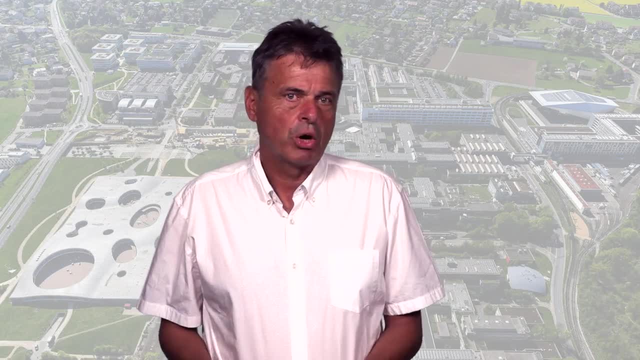 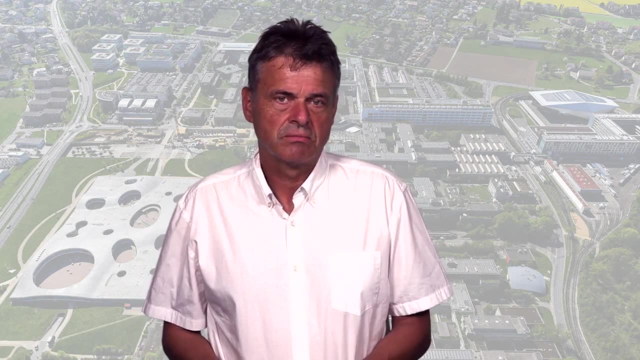 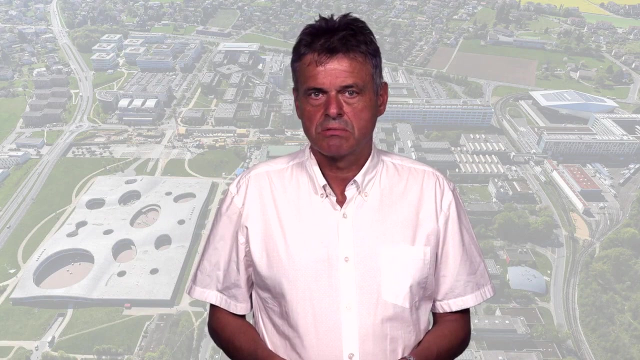 of important concepts and invite you to play with them, modify and improve them. The course is also complemented by a series of programming projects as homework assignments. What about the recommended background? Well, you should have at least one year of programming experience. Proficiency with Java or C-sharp is ideal, but if you are experienced with 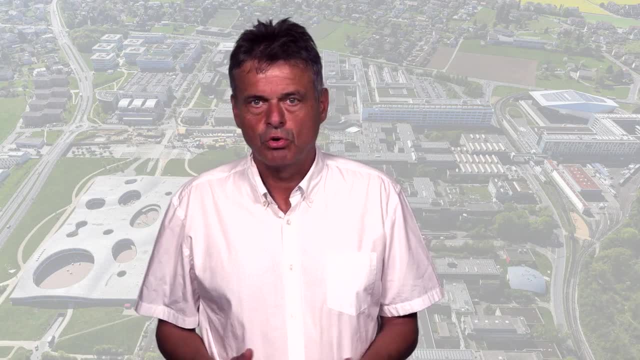 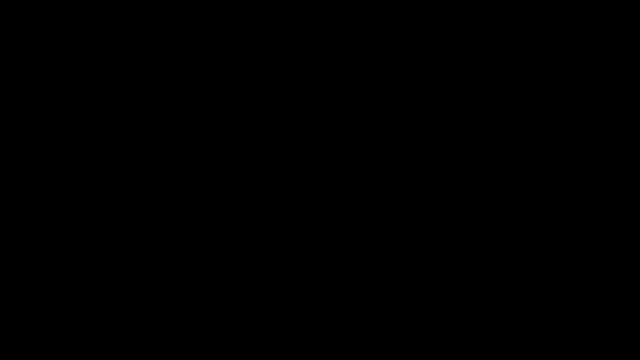 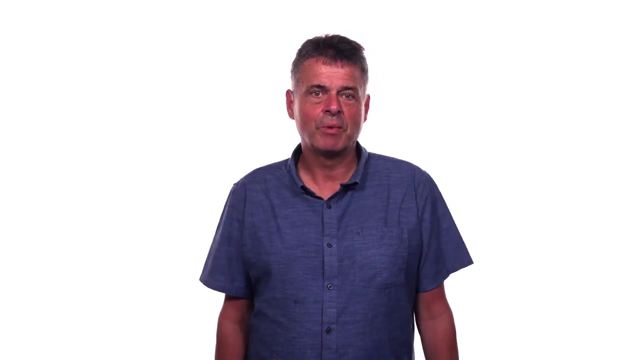 other languages such as C, C++, Python, JavaScript or Ruby. that's also sufficient. You also should have some familiarity using the command-line. Welcome to my course on functional programming: programming principles in Scala. As the name implies, we're going to do quite a bit of Scala. 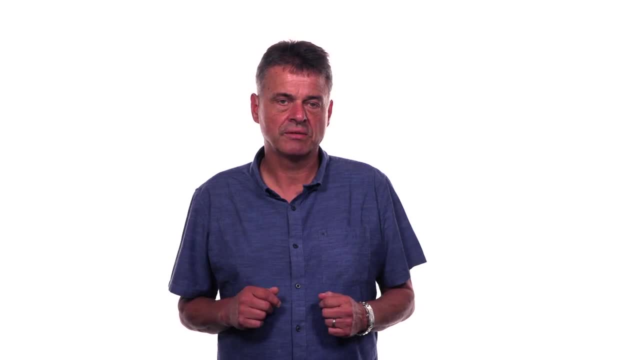 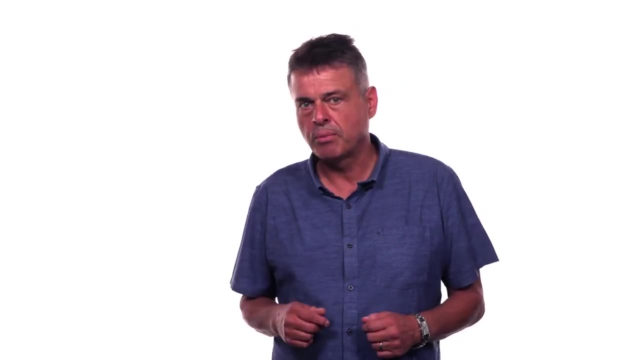 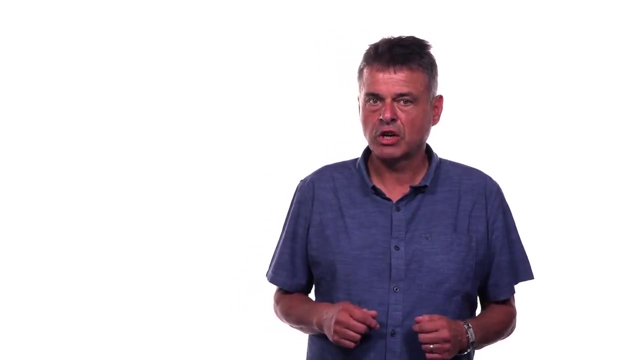 programming. but that's not the primary objective of the course. The primary objective is to teach you functional programming from first principles. You're going to see functional programs, methods to construct them and ways to reason about them. You're going to find that functional programming. 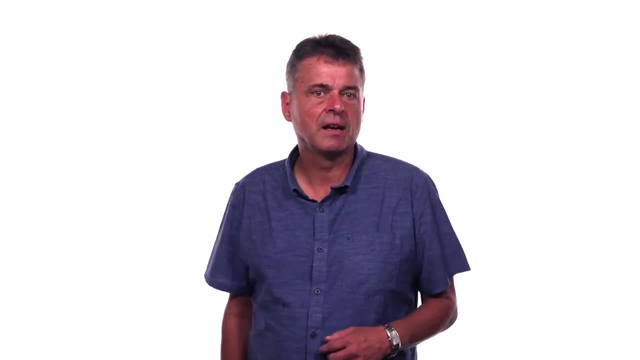 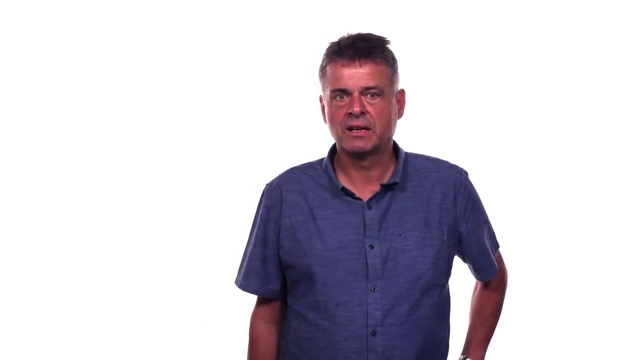 is a paradigm that's quite different from the classical imperative paradigm that you know from languages such as Java or C. In fact, you can combine the two paradigms and it's one of Scala's strengths that it provides a gradual migration path from a more concise, Java-like language. 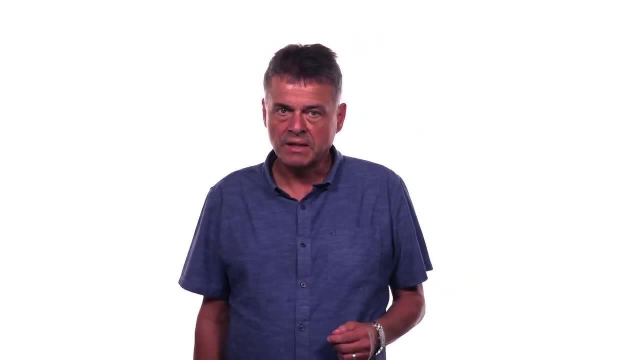 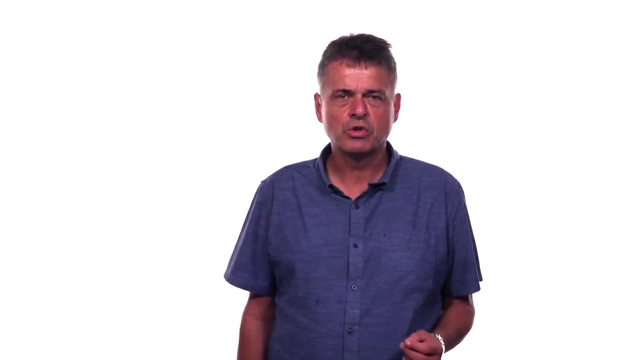 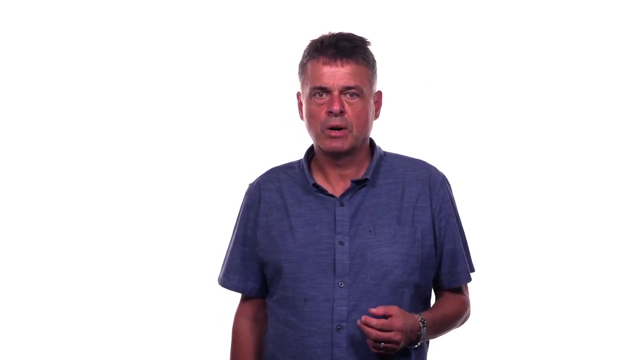 to full functional programming. But in this course we're not going to be gradual, We're going to take a clean break. I'd like you to suspend for the time being most of what you know about programming and look at programs with fresh eyes. That way, I believe, you'll be better placed to absorb. 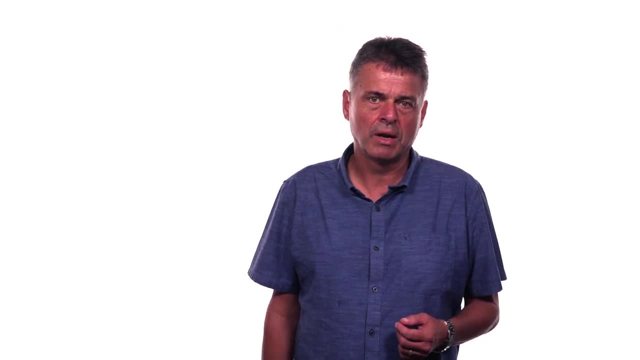 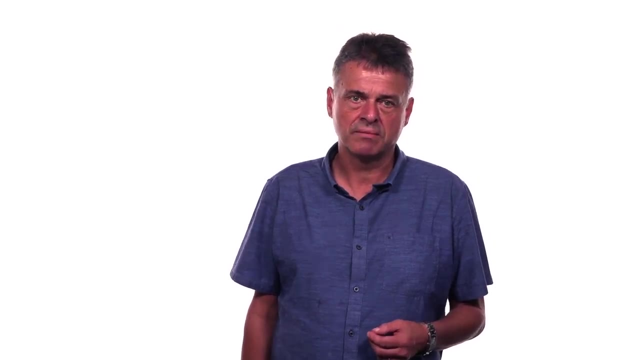 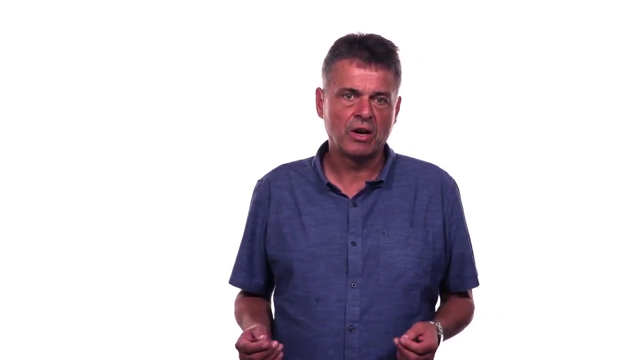 the new knowledge that you're learning. You'll have a new way of thinking, promoted by functional programming, and once you've done that, you'll also be able to integrate what you have learned back into your daily programming practice. A couple of remarks on the organization of the course. It will consist of a sequence of videos which will introduce the elements of the course one by one. 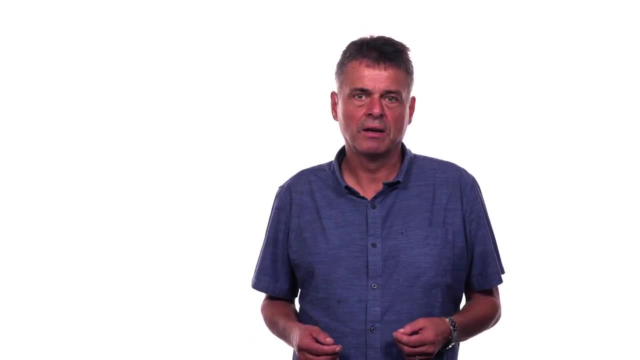 We'll typically have five or six videos per week. The videos will often have quizzes where you're asked to fill in some questions. Those questions could be multiple choice, or I might ask you to code something After the quizzes. you will always see the answer in the videos. 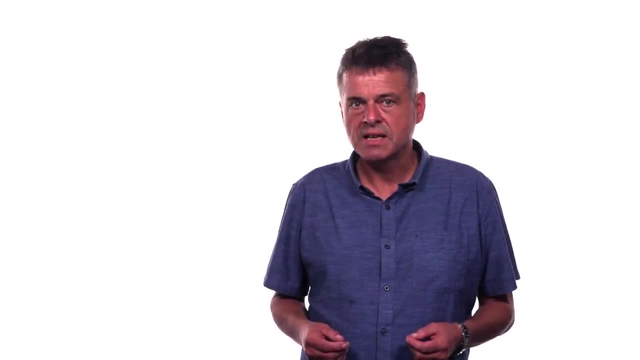 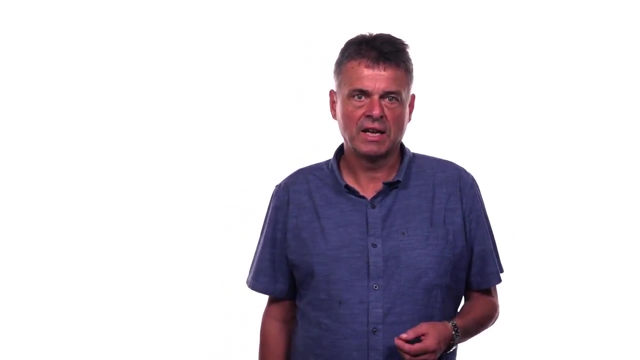 Besides the quizzes, there are also assignments. The assignments you have to hand in and you're going to be graded on them, And if you pass the assignments, then you will get a certificate at the end of the course. The quizzes, by contrast. they're just for your own education. There's not 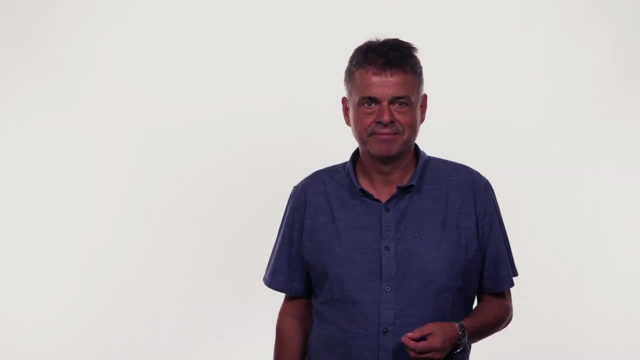 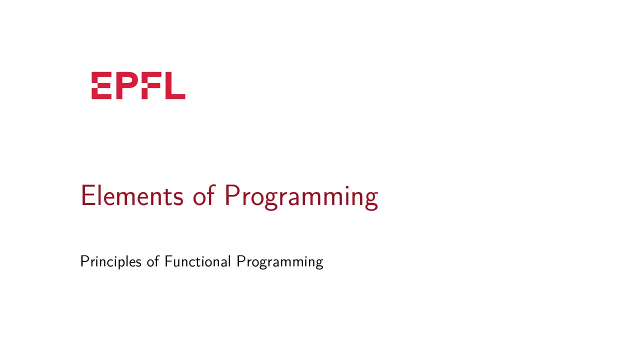 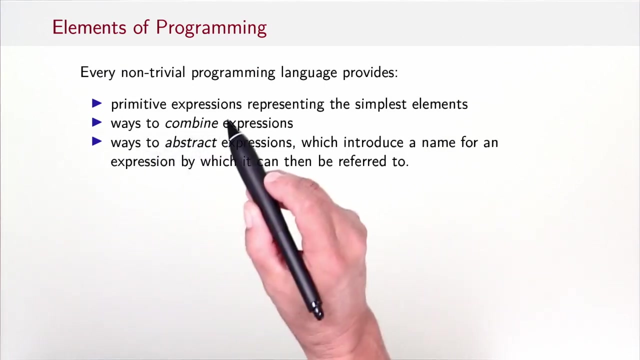 there are no grades for these, So let's get started. Web site. Welcome to this first hands-on lecture on how to do functional programming with Scala. In this lecture, we're going to look at the most fundamental elements of programming. In fact, every non-trivial programming language provides primitive expressions that represent: 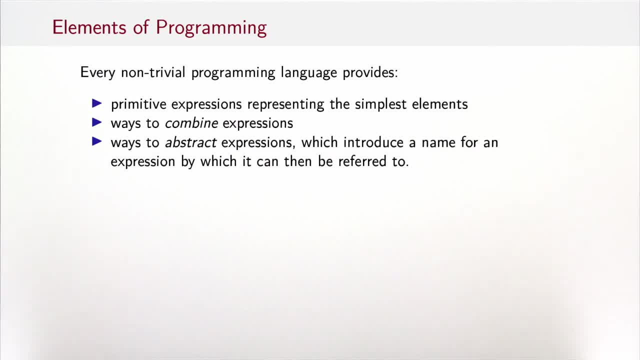 the simplest elements of the language, so that would be something like a number or a string. Then it combines ways to combine expressions for a string or a number, Then it combines ways to combine expressions for a number, and then it combines ways to combine expressions. 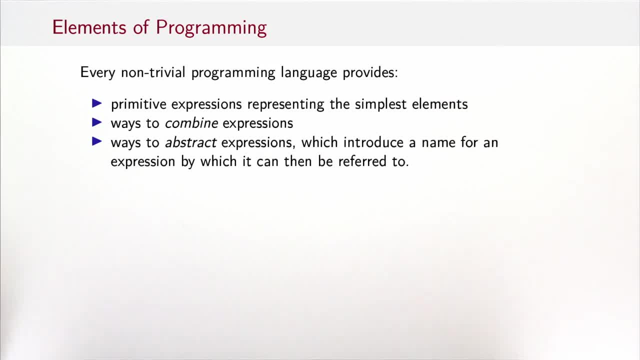 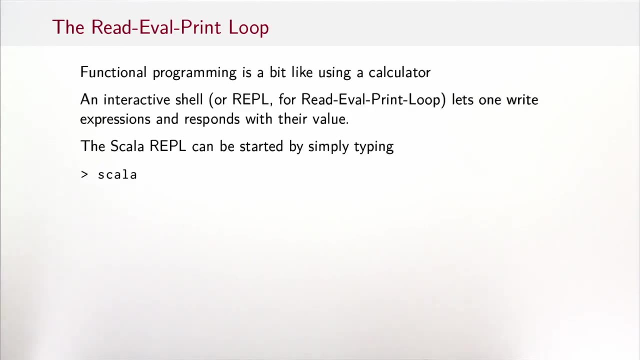 like: add two numbers, concatenate two strings and finally it will provide ways to abstract expressions. Abstracting means we introduce a name for an expression and then afterwards we can refer to the expression by its name. So a good way to approach functional programming is to think: 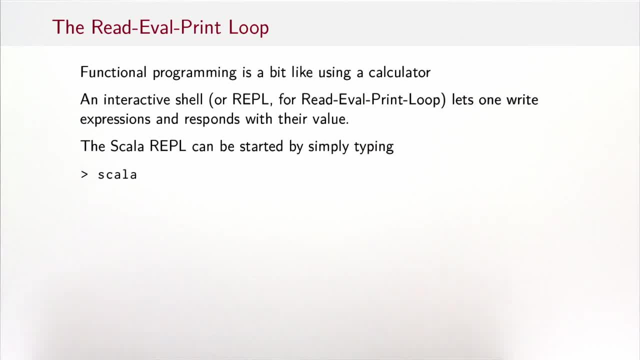 of it as a very powerful calculator. In fact, most programming languages, Scala included, have an interactive shell, which is often called a REPL. REPL stands for read eval print loop. The REPL lets you write expressions and it responds with the value of those expressions. If you want to. 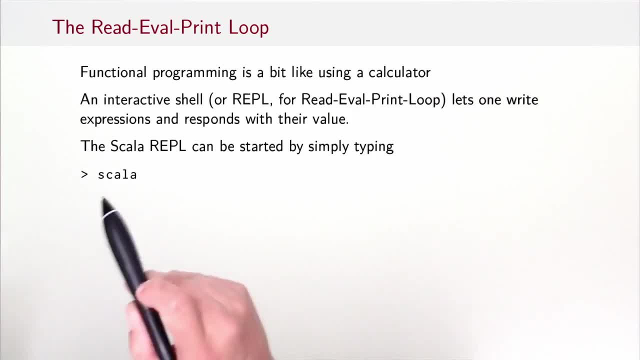 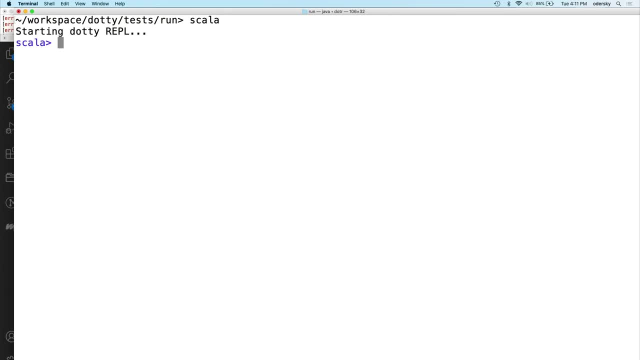 start the Scala REPL. you can simply type Scala at the command prompt. So let's do that. We type Scala and we get a REPL. It says here starting Dottie REPL, because at the time I record this lecture we are still having a pre-release of Scala 3 called Dottie. 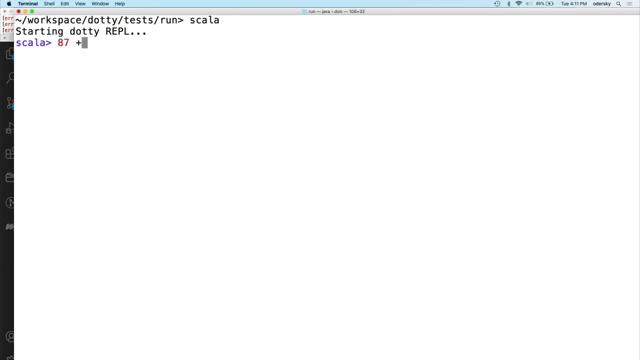 So we have the Scala prompt and now we can type expressions like this one here, and the REPL will respond with the value 232 and also its type, which is int in this case. We'll learn more about types later, But functional programming languages, of course, are stronger than REPLs. For a starter, they 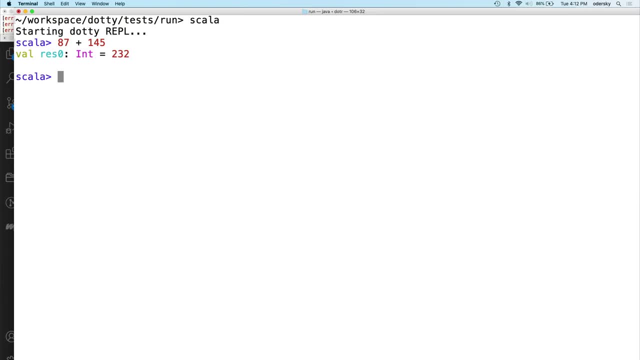 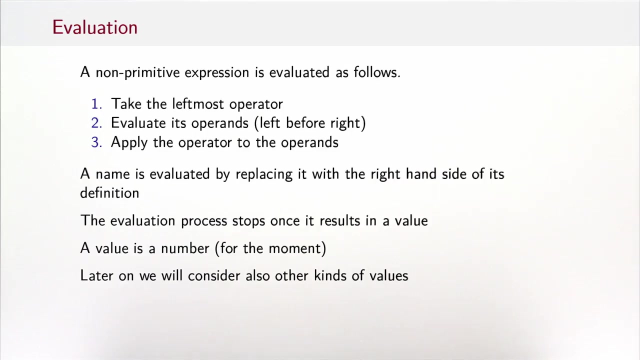 also let you define values and functions and you can give them names. So, for instance, you can write def- size equals, And now we have defined size and you can use it in another expression like this one. So how are expressions in a functional language evaluated? In the end it's, of course, the computer, but a good 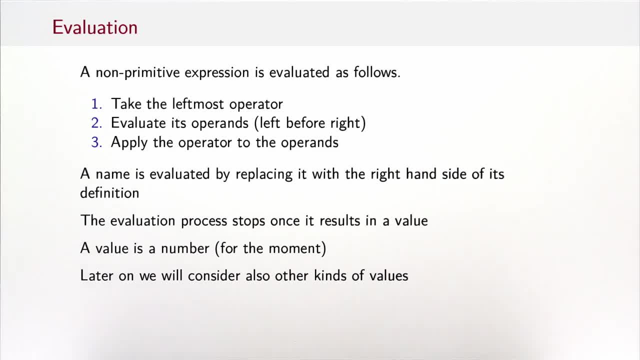 high-level way to think about it is in very much the same way. you would simplify an expression with a pen and paper, So you would typically take the leftmost operator, evaluate the operands going left to right and then apply the operator to the operand. 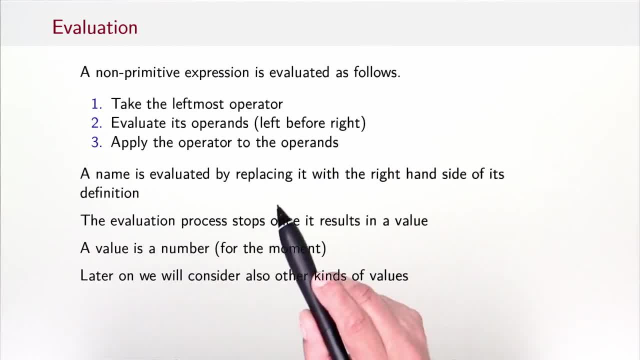 Now we have defined the number of differences to get to our experimental data as well. So I guess we will do this experiment after we've speak about the name first. OTHER EXERCISES: You can create a shift-fold governments. To do that, you put the數 to the shoot. 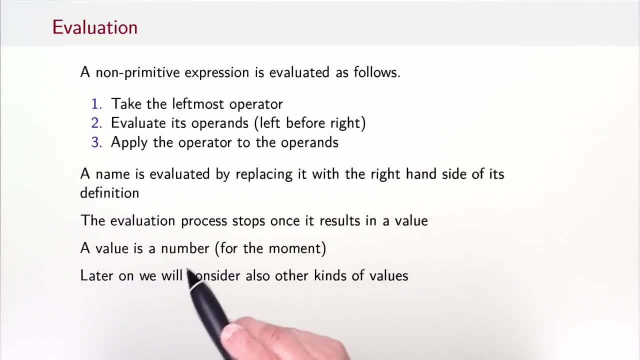 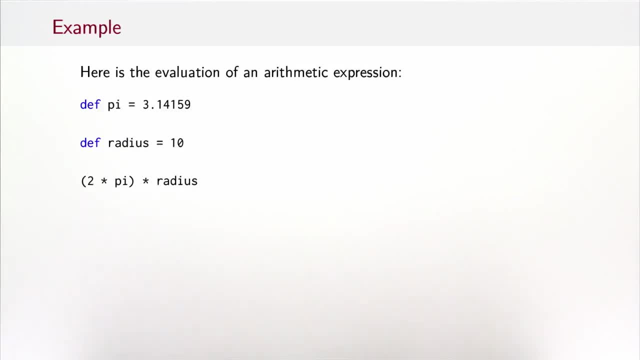 And let's sayды V's are the zero colors kept in the model where items landed on a circle and received a number of values. OTHER exemples: If you have a name like size, then you evaluate that by replacing the name with the right-hand sides of it's definition. so size would be two performed in the examples that you saw previously. 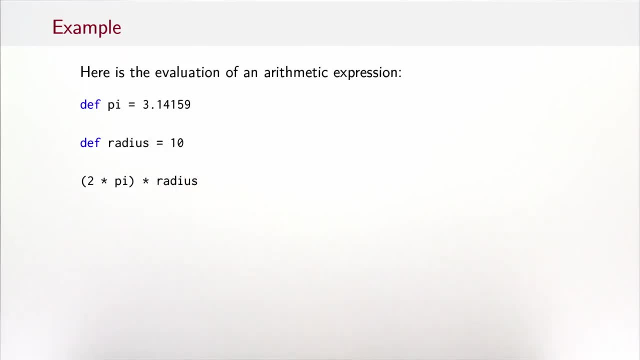 radius, where pi and radius are defined like you see here. So that would evaluate like this: You first take the name pi and replace it by its definition, You perform the multiplication. You take the name radius and replace it by its definition, You perform the multiplication and 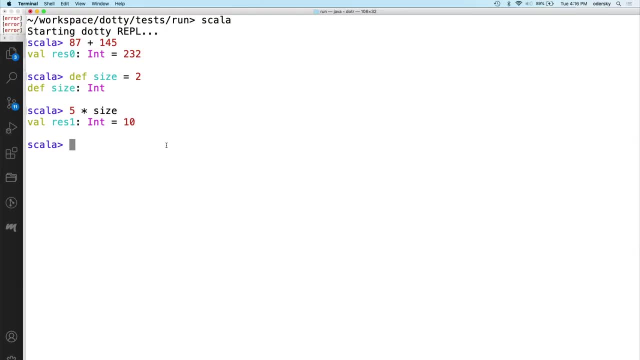 you arrive at the result. Now let's do something a little bit more interesting. We can also define functions that take parameters. For instance, here's one. Now the REPL responds with a def: the name of the function, its parameter and its result value. 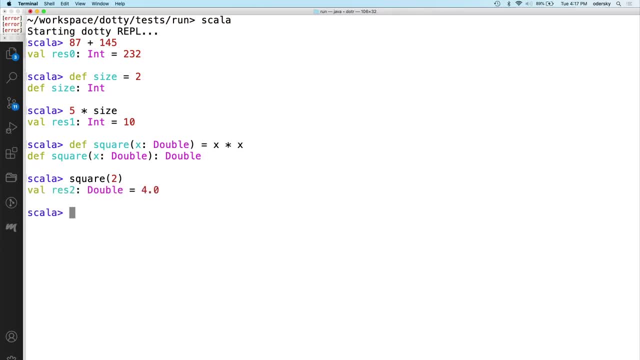 You can write then a square of two, you get four. You can write square of five plus four, and you get 81.. Or you write square of four, and you always get the result. Of course we can push this further and now define a function that in turn calls square, So let's call it sum of. 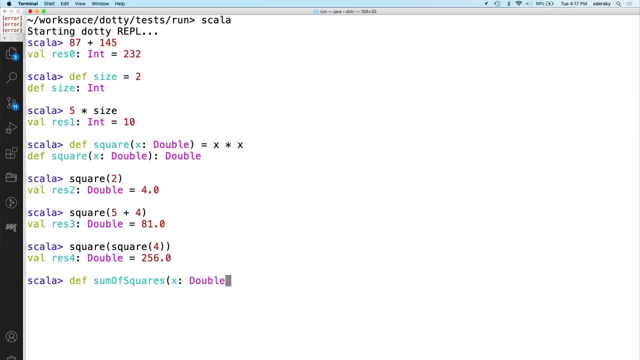 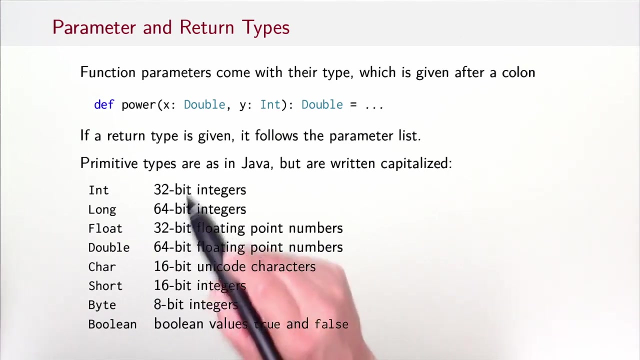 squares And we have defined a function that takes two double parameters and a double result. So let's look at the syntax of what we've done here. So we can have function parameters- They are given by a name and a colon and a type, And functions can also have result types in which 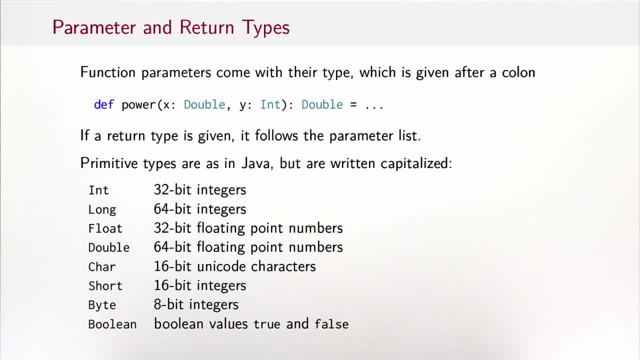 case also, we have a colon at the end and its type Types for now are basically just primitive types and those are, as in the case of a function that takes two double parameters and a double result, So like in the case of an integer, as in Java, But they all start with a capital letter. So we have 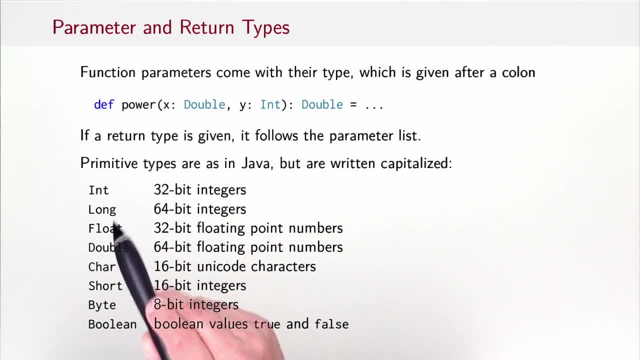 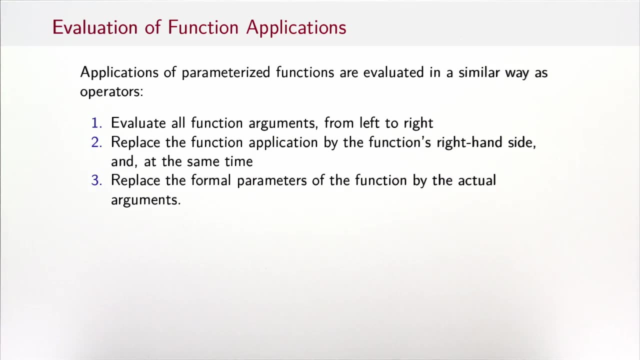 int for the usual integers, long for 64-bit integers, float double for floating point values, curve for characters. short and byte for shorter integers. and booleans for the boolean values: true and false. So let's look at evaluation again. How would we ever evaluate an application? 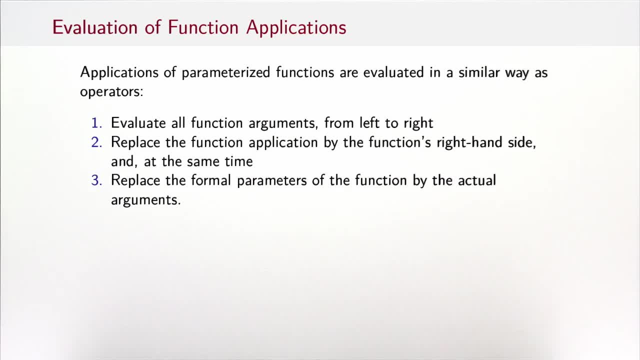 of a parameterized function. In fact, it's done in a similar way to what we already know from operators. We evaluate all the functions in the set And we find that we have two positions. We have one on each of these two functions, one on each of the other. We see that the set has two. 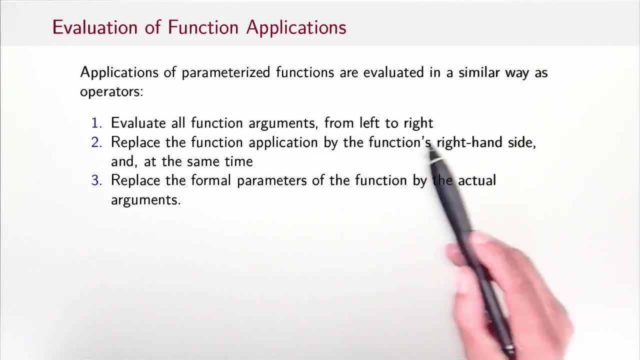 or in this case, in the set. we see that the set has four, The set has two, And then we find that all the function arguments from left to right. We replace the function application by the right hand side and at the same time we replace the formal parameters of the function by the. 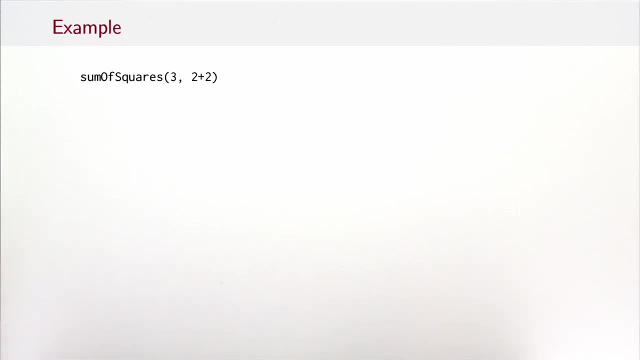 actual arguments. So let's do this for the sum of squares example. Let's say we start with sum of squares 3 and 2 plus 2. We simplify the arguments. that simplifies 2 plus 2 to 4. We replace it with the body of the function and at the same time we replace the formal. 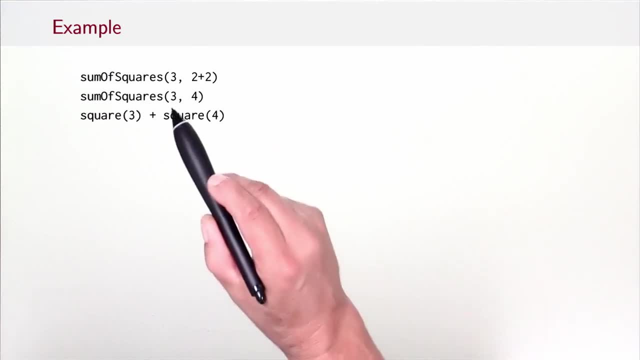 parameters of sum of squares, which were x and y, by the actual arguments, which were 3 for x and 4 for y. Now we are left with square of 3 plus square of 4.. We simplify and turn square of 3, that gives the body of square 3 times 3 plus square of 4.. After simplification: 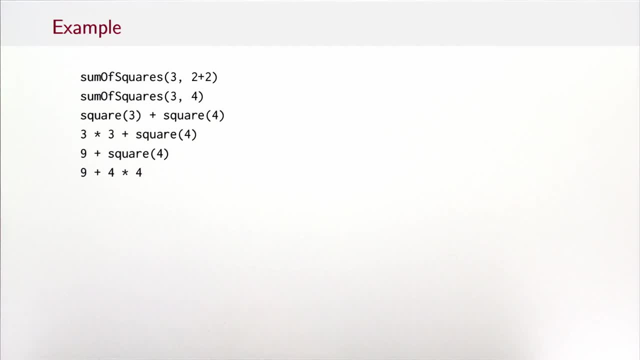 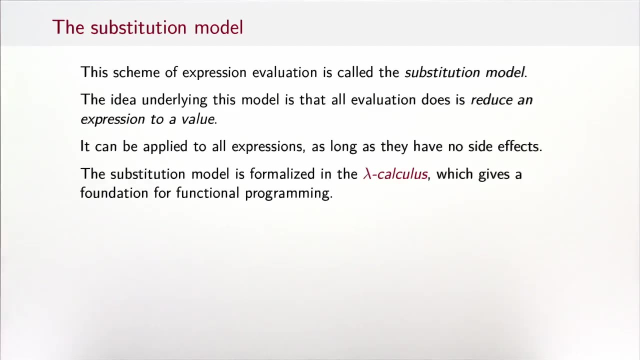 we take the right operand call, that expands to 4 times 4.. Now we get the result 25.. Now this will probably seem complicated, Trivial to you, and you might wonder why I insist so much of the details of evaluation. In fact, it turns out that this evaluation model, which we also call the substitution, 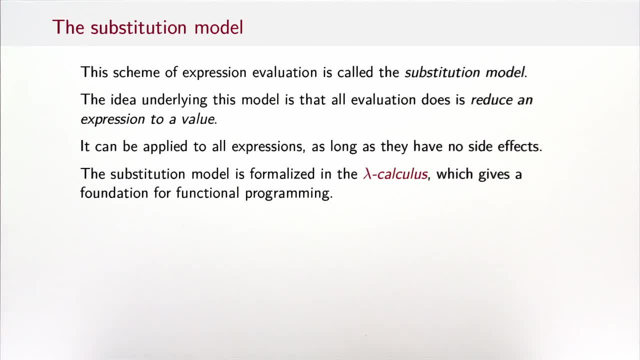 model, simple as it is, is universally powerful. That means we can express every algorithm with that model. The idea underlying the model is that all an evaluation does is reduce an expression to a value. It can be applied to all expressions, as long as those expressions 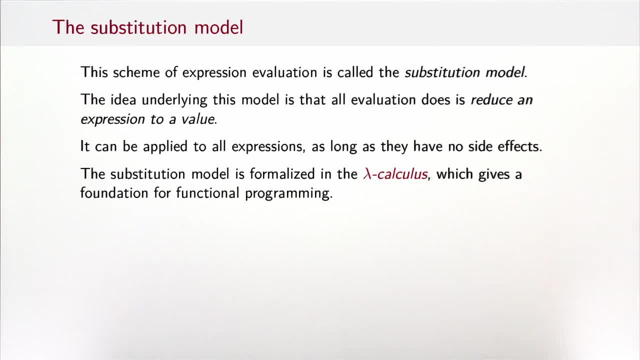 have no side effects, which means that those expressions are functional or purely functional. The substitution model has been formalized in the lambda calculus, which gives a foundation for functional programming and for programming in general. In fact, the lambda calculus is older than computers are. It was first invented by Alonzo Church and it was intended as a 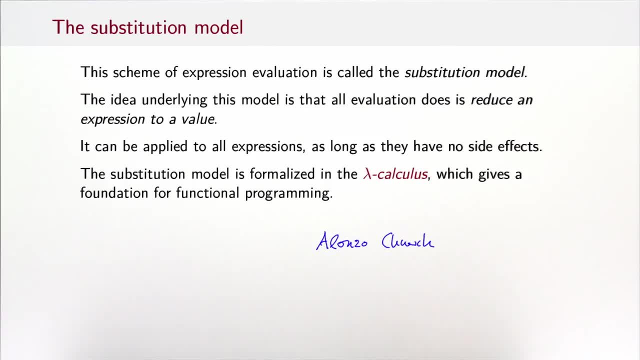 foundation of mathematics. In fact, a couple of years later, another logician, Kurt Gödel, showed that a complete and complete algorithm can be applied to any function, of any function. In fact, a couple of years later, another logician, Kurt Gödel, showed that a complete and complete 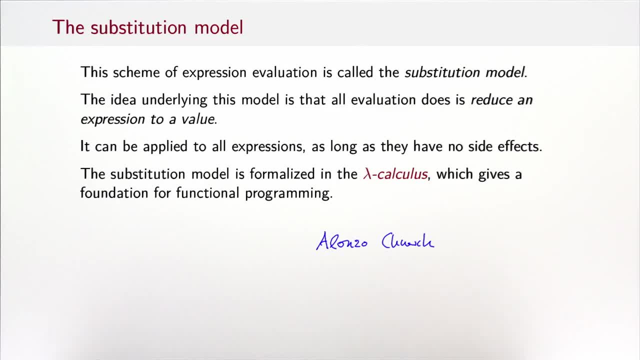 algorithm can be applied to any function, of any function. In fact, a complete and complete formalization of mathematics is impossible. so lambda calculus was left as a model, more for computable mathematics and for computing. So now that we know what evaluation is, we can ask interesting questions. One interesting: 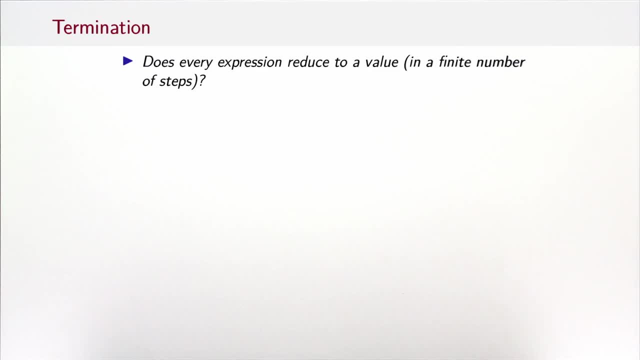 question is: does every expression reduce to a value in a finite number of steps? Does every evaluation terminate? So let's think a little bit. Can we find an expression whose evaluation would not terminate? In fact, yes, here is one, So we can write an expression. 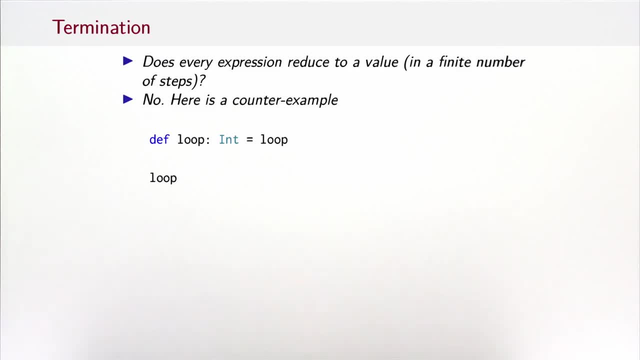 loop. It's of type int, say, and its body is loop. So if we reference loop in an expression, then by our rule the reference would be replaced by the body, which is again loop. So we get a beautiful and very tight loop of an expression that only evaluates to itself and therefore 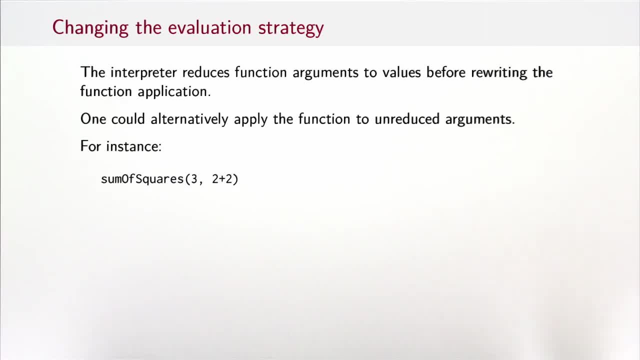 evaluation of that expression will never terminate. Another interesting question to ask is whether the evaluation strategy we've seen is the only possible one, or were there other possibilities? One particular detail is that our interpreter reduces function arguments to values before rewriting the function application. Can we? 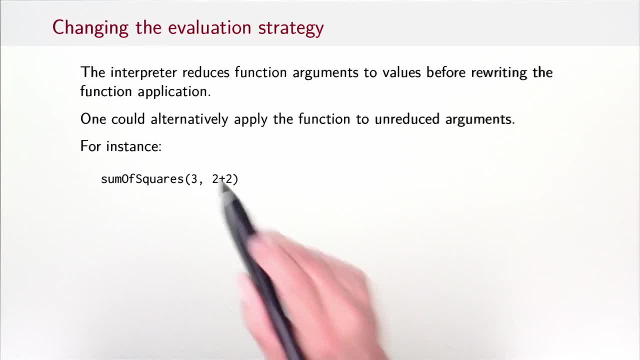 change that? In fact, yes, we could alternatively apply the function to un-reduced arguments. So, for instance, if we start with the same expression as before, three, sum of squares two plus two, then we would get square of three plus square two plus two. so I haven't. 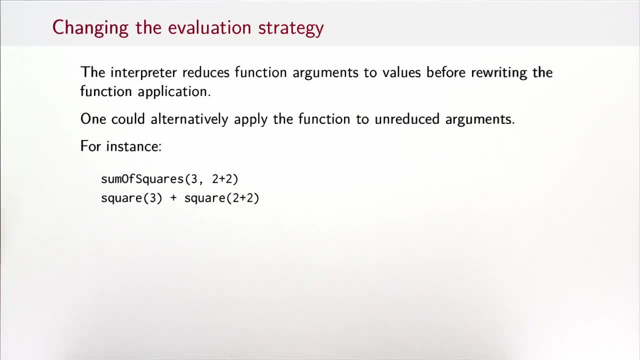 evaluated two plus two. I just pass it like this, And then we would continue as before on the left and on the right. we would now replace square of two plus two by two plus two times two plus two, so the parameter of square x gets replaced by the expression. 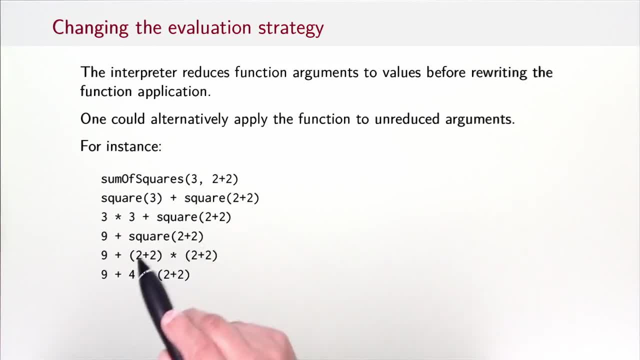 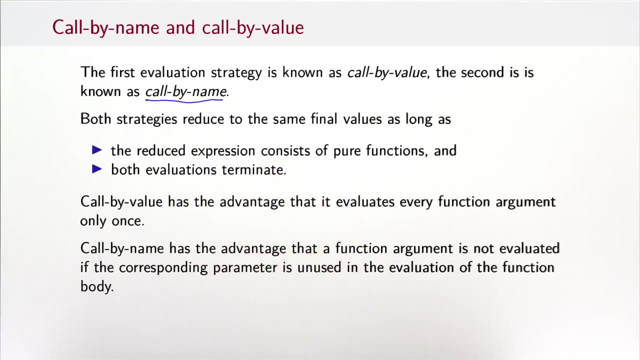 not its value. And now, finally, I have to reduce the two plus two here and the two plus two here and arrive at the same result, So that alternative evaluation strategy is known as call-by-name, whereas the one we saw previously is called call-by-value, because we evaluate things before we pass them. so 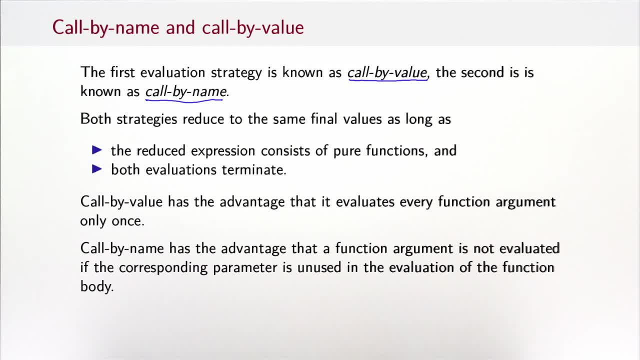 we pass only values and not full expressions. In fact, it was no accident that both reduction sequences reduced to the same value, twenty-five. That's always the case, so both strategies reduce to the same final values, as long as the reduced expressions consist of pure 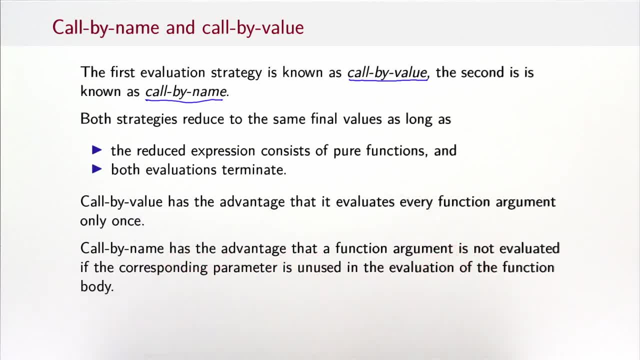 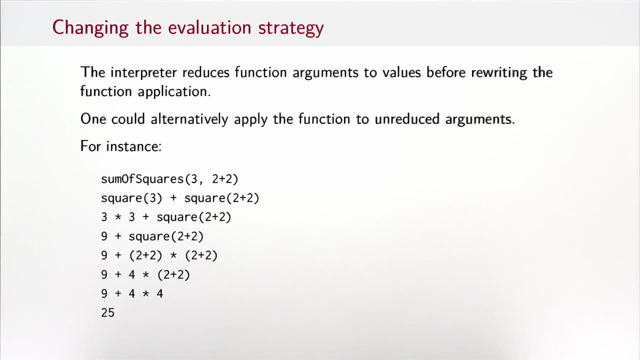 functions no side effects and both evaluations terminate. So which one is better, Call-by-value or call-by-name? So you might think that call-by-value is better because it evaluates every function argument only once. If you go back to the sequence that you saw here, you notice that 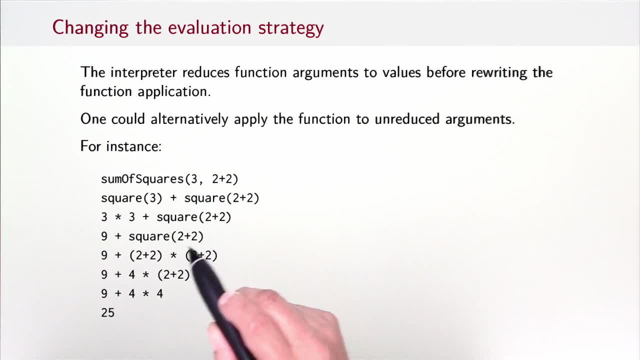 the evaluation of two plus two is done twice because we passed it to square here and here. Now we have duplicate work to simplify 2 plus 2 to 4.. Now that's, of course, in this case completely trivial, but instead of 2 plus 2 you could have an arbitrarily complicated expression. 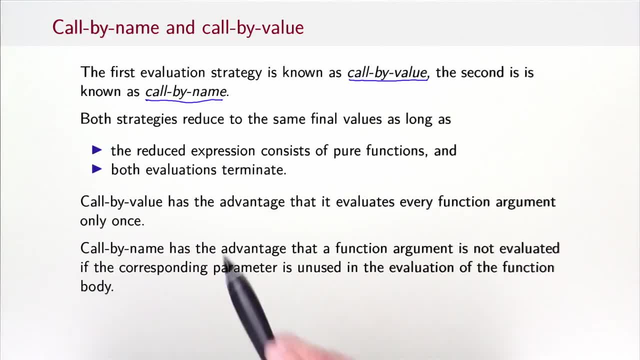 and then it starts to matter. So call-by-value definitely has the advantage that it evaluates every function argument only once. But call-by-name also has an advantage, which is that well, if a parameter is completely unused in the evaluation of a function, 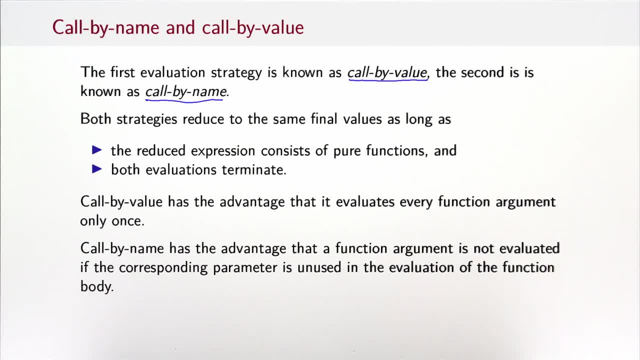 then the function argument is not evaluated at all. So call-by-name can evaluate function arguments 0 times, 1 times or multiple times, whereas call-by-value always evaluates them exactly once. And sometimes when it's 0, then call-by-name has an advantage. 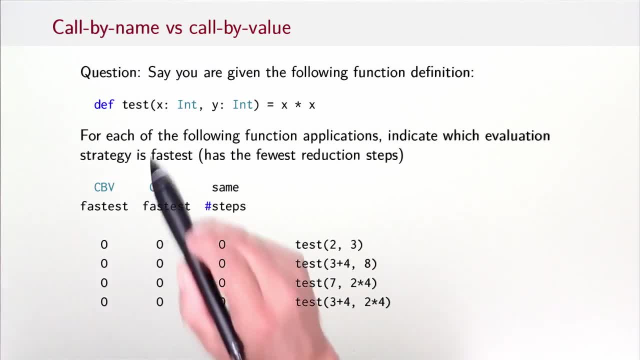 So let's make a little quiz about that. Let's say you have the following function definition: def test takes two parameters, x and y, and its body is x times x. So So for each of those function applications that you see here, 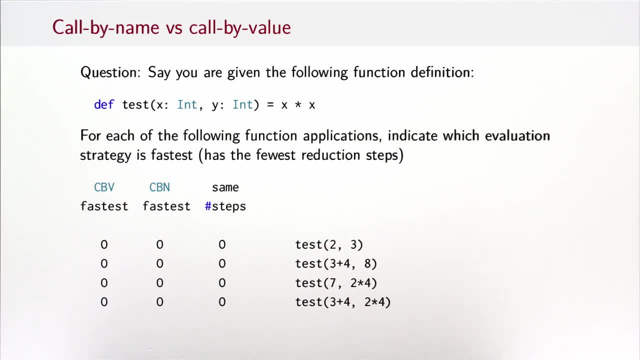 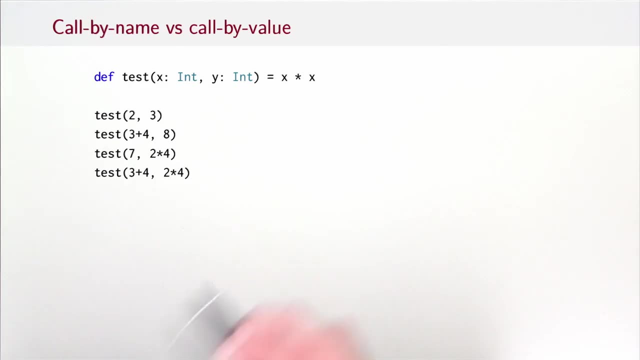 indicate which evaluation strategy is fastest, That means has the fewest reduction steps, Call-by-value, call-by-name, or maybe sometimes they have the same number of steps. So let's see what the answers will be. If we write test 2, 3,, then well, you have in both cases the evaluation 2 times 2,. 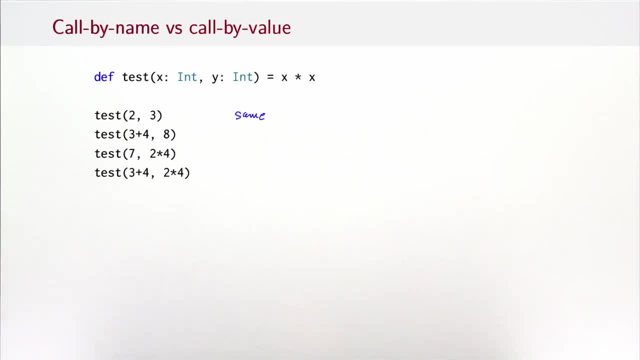 so they are the same. If we write test 3 plus 4, 8,, then call-by-value is better, because the expression 3 plus 4 will be evaluated only once before it is passed into test. If you write test 7, 2 times 4,, then call-by-name is faster. 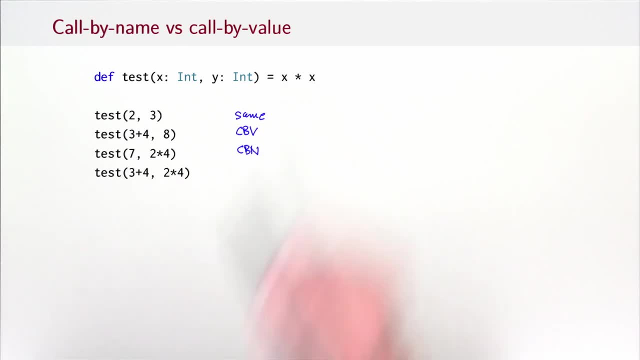 because the evaluation of 2 times 4 is omitted altogether. And finally, if you write test 3 plus 4, 2 times 4, then essentially call-by-value has an advantage for the first parameter, call-by-name for the second parameter. 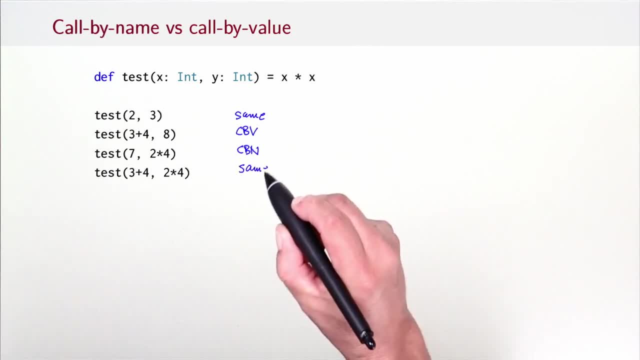 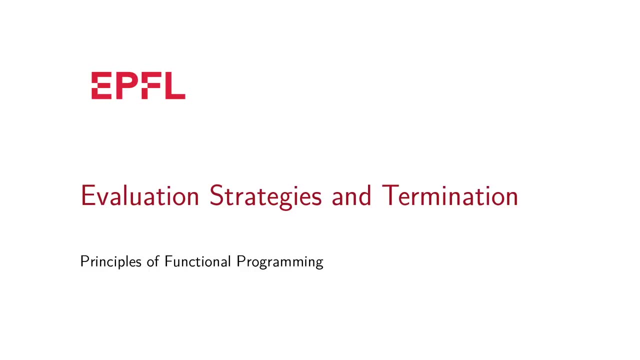 and the two cancel each other out. So you will have again the same evaluation complexity. In the last session you've seen a formal model of evaluation, which we call the substitution model, and you've also seen that there was more than one way to evaluate. 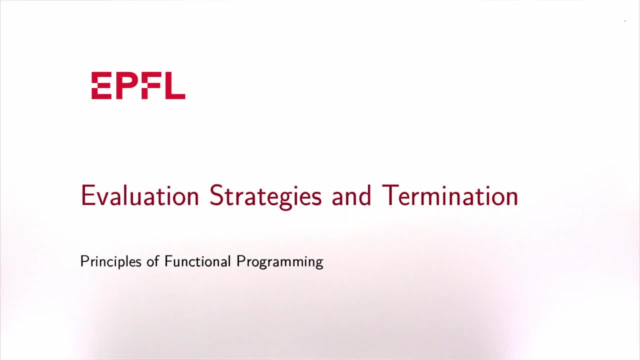 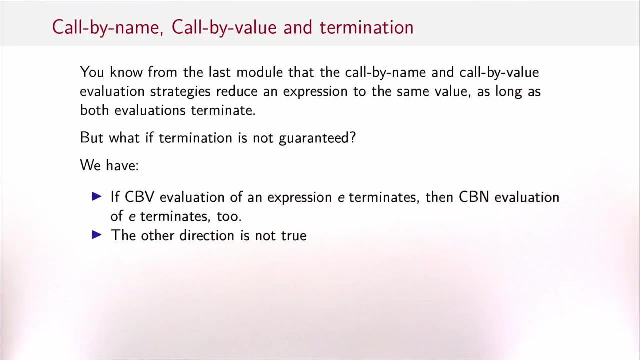 an expression. We identified two evaluation strategies, which were called call-by-name and call-by-values. In this session, we are going to go into a bit more detail about these strategies, in particular with a view on termination. So what we've learned in the last session is that the call-by-name 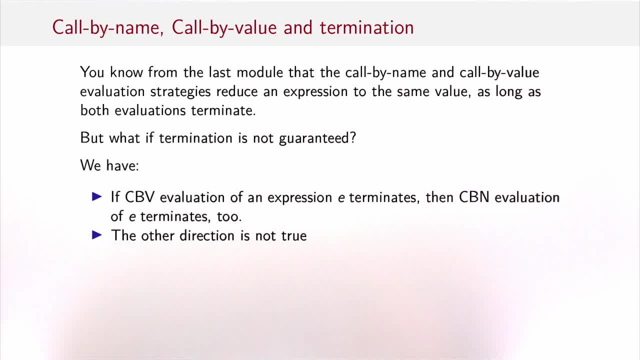 and call-by-value evaluation strategies reduce an expression to the same value as long as both evaluations terminate. But what if termination is terminated? What if termination is not guaranteed? In this case, there's an important theorem to remember. The theorem says that if a call-by-value evaluation of an expression terminates, 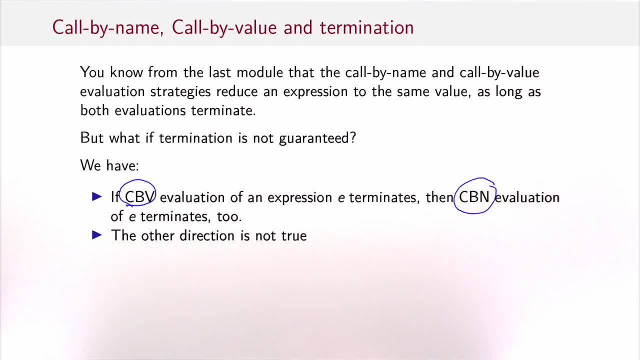 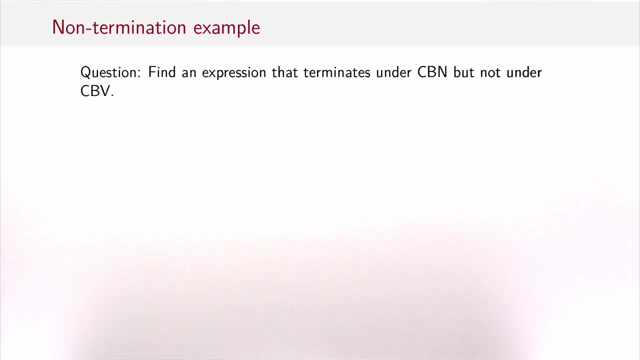 then the call-by-name evaluation of the same expression terminates as well, But the other direction is not true. So there are expressions that terminate under call-by-name and that do not terminate under call-by-value, So let's try to find such an expression. 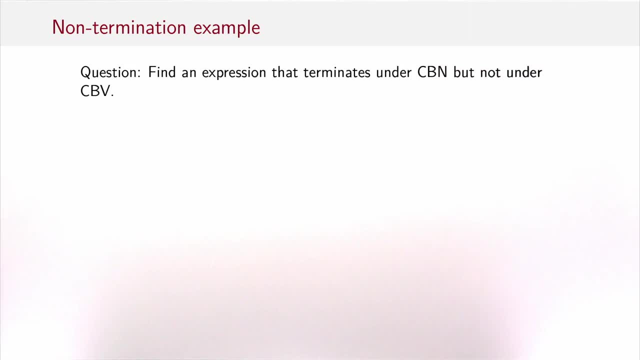 that terminates under call-by-name but not under call-by-value. What could there be? Think a little bit. Well, here's a candidate expression Let's define first. It takes two integers, x and y, and just returns the first one. 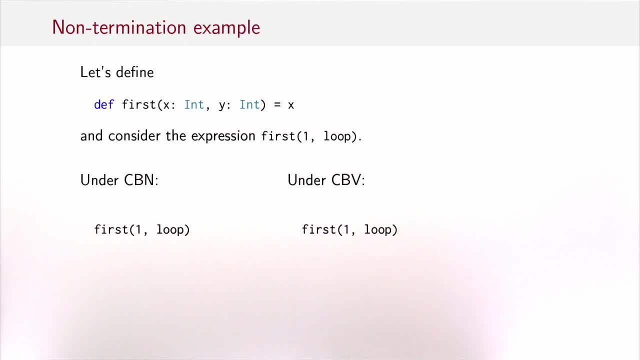 And now we consider the expression first of one and loop. So under call-by-name we have that the arguments one and loop are passed as they are. So we immediately replace first by its body x, which in this case would be one, because one is the first. 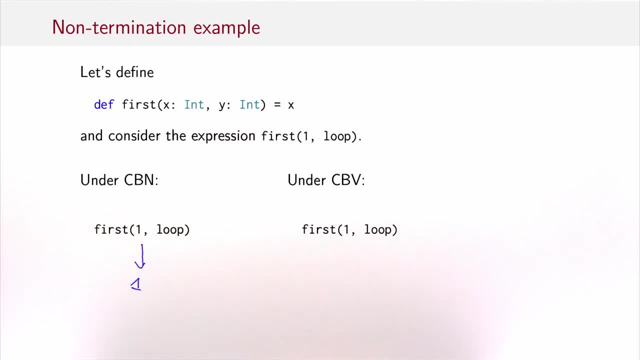 And one is the argument that's passed to x. So we evaluate in one step to one Under call-by-value. on the other hand, we evaluate the two arguments first. So one evaluates to one- no problem there- But loop, as we've seen, evaluates to loop. 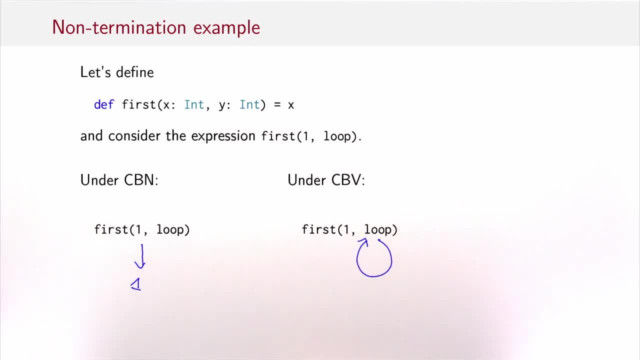 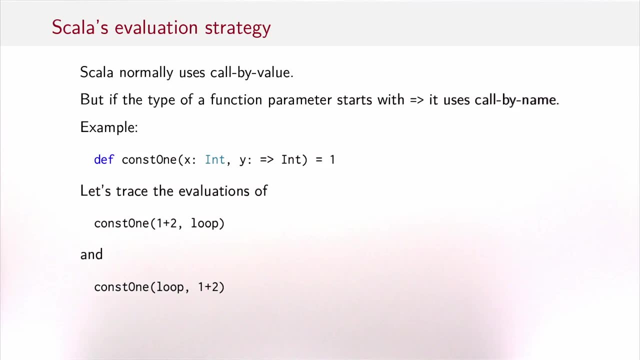 And so we get stuck literally in this loop. that first one loop always evaluates to itself, and term evaluation does not terminate in this case. So if you just look at termination, it might seem that call-by-name is a better evaluation strategy than call-by-value. 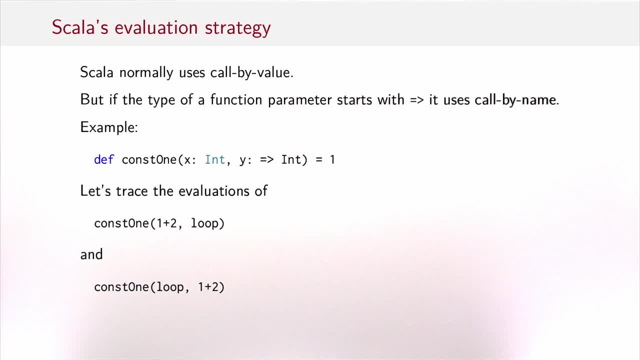 But Scala, like most languages, actually uses call-by-value by default. There are two reasons for this. One reason is that call-by-value can avoid- sometimes exponentially- many reduction steps because it avoids duplication of evaluations. And the second reason is that, as long as a language 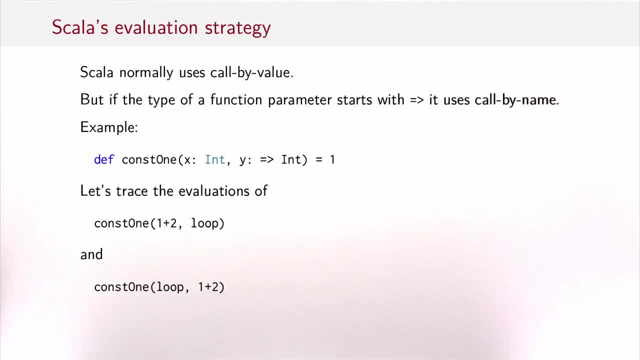 has some imperative side effects, which is the case for Scala. call-by-value is actually much more predictable than call-by-name. That means it's much easier to tell when the effects of an expression actually happen if the evaluation strategy is call-by-value than if it is call-by-name. 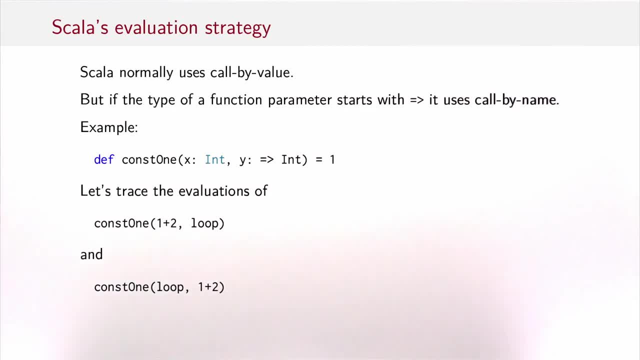 So for both of these reasons, Scala uses call-by-value, But it gives you the choice to choose call-by-name explicitly, and you do that by adding an arrow in front of a function parameter, as you can see in this example here. So here we have a function const1.. 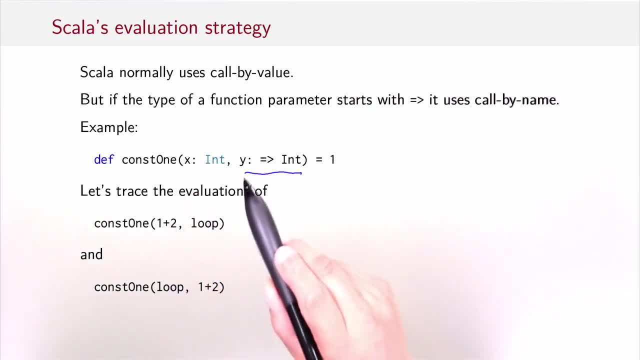 It takes a call-by-value parameter x and a call-by-name parameter y, because you have the arrow here And it just evaluates to 1.. So now let's look at two evaluations. The first evaluation would be of the expression const1 loop. 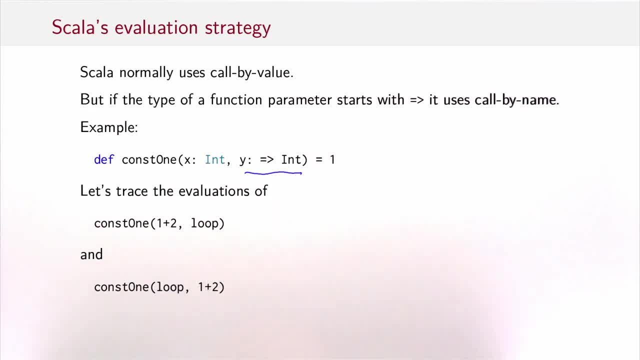 So loop is in the second call-by-name position And the second expression would be the same, but with the arguments reversed. So loop would now be in the call-by-value position. So let's look at call-by-name first. So if we start with const1 loop, 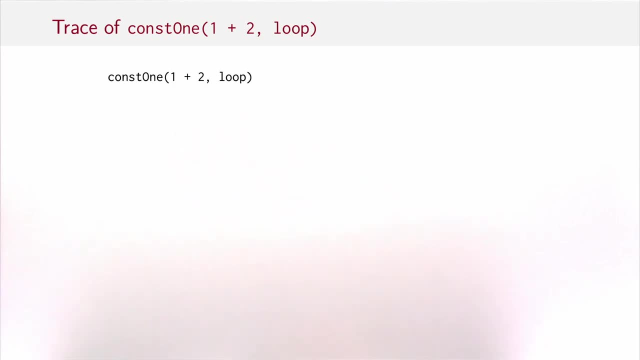 then we have to evaluate call-by-value arguments left to right, So we would evaluate 1 plus 2 to 3.. And then, as a next step, we would simplify the call to the body of const1, which is essentially just its first argument. 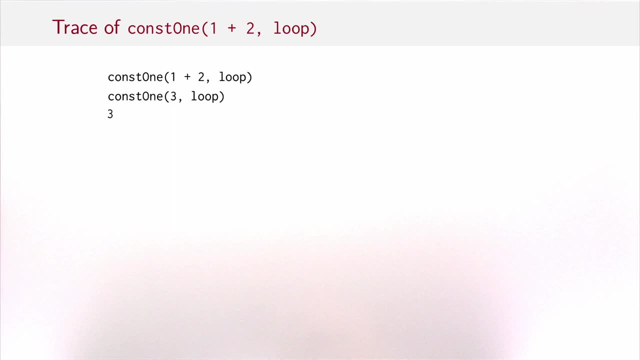 So 3 is the result. But the important thing to note here is it terminates. So let's look at the reversed arguments now. Loop appears in the call-by-value position. If we have this expression here, then we have 3.. So we have to evaluate loop as first call-by-value argument. 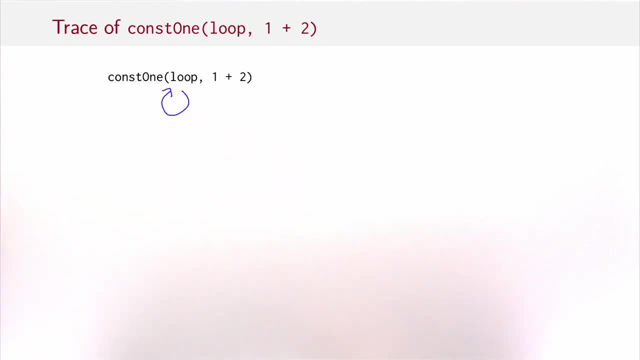 And that would just essentially evaluate to itself, which means that we get an infinite sequence of steps where the function just evaluates to itself And evaluation never will terminate. So in this unit we will learn about two new constructs in our toolbox: conditionals and value. 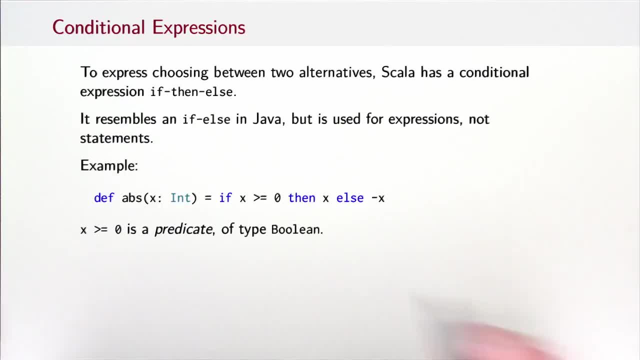 definitions. So the first construct is if-then-else. It allows you to choose between two alternatives, And the if-then-else in Scala resembles an if-else in Java, but it's an expression, not a statement. So let me explain what that means. 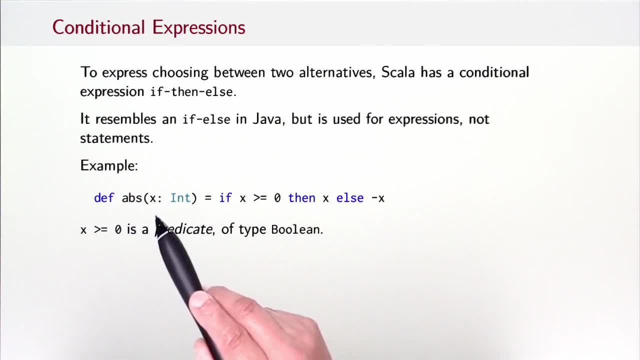 If you have a function like apps for absolute value that takes an x int, and then the right-hand side would be: if x greater or equal 0, then x else minus x. So here, that right-hand side, it's an expression. 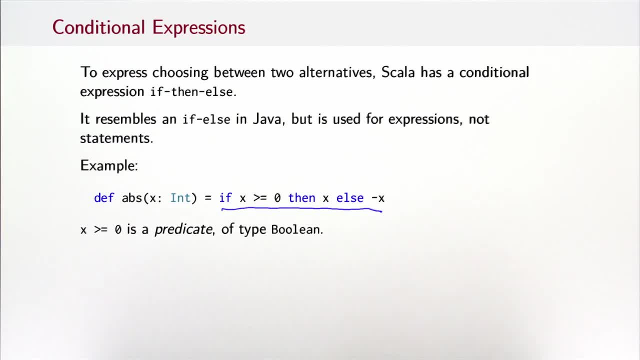 It returns a result. In Java you would use the if-then-else for a statement that has a side effect. For instance, it would maybe assign to a variable, But that's not available to us in purely functional programming. So of course a Java buff would know that Java also. 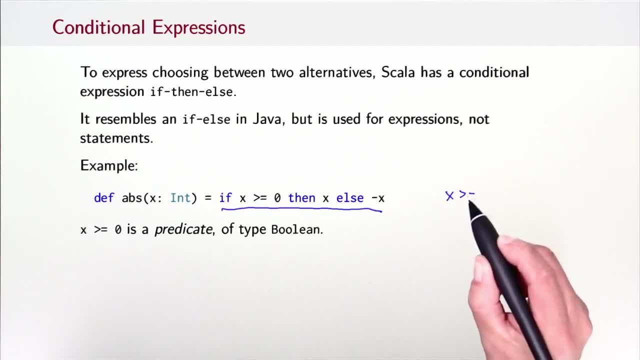 has a conditional expression. It would look differently. You would write it like this, But that's actually rather cryptic. So most people prefer the if-then-else, And in fact that's the only form that's available. That's available in Scala. 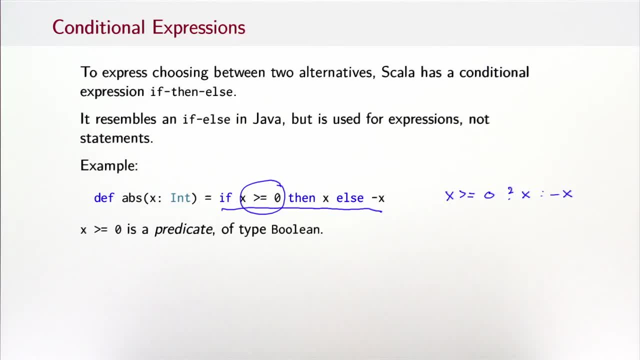 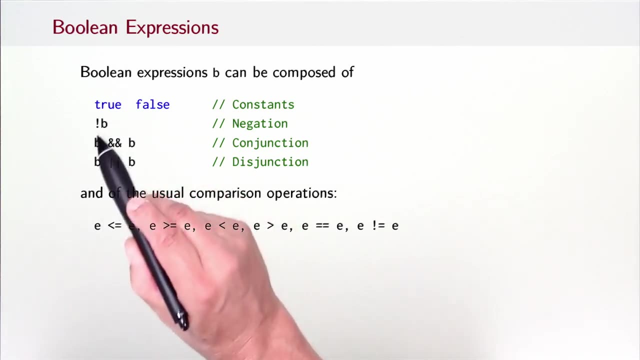 The x greater than or equal 0. here is a predicate. That's an expression that has boolean, the type of truth values- true and false- as its type. So you can form boolean expressions from the two constants, true and false, negation which is expressed with a bang. 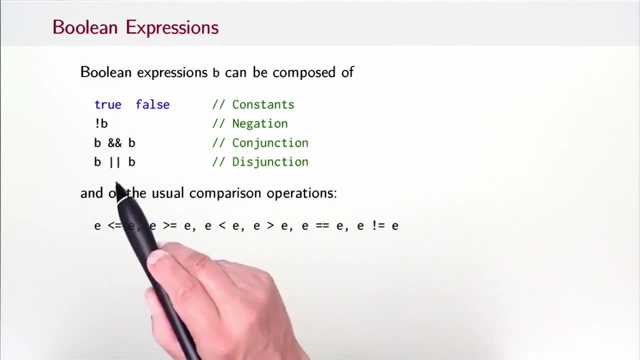 conjunction which is expressed ampersand, ampersand disjunction, or which is represent bar bar, And then you have the usual comparison operators: less than equal, greater than equal and so on. You will note that that's exactly the same operators as in Java. 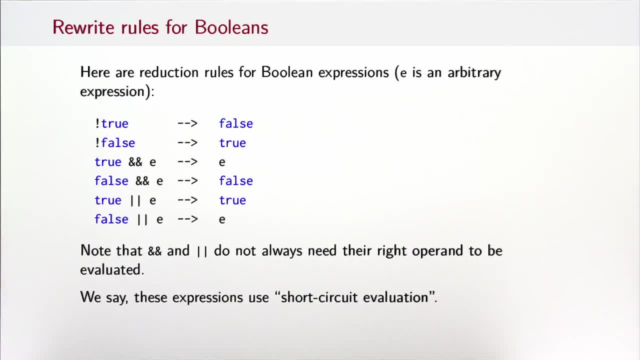 So that's the syntax of boolean expressions. What about their semantics or meaning? In fact, we can express the meaning of a boolean expression by giving a reduction rule similar to the simplification rules that we've seen so far. So here we would say that not true gives false. 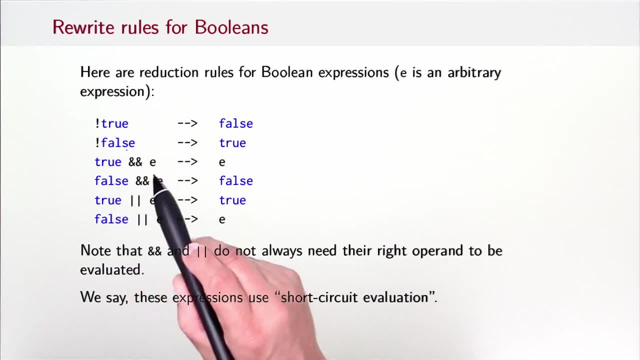 not. false gives true, Then true and some arbitrary expression gives that expression. and false and some arbitrary expression always gives false. True or some arbitrary expressions gives true and false, or some arbitrary expression gives that expression. So why did I write it this way? 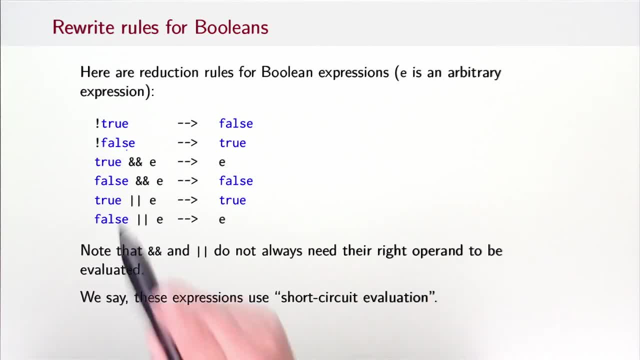 Well, one particularity here is that for these evaluations you don't need to have a value. here I said it's an arbitrary expression, So if I have something, for example something like, let's say true or loop, where I assume now that loop is a function defined on booleans- 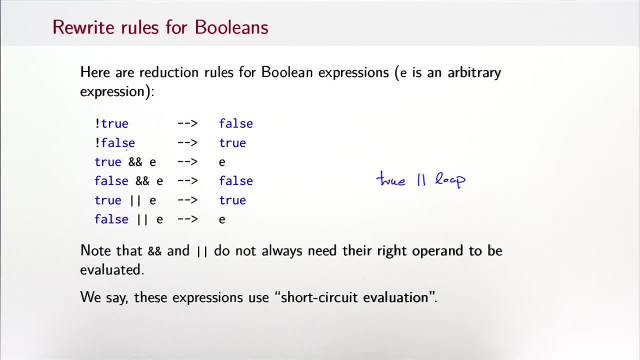 but that's still loops. So is that an expression that will terminate or not? In fact, it will terminate. I just used the rewrite rule that I have seen here And I said: well, that reduces to true. So this idea that sometimes we actually do not need to evaluate expressions. 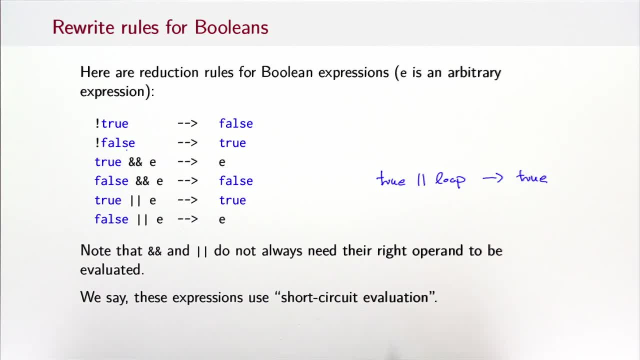 to know the result is called short-circuit evaluation, And most programming languages have boolean expressions that use short-circuit evaluation, and Scala is no exception. The difference and the nice part is that, instead of having something very operational, we can explain what a short-circuit evaluation is simply by giving the rewrite rules. 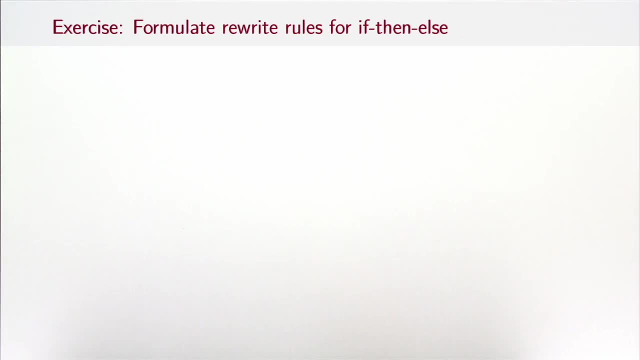 So, as an exercise, what would rewrite rules for if-then-else be? We have a boolean- conditional expressions. We should fill it with meaning. So let's set that up and say: well, if we have an if-then-else and the condition is: 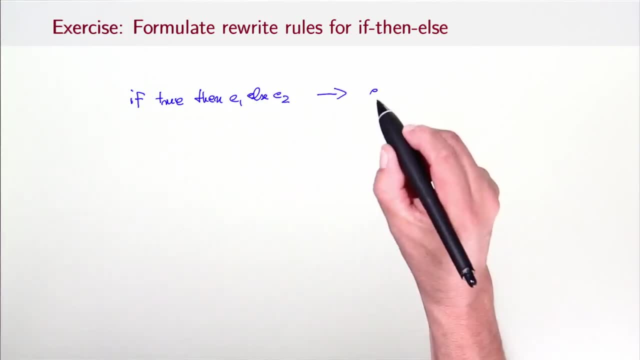 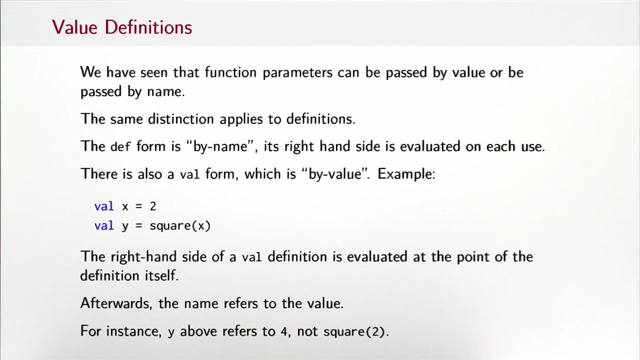 true, then that rewrites to the first part, e1.. On the other hand, if the condition is false would rewrite to e2.. So much for conditionals. Now. the second construct we're going to look at in this unit is value definitions. 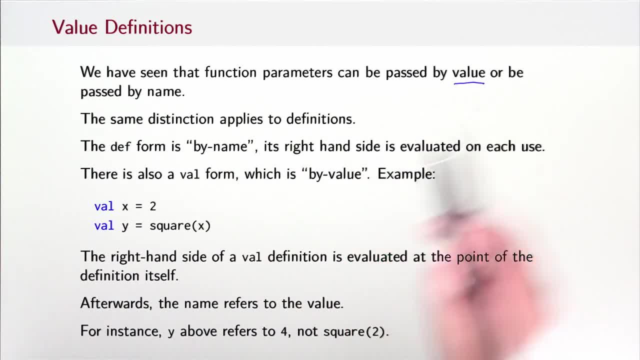 So we've already seen that function parameters can be passed by value or by name, as expressions or as values, And in fact the same distinction applies to definition. What we've seen so far is the def form of definitions, and that one is by name. 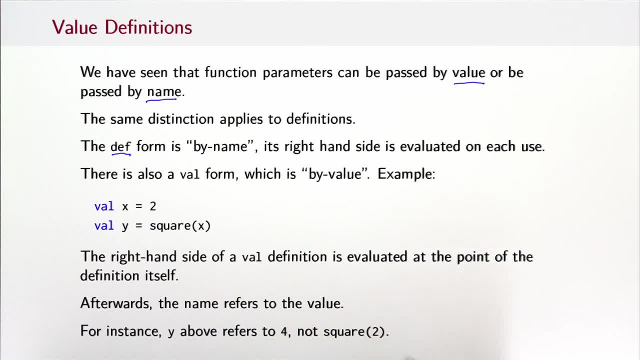 We said that each time we mention the name, we replace the name by its right-hand side by the full expression. There's also a val form which is by value, as the name implies. So, for instance, if you write val x equals 2, and then val y equals 1,, and then you have. 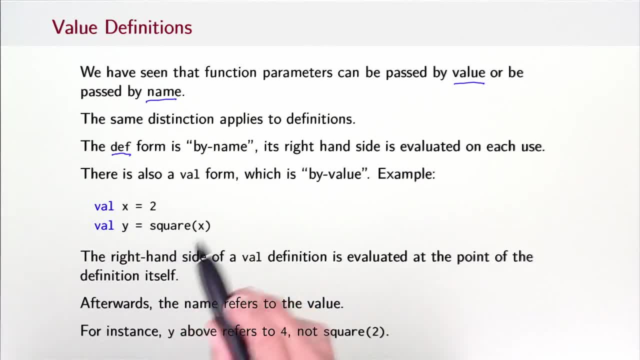 y equals square of x, then the right-hand side of that definition will be evaluated immediately at the point of definition. Afterwards, when you write y, you will essentially replace y not with square of 2, but immediately with 4, with the value that you have already pre-computed. 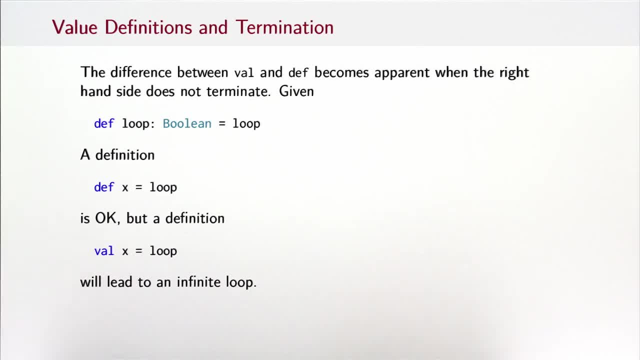 The difference between val and def becomes apparent when the right-hand side does not terminate. So if you have a function like loop boolean equals loop again, then if you have a definition x equals loop, then that's okay, but a definition val, x equals loop. 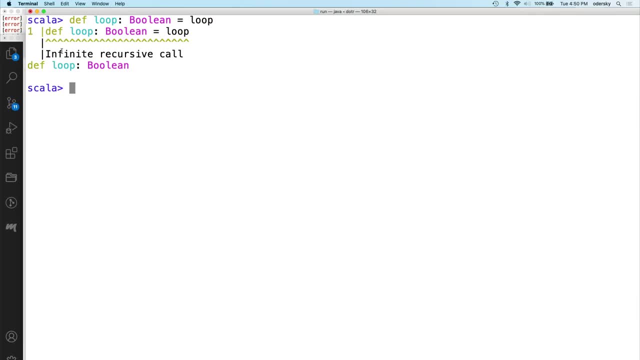 would lead to an infinite loop. So here's my loop function. Instead, our wrapper is smart enough to detect that this is an infinite loop and it warns us with infinite recursive core. But that yellow expression here and the yellow twiddles, that's just a warning. 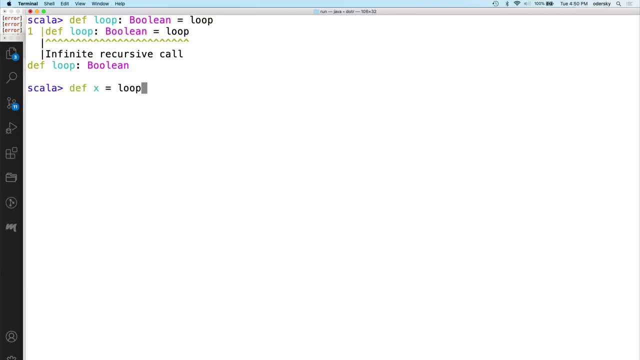 We can still use loop, for instance like here, And that's fine. So we have defined x to be equals to loop, So we are still in the REPL. On the other hand, if we would write val x equals loop, what would happen? 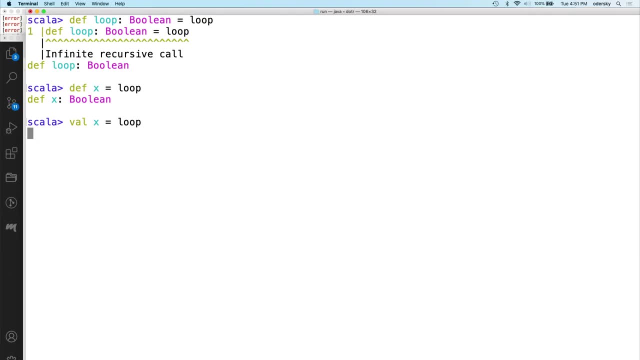 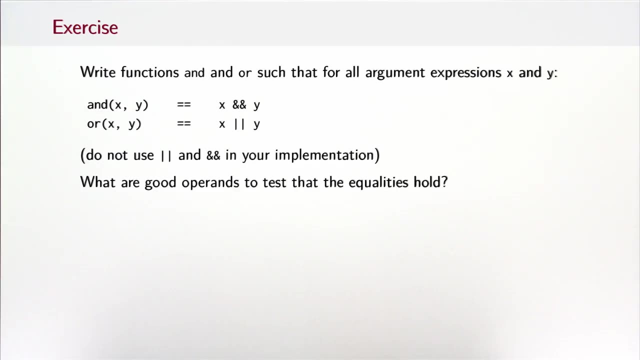 Well, nothing, That's the infinite loop for you. We have to take it out with control-c, And that will lead us back to the command line. So here's another interesting exercise: Write functions, AND and OR such that, for all argument expressions, AND is the same. 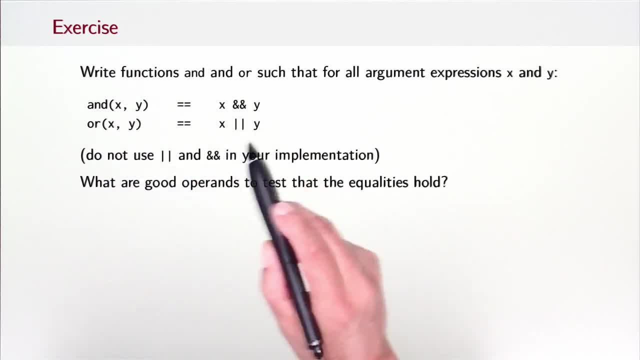 as X AND Y And OR is the same. It's the same as X double bar Y. Of course you should use not the double ampersand and double bar in your implementation, otherwise it would be too simple. What are good operands to test that the equalities hold? 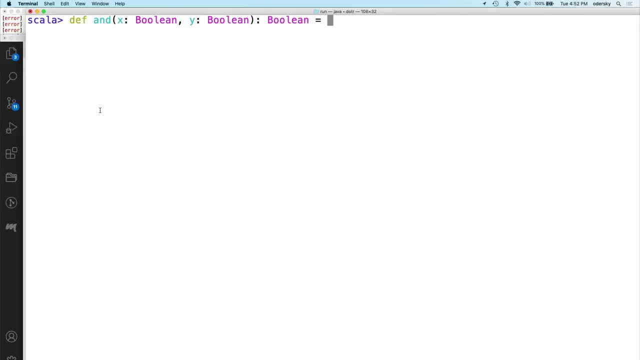 Okay, so I'll show you how to do it with the AND function and I'll leave the formulation of the OR function to you. So here's the signature of AND. It takes two booleans and gives back a boolean. How could we implement it? 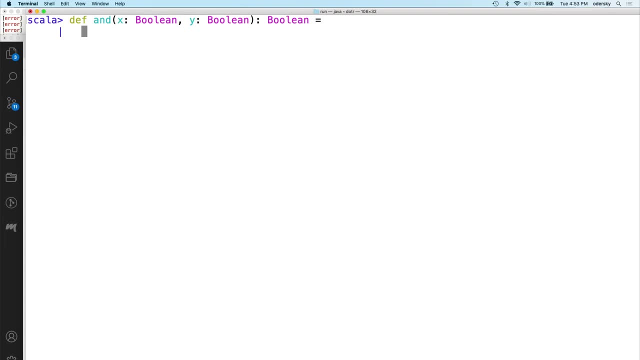 Well, we're not allowed to implement it. We're not allowed to implement it, We're not allowed to use ampersand, ampersand, But we can use an IF. So let's see If X, so if X is true, then the AND of true AND something else. what did our rewrite rule? 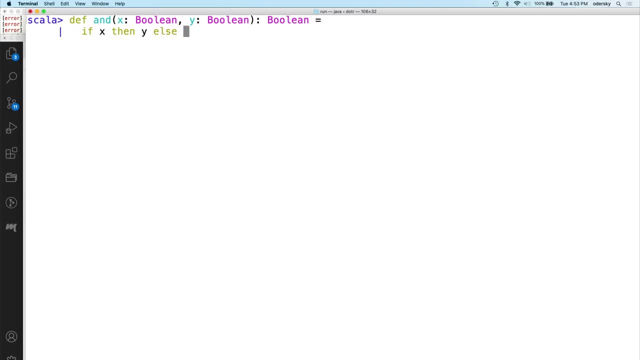 say, Then it's the, something else, And if X is false, then our rewrite rule said that the whole result will be false. Okay, so we have defined the AND function. Now let's test it, Let's see: AND- true, false. 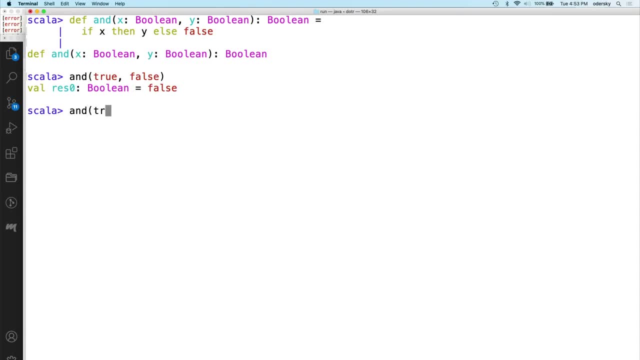 And true false That gives false AND true true That gives true. And you trust me that the other combinations will also hold. But is that everything that we need to test it with? No, In fact, we should also test it with non-terminating expressions, because short-circuit evaluation. 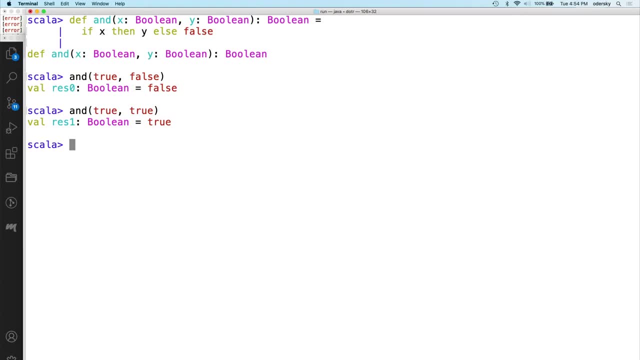 can handle those as well. And we said: AND should behave just like double ampersand, so it has to handle those. So let's see What would we, What could we do with AND false loop, So that should give false right. 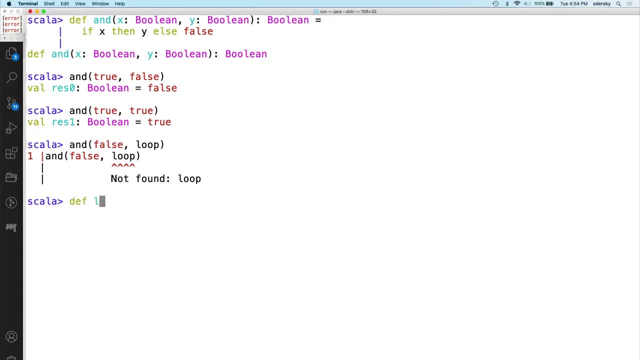 Oops, I haven't defined loop yet, So let's quickly do that. And AND false loop. Oops, we got non-termination. So where did we go wrong? Well, in fact, it turns out that the second parameter, the Y parameter, 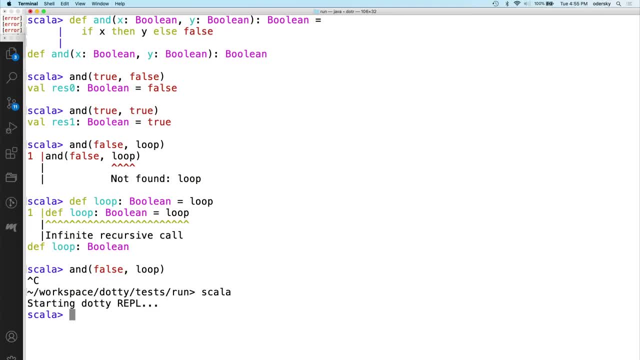 That one is called by value, And that means that the expression, in this case loop, will be evaluated, And that's not what we want. So let's change that and make it called by name. So we add an arrow in here. 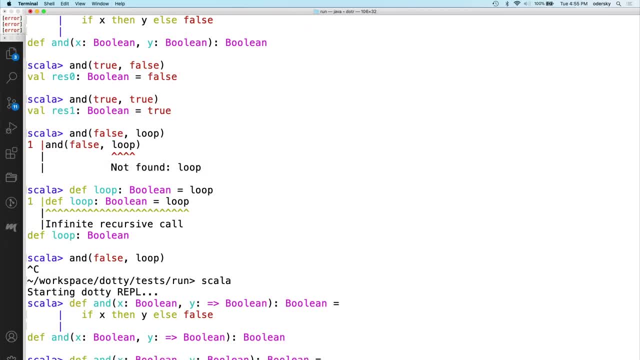 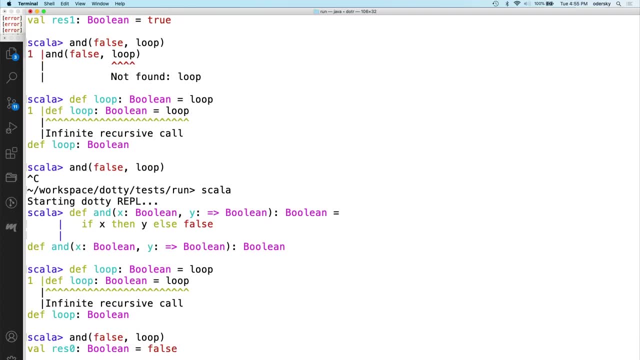 And now we test it again. We have to define loop first, And now we can define the test case, And now it works. So with that change in the definition of AND, it turns out that all the test cases that we need actually pass. 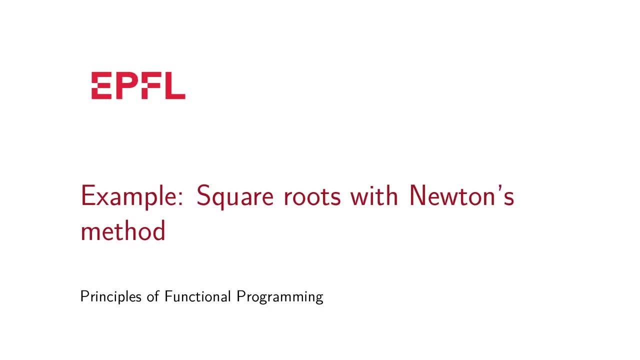 Okay, I think you're ready for your first example, which is a little bit larger than a single line. What we're going to do in this unit is define a function. We're going to define a function. Define a function to compute square roots with Newton's method. 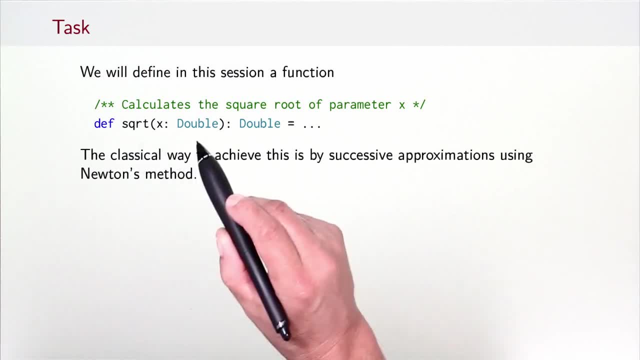 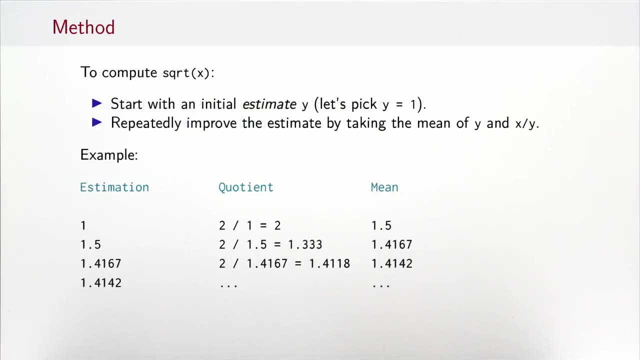 So, specifically, we define a function def square root which takes a double parameter and returns a double result, And it calculates the square root of the parameter x. The classical way to achieve this is by a successive approximation technique that dates back to Isaac Newton. 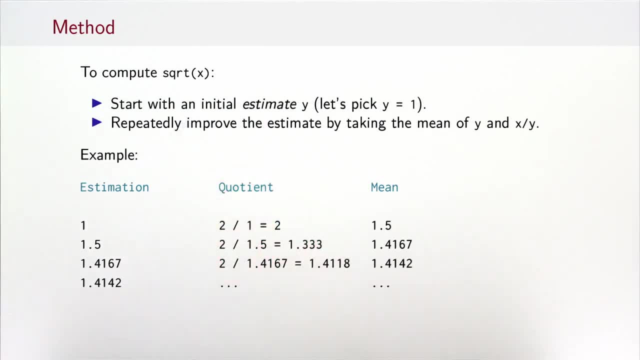 So the idea is as follows: To compute square root of x, we start with an initial estimate, Let's call it y and pick: y equals 1. And then we repeatedly improve the estimate by taking the mean of y and x divided by y. 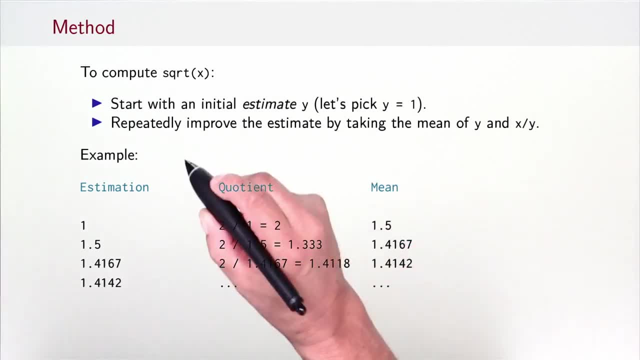 So let's look at the first elements of the sequence of computing square root of 2.. So we start with 1.. The quotient then would be: 2 divided by 1 equals 2.. The mean is 1.5.. Our next estimate is 1.5.. 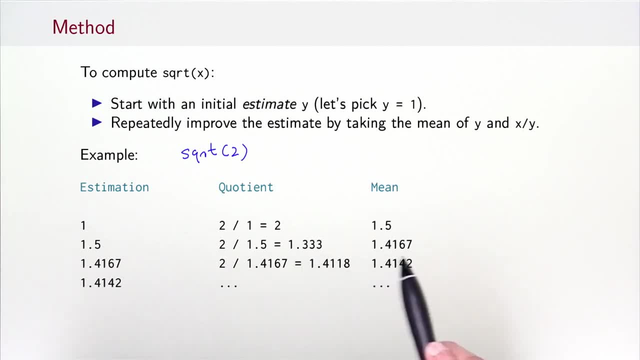 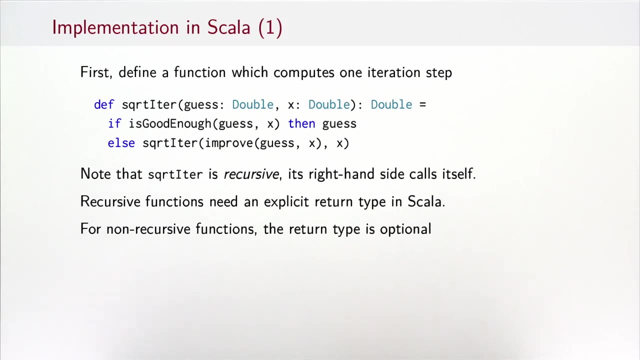 The quotient is 1.33.. And our mean is 1.4167.. And you see that it converges actually quite rapidly to the true value of square root of 2.. So let's define a program that does this approximation. Our first step towards this program is to define a function which computes one iteration. 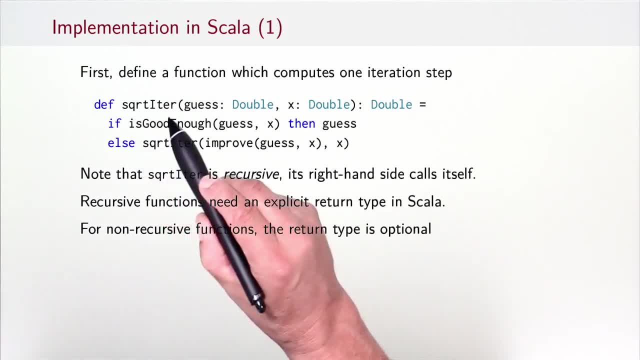 step, So the iteration step, call it square root iter. for square root iteration It takes a guess, an estimate, And the value for which we want to compute. And the value for which we want to compute, We compute the square root, which is called x here. 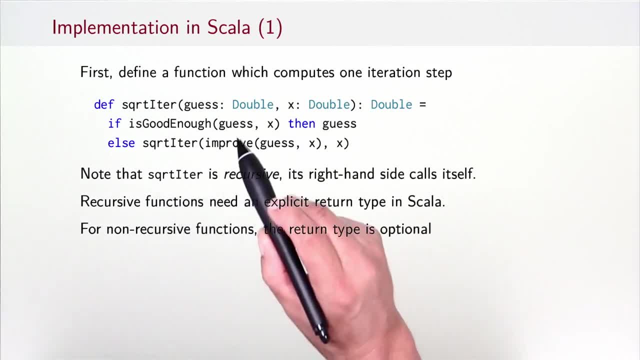 And the implementation says: well, if the guess is good enough already, it means close enough to the real value. then stop and return the guess And otherwise we call square root iteration, again with an improved guess and the original value for which we want to take the square root. 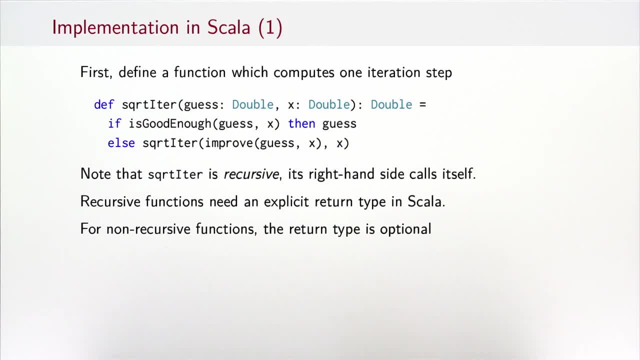 So this example already shows two quite fundamental techniques of functionalization. One is we split our program up into lots and lots of small functions, And the second one is we make use of recursion. Here we have square root iter that calls itself with an improved guess, unless the guess is. 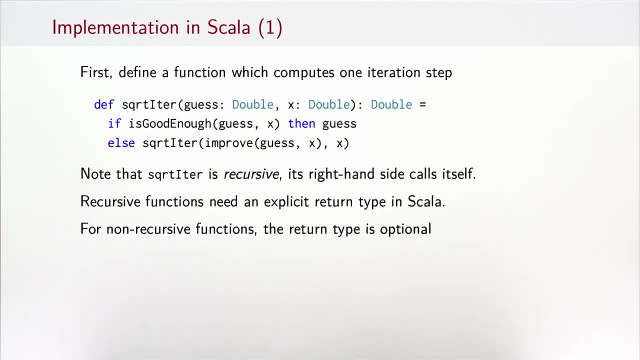 already good enough in which it terminates. Recursive functions need an explicit return type in Scala, otherwise the type inferencer will get confused. so we have written colon double here. For non-recursive functions The return type is optional. However, if a function is public, that means used by others than yourself, then it's always. 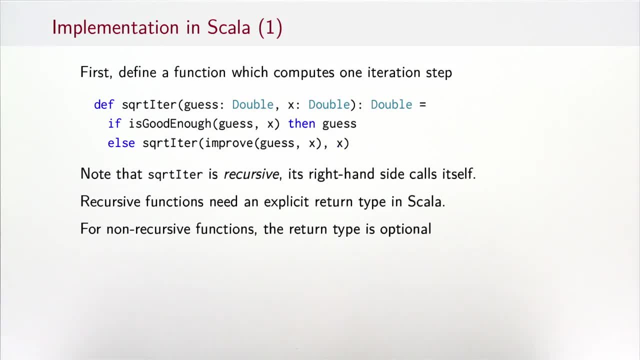 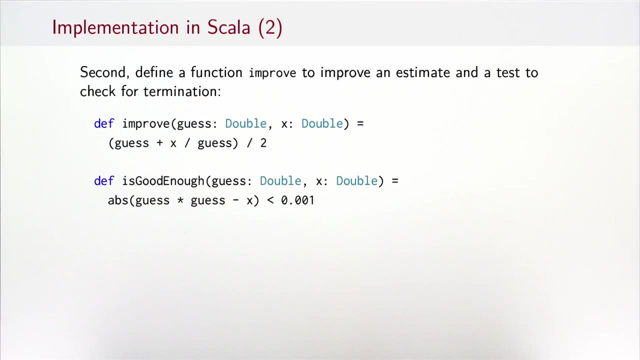 good practice to add a return type for documentation. So our high-level design has left two things open: First, how to define is good enough And second, how to define improve. So let's get to these now. Improve is straight out of the textbook. 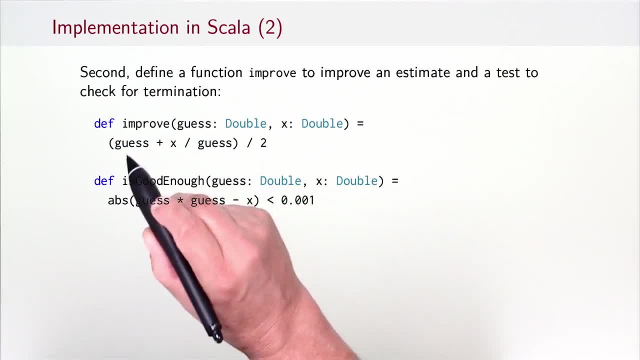 We say to improve a guess we take the mean Between the original guess and x divided by the guess. So the mean is the sum divided by two Guess plus x divided by guess. divided by two, For is good enough. we have a number of possible choices. 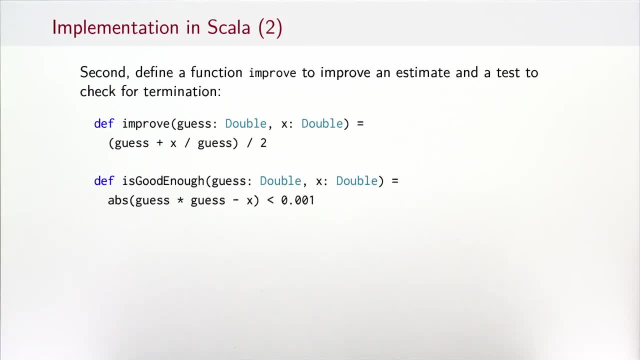 Here we pick a particularly simple one, which we will improve on later. So our choice for is good enough. just says: well, take the square of the guess and the difference between the square and the original value, and that must be a small number. 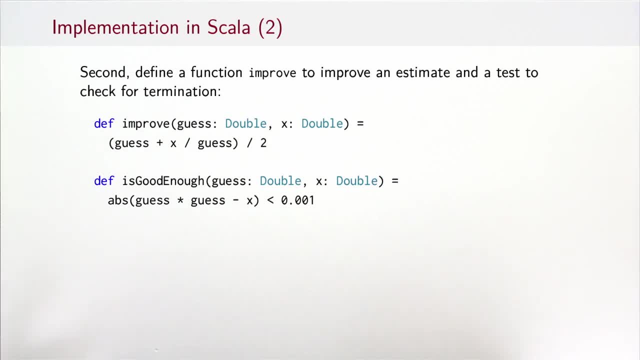 So a guess is good enough If the guess multiplied by x By itself is close to the original value x. So now we're almost done. We just have to define the square root function, which is square root iteration with the original guess. 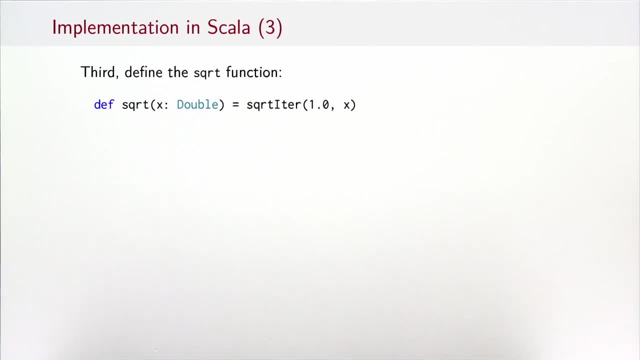 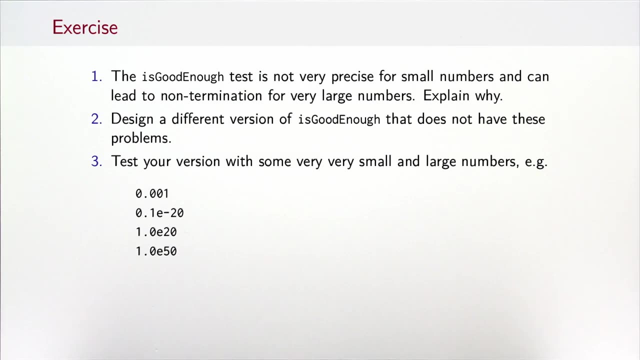 We pick 1.0 and the value x and we're done. So here's an exercise for you. I suggest you take out the Scala REPL type in the function or copy them and then play with it. So one shortcoming of is good enough is that it turns out it's not very precise for small. 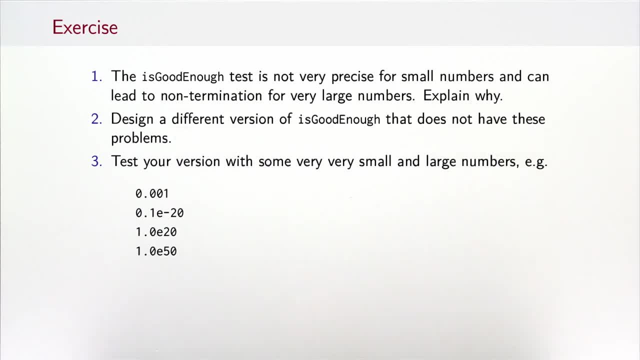 numbers x, and it even can lead to non-termination for very large numbers. Can you explain why? So, to explain why you have to know a little bit about floating point numbers. If you don't know anything about floating point numbers, then after you can skip this. 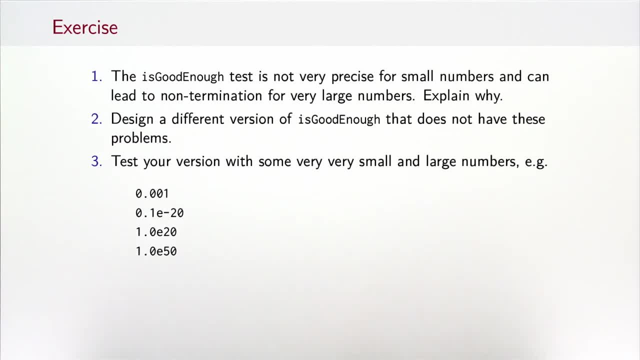 exercise. knowledge of floating point numbers will be, by and large, not necessary to complete this course successfully. Second, If you know what the problem with this good enough test is, Then you define a different version that doesn't have the problems. And three, 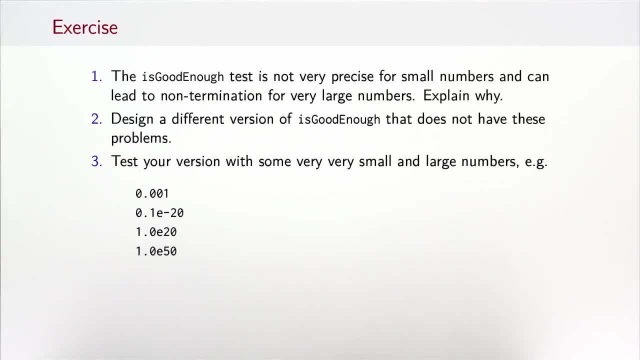 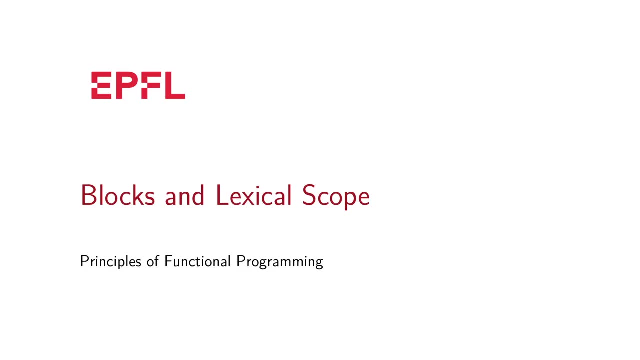 Test your versions with some very small and some very large numbers. For instance, try to take the square root of 0,, 0, 1 or something even smaller, or something very large or something even larger than that. In this unit we are going to stay with the square root. example. 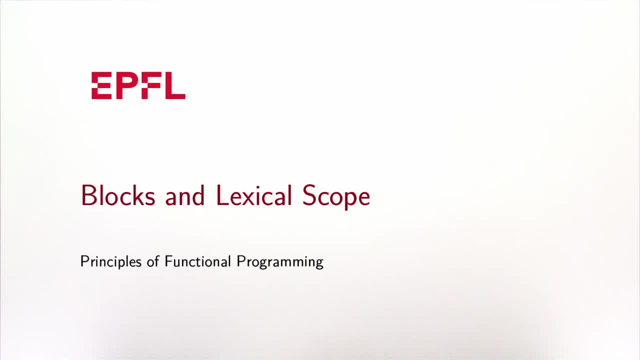 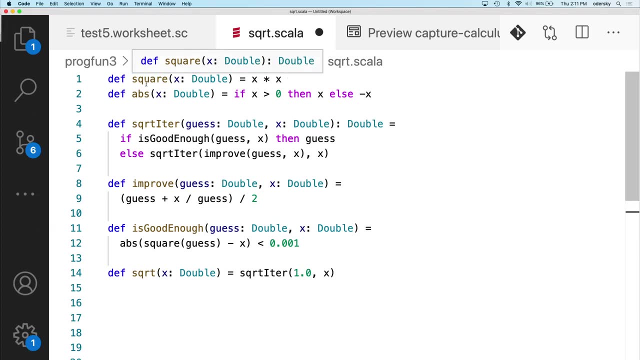 And learn several tools. So let's get started. First of all, let's take a look at some of the techniques, how to organize it better. So I've written all the essential things we did last week into this editor in a program called square root dot Scala. 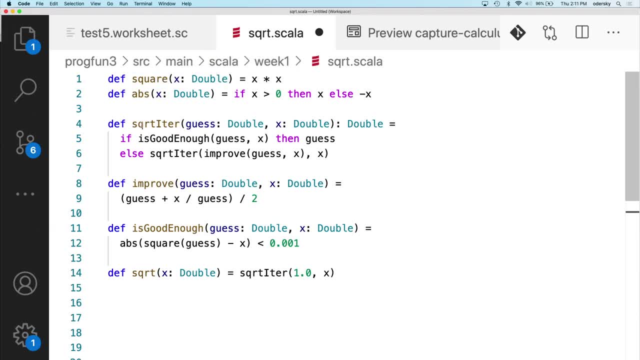 So you see here the square method, The square root, iter, improve is good enough And finally, square root, We can also add a test method. So here's the test method, And here's the test method, And we can also run it. 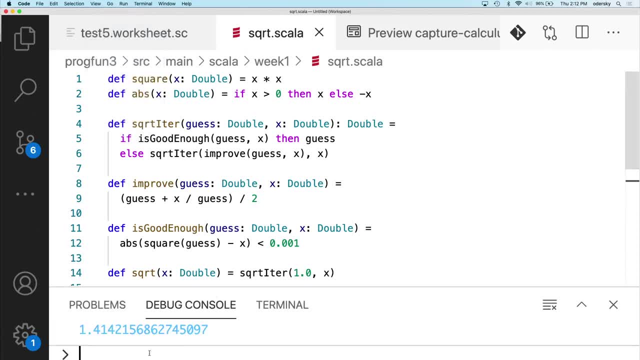 Let's open the debug console here, And that gives us the number, the square root of 2, as expected. Now, things are fine so far, But there's one problem, And that problem is that we have many, many functions that essentially all sit here: equals. 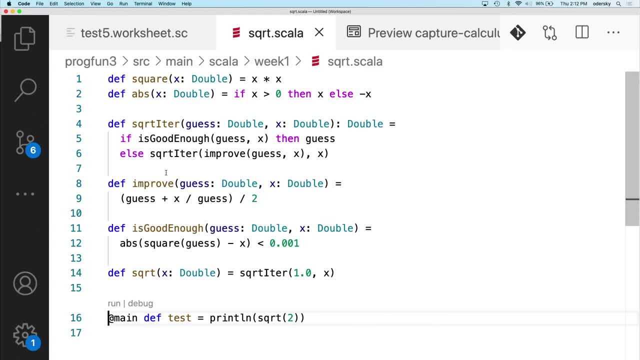 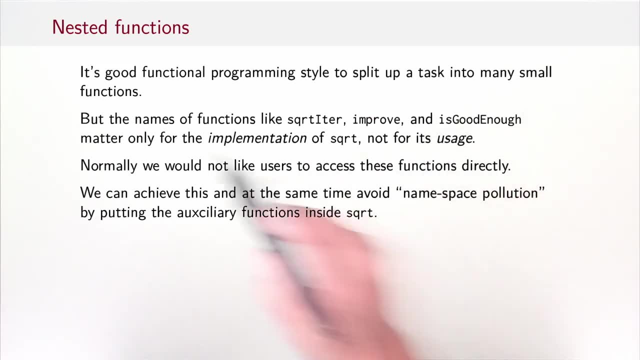 One is equal to the other And they're all together pollute a little bit the global namespace. So in fact, Let's see, In fact it's good programming style to split up a task into many small functions. We've seen that in the last week. 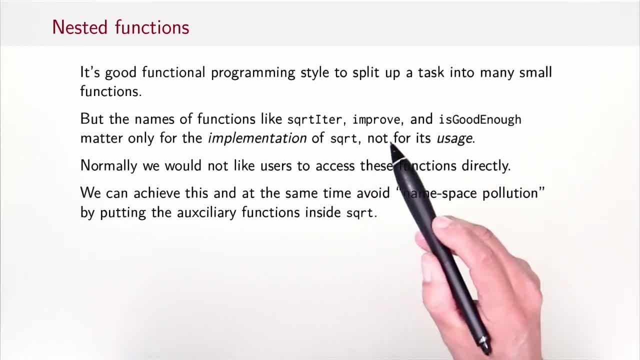 But it turns out that the names of the functions- square root, iter, improve and is good enough- They really matter only for the implementation of square root, not for its usage. So normally we wouldn't like users to access these functions directly. So if a user shouldn't access the functions, then why should they be there, visible and 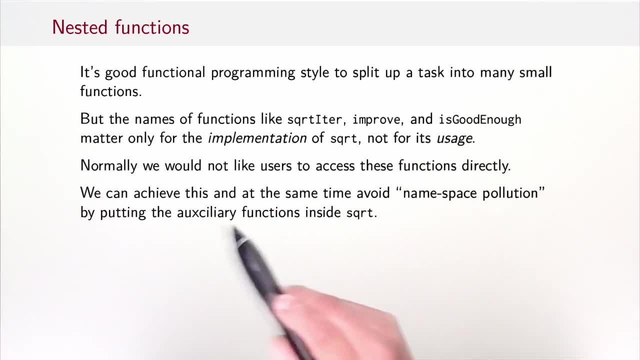 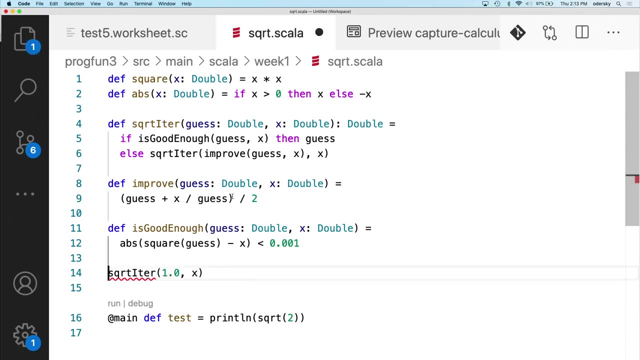 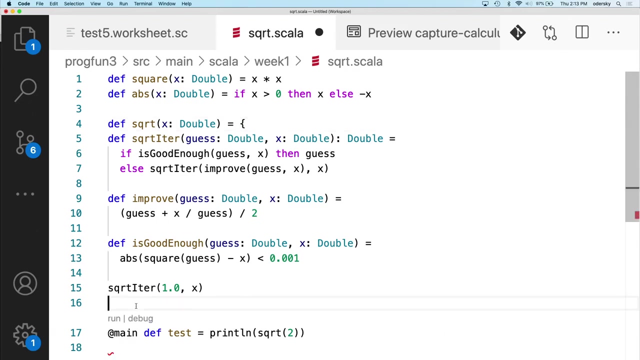 callable to the user. So we can achieve The hiding of the function and avoid namespace pollution by putting the auxiliary functions inside square root. So let me do that in this example I take: I take square root, Put it on top And then put everything inside. 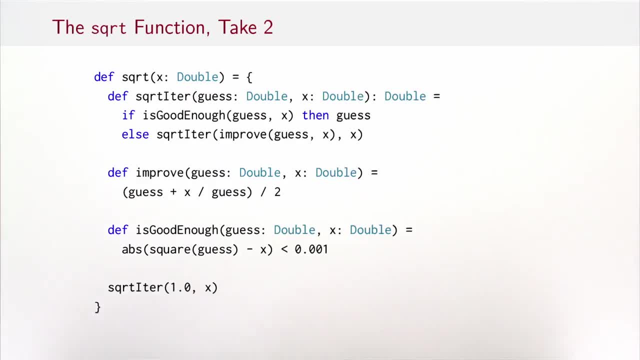 So now it's going to look like this. So here you see that the square root iter improve and is good enough. Now, all inside square root and square root itself, the body of square root. It consists of this last statement, which in turn is called square root iter and starts: 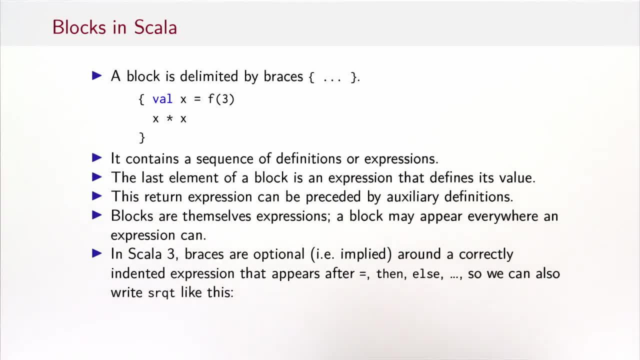 the iteration. So what we've seen here is a block. A block is delimited by braces. Here's a simple example of another block. It can contain definitions like a well definition. here, Or in the square root example, we've seen several def definitions. 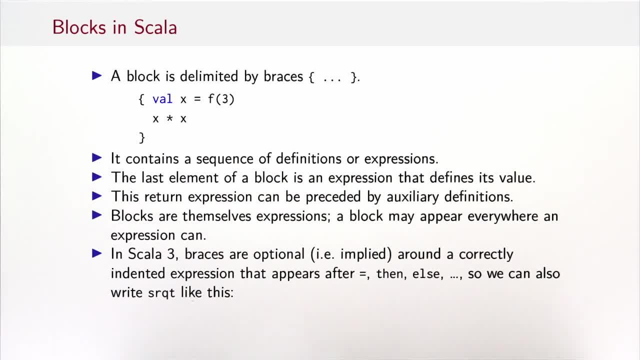 And then it ends in a final expression, And that expression is the result of the block. A block is itself an expression, So a block can appear everywhere an expression can, And furthermore, in Scala 3, the braces are optional around a correctly indented expression. 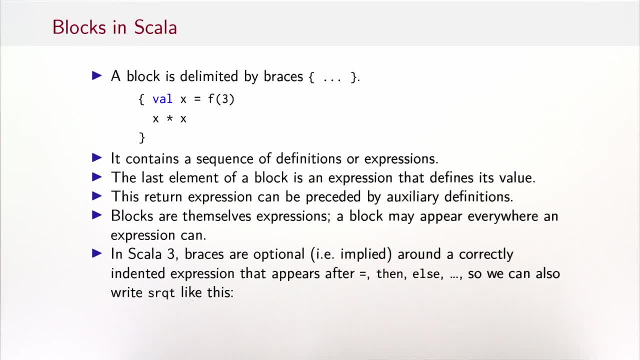 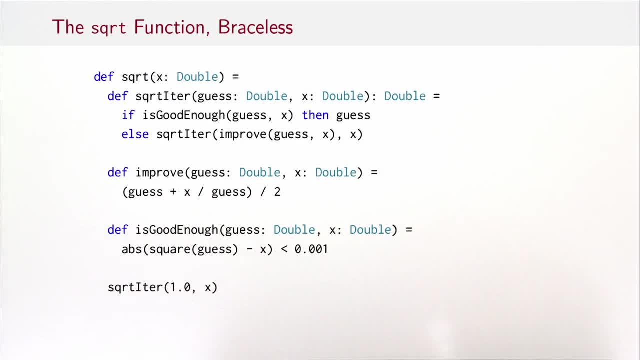 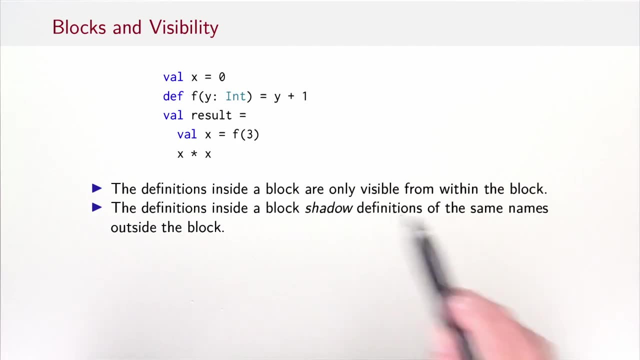 that appears after equals, then else and so on. So we can also write square root like this: We can leave out the braces And that's it And have it look a little bit cleaner. So blocks influence visibility. In fact, the definitions inside a block are only visible from within the block. 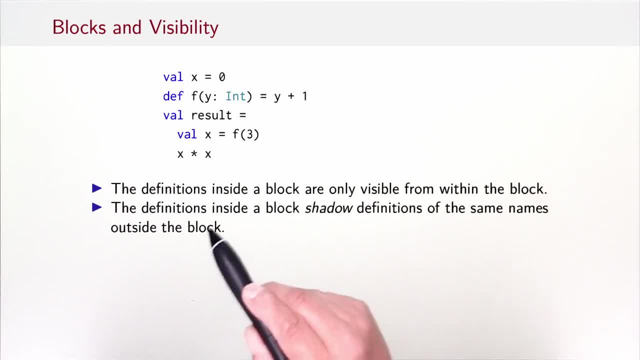 They cannot be accessed from the outside, And furthermore, the definitions inside a block shadow definitions of the same names outside the block. So, for instance, in this case, here the value x, it would go to this x, which is the definition inside the block, which is implied by the indentation. 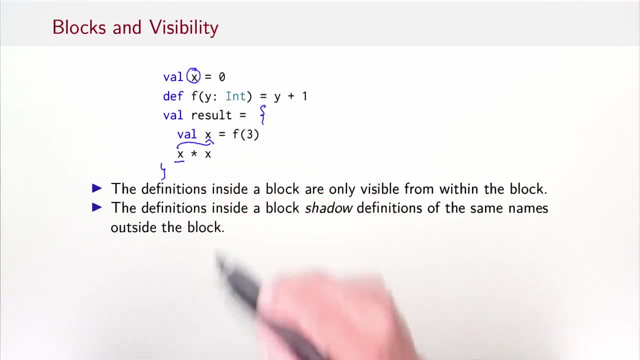 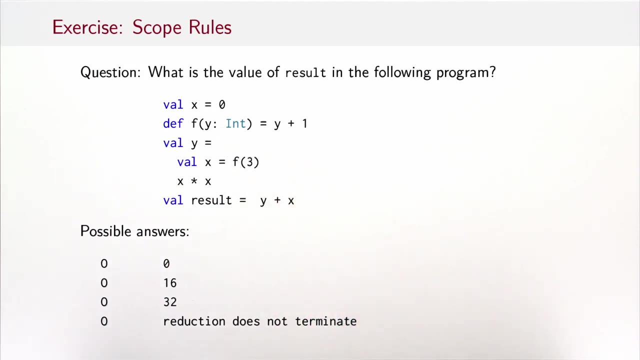 It wouldn't go to this outer x. The outer x is essentially shadowed. That's a shadow from the inner x that essentially hides the outer x here. So let's put this to an exercise. We have another program here: lots of uses of x and y. 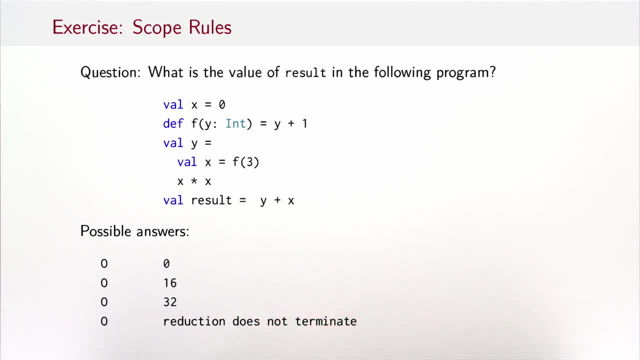 What's the value of result in that program? Take a look and digest it a little bit and then answer. The possible answers are x, They are 0,, 16,, 32, or. reduction doesn't terminate, So let's see. 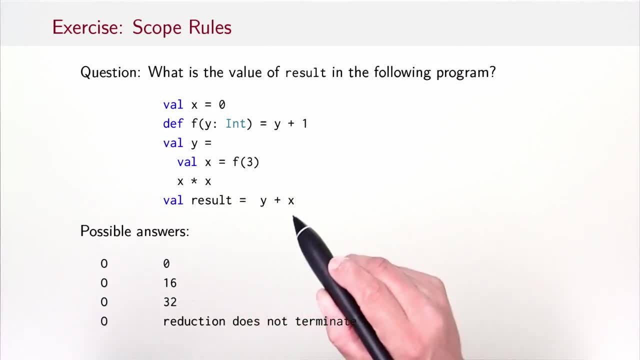 The result expression consists of the y plus x. So where does the y go to? The y gets accessed. the y here. It certainly doesn't see the y here because that's a parameter. so it's local to the def here. Where does the x go? 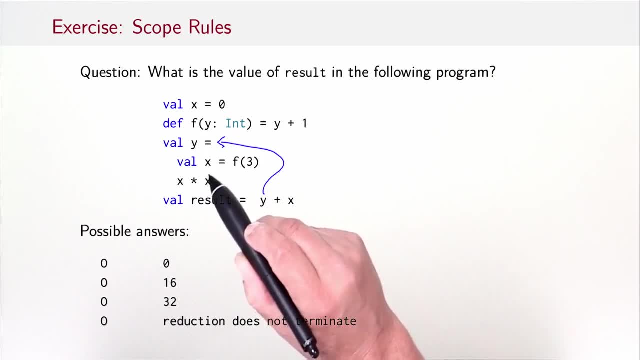 Well, the latest definition of the x was here, But again, the x is inside the block which is implied here, So it's not visible at this point. So that means the x goes here. Okay, So the x is definitely 0 here. 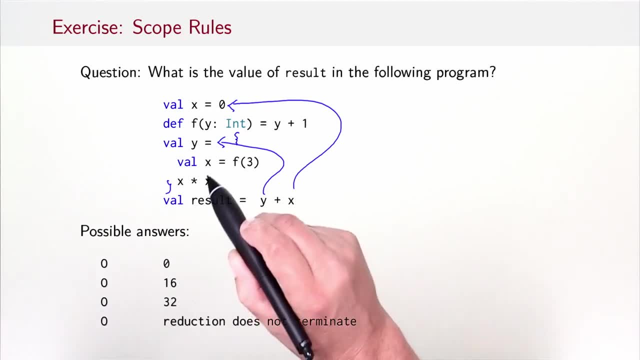 What's the value of y? Well, the value of y says it defines its own local x, which is f of 3.. f of 3 would be the parameter 3 passed to y, So that would be 3 plus 1 equals 4.. 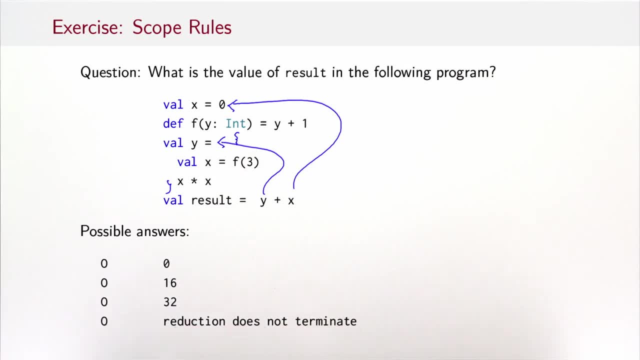 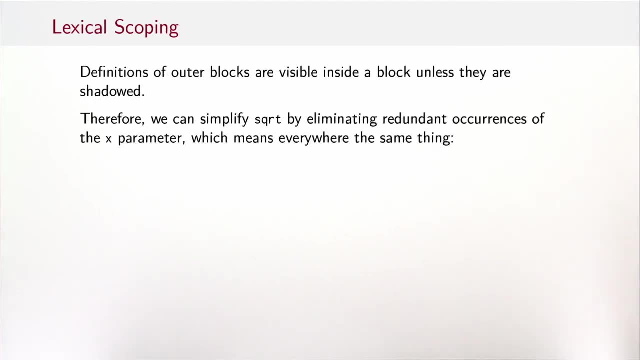 And then it returns x, So that's the value of y 6 times x, So that's 16.. So 16 plus 0 is 16.. So 16 is the correct answer. So one consequence of lexical scoping is that definitions of outer blocks are visible inside. 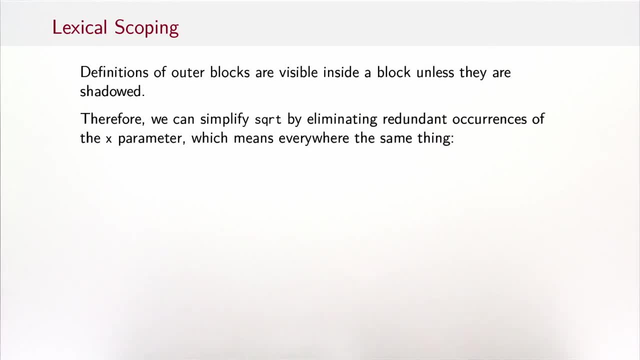 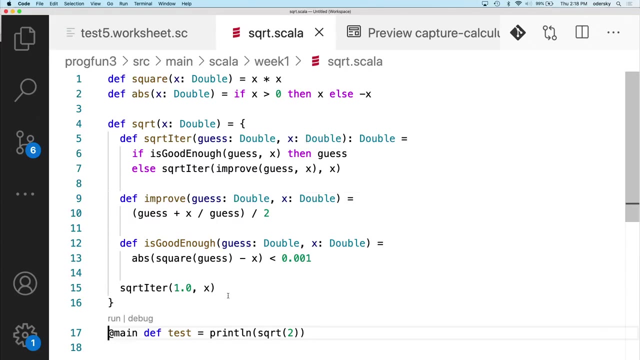 a block, unless they are shadowed, And that's actually very useful because that lets us simplify square root by eliminating redundant occurrences of the same parameter, the x parameter, which means everywhere the same thing. So we see here that the parameter x is repeated all over again and it's always the same value. 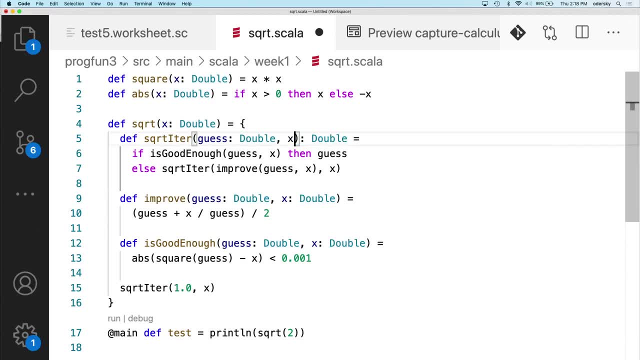 It's always passed as x again to the result. So what we can also do is we can simply delete it in all the nested occurrences here, here and here, And the program would still work. Now we get errors. Why do we get errors? 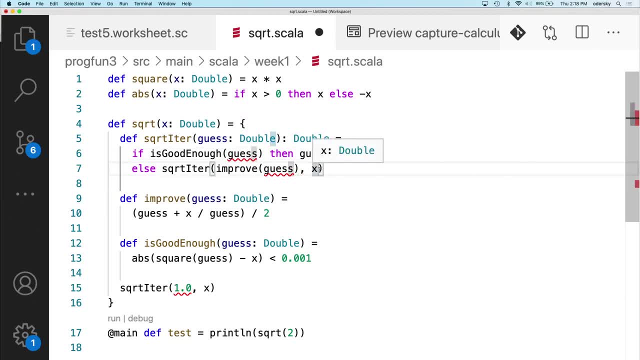 Well, because we have passed it on. Okay, And we need to pass it on because it's no longer a parameter, So we can simplify the calling positions as well. Now we have a program which is shorter, clearer and does exactly the same as the previous. 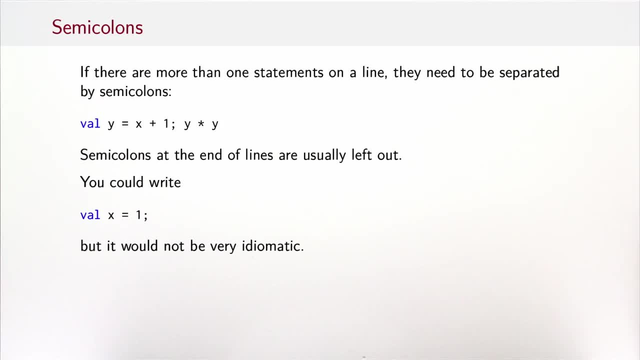 one. So so far we have seen definitions and expressions, And definitions and expressions together are called statements. And again, so far we used one line per statement. Every statement was on its own line. But in fact we can write more than one statement on a line, but then they need to be separated. 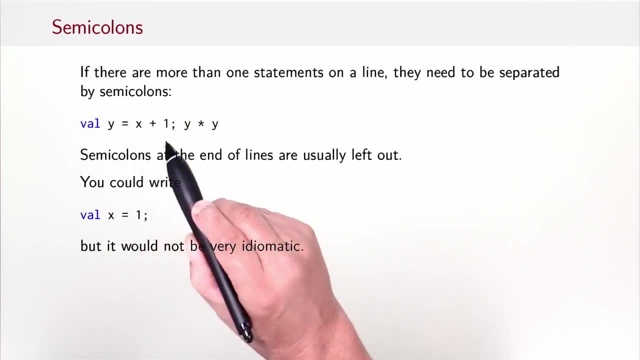 by a semicolon. So here you have an example. You can have a definition of y and then you immediately follow that with the expression y times y. But here you need a semicolon, otherwise it wouldn't work. Semicolons can be written at the end of lines but are usually left out. 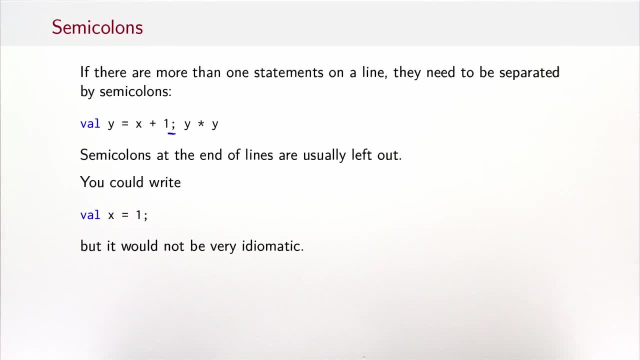 So if you write this, then that probably means that the person came recently from a language that required semicolons, such as Java. It isn't yet used to the new style that leaves the semicolons out. In fact, one way to use Scala is very much as an imperative and object-oriented language. 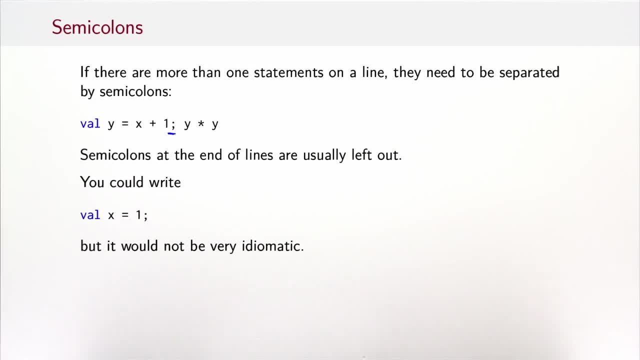 in the style of, let's say, Java or C-sharp, And if you use it that way, then often people say Scala is like Java, without the semicolons, because you don't need the semicolons. But in fact there's much, much more to Scala and to functional programming. 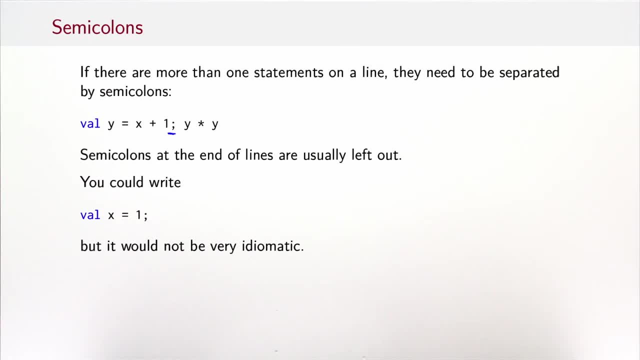 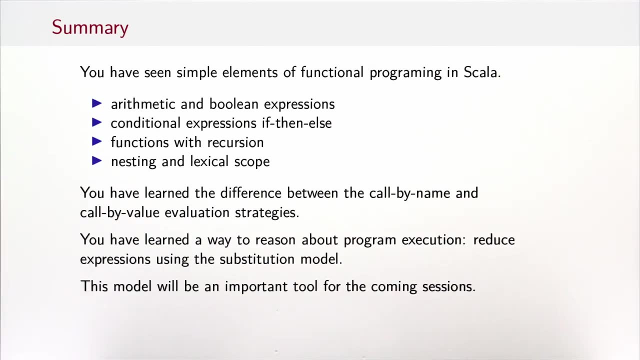 So this is essentially just typically the first steps in the long journey Towards a completely different programming style. So, in summary, you've seen simple elements of functional programming in the Scala language. We've seen arithmetic and Boolean expressions. We've seen if-then-else conditional expressions. 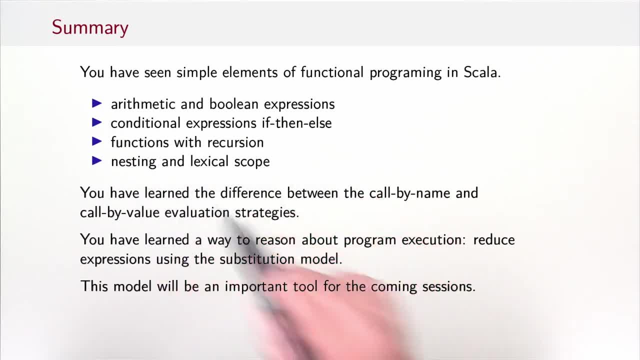 We've seen functions and recursion, And we've seen nesting and lexical scope. You've learned the difference between call-by-name and call-by-value, which are two really important concepts, And, even more importantly, you have learned a way to reason about the function of the 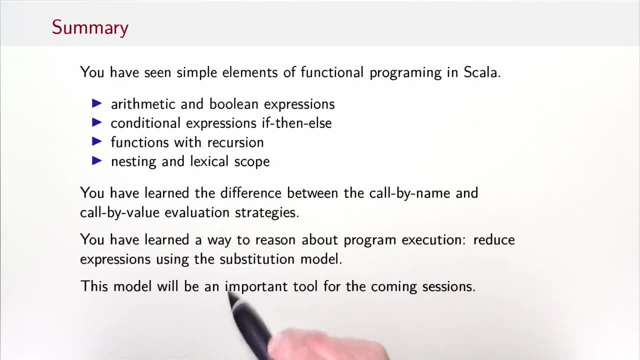 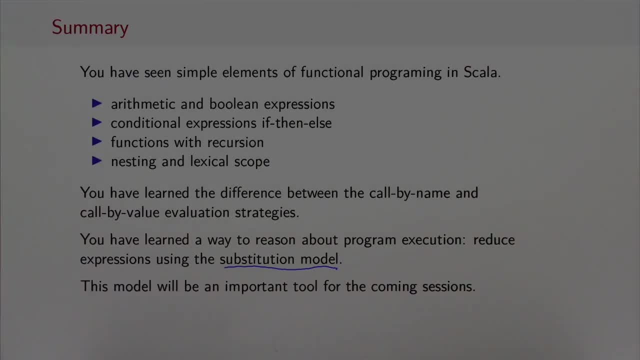 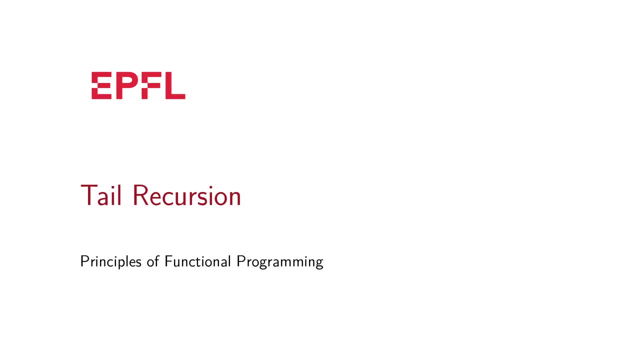 function. You've learned to reason about program execution. reduce expressions using the substitution model. This model will be an important tool for the coming sessions. So you've seen in the last sessions that recursion is a fundamental tool for functional programming, Whereas in an imperative language you would probably rather use a loop like a while loop. 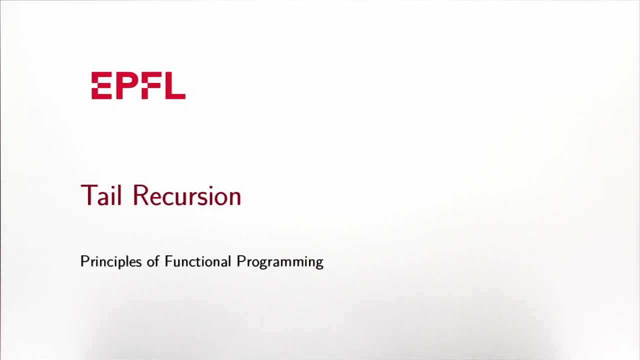 or a for loop. Now it turns out that recursion and loops have a lot to do with each other, And there is a form of recursion that is essentially exactly the same as a loop, So that form of recursion is called tail recursion, And we're going to find out more about it in this session. 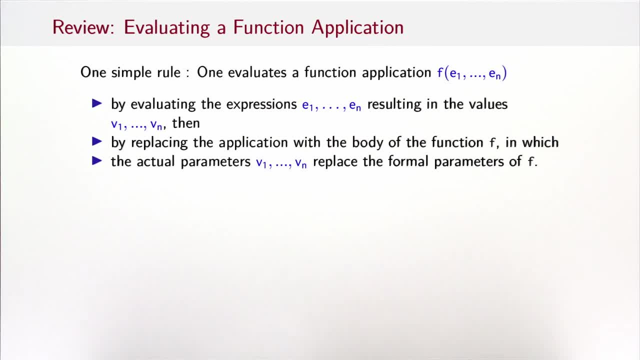 Before we do that, let's review again how we treat function applications in our evaluation model. So there's one simple rule. One evaluates a function application f, applied to arguments e1 to en, By evaluating the expressions resulting in the values v1 to vn and then replacing the 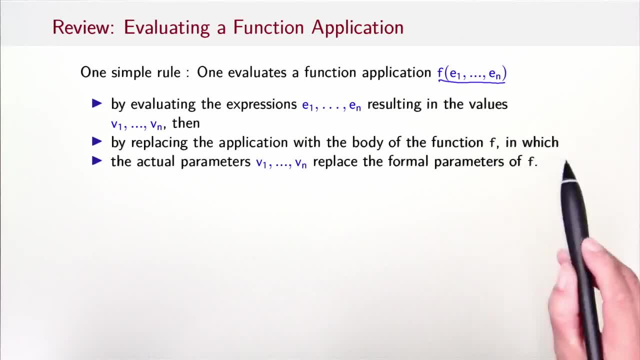 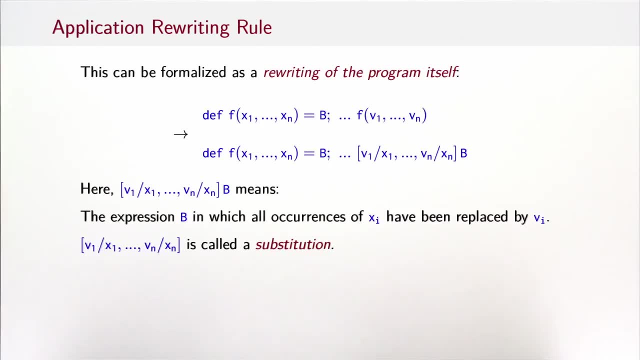 application with the body of the function f, in which the actual parameters values v1 to vn replace the formal parameters of f. Now that notion is so important that it warrants to have a notation for it, a specialized notation. So we can visualize that by a rewriting of the program itself. 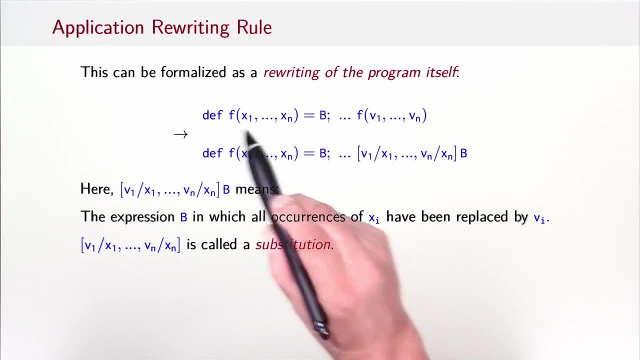 So Here we would have a program that has a definition of the function f with these parameters- I've left out the types and the body- And here we have a call of the same function, So that program can be rewritten to a program with the same definition and the same dot. 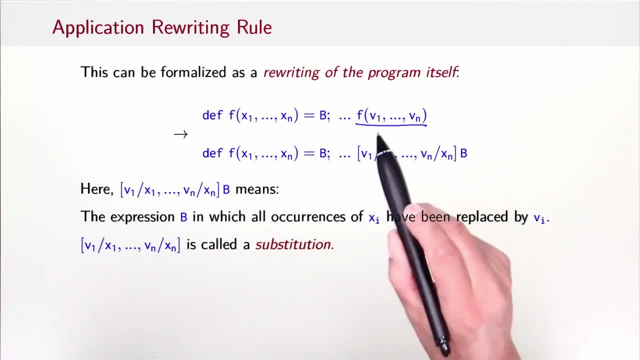 dot, dot in between, the filler in between here, But the call here would be replaced by the body with the substitution where every formal parameter x gets replaced by the corresponding value v. So this notion, with this in brackets: v1- slash x1, vn slash xn, that means precisely the expression. 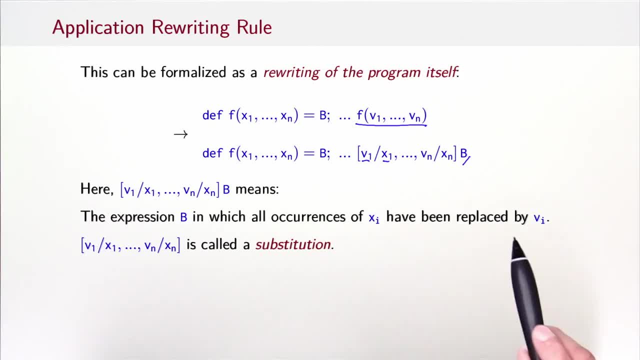 b, where all occurrences of an xi have been replaced by the corresponding vi, And that whole block is called a substitution, and that's where the name substitution model comes from, because essentially that's the core step of evaluation in that model. So let's do an example of this rewriting. 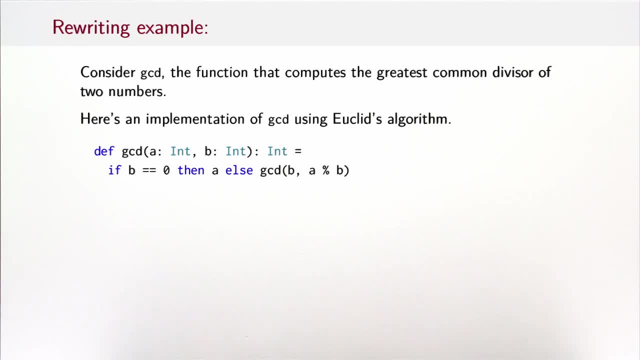 We consider a new function, gcd or greatest common divisor. So the greatest common divisor of two numbers is the greatest number that divides both a and b, And there's a very old algorithm that goes back to Euclid in the Antiquities, So that algorithm is like this. 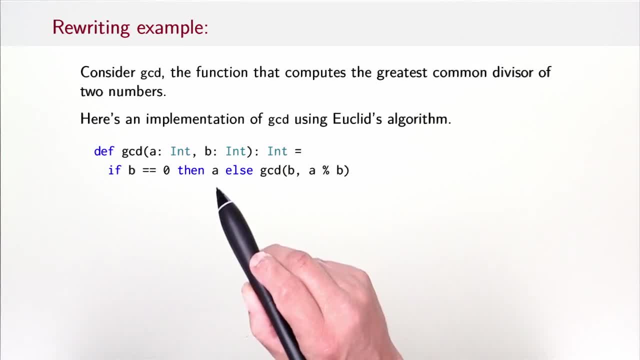 It says: well, if the second number is zero, then it's the first, And otherwise you call gcd again. with the first argument is now the second argument b, And the second argument is the first argument, a modulo b. So that operator- here the percentage is modulo- is a modulo operator in Java and also in Scala. 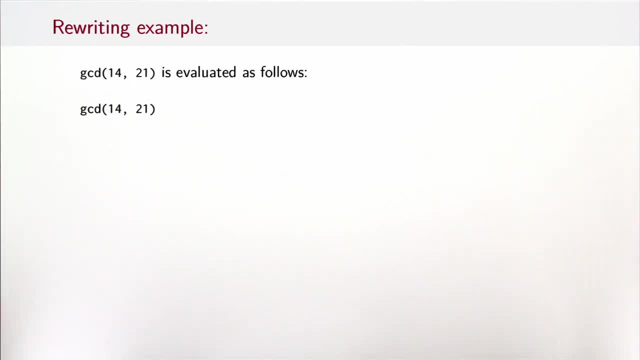 So now, if we have a call gcd, we can visualize its evaluation as follows. So we start with the call, then we expand it to the right hand side of gcd. that would be this one: here, with the correct parameters, We simplify the condition to false. 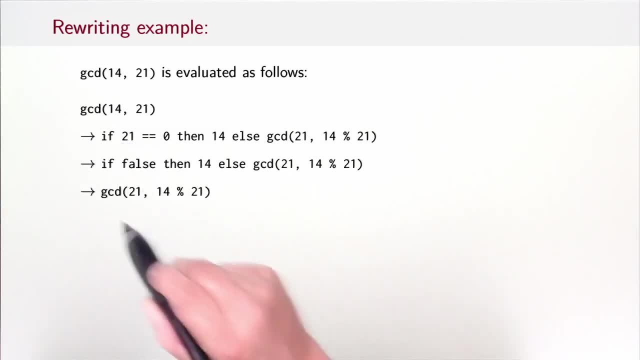 We simplify the if-then-else, since it's false. it's the else part. so it's this one here And we go on into the next call. Now we simplify the argument: 14 modulo 21 is 14.. And we go on, we expand to the call. 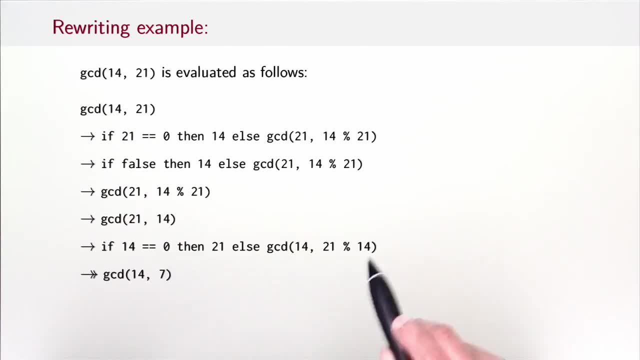 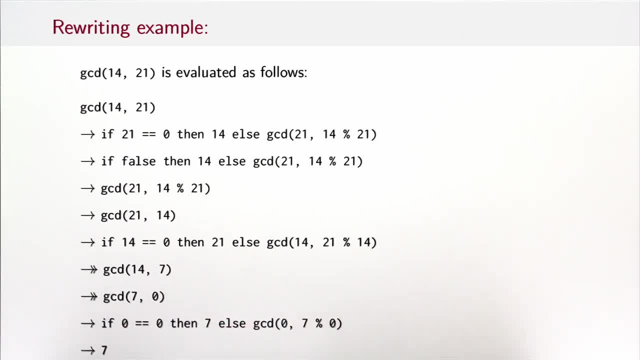 So this double arrow here means reduction by several steps, So I have left out some steps between here and here, but it should be clear what they are, OK. So now that we've seen that, let's try another function. Consider factorial. 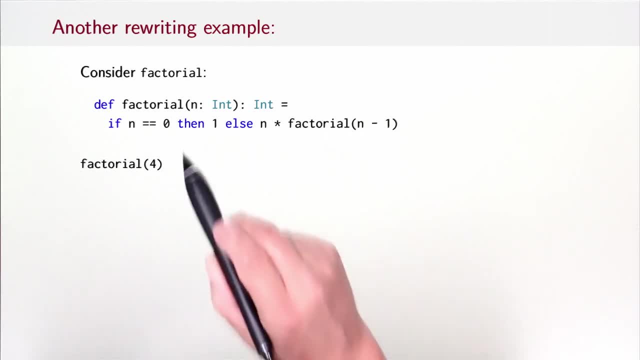 So if the factorial function is defined like this, it takes an int and gives you an integer result. It says: if the argument is false, then we can guide. it says: if the argument is 0, then the factorial of 0 is 1. Otherwise, the 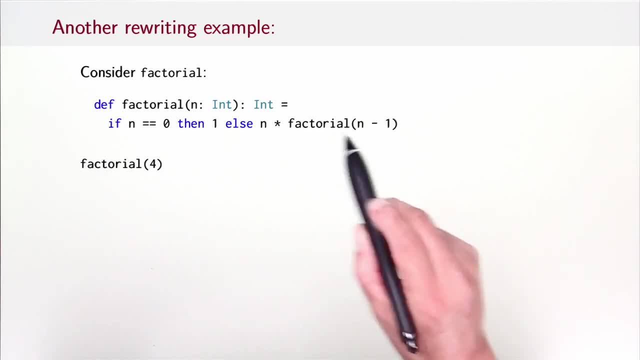 factorial is the number n times factorial n minus 1.. So let's consider factorial 4.. So that would be the body of factorial that we see here. So there's really two reduction steps: One is the body here and finally that one. 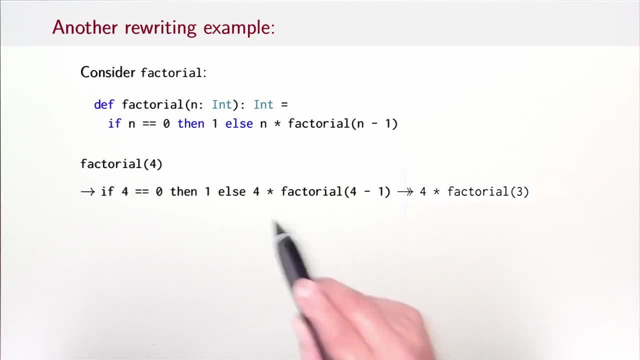 reduces to 4 times factorial 3, the right-hand side here. So if we go on, then factorial 3 reduces to 3 times factorial 2.. That reduces to 2 times factorial 1.. Finally, we have 1 times factorial 0. Finally we have the. 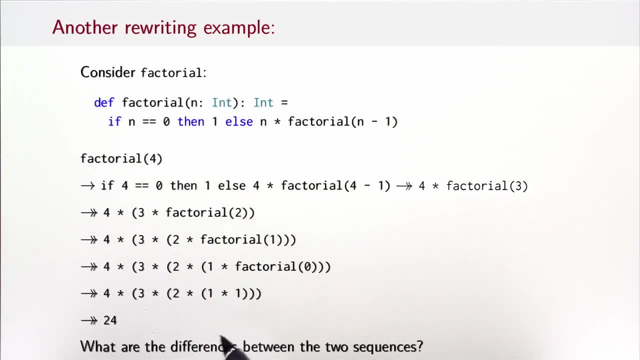 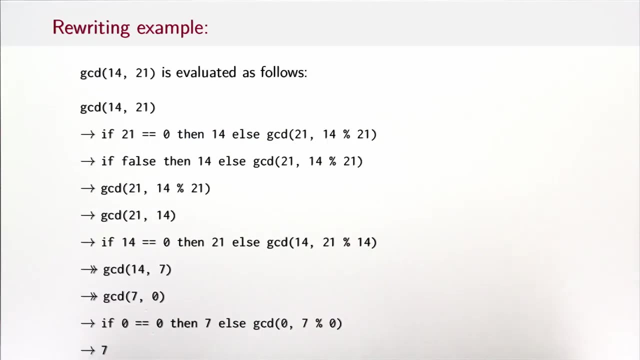 argument equals 0. So that would give us 1. And then, finally, the whole reduction will go back to 24.. So do you see a difference between the two reduction sequences, The one for GCD and the one for factorial? So if we look at the reduction sequence for GCD, we see: 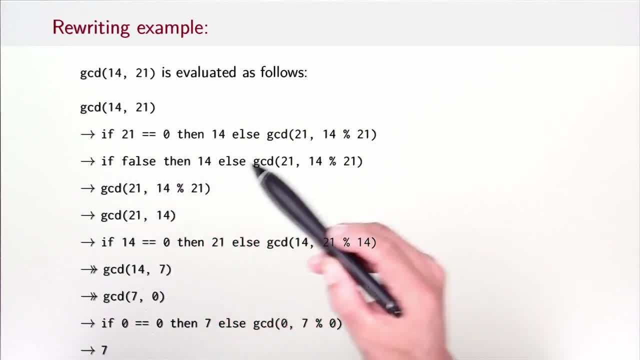 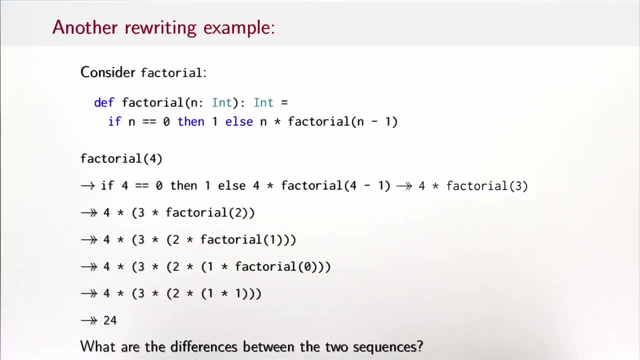 it's essentially flat, So it will oscillate between if-then-elses and recursive calls. But essentially the expression we reduce to always follows the arrow immediately, Whereas if we see the reduction sequence for factorial then we notice that we have deeper and deeper nesting. So we have essentially 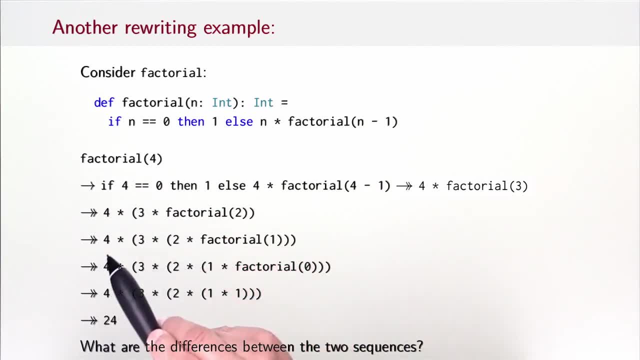 something that we have No, or no already in some operands- 4,, 3,, 2, and then the recursive call of factorial, and here we reach a four times level of nesting, and then it unravels again until we have 24.. So why is that? Why do we? 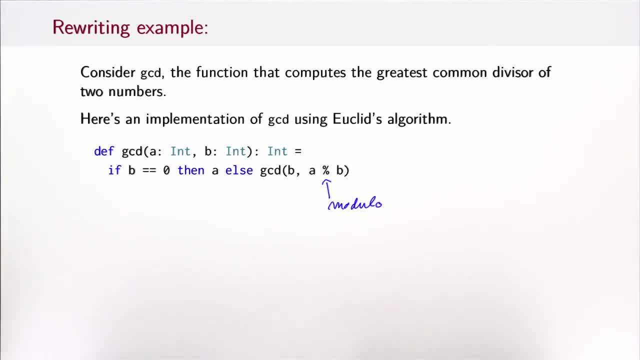 have the difference between those two reduction sequences. Well, if we look at GCD, then we see that GCD calls itself recursively as its last action. There's nothing after the recursive call. The recursive call is at the same time the result of GCD, Whereas if we look at factorial, then we 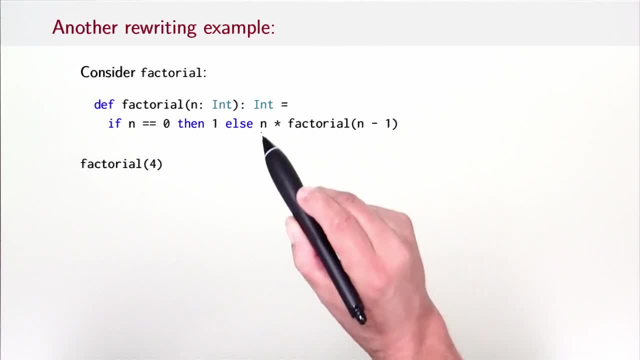 notice that after the call there's still work to do. We still have to multiply with n, So here the call is not the last action of the body, of the function and that leads to the different reduction traces. If the call is the last action, then essentially the intermediate expression in the 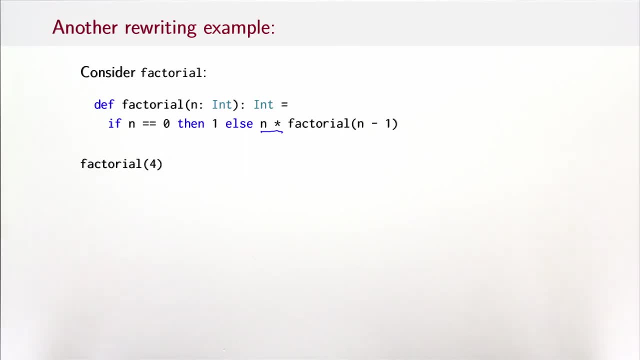 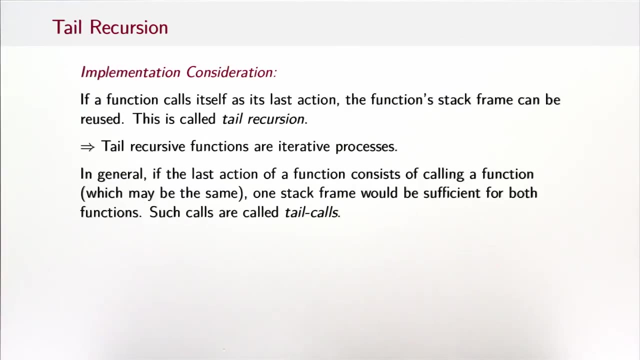 reduction has always about the same size, whereas if the call is not the last thing, then we essentially goes deeper And that observation, which we have done on a very high level and on a very abstract level on the reduction traces, translates directly to an observation on the actual implementation hardware. 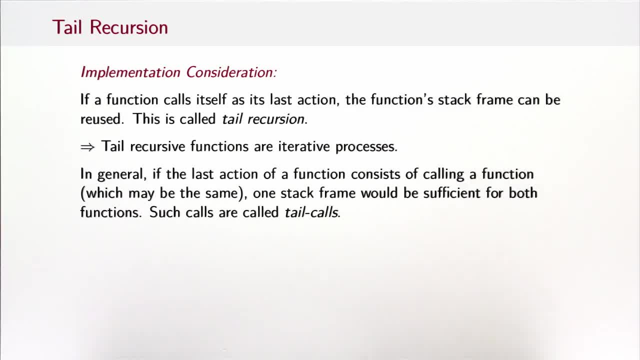 because for function calls we have things called stack frames in a call stack and if a function calls itself as the last action, that stack frame can be reused. We can immediately use the same stack frame for the recursive call, and that is called tail recursion. So tail recursive functions. 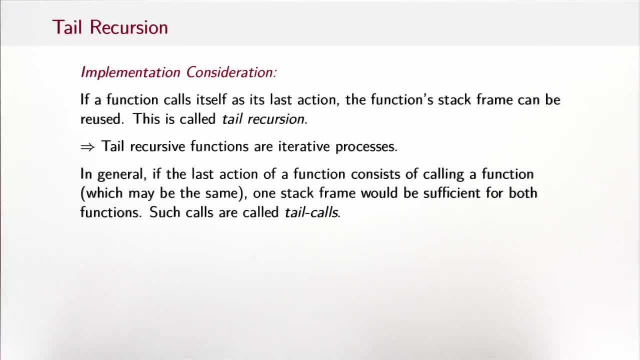 are in a recursive call, So we can immediately use the same stack frame for the recursive call. In essence, iterative processes, There's nothing different between a while loop and a tail recursive function. In general, if the last action of a function consists of calling another function, or maybe. 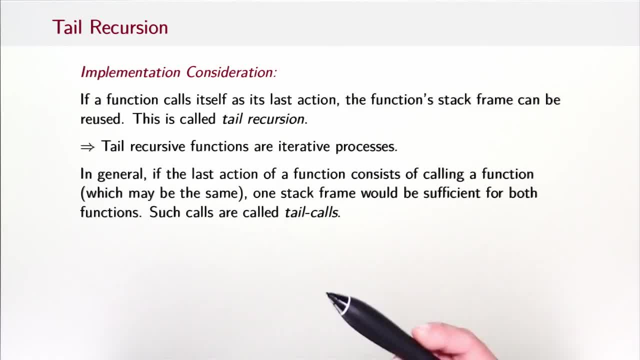 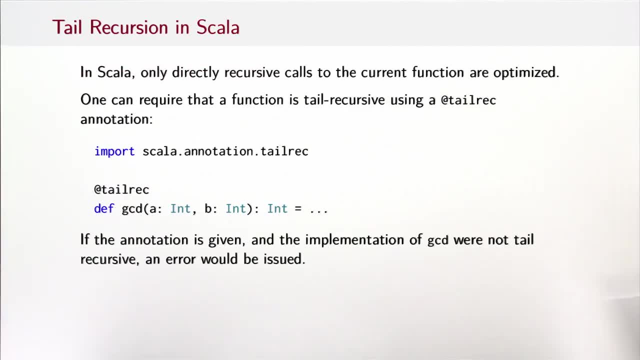 the same one, then we only need one stack frame for both functions. Such calls are called tail calls In Scala because it runs on the JVM. we can only optimize directly recursive calls to the current function. Such an optimization can help runtime speed speed of the function and it also can avoid stack overflows. It turns out that in a normal stack on 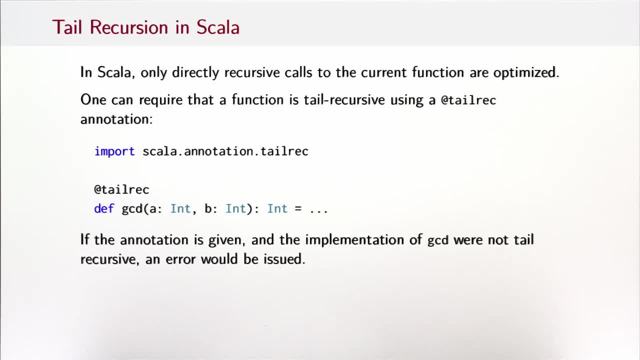 the JVM you have maybe 2,000, 3,000 recursive calls until you get a stack overflow. So if your programs are large enough and your data structures are large enough that that isn't sufficient, it's very important that your calls are in fact tail calls So you can in fact know that at compile time. 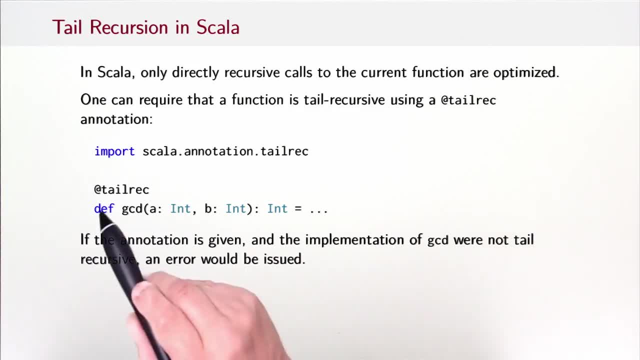 without running the program, because you can tell the compiler that you require that the function must be tail call optimizable, And you do that with an annotation which is called tailrec. You import it from Scala annotation tailrec and then you can use tailrec. and that means that if the implementation of gcd for some reason is not tail recursive, 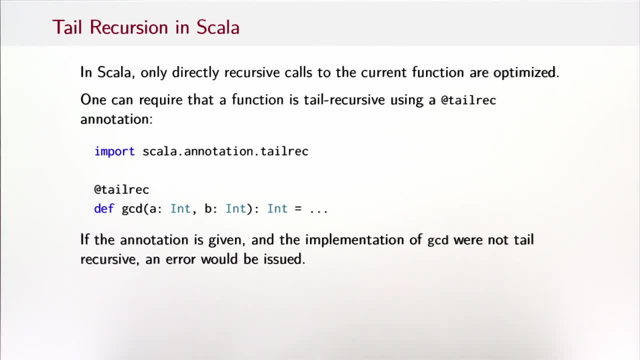 then the compiler will tell you. It will say: give you a warning that says this function is declared tailrec but it's actually not tail recursive. On the other hand, even if you leave tailrec out, the compiler will still optimize your gcd function to be tail recursive when it can. 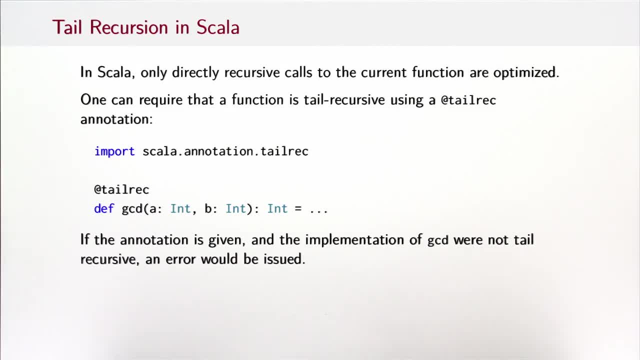 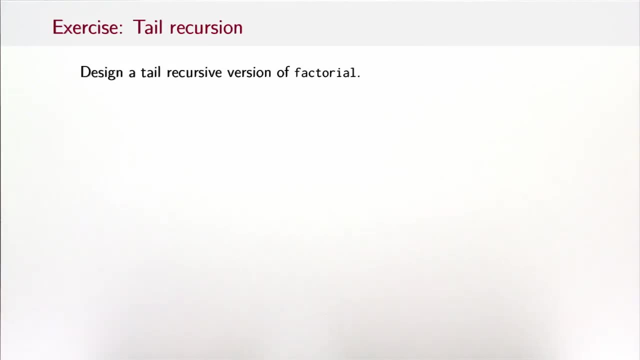 So basically, tailrec is not a command that tells the compiler it must optimize, will optimize in any case. It's just essentially a check for you to know that the compiler could actually do that in the end. So an exercise for you open ended. You've seen factorial. 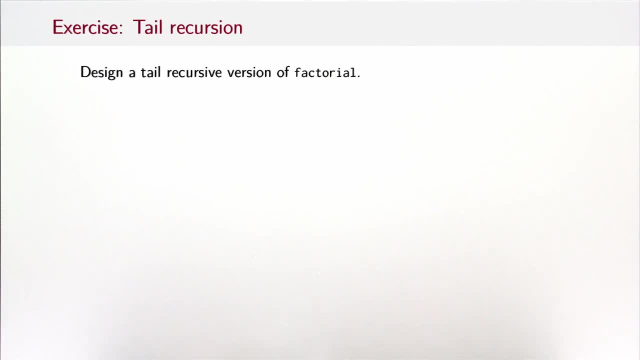 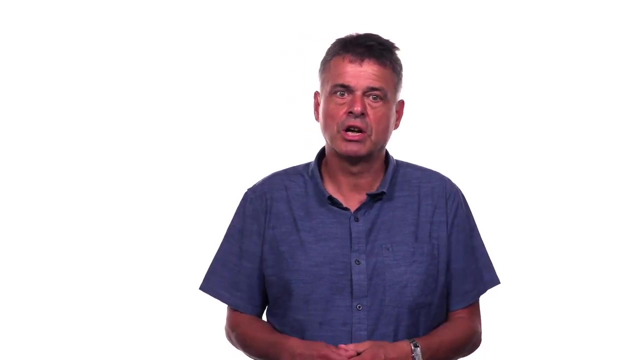 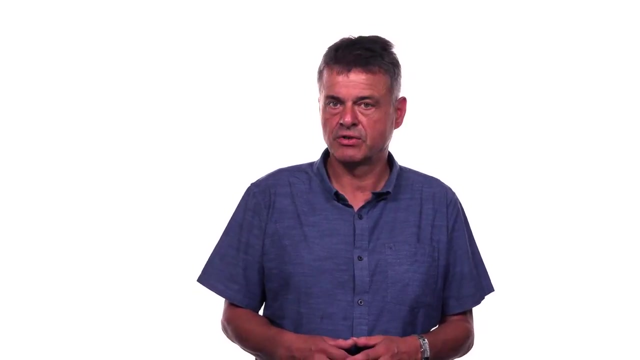 and we've seen that it's not tail recursive. Can you design a tail recursive version of Factorio? In this session we're going to cover an important concept in functional programming: higher order functions. They let you pass functions as arguments and return them as results. You'll 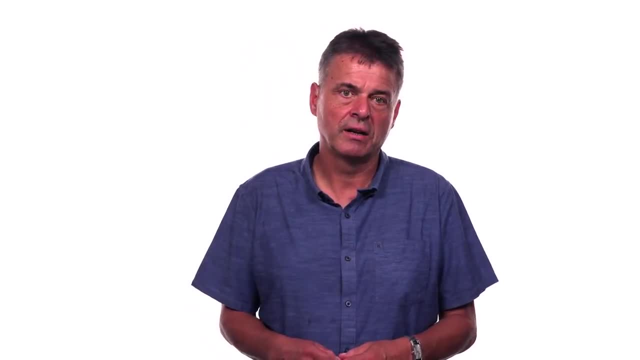 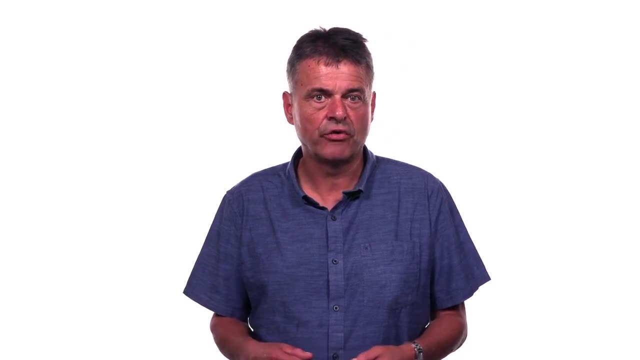 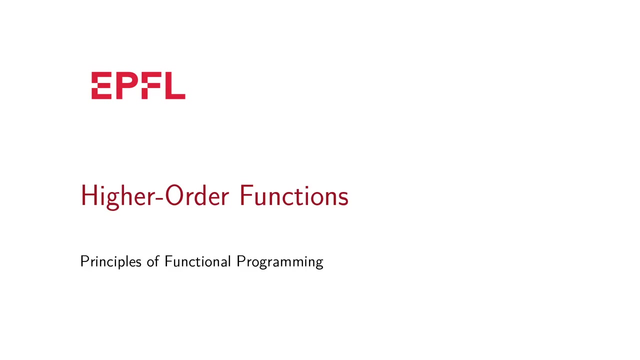 also learn about scalar syntax and how it's formally defined. Finally, you'll learn about classes, methods and data abstraction through the design of a data structure for rational numbers. In this unit, we're learning several new ways: how to compose functions into more interesting 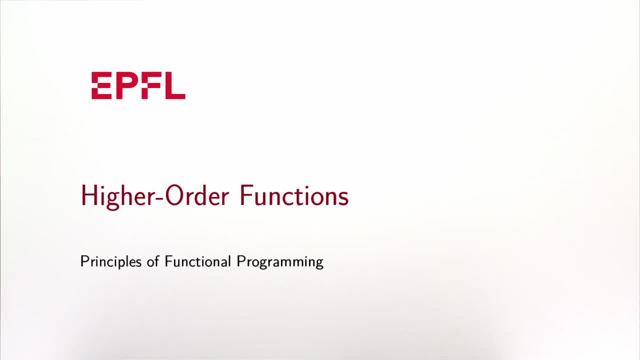 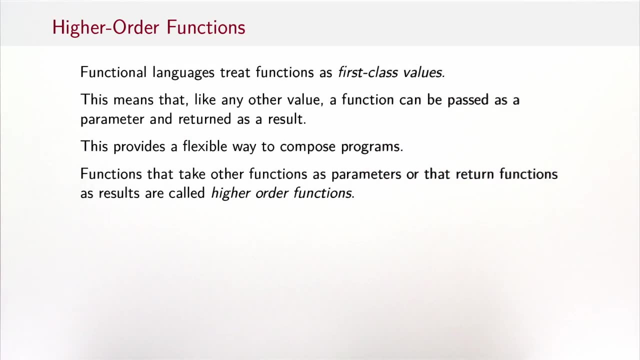 functions. The key concept here is called higher order functions. In fact, functional languages treat functions as first class values. That means, like any other value, a function can be passed as a parameter and returned as a result, And we'll see that this provides a flexible way to compose programs Functions. 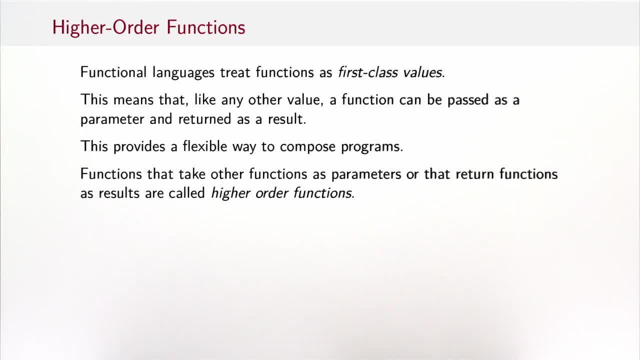 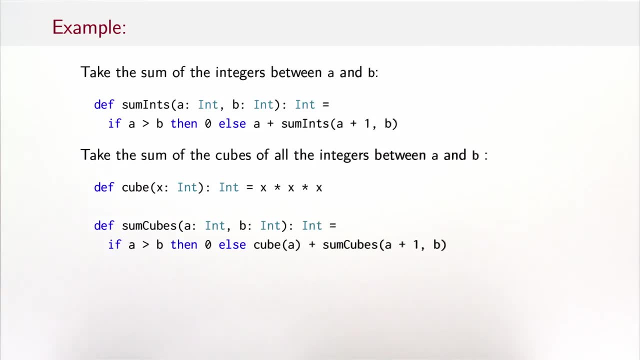 that take other functions as parameters or that return them as results are called higher order functions. So let's start with an example. Take the sum of the integers between a and b. So we have a function sumInts- lower bound a, upper bound b- and we have a recursive definition. 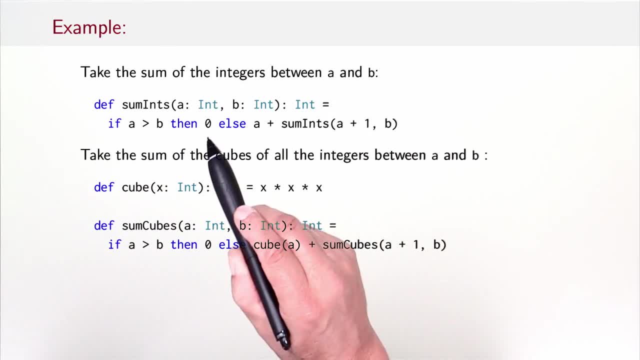 if a greater than b, then the interval is empty and the sum is 0.. Otherwise we take a plus sumInts of a plus 1 and b. Good, so far. Now let's take the sum of the cubes of all the integers between a and b. So the cube function would be just like the square. 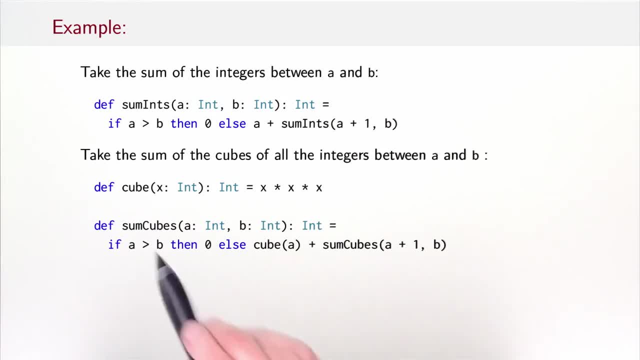 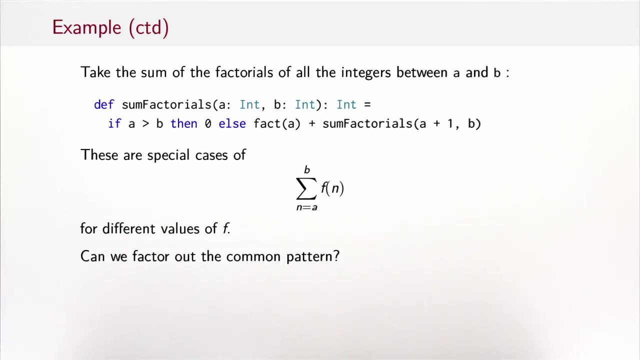 function only 3 times x multiplied. So sum cubes. you could write this: if a greater than b, then 0, else cube of a plus sum cubes a plus 1 b. Ok, Ok, Ok, Ok. Now let's take the sum of the factorials of all the integers between a and b, So we 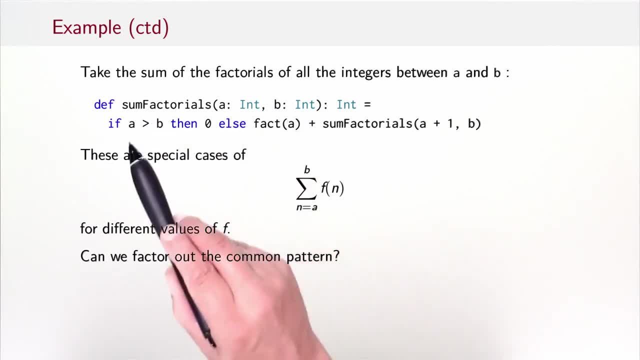 could write a function sum factorials from a and b. and then it's the same thing here, except where we wrote cube we write fact for factorial of a plus sum factorials a plus 1 b. So I assume here that fact is the factorial function. 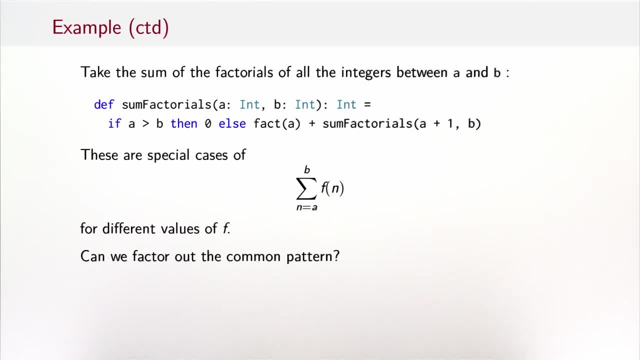 Now, a mathematician would get bored very quickly And they would say: well, these are just some special cases. These are all special cases of what we know as the sum functions, And here's the way mathematicians would write it. So it's a big sigma, and we say: the lowest, the start value is a, the. 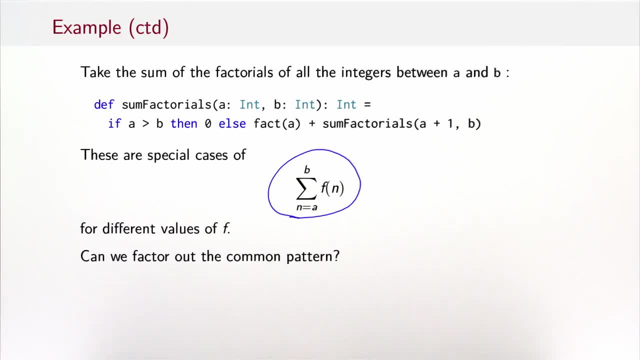 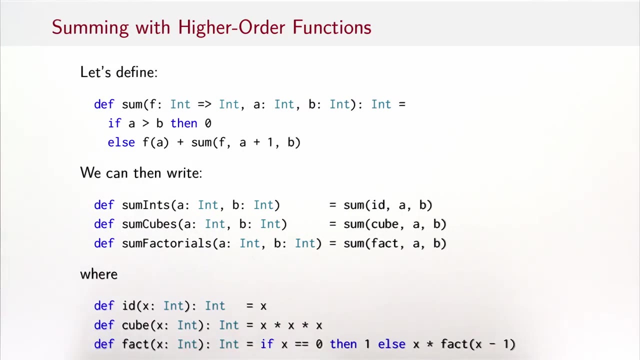 end value is b and we take essentially the sum of all the values of f, of n, where n goes from a to b. Can we do the same in programming? Can we factor out the common pattern? So what varies in these things? Well, the thing that varies is the functions, that 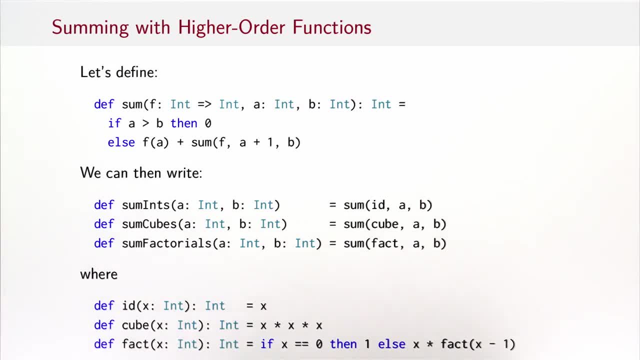 I pass into the summation function. So what we can do in function programming is we can make a parameter that is a function. So here we have a new definition of sum that takes now a function f and a lower bound a and an upper bound b, and it has exactly the same pattern as before, only it uses the function. 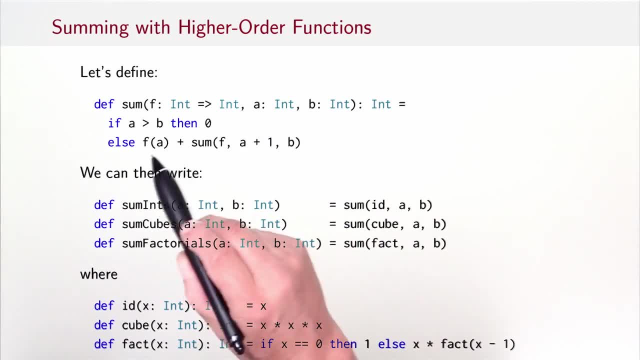 parameter f at this position here. So if the interval is non-empty, then we take f of the lower bound and then we go on with sum of f, f and a plus 1 and b. So once we have that we can write our sum functions in this way We can say: well, sum. 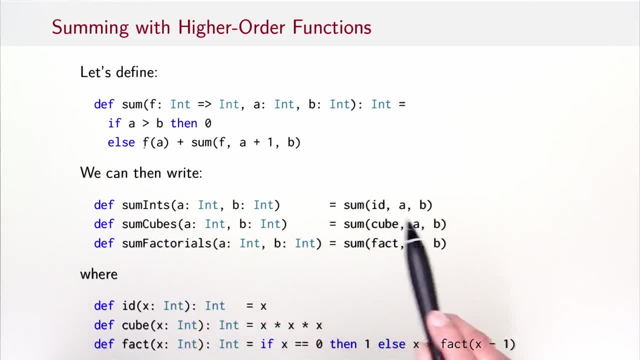 ints is the sum of the identity and a and b sum cubes is the sum of the cube function and a and b and sum factorials is the sum of the factorial function and a and b. where the id function is just x, the cube function is x times x times x and the factorial function 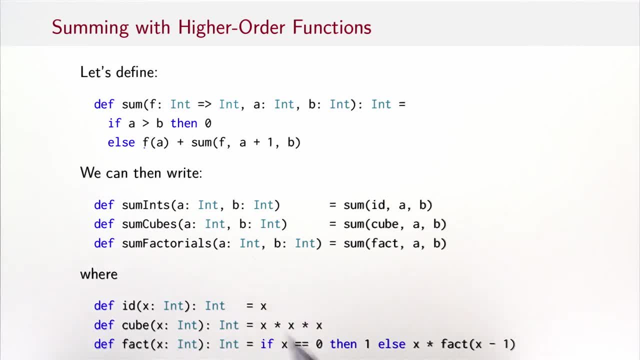 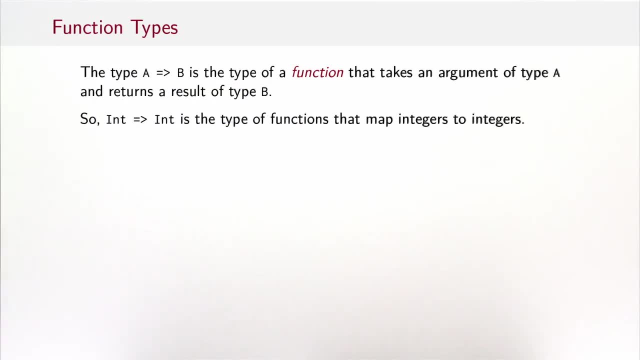 is the usual definition of f. So what we've seen here is a new type int to int, and that type is a type of a function. So generally, the type a- arrow b is a type of a function that takes an argument of type. 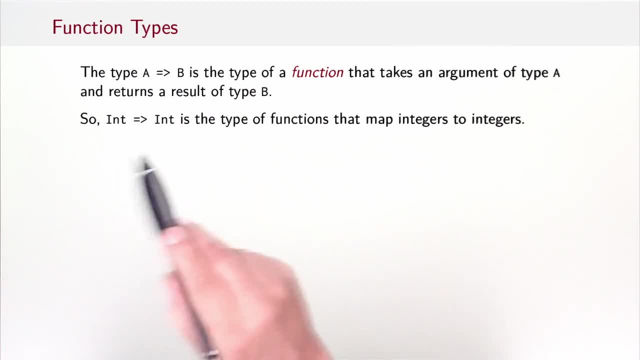 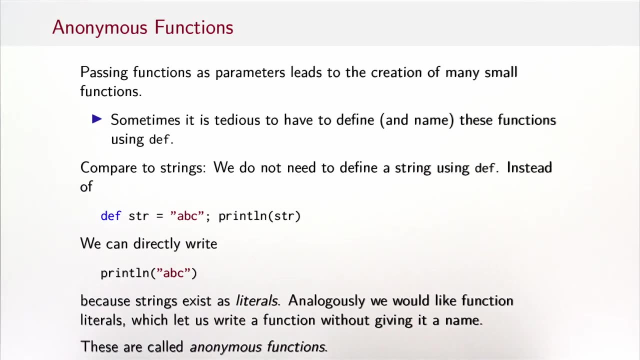 a and returns a result of type b. So int to int is the type of functions that map integers to integers. So generally passing functions as parameters leads to the creation of many small functions and sometimes it's tedious. It's tedious to have to define and invent a name for all these functions using a def. 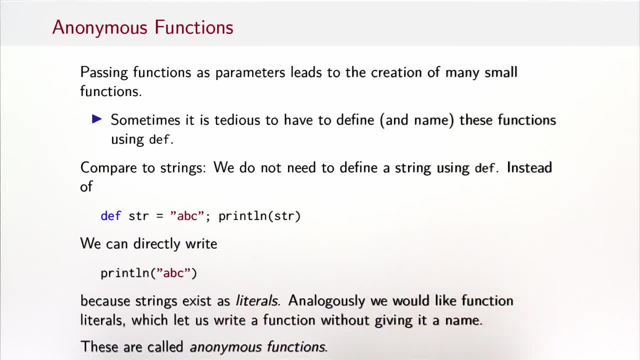 Compare that to strings. We do not need to define a string using def. Instead of def, string equals abc println string. we can directly write println abc because strings exist as literals. Analogously, we would like a literal for a function that lets us write a function without. 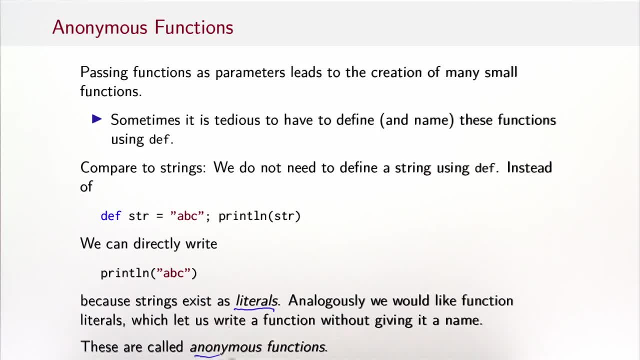 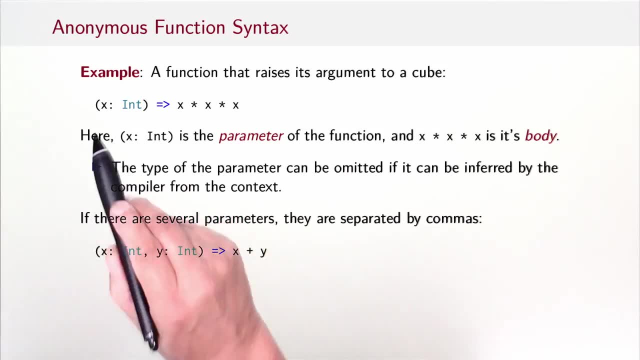 giving it a name. And these literals exist. They are called anonymous functions. So, for instance, here is a function that raises its argument to a cube. It takes a parameter x of type int and returns x times x times x. So that function doesn't have a name. 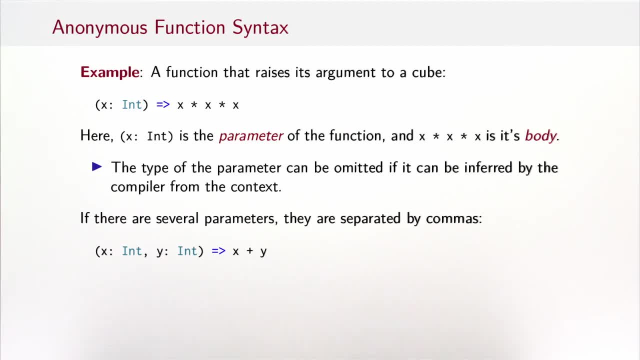 We haven't given it a name. That's why it's an anonymous function. x colon int is the parameter and x times x times x is the body. The type of the parameter can be omitted if it can be inferred by the compiler from the context. 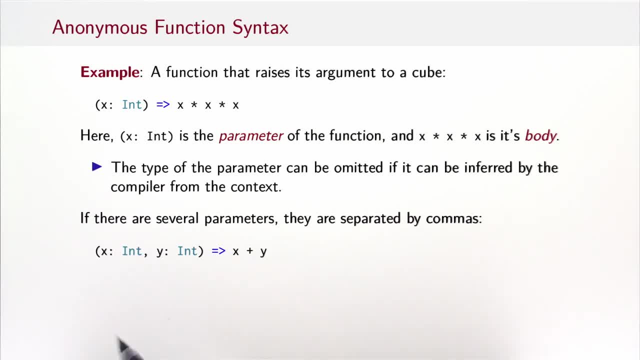 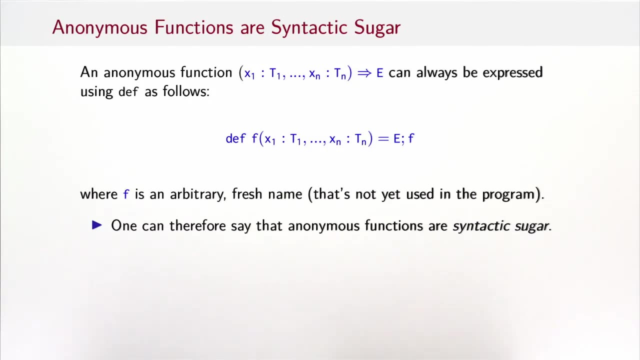 So, for instance, x, int, y int arrow, x plus y would be the function that sums its two arguments, x and y. Anonymous functions are very convenient sometimes, but they're not essential. In fact, we can always express an anonymous function like this one here using a def. 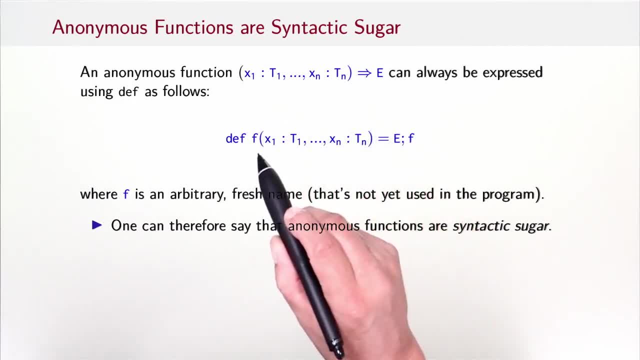 So instead of writing the anonymous function, we give it a name. call it f here, but it could really be any name. Write the same parameters, the same body and then follow that by f And put it in braces to make it a block. 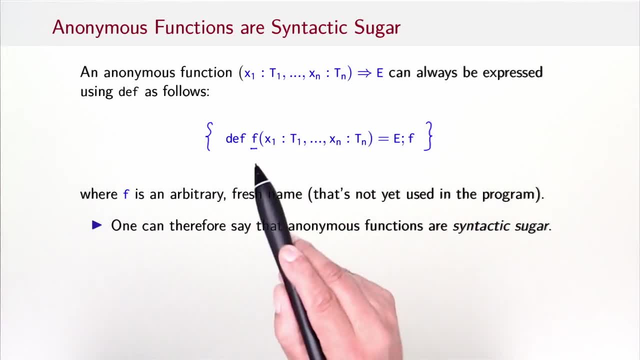 So that's exactly the same as the anonymous function. The name here doesn't matter because it's inside the block, so nobody can refer to it from the outside, Because anonymous functions expand like this to something that we know already. we can therefore say that anonymous functions are syntactic sugar. 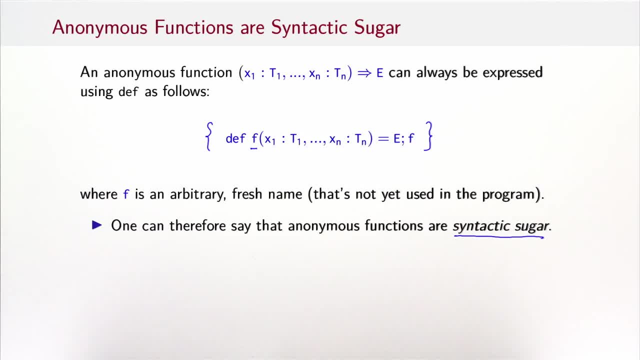 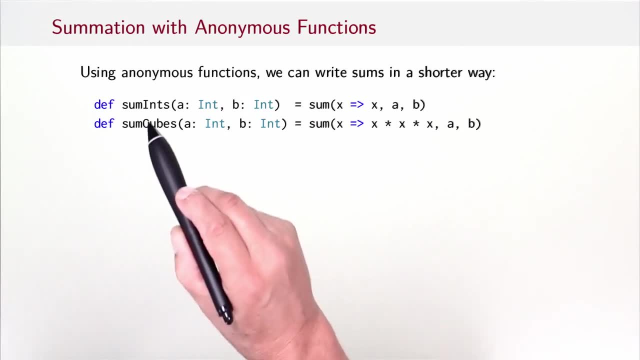 Syntactic sugar means it makes life nicer, But it's not. It's not essential. So with anonymous functions we can now write sums in a shorter way. So, for instance, sum ints would be simply sum functions, where the function that we pass 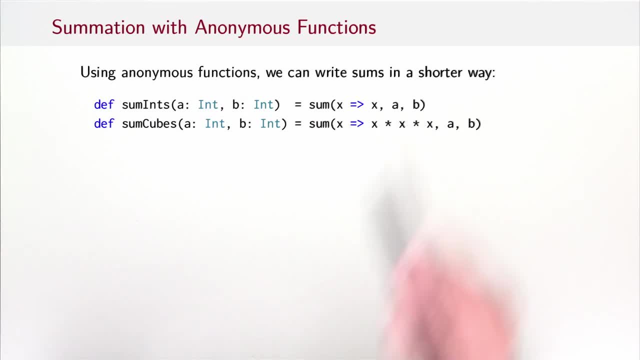 is the identity. It takes an x, gives us back the x and the bounds are a and b, And sum cubes would be the function that calls sum with an anonymous function, and the anonymous function takes an x and returns x times x times x. 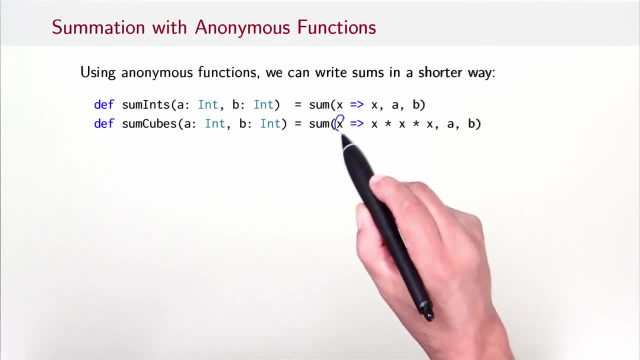 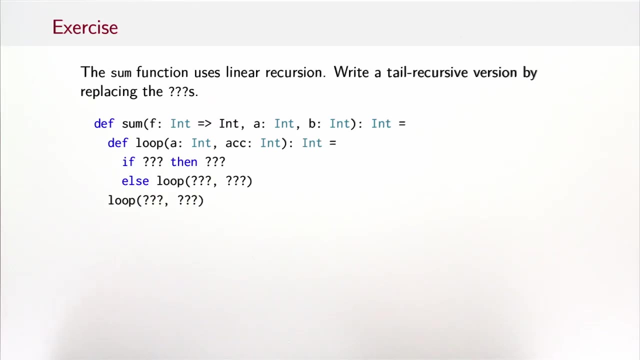 What you've seen in both of these examples is that we don't need a type. We don't need a type, We don't need a type for these parameters. That's because, essentially, the compiler knows that the sum function expects a function from int to int, so it can infer that the parameter must necessarily be of type int. 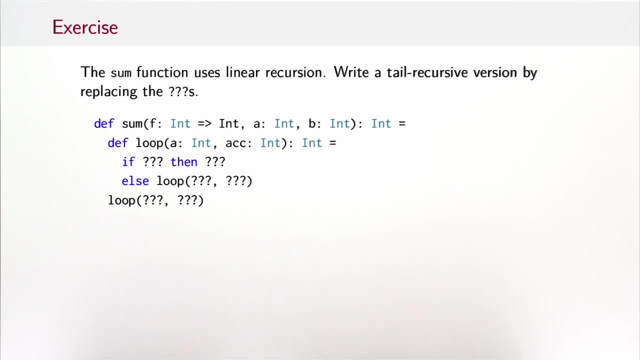 So here's an exercise for you. The sum function uses linear recursion. That means the stack grows as the sum function sums up its operands. Can you write a tail recursive version? So I'll give you a hint. Here's the general scheme. 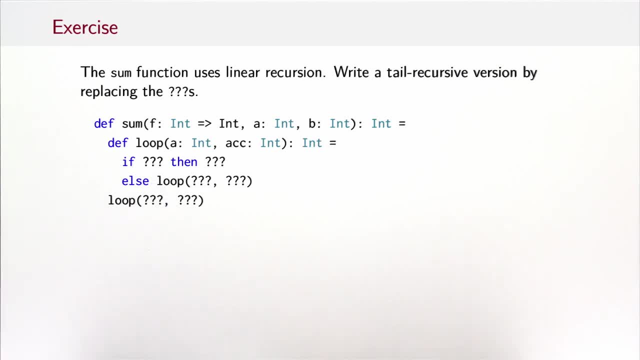 And what you should do is replace the triple question marks With expressions of your own. Okay, so let's see how we would write the body of loop. It essentially follows the scheme that we've seen before. So we say, if a is greater than b, then we have the case where, essentially, we can return. 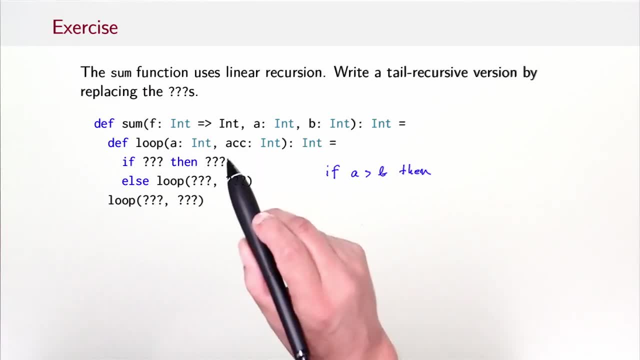 what we already computed. And the idea is, what we computed we put in this accumulator which we call ack. So ack is essentially the intermediate result. So we return ack, And if not, then we go on with the loop. So the loop takes a new, lower bound. 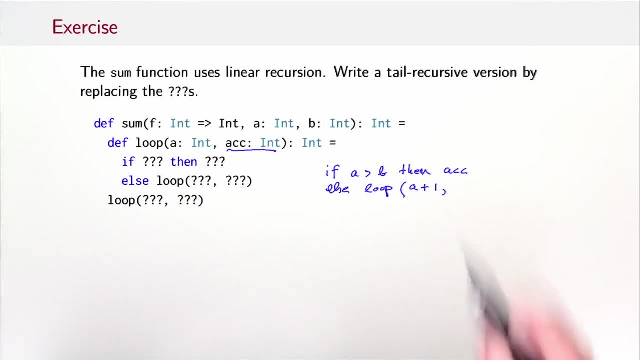 That would be a plus one And it takes an accumulator of the things that we have already summed up. So that would be the old accumulator plus f of a, The initial call. So how do we set off the iteration? Well, we call loop with the original lower bound a. 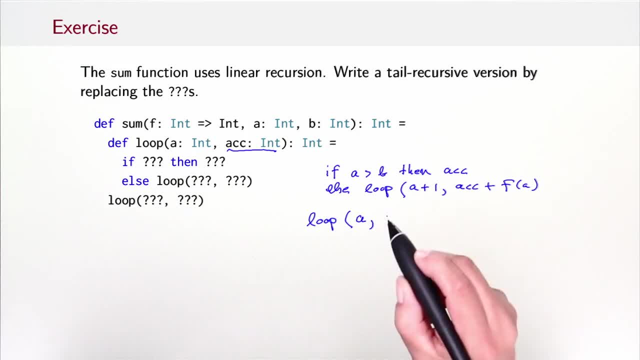 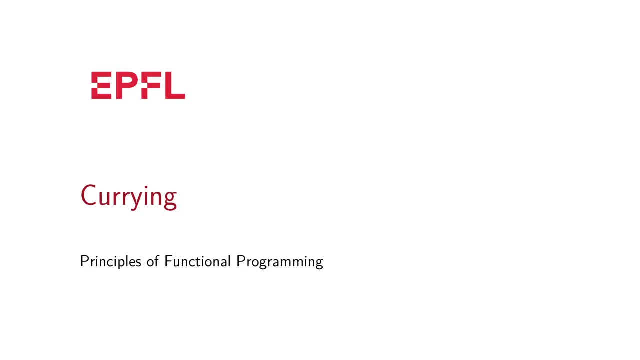 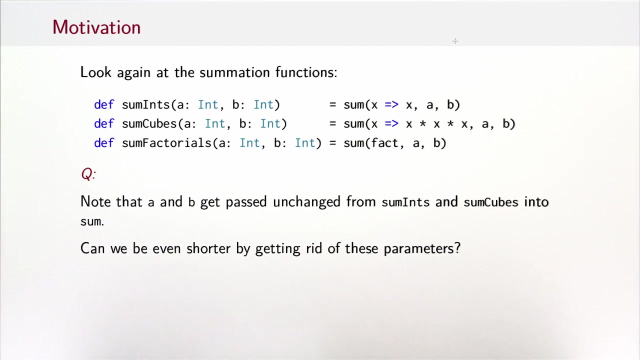 And what is our accumulator? Well, it's a zero value for the sum, So it's zero. So in this section you'll learn about a particular way to compose and abstract functions. that's called carrying. Okay, Let's look again at the summation functions. 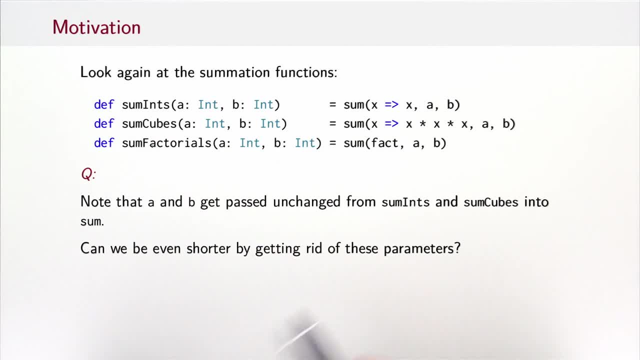 Some ints, some cubes, some factorials. Note that a and b get passed unchanged in each case to the sum functions. Now, whenever there's a common pattern like this one, you should ask yourself whether it's possible to eliminate the repetition. So can we be even shorter by getting rid of the a and b parameters? 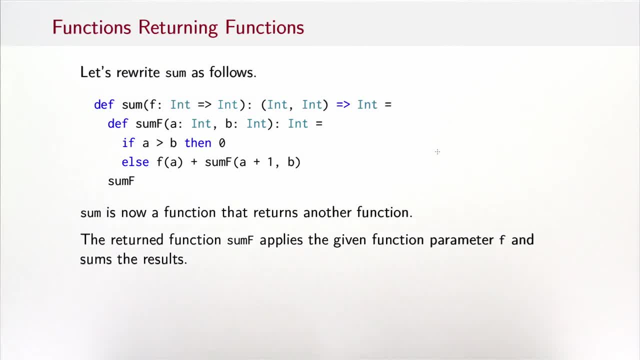 At first this looks difficult, But here's an idea. Let's use the fact that a and b are equal. Let's use the fact that a and b are equal. Let's use the fact that in our language, functions can return other functions. 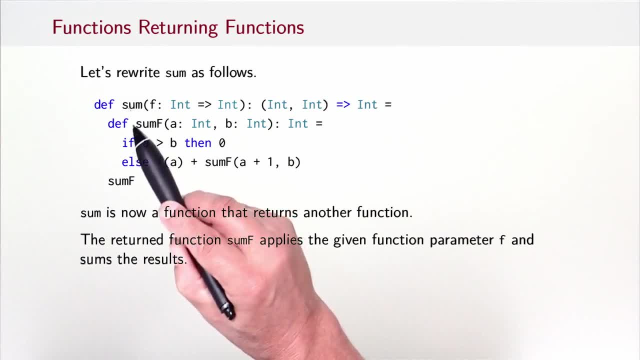 Let's redefine sum as follows. So here we have the sum function, And it takes now a single parameter, the function f, and it returns a function that takes two ints, which are the bounds a and b, and gives you back the final value. 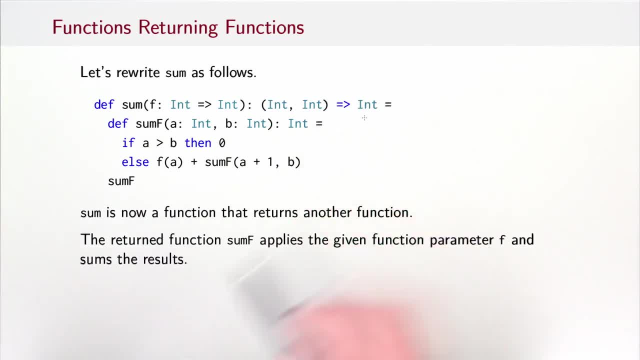 How can we formulate f? Well, f has to return a function. Let's call that sumf. Let's call that sumf And the sumf function. it takes the bounds And then it has the usual pattern. So if the lower bound is bigger than the upper bound, it returns zero. 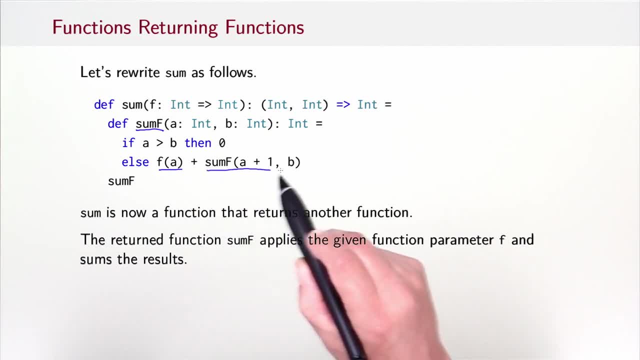 And otherwise it returns f of a plus. and now we have the sumf function applied to a plus one b, So that function captures the common pattern where the two bounds, a and b, are still left open. They're parameters to the function sumf. 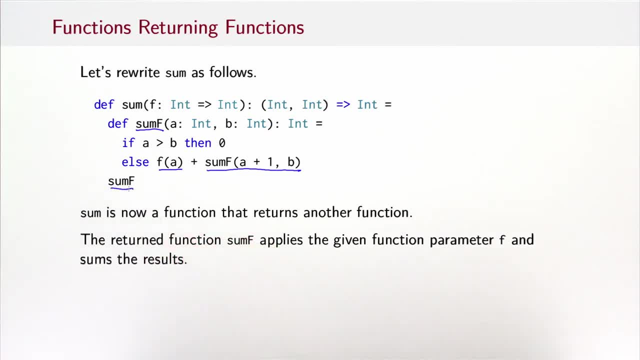 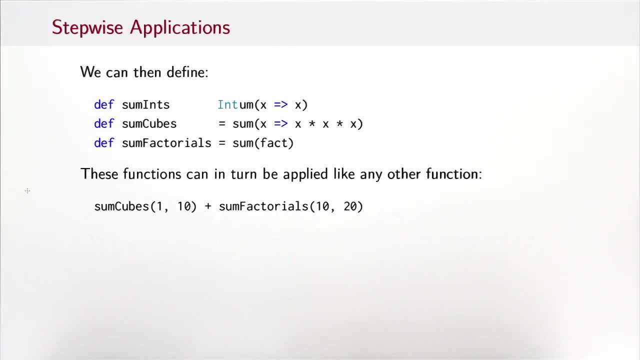 So all sum then returns is the sumf function. So that's it. Sum is now a function that returns another function. So how do we apply sum? Sum now returns a single argument, so we can define a function sumints, that applies sum. 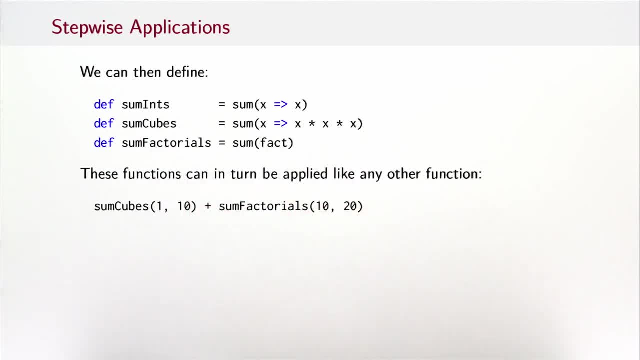 to the identity function, sumcubes to the cubing function and so on. So what's the type of sum x to x? Its type is int and int to int. So that's the return type of the sum function. Okay. 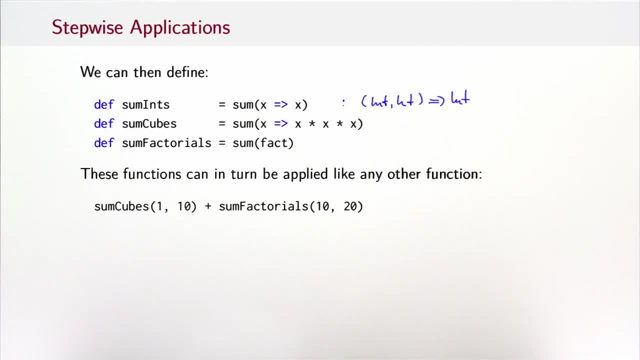 So if these things are functions, they can be applied in terms. So one could write: then sumcubes plus sumfactorials. All this is possible because we have returned a function that takes the bounds separately. Okay, So you've seen, we have now proceeded in two steps. 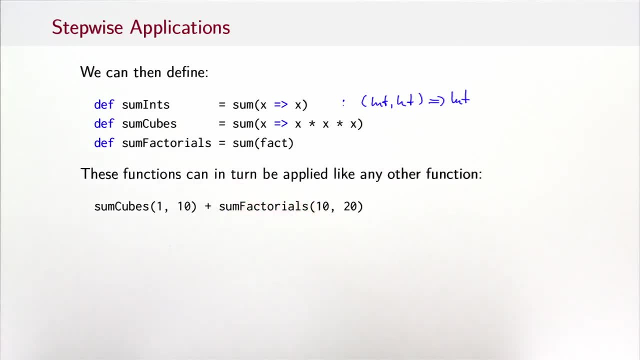 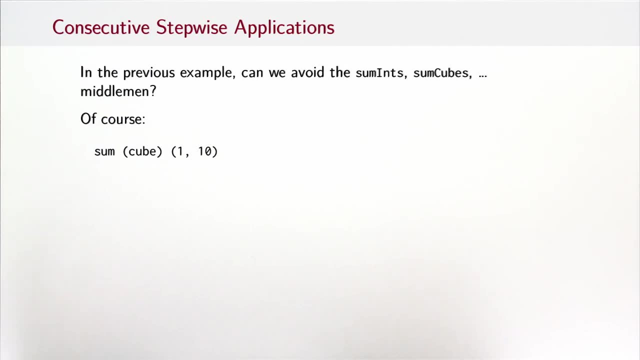 We first define the intermediate function- sumints, sumcubes, sumfactorials- and then we apply them to the actual bound arguments. You might have noticed. You might ask: can we cut out the middleman and avoid the sumints and sumcubes? and so 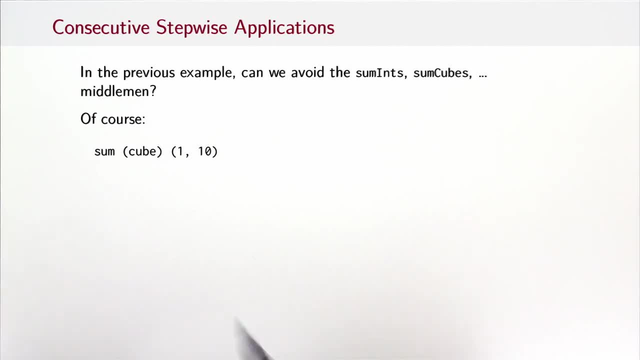 on intermediate functions. And the answer is, of course You can write sum applied to cube, applied to. Well, let's analyze that a bit further. So we have first the function sum of cube That applies sum to the cube function, and it returns another function, one that takes 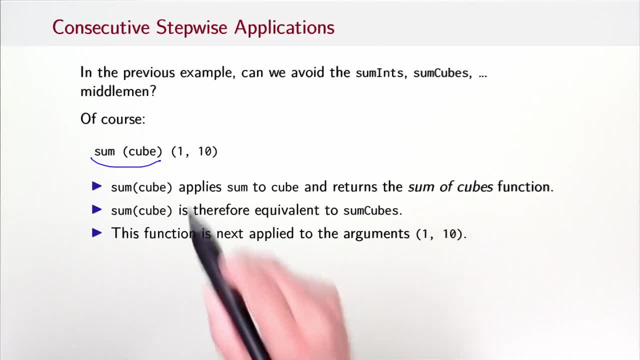 two integers which are the bounds. So this sum of cubes function, This function gets in turn applied to the two bounds 1 and 10.. So sum of cube is equivalent to sumcubes that you have seen previously And that function gets applied to the arguments. 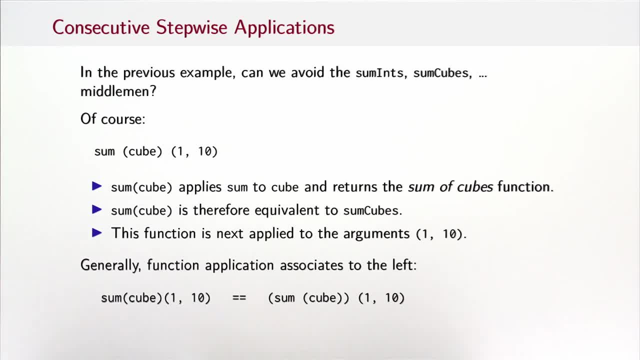 Generally function application associates to the left. So if you write sumcube, that means you first apply sum to cube- The parents go like this- And then you apply the result to 1 and 10.. Now this might look quite weird to many of you. 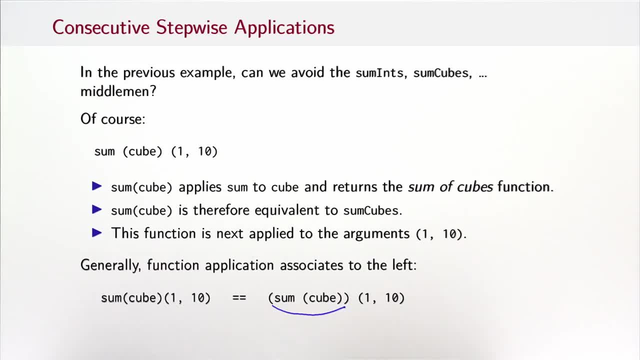 But in fact, there is something that you probably know that is quite close to that and behaves in exactly the same way. What is that? Well, what I have in mind is arrays. In a language like Java or C-sharp, you write array selection with a single argument. 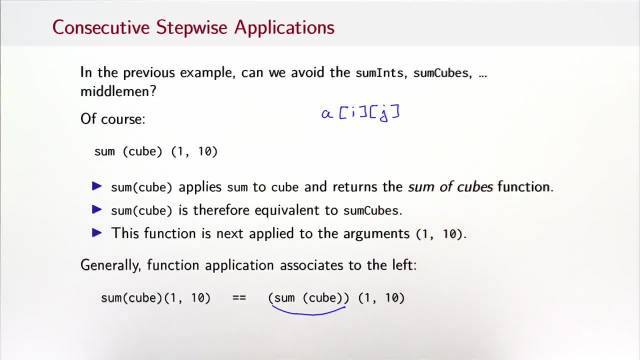 And if you have several dimensions, then you write them one after the other with brackets. So A, I, J would be a selection into a two-dimensional matrix with indices I and J. In fact, you can think of an array as a function from the index to the element type of the array. 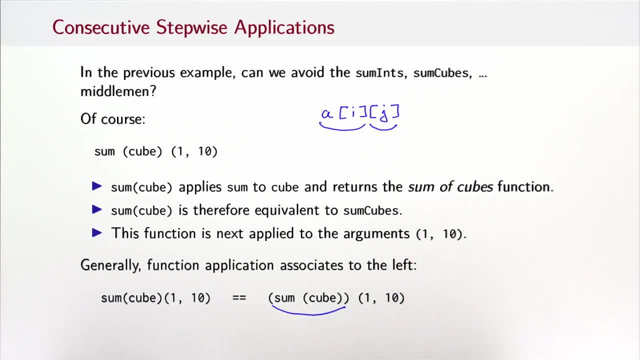 So here you have the first function application and here you have the second. Now you might ask yourself: well, if arrays are like functions, then why do we write array application or array indexing with brackets instead of parents? And the answer is no good reason. 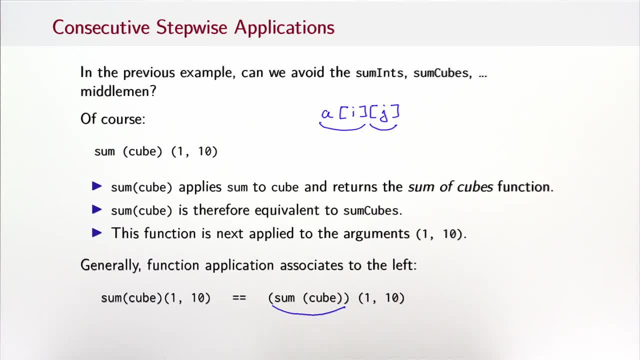 It's really historical reasons only. So in fact, in Scala, when we will introduce arrays at some later point, you will find that in Scala We will write arrays, We will write array selection with parentheses like this, because, after all, arrays are morally. 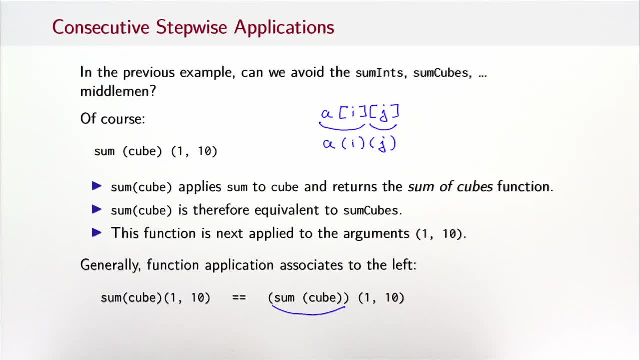 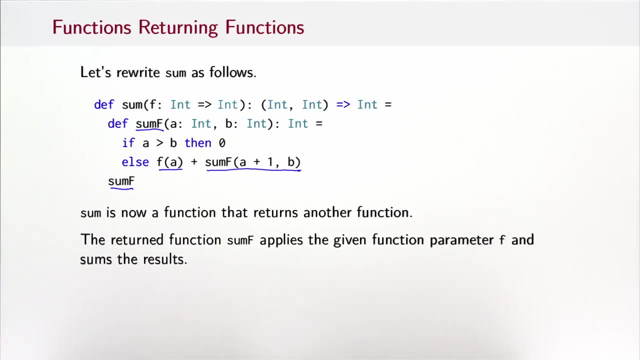 just functions, and so you should write array indexing as function applications. But we will not see arrays for quite a while because they are a mutable concept and we want to concentrate on the purely functional aspects of the language first. Now, one downside of this new way of writing functions with arguments given one after each. 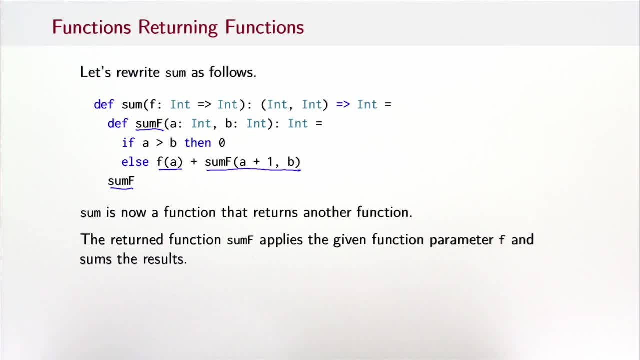 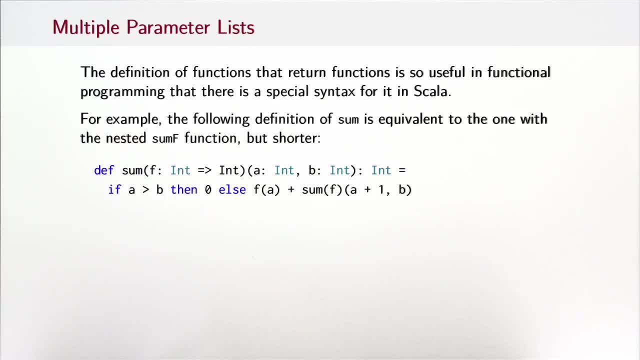 other in separate parameters Is that defining a function like that is a bit clumsy. So this thing is a bit scary the way we set up these functions. But in fact the definition of functions that return functions is so useful in functional programming that there is a special syntax for it in Scala and many other functional 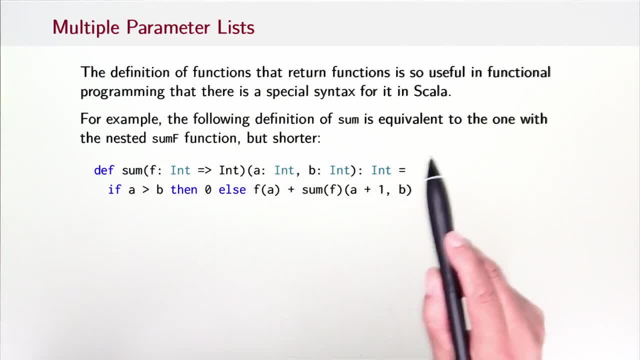 languages. So for instance, the following definition of sum is equivalent to the one with the nested sum f function, but clearer and shorter. Here you just write two parameter sections. You write sum takes first The function is a parameter And then you follow immediately with the second parameter, section a and b. 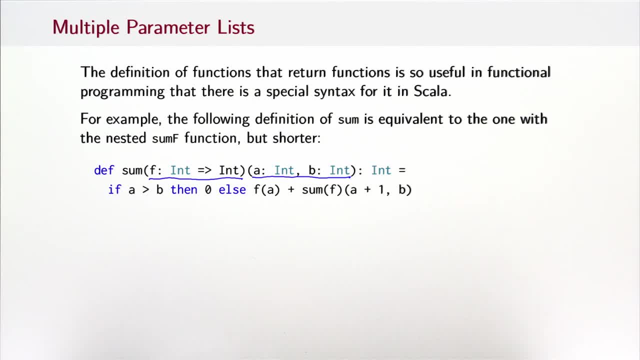 And the result is int and the body is just what you've written before. So what that implicitly defines is a function that takes a single parameter f and that returns a function that takes the two following parameters a and b. But you don't have to invent a name and an inner function to do it. 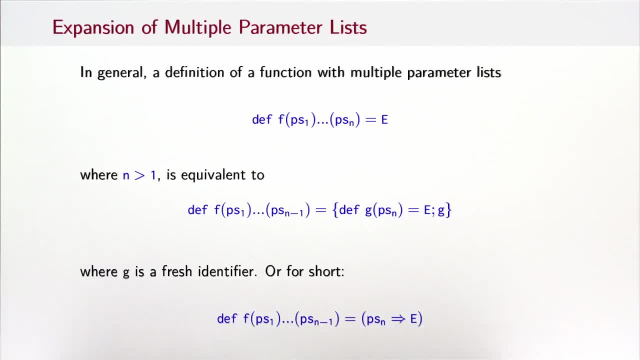 You can write it all in one line, So let's play with this. Let's say you have a function that takes a number of parameter lists. That function would be equivalent from what we've seen, to a function where the last parameter list becomes essentially this nested function. 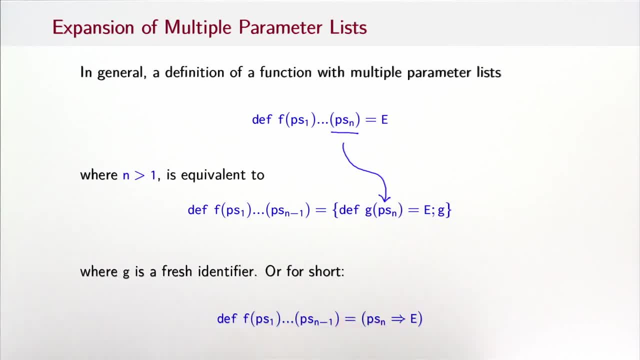 That's how we have defined this idea of writing many parameter lists on one line. They expand to essentially defining nested functions with arbitrary names. Here the name is g Or, for short, this thing. here It's just an anonymous function, as we've also seen. 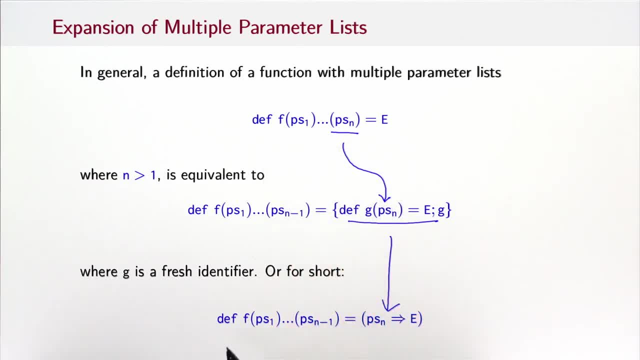 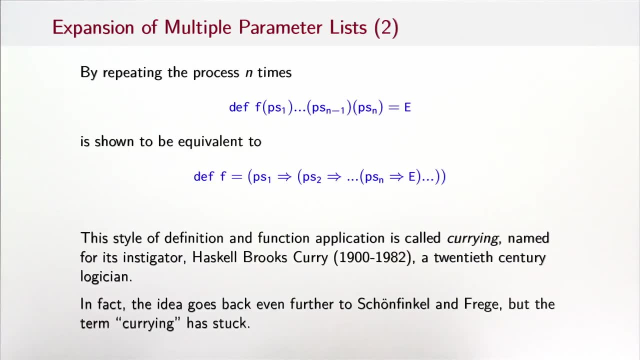 So the function definition that you saw up here would be equivalent to a function definition with one fewer parameter lists that has an anonymous function on the right-hand side. Now we can repeat the process and do that for every parameter list of the function And that will end up in a function with no parameters at all. that is an anonymous function. 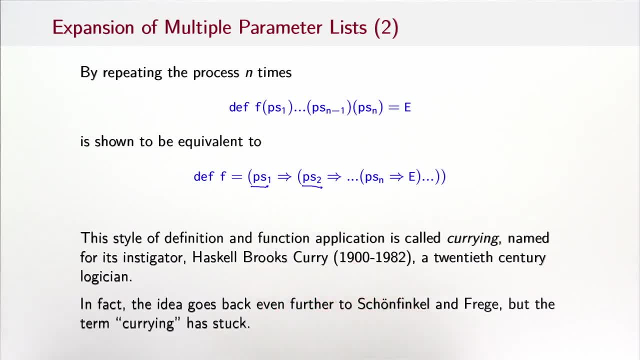 of the first parameter list, that returns an anonymous function of the second parameter list, And so on. finally, that returns a function of the last parameter list and that returns a body e. So that means that theoretically you wouldn't need function parameters in defs at all. 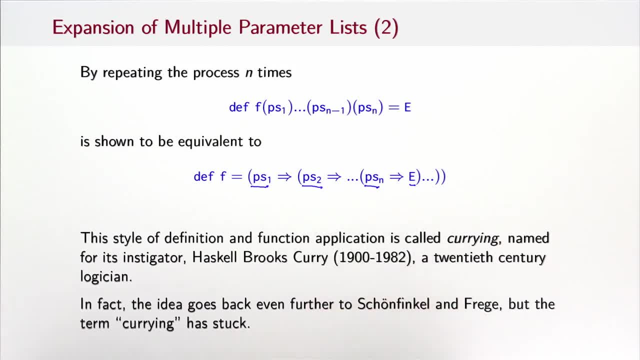 All you would need is anonymous functions like that, And that style of definition function application has a name: It's called currying, named for its instigator, Haskell Brooks Curry, who was a logician in the 20th century, So it's no coincidence. 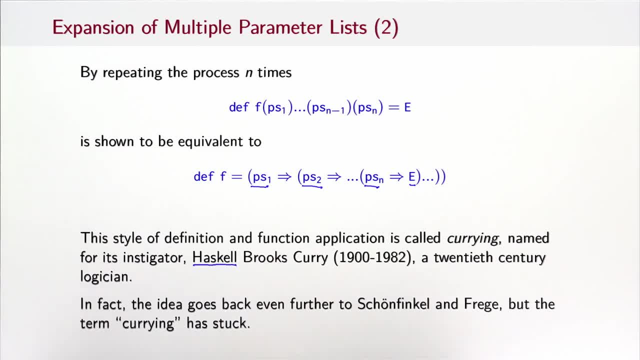 It's not that Haskell is a very well-known functional programming language. It was named after the same logician. In fact, this idea that you can write every function as essentially a sequence of anonymous functions that each take a single parameter goes back even further to Schoenfenkel and 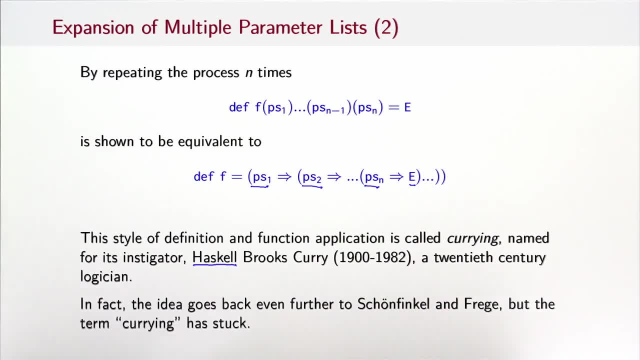 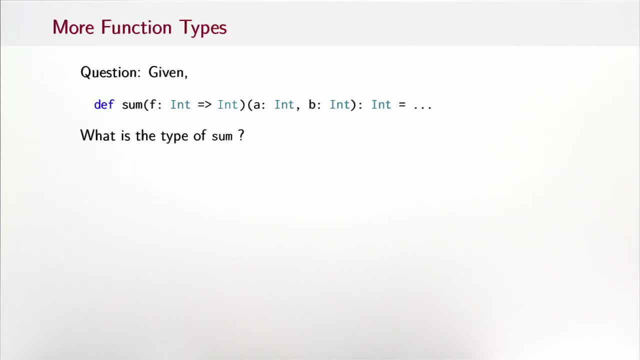 Frege, but the term currying has stuck. So let's look at the sum function again. Given this function here, what is the type of sum? Well, Here we can read it off the parameter list. It takes a parameter of type int to int. 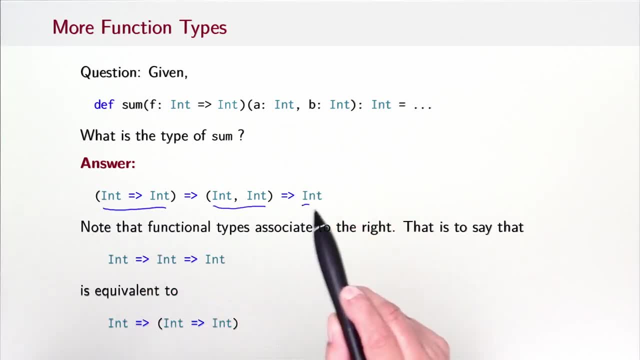 Then it takes two parameters which are both ints, and then it returns a result of type int. So if you're picky you might want to write parentheses around here, because the thing in the red parentheses is the result type of the sum function, but in fact functional. 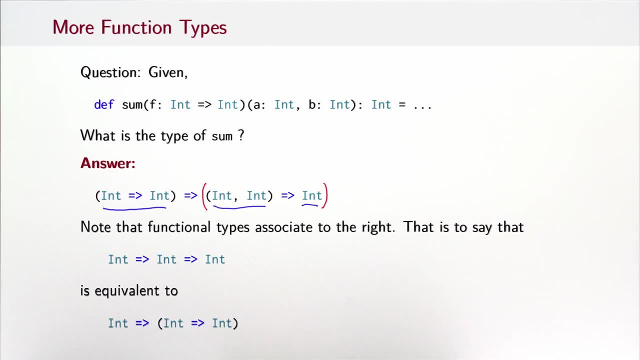 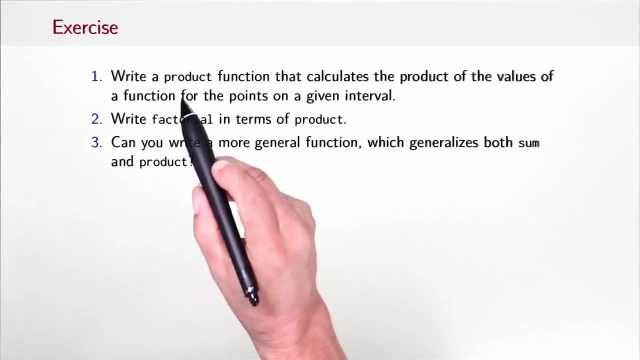 types associate to the right. That means that int arrow, int arrow, int is in fact equivalent to putting the parentheses here the way you see it here, So these red parentheses can also be left out. So here's an exercise: Write a product function that calculates the product of the values of a function for the. 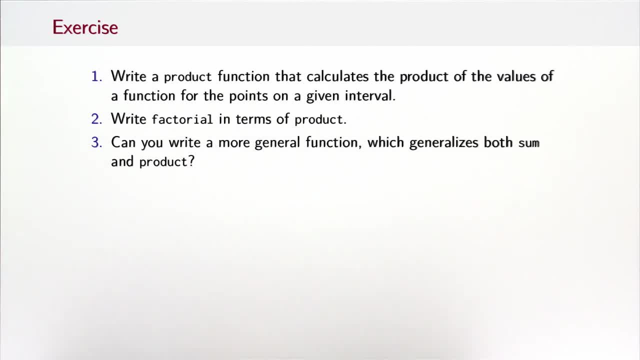 points of a given interval, similar to what we did with the sum function. As a second step, write the factorial function in terms of product And as a third step, can you maybe write a more general function that generalizes both sum and product. 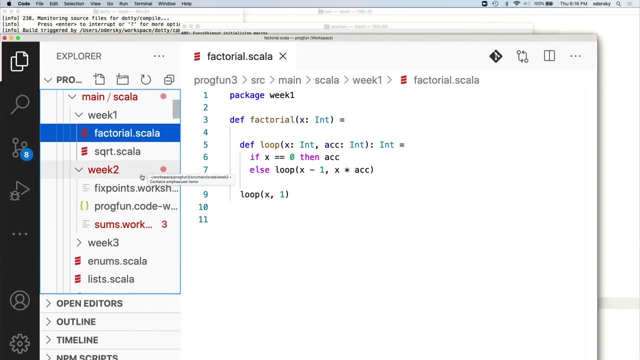 OK, So to solve this exercise, I'm going to make use of a new tool which is called Worksheets. So a worksheet is like a REPL, a thing where you can type in definitions and expressions, but it's more like a complete editing surface, and you will see that the answers together. 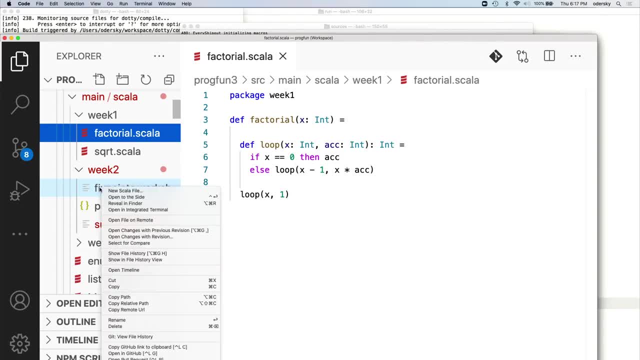 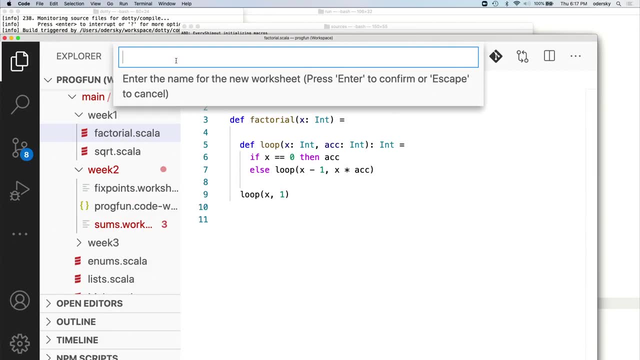 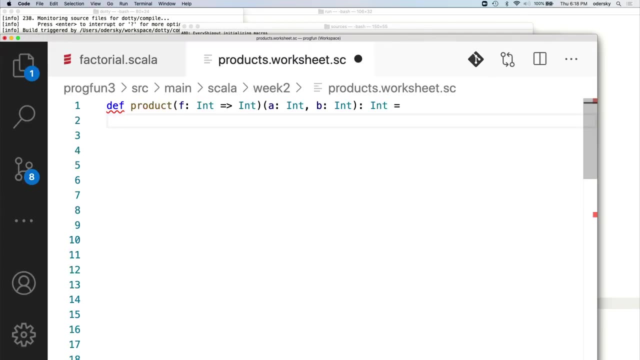 with the expressions that you type. So to start a worksheet. we select a new Scala file of type- worksheet, OK, And we write: give it a name. let's call it products, OK. So how would I define product? Well, a similar way to how I define sum. 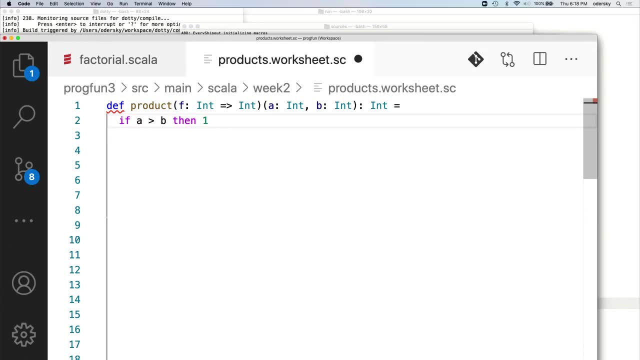 If a is greater than b, then the product is empty. so I give you back the unit for products And otherwise I apply f to a and I multiply that with product of f, a plus product. OK, OK, So let's test this. 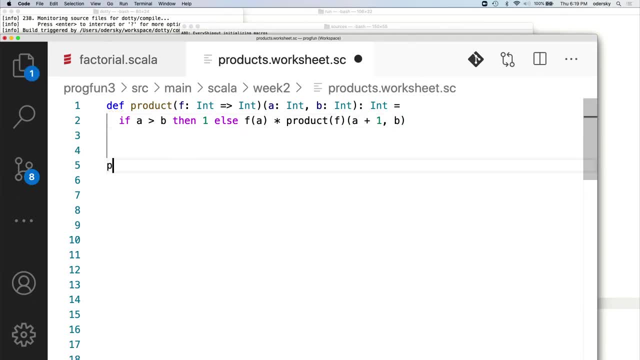 Let's say write product of the square function, and it bounds 1 and 5.. So the worksheet responds and says: well, you've defined an integer and it is 14,400.. Once more, OK. So let's use that to define factorial. 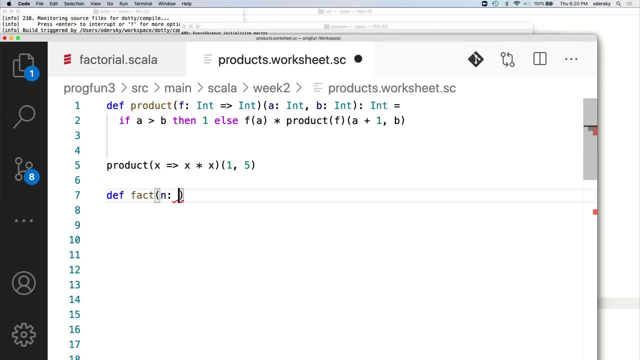 So what would factorial be? Well, it's a function of a function. OK, So what would factorial be? It's the product of the identity function. So that's x to x and 1 up to n. So it's 1 multiplied by, 2 multiplied by, and so on until n. 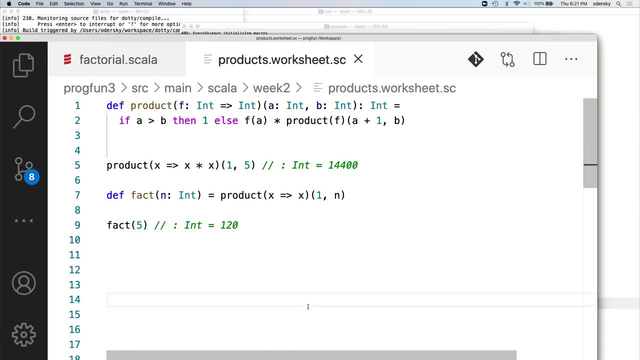 OK, So factorial of 5, just to test, it would be 120. OK, So what about the third question? Can we write a more general function that generalizes both product and sum? So what would this function do? Well, essentially, it would say: well, we want to abstract over the way we combine things. 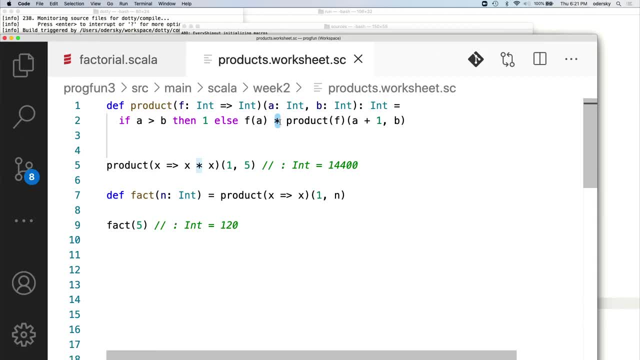 So we had a plus for sum and a times for product, And also we have to abstract over the case which should be returned when this interval is empty. It was 1 for products and 0 for sums, So let's define a function that keeps both of these values as parameters. 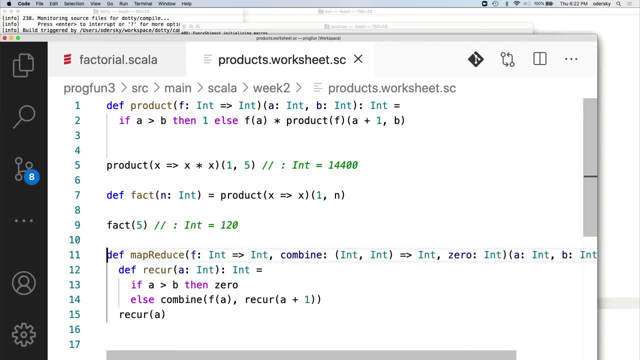 So I call this function mapReduce, because it takes a map function, a thing that gets applied to every element, That's those things we usually call a map. I call this f here- And it takes a reduce function, which is called combine here, that then takes two of the results of maps and combines them into a single int. 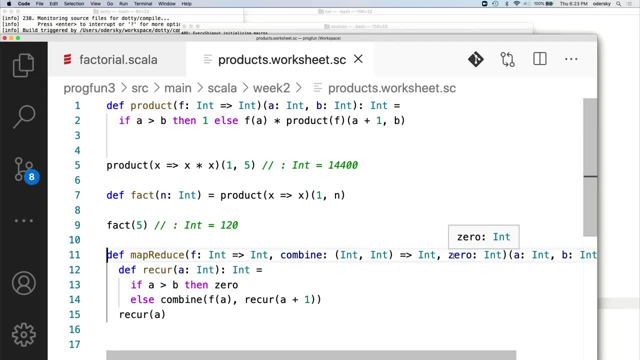 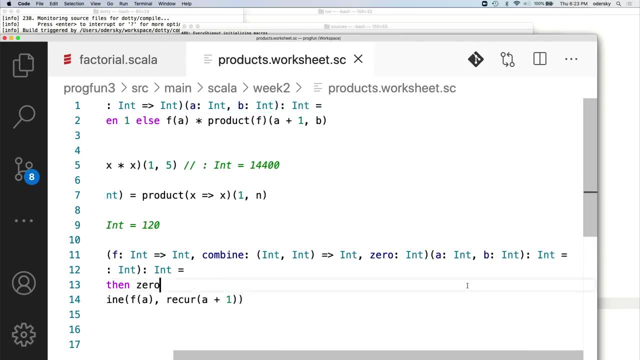 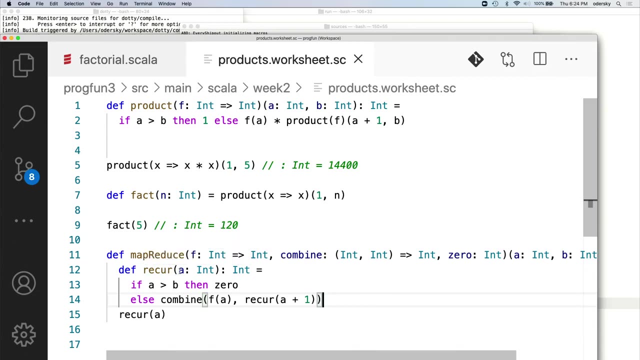 And it also takes a 0. That's the thing to return in case the interval is empty. And that function returns a second function that essentially takes our interval of bounds from a to b. So I define mapReduce with a helper function that's called recur here. that takes essentially the next value in the reduction to apply. 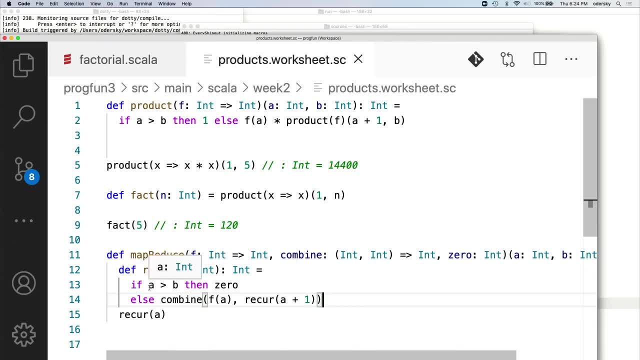 So the pattern of recur is very much like what we've seen before. It says if a is greater than b, then we return the 0. Whatever the 0 is, And otherwise we combine the application of f to a. So that's my next value and the result of recurring with the next step value. 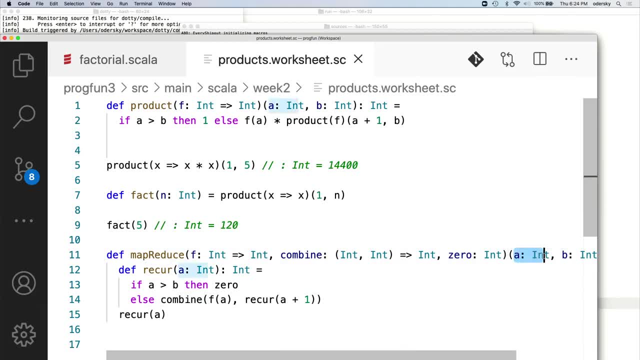 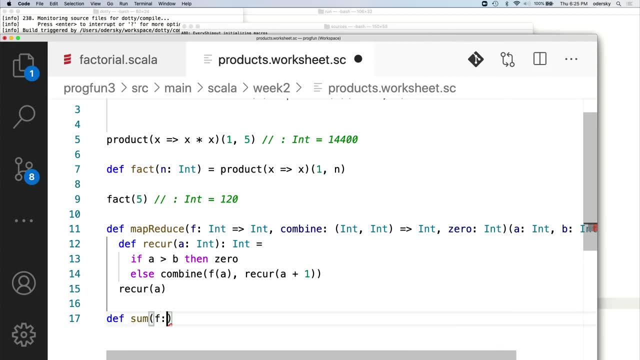 Then the result of mapReduce will simply be recur with the current lower bound a, This one here. So now that I have mapReduce, how can I redefine sum? So the sum function would take a function f, its map reduce of f. The combine function is the function that takes two integers. 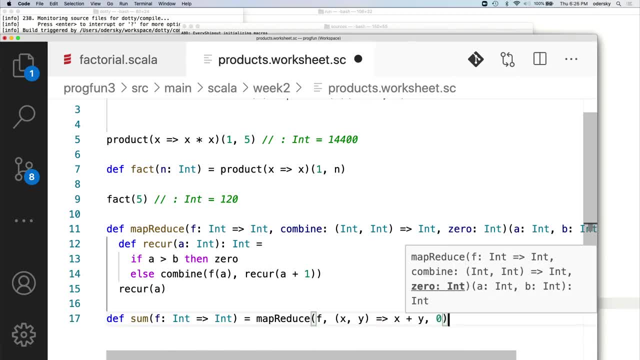 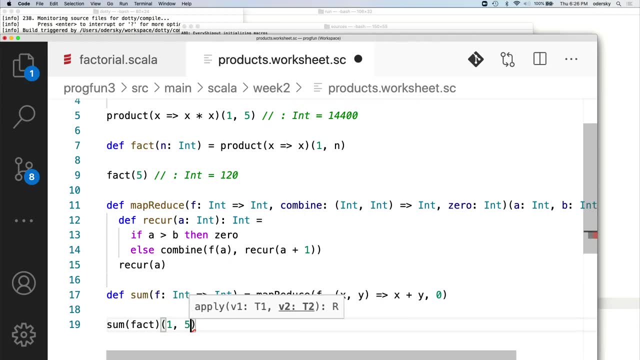 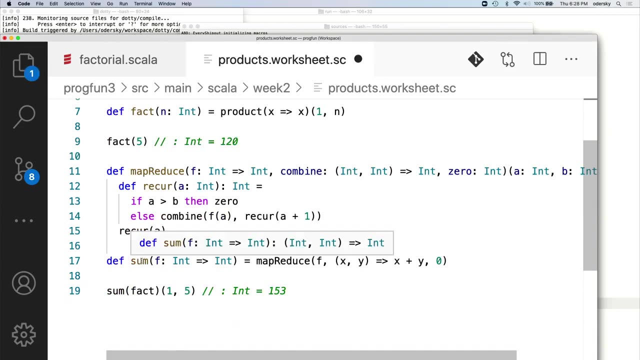 and sums them and the zero is zero. So let's try it. Let's say we want sum of factorial between one and five. Here you go. So one thing which is interesting for sum is that I haven't bothered writing the two arguments for the bounds and I 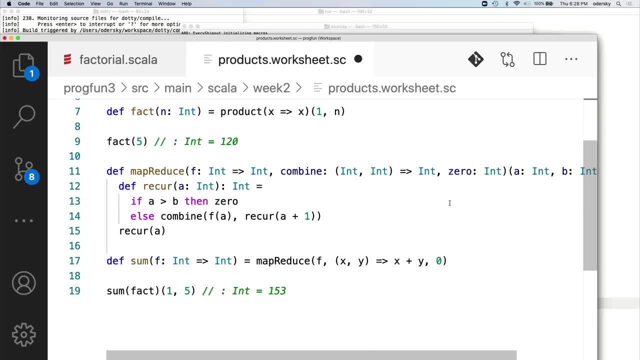 don't need to pass them on to map reduce either, because both sum and map reduce are curate functions. That means what we do here is we just compute the final function that then works on an interval, and we don't need to mention that interval yet. The interval will be mentioned only later, when we apply the 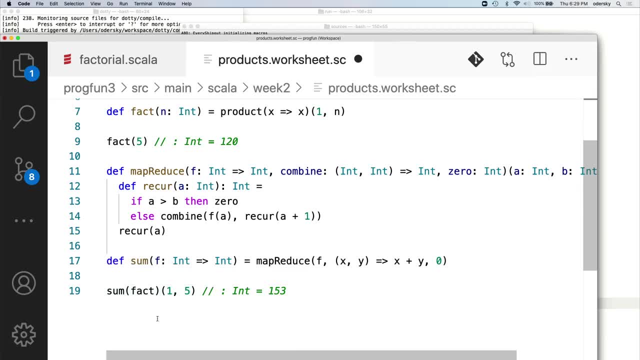 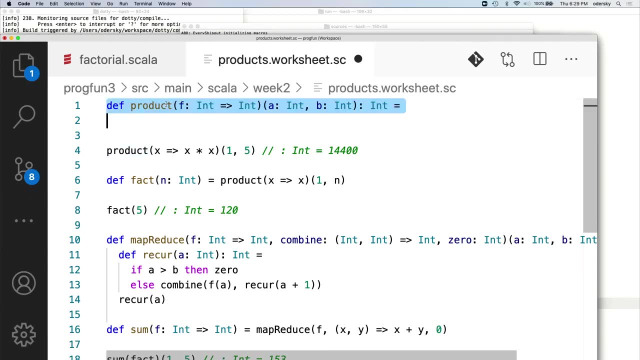 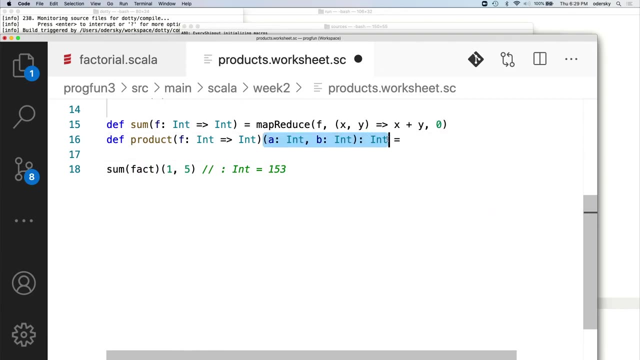 result of sum and fact. So how would we define a product function using map reduce? So let's take, so let's delete the body here and just take the signature and drop the a and the b. We don't need them anymore. So product would. 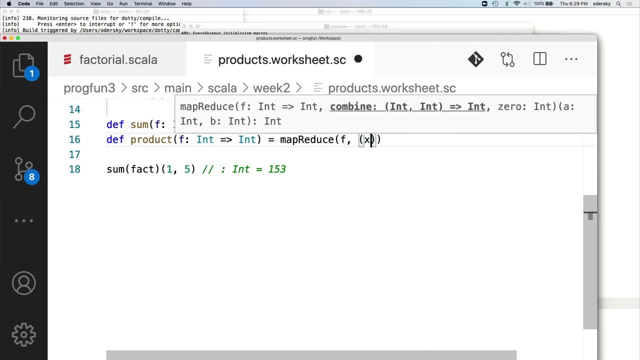 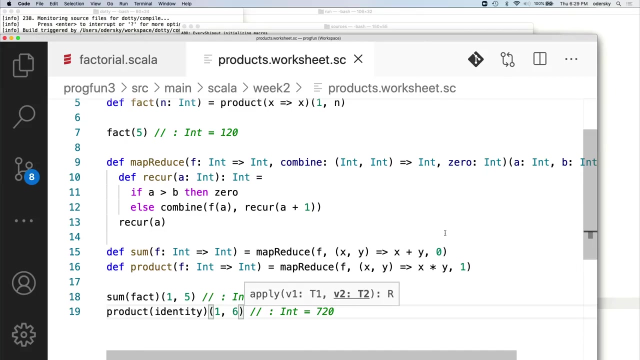 be map reduce of the function f. Now our combination function is multiplication and our zero is one. Let's put that to the test. Let's say: product of identity: one and six, Seven, twenty. Good, So you've seen how we can become very abstract and very concise. 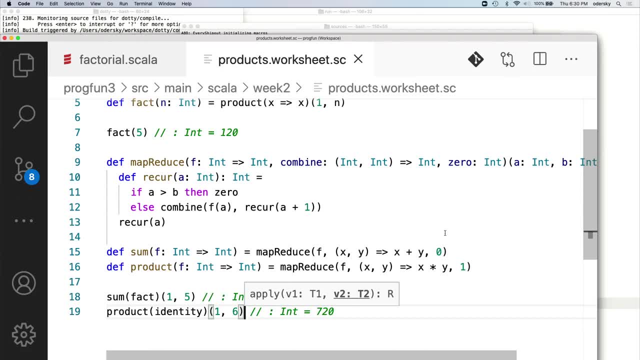 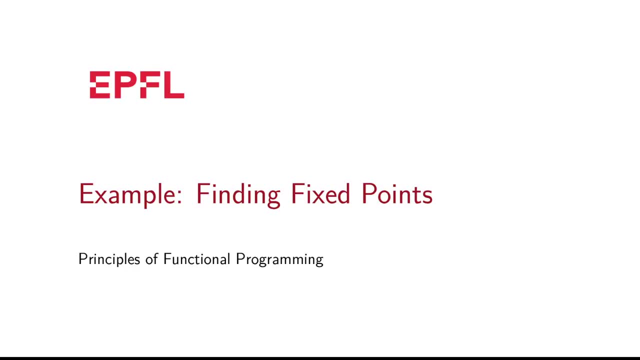 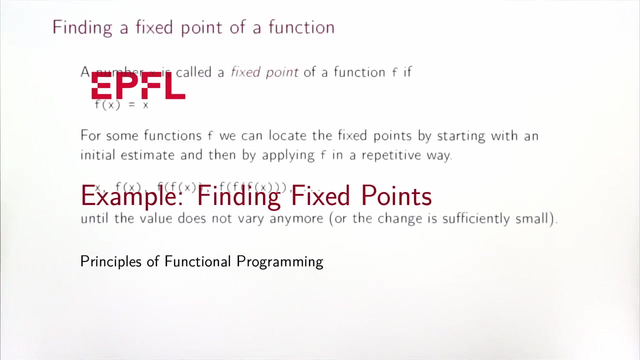 defining functions that take functions as arguments and that return functions as values. In this section we are looking at a somewhat larger example, using higher order functions. in interesting ways, The example is about finding fixed points of functions. A number, x, is called a fixed point of a function if f of x equals x, So f maps x to itself. 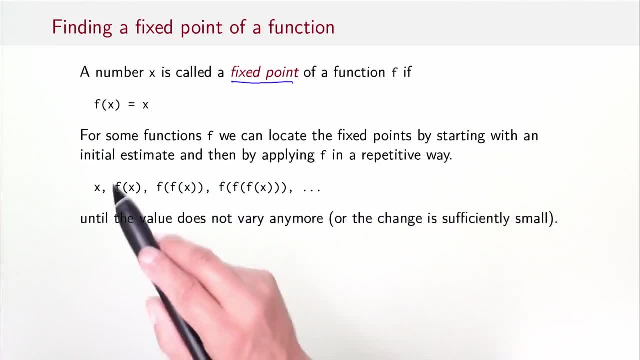 For some functions, f, we can find the fixed points by starting with an initial estimate and then applying f repetitively. So it's x, f of x, f of f of x, and so on, until the value does not vary anymore or the change is sufficiently small. It doesn't work for all functions, but 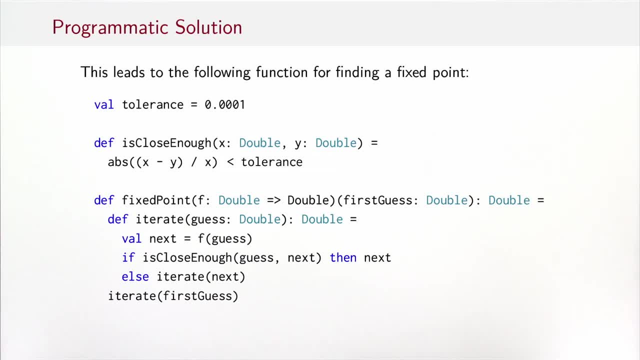 for quite a few it does. So that leads to the following set of functions for defining a fixed point. The idea is we take a function from double to double in that case, and a first guess, And then we iterate until we are close enough. So iteration means we define. 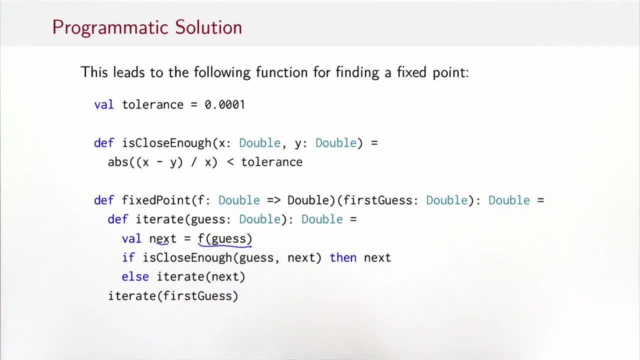 the next function as the application of f to the guess. if we're close enough with the next value, then return the next value and otherwise iterate recursively So to find a fixed point. we then iterate from the first guess. The only thing to do is define. the function is: 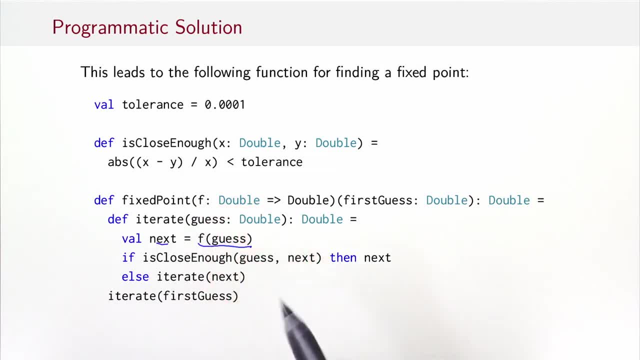 close enough. So the idea of is close enough was that the difference between x and y divided by x should be smaller than some tolerance. So the absolute value of x minus y divided by x should be smaller than some tolerance, which is some small double value. 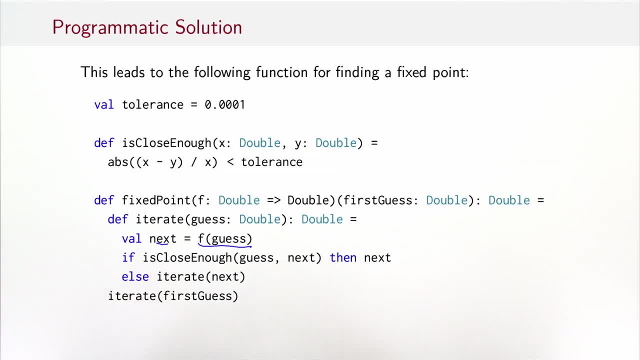 That definition of is close enough is quite similar to what we did for square roots, but it answers the question that I asked when we did. the square root example that we want a definition from for is close enough? that's robust for very small as well as very large numbers. So 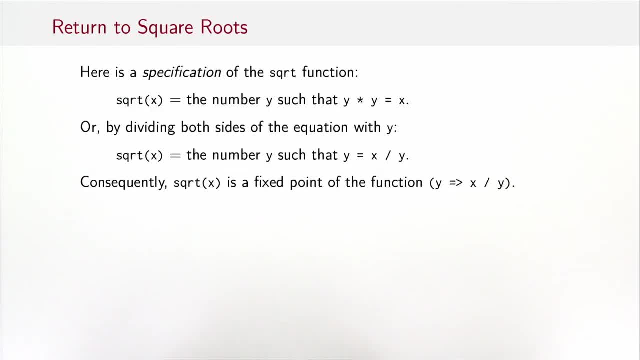 this one is better than what we had before. So let's return to square roots. We can actually use the fixed point function to come up with a new and more principled definition of what the square root function is. So the idea is that if we look at the specification of the square root, 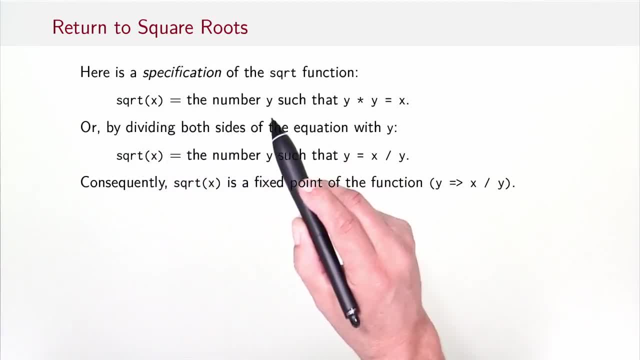 function. then square root x is just the number y, such that y times y equals x. We can also divide both sides of the equation with y, so that means square root x is the number y, such that y equals x divided by y. That means that square root x is a fixed point of the function. that takes a y and gives you x divided. 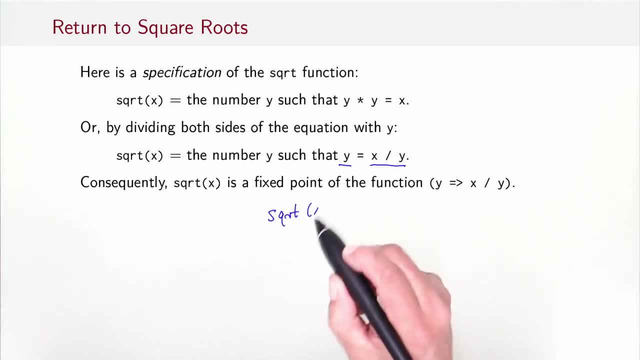 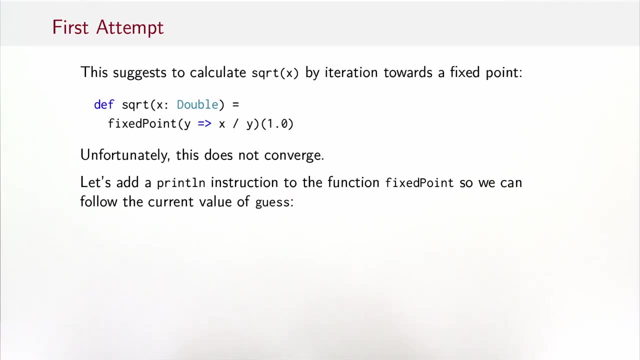 by y. Indeed, that function would map square root x to x divided by square root x. Well, and that's just square root x. so a square root x is a fixed point of that function. So now that we know how square roots can be expressed as fixed points, we can try to calculate square root of x by iteration. 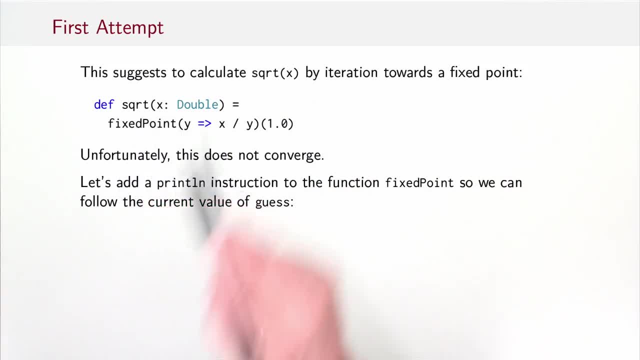 as a fixed point. So we could try this to say: square root of x is simply the fixed point of this function that we've developed previously, and 1.0 as a first guess. Unfortunately, if we try that in a worksheet or rappel, it doesn't converge. It will loop forever. I've copied the fixed point. 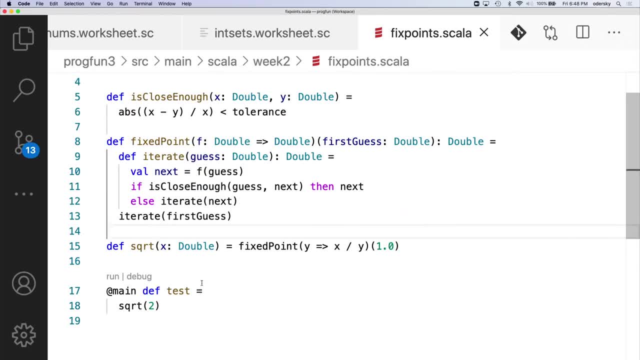 program to a program with a main method test that runs square root of 2.. Let's try to run that. Nothing happens. We stop it. Let's see what goes on. We can try to find out what goes on by putting a strategic. 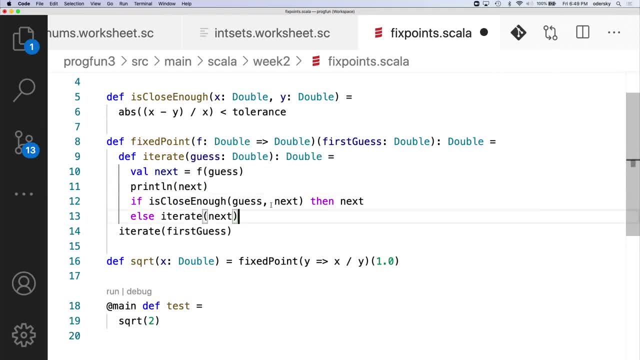 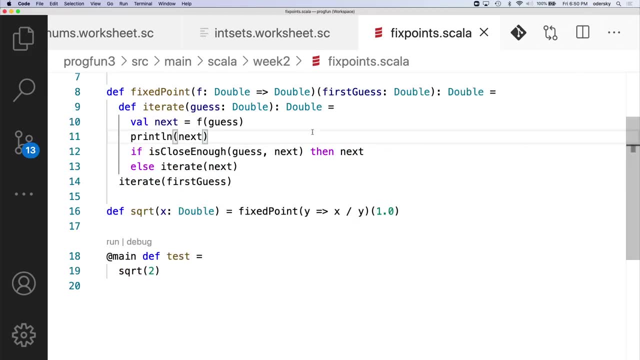 println statement here. So we want to. for each iteration we want to print the value that it just computed at that iteration. So to see what comes out of the println statement, I have to add a debug console here. Okay, let's run the program. So we've seen that. okay, it's an infinite. 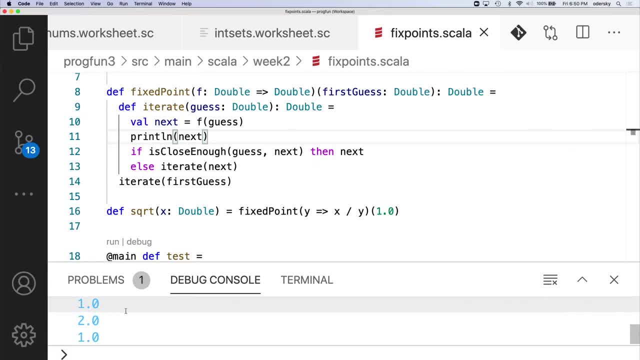 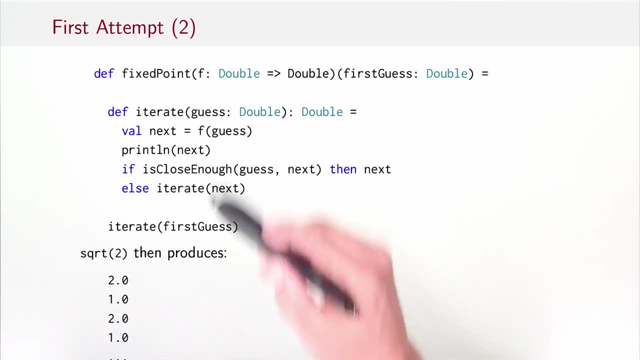 sequence of ones followed by twos. So it doesn't converge. It always oscillates between one and two. So here I've written the same thing. If we do add the println to the iterate, then square root of two produces as output two, followed by one, followed by two, followed by one, and so on. One way to control. 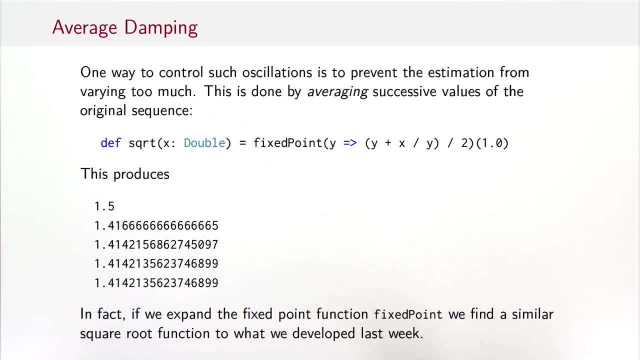 such oscillations is to prevent the estimation from varying too much. A good idea to do that is by averaging successive values. So let's run the program and see what happens. Let's see what happens. So what we could try to do is take the fixed point, not of the function x divided by y. 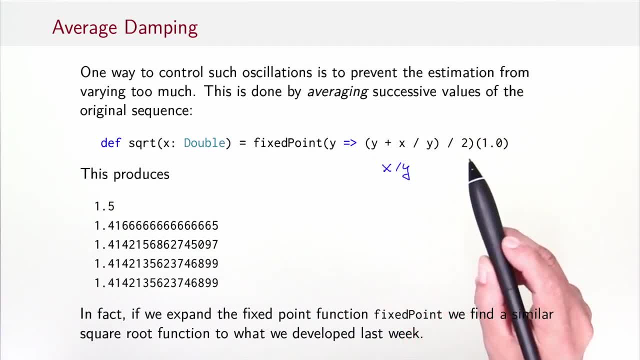 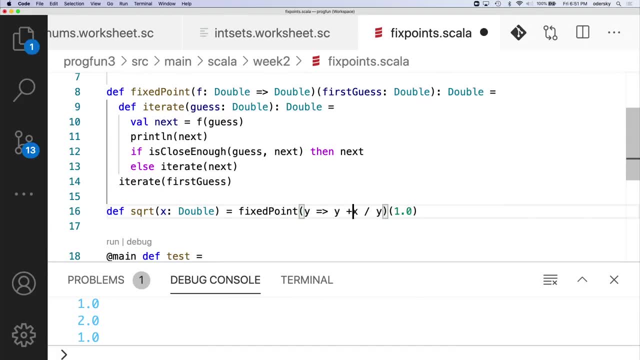 but y plus x divided by y divided by two, So it's the average of the previous value y and the new value x divided by y. So let's do that And run the program again. Okay, so now we see something much nicer. 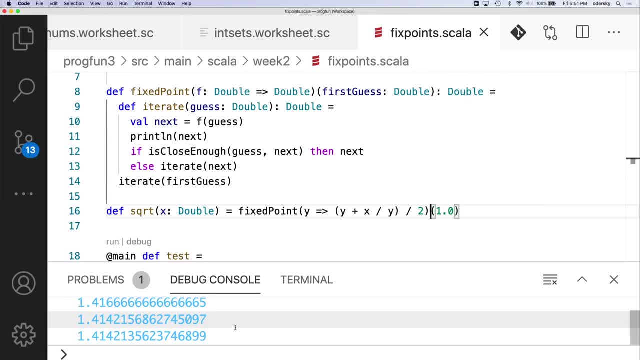 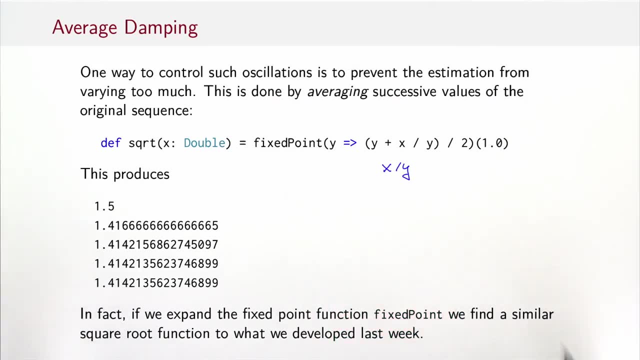 So after we've done that, we can run the program again. So after we've done that, we can run the program again. After four iterations already we are close enough. So it converges very rapidly. In fact, if we expand the fixed point, replace this call to fixed point by the body, by its definition. 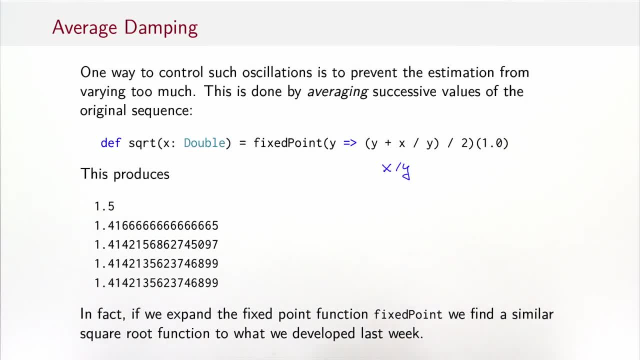 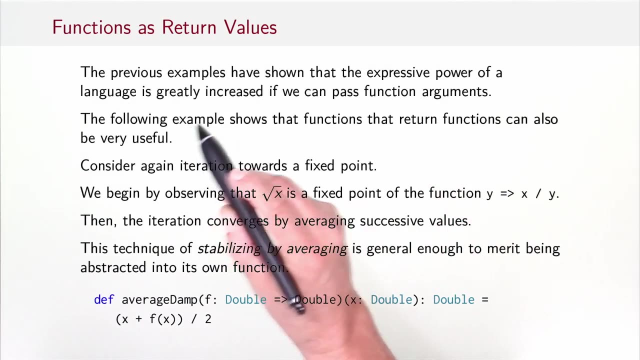 then we'll find a square root function that's quite similar to what we developed last week. So in a sense, fixed point really captures the essence of what we did with square root and generalizes it to other functions as well. So you've seen in the previous examples that the expressive power of a language is greatly. 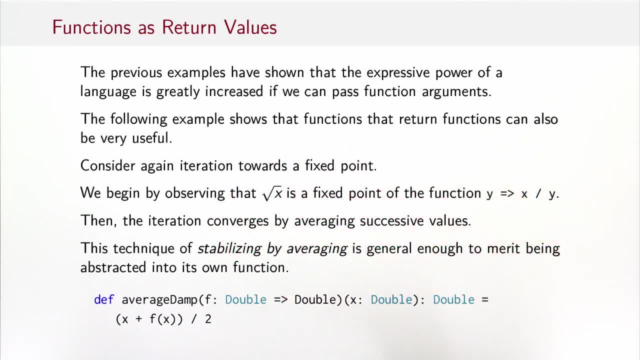 increased if you can pass function arguments. Sometimes it's also useful to return functions as results. For instance, if we look at the iteration towards a fixed point, we began by observing that square root of x is a fixed point of this function. Then we noted that we need to average successive values, And this technique of stabilizing by 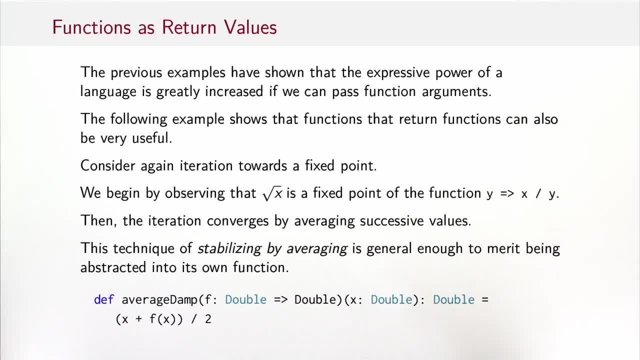 averaging is quite general. It's general enough to merit being abstracted into its own function. So what would this function look like? Well, average damp would take a function from double to double and an argument of type double. It would return the average of the previous value x. 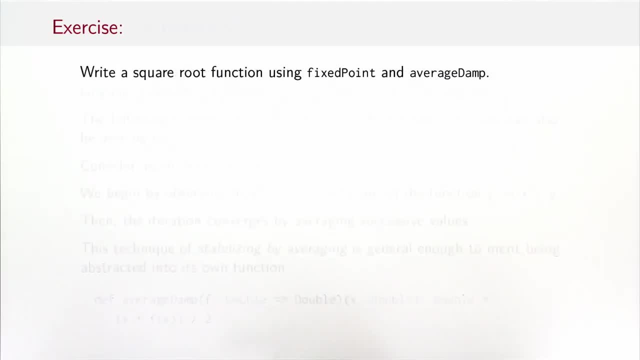 and the new value f applied to x. So now that we have average damp, let's rewrite the square root function using it and the fixed point function that we've seen before. What would that look like? Well, here's the answer. Square root of x would be the. 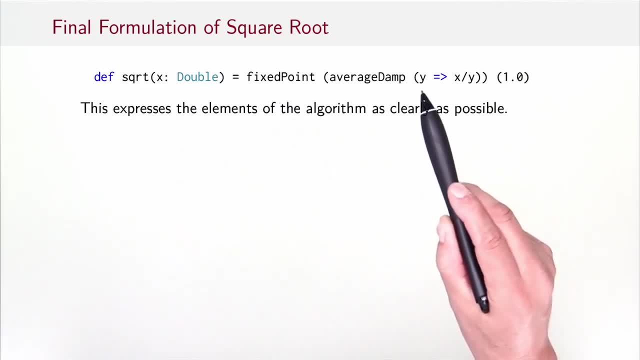 fixed point of the function y maps to x divided by y, subject to average damping. So its fixed point of average damp of the function y goes to x divided by y. I believe you'll agree with me that this expresses the elements of the algorithm, Why square root computes what it computes and 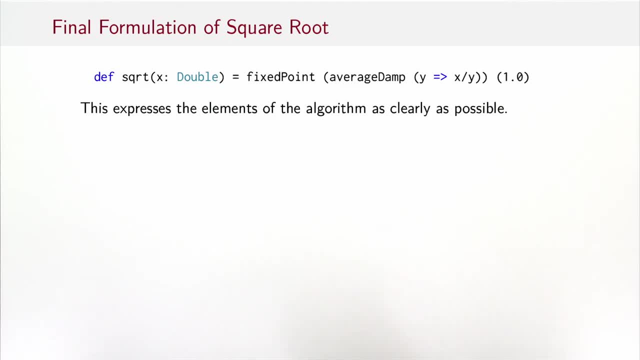 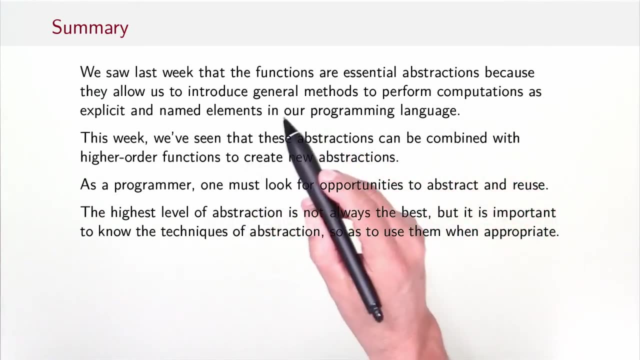 why it has to be written this way as clearly as possible. So to summarize, we saw last week that functions are essential abstractions because they allow us to introduce general methods to perform computation as explicit and named elements in our programming language. This week we've seen that these abstractions can be combined with higher order functions. 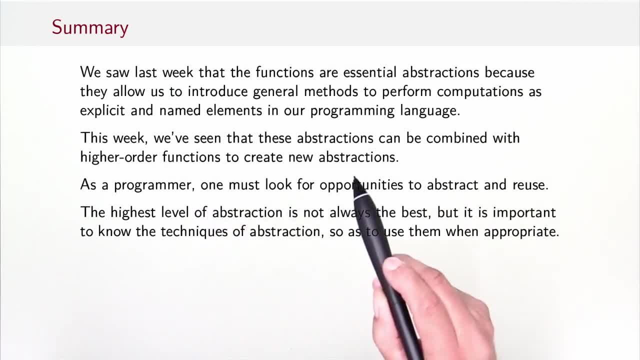 function parameters and function results to create new abstractions. As a programmer, one should always look out for opportunities to abstract and reuse. The highest level of abstraction is not always the best, but it's important to know the techniques of abstractions so as to use them when appropriate. 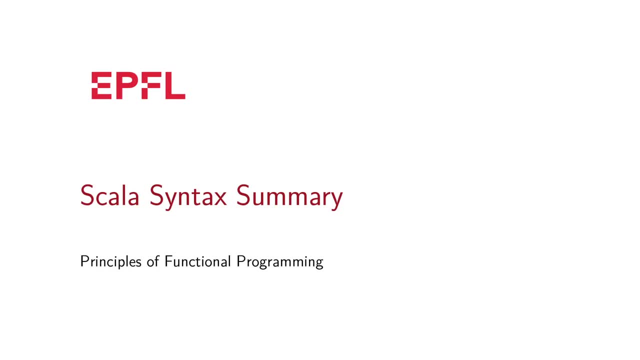 By now you have a useful set of tools to work with functions, including higher order functions. It's time to take a step back and summarize what kind of language constructs we have encountered. So when I describe this language construct, I use a formal notation called extend. this 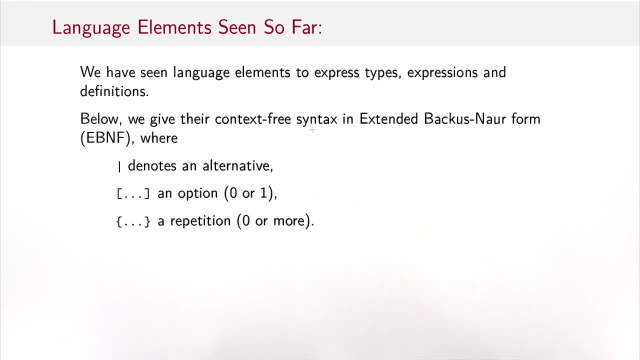 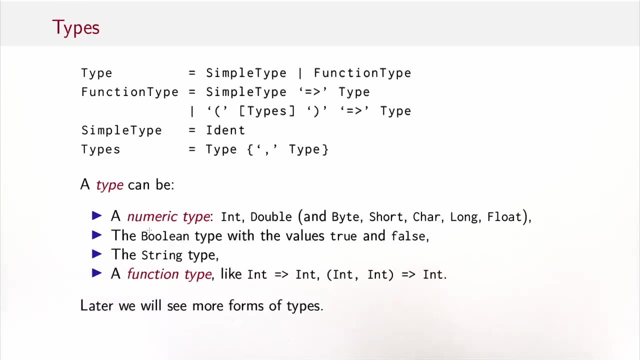 buckles now form. that describes what's called context-free syntax. Essentially, we describe the language by alternatives, by optional elements and by repetition, as well as simple elements. We'll see that in the next slide in an example. So let's start with types. What kind of types have we seen? Well, here it says a type is either: 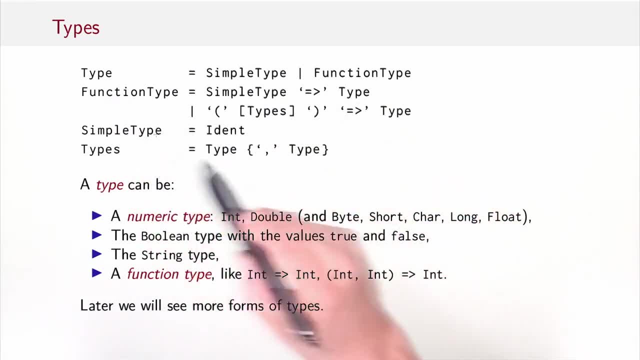 a simple type or a function type, and a simple type is just an identifier and a function type is a simple type followed by an arrow, followed by a type, or that's the bar. it can also be a list of types, in parentheses followed by an arrow and a type. So, types is a type, followed potentially by. 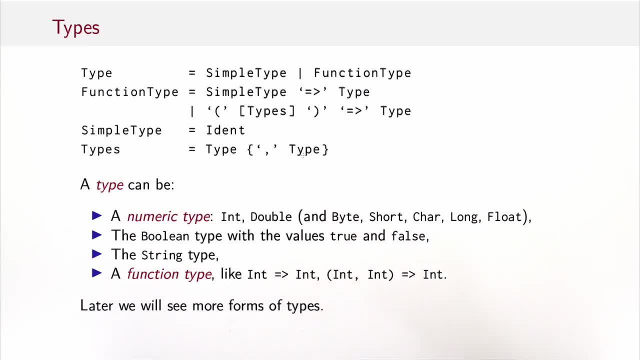 one or more commas and a type. So if we look at the identifiers that can be types, then what we've seen are numeric types like int and double, and they also bite, short character, long and float. We've seen the boolean types with the values true and false. We've seen the string type and then 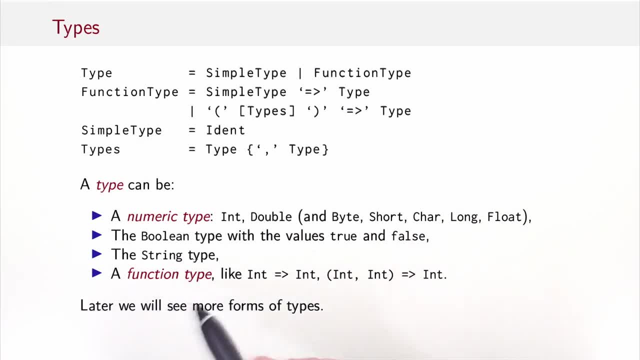 in the compound types. in the structured types we have function types such as int to int or int and int to int. Later we'll see more forms of types, but for the moment that's all we need. Now let's look at expressions. What kind of expressions are available? 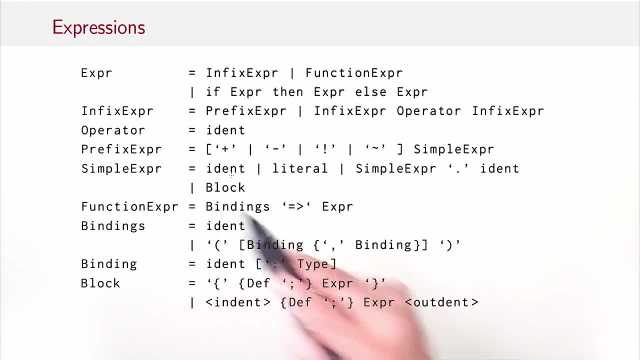 Well, the simplest expressions are listed here. They're just identifiers or literals like five, or a, b, c or that. you can also have an expression followed by an another expression like x, dot, y. Then expressions can also be formed from operators like minus x or plus x. There's also 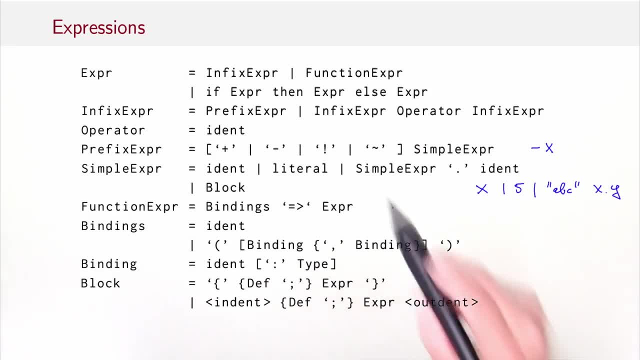 bang for a knot and there's a tilde for one's complement. Then you have infix expressions like x plus one. So that would be an expression that consists of an infix expression and an operator, in this case plus, plus, and an infix expression. And finally you have the conditional expressions like: if x greater zero, then minus x. 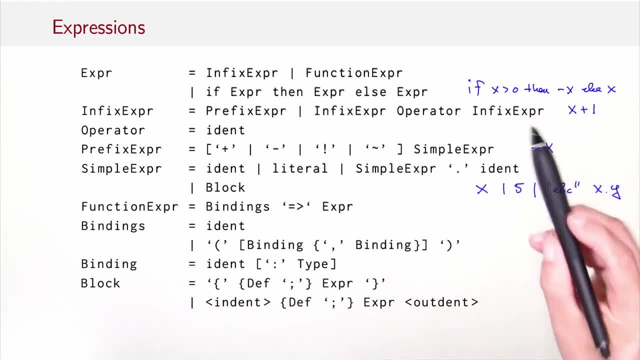 else x. So that would be composed of an expression here, an expression here and an expression here, And you have function expressions like x, x times x. So a function expression is given here. It's a list of bindings followed by an arrow and an. 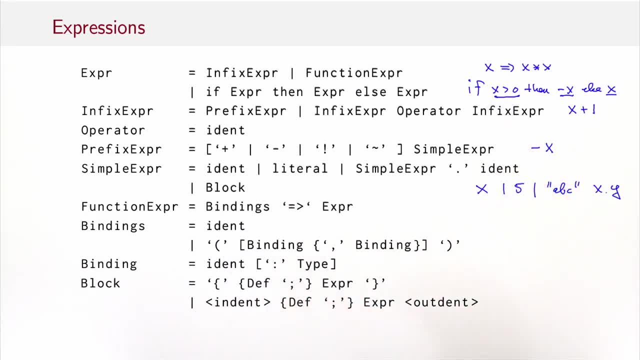 expression and the binding is either a simple identifier- what we've seen here- or it's a list of identifiers in parentheses, like in this binding here, where we describe the anonymous summation function. Finally, we have blocks, So a block is listed in braces like val. x equals two. 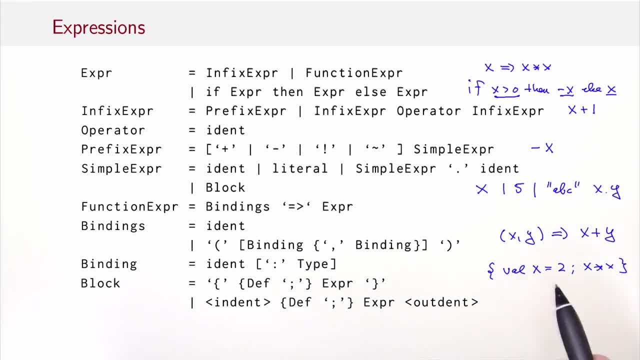 x times x. So that would be a definition and that would be an expression. And, as we've seen, instead of the braces we can also use indentation here and here. So these indent outdent markers, they indicate essentially that here we have the next columns to the right and here we go left again. 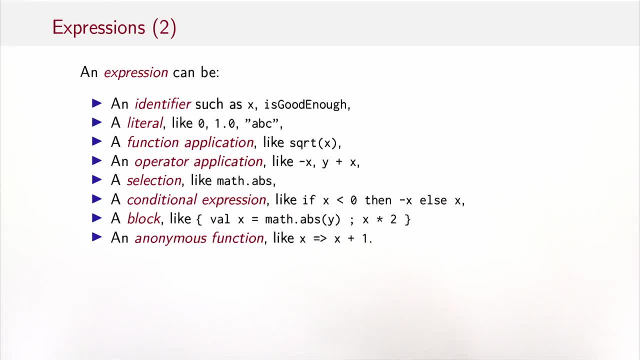 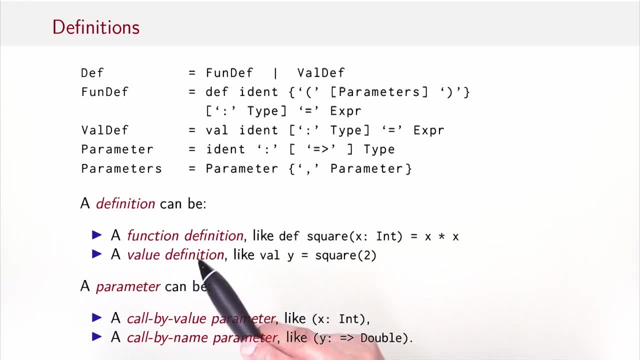 So here you see again a list of all the expressions with examples. Finally, a definition. So a definition can be a function definition, such as def: square x equals x times x, or a value definition, such as val y equals square of two, And the parameter of a function definition can be: 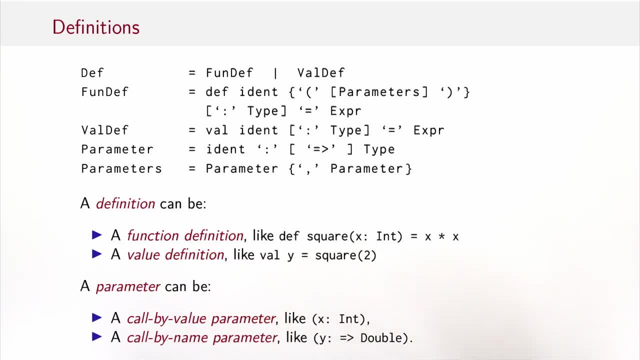 a call by value parameter or a call by name parameter. So that's indicated here by this production for parameter, which says a parameter starts with an identifier, it's followed by a colon, Then there's an optional arrow which indicates a call by name parameter and finally there's the 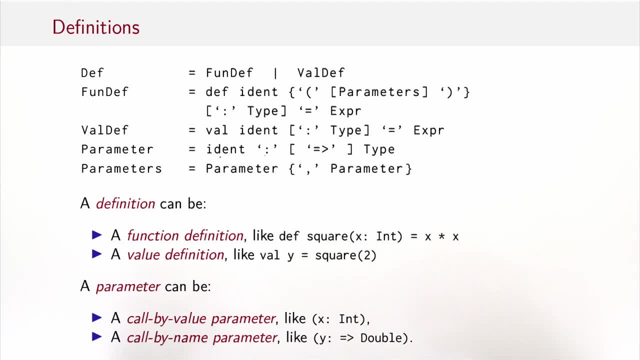 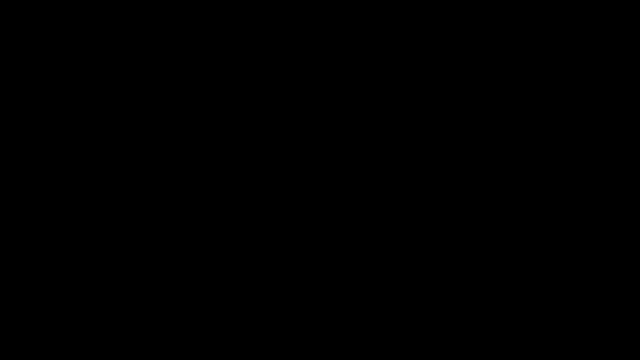 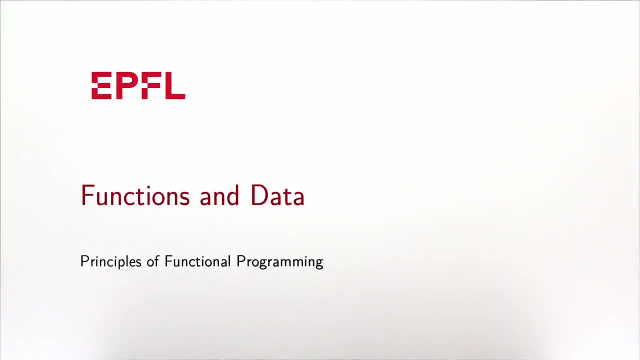 type of the parameter. You can think of this as the basic syntax that describes the core functional features of the language. So far, all our programming was about functions that were operating on values of primitive data types. So, for example, if we want to write a function that is int or string, This will change from now. 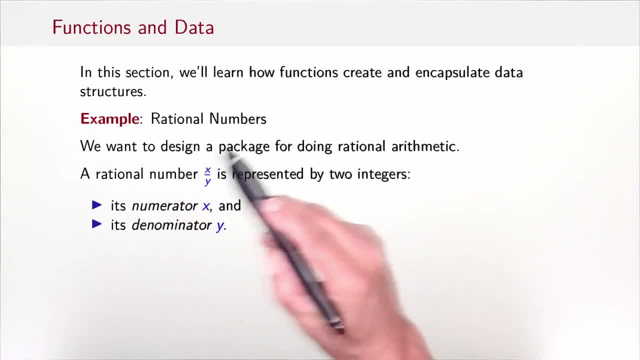 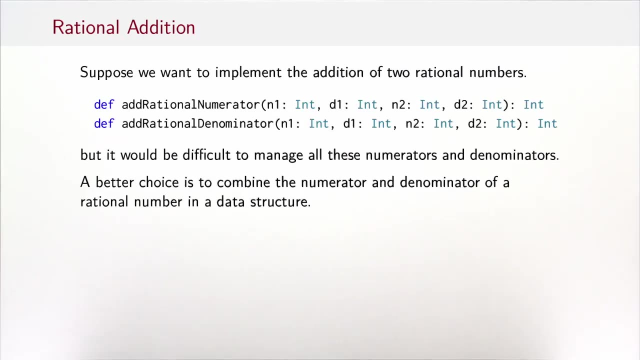 We'll introduce ways to introduce new customized data structures. We'll do that with an example, namely rational numbers. So we want to design a package for doing rational arithmetic. A rational number, x over y, is represented by two integers: It's numerator x and its denominator y, Suppose 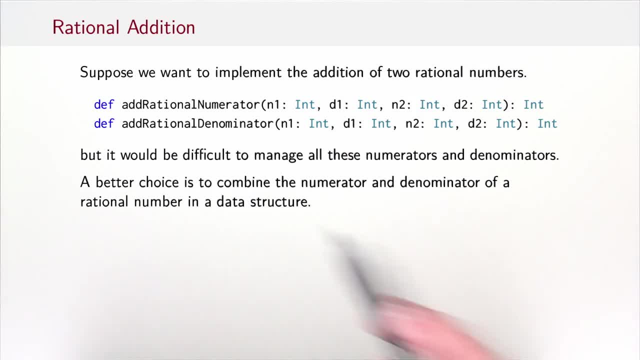 we want to implement addition over rational numbers Without having a special type for rational numbers. we could still write something like this: Add rational numerator and it gets the rational numbers in pairs of two integers here and here. numerators here, denominators here. It would give you, according to the formulas, the numerator. 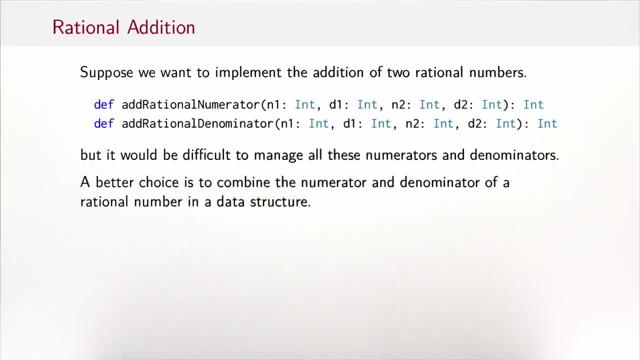 of the new rational number. and then you'd need another complementary function: Add rational denominator. that would give you the denominator. But of course it would be really difficult to manage all these numerators and denominators separately. A better choice is to combine the numerator and denominator of a rational number in one data structure. In Scala we do this by: 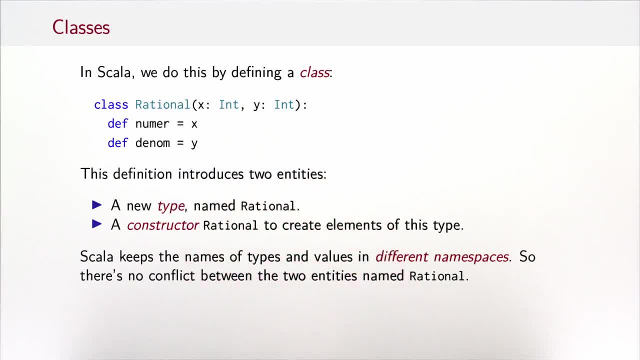 defining a class. Here you see a possible start of a class Rational. You see two parameters here, which are the parameters that become the numerator and the denominator. Numerator and denominator are methods, so-called methods inside class Rational. So a class definition like Rational introduces 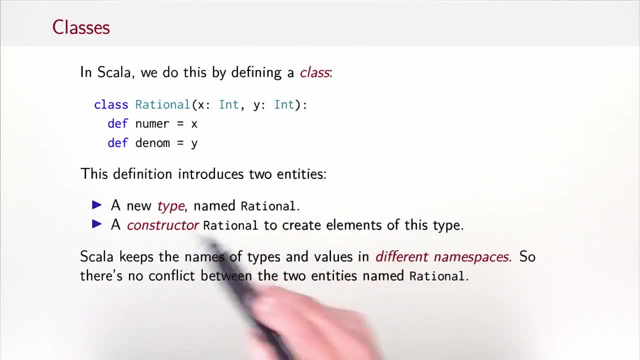 two entities. It introduces a new type named Rational. In the future one can use Rational just like one can use int or string. And it also introduces a constructor, also named Rational, to create the elements of this type. There's no confusion, because Scala keeps the names of. 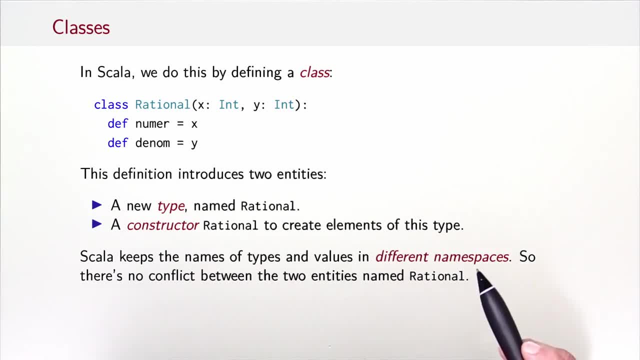 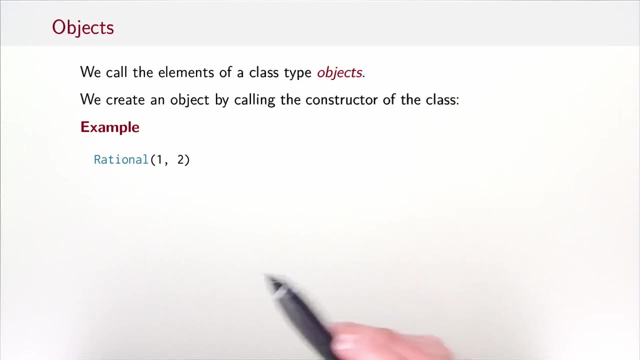 types and values in different namespaces. Otherwise put, it's always clear from the context whether we talk about a type or about a value and constructors. We call the elements of a class type, objects. We create an object by calling the constructor of the class. So Rational would create the Rational. Once we have a Rational number, we 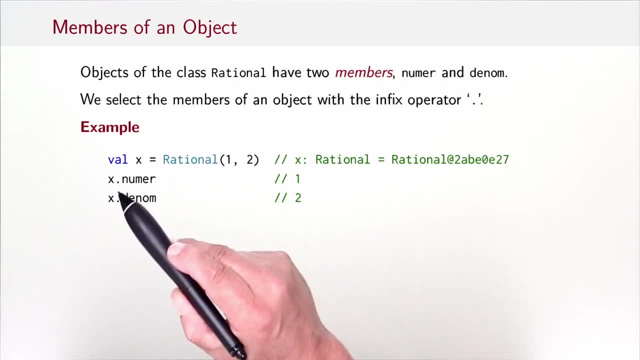 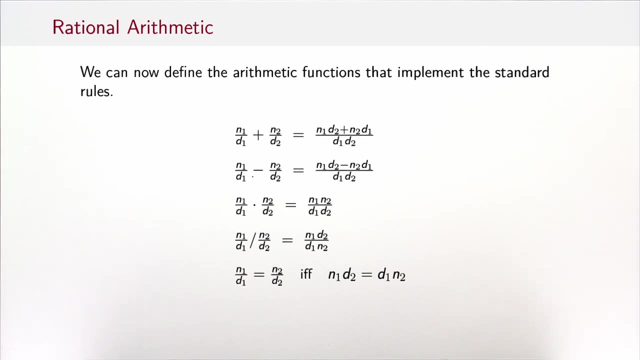 can select its members using the infix operator dot. So if x is the Rational, then xnumer would give you 1 and xdenum would give you 2.. We can now define the arithmetic functions that implement the standard rules. So here you see the formulas for the addition of two Rational numbers: subtraction, multiplication. 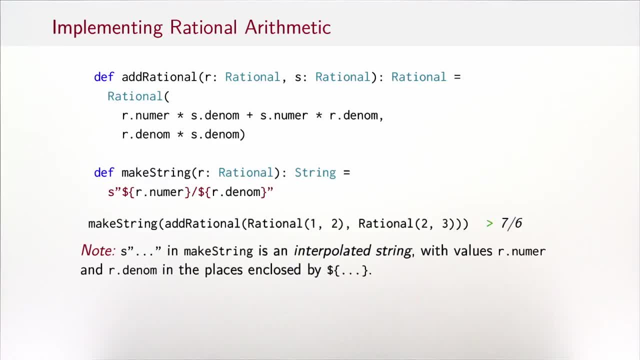 division and equality. So one way to do that would be to add new functions outside class, Rational, For instance. the addRational function would take two Rationals, r and s, and implement the standard formula for addition: It takes the numerator of the left. 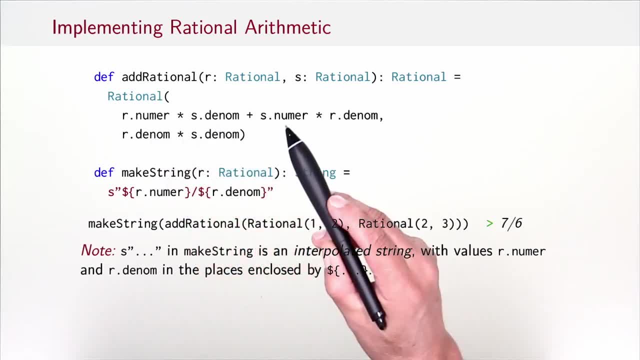 multiplies with the denominator of the right, then the numerator of the right gets multiplied with the denominator of the left, and the denominator of the whole thing is the product of the denominators of the two Rationals. Another thing we might want to add is a method. 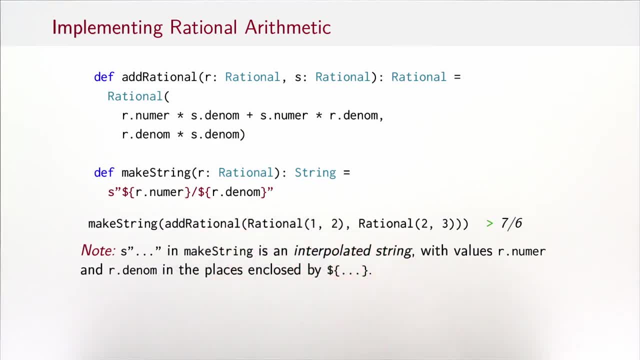 makeString, which takes a Rational number and turns it into a string. So our Rational number one half should be printed as 1 slash 2.. The way we do that is we use here what's called interpolated string. That syntax s quote mark to quote has a special meaning in Scala. 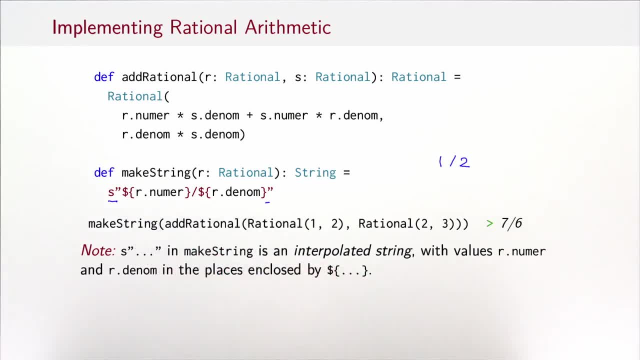 It means that inside these interpolated strings anything that follows a dollar is treated as an expression, So it's evaluated, and then the string value of its result is inserted into that string. So what this expression here would do is it would take the numerator that's 1, convert it to the digit 1.. 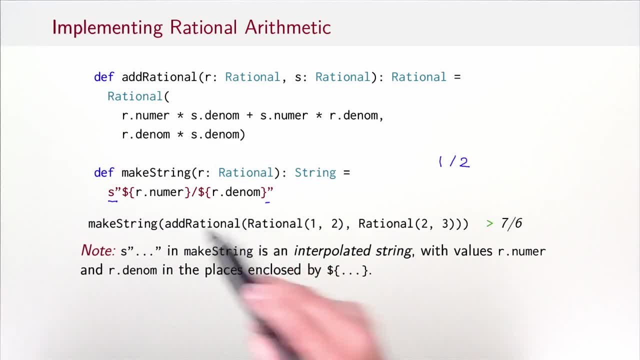 It would take the denominator, convert it to the digit 2 and then splice these results into the resulting string with the slash in between. So that's what you will get. Once we have makeString, we can write expressions like this one: here We can add two Rational: 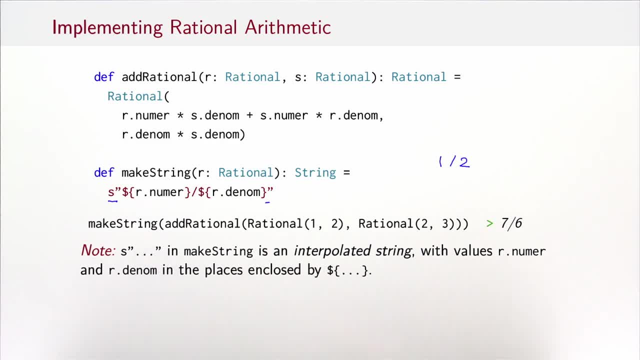 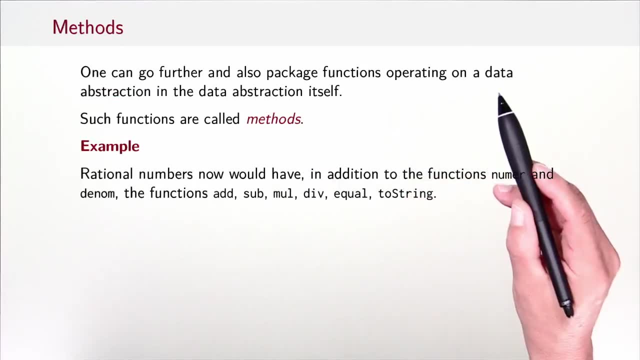 numbers 1, 2 and 2, 3 and convert the result to a string, and we would expect to see 7 slash 6.. One can go further and also package functions that operate on a data abstraction in the data type itself. Such functions that are inside a class are called methods. 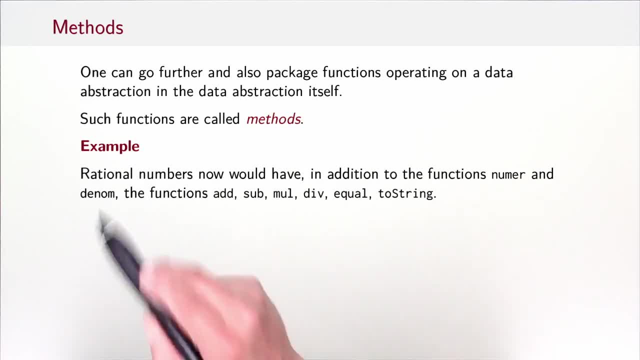 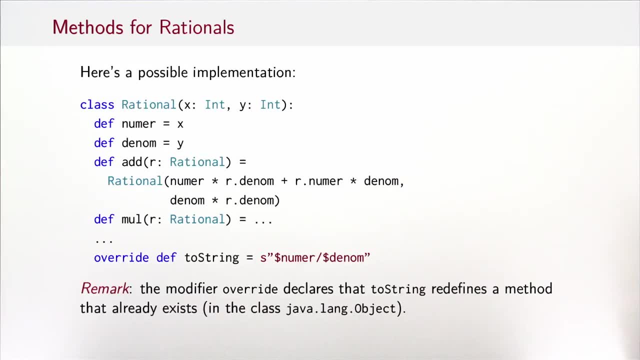 Rational numbers now could have, in addition to the functions numer and denom, the functions add, subtract, multiply, divide, equal and toString. So here's a possible implementation. We have the class Rational. that starts as before, and then we could add a method add that takes a Rational number as arguments. 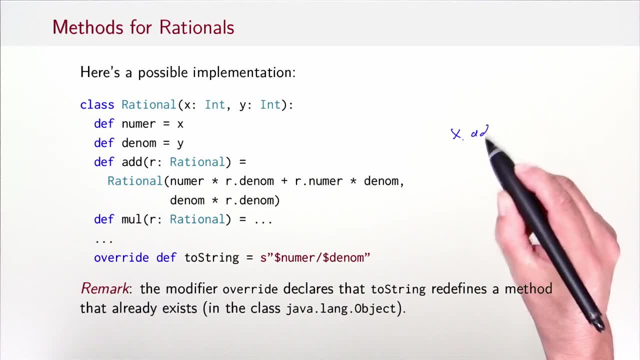 If you have a Rational number x and one which is y, then you would invoke it like this: xadd of y. So it's like numer, but you add an argument here. That means that what the argument here is the right operand of the addition operation and the left operand is the Rational number. 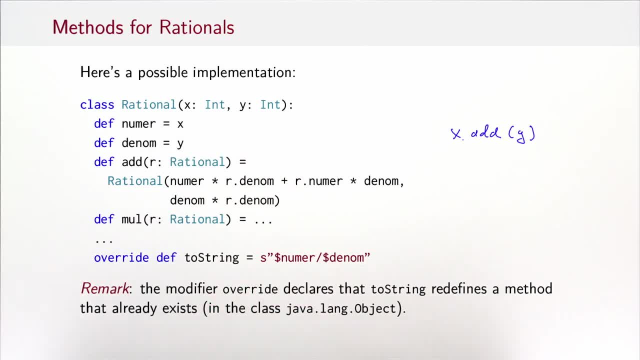 itself in which the add occurs. So, consequently, the formula to create a new Rational number is almost the same as our previous stand-alone method: addRational, but instead of writing the left hand side numerator, we just refer to numerator directly. It's that numerator of the current Rational. 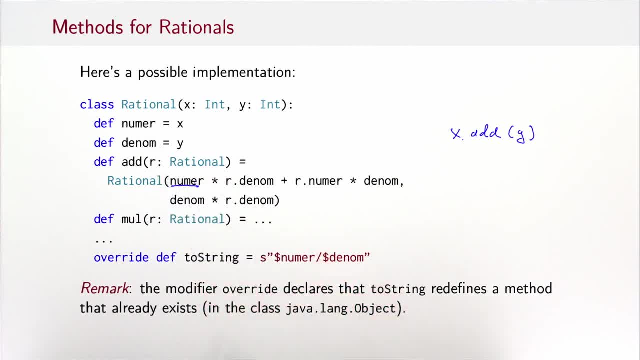 and we multiply it with the denominator of the other Rational number and analogously for the other parts of the formula. So that was addition. In the same vein I can define multiplication. And what about makeString? In fact there is already a standard method toString that all Scalar classes support and that 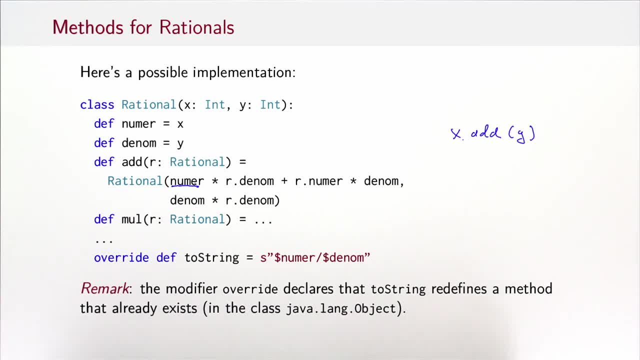 you can customize as you want. So the idea is that for Rational we would customize this toString method to just return the interpolated string. So it's numer denom. We could put it in braces as before, but if the expression is a simple identifier, like numer denom, 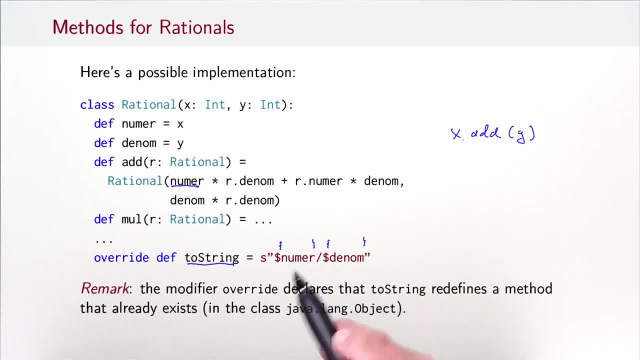 we don't have to, So we can write it shorter: just $numer divided by numer. So we just specify $numer as well. that's what we require. So one thing to notice: that we had used the modifier override in front of the def, That's. 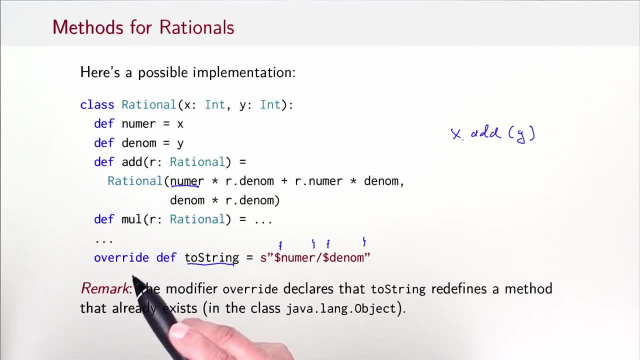 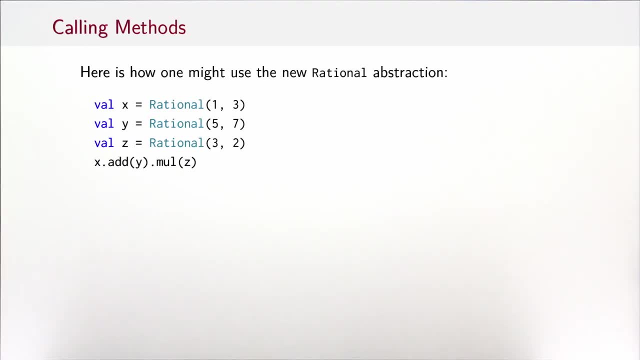 because, like I said, every class already defines a toString method now and the override modifier essentially states that we do not want this default definition of toString, but we want to use our own in class Rational. So here's how one might use the new Rational abstraction. 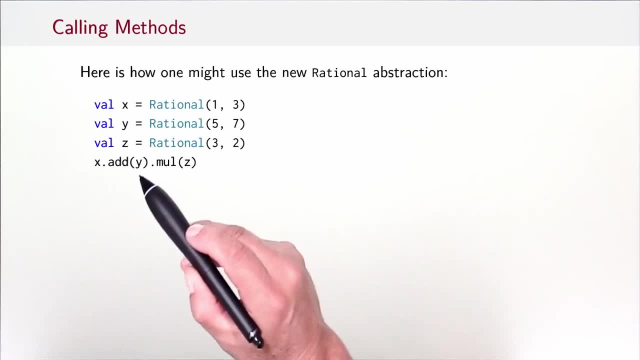 and then add x and y and then multiply the result with z. So in each case the method gets called with the infix dot and the argument of the method is just passed, as you would pass a function argument. So let's put this to the test. 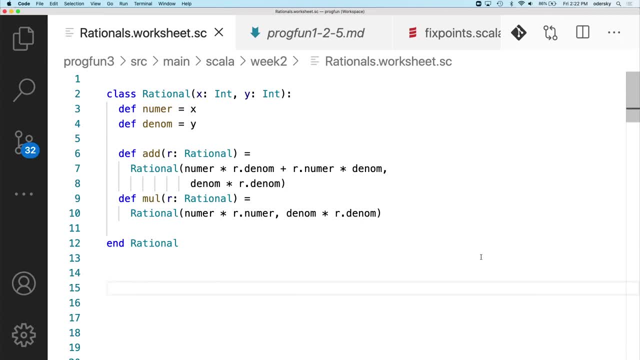 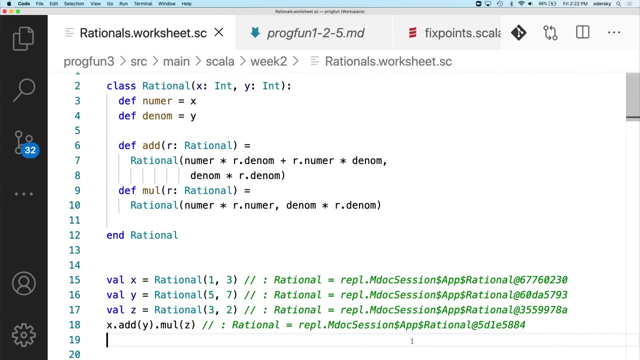 I have defined my class rational, I've added a multiplication method, And now let's just define three numbers and add them and multiply them, And so what we see is not very comprehensible. So what we got here is actually the toString that the class rational got by default. 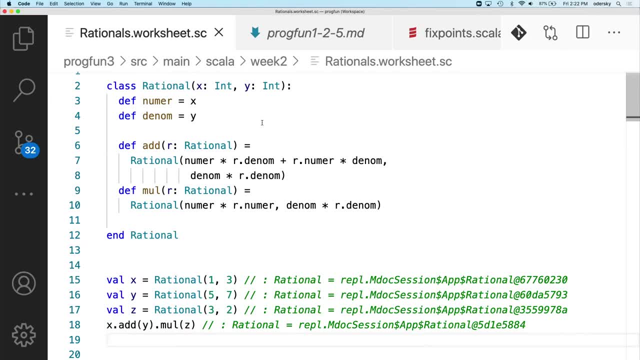 It's so-called inherited from class javalongobject, And that one is not very nice because basically it just tells you what the type is and then it tells you a hash code afterwards- not something for human consumption. So what we need to do is we need to add the toString method as indexed. 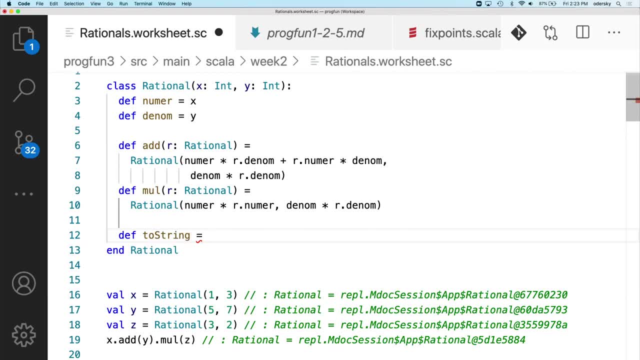 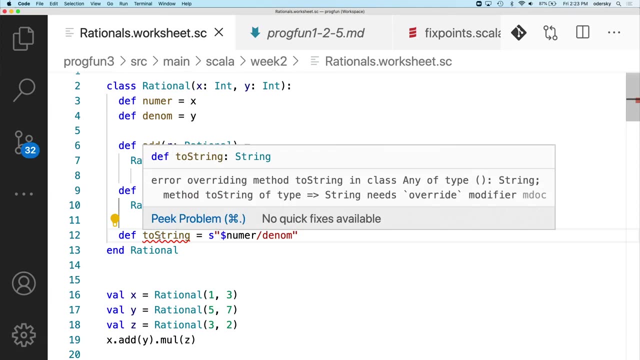 So we say def toString equals interpolated string of nummer and then denom, And then we get an error that says we can't override this method toString in class any because we need an override modifier. So the compiler helpfully tells us that we are changing the 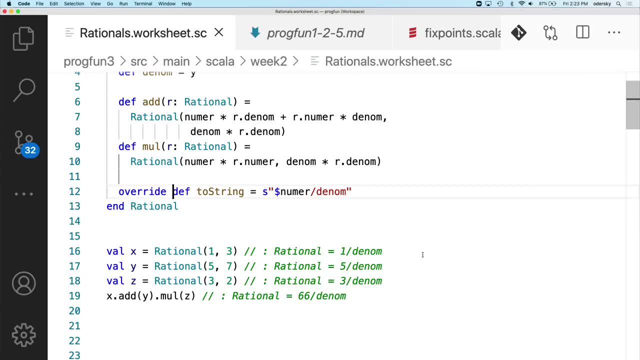 the default behavior and we have to be explicit about it. Once we do that, then we get still not quite the right thing because we forgot to put a dollar here. So let's do that. And now everything looks nice and tidy. So let's finish this session with an exercise. 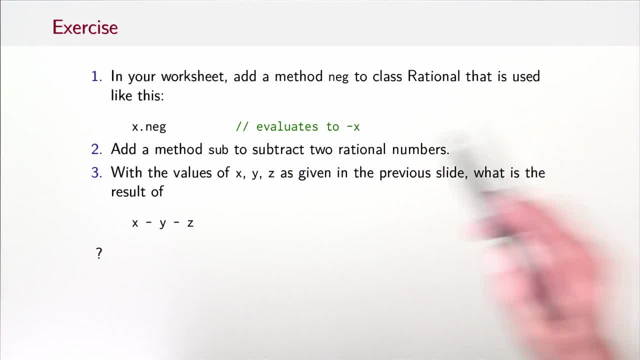 In your worksheet. add a method neg to class rational that's used like this: xneg should evaluate to minus x. Once you've done that, add a method- subtract or sub- to subtract to rational And then you need to add the expression x minus y, minus z. 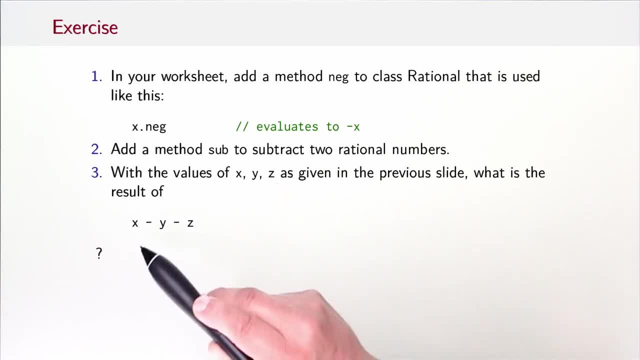 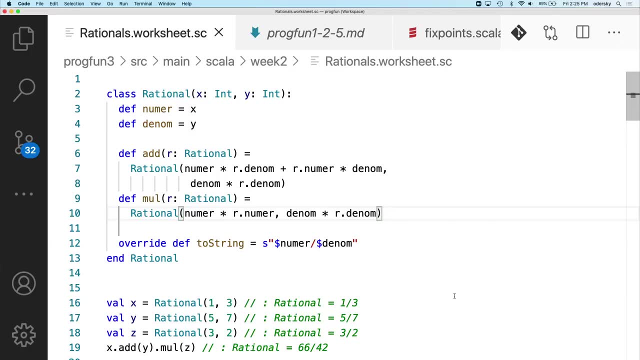 And as a test you might want, with the numbers x, y, z, as given in the previous slide, try out the expression x minus y minus z. So let's get to that. How would we define the neg operation? Well, a simple way to do it is to just create a rational with a negated numerator and denominator. 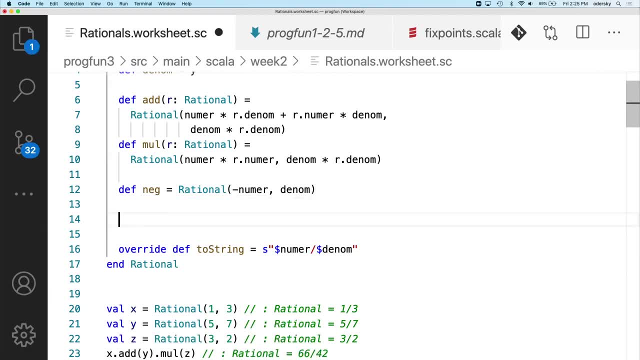 Okay, now for subtraction. So we subtract a rational from the current object. Well, we could alternatively write a expression just like this one here, except with a minus. Or maybe more elegantly, we just make use of neg. So it would be: add rneg. 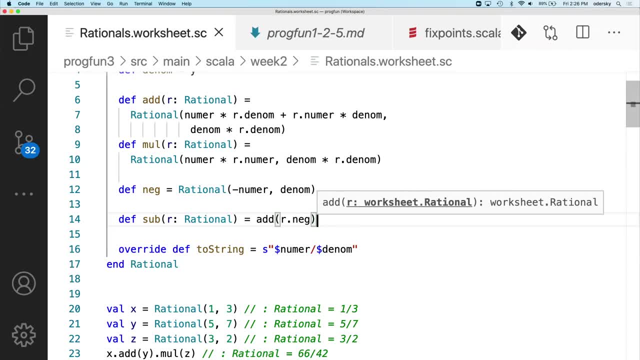 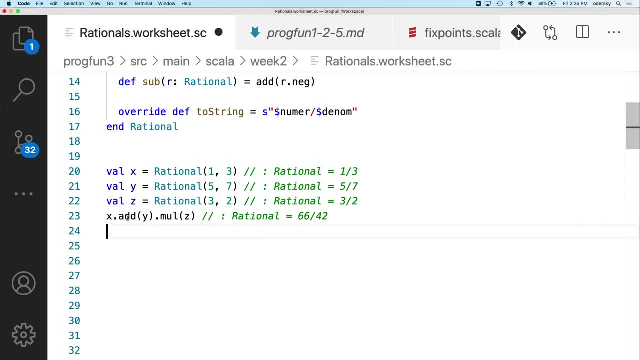 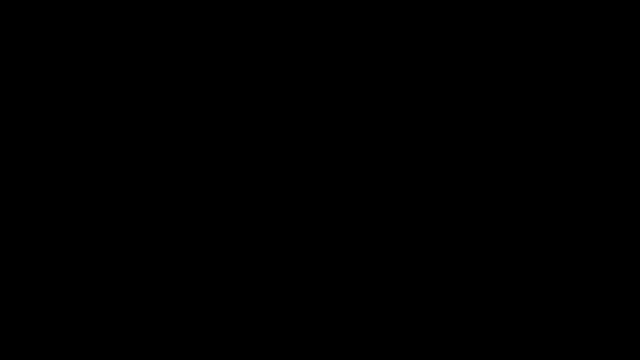 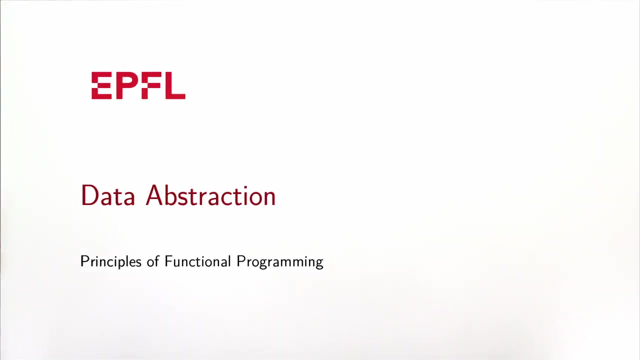 So we add the negated rational and that gives us subtraction. Now let's do the x subtracted by y, subtracted by z, And that gives us the result that you see here. So in this unit we are going to learn about data abstraction. 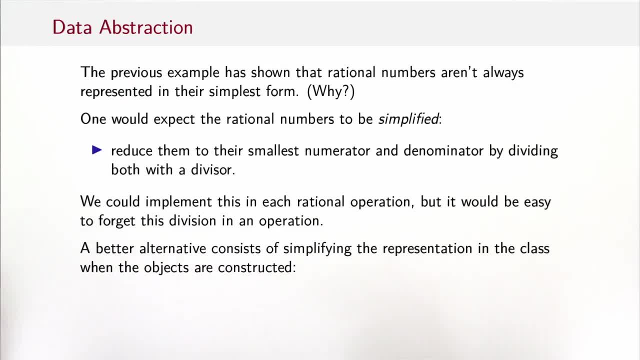 So the previous example has shown that rational numbers aren't always represented in the simplest form. For instance, we saw a rational number 66 to over 42. So you might have expected to see 33 over 21 instead, which is the same rational number. 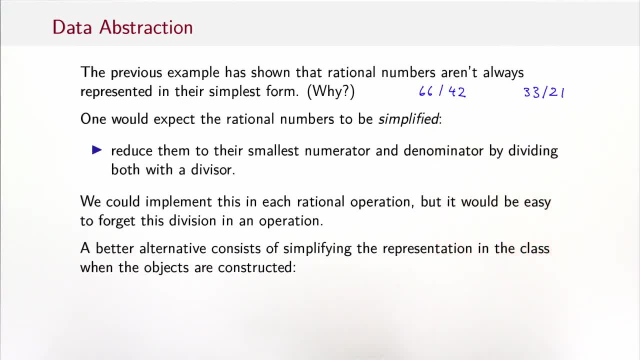 but reduced. the numerator and denominator are both the smallest possible. So what we would like to do is simplify rational numbers, which means reduce them to the smallest numerator and denominator By dividing both with a divisor. We could, of course, implement this in each rational operation. 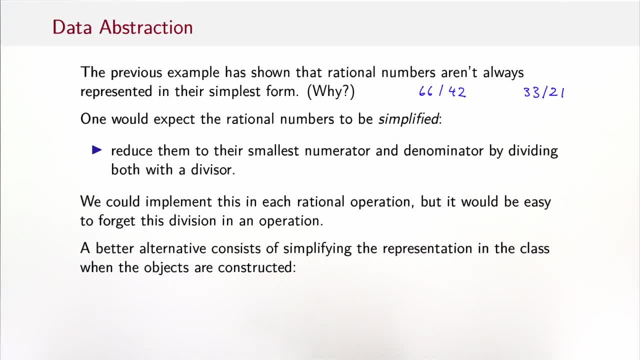 but it would be easy to forget this division in an operation And besides, we don't want to repeat ourselves over and over again for each of the implemented operations. So a better alternative is to simplify the representation of the class when the objects are constructed. 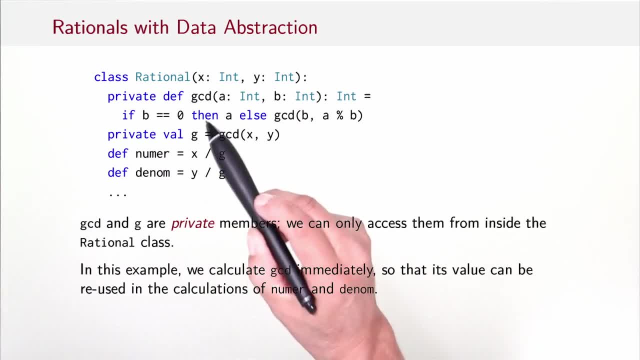 So the way we could do that is, we can define a method, gcd. that's the greatest common divisor function that you've already seen in class rational. Now gcd is used only internally, so it's labeled here. private Clients of class rational can't call gcd directly. 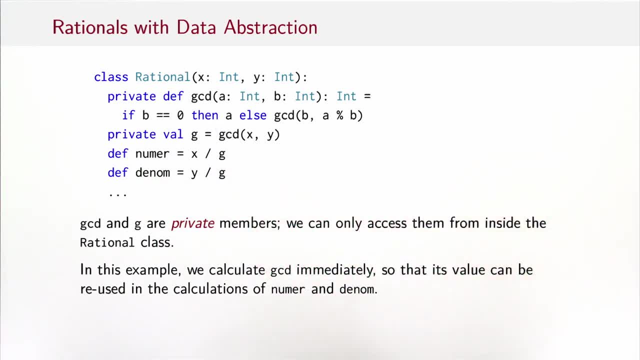 It's used only for the internal functioning of class rational. Then we have another value, g, which is the gcd of the numerator and the denominator, which is always also private. You shouldn't access it from the outside. And then, finally, we have the numerator and the denominator: is x divided by g and y divided by g. 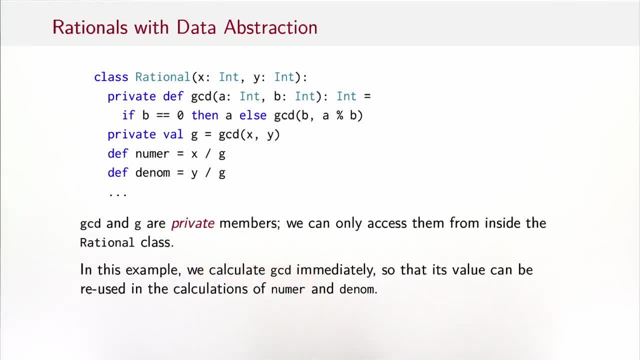 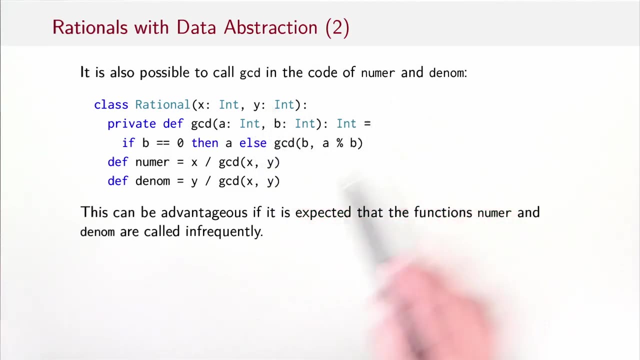 So that gives us the smallest possible numerator and denominator. So in that example we have calculated the gcd immediately so that its value can be reused in the calculations of numer and denom. It's also possible to call gcd in the code of numer and denom directly. 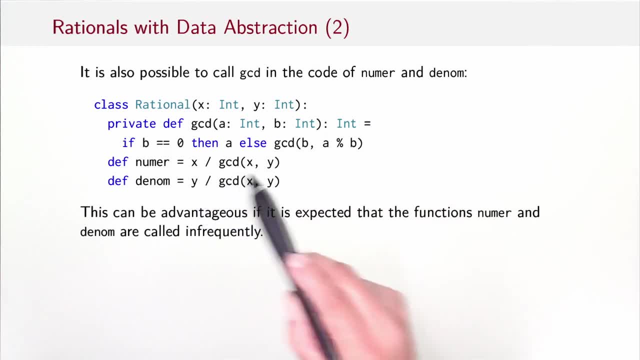 So here, instead of having a separate variable, we would just divide by gcd here and here, And that can be advantageous if we wouldn't expect the functions numer and denom to be called very often. It's equally possible to turn numer and denom into vowels. 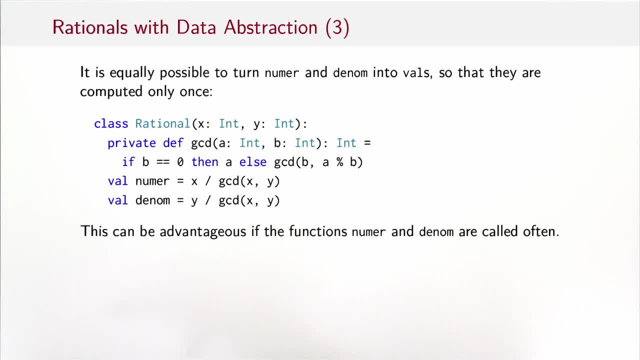 so they are computed only once, And that can be advantageous if the functions numer and denom are called often, which we would expect is the normal case. So the normal case would be a private method, gcd, which is called in the initialization, but it's also a supervisor for the numer and denom values. 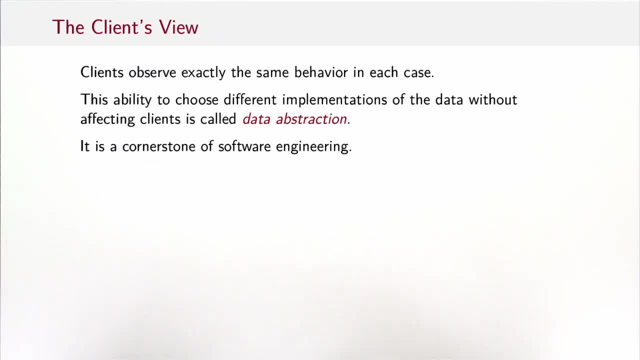 So the point is that if you're using rationals, clients of class, rationals observe exactly the same behavior in each case. It doesn't matter where exactly you define the gcd, whether you create a separate value to hold it, or whether numer and denom are values or methods. 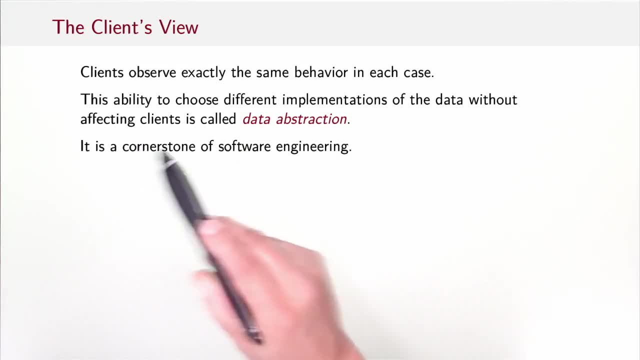 This ability to choose different implementations of the data without affecting clients is a cornerstone of abstraction, And it's a cornerstone of software engineering really, because it allows you to adapt and refine the implementation without affecting the clients. You can see locally in a class. 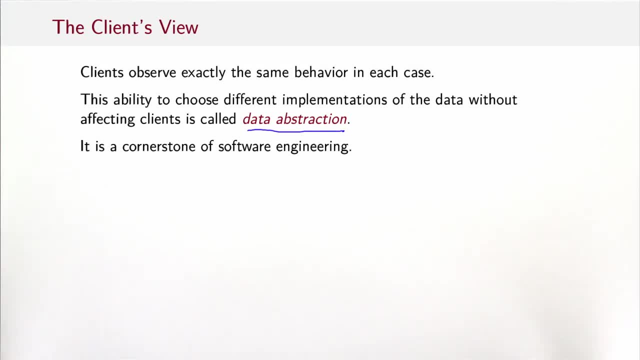 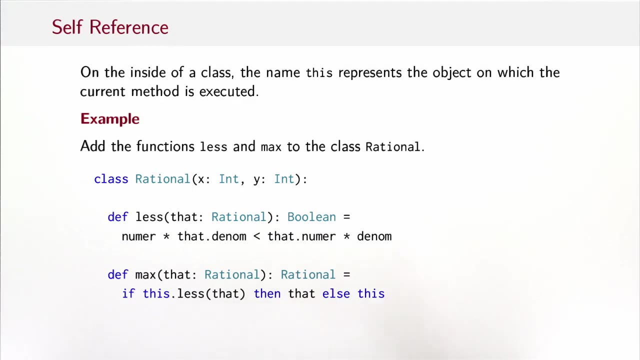 you can reason locally about a class without having to keep the whole program in your head and track the side effects that your class might have on all the rest of the program. So another important concept when we talk about objects and classes is self-reference Inside a class. 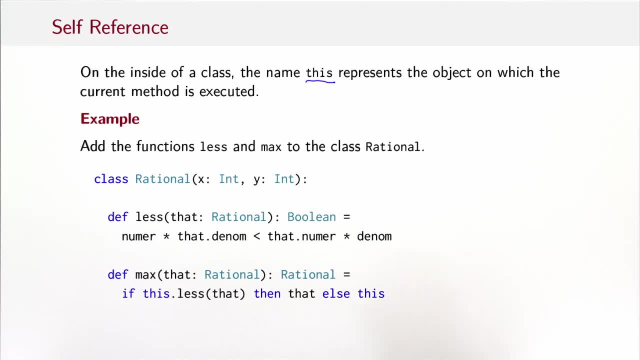 the name. this represents the object on which the current method is executed. So, for instance, if you would like to add functions less and max to the class rational, then here's what you would do. We define the less method as usual. So if you want to say x1 over y1, 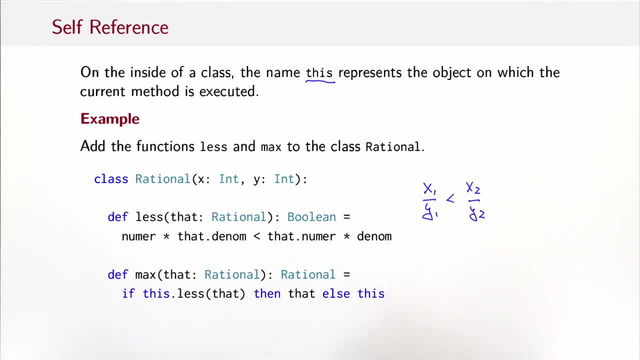 is less x2 over y2, and that's equivalent to: essentially, we just multiply everything by y1 and y2, so that's equivalent to x1 over y2, less than x2 over y1. And that's what we implemented in this formula here. 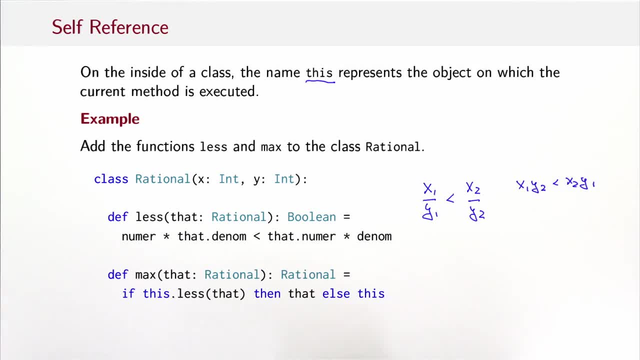 Now let's look at the max method. To implement max, we would ask whether the current rational number is less than the right-hand side argument. In that case we return the right-hand side arguments and otherwise we return the rational number itself. So you can see here that the ability 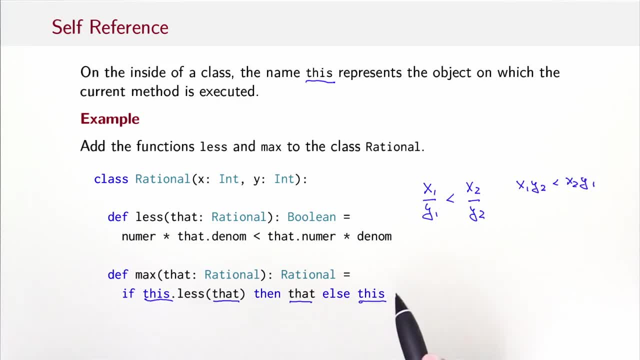 to name the current object with. this is essential because otherwise we couldn't return the current object as a result of an operation. The other occurrence of this was here, where we used the less method on the current object. That one is equivalent to just writing less of that. 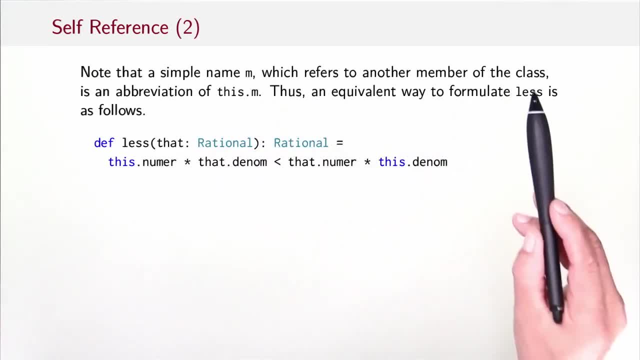 So, in general, a simple name that refers to another member of the class is just an abbreviation for thism. Thus, an equivalent way to formulate less is as follows: thisnumer times thatdenominator. less than thatnumer times thisdenominator. 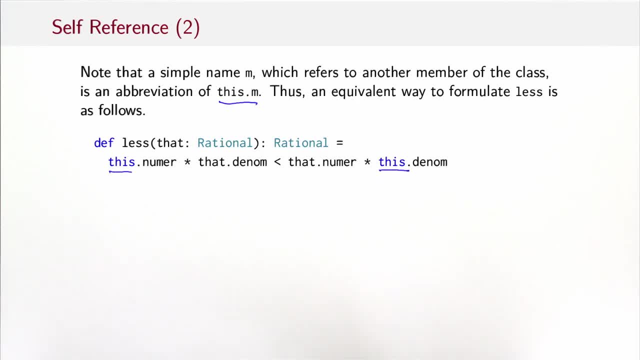 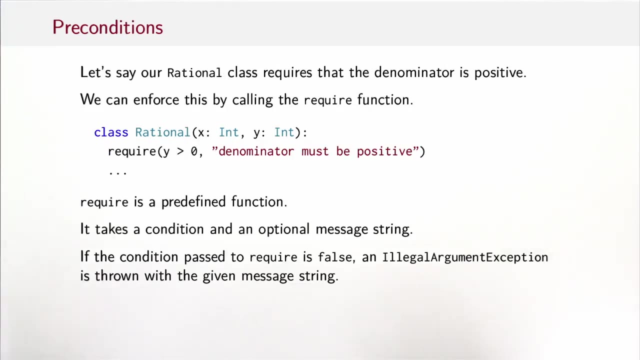 So now we have made it explicit everywhere that we mean the current object, But we can also leave out these two references to this and just write numer and denom as before. The meaning is exactly the same. So let's look at more tools that are useful for dealing with data abstractions and classes. 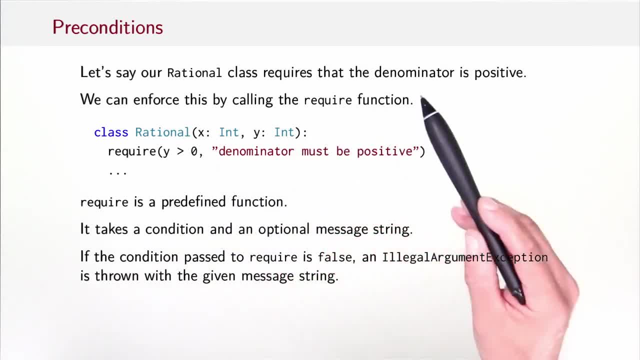 Let's say in our class Rational we want to require that the denominator is positive. We can enforce that by calling the require function. So we could start class Rational with a function which is require y greater 0. Denominator must be positive. require is a predefined function. 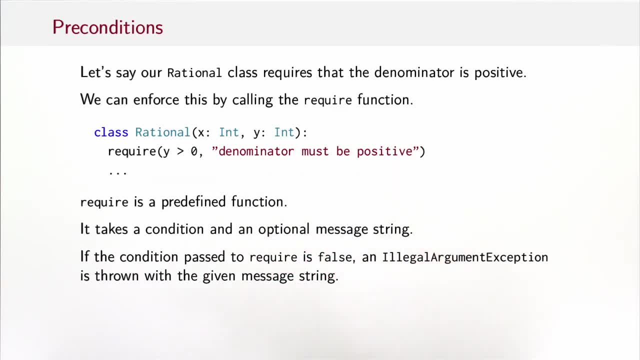 It takes a condition and optionally a message string. If the condition is false then it throws an exception called an illegal argument exception and that takes the message string as an argument. Throwing an exception will usually terminate the program with the message string, but there are ways to handle it later. 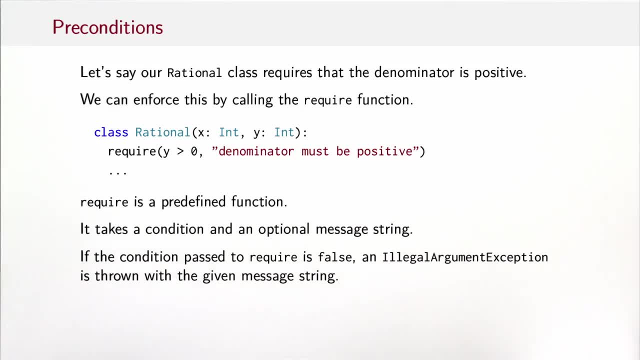 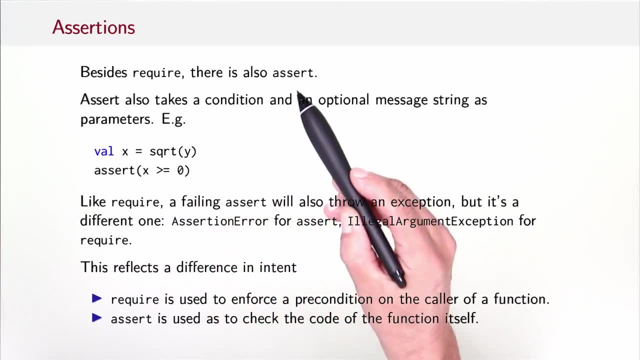 and we'll learn about those later on. For now, we can think of throwing an exception as just a way to terminate the program. Similar to require, we also have the predefined assert function. Assert, like require, takes a condition and an optional message- string as parameters. 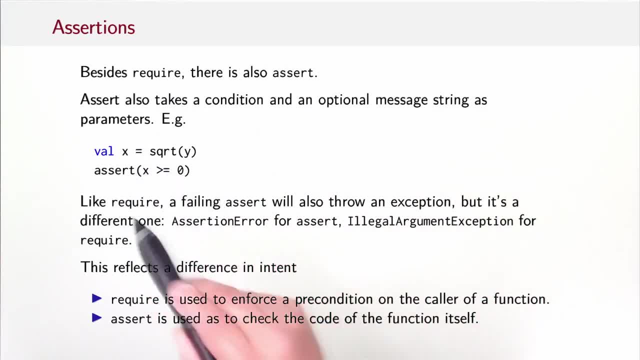 So, for instance, we could write: val x equals square root y, assert x greater or equal 0.. An assertion like this states something that should be true. If the condition is false, then it will also throw an exception, but it's a different one. It's called an assertion error for assert. 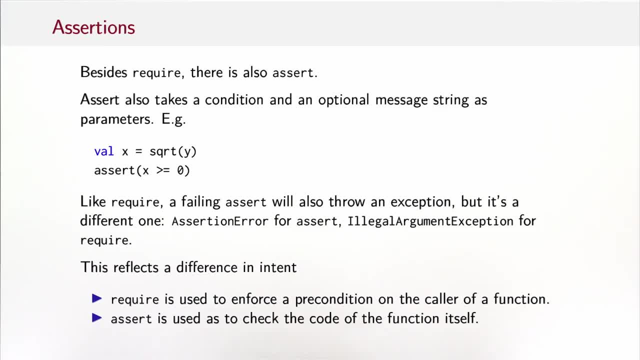 whereas it was an illegal argument. exception for require: That reflects a difference in intent. Require is used to enforce a precondition on the caller of a function, So if require goes wrong then the fault is with the code that called the function, whereas assert is used to check the code of the function itself. 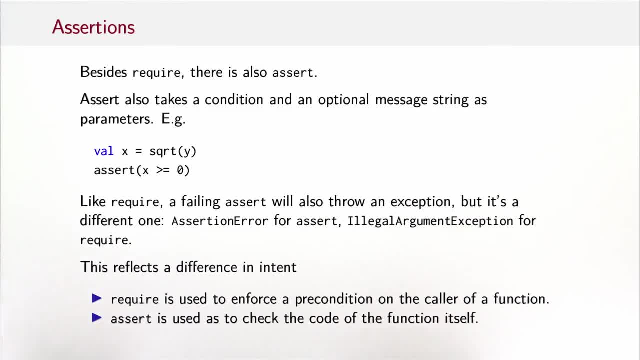 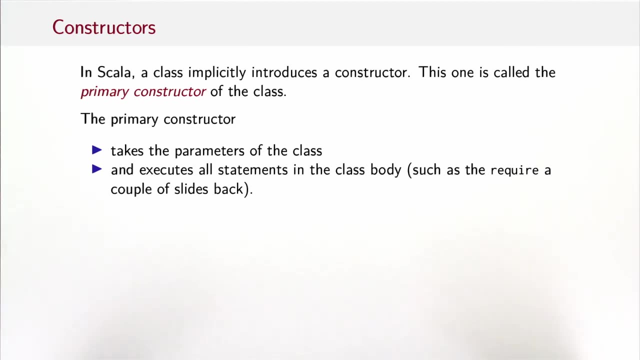 So if assert is wrong, then essentially we have a bug in the implementation of the function. It was called, probably with the correct arguments, but the implementation is wrong. So we've seen that a class implicitly introduces not just a type but also a constructor, a way to construct elements of that class. 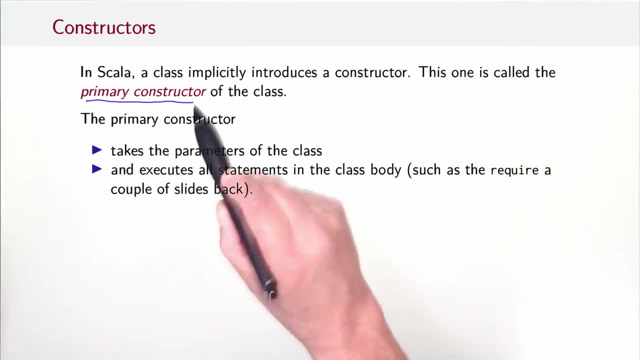 This implicit constructor is also called the primary constructor of a class. So the primary constructor takes the parameters of the class and executes all statements in the class body, such as the require a couple of slides back, or the value definitions of numerator and denominator or any other statement that's in the body of a class. 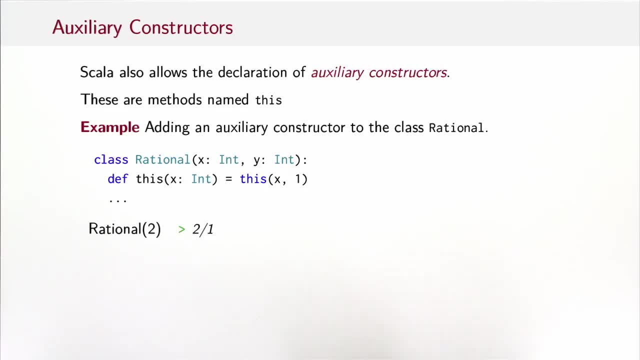 So when I said primary constructor, that implies that there could also be other constructors, and in fact that's the case. Scala allows the declaration of auxiliary constructors, which are just methods named this. So here's an example. let's say you want to have a constructor for a class Rational. 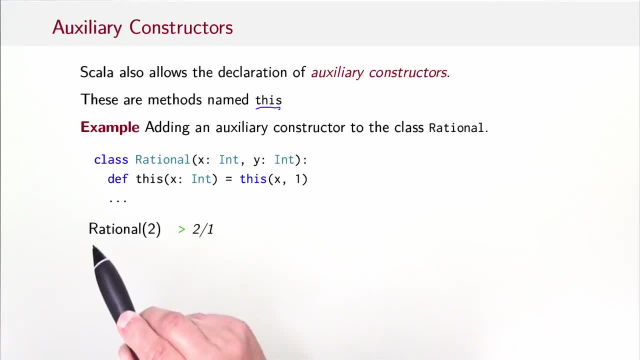 that takes a single argument. So we want to be able to write something like Rational of 2 and that should just give the number 2 over 1, so the integer number 2 expressed as a Rational. So we can do this by defining an auxiliary method. this: 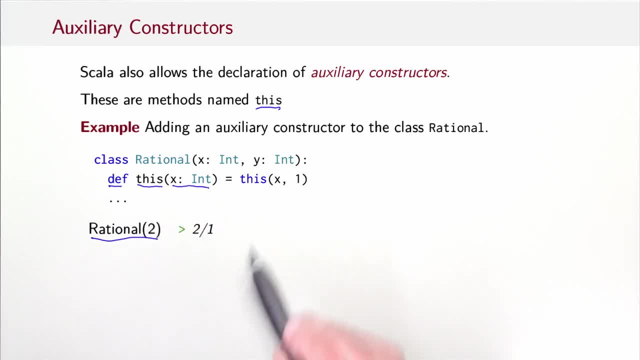 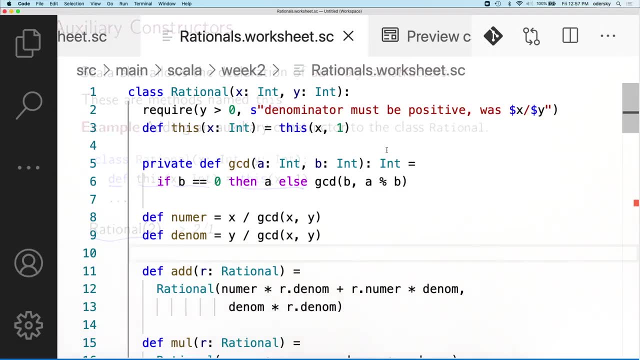 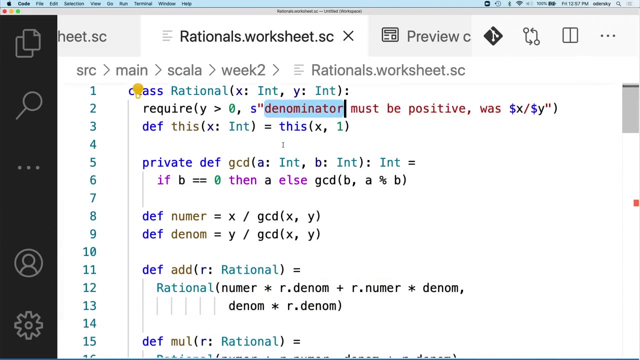 that takes the single integer, the numerator, and that creates a Rational with the numerator and 1 as the denominator. Now I've put everything we've covered so far in the worksheet with the definition of the class Rational. so we have the require, the secondary constructor, the. this 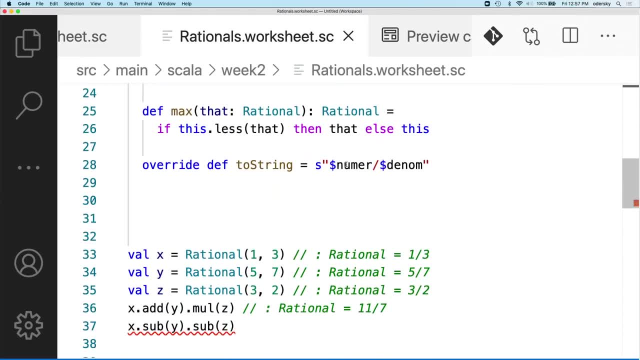 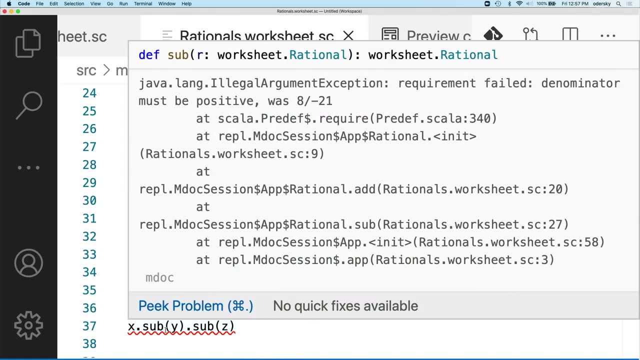 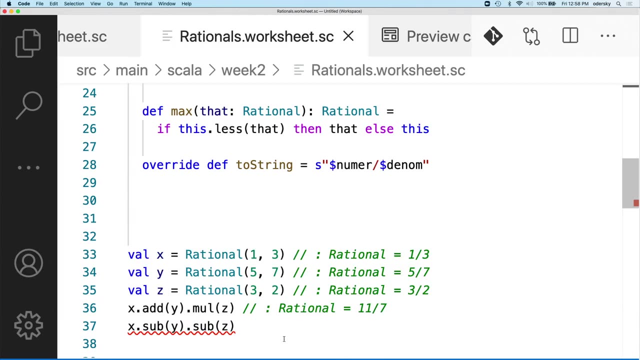 then the normalization with GCD, then all the methods and so on. So in the examples we see that something doesn't work. So what do we see? Well, it said denominator must be positive. but we got 8 divided by minus 21, so the denominator was negative. 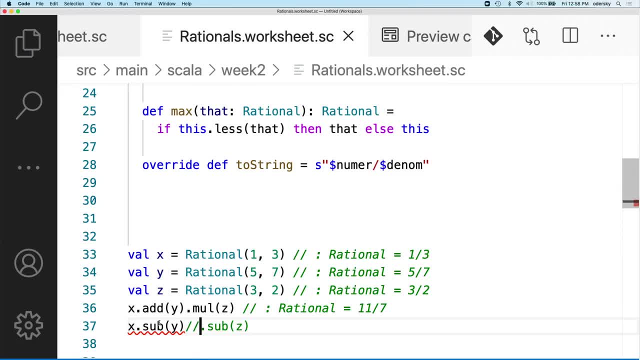 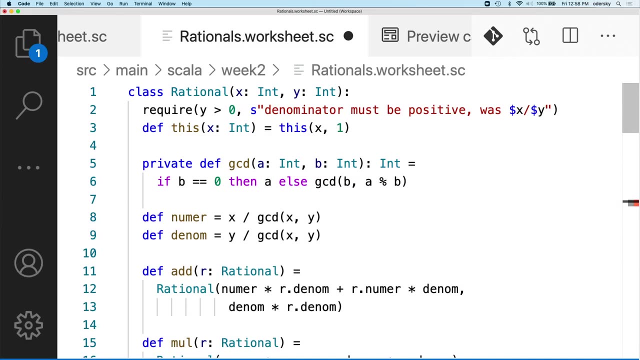 Where did it go wrong? So we can debug it a little bit and comment out the thing. so it was the first subtraction that is already the case, that went already wrong. So if we think about it, where could the problem be? In fact, it turns out the problem is in. 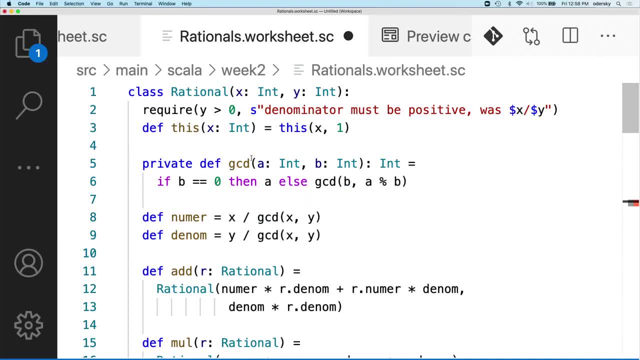 the definition of GCD. and it calls to GCD here, because the definition of GCD assumes that the two operands are both positive, whereas here the denominator, the Y, must be positive but the X can be negative. So the GCD with a negative number. 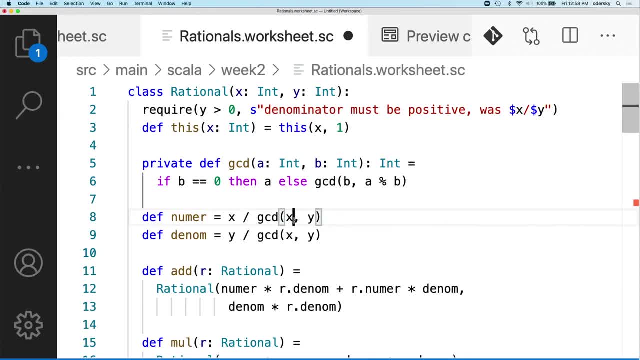 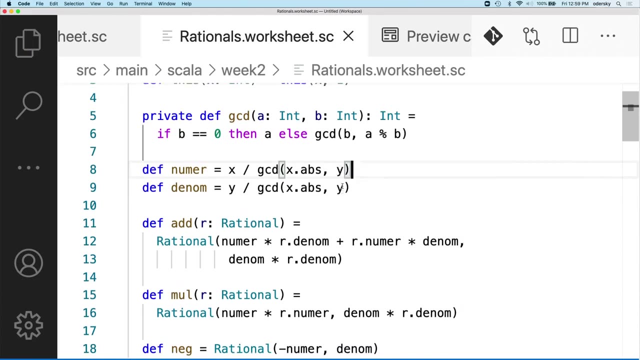 the way we've defined, it would come out as negative again, And to fix that we would have to define the absolute value of the X value. So that's in fact the greatest common divisor through which we have to divide. There's no need to take the absolute number value from the Y. 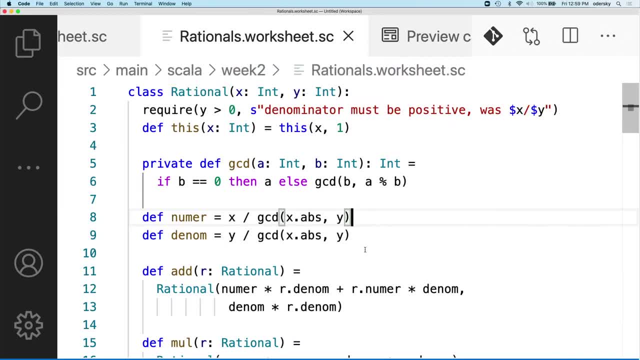 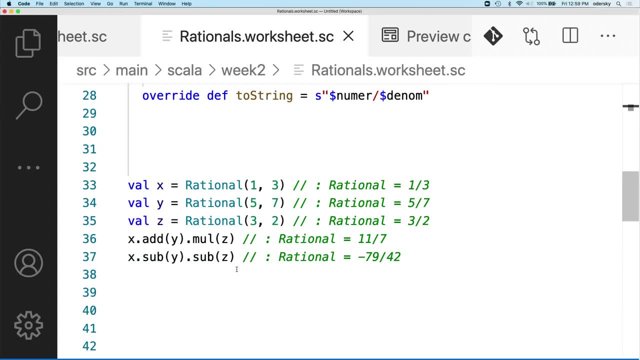 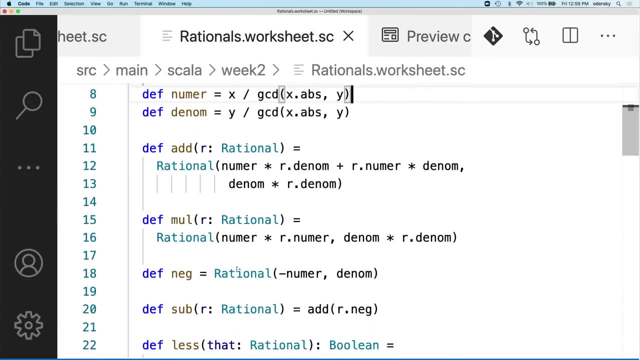 because the require here already indicates that Y must be positive. So with that change we have that the final expression evaluates correctly, without throwing an exception. Another thing you saw is that the class is getting quite long, So it's sometimes hard to see where it ends. 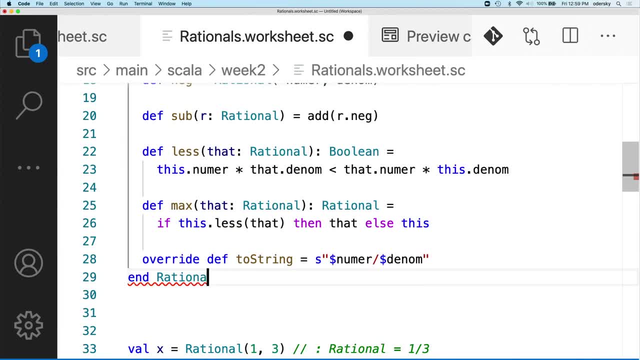 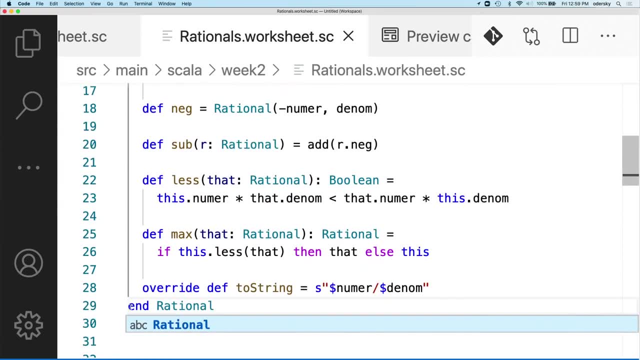 and to help here, there's a way to specify that. so in Scala you can write a so-called end marker which tells you what's the end of the class. If you get the column wrong like this, then you would get an error which says that the end marker is misaligned. 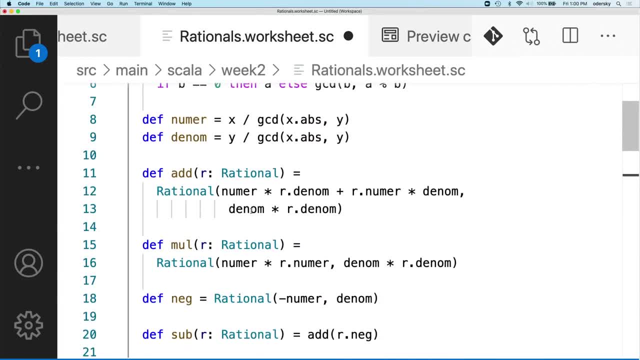 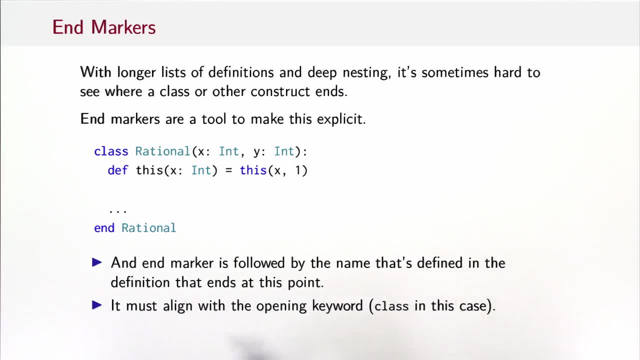 So the end marker has to start at exactly the same column as the class that it closes. So generally, an end marker is followed by the name that's defined in the definition. that ends at this point and it must align with the opening keyword. In this case, the end must be in the same column as the class. 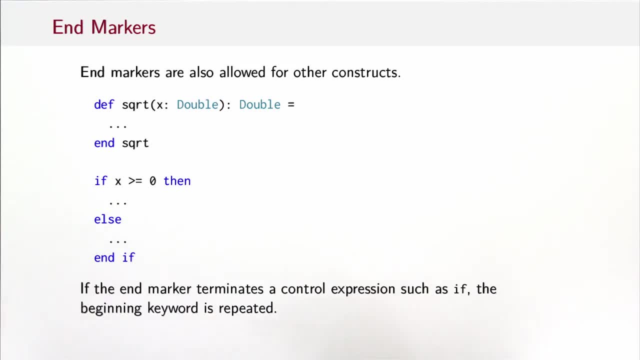 End markers can also be used for other constructs. For instance, they can be used to terminate a def or a val, like what you see here, to terminate a control construct like an if-then-else that spans several lines. If it's a control construct, that's terminated. 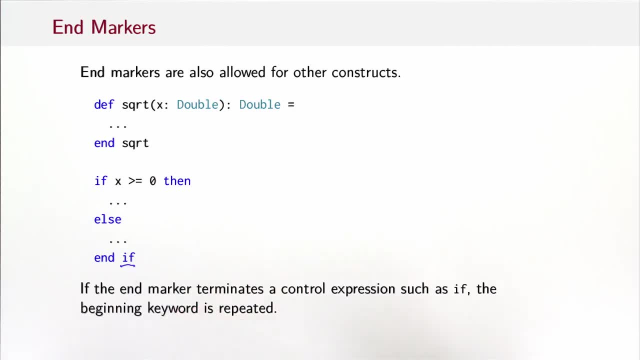 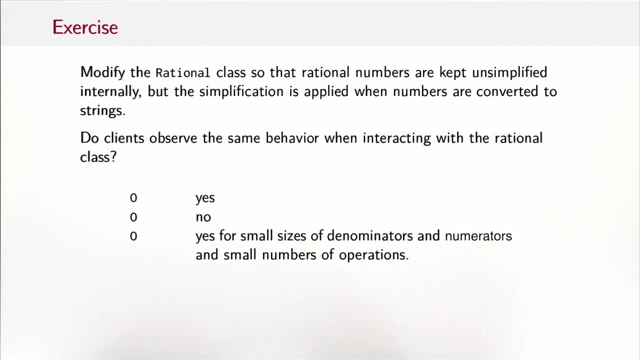 you follow the end by the name of the control construct instead of the name that's being defined, because of course, for control constructs there is no name that is defined. So here's an exercise for you: Modify the rational class so that rational numbers are kept unsimplified. so no GCD. 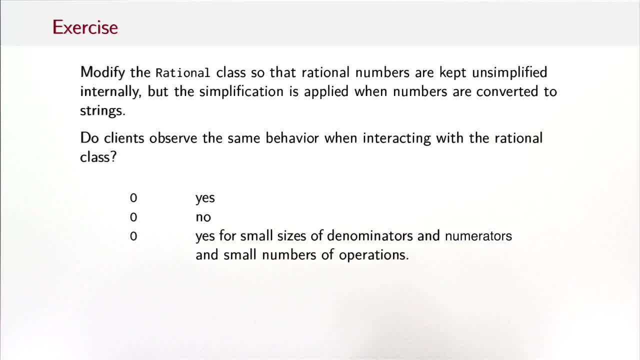 but the simplification is applied when numbers are converted to strings. Do clients observe the same behavior when interacting with the rational class? Yes, no. or the third choice is yes for small sizes of denominators and numerators and small number of operations. 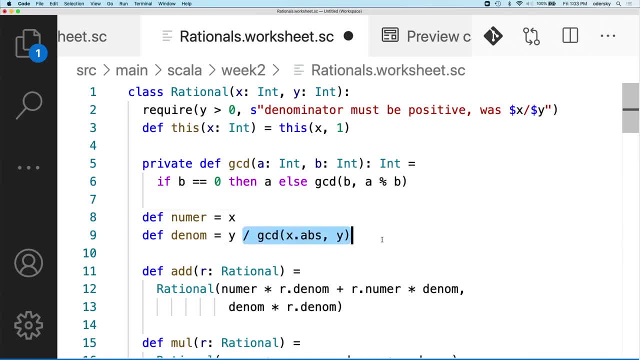 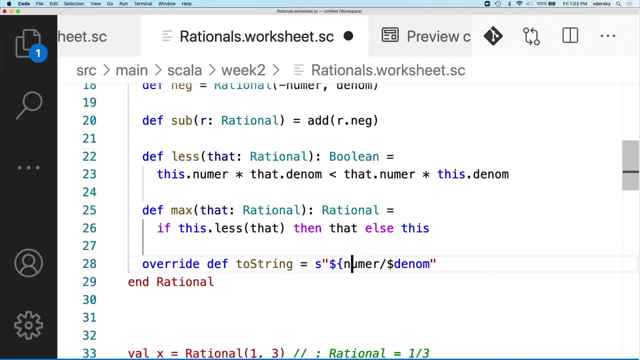 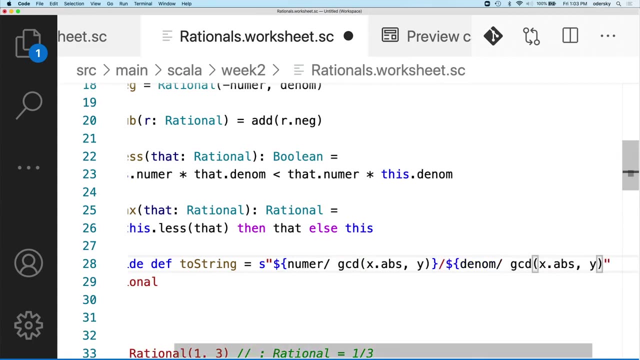 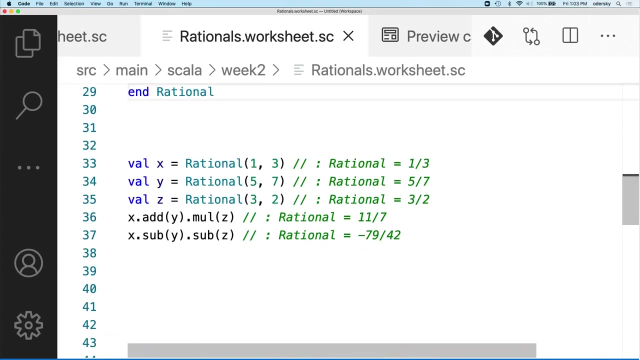 So let's see: We would delete the simplifications of the numerator and denominator- They're now unsimplified- and we would add the simplifications when they are printed. That's all we have to do Now. in this example, we see the same output. 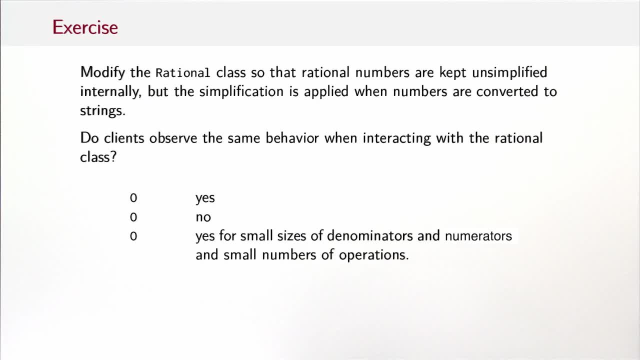 So the question is: is that always the case? Let's think a bit about it And I believe the fair answer is really 3. For small sizes of denominators and numerators, you wouldn't see a change as long as the number of operations 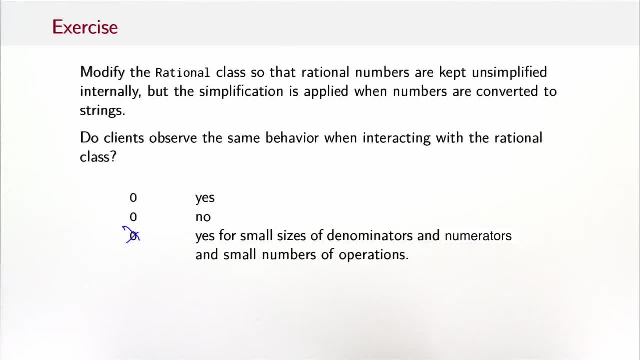 is small. Why would you see a change if denominators and numerators can get very large Because of the problem of overflow? If the rational numbers are not simplified, the denominators and numerators can get increasingly larger until they don't fit into the range. 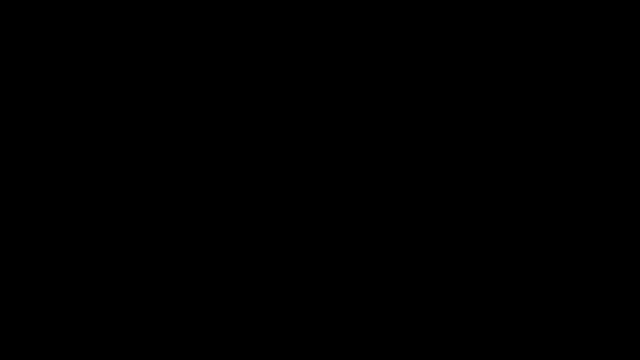 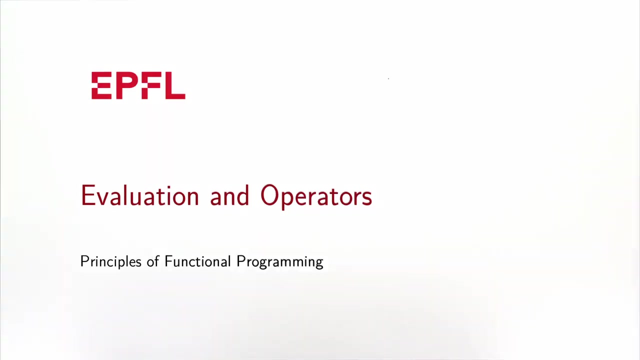 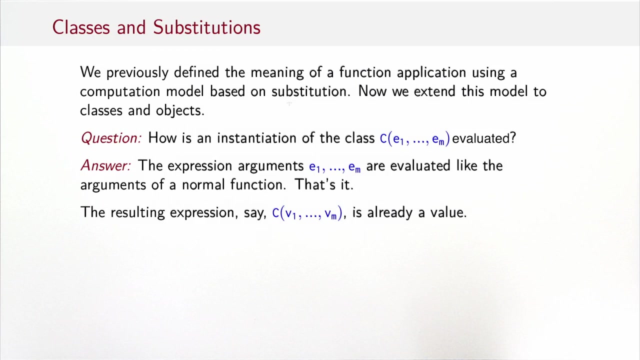 of an integer anymore. In this unit, we are going to look at how operations on objects evaluate and also we are going to learn some handy new syntax for defining operators. Previously, we defined the meaning of a function application using a computation model based on substitutions. 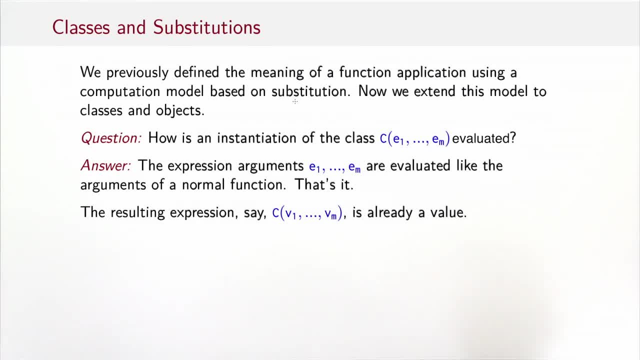 Now we extend this model to classes and objects. The first question is: if we have an instantiation of c to e1 to en, how is that evaluated? And the answer is: well, the class arguments e1 to em are evaluated just like the arguments of a normal function. 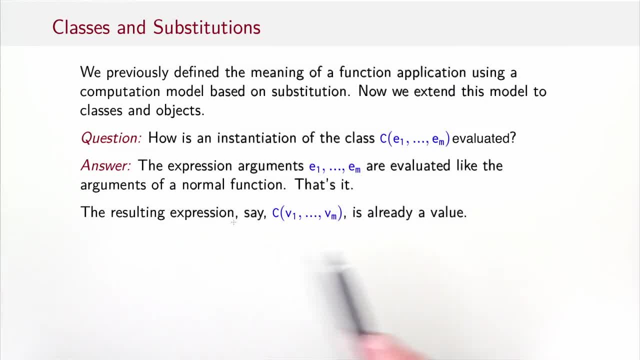 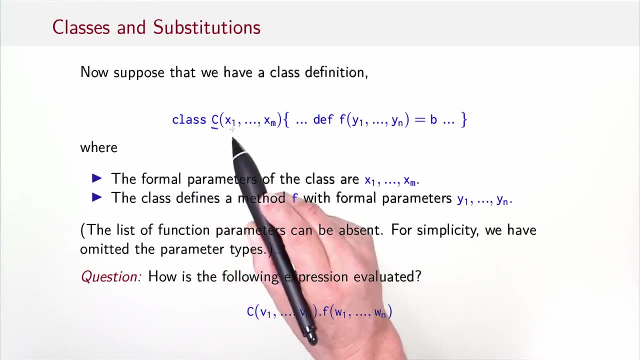 And that's it. The resulting expression is already a value. So if e1 to vm are values, then passing them to a class constructor c gives you another value. Now let's suppose we have a class definition of a class c which takes formal parameters x1 to xm. 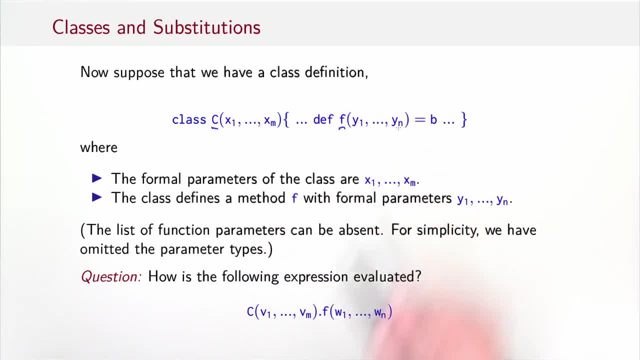 and it has a method f which takes another set of parameters, y1 to yn, and has a body b. For simplicity, we have omitted the types of the formal parameters because they are irrelevant for the discussion here. The question is: how is the following expression evaluated: 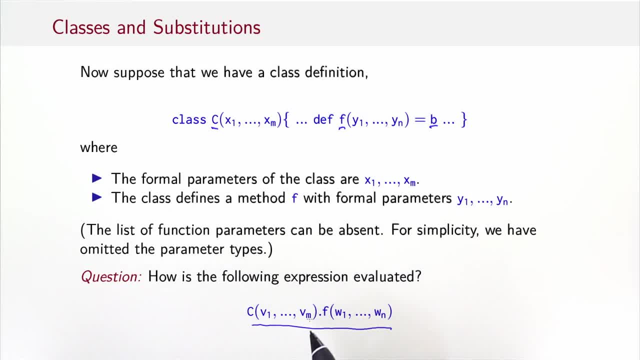 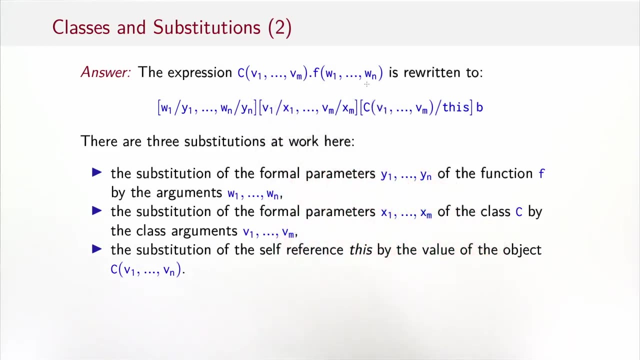 c applied to some values that are the class arguments. select f and then apply to some further values that are the method arguments. The answer is that we can rewrite that expression using substitutions, and in this case we actually need three substitutions. Let's analyze them one by one. 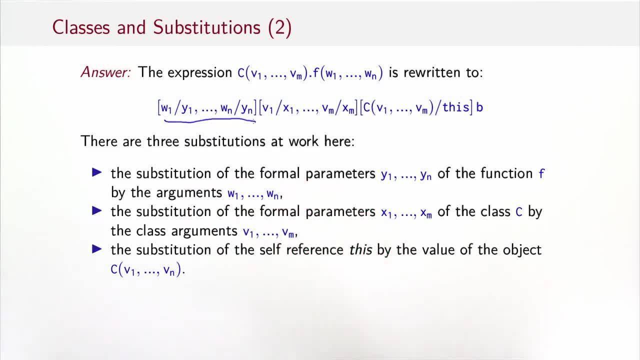 So the first substitution here passes the actual function arguments for the formal parameters of the function, as we do that for normal functions. The second substitution passes the class arguments v1 to vm for the class parameters x1 to xm, And the final substitution passes the class value. 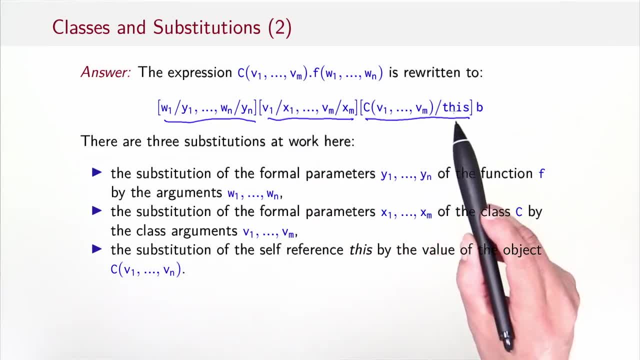 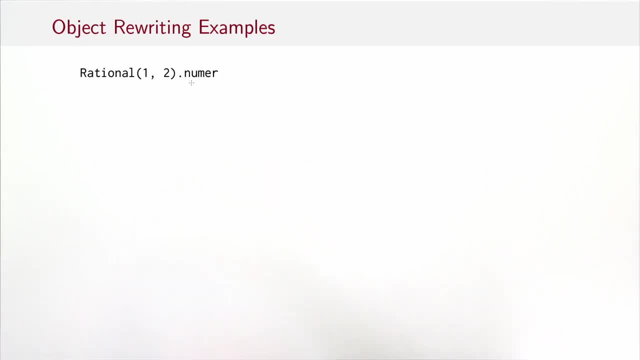 c1 to vm itself for any references of this in the body. So let's see that with some examples. Let's say we have rational 1,, 2 dot numer. So that would be, according to the definition, substitute 1 for the class argument x. 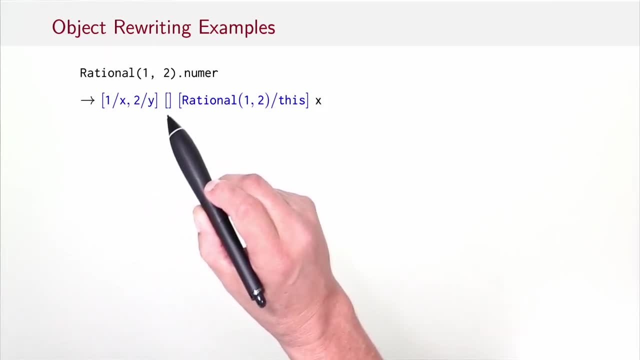 2 for the class argument y. there are no function arguments, so the second substitution is empty. And finally, substitute rational 1, 2 for this nx. So that gives simply 1, because x gets substituted by 1, as expected. So let's do. 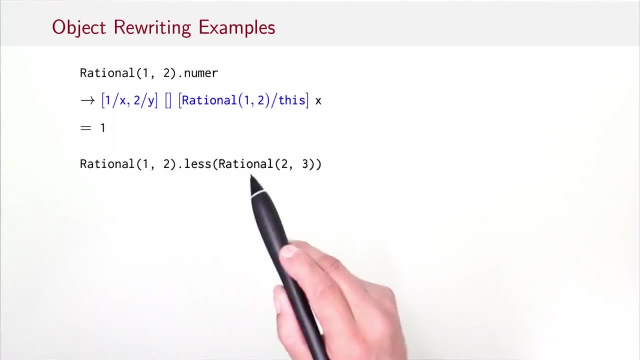 a more complex example. Let's say rational 1, 2 dot less rational 2, 3. What would that evaluate to According to the definition? we again pass 1 for x, 2 for y. then the argument of less is the rational. 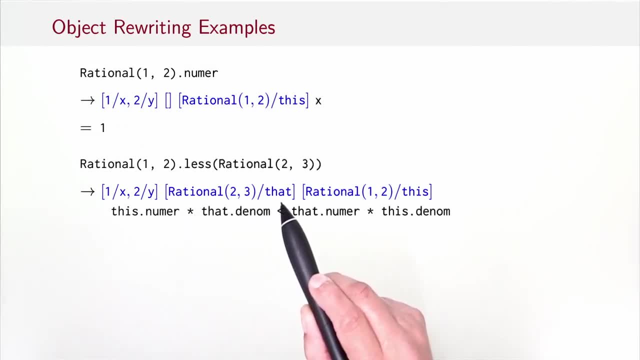 number 2, 3, so that gets passed for the formal parameter that, and the rational 1, 2 gets passed for this. And the body of less is that expression that you see here, this dot numer, that denom, less than that dot numer. 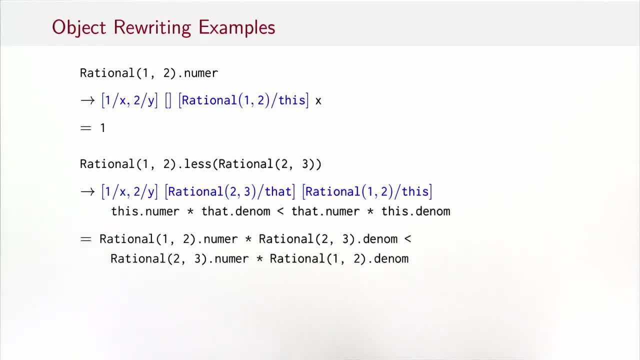 times this dot denom. So that then would substitute to rational 1, 2 dot numer times rational 2, 3 dot denom, less than rational 2, 3 dot numer times rational 1, 2 dot denom. And if we apply the 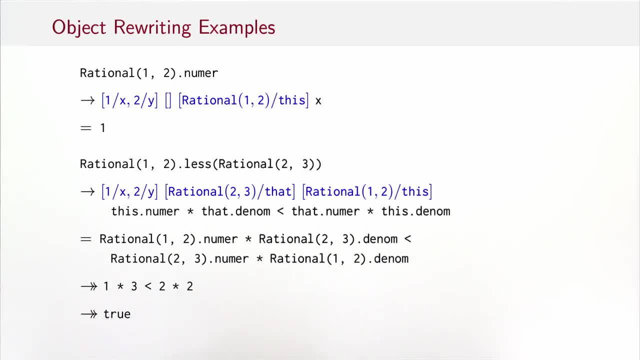 definitions of numer and denom. that would substitute to 1 times 3, less than 2 times 2, and then to true. So you see that calls of methods can be described very much like calls of normal functions, only that now we have not just a substitution. 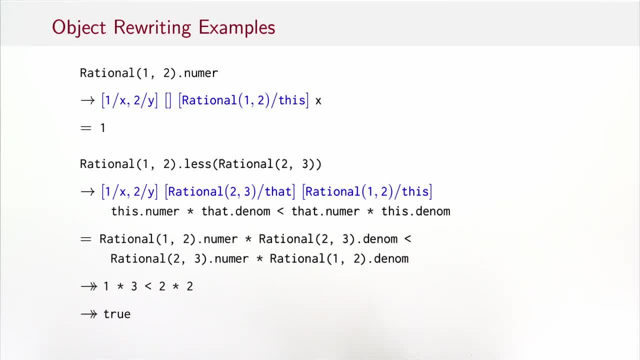 of actual arguments for formal parameters. we have a similar substitution for the class arguments and the class parameters and finally, we have the substitution of the left hand side from the dot that value here for the reference to this in the class. So here's a variant of what we've. 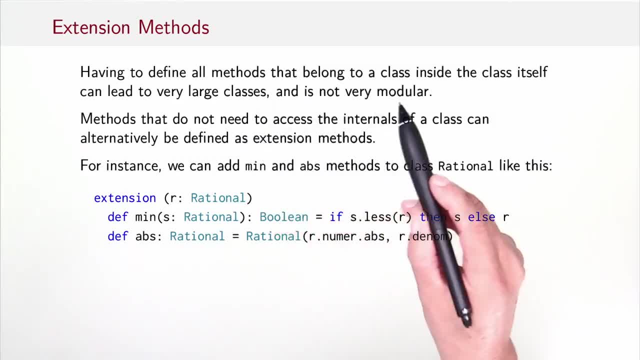 seen before. So far we defined all the methods of a class inside the class. That can lead to very large classes and it's not very modular. A lot of the methods we defined don't really need access to the internals of a class. They could have alternatively. 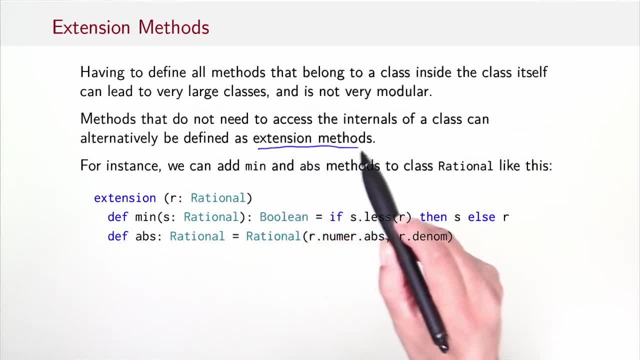 be defined as so called extended methods. For instance, we could ask further methods- call them min and abs- to class rational like this: So now we are outside class rational, but we define an extension of a rational number, r, and we add the two methods min, that takes another rational. 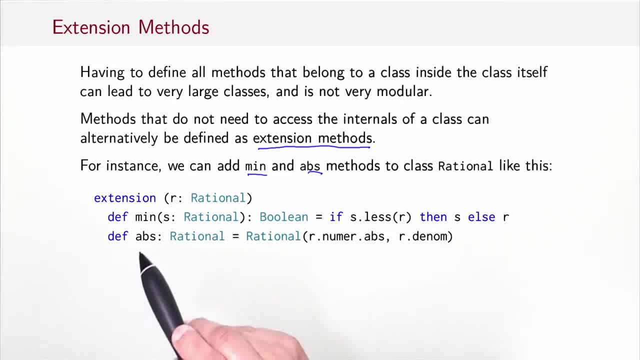 number with the usual definition and abs. that takes a rational number and gives you the absolute value of that rational number. The advantage of using extension instead of class methods is that you can define an extension anywhere. You can define it together with the class, but you can also define it. 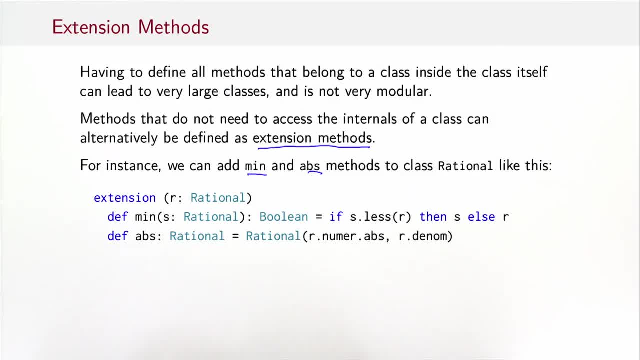 in different modules and there can be different people who can define different extensions of the same class without having to step over each other's feet, changing the same source code. Extensions of a class are visible if they are defined together with the class, or if they are visible. 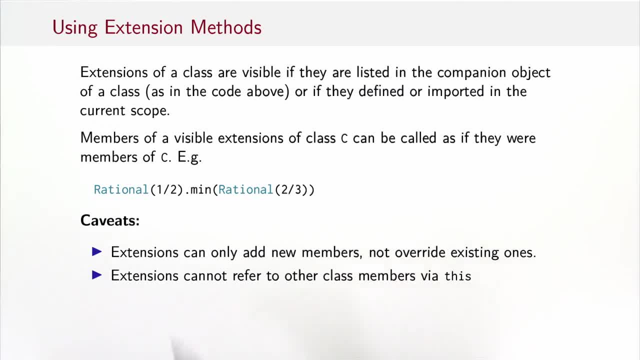 in the current scope, where they are defined or imported And members of an extension of a class C can be called as if they were normal methods of that class. So, for instance, you could write rational one, two, dot, min, rational two, three, no matter whether min was defined. 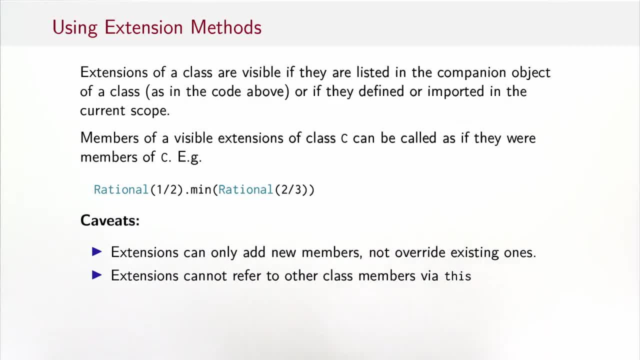 as a method of class, rational or as an extension of it. So the idea of an extension is that it adds new functionality to a class without changing existing functionality. That has two consequences. The first is that extensions can only add new members, new methods. 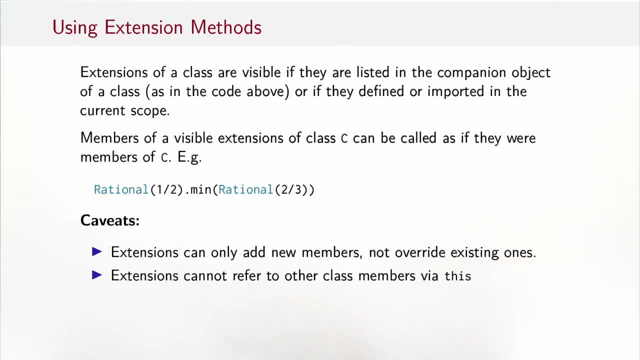 not override existing ones. And the second is that extensions cannot refer to the internals of a class or to other members of a class via this, because this is not available in the extension. You see the instance from the outside, not from the privileged access that can see this. 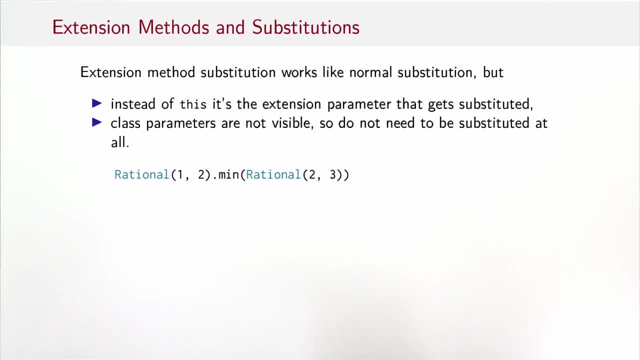 So if you look at the operations of extension methods using substitutions again, then we find that extension method substitution works basically like normal substitution, but instead of this it's now the extension parameter that gets substituted And furthermore, since class parameters are not visible, they don't need. 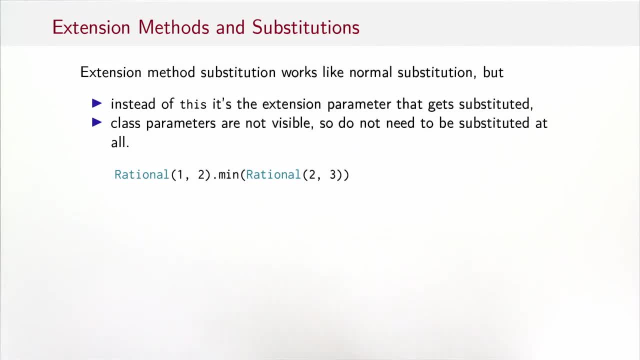 to get substituted at all. So we see here this example for the extension. So what happens here is that the value to the left of the dot replaces the extension parameter, that was r, and the argument rational two, three replaces the method parameter of min, that was s. 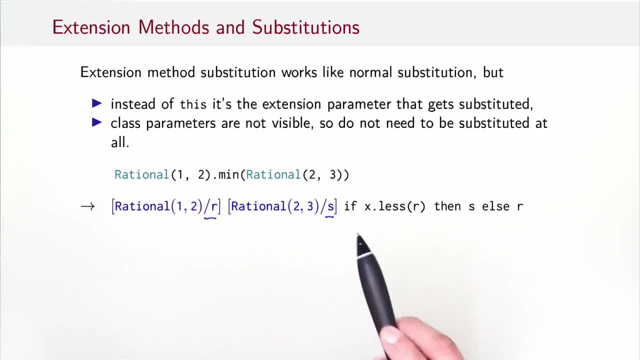 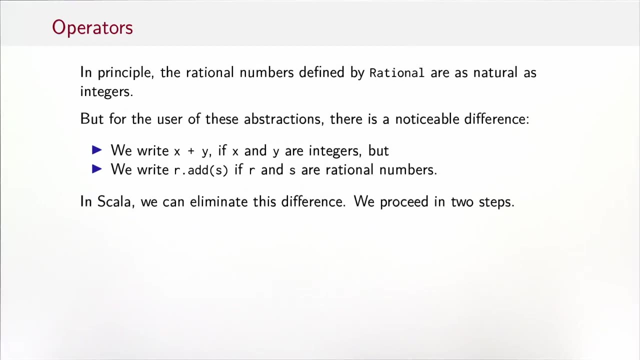 And under these replacements we replace the call with the body of min, which is this expression here. So if we perform these substitutions, we get what we would expect: this expression here. Here's a final tweak to make dealing with rational numbers more convenient. In principle, the rational numbers we've 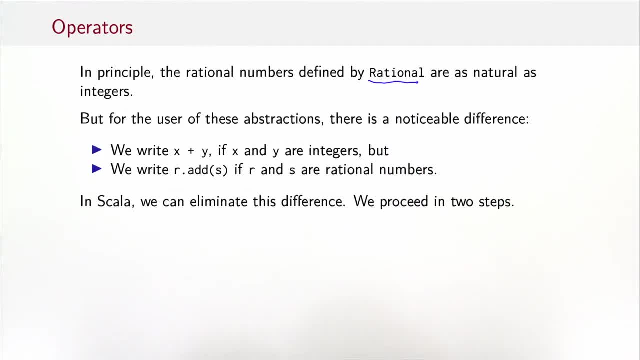 defined by our class, rational are as natural as integers, But for the users of these abstractions there's still a noticeable difference. For integers we would write x plus y, but for rational numbers so far we wrote r, dot, add s. so we used method syntax, And that's in a sense. 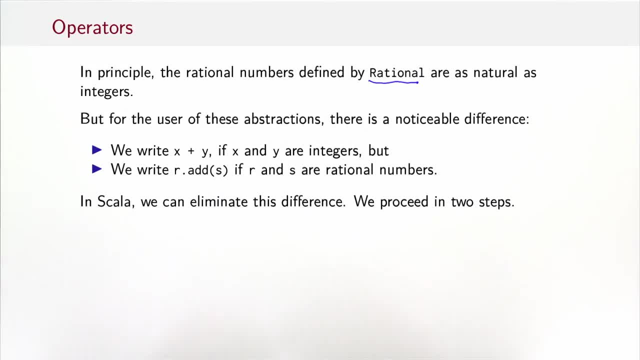 a shame. If rational numbers are as natural as integers, then we should be able to use the same natural and convenient notation for dealing with them. And in fact in Scala we can do that. We can eliminate the difference, and to do that we proceed in two steps. 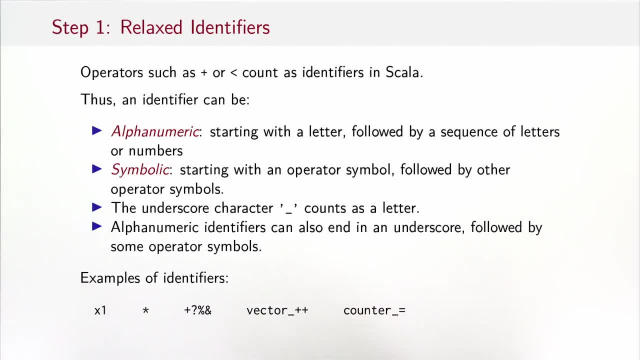 The first step is to relax the notion of what an identifier is. In fact, in Scala, an operator such as s or less counts as an identifier, So in general, an identifier can be alphanumeric: It starts with a letter, followed by a sequence of letters or digits. 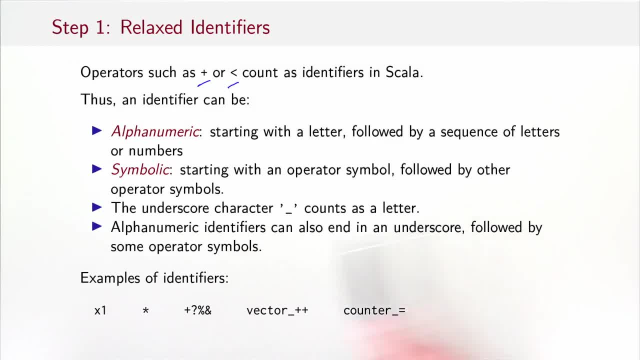 Or it can be symbolic: It starts with an operator symbol followed by other operator symbols. It's also possible to combine the two. You can have an alphanumeric identifier that is followed by an underscore and then followed by some operator symbols. So all these would be valid. 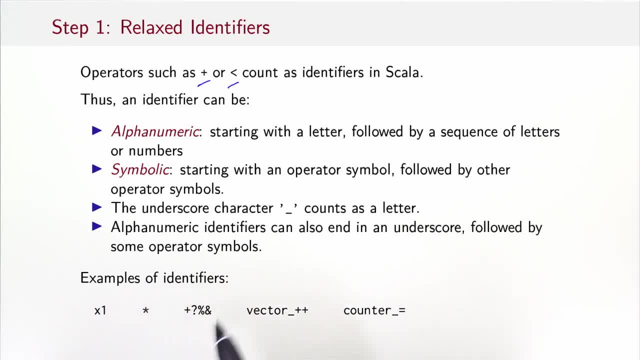 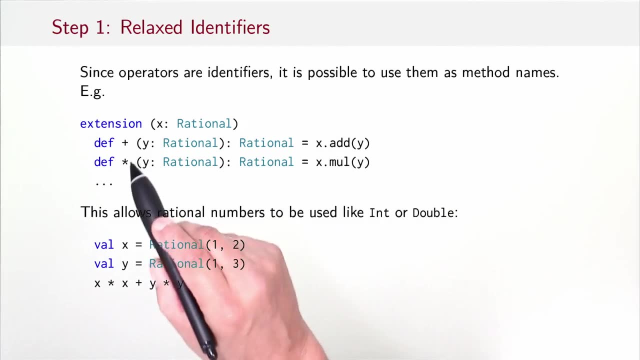 identifiers in Scala x1: asterisk and this funny thing here- Probably not recommended to use that Vector underscore plus plus or counter underscore equals. Since operators are identifiers, it's possible to use them as method names. Here we use plus and times as method. 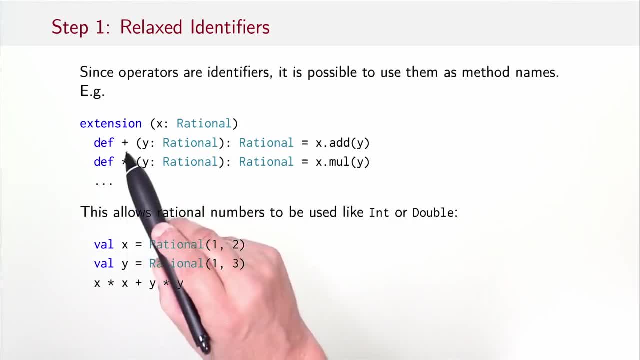 names for an extension of class rational. So plus is just an alias of add and times is an alias of multiply. You could also use plus and times as methods in class rational itself. So that's your choice. Here we have made the choice to use the. 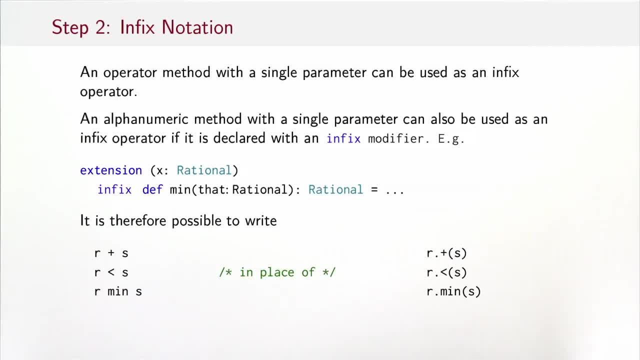 operator names, preferably as extensions. The second step is that an operator method with a single parameter can be used as an infix operator. So, for instance, you can write r plus s and what it means is you call the method plus on the left hand value r, with. 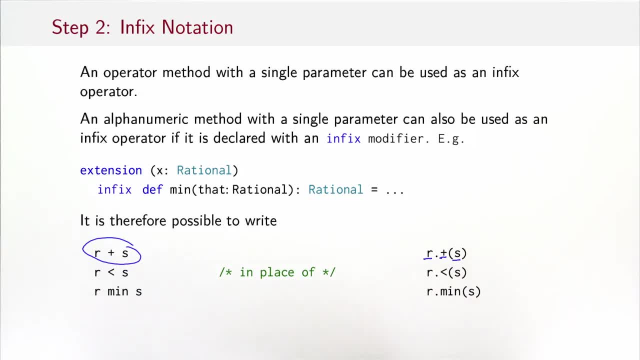 the argument s. The two are completely interchangeable. Likewise, r less than s is just a shorthand syntax for r dot method call less than with the argument s. So that explains what operators are. They're just essentially a more convenient notation for method calls. 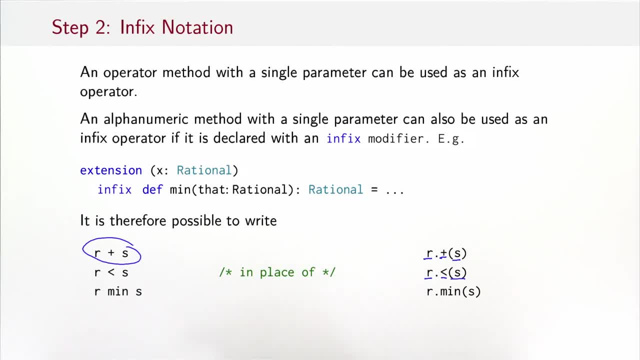 We can use the same trick for alphanumeric methods. So we might want to write, for instance, r min s with infix operator syntax instead of r dot min s. If we want to do that, then we have to declare the infix operator with an infix modifier. So here: 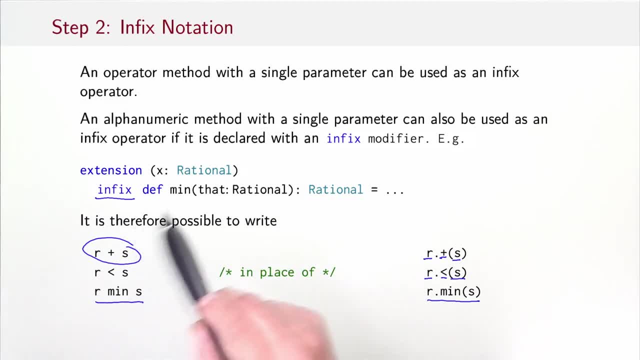 to be able to use min like that. you should define min with this infix modifier as an extension of class rational and that means it's usable like that. The reason for demanding an explicit modifier is that that enforces a certain uniformity between usages. So 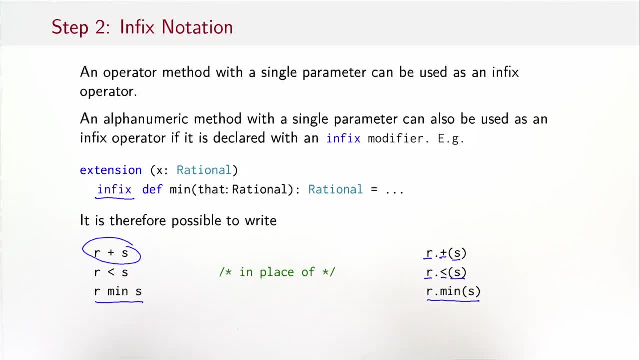 we do not want users to essentially freely mix infix and method syntax, so it is the designer of an abstraction and a method that decides whether the method should be called infix, in which case it gets an infix modifier, or whether it should be called as a normal method call, which is: 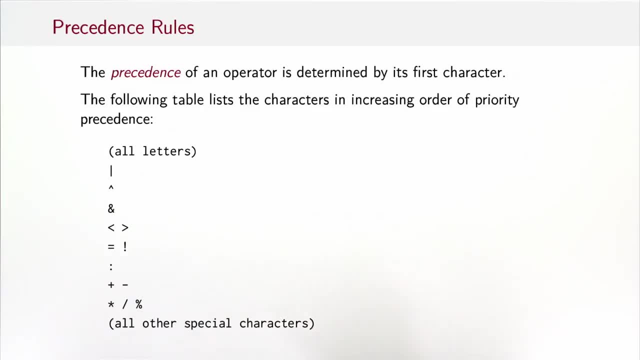 the more common case. So once you have operators you need to worry about precedence. For instance, if you have 1 plus 2 times 3. so how is that parsed? Where do the parentheses go? What Scala does here? it has a fixed order of precedence. 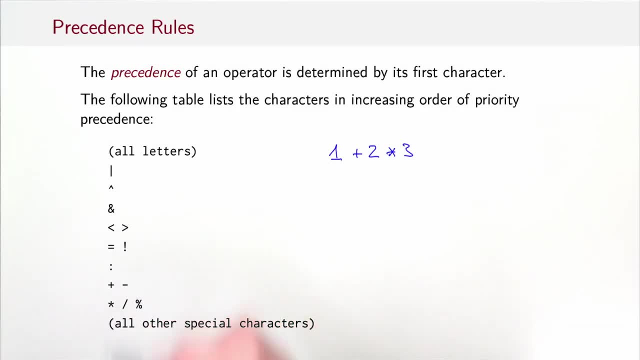 that depends on the first character of the operator. So the highest precedence is times, divide and modulo, followed by plus or minus, followed by a colon, equals, bang, less than greater and up arrow bar, and then the lowest precedence are all letters. so min would have a lower precedence than any operator. 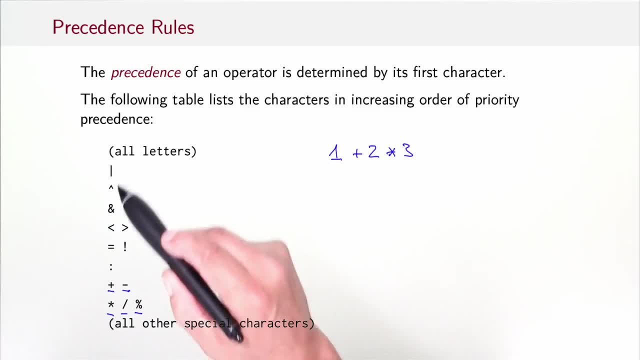 and the highest precedence are all special characters that are not in this list. You will notice that from here, this is actually the same precedence that operators in Java would have. of course, in Java you have only a fixed set of operators, but their precedence is exactly in that order. 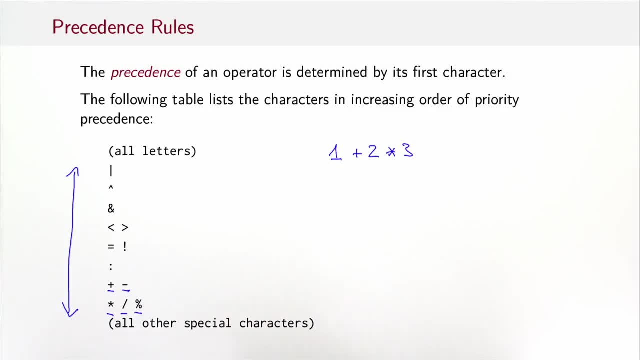 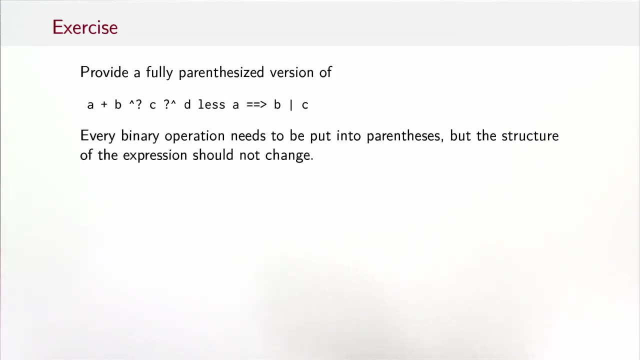 So Scala reuses that notion and generalizes it by allowing you to define your own operators that are not only in this set, but can also use other special characters or be followed with other operator symbols. So here is an exercise for you. We provide a fully parenthesized 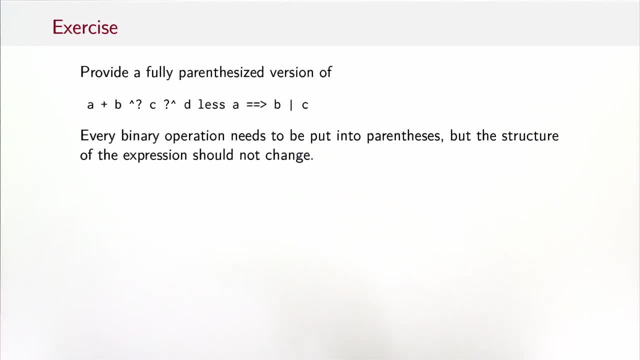 version of this expression. here Every binary operation needs to be put into parenthesis without changing the structure of the expression. So the conceptual structure of the expression should be the same with or without parenthesis. So let's see how would we go about this. Let's go. 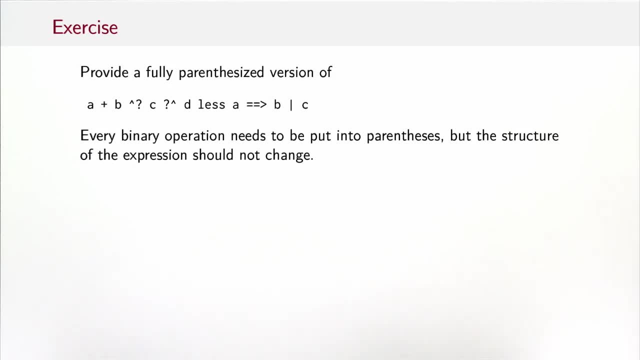 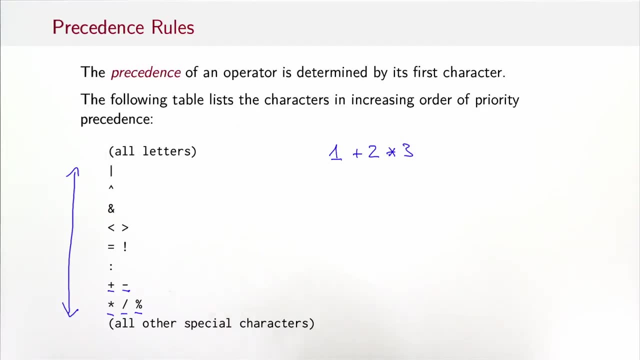 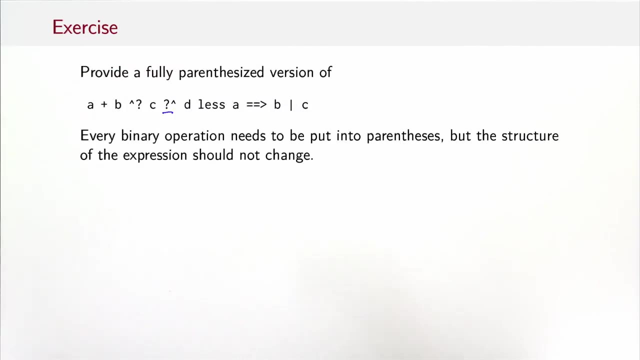 from highest to lowest precedence. Which of these operators has the highest precedence? It's this one here because it starts with a question mark which was not in our list of operators. So all our other special characters have the highest precedence. Question mark is one of those, So that's. 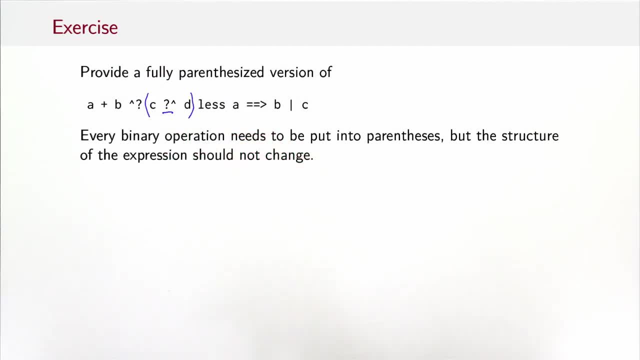 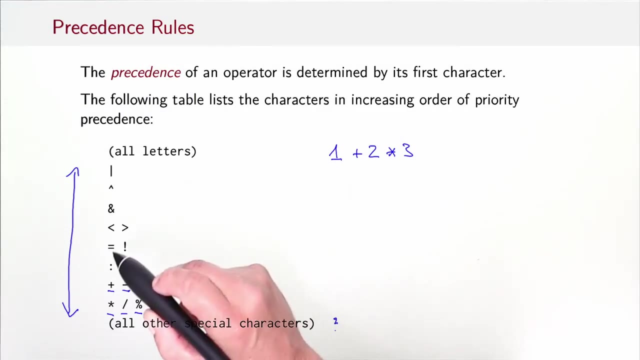 the highest precedence. We put the parenthesis like this: The next highest then would be the plus operation here, So plus. the parenthesis would go like this: The next highest operator is the equals. here That follows up after the plus in our list of expressions. 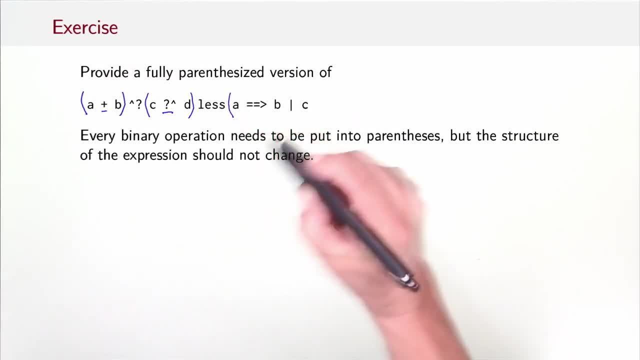 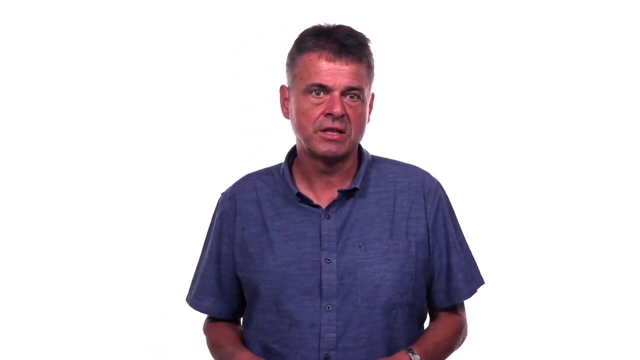 So that would be this expression here. We would do the parenthesis like this: That one is followed by the up arrow And that one is followed by the bar, And finally, less is the operator that remains with the lowest precedence. Over the last sessions, you've. 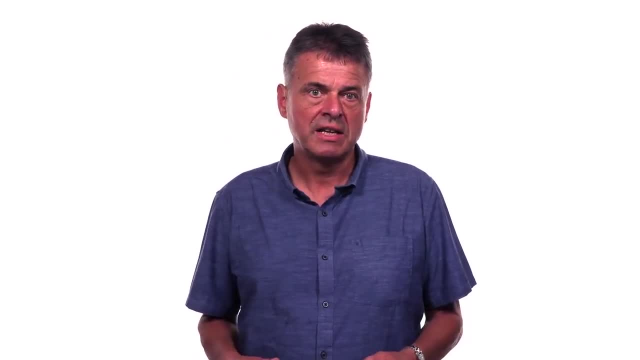 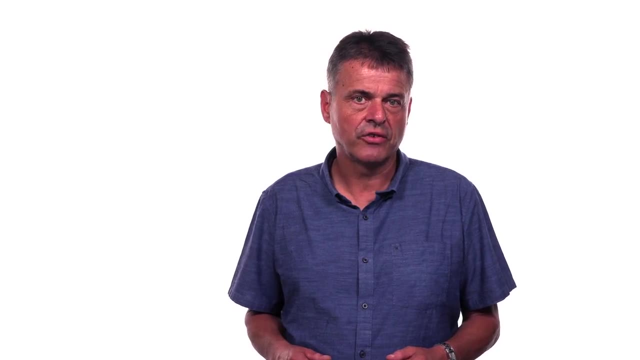 learned about objects and methods. So far, these are all instances of a single class. This is going to change in this session. We are going to introduce hierarchies of classes that extend each other. Once we have class hierarchies, an important 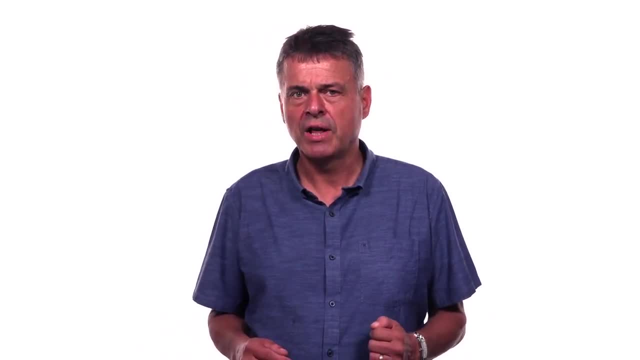 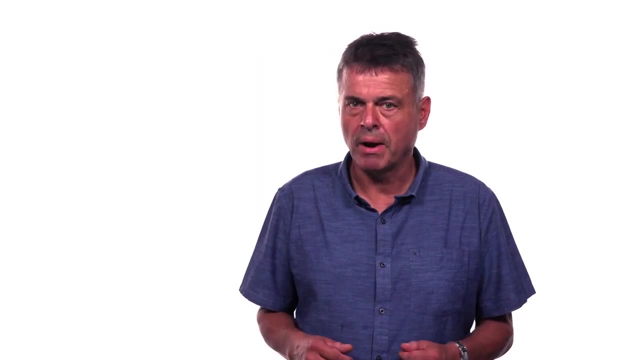 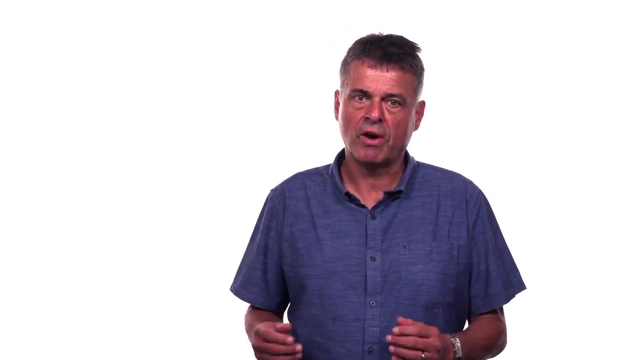 aspect is the model of evaluation. Now, the actual method might depend on the runtime type of the receiver of that method. This concept is called dynamic binding. It's one of the key aspects of object oriented programming. You're going to find out how our model of term rewriting 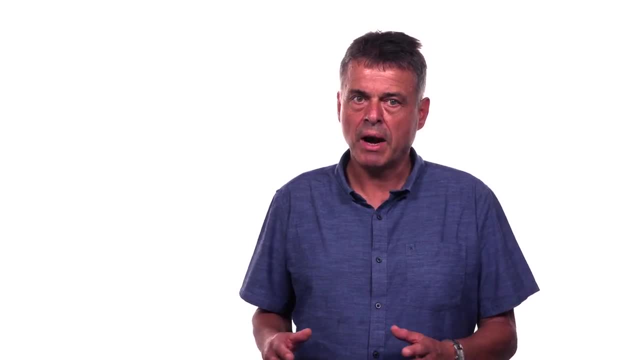 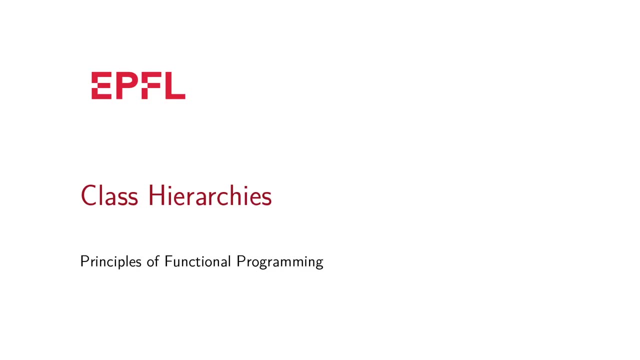 already supports this concept, So dynamic binding and term rewriting go very naturally together. In the last units you have seen a data type rational described by a single class, But there are also situations where it's natural to describe what's conceptually a data type. 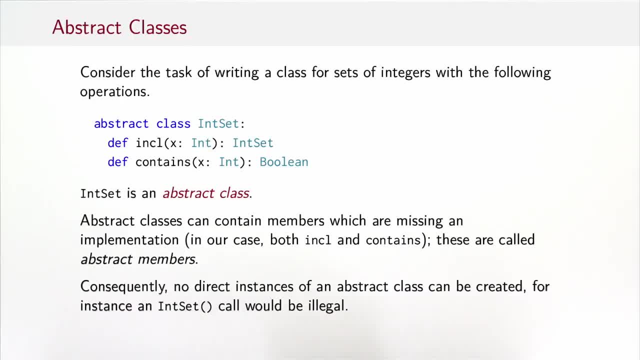 by a hierarchy of several classes. For instance, consider the task of writing a class for sets of integers with the following operations: include and contains. So include: takes an integer and returns a set that contains the previous set plus that integer that got added and contains. asks whether a given integer 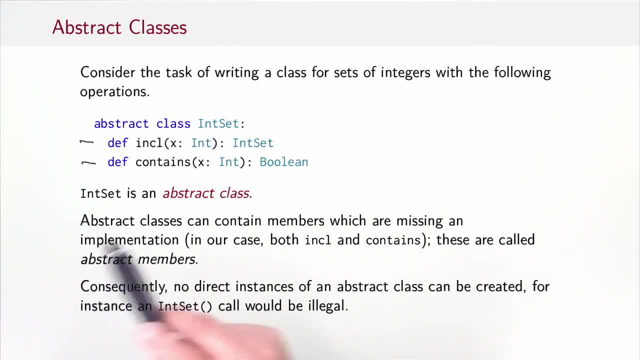 is in the set and returns a boolean. Int set is an abstract class, which is made clear here with this modifier. Abstract classes can contain members which are missing an implementation. In our case, both include and contains are not implemented. These members that are not implemented. 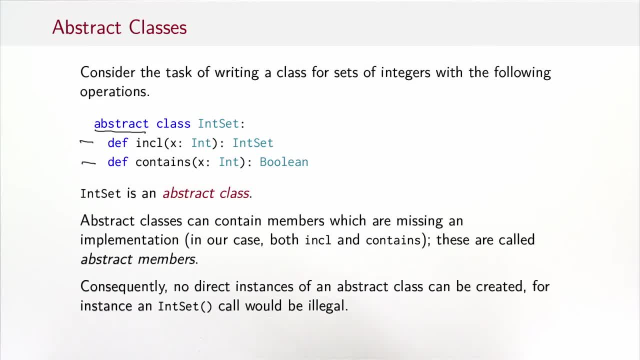 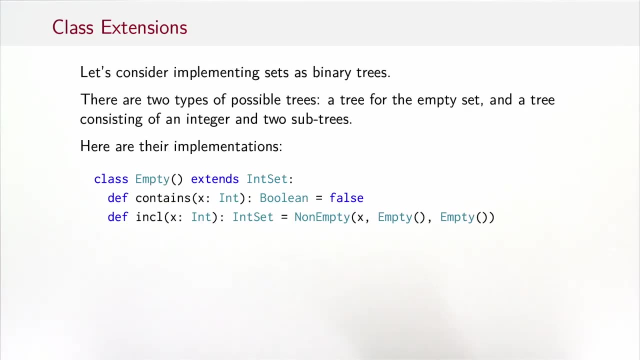 are called abstract members, Because abstract classes can contain abstract members that are not implemented. it follows that we cannot create instances of abstract classes because they would miss implementations. So a call like int set would be illegal. Let's consider implementing sets as binary trees. 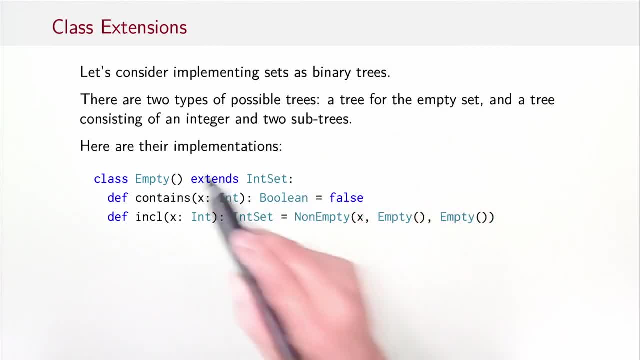 There are two types of possible trees: A tree for the empty set and a tree consisting of an integer and two subtrees. For instance, the set 1,, 2,, 4, 5 could lead to the following tree. It could have. 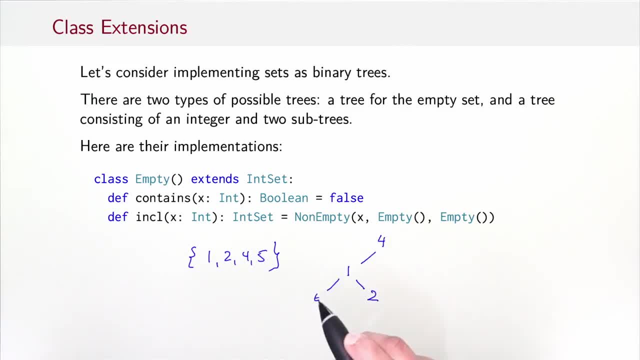 let's say a 4 at the top, then a 2 and a 1 at the left, and there would be empty 5 and there would be empty and the 2 has again two empty subtrees. So that's one possible representation. We start. 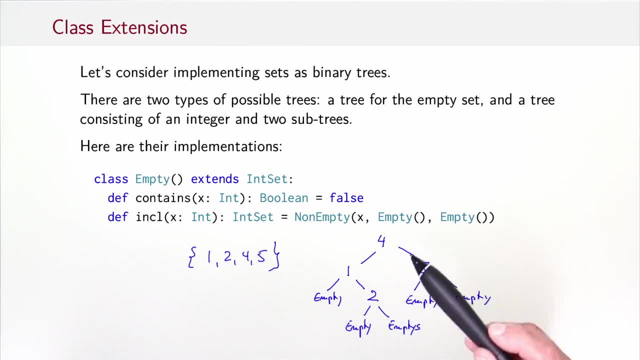 with one of the numbers 4, and then we notice that on the left subtree there are all the numbers which are smaller than the root number and on the right subtree there are all the numbers that are larger. So that's an invariant that we want to keep for the sets because it makes 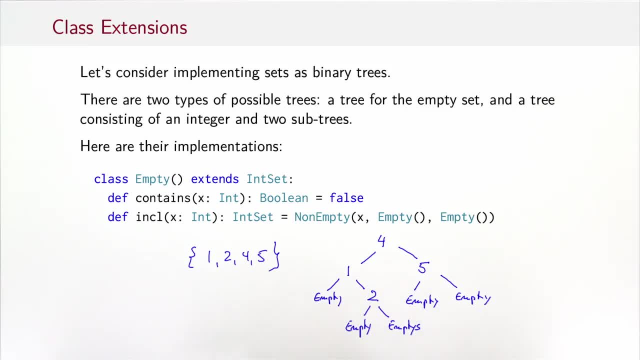 it efficient to both query with the contains method and add new members with the include method. So let's look at the implementations of the empty set and the non-empty set. The empty set you see here, For it, the contains method is always false. 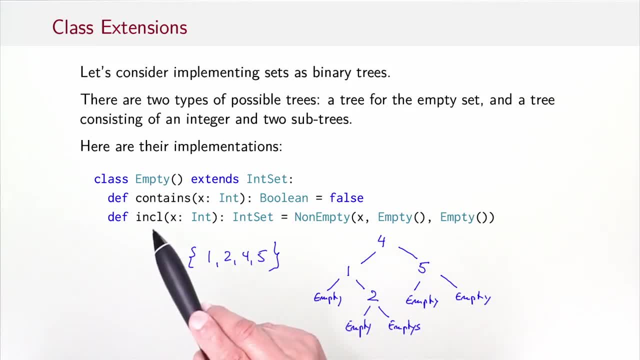 The empty set doesn't contain an element and the include method would create a non-empty set with the included element and two empty subtrees. So if we start with the empty set and we include 2, then we would get the tree that you see here: 2, empty, empty. 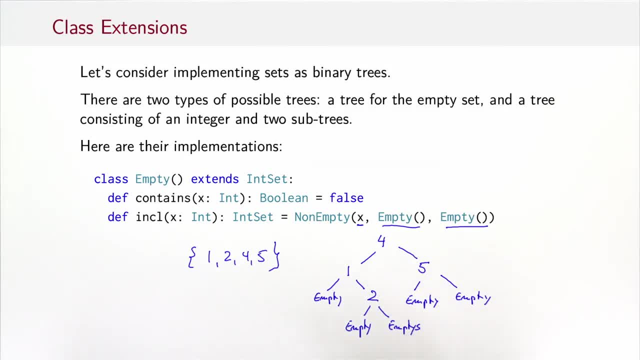 Empty sets are a special case of an inset. They are one of the possible implementations and that we made clear with this extends clause. We say the class empty extends inset, which means that it conforms to the interface of inset. It implements all the methods that are defined. 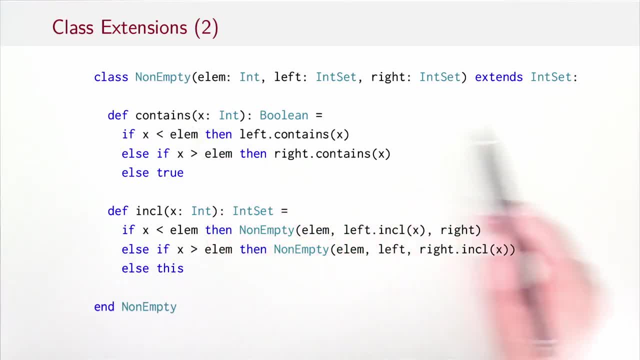 in inset. So now let's look at the non-empty set. It's another extension of inset. It takes an element as the first parameter and 2 insets as the left and the right subtree. Now let's look at the method implementations. Let's take contains first. 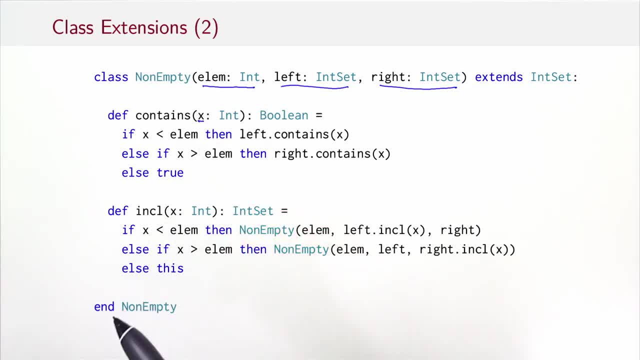 So to ask whether the set contains an element x, we ask whether the element x is smaller, larger or equal to the root element. If it's smaller, then we know that we have to look in the left subtree. If it's larger, we look in the right subtree. 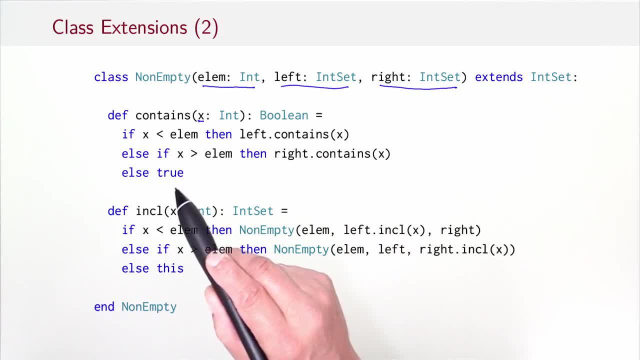 and if it's equal, then yes, the set contains the element and we return true. What about include? So include is similar to contains in that we also ask whether the included element is smaller, larger or equal to the root element: lm. If it's smaller. 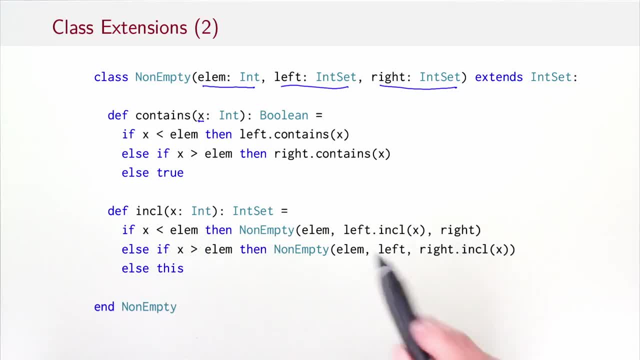 then we insert it in the left subtree, But this insertion- remember, we are in a functional language, so this insertion- would return a new tree, It wouldn't change anything, and that means that that new tree would have in turn to be wrapped with a tree. 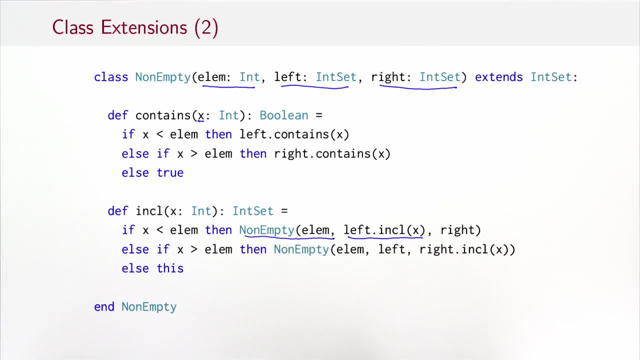 that adds the element and the right subtree. If the x is greater than the element, then we go analogously on the right element, So we include in the right subtree and we wrap with element left, and if it's the same as the element x, then there's nothing. 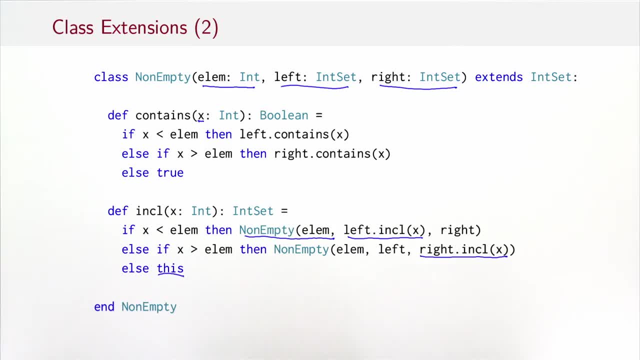 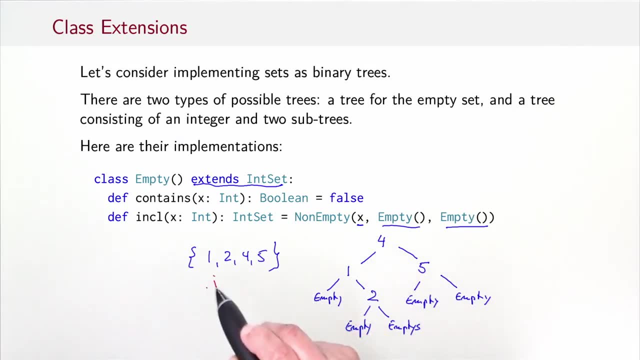 to do. The element is already in the set and we can return the set itself. So let's look at the operation on include with this set that we have formed here. Let's say we want to include the element 3 in the set. How would 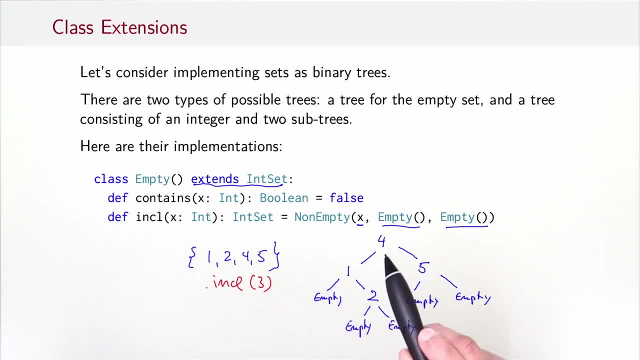 we go about. So we would ask: is 3 greater or smaller, or equal to 4?? Well, smaller. we go to the left subtree: It's greater than 1. so we go to the right subtree: It's greater than 2. so we go on the right. 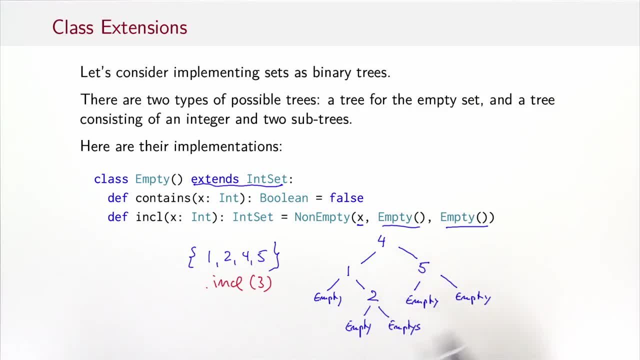 subtree. Now we have an empty tree, and empty tree include would then give us 3 empty empty as the new subtree. So now we wrap with 2 and the empty set. Now we wrap with 1 and its left empty set and finally we wrap. 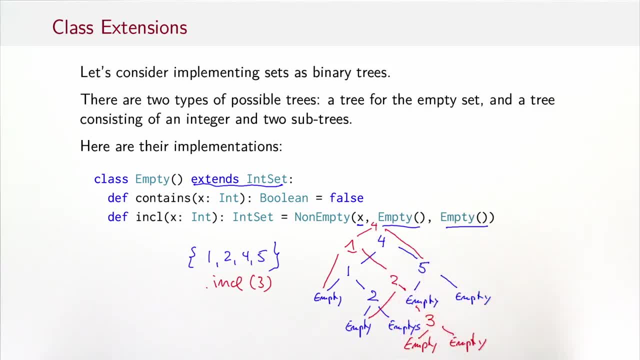 with 4 and its right tree. So we form the new tree. We left the blue tree alone. We form the new overlay tree, which is the red tree that now contains 3, as well as the elements that are in the blue tree that are reachable through the blue tree. 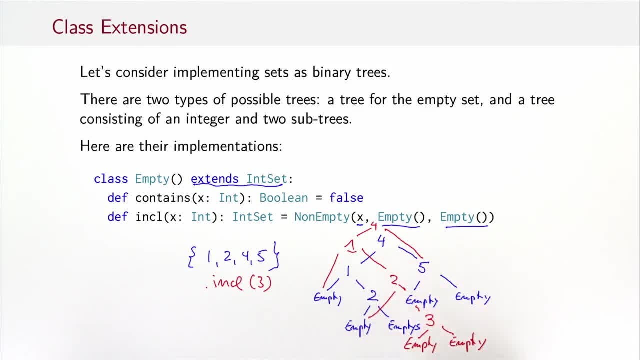 At the same time, the red tree doesn't completely copy the blue tree. It contains some elements that are left untouched, For instance, this subtree here That's now a part of the blue tree and it's a part of the red tree. So this idea that 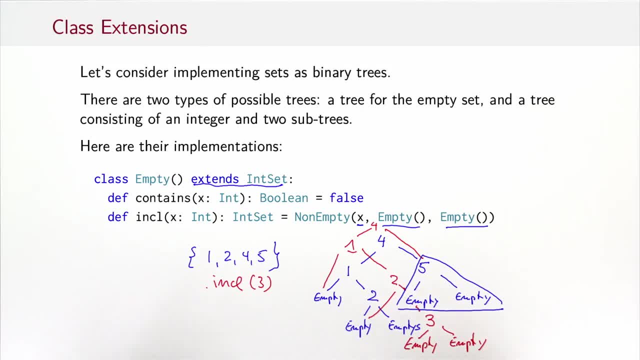 we can create new data structures from old ones without changing the old ones incrementally is called persistent data structures, Because the old one persists. we just create new ones out of the old ones, And it's one of the standard techniques in functional programming. Some more terminology. 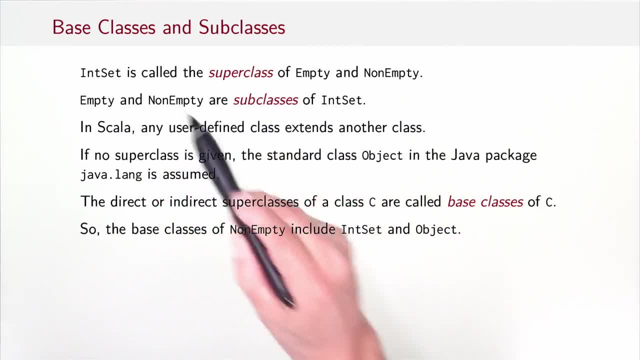 IntSet is called a superclass of empty and non-empty, and empty and non-empty are subclasses of IntSet. In Scala, any user defined class extends another class. If no superclass is given, the standard class object that's defined in the Java package- java-lang- is assumed. 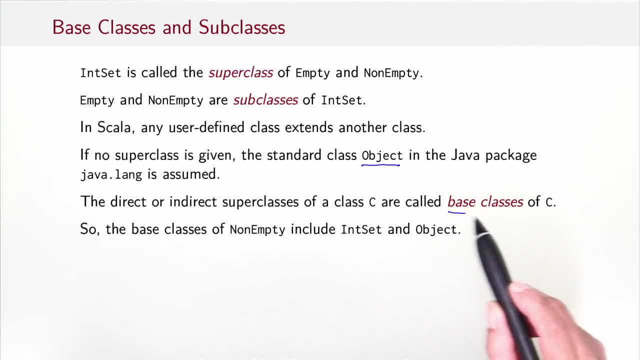 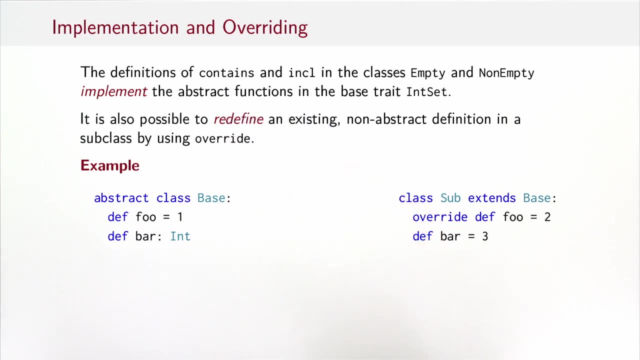 The direct or indirect superclasses of C are called the base classes of C. So the base classes of non-empty would be first IntSet and then object. We've seen that there are overall three deaths for contains and incle. One pair was abstract. 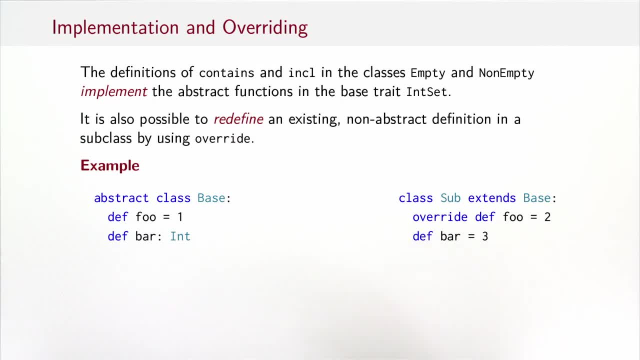 that was in the class IntSet where we have left out the implementations. And then there were two implementations, one for in class empty and the other in class non-empty. In that case we say that the definitions of contains and incle in empty and non-empty. 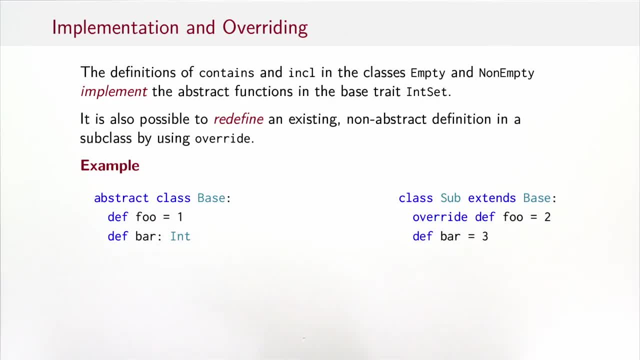 implement the abstract functions in the base trait IntSet. It's also possible to redefine an existing non-abstract definition in a subclass by using override. So if you have, say, a class base with a concrete method foo and an abstract method bar, then you can define. 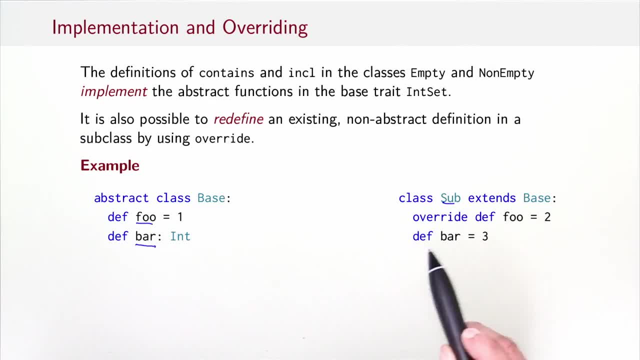 a subclass that extends base and you can just implement bar like this. But if you want to change, if you want to reimplement foo to be two here, then you need the override, So you can't just write def foo, that would give an error. 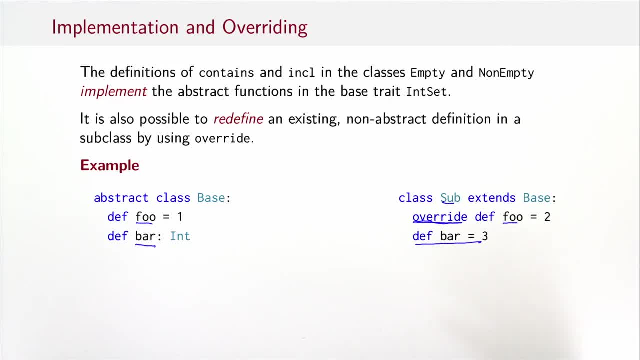 The reason why you're forced to do that is that the compiler wants to make sure you don't have an accidental collision where you just define a method, think it's a new method, but that method accidentally replaces a method in the subclass. So override is essentially an. 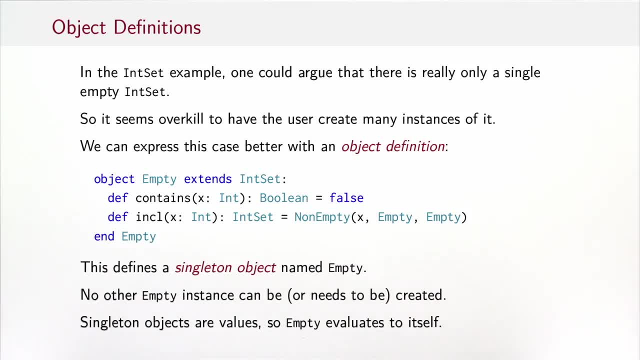 opt-in marker that says that's what I intend. So in the IntSet example one could argue that there's really only a single empty IntSet. It makes sense to have many instances of non-empty IntSets, but all empty IntSets really are alike, So it seems overkill. 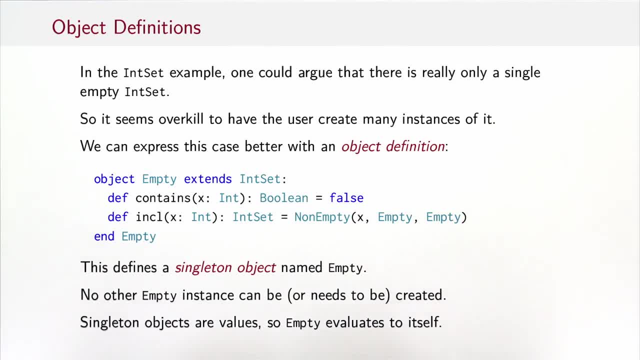 that the user needs to create many instances for the empty IntSet, And in fact we can express this case better with an object definition. An object definition would look like this object empty extends IntSet, and then come the two implementations of the method and then comes the. 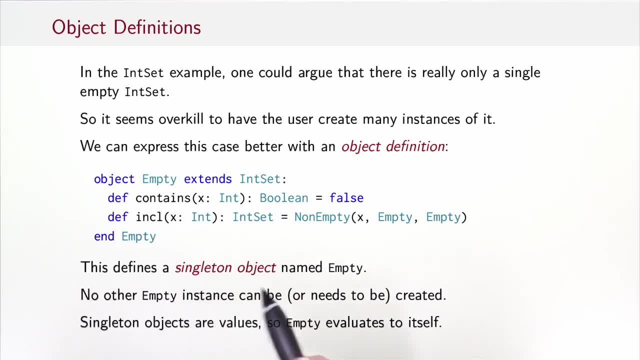 optional end marker. This defines a singleton object named empty. The structure is exactly like a class, but instead of a class that needs to be instantiated, an object exists already, and there's exactly one object that exists, which is called empty. here, No other empty instance can be or needs to be created. 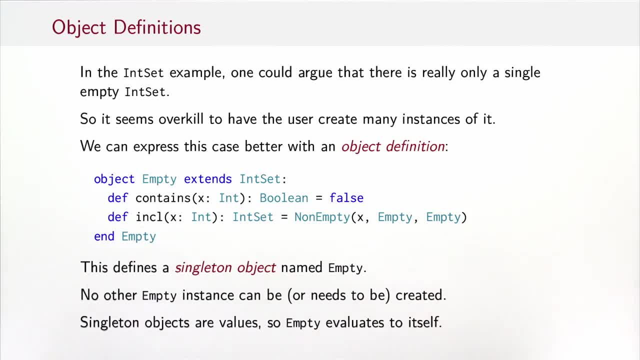 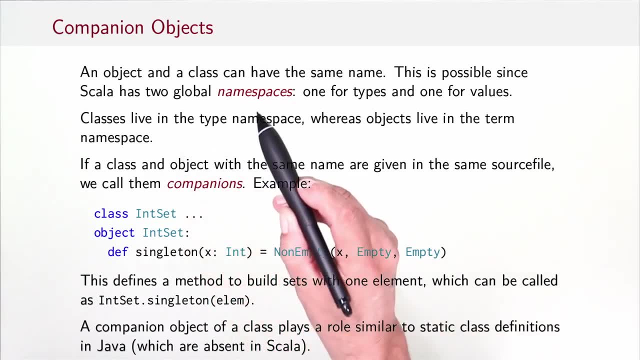 Singleton. objects are values, so empty evaluates to itself, An object in a class can have the same name. This is possible since Scala has two global namespaces, one for types and one for values. Classes live in the type namespace, whereas objects live in the term namespace. 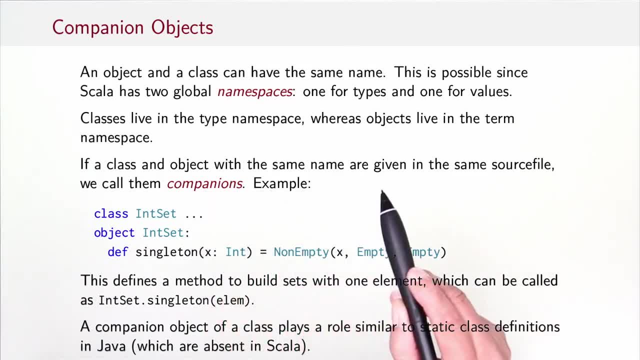 If a class and an object with the same name are given in the same source file. we call them companions. So for instance, you could have a class IntSet with the usual methods and then you could have in the same source file an object IntSet that adds: 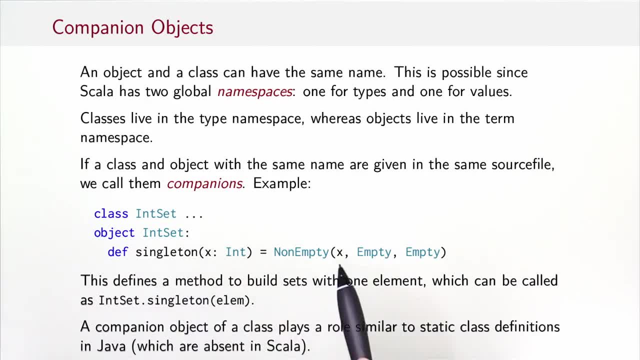 a method, let's say singleton, that creates a set consisting of exactly one given element. A companion object of a class plays a role similar to what static class definitions are in Java. That means in the companion object you would typically put methods that exist only once per class and not once. 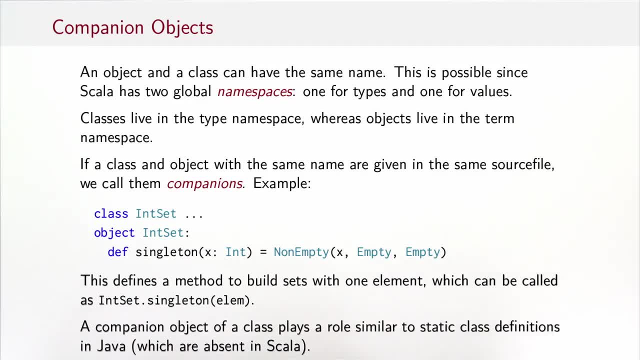 per class instance. Static methods are absent in Scala because Scala is a purer object oriented language than Java. So in order to emulate what you would do with a static method, you define a singleton object with the name of the class and you put the methods in that singleton object. 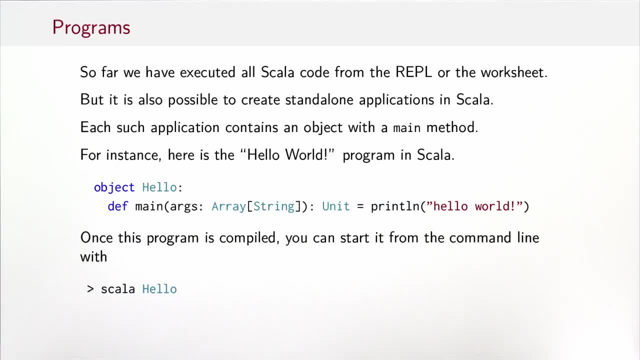 So far, we've mostly executed Scala code from the REPL or the worksheet, but it's also possible to create standalone applications in Scala. Typically, such an application takes the form of an object that has a main method, and the main methods have to follow a particular convention. 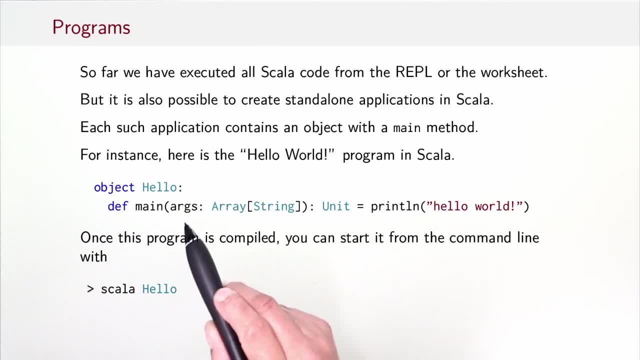 which is inherited from Java. They have to take a single argument of type array of string and they return unit. A main method then has a body that is executed when the program is called. So you call the program by typing Scala in the command line and then the name of. 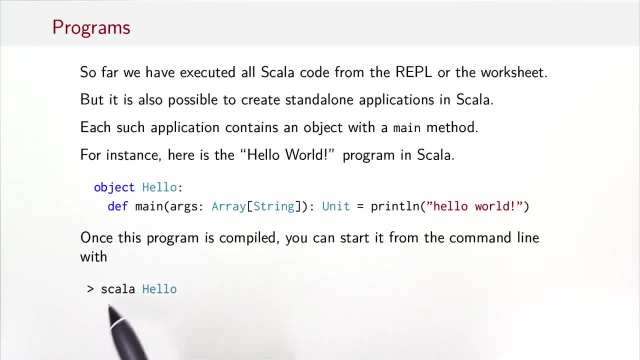 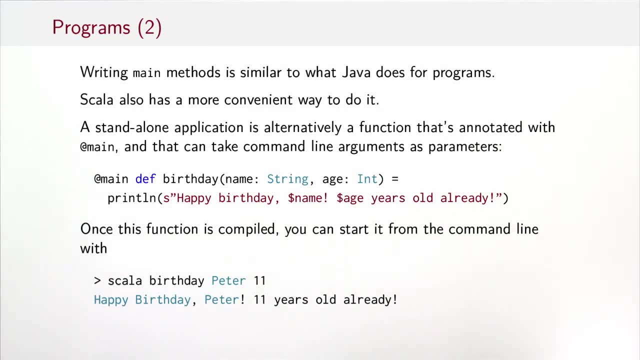 the object. So once this program here is compiled, you can start it with Scala hello and you would see hello world. So writing main methods is similar to what Java does for programs, but Scala also has a more convenient way to do it, and you've seen. 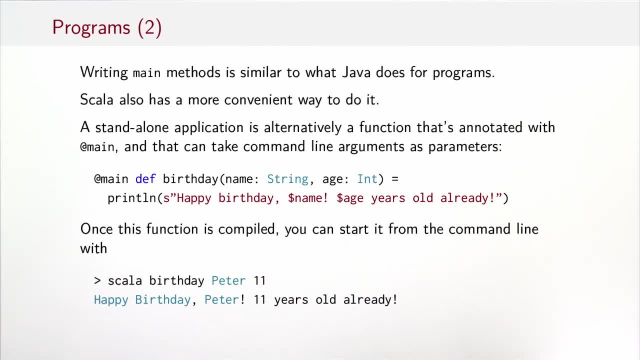 it already that you can have a Scala program, a Scala text, and you can just put in the Scala program a single method that's annotated with main, So that method then also gives you a main method for the program. You can have a method here. let's 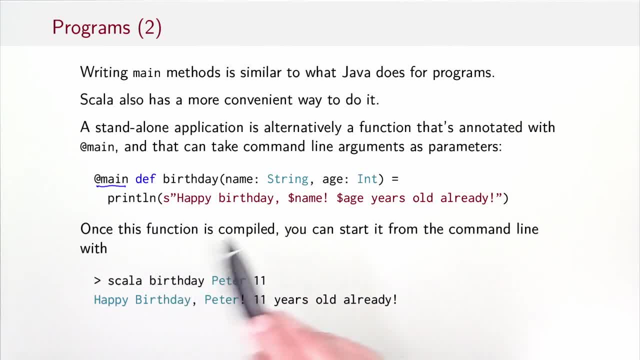 say birthday, that takes a name and an age and it prints happy birthday. name. age is already. Once this function is compiled, you can call it from the command line with Scala birthday and then you pass just arguments for the two parameters here: Peter for the name and 11 for the age. 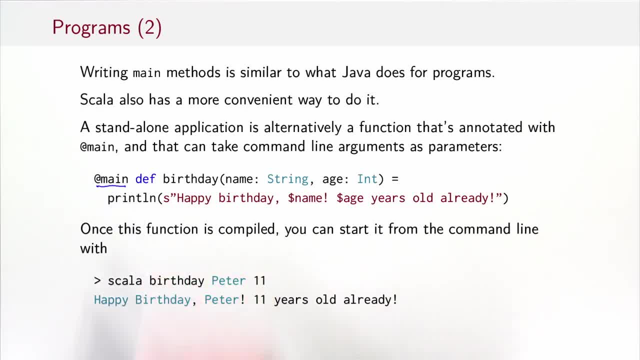 And that's what you would get. So typically, using main as an annotation is a more convenient way to start a whole or to define a whole program Under the covers. then it will translate into an object with a main method as the JVM prescribes, but you won't see that That's. 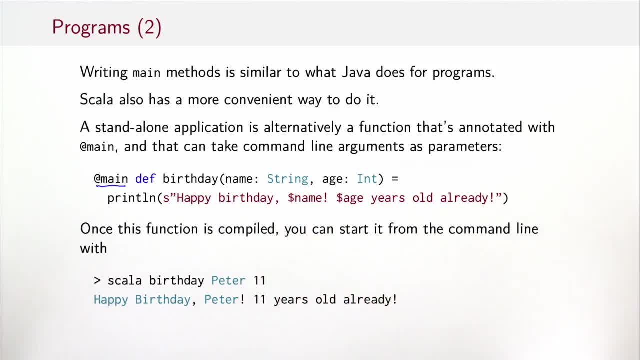 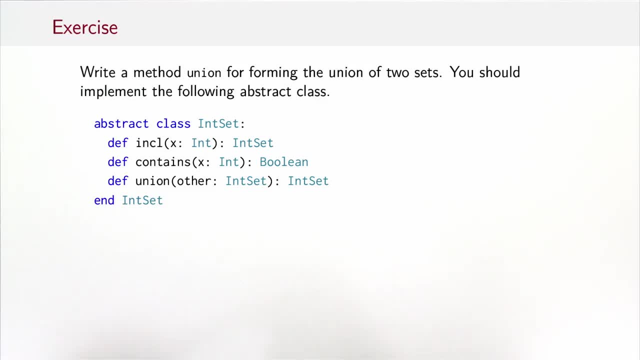 essentially the compiler wrapping this birthday method for you in a synthetic object that has the correct main method. So here's an exercise. Let's write a method union for forming the union of two sets. So you should implement the following: abstract class, class inset: as before. 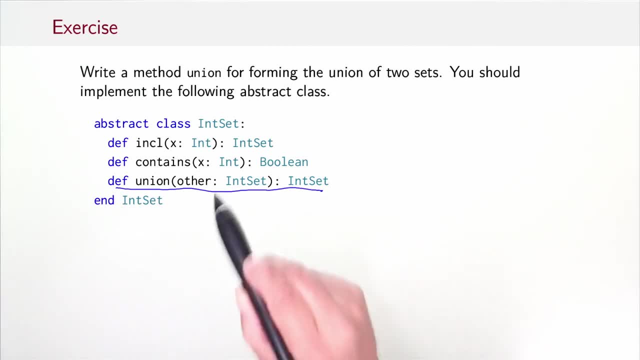 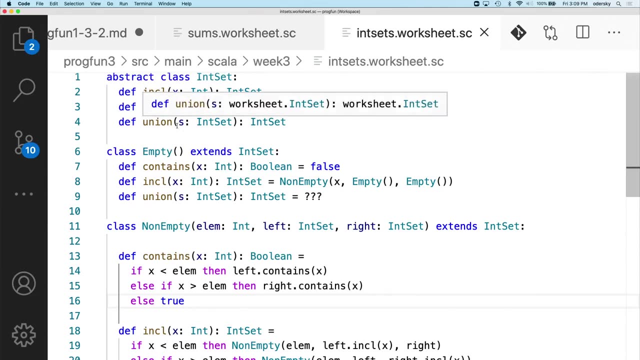 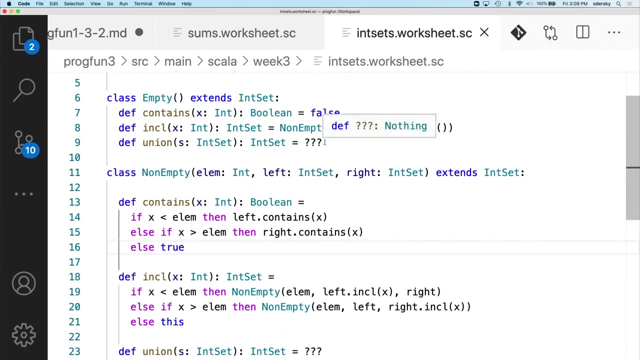 but now it has a third method, union that takes another inset and returns an inset. So I have prepared a worksheet here where we see the union method up here and already templates for the union method in empty and non empty, and so far the implementation is missing. 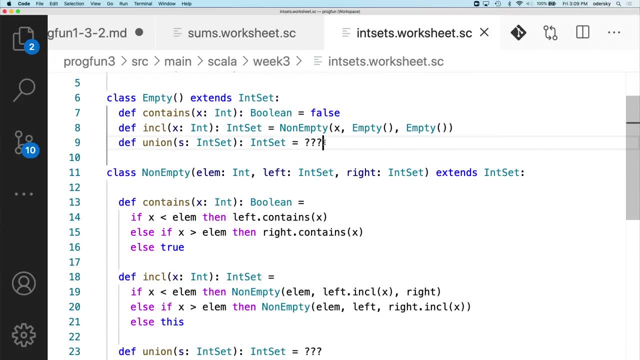 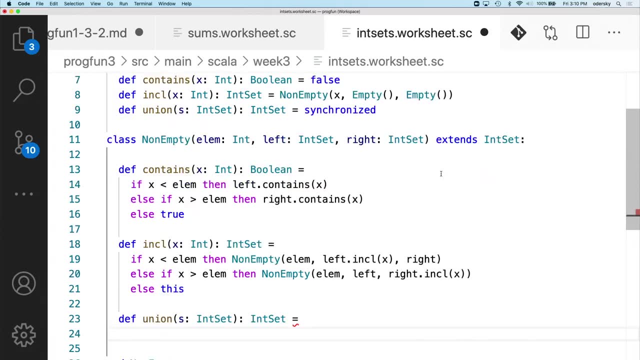 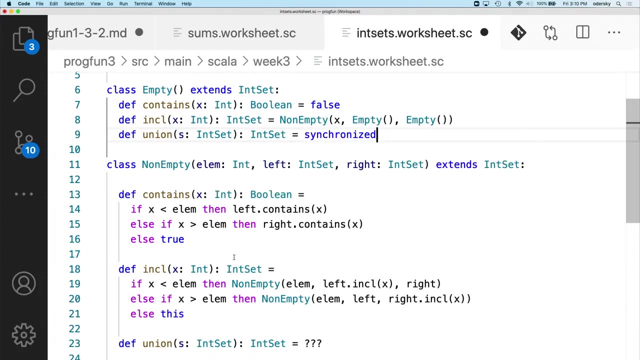 which is indicated by this triple question mark. So the task is to replace the two triple question marks with something that implements union. What's the union of the empty set and another set? S? Well, that's obviously S, so that was simple. What's the union? 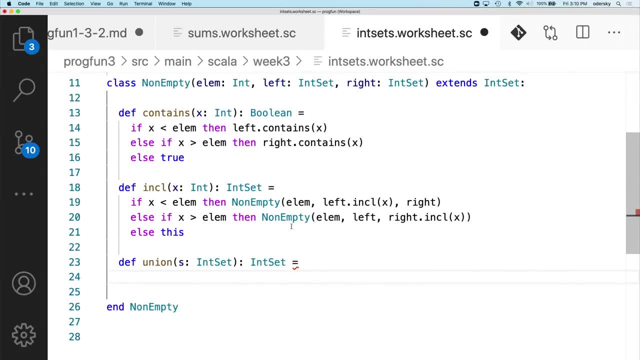 of a non empty set consisting of an element and a left and right subset and some other set S. That's actually harder, So here's one way to do it. The idea is that what we need to do is we need to reduce it somehow to include. 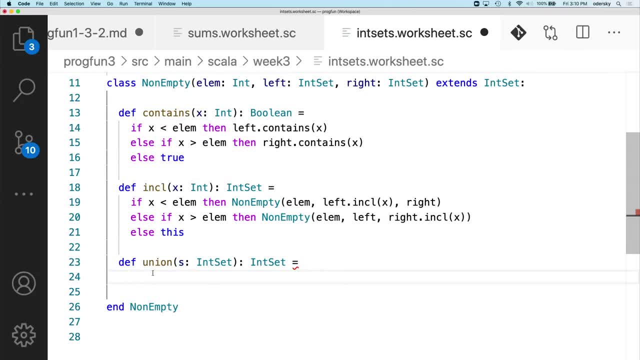 So we need to include with the union of something that is smaller. So one way to do it would be to say we take the left set and form the union with the right set and the union with S, and then we finally include lm in that. 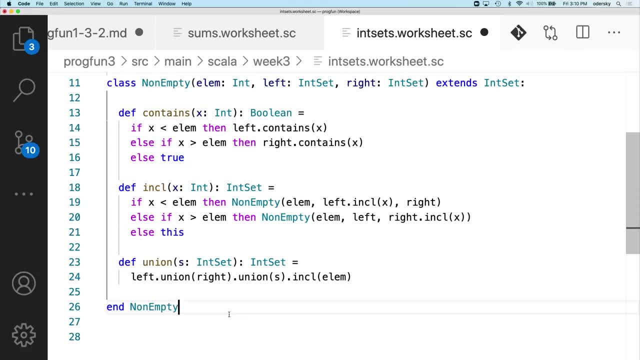 So this is very recursive. One union call gets replaced by two more and a call to Inkle. How are we sure that this terminates? Well, the argument here would be to say: well, each of these following unions here, union sets that are smaller than the sets we started with. 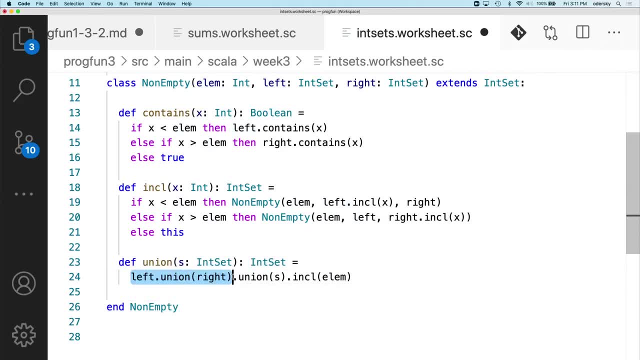 So we started with the current set. that set is clearly bigger than left or right, so that union here will essentially work on something which is smaller. And then, finally, we take the union with S, and that union here has to work on the right set. So we have the same right hand side, but 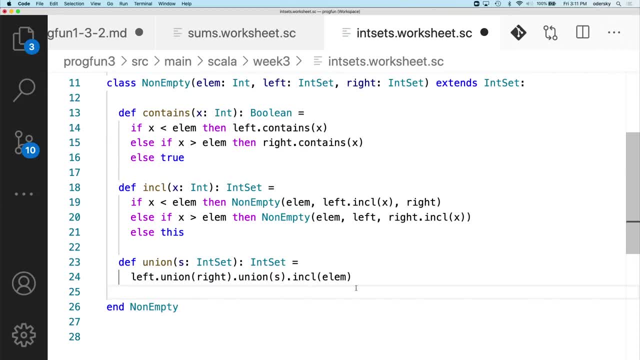 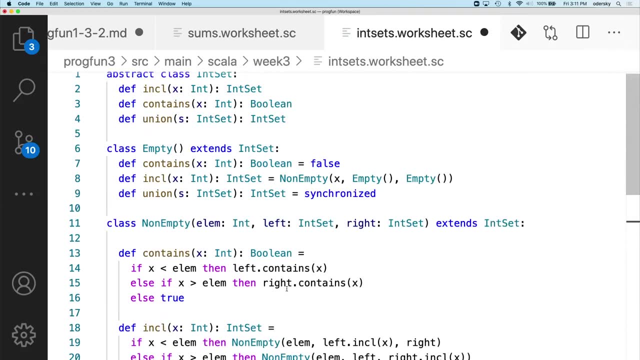 the left hand side is one element smaller And then we compensate, finally by including the element at the end. So if we do that, then the left hand set will get smaller and smaller and smaller until finally it will be the empty set. and when it's the empty set, 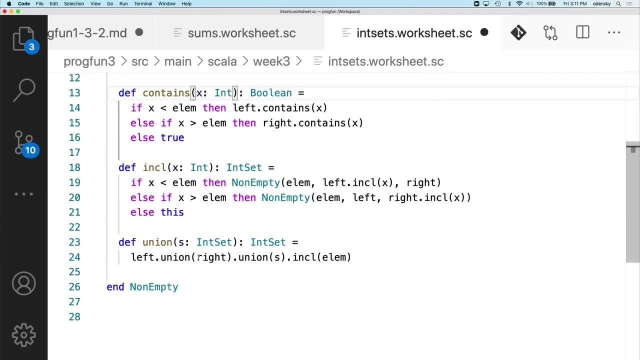 then okay, then we know what it is. It's just S, So then the recursion terminates. So that's the termination argument and it's correct. But nevertheless, a call to union like that is pretty inefficient, because essentially we decompose and reconstitute. 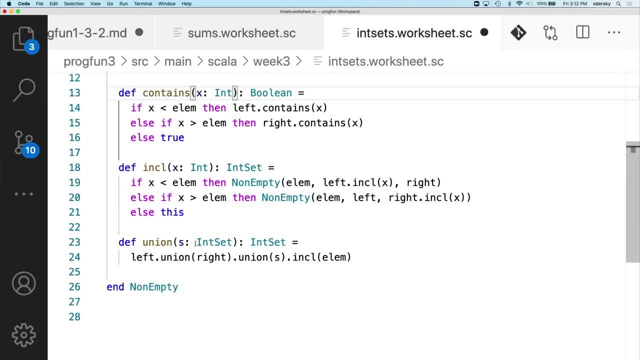 that set multiple times and it would be much, much nicer if we could simply go through the second set inset and say, well, pick all the elements of that set and just include them one by one into the current set. But for being able to do that we'd have to look. 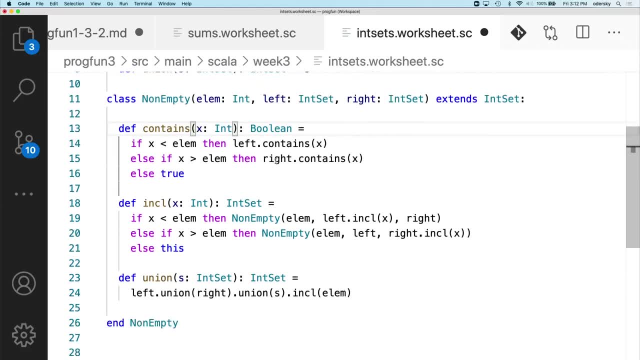 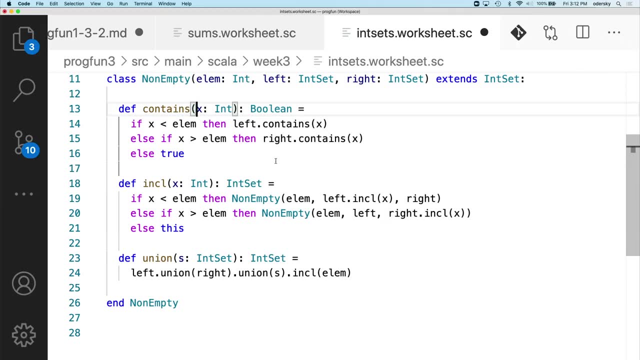 inside the second set and say, well, what are the elements of the second set? and so far that interface doesn't give it to us. So we'll learn techniques to decompose data structures, to find out what's inside data structures in the units that follow this one, So one. 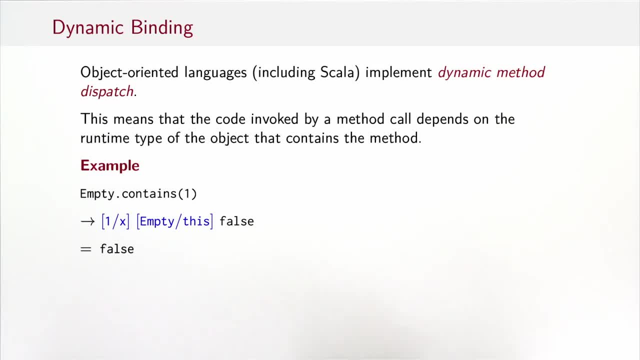 interesting consequence of class hierarchies is that they lead to dynamic method dispatch. That means that the code that's invoked by a method call depends on the runtime type of the object that contains the method, And in fact that falls out directly from our substitution model. 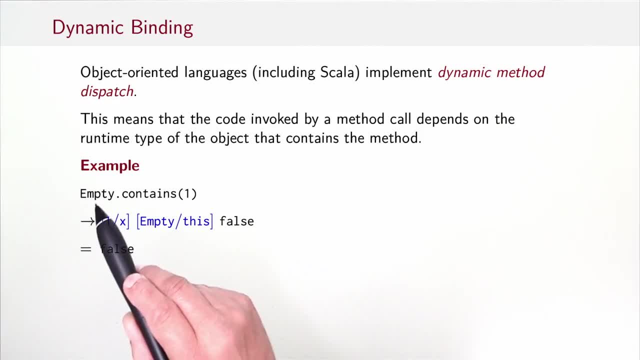 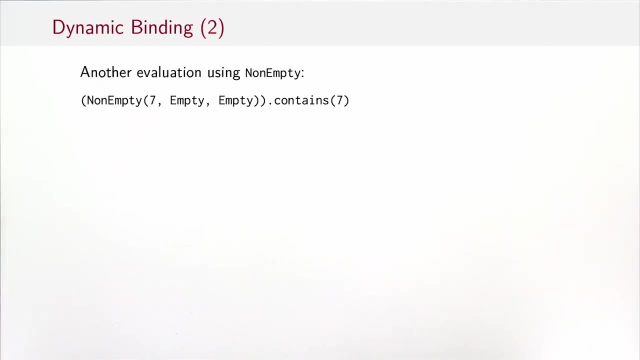 So we can put that to the test and just ask: let's say, for the empty set contains one, So that would be the contains method in the empty set, which is simply false with these substitutions, and that would give us false Now if we use the same. 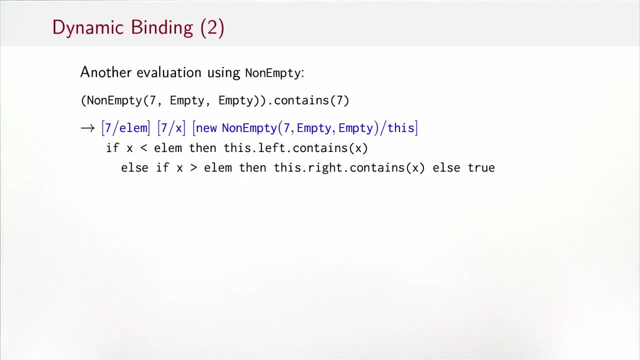 method call contains seven with a non-empty set, then what that would give us is the implementation of contains in the non-empty set. So that's this one here, Subject to the substitutions is substitute formal for actual parameters and then substitute the non-empty set here for 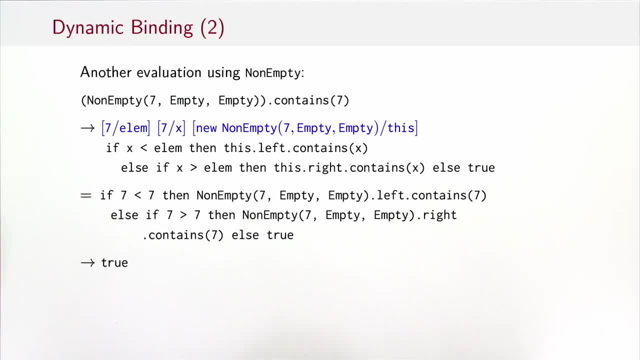 this And we can trace the substitution and that will eventually give true. So what we've seen here is that the sequence of reductions that gets performed depends on the value to the left hand side of the method, And that's what we call dynamic binding. 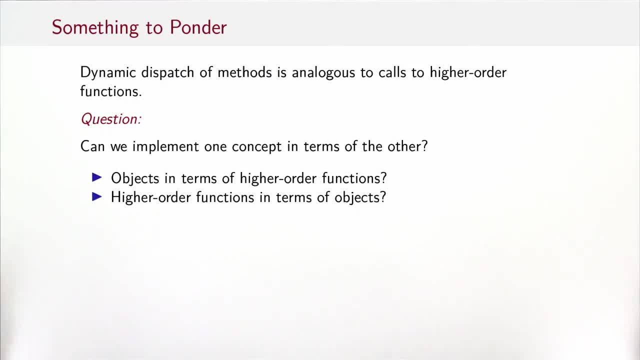 or dynamic dispatch. So here's something to ponder for you. Dynamic dispatch of methods looks quite analogous to calls to higher order functions. In each case, the target where the call goes is not obvious from just looking at a single expression For higher order functions. 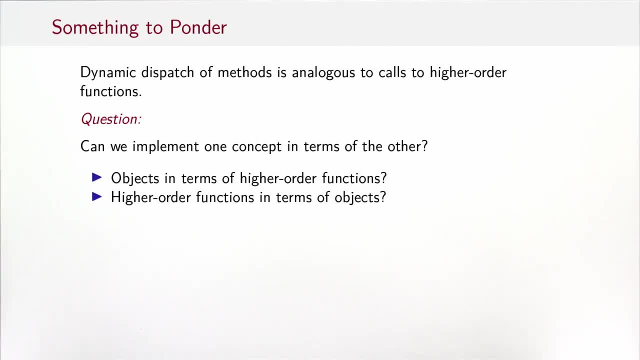 it depends what got passed as the actual argument to the parameter and for dynamic dispatch it's what is the value to the left of the dot. So the question is: can we implement one concept in terms of the other? Can we implement objects in terms of higher order functions? 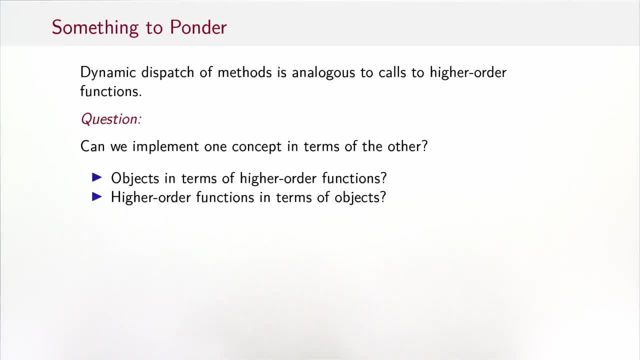 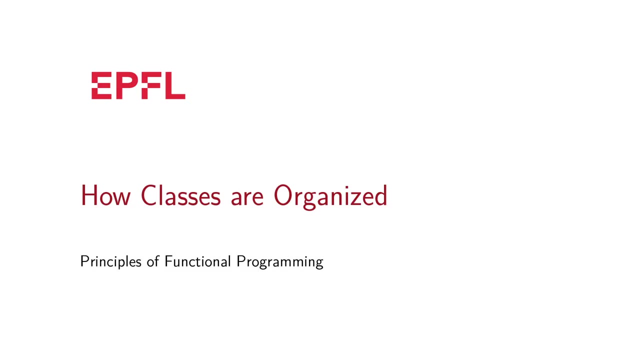 or can we implement higher order functions in terms of objects, Or maybe can we do both Implement one concept in terms of the other, in either direction. In this unit, we are going to learn a little bit more how classes are organized into larger programs. 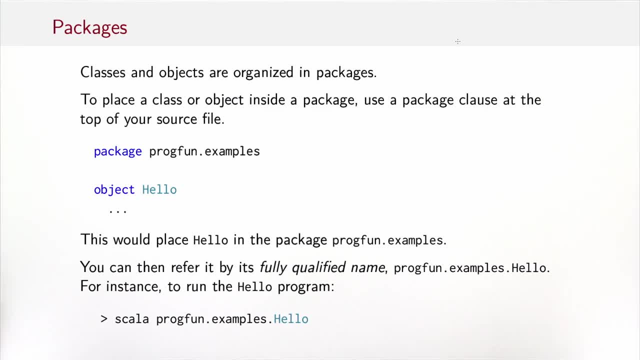 Classes and objects are conceptually members of packages. You can think of a package as similar to a directory in a file system. In fact, packages often correspond one to one, to directories. To place a class or object inside a package, you use a package clause. 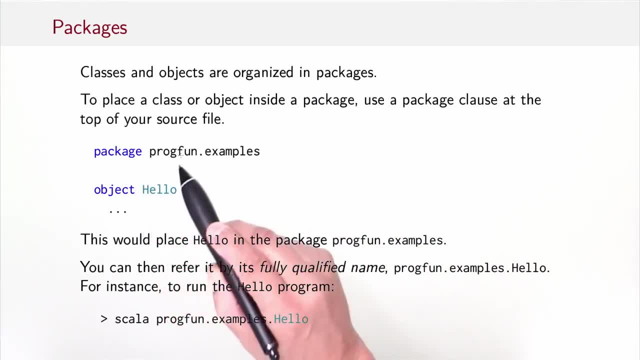 at the top of your source file. So you write package proc fun- examples and then object: hello, and that would give you an object in the package proc fun dot examples. Usually you organize your sources so that you would have a directory proc fun and that directory would. 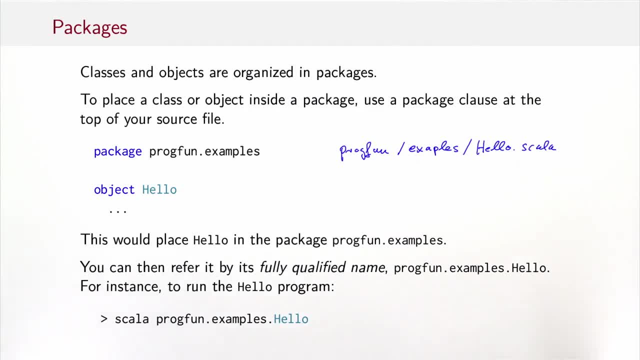 contain the file hello dot Scala. So that's the normal way you organize source files, but it's not enforced by the system, it's just a convention. Once you have an object in this package, you can refer to it by its fully qualified name. So to refer to hello, you would write: 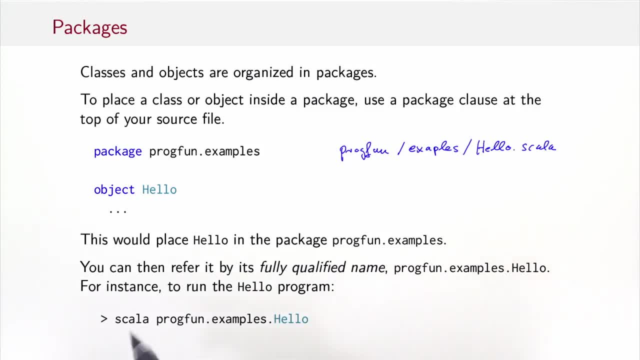 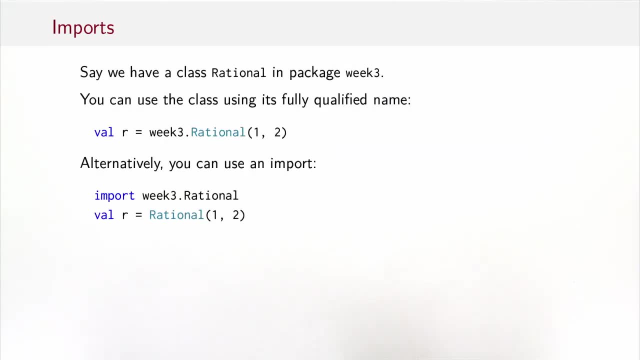 proc fun dot. examples: dot hello. For instance, to run that hello program you would write Scala proc fun examples: hello. Now, to avoid having to write long package names over and over again, you have imports. Let's say we have a class rational in package week. 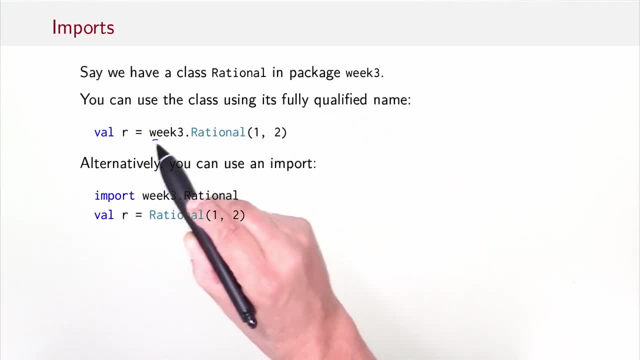 three. We can use the class using its fully qualified name, like this: week three, rational. Alternatively, you can also use an import. You can say import week three, rational and that makes rational known under its simple name here, So you don't need the week three dot prefix. 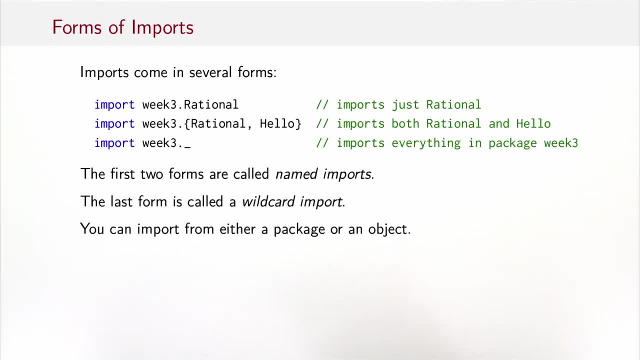 Imports in Scala are quite flexible. They come in several forms, so you can either have an import that imports a one specific thing or several things. So import week three: rational hello in braces would import both rational and hello. or you can have a wildcard import which we write with an underscore. 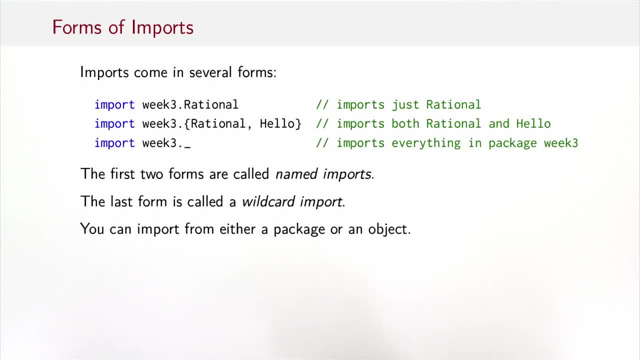 So that third import would import everything in package. week three: The first two are called named imports and the last is a wildcard import, And you can import from either a package or an object. In fact, conceptually, packages in Scala are just essentially very large. 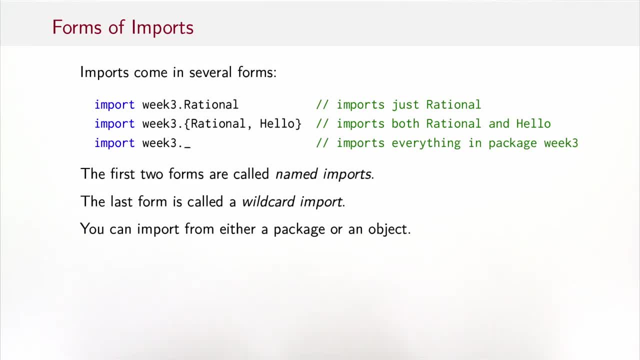 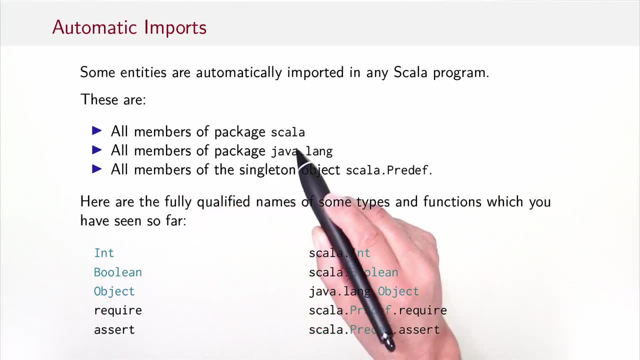 objects that have members that are each in individual source files. Some entities are automatically imported in any Scala program. These are all members of the package Scala, all members of the package java dot lang and all members of the singleton object Scala dot predef. So some. 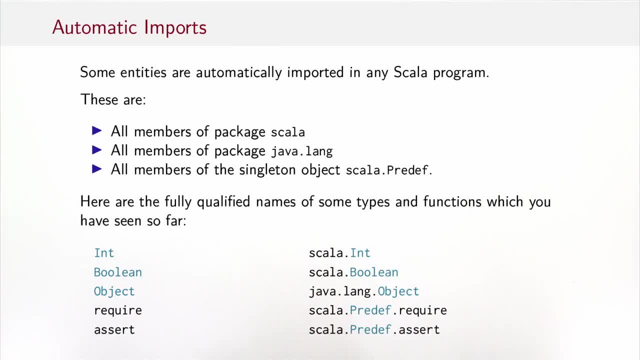 of the names you've seen before actually live in these packages and objects and are imported automatically. The int type is really Scala dot int, so it's the same as defined in the Scala package and it's made available because of this first automatic import. The same happens for the boolean type. 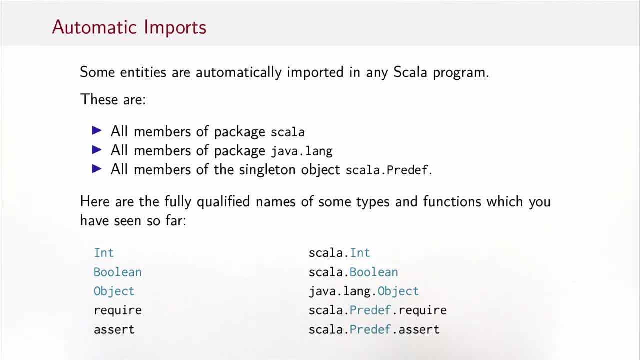 and object which you get from java dot lang object. The require and assert methods that we've used in the rational example are actually defined in the Scala predef object as methods and you get them by the automatic import from the Scala predef object, So they're really Scala predef require. 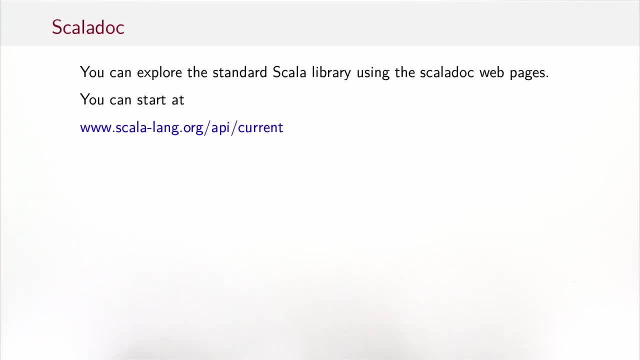 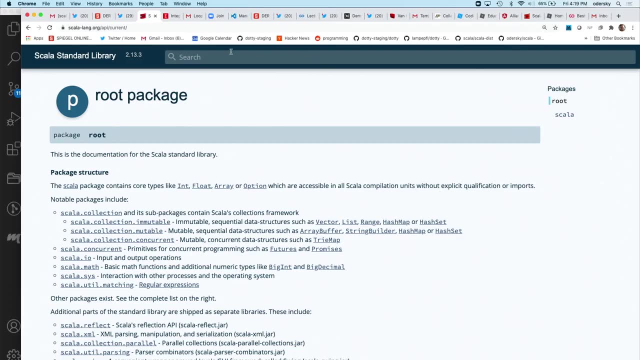 and Scala predef assert. You can explore the standard Scala using the Scala doc web pages. You can start at this web address. So here we see the root page of the web pages and we can look for the definition of a type. let's say: 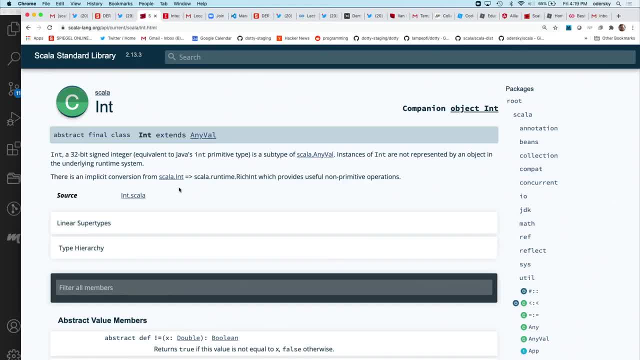 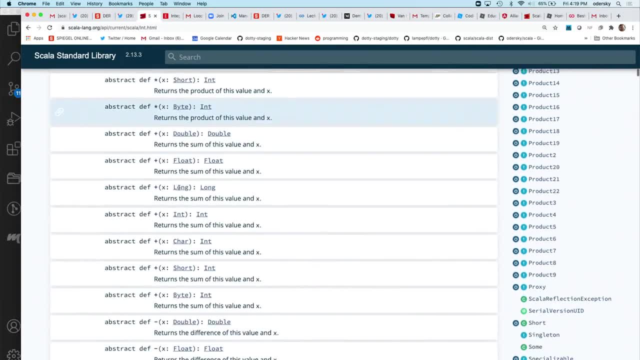 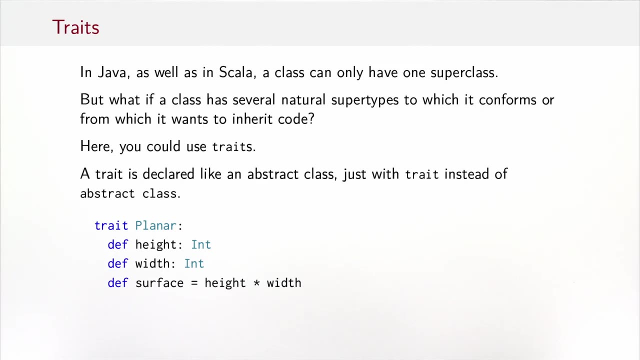 int and that would then give us the Scala int type and all the methods that are defined on that int type. So you see the usual suspects, all the operators that you can have on int and several others more. Another important concept in Scala are traits. 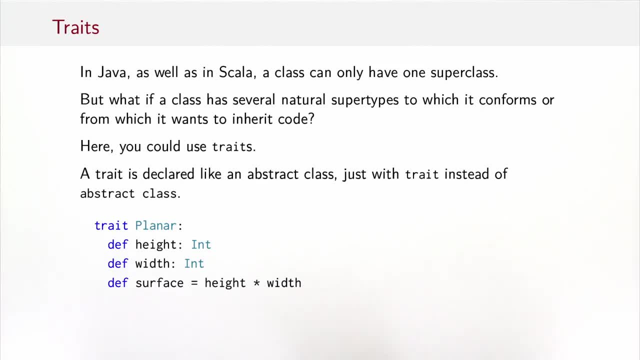 So traits are similar to classes. The difference is that in Scala, as well as Java, a class can only have one superclass. It can extend only one class. But it often happens that a class has several natural supertypes to which it should conform and from which 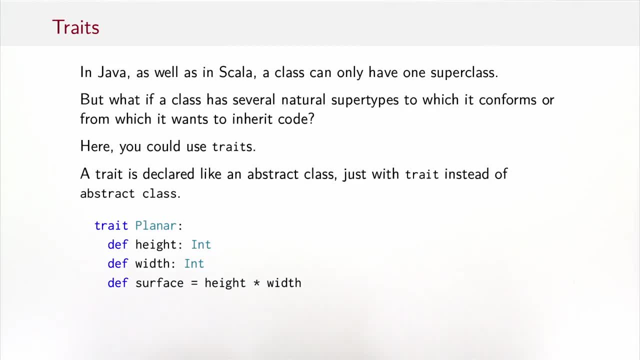 it sometimes wants to inherit code. In that situation you could use traits. A trait is declared like an abstract class, just with trait in front instead of abstract class. So here we have a trait planner that has height and width, which are kept abstract, and surface, which is defined as. 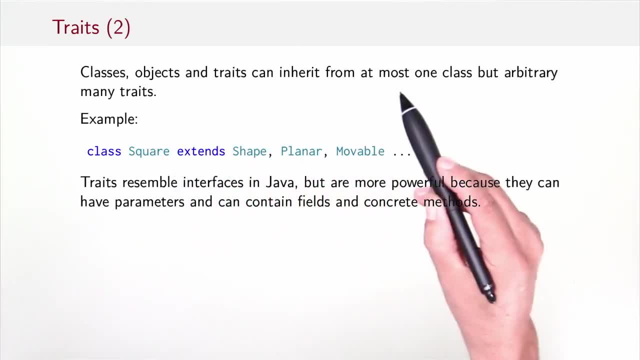 height, times, width, Classes, objects and traits can inherit from at most one class, but arbitrarily many traits. So, for instance, you could have a class square that extends shape, which might be a class, and then it also extends traits. planner and movable Traits resemble interfaces. 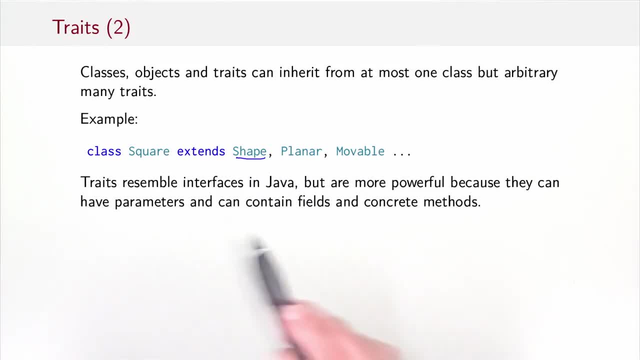 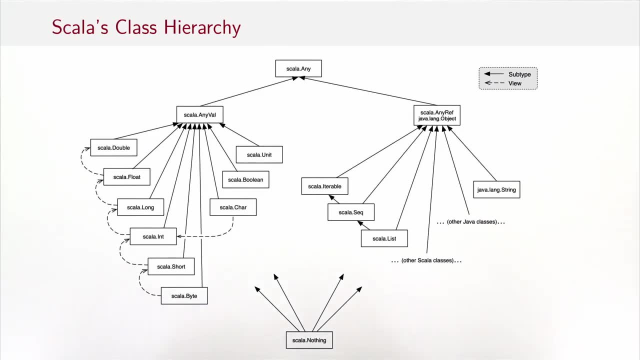 in Java, but they are more powerful because they can have parameters and they can contain fields and concrete methods. Here is an outline of the class hierarchy as seen from every Scala program. The any class has two subtypes: anyval and anyref. Anyval. 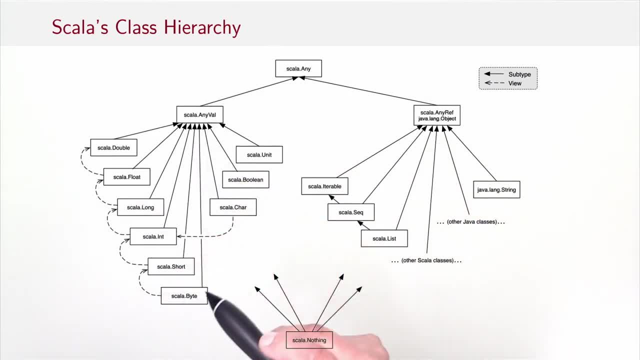 is the common superclass of all primitive types. So we have nine primitive types in Java as well as Scala. They are: double float, long int, short byte. Those are the numeric types, And then character, boolean and unit. On the other side are 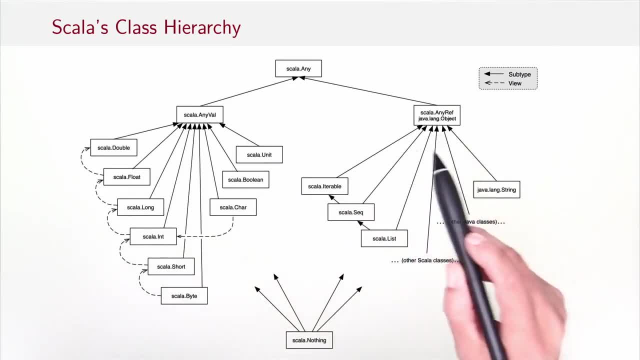 most user defined types. They are all subclasses of Scala anyref, which is just another name and alias for Java long object, The Java's root class. So typical subclasses of object would be string or Scala classes like Scala list, Scala sequence, Scala iterable. 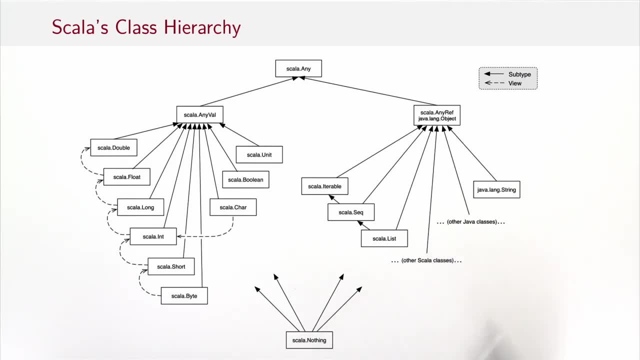 other Scala classes defined by the system or defined by you or other Java classes. They are all inherit from anyref aka object And then, duly to the top type, any scala also has a bottom type: nothing. So the nothing type is a subtype of all the other. 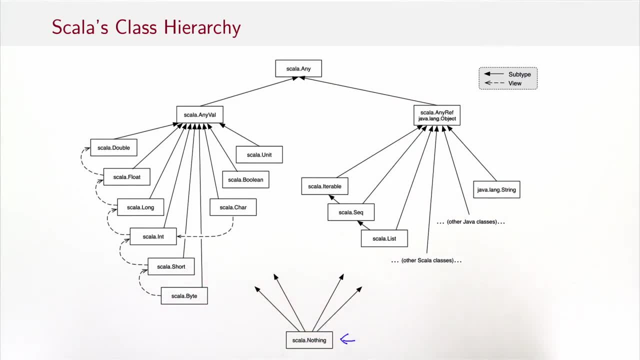 types and it doesn't have a value. So nothing essentially represents a computation that never returns a value. It could be a computation that loops forever, never terminates, or a computation that finishes with an exception but not with a normal value return. So the arrows here mean subtyping. 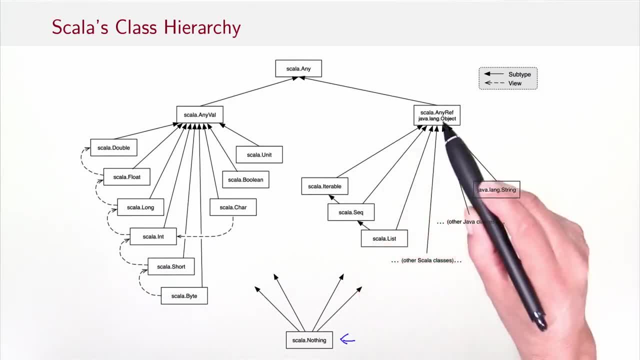 That means everything at the bottom of an arrow conforms to the thing at the top of an arrow. There's also the dashed arrows here. They are conversions, So you have implicit conversions along these edges. For instance, you can convert a byte to a short. 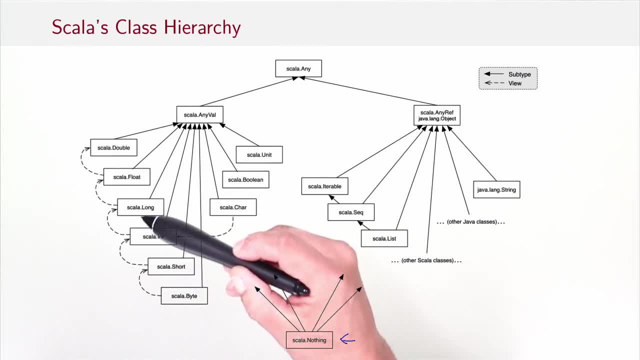 can convert that to an int, can convert that to a long. you can convert a long to a float or a float to a double, and you can also convert a character to an int. They're similar to subtypes, but there's also a difference. 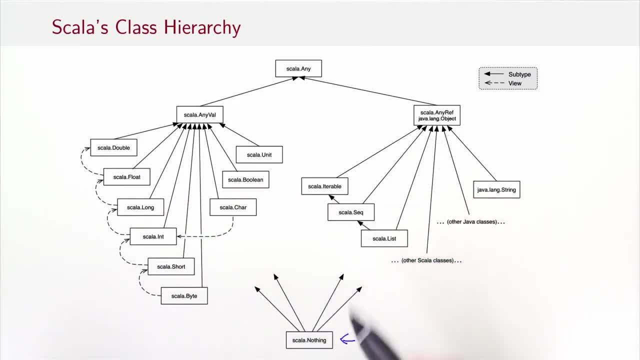 When you have a subtype relationship, the two classes on either end have typically the same representation, whereas for a conversion the representation changes Internally. an integer is not represented the same way as a long. A long has twice the bits of an integer and again a long is not represented the same. 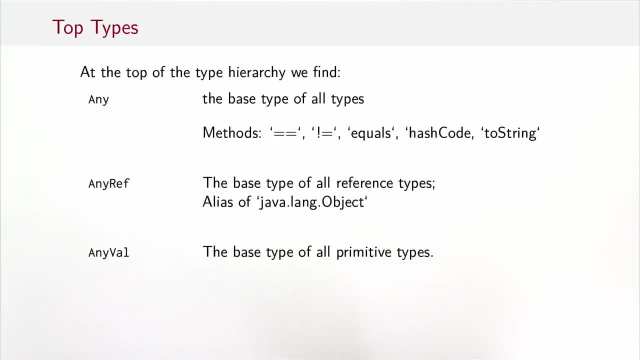 way as a float and a double. So let's take a closer look at the top types of this hierarchy. At the very top we have any, which is the base type of all other types. It has methods for comparisons, equals, not equals, or an alphanumeric equals. 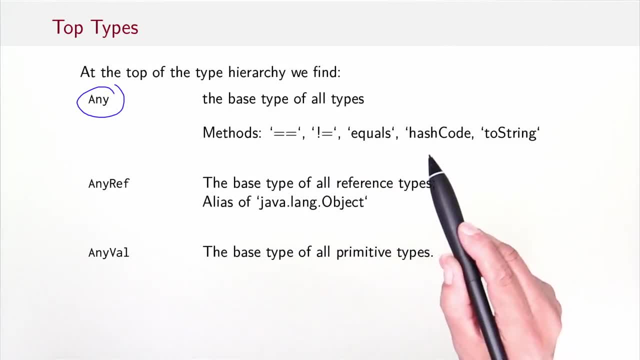 method that's inherited from Java. You can take the hash code of every object and you can turn every object into a string using the toString method. The two child classes are anyRef and anyVal, So anyRef is an alias for JavaLangObject. 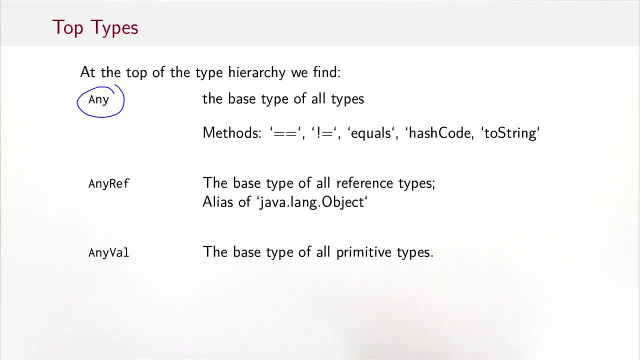 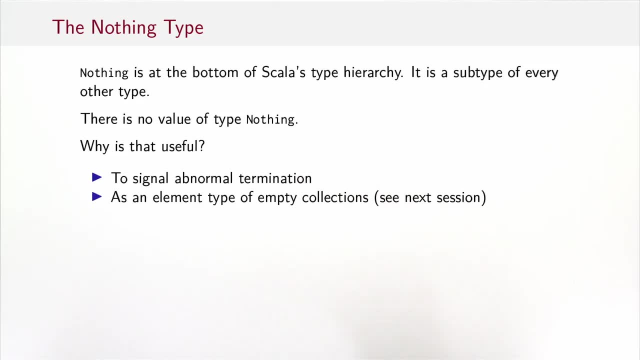 and anyVal is the base type of all primitive types. So we've seen also nothing at the bottom of Scala's type hierarchy, which is a subtype of every other type. There's no value of type nothing, but nothing is nevertheless very useful as a type to signal abnormal termination. 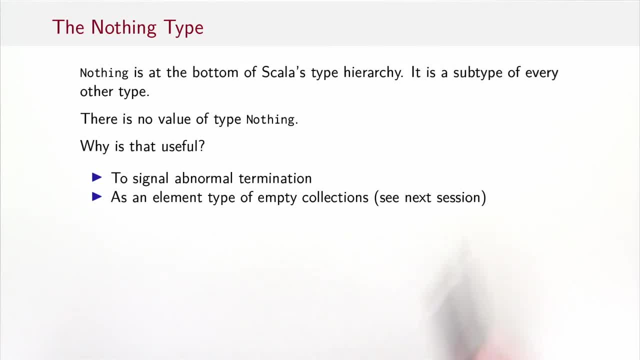 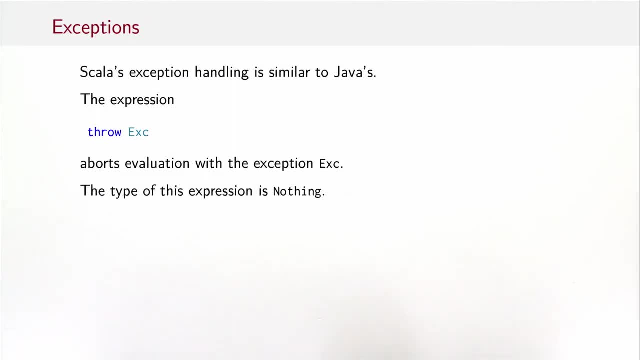 and also as an element type of empty collections. We'll see that in the next week. Another issue we should briefly touch on are exceptions. So Scala's exception handling is quite similar to Java's. The expression throw exception with a type of an exception aborts the. 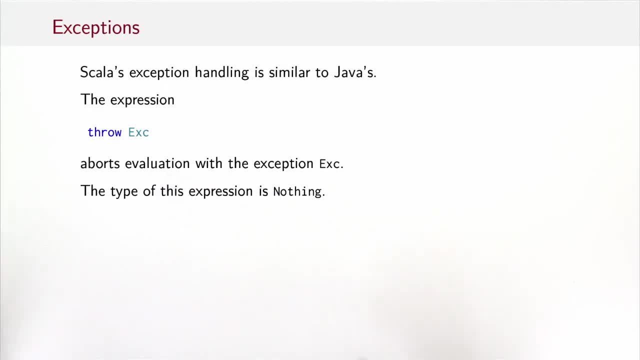 evaluation. with the exception xc And the type of this throw expression is nothing, because there's no value that's returned from the expression. So let's finish with an exercise. What's the type of this expression? If true, then one else false. Is it int or boolean, or 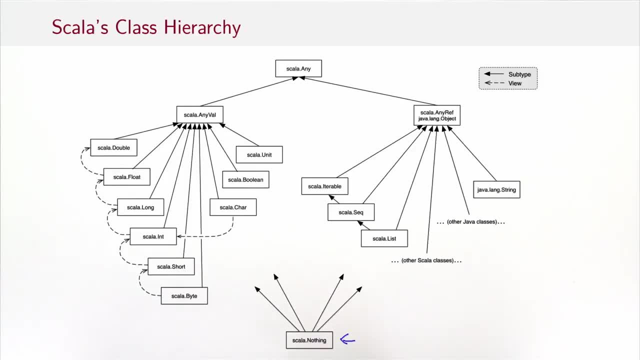 anyVal or object or any? To answer this question, let's look at the class hierarchy. So we had two branches of the if, an int and a boolean One and false. So their common supertype is anyVal and indeed that's also the type of the if. then else, 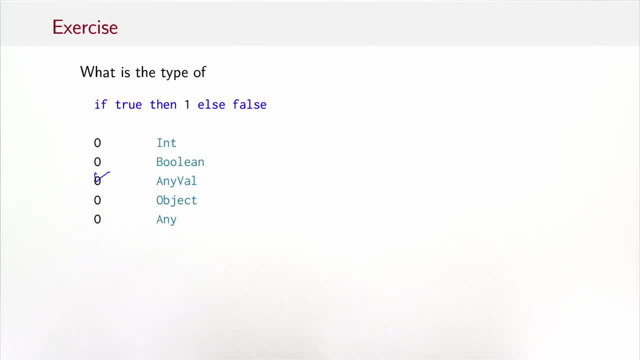 So anyVal is the correct answer here. You might have said: well, why isn't the compiler smart enough to say, well, the condition is always true. so the if statement will evaluate to the first side, which is an int, In which case the type maybe should. 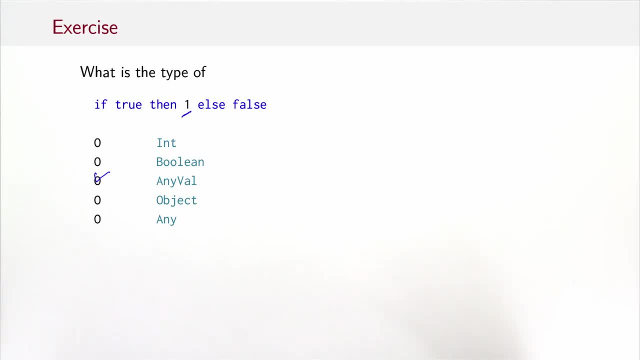 be int, which is a subtype of anyVal, and subtypes are considered as better types of the supertypes. The compiler is intentionally not doing that because it would lead to instability of programs. If you change this condition to something that was less obviously true, some condition. 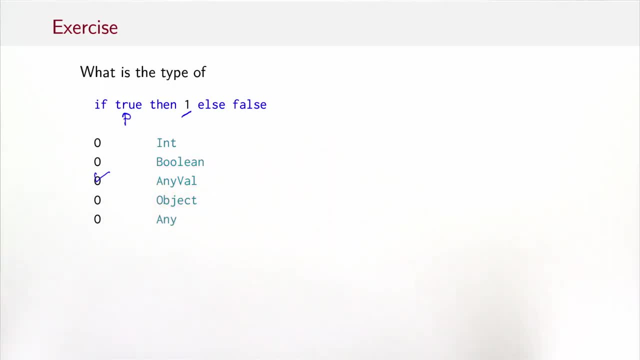 p, let's say. then suddenly the type of the if would become less good. It would go from int to anyVal and that might break your program. So that's one of the things where a programmer would know more than what the type system of a compiler. 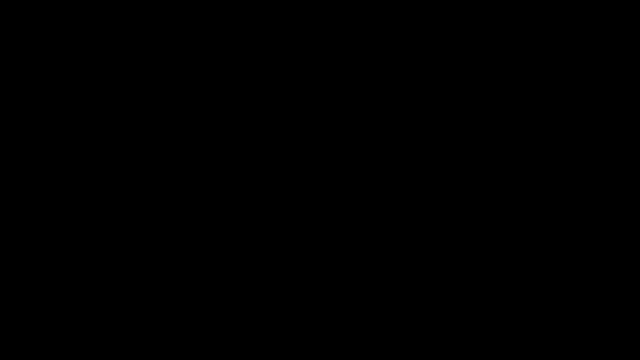 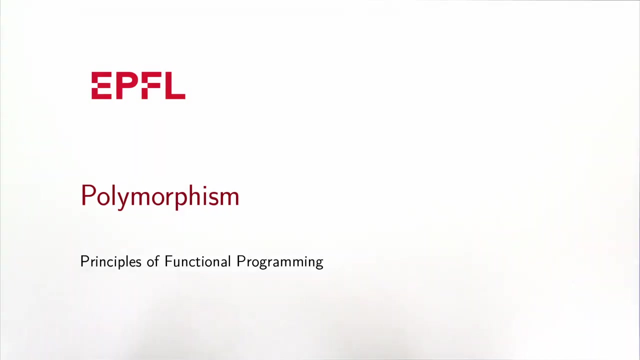 actually gives you. In this section, we are going to introduce polymorphism, which is a way to define classes so that they can be used more flexibly. Before we get there, let's introduce a data structure that's truly fundamental for most functional languages: The immutable. 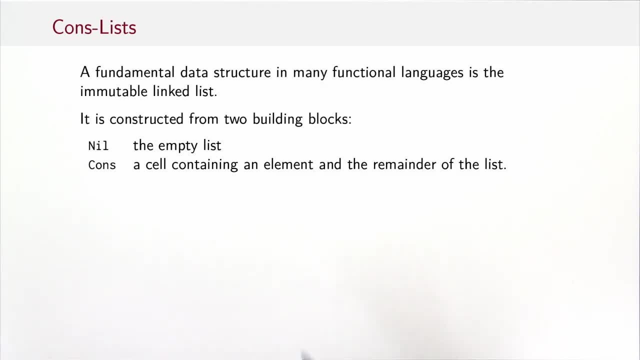 linked list. An immutable linked list is constructed from two building blocks. nil is the empty list and cons is a cell containing an element and the remainder of the list. Let's look at some examples for cons. The first list is list of 1,, 2, 3.. That would be. 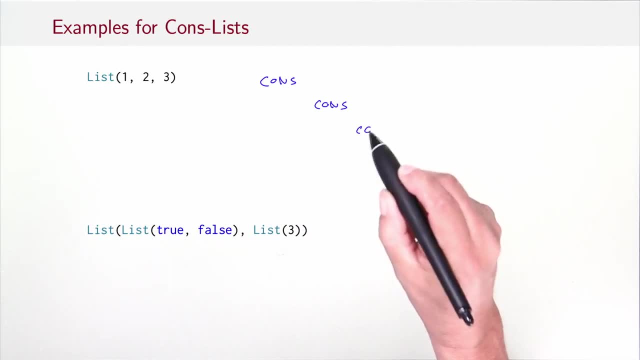 represented as three cons cells. Each cons cell contains one of the elements of the list and the remainder is the list that contains the other elements. So the list 1,, 2, 3 would start with a cons cell containing the element 1 and would 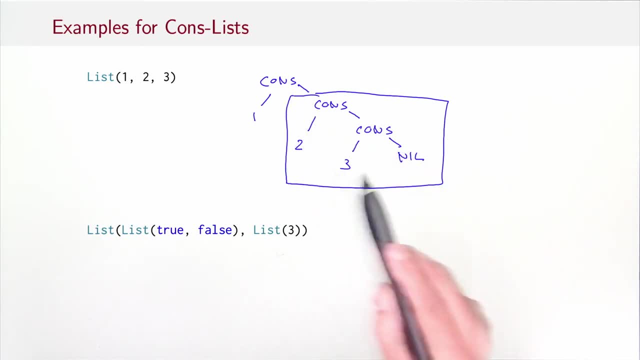 contain as the second half the list 2, 3, and that would contain as the third half the list 3, nil, and that finally has the rest, nil. So that's so. you construct lists recursively by adding progressively more and more elements at the front. Lists can also. 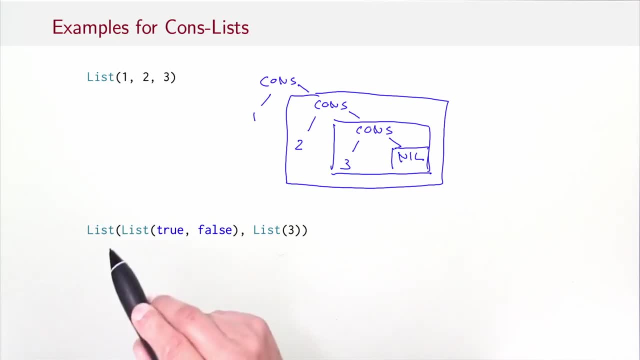 contain lists, and they also contain lists of different types. So here we have a more complicated list, a list whose first element is a list that contains true and false and whose second element is a list of three. So that would look as follows. So here, 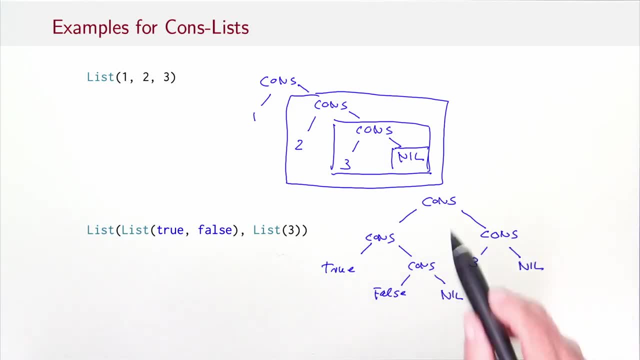 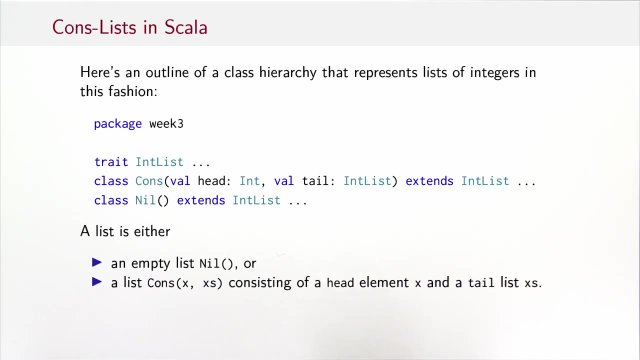 you see the structure of the second list. Its structure is a cons cell that contains a list as its first element and the rest of that list would be a list containing 3 as its element and nil as its rest. To represent lists like this, we can define a class hierarchy. 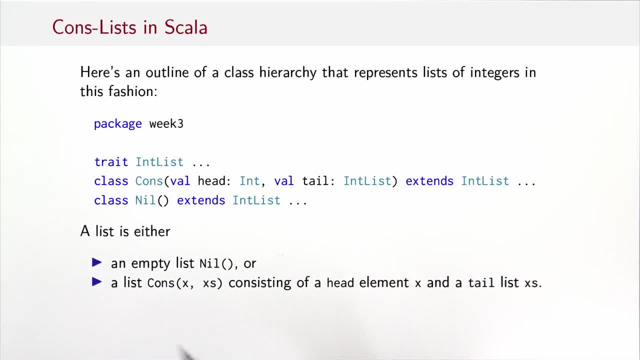 For the moment let's keep it to list of integers only, So we would have a trait int list at the top could also be an abstract class And two subclasses- cons and nil, that both extend int list. So the nil class doesn't have any arguments, The cons- 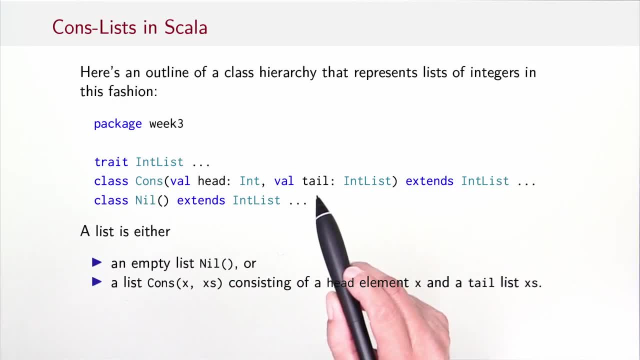 class takes two arguments, which is the head of the list and the tail of the list. So that means a list is either the empty list or it is a cons object that contains a head x and a tail list xs. So we used a new abbreviation. 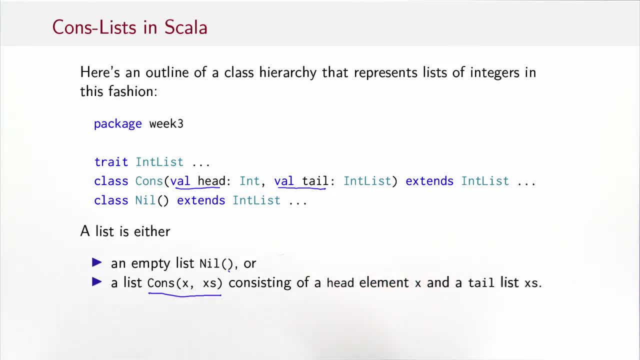 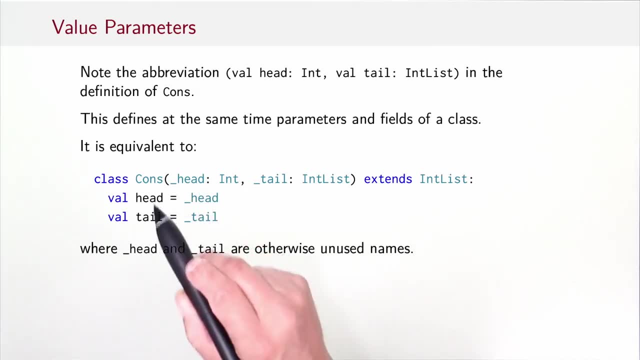 here, where we defined a val head and a val tail directly as parameters of the list. That just means that the parameters are taken also as fields in the same list. So a val head int, val tail, int list means exactly the same thing as if we had defined parameters with some. 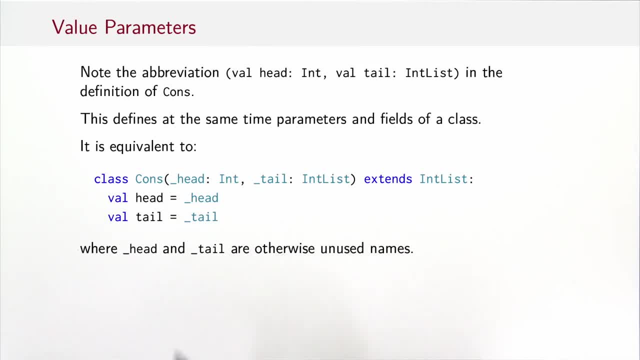 different names, Let's say underscore head and underscore tail, and then had defined two value definitions: head, which is underscore head, and tail, which is underscore tail. So using val's in parameter position, we can define at the same time parameters and fields of a class, which is sometimes 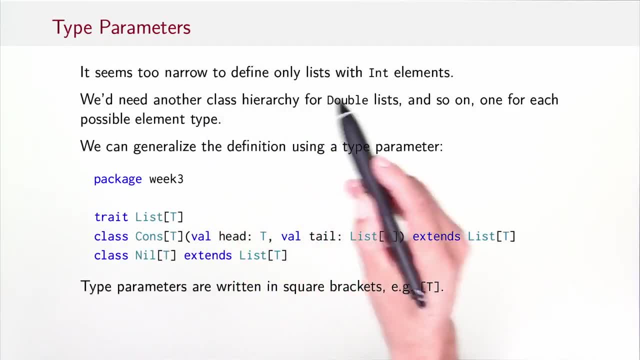 handy. However, it seems too narrow to define only lists with int elements. We then need another class hierarchy for double lists and one for booleans, and so on, One for each possible element types. That's clearly not sustainable, So we can generalize the definition using 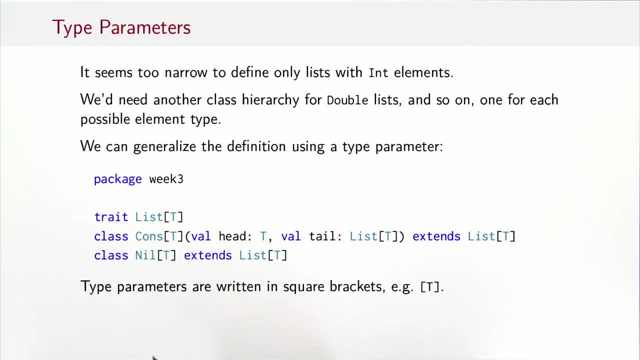 a type parameter. The way we do that is that we add a type parameter, t, in brackets to the definition of class list and the definitions of the two subclasses cons and nil. So type parameters are written in square brackets. That's how you see that you. 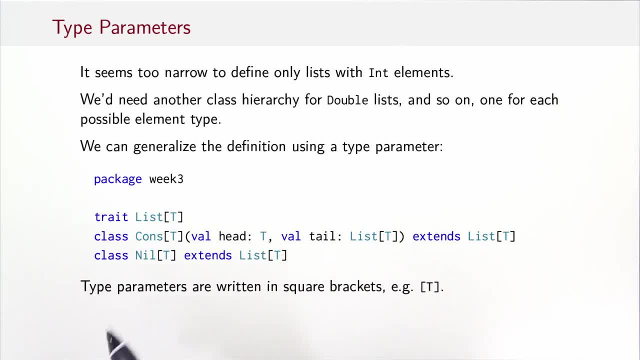 pass a type and not a value. So let's analyze this in more detail. We have a list of t where t is the element type and that has two subclasses. cons of t is a cons cell of type t. That would have a head of that very same. 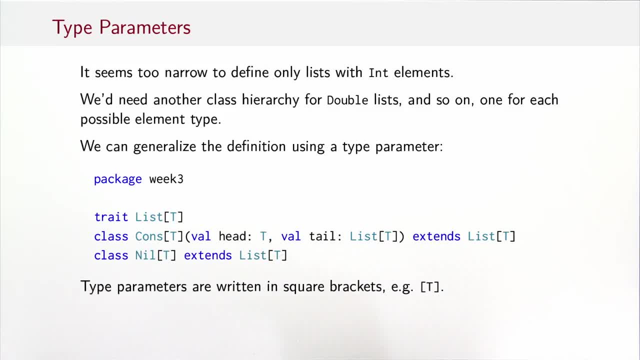 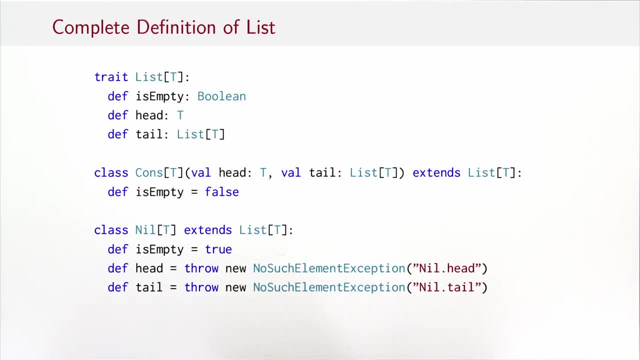 type and a tail of type list of t, Whereas a nil of t is another subclass of list of t. Using type parameters, we can give a complete definition of the list class hierarchy as follows: We have a base trait list of t. It has methods. isEmpty. 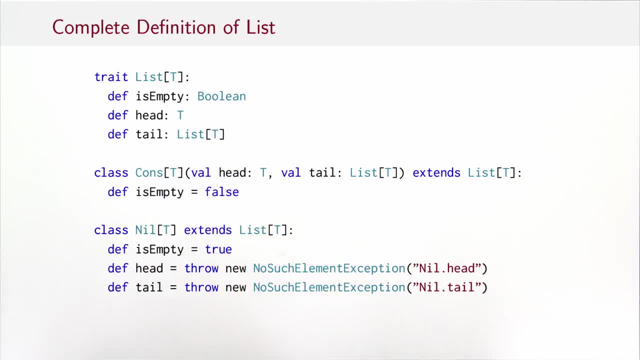 head of type t. tail of type. list of t. We have a cons subclass that defines the head and the tail as the parameters that are given. So that would contain already implementations for the head method here and the tail method here, because the value parameter here 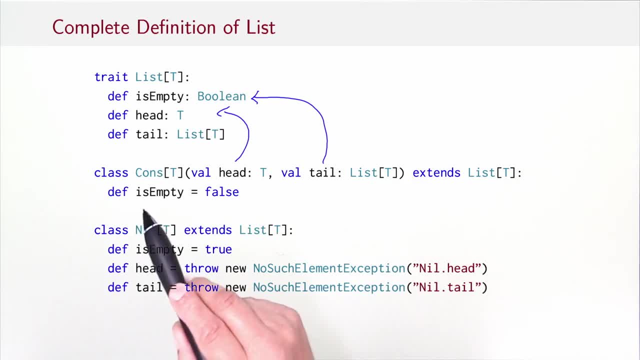 also defines a field. So all that needs to do is really to define the isEmpty method, which for a cons class would be false. And finally we have the nil subclass of list, For nil isEmpty is true, and for head and tail we don't really. 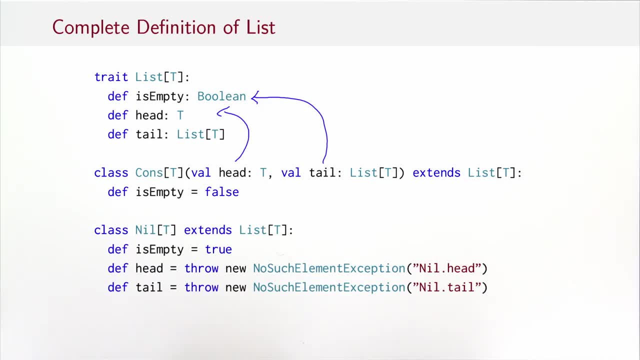 know what to do, because nil doesn't have a head nor a tail. So what we do? instead, we throw an exception. So if somebody would try to call head or tail on a nil instance, they would get a no such element exception. nilhead and niltail. 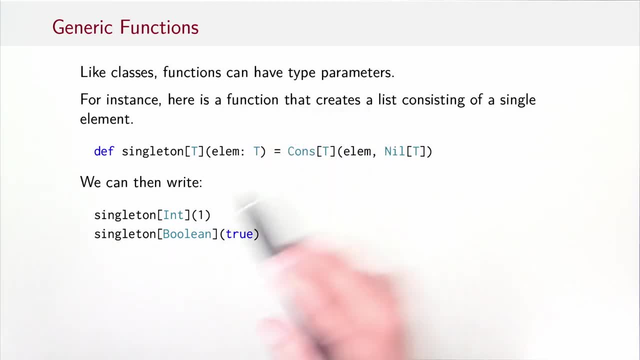 Just like classes, functions can also have type parameters. For instance, we can define a function, singleton, that creates a list consisting of a single element where we leave open what the type of that element is. That means singleton takes a type parameter t and an element of type t and it. 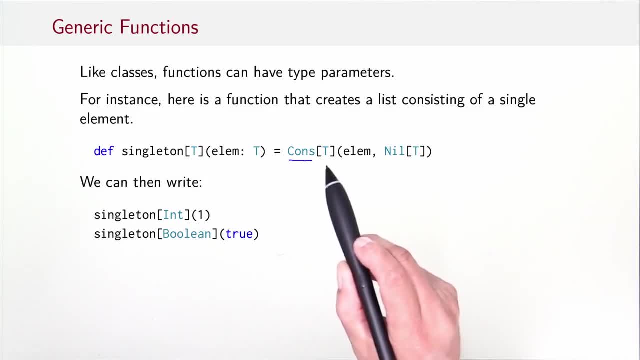 returns a cons instance with that type t and the element and nil as the tail. That means we can now write singleton of int and one that would give the list one cons nil, or a singleton boolean and true and that would give the list cons true, nil. 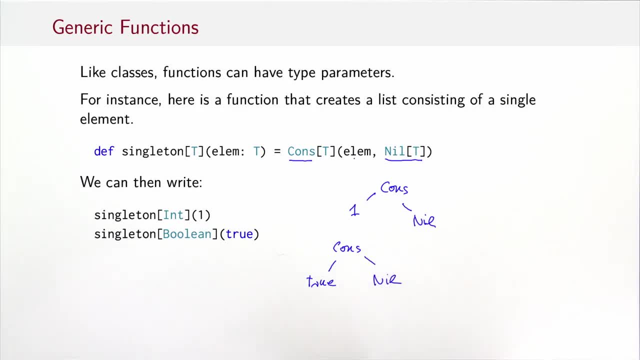 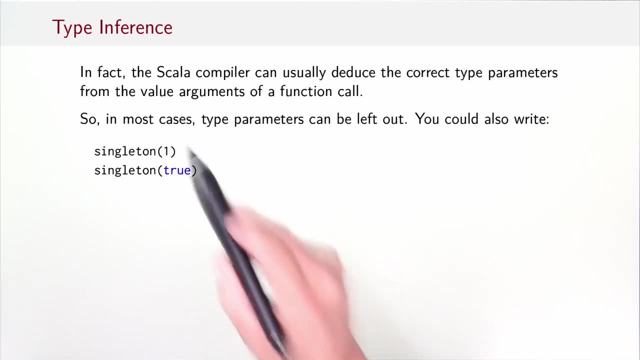 of type. list of boolean. In fact, the Scala compiler can usually find out what the correct type parameters are by looking at the value arguments of a function call. So in most cases type parameters can be left out, and that means concretely for singleton. you could also write: 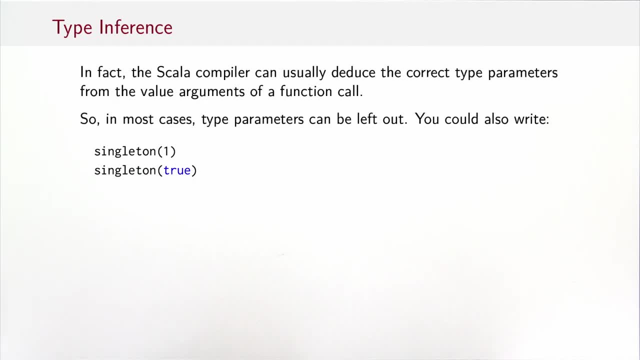 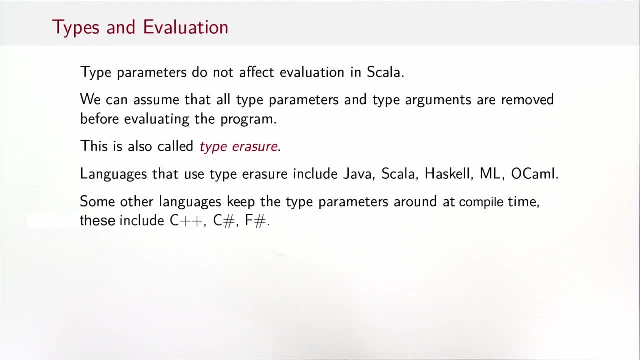 singleton of one and singleton of true, and the compiler would figure out that the correct type parameter is int in the first case and boolean in the second. So now that we have type parameters, do we have to change our model of evaluation? by substitution, Turns out the answer is. 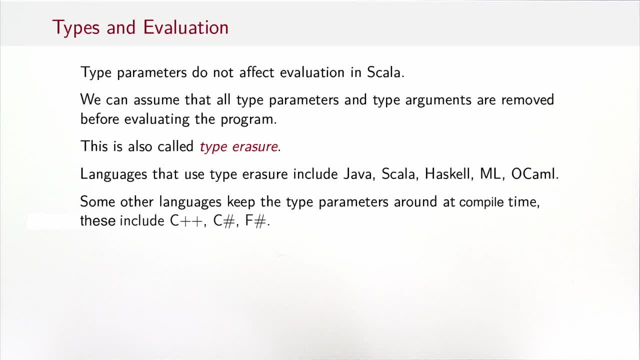 no, Type parameters do not affect evaluation in Scala in any way. In fact, one can assume that all type parameters and type arguments are removed before evaluating the program. So type parameters are a compiler only property. This property is also called type erasure. Types get erased. 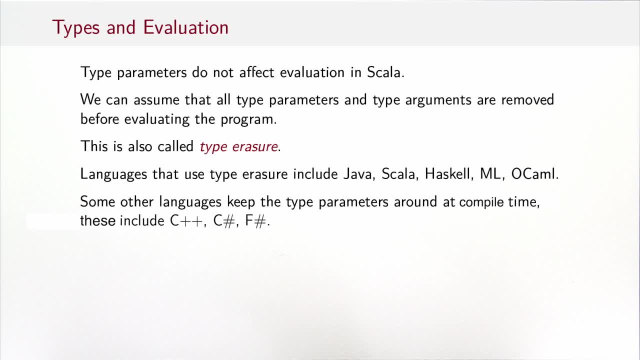 during the compilation process. Many languages that have type parameters use type erasure, including Java, Scala and most other functional languages like Haskell, ML or OCaml. Some other languages keep the type parameters around at compile time. These include C++ and NET languages like C Sharp. 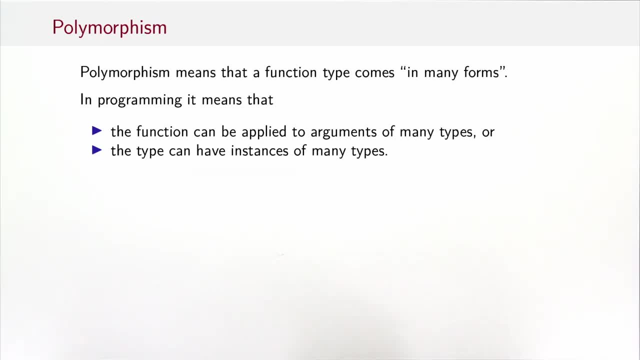 and F Sharp. When we talk about type parameters, often the word polymorphism comes up. Polymorphism means that a function type comes in many forms. Poly means many and morphism means many forms. In programming that means that a function can be applied to arguments of many. 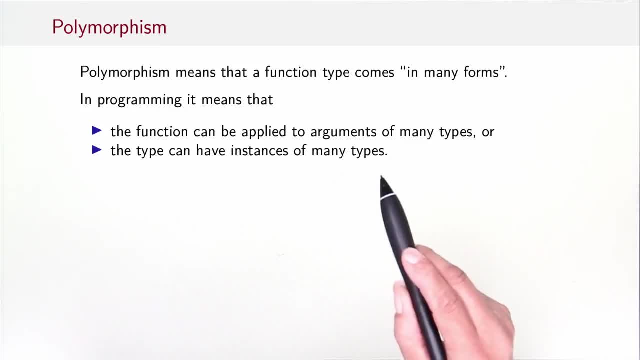 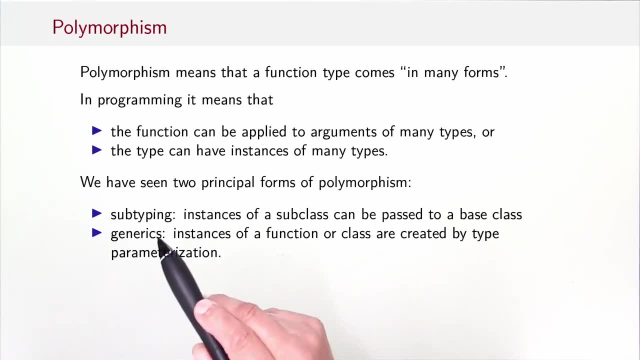 different types, or also that a type can have instances of many types, And we've seen those two forms of polymorphisms by now. In fact, the subtyping that arises in class hierarchies means that instances of a subclass can be passed to a base class. 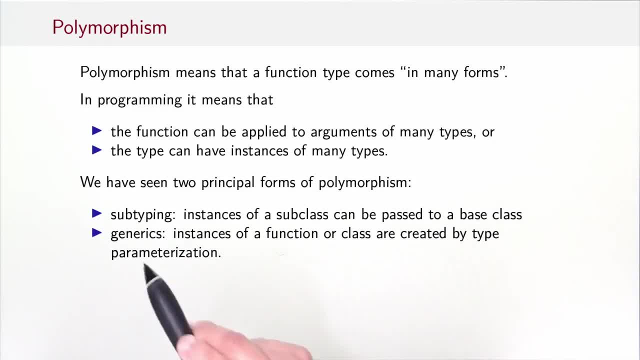 That's sometimes called subtype polymorphism. And then we have the second form with type parameters. that's sometimes called generics. That means that instances of a function or class are created by type parameterization, So we can have many different instances that work on different. 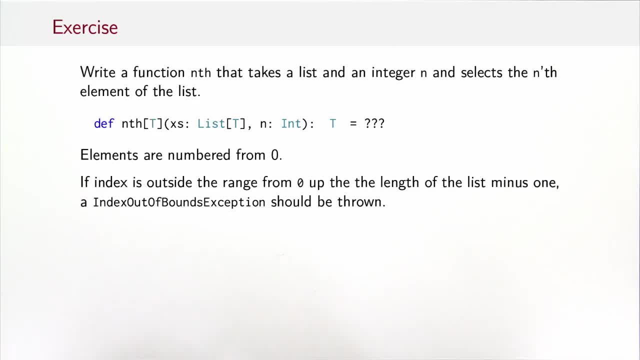 types by passing type parameters. So here's an exercise that uses type parameters. Write a function- nth- that takes a list and an integer and selects the nth element of the list. So the signature of this function should look as follows: We have def: nth. 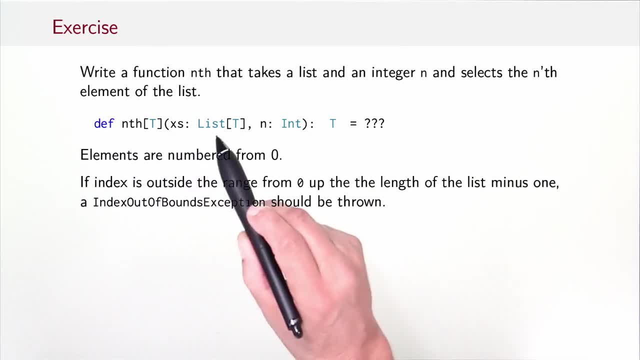 it should take a type parameter t xs, which is a list of t and an index n, and it returns t and you should fill in the body of the function indicated by the three question marks. here. Elements in the list are conceptually numbered from zero, so nth of a. 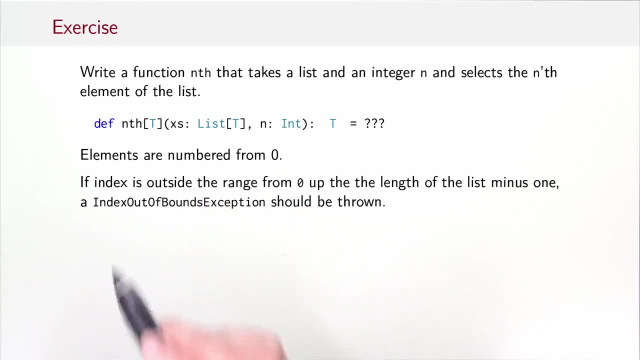 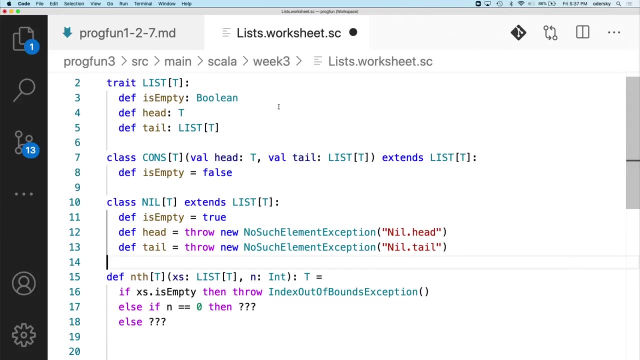 list and zero should return its first elements, And if the index is outside the range from zero up to the length of the list minus one, then an index out of bounds exception should be thrown with a throws statement. So I've copied the list class hierarchy into the worksheet. 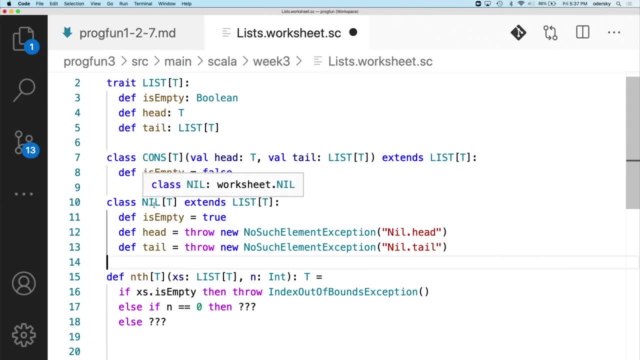 I've renamed all the class names to all uppercase to avoid conflicts with Scala's predefined list and nil classes, And I've already given the outline of the nth method with the types as given. and the first clause of the nth method says: well, if the list 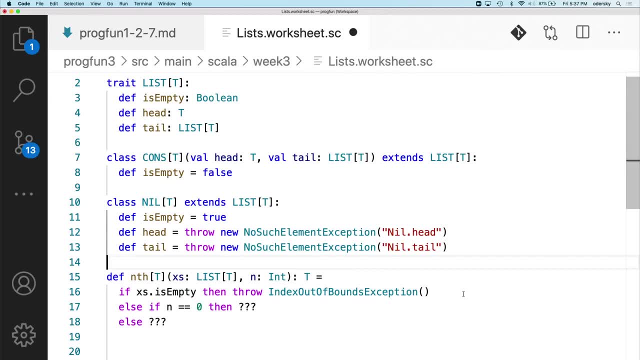 here is empty, then we throw an index out of bounds- exception, Because we can't take the nth element of an empty list. And then we have two other clauses. one is: if the index is zero, then we need to do something, and we need to do something else. 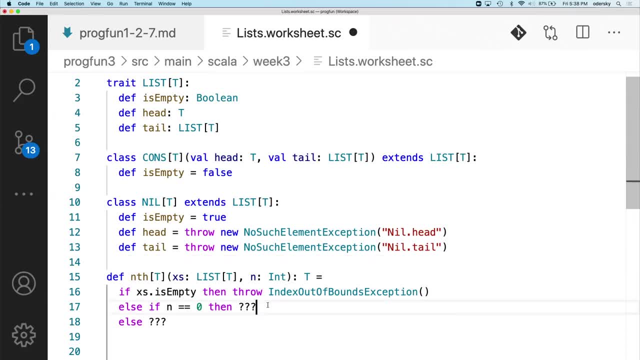 if the index is non-zero. So what do we need to do if the index is zero? In that case we return the head of the list, the first element of the list, And if the index is not zero, then we do a recursive call to nth. 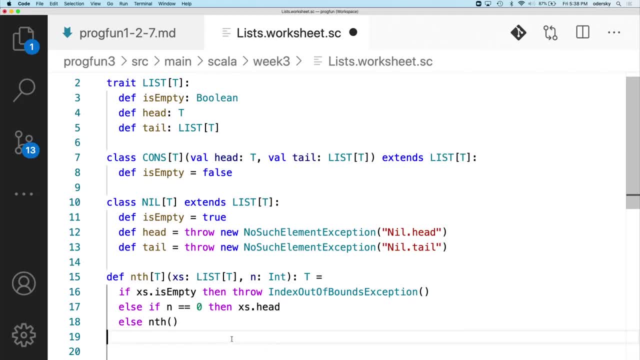 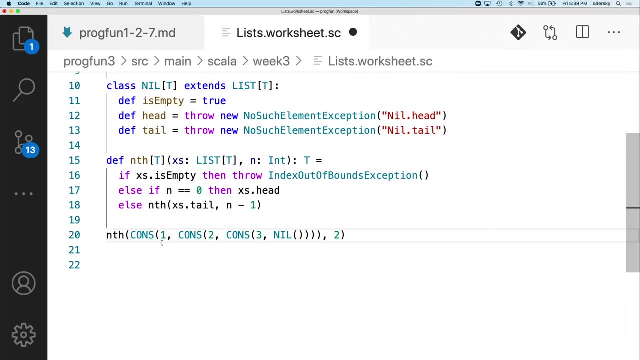 with the list would be xstail and the index would be n-1.. So we can test this by defining a list of three elements: 1,, 2, 3, so that would be cons of 1, cons of 2, cons of 3, nil. 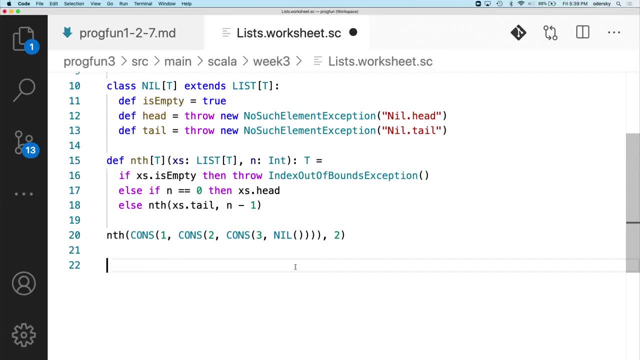 and take the second, the element at index 2, so that would really be the third element, because elements start at zero. so indeed, that would be three. We can test it and say: well, what would we get for the zeroth element? yes, that's one- What would we get? 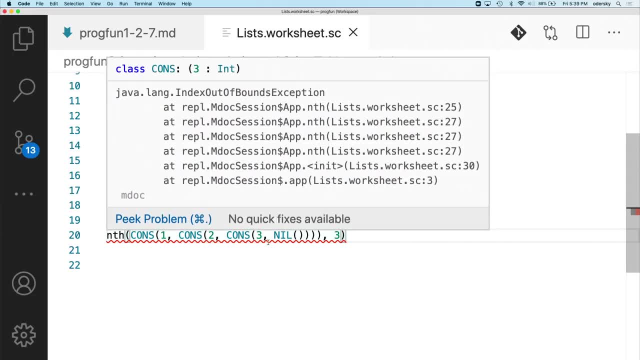 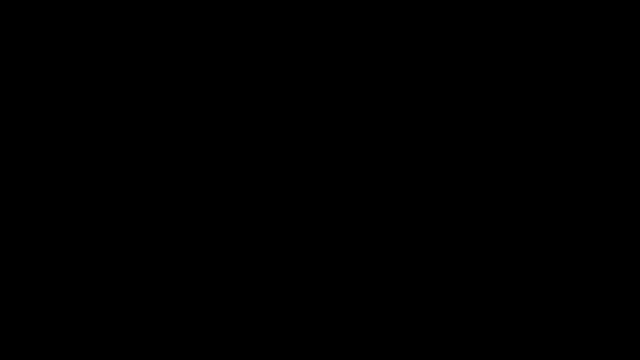 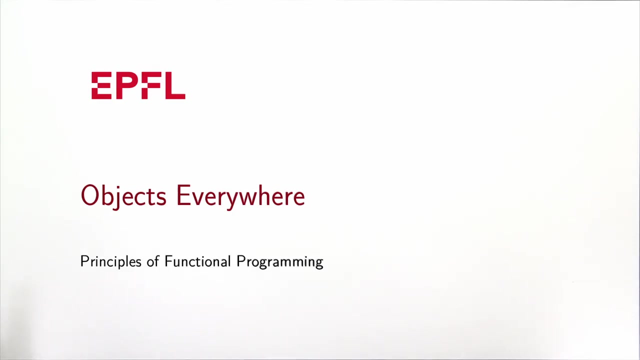 if we put in three here, then we get a red underscore twiggle and it says that there was an index out of bounds exception. as expected, as we have implemented in the nth method that you saw, This section is titled Objects- Everywhere The topic of the section is: 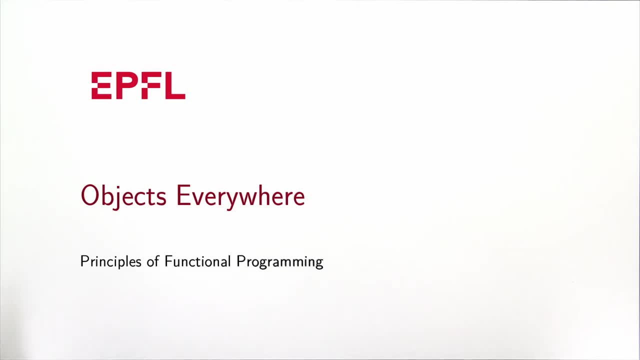 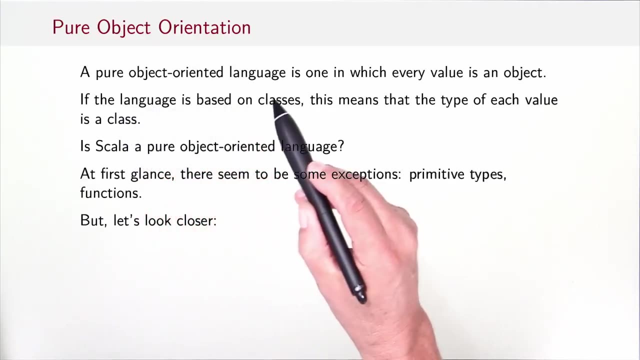 that this model that values are objects and operations are methods can really be applied quite universally in Scala. So we say: a pure object oriented language is one in which every value is an object. If the language has classes, this means the type of each value is a class. 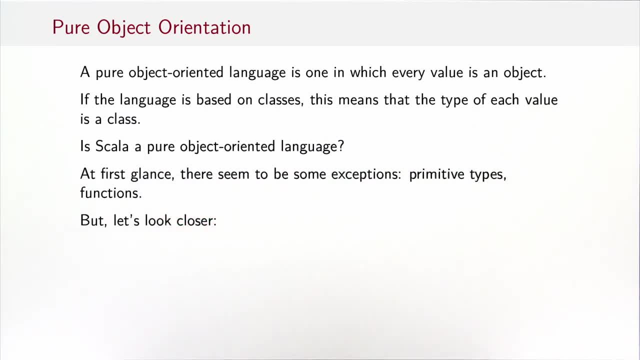 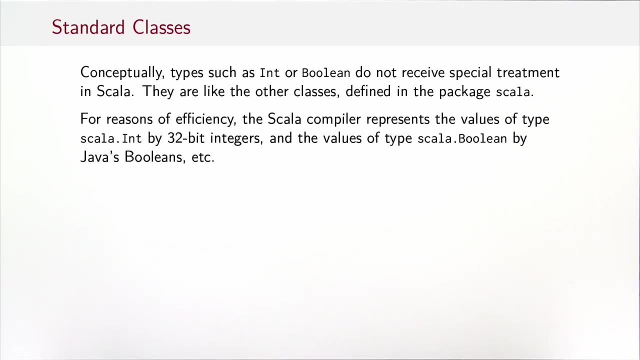 Is Scala a pure object oriented language At first class? there seem to be some exceptions. For instance we saw primitive types or function types. But let's take a closer look. A class such as int or boolean is represented by the computer quite differently from an object. An object is: 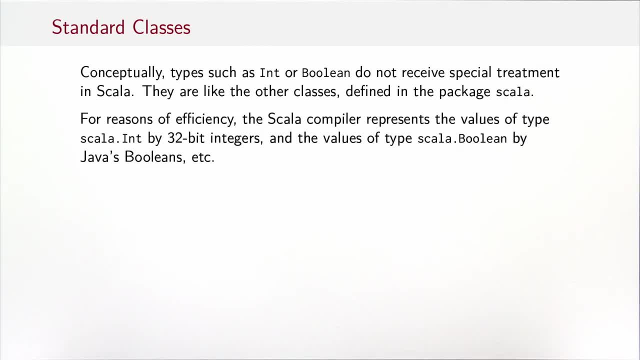 typically a multi word record on the heap and an integer on boolean is just a primitive value that can sit in a register Conceptually. types such as int or boolean don't receive any special treatment in Scala, Just like the other classes defined in package Scala. 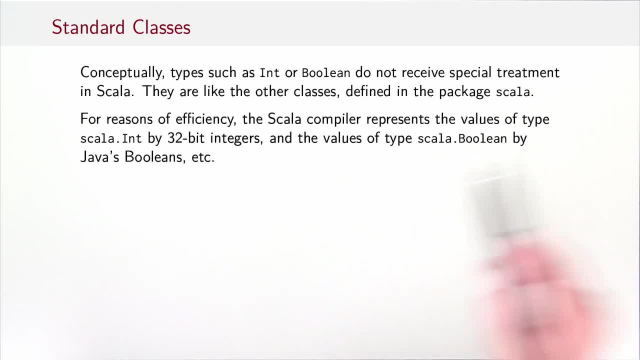 It's true that, for reasons of efficiency, the Scala compiler represents values of type Scala int by 32 bit integers and values of type Scala booleans by Java's booleans, and so on, Whereas a normal object would be represented as some form of record with multiple fields in the heap. 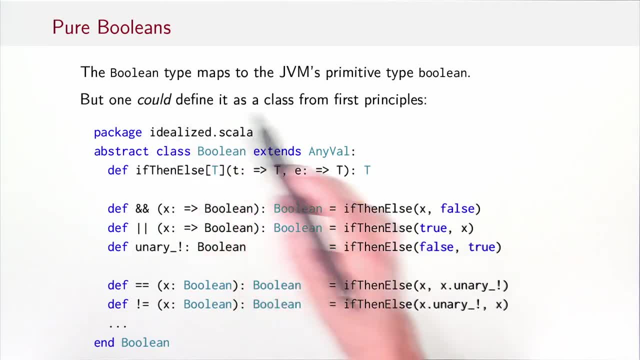 of the program execution, So for efficiency. the boolean type maps to the JVM's primitive type boolean, But conceptually one could define it as a class from first principles. Here's a way to do it. Let's say we are in a package, idealized Scala, We define 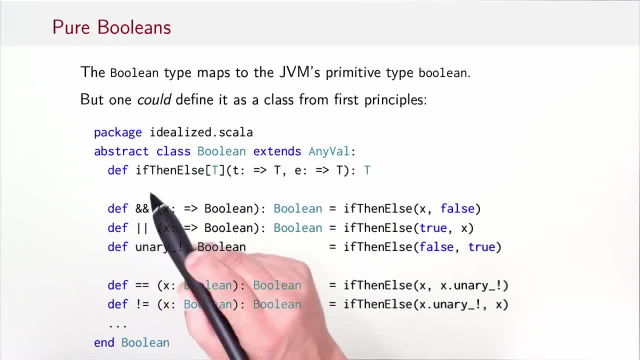 an abstract class boolean that has a single abstract method called if-then-else. If-then-else resembles an if expression. It takes two parts, a then part and an else part, which are both by name parameters and their type is arbitrary. 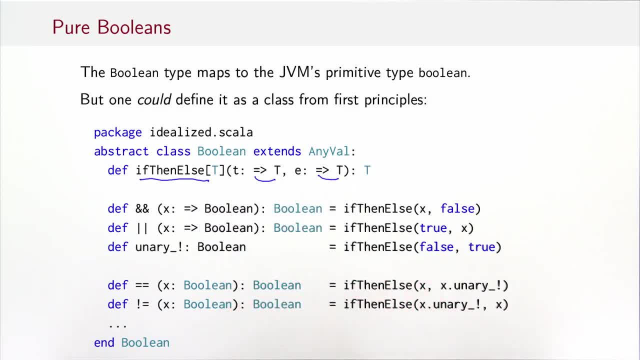 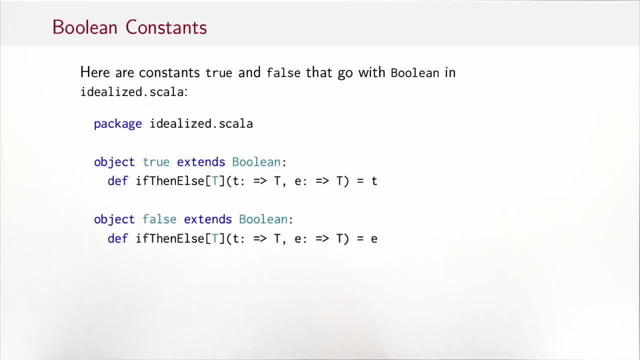 So if-then-else takes a type, parameter t, which is the type of the then part and the else part. So we'll get to the other operation shortly. Let's skip ahead and see how if-then-else would be implemented. So the type. 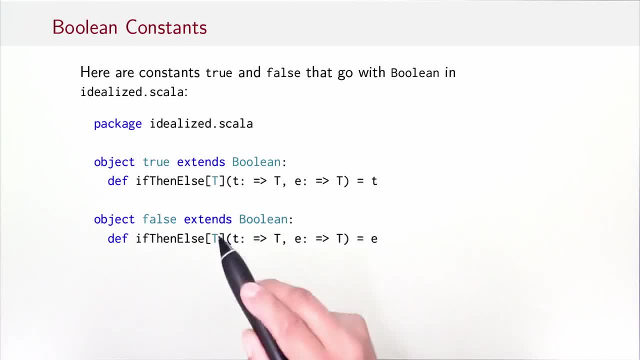 boolean would have two concrete objects, true and false, that both extend boolean, And for true, if-then-else is implemented to always pick the then part, and for false, the if-then-else would be implemented to always pick the else part. So what we would have as 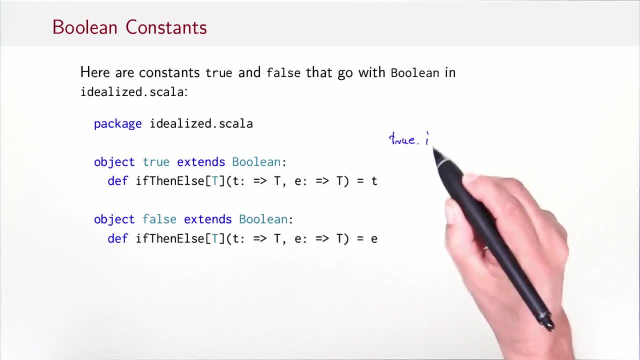 expressions is if we write true dot, if-then-else a, b, that always gives a, And false if-then-else a, b always would give b. So what you see is this if-then-else method is really the same thing as writing if true. 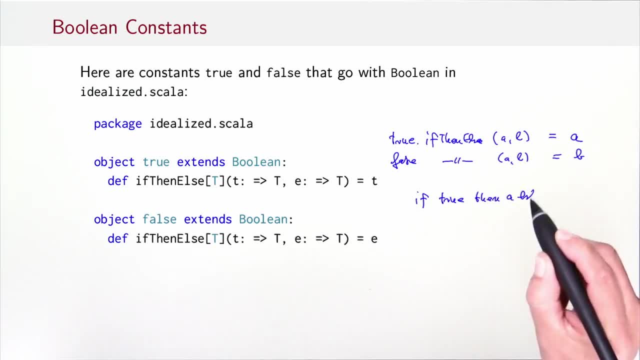 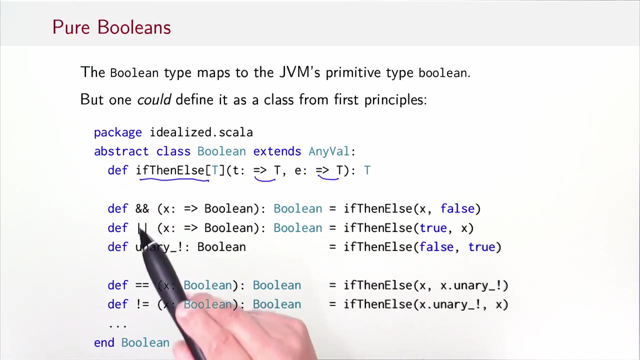 then a else b. That's what it encodes. Okay, so now that we've seen how if-then-else is implemented, let's see how we can put it to use. I go back to the previous slide, So the definition of the. 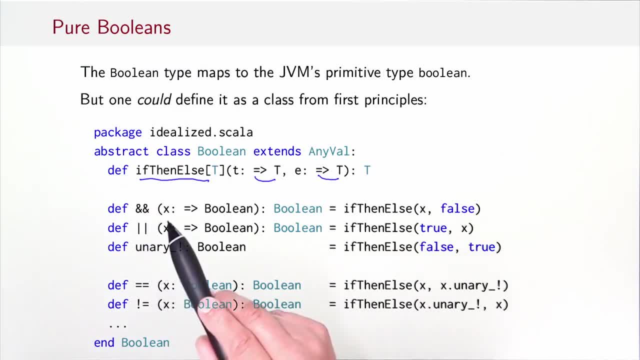 and method on booleans would then be: and takes a by name parameter x, and it returns if-then-else x- false. So let's see how this would work. So if we have true and let's say false, So that's the same thing. 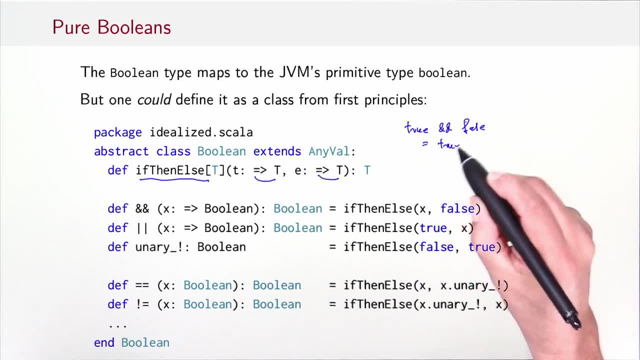 as the and method applied on the true object. That's just what the infix operator and and means. And then, if you look it up, then the- that would be true dot, if-then-else abbreviated like this: false, false. and that would be false because 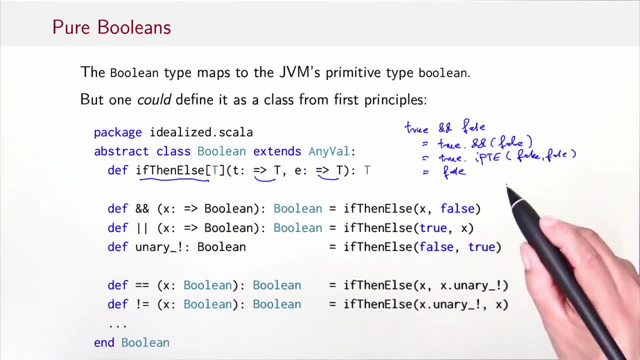 either operand is false. On the other hand, if we do true and true, that would be true. dot if-then-else true, false and that would be true because if-then-else on true picks the first argument. So that's okay, You can write. 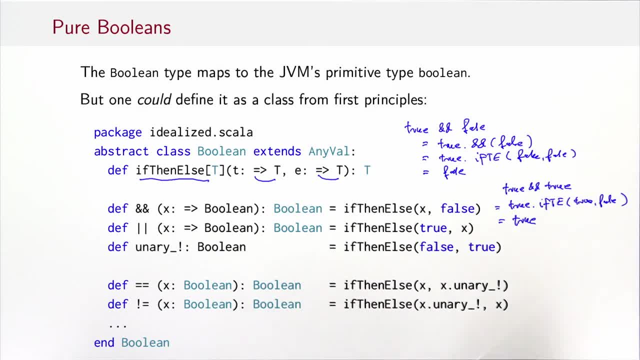 by hand yourself. The case is false and false and false and true, and you will find out that the answer is always the right one. Similarly, the or operation would then, if-then-else true and x- The negation would be if-then-else false and true. 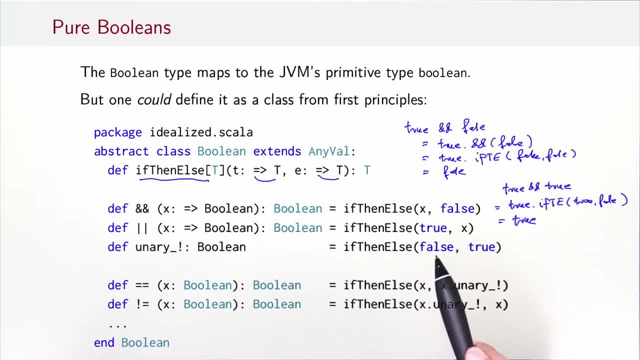 So that means if the boolean in question is true, then it returns false. If it's false, it returns true. So equals and not equals can also be defined in if-then-else, and here you find the definitions. I invite you to try that out for yourself. 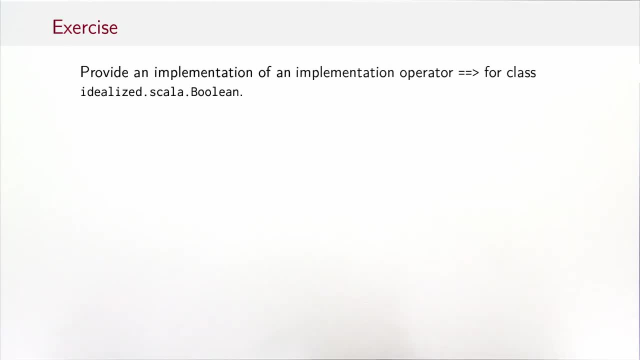 that you get the right values each time. So here is an exercise. Provide an implementation of an implementation operator for class idealized scalar boolean. So the implementation should be true if A implies B. So A is either false or B is true. So let's see what that. 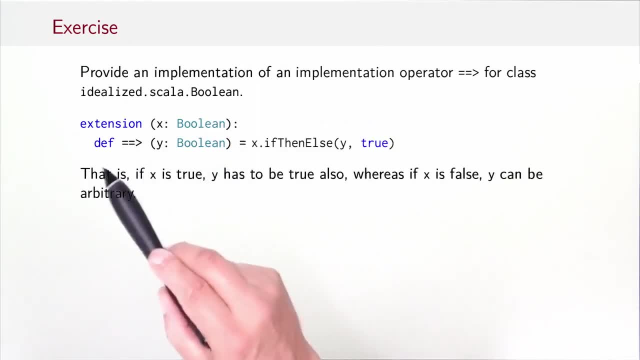 would look like. So we can define it as an extension method. def: equals, equals- arrow between two booleans and that would say if-then-else y true. So if A is false, then we return the second part. That's true If A or x. 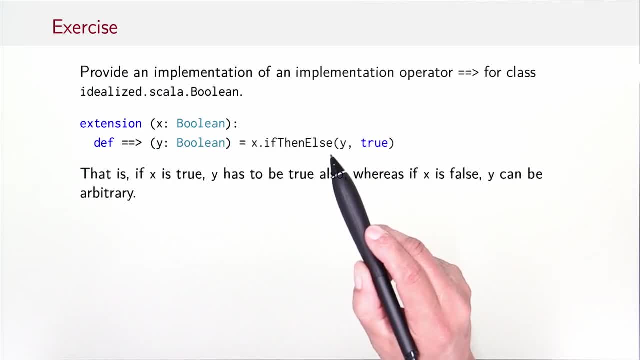 here is true, then y must be true also. So we return the first part. Okay, So you can see that you can define any operation on booleans by instantiating if-then-else in the right way, where if-then-else is really just. 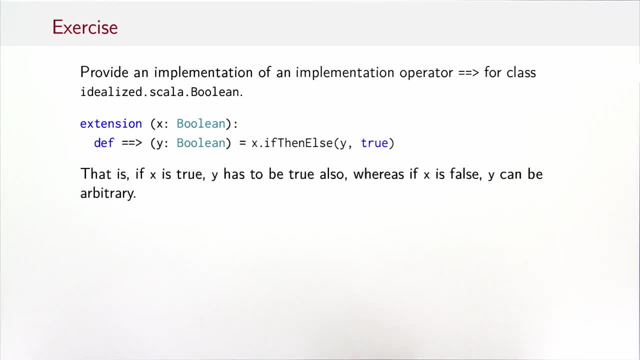 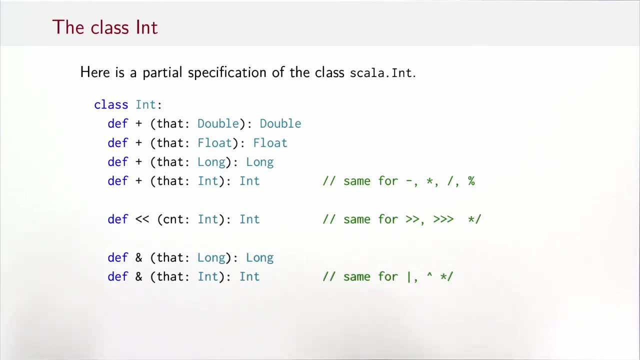 a proxy for the if-then-else expression that you have with boolean conditions. So boolean was a simple class because it had only two possible values, But we can do similar techniques for other classes. So here's a partial specification of the class scalaint. So int would: 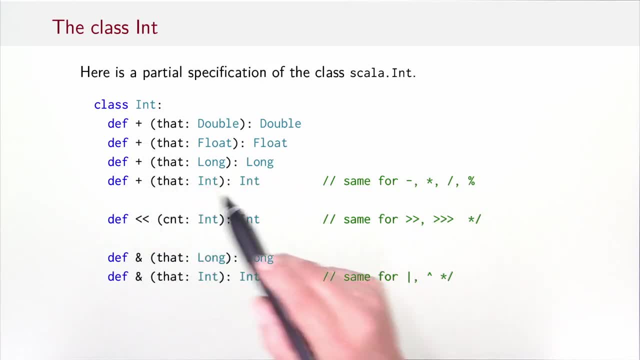 have methods plus that take an int and an int and give you back an int. but you can have several overloaded variants of such methods, so you can also add an int to a long giving a long, or add an int to a double- giving a double. Then you have shift operators. you 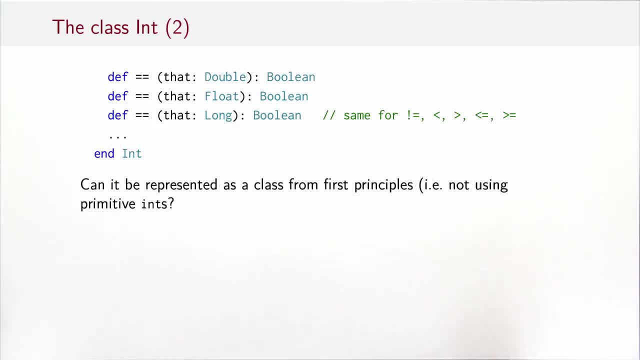 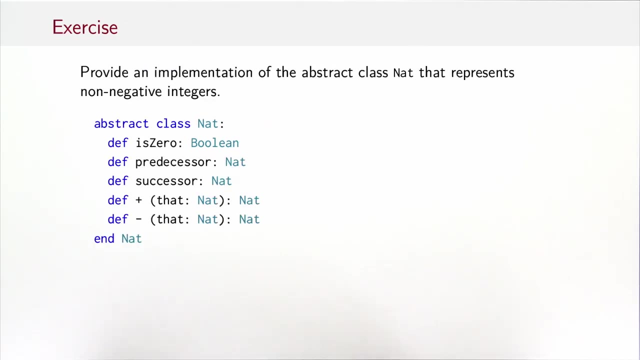 have bit mask operators and so on. So you have a whole set of these operators that can all be defined as methods. on class int Question, Can this class int be represented as a class from first principles? That means not using primitive ints To answer this. 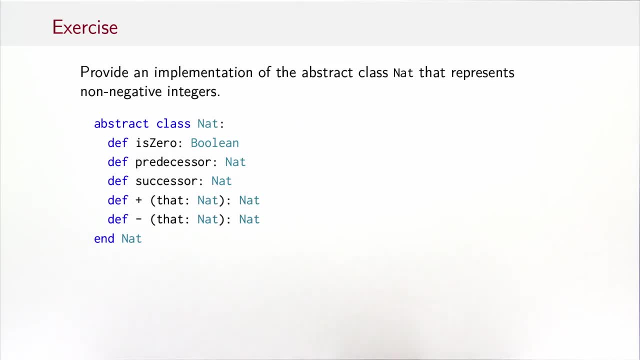 question. it's better to look at a slightly simplified version. We look at a class nat for just natural numbers. That means numbers that are non-zero, And we reduce the set of operations that we look at. We want essentially just those five operations. an is zero operation that. 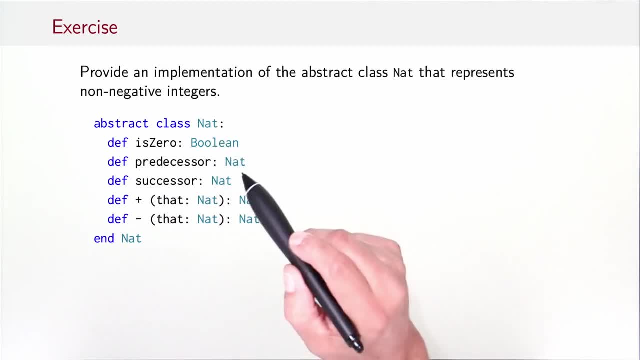 returns whether the natural number is zero, The predecessor of the natural number. in case it is not zero, it can throw an exception for zero, The successor of the number which gives the next higher number. and then we want to implement addition and subtraction on those natural numbers And we 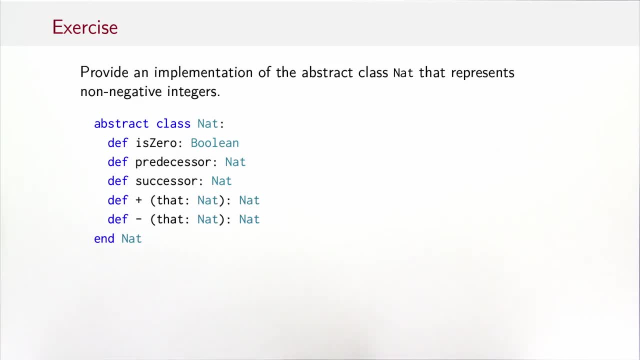 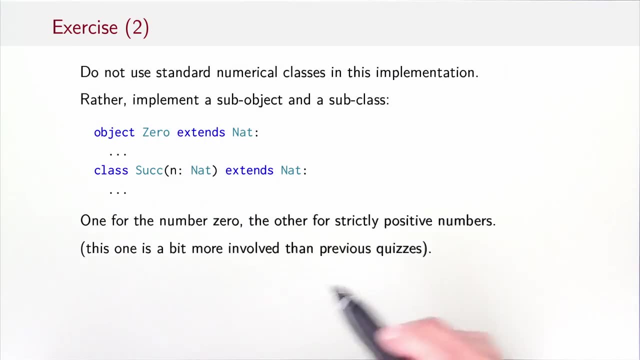 should do that from first principles, without referring to class int or any of the other primitive number types. So what we want to do instead is we want to have an object zero, which is a sub object of class nat, And we want to have a class successor. 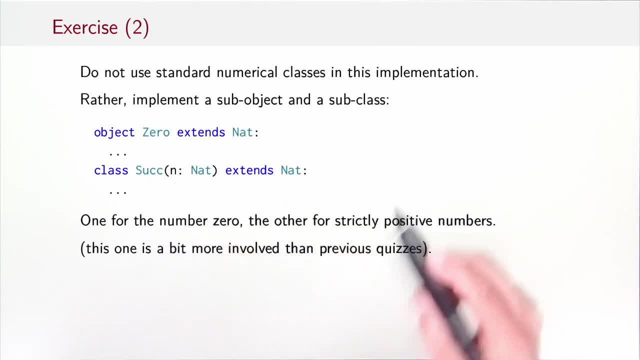 of n. that is another subclass. So successor of n would be the instance that represents n, plus one for any number, n. So this is an open ended puzzle for you. It's quite a bit more involved than the previous quizzes, But it's quite illuminating if you manage to. 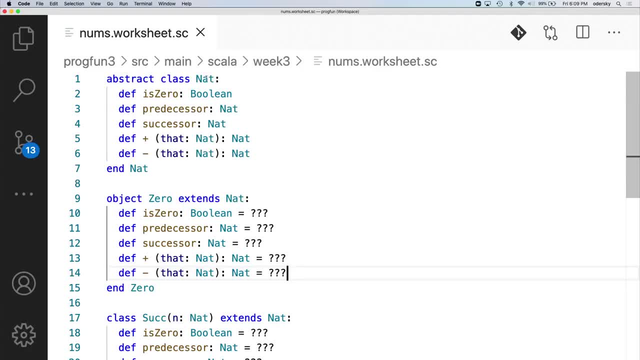 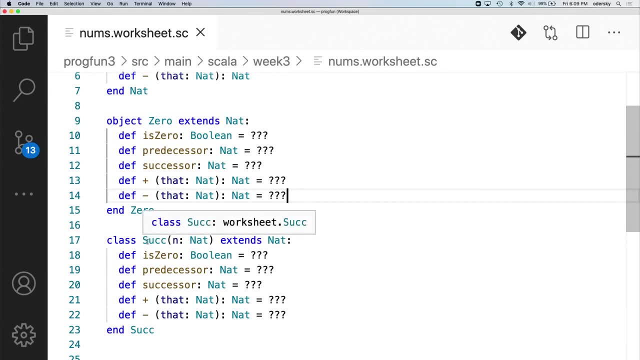 solve it. So I've given the class hierarchy as specified in a worksheet. We have the abstract class nat with the five methods to implement, And then we have the sub object zero and the subclass successor, And I've already added the method definitions. but 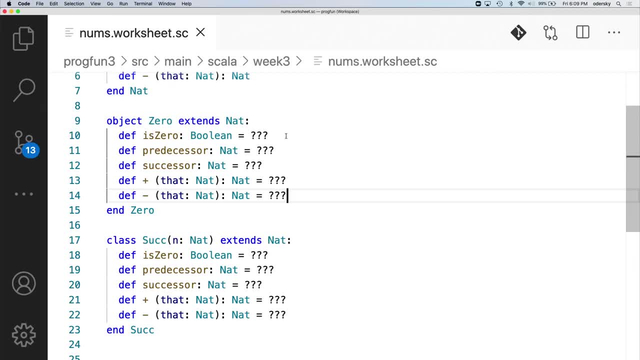 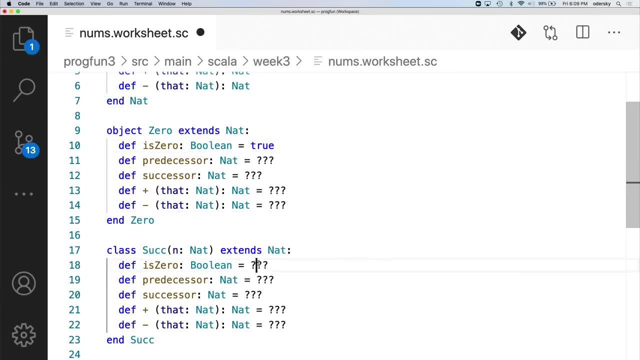 the method bodies are all the triple question mark, which means they still need to be implemented. So let's start with: is zero Is zero for a natural number? well, if the natural number is zero, then obviously zero is true, And for the successor it would be. 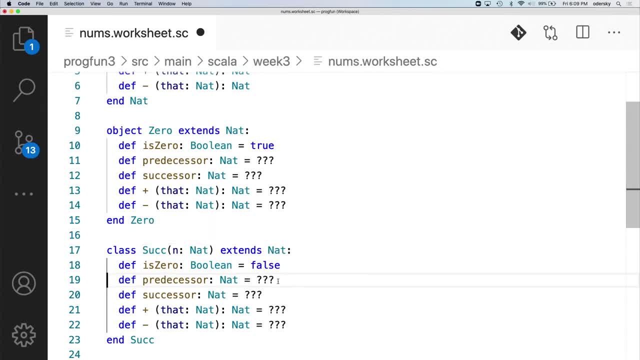 false. What about predecessor? Predecessor is defined only for successors. We don't know what it is for zeros. So for the successor object it would be n. That means the number from which we took the successor, that's the predecessor of that. 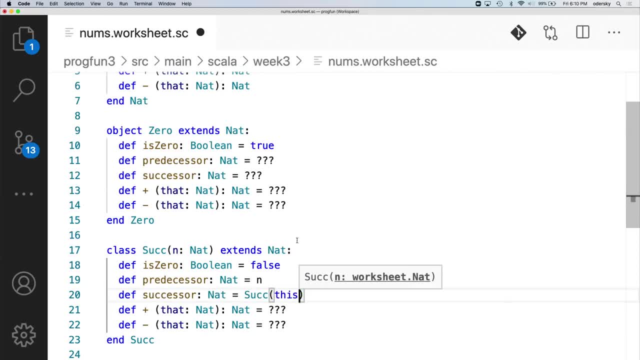 number. What about successor? So successor of a number would be simply, we wrap it in successor, So the successor of this number is successor of this and the successor of zero is also literally successor of zero. Or we can write this, because this in this: 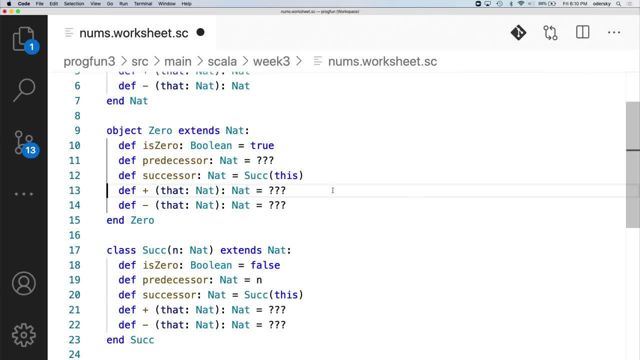 case is zero. What about plus? To add a zero and any other natural number that? so the result would obviously be that: What about adding a successor to a number that? So here the idea is we can say: well, that's the successor of n plus. 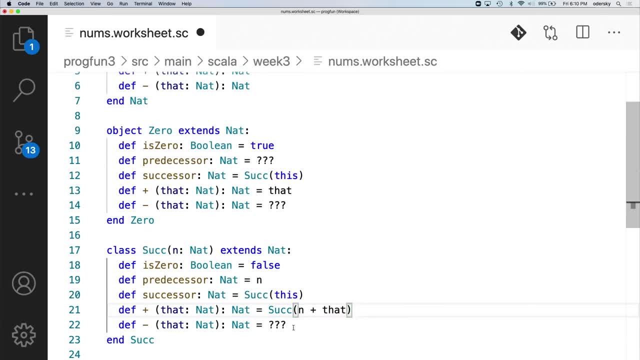 that. So we take the addition on the number which is one smaller and we form the successor. That's the same thing. So that leaves subtraction. Subtraction on a zero number. that would be defined only if the that number is in fact zero as well, because otherwise 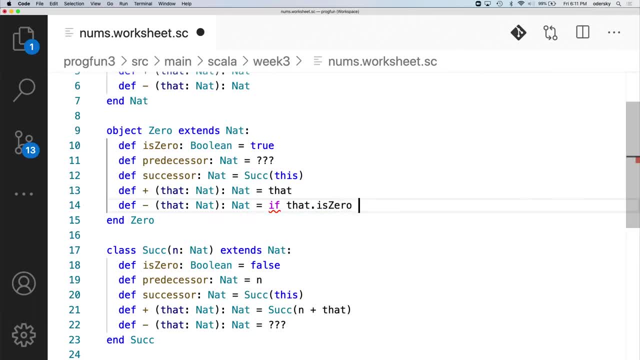 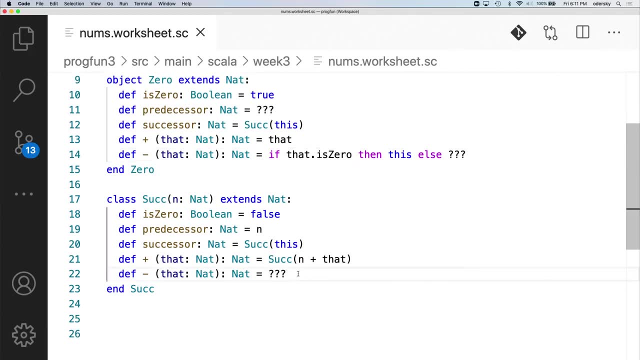 we would go in the negatives, which cannot be represented as natural numbers, So let's write that. So again, I've left the case where the number is not zero open with triple question marks, meaning that I don't really know what to do there For successor. 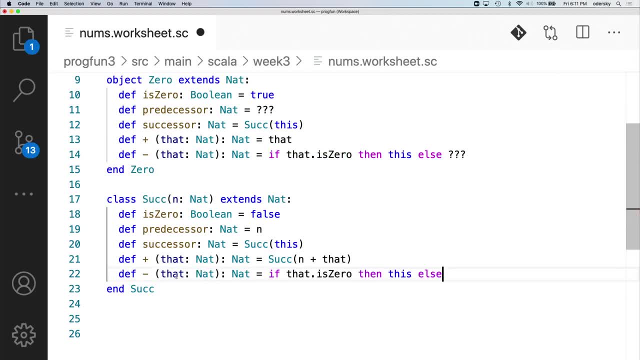 what do I do for successor? So I start off in the same way. So if the other number is zero, then this number minus zero is this number. That's fine, And otherwise what do I do? So otherwise, I take the predecessor n and I subtract. 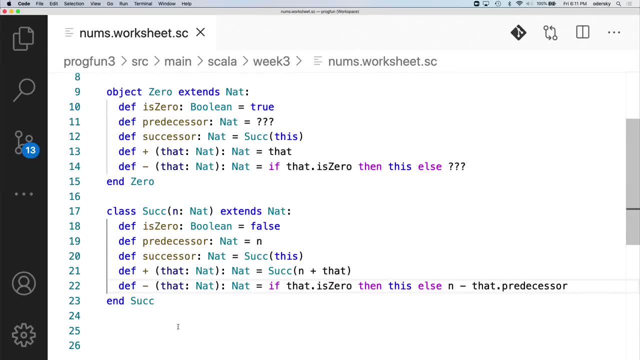 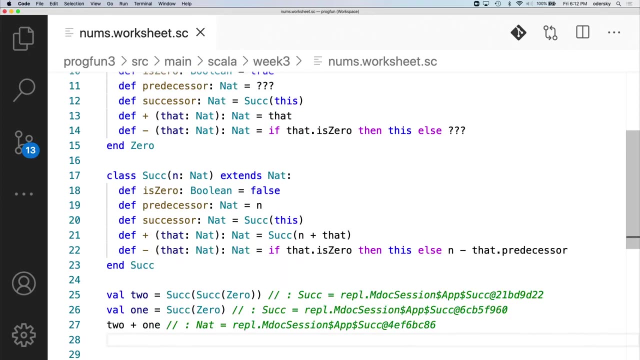 from it the predecessor of nat, And that's it. So we can already test the worksheet. So let's define natural numbers. So I defined one and two. Let's add them. Ah, we don't really see much. so what's missing here is: 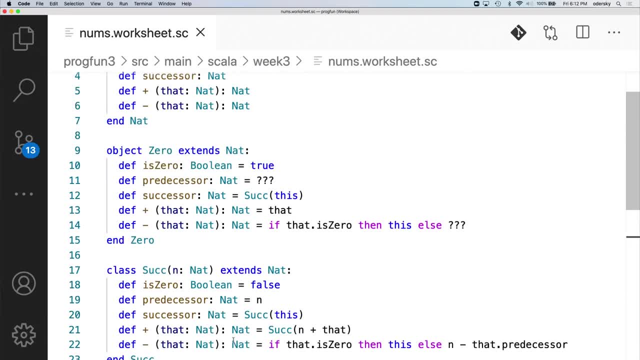 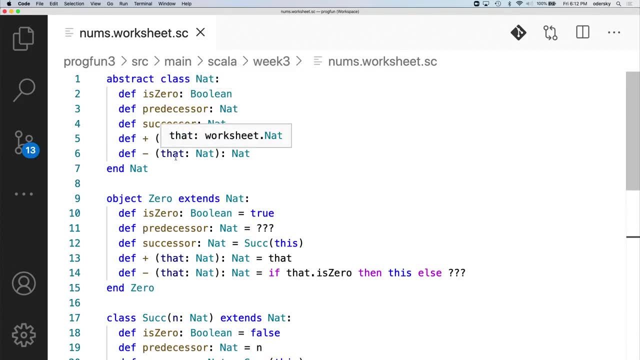 we need to add a two string method so that we can actually make sense of these things. So let's add this method as a sixth method. We don't need to add it here, because two string is already implemented in object anyway, So we just have to override it. 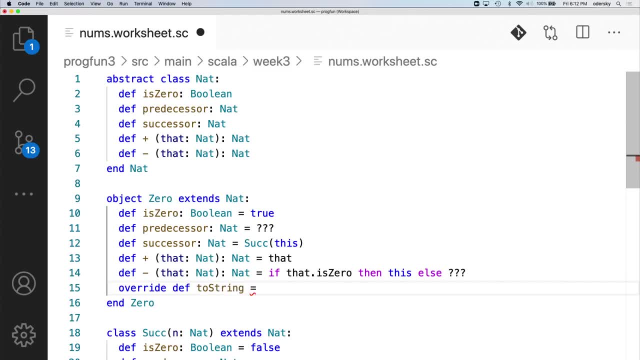 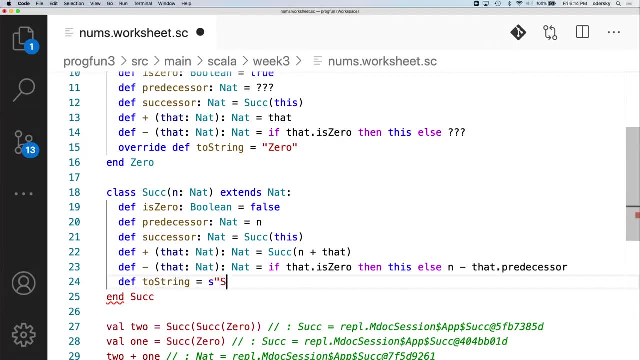 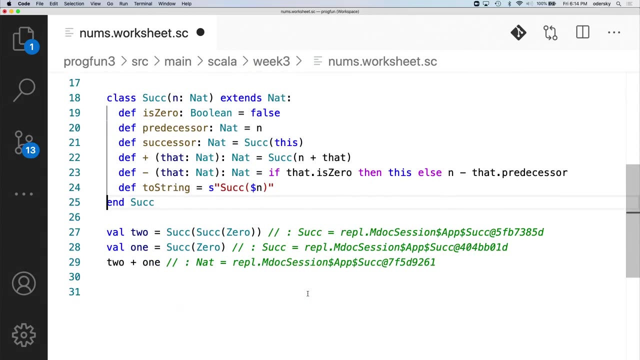 in the two implementations here. So for zero the two string would say zero And for successor I can define two string like this, So I literally write successor and then recursively the two string of the predecessor number. So if I do that, Oh I. 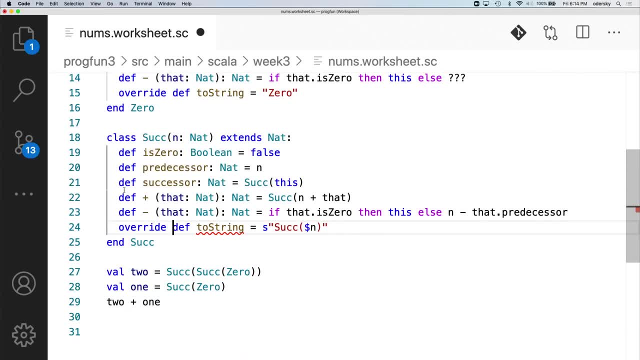 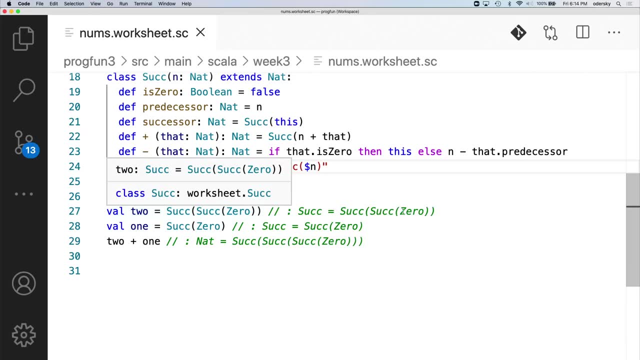 get an error because I forgot the override. Yes, Two string needs an override, because we've seen that they are already implemented in objects. So now I get something that is more reasonable. I get here the same things that I have defined, and two plus one. 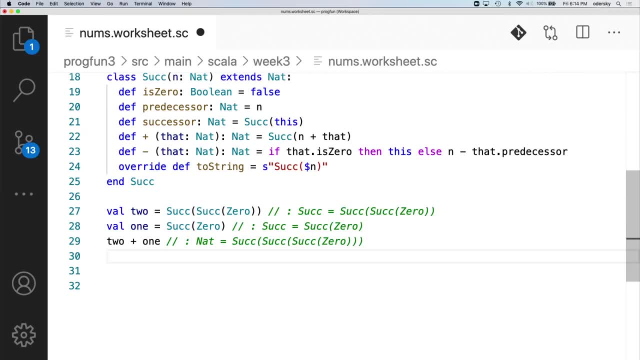 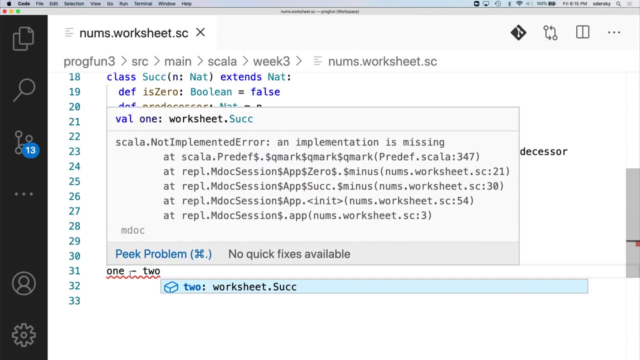 is three? No big surprise. So what do we do with, let's say, two minus one? Just look at that. So that would be one Also, fine, What would we get for one minus two? And that's an error. So what we would get is a not implemented. 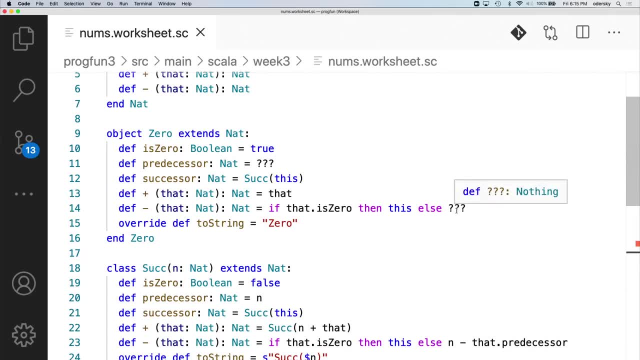 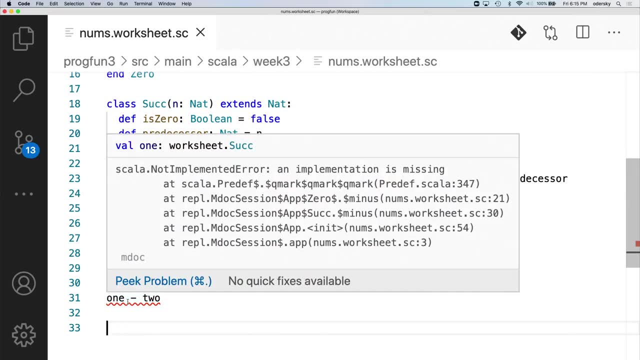 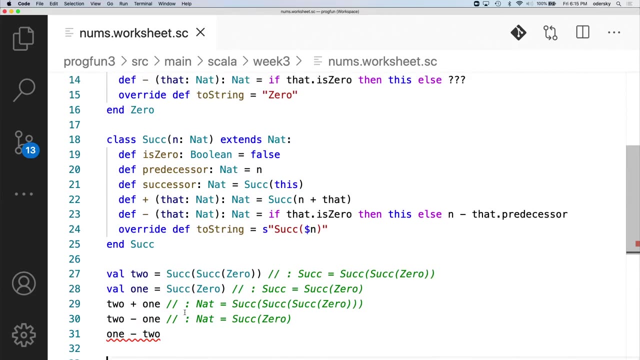 error, An implementation is missing, In fact, the things that we have left open, this triple question mark is a predefined operation scalar which gives you an exception called a not implemented error. So that's a good approximation if you don't want to be bothered defining your own exceptions, which 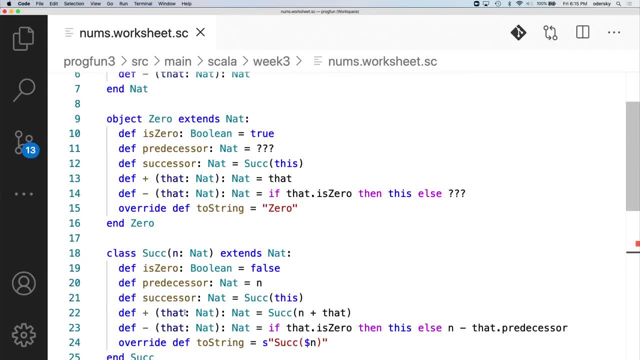 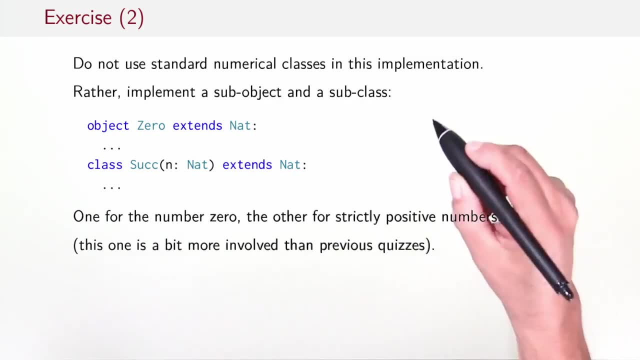 in this case is not really relevant for the project, for the problem at hand. So we've seen how to construct natural numbers from just three classes: A base class, NAT, and then an object zero and a subclass successor. In fact, that's a well known 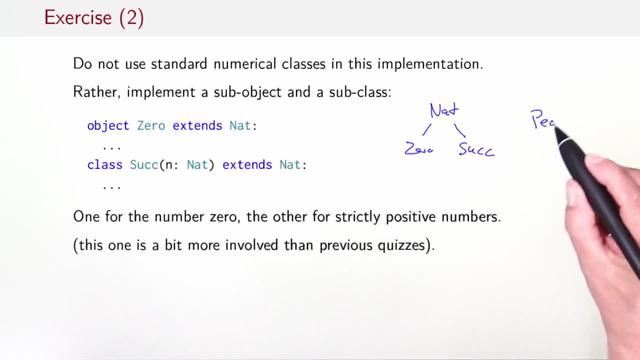 concept. in mathematics, These numbers are called Piano numbers after the Italian logician Giuseppe Piano. And it doesn't stop there. You could now also add multiplication, division or other operations to natural numbers, and you can then extend the concept to more complicated number types. 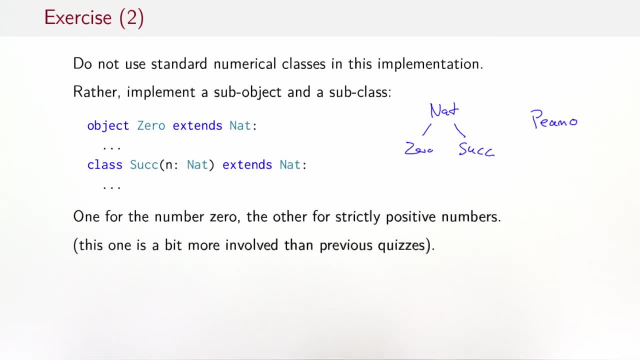 such as integers or rational numbers or any other kind of numbers, or really any other kind of data structures. In fact, it's possible to build up the whole of computable mathematics on just this simple basis. Efficiency is another matter, of course. These piano numbers in the implementation. 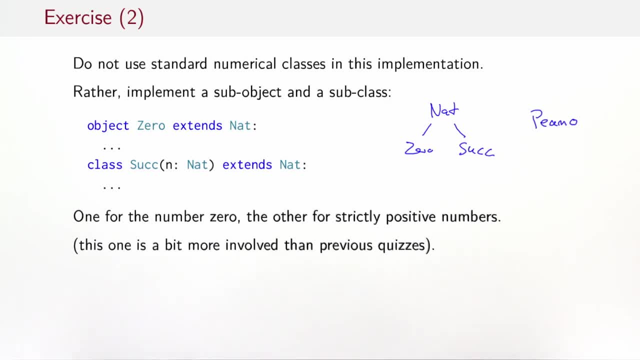 that we've given are notoriously inefficient, because even a simple addition would be linear in the size of the numbers. So the bigger your numbers are, the longer you have to hunt down a chain of successors. So while these things are quite beautiful in their simplicity, they're far from an efficient 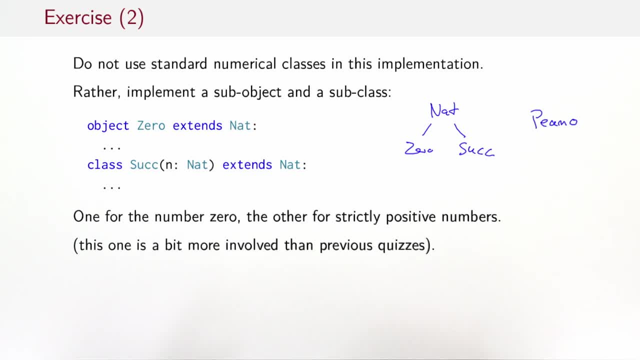 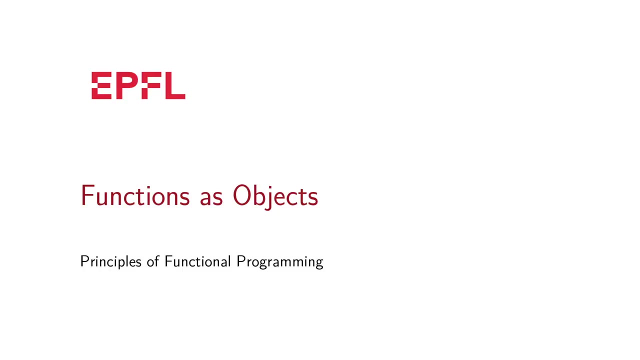 implementation. But that's not a problem. We can very well keep apart the abstract concepts and the actual implementation. One should be simple and elegant, and the other should be efficient and fast. In this session we're going to take a closer look at the relationship between functions and 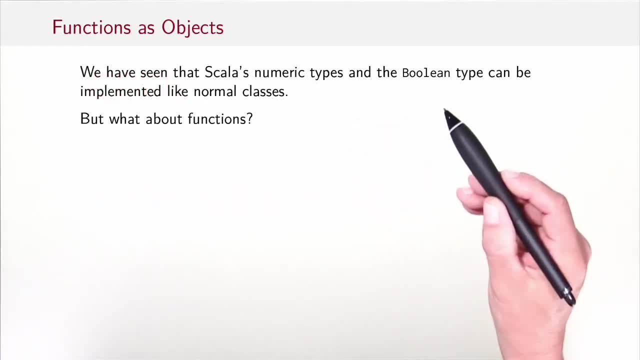 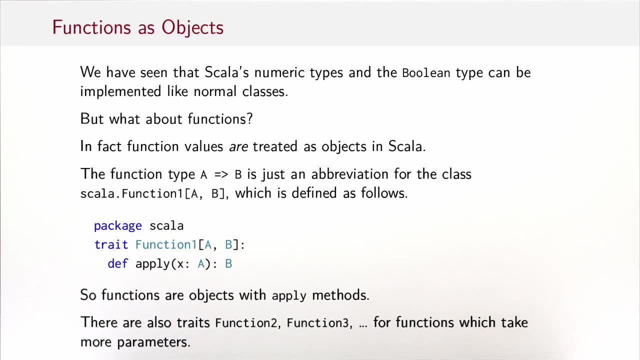 objects. We've seen that scalar types and the Boolean type can be implemented like normal classes. But what about functions? In fact, function values are treated as objects in Scala. The function type is just an abbreviation for the class type ScalaFunction1, where the class ScalaFunction1 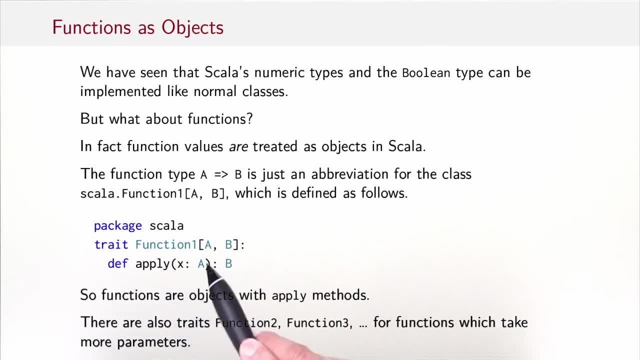 is defined as you see here. It's a trait, It has two type parameters and it has as only member an apply method that takes an a and returns a b. So functions are objects with apply methods. There are also traits: function2, function3. 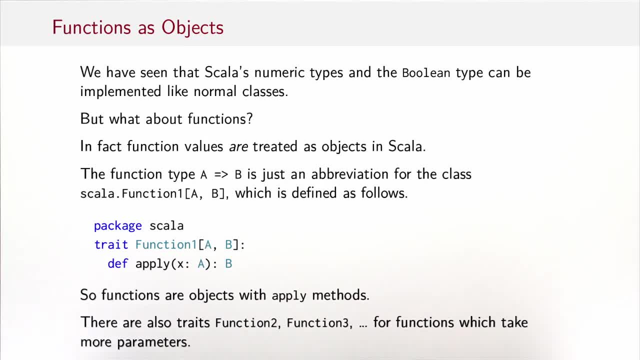 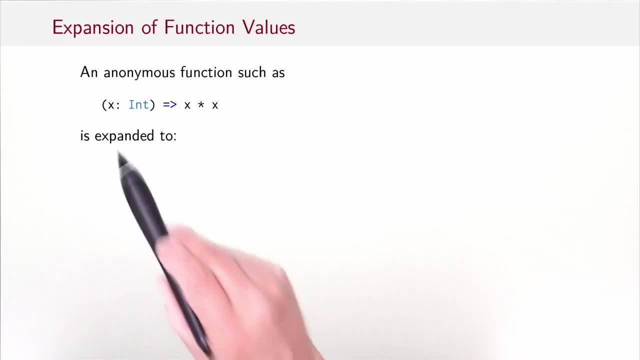 and so on, for functions which take more than one parameter. So much for function types. What about function values? Well, the classical function value is an anonymous function like the one you see here. It takes an x and, let's say, it squares the x. 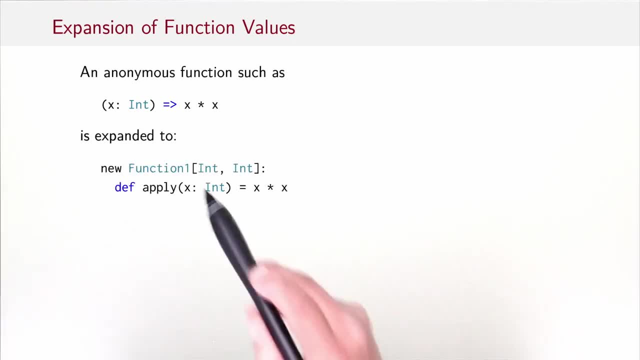 That function value is expanded to what you see here. It's an anonymous class function1 with the type of the parameter and the type of the result type and an implementation of the apply method. In this case, the implementation of the apply method is simply the body of the anonymous function. 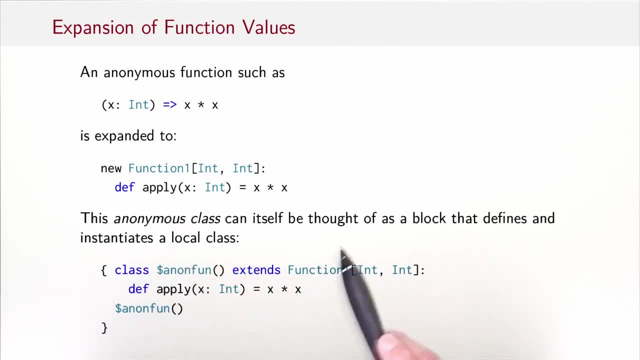 An anonymous class like this can itself be thought of as a block that defines and instantiates a local class. So this syntax here is available for any class. You can have new and then a class name and then some method definitions or some other member definitions. 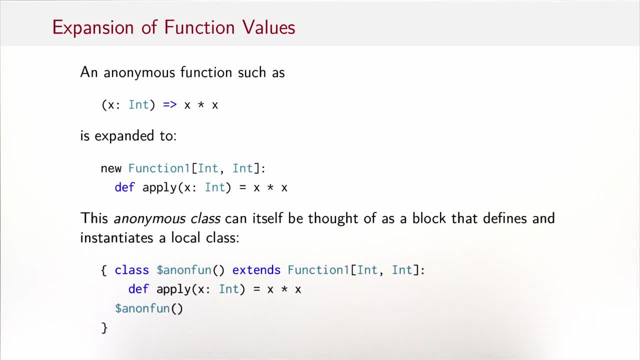 in a block that follows the class name. Such an anonymous class is a shorthand for what you see here. It's a class with a compiler synthesized name. in this case it's $anonfun. It extends what you wrote here. function1 int, int. 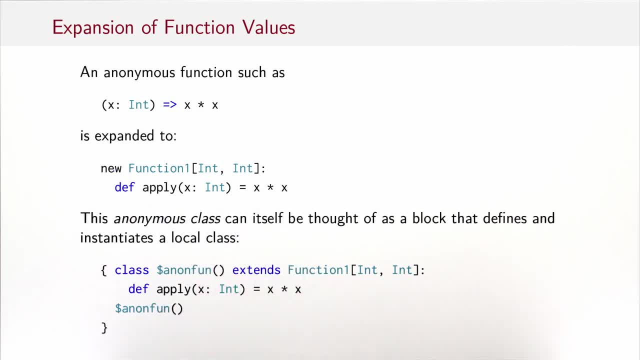 It has the definition that you give in the anonymous class and at the end of the block you just return an instance of that class. So an anonymous class like this one creates a class with a name that is compiler generated and creates an instance of that class, which is the value. 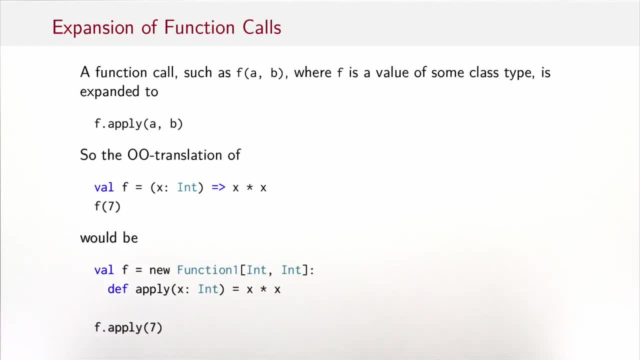 of that expression. Now let's look at function calls. So let's say we have a function called f, where f is a value of some class type, then that call is expanded to fapply. So we're looking for an apply method that we can select from that value. 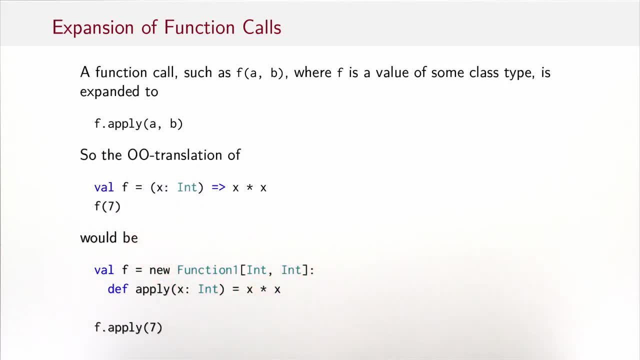 and that will be the method that gets applied to the arguments a- b. So the object-oriented translation of this anonymous function value, followed by this call, would be an anonymous class that you see here, followed by an invocation of the apply method that we have defined here. 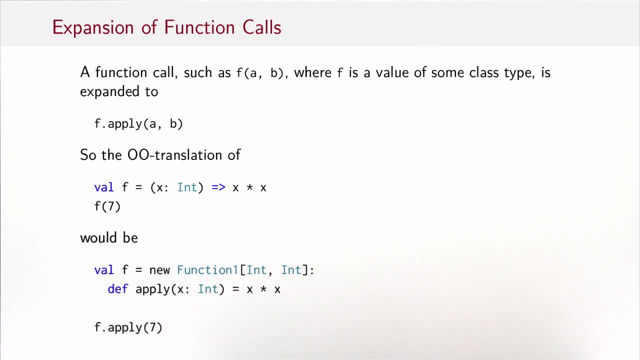 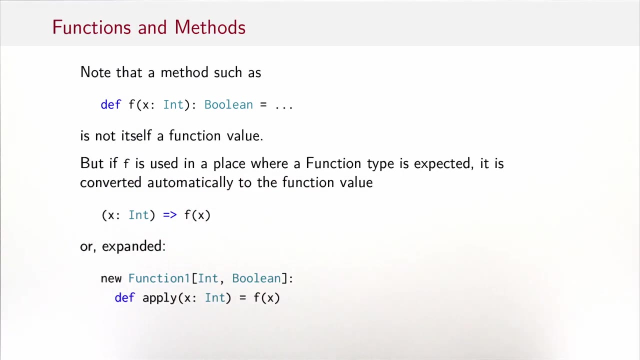 with the given argument. So that means that we can use the same syntax for method calls also in the application of function values. Note that a method that's defined with a def like this, f here- is not itself a function value, but if f is used in a place. 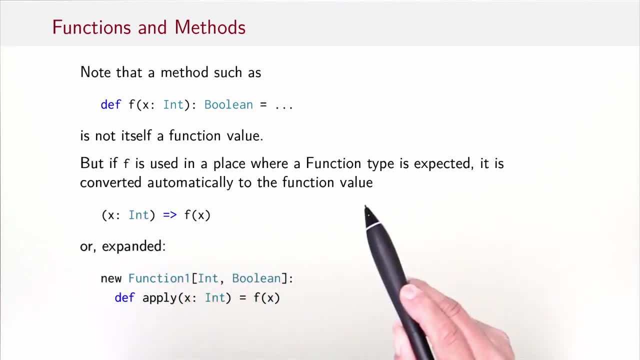 where a function type is expected, it's converted automatically to a function value by converting the f into an anonymous function that takes a parameter as indicated here and applies f to that parameter. So an example where this happens would be the following: So here I've defined a function g. 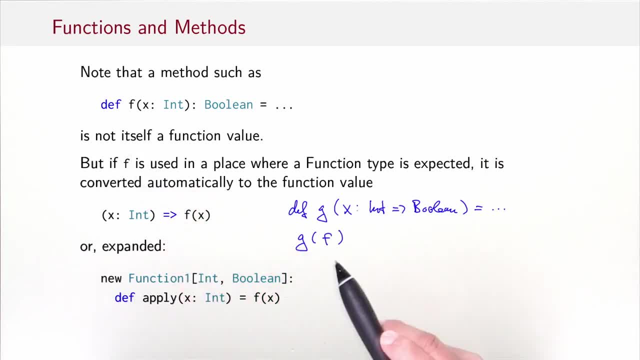 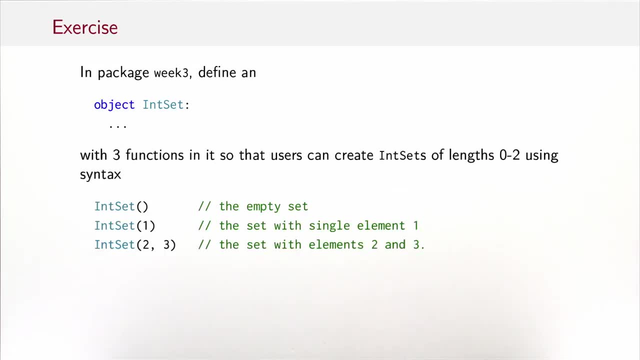 to boolean, and I can pass my method f to g because f can be converted to a value of that type by the conversion that you see here on the left. So let's finish with an exercise in package week 3, where we have defined the inset class hierarchy. 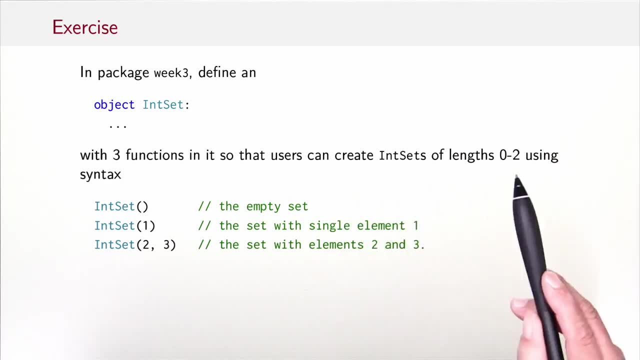 define a companion object inset with three functions, so that users can create insets of lengths 0 to 2 using the syntax that you see here. inset of 1 would create a set with single element 1, and inset 2, 3 would create a set. 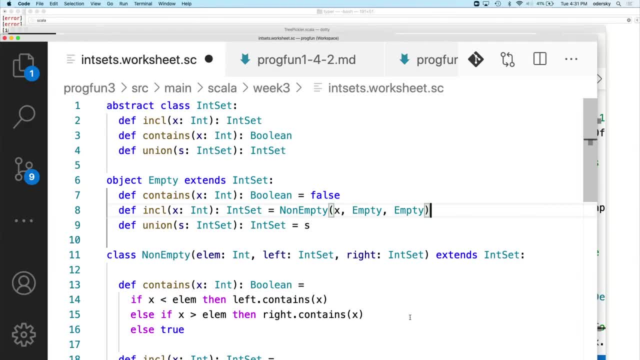 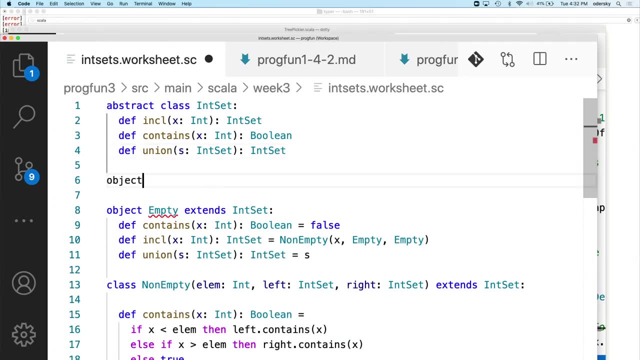 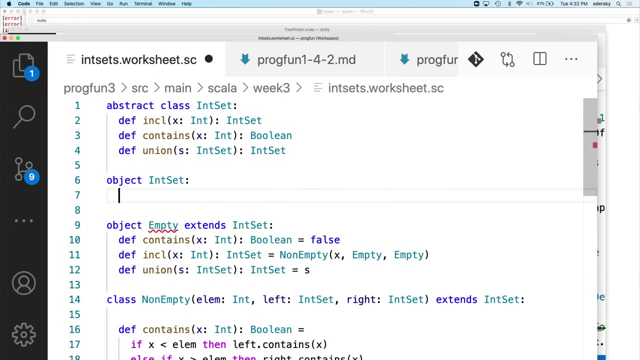 with elements 2 and 3.. So let's see how this would work. So here we have our original inset class and two subclasses. Let's create an object inset and then we need three apply methods. So for the empty set, that's simple. 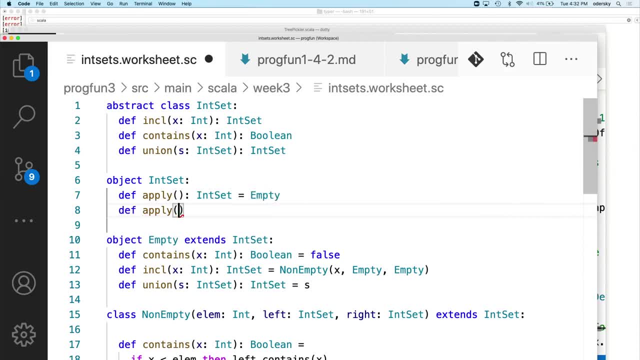 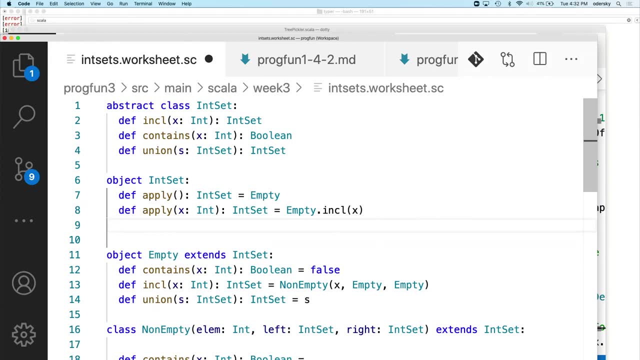 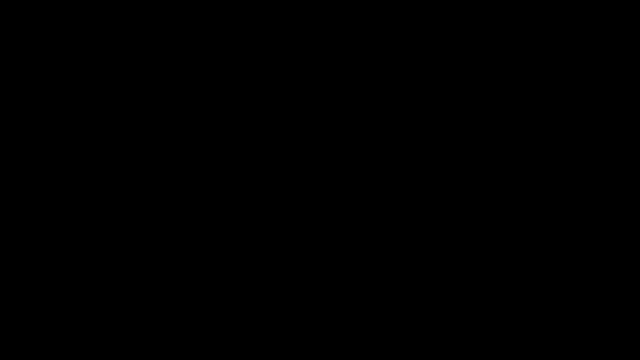 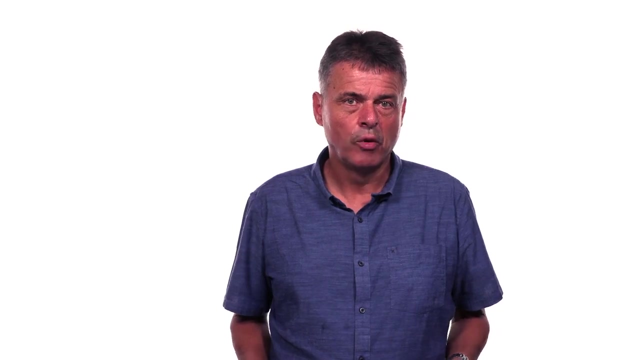 that's an apply method here. for a set with one element, we take the empty set and include x, and analogously, for a set with two elements, we take the empty set and include first x and then y. So far, we were mostly concerned with building up data. 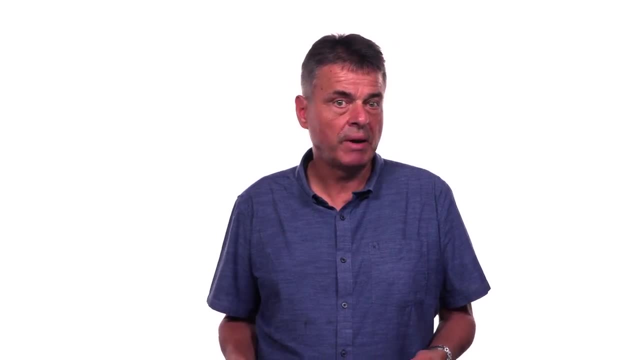 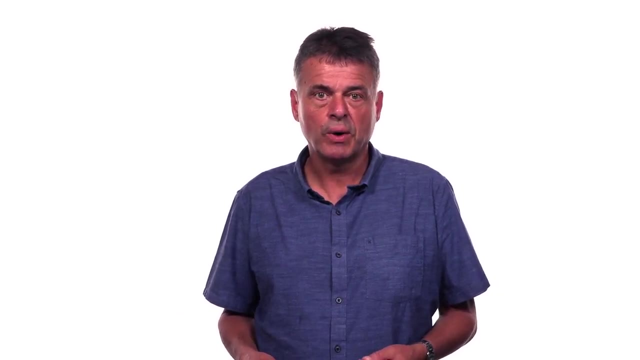 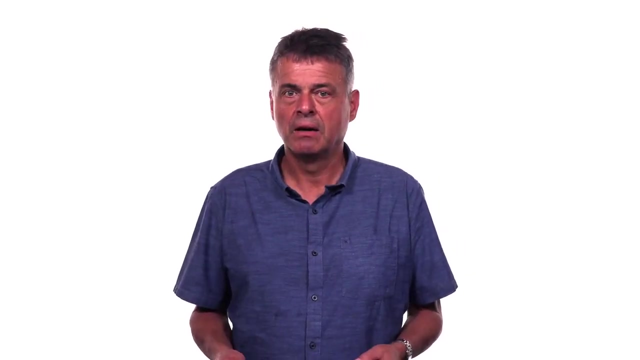 from objects and functions. We have learned that functions can be data values themselves and have seen the relationship between functions and objects. In this week, we'll shift the focus from data construction to data decomposition. If you have some data, what are good ways to find out? 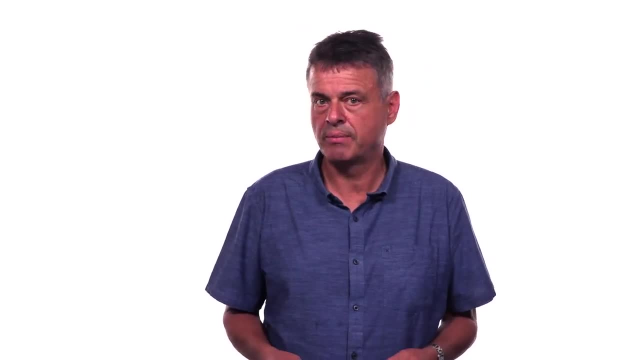 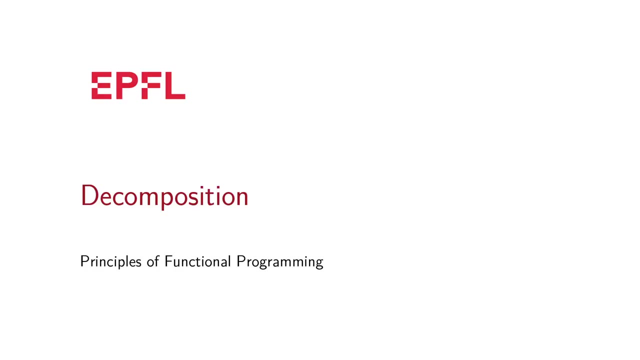 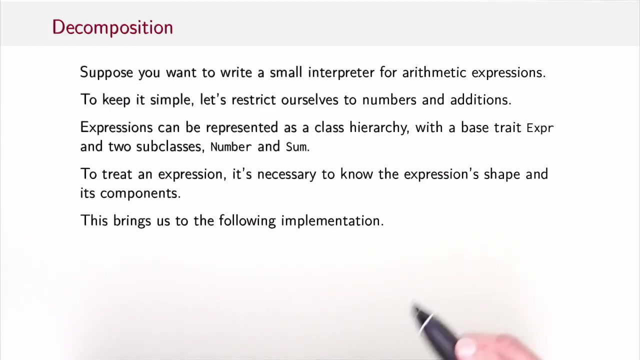 what's in it and to act on that knowledge. In this unit we're going to look at decomposition- how to inspect a value and break it up in smaller parts. For instance, suppose you want to write a small interpreter for arithmetic expressions, To keep it simple, 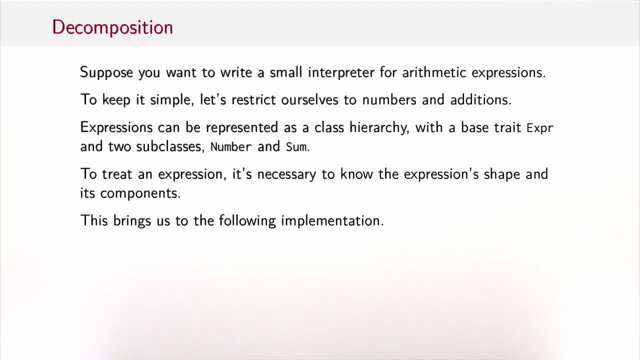 let's restrict ourselves to just numbers and additions. Expressions can be represented in the form of numbers as a class hierarchy with a base trait, expr, and two subclasses, number and sum. So it would look like this: So to treat an expression, it's necessary to know. 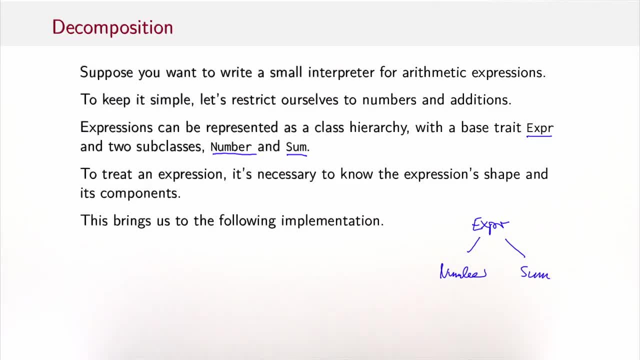 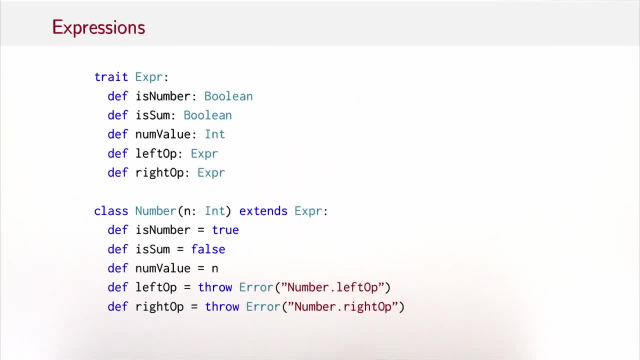 which shape it is and also to access its components. This brings us to the following: object-oriented implementation. Here we see a trait expr with five methods. Two of the methods allow us to find out what kind of expression it is. One is sum and the other three. 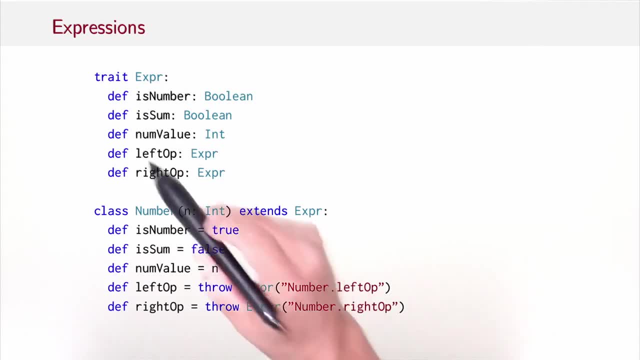 allow us to access the components of the expressions. In case the expression is a number, numValue would pull out its numeric value as an integer. In case it's a sum, leftOp and rightOp would pull out the left and right operands. So these five methods. 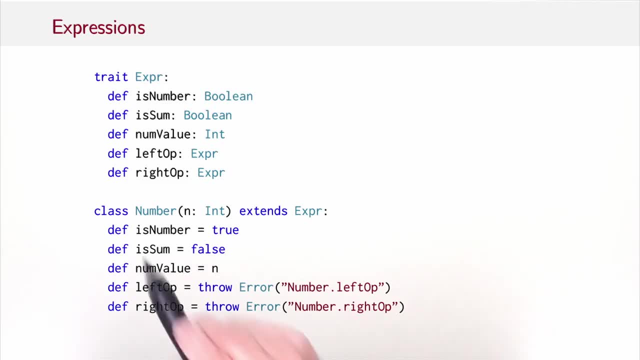 now have to be implemented in the two subclasses of expr. Let's look at class number first. So a number is defined as an expression. It is a number, It's not a sum. Its numeric value is the given integer and its left and right operand. 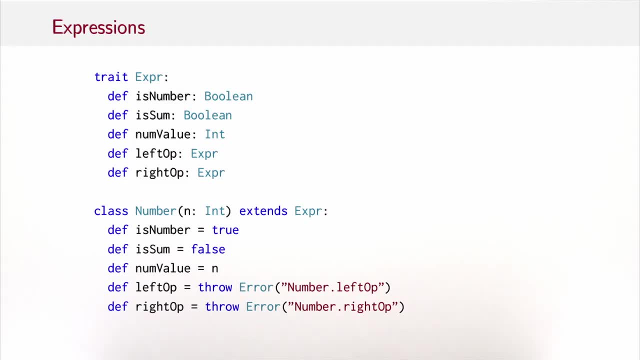 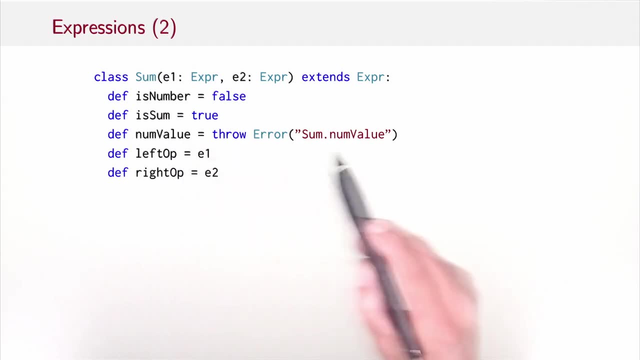 are both undefined, which we model here by throwing an exception. So that would be an illegal call. if the expression is a number For sum, it goes the other way round. so a sum is not a number, but it is a sum. Its numValue would throw an error. 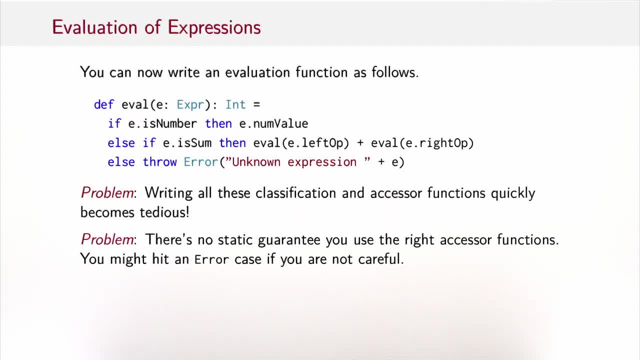 Its left operand would give you the first parameter And then it would operate on expressions. So, for instance, here is an evaluation function that evaluates an expression to the integer number it represents. So we would have defEval: it takes an expression and returns an int. 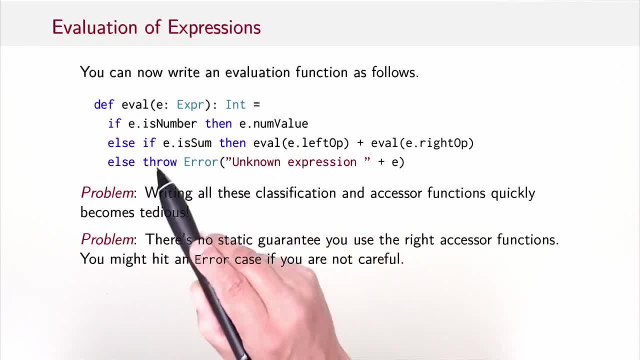 If the expression is a number, then return its numeric value. Otherwise, if it's a sum, then evaluate the left operand, evaluate the right operand and add the two values. And finally, in case we find another subclass of expression, we throw an error with unknown expression. 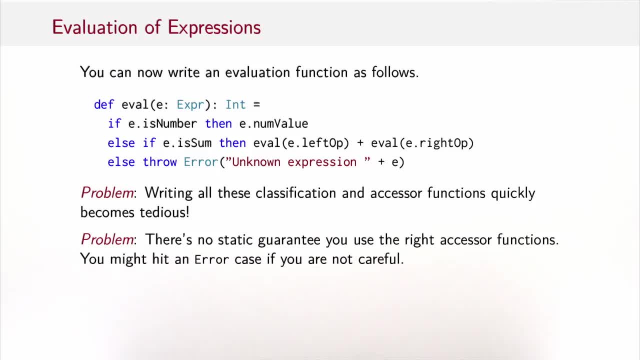 Now that works, but there are also problems. One problem is that writing all these classification and accessor functions quickly becomes tedious. It was already tedious for something as simple as an expression with two subclasses. We will see how much more tedious it gets once we add. 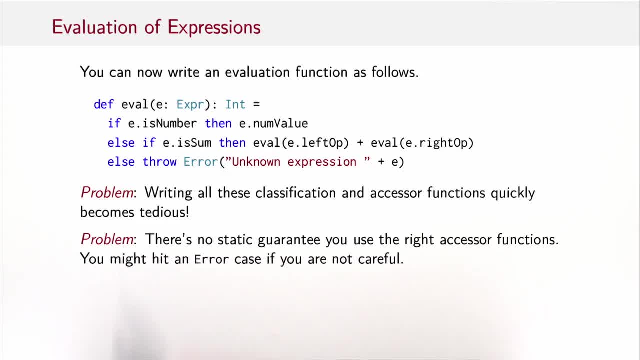 further cases to expressions. And the other problem is it's not really very statically safe. There is no static guarantee that you use the right accessor functions. Many of the functions throw exceptions when they are called, which means you don't have a compile time guarantee. 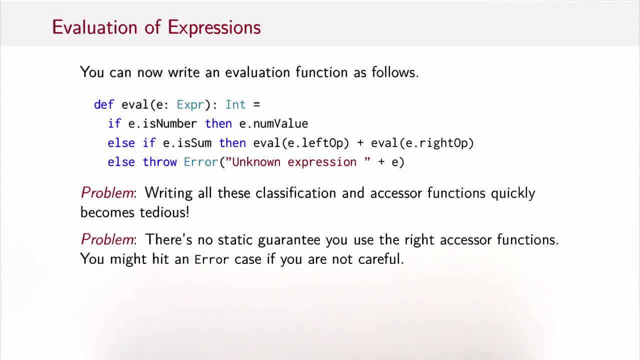 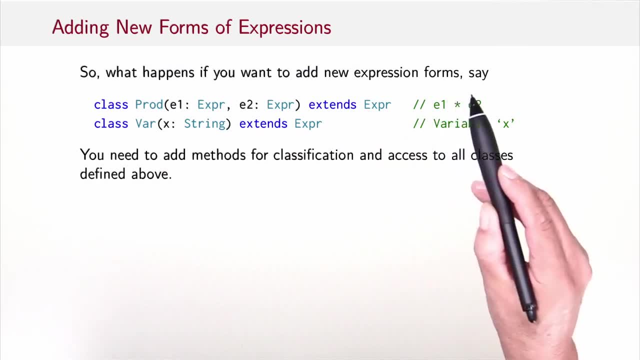 that your program will execute without exceptions being thrown. So to illustrate the first problem, let's study what happens if we add two new expression forms. Say, we want to add a product expression that takes two operands and a variable expression that takes a string and represents a variable. 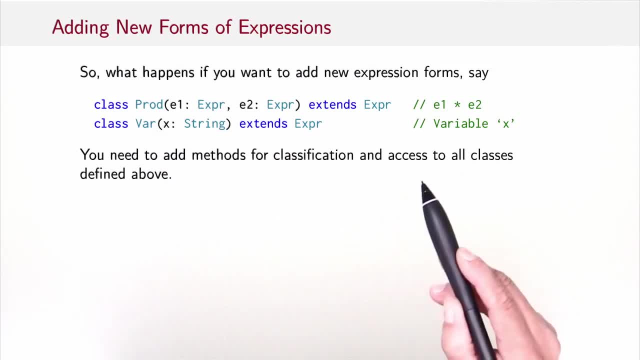 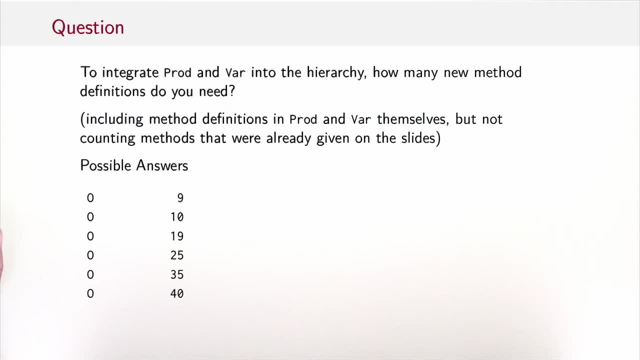 We need to add methods for classification and access to all the classes defined above, and we have to define the methods for these two new classes. So think about it: If we integrate product and variable into the hierarchy, how many new method definitions do we need? 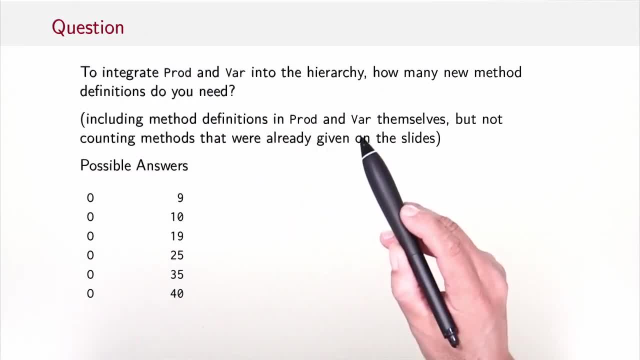 I include here method definitions in product and variable themselves, as well as any new methods that we have to add to sum and number, but not the methods that we have already shown on the slides. Possible answers would be 9,, 10,, 19,. 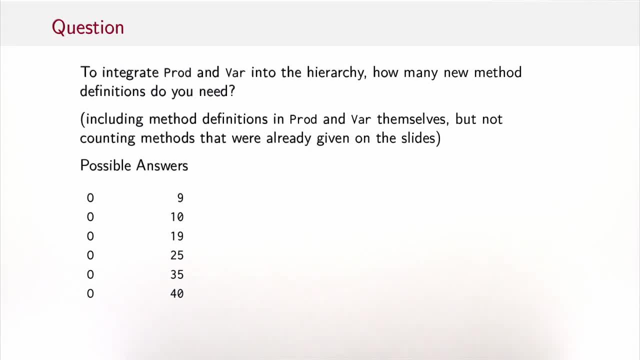 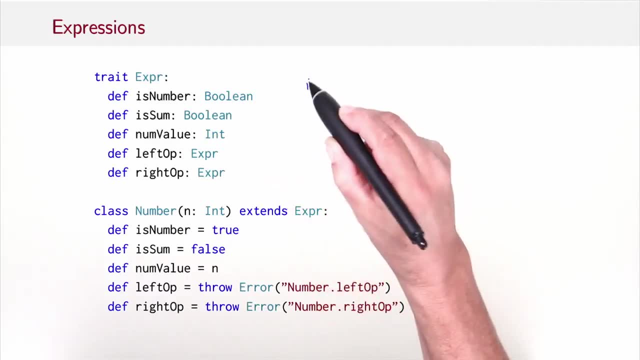 or is it 25,, 35, or 40?? So to come up with an answer, let's look at the existing classes first. We need two new methods- isVar and isProduct- in trait expression that have to be implemented everywhere And furthermore, if it's a variable, 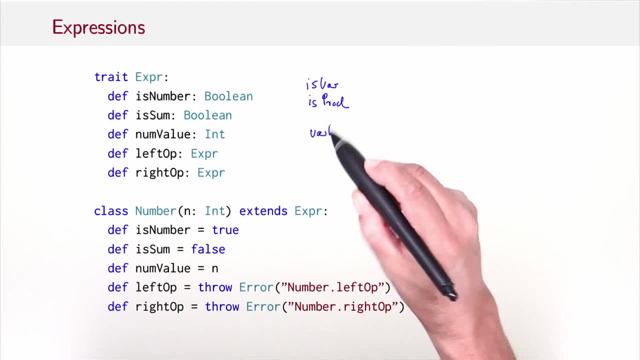 we need a method called var name or something like that to get out its name, and if it's a product, we might need product left op and product right op, but we could maybe also reuse the left op and right op operations here, So maybe there are two more op. 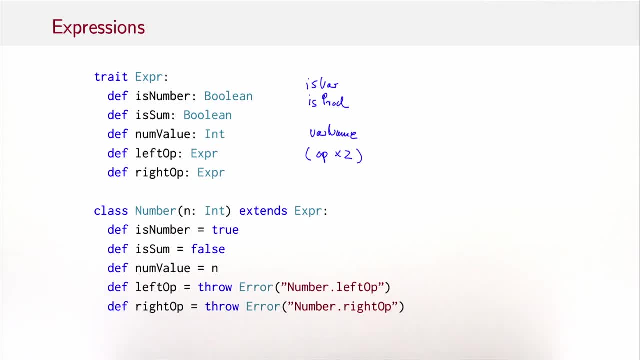 operations, depending on how far we want to separate things. So it makes, depending on how we count, three or five methods in expra that have to be added, that have to be added also to number and also to sum. So if we do the sums, 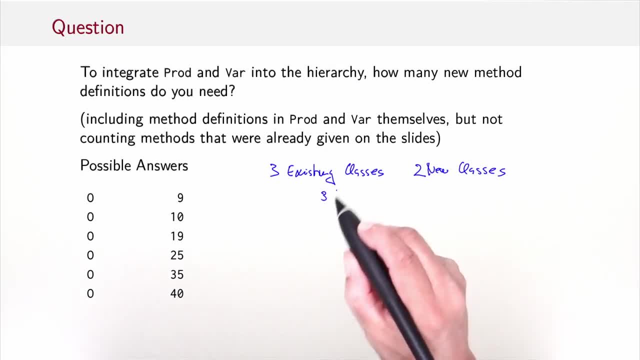 then, depending on how we do things, we need either three or five methods in addition per existing class and either eight or ten methods in a new class, because a new class has to contain the previous five methods that we've seen already as well. So there are three. 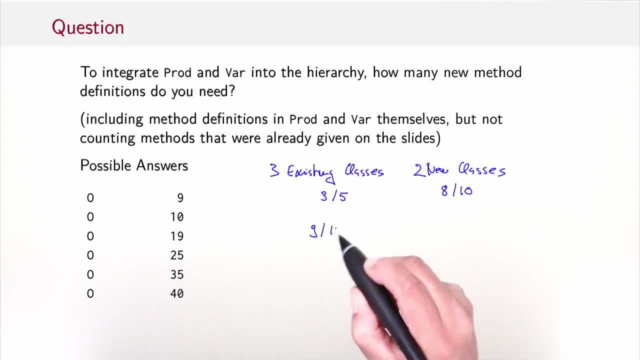 existing classes, so that makes nine or fifteen, and there are two new classes, so that makes sixteen or twenty. So that means if you do the sums, it's either twenty-five or thirty-five. That means both of these answers would be plausible. It's either twenty-five or thirty-five. 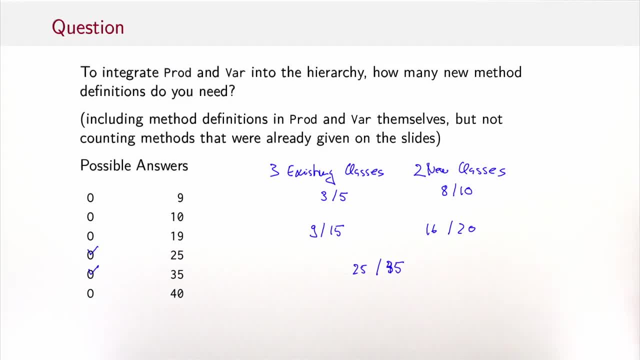 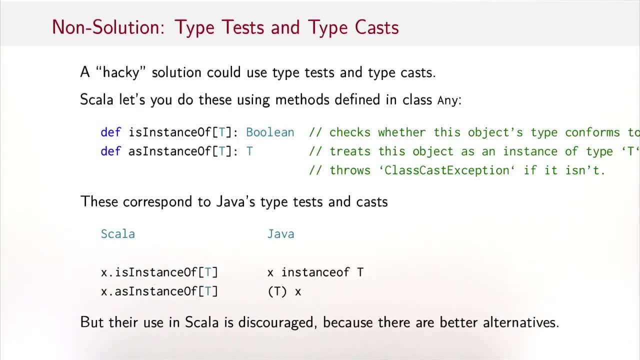 Which means it's quite a lot. even at twenty-five it's quite a lot. Okay, so we conclude that this is not very scalable. What else can we do? So one thing one could try is using type tests and type casts, but I find that quite hacky. 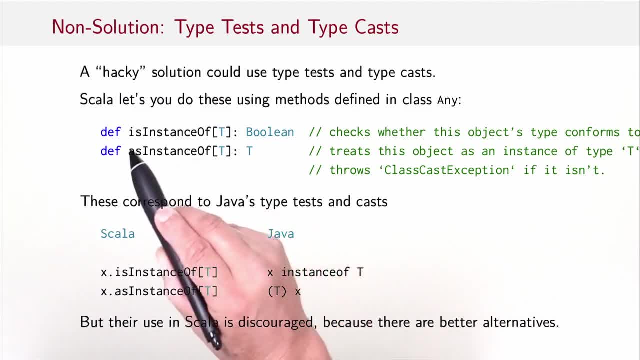 So in Scala you can test whether a value is of a certain type with the instance of operation. So x is instance of t tests whether x is at runtime, a value of type t And x, as instance of is a cast. It simply treats an object. 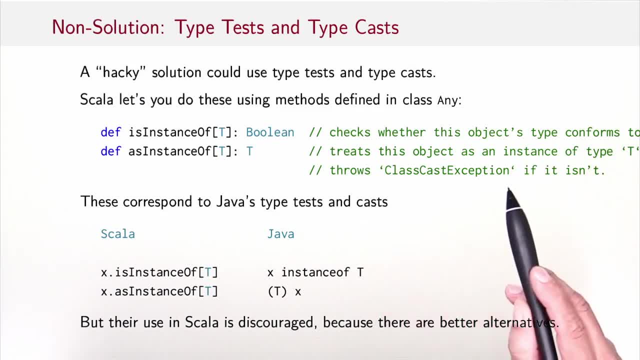 as an instance of type t and throws a class cast exception if it isn't. These correspond in Java to instance of and to the special cast syntax that you see here. But the use of type tests and type casts in Scala is actually discouraged because there are better alternatives. 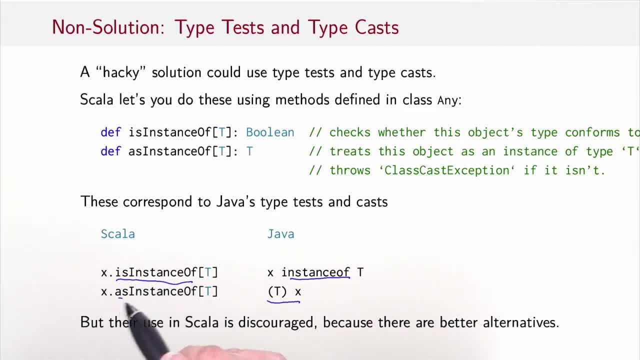 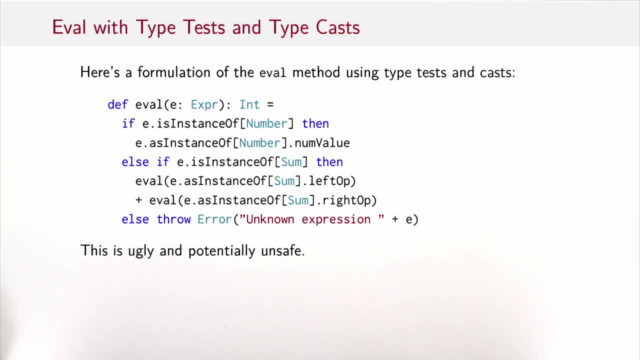 That's also the reason why we've chosen very long name for them. that are intentionally hard to type, So staying with type tests and type casts. here's a formulation of the eval method, But, as you can see, it's actually quite ugly. It's also potentially unsafe. 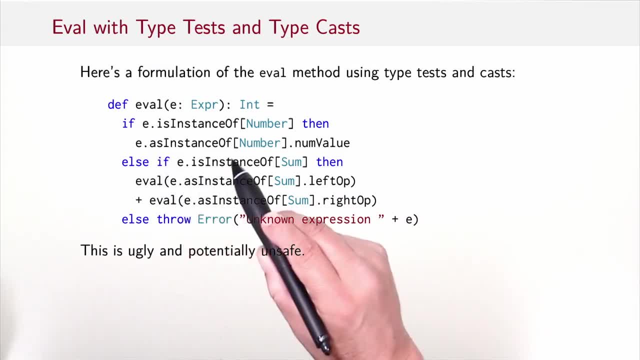 because we don't have usually a guarantee that a type cast which can throw an exception is always protected by a type test of the same for the same type. That's the case here, but you might easily make a mistake in a better program. So something. 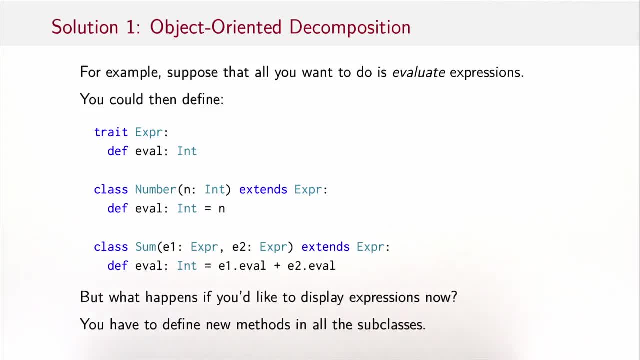 which is a more reasonable solution, is called object oriented decomposition. For instance, suppose all we want to do is evaluate expressions. Then we could define an abstract method, def eval inside the expression trait itself. that gets implemented in both of the subclasses. So for number eval would be n. 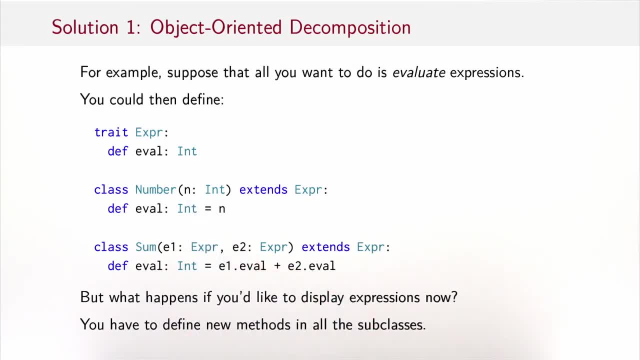 and for sum eval would be e1.eval plus e2.eval. So this looks quite concise. But what happens if we'd like to display expressions now? Well, we'd have to add a new method in each subclass. Let's say def show here. 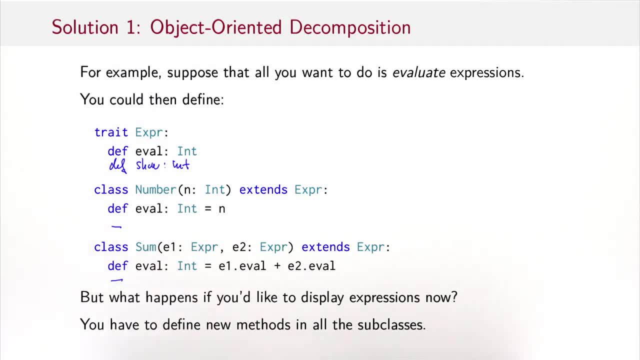 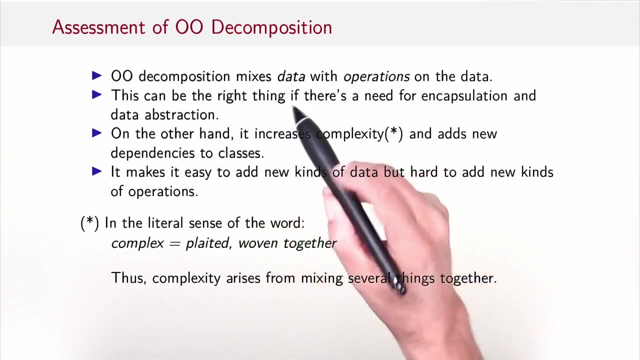 and we need one here and we need one here as well. So we need potentially to touch a large number of classes to add some piece of new functionality. So we've seen that object oriented decomposition mixes data with operations on the data. The data are. 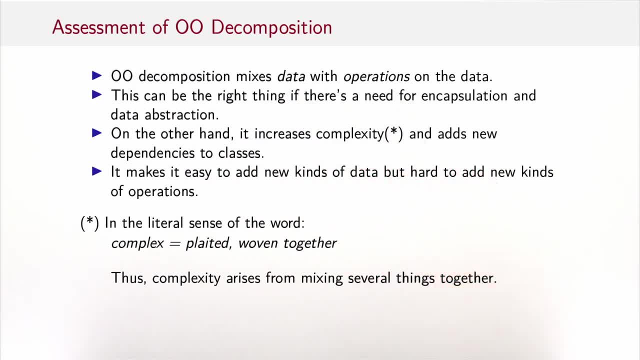 the fields and the classes, and the operations are the methods. This can be the right thing. if there's a need for encapsulation. We want to hide the data and data abstraction. On the other hand, it increases complexity and adds new dependencies to classes. 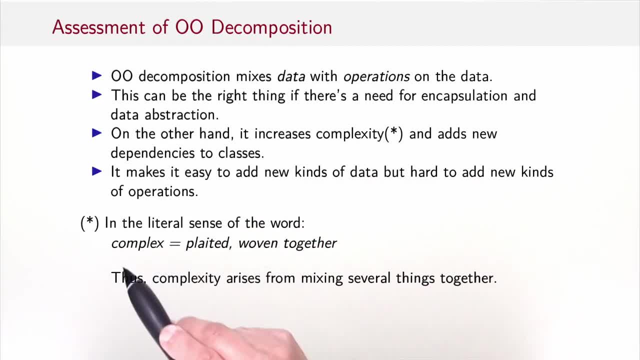 It increases complexity in the literal sense of the word, where in Latin complex means plated or woven together. Thus, complexity arises from mixing several things together, which is the case for object oriented decomposition. Of course, complexity is not by itself bad, and often there's no way to avoid. 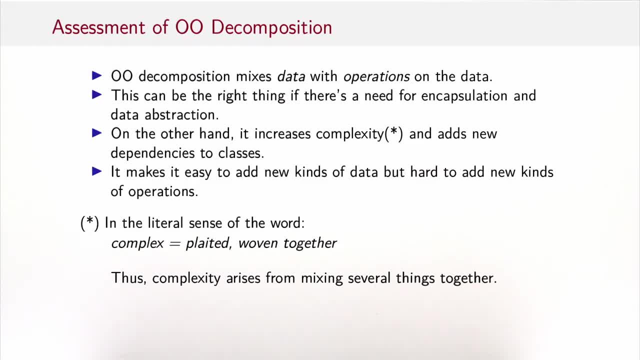 it one way or another, But we should use it only if there's a tangible advantage, And the tangible advantage could be that we need encapsulation or data abstraction or another advantage of object oriented decomposition is that it makes it very easy to add new kinds of data. 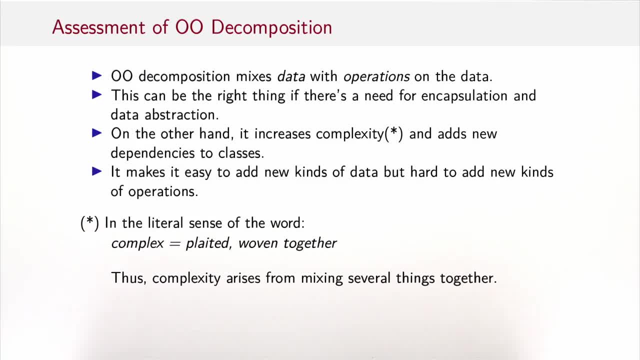 Because in that case we just have to invent a new class and give it all the operations that we have predefined and done, Whereas it makes it much harder to invent new kinds of operations. If we want to add a new operation, like show, we would have to touch all the 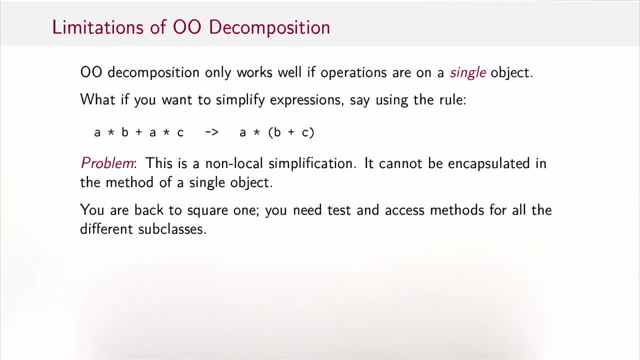 classes that we currently have. One other limitation of object oriented decomposition is that it works only well if operations are on a single object. To illustrate that, think about what you have to do to simplify expressions, say using the rule a times b plus a times c. 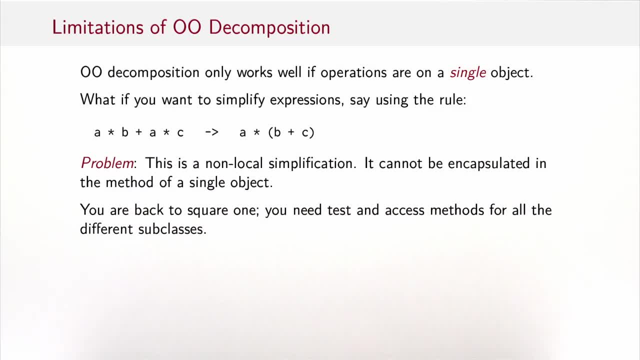 becomes a times b plus c. so we pull the b and the c together into an addition. The problem here is that this is a non-local simplification. It can't be encapsulated in the method of a single object. So you're back to. 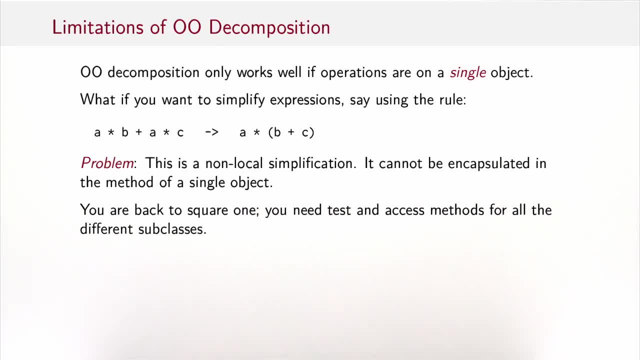 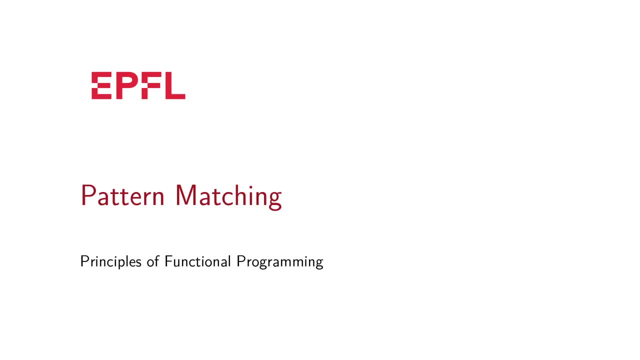 square one. You need test and access methods for all the different subclasses. In this unit we are going to learn about a functional way to do decomposition, which is called pattern matching. So the task we are trying to solve is to find a general and convenient way. 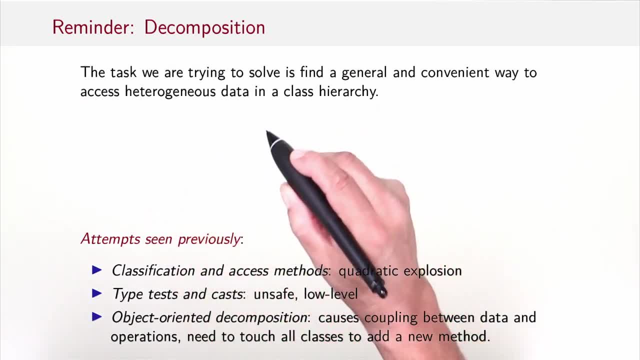 to access heterogeneous data in a class hierarchy. The example we had was a class of expressions and then that had subclasses- number and sum, and then possibly others- product variables and so on. Our first attempt was to use accessor and classification functions that suffered from quadratic explosion. 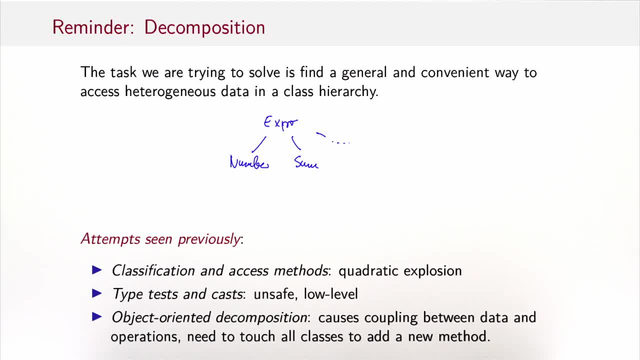 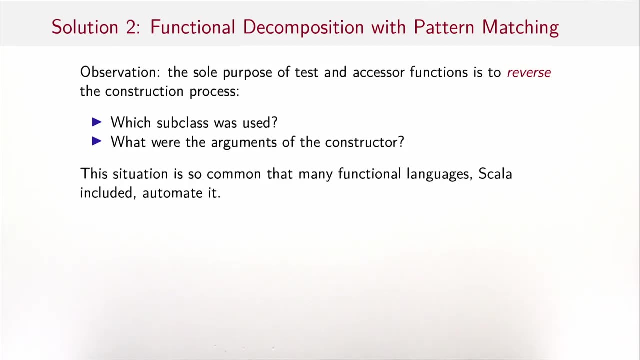 Our second attempt to use type tests and typecasts wasn't very safe nor pretty, and the third attempt to use object oriented decomposition, worked in some cases but had limitations. So another solution is to use functional decomposition with pattern matching. This relies on the observation that the only purpose of test and 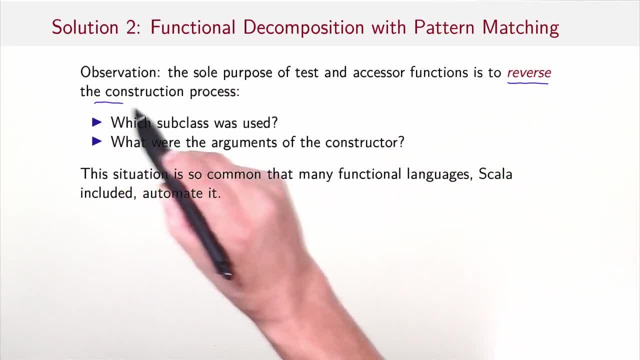 accessor function is to reverse the construction process. Namely, we want to know which subclass was used for the construction of this value and what were the arguments to the constructor. That situation is so common that many functional languages, Scala included, automate it. Scala supports. 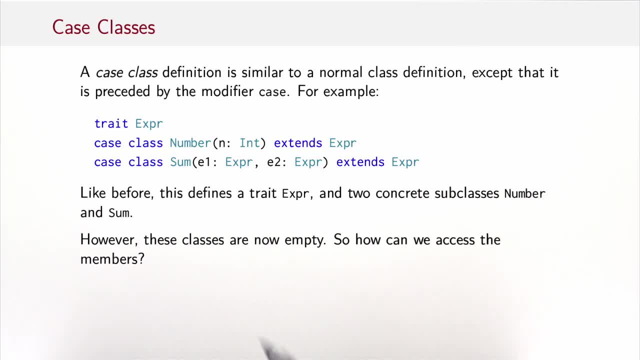 functional decomposition through case classes. A case class definition is similar to a normal class definition, except that it is preceded by the modifier case. So here we have our expression class hierarchy, and number and sum are now case classes. Those two classes are now empty. There are no. 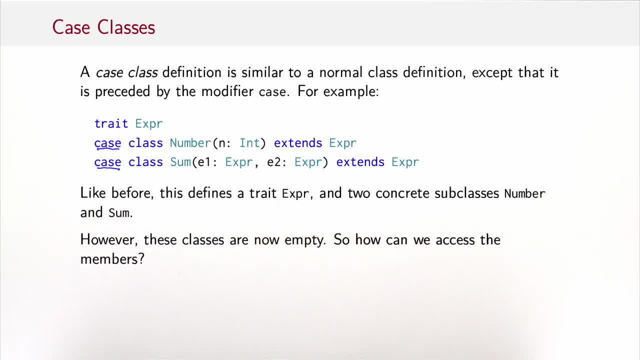 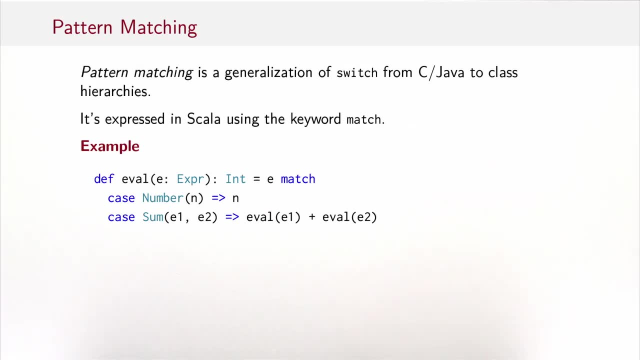 methods given in either one. So how can we access their members? That's where pattern matching comes in. Pattern matching is a generalization of switch from C Java to class hierarchies. It's expressed in Scala using the keyword match. So, for instance, to define an: 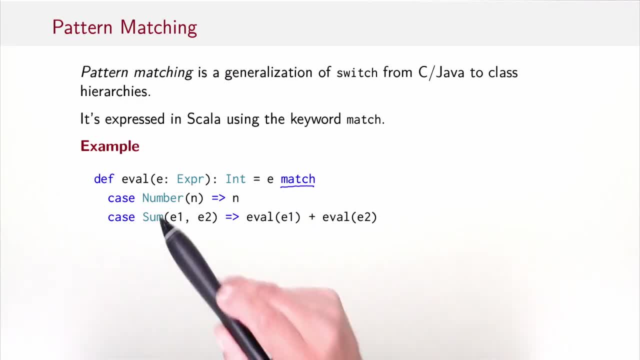 eval function on expressions. what we could do is do a pattern match on the expression in question. There are two cases. If the expression is a number, then we return its numeric value n. If it's a sum over expression e1 and e2, then we evaluate e1. 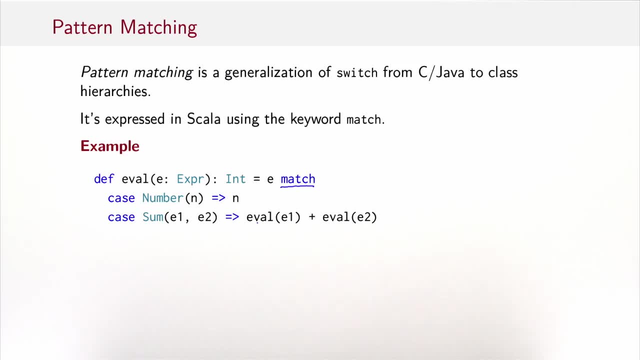 and evaluate e2 and add the two results. So what you see here is that a pattern at the same time identifies a case number or sum and names the elements in that case, Here the n for the numeric value or the expressions e1, e2. 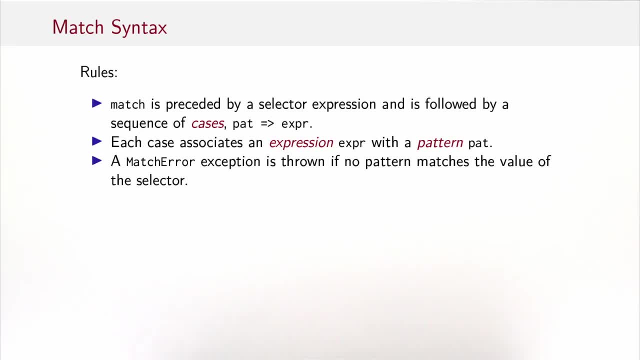 for the left and right operands of the sum. So, in general, match is preceded by a selector expression and is followed by a sequence of cases that all take the form pattern arrow expression. Each case associates an expression with a pattern. If no pattern matches the value of the selector. 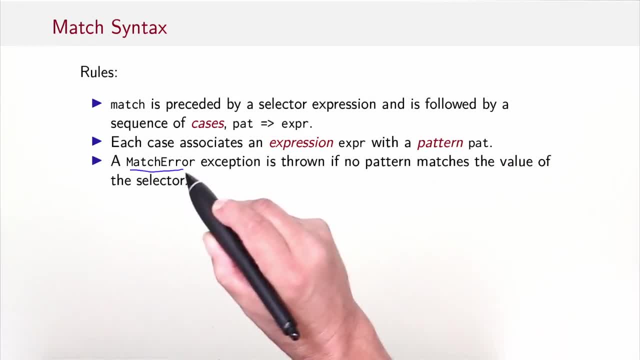 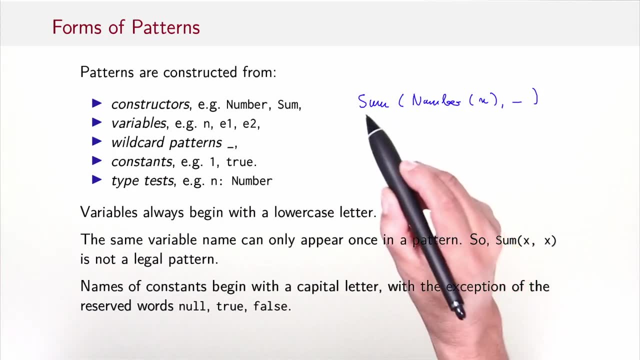 an exception is thrown and the exception is of the class match error. Here is a more complicated pattern, So that pattern is formed from a constructor sum that gets applied to arguments. The first argument is a constructor number that gets applied to a variable pattern. So that's. 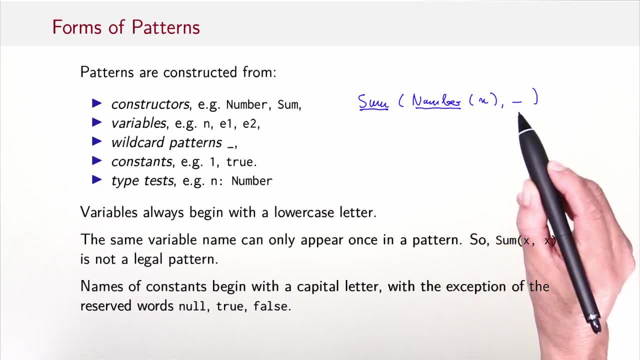 a second form here, And the second argument to sum is a wildcard which says it's essentially a don't care operation. It says it can match anything and we don't bother to give it a name. Besides these forms of patterns, you can also have: 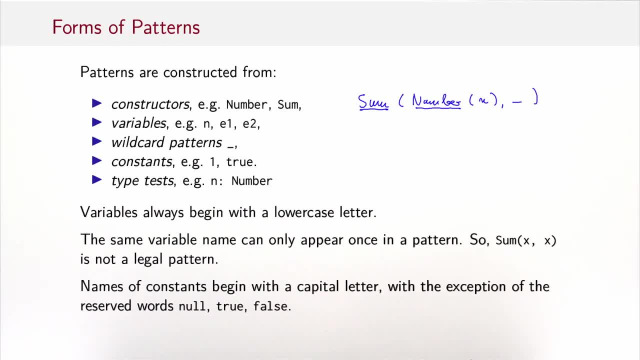 constants in patterns such as 1 or true, and you can also have type tests in patterns such as n colon number. So we could for instance say here x colon number as the second argument, and that would match any number, so not another sum, and name it x. 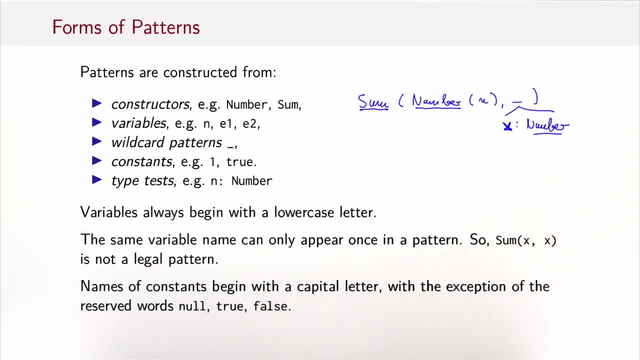 Variables such as x or n always begin with a lower case letter in patterns. If they would start with an upper case letter, they would be interpreted as constants, And the same variable name can only appear once in a pattern. So sum x- x is not a legal pattern. 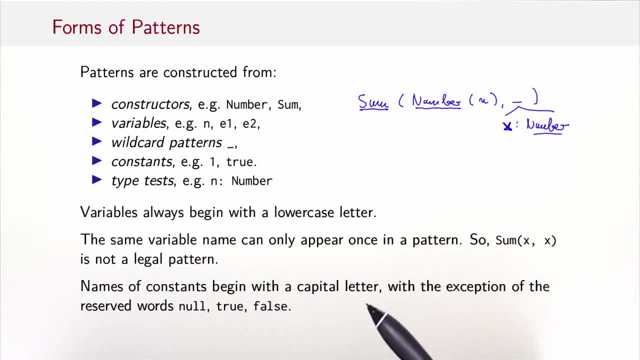 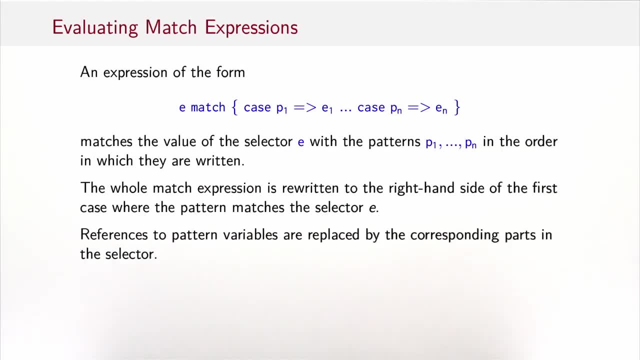 Names of constants should begin with a capital letter, with the exceptions of the reserved words null, true and false. So let's look at evaluation. If we have a match expression of this form, that expression matches the value of the selector e with the patterns p1. 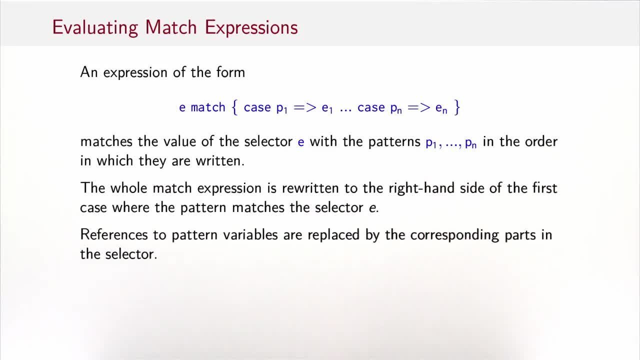 to pn in that order, in the order in which they are written, And the whole match expression is then rewritten to the right hand side of the first case, where the pattern matches the selector And references to pattern variables in the pattern are replaced by corresponding. 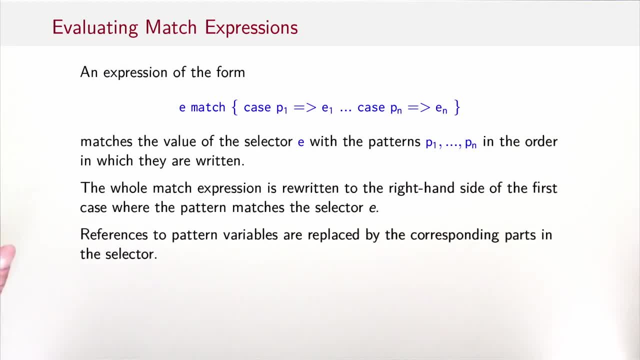 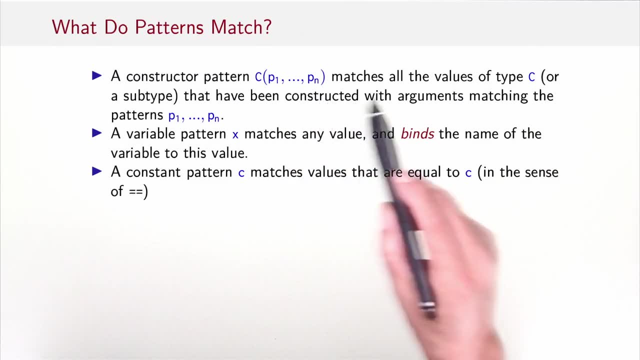 parts in the selector. We'll see how that works in an example shortly. So what do patterns match? If you have a constructor pattern like this, then that matches all values of type c or a subtype that have been constructed with arguments that in turn match the. 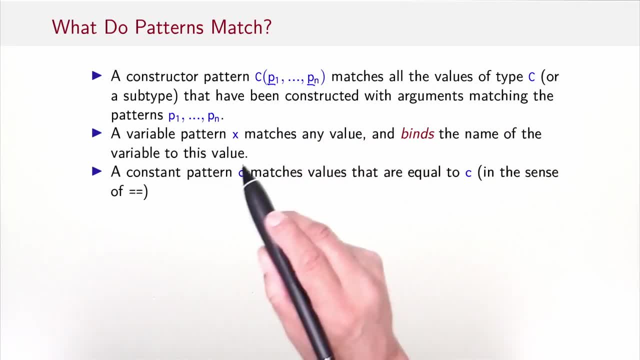 patterns p1 to pn. A variable pattern matches any value and binds the name of the variable to this value. The same thing is a wildcard pattern matches any value and does not bind any name to that value. A constant pattern c matches values that are equal to. 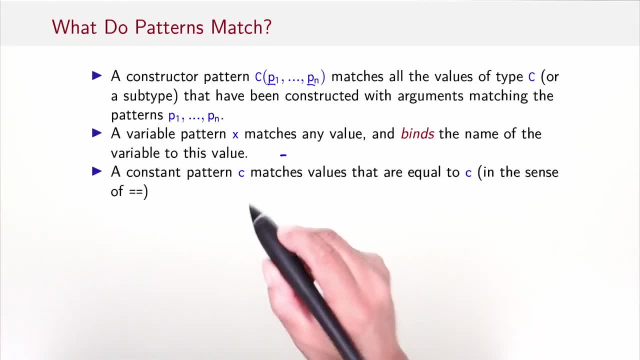 c in the sense of equals equals. So if you have, let's say, 22,, then that would match the value 22 and no other value. And finally, a type pattern like n number would match any value that is equal to a number and name it with the name n. 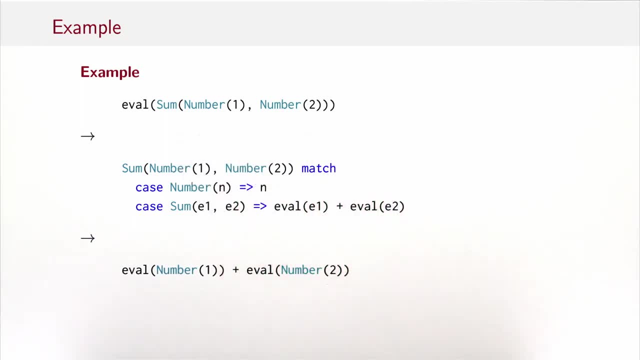 So here's an example. Let's evaluate sum of number 1, number 2.. So as usual, we replace the call to eval by its right hand side, where the parameter e of eval would be replaced by the argument here. So that gives the argument here in. 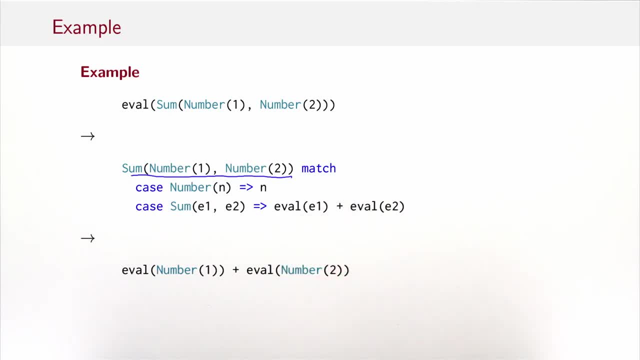 selector position of a match that you see here. Now we match this selector with the patterns one by one. The first pattern does not match because this one is a sum and that one is a number, but the second pattern matches, So we replace that match expression. 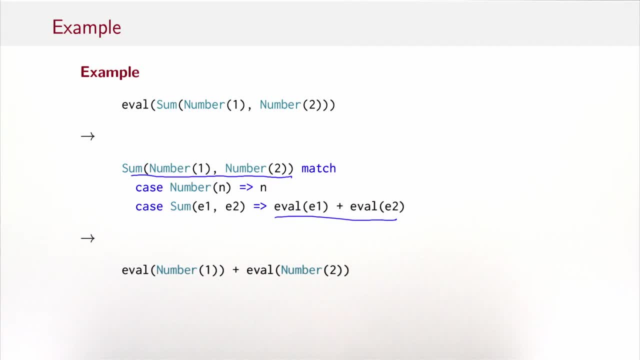 by the right hand side, This one here- Where, furthermore, e1 gets replaced by the corresponding part in the selector, So that's number 1, and e2 gets replaced by number 2, because that matches this part of the selector. Now to evaluate that expression further. 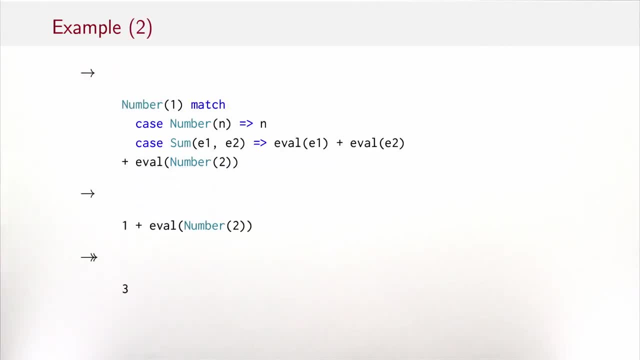 we replace the first call of to eval here by its right hand side. That would give number 1 match again the same two cases, and then, once we've done that, we still have to add with eval number 2.. Now we see that it's the first pattern. 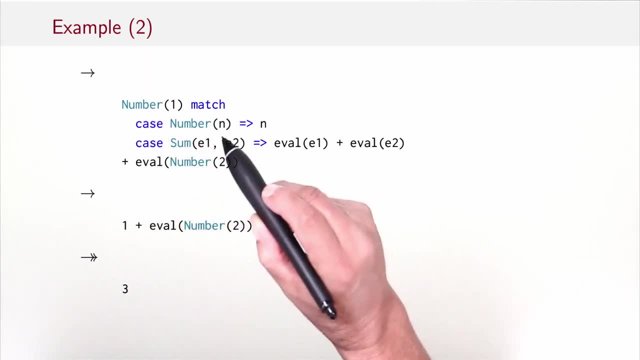 that matches So number number line up here and the variable n gets replaced by the selector expression 1.. So that leads to 1 plus eval number 2, and proceeding in the same way we get eval number 2, gets 2 and the whole result becomes 3.. 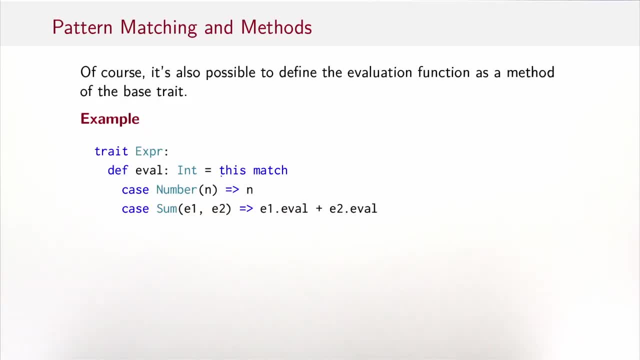 Pattern matching functions can be defined anywhere. So far we've defined eval outside the expression type hierarchy, but we could also put it as a method inside trade expression, and in that case the match would be on the current values on this instead of a given parameter Otherwise. 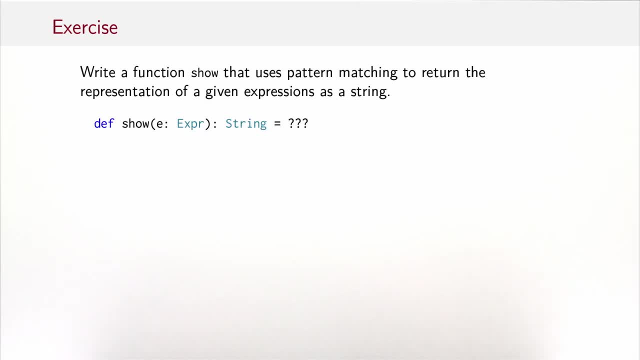 it would be exactly the same match. So here's an exercise for you: Write a function show that uses pattern matching to return the representation of a given expression as a string. So we want to write this method and you should fill in the triple question marks. 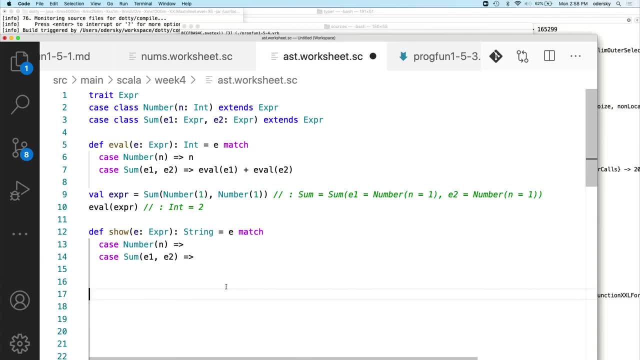 here. Okay, So I've added what we had so far into a worksheet. We have the expression, class hierarchy, the eval function. I have a sample expression which is just 1 plus 1 and we evaluate it. Now we have to define a. 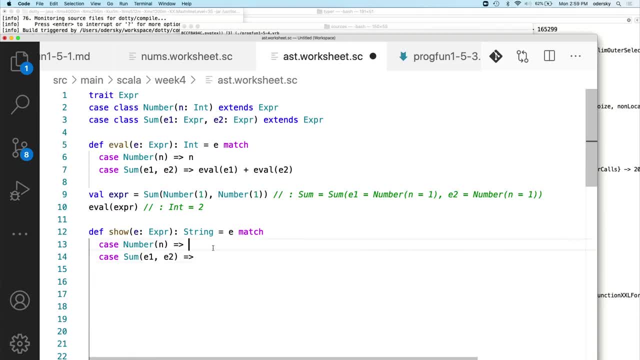 show function and the template is quite obvious. We will match on the expression: If it's a number, we have to do one thing, and if it's a sum, we have to do another thing. So if it's a number, what do we need to do? 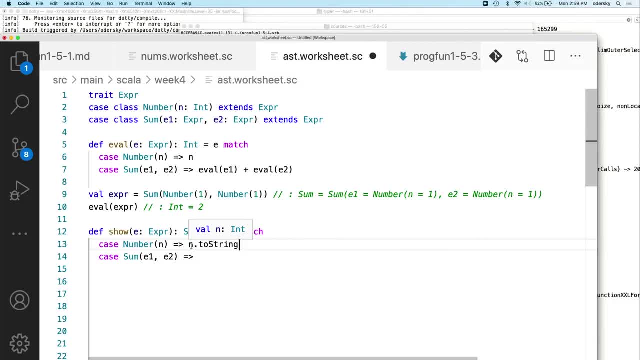 Well, we just return the number here as a string, because that's the result type of show. So it's n dot 2 string. Remember, all values in Scala have a 2 string object that converts them to a string representation. Or we have a sum expression: sum e1. 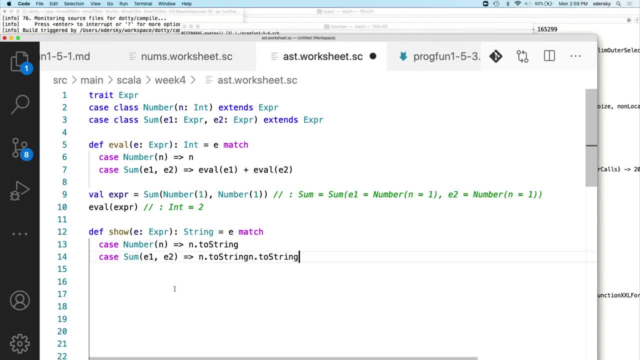 e2.. What do we do in this case? In this case, we return a string that contains the recursive calls of show on the two operands and a plus in the middle. Let's put that to the test. Let's say: show of expression. 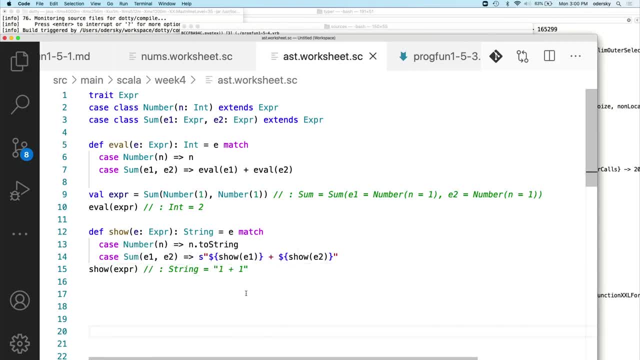 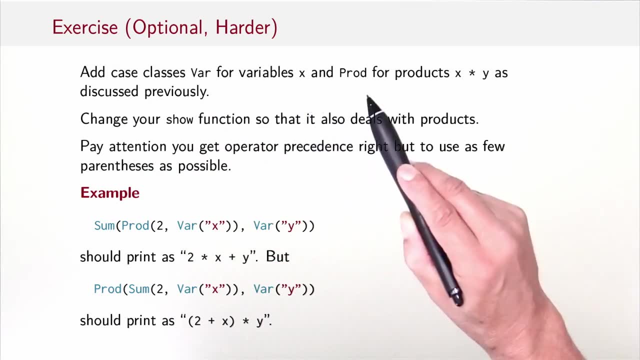 What do we get? We get 1 plus 1, as expected. So here's a second exercise which is a bit harder. Add case classes: var for variables x and prod for products, x times y, as discussed previously. Change your show function so that it also deals with 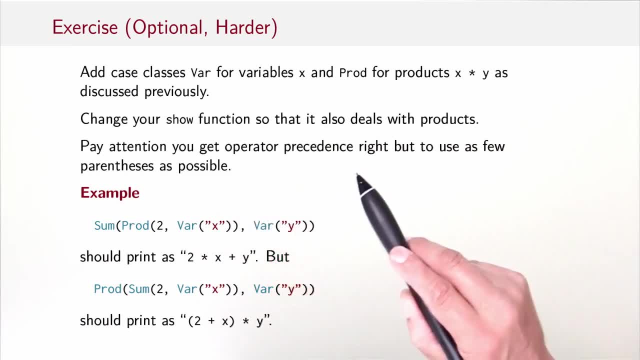 products. But pay attention that you get the operator precedence right and at the same time use as few parentheses as possible. So, for instance, if you have a sum of products, then you can leave out the parentheses. That's a valid output. But if you have a product of, 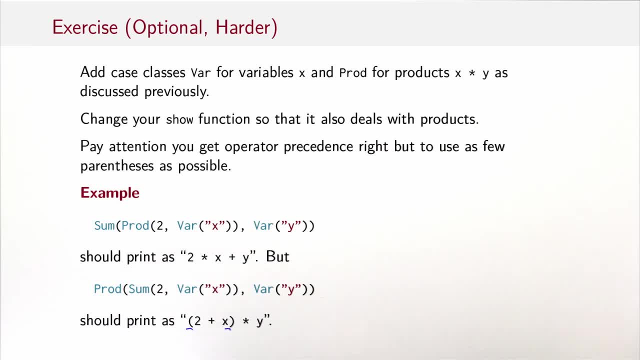 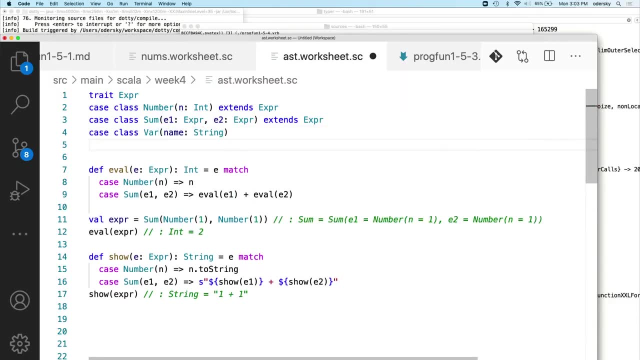 sums, then you need the parentheses around here, because otherwise it would change the meaning of the expression. Okay, let's see what we have to add to the worksheet. First, the two case classes: Here's the var class And here's the product class. 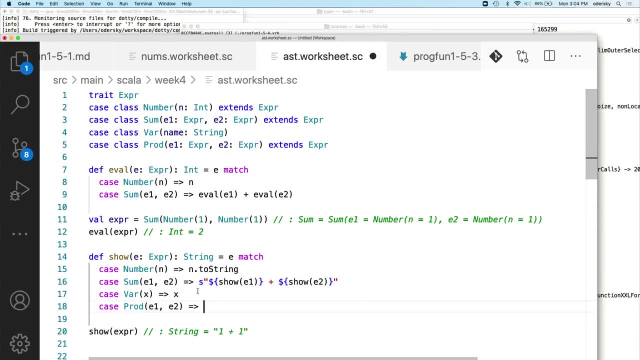 How do we change show? So for the var class we just return the name of the variable, And for the product class we might try this. so essentially treat it like the sum class. Okay, let's put it to the test. Define another test value. 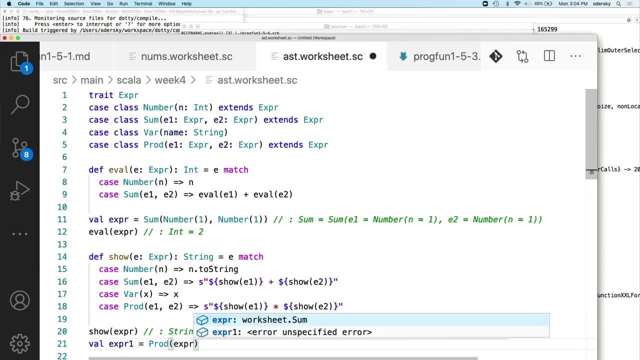 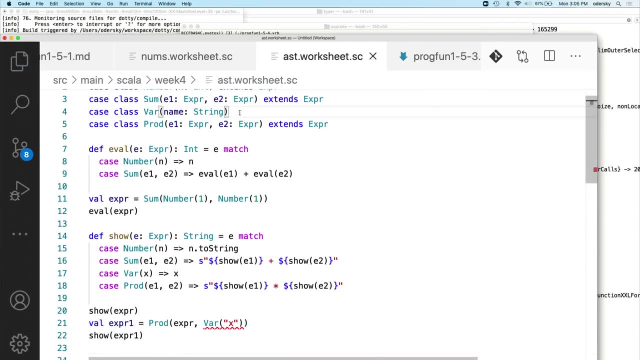 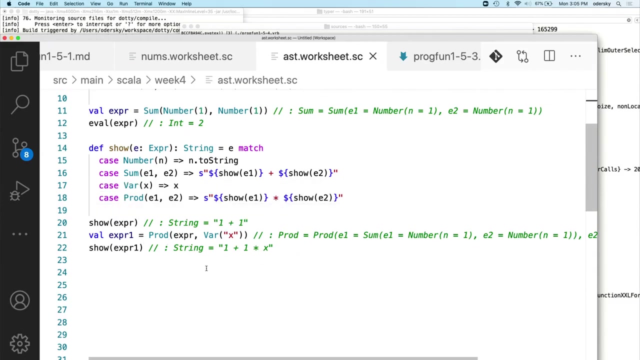 x per 1 equals. let's say product x per var x and show x per 1.. I forgot to make var extend expression. Good, now we see something, So we have the x per 1.. But if we show it, then it's actually. 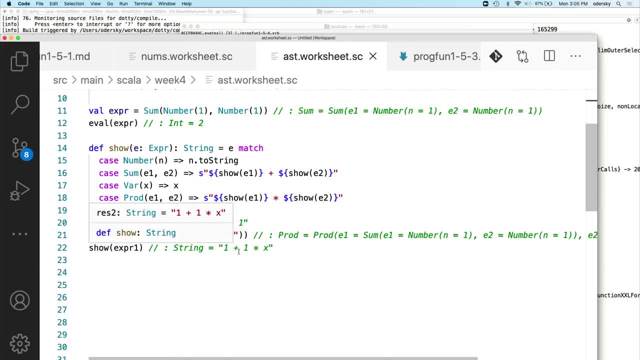 wrong, because it looks like we multiply x by 1 and add 1, where in fact we wanted to multiply x by 2.. So how do we fix that? Well, the problem is that we can't really use show here, because it doesn't put in the right parentheses. 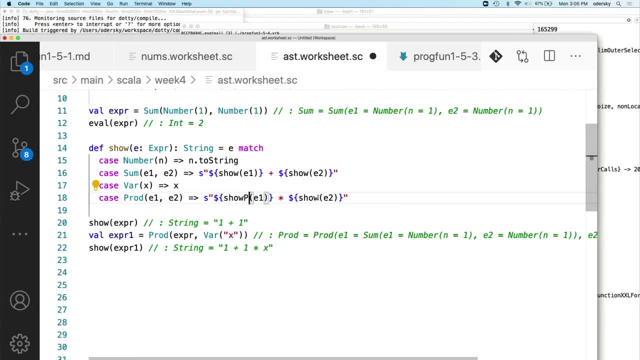 So what I propose is we call another function, call it showP. that puts the proper parentheses around the operands of our product. So how do we define showP? So showP starts like show but says well, if the result is a sum, then the expression: 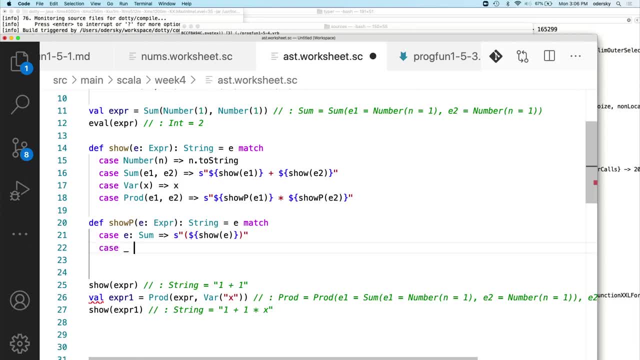 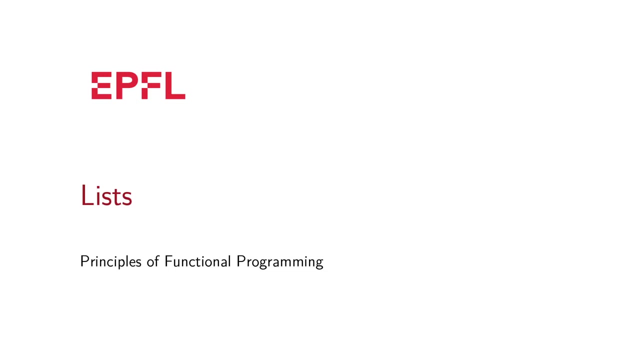 in parentheses and otherwise just show the expression as usual. And now we see that indeed, here at the bottom the two parentheses are put around the right expression: 1 plus 1.. In this section we are going to introduce one of the most fundamental data structures in functional programming. 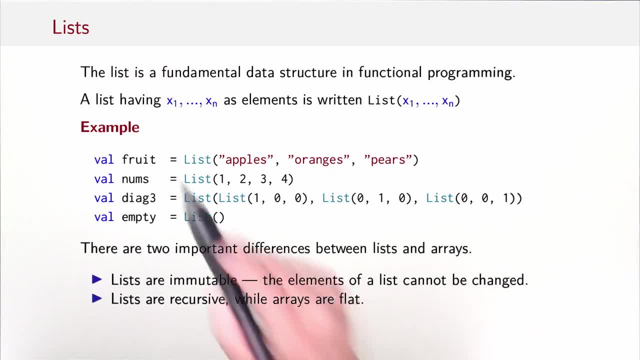 which are lists. A list with elements x1 to xn is written list of x1 to xn, like you see here. For instance, here's a list of fruit, list of apples, oranges, pears. Here's a list of numbers. Here's the diagonal of a 3 by 3. 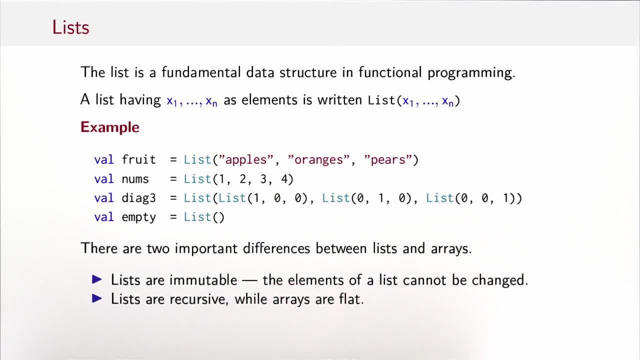 matrix, That's a list that consists of three lists as sub elements, And here's the empty list. Lists resemble a lot arrays, which is another fundamental data structure used in imperative programs, But there are two important differences. The first difference is that lists are 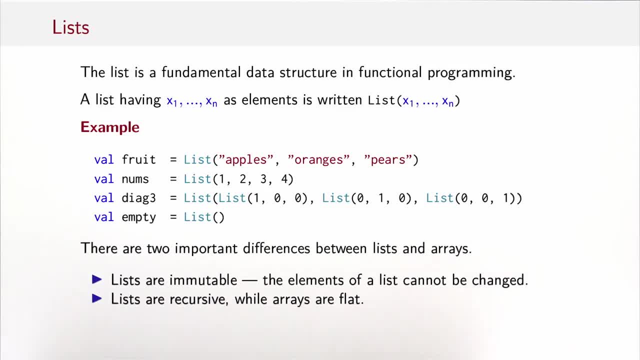 immutable. The elements of a list cannot be changed after the list is constructed. And the second difference is that lists are recursive while arrays are flat. So to see that, let's draw the structure of some of the lists that you've seen here. Let's start. 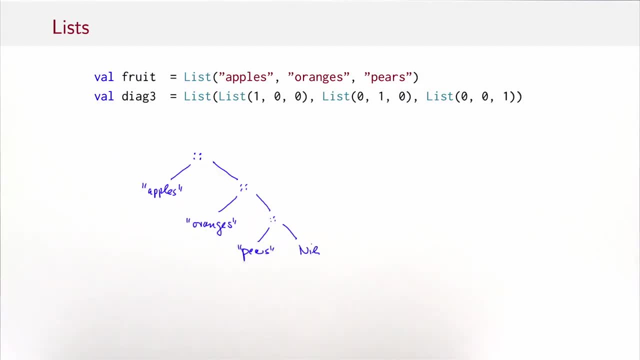 with the first list of fruits. So you see, the fruit list consists of a cell which we call a cons cell, Which we often write with a double colon. That cons cell has a head element, which is called apples, and a tail, which is another list. 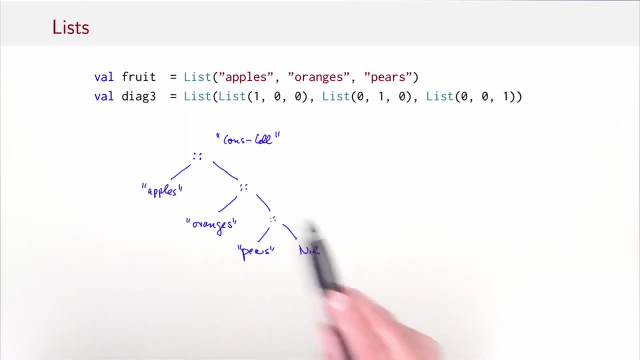 which has a head element- oranges- and a tail element, which is another list. And that third list has a head element called pears and its tail is nil. So lists are recursive. Every list contains in its tail position another list that can be nil. So they're a little. 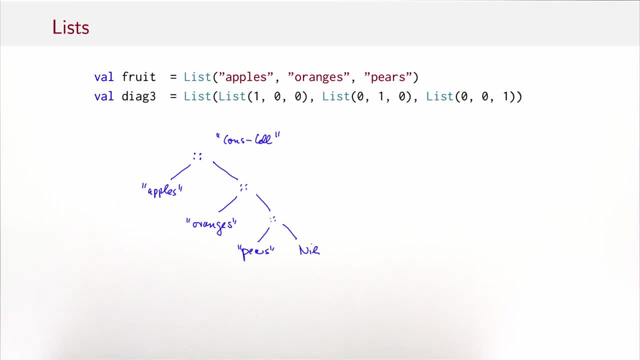 bit like Russian dolls. Each doll contains a slightly smaller doll inside. The elements of this list are simple values, but it's also possible to design lists of lists. An example is the second list that we see here, diagonal three. So here you see the structure of diagonal. 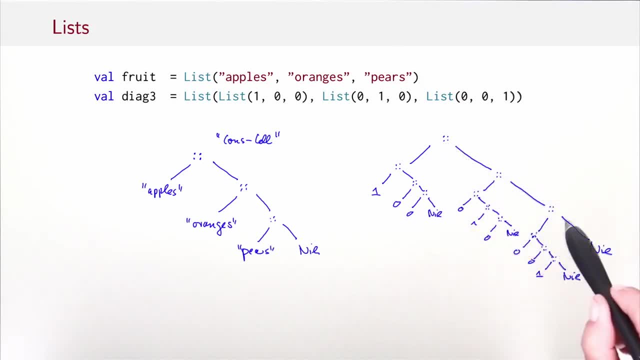 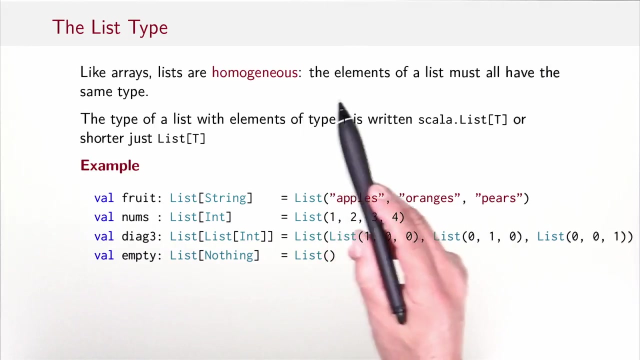 three. It has, at the top level, three cons nodes: one, two, three, And each cons node has a head element, that is another list, One of each of these three lists of three numbers, each. Like arrays. lists are homogeneous. The elements of a list must all have the same type. 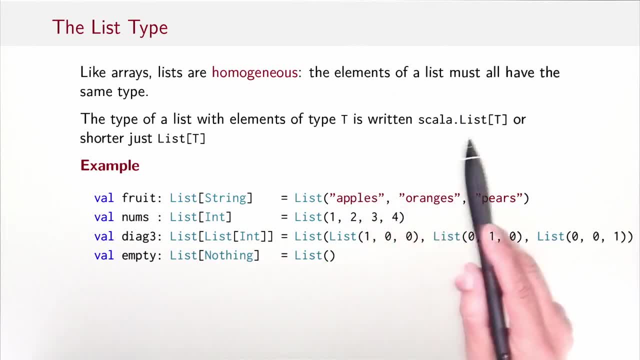 The type of a list with element of type t is written: scalar dot list of t or, shorter, just list of t. So if we add the types to the lists we've defined before, then fruit would have type list of string because its elements are strings. Nums has type. 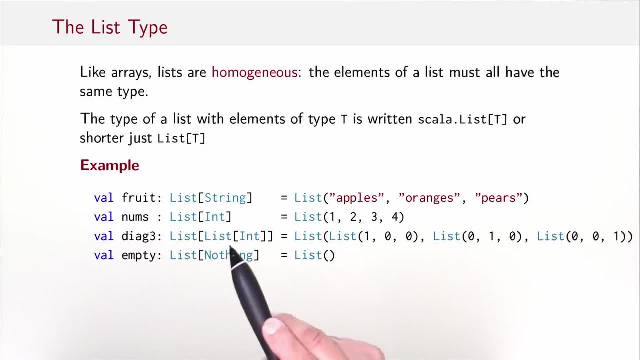 list of int. Diagonal three is a list of list of ints. Its elements are list of ints And finally, empty, is a list of nothing. We will see the significance of this nothing value later on. We've seen that all lists are constructed from the. 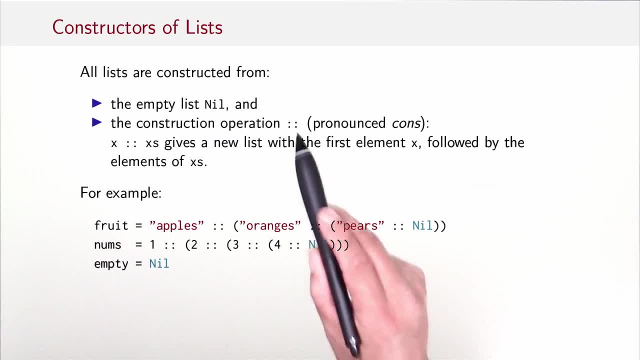 empty list, nil, and the construction operation double colon, which is pronounced cons, So x, cons, xs, gives a new list with the first ahead, element x, followed by the elements of xs, where we say those elements form the tail of the list. So for instance, the fruit list that we've seen. 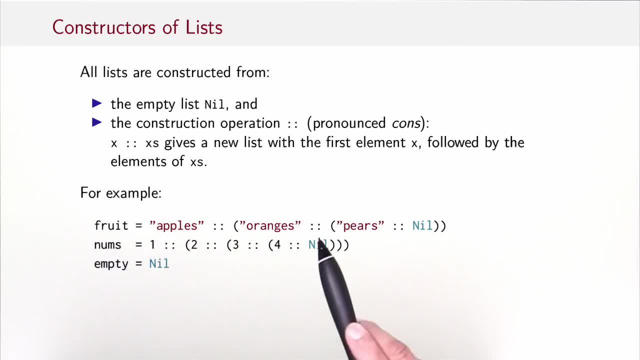 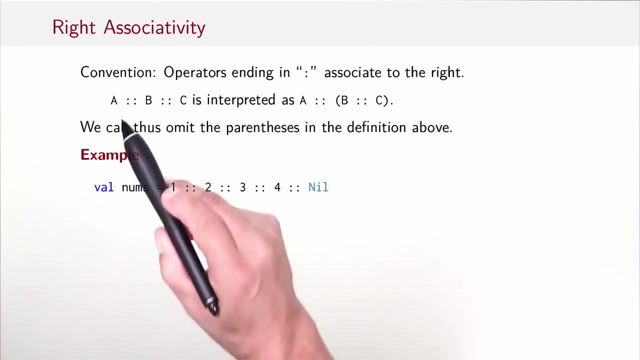 can be written like this: Apples cons, oranges cons, pears cons- nil. or the numbers list can be written like this: or empty is simply nil. In fact, we have a convention that operators that end in a colon associate to the right, So that means you can write: 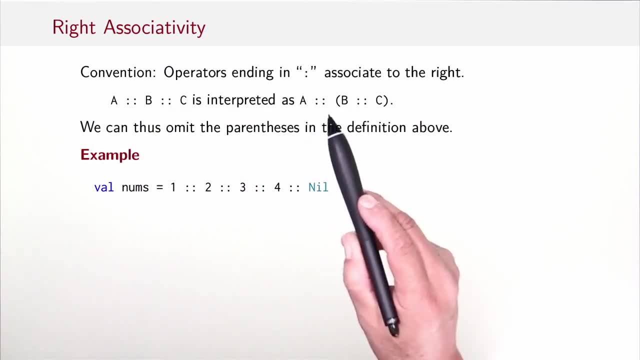 a colon b, colon c, and it means the same thing as a double colon b, double colon c in parentheses, And that means we can omit the parentheses in the definitions above. So val nums, which was list of one, two, three, four can be written: one cons two. 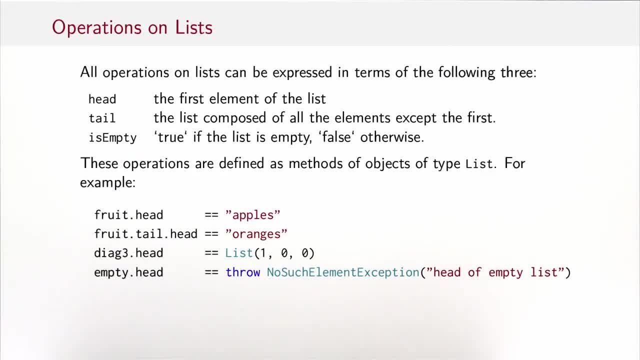 cons, three cons, four cons, nil. There are three fundamental operations on lists, and all other operations can be expressed in terms of those three. The first fundamental operation is head, which returns the first element of the list. The second fundamental operation is tail, which returns the list composed of all the 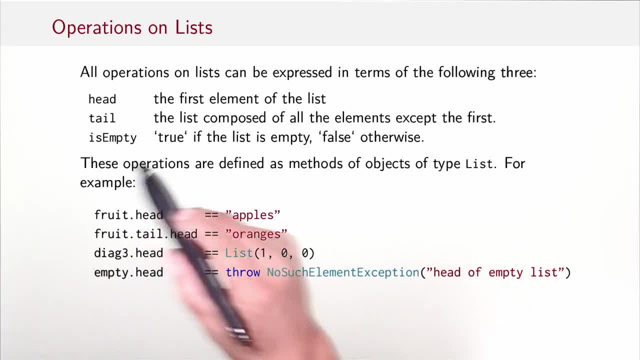 elements, except the first And the last fundamental operation is empty, which is true if the list is empty and false otherwise. So these operations are all defined as methods on objects of type list. For instance, fruit dot head would be apples. fruit dot tail dot head would be: 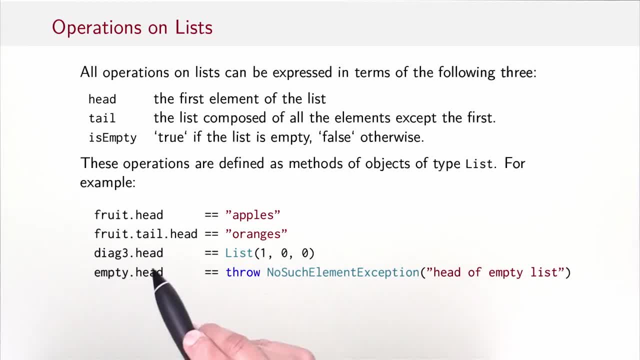 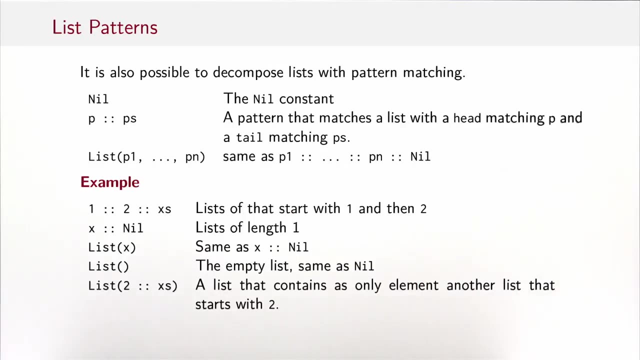 the second element of fruit, that is, oranges. diagonal three dot head would be the list. one, zero, zero and empty dot head is not defined and in fact it throws an exception and no such element. exception which says head of empty list Instead of using head and tail. it's also: 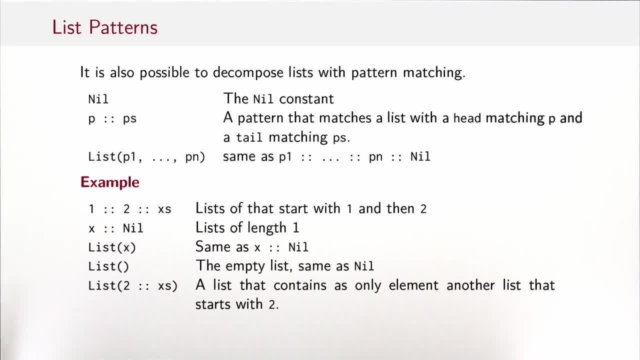 possible to decompose lists with pattern matching, and that one is often preferred. Patterns for lists follow exactly the way we construct lists, So the nil nil constant can be used as a pattern. The pattern p cons ps is a pattern that matches a list with a head that matches. 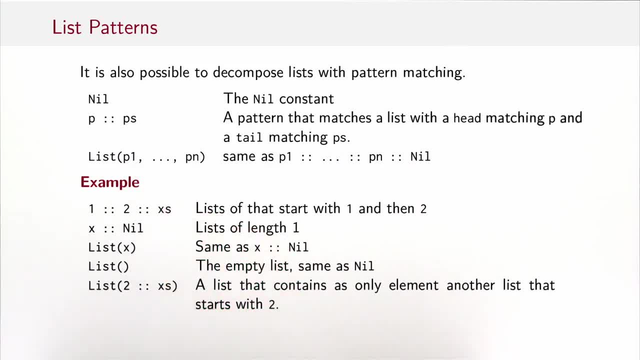 p and a tail that matches ps, And the pattern list of p1 to pn is actually the same as p1, cons and so on: pn cons nil, So it matches a list consisting exactly of n elements that each match patterns p1 to pn. So here are some examples. 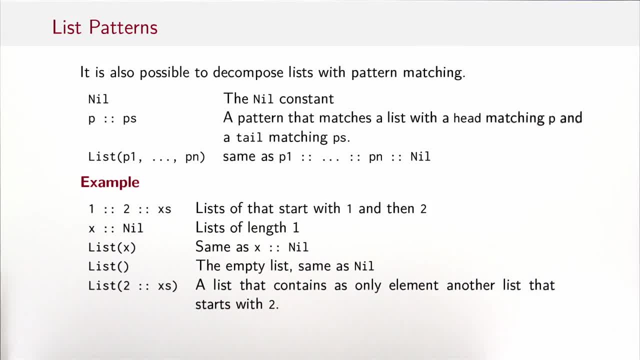 of list patterns: 1 cons. 2 cons xs. that matches all lists that start with 1. are followed by 2 and then can be followed by arbitrary elements that are captured in the variable xs. x. colon nil matches all lists of length: 1.. List of 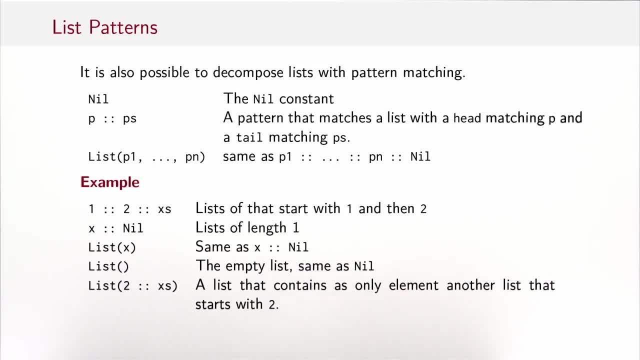 x is the same as x colon. nil also matches all lists of length 1. List, simply like that is the empty list, that's the same as nil, and list of 2 colon xs. what is that? well, that matches a list that contains one element and that element is another. 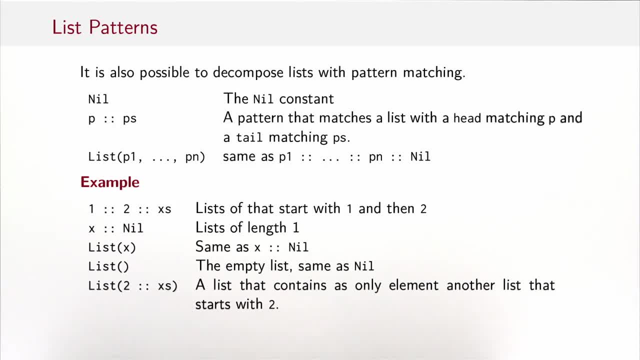 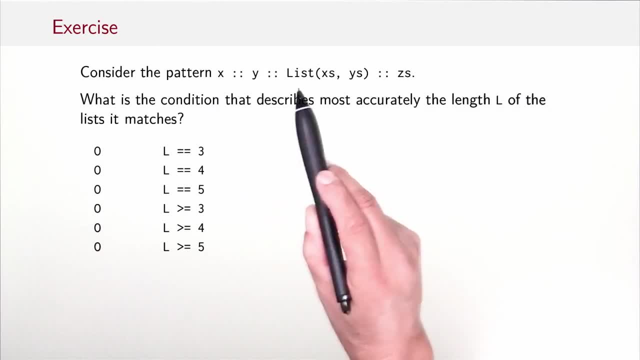 list that has starts with 2 and is followed by arbitrary elements. So to check whether you've understood that, let's consider the pattern: x cons, y, cons list xs, ys, cons, zs. What is the condition that describes most accurately the length l of the listed? 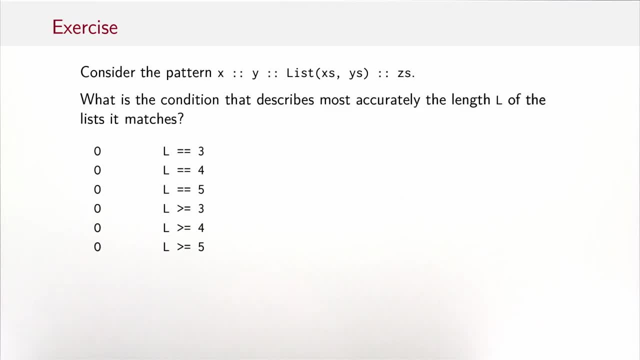 matches. Here you have 6 choices. So the answer is: it describes lists of length at least 3.. Let's see why. So we have a pattern that matches a head: x, a second element, y, a third element. that must be of this form, So that's a. 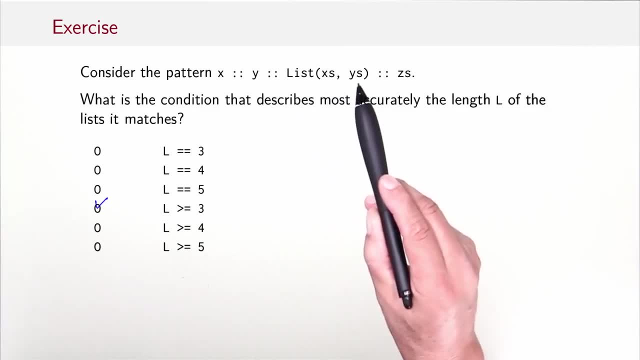 single element, but it must be a list. So that makes 1,, 2,, 3 elements and then it can be followed by any tail. zs including the tail could be nil. So if the tail is nil, then that list would have 3. 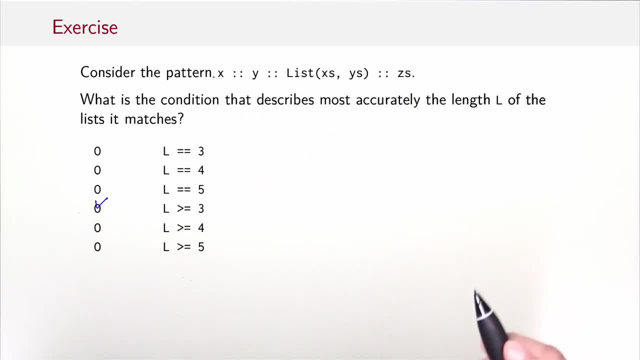 the length of that list would be 3.. Some people might get confused and say: well, I see 1,, 2,, 3,, 4 elements here. Why does it not say list length greater or equal 4?? Well, it helps if we draw that list. 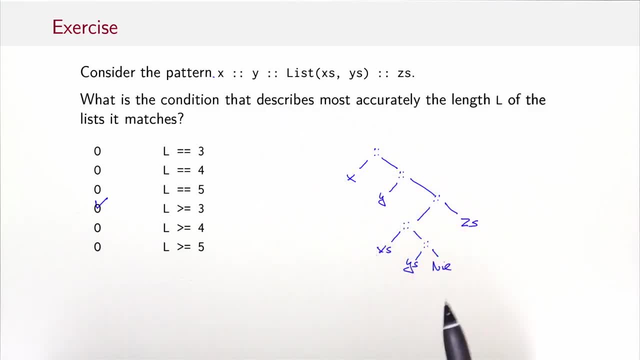 So that's the structure of the list that you see here above, and you see, indeed, if you count the cons node here, it's 1,, 2, 3 and then it's followed by some arbitrary tail zs. So the xs, ys, they don't count. 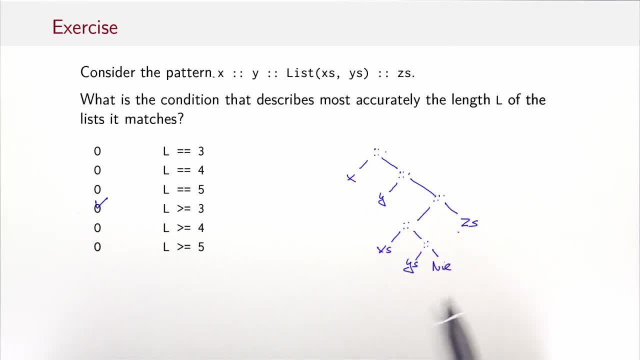 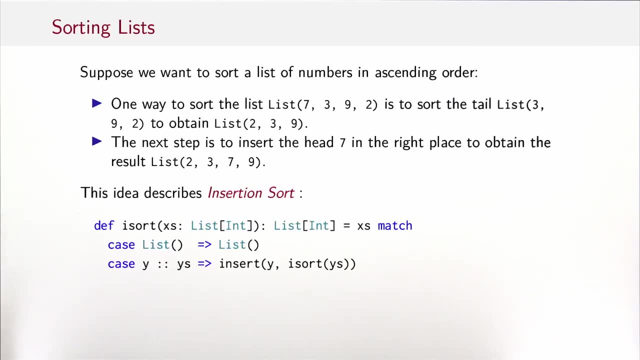 towards the length of the outer list because they make up together an element of that list, Namely the third element of the outer list. Okay, so let's start with writing simple functions over lists. One common function is sorting a list of numbers in ascending order. 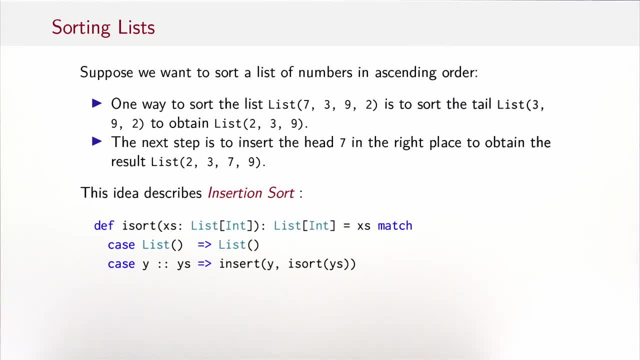 There are several ways to do it. Here's a particularly simple one which is not very efficient. So one way to sort the list 7,, 3,, 9,, 2 is to say: well, let's sort the tail of the list first. 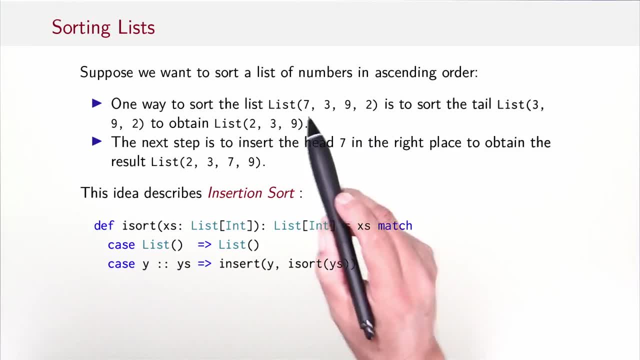 that would give the list 2,, 3,, 9, and then let's insert the element 7 at the right position in that list, Functionally of course. So we can't change the list, but we would return then a new list which would be 2,, 3,, 7,. 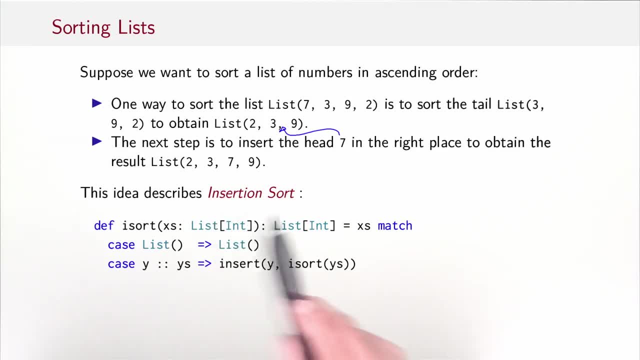 9. So that idea describes insertion sort, a particular sort algorithm, And here's the outline of insertion sort. It takes, if we work with integers, a list of integers and gives us back a list of integers. We do a pattern match If the list is. 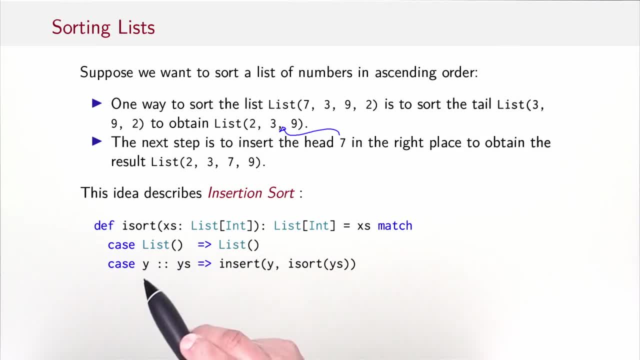 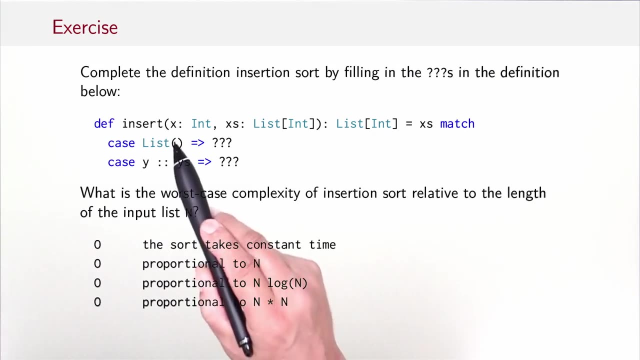 empty, then we return the empty list. otherwise, if the list is non-empty, then we recursively sort the tail of the list and we insert the head of the list into that sorted tail. So it remains to define the insertion function that inserts an element x into a list xs at the right. 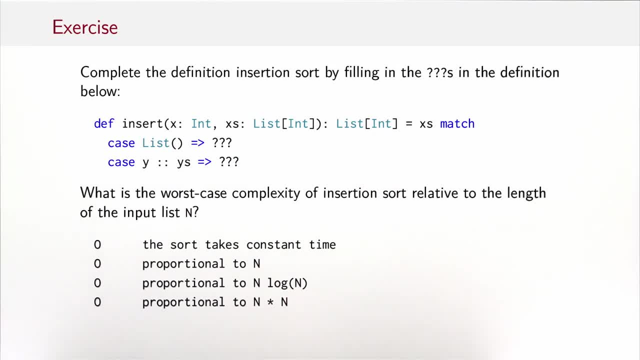 place returning a list of the new elements. So again, we do a pattern match over what kind of list it is. If we want to insert an element into the empty list, what would we get? Well, that's simply the list x, right? 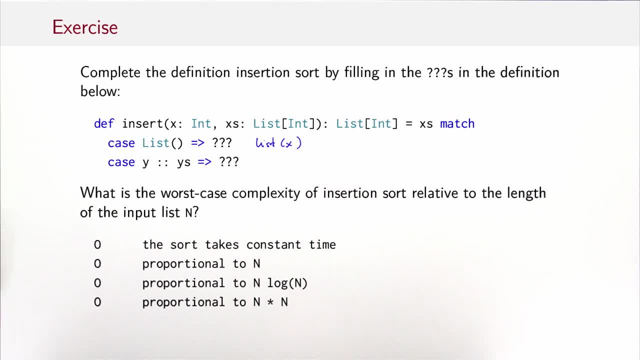 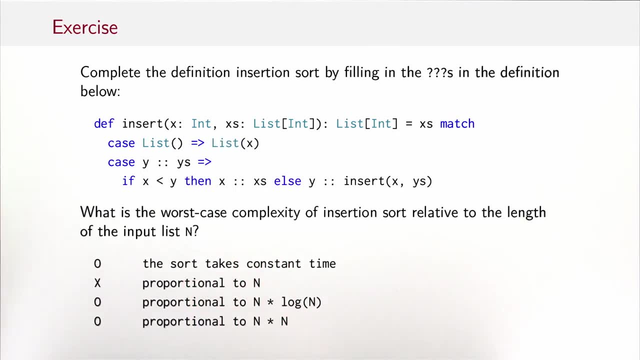 And what about if it's a non-empty list? So what do we need to do in the case where the list is not empty? Let's say it has a head y and a tail ys. Well then it depends whether the element we want to insert the x here. 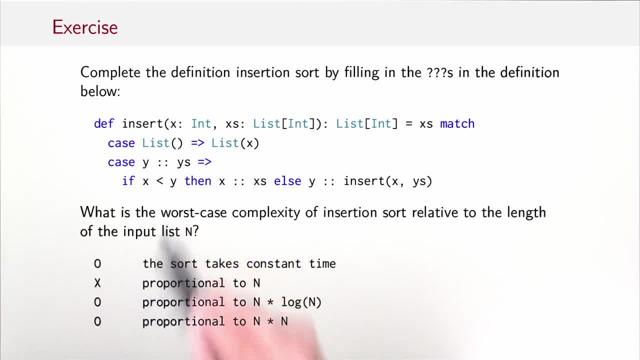 is less than y or greater or equal to y. If the element we want to insert is less than y, then it will be the first element of the result list, Because we start with smallest elements first. So we simply return x and then xs. 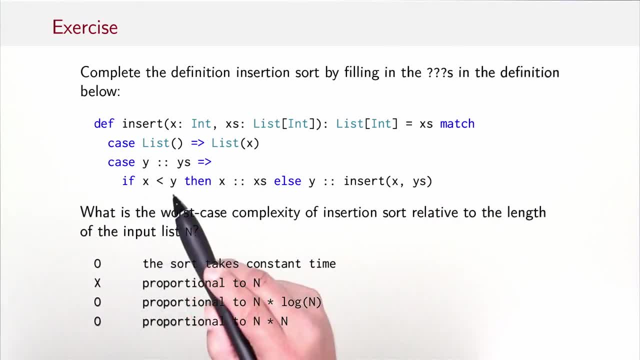 the list itself. If the element is greater or equal to the head element y, then the list keeps its old head element and we insert x recursively into the tail of the list. So that leads us to this else branch. Now, if we look at 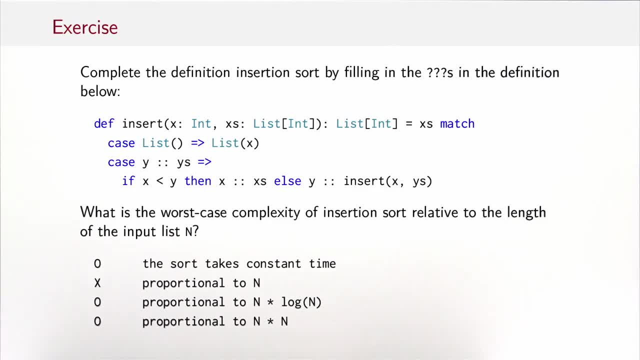 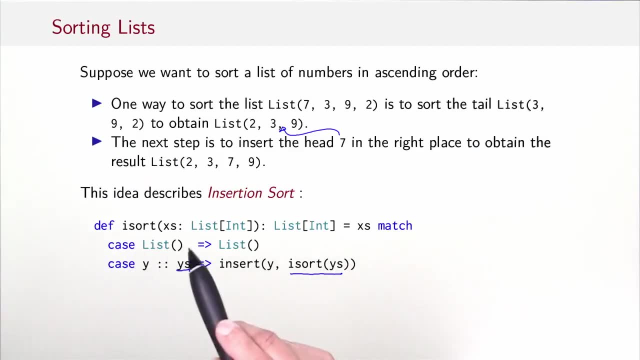 complexity. what's the worst case? complexity of insertion sort relative to the length of the input list n. So here we see that insertion sort would go linearly through each element, So it has one pattern match and one operation per element of the list And each. 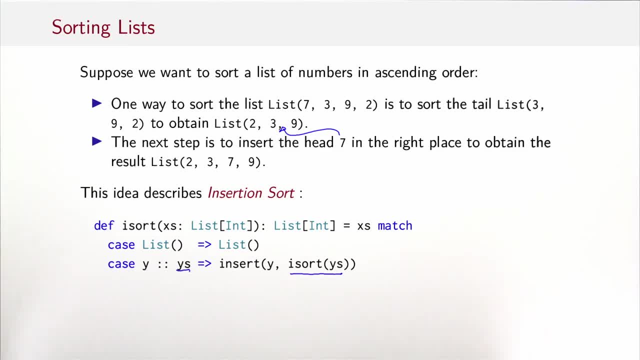 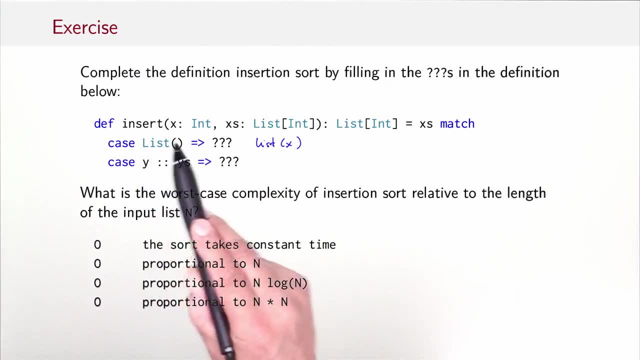 of those operations. calls the insert. call on the remaining list. So what's the complexity of insert? Well, insert is again its worst case. complexity is it has to go through the whole list And that would give a complete complexity proportional to n times n. 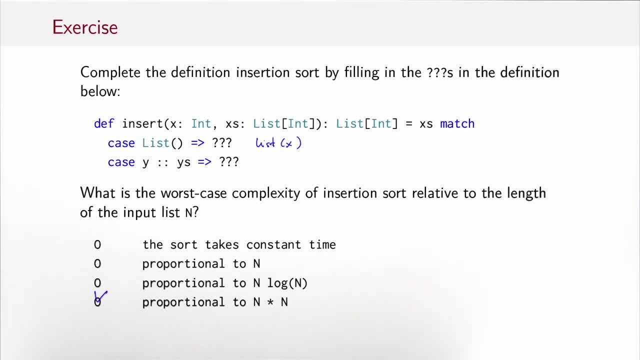 where n is the length of the list. So the first n comes from essentially having to insert each element of the outer list, and the second n comes from having to traverse the inner list, potentially up to n for the longest and then successively smaller ones, But it's still. 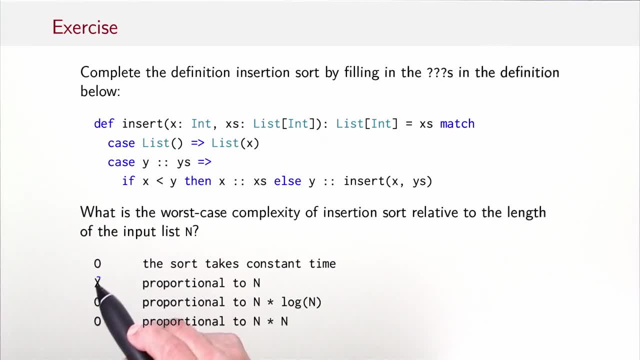 n times n. So here that's actually wrong, because the question was: what's the worst case complexity of insertion sort? So the worst case complexity of insert is proportional to n, and that means the worst case complexity of insertion sort is proportional to n times n. 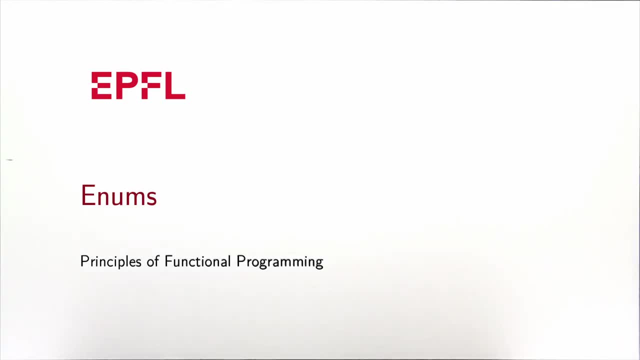 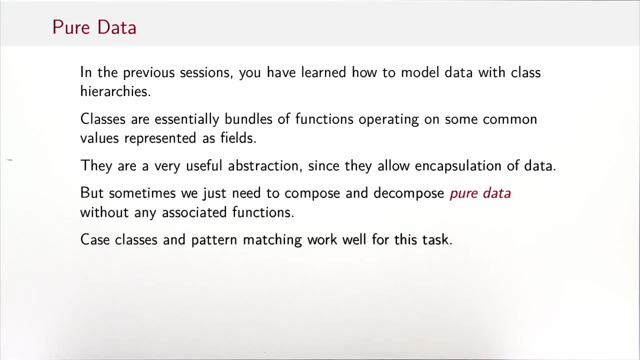 In this section, you'll learn about enums, which are a convenient way to construct data composed from cases. In the previous session, you've learned how to model data with class hierarchies. Classes are essentially bundles of functions that operate on common values that are represented. 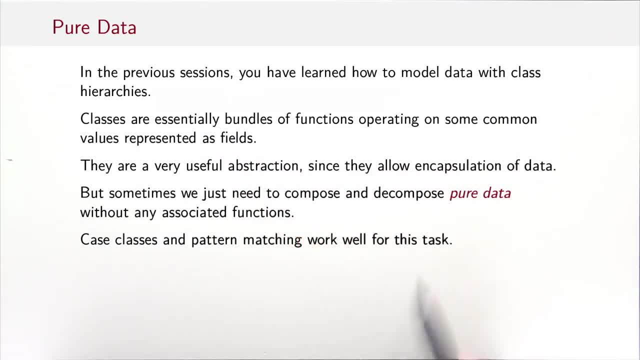 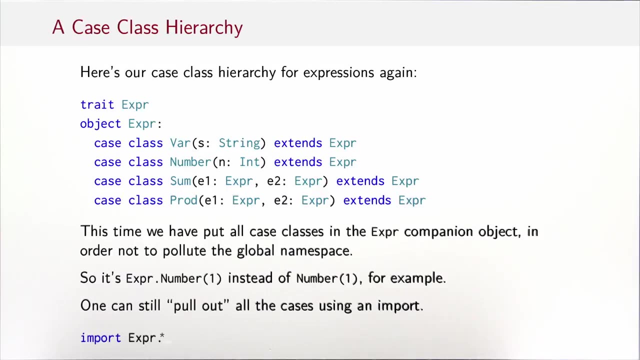 as fields. They are very useful abstraction, since they allow encapsulation of data, But sometimes we just need to compose and decompose pure data without any associated functions. Case classes and pattern matching work very well for this task. Here's our case class hierarchy for: 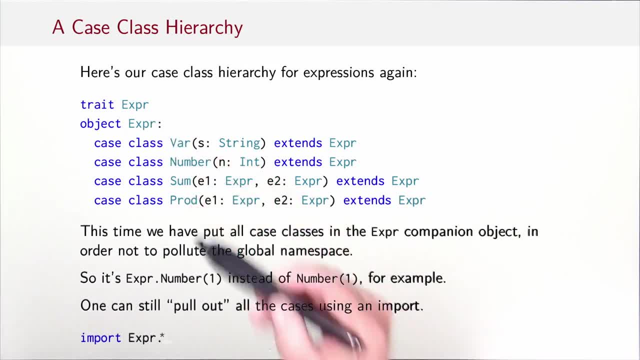 expressions. again, We have the base trait expression and then we have four case classes for variables, numbers, sums and products that all extend expressions. This time we've put all case classes in the expression companion object in order not to pollute the global namespace. 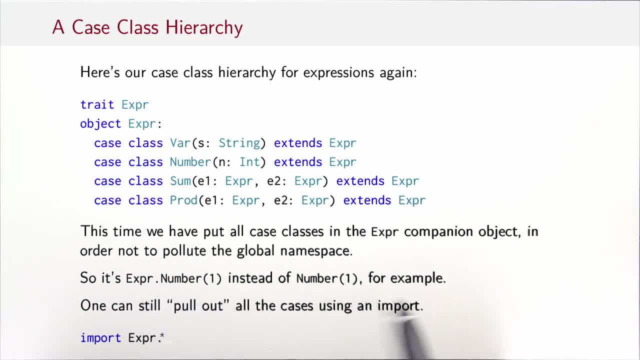 So here it's expression dot number one instead of just number one, for example. So that means the type number or var couldn't accidentally clash with something of the same name that we have defined on the outside. Of course, one can still pull out all the cases using an import. 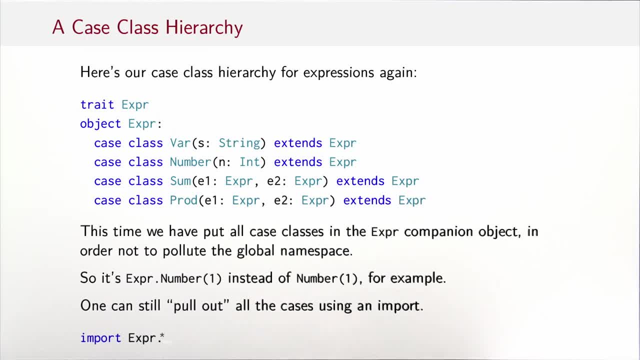 So you can write import expression dot underscore. That would pull out everything that's defined in object expression and make it available in the global namespace. So note that there are no methods in these definitions. All we've done is define some base trait and case classes that extend the. 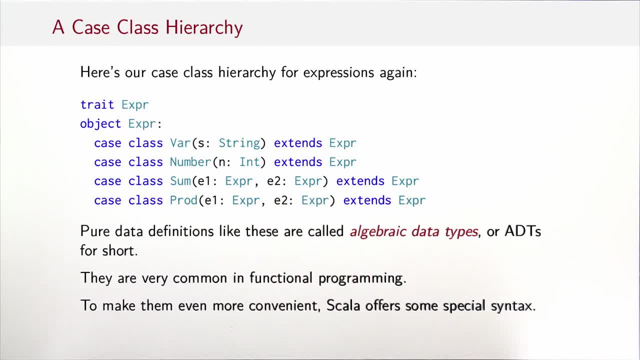 base trait and thus define in particular cases how data of the case trait can be constructed and pattern matched upon Pure data. definitions like these are called algebraic data types, or ADTs for short. ADTs are quite pervasive in functional programming. To make them even more, 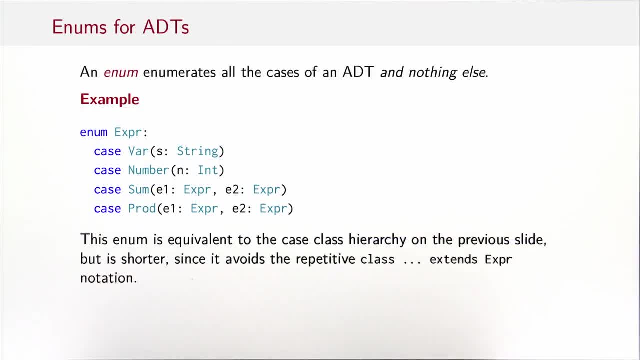 convenient. Scala offers some special syntax. What you can do, alternatively, is use an enum to define an ADT. An enum enumerates all the cases of an ADT and nothing else. So the way to do it here would be to write enum expression instead of the base trait and then 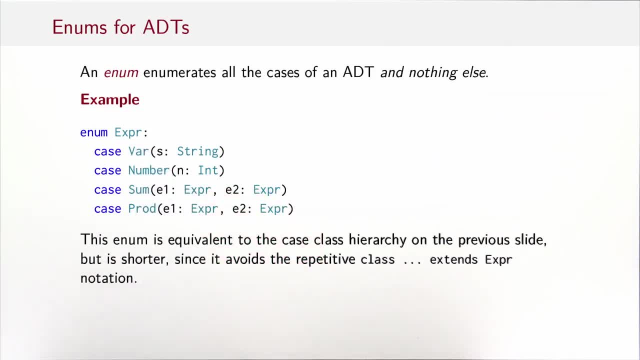 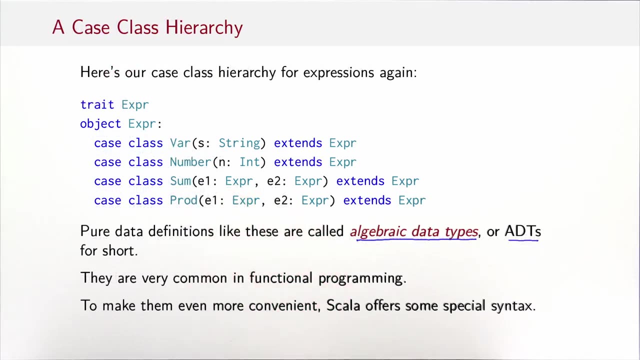 simply the cases var number sum prod inside. That enum is equivalent to the case class hierarchy of the previous slide, but it's shorter since it avoids the repetitive class blah extends expression notation. So that was the case class hierarchy and that's the equivalent enum. 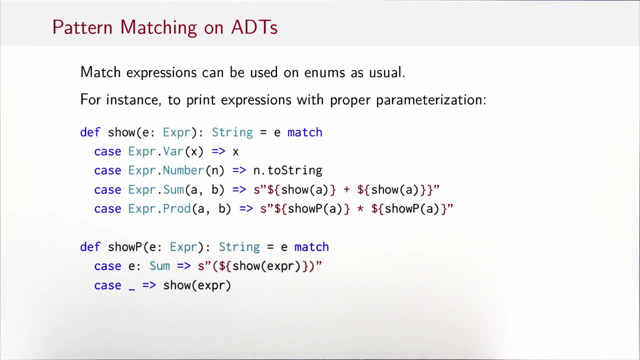 Since enums are just shorthands for case class hierarchies, we can use match expressions on them as usual, For instance, to print expression with proper parameterizations. we could use this show method here. This implementation is like the one we did in the exercise two sessions ago. 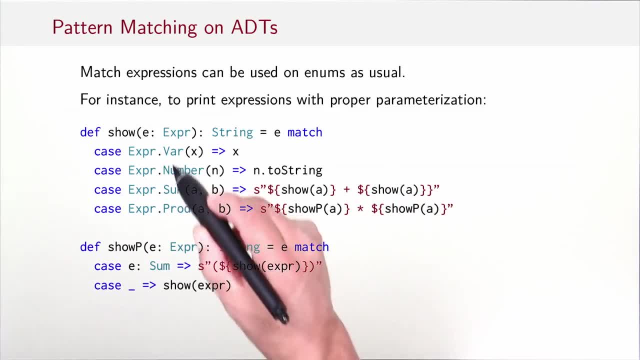 The only difference is that now, since the pattern, since the case classes are inside the expression object, I have to prefix them with expression dot, as you see here. Of course, I could also import the expression object like this, and then I could use the normal patterns which you can see. 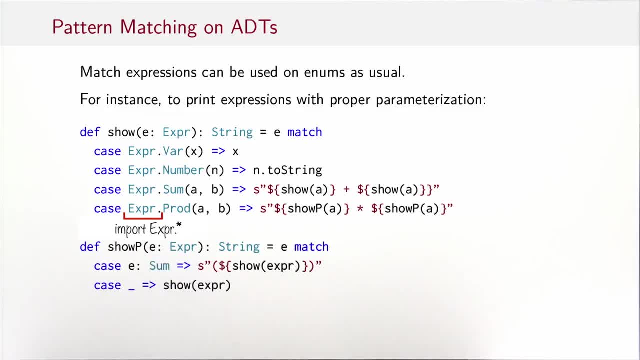 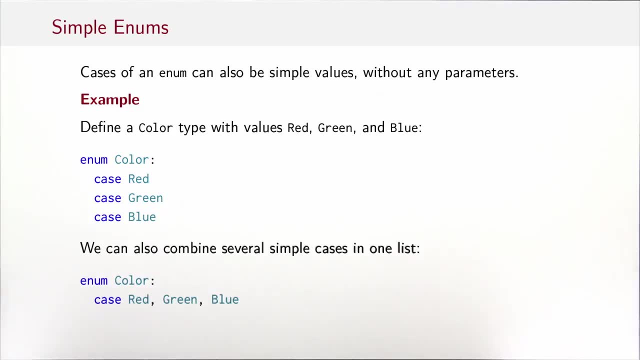 here in the show p method, where we used some without an expression prefix, Even simpler enums. The cases of an enum can also be simple values. so no case classes, just constants, in which case they wouldn't have any parameters. So, for instance, we can define a: 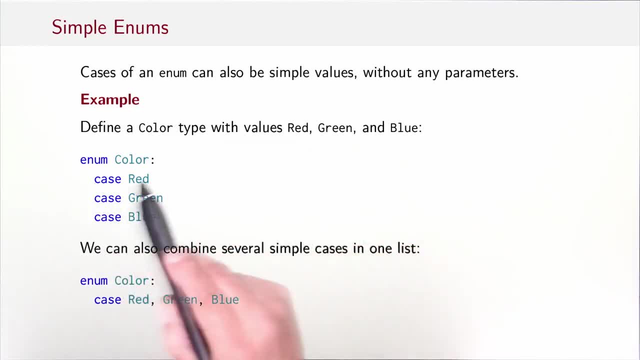 color type with values red, green and blue, like this: Enum color case red case, green case, blue, or even shorter, we can put the three cases on a single line. so enum color case red comma green comma, blue would give us a simple color type For pattern matching these simple cases. 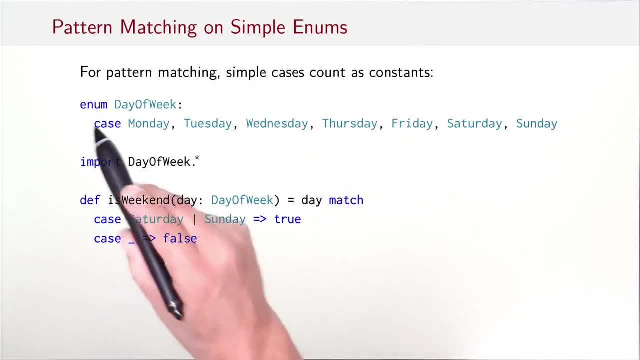 count as constants. So, for instance, I could define an enum day of week with the seven days I can import it, and then I could have a function is weekend that says it takes a day and matches the day. if it's a Saturday or a Sunday, it returns. 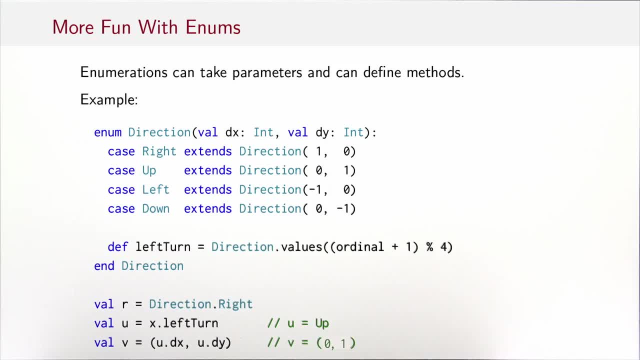 true and otherwise it returns false. Here's some more refinements of enums. Enumerations can also take a parameter and they can define methods. So here we have an enum direction that has two parameters, which have happened to be val parameters, dx and dy. 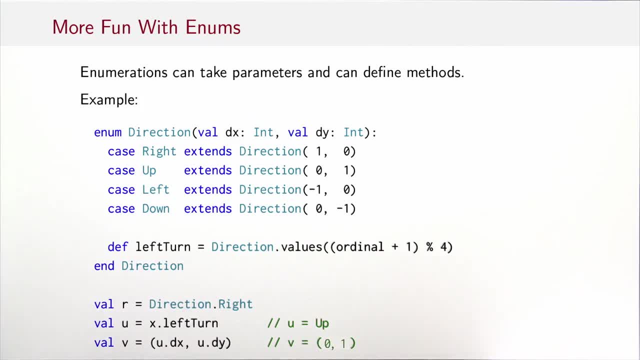 So that's the displacement in the x coordinate and the y coordinate. So right would be the direction, one zero, that's x, that's y, up would be zero, one, left would be minus one zero and down would be zero minus one. The other thing we define here is: 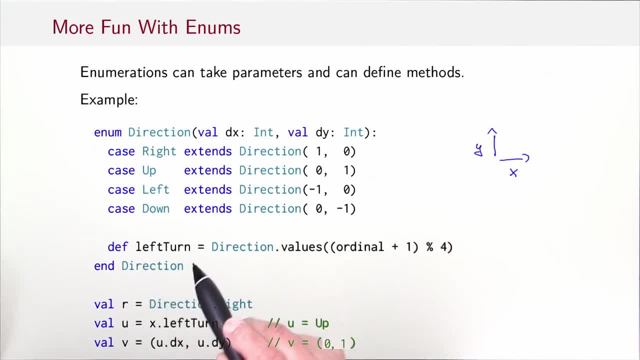 the method left turn, which is a method defined on enums of this direction type. The way we do it is that we make use of two auxiliary functions: ordinal and values. So ordinal is the ordinal number of an enum value. that's essentially just a number that starts. 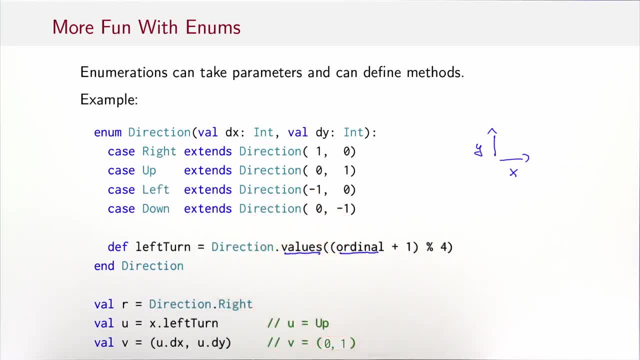 with zero and goes up one per case that we have defined. So what we do here is we take the ordinal number plus one, so the next one modulo four, so we have a wrap around and go from down to right And that gives us an integer number. 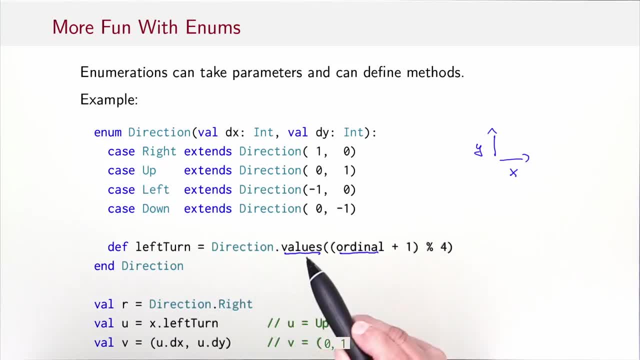 and then we can make use of the second method, which is called values. So values takes an int and gives us the enum that has the ordinal number that's given as the int. So in this case, left turn would be direction dot values of ordinal plus one modulo four. 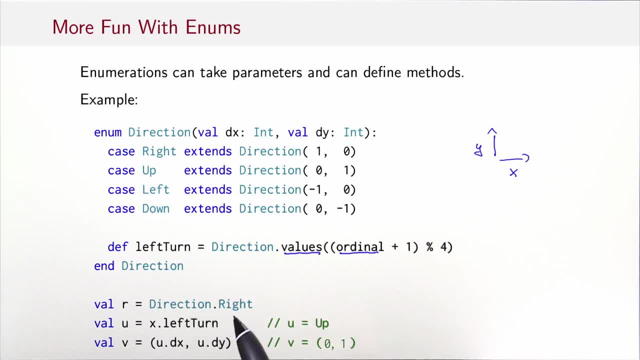 So let's do an example. Let's say we start with direction right and we want to do a left turn on that, So right has the ordinal number zero. So if the next ordinal number that we compute here is one and the direction values of one, 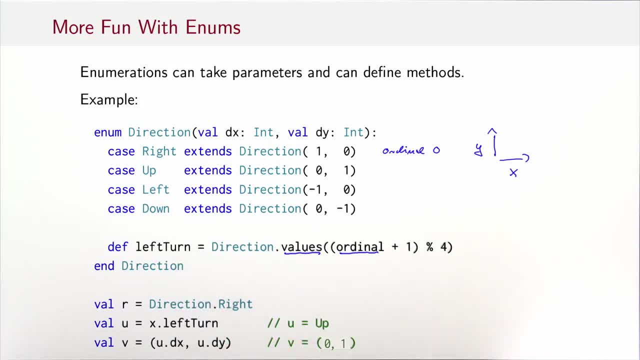 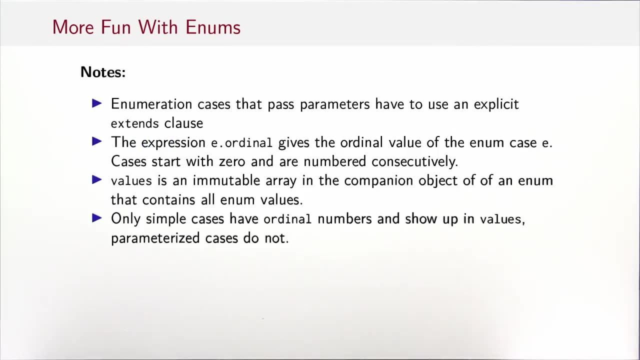 would be up. So we get up as the result of left, turn on right And then if we want to get the fields of the up value, So dx would be zero and dy would be one. So here are some further explanations for this example. 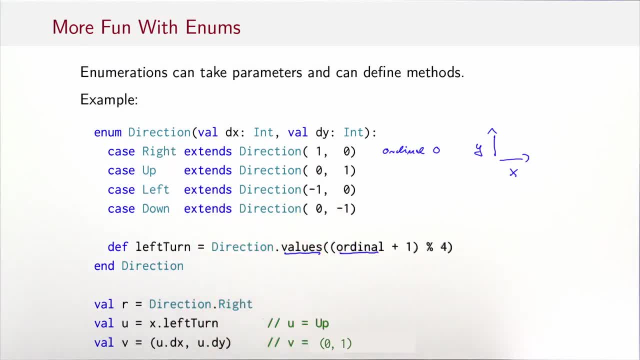 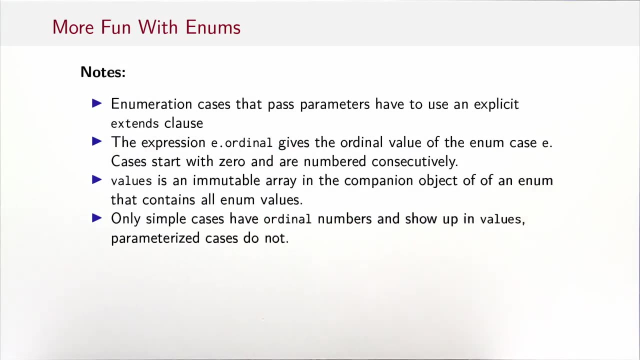 Cases that pass parameters to their enclosing enum always use an extends clause, So it extends direction, and then that's followed by the actual arguments for those parameters. Expression e dot ordinal gives the ordinal value of the enum case. e Cases start with zero and are numbered. 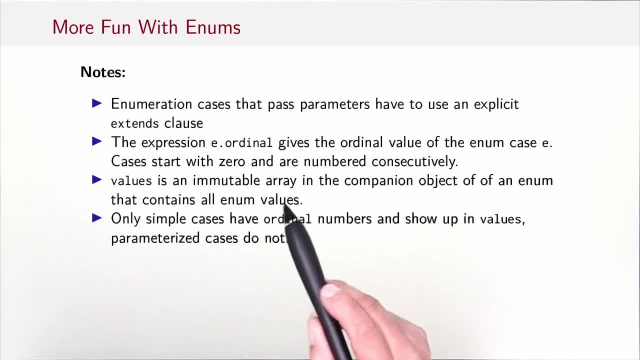 consecutively Values is an immutable array in the companion object of an enum that contains all enum values And furthermore, only simple cases have ordinal numbers and show up in values. Parameterized cases do not, because there's not a single value that represents a parameterized. 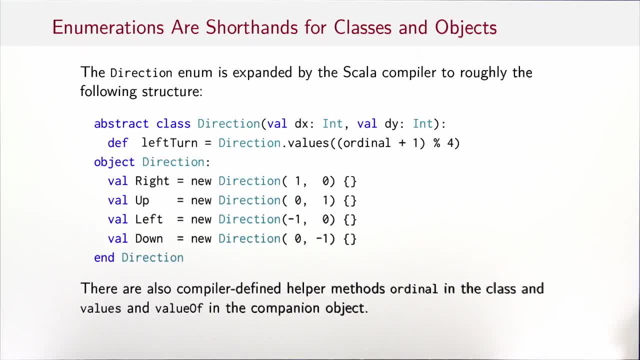 case. So you've seen that ADT enums are shorthands for class hierarchies with case classes. Similarly, enums with simple cases are shorthands for classes and simple values. So the direction enum that we've seen is expanded by the Scala compiler. 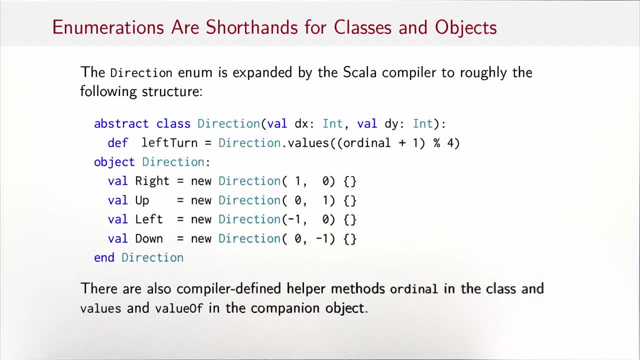 to roughly the following structure that you see here We have a base class direction that takes the parameters as given. So we would see a left turn here as the method And then in the companion object of direction we would have the four cases which in: 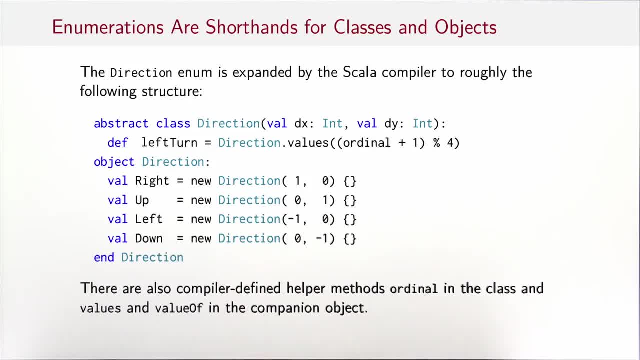 this case are all individual values, right up, left and down. Each value is an instance of an anonymous subclass, of class direction with the proper values for the parameters. And then, of course, there are also the compiler defined helper methods, ordinal in each case, and values, and 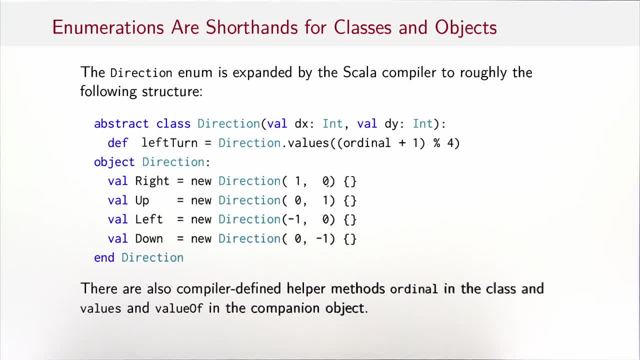 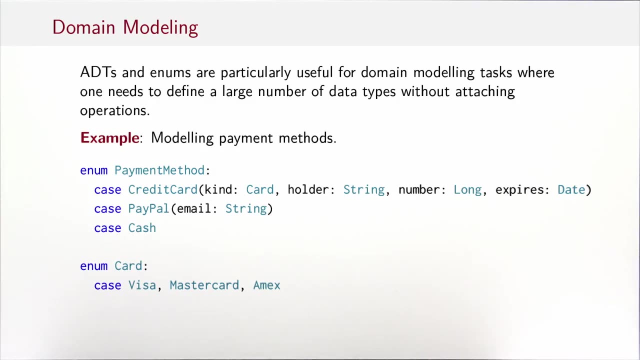 there's another method, valueOf in the companion object. valueOf lets you get the enum case that corresponds to a string which is the name of that case. ADTs and enums are quite common in more applied functional programs where the task is often to model. 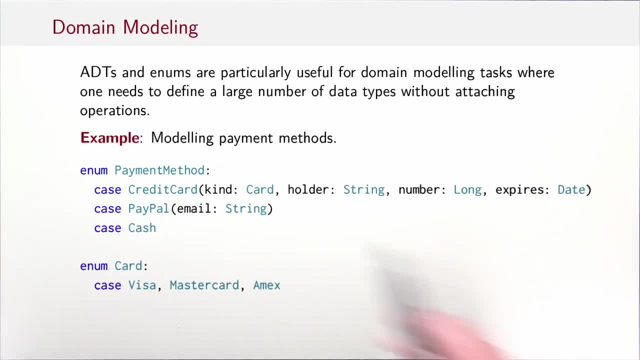 some domain. In that case one often needs to define a large number of data types without having to attach any operations. So as a small example of this, let's say we want to model payment methods. There could be an enum payment method where we could say: well, one payment method. 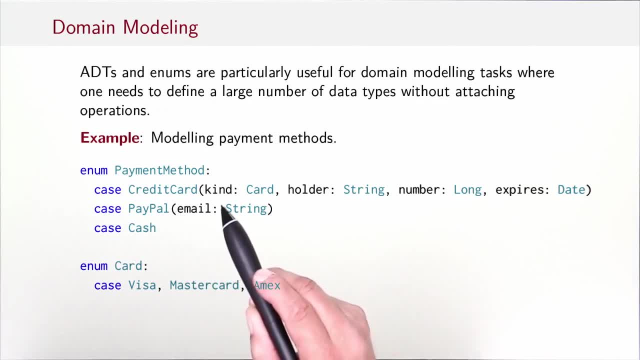 would be by credit card, in which case we want to know the kind, so what card it is, who's the holder, what's the number of the card and what's the expiry date. Or a payment method could be paypal, in which case we would want the email. 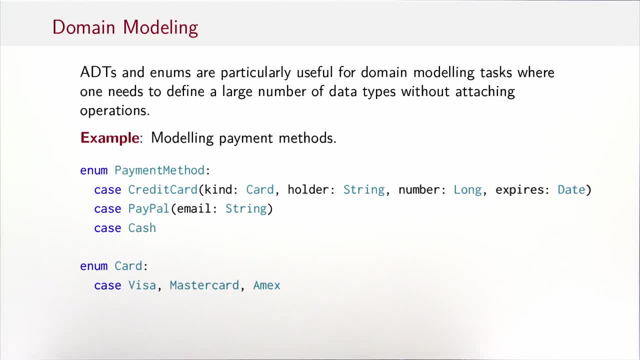 or a payment method could be cash. The most concise ways to write these things down is as an enum in the way you've seen here, Or here's a simple enum for credit cards, where we just say a credit card is Visa, Mastercard or Amex. 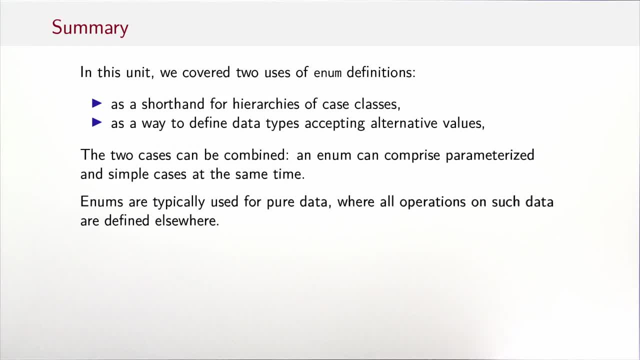 So, to summarize, in this unit we've covered two uses of enum definitions: First as a shorthand for hierarchies of case classes, in which case we talk about an ADT typically, And second, as a way to define data types that accept alternative values similar to enums in many other. 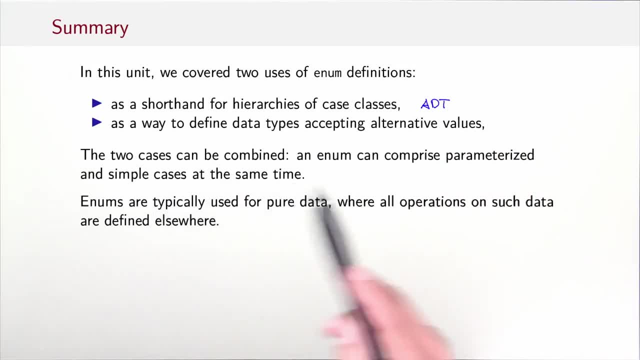 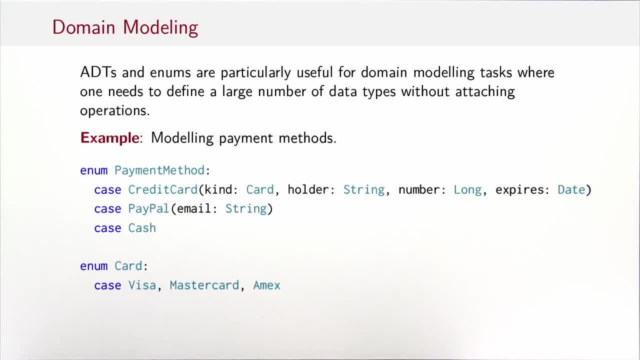 languages. The two cases can be combined in Scala. An enum can comprise parameterized and simple cases at the same time. We've seen an example in payment method where a payment method has two parameterized cases here credit card and paypal- and a simple case cash. 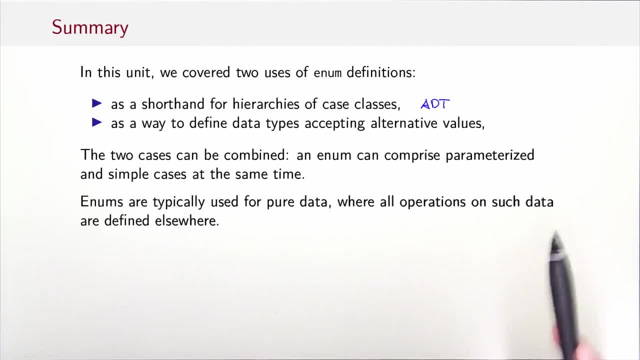 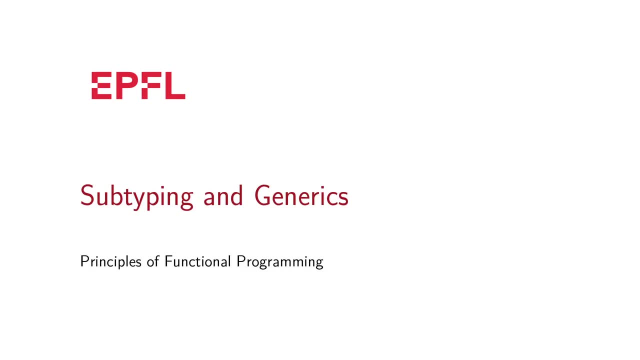 Enums are typically used for pure data, where all operations on such data are defined elsewhere. In this session, we're going to take a closer look at the interactions between subtyping and generics. We've already seen the two principal forms of polymorphism. One was subtyping. 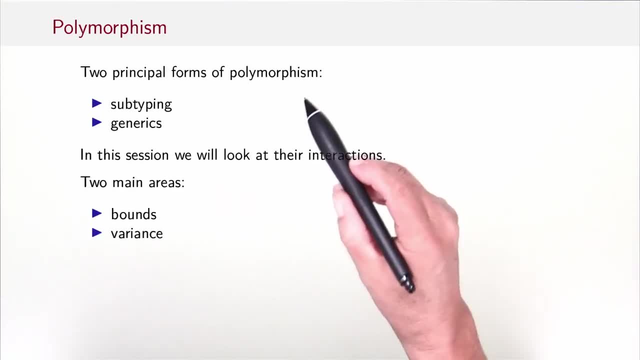 and the other was generics. In this session, we'll look at the interactions. In fact, there are two main areas of interactions. One is bounds of type variables and the other is variance. In this session, we'll look at the interactions. So let's look at type bounds. 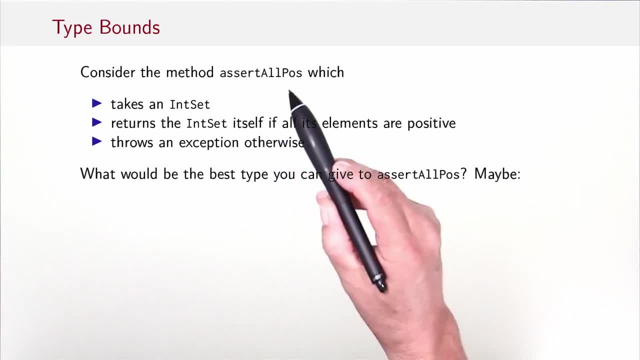 first Consider a method- assertAllPos- which takes an inset, returns that same inset if all its elements are positive and throws an exception otherwise. What would be the best type you can give to assertAllPos? Maybe this one: assertAllPos: it takes an inset and returns an. 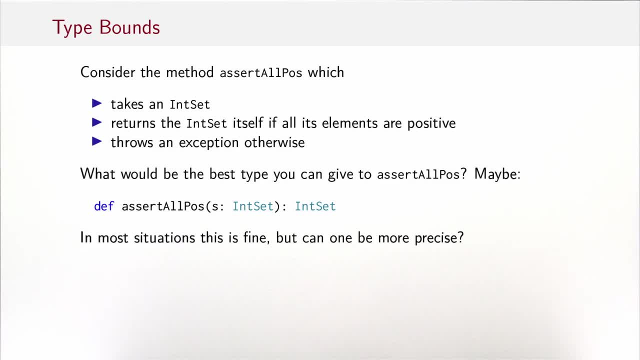 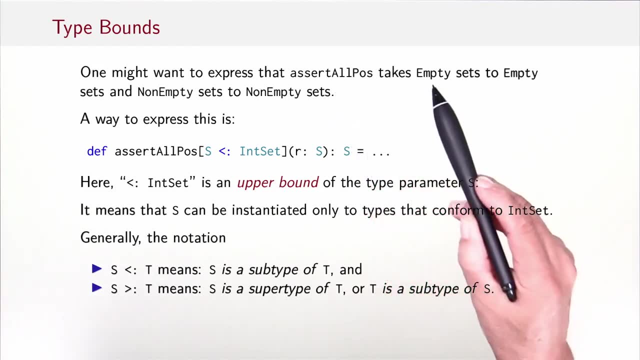 inset. In most situations this would be fine, but can one be more precise? Well, one observation is that assertAllPos would take empty sets to empty sets and non-empty sets to non-empty sets. If you want to express that in the type, then a way to do so is like: 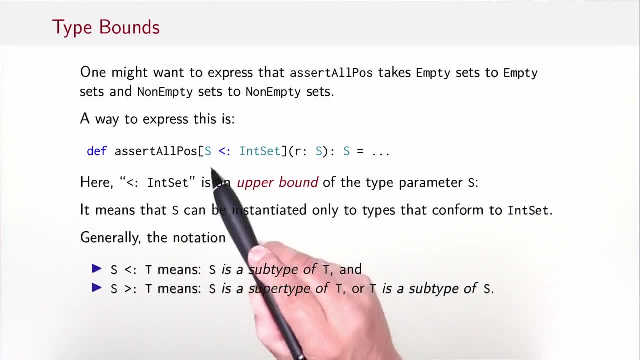 this We can say: assertAllPos takes a type parameter s, which must be a subtype of inset and a value r of type s, and it returns that type s. Here the less than colon inset is an upper bound of the type parameter s. It 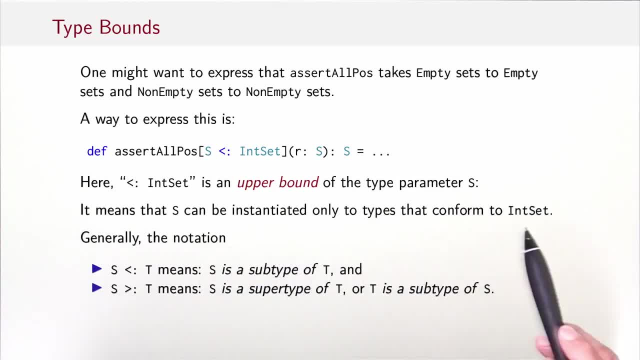 means that s can be instantiated only to types that conform to inset. So let's see what one can do with assertAllPos. Can one pass an empty set to it? Yes, because we can instantiate s to empty, and then the actual set is an empty set and we get back an. 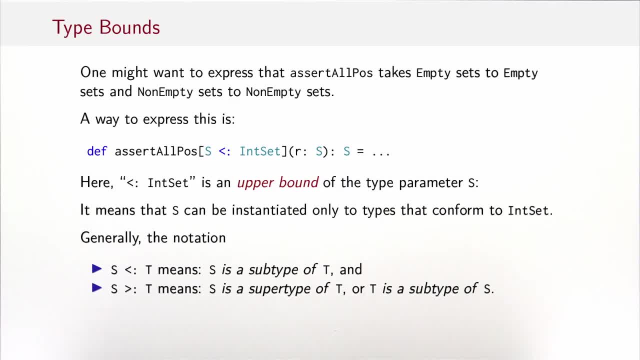 empty set, Can we pass a non-empty set to it? Yes, for the same reason. s can be instantiated to non-empty set, which is a subtype of inset, and we can pass a non-empty set and get back a non-empty set. So how is this new version assertAllPos. 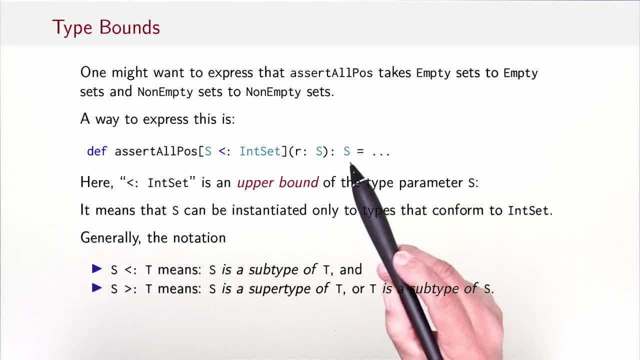 better than the old one. Well, in the return type, because now the return type is coupled with the parameter types. it expresses that whatever we put in, we get out. If we put in a specific subtype of inset, we get out that same inset. 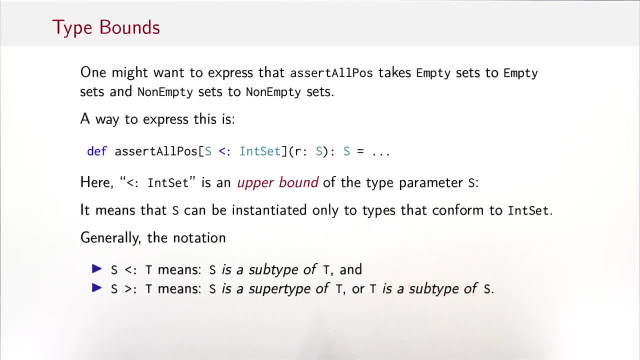 That was lost in the previous version, where the return type was always inset, so the information what kind of inset it was was lost. Generally, the notation s less than colon t means s is a subtype of t, and s greater colon t would then mean s is a supertype of t. 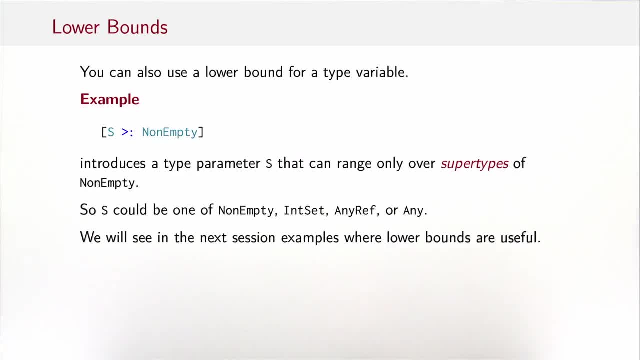 or t is a subtype of s. In fact, the supertype notation can also used as a bound and then it forms a lower bound. So you can write a lower bound for a type variable like this. So that would introduce a type parameter s that can range. 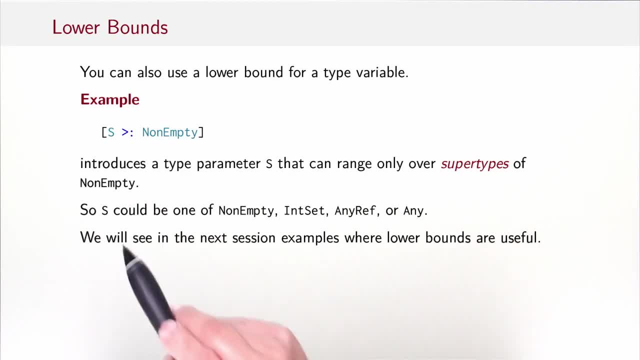 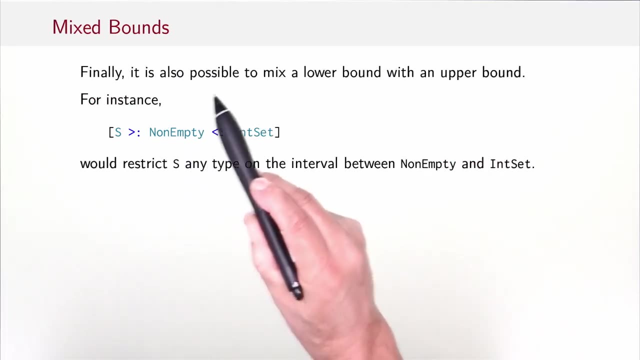 only over supertypes of non-empty. So specifically, s could be non-empty or inset, which is a supertype, or any ref or any. We will see in the next session examples where lower bounds can be very useful. Finally, and for completeness, it's also possible: 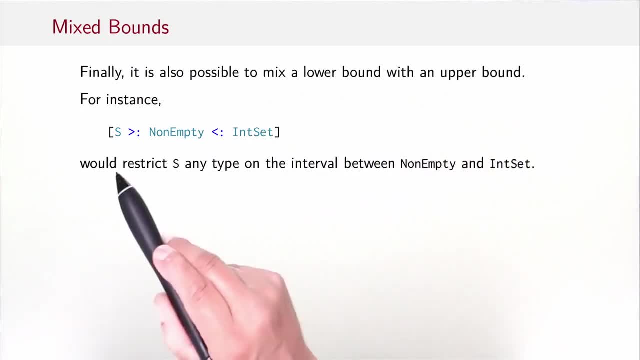 to mix a lower bound with an upper bound. In that case the lower bound comes first. So to write an s which is lower bounded by non-empty and upper bounded by inset, you would write s: greater colon non-empty, less colon inset. And that means: 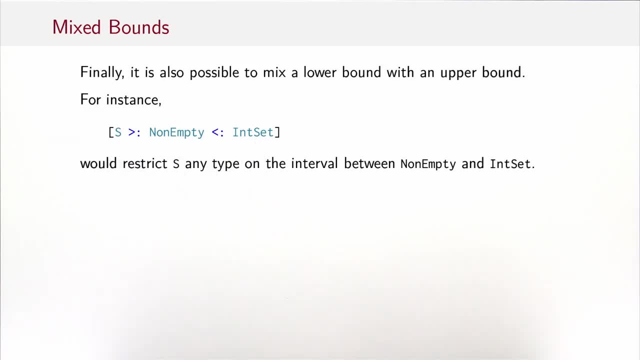 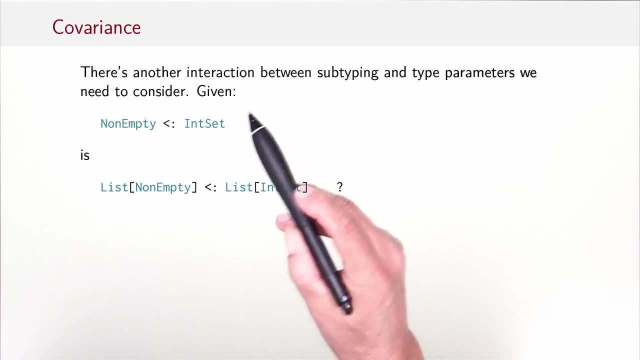 s can now be either inset or non-empty, but no other type. So much for bounds. Let's look at variance next. In fact, there is another interaction between subtyping and type parameters we need to consider, Given that non-empty is a subtype of inset. 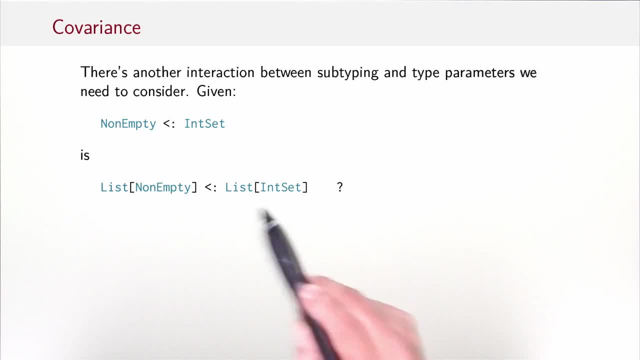 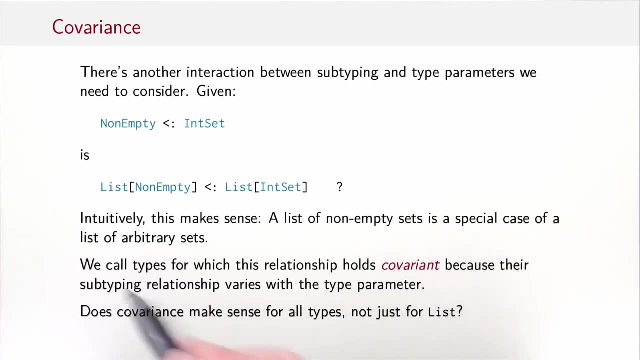 do we also have that? list of non-empty is a subtype of list of inset. Intuitively this makes sense. A list of non-empty sets is a special case of a list of arbitrary sets. We call types for which this relationship holds covariant because their 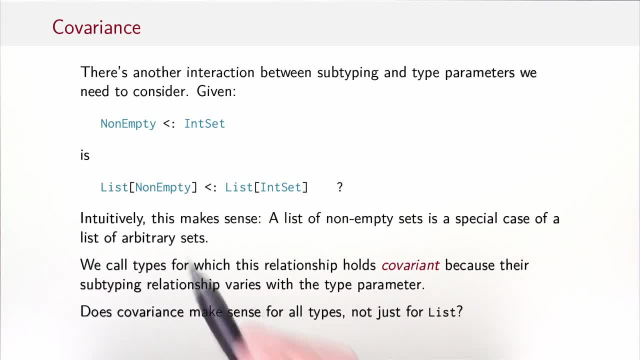 subtyping relationship varies with the type parameters. So if the type parameter goes up, then the type as a whole also goes up. They vary in the same direction and that's why they're called covariant. So one question that's fair to ask is whether covariance makes sense for. 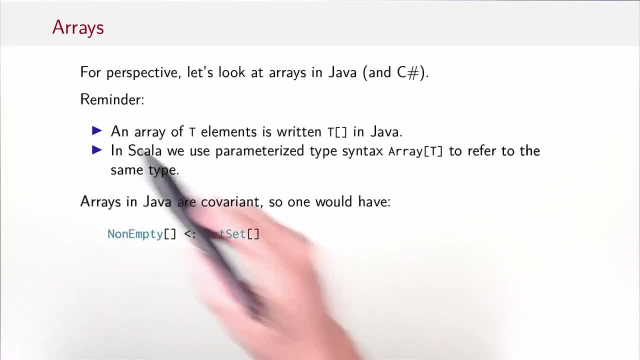 all types and not just for list. For perspective, let's look at arrays in Java and C-sharp, where they're similar to each other. As a reminder, an array of elements of type T is written T brackets in Java, and in Scala we use instead. 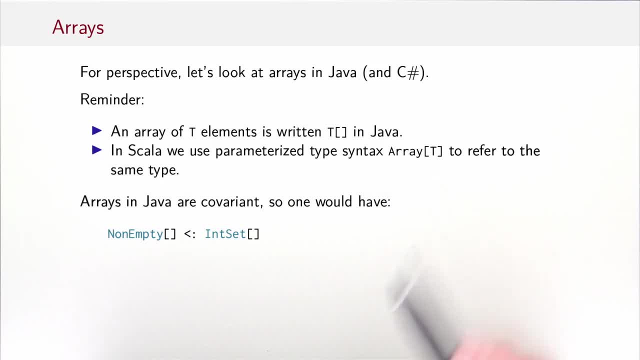 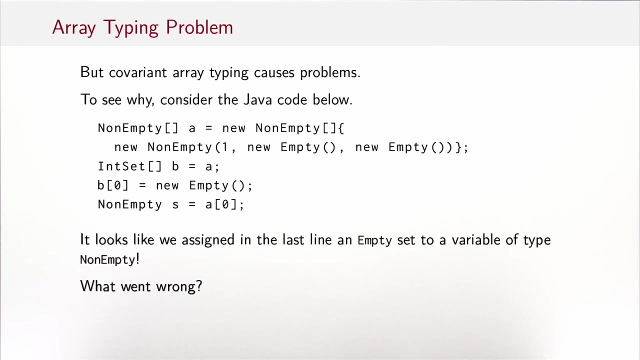 the parameterized type syntax array of T to refer to the same type. In fact arrays in Java are covariant. so one would have in Java that non-empty brackets is a subtype of inset brackets. But in fact that covariance rule for arrays causes a lot of. 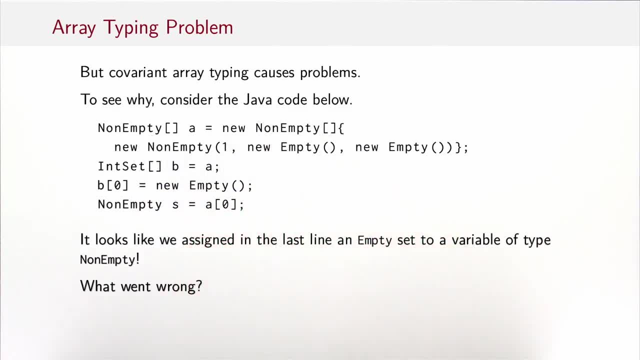 problems. To see why, consider the Java code below. We create a non-empty array which has a single element which is some non-empty set. We then assign that array to an array of insets. Then we create an empty array and put that into the. 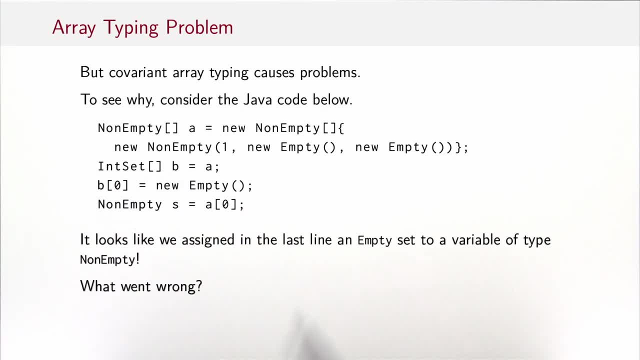 first element of the inset array B, And finally, we pull out the first element of the A array and put that in a non-empty set, S. Now what you need to know is, when we have an assignment of arrays in Java like this one here, then those two arrays really. 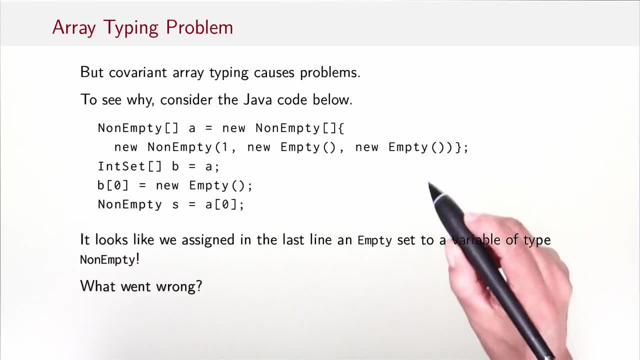 point to the same object. So after the assignment it would look like this: We would have the A array, which is an array which contains a single non-empty element, And the B array, which is an inset array, points to the same array. So by the third line, 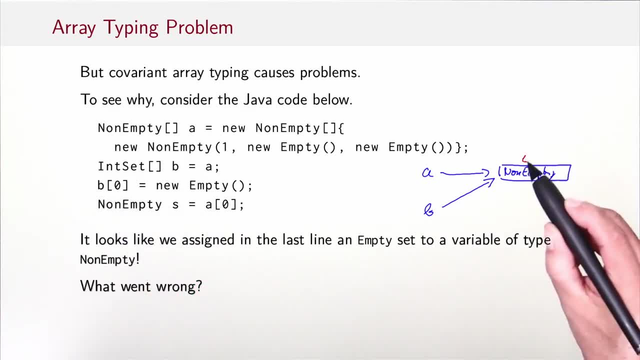 we don't have a non-empty element in the array anymore. The element here is now empty, And that means by the fourth line it seems that we assign an empty element into a variable of type non-empty, Which is of course a violation of type soundness. That means: 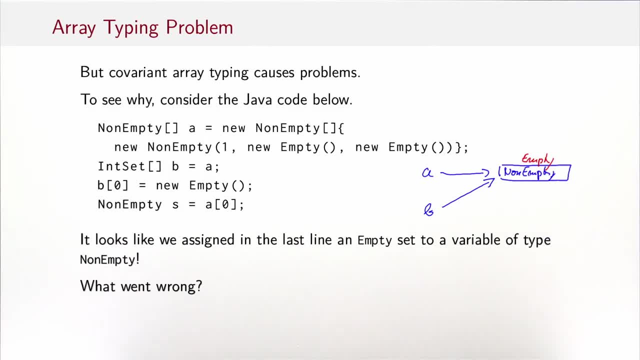 our type system lets us do something at runtime, which is clearly wrong. In fact, the Java runtime system patches this security hole by storing a runtime tag in arrays that remembers with what type it was created. So the non-empty array here would remember that the only non-empty 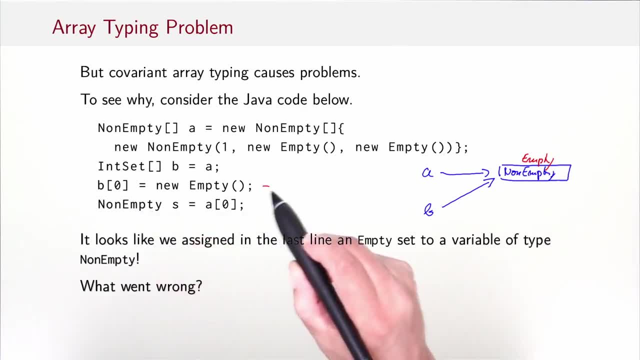 elements can be stored, And that means by the third line, this one. here you would actually get a runtime error similar to a class cast exception that says: well, you can't store an empty element in an array that was created by non-empty, But that's still. 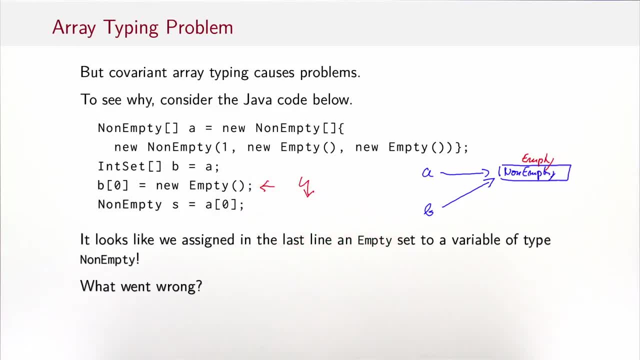 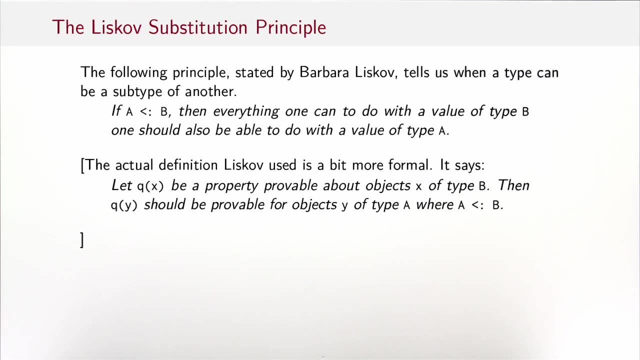 troubling because we write something which looks completely reasonable and the end result is a runtime error, which is an array store exception similar to a class cast exception. So those things normally shouldn't happen. So now we're confused. Arrays can be covariant in Java. 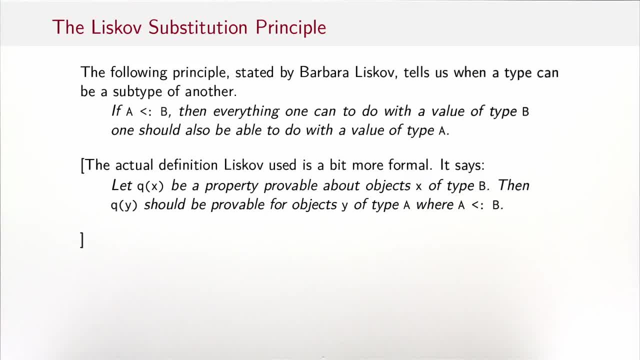 but when we use that, then we get into trouble: runtime exceptions. So when is it sound to state that a type should be a subtype of another type? In fact, we can base reasoning on a principle that was first stated by Barbara Liskov, which tells: 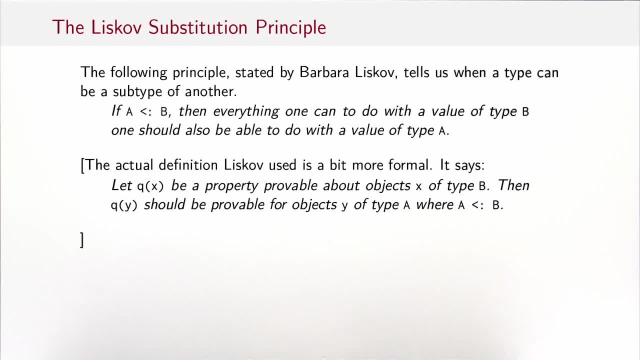 us when a type can be a subtype of another. The principle says: if A is a subtype of B, then everything one can do with the value of type B, the supertype, one should also be able to do with the value of type A. 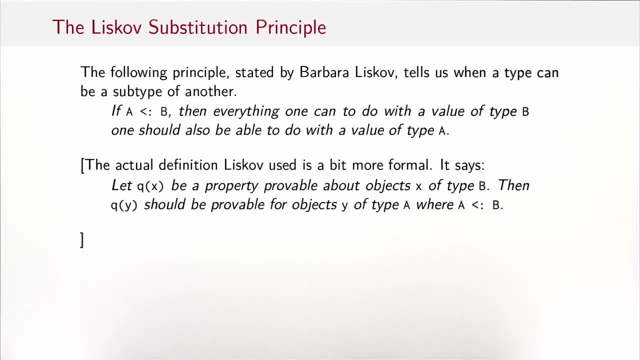 So it means everything I can do with B. I can also do with the subtype A and potentially I can do more things with A. In a sense, A is better than B. It can fulfill every role that B plays, plus potentially more. The actual definition. 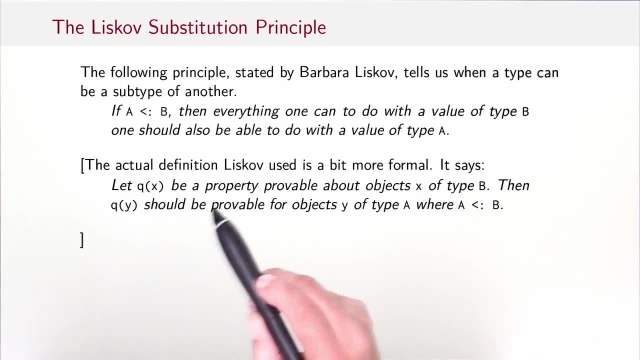 Liskov used is a bit more formal. It says that Q are property provable about objects X of type B. Then Q of Y should be provable for objects Y of type A, where A is a subtype of B. So these characterizations. 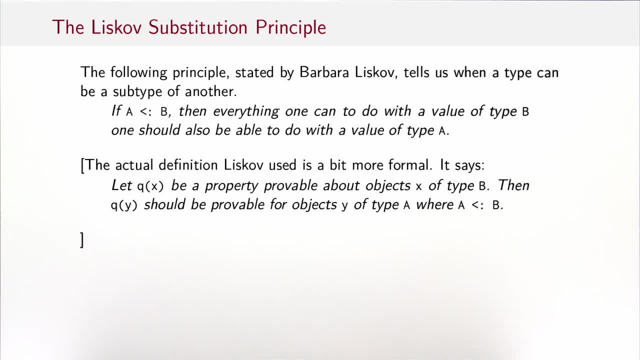 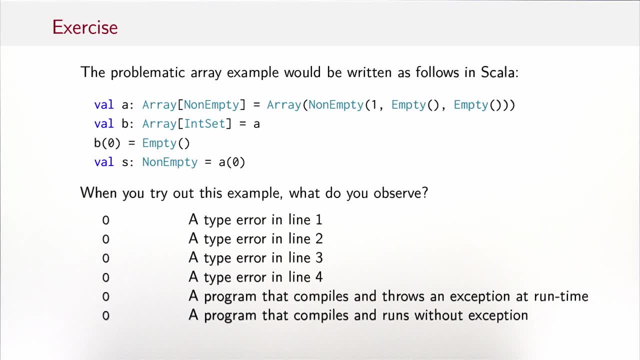 together have the name Liskov substitution principle. Now consider arrays again. Can an array of non-empty be a subtype of an array of int set? That would mean that everything I can do with an array of int set, I can also do with an array. 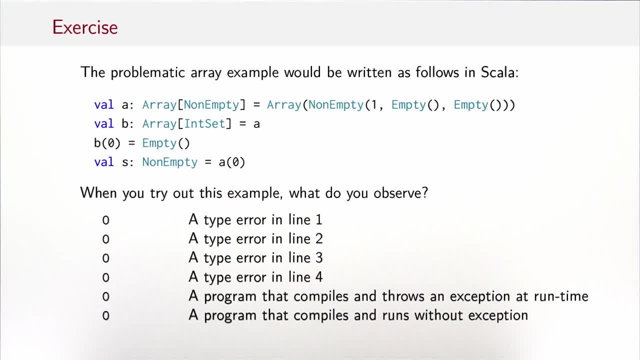 of non-empty. But if you think about it, there is one thing I can do with an array of int set that I cannot do with an array non-empty, and that's store an empty set in it. I can store an empty set in an array of int set. 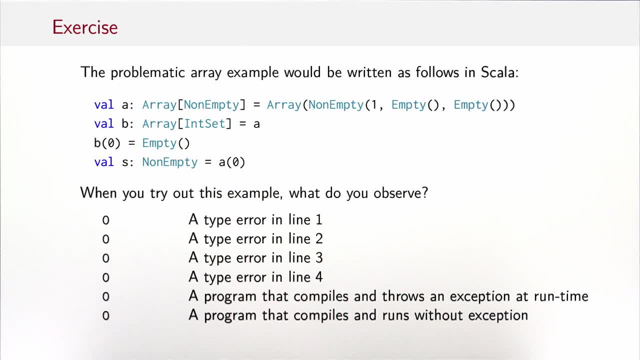 but it's definitely not in an array of non-empty. So by that logic arrays cannot be covariant, because covariance of arrays would violate the Liskov substitution principle. So let's look at the example again. in Scala, What do you think If you see the same four? 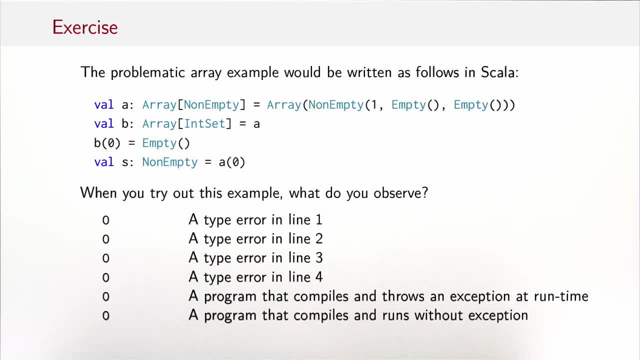 statements that we've seen before in Java but now written in Scala. would you observe a type error And, if yes, in what line? Or would the program compile and maybe throw an exception at runtime, like it does in Java, Or would the program compile and run without? 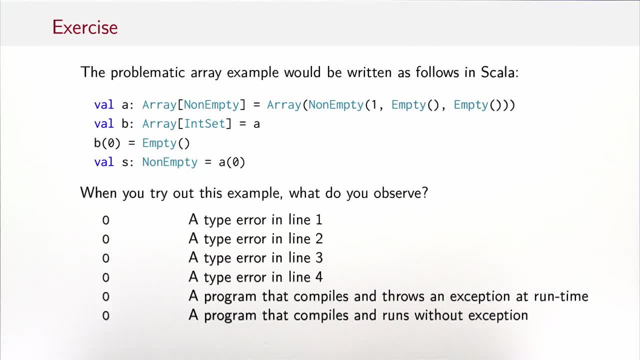 exception. In fact I've already given it away since, I said, arrays cannot be covariant in Scala. That means that that assignment here, that assigns an array of non-empty to an array of int set, that's illegal Because an array of non-empty 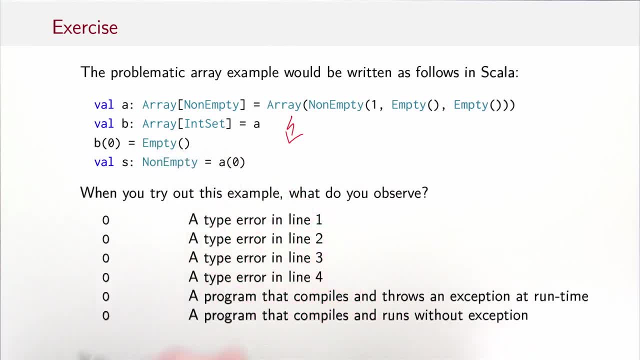 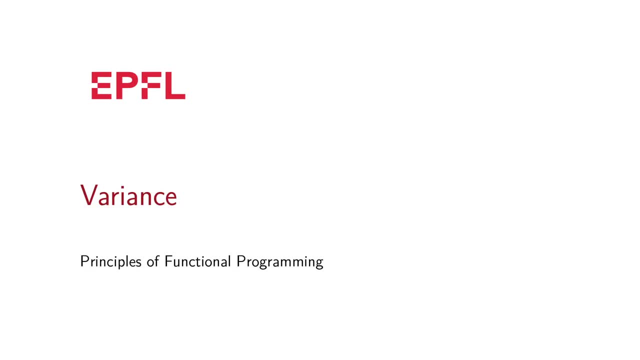 is not a subtype of an array of int set, So we would get a type error in line 2.. In this session we are going to take a closer look at variance, how variance is computed and how you can structure your program to make them variance correct. 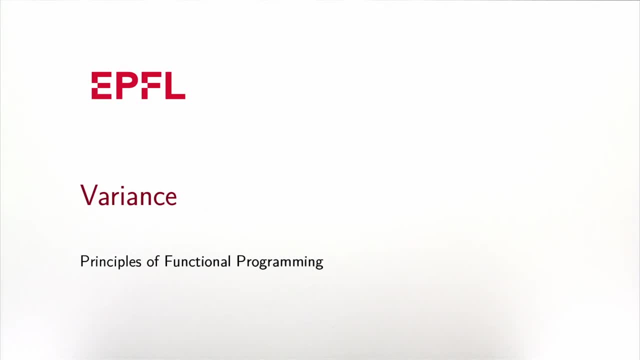 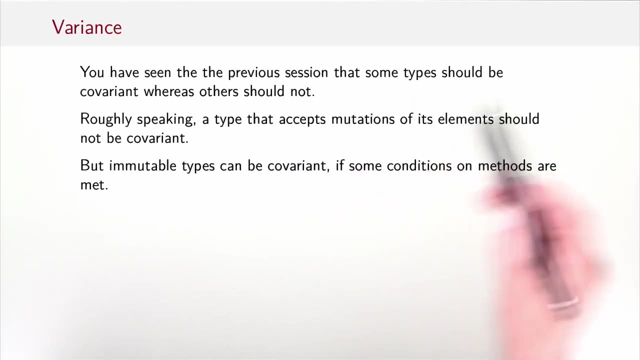 The material in this session is a bit more advanced than the other sessions so you can also skip it in a first pass through that course. So we've seen in the previous session that some types should be covariant whereas other types should not Roughly. 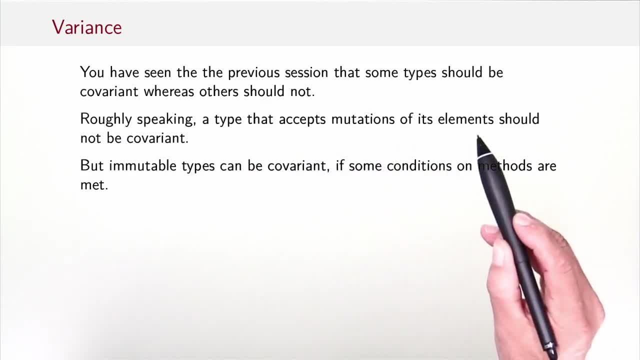 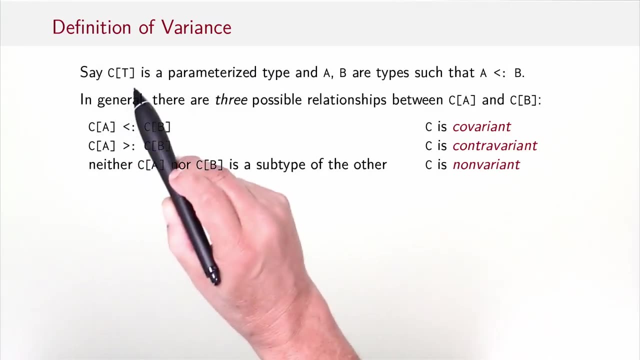 speaking, a type that accepts mutations of its elements, like array did, should not be covariant. But immutable types can be covariant if some conditions on methods are met. Before we go on, let's define what we mean by variance. Say C is a. 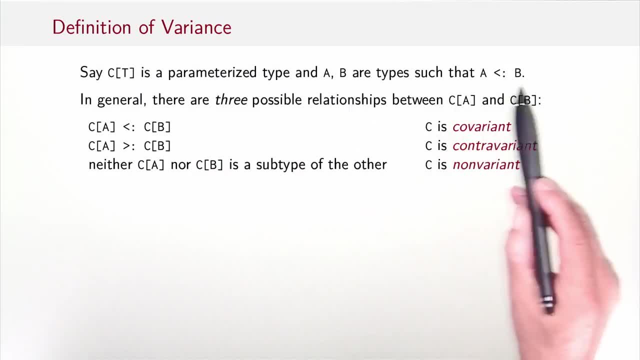 parameterized type and A are types such that A is a subtype of B. In general, there are three possible relationships between C of A and C of B. C of A could be a subtype of C of B. We say then: C is covariant. 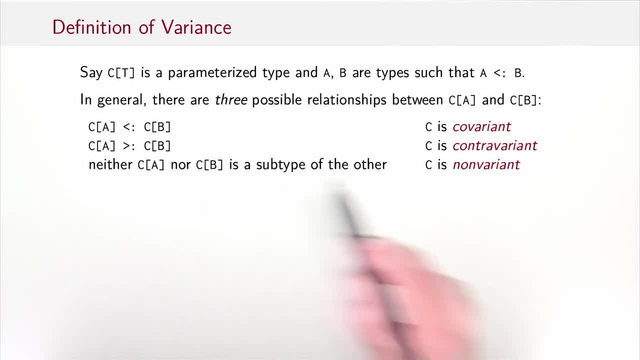 Or C of A could be a supertype of C of B. Then we say C is contravariant, Or neither C of A nor C of B is a subtype of the other. Then we say C is nonvariant. So covariant means the application. 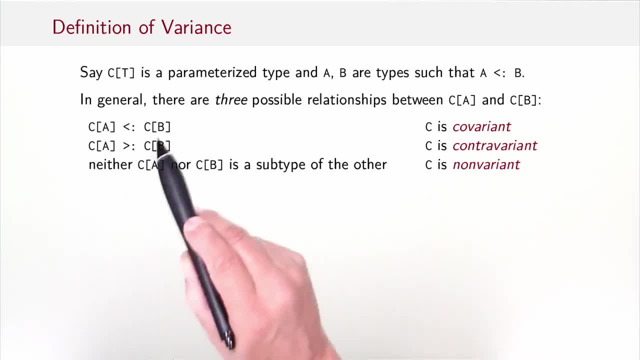 with C varies in the same direction as the elements. contravariant means it varies in the other direction, and nonvariant means the two types are unrelated. In Scala you can declare the variance of a type by annotating the type parameter. So you can declare a. 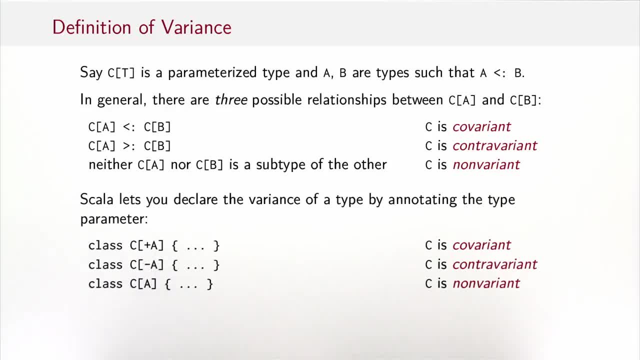 class to be covariant by writing a plus in front of the type parameter- A in this case- Or for contravariant classes, you would write a minus in front of the type parameter. If you don't write anything, then the class is assumed to be nonvariant. 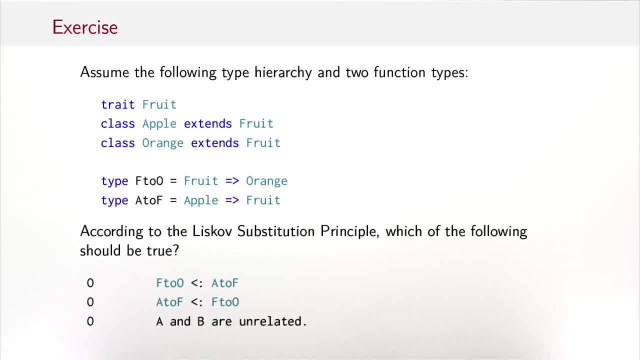 So here is an exercise that requires some thought. Let's say we have a type hierarchy- fruit- with subclasses for apples and oranges, And then we have two functions: One converts a fruit to an orange and the other takes an apple and returns a fruit According. 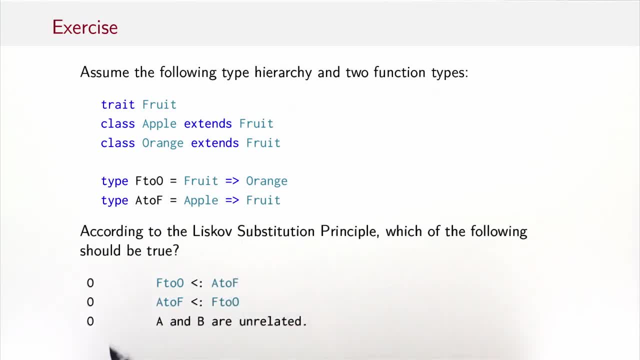 to the Liskov substitution principle, which of the following should be true: Should fruit to orange be a subtype of apple to fruit, Or should apple to fruit be a subtype of fruit to orange, Or should the two types be unrelated? So let's look at the first subtyping. 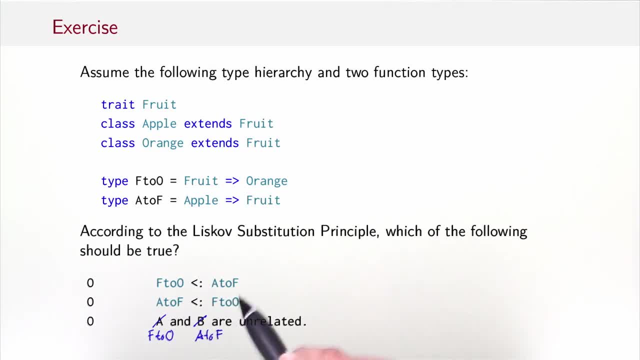 relationship. What can I do with the second function, apple to fruit? Well, I can pass it an apple and obtain a fruit. Can I do the same thing with the first function? Yes, you can pass an apple to the first function. Apples are fruit And. 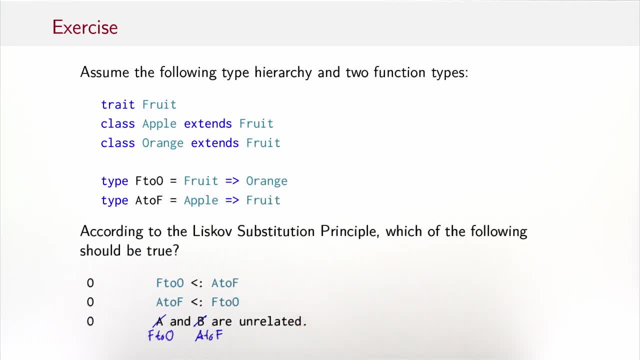 you will obtain a fruit, because oranges are fruit as well. So this one seems to be true. What about the second relationship? Is apple to fruit, a subtype of fruit to orange? Well, what can I do with the fruit to orange function? I can pass it a. 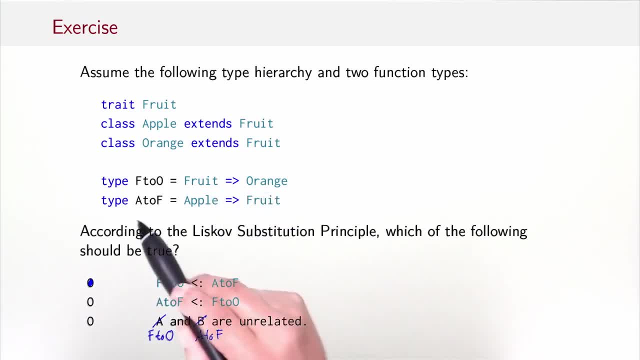 fruit and obtain an orange. Can I do the same thing with the second function? No, because the second function requires an apple To the first function. I could also pass an orange. Oranges are fruit, but oranges are not apples, So I can't. 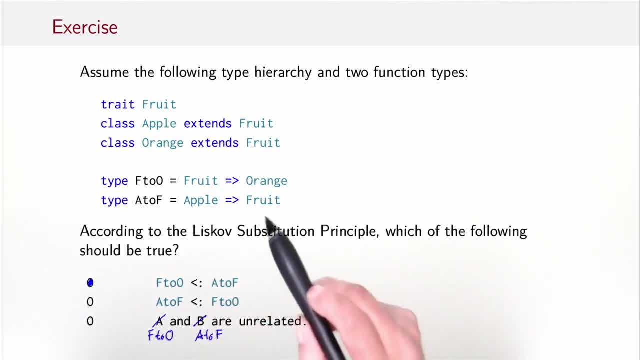 pass the same things to the second function. Furthermore, the second function actually returns a type that is less precise than the first one. The first guarantees to give back an orange, whereas the second only guarantees to give back some fruit. It could be an. 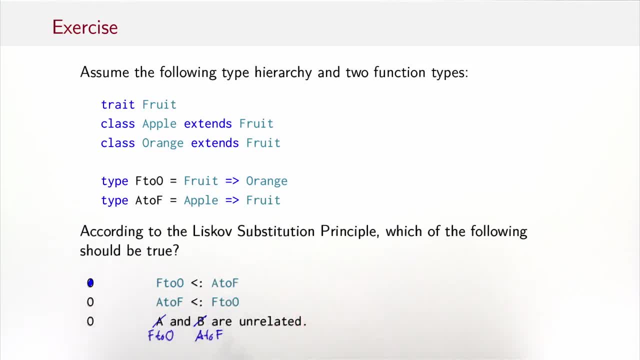 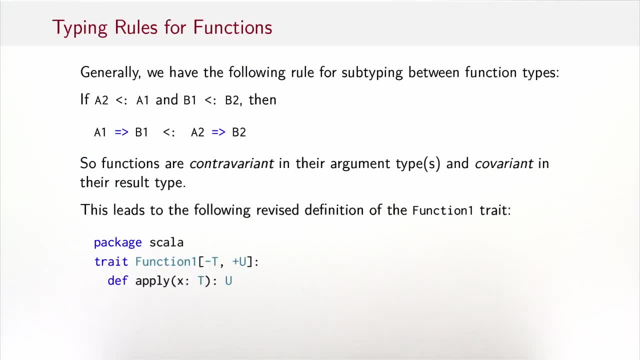 orange, but it could also be an apple. So that relationship is not true And so the correct answer is one in this case. So we can generalize from that reasoning to arrive at a rule for subtyping between arbitrary function types. Here's the rule. 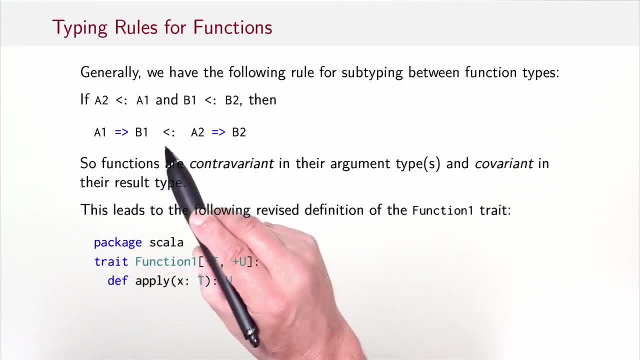 We say the function type A1, arrow B1, is a subtype of the function type A2, arrow B2. if B1 is a subtype of B2, so that's covariant And the arguments there. it goes in the other way: A2 must be a subtype. 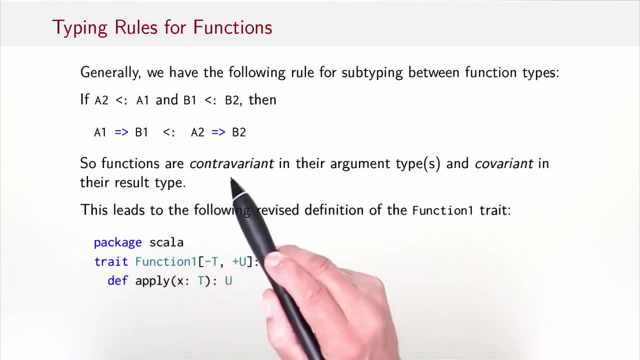 of A1.. So functions are contravariant in their argument types and covariant in their result type. So that means that if we want to come up with a revised definition of the function, one trait that takes account of variance, we have to write it like this: 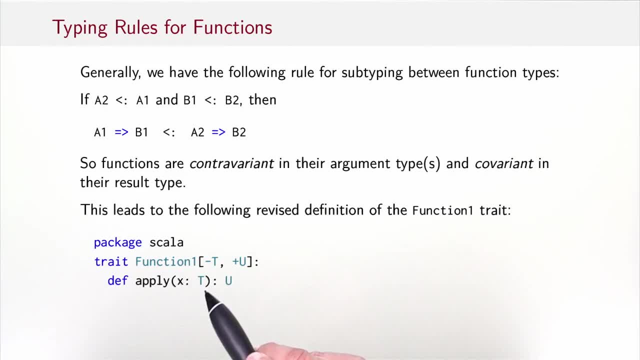 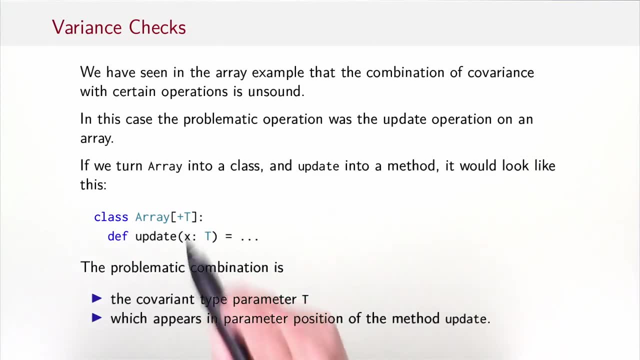 Function. one is contravariant in its argument, type T- and covariant in its result, type U. So how does the compiler verify whether your variance annotations are correct? We've seen in the array example that the combination of covariance with certain operations is unsound In this case. 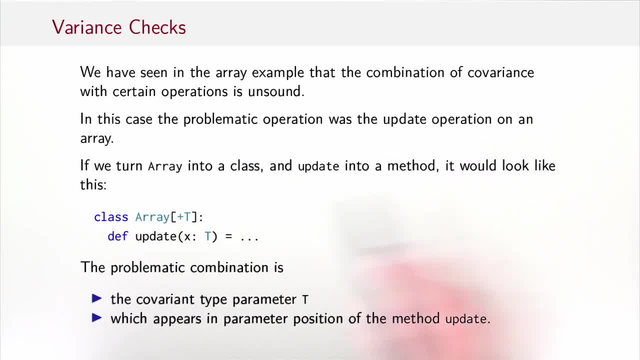 the problematic operation was the update operation on an array. If we turn array into a class and update into a method, it would look like this: Class array- let's assume it should be covariant- and then we have the update method that takes a parameter. 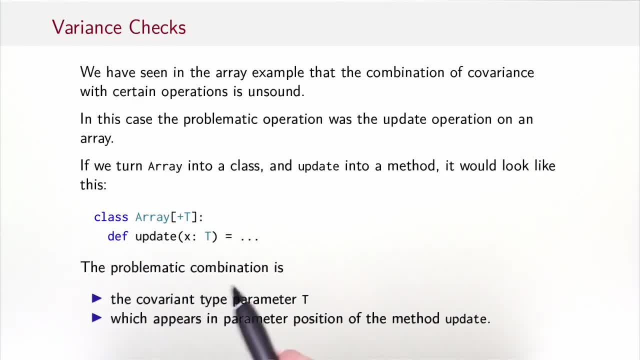 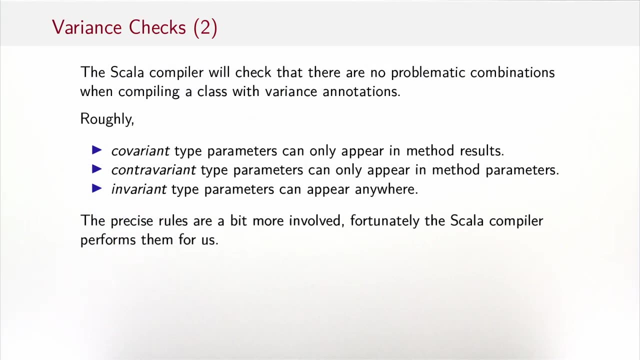 x of type T. The problematic combination here is the covariant type parameter T which appears in parameter position of the method update. So that led to problems and that's probably something that the compiler should disallow. So the Scala compiler will check that there are no. 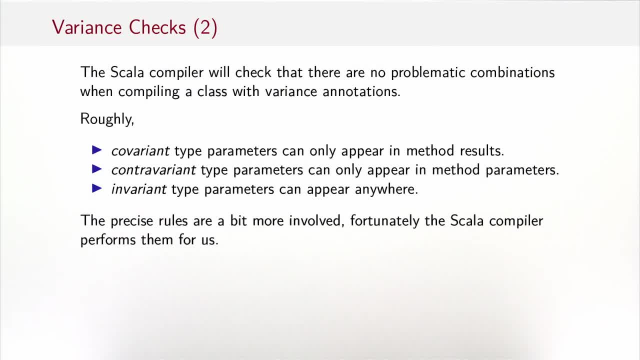 problematic combinations when compiling a class with variance annotations. Roughly covariant type parameters can only appear in method results, contravariant type parameters can only appear in method parameters and invariant type parameters can appear anywhere. The precise rules are a bit more involved, but fortunately 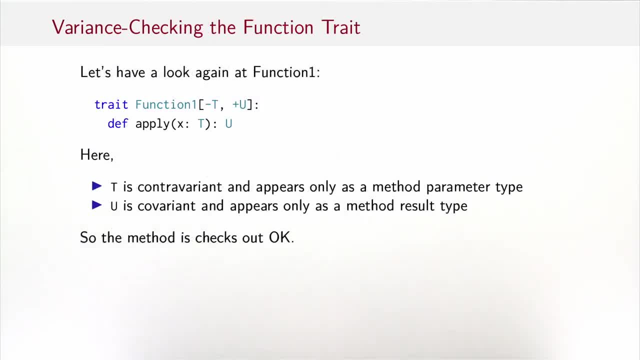 the Scala compiler checks them for us. So let's see whether the rules work out for our function type that we've just defined with variances. Here's the function type. here T is contravariant and it appears only as a method parameter type. so that's okay. 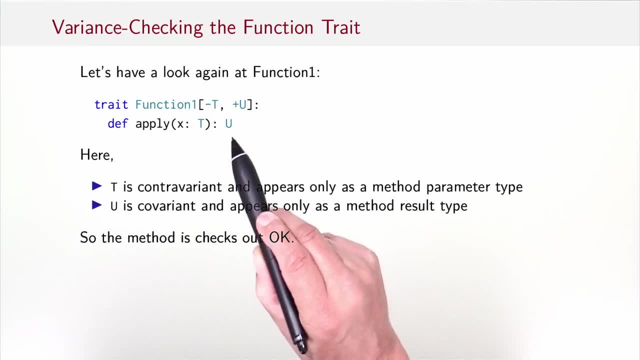 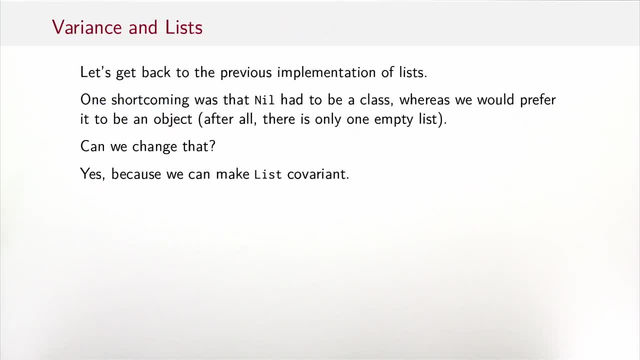 And U is covariant and appears only as the result type of the apply method. So that's also okay and the method checks out correctly. Let's get back to the previous implementation of lists. One shortcoming was that nil had to be a class because 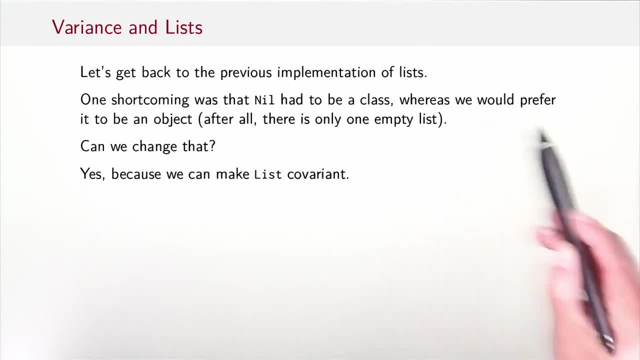 it needed a type parameter that indicates the type of the list, whereas we would prefer it to be an object. after all, there's only one empty list. Can we change that? The answer is yes, because we can make list covariant. So here are the essential modifications: 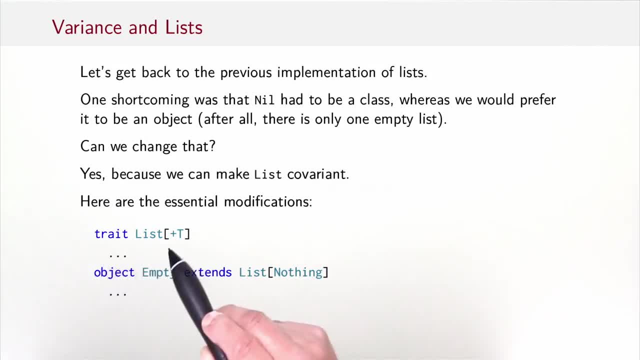 We would give the list trait a covariant type parameter T. We have already seen that a list of apples is a subtype of list of fruit And then the object empty can be a list of nothing. So we can write: object empty extends list of nothing. 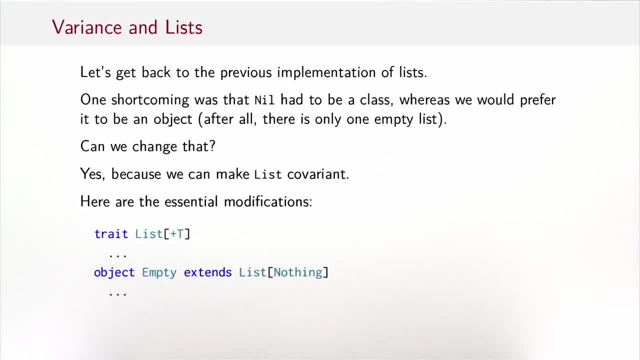 Now that's beautiful because it works on two different levels. On the one hand, we have nothing is a subtype of T For any T and lists are covariant. so list of nothing can be used for any list type T. On the other side, the type list. 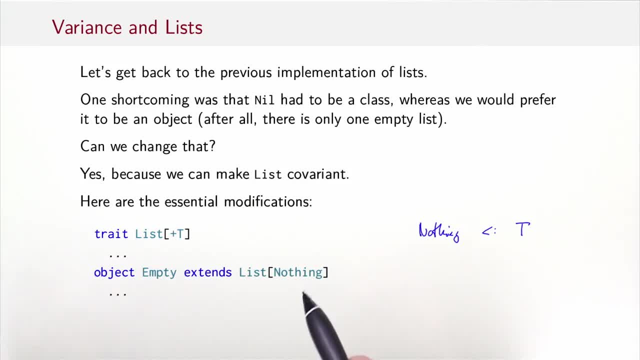 of nothing really conveys the information that there's nothing in the list. So list of nothing. on the one hand says well, there's nothing in the list and on the other hand ensures that that object is a subtype of any list type that the user might care to give. 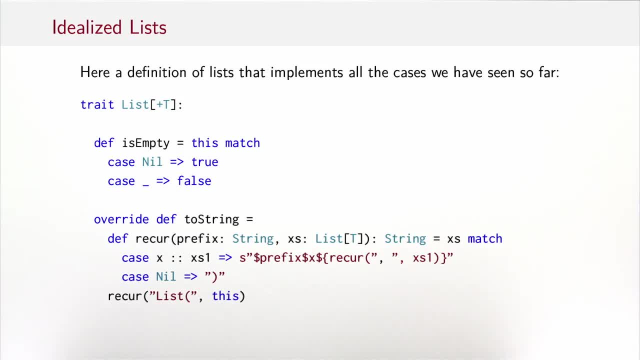 So far we have followed in this course the no-magic rule. Everything you see should be constructible from first principles, and those principles are stated explicitly. So now we have enough machinery to apply the no-magic rules to lists as well, So we can. 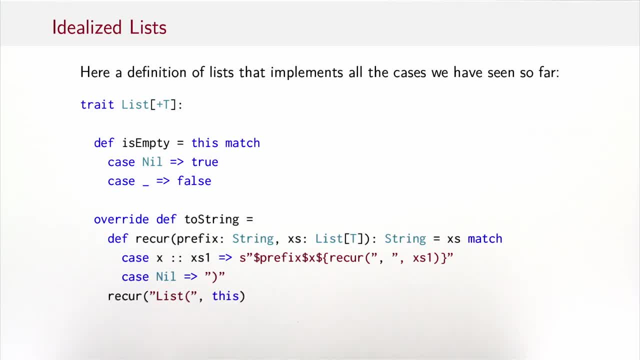 show you how one could write lists as they are used in Scala in a library, at least roughly and approximately. So lists would be a trait with a covariant type parameter. The isEmpty method would do a pattern match and say: well, if the list is. 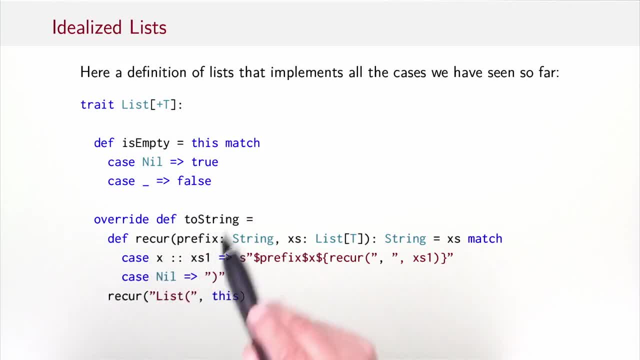 nil, then it's true and otherwise it's false. The toString method is a little bit more involved, so it would use a local function recur that takes a prefix and the list of elements that should be still converted to a string and it returns. 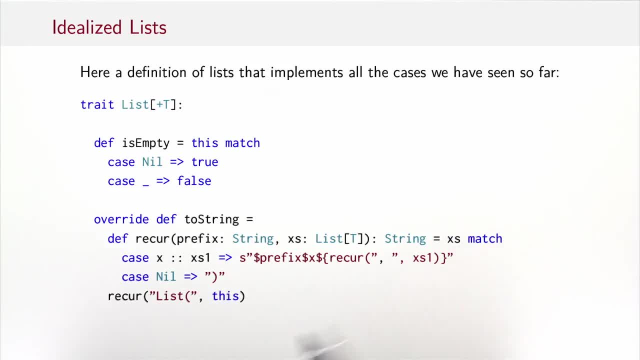 a string. So it would say: okay, if the list is empty, then I close my string with a closing parent, If it's non-empty, then I print the prefix, I print the head element and I follow with a recursive call to recur where. 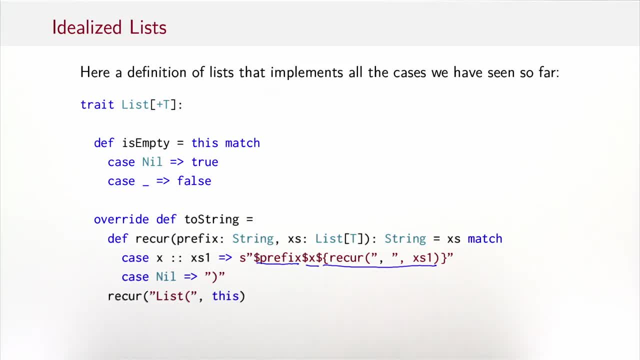 I say the new prefix that should follow x, if there are more elements, is a comma And I start the recurrence with the prefix list open parents. So the first time we print an element we print it after list open parents, and every other time 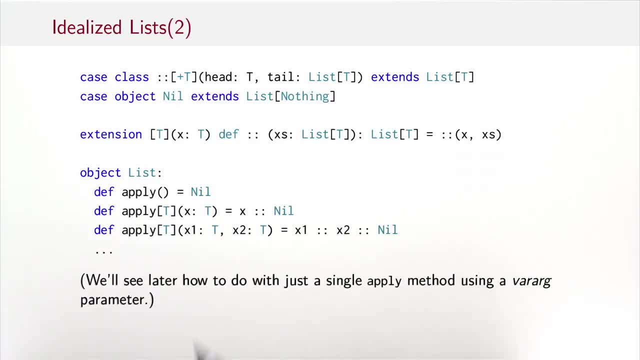 we print it after a comma. So, to continue, there would be a subclass and a subobject of lists. The subclass is called cons, It's also called covariant, It's a case class and it has a head parameter of type t and a tail parameter. 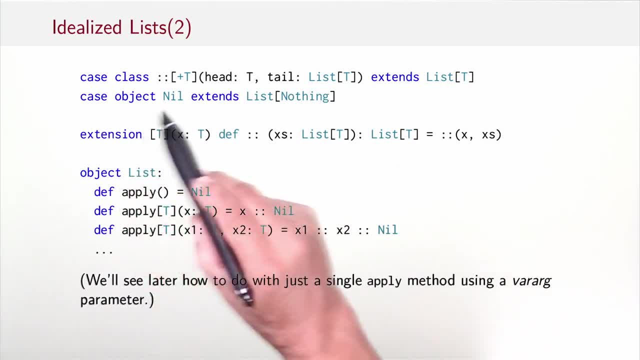 of type list of t And the other case is a case object: nil that extends list of nothing. as we have seen, The final thing we need is cons as a method. We want to write one cons nil as an infix method. 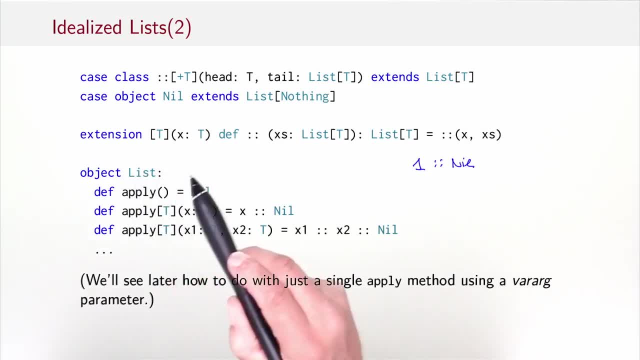 and we do that by defining an extension method. We say, okay, cons is written like this: It takes a first parameter, x, which is of type t, a second parameter, xs, which is of type list of t and its right hand. 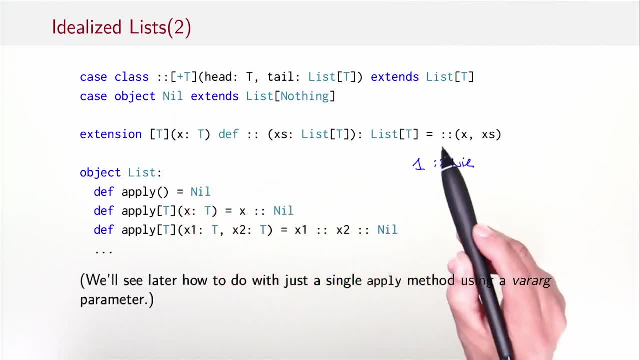 side would be the class creation, which now is written prefix, so that now here we create a new object with the parameters x and xs And finally, we still need to implement calls like list of one, two, three things like that. 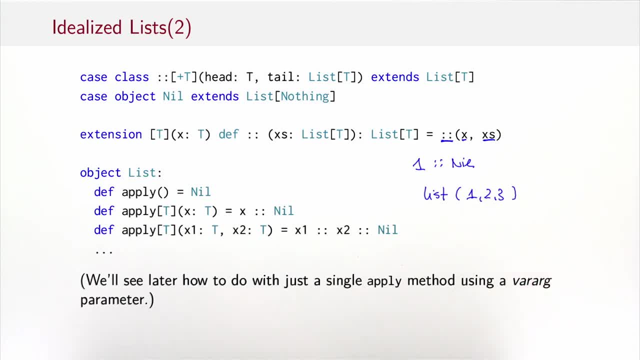 For that. it turns out that we don't have quite the machinery yet to do it in general. so essentially we do a fallback and we just give you an overloaded apply method with several cases for essentially lists of parameters of smaller size. So apply without parameters would be nil. 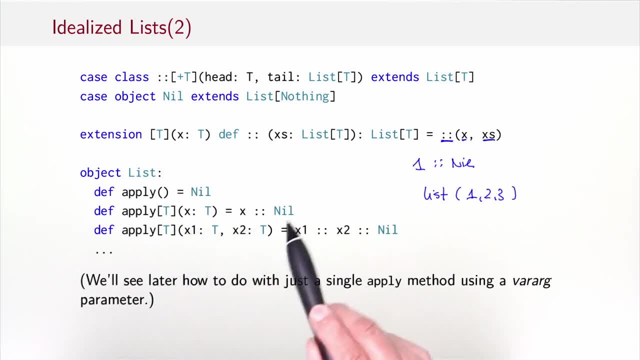 of course, Apply with a single parameter would be x, colon, nil. The two parameter case is here and we would go on with apply methods as many are needed. Later on we'll see that we can do with just a single apply method that uses a var. 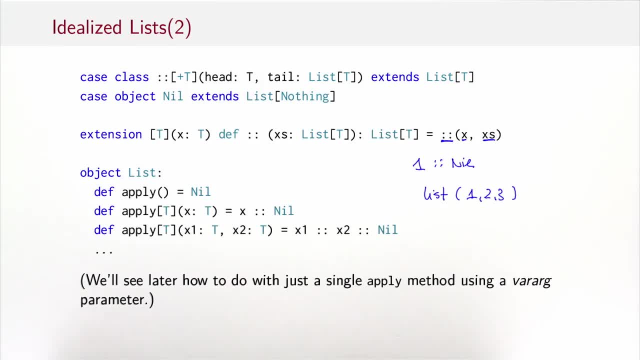 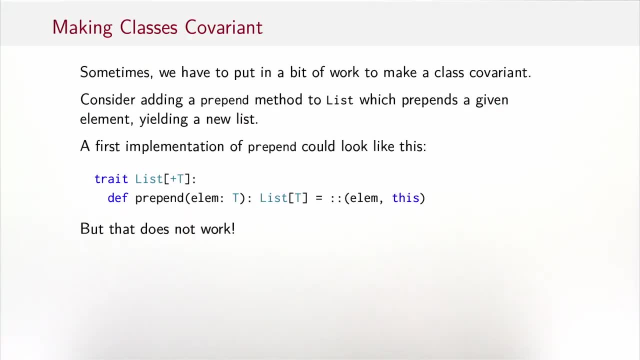 arg parameter. but to introduce var arg parameters we need a little bit more machinery for them. so for the moment we should leave it at that. Sometimes we have to put in a bit of work to make a class covariant, For instance, consider adding a prepend method. 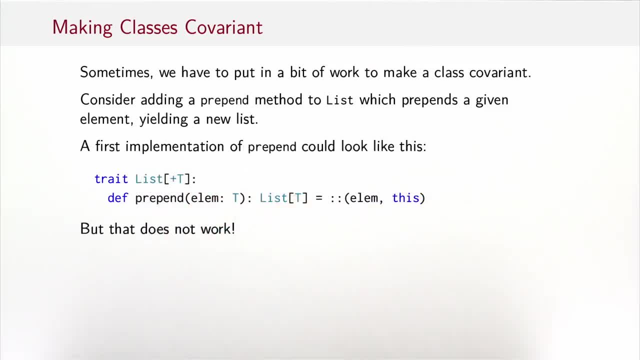 to list which prepends a given element, yielding a new list. A first implementation of prepend could look like this: We are in trade list with covariant type parameter t. Prepend takes an element of type t, returns a list of t and is implemented. 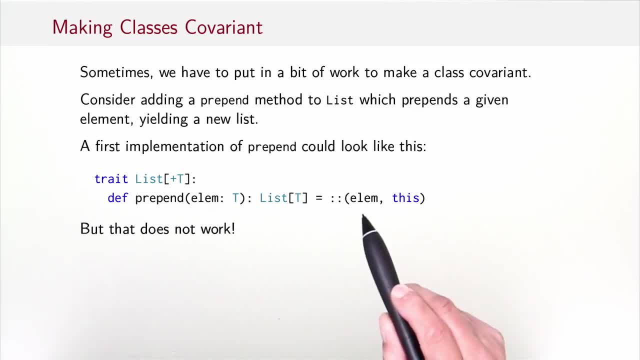 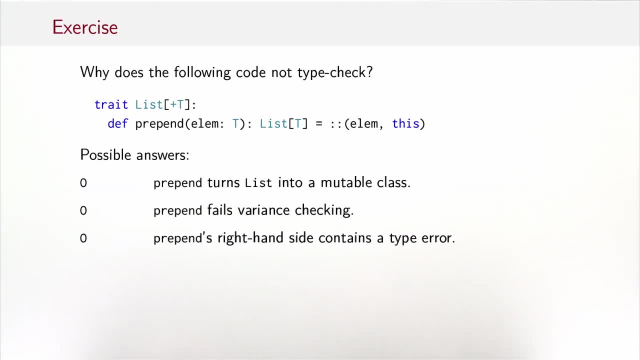 by essentially calling a new cons node with the given element and the current list as the tail, But that doesn't work. So what do you think? Why does the following code not type check? Because prepend turns list into a mutable class and that violates variance. 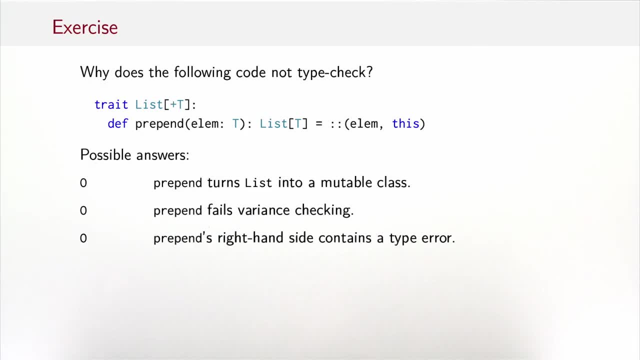 Because prepend fails variance checking in other ways, Or because prepend's right hand side contains a type error. Well, let's look at these possibilities. Prepend gives you back a new cons node. so no, there is no mutation involved. It doesn't turn list into a mutable class. 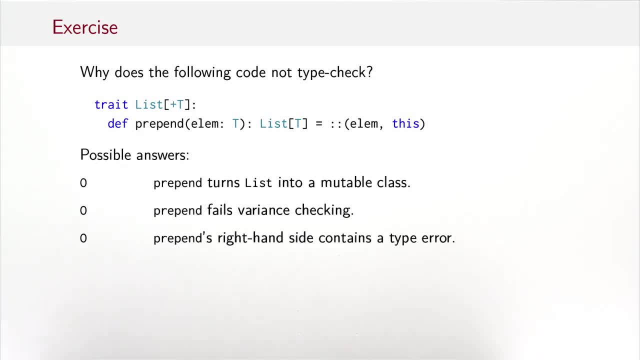 But it still fails variance checking. Why? Well, because the type parameter t is used as the parameter of the prepend method And we have seen that's illegal only for contravariant type parameters or invariant type parameters. But t is declared covariant. 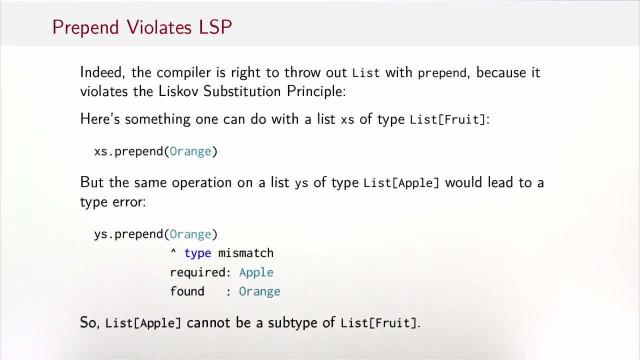 So that's a variance error. So is the compiler over zealous in rejecting prepend? In fact, no, Indeed, the compiler is right to throw out list with prepend because it violates the LSP, the Liskov substitution principle. How? 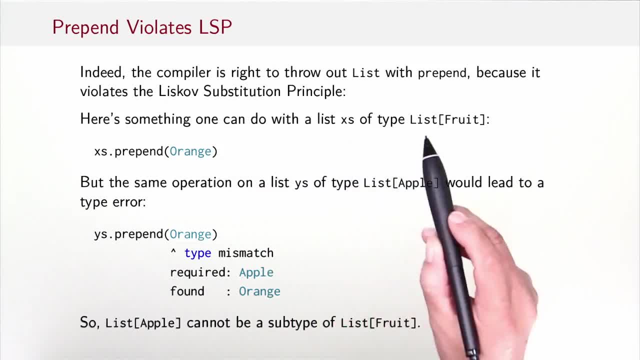 Well, here's something one can do with a list xs of type list of fruit. Prepend an orange, You would still get a list of fruit. But the same operation on a list ys of type list of apple would lead to a type error. So if I do the 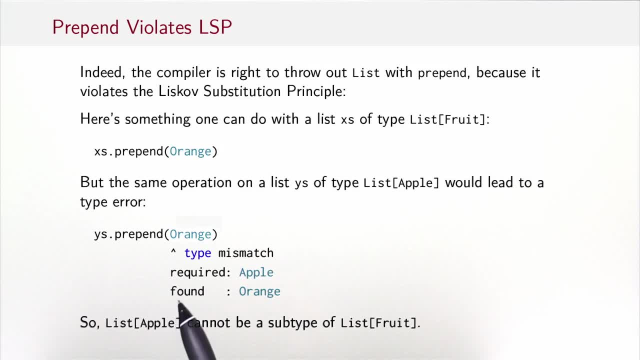 same operation. then the compiler would complain and said: well, I required an apple, but I found an orange. So I can't prepend an orange to a list of apples, which means that list of apple cannot be a subtype of a list of fruit. But you might argue, prepend. 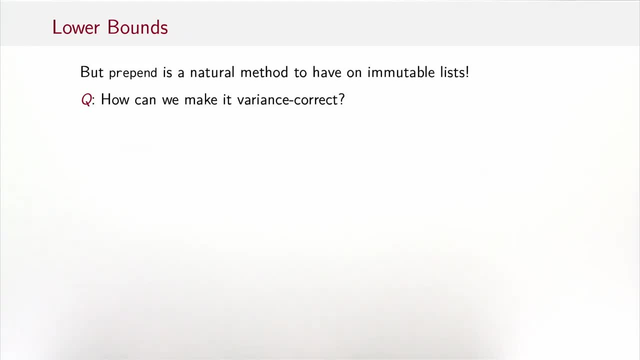 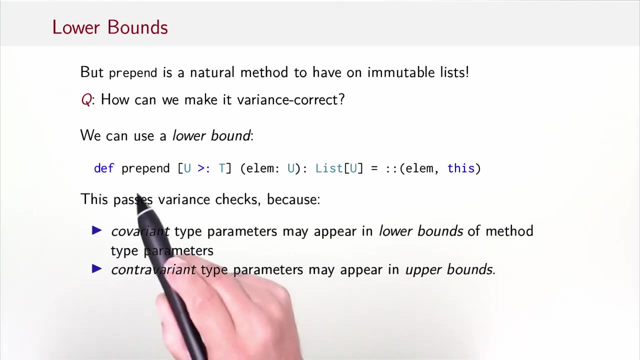 is such a natural method to have on immutable lists, Is there a way to make it variance correct? In fact, yes, We can use a lower bound, So we can write prepend like this: Prepend takes a new type, parameter u, which is now a supertype. 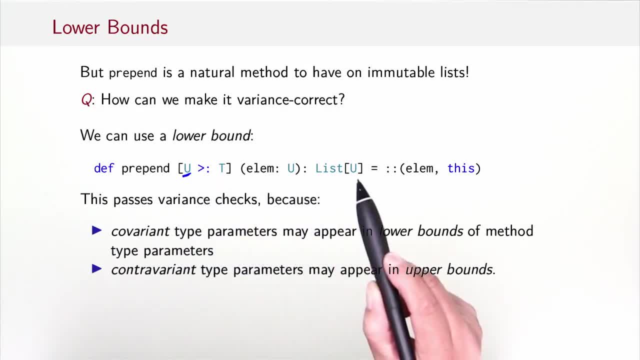 of t and an lm of type u and returns a list of u and it has the same body with the cons as before. This passes variance checks because covariant type parameters may appear in lower bounds of method type parameters, whereas contravariant type parameters may appear only. 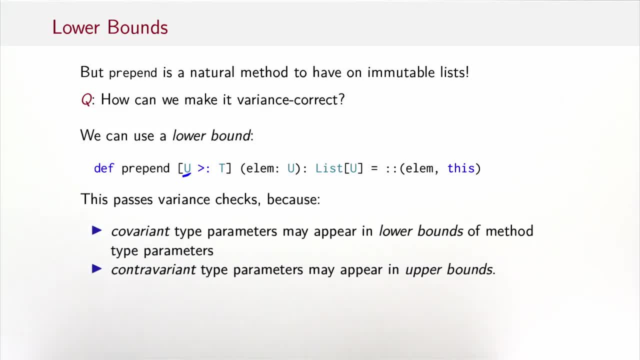 in upper bounds. So in a sense we have a double flip: We go to a parameter, but then we go to the lower bound of that parameter and that turns variance around again and makes covariant parameters legal to appear. Okay, but is this more than? 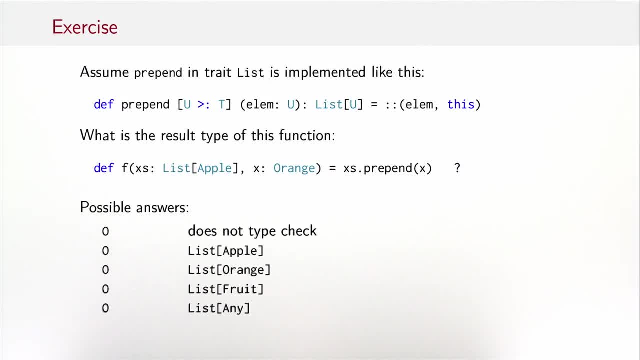 just a trick to make the variance check happy. In fact, yes, we have added some useful functionality to prepend. If we look at prepend again, the question is: what is the result type of this function? We take a list of apples and an orange. 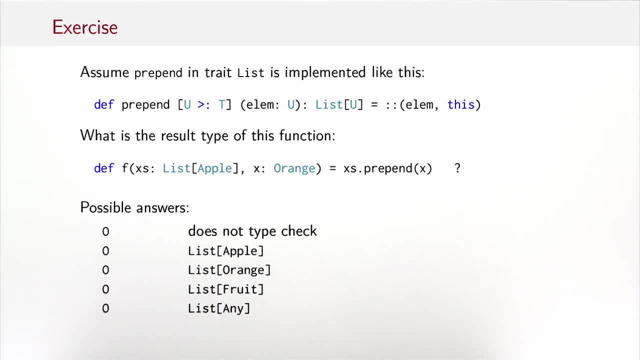 and we call x as prepend x. Previously that wouldn't have worked because we said I can only prepend an apple to a list of apples. but now I can prepend an orange and what do I get? Well, it does type check and I get a list. 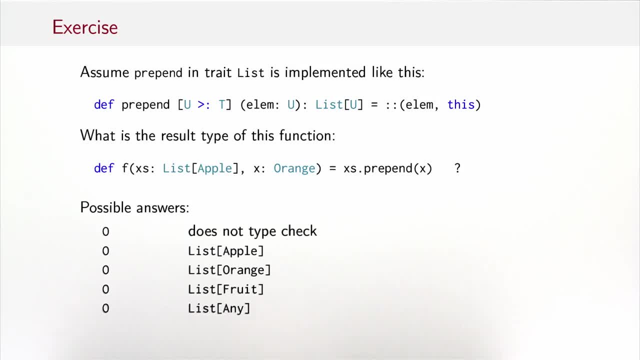 of apple. No, the list would contain an orange. A list of orange? Surely not A list of fruit. Yes, that's the answer. I would obtain a list of fruit. So how does that work? Well, I'm in a list of apples. 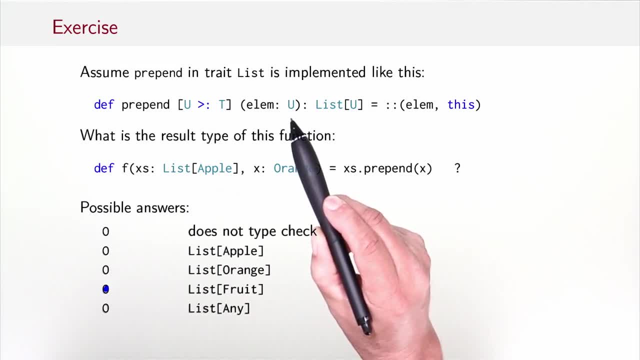 I get the element, which is an orange, The compiler will have to find a type u which is a supertype of an apple and can take an orange, and the smallest such type is indeed fruit. So the compiler will instantiate my type u with fruit and that's the result. 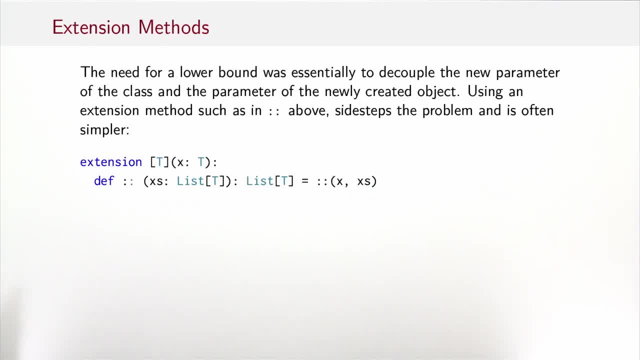 type list of fruit. then that I get back. But there's a simpler way to obtain the same functionality, and we've seen it already. It's called extension methods. In fact, the need for a lower bound was essentially to decouple the parameter of the class and the 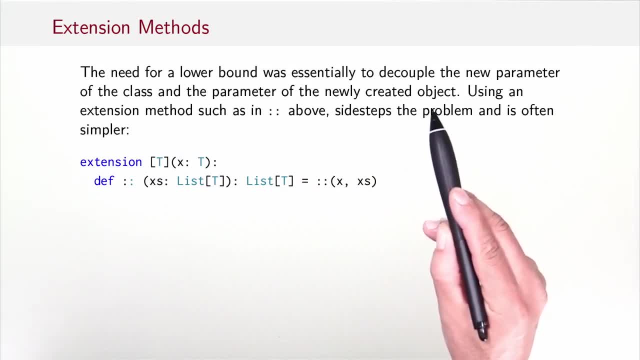 parameter of the object that is newly created. The newly created object could be a fruit, where the class was a list of apple Using an extension method, such that the cons method that we've already constructed sidesteps the problem and leads to the same result. So if we 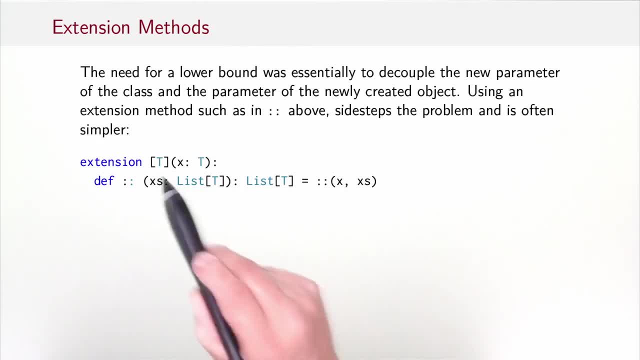 define an extension method here, then the compiler will also instantiate the type t to be a supertype of the type of the element that we prepend and the type of the tail that we pass here. So we would if we prepend an orange to a list of apples. we would. 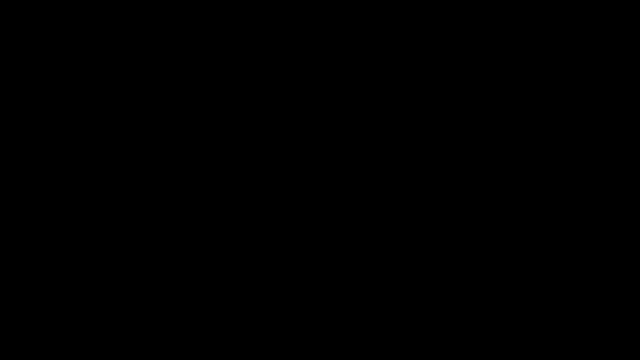 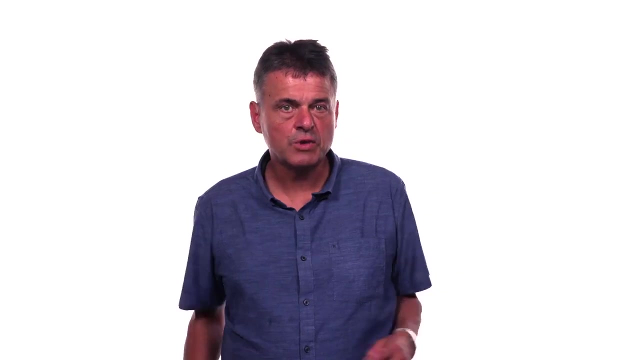 again obtain a list of fruit. This week, we're going to put the spotlight on lists. The list type is one of the most common data types in functional programming. You'll find out about many useful list processing methods, and you'll also learn how some of these methods are implemented. 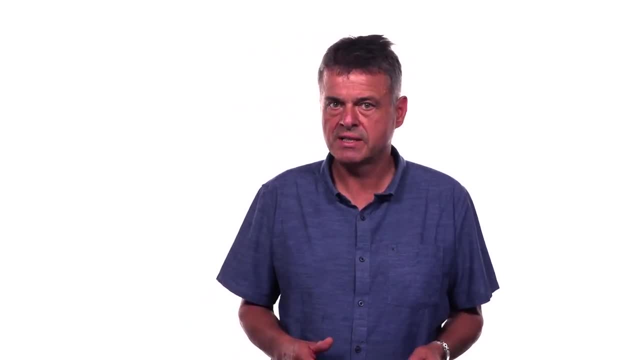 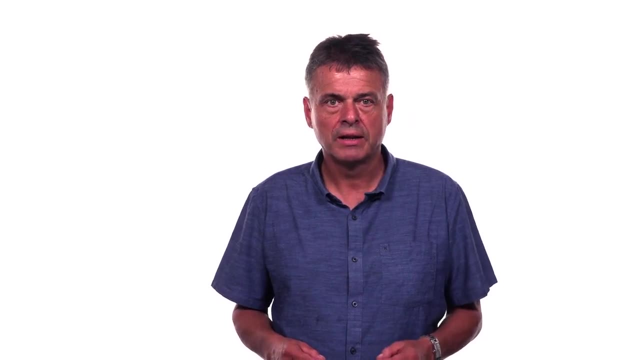 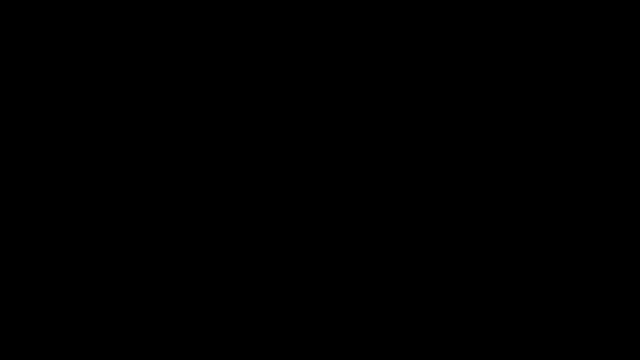 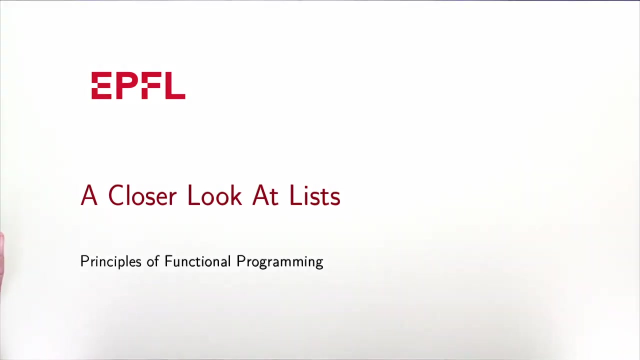 in terms of the fundamental operations on lists, as well as pattern matching. Finally, you'll learn about structural induction, which is a powerful method that can prove the correctness of algorithms over lists and other recursive data structures. In this session, we're going to take a closer look at 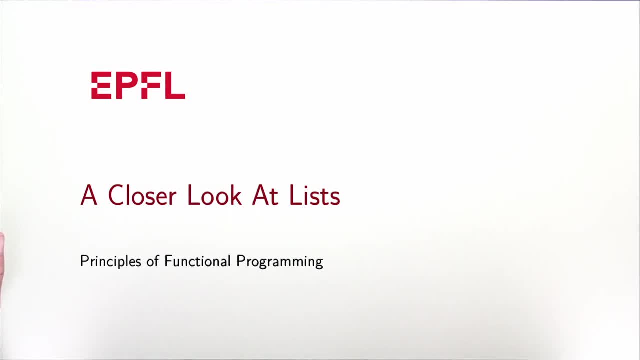 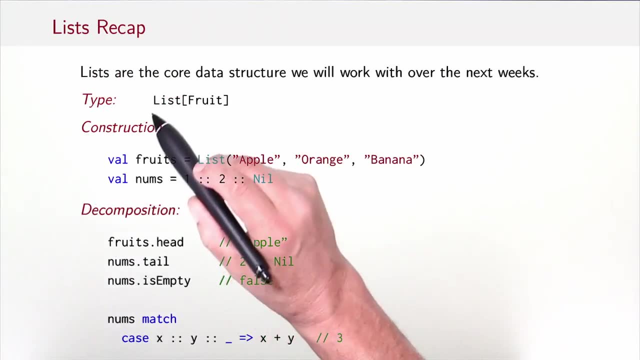 lists. Lists provide quite a rich catalog of operations and we'll learn how to use some of these operations in our work. So, to recap, there's the type list, which takes the type parameter of the list elements. We can create lists by writing list in front of. 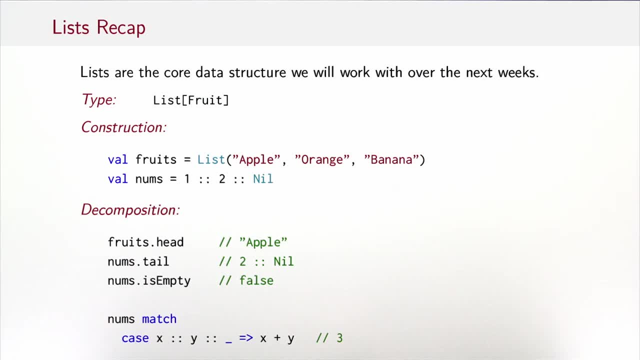 the elements of a list we want to create. or, alternatively, we can create lists using a sequence of cons- operations, like you see here for nums To decompose lists. we can do that either with the three standard methods- head, tail and isEmpty, or, preferably with a pattern. 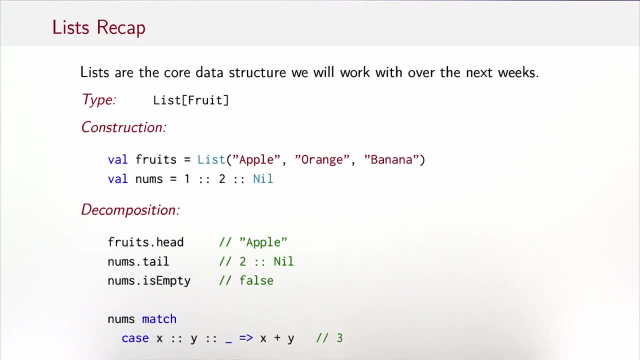 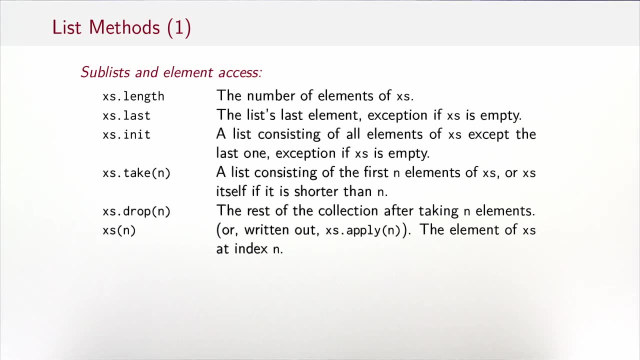 match, like what you see here for the example where we pull out the first and second element from the list nums. So here are some of the most commonly used list methods. First there's length. that gives you the length of the list. that means the number of elements in the list: xs. 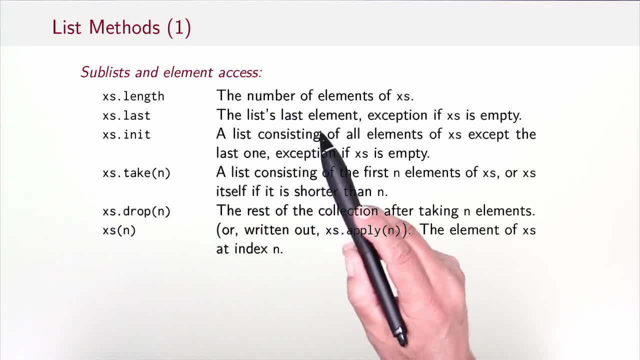 Last gives the list. last element, exception if xs is empty. So last is the analog of head. Init gives you the list consisting of all elements of xs except the last one, exception if xs is empty. So init is the analog of tail. 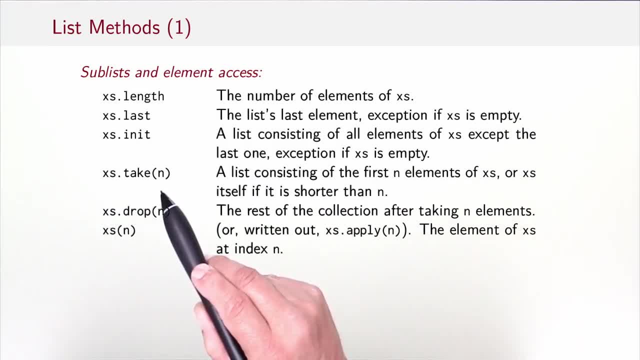 XstakeN gives you a sublist that consists of the first n elements of the list xs, or of the list xs if the list is shorter than n. So let's say you have the list 1,, 2,, 3 and you take 10 elements, you still get the list. 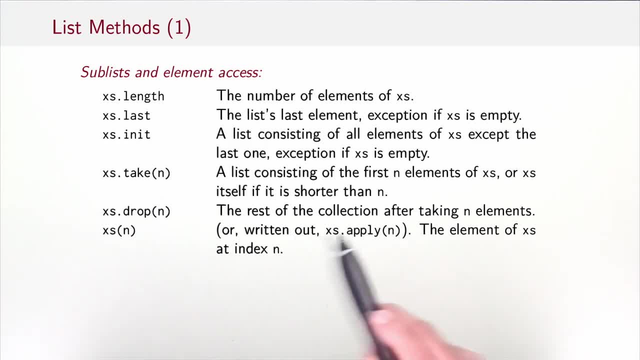 1,, 2, 3.. XsdropN gives the rest of the list after taking n elements Or nothing. if the list is exhausted before getting to the nth element. XsapplyToN, or written out simply: xsapplyN is the element of xs. 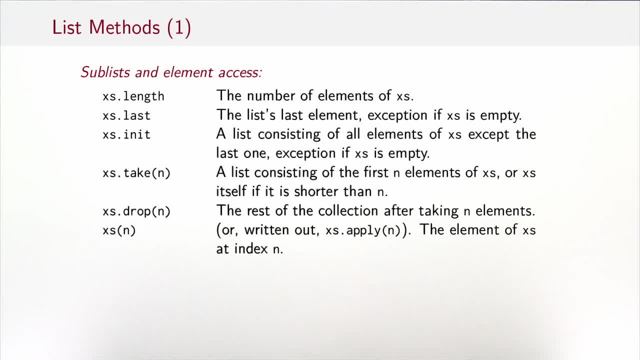 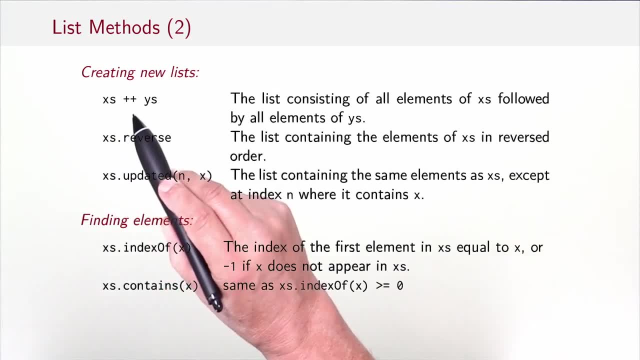 at index n, And if the index is out of range of the list you'll get an exception. So to create new lists, there's first concat, written double plus. That gives you the list consisting of all elements of xs, followed by all elements of ys. There's also: 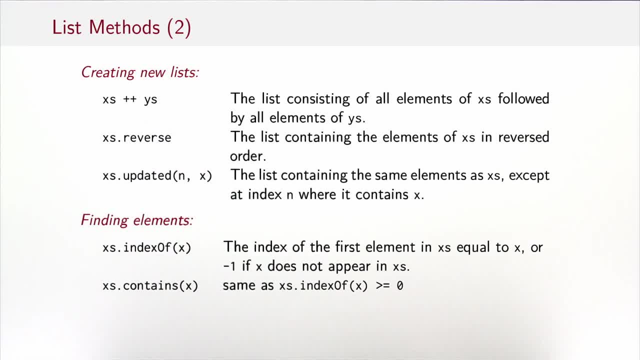 reverse. that reverses the elements of xs. That means it gives you a new list where the elements of xs appear in reversed order. And finally there's updatedNx. that gives you a new list that has the same elements as xs, except at position n, which must be in range. 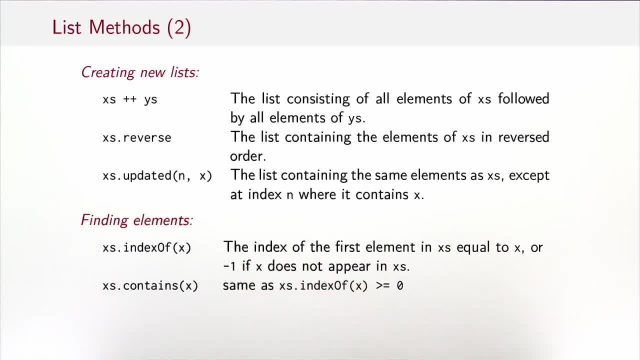 it gives you x. So updated is still purely functional. It doesn't touch the list xs but it gives you a new list with the properties I've described. The following two methods are useful for finding elements. First, there's indexOf. indexOf gives you the 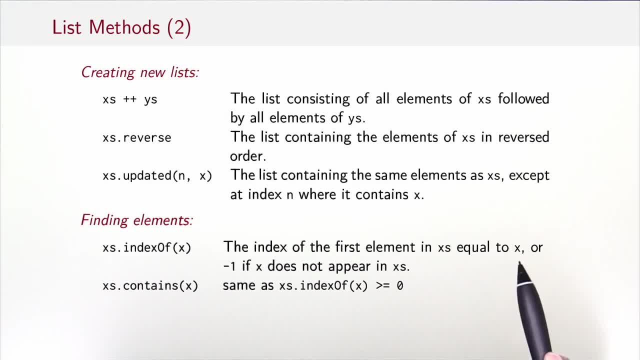 index of the first element in xs. that's equal to x or minus one. if x doesn't appear in xs, xsContains gives you a boolean that tells you whether x is an element of xs. xsContains is thus the same as xsindexOf equals zero. 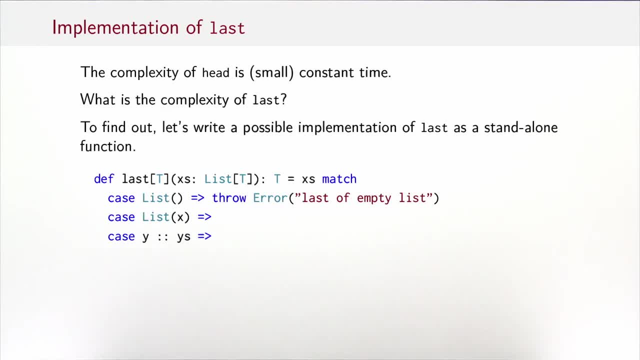 So let's take a look how some of these methods are implemented. We know that the complexity of head is small, constant time, because head just pulls out one of the fields of a cons node. What is the complexity of last? To find out, let's write a possible. 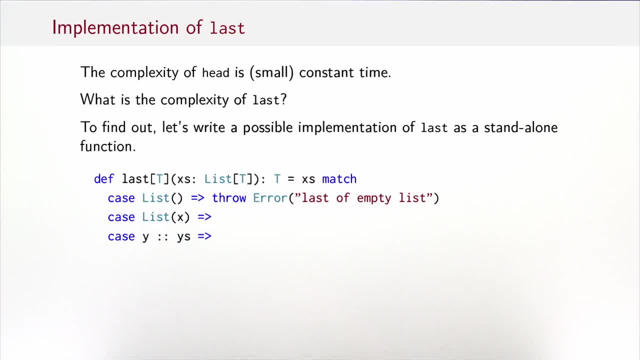 implementation of last as a standalone function. So here's what we could write last of a list xs of type list of t, is we match on xs? if it's the empty list, then that would be an error. if it's a list consisting of just one element, x. 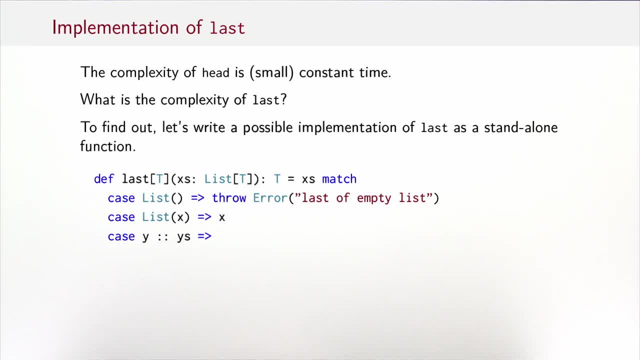 then the last element of that list would be x itself. and the third case would be: it's a list consisting of a head y followed by a list ys. in this case we have to search for the last element in the list ys, so the result is last of ys. So if you look at 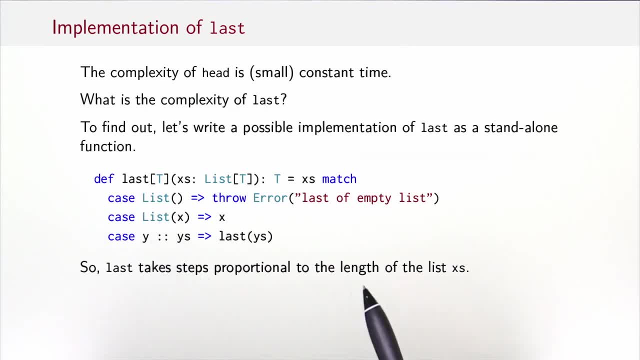 this implementation, we see that last takes steps proportional to the length of the list xs. it has to go through the length of the list to find the last element, and that makes last a lot less efficient than head. so, if possible, always define your operations in terms of head and tail. 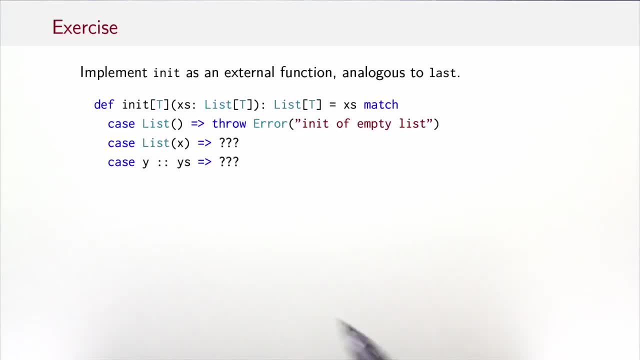 and not last, and init. In fact, looking at init, we can see here a possible implementation scheme. we have the same triple pattern match. if the list is empty, then init is not defined, so we get an error. if the list consists of just a single element, then init is the list. 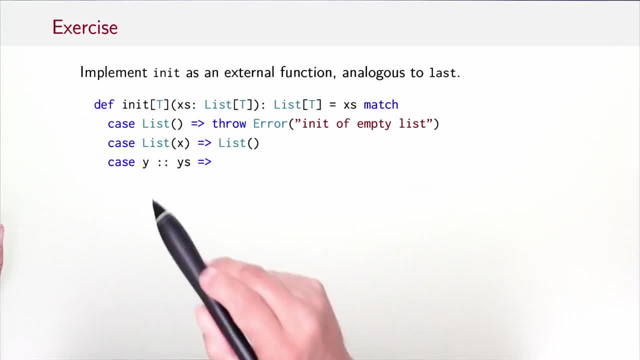 without that element. so that would be the empty list. and if the list consists of an element, y, followed by a list, ys, then init would definitely contain y and the initial elements of ys. That's a complete implementation of init and, like last, its complexity is proportional to the 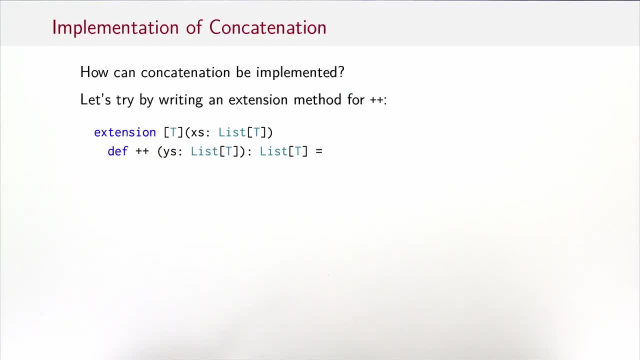 length of the argument list xs. as a third method, let's look at concatenation. how could concatenation be implemented? let's try for a change to write an extension method for plus plus. So we have an extension method plus plus that follows a list xs and. 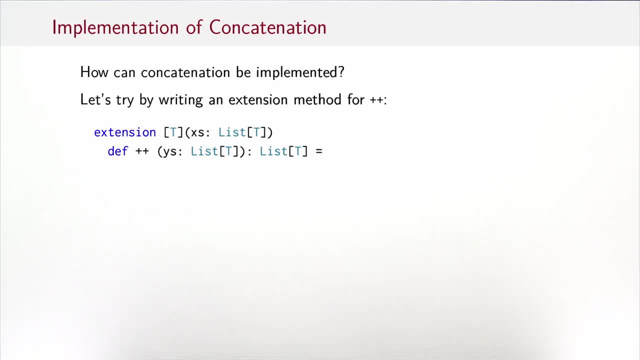 has as additional argument a list: ys. as usual, we'll start with a pattern match. but a pattern match on what list should we match? on xs or should we match on ys? turns out that its advantage is to match on xs, so let's do that. so we write xs match. 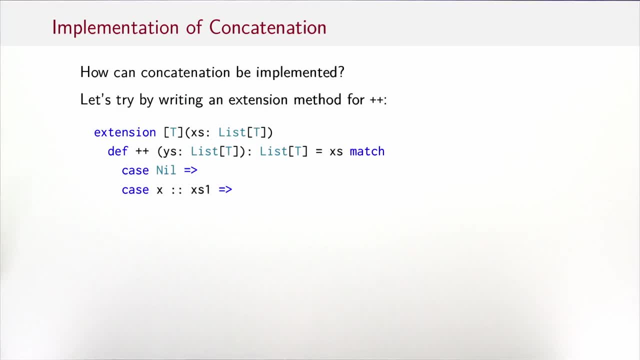 if xs is nil, what do we return? Well, in that case the concatenation of nil and ys is ys. if xs is not nil- let's say it's an element, x, followed by a list, xs1- then the concatenation would start with x and be followed. 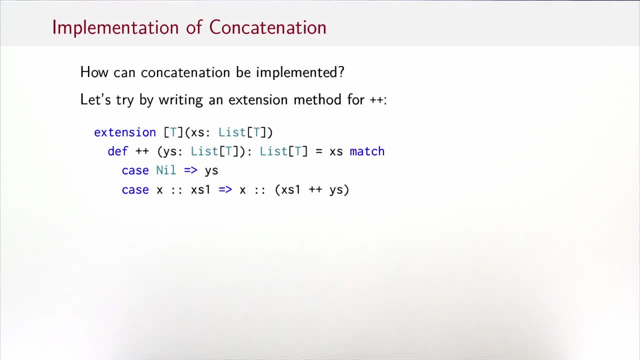 by the concatenation of x1 and ys. what's the complexity of plus, plus concat? well, we have to do a pattern match only on the left list, but we go to the end of that left list, so the complexity would be proportional to the length of the. 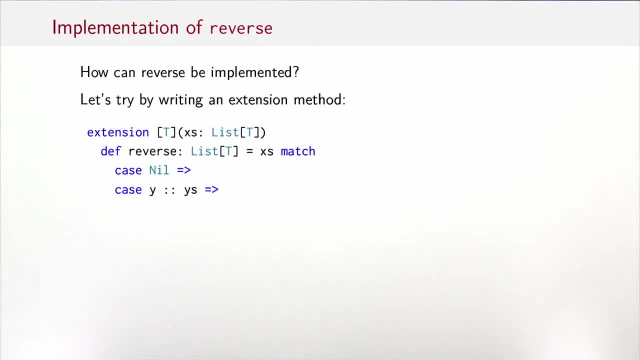 left list xs. as another example, let's look at reverse. how can we implement reverse? let's try again by writing an extension method. in this case there's only one list, xs, so let's try to pattern match on that list. if the list is nil, reverse of the empty list is: 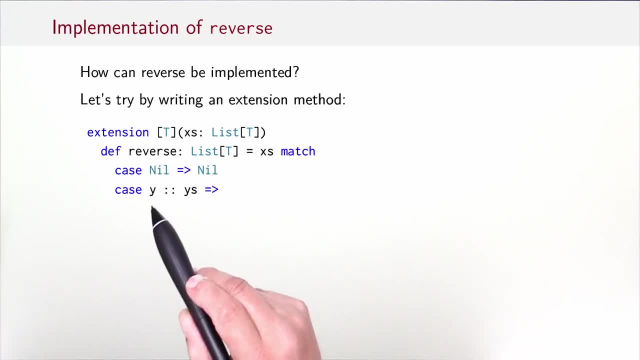 the empty list. of course, reverse of a non-empty list starting with y and being followed by ys is well. one way we could do it is to say: well, let's reverse the list ys and append the y as the last element to that list. so it's ys, reverse, concat. 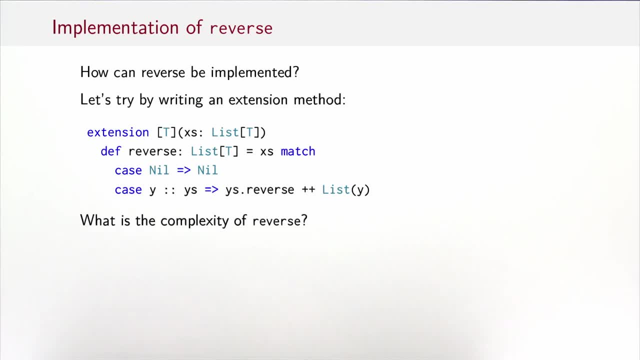 list of y. what's the complexity of reverse? well, we go through the list xs. that gives us a factor linear in the length of the list, and then, for each of the sub-lists, we call concat, and that concat is, as we've learned, proportional in the 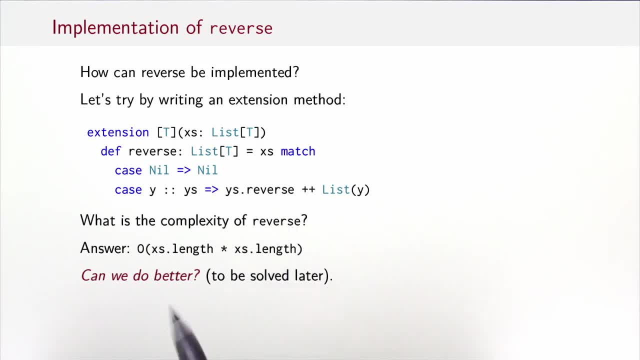 length of the left list. so that gives us a factor of x dot length times x dot length. so the complexity of reverse is quadratic in the length of the list xs. that's a bit disappointing, because if we had an array we would know of course how to reverse. 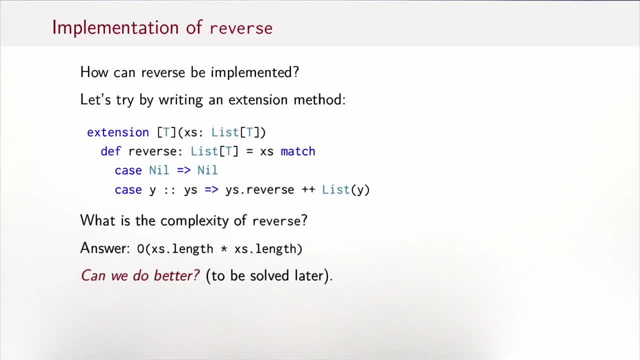 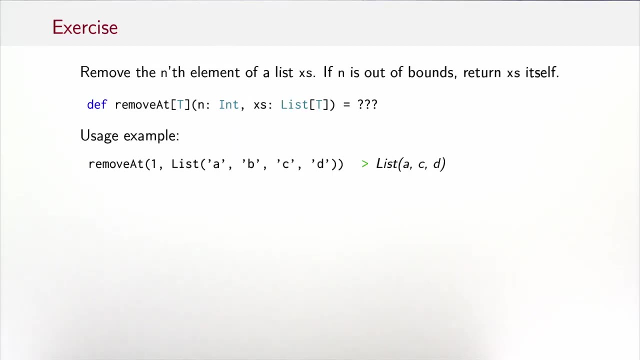 it in linear time, just swap the layers of corresponding elements. so one question is: does functional programming in this case have an inherent performance overhead or can we do better? and we'll solve that question later. but before that, let's do an exercise, let's write a function. 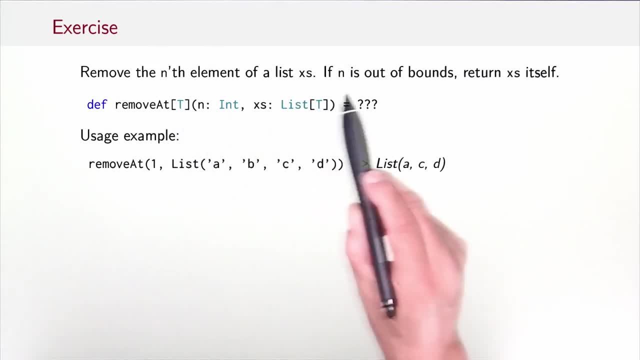 to remove the nth element of a list xs. if n is out of bounds, it should return xs itself. so we're after a function with this signature. it takes an index n and a list xs and the implementation should satisfy a usage example like this one here. let's say, if we remove the element 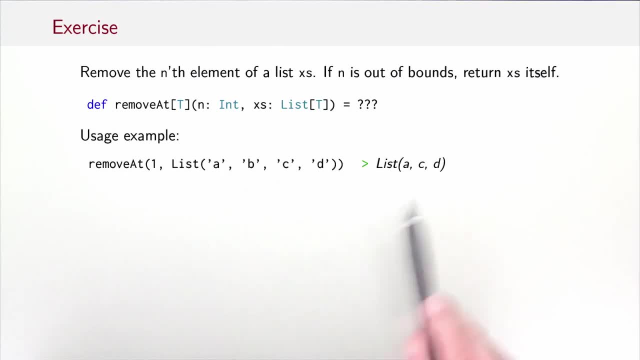 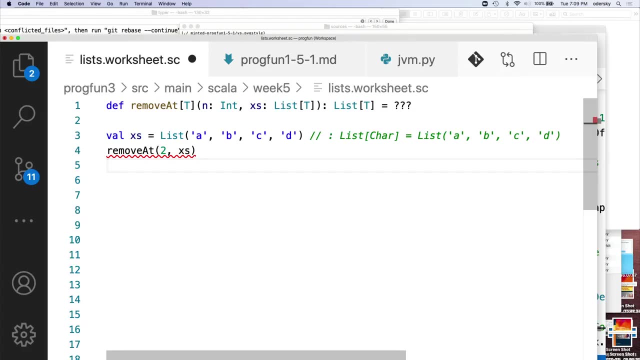 at index 1 of the list abcd, we should get the list acd, because the element at index 1 is b, so that element should be dropped. ok, so I have set up the worksheet with the signature of the removeAt method and the example list xs. 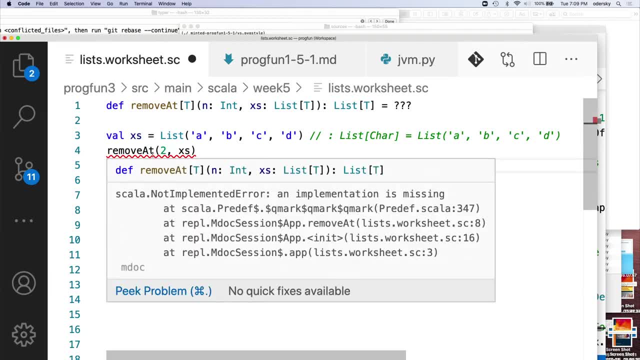 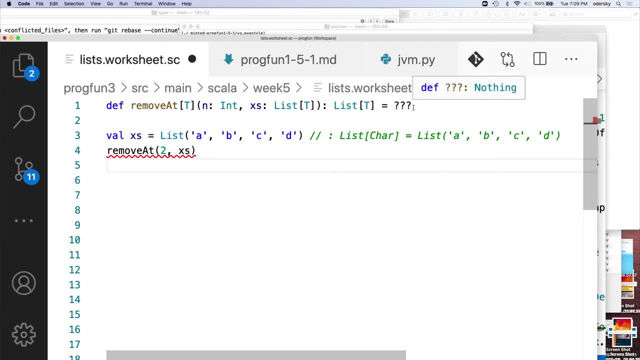 for the moment it doesn't work. so if we look at the removeAt call then it says not implemented error. yes, of course we have still a triple question mark as the body. so the task now is to fill in the body of removeAt. so one proven strategy is: 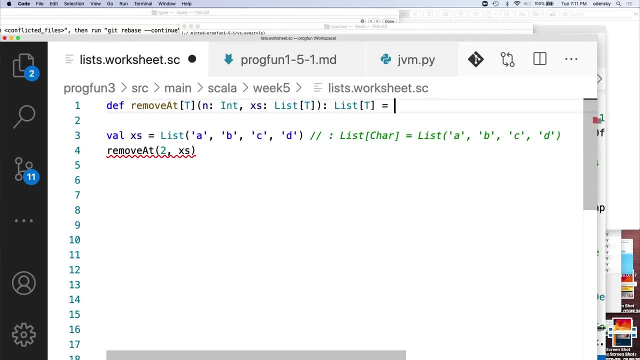 we pattern match on what xs is, so we write xs match. if it's nil, then we said: well, remove anything from the list where the index doesn't exist should return the list itself. so we return nil. if the list is not nil, say consists of y followed by ys. 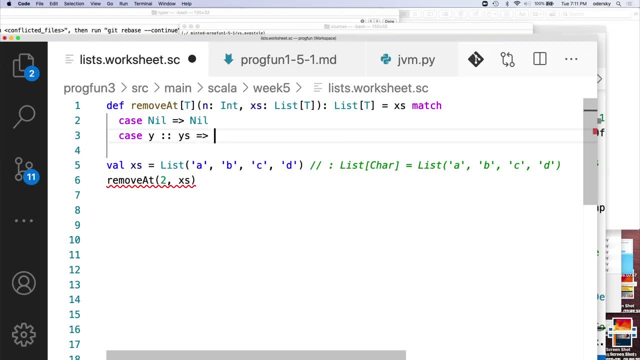 what do we do? well, now we look at the index n. if n equals 0, then we should return the list consisting of all elements except the first, so that's ys. if n is not 0, then we'll have to do a recursive call, so y. 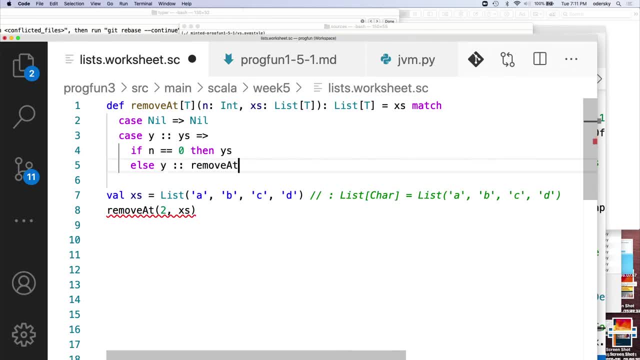 would be part of the list and that would be followed by removeAt and ys. ok, so we, if we test that, then removeAt indeed gives us the list. we can do some other elements, let's say 4. that doesn't do anything because there is no fourth element. 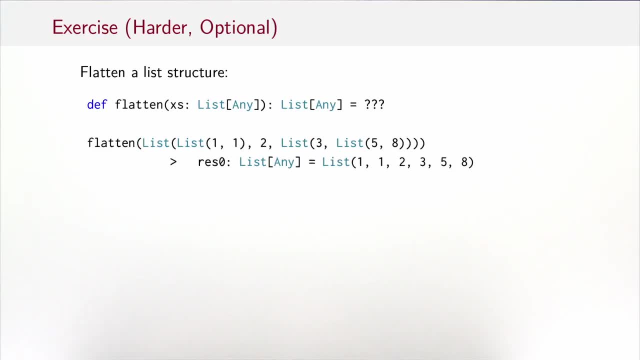 3 would remove the last element, and so on. the second exercise is a bit harder. we want to flatten a list structure, so we're after a method with a signature like this one. it should take a list of any and it gives us a list of any. 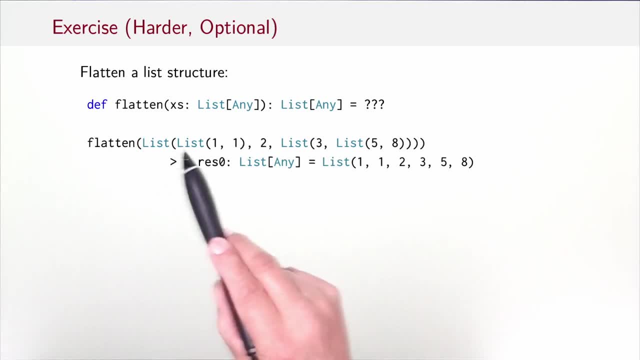 and what it should do is if we have a list that has nested lists as elements, then those nested lists should all be flattened so that we get a single list that contains just the elements themselves, without any embedded sublists. so if we take flatten of that import and we 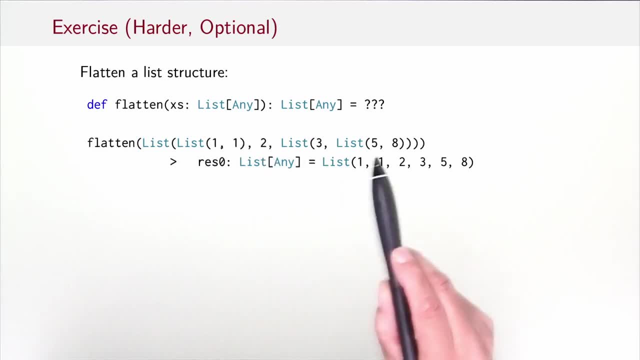 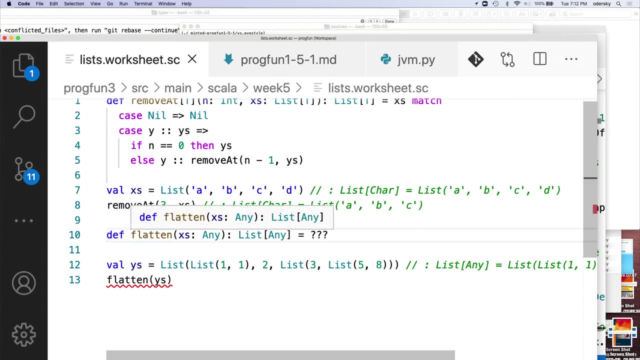 should just get the leaf elements 1,, 1,, 2,, 3,, 5,, 8 in that order in a single list. again, I've given the setup here. we have the signature of flatten, the example list that was given in the exercise, and 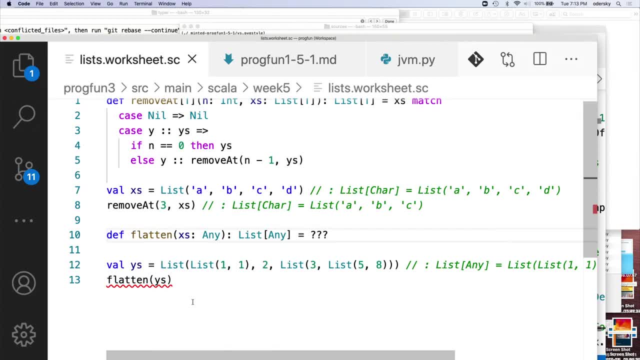 if we look at the call then it says again not implemented. in fact it turns out that it's advantageous if we give flatten a somewhat more general type. so it takes an any and gives us back a list of any, and the understanding is if the argument that it takes is not a list, 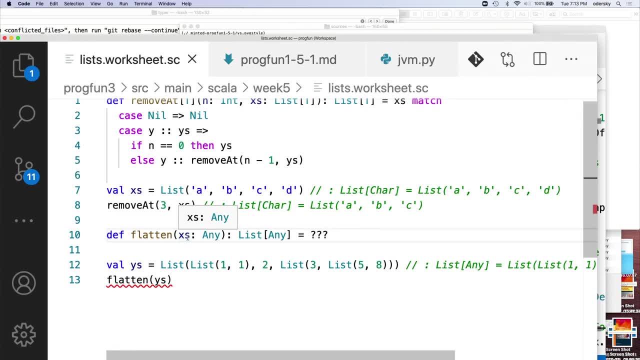 it would just return a list consisting of that single argument. so flatten takes any combinations of arguments and it will always return a single list. so let's do that. so what we do is we match on xs, so we see we can match on more things than lists. it can also be any. 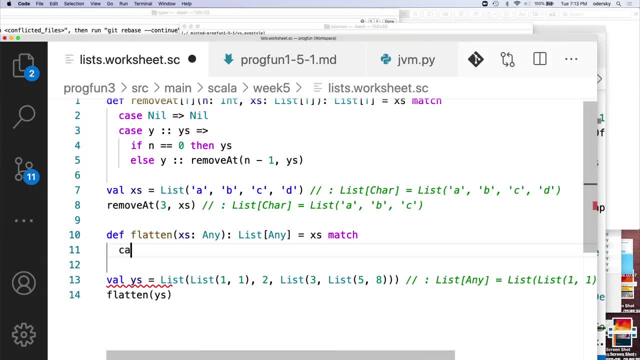 so if the list xs is nil, then flatten the list of nil gives us nil. if it's another list consisting of a head y followed by ys, then what do we do? well, y could have embedded sublists, so let's flatten those. and so could ys, so let's. 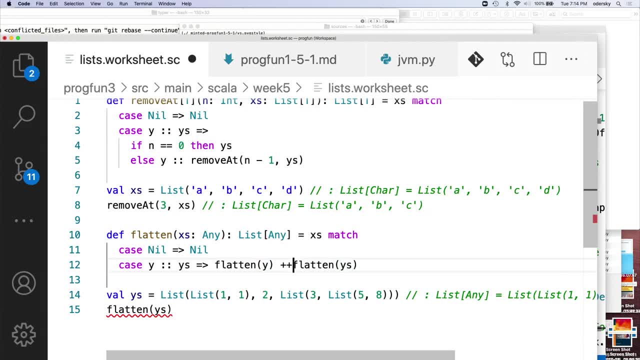 flatten ys and then we concatenate the results because we are interested in a single list, the. the other case is it is something that we don't know what it is. in this case we return the xs followed by nil. so if it's not a list, then just turn it into. 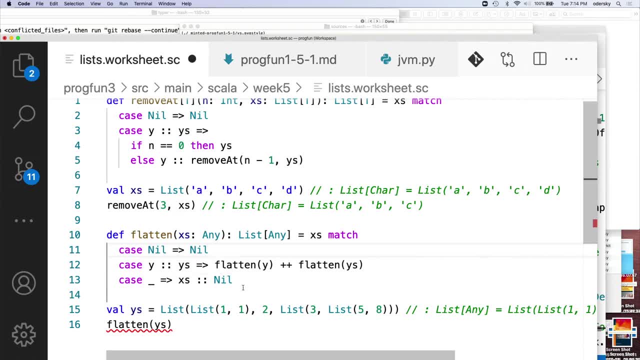 a list by making it the only element of the list we return okay, so let's try that. so if we do that, then indeed flatten of ys gives us one, one, two, three, five, eight. so what we've seen here in the example of flatten is that pattern matching can be. 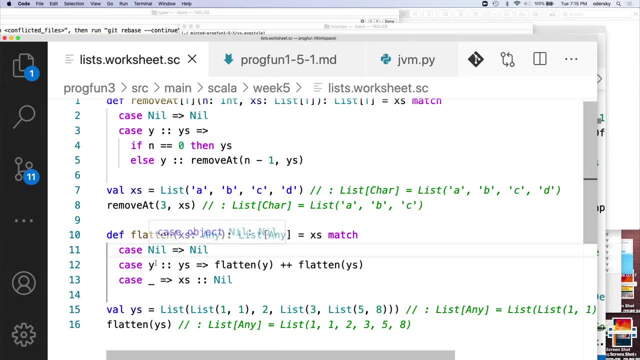 done on very general types, including any, so the patterns will always essentially pick out the right sub parts and match it with the right hand side. this can be quite useful for code that is weakly typed so that works on on many different types in a homogeneous fashion. 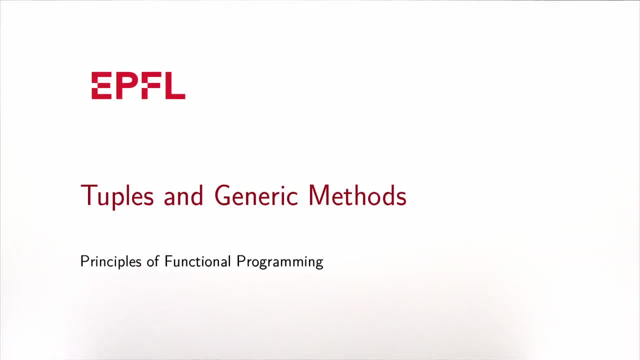 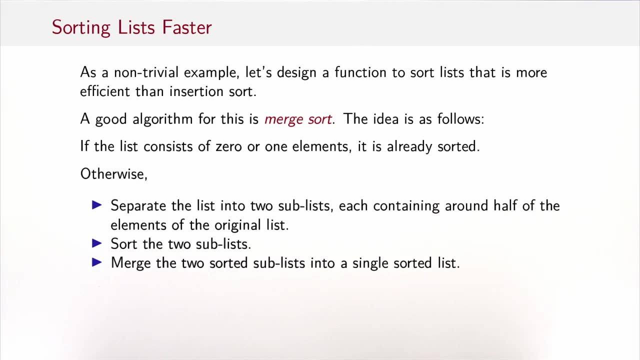 in this session we'll learn about more methods on the list type and we'll also introduce a new data type, the tuple. we look at these things in the context of a somewhat larger example, namely, we want to design a function to sort lists that's more efficient than 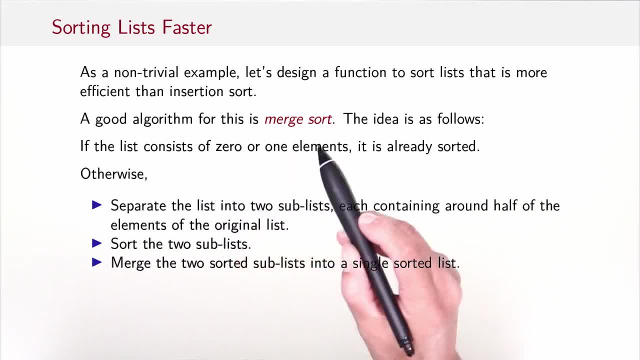 insertion sort. a good algorithm for this is merge sort. the idea is as follows: if the list consists of zero or one element, it's already sorted. otherwise we separate the list into two sub lists. each sub list should contain about half the elements of the original list. then we sort the two. 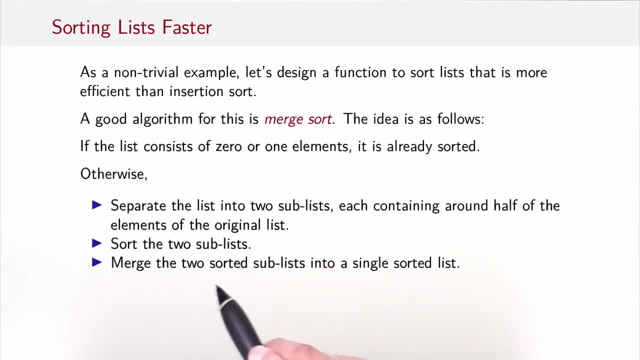 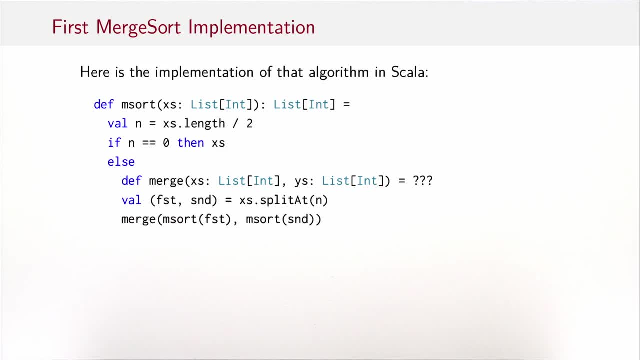 sub lists each in turn and finally we merge the two sorted sub lists into a single sorted list. here's an outline of the implementation of that algorithm. in Scala we define a function- msort- short for merge sort- that takes a list of ints and returns a list of ints. 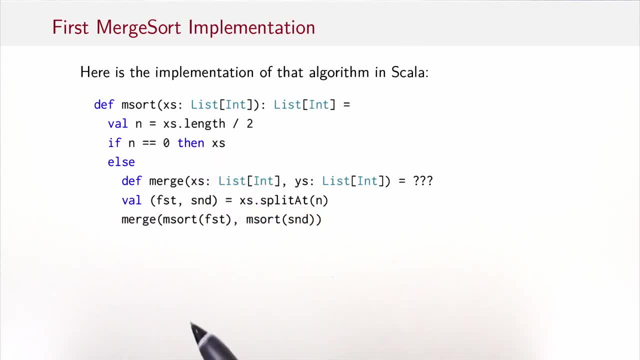 we compute the length of the list divided by two. if that is zero, the original list was of length zero or one- then we return the original list. otherwise we postulate a merge function for two sorted lists. so it remains to the triple question marks here remain to be. 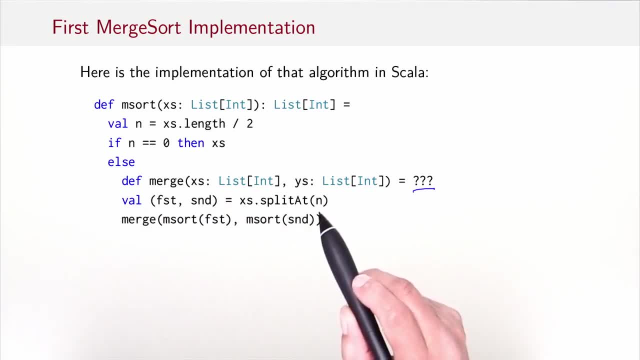 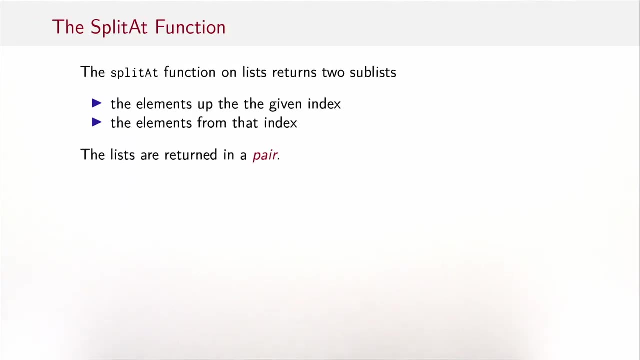 filled in. we split the list at the point in the middle. that gives us two sub lists, first and second. we recursively sort first and second using merge sort and we merge the results of those two recursive sorts. that sorting function uses the split add function on lists that returns two sub lists. 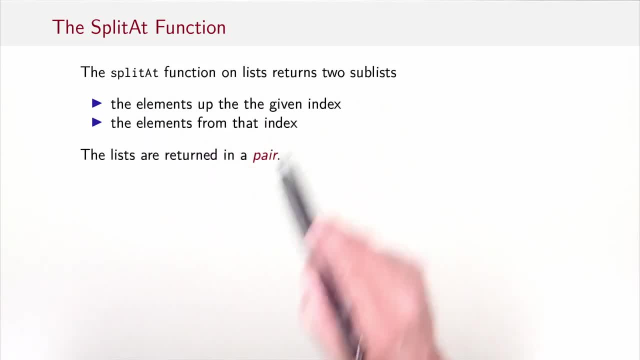 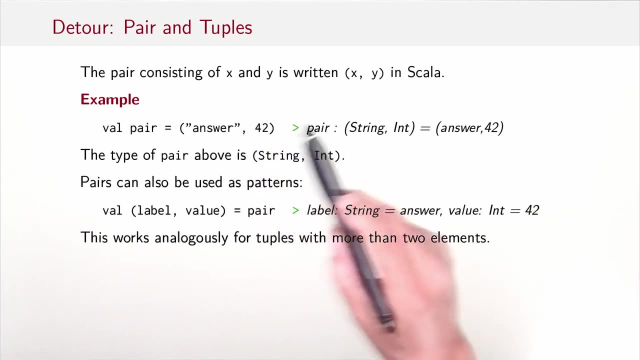 the elements up to the given index and the elements from that index. and those lists are returned in a pair. a pair consisting of the two halves x and y is written x, comma, y in parenthesis in Scala, for instance. here you can say: val pair equals answer 42 and that 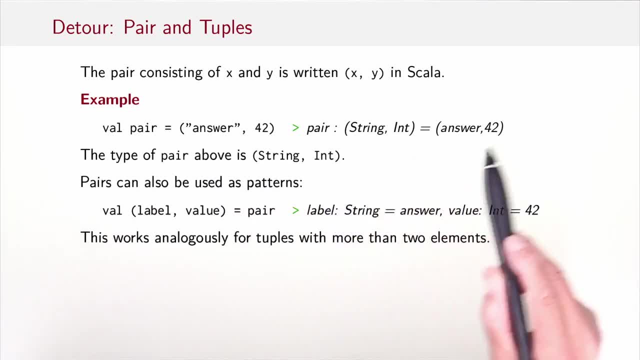 would give you a pair of type string int and value answer 42. so the type of the pair is string int. it's again the individual types in parenthesis, separated by commas. pairs can also be used in patterns, so you can decompose that pair by writing val label value equals. 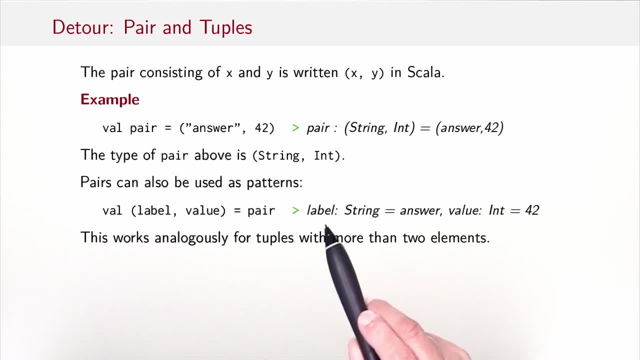 pair, and that would give you two values: a label, which is the answer, a string, and a value which is an integer 42. the whole thing works analogously for tuples with more than two elements, so you can have as many parts in a pair as you want. 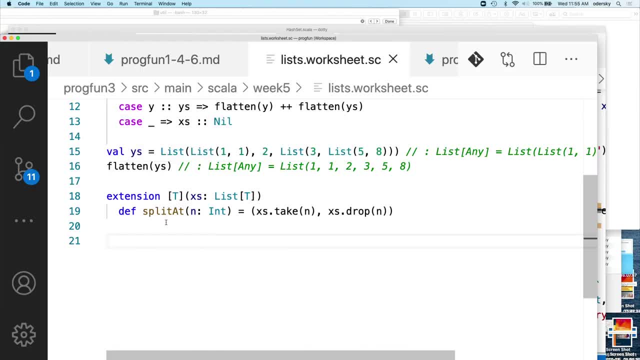 so using pairs, we can write the extension method split at, like you see here. so it's defined on lists of t for arbitrary t, it takes an int and it gives you back a pair where the first element of the pair is xs. take n, so the elements of the list. 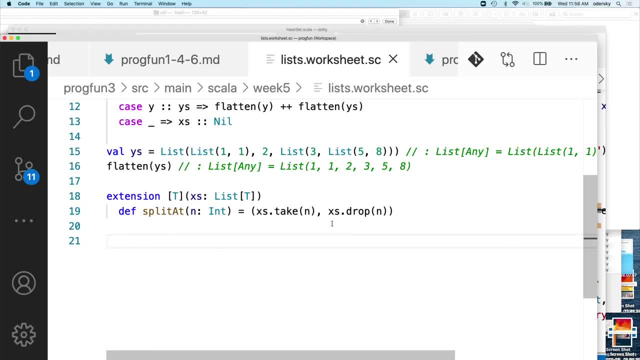 up to index n and the second half is xs, drop n. so all elements of the list except the n first ones. now we can test that by writing. let's say, split at two with our list of xs from the last section, and that would give us a list where the original list 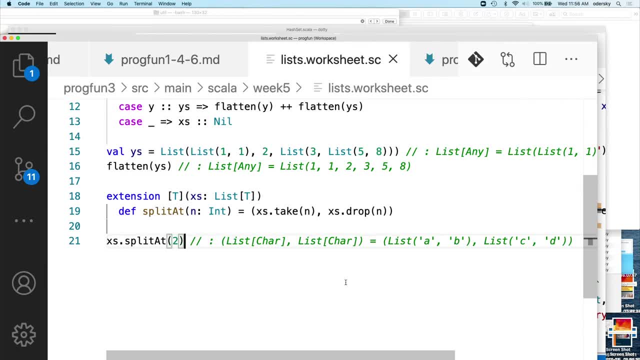 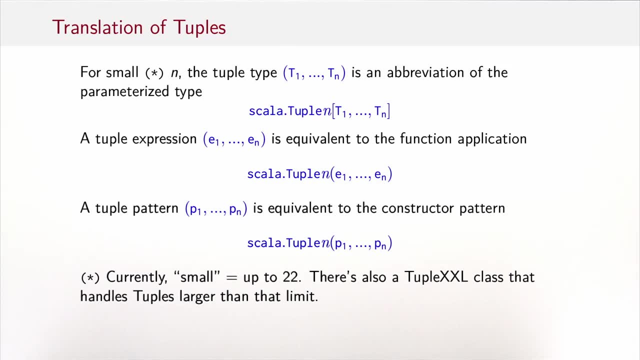 a, b, c, d was split into two halves, a, b and c d. so so far every type in Scala was an instance of some class. the same holds for tuples, so for smallish n the tuple type t1 to tn is just an abbreviation for the parameterized type. 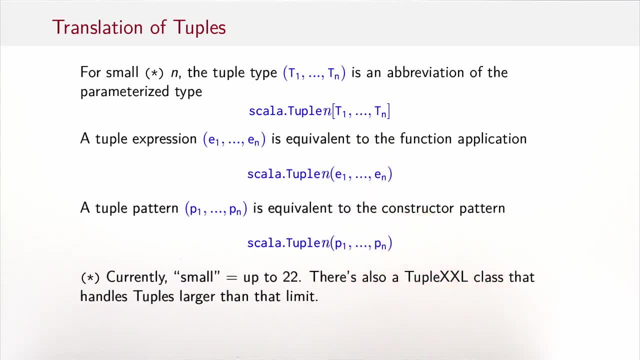 Scala tuple, then the number n and then the arguments t1 to tn. so the pair int string would be an abbreviation of tuple 2. I leave out the Scala prefix of int string. for larger tuples, tuples with length more than 22, we have a special class. 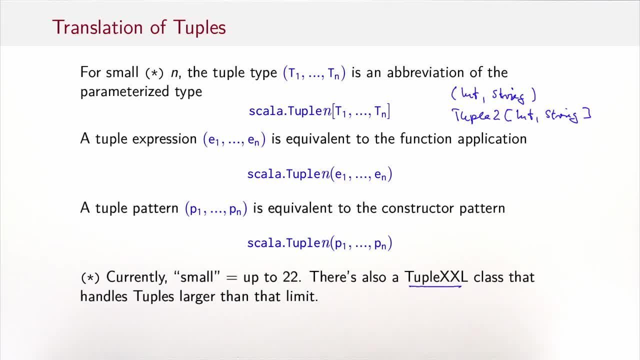 tuple xxl. that essentially collects all elements in an array and then stores them in the tuple xxl class. so yes, tuples are instances of classes, but there is a difference whether the tuple is of moderate size, so up to 22, or beyond that, where we have 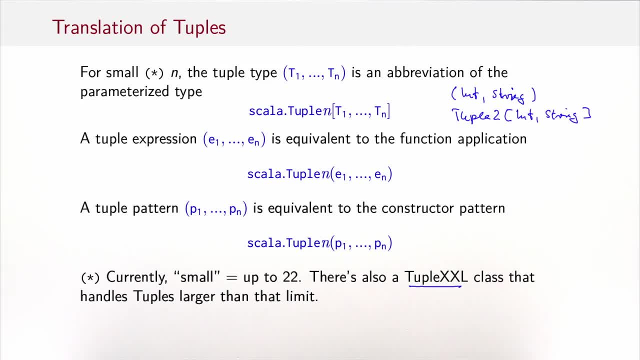 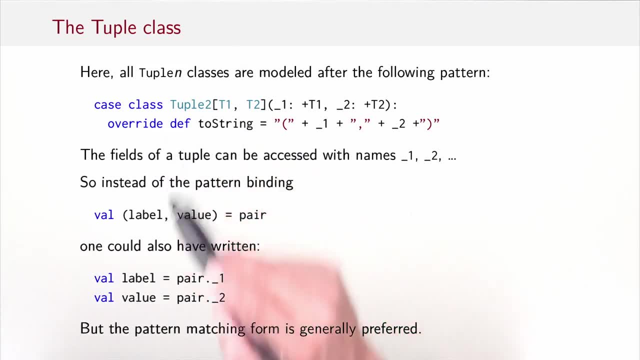 essentially a class that collects tuples of all different sizes. so if we look at each of the tuple classes, then they are all modeled after the following pattern. here we have the example with tuple 2, the pair class, so it takes two type parameters, t1 and t2, and it takes two. 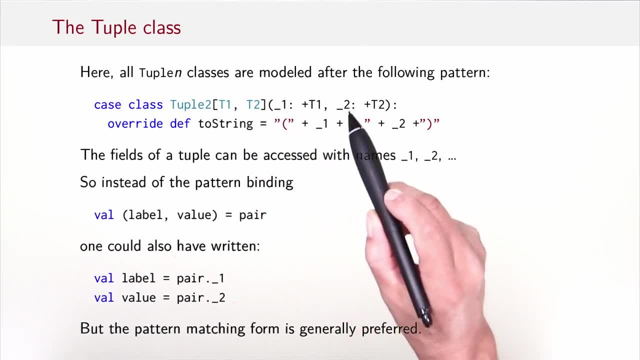 selectors which are written underscore 1 and underscore 2, and the first one is of type t1, the second is of type t2. they are both covariant. so tuples are covariant in both of their argument types and they override the two string method so that they look like a pair. 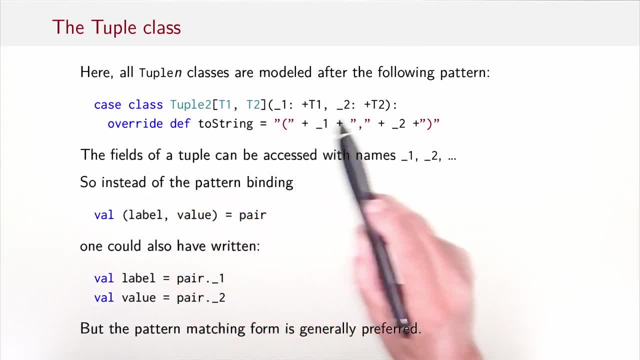 because tuples are case classes, it means that these selector values are also available as fields. so instead of the pattern binding: val label value equals pair, you could also have written: val label equals pair. dot underscore 1, which selects the first half of the pair, and val value. 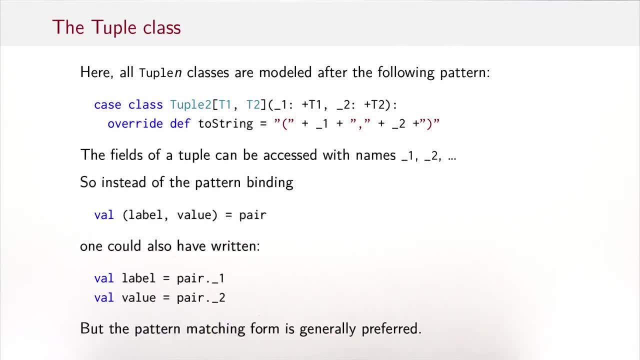 equals pair underscore 2. normally, at least if you want to match on all elements of a tuple, the pattern matching form is more concise and it's clearer, so it's generally preferred. the individual selectors can sometimes be useful if you have a long tuple and you just want. 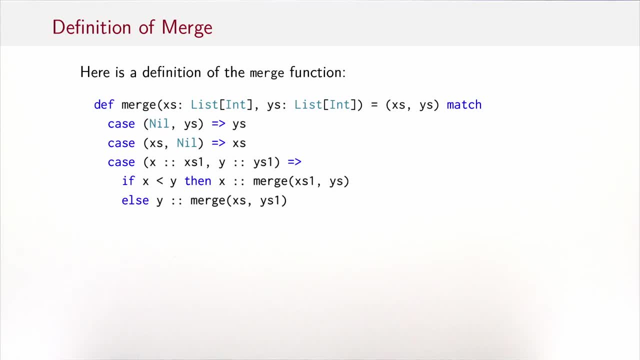 to select a single element, for instance. so to complete merge sort, we still have to define the merge function here it is. so merge takes two lists of integers which are both assumed to be already sorted. it then does a pattern match on the pair of xs and ys. 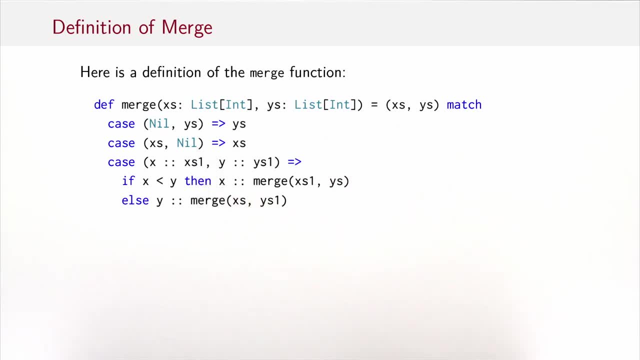 so we form a pair of the two lists and we match with pairs in turn. so if the two lists are nil, ys, that means the first list is nil, the second list is arbitrary. then we return the second list. there's nothing to merge if the second list is nil. 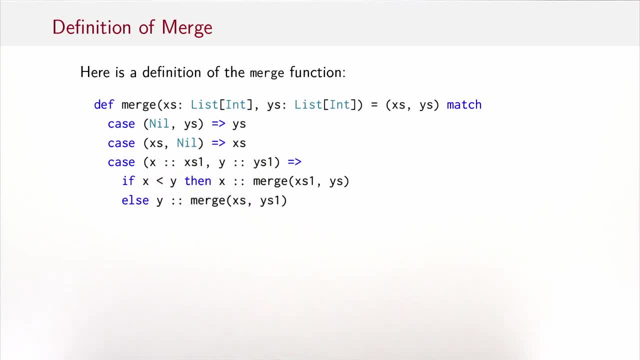 and the first list is either nil or has some elements. we return the first list if both lists are non-empty. so the first list, let's say, starts with x and the second list with the variable y. then we have a distinction whether x or y is the smaller elements. 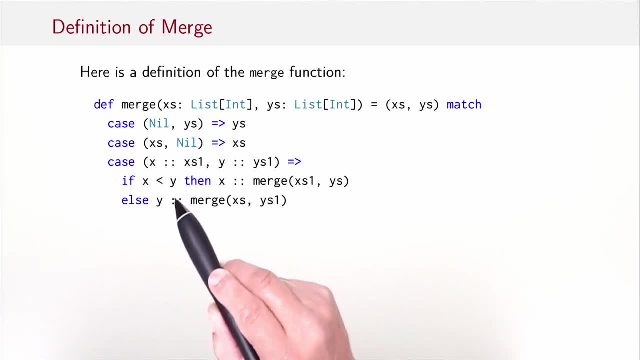 so if x is less than y, then the merged list would start with x and be followed by the merge of the rest of the xs list and all of the ys list. otherwise, it would start with y and be followed by the merge of all of the xs list. 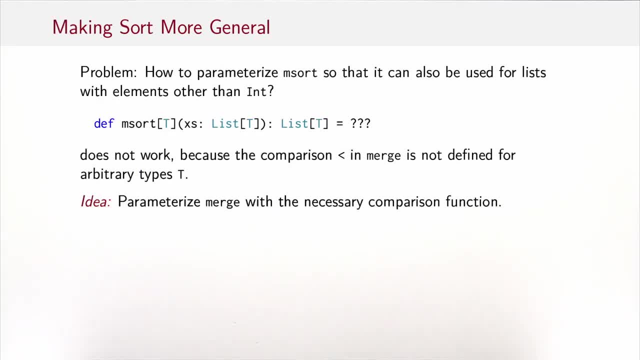 and the rest of the ys list. ok, so that was merge sort on int lists. but of course we'd like to generalize it so that it can also be used for lists with elements other than int, if we just add a type parameter to msort, like this: 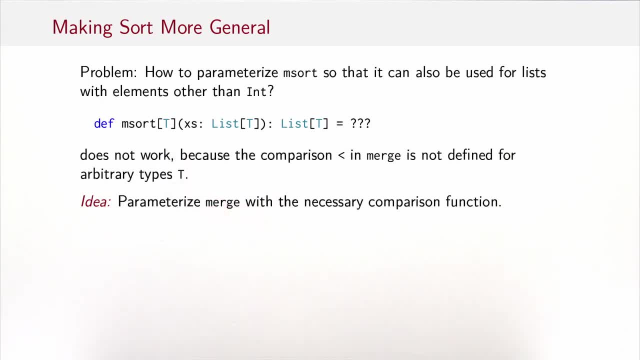 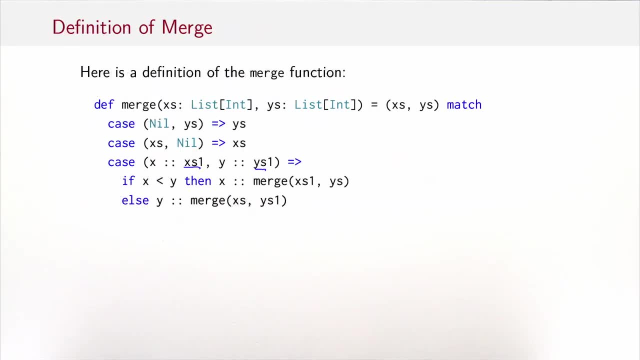 so we replace the int by t, which is a type parameter. that wouldn't work. why? well, because the comparison in merge is not defined for arbitrary types t. so let's look at merge again. here is the comparison. it is defined for int, of course, but it wouldn't be defined for arbitrary types t. 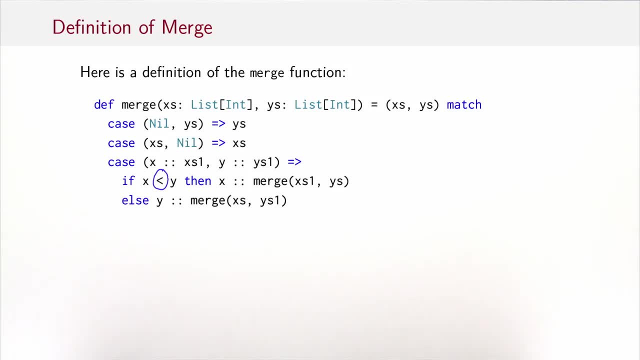 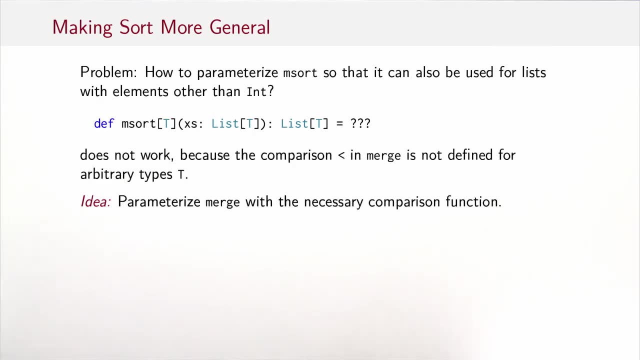 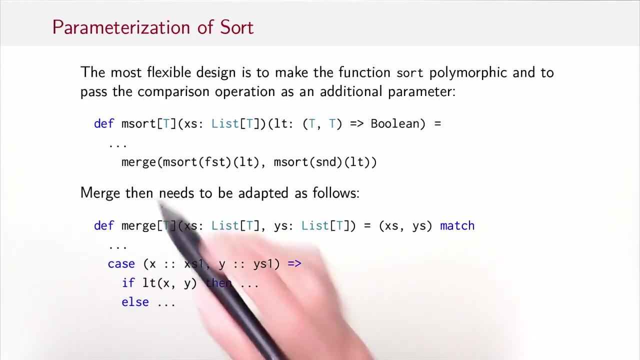 if we just given a type t of which we know nothing, then we cannot assume that it has a comparison function less than defined on it. but what we can do is to merge with the necessary comparison function. so let's do that next. so here we have a new version. 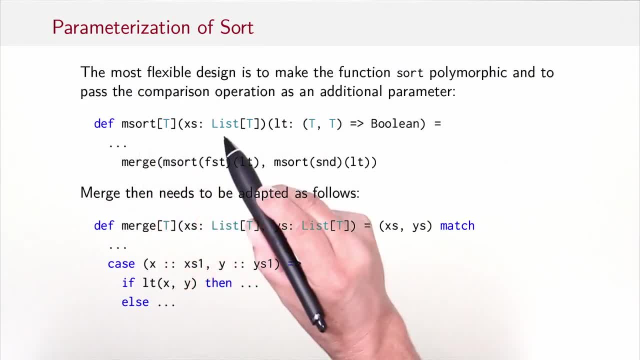 of merge sort, which is now polymorphic. it takes lists of t for arbitrary t and it also takes a comparison function, less than that, takes two elements of type t and returns a boolean. so if we have set up things like this, then in the recursive call we have to go on and pass less than. 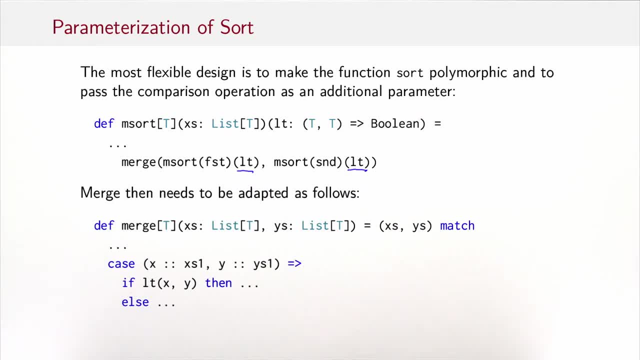 to the two recursive invocations of merge sort, because otherwise we would miss a parameter and then merge also needs to be adapted. the merge function is defined inside merge sort, so it would see the less than function. that's ok, but here at the comparison we would have to call that comparison function. 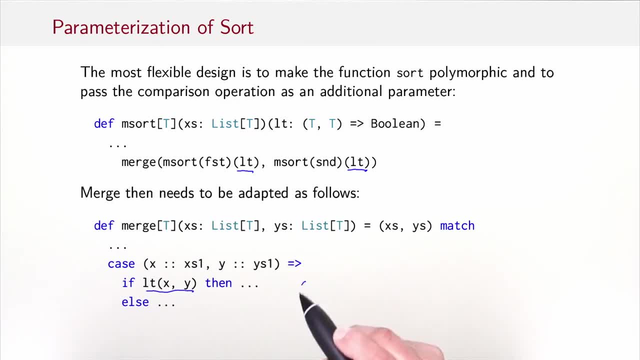 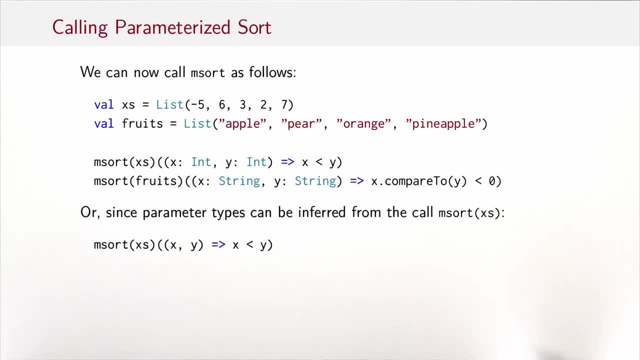 less than x and y. instead of calling x less than y, what we did previously, we can now call msort as follows: to sort a list of integers, we pass that list xs and the comparison function less than on integers. to sort a list of fruits, which is a list of string. 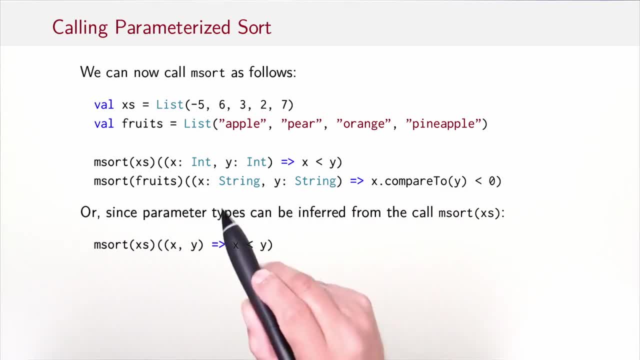 we pass the comparison function on string, which in this case would be the function that takes two strings, applies the compare to function, which is a function known in java from strings, and says the value of compare to should be less than zero. so that's equivalent to a less than. 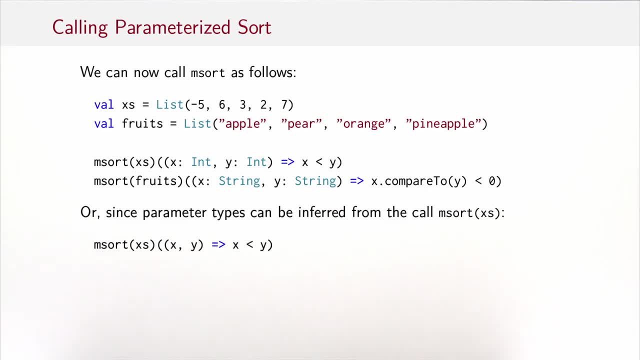 on strings, note that the type arguments of msort have been inferred in each case, so we could have written int here and string here. but that's not necessary because the compiler will infer it from the types of the arguments. and as another simplification, the compiler can also: 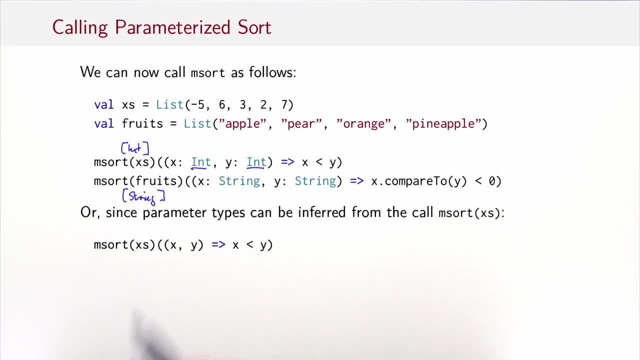 infer the types of the parameters here, because it knows when it sees the list xs that we intend to do a merge sort on int. so we need a comparison function on two ints. so that means we can write it even shorter: merge sort xs and y arrow. x less than y. 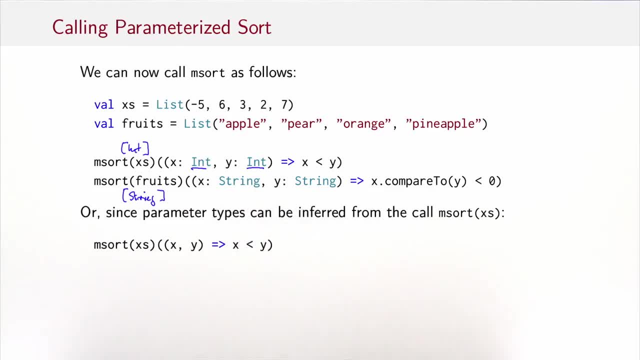 so we don't really need the parameter types here, nor do we need them in the string example. now you could say: well, even that is too much noise for me, couldn't the compiler have inferred the correct comparison function for the parameter type? so that means we now ask the compiler. 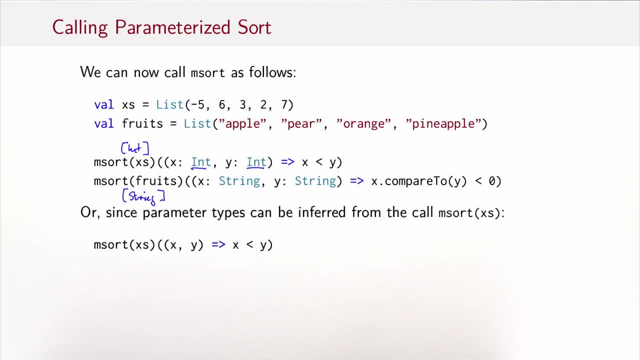 not just to infer a type, but to infer a value that we say: well, for int, what's the correct comparison function? or for strings, what's the correct comparison function? and in fact we will see that this is possible, but it will take us several weeks to get there. 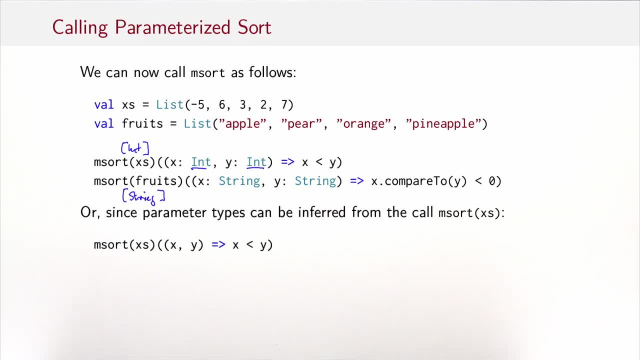 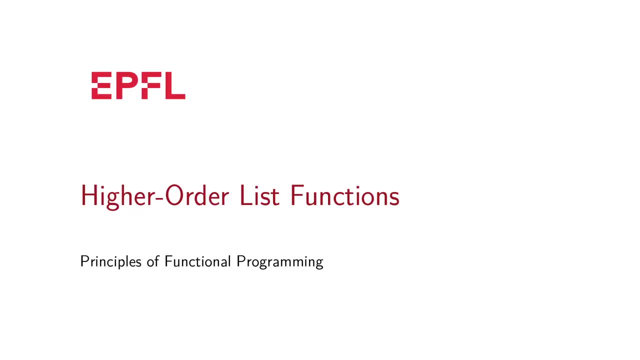 we will have a week on implicit parameters. that does precisely that- that it can infer missing parameters from their types. in this session we'll introduce higher order list functions. you've seen already that they can be very useful. that holds particularly for lists where there are many very common operations. 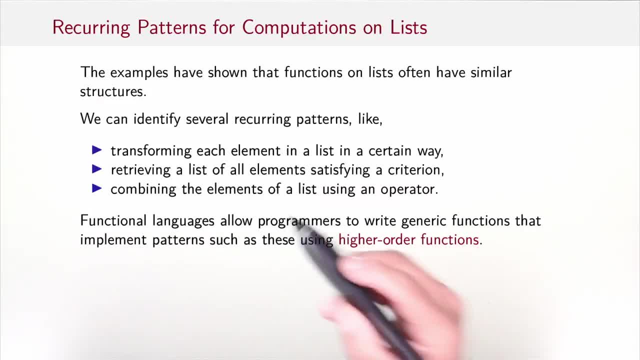 that can be abbreviated with higher order functions. the list examples we've seen have already shown that functions on lists often have quite similar structures. we can identify several recurring patterns, like transforming each element in a list in a certain way or retrieving a list of all elements that satisfy some criterion. 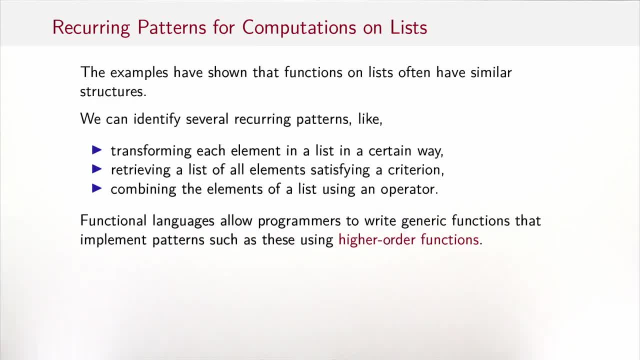 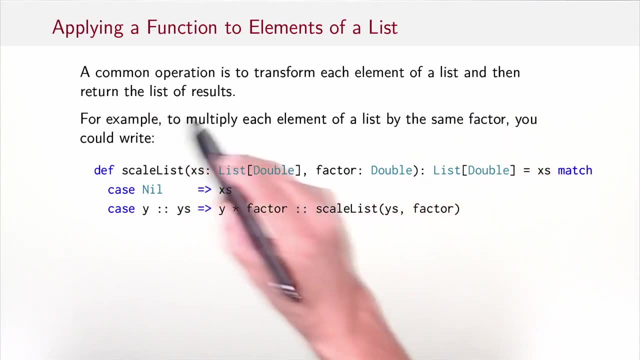 or combining the elements of a list with the operator function. languages allow programmers to write generic functions that implement patterns such as these using higher order functions. so here's an example of the first category. a common operation is to transform each element of a list and then return the list of results. 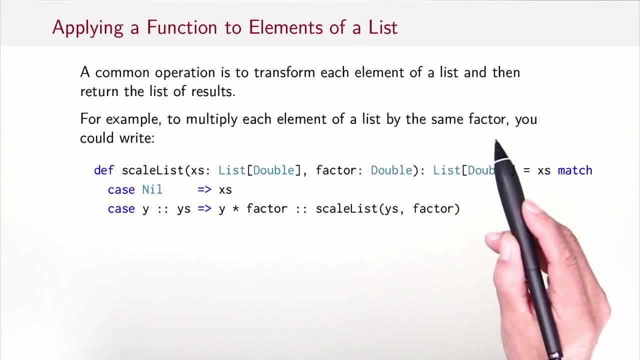 for instance, we might want to multiply each element of a list by a given factor. we could do this with this function here, scaleList. it takes a list and a factor to return it. if it's non-nil starting with y, then multiply y with factor and do a recursive call of scaleList. 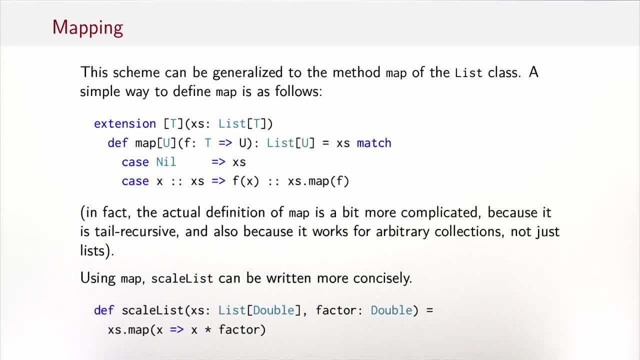 of the rest with the same factor. this scheme can be generalized to the method map of the list class. a simple way to define map is shown here. we've defined it as an extension method on lists of arbitrary type t map takes a function from t to some new type u. 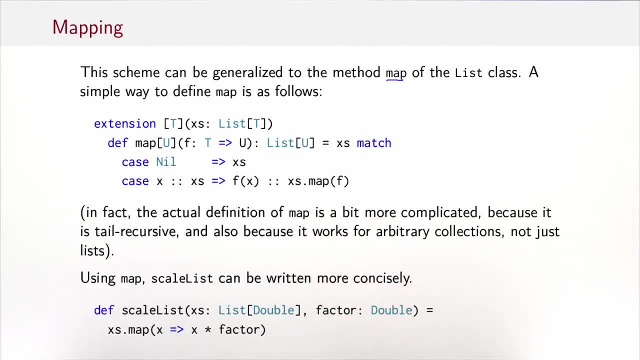 as additional parameter and returns a list of u's, and it's implemented as follows: we do a pattern match on xs. if the list is nil, then we return the empty list. if the list is non-nil, with head element x, then we apply the function f to x. 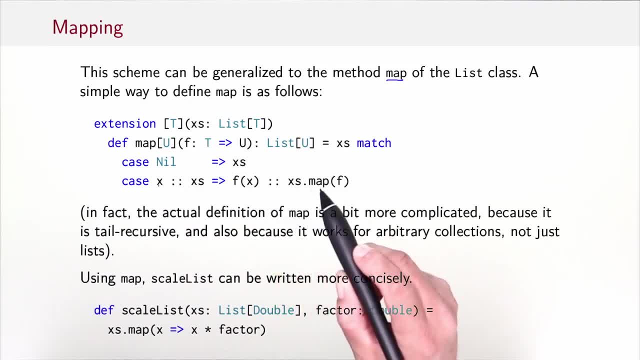 and cons it with the recursive call on map over the rest of the list with the same function f. in fact the actual definition of map is a bit more complicated because it is tail recursive and also because it works for arbitrary collections, not just lists. but to understand the functioning on map for lists, 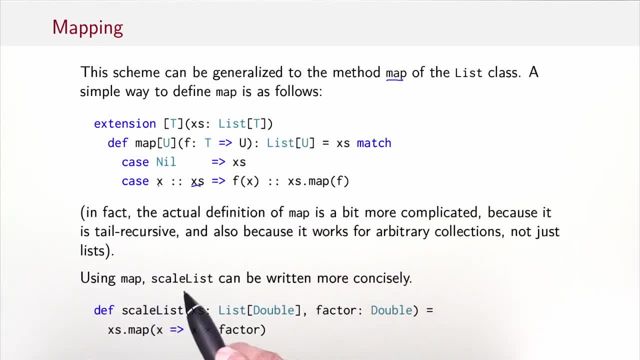 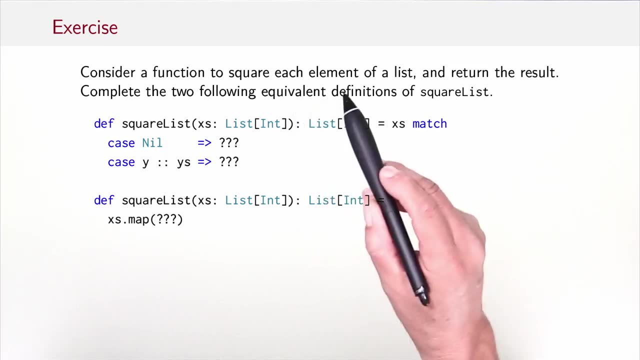 this will do using map. we can now write scaleList more concisely. we can just say: scaleList is xsmap of x taken to x times factor. so let's do a similar exercise. let's consider a function to square each element of a list and return the result. 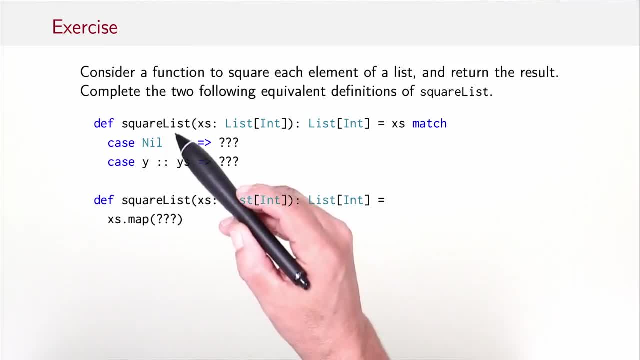 there are two equivalent ways to do it: one as a recursive definition and the other as a call to map. let's fill in the question marks for both of the alternatives. so the recursive definition: we map nil to nil. we map y, followed by ys to y times y. 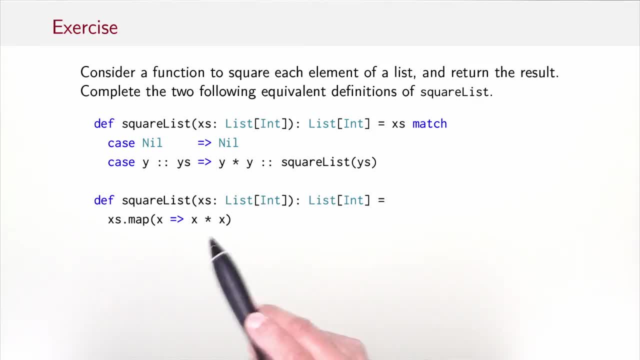 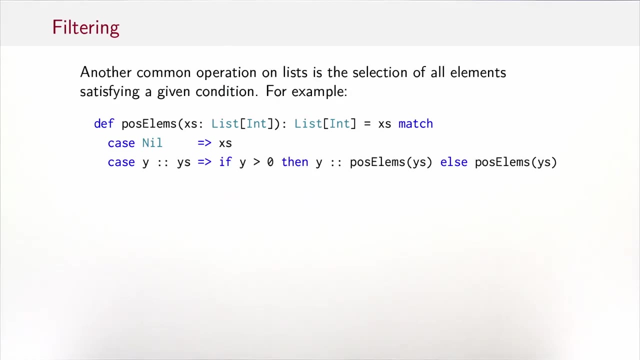 cons: square list: ys as usual, and for map it's a lot simpler. square list is simply xsmap with the squaring function. so we see that map is a very handy tool for all cases where we transform each element of a list into a transforming function. another common operation on lists: 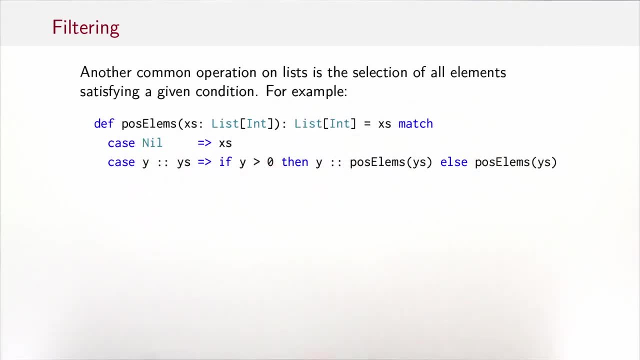 is to select all elements that satisfy a given condition. for example, here we have a function that takes the positive elements of a list of integers. poslms is defined with a usual recursive pattern: match. if the list is nil, we return xs. if the list is not nil. 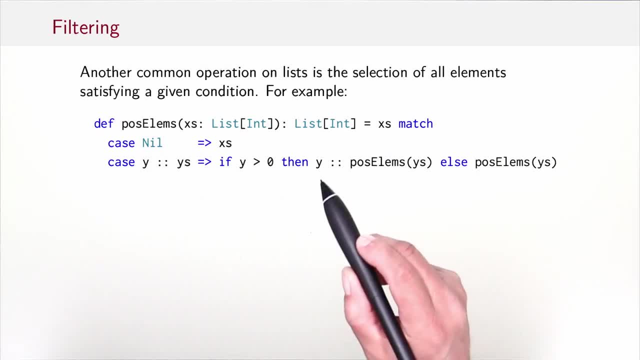 with head element y and y is greater than 0, then we return a new list with y followed by poslms ys, and otherwise we just return poslms ys without the head element y. this pattern is generalized by the method filter of the list class. 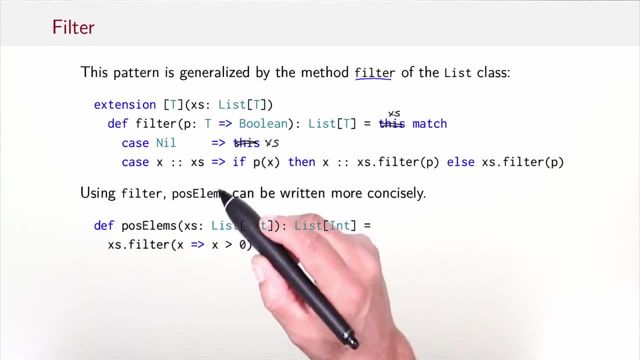 here is a possible definition of filter as an extension method. it's defined on lists of arbitrary type t. it takes a predicate function that maps values of t to type boolean and returns a list of t, and its implementation is a pattern match on the list xs. so if xs is nil, 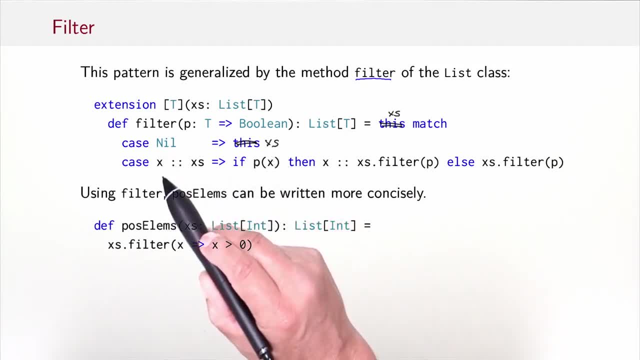 we return xs unchanged. if xs is not nil, then if the predicate holds for the first element of the list, then that gets included in the result and we follow with the recursive call filter p on the other elements- xs, and otherwise we just return filter p over the other. 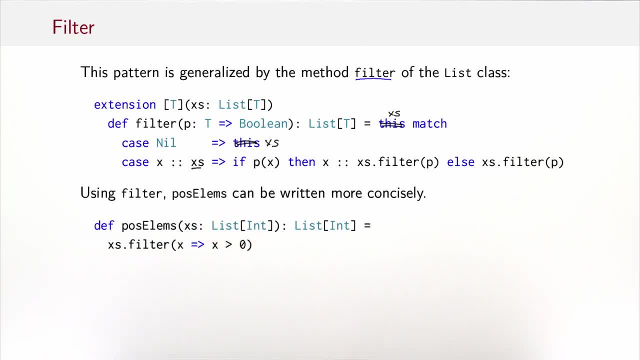 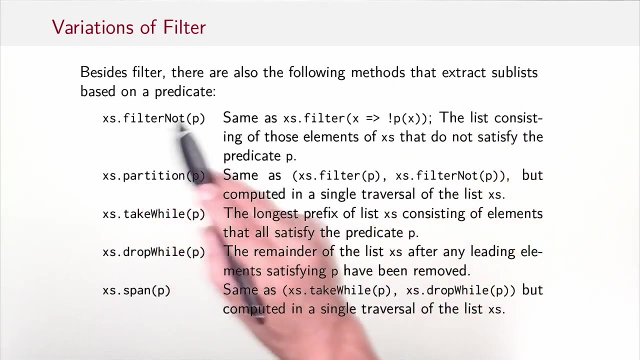 elements xs without the head element x. using filter, we can now write poslms more concisely like this: it's just xs filter with the function x that tests whether x is greater than zero. besides filter, there are also the following variations that extract sublists based on a predicate. 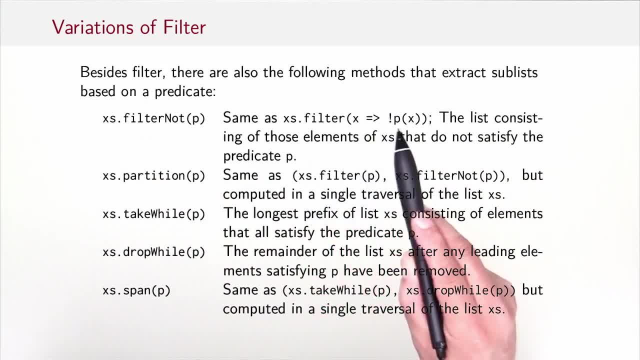 we have filter not, so that's the same as filter- with the predicate that negates p. so it's the list consisting of those elements of xs that do not satisfy the predicate p. then we have partition, that's the same as the pair of lists. the first list is xs, filter p. 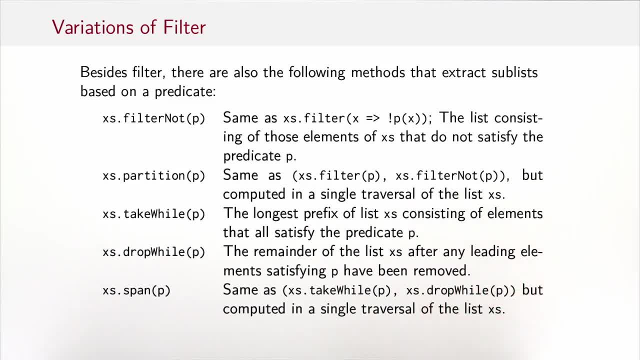 the second list is xs filter, not p. so the first list gives you all the elements of xs that satisfy p. the second list gives you all the elements in xs that do not satisfy p. but the two lists are computed in a single traversal of the list xs. 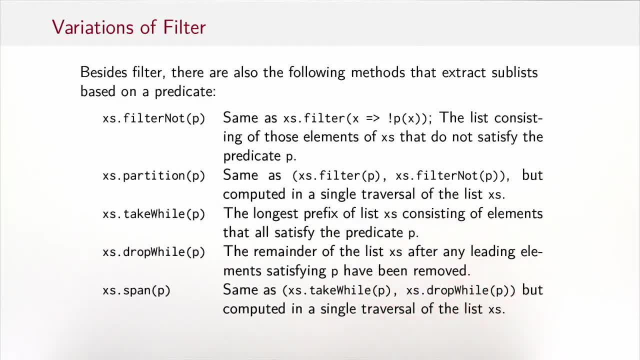 so it's more efficient than two separate calls to filter and filter not the take. while method is a bit like filter, but not quite. it gives you the longest prefix of the list xs consisting of elements that satisfy the predicate p, so the first element that does not satisfy p. 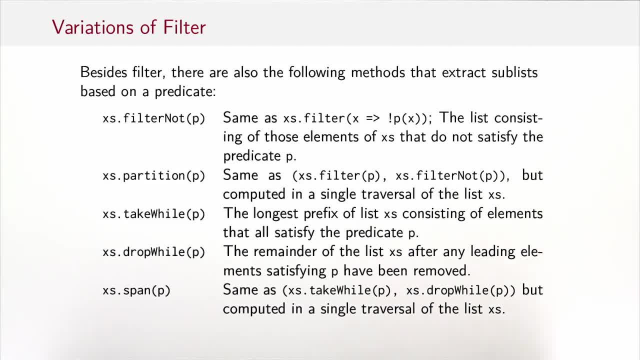 terminates the output, whereas filter would go on and look for other elements that satisfy p in the rest of the list. drop while is the dual of take while, so that means we drop elements of the list until there is an element that does not satisfy p. we drop the longest prefix of the list. 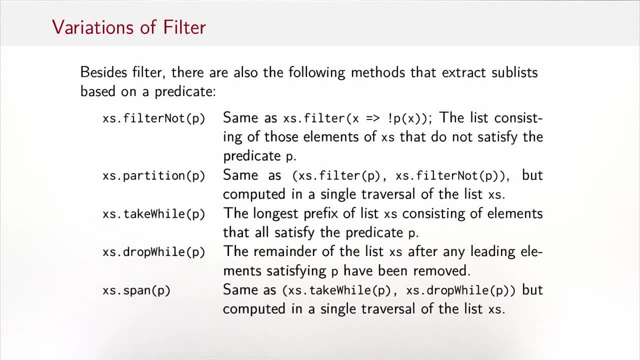 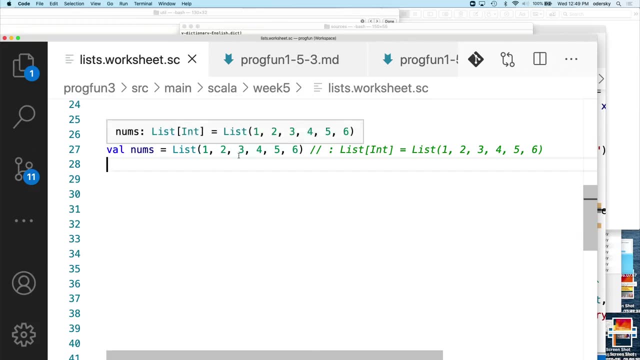 of elements that do satisfy p. and finally we have xs, span. p, that's the same as take while, drop while, but computed in a single traversal of the list: xs. so to illustrate the difference between partition and span, let's write a list of numbers and partition, the list. 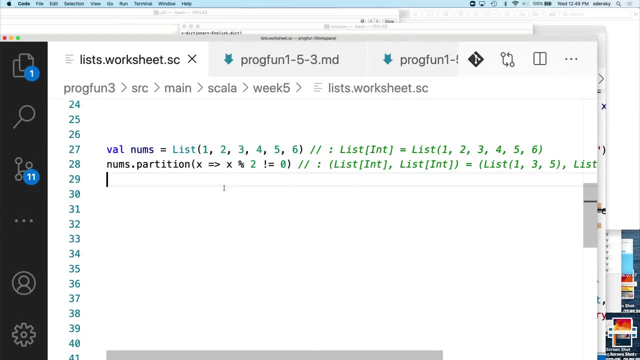 with the predicate testing whether an element is odd. so what we get is two lists. the first list are the list of odd elements and the second list is the list of even elements. let's do the same thing now, but with span instead of partition. we get a list one. 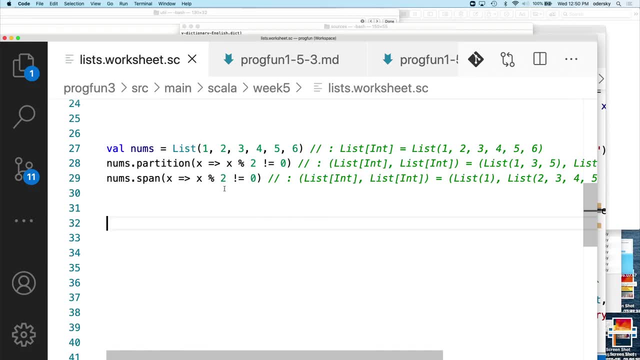 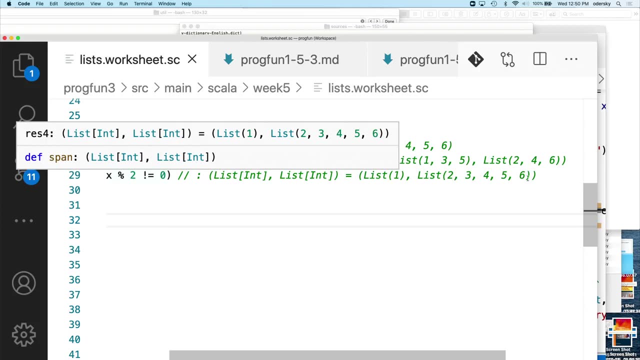 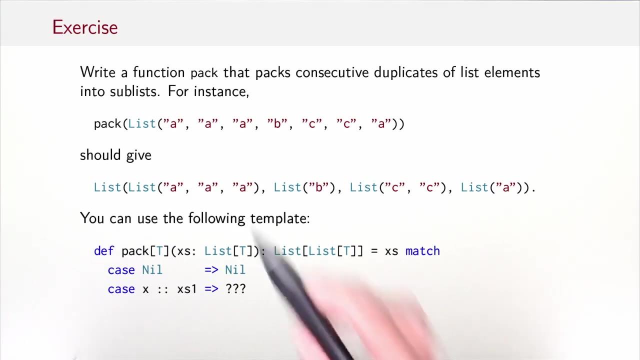 as the first element. so that's the longest prefix of the list that consists of odd elements. that's just a single element and the remaining list is all the elements after this first element. so here is an exercise for you: write a function pack that packs consecutive duplicates. 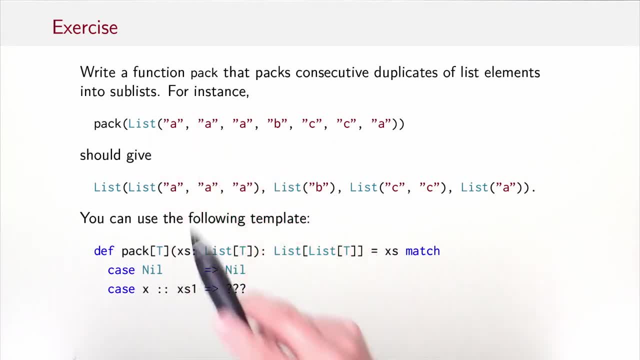 of list elements into sublists. so, for instance, if you have a list consisting of three a's, a b, two c's and an a, then we should return a list consisting of four sublists: first the three a's, then the single b, then the two c's. 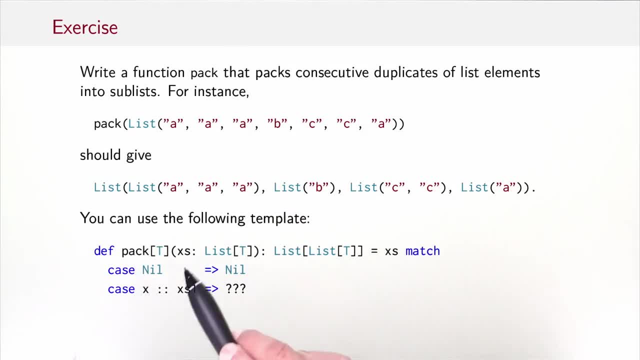 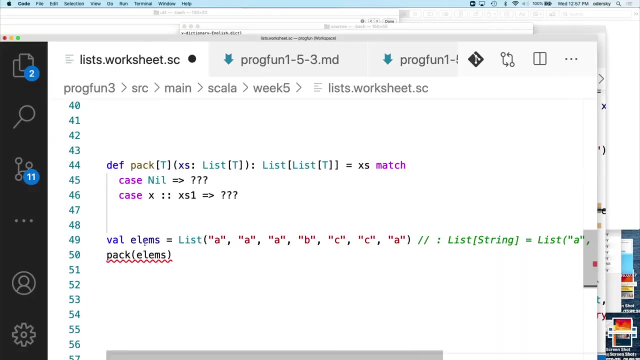 and finally the remaining a. you can use the following template: pack takes a list of arbitrary type t, returns a list of list of t and it uses the usual pattern match between nil and non-empty lists. so I've set up the example in the worksheet. we have the template for the pack function. 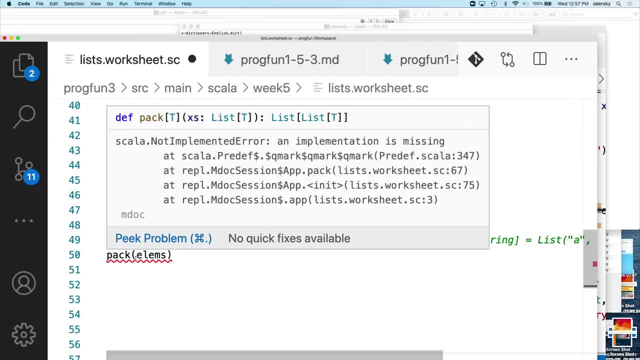 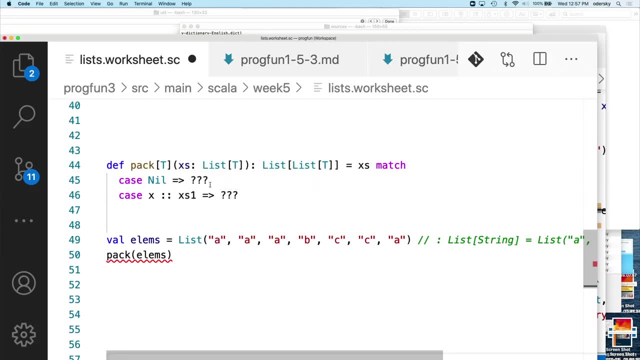 we have the example list elements and the call pack elements right now gives us a not implemented error because of the triple question marks here which we have to replace. so what do we do in the case of nil? well, if the list is empty, then we should return the empty list. 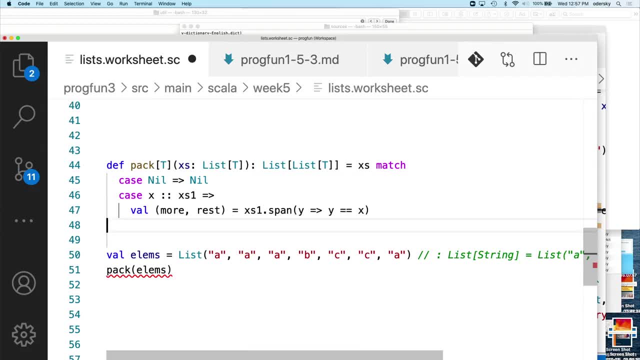 because there is nothing to pack. what if x is not nil? let's say, it starts with x and is followed by xs, then one thing we should do is collect all elements that are equal to x, and they will be collected into the more list, and then that should be followed. 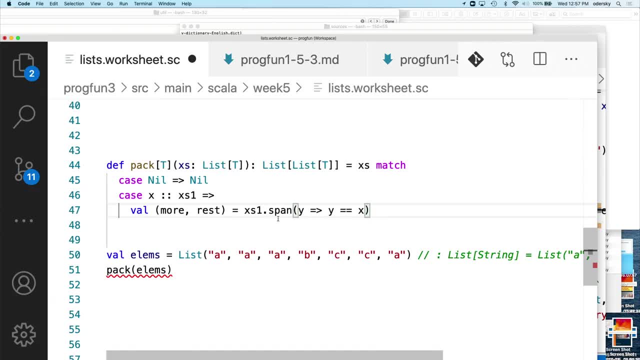 by all elements that remain in the list. so we can do that with the call to span and the predicate that tests whether a given value is equal to x. so once we have that, what do we do? well, we could return more, followed by pack of rest. let's see whether. 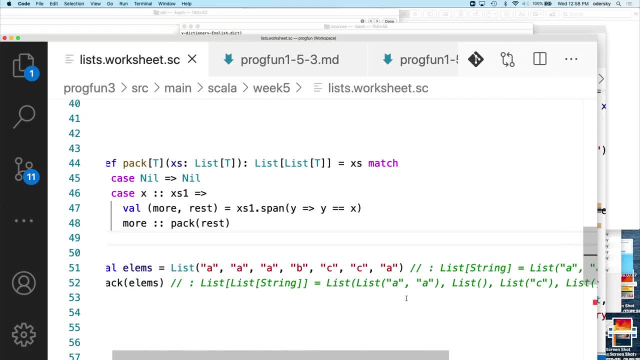 this would work. we get a result, but there is always the first value missing. we get only two a's instead of three, no b instead of one, one c instead of two. so where did we go wrong? well, we haven't included the x in the result list. 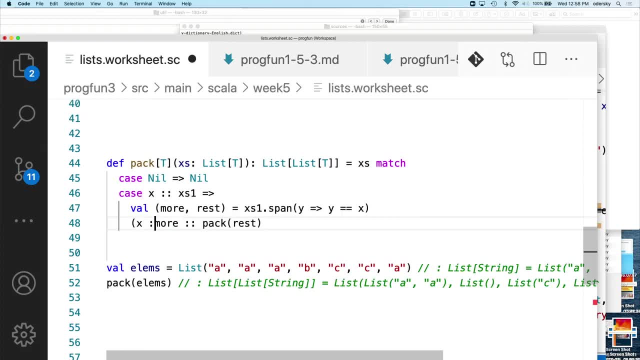 it's just the following elements that equal x that we excluded, but we forgot x, so let's add x to the first element as the first element of the first element of the result list, and that would now give us a result which is correct and the logic looks good as well. 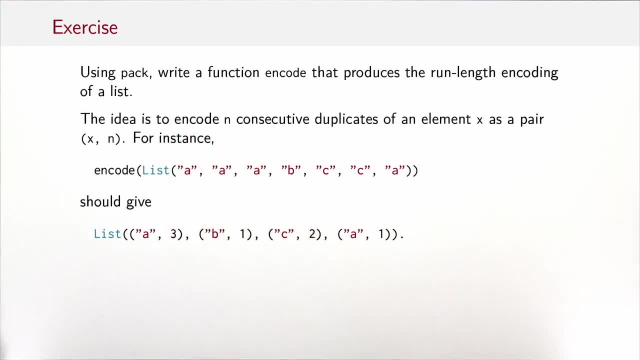 now let's follow this up with another exercise. using the pack function that you've written before, write a function encode that produces the run length encoding of a list. the idea of a run length encoding is that we want to encode n consecutive duplicates of an element x. 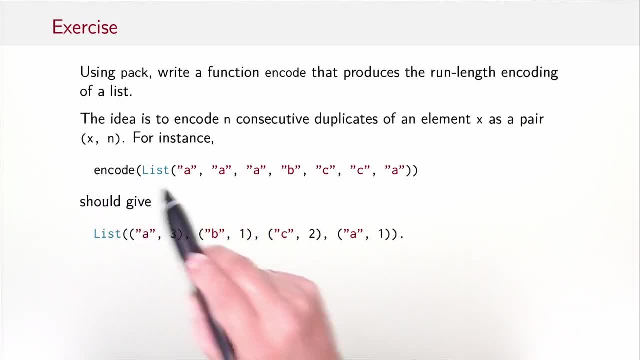 as a pair: xn. so for instance, the encoding of this list here is a list of four pairs. the first pair says we have three a's. the second pair says we have one b, two c's and finally one a. so a run length encoding of a list can compress a list. 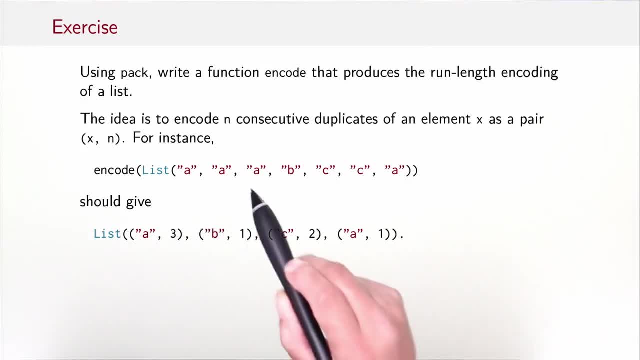 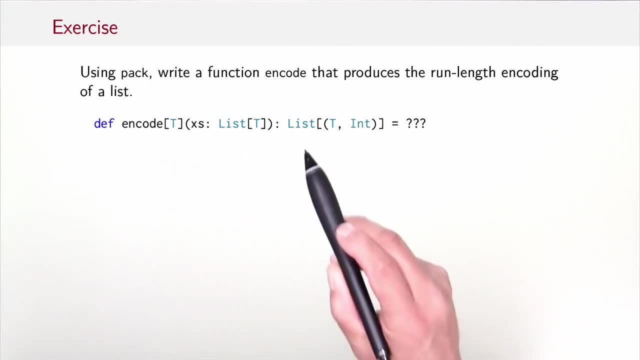 if it is quite common that an element appears several times consecutively in the list. so here is the outline of encode. it takes a list of t and returns a list of pairs of t's and ints. that's the length counts and all that remains is implemented. 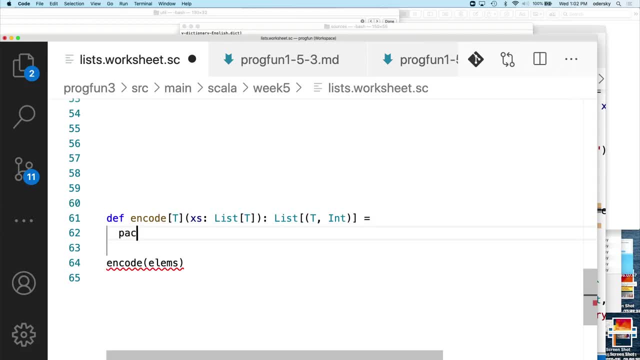 so I've given the template for encode in the worksheet to implement it. let's start with packing elements, so that would give us a list of list of t's. now what we have to do is get from this list of t in the element list to a pair, which is the element in the list. 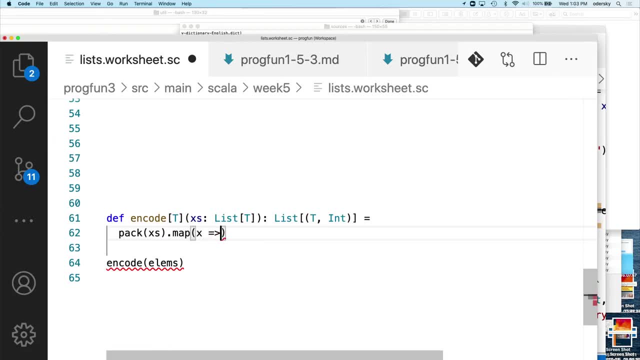 plus the length, and we do that with a map, so we say map with the function x that returns xhead as the element and xlength as the list, and if we do that, then we get a list of pairs of strings, of integers, which consists indeed of: 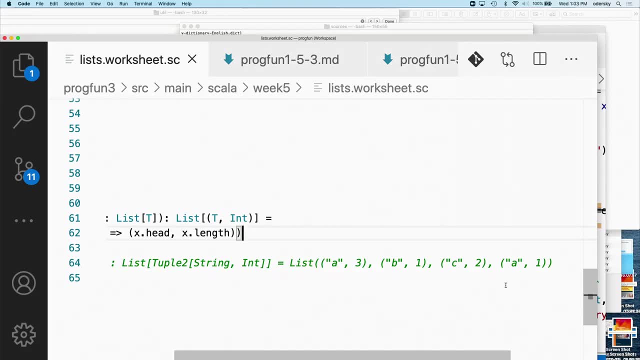 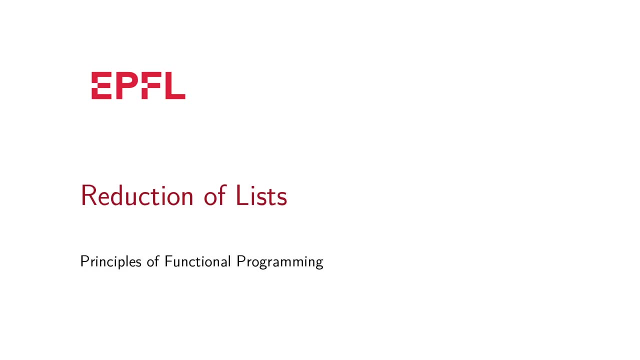 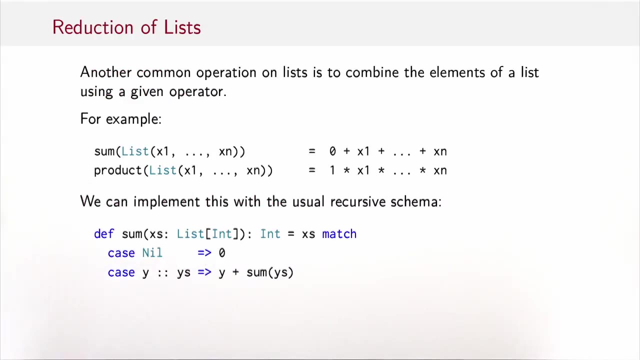 three a's, one b, two c's and one a. in this session we are going to look at another set of operators that serve for reducing lists. in fact, it's quite common to combine the elements of a list with a given operator. for instance, to sum all the elements of a list. 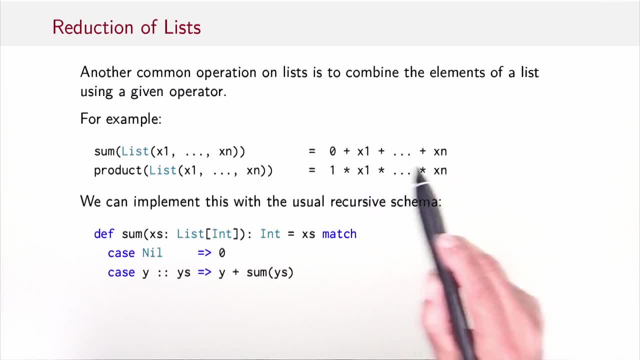 you could use an operation like this one: so x one plus x n, and for the empty list you would return zero. or to take the products of all elements, you would arrive at this formula: multiply all the elements of the list and multiply by one, which gives you one for the empty list. 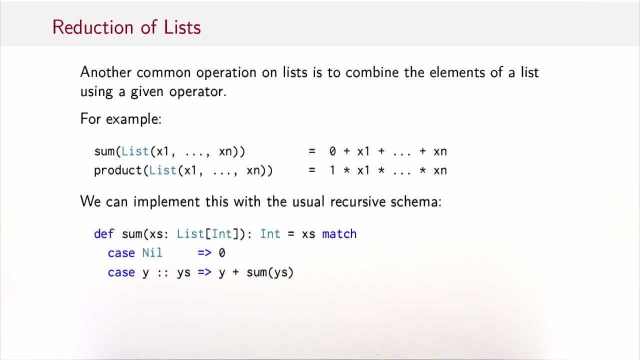 we can implement this with the usual recursive schema. so, for instance, for sum, it would look like this: sum takes a list of int, returns an int x match. if it's nil, then it's a zero. otherwise, if it's a list starting with y, it's y plus. 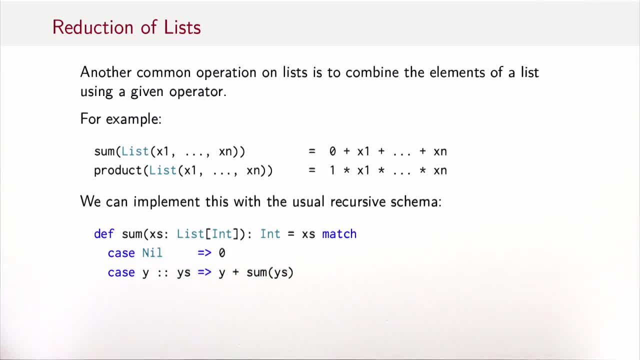 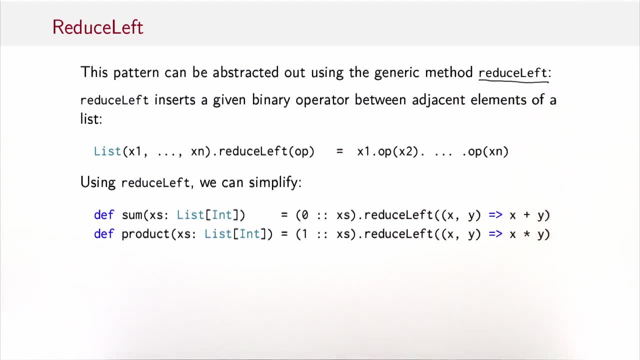 sum of the remaining elements, y. this pattern can be abstracted out using the generic method, reduceLeft. reduceLeft inserts a given binary operator between adjacent elements of a list, a list of x, one to x n, and you do a reduceLeft with op and that would give you 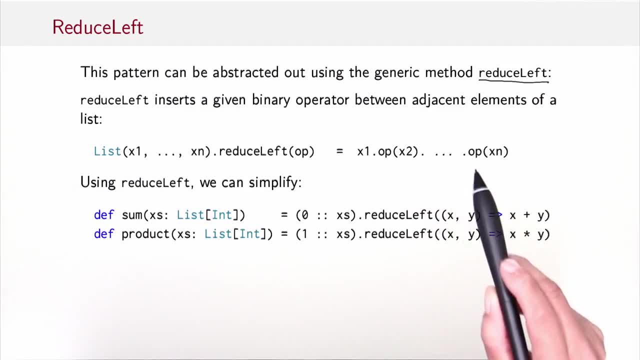 x one, dot op x two, dot op x three, and so on until dot op x n. if you have reduceLeft, then we can simplify sum it product as you see here. sum would be just zero cons xs, reduceLeft, with the summation function and product would be: 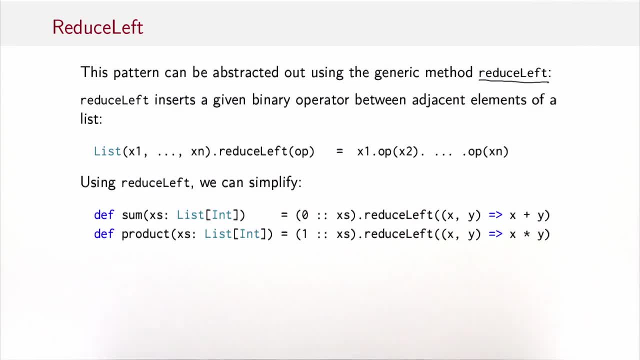 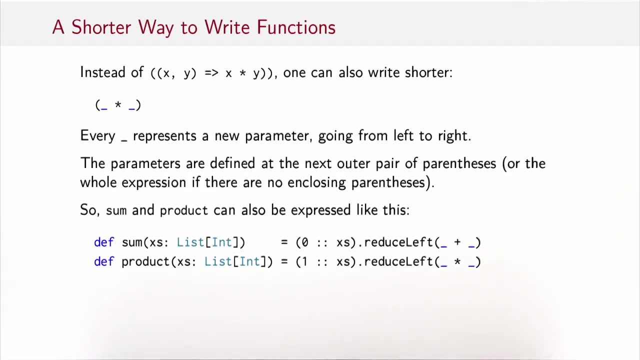 one and xs reduceLeft with the multiplication function as an aside, we can write these functions that we pass to other functions also in a shorter way. instead of x y arrow, x times y, for instance, one can also write shorter underscore times underscore. every underscore in a formula represents. 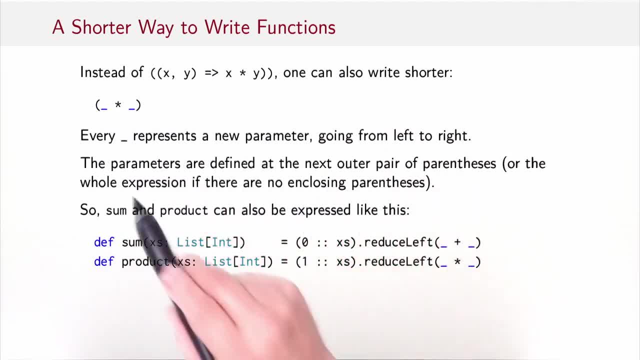 a new parameter going from left to right, and the parameters are then defined. so this thing here would be inserted at the next outer pair of parentheses, or the whole expression if there are no enclosing parentheses. so essentially, you go left to right, you note the occurrences of an underscore. 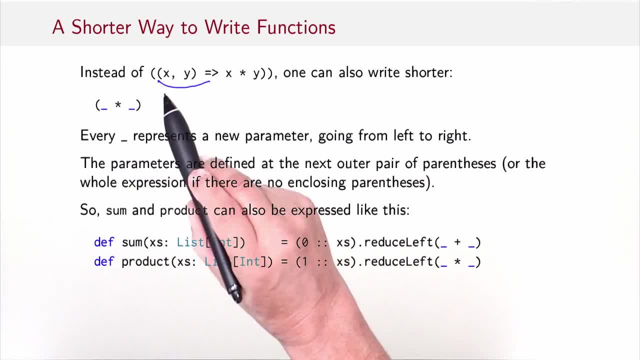 once you hit a pair of parentheses, you insert a parameter section, one parameter for each underscore that you have encountered. so with that, sum and product can also be expressed like this, which is aesthetically a bit more pleasing. so sum would be zero, followed by xs reduceLeft. 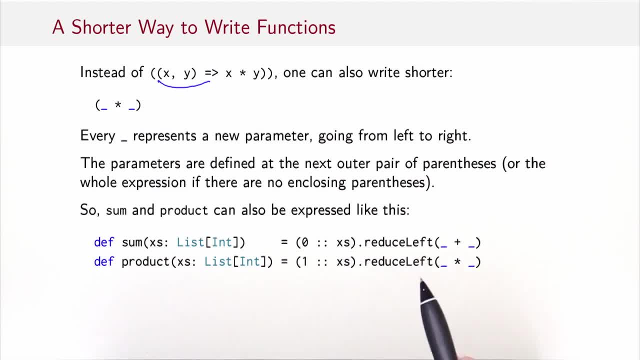 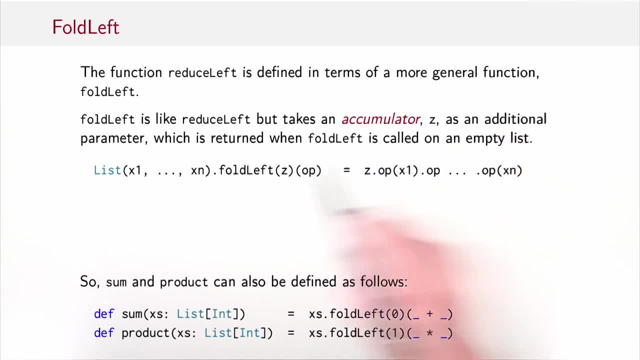 with plus and product would be one followed by xs, reduceLeft and multiply. the function reduceLeft is defined in terms of a more general function: foldLeft. foldLeft is like reduceLeft, but it takes an additional argument: an accumulator named z. here. that accumulator is returned when foldLeft is called. 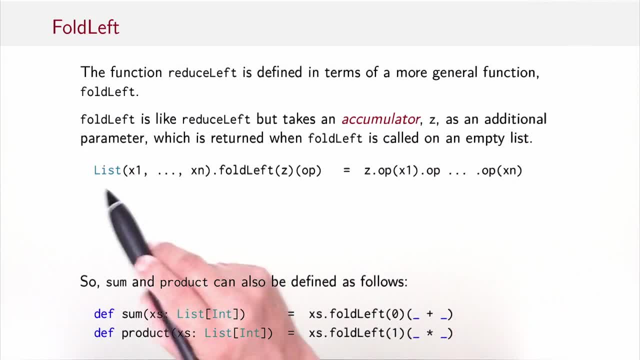 on an empty list. so if we take a list of elements x1 to xn and we do a foldLeft with the zero z and the operation op, then that would be zero dot op x1, dot op x2 and so on until dot op xn, or visually. 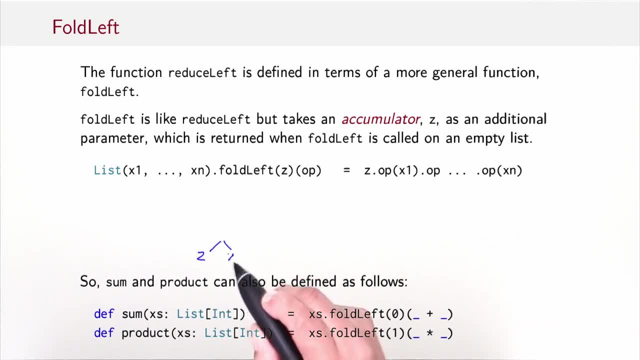 it would look like this: so you have the zero on the left and you have the x1 here and you have the operation and you build up operations until you finally combine with xn. so it's a left leaning tree with operations at the node and zero at the lower. 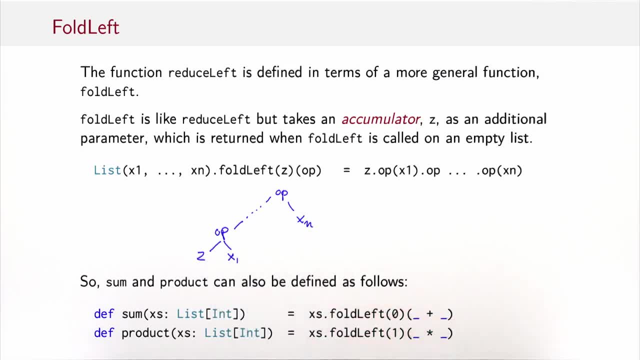 left corner and the elements x1 to xn as the leaves on the right. so with foldLeft, we can now define sum and products as follows: sum of xs would be xs- foldLeft, with zero as the identity and plus as the operation, and product of xs would be xs. 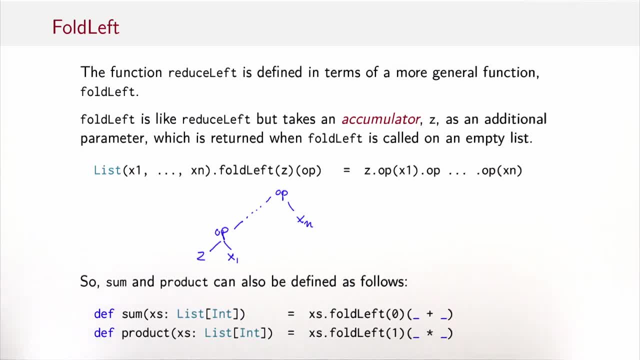 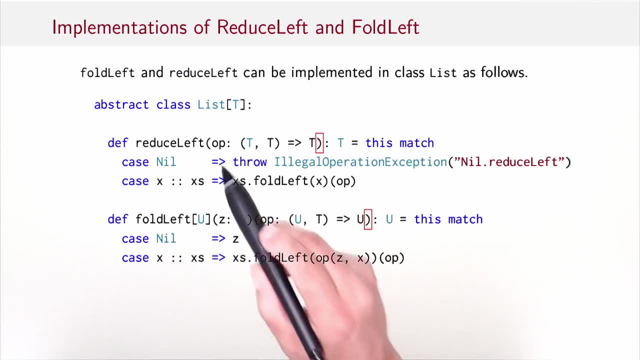 foldLeft, with one as the identity and times as the operation. so now that we have foldLeft, we can define reduceLeft in terms of it. so reduceLeft takes an operator from t and t, the list element type to t, and returns a t and its body is defined. 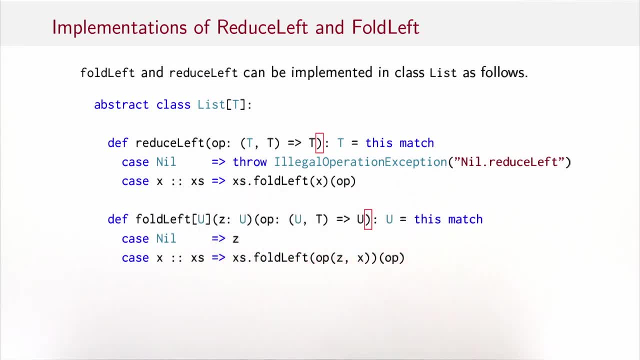 only for non-empty lists. so if the list is empty, we throw an unsupported operation exception. if the list is non-empty- x followed by xs- then we do a foldLeft on xs with the zero element, x, so the first element and the given operation. so we've seen that applications of 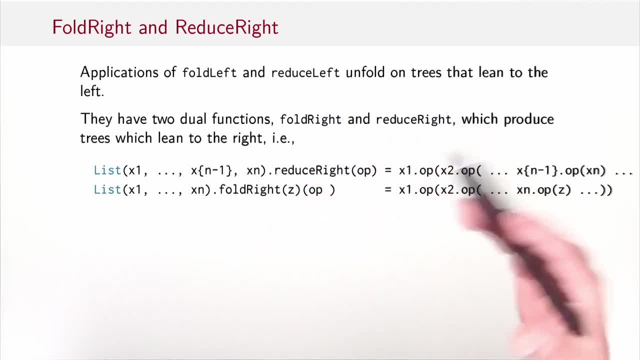 foldLeft and reduceLeft can be visualized as trees that lean to the left. there are also two dual functions, foldRight and reduceRight, which produce trees which lean to the right. so here are the definitions of reduceRight and foldRight. let's look at foldRight first. 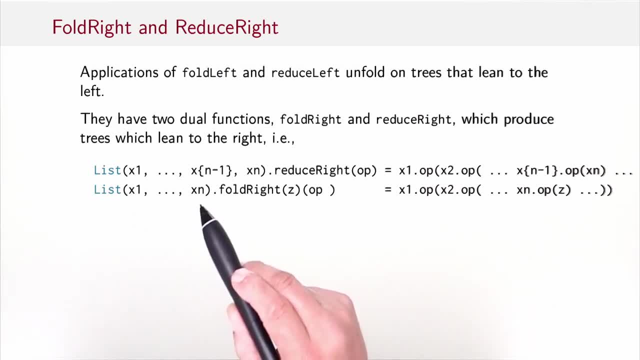 so if we do a foldRight on a list x1 to xn with a zero z in our operation and we get this right hand side, and if we want to draw that, then it looks like this: so it's x1 up, x2 up and then the list goes down. 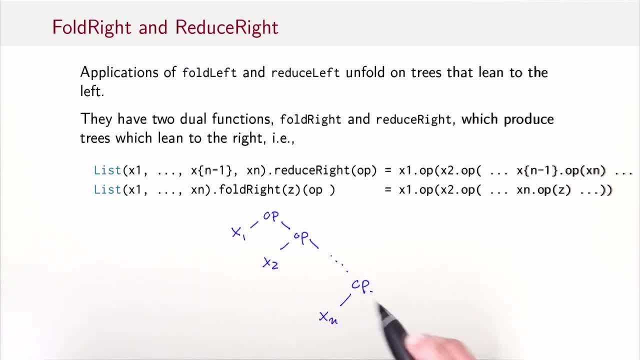 until finally we have xn up and z, so we get a right leaning tree. the spine of the tree is again the operations. the elements appear from top to bottom, x1 to xn, and the zero is on the low right corner and reduceRight is like foldRight. 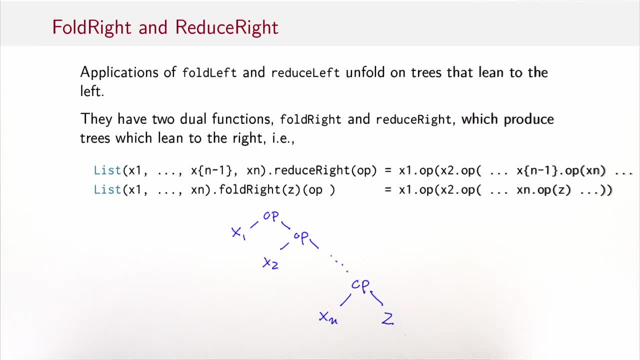 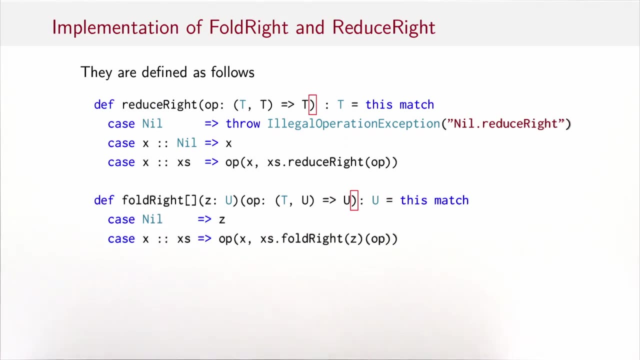 but instead of having a separate zero, it just combines the elements in the list itself, so it would look like this: so foldRight and reduceRight can also be seen as functions inside class list. let's look at foldRight first. it takes a zero and an operation. 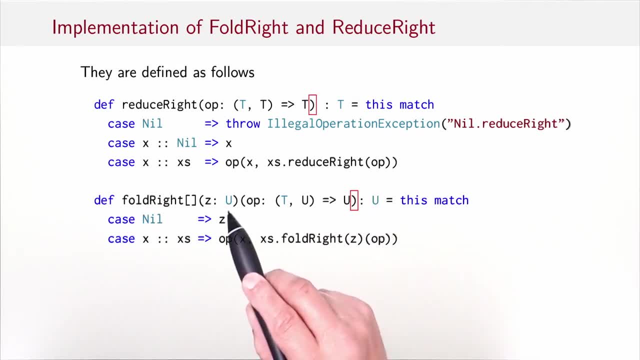 and it returns the result: type of the zero or of the operation, which is a type parameter which we didn't write here, so the u here goes in the brackets. that was a typo in the slide. so the implementation of foldRight would be: we match on the current list. 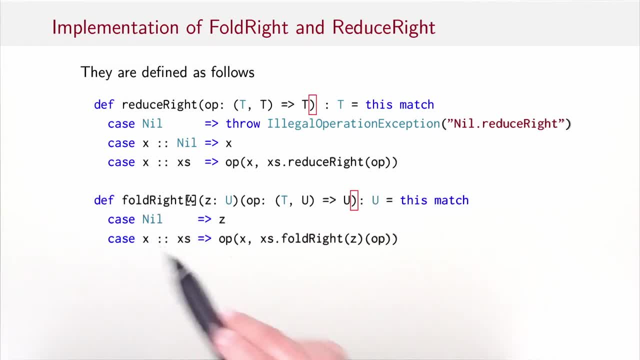 that's this: if it's nil, then we return the zero, if it's not nil, then we perform the operation with the first element of the list and a foldRight of the rest of the list with the same zero and the same operation, and reduceRight is essentially like foldRight. 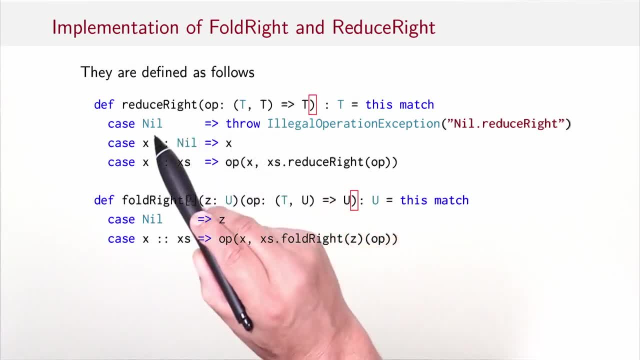 but only defined on non-empty lists, so it gives an unsupported operation exception for the empty list. if the list consists of a single element, then that element is the result if the list consists of a single element. if the list consists of more than one element, then it does the operation. 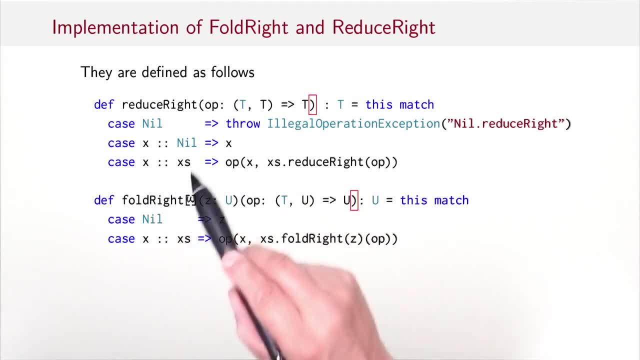 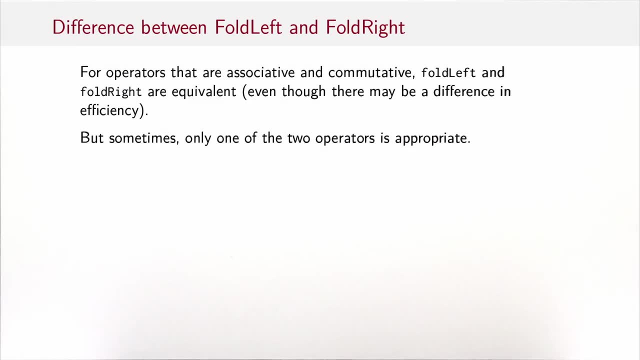 with the first element and a reduceRight of the remaining elements. so does it make a difference whether you use foldLeft or foldRight, or reduceLeft or reduceRight? well, if the operator op is associative and commutative, then foldLeft and foldRight are equivalent. 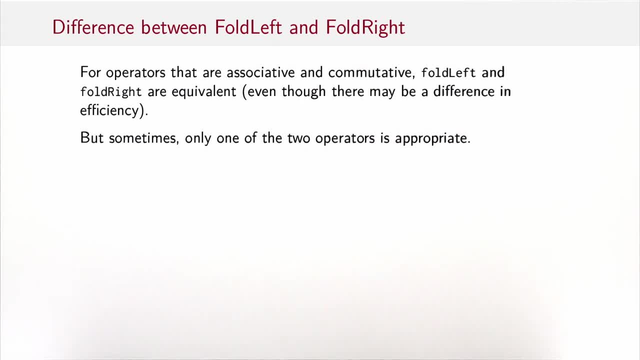 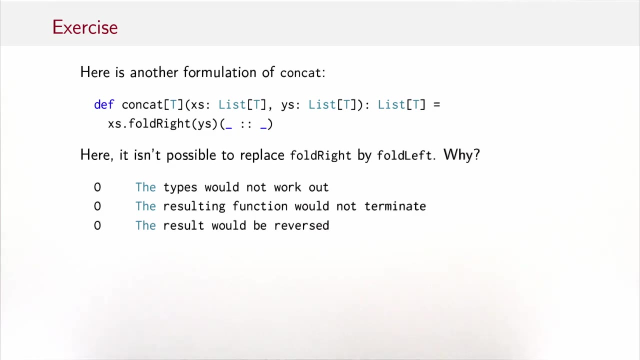 even though there might be a difference in efficiency. often foldLeft, for instance, can be implemented in a tail recursive way, whereas foldRight is not tail recursive, so it needs more stack space. but sometimes only one of the two operators is appropriate, so you can find it out yourself. 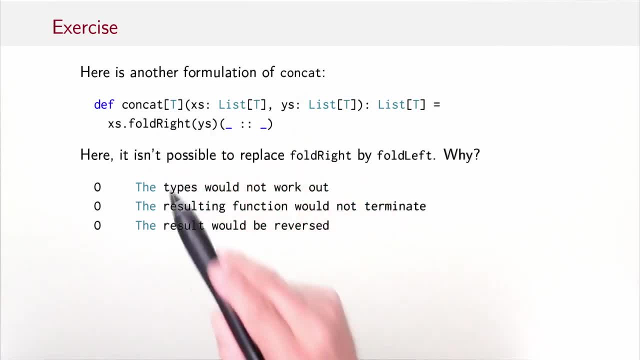 here is another formulation of concat. so we can say: concat of two lists, xs and ys, is the first list, xs, foldRight, with zero ys and the cons operation as an operation. we can visualize the operation of concat by just drawing this operation with a diagram. so we have 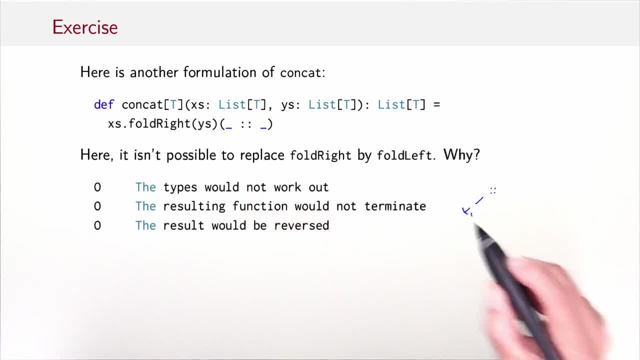 defaultRight. that would be here the cons operation as the operation. so it takes elements x1 to xn, one after another, and the zero then is the list ys. so let me just write out the list ys. what would ys look like? it is ys1 to y1. 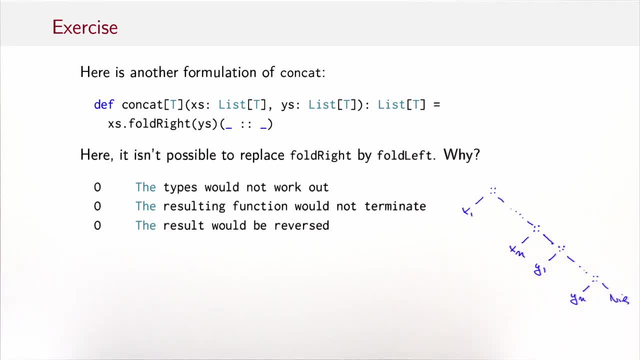 to yn and nil. so we see, indeed, this version of concat neatly aligns all the elements of x, followed by all the elements of y, followed by nil, which is exactly what we want. ok, so could we have also used foldLeft instead of foldRight for this? 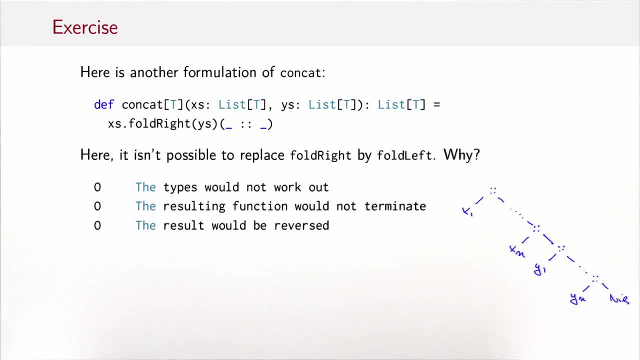 the answer is no, and the question to you is: why is it? because the types wouldn't work out or the resulting function wouldn't turn to terminate, or the result would appear in reversed order. I invite you to copy the function concat in the worksheet. verify that it works correctly. 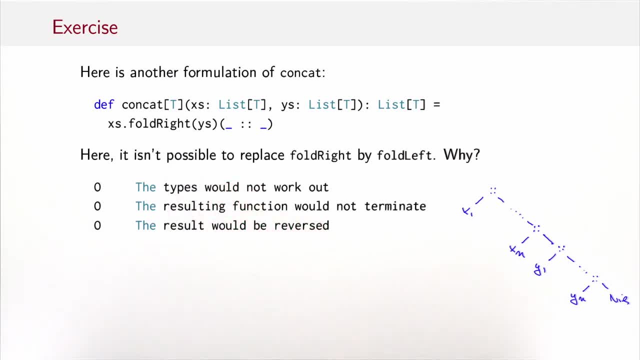 and then replace foldRight with foldLeft, what you will find is that the types would not work out. indeed, we can again visualize that if we do a foldLeft, then we would have as a zero the list x1 to xn, and then we would actually apply the same. 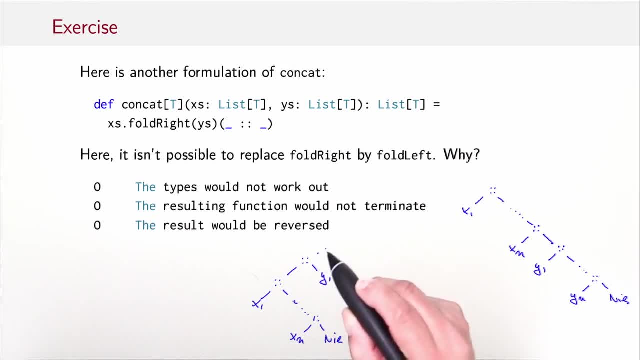 cons operation on y1 to yn. but that's not type correct, because here we are mixing a list with single elements for the y1 and yn, so the two don't have the same type and that's why it doesn't work out. so remember that some. 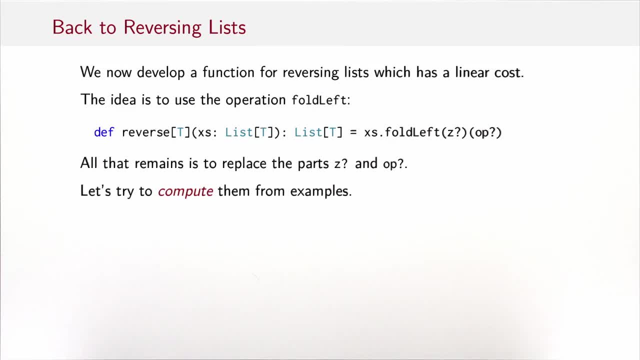 sessions back, we wrote a definition of reverse which was not very performant. it had quadratic complexity where linear is what we want to achieve. we will now fix that problem. so we develop a function for reversing lists which has a linear cost. the idea is to use the operation foldLeft. 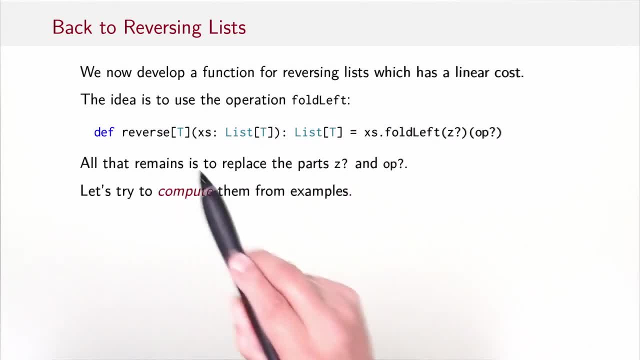 for this. so our template will look like this: the reverse function: it takes a list, returns a list, and its body is xsfoldLeft, with some zero which we have to determine and some operation which also leaves to be determined. so all we need to do is replace: 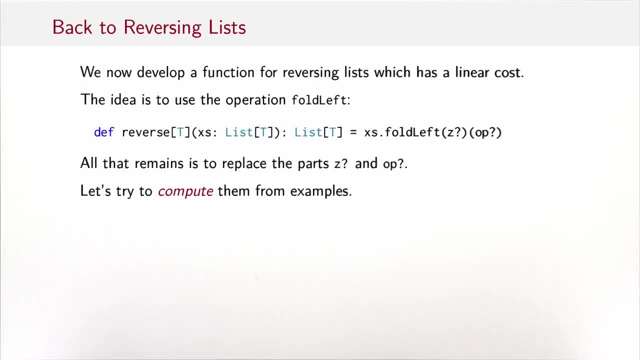 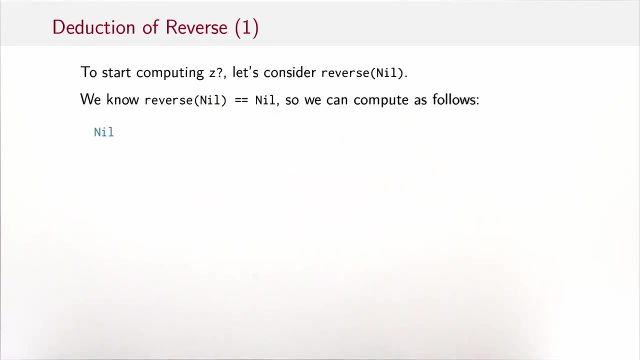 the zero question mark and the operation question mark. now we could guess what they are, but the interesting bit here is that we also can compute what they are. we can try to compute zero and operation from examples to compute z. let's consider reverse of nil. we know reverse of nil is nil. 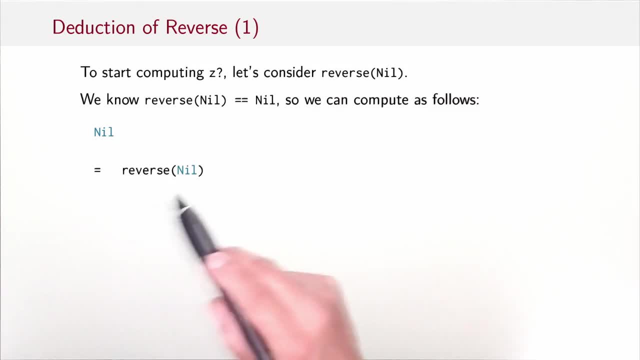 so we can compute as follows: nil is reverse of nil. now we plug in the template of reverse, so that would be nil, foldLeft, some operation, z and op, and now we plug in the definition of foldLeft where we say nil, foldLeft is z, so foldLeft of the empty list is always. 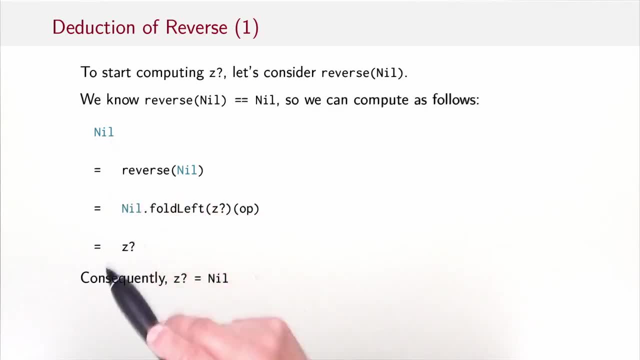 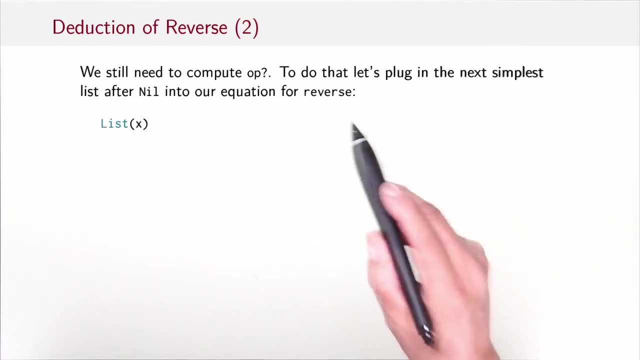 a zero, so that gives us z and consequently, because all these are equalities, z equals nil. so we still need to compute op question mark. to do that, let's plug in the next simplest list after nil into our equation for reverse. so we start with list x. 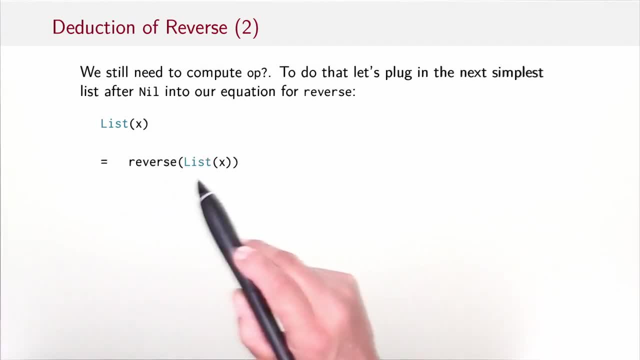 and we know that's the same as reverse of list x. reversing a singleton list gives the list itself. now we plug in our template so that would be list of x- foldLeft, nil op, and now we apply the definition of foldLeft. so on a single element, list foldLeft. 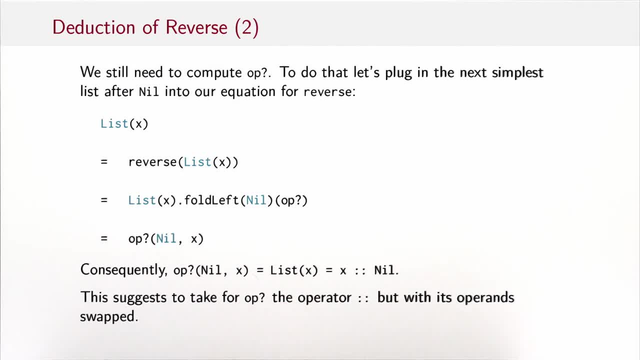 is the zero and the element with the combined with the operation. so that means operation of nil, and x is the same as list of x, and list of x is of course x, colon, nil. so that suggests we should take for the operation the cons operator, but with its operands. 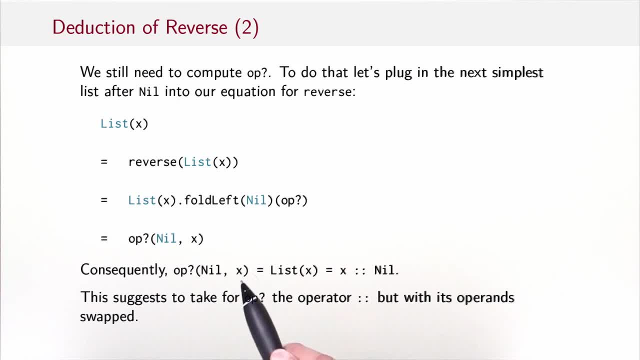 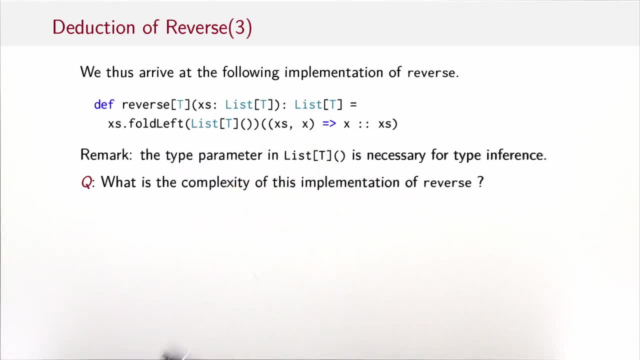 swapped. so here we have the nil on the left hand side and x on the right hand side, and here they are in the other order. so, putting everything together, we get this definition of reverse. so reverse is a fold left with the empty list and the operation that. 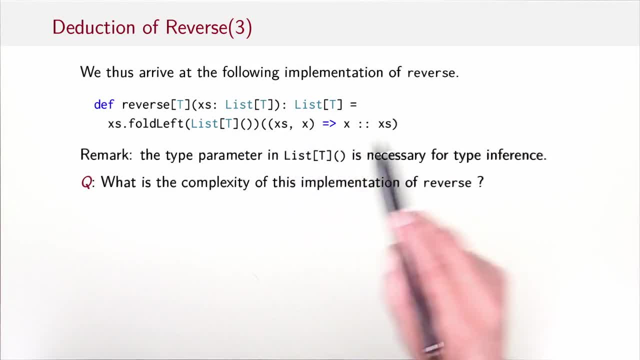 performs a cons on its operands but with the operands swapped. so it takes a list and an element and it returns the element prepended in front of the list. so there is a remark that this type parameter list of t here. that's necessary because otherwise the type inference. 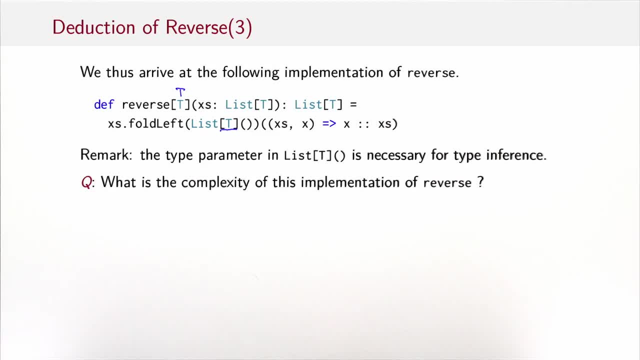 of Scala will get confused. we are working on that and maybe we can improve it in a future version, but it's not easy given the type inference algorithm that Scala applies. so it's one of the cases where you actually do have to write an actual type arguments. 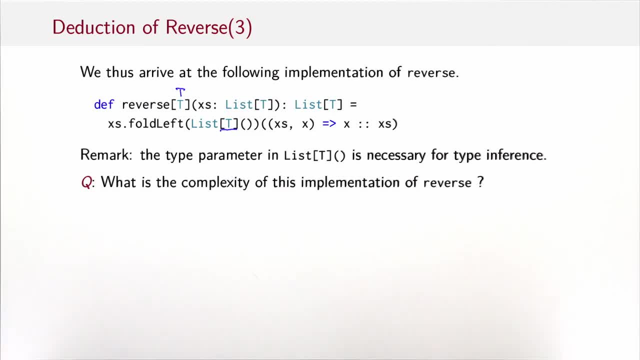 now, what's the complexity of this implementation of reverse? well, let's see. we've seen the operation tree of fold left. that's obviously linear in the length of the list x as it goes once through the list x as, and combines all elements with one operation. 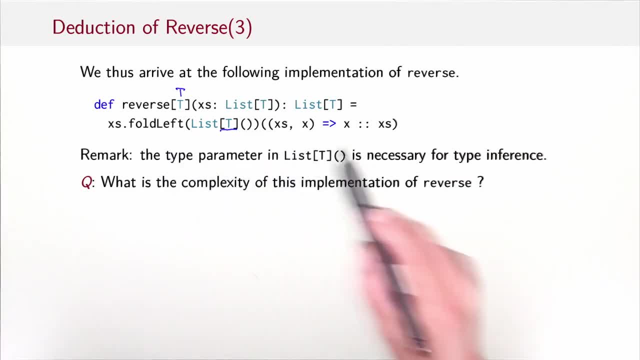 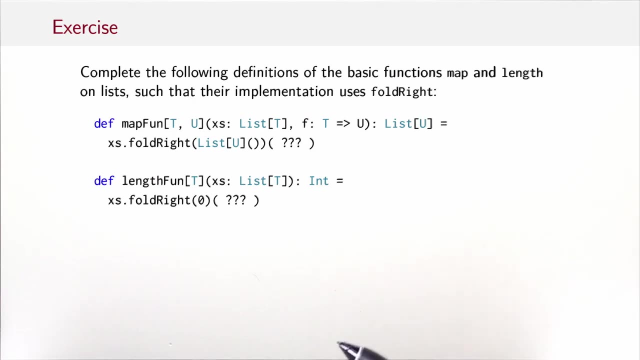 and here it's just a fold left with an operation which is constant time. so the answer is: it's still linear in the list x as linear instead of quadratic. so we have achieved our objective. so here's an exercise for you. we have two functions that you know. 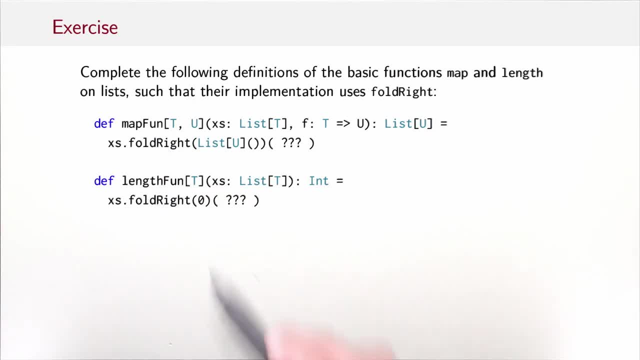 by now. that's the map function and the length function. I've just wrote them outside of list as functions like this. can you implement them in terms of fold right? so I've already given you the outline. so for the map function we would do a fold right. 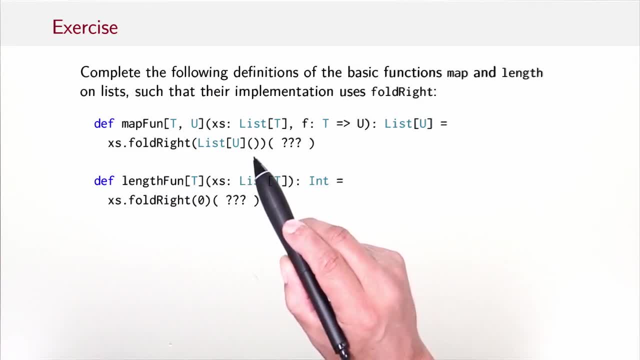 on the empty list, because map on the empty list gives the empty list and an operation that we have to fill in and the length function would give you a fold right with zero for the empty list and again an operation that you have to fill in. so let's see. 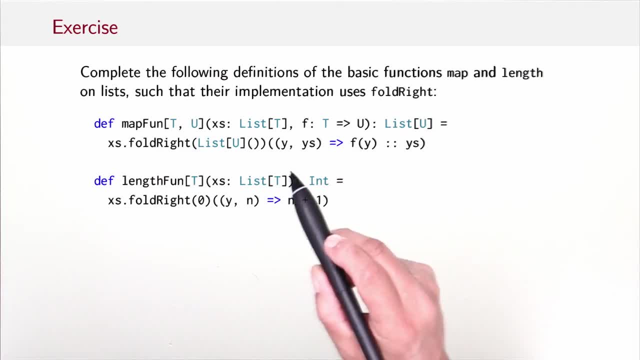 for the map function what we need to do if we have a fold right, so we get an element and the remainder of the list and we do apply the function and we do a cons with the remainder of the list if we show that together with fold right in a diagram. 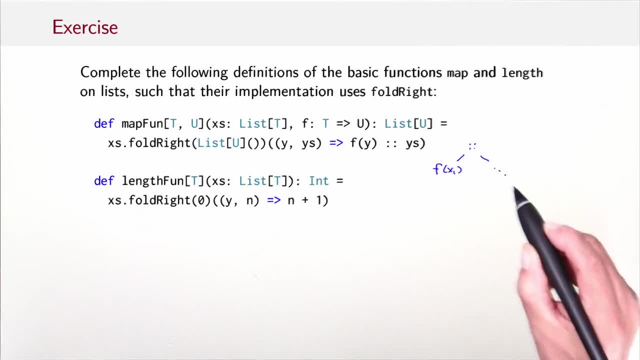 it would look like this. so it would be f f zero, which is exactly what you would expect for the map function. so what about the length function? the length function can also be expressed with fold. right here, the operation we need to use is the operation that takes a list element. 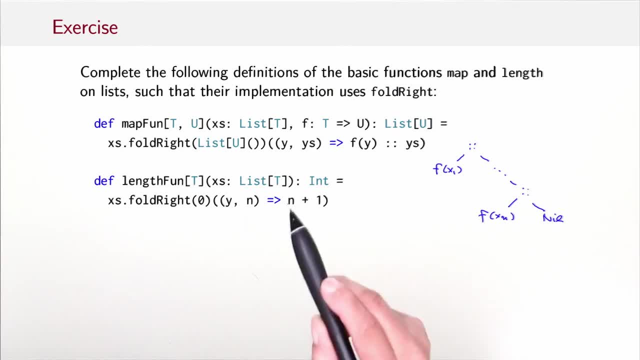 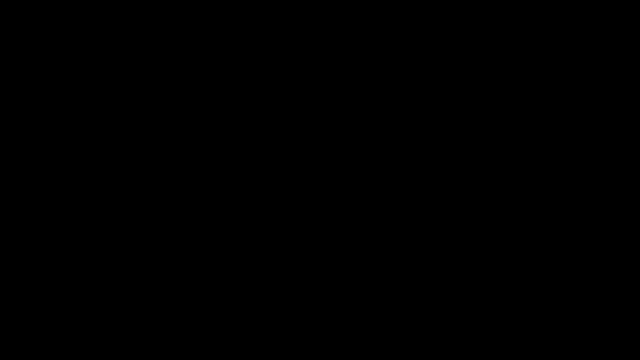 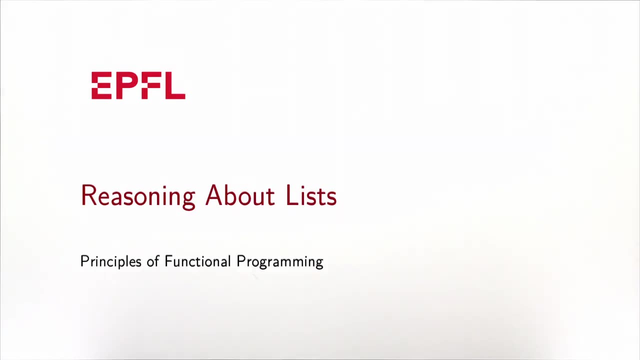 and a length that was computed so far on the right and just returns the length plus one. so the element and the contents of the element are ignored. here in the last session we've seen that our function definitions give us certain equations that can be used to compute. 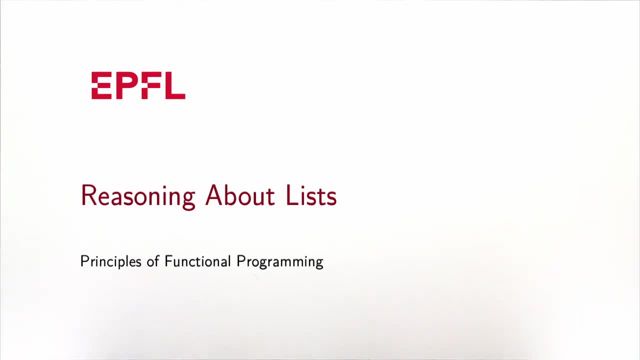 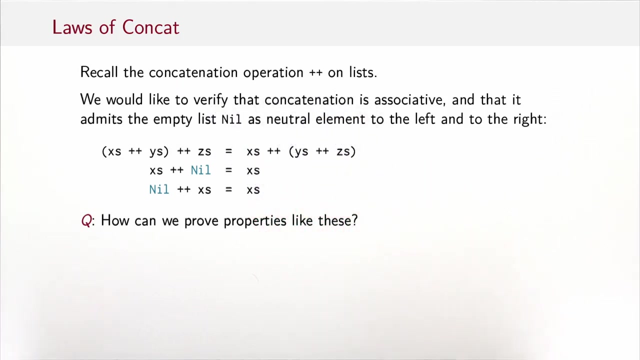 parts of an expression. in this session we go on in the same direction by showing that the same equations also allow us to reason about the correctness of our operations. recall the concatenation operation plus plus on lists. what would it mean to say plus plus is correct. correct in what sense? 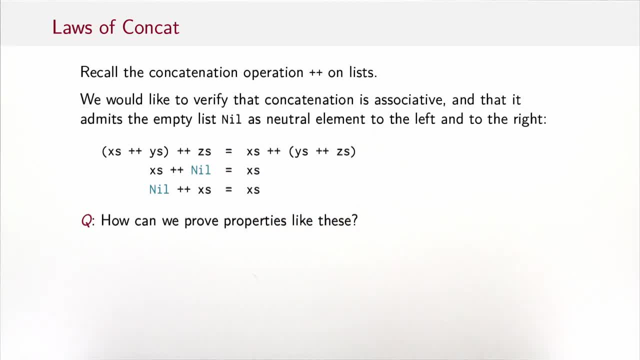 so one thing we could do is verify that concatenation satisfies certain laws, for instance that it's associative and that it admits the empty list nil as neutral element to the left and to the right. postulate these three laws that we say xs plus ys in parenthesis on the left. 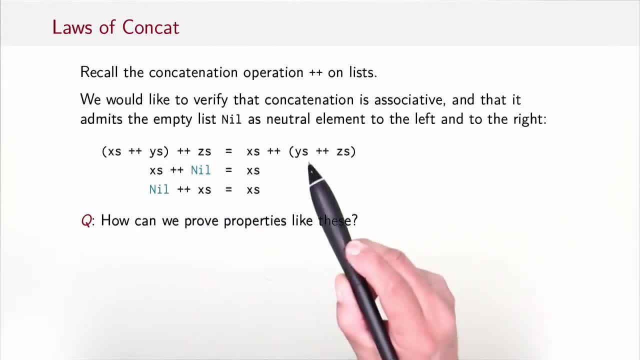 followed by plus zs is the same thing as xs plus ys plus zs. xs plus plus nil is xs. nil plus plus xs is xs. ok, so now that we've established the properties, how can we prove them? and the answer is by using structural induction on lists. so what is structural induction? 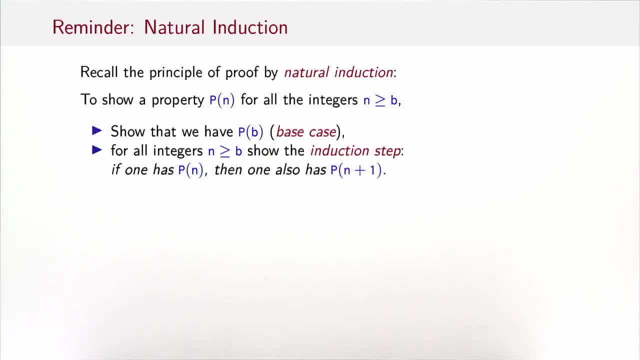 well, let's take a step back and first have a look at natural induction. probably most of you know that already. to show a property, p of n, for all integers, n greater or equal one base, case b, we show that p of b holds and for all integers. 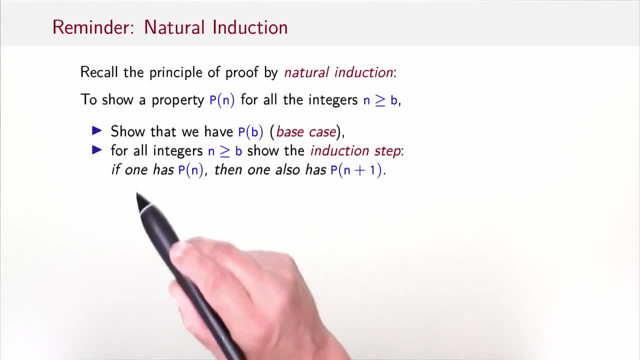 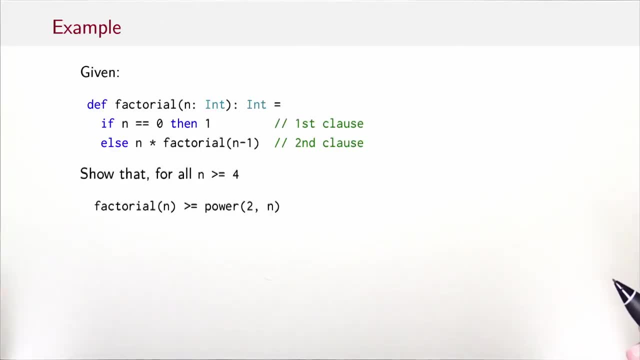 n greater than b, we show the induction step. if one has p of n, then one also has p of n plus one. natural induction can be used also in programming, for instance in this example. here we have a factorial function that you know and we want to show that for all n. 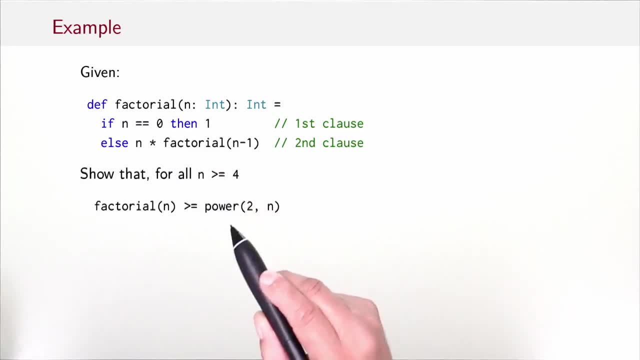 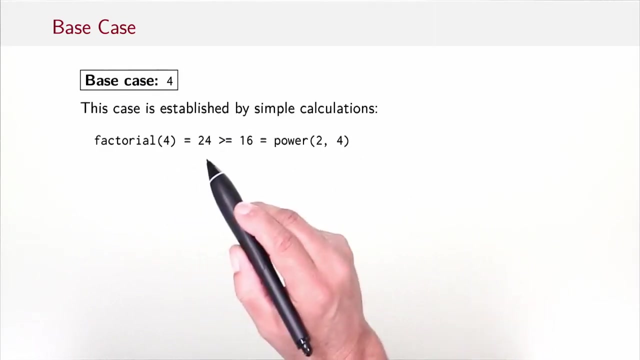 greater or equal four. factorial of n is greater or equal power of two to the nth. so that's the implementation of two to the nth. so to prove that, we start with the base case, which is four, and that case is established by simple calculation. factorial of four is twenty four. 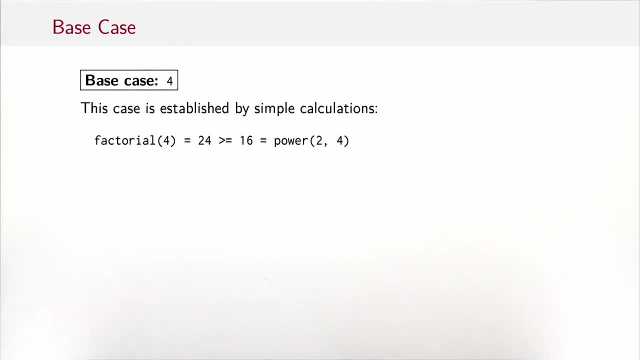 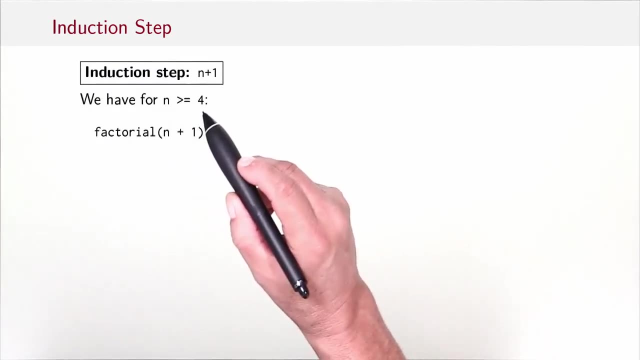 two to the fourth is sixteen. so twenty four is greater or equal sixteen and we're done for the induction step. we proceed as follows: we have for n greater or equal four that factorial n plus one is greater or equal n plus one times factorial of n, and that's simply by the second clause. 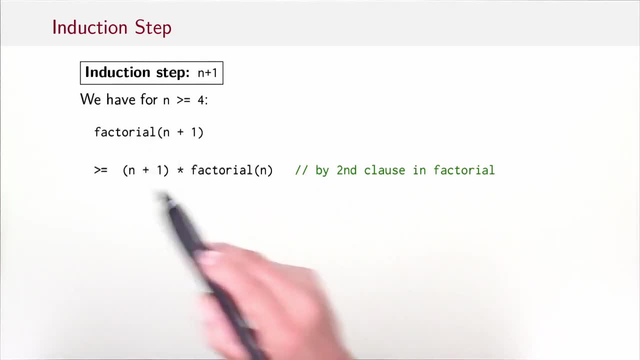 of factorial. that's an equality. factorial n plus one. is that? so if we have equality here, we can also assume greater or equal, and that's in turn greater than two times factorial of n. simply by calculation, n plus one is at least five. so by the induction hypothesis, 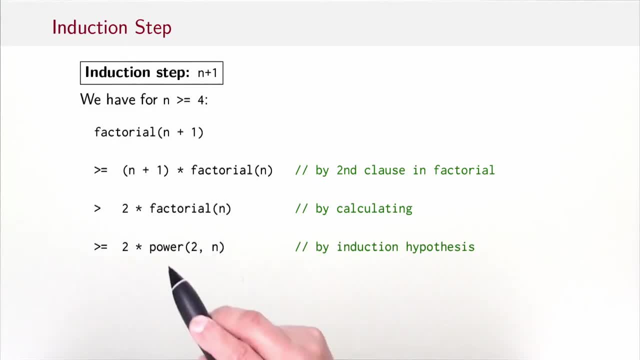 we know that for n, factorial of n is greater or equal power two to the nth, and that by the definition of power is power of two to the n plus first. so we have again a chain of greater or greater or equals that starts with factorial n plus one. 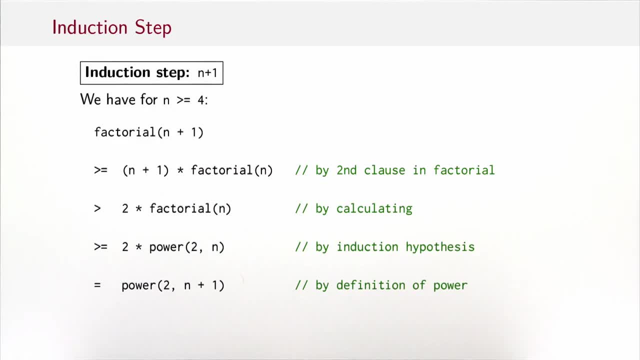 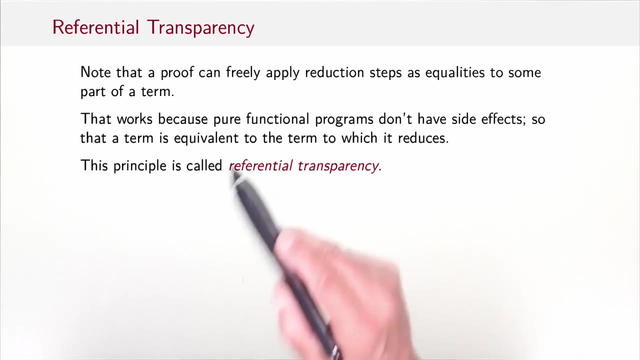 and ends in two, to the n plus first and in the sequence. we used here the induction hypothesis, which says we are allowed to assume, if we want to prove the case for n plus one, that the case for n already holds. in these proofs we have freely applied reduction steps as 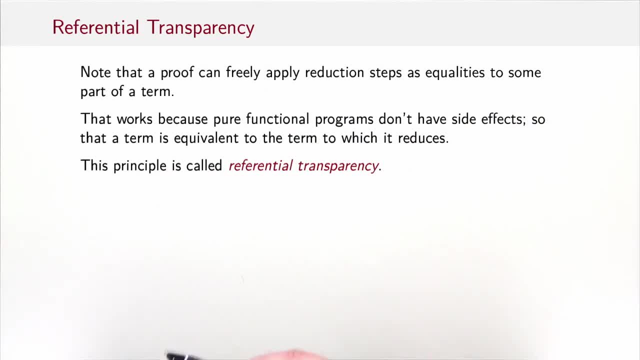 equalities to some part of a term. that means we have replaced the left hand side of a function with its right hand side, or vice versa. that works, because pure function programs don't have side effects. so a term is equivalent to the term to which it reduces. 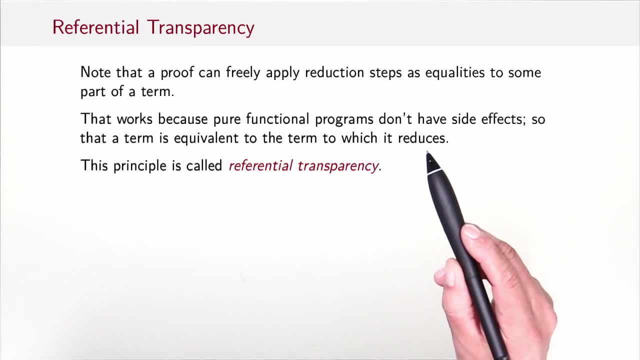 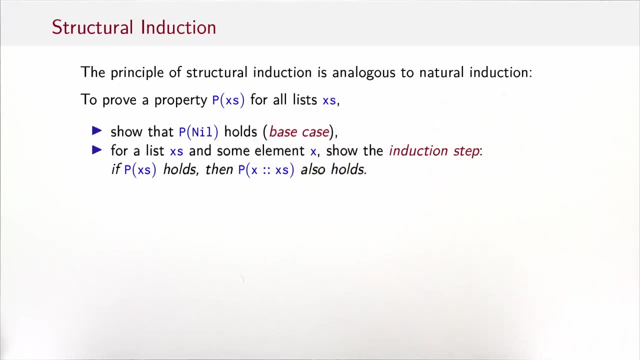 and a function left hand side is equivalent to its right hand side. that principle is called referential transparency and it's really the basis that makes everything in this kind of proof system work. so the principle of structural induction is analogous to natural induction. it goes like this: 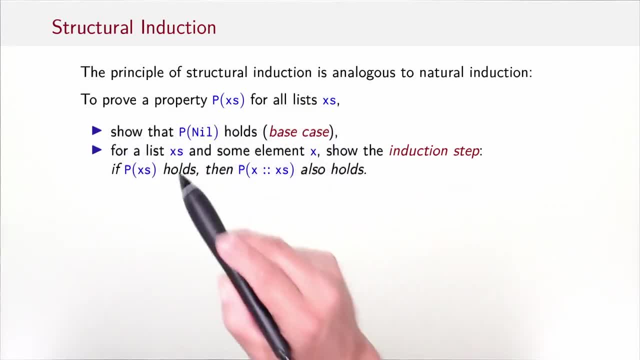 to prove a property, p for all lists show that p holds. that's the base case. and for a list, x and some element x show the induction step. the induction step to show is: if p holds, then p also holds. so let's apply this principle in the proof of. 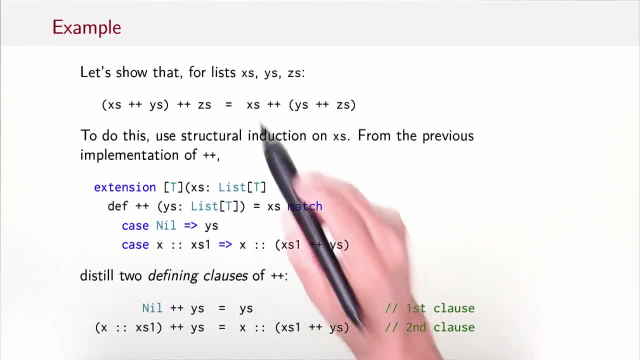 associativity for concat. so we want to show that for all lists x, y and z, this equation holds. to do this we want to use structural induction on x, the left most list. so we saw the previous implementation of plus plus that you saw here and we can distill from this two defining. 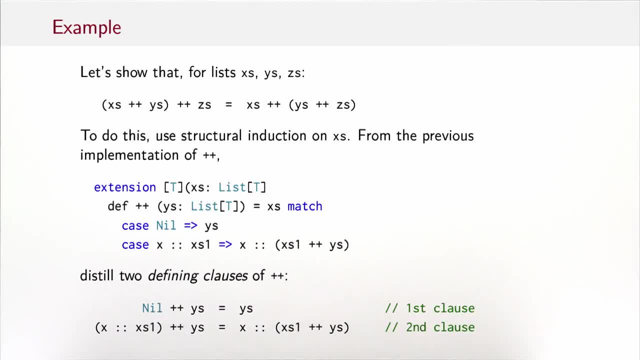 clauses of plus plus that state how plus plus works on its left operand. so we know that nil plus plus ys is ys and that x followed by xs1 plus plus ys is x followed by xs1 plus plus ys. so we read that of the second clause here. 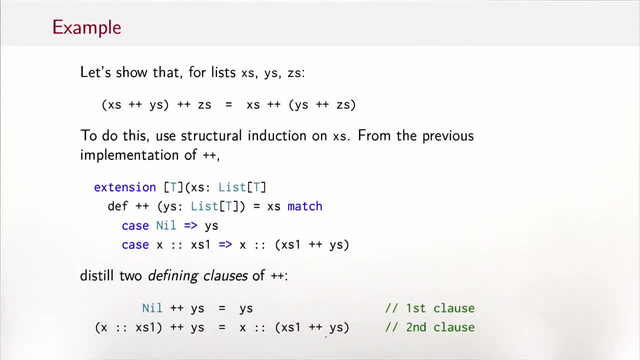 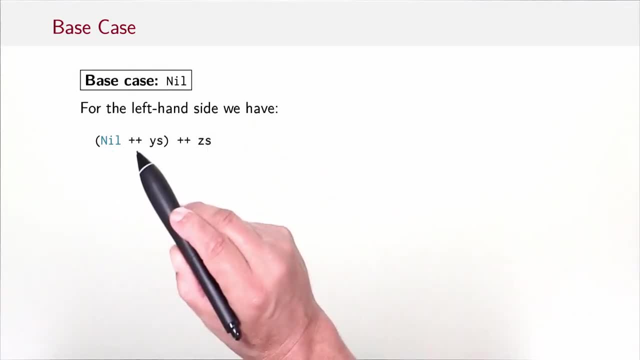 and we are going to use these two clauses in turn for our proof. so let's look at the base case for the left hand side. we have nil plus plus ys plus plus zs by the first clause of plus plus nil plus plus ys is ys, so that's ys plus plus zs. 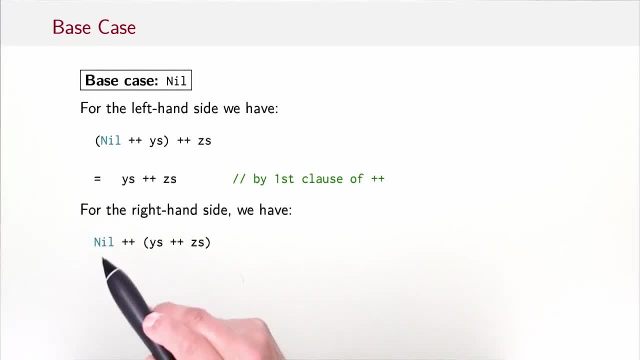 and for the right hand side we have nil plus plus ys plus plus zs, again by the first clause of plus plus, that's ys plus plus zs. so the two are the same and that in turn proves that This term here is the same as that term here. 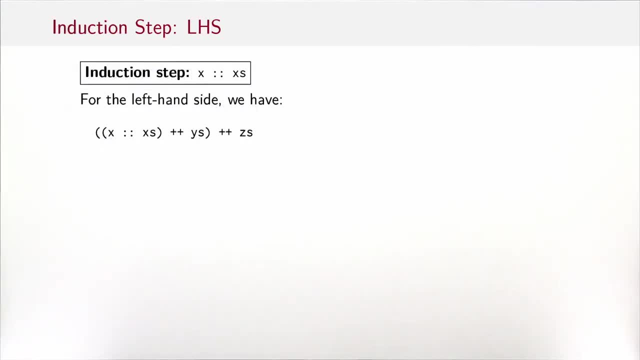 The case is therefore established. So now let's do the induction step, where our left-hand list is assumed to be of the form x cons xs. So the left-hand side now looks like this: x cons xs plus plus ys plus plus that s. 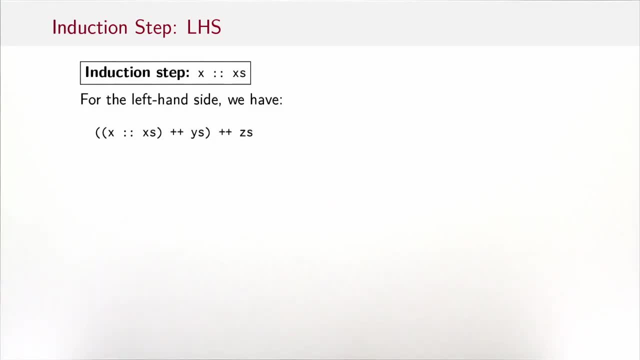 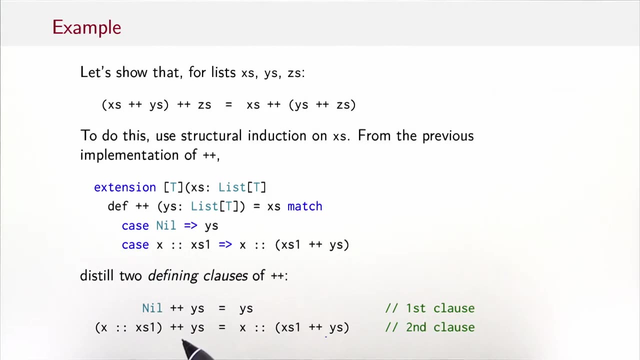 Let's simplify that. To do that, we have to look at the second clause of plus plus. So the second clause is here. It says essentially that if I have a cons and a plus plus, I can move the parents from the left to the right. 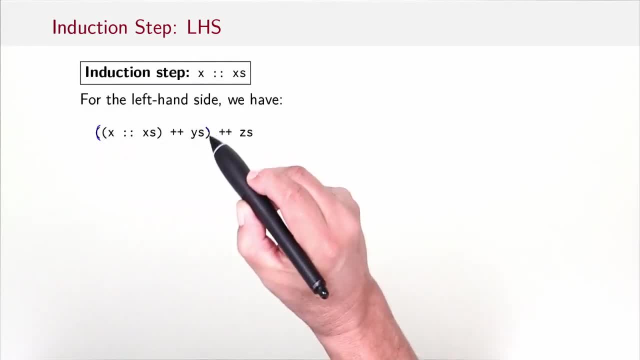 So that's the case here. We have the parents here. Let's move them to the right. That gives this term here. So we now have x colon. xs now associates with ys plus plus that s. Now we can simplify that further using the same trick. 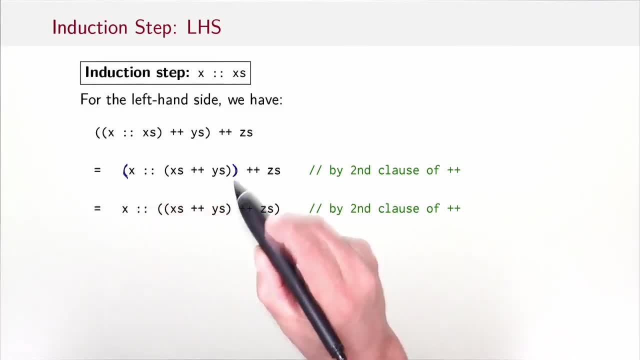 So we now move these parents to the right. So that gives us x, and then xs plus plus ys, together with that s. Now we can apply the induction hypothesis. We have x plus plus ys plus plus that s, So we can assume that one is associative. 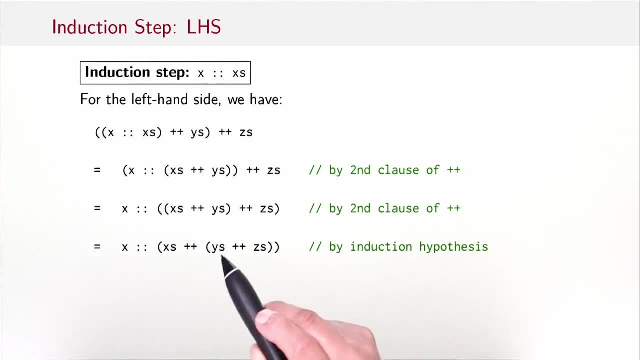 So by the induction hypothesis we get xs plus plus and ys and zs then in parenthesis together, And that's as far as the left-hand side goes. So let's stick with that and concentrate on the right-hand side. So for the right-hand side we have 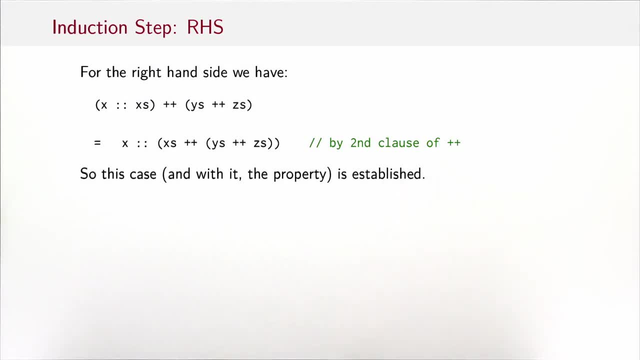 this. By the second clause of plus plus, we can move the parents here from the left to the right, so that gives x, colon, colon, xs plus plus ys plus plus zs, and that's actually exactly the same as what we have seen here before. So the equality is established. we have the left hand side, which 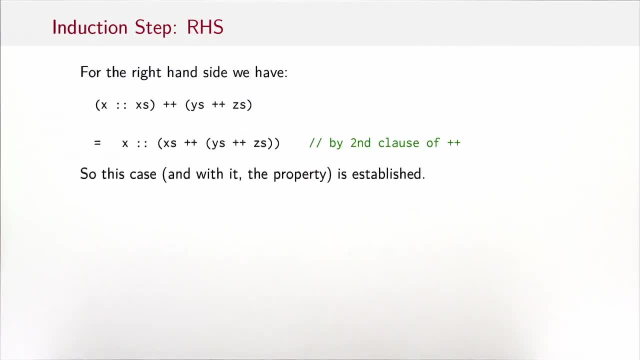 is equal to this. and then that's where we picked up. and that's again equal to the right hand side going up. So we have a series of equalities which established the inductive case. So here's an exercise for you. Show by induction on xs that xs plus plus nil is xs, so that nil. 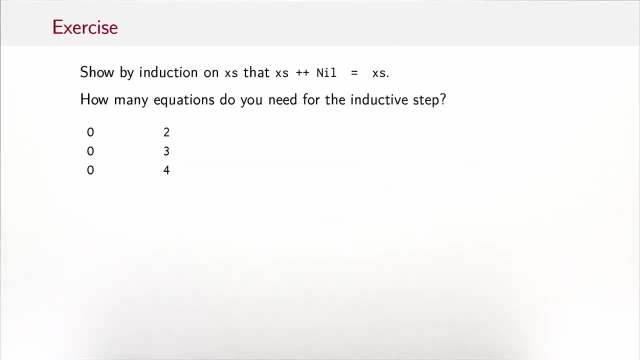 is a neutral element on the right. How many equations do you need for the inductive step? Two, three or four? Well, let's see. the inductive step would look like this, so it would be x, followed by xs plus plus nil, so by the second clause of plus plus. that's the same as x. 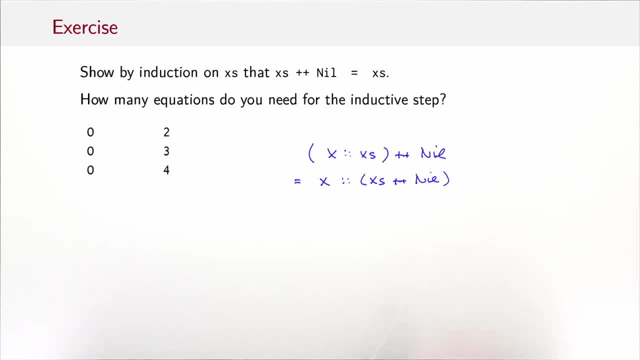 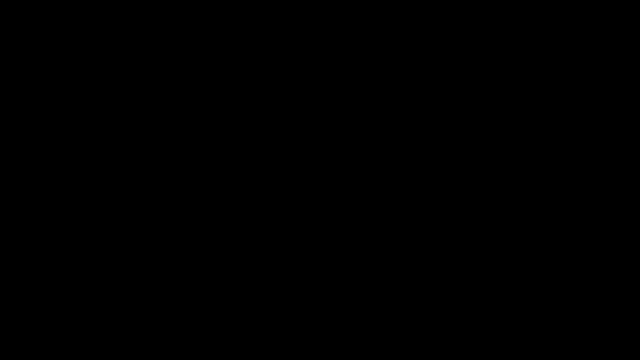 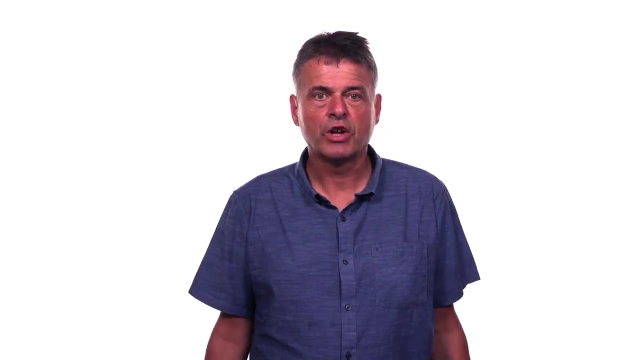 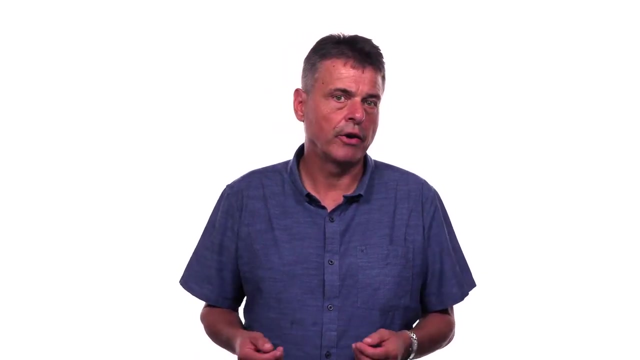 xs plus plus nil and by the induction hypothesis that's the same as x colon, colon xs. So two is correct. we need two equations to get there, Ralph. After our deep dive into lists, this week we'll explore other data structures: vectors, maps, ranges, arrays and more. They differ from lists both in their functionality. 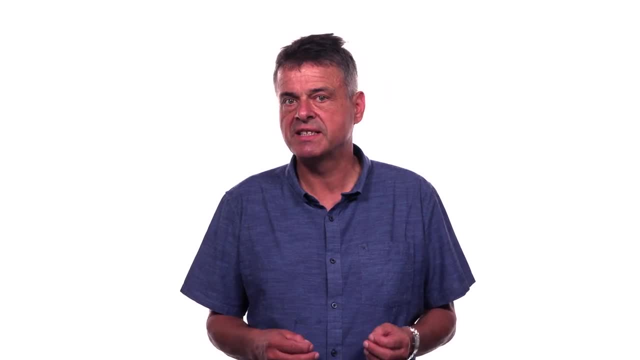 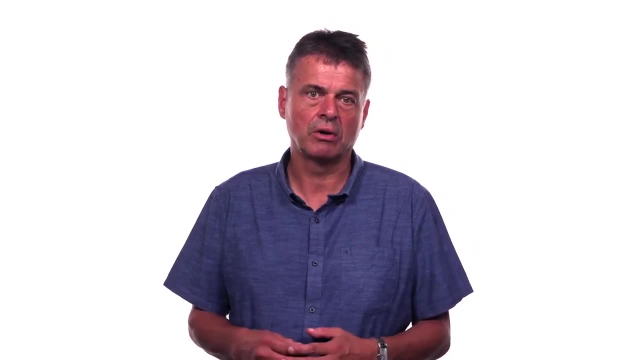 and in their performance. One thing will stay the same, however: all the collections we're going to study in depth are going to be immutable. No mutations allowed. we're going to start this session by looking at different kinds of求 is some of the functions that are involved, But those 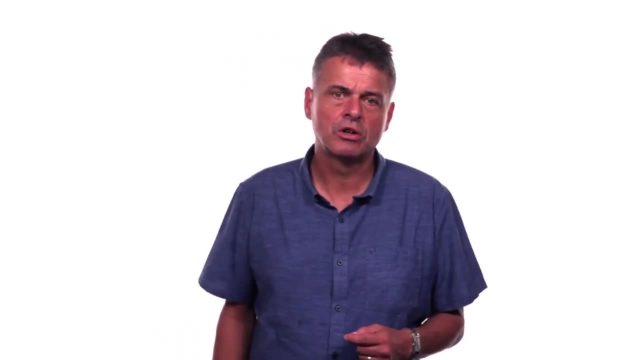 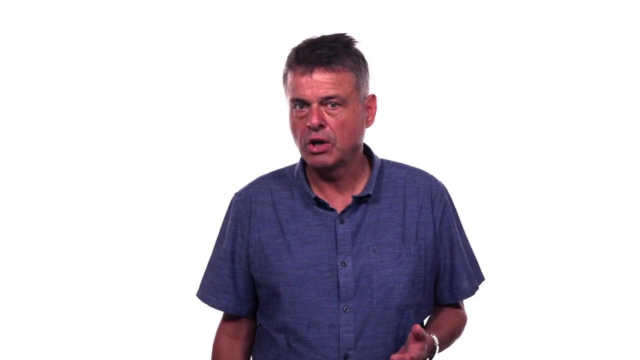 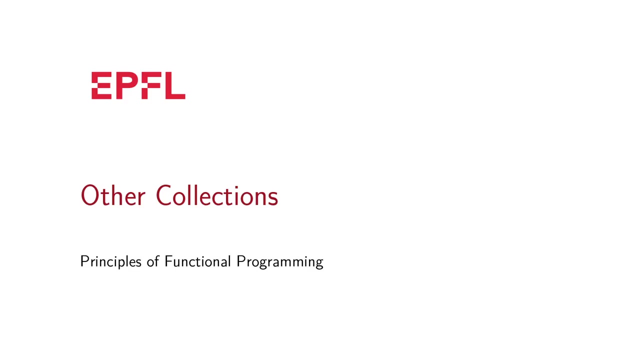 of sequences. The second important topic of this week are SCADA's powerful and flexible four comprehensions for querying data. You'll learn how to use this construct to solve some non-trivial combinatorial search problems. In this session we are going to look at some other sequence collections beyond lists. 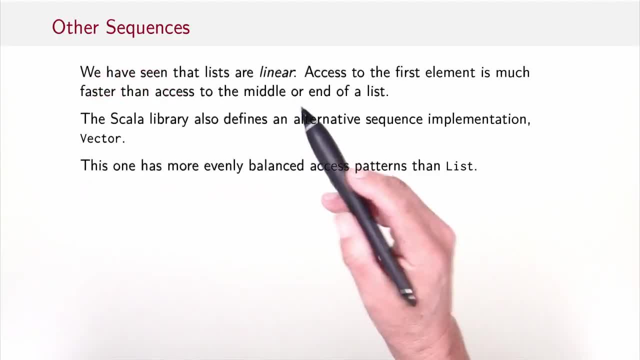 We've seen that lists are linear. that means access to the first element is much faster than access to the middle or end of a list. The SCADA library also defines an alternative sequence implementation, which is called vector. This one has a more evenly balanced access pattern. 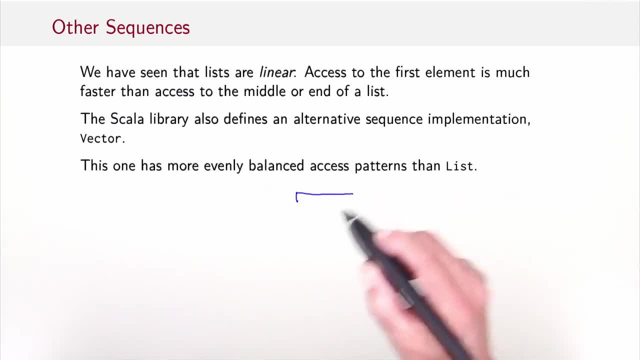 than list. The idea with a vector is that it's essentially a tree with a very high branch out factor. So you have essentially here, if the vector is small, up to 32 elements, then it's just an array. If the vector grows beyond 32 elements, then it becomes an array of. 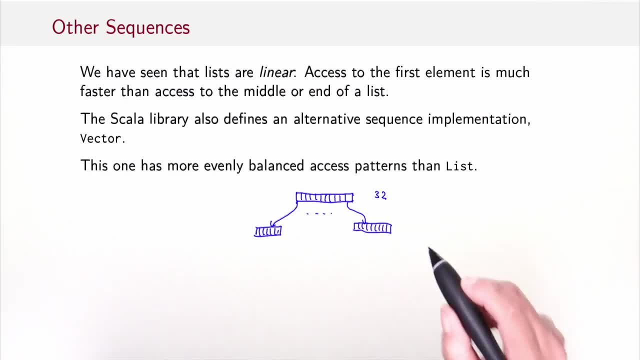 arrays, each of which has 32 elements. So we have 32 times 32 equals 1024 elements, And if the vector grows beyond that, then each of the sub-arrays will again spawn 32 children of 32 elements each, and so on. 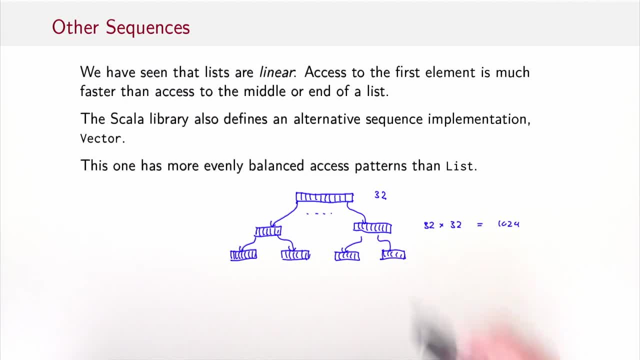 So that one gives now 32 times 1024 elements and so on. The vector could have a maximum of 5 levels, which would give you 2 to the 5 times 5.. So that's 2 to the 25th elements, That's the. 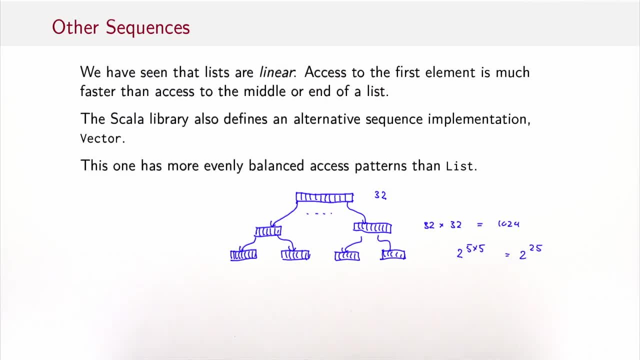 maximum size of a vector. Now, if you have a structure like that, then let's see what would happen if you have to change the structure. For example, if you have a structure like this: a single element functionally, without actually modifying the vector, creating a new vector. 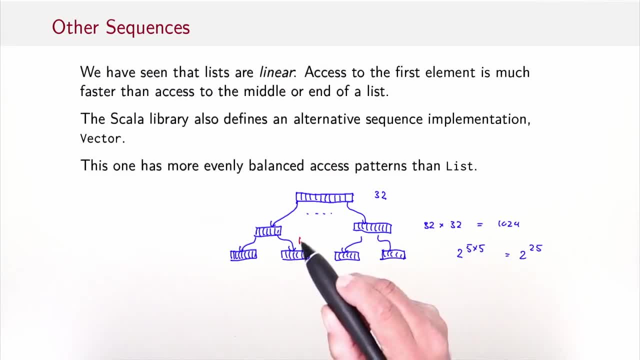 So let's say you change an element in this subarray here. What you would need to do is essentially create a new array of 32 elements which contains the changed element. Let's say, this one is this one here, So that's the one you changed, And then its parents. 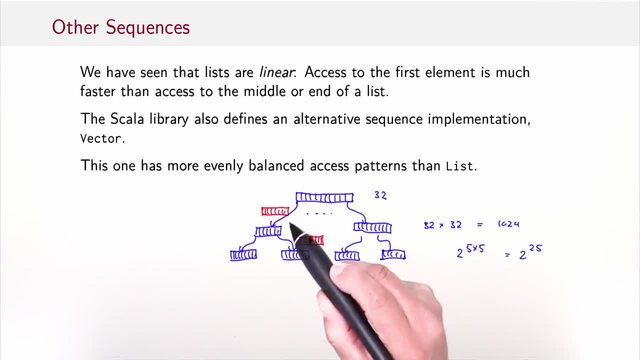 need to change as well, So that one would go here and here and to all the other ones And then finally the root has to change as well. So it's not free to change a single element functionally. You have to create, in this case with a depth 3. 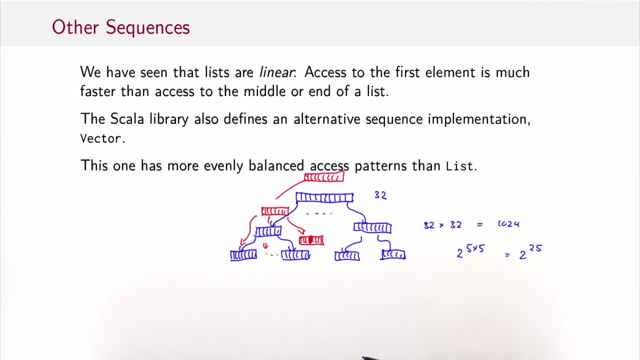 arrays. So in general you have to modify as many arrays as is the depth of your tree. But the depth of your tree is very shallow. Maximum is 5.. But it's still much, much better than having to copy an array of 1,000 or 32,000 or 2 to the 25th element, scaling. 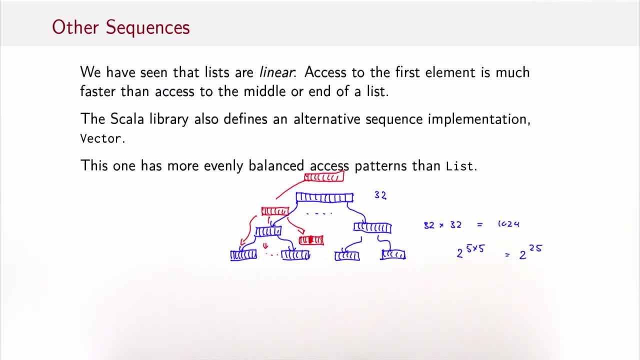 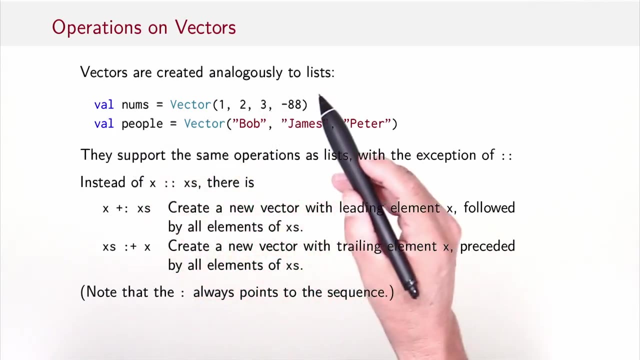 So it's essentially: what you have here is a compromise to have reasonably fast access times and reasonably fast update times in all situations. Now, how can you use vectors? They are created analogously to lists, only you write vector instead of list. So here you define two vectors: a vector of numbers and a vector of people. 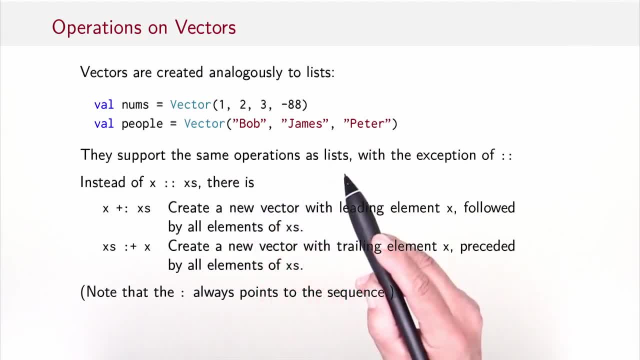 Vector support by and large the same operations as lists, with the exception of cons. So there's no cons, but there are two operations: that add an element to the left of the vector or add an element to the right. Since vectors are symmetric, there's no bonus anymore to only add elements. 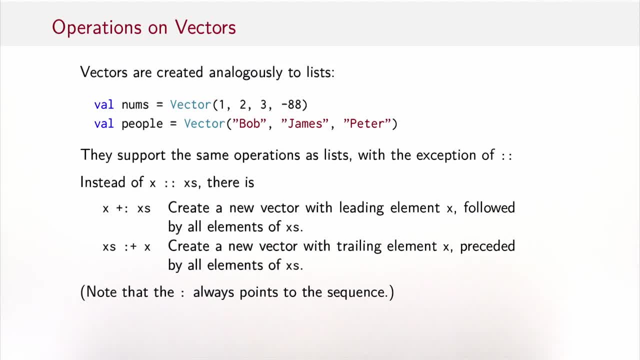 to the left. Adding them on the right is just as efficient as adding them on the left. So note here as a reminder: the colon always points to the sequence. So x plus colon xs means add a single element to the left to the sequence xs and xs. colon plus x means the opposite. The sequence goes left. 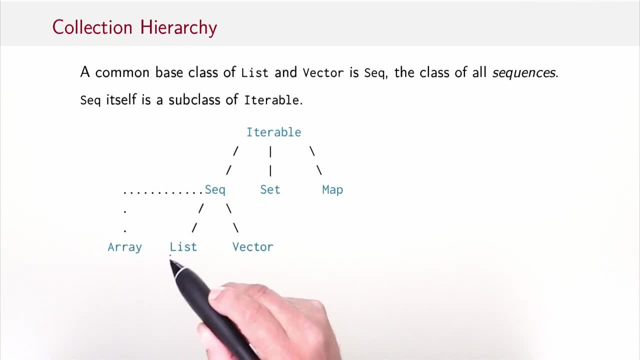 and the element goes right. So we've seen list and we've seen vector, and those two are in fact instances of a larger class hierarchy of collections. in Scala The common super trait of list and vector is called seek for sequence, And that is again not the most general one. So that is again an instance of an 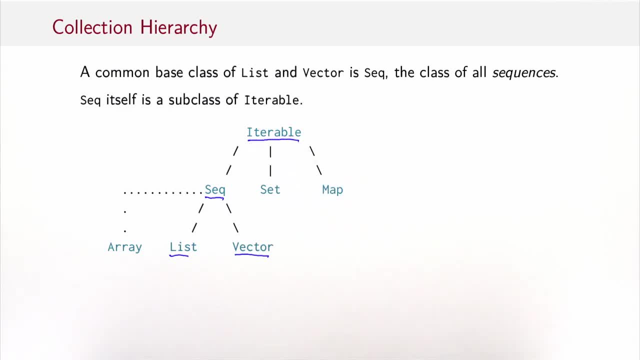 even more general trait, called iterable, And iterable has other sub-traits, namely set and map, that we are going to see in the sessions that will come. You might ask: what about array? Is that not a collection? Yes, you can see it as a collection, but since it's defined in Java, it can't. 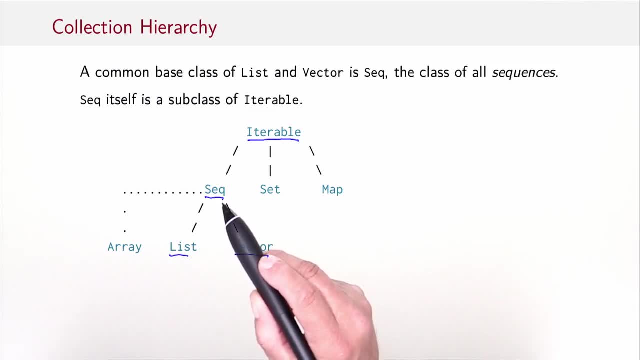 be a direct sub-trait of sequence, because sequence is defined in Scala. What happens instead is that array is a separate class, but there are automatic conversions that upcast array to sequence and that also give array again all the operations that you find in sequence. So arrays and also strings. 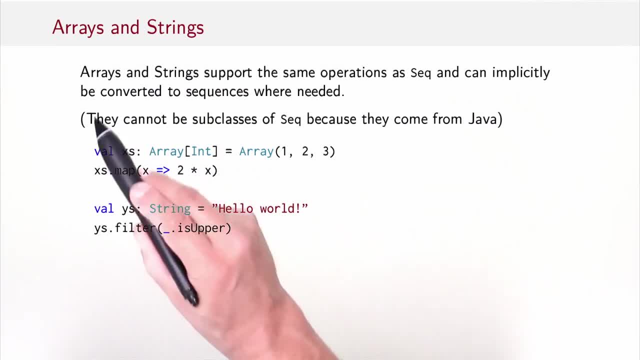 support the same operation as seek and can implicitly be converted to sequences where needed. So, for instance, you can write: xs equals array one, two, three, and then you can use a map on an array. or you can write val- ys equals a string and you can use a filter on the string. 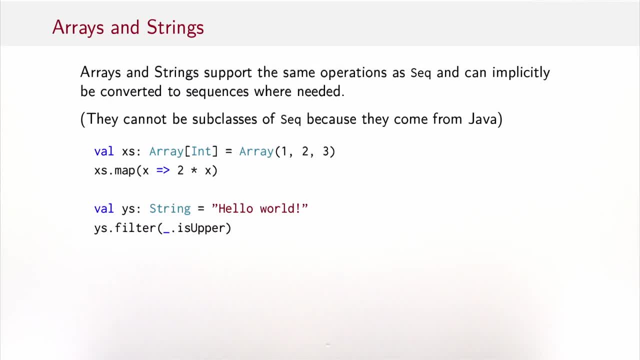 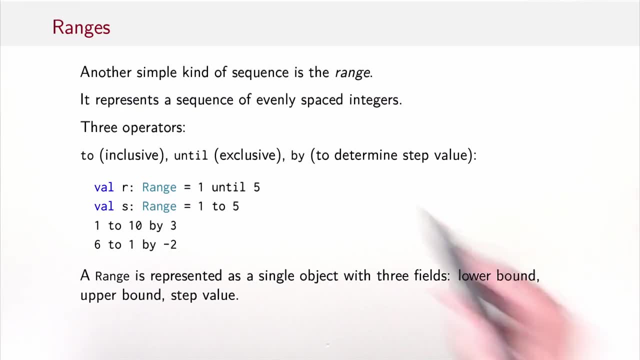 This filter here would pick all the characters which are in uppercase. Arrays and vectors are not the only kind of sequences in the Scala collection library. Another important one is the range. That's a very simple kind of sequence of integers. only It represents a sequence of evenly spaced integers. It has three. 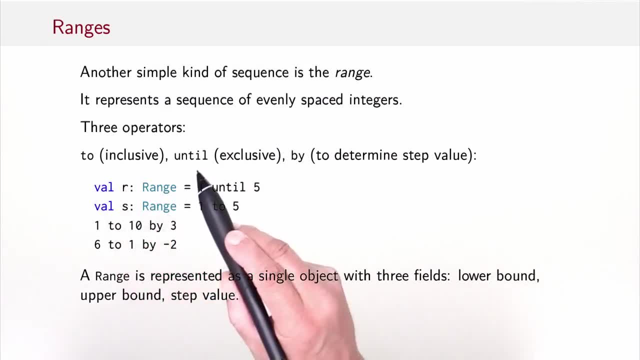 operations to build ranges to until and by. So one until five would give you the range consisting of the numbers one, two, three, four, So the five is not included. Whereas one to five would give you the same numbers with the five, So two is inclusive. and 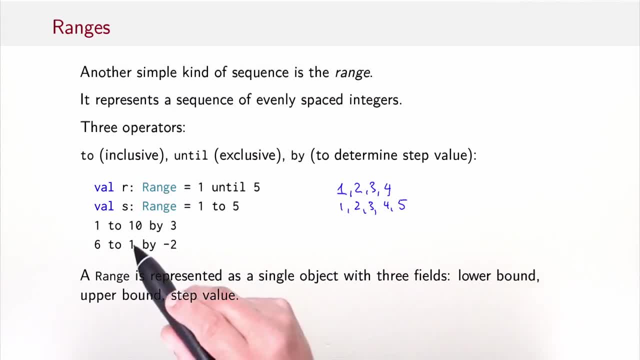 until is exclusive. And then you can also vary the step of the range using the by clause. So one to ten by three would give you the sequence one, four, seven, ten, And six to one by minus one would give you six, four. 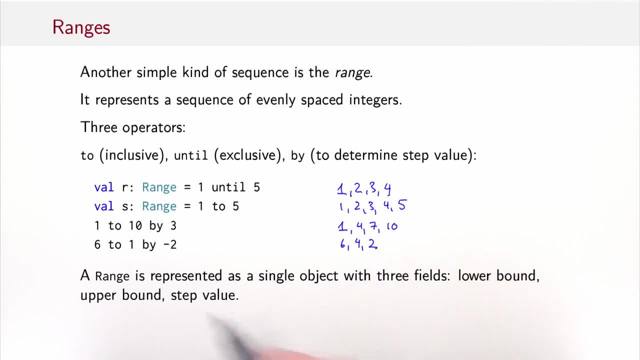 two, and the zero would no longer be included because it's already smaller than the end one. Ranges have a particularly compact representation. A range is represented as a single object with just the three fields: the lower bound, the upper bound and the step value. Here are some more operations that work on all. 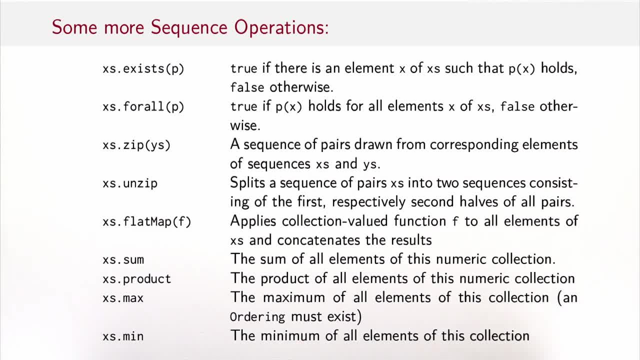 sequences, on vectors, on lists, on ranges. So you can ask whether there is an element in the sequence that satisfies a predicate p, that is called xs, exists p, And dually you can ask whether all elements in the sequence satisfy predicate p. That's done with a for all. 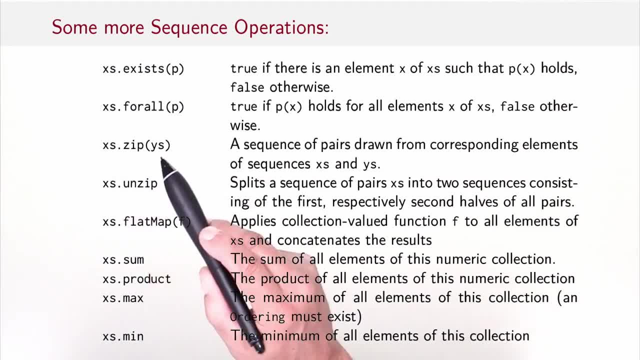 You can have a zip. A zip takes two sequences and it forms a sequence of pairs drawn from corresponding elements of sequences xs and ys. If one of them is longer than the other, then it's truncated to make them fit. So, for instance, 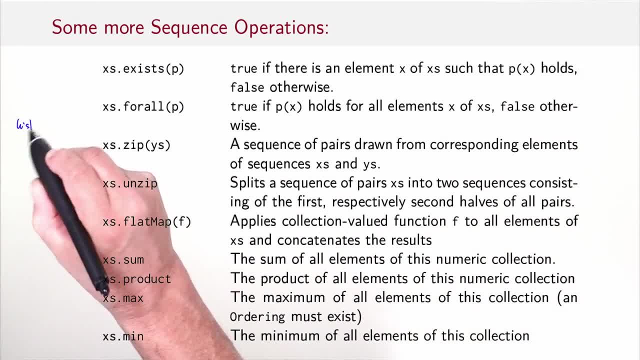 if you had, let's say, the list one, two, three. zip vector a, b. you can zip sequences of different type and the result will always be the same type as the first sequence. So that would give the list of pairs, namely one and a and two and. 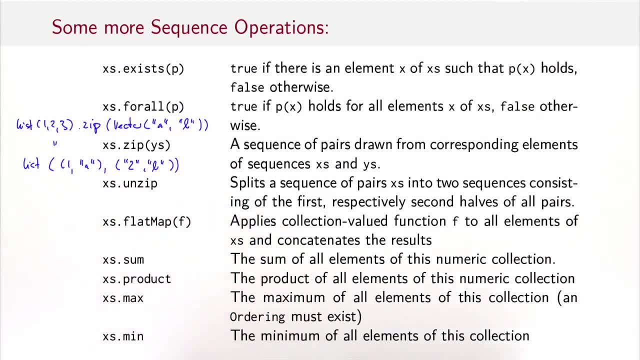 b. Unzip is the opposite of zip, So it takes a list of pairs and gives you two lists: one list consisting of the first half of the pair and the second list consisting of the second half of the pair. Flat map is an important function. It's a little bit like map, but it takes a. 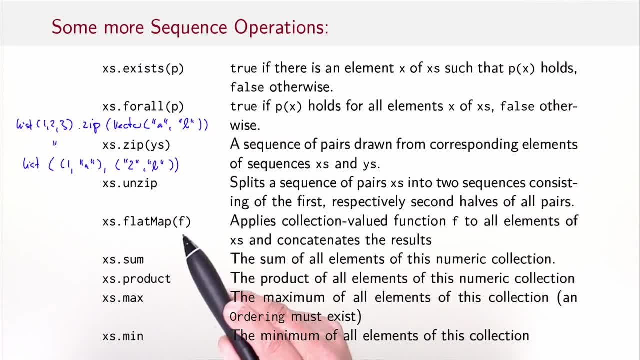 function that returns itself a collection. And what it will do is it will apply f to each element and then concatenate all the results. It will concatenate all the collection results to give a single sequence, Sum and product form: the sum and product of a sequence of numbers Maximum. 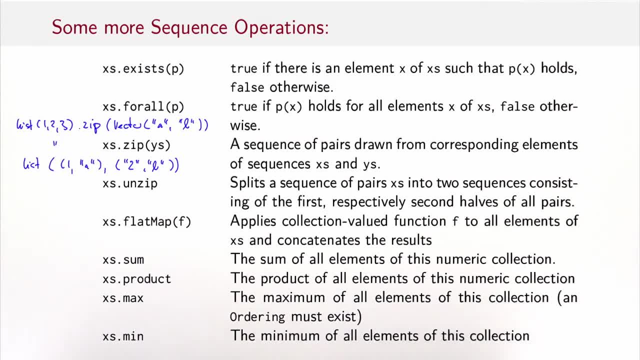 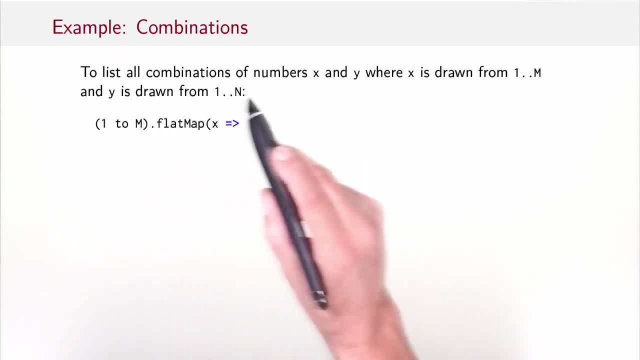 gives you the maximum of all elements of the sequence and minimum the minimum. Let's do an example that uses some of the operations that we discussed To list all combinations of numbers x and y, where x is drawn from one to n and y is drawn from one to n. What would we do? Well, we start with. 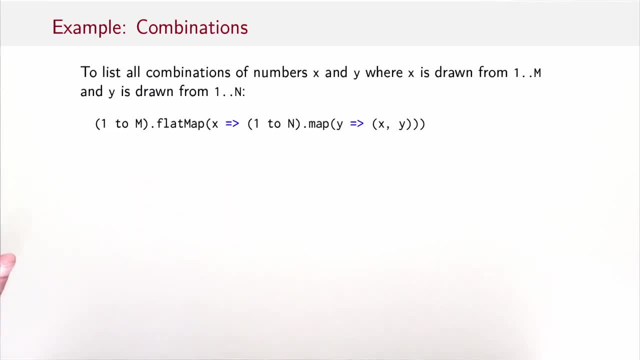 the range one to n and then we do a flat map of the following operation: We have the range one to n and for each element in that range- call that y- we give you the pair x- y. So the x comes from the first range, the y comes from the second range and with the pair we 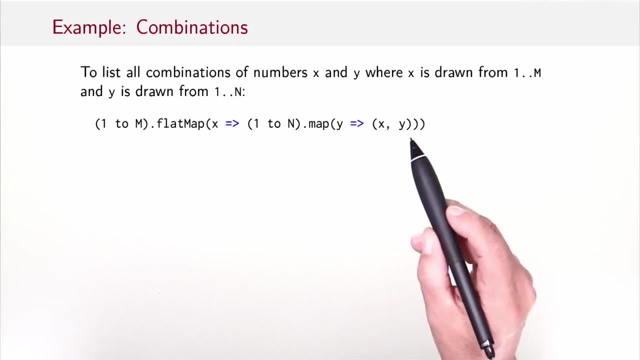 do all combination That by itself the one to n map operation gives you a sequence, and all these sequences are concatenated by this flat map call that you see here. So if you're curious you might ask: well, this is a range and 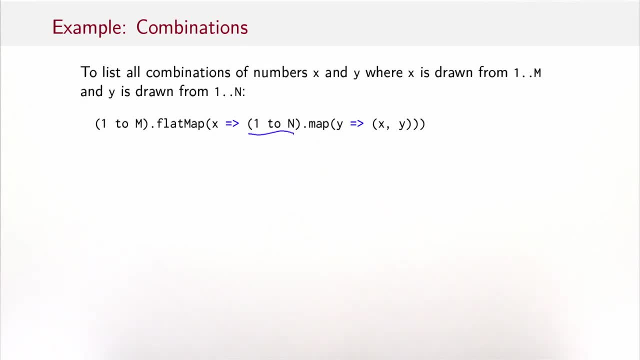 I do a map on a range. What kind of collections do I get back? It can't be a range, because the elements of that collections are pairs and not integers. The answer is: what I get back is the default sequence type, which in this case would be a vector. 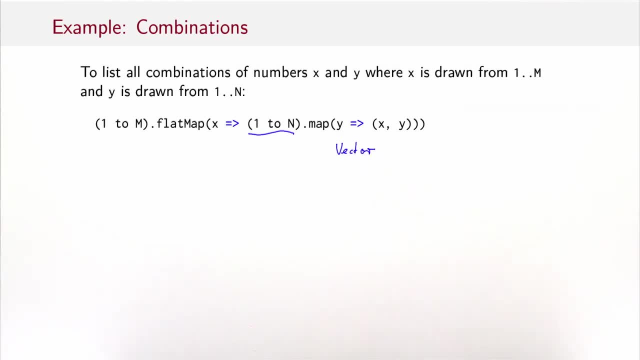 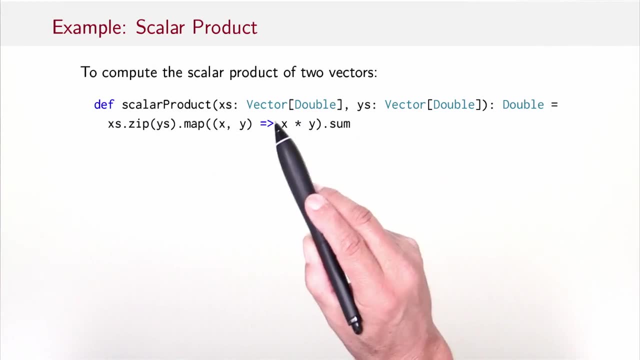 The runtime type of this thing is vector. Here's another example: To compute the scalar product of two vectors, we can write a function like this: def: scalar product of xs vector double ys vector double It's xs zip, ys map the function. 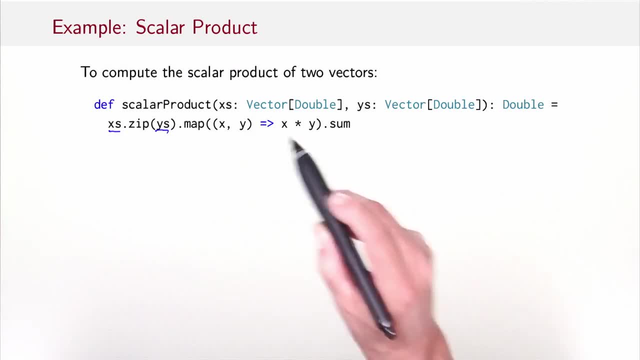 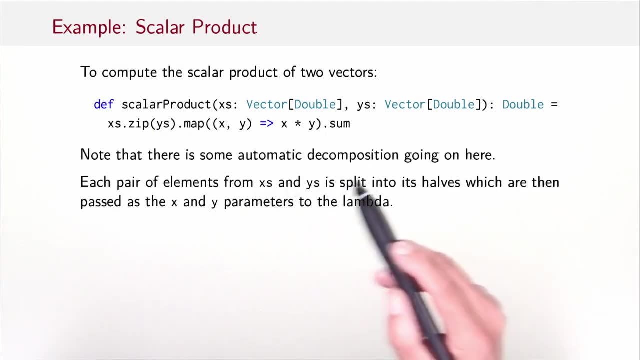 that takes corresponding elements x and y forms the product of x and y, and afterwards we sum it all up with dot, sum. Note that there's some automatic decomposition going on here. xs, zip, ys gives a list of pairs, So map takes a pair, But here, the lambda, we pass. 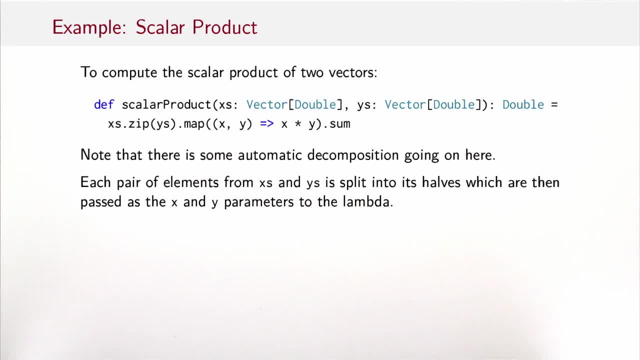 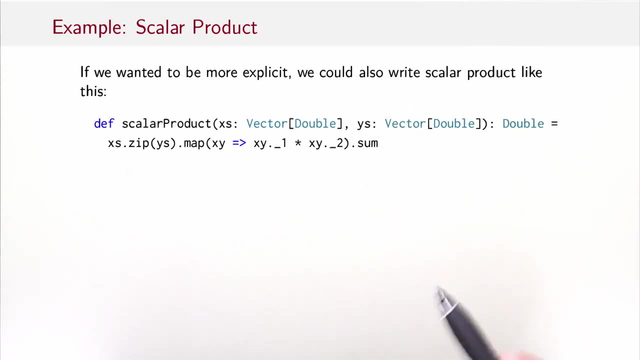 to the map is a function of two parameters. So behind the scenes, the compiler will automatically decompose the pair and put the first half in x and the second half in y. If we wanted to be more explicit, we could also write scalar product like that. So instead of decomposing the pair and letting the compiler do it, we 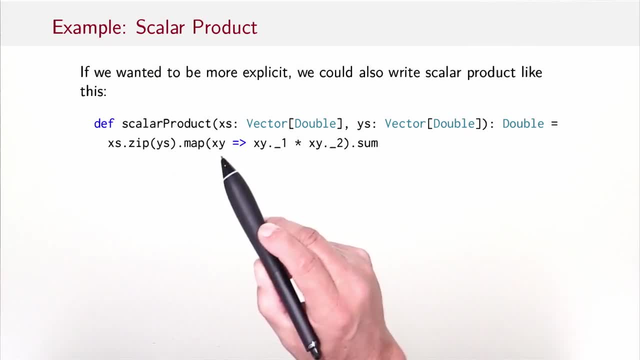 take the xy, which is now the parameter that ranges over the pair, and we take the first half of xy and the second half of xy and multiply it. On the other hand, if we wanted to be even more concise, we could also write it like: 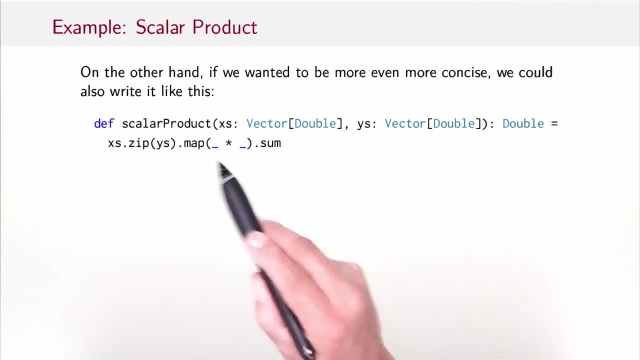 this xs, zip, ys map of underscore times: underscore dot sum. As we've seen before, the function underscore, star underscore, is the function that takes a parameter x and a parameter y and multiplies them. Most people would write scalar product like this. It's clearly the most elegant way to express. 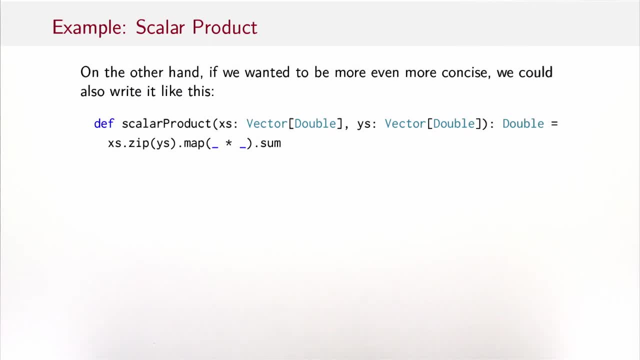 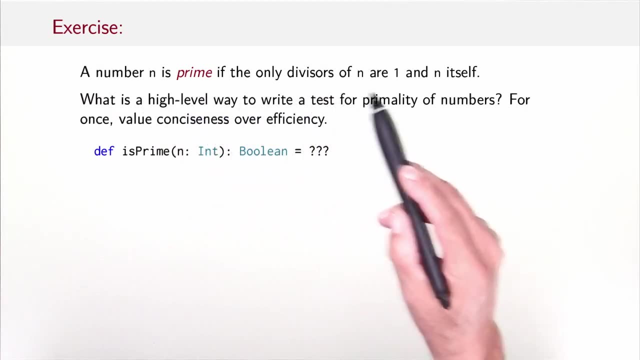 it, And in terms of runtime performance, all three versions are basically equivalent. Here's an exercise for you. A number, n, is prime if the only divisors of n are 1 and n itself. What's a high-level way to write a test for? 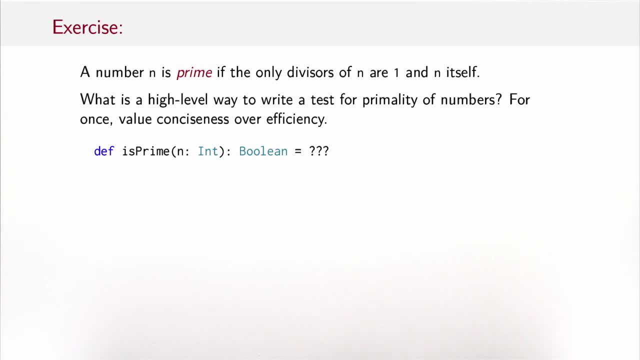 primality of numbers. For once value conciseness over efficiency. So fill in the triple question marks here for the test whether a given integer n is prime. So let's see how would we write that test. So if we go literally we say for all numbers between 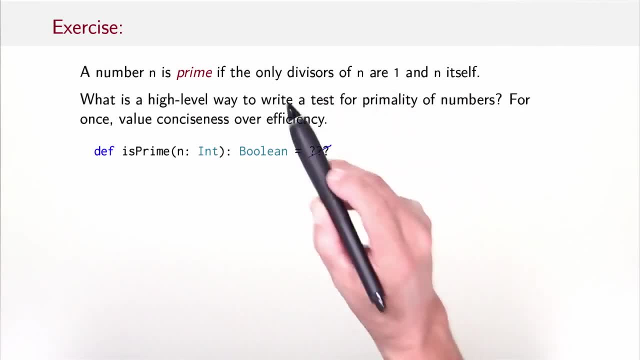 1 excluded and n excluded. that number is not a divisor of prime, So let's just write that literally. So we say 2 until n for all, For all these numbers, we have that n modulo the parameter not equal 0.. 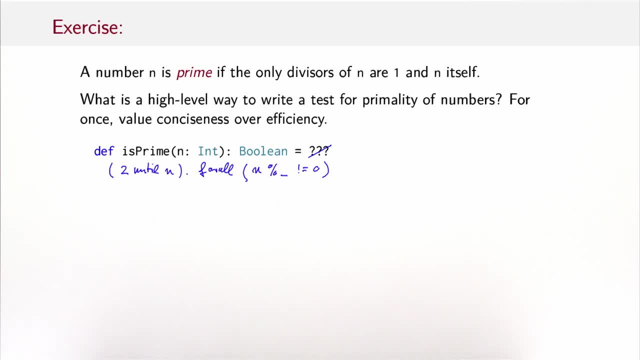 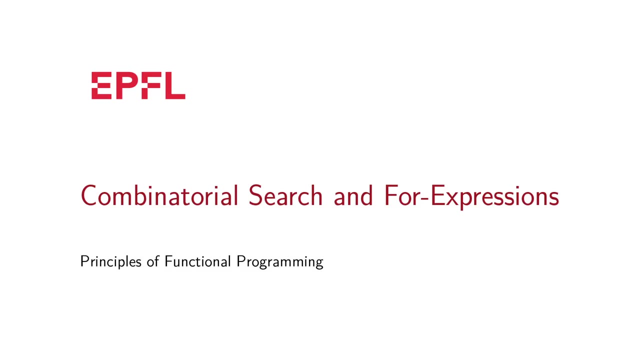 So you see, one of the nice aspects of functional programming and powerful collection operations is that you can write very, very high-level code that directly translates a mathematical specification into code. In this session we're going to take a look how we can use scalar collections for combinatorial 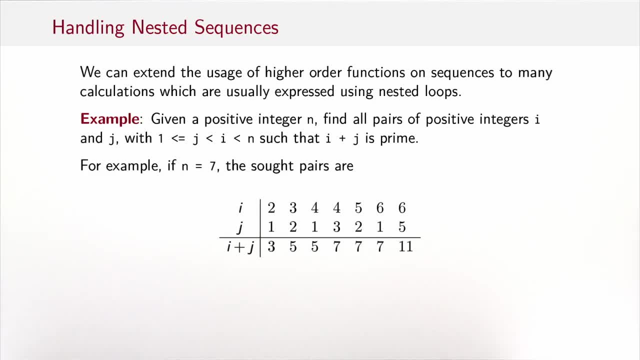 search. In imperative programming, when you search for something, you often do that by means of a loop or a series of nested loops. The loops would terminate when an element that matches the condition is found. In functional programming. you don't have loops at your. 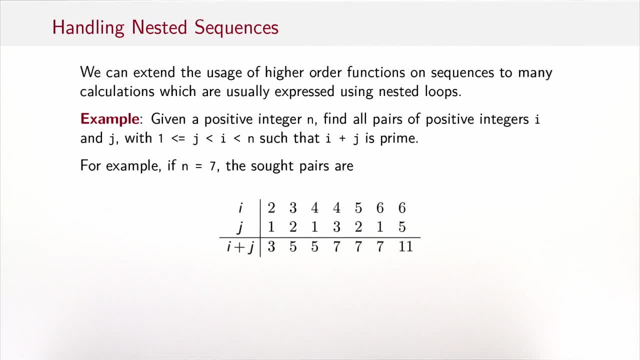 disposal, but you do have higher-order functions, And it turns out that higher-order functions on sequences are a very good toolbox to achieve the same objective- combinatorial search- and they often lead to code that is clearer and shorter than using loops, For example. let's look at this problem. We are given a positive 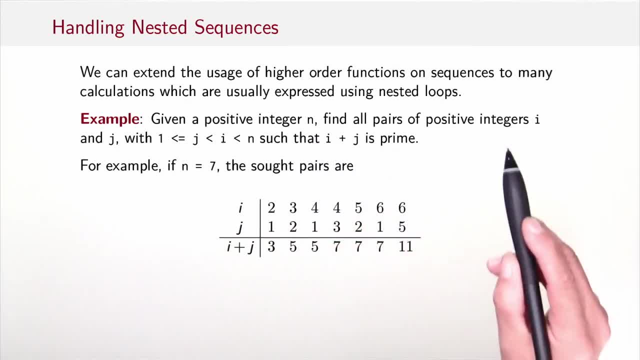 integer n. We want to find all pairs of positive integers, i and j, such that j is between 1 and n, exclusive, and i is between j and n, both exclusive, And a pair of those two integers should meet the condition that i plus j is. 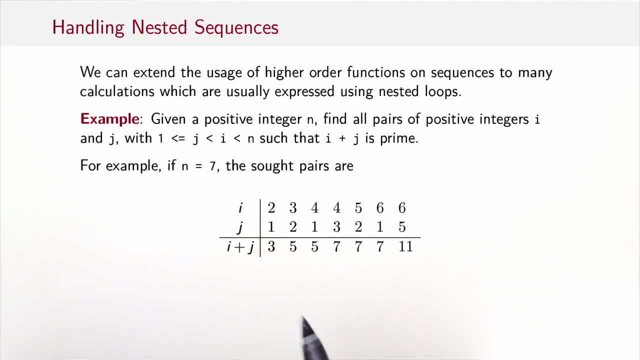 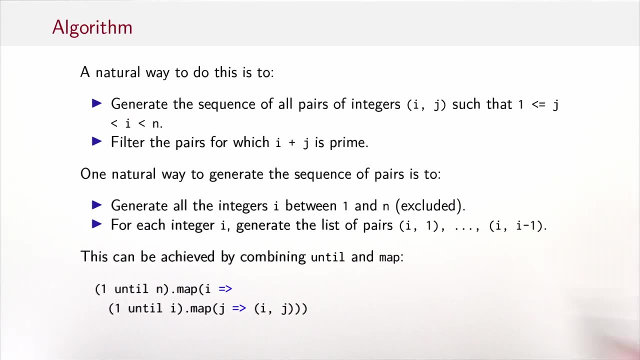 prime. For example, if n equals 7,, then the pairs of the solution are here: in this list, The smallest set of integers with a prime set sum is 2 and 1, and the largest is 6 and 5.. So how do we find a solution to this problem? A natural way to do so is to generate 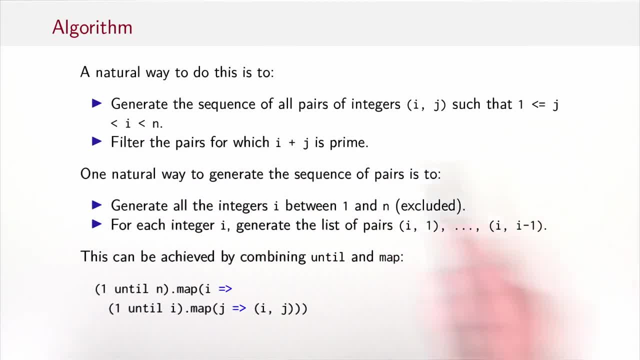 the sequence of all pairs of integers i- j that are within bounds as a specify, and then filter that sequence for the pairs for which i plus j is prime. So how do we generate the sequence of pairs? Well, we first generate all the integers i between 1 and n excluded, and then, for each integer, 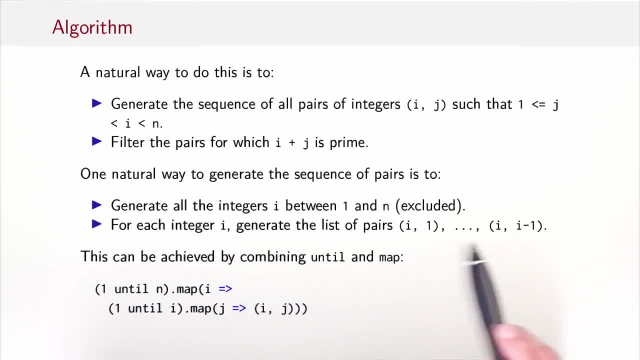 i given. like that, we generate a list of pairs i, 1, and so on up to i i minus 1.. And that can be achieved by combining until and map. So we start with the list 1 until n, We map it. 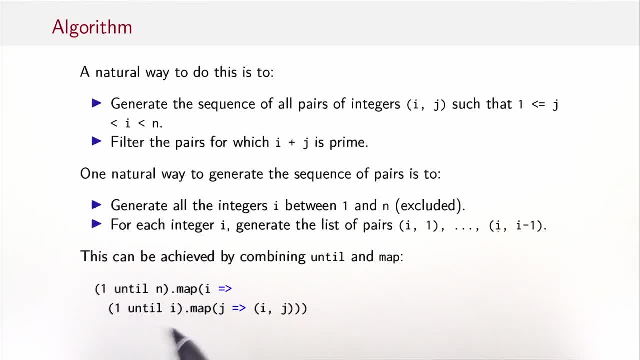 so that for each of those we get the list 1 until i and we map that list with a j so that we can get back the pair i and j. So that's close to the solution, but not quite yet, because, like that, 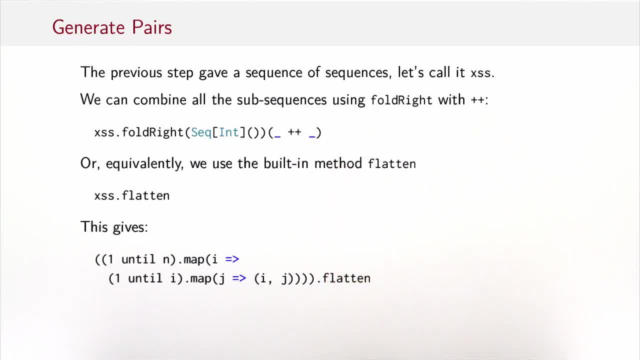 we get a sequence of sequences. Let's call that sequence of sequences xss. So that's a good step towards a solution, but it's not quite what we need yet, because the previous step gave us a sequence of sequences. Let's call it xss- What we still have. 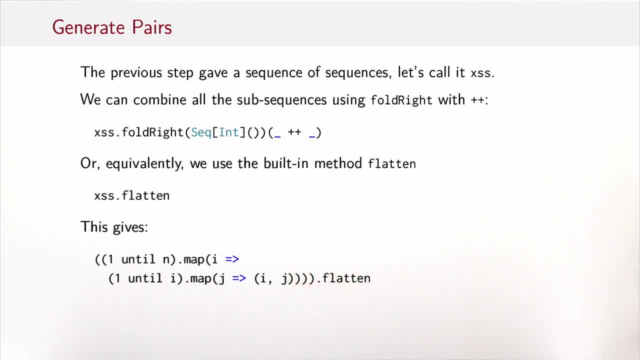 to do is combine all the subsequences into one single sequence, and we can do that with fold right and plus plus, So for instance, xss fold right with the empty sequence and plus plus with the operation. Or equivalently and simpler, we can use the built-in method flatten, So we can just 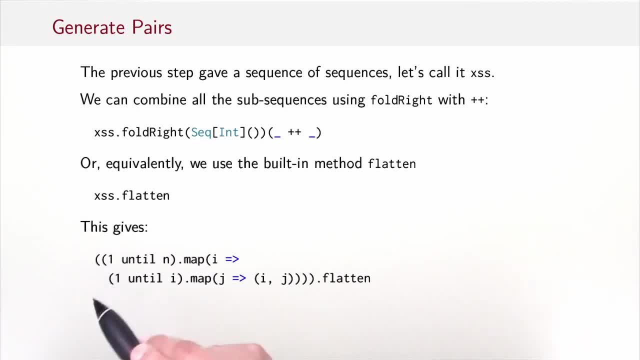 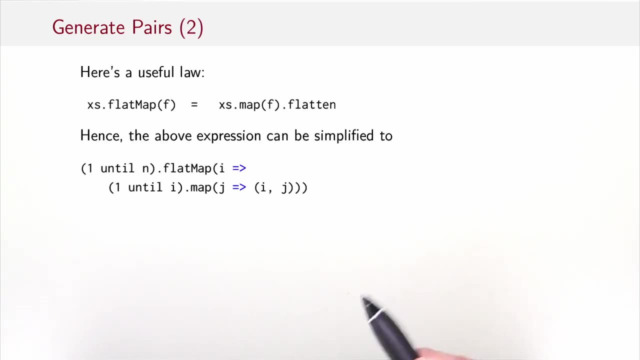 write xss, dot, flatten. So that gives together the expression that you see here. We map over 1 until n, We map over 1 until i, We form the pairs of i and j and we flatten the results. Here's a useful law For any collection: xs, xs, flat map. 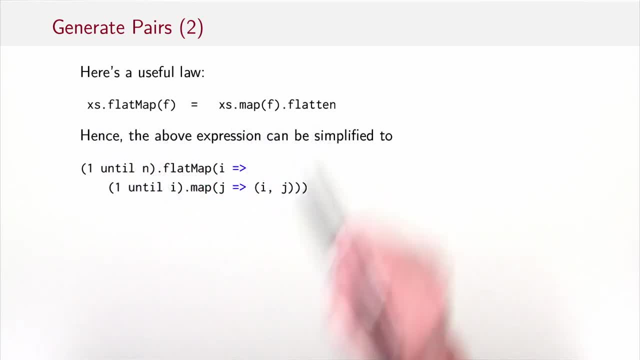 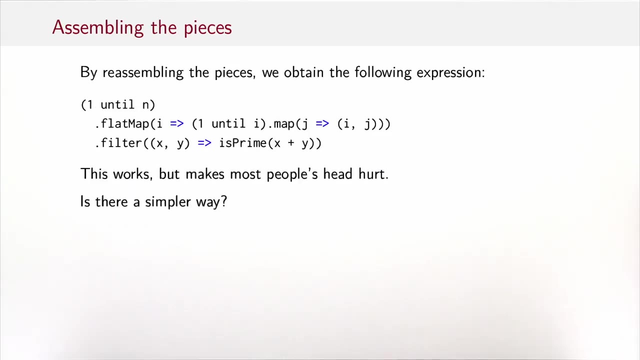 f is the same as xs: map f and then flatten. So the above expression can be simplified to: 1 until n flat map i. 1 until i map j form the pair of i and j. So now we need to reassemble the two pieces and we obtain the following expression: 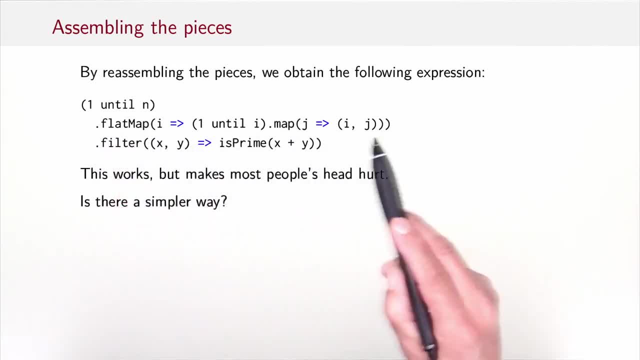 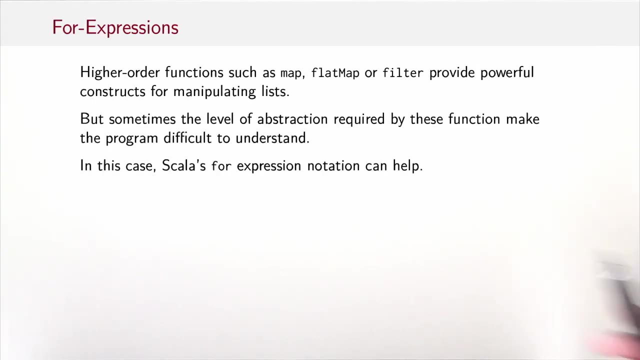 1 until n- flat map. i map j, i, j and then we filter the pairs x- y to keep only those pairs where x plus y is prime. This works, but it makes most people's head hurt. Is there a simpler way? Generally higher-order functions such as map, flat map or filter. 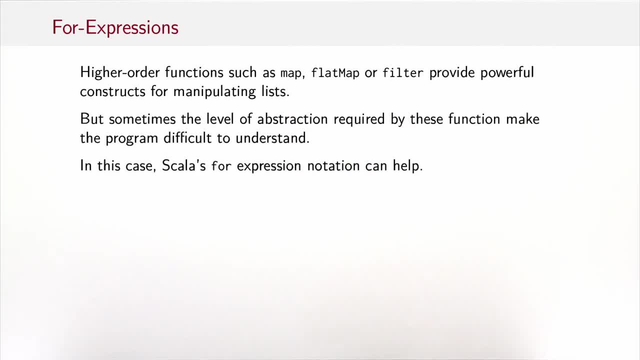 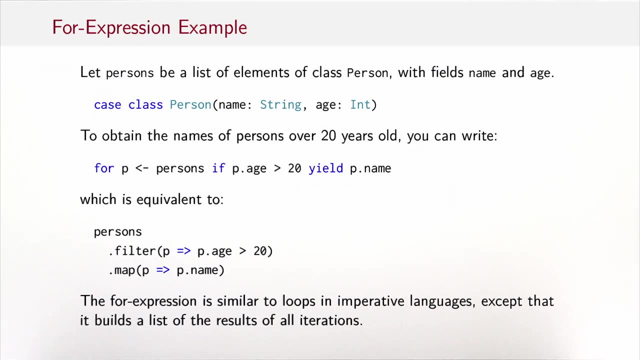 provide powerful constructs for manipulating lists, But sometimes the level of abstraction required by these functions make the program difficult to understand. In this case, Scala's four-expression notation can help, And that's what we are going to discover. next. We introduce four expressions with an example: Let persons be. 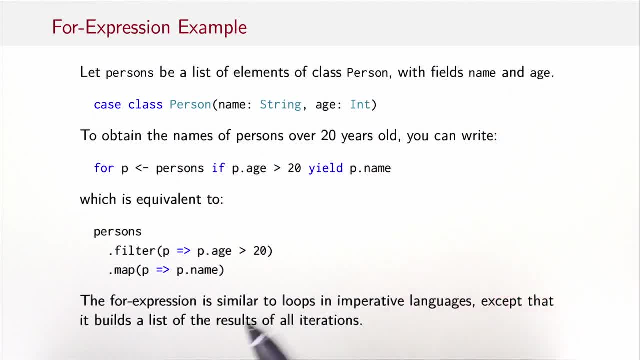 a list of elements of class: person with fields name and age. So here's the definition of that class. To obtain the names of persons over 20 years old, you can write for p left arrow. so this is pronounced taken from persons if p dot age greater 20. 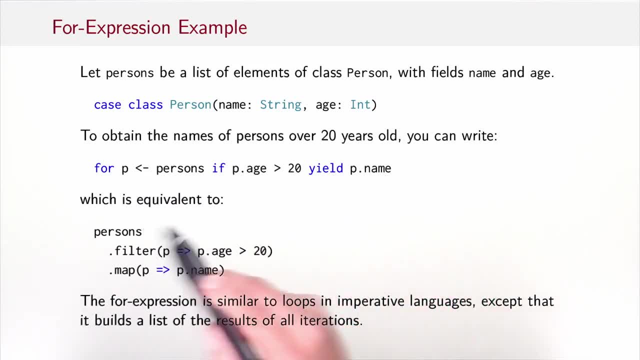 yield p dot name. This four-expression is equivalent to writing persons dot filter such that p dot age is greater than 20, and then dot map take the name of the person. So that four-expression looks a bit like a for loop in an imperative language, except that it builds a list of the results instead of working by. 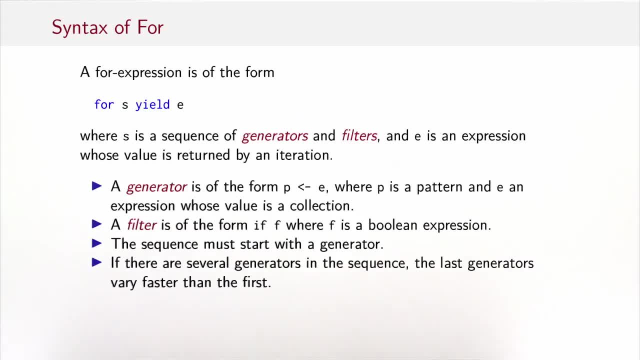 side effects. So you've seen a particular example of a four-expression. In general, four-expressions are of this form: for s yield e, where s is a sequence of generators and filters and e is an expression whose value is returned at each iteration step. So each e 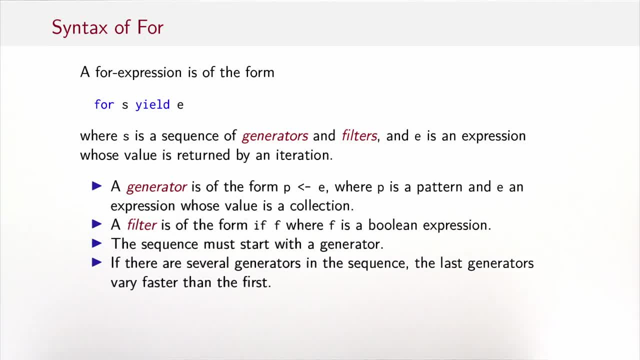 designates one element of the collection that is returned by the four as a whole. So what are generators and filters? Well, a generator is of the form p, left arrow, e, where p is a pattern and e is an expression whose value is a collection. 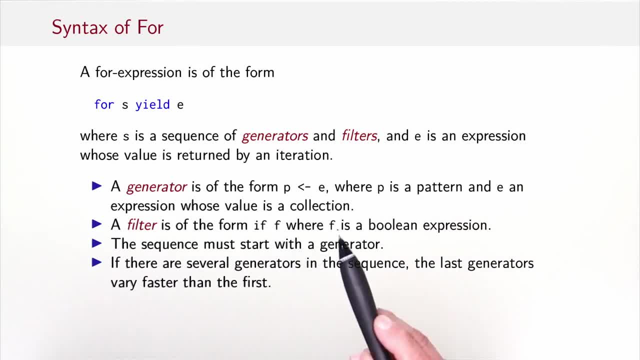 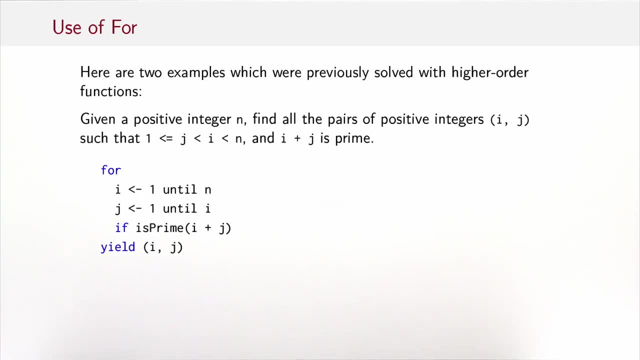 And a filter is of the form: if f, where f is a Boolean expression, The sequence must start with a generator, and if there are several generators in the sequence, the last generators vary faster than the first. Here are two examples which were previously solved with high-order functions. The first example was given. 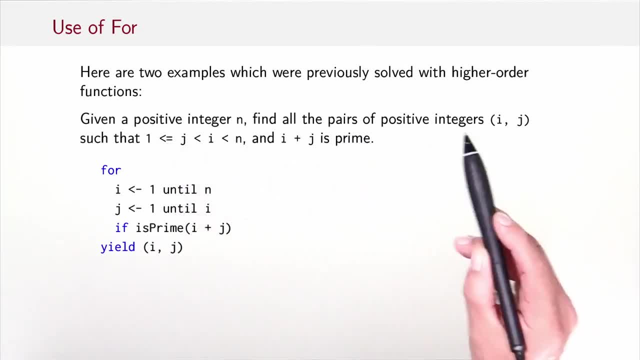 a positive integer n, find all pairs of positive integers with these range conditions, such that i plus j is prime. So that can now be written like this We can write for: let's take i from 1 until n. let's take j from 1 until i, if is. 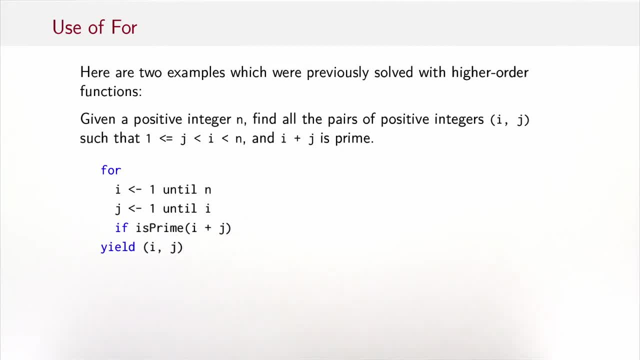 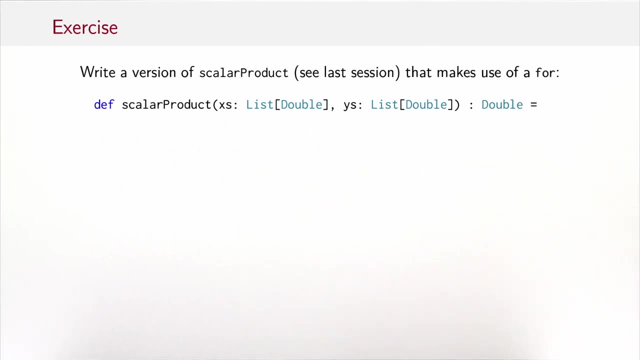 prime i plus j, then yield i- j as a pair. So this is clearly clearer than the previous example using high-order functions. As a second example, let's write scalar product with the use of a for. So here you have the outline of scalar product. What would it look like if you? 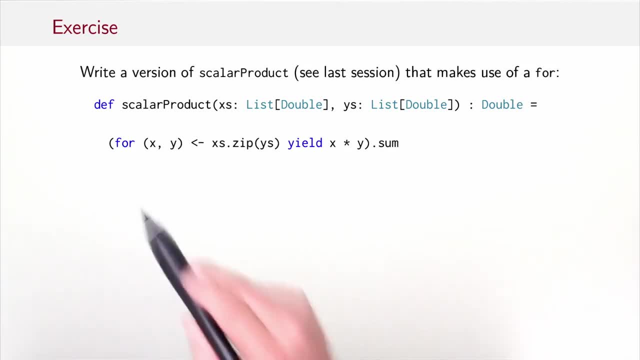 write it with a for. So here's the answer. We would have a for expression that still needs to zip xs and ys. It matches that with the pair xy, and for each xy that comes from this range it yields x times y and finally we have a sum of the whole sequence. 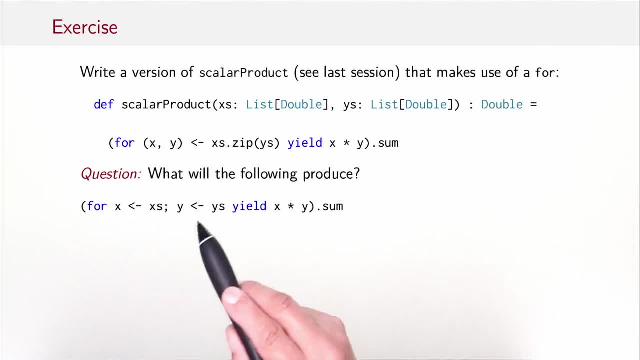 You might ask the question: well, why couldn't we write it like this For x taken from xs, y taken from ys: yield x times y. Would that work as well, or would it do something different? or maybe not compile? 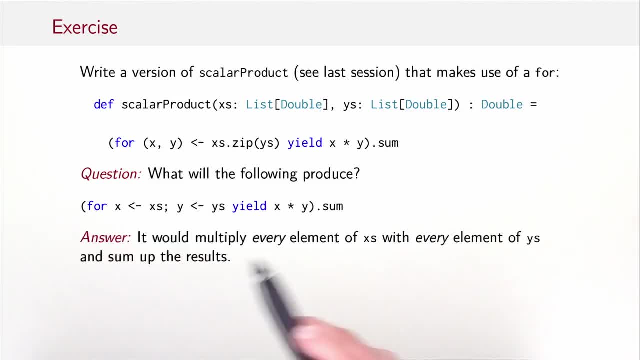 The answer is it would compile, but it would do something different. It would multiply every element of xs with every element of ys, So not just corresponding elements, but every element of xs times every element of ys, So it would be a quadratic number. 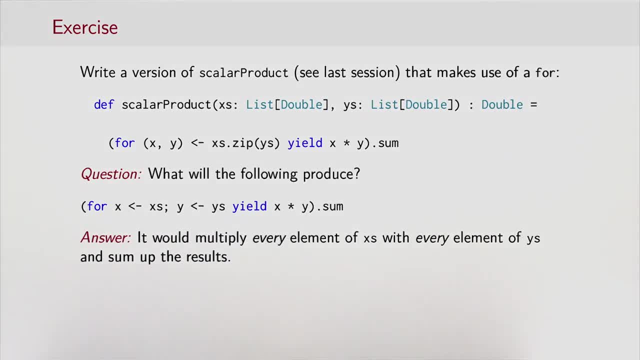 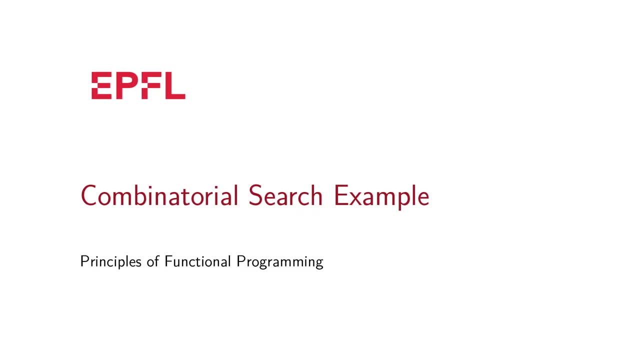 of terms that we multiply and then sum up. In this session we'll use the techniques we have explored in the previous sessions in a larger combinatorial search example. Before we do so, we need to introduce one more collection type: sets. Sets are another basic abstraction. 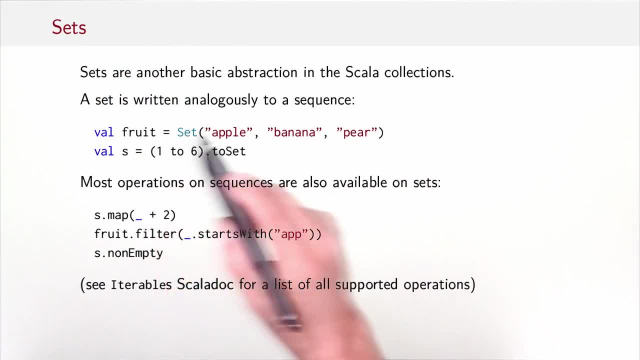 In the Scala collection. a set is written analogously to a sequence. So we write: while fruit equals set of apple, banana, pear, or here we have the range one to six, dot two set. That would give us a set of the numbers one and up to six, Most operations on sequences. 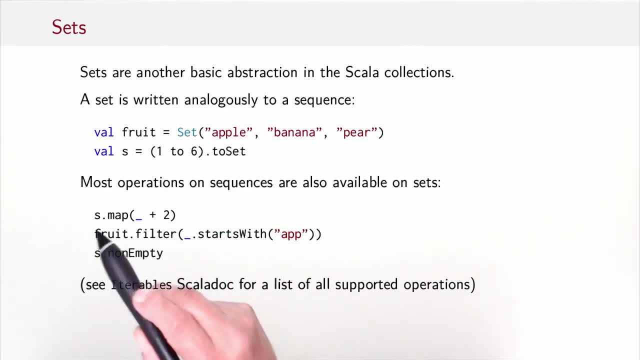 are also available on sets So we can map sets s dot map. underscore plus two would add two to each element of s, giving you the set Three, two, eight. Fruit filter starts with app. That would give you the set of fruits. 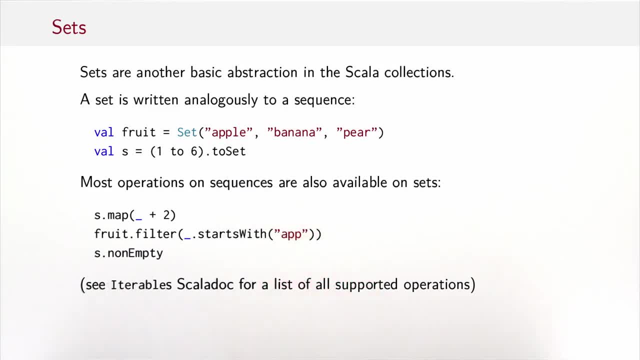 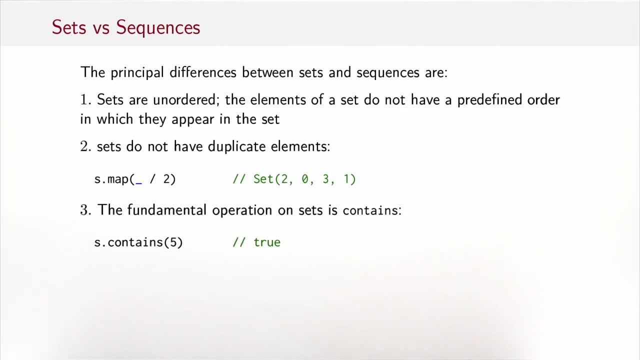 that consists just of apple And s dot. non-empty would return true. Here are the principal differences between sets and sequences. There are three overall. The first difference is that sets are unordered. The elements of a set do not have a predefined order in which they appear in the set. 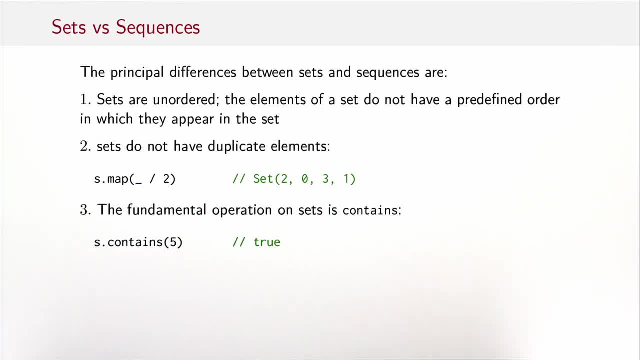 So if you print out the elements of a set, you do not know a priori which element will come first. The second difference is that sets do not have duplicate elements. So, for instance, if we take the set of numbers one to six and we map it with a division by 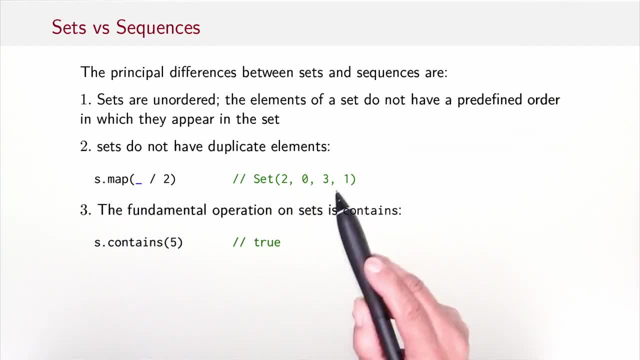 two operation. then we get a set of numbers, one to three, and each number appears only once in that set, even though six and five both would map by division of two to three. But you do not have a duplicated three, you have a. 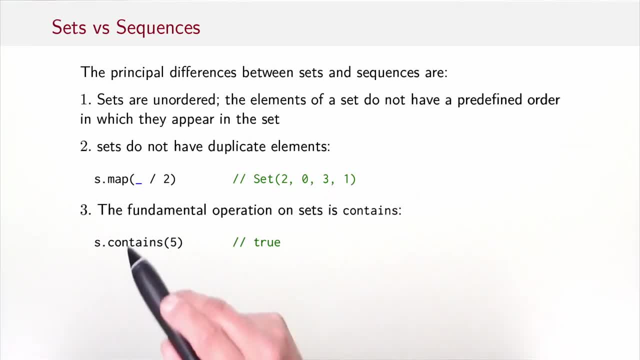 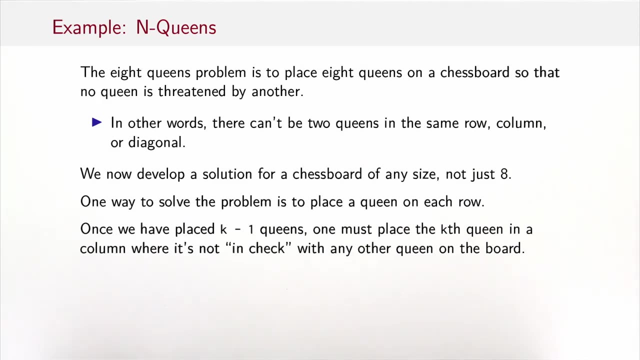 single one here. And the third difference is that the fundamental operations on sets is contains, So s contains five, would give you true. So now let's get to the combinatorial search problem that we want to tackle. The problem is the n queens problem, The eight queens problem, 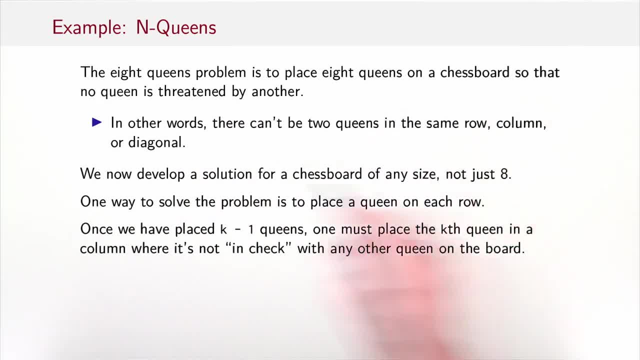 is to place eight queens on a chessboard so that no queen is threatened by another. In other words, there can't be two queens in the same row, column or diagonal. We now develop a solution for a chessboard of any size, not just eight. 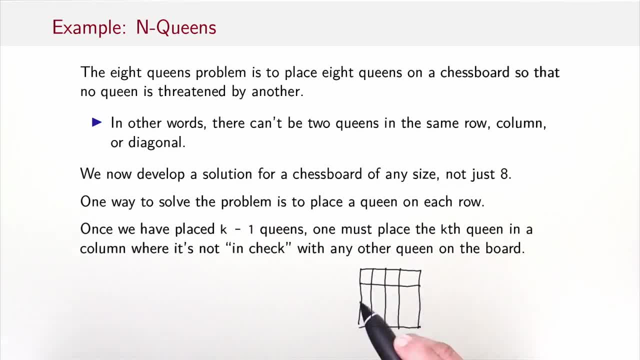 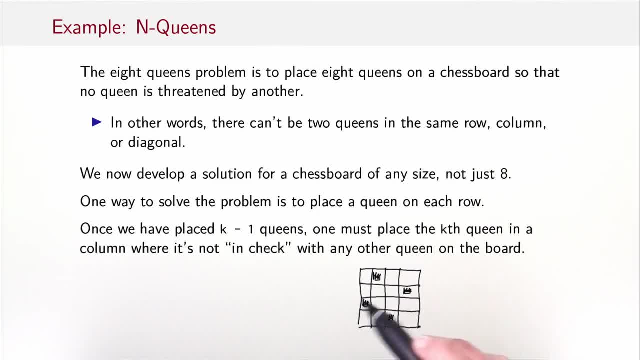 each queen is in its own column, in its own row, and none of them checks the other by a diagonal. This is not the only solution. You can find other solutions by rotating that image or taking the mirror image according to one of the axes. It turns out that for larger boards, there are many, many more solutions. 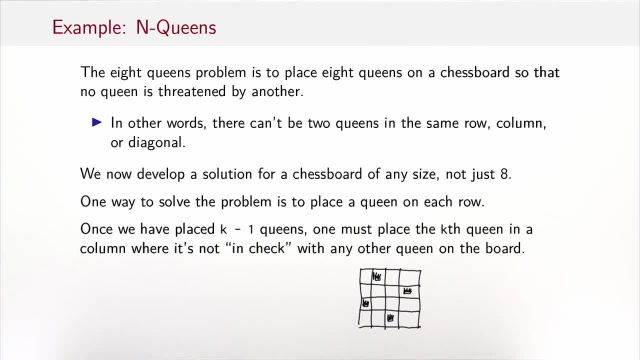 so the number of solutions grows as the board grows. So let's now develop a solution for a chessboard of any size. So one way to solve the problem is to place a queen on each row. We start with the first row and the queen is arbitrary. Then we go to the next row and we pick a. 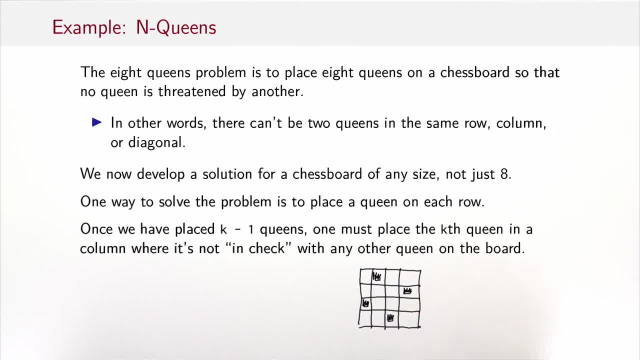 column where the queen is not yet in check with the previous queen, and so on. Generally, once we have placed k-1 queens, we must place the kth queen in a column where it's not in check with any other queen on the board. 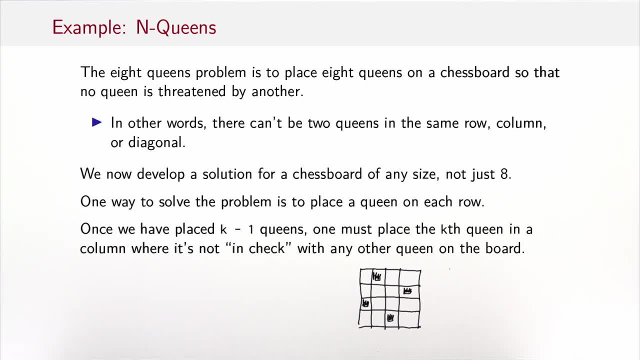 Of course it's possible that one gets into a dead end, that one ends up in a row where no position of a queen would be legal. In this case you have to backtrack and change some of the previous queens so that a place becomes free in that row. For instance, 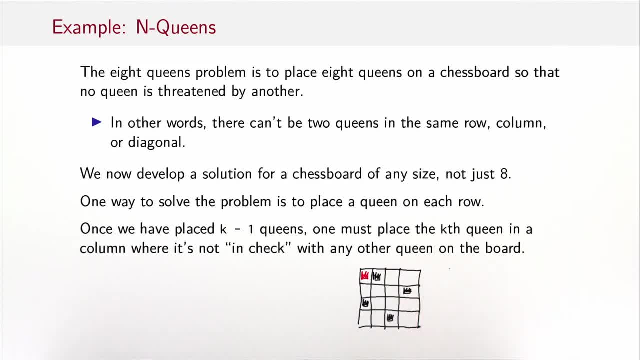 if we had placed the first queen here instead of one to the left, then it would have turned out that there is no way to complete the puzzle, so one would have to backtrack all the way to the first queen and say, no, that we can't place it here, We have to place it one. 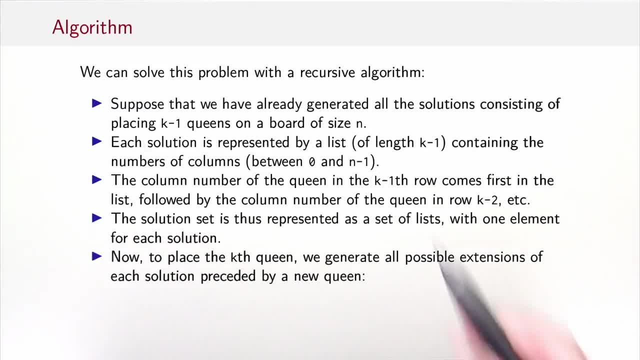 field to the right, So we can solve this problem with a recursive algorithm. The idea is- let's suppose that we have already generated all the solutions consisting of placing k-1 queens on a board of size n. Each solution is represented by a list of length- k-1- that contains 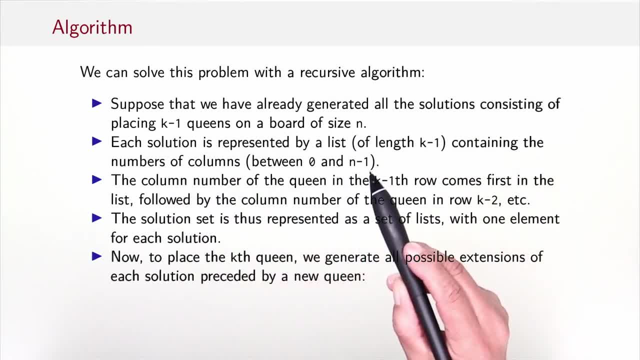 the numbers of the columns between 0 and n-1 of the queens that have been placed: The column number of the queen in the k-first row, so the last queen that was placed comes first in the list, followed by the column number of the queen in row k-2, and so on, and the last queen in the list is the. 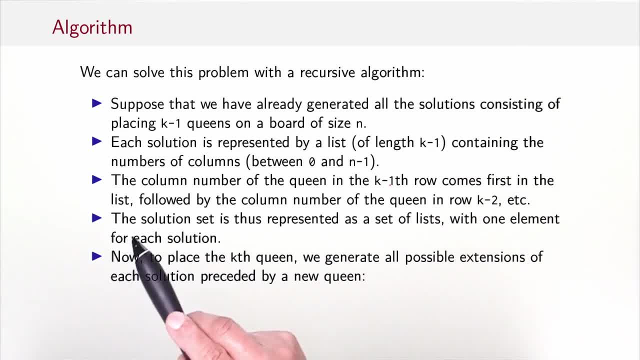 queen on row number 1.. The solution set is thus represented as a set of lists with one element for each solution. So all solutions are a set and each solution is a list of column numbers. Okay, so now to place the k-th queen, we generate all possible. 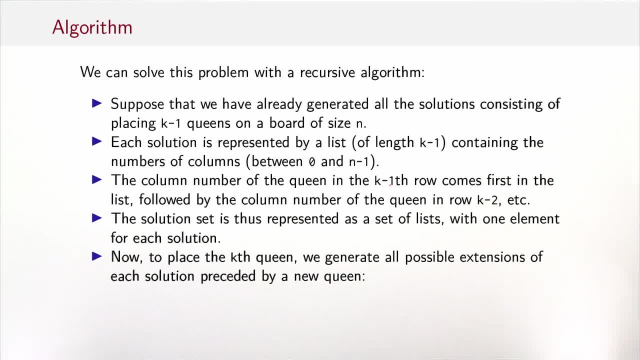 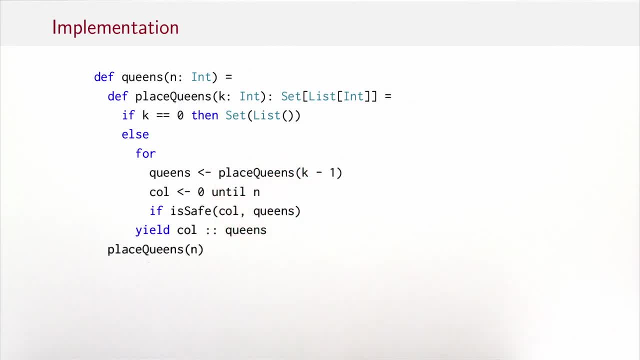 extensions of each solution preceded by a new queen. So here's the implementation. We have this method: def queens. it takes the size of the board n and it simply consists of a call to place queens n. Place queens takes a parameter k which says how many. 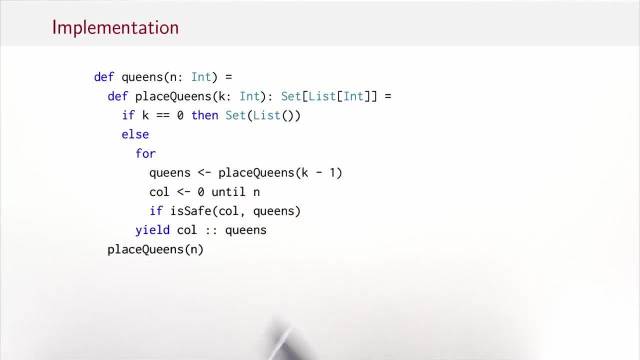 queens are still to be put on the board And it returns a set of list of integers, as discussed. A set of solutions is a solution is a list of int. So if k equals 0, that means we don't need to place any queens, so we can respond with the empty list. that's the. 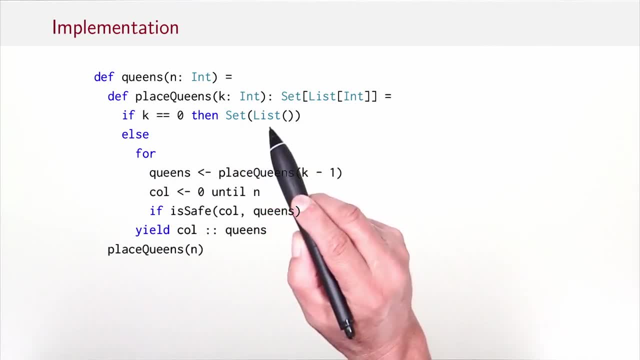 solution and we return with a set that consists of just this solution. So if k is not 0, then we recursively call place queens of k minus 1.. So we have a problem that is 1 simpler than before And we let queens range over the result. So place queens k minus 1 is 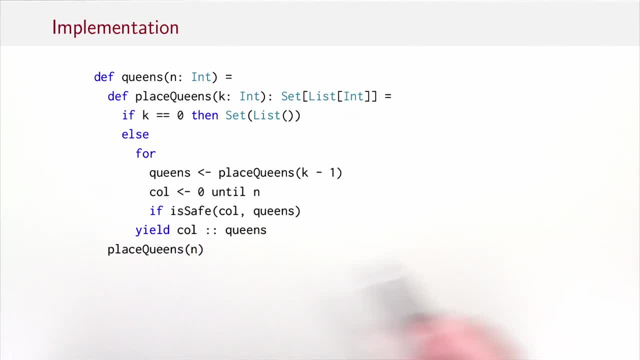 a set of solutions. Now each queens here is a solution, so it's a vector of column numbers. Now the task is to place the k-th queen. So we do that by letting col range from 0 until n. that's the possible columns of the board where we could place the queen And we 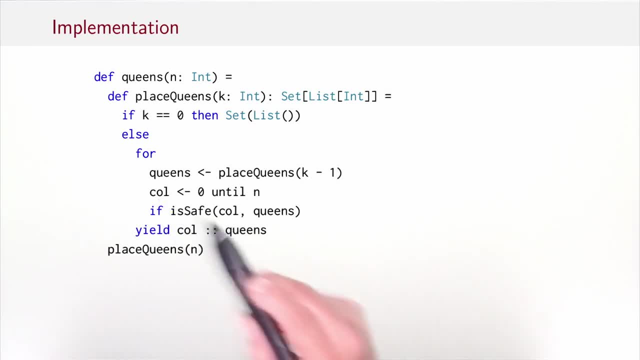 ask whether the queen would be safe in this column relative to the queens that already have been placed. If that's the case, we yield the column, the new column preceding the queens that have been placed, And that's it. It's actually surprisingly simple. 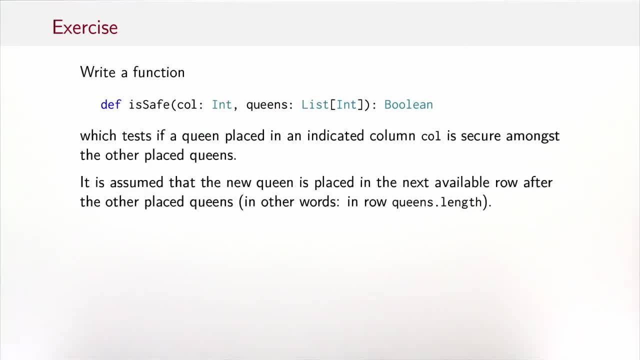 And concise as a solution for this problem. Well, it's not quite the solution yet. We still have to write the function isSafe. So isSafe takes a column where we want to put the new queen and a list of ints, which is the. 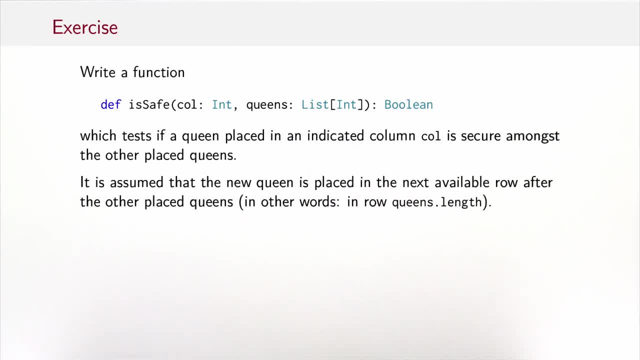 column numbers of the queens that have been placed so far And it should test whether a queen placed in that column is secure amongst the other placed queens. So it's assumed that the new queen is placed in the next available row after the other placed queens. 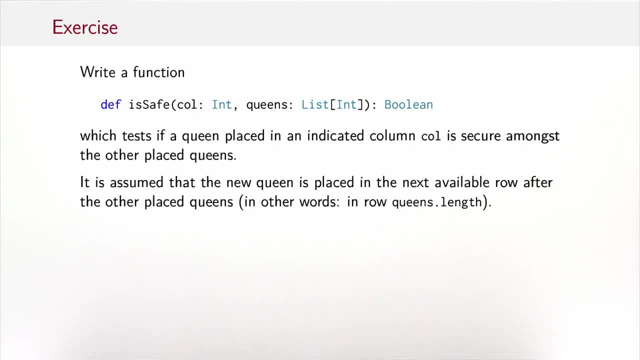 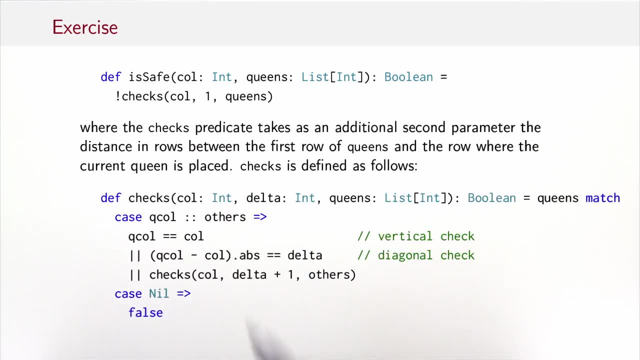 In other words in row queenslength. So try to come up with an implementation of isSafe as an exercise. So here's a possible solution. isSafe of column versus queens is that the column is not in check with a distance of 1 to the list of queens. 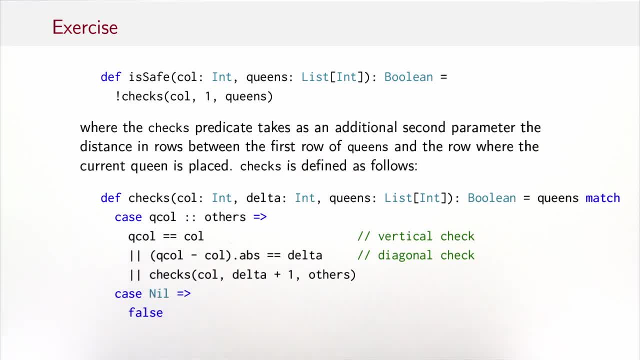 Which uses an auxiliary method, checks. that takes an additional parameter, delta. So it takes a column number where the new queen is put, The queen that remains to be checked, And delta, which is the distance of the row where the new queen should be placed And the last row, the first queen. 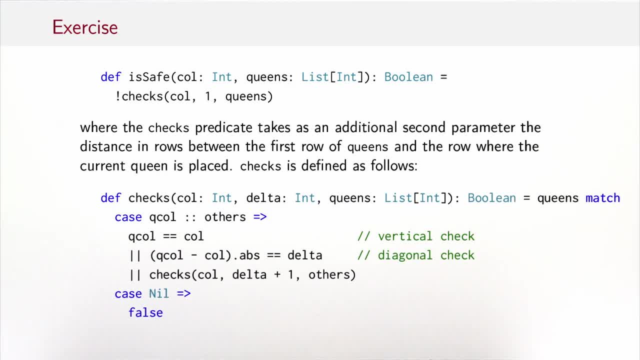 of the list here was placed Initially. delta is 1 because we follow the queens directly by the column we place. So the checks method now is implemented like this. It says: well, if the queens is empty, then the result is false, The queen is not in check. If the queens 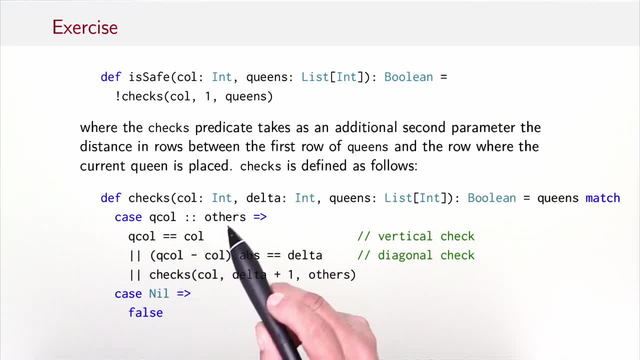 is non-empty. so let's say we have a queen column and some others, then if the queen column is the same as the column, that's a check. That's a vertical check. Or the queen column minus the column absolute value is the same as the distance delta here. That's a diagonal check. 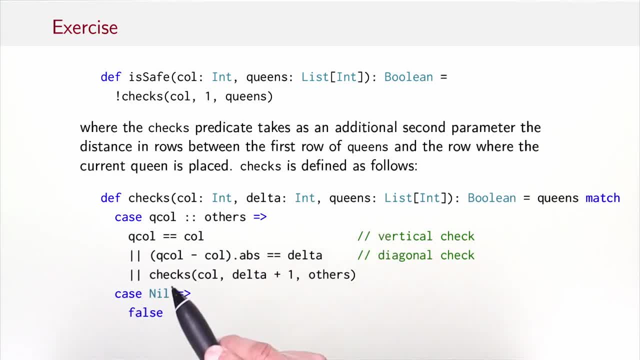 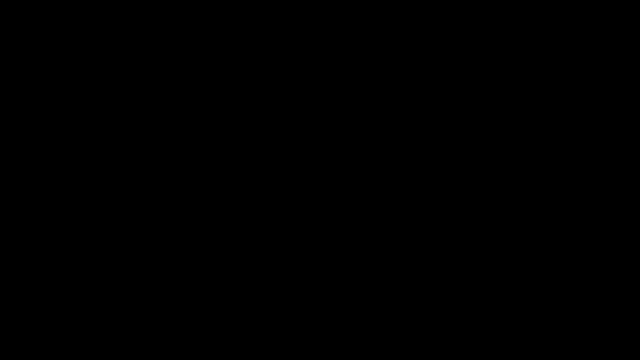 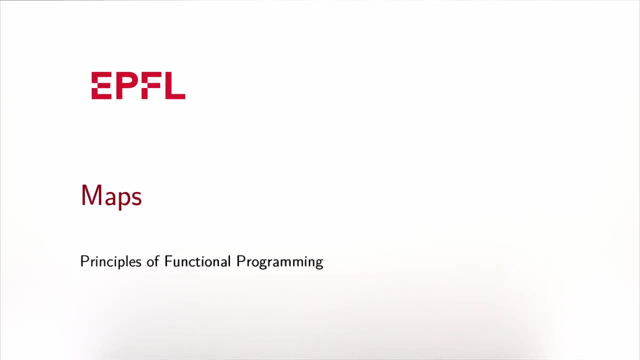 Or it might be in check with some of the remaining queens. So that's a recursive call. Checks with the column delta plus 1 and the others. So you know by now how to deal with sequences and sets. In this session we'll get to know the third fundamental. 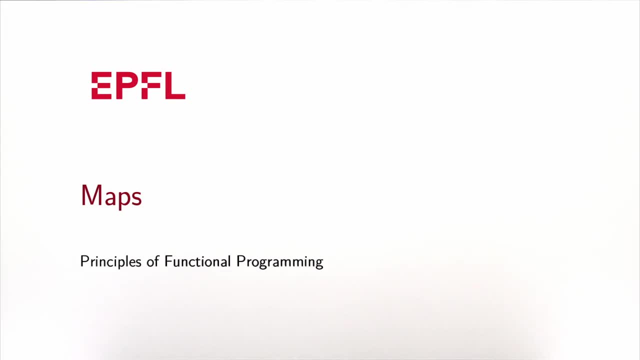 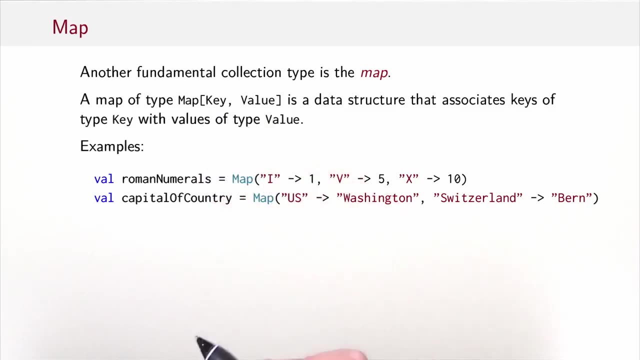 collection type, namely maps. Map takes two type parameters: a key type and a value type. It is a data structure that associates key of type key with values of type value. Here are two examples of maps: Roman numerals: It's the map that goes from the letter i to 1, the letter v to 5,. 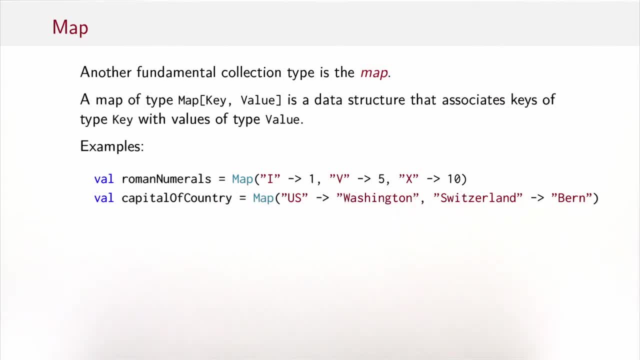 the letter x to 10. You can extend that to further letters, of course. So that's a map from strings as the key type to numbers as the value type. The second map we have here is capital of country. That's written map: US, Washington, Switzerland, Bern. So that's a map from. 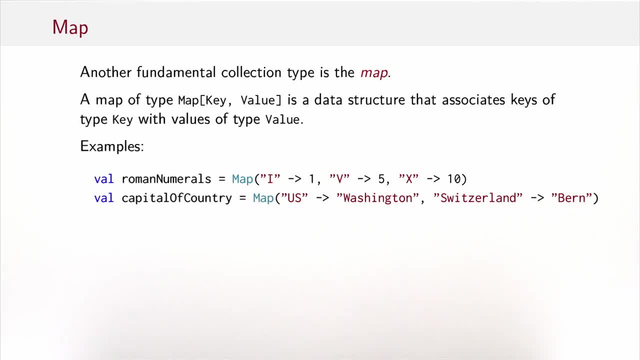 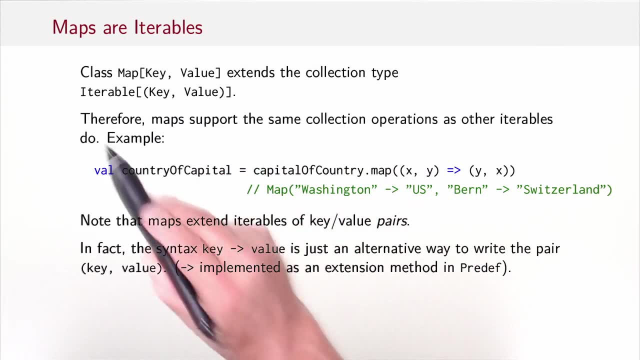 strings to strings. The key type and the value type are both strings. Maps are a special subtype of iterables. The type map key of value extends the collection type- iterable- of pairs of keys and values. So since maps are iterables, they support the same collection operations as other iterables. 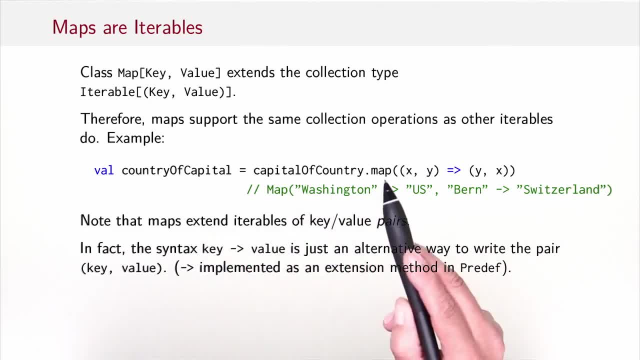 do. For instance, we can map a map itself. So we can write: country of capital is capital of country map, And then it takes the key and the value. So that's the country and the capital And it reverses the two. So now we have the capital first and the country second. 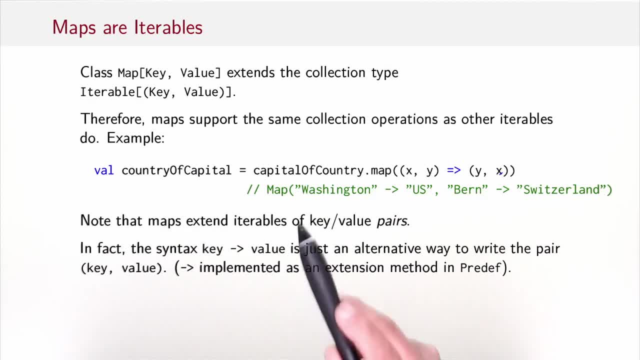 And that would give the new map country of capital, And if we print it out it's Washington, US, and Bern, Switzerland. Note that maps extend iterables of key value pairs. In fact, the syntax key arrow value is just an alternative way to write the pair key value, The right arrow. 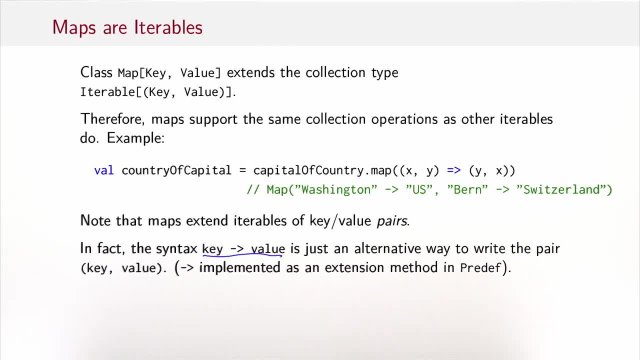 here is implemented as an extension method in predef, which is an object that's implicitly imported into every Scala program. So the right arrow here is not syntax, it's just essentially another method definition. You can think of the extension method to be defined like this, So it would be extension with 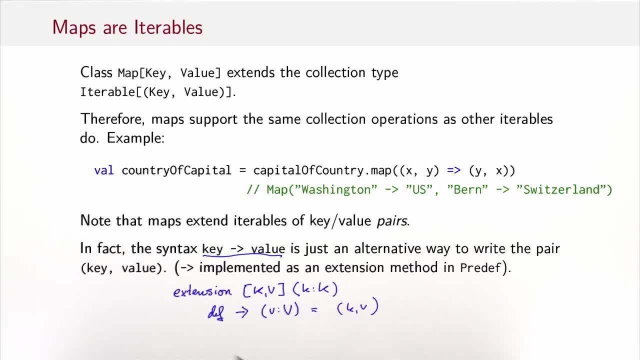 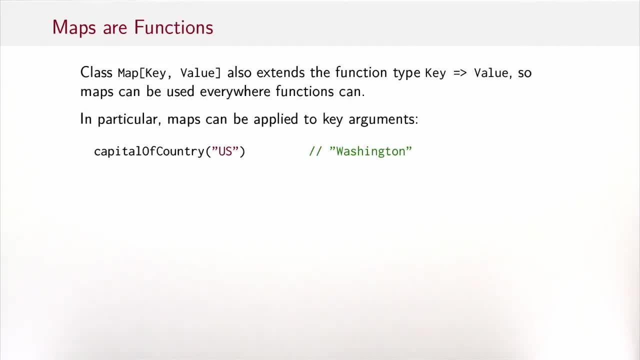 arbitrary parameters k, v. A key of type k, a value of type v, returns the pair of k and v. So we've seen that maps are iterables and we've put that to good use. But maps are also functions, So the class maps. 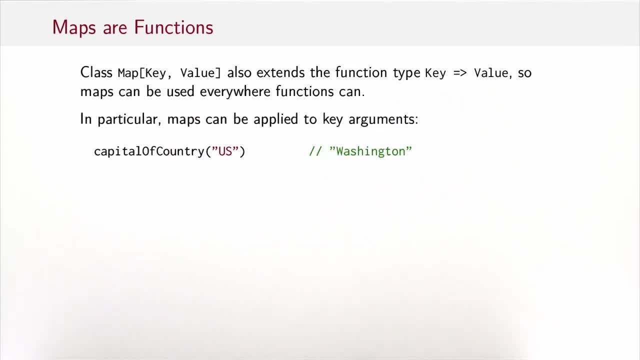 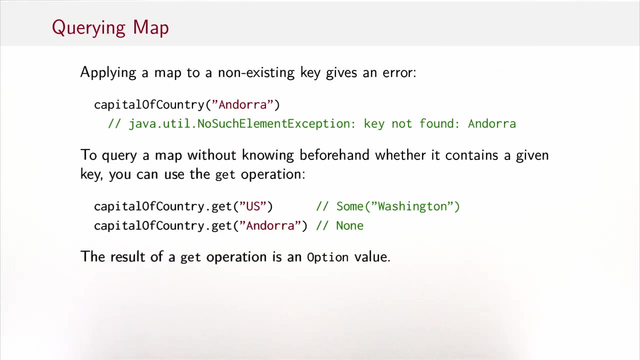 key value also extends the function type key arrow value. So that means that maps can be used everywhere functions can. In particular, maps can be applied to key arguments So you can write capital of country US and that would give you Washington. What happens if you apply a map to a key? that's: 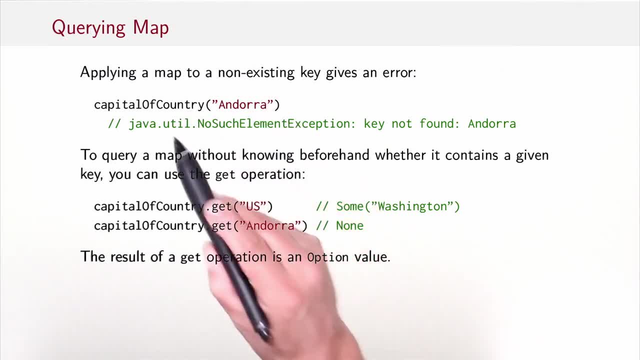 not defined in the map. Well, applying a map to a non-existing key would give you an error. If you tried capital of country Andorra, then you would get an exception. a Java user would tell no such element exception. That would tell you, furthermore, that the key Andorra was not. 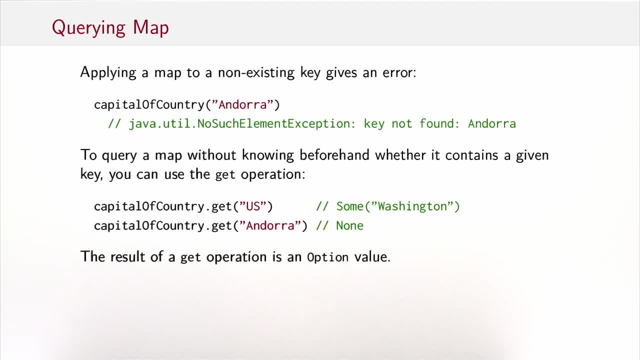 found. So you should use the application syntax for maps only if you're sure that the key is in fact in the map, But in most cases you're not. So in that case there's a second operation, which is called get. that doesn't throw an exception if the 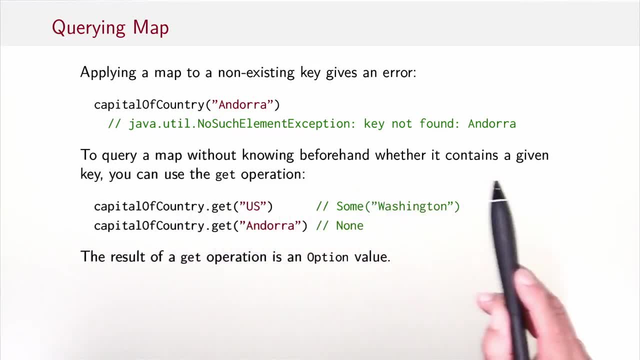 key is not in the map. So to query a map without knowing beforehand whether it contains a given key, use the get operation. Here's what it's used like Capital of country: dot get US. that would give you a value called sum Washington. So it. 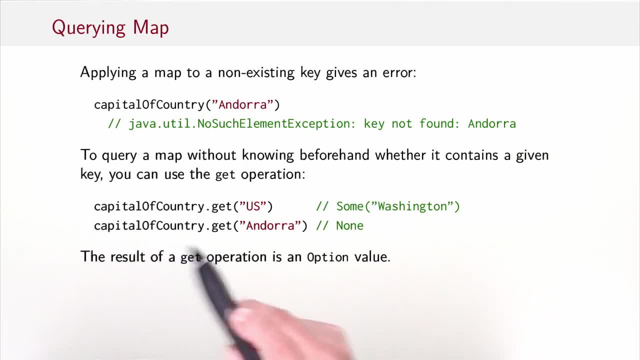 says there's something there and it's Washington. And if you say capital of country, get Andorra, then you would get a different value which reads none. The result of a get operation which has these values sum and none is of type option. So the option type is: 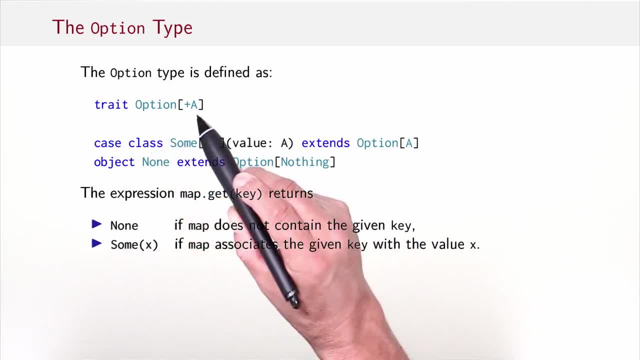 defined as you see here. It's a trait with a single type, parameter a, which is covariant. It has two cases: sum and none. Sum is a case class that takes a value of type a and extends option of a. None is an object and it extends option of nothing. So 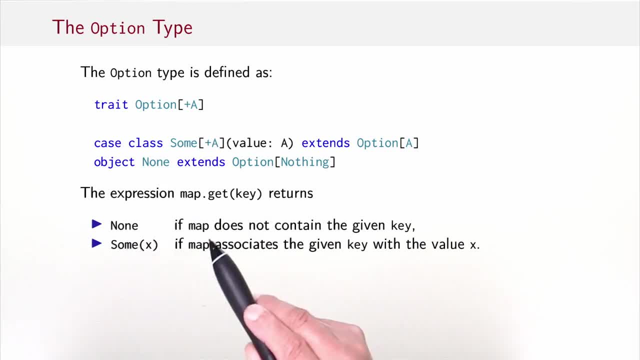 an expression map dot, get key would return none if the map does not contain the given key and sum of x if the map associates the given key with the value x. So how do you work with options? Well, since options are defined as case classes, 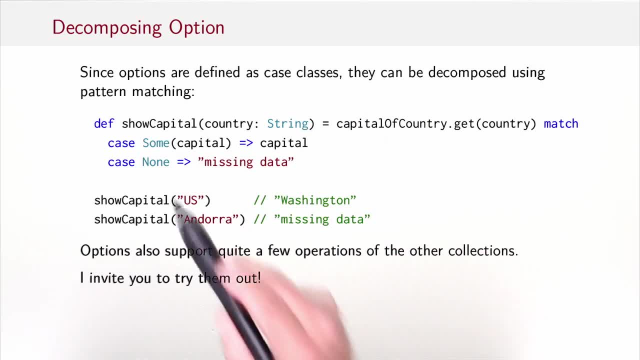 they can be decomposed using pattern matching. So here's a typical method. let's say we want to show the capital of the given country and not fail with an exception if the country is actually not in the map. So here we would say: capital of country dot get country match If we found a capital. 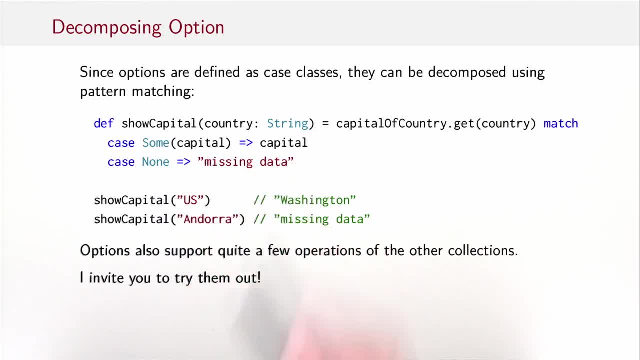 then report that If we found nothing, then return missing data instead. So here we would now have show capital- US would give us Washington. Show capital- Andorra would give us missing data. Options also support quite a few operations of the other collections, even though they are not a collection type, because 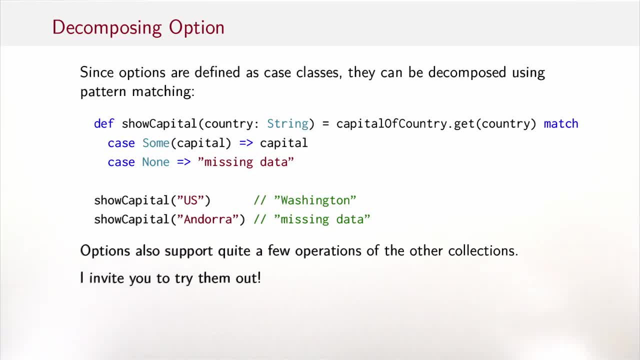 common to all collections is that I can add arbitrary data to a collection, Since an option has only zero or one elements. it's not a collection in that sense, But it supports quite a few operations such as map or fold or filter. I invite you to look at this color dog pages for option and try them out. 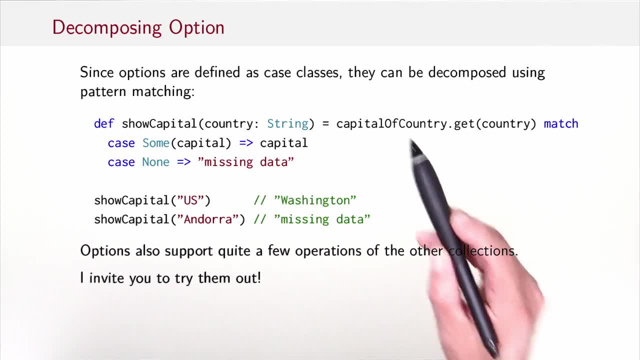 So you might ask: why does capital of country or any map really return an option in the get method? In some other languages it would return either the country or a null in case of a missing string. So why not use null? Well, it turns out that null is actually really dangerous, because if any value 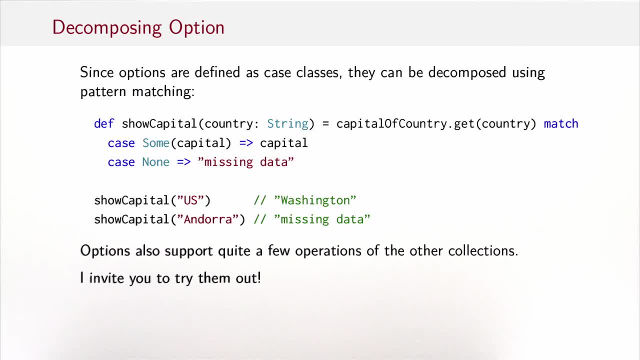 can be null, then you never know beforehand whether certain operations on that value are defined or not. If the value is null, you would get a null pointer exception. So that's why the inventor of null, that was Tony Hoare. he was also the inventor. 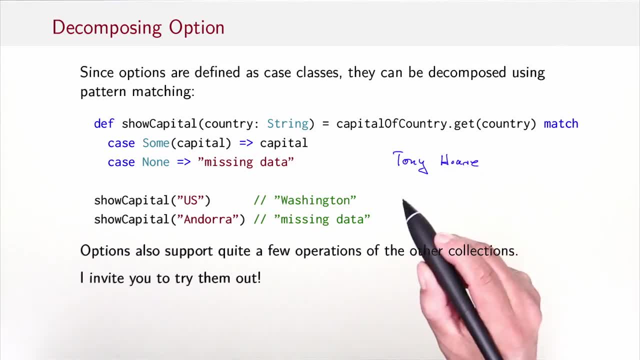 of Quicksort and many other things. So the inventor of null called it his billion dollar mistake. In Scala, null is actually available. We need it already for interoperation with Java, but it's generally considered bad style to use it. So this course will generally not use null and 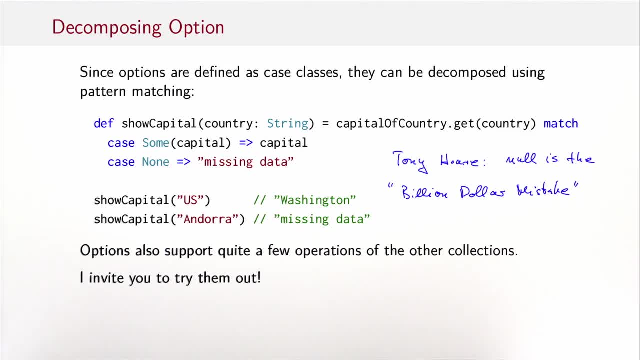 replace it with safer alternatives, such as option. So why is option safer than null? After all, in an option also, I mean I have either something or nothing. Well, it's safer because the types force you to handle both cases. So if you 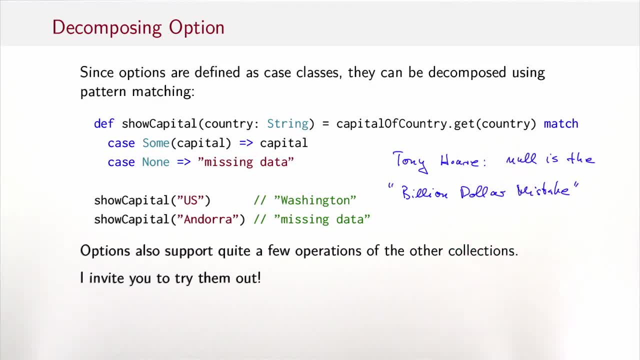 do a capital of country get country, then that doesn't pretend to be a string, It's an option of string and you have to process it further by typically pattern matching on the some case, And if you forget the none case, then the compiler will complain. 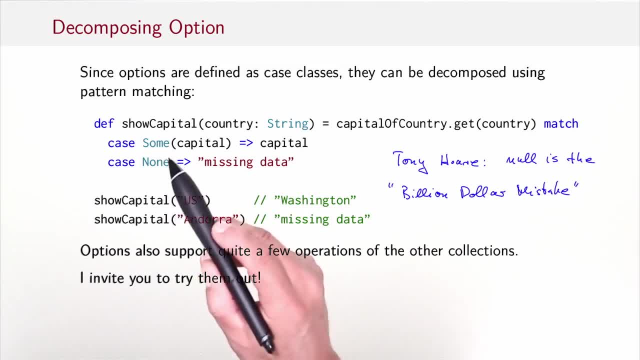 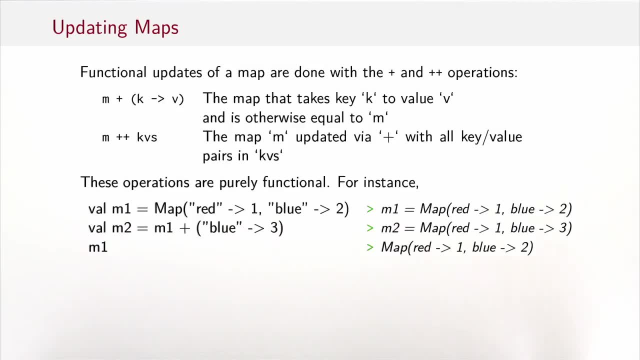 and say the pattern match is not exhaustive, So it will essentially nudge you to really handle both of the cases. That makes option so much safer than null. Back to maps. we've seen how we can query a map and how we can define a map from a sequence. 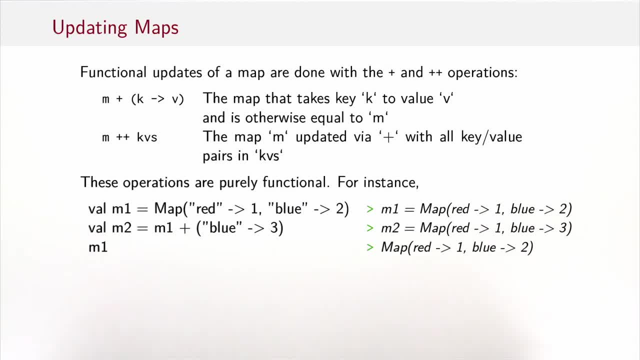 of key value pairs. But can we also update a map? In fact, yes, that's available, So we can have functional updates of a map and they are done with the plus and plus plus operations. So this operation here, m plus key value pair. 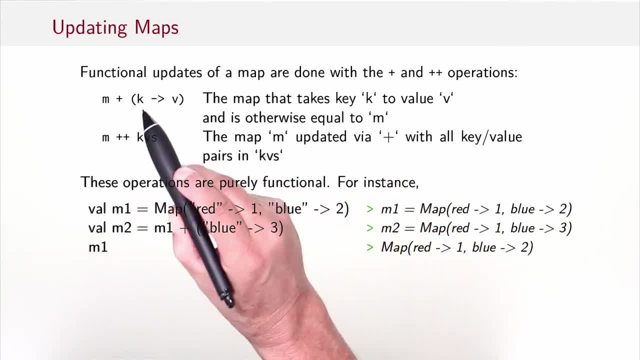 that would give you the map that takes key k to value v and is otherwise equal to m. So k might already be defined in m, in which case it will be overridden The new binding maps k to v, Or it might not yet exist in. 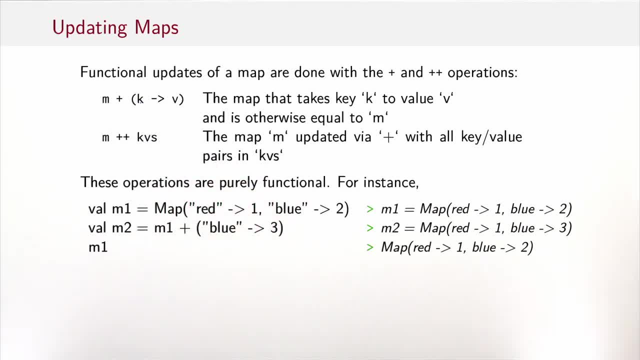 m, in which case we add a new binding for k. Then there's also a bulk operation: m plus plus key values. So that would update map via plus with all key value pairs that are given in the collection k vs. Let's go back to this. Then there's also a bulk. 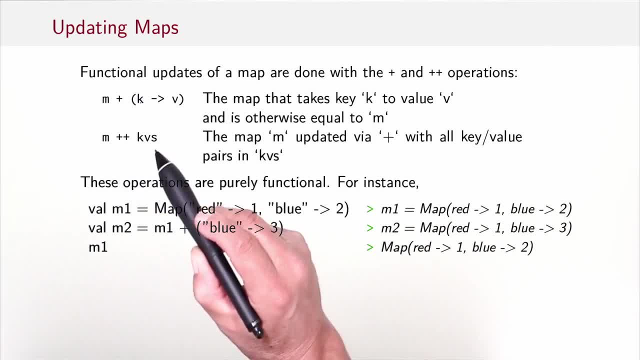 operation plus plus m plus plus key value pairs. So here k vs is itself a collection of pairs of keys and values and the map that gets then updated via plus with all the pairs in the k vs collection. So of course these operations are purely functional. They don't change the map m They create. 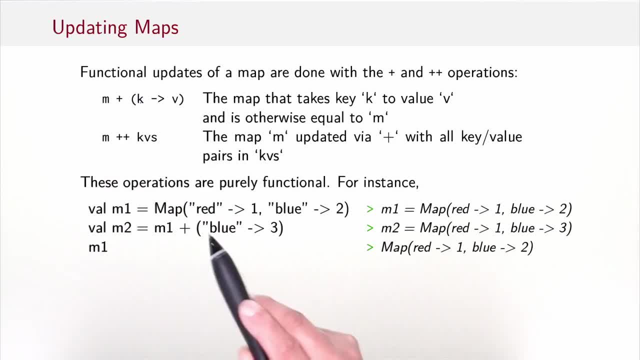 a new map. So, for instance, if I define a map m1, red becomes one, blue becomes two, And then I add blue becomes three to that map with a plus. Then I get the new map. Red becomes one, Blue now maps to three. 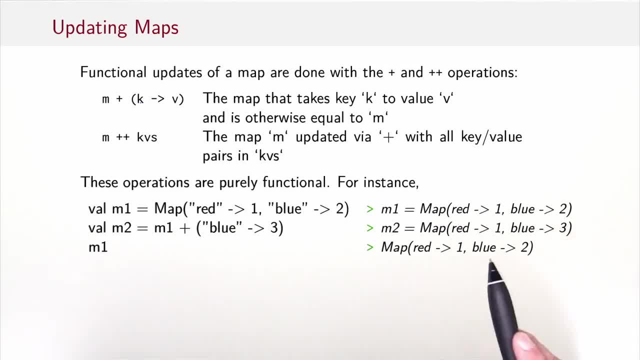 But the old map, m1, is still the same. Red becomes one, Blue becomes two. You might wonder how can we implement maps like that so that the old map stays in place while we update the new one? Well, for small sizes maps are just essentially single objects, and we do copy the whole object that holds for sizes. 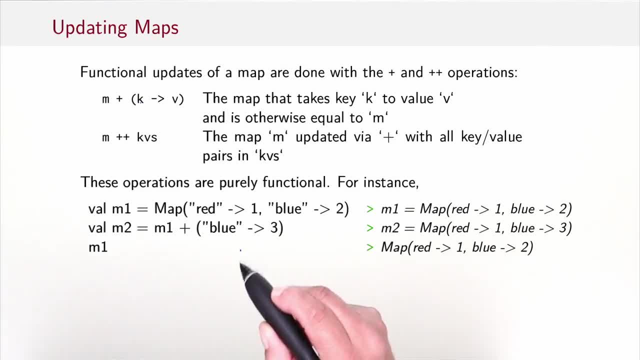 up to four And for larger sizes. what we do is we essentially use a scheme similar to the vector scheme. So we have essentially arrays of arrays of a shallow depth up to five, And in each array we have essentially key value pairs And we use a hash function to essentially 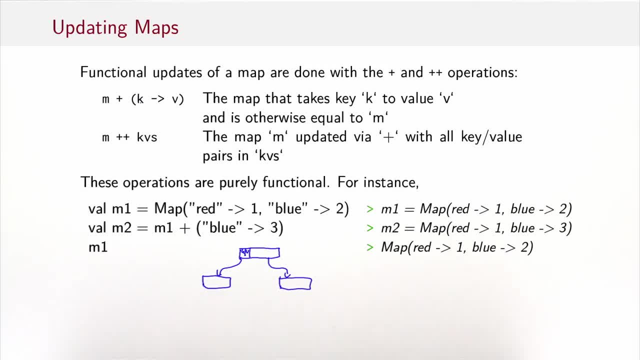 select either the right subarray or the right element in that array, Similar to vectors. if we update, we get essentially a log n update of these subarrays, where n is the depth of the tree. So basically we copy between one and five of these subarrays, which is still a reason. 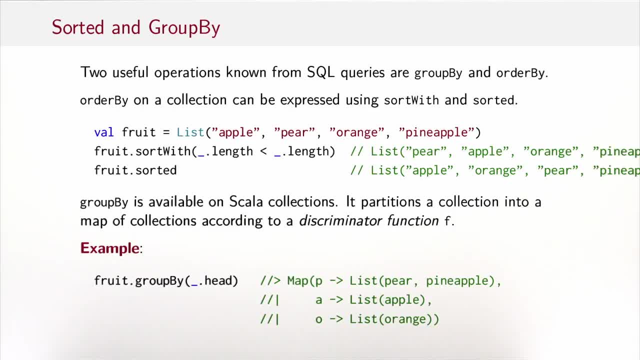 why we have a relatively bounded cost for updating a map. So if you know SQL from databases, then maybe by now you have realized that a lot of the collection operations we have really correspond to what you can do in these database queries as well. And that's no accident because essentially both of them are rooted in the same. 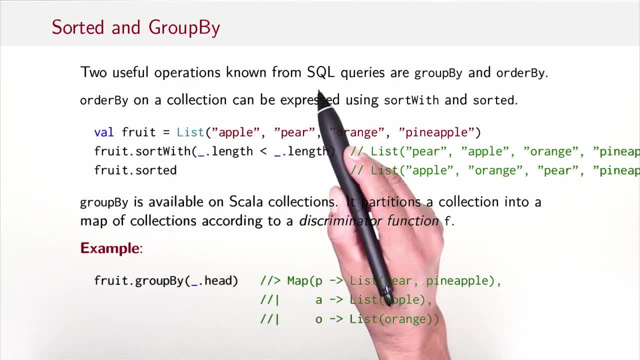 theory, relational calculus. So two other common operations from SQL queries are group by and order by. Order by. we don't have directly collections, but they can be expressed using the function sort with and sorted. So here I present them with an example. Let's say we have this fruit list. 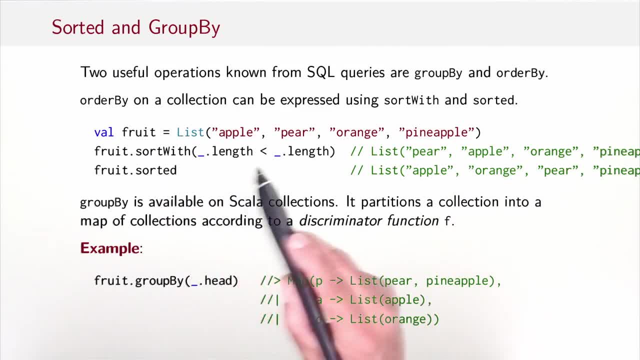 and then fruit: sort with underscore length, less than underscore length. So that would sort the list with the function that shorter strings appear first. Consequently, that would give you the list: pear, apple, orange, pineapple. There's also another function that is written sort. 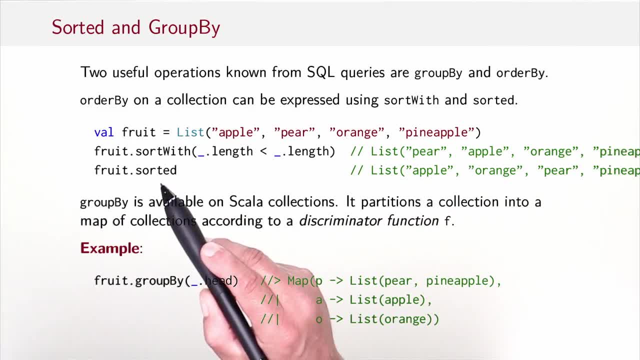 with and sorted So fruit dot, sorted sorts with the standard comparison function for the underlying type. Here the standard comparison function for strings is lexicographic ordering. So essentially we compare first the first letter, if it's the same, the second letter and so on. So that would give you this. 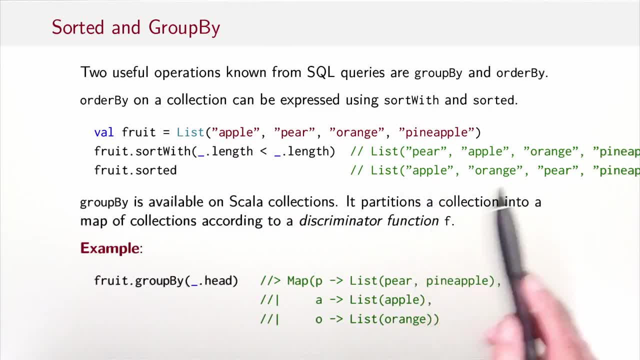 ordering instead. So here apple comes first because it starts with an A, then orange, pear and pineapple. So so much for ordered by, or rather sort with and sorted. What about group by? So group by is directly available on Scala collections. What it does is it partitions a collection into a map of collections. 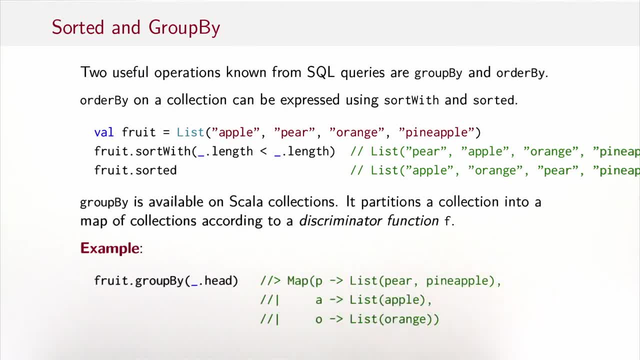 according to a discriminator function: f. So again, it's best explained with an example. Let's say we have the fruit list and we want to group it by its head. So that means we take the head of each element. Here we have an A, a, P. 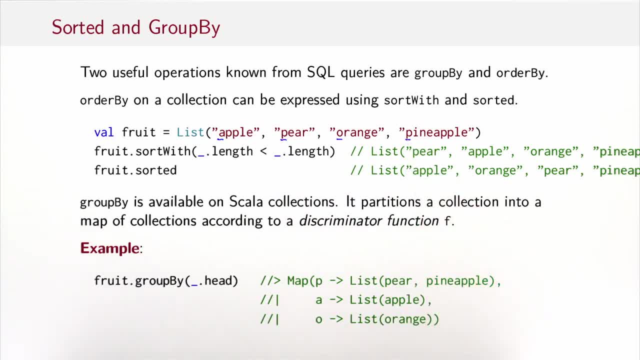 an O and another P And we create a map from these heads to the lists of original elements. So what we would get here is that P now maps to the list of pear and pineapple, A maps to a single element list- apple and O maps to a single element list- orange. 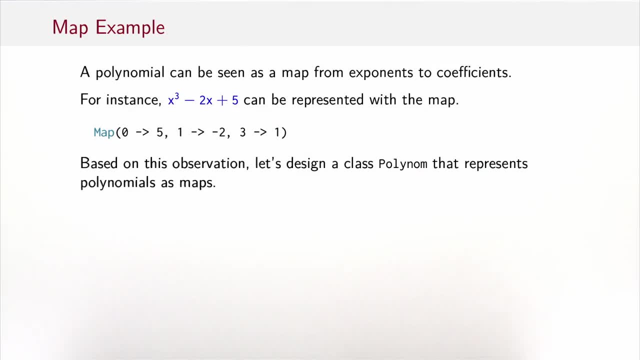 So let's use these operations in an extended example, which is to construct a class for polynomials. One way to look at a polynomial is as a map from exponents to coefficients. So, for instance, the polynomial x to the third minus two, x plus five could be expressed. 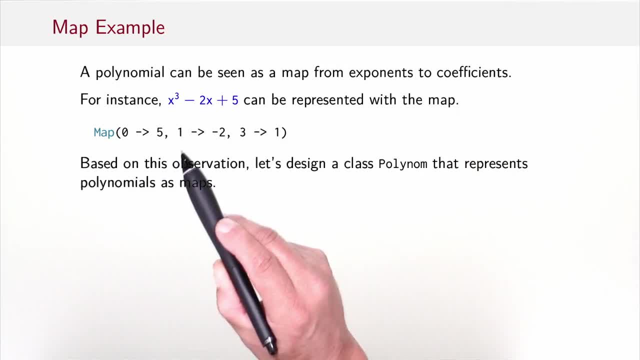 with the map that says: exponent zero maps to five, exponent one maps to minus two and exponent three maps to one. Based on this observation, let's design a class polynomial that represents polynomials as maps. In fact, there's one other operation that comes in handy to treat this use. 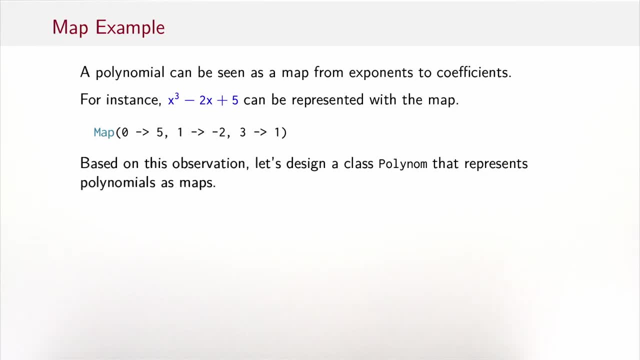 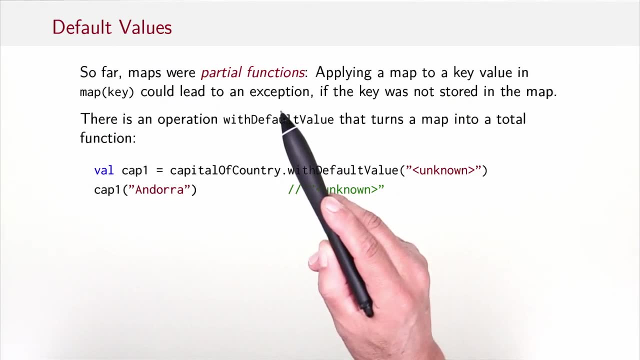 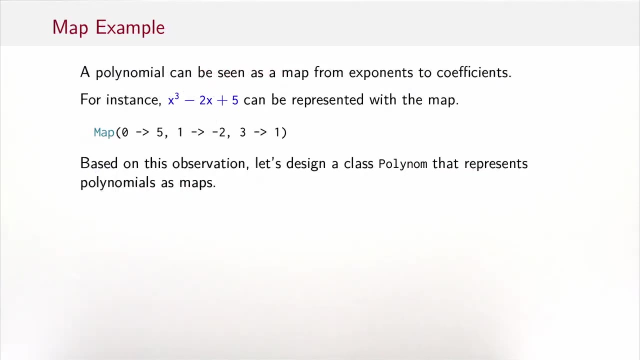 case and that has to do with default values. So we've seen that previously maps were partial functions. Applying a map to a key could lead to an exception if the key was not stored in the map. But for polynomials that's actually not very useful because we could say: well, it does make sense. 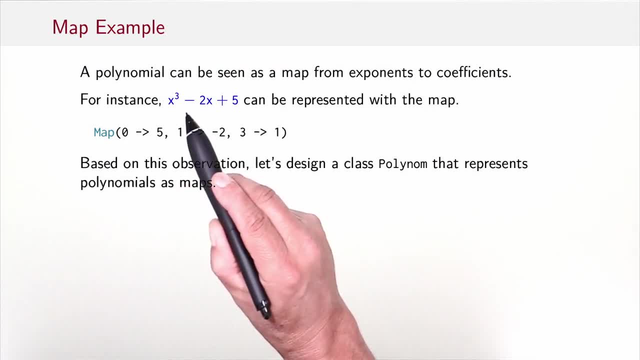 to ask: well, what is the exponent two coefficient for a polynomial? even if it's not given, you could just say it's zero. So basically you could say x three plus zero, x two is the same thing as x to the third. So we can treat missing coefficients as 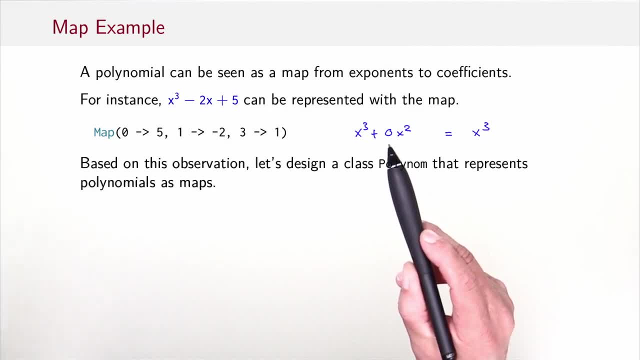 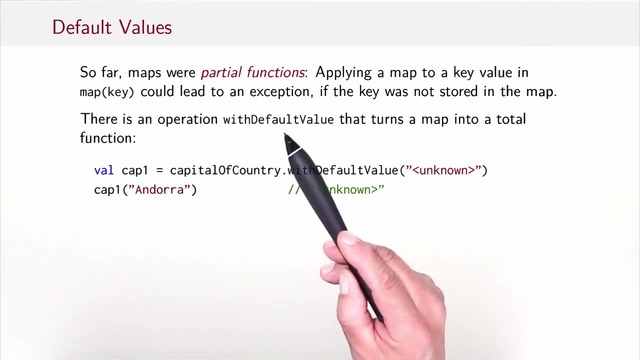 just coefficients of zero. So the fact that these maps are partial and might fail is actually inconvenient. We would like the map to just give us back a zero for the cases where it's not defined, And we can do that with the operation with default value. So the operation with default value turns a map. 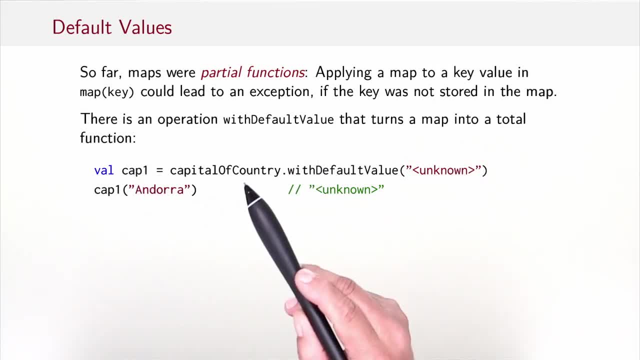 into a total function. So here we have capital of country. that was a normal map that could fail and we can give it the default value, or we can create a new map. rather that is the old capital of country map, but now with the default value unknown. 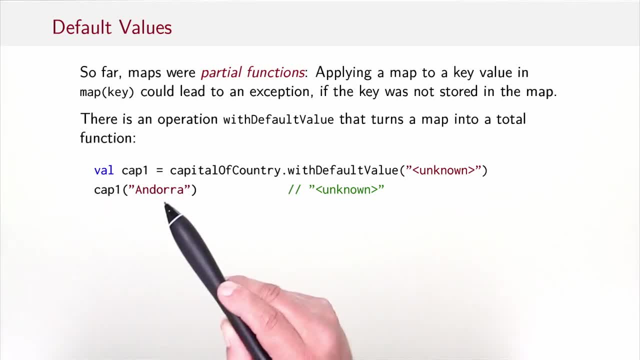 And that means we can now apply cap one to Andorra directly, and we would just get back the string unknown instead of an exception that an element was not found. So with these tools, I think we have enough now to embark on the design of the polynomial class. Okay, so I've given you the outline of 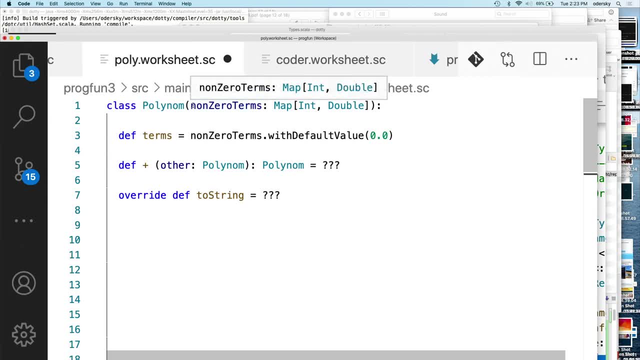 the class polynomial. It takes a map from int to double as parameter, which is a normal map, which I call here non-zero terms. So that's essentially that's the terms consisting of coefficient and exponent that are not zero. So the map maps the exponent. so 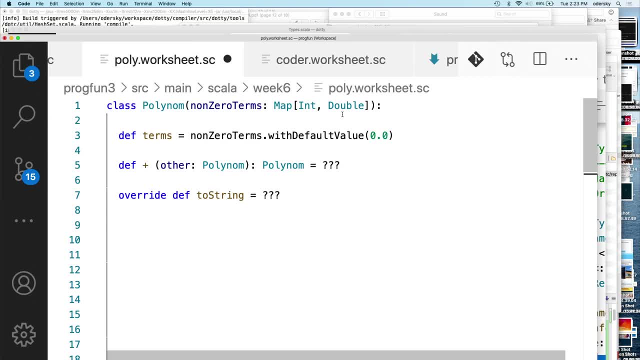 zero, one, two, three and so on, to the coefficient, which is a double number. Then we have the terms, which is non-zero terms, with a double number, which is the default value of zero point zero, and that could, should actually be a vowel, because we probably use it several times. Okay, then we want to: 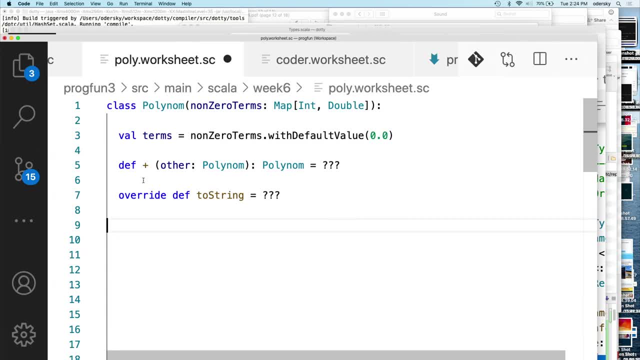 define two operations: One is the addition, so that adds two polynomials, giving a polynomial, and the other is two strings, so that should print or show a polynomial in a nice way, in a nicely formatted way. So let's do two string first. So let's start with something really simple. Let's say the two string. 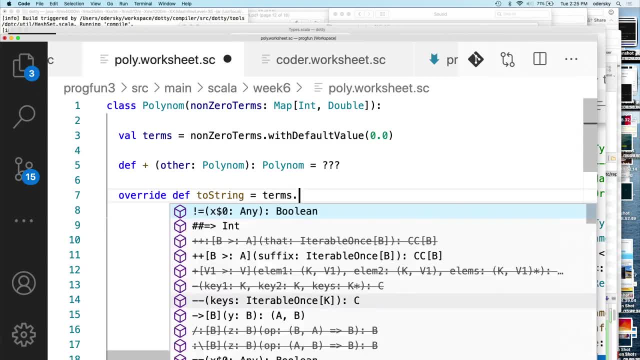 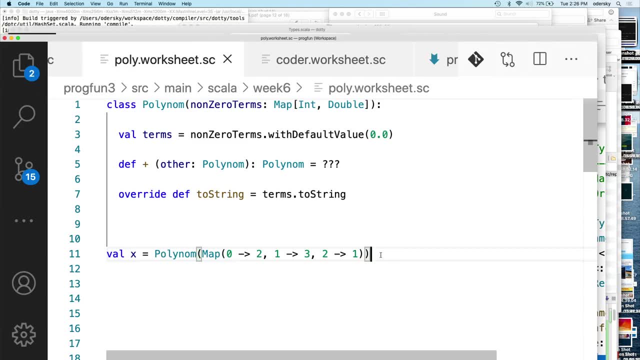 of a polynomial is this two string of its terms: map. We can test it by creating a polynomial- Let's say this one here, And then it would indeed print us the map in the way we would expect it. But that's of course not very nice, because the 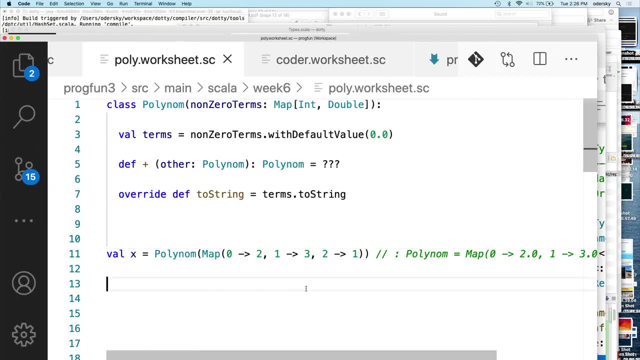 two string method exposes the internal implementation of a polynomial in terms of a map. So you would rather want to see something that has recognizable coefficient and exponents. So how do we do that? So one thing we could do is first define the right coefficient exponent pair for each of the 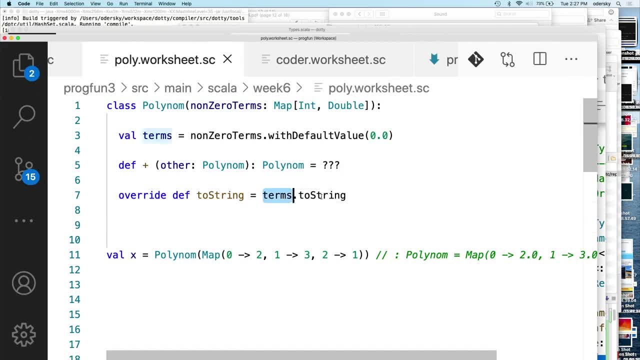 terms that we have in the map and then essentially create a string that just concatenates them all with pluses in between. So let's do that, So we can improve that, by taking each of the terms of the polynomial, printing that out as an exponent coefficient pair and then concatenate. 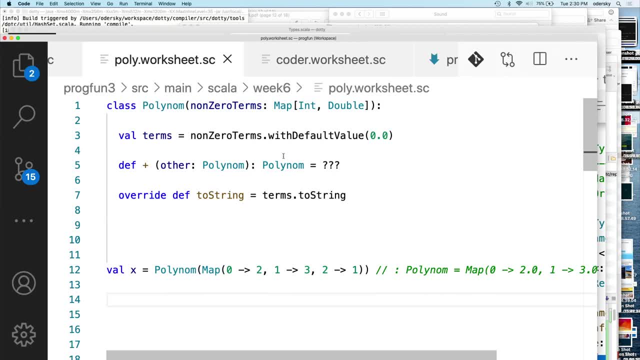 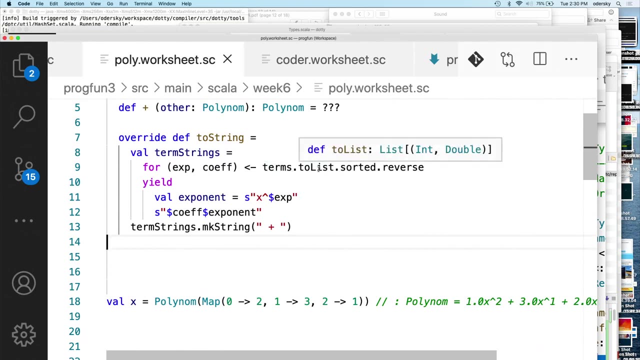 all those strings with pluses in between. So let's do that, I'll delete the old version and I write the new one here. So what happens here is: we take the terms, we map it to a list, we sort it so that gives. 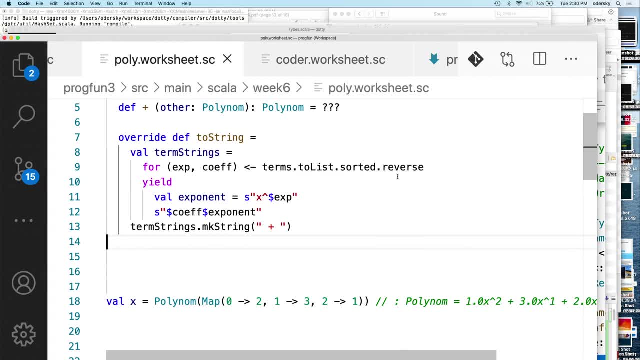 us the lowest exponents first, and then we reverse the sorted list so that gives us highest exponents first. So now we let exponents in coefficient range over those terms and we print the exponent as x up arrow exponent and we print the coefficient as it is and then we 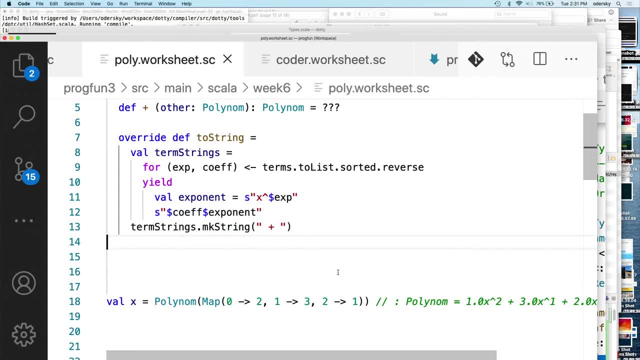 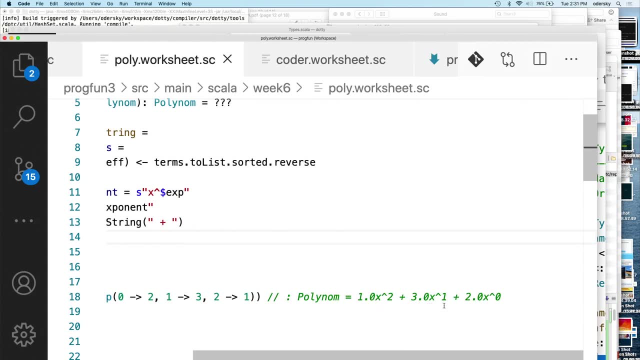 concatenate the whole thing with pluses in between. So now my polynomial would read like this: 1.0x to the second, plus 3.0x to the first, plus 2.0x to the zeroth. Now there's room for improvement, in particular. 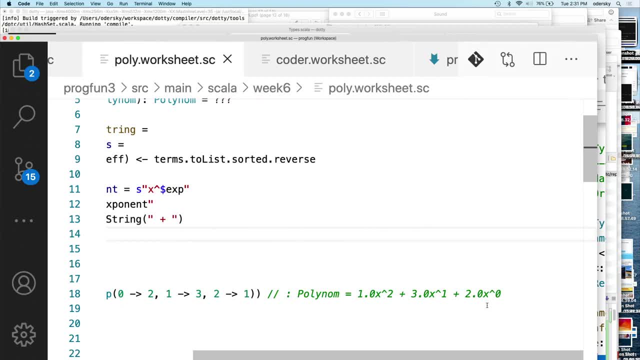 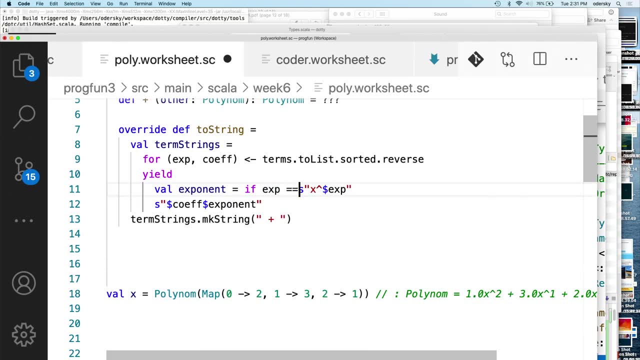 x to the zeroth, that's one. So we typically don't print that. So let's try to change that So that would simply say: if exponent equals zero, then we don't print an exponent and otherwise we print that, So that one looks better now. 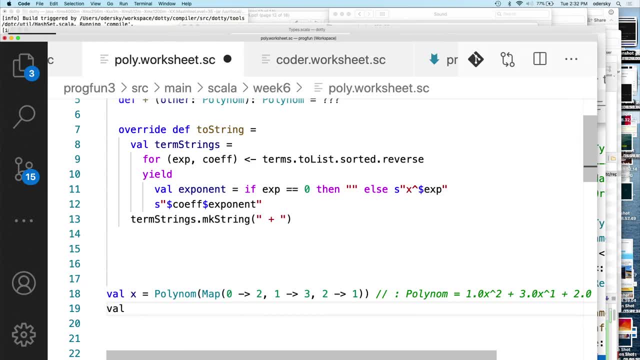 Another thing to improve would be what happens if we take the zero polynomial? So that would be the empty map, no coefficients at all, And that would give us the empty string, which is not ideal. So what do we do about that? Well, we have to create another special case. 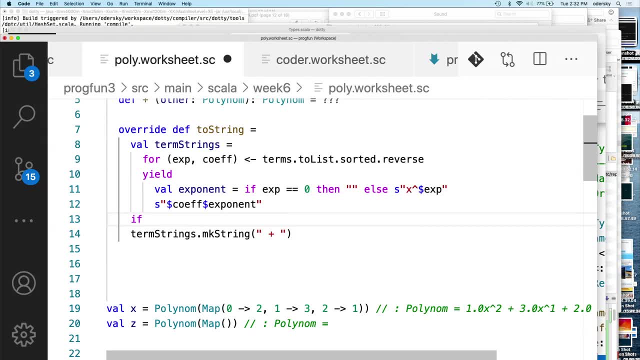 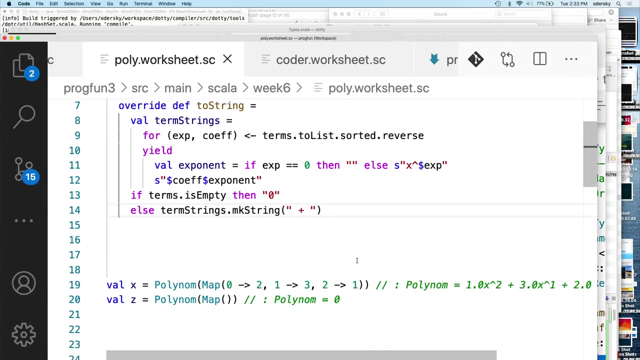 and say: well, if the term map is empty, so no coefficients at all, then let's print a zero as the only element and otherwise print term strings, mixed string plus, as before. So now we have handled that as well. A third improvement I leave up to you. it's a little bit more involved. 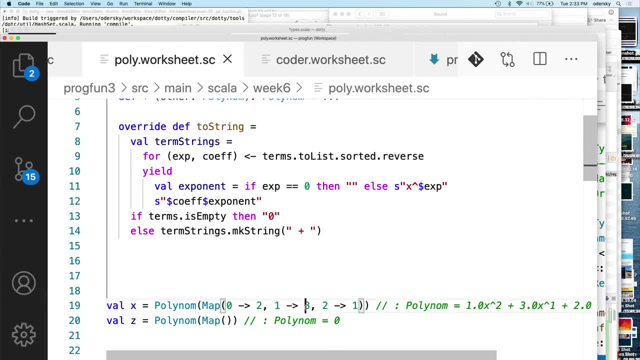 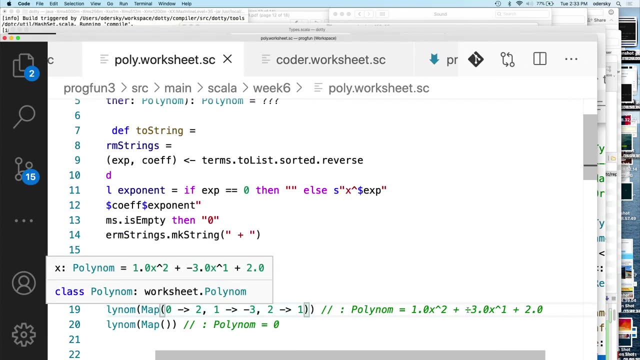 would be to handle negative coefficients gracefully. So let's say I have actually minus 3 here. What would I get? Well, I would get plus minus 3.0x to the first, which is legible but which could be improved by essentially removing the minus here. 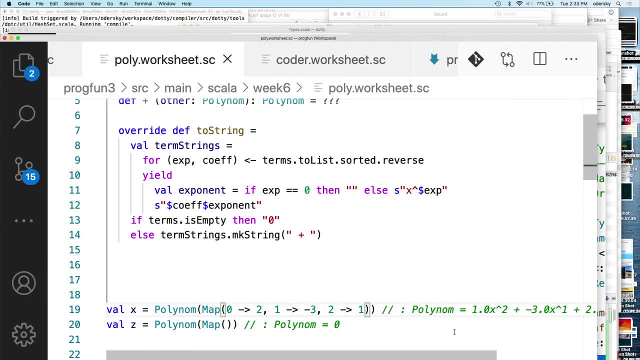 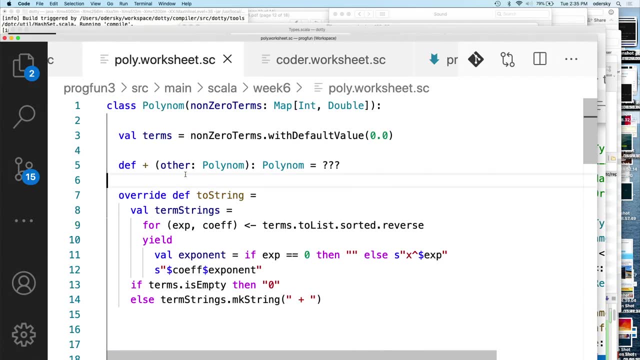 and changing the plus with a minus. So that's a little bit more involved and I leave that up to you as a polishing exercise. So let's turn now towards the plus operation To add two polynomials. we have to combine their terms If a term has an exponent which is only 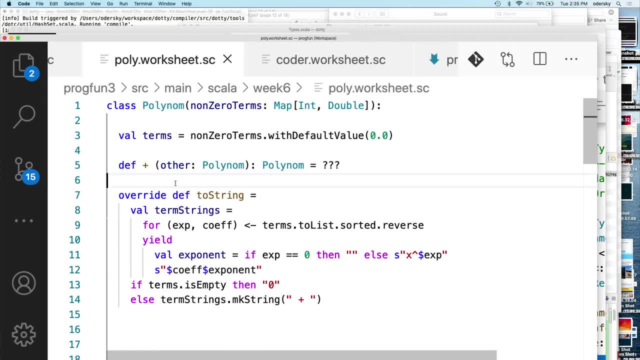 in one of the polynomials, we can just keep it like it is in the result. But if a term has an exponent that figures in both this polynomial and the other polynomial, then we have to add the coefficients. So here's a way to do this. 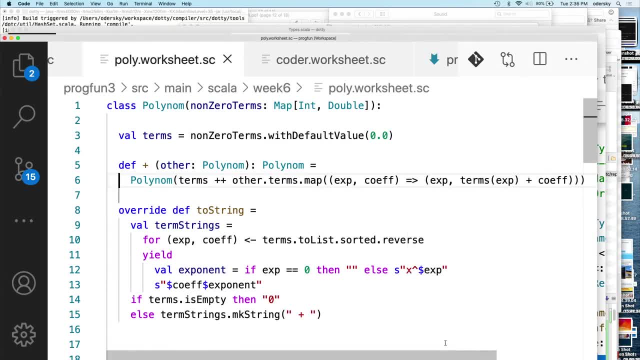 So let's analyze this expression in detail. So if we return a polynomial, it takes a map. The map contains the current map terms updated by this other map, And this other map is the terms of the other map that are then mapped, so that if we have an exponent with coefficient in this other map, 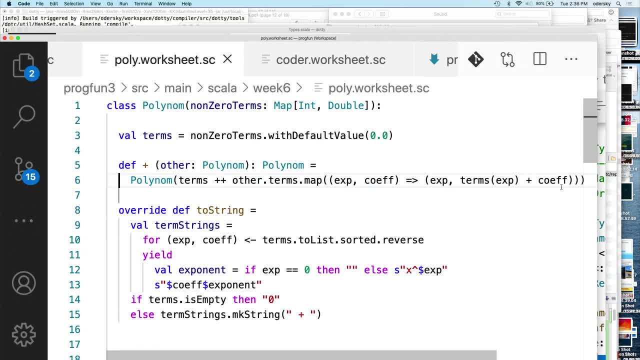 then we take the exponent and the coefficient plus the value of the current map terms at this exponent. So we add up the coefficients of both maps And we do that for all terms that are in both this map and in the other map. If a term is only in the other map, then terms of exponent would be zero. 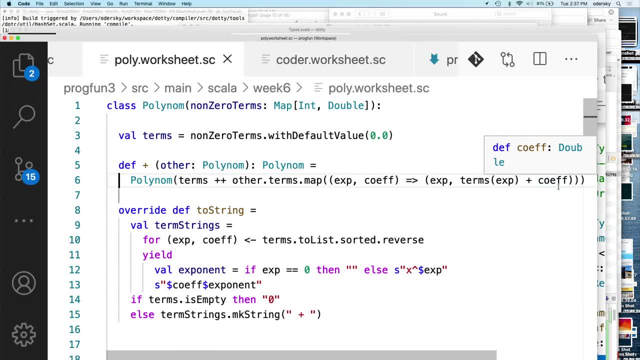 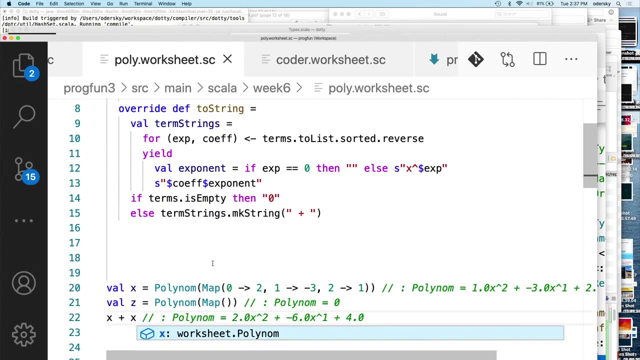 So that would effectively return exactly the same term that we had in the other map, And if a term is only in terms, then that wouldn't be updated. So again, it would stay as it is. So we can test the operation by just, for instance, taking x plus x or x plus x plus zero. 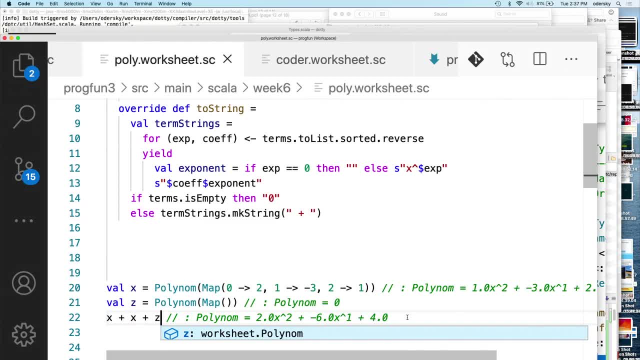 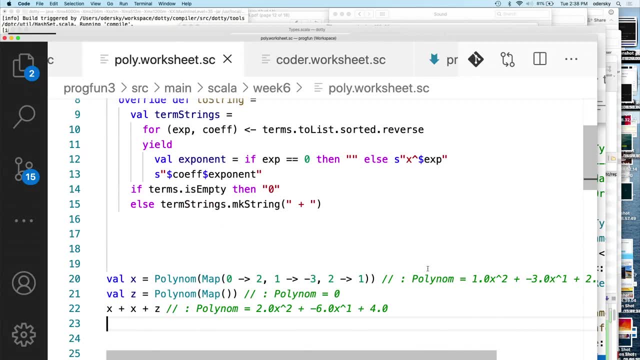 And that would give you the polynomial that has all coefficients doubled, as expected. So there's one further refinement I'd like to do. It's a bit awkward to have to write polynomials like this because again it exposes the implementation strategy. Implement polynomial in terms of a map. 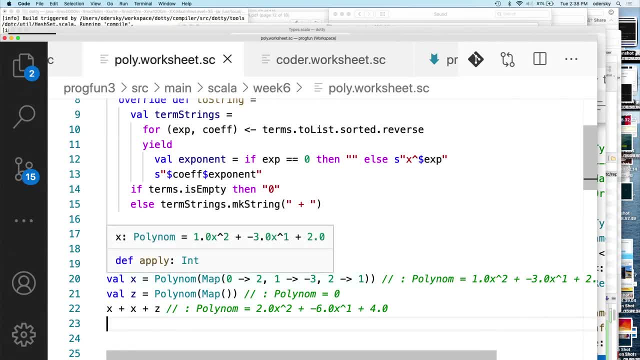 And second, there's this nested call- polynomial of map- where it should be clear that if we want to create a polynomial, we want to create it with just, essentially, the elements that are here. So the question is, could we get rid of the map call like this? 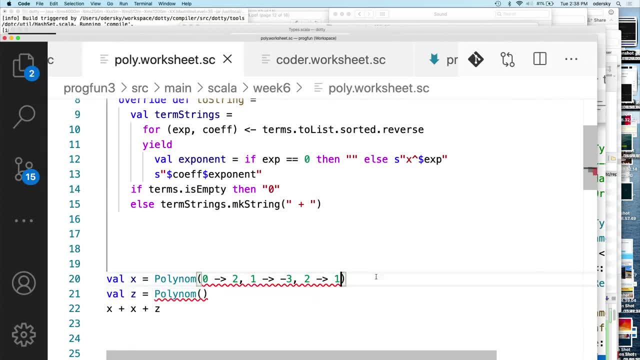 and write polynomial like that. For the moment, of course not, There's not an operation. So it said: well, it found the three int pairs and it needs a map. So what we can do is we can give a map a secondary constructor. 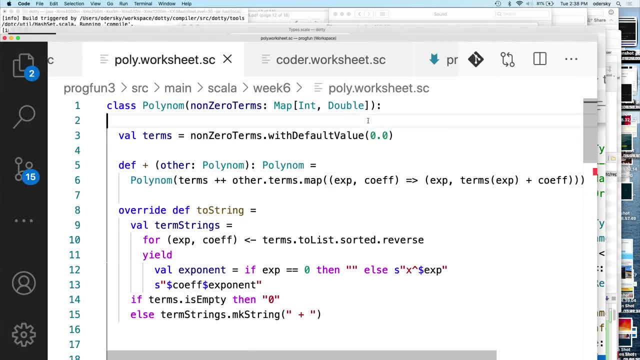 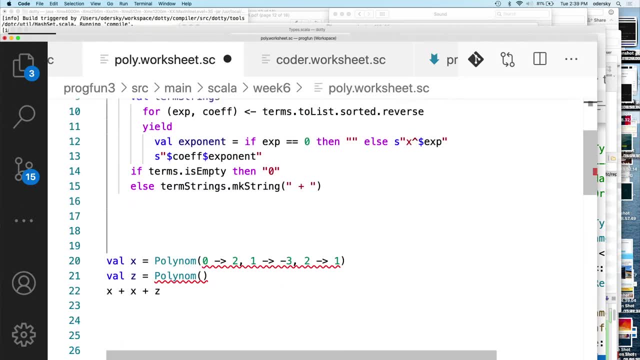 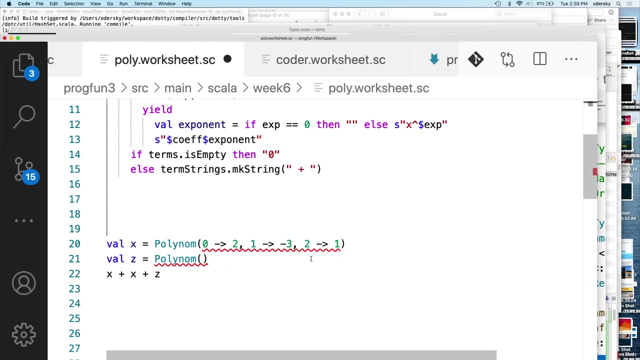 that would work with these parameters. So what we would do here is we can define a secondary constructor, this And that would take. well, what would it take? The problem is that we have to deal with a varying number of parameters. A polynomial could have any number of terms that should be given in this parameter list. 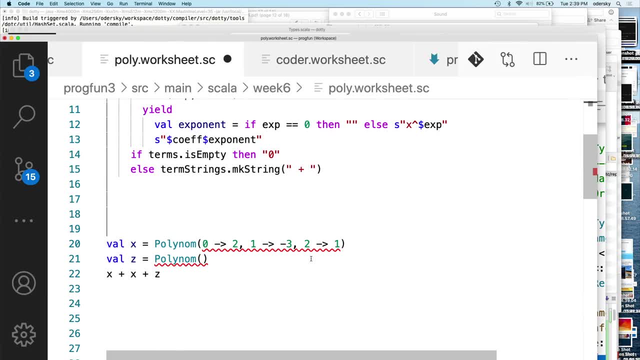 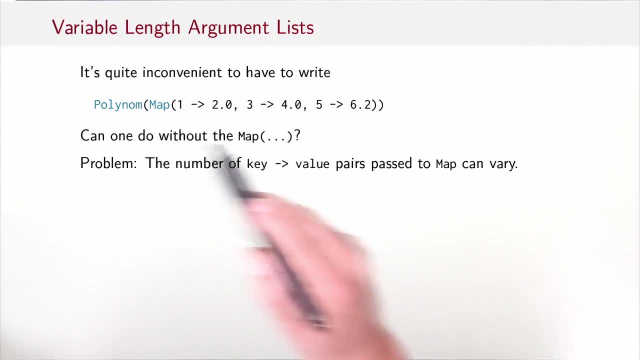 So for that we're going to introduce another language feature of Scala that you haven't seen yet and that's vararg parameters. So we've seen that it's quite inconvenient to have to write polynomial of map everywhere. Can one do without the map? 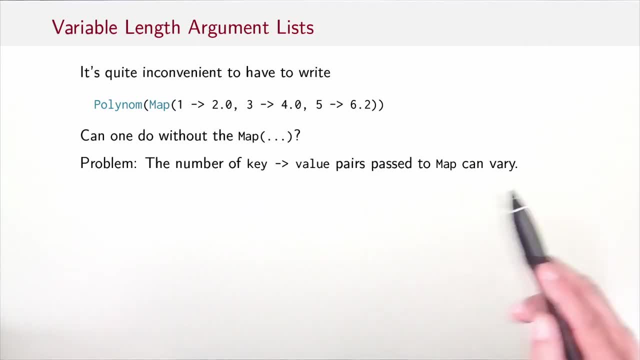 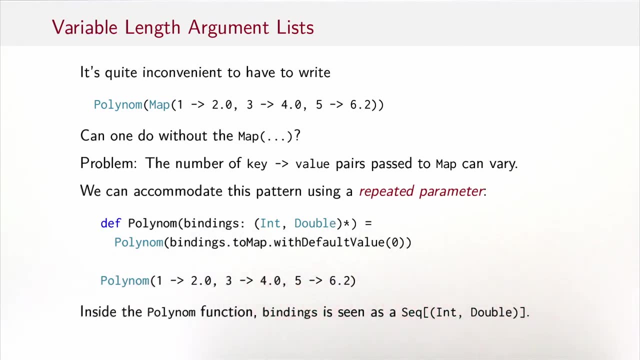 The problem is that the number of key value pairs passed to map can vary, But we can accommodate this pattern using a repeated parameter. So the idea here is that we can give a definition bindings that takes a list of int doubles, So this list is represented by the star here. 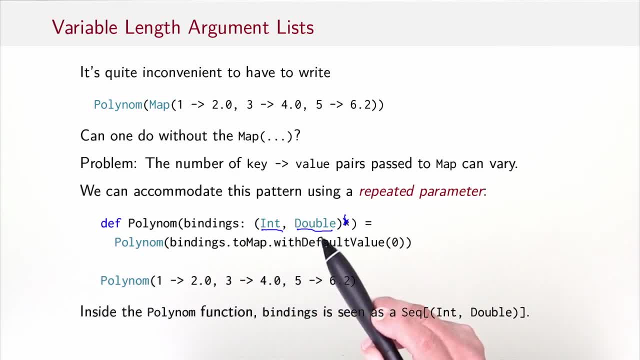 So vararg parameter is given by a parameter type followed by an asterisk, And what that gives internally is a sequence, And what we can do then is essentially convert the sequence to a map. There's a handy to map function for that. Give it a default value: zero. 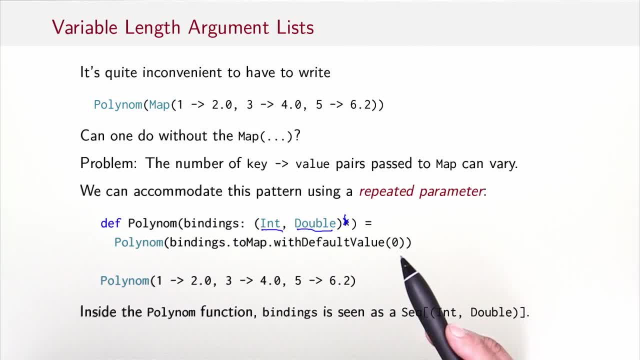 And that would essentially create a polynomial with the correct map. And if we do that, then we could write polynomial of and then just the bindings, like that. That's just three pairs And so that would match this type int double star And that would invoke this method. definition of polynomials. 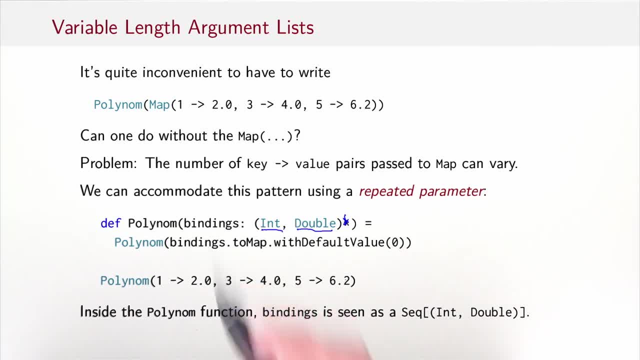 So inside the polynomial function the bindings here are seen as a seek of int and double. So generally a vararg parameter, a repeated parameter like this, generates a sequence of the element types that precede the asterisk. So back to the worksheet. 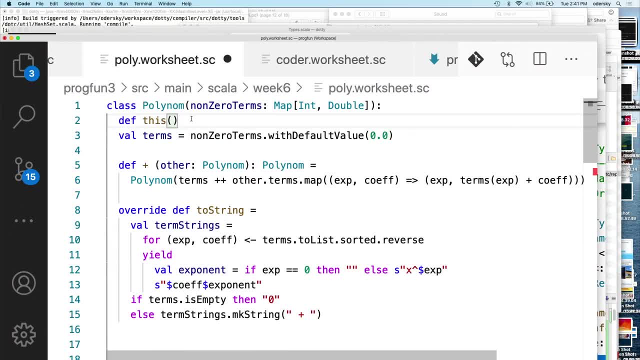 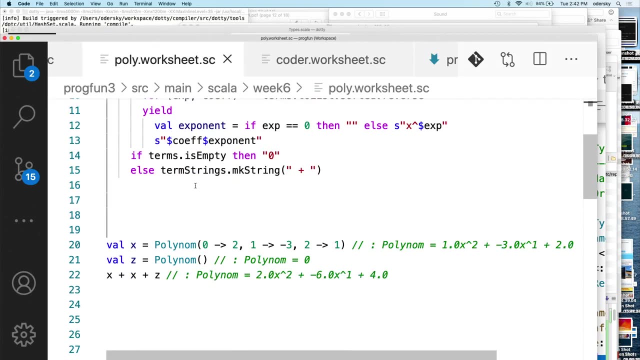 In my worksheet I'm going to do it slightly differently. So instead of creating a separate def that creates a polynomial, I create a secondary constructor directly, So it would be bindings And that would say So with that secondary constructor. now we see that our polynomial syntax works. 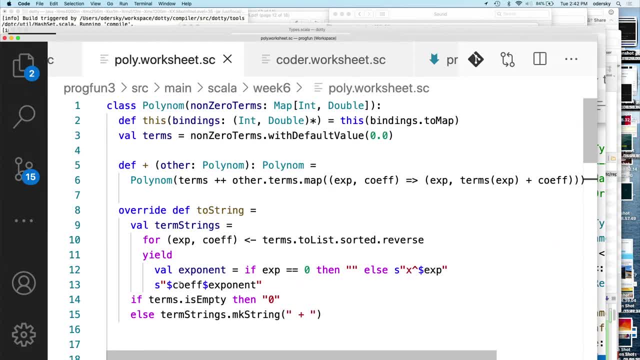 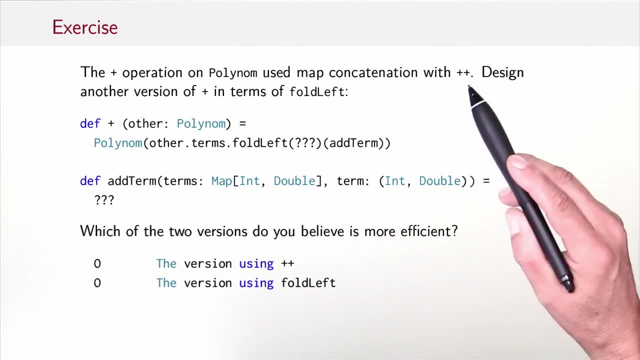 and we don't need the intermediate map anymore. So here's an exercise for you: The plus operation on polynomial used map concatenation with plus. plus Design another version of plus in terms of fold left. So that version would look like this: So plus takes another polynomial, creates a polynomial. 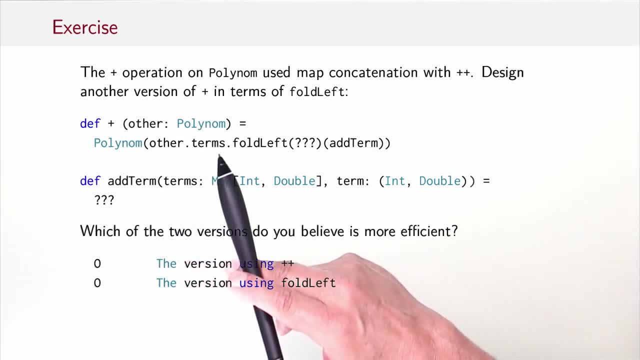 and it essentially folds the other terms with something that you have to fill in and an add term method. So the type of the add term method is known from the outline here. So it would have to take a map of int and double and a term which is an int and double. 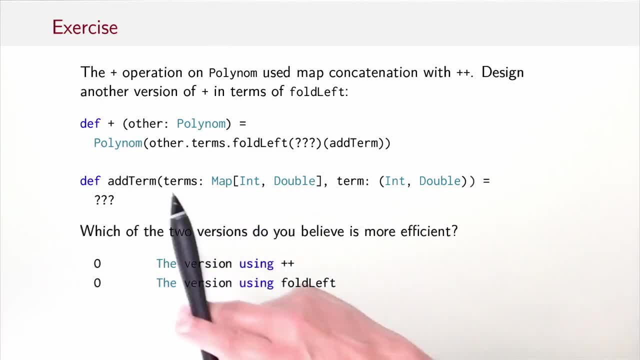 and would have to create the map that consists of the terms map plus the additional term, So overwritten with the additional term. So once you've solved the exercise, then try to answer the following question: Which of the two versions do you think is more efficient? 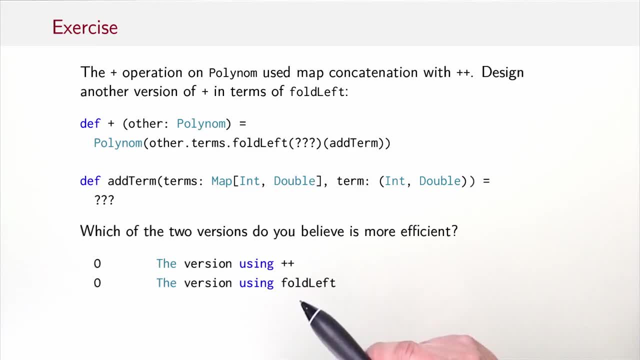 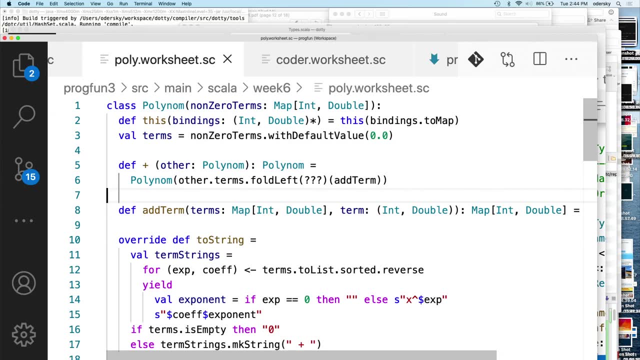 The previous version using plus plus or the version using fold left. So I've added the outline from the slide to the worksheet. We have the plus operation, which is defined in terms of fold left, and we have the add term operation, which also remains to be defined. 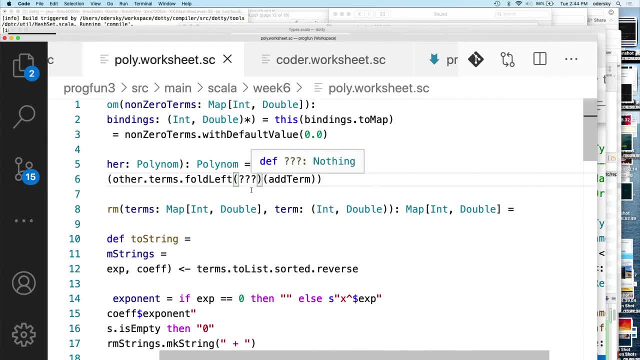 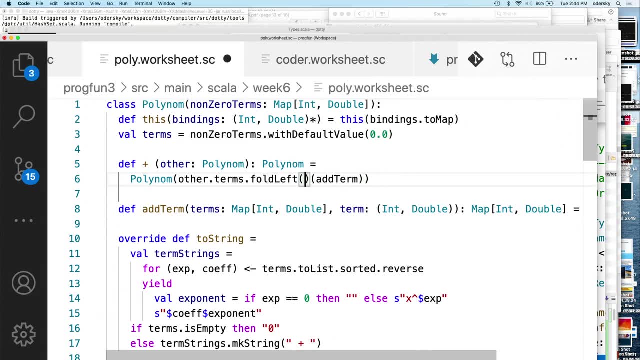 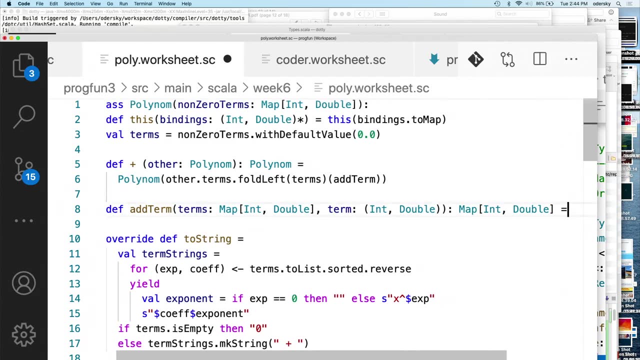 So let's try to fill in the triple question marks here first, If we do a fold left. so what's the map we start with? Well, that's, of course, the map, the our own map. So that would be terms. Okay, and how do we add a term to a map? 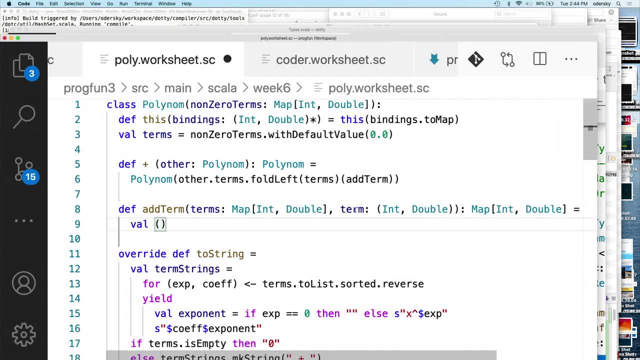 So one way to do it would be to first decompose this term So we say, okay, we know that's the exponent and the coefficient, That's my term. This just gives me a handy way to talk about the two parts. And then it would be what? 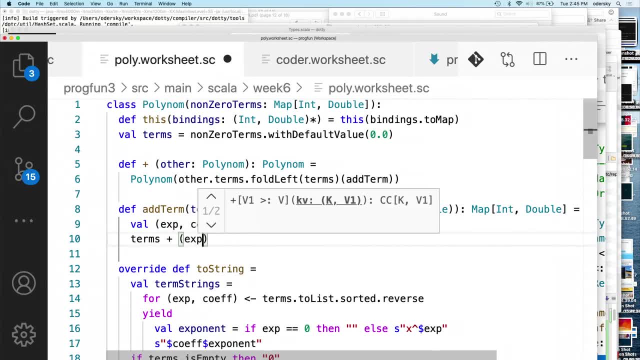 It would be terms plus the exponent maps. to what does it map to? Well, the terms of exponent, what I have in the current map, plus the coefficient that I have given here, And that should be it. So let's see whether my examples still work. 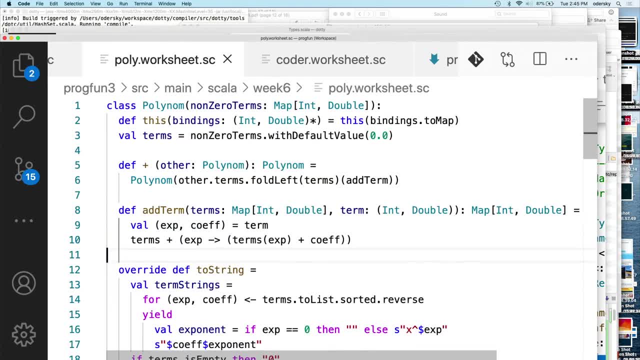 Yes, everything still works. So, judging by these tests, the new implementation of plus is equivalent to the old one. But is it faster or slower? What's the answer here? Well, I would think it's probably faster. So the reason is that with the new implementation of plus, 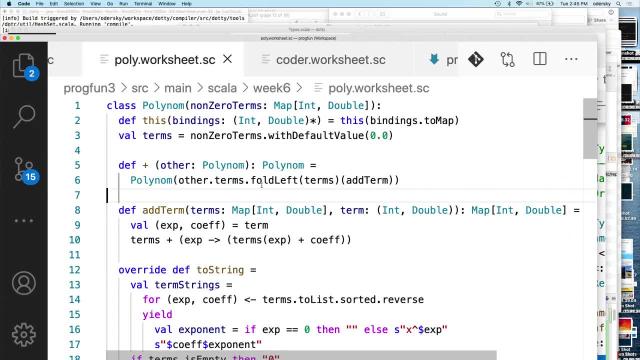 essentially we go directly on the terms and we do a single scan with the fold left. We add essentially each term in a single scan, Whereas the previous implementation that built up a map of all the common terms, and building up a map is costly- then we are left with two maps and then the maps were essentially folded with plus plus. 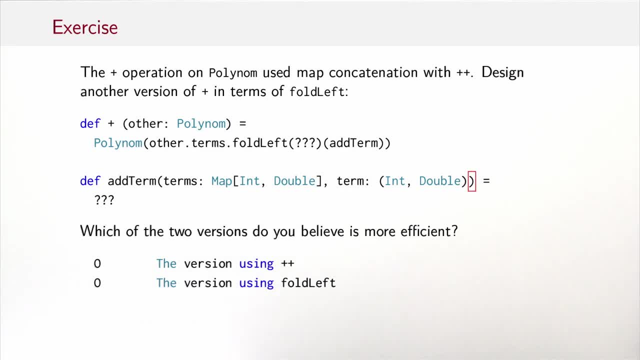 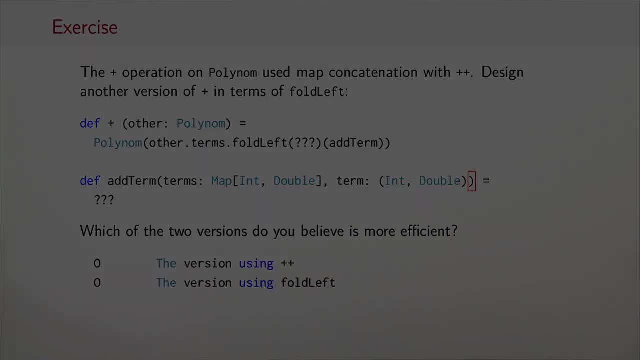 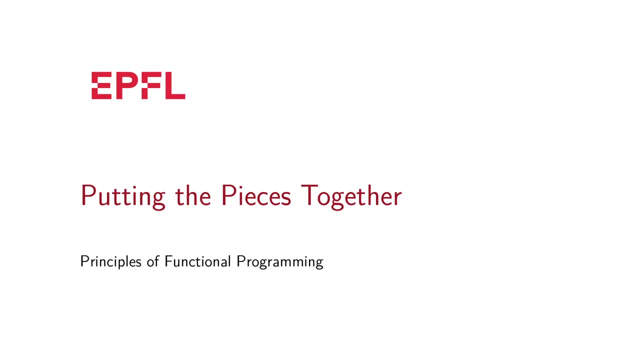 So this intermediate step to going through a second map probably costs some time, So I would imagine that the fold left version is faster than the other. So to conclude this week, let's put the pieces together. You're going to use what you've learned about collection operations. 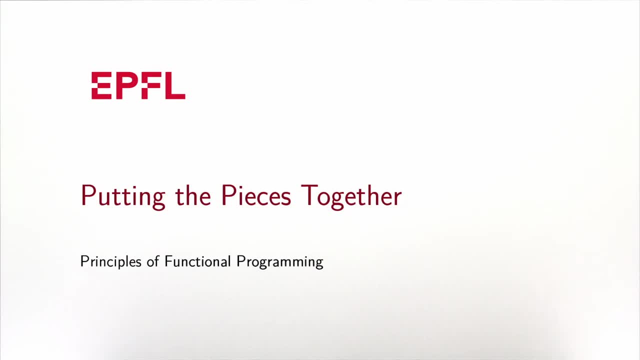 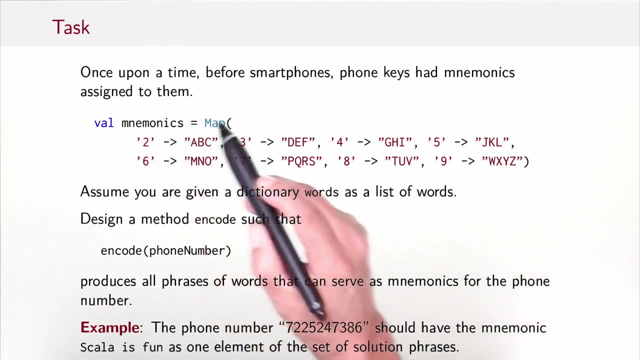 together with some of the other functional techniques, to solve a non-trivial programming problem. The task you want to solve is the following: Once upon a time, before smartphones, phone keys had mnemonics assigned to them. The mnemonics were always the same. 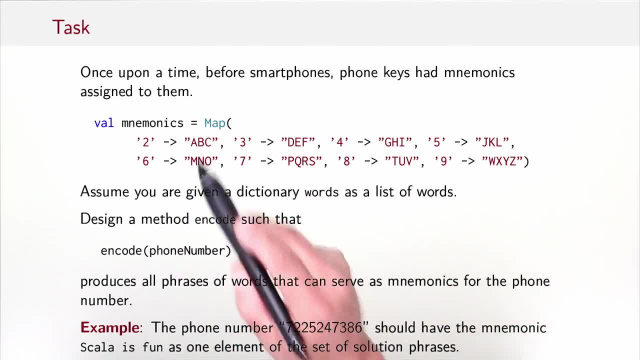 so each digit from 2 to 9 had a string of 3 or 4 letters assigned to them. The purpose of these assignments were as a way to remember phone numbers better. So, for instance, if I wanted you to remember the phone numbers. 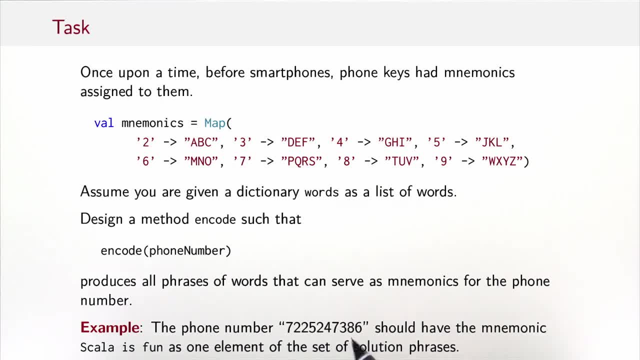 722-524-7386,. I would have to come up with a phrase that you could type, or rather, you would type the digit corresponding to every letter here, and that would then, in the end, give you the phone number that we wanted you to dial. 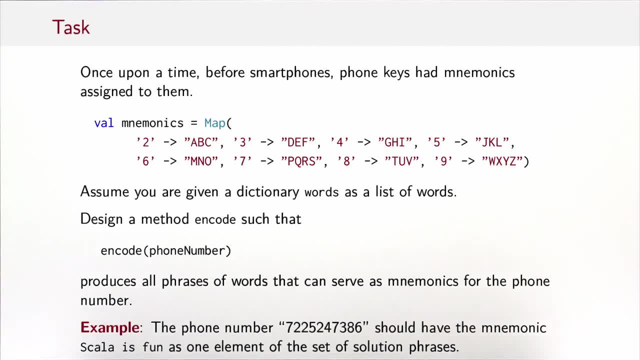 The point of this map was as a help to remember phone numbers. So, for instance, if I wanted you to remember this very long phone number here, then I could have given you a number or I could have given you a phrase instead. In this case, maybe I could give you the phrase. 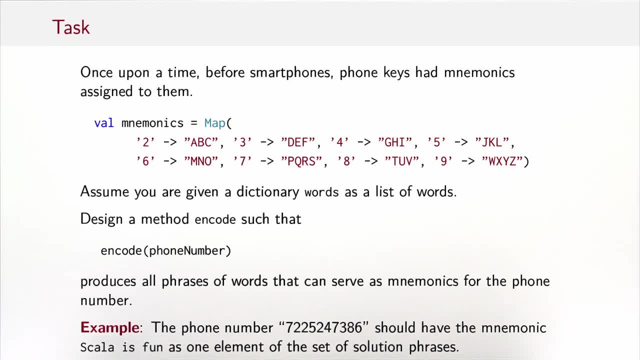 Scala is fun, And the idea then is, you would just essentially type out the letters instead of the digits. So you would type the letter S: well, that corresponds to the digit 7, so that gives you the first digit of the number, and SC and A would both map to 2,. 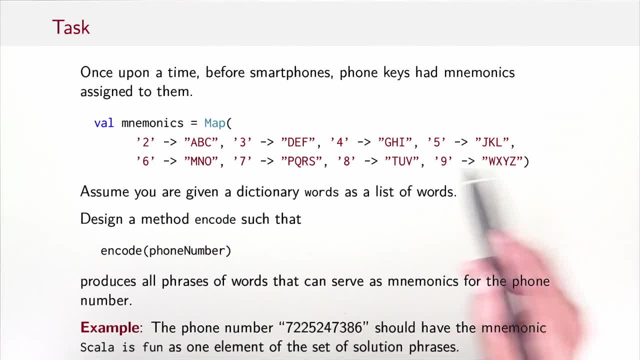 so that gives you 22,, and then L would map to 5, and so on. so you get the principle. It's easier sometimes to remember that than to remember a phone number, And of course at about the same time that phones had these mnemonics. 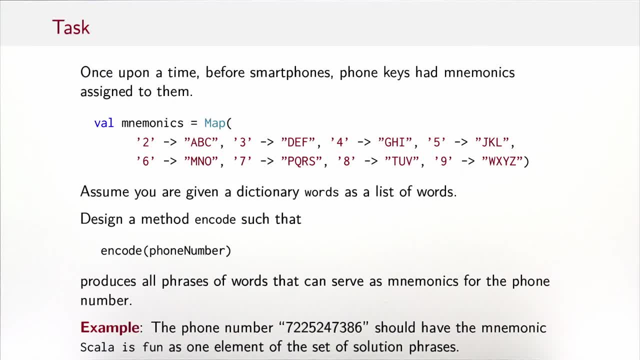 there were no URLs or internet addresses, so the way to contact a business was to dial a phone number, and that's why there were a lot of radio ads or other things that gave you essentially these mnemonic strings instead of the real numbers, which nobody can remember. 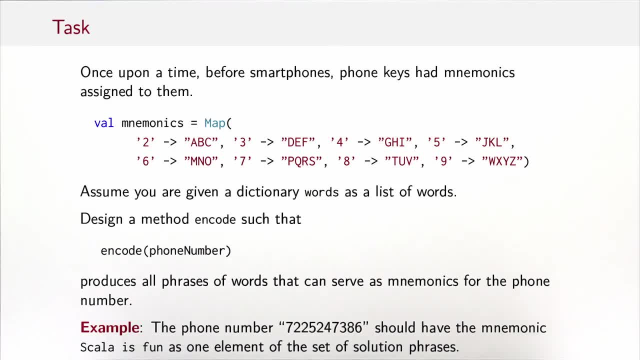 Okay, so the aim now is that you're given a dictionary of words that you can use and a phone number, and you should encode the phone number that gives me all phrases of words that can serve as mnemonics for that given number. 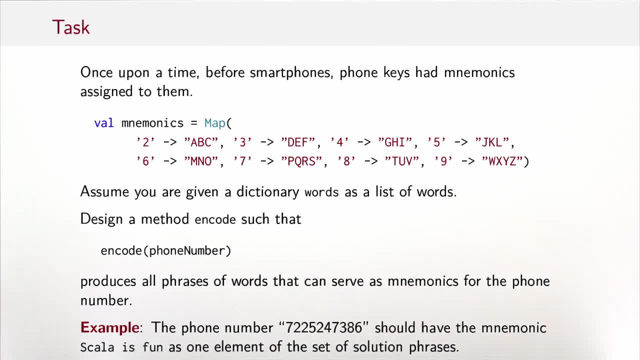 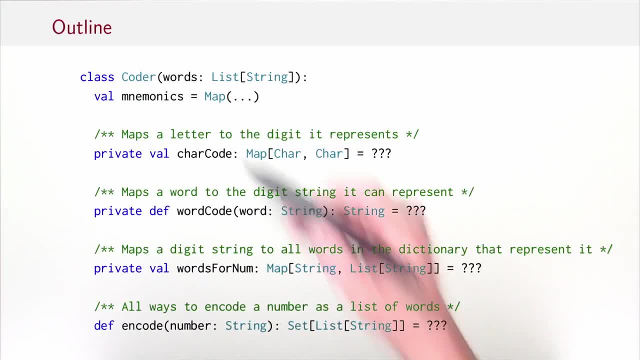 Typically there would be more than one phrase. I want them all so that I can pick the one which is nicest or cutest or most easy to remember. So I've given you the outline of a class to do that here and we are going to proceed to the solution in four easy steps. 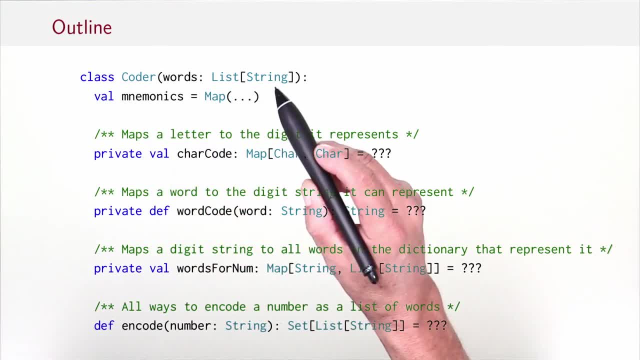 So the class is a class coder. It contains the dictionary, which is a list of strings, as a parameter. It has a field- mnemonics- which is exactly as it was given here, so I haven't bothered to repeat the definition. And then we have four methods that we should implement one by one. 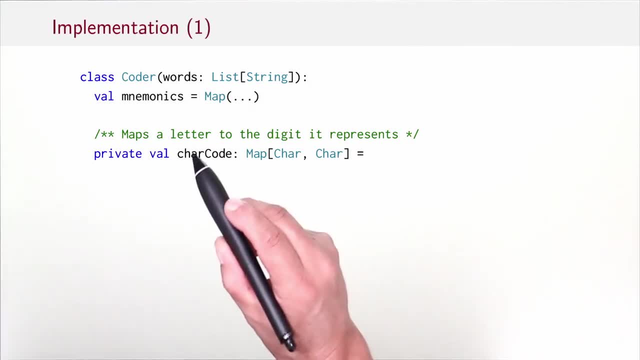 So the first method- carcode- maps a letter to the digit it represents. So mnemonics was a map from digits to letters in these strings. Now we want to go the other way, So that amounts to essentially inverting the map. 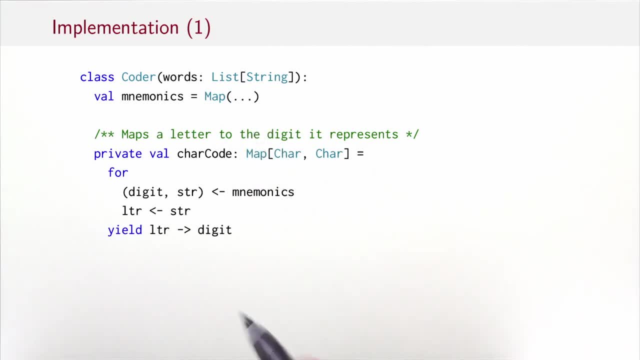 We want to swap essentially keys and values, but it's a little bit more complex because one half is essentially buried in the string. So what we do is we let digit and string range over all the pairs in mnemonics and we let letter range over all the letters in string. 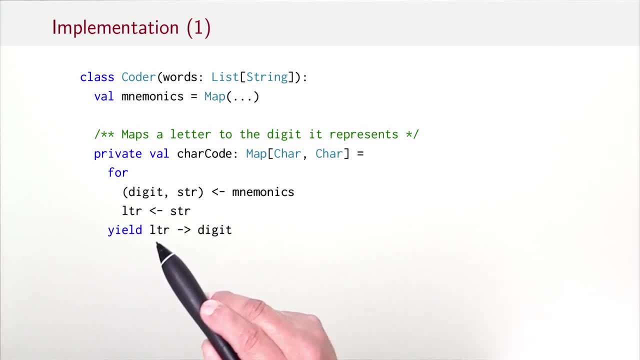 and then we return the pair of letter to digit. So each letter that we find here corresponds to this digit, of course. so we just return these bindings as individual pairs. Good, so now that we know carcode, let's scale that up to word code. 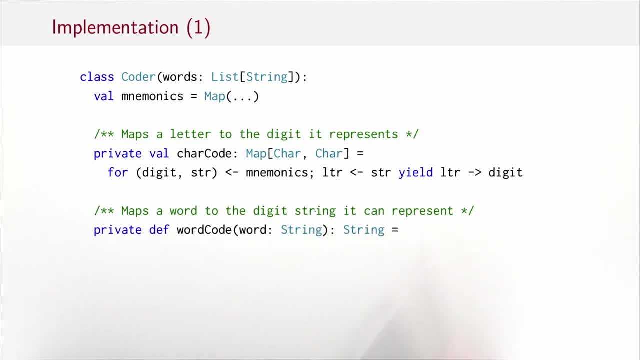 So we want to map a word to the digit string it can represent. So here's the implementation. Essentially we map each letter in the word with carcode. So for each letter in the word we want to know the digit it can represent. 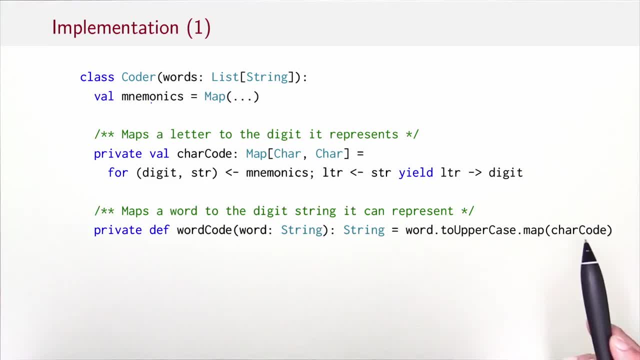 We want to concatenate all these digits. That gives us the digit string that the word as a whole represents. Before doing that, however, we should convert all the letters in the word to uppercases, because carcode is only defined for uppercase characters. So that leads to this right-hand side here. 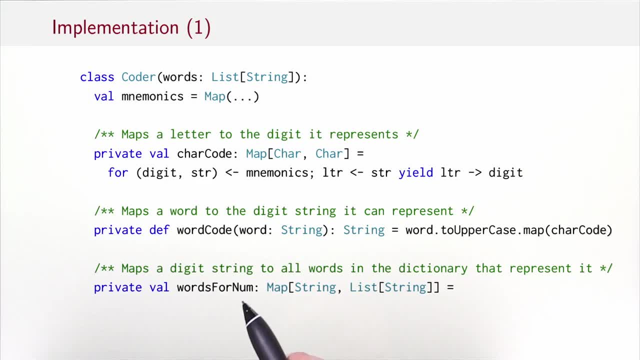 The third definition is words for num. What we want is a map from strings to list of string, that maps a digit string to all words in the dictionary that represent it. So it's again, in a sense, the inverse of what we've done here. 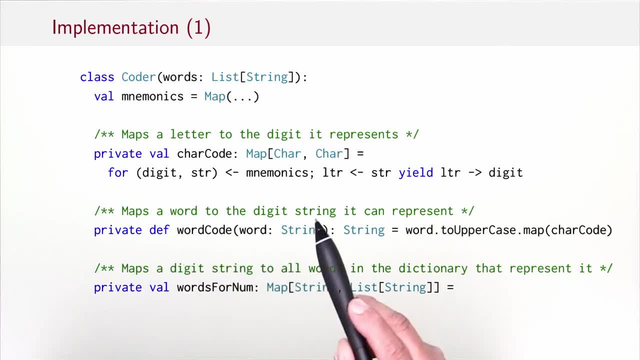 Here, given a word, we know the digit string it can represent. And now, given a digit string, we want all words that represent that digit string. So is there an operation in the collection library that corresponds to that? And the answer is yes. 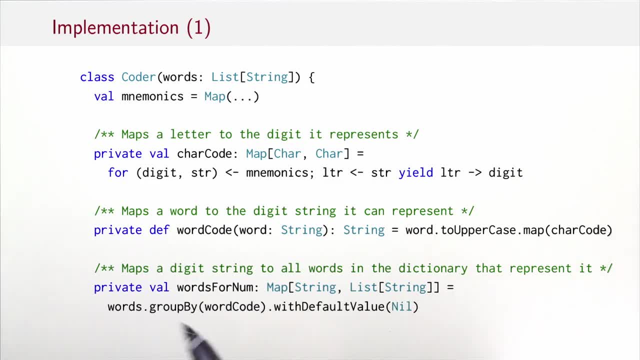 That's a groupby, So it's words grouped by word code. Indeed, if we look at it, we say OK for each word. take the word code, That's a digit string represented by it, And then that becomes the key of the map. 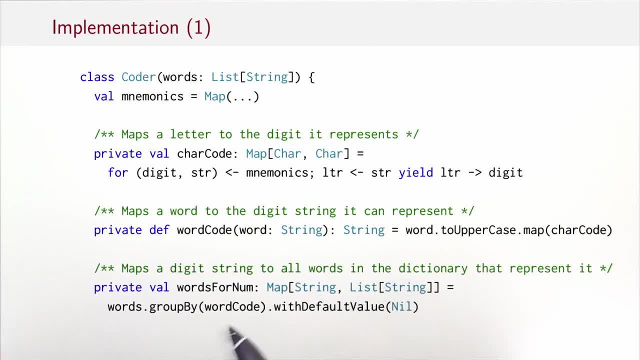 And we add to the key, as a list of strings, all the words that have this word code. that's exactly grouped by. Furthermore, what we want for words for num is a total map. So we want to say, even if a string doesn't appear, 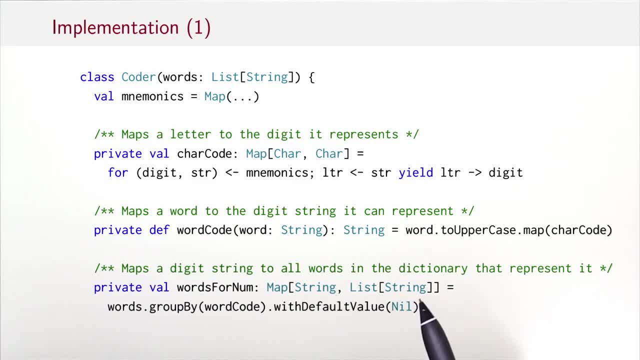 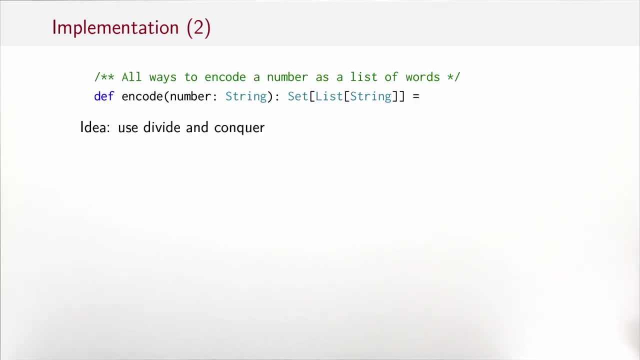 in the map. we still want to map it to something. In this case we map it to nil. That means that digit string doesn't correspond to any word in my dictionary. So now we're just left with the ENCODE method. ENCODE is the method that essentially does the main work. 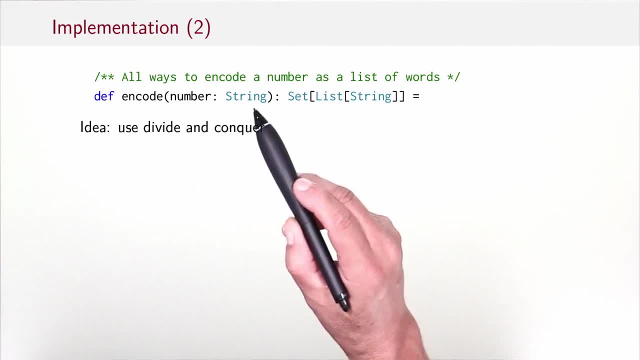 So it takes a number, a digit string, and it should give us back a list of strings where each of these is a phrase that essentially maps to the number, And we want to have a set of solutions. So, because we said we're interested in 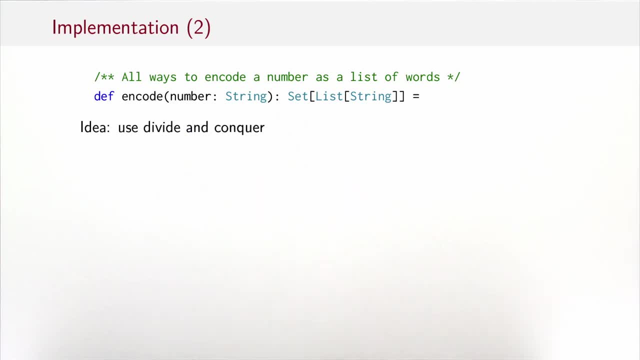 all the possible word combinations that map to the given number. So our result type is a set of list of strings. So it's a set of phrases. Each phrase is represented as a list of strings. So to implement ENCODE we use a principle. 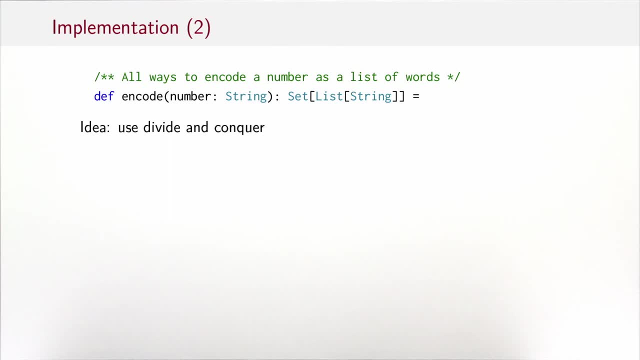 which is very common in functional programming, In fact, which we have used time and time again without calling it as such. The principle is called divide and conquer. So the idea with divide and conquer is that we split the problem into essentially two or more easier sub-problems. 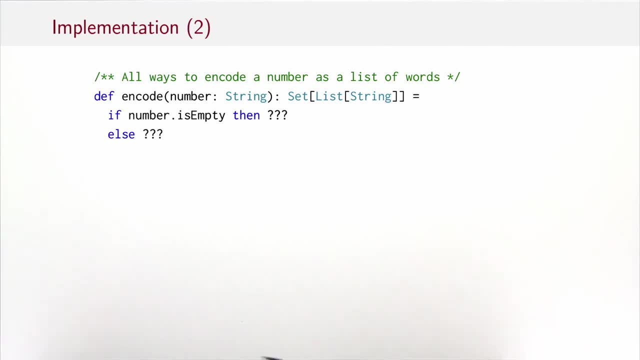 We solve the sub-problems and then we put back the solutions together for the final solution. So what are two sub-cases for splitting a number? So I guess the first distinction would be: is the number empty or not? We have to handle either case. 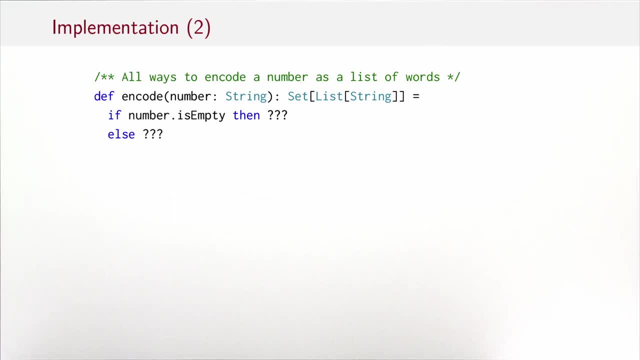 So if the number is empty, what do we return? So we want to have a number, or we want to have a phrase that corresponds to the empty number. That's easy. That's just the empty phrase. So we get a set consisting of a single solution. 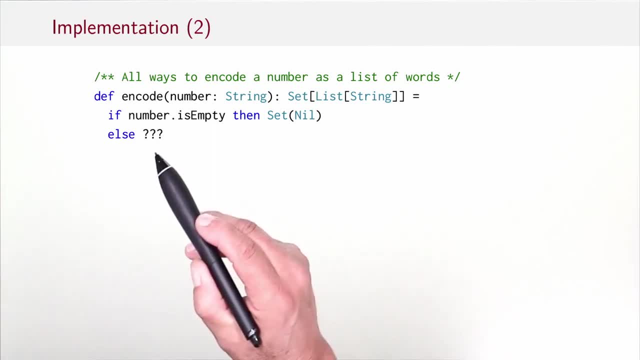 which is the empty list. So what do we do if the number is not empty? We have to find another divide criterion to split the problem into two simpler sub-problems. So one divide criterion could be to say: well, we have this digit string. 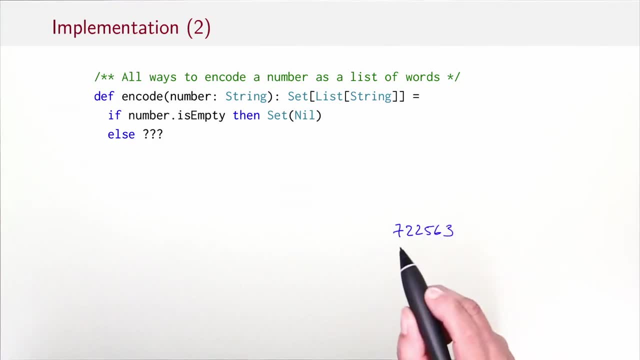 Let's say 722563.. And then we want to say: well, how many digits do we use for the first work? We have a choice: It could be one, or it could be the whole digit string or anything in between. So that would be a possible split point. 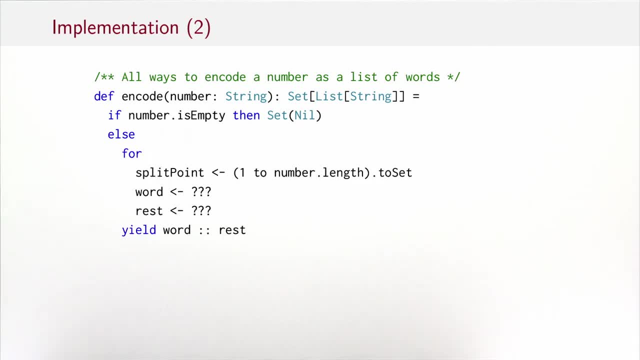 and we work from there. So that leads to the following outline. So we say we take the split point which starts at one and ranges up to the length of the number, And that gives us a point where we want to split it. Then we compute the word. 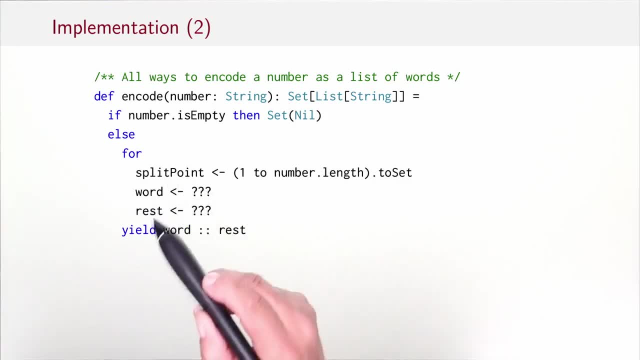 that contains the digits up to split point. We compute the rest of the phrase that contains the digits following split point And we compose the rest and the word together to our solution. So that's the outline. Why did I write .2set here? 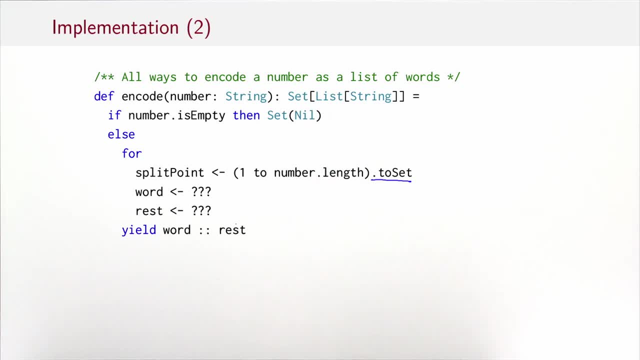 Well, it's because in the end, I need a set of list of strings, whereas here I have a sequence, I start with a range and that will get transformed to other sequences- vectors, normally- But that's not what I want in the end. 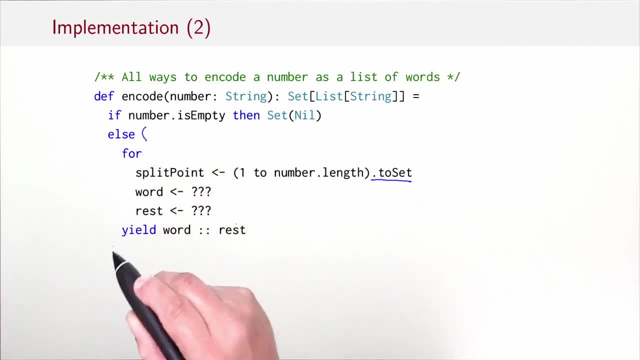 So I could either have written here the whole thing .2set- That would have worked- Or, like I did it here, I put the 2set immediately around the range. Now I'm working with sets here and in these four expressions, essentially the collection you start with. 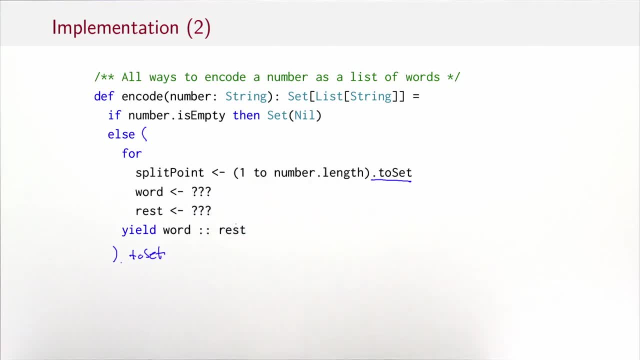 is also the collection of the result. So the result then in this case will again be a set. But I have still two things to fill in, Namely how to compute the leading word and how to compute the rest. Okay, so to fill in the first triple question mark. 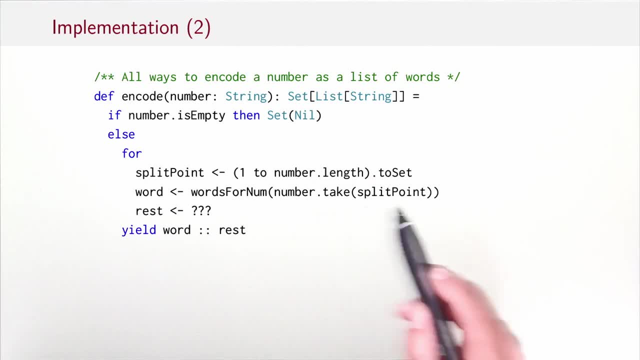 here's the solution: We take the digits of number up to split point and pass them to words4num. So words4num will give us back a list of words that correspond to these digits, And we let word range over the elements of that list. 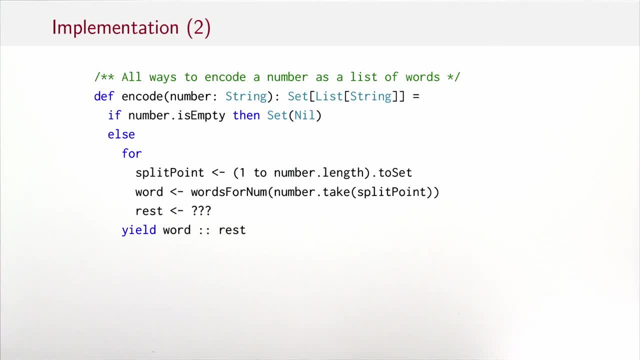 So each word is a possible solution for the first part of the phrase. So how do we define rest? Well, rest is just a recursive call, where we now encode a number without the first split point digits. So what we've done is we've reduced the encode problem. 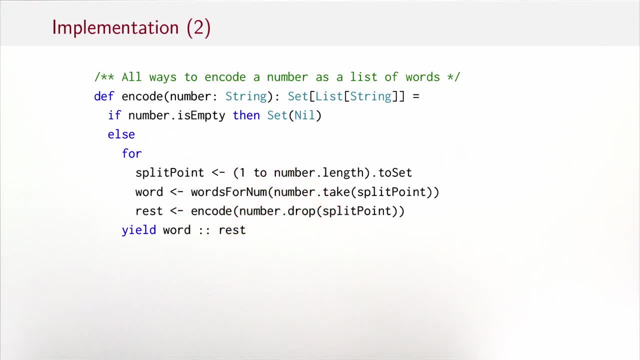 by two case distinctions: One was number is empty or not, and the other was essentially, where do we have the split point? and the other was a simpler problem, Namely a recursive call of encode where the number is smaller. We have dropped at least one element. 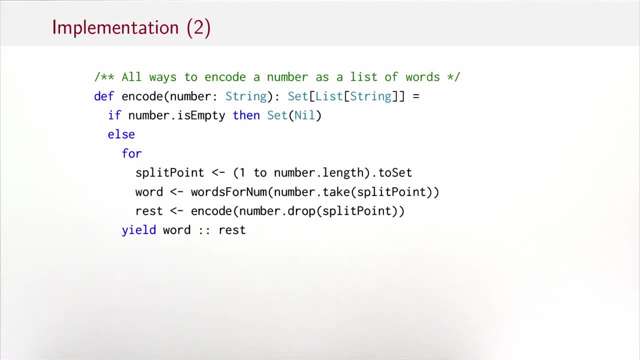 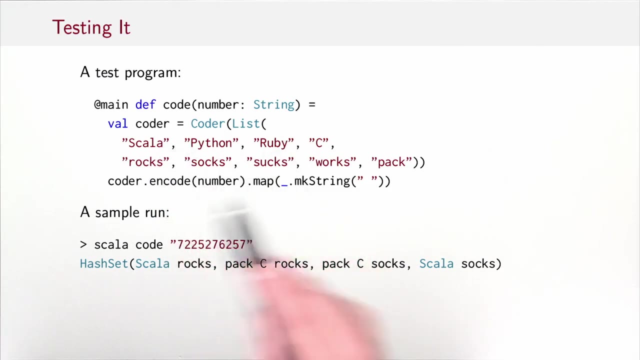 from our number here in the argument to encode, And the conqueror then is essentially putting the things together, and that was just word const rest. So here's a little test program, So we can have a function code which takes a number, and we build up a coder with some sample words. 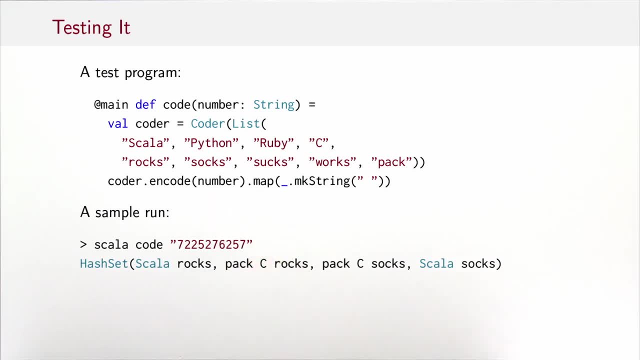 in the dictionary We encode the number and essentially that would give us a set of lists And what we do is, for each element of the set we just form a phrase from the list by putting spaces between the words in the list. So if you have a sample run, 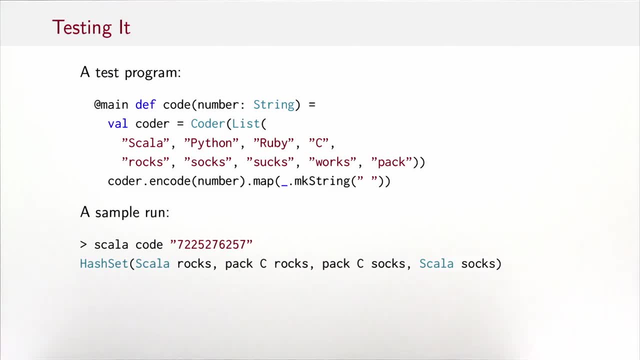 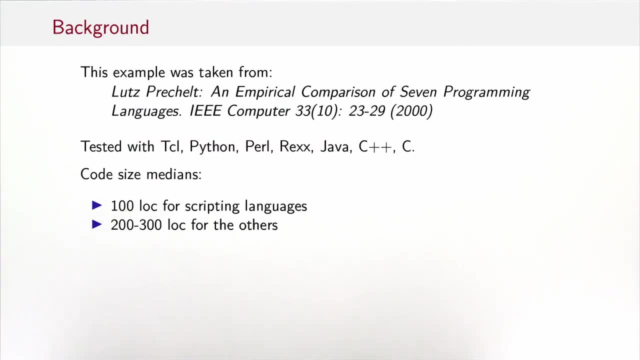 scalar code and then that number, then that would be the resulting set that you get. So this example actually has a history. It was taken from a paper by Lutz Brechelt which is called An Empirical Comparison of Seven Programming Languages. So the languages also show the time when it was taken. 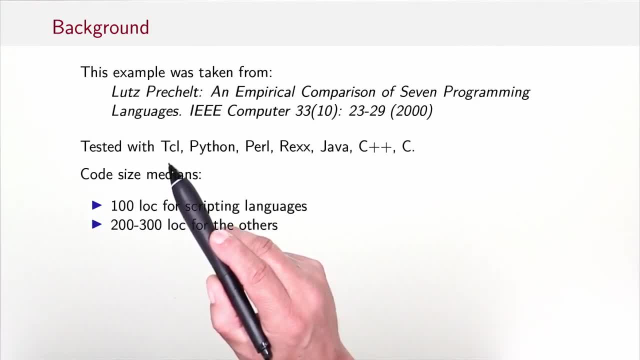 It was essentially the task was for students to solve this problem in different languages. Each group of students had a different language, so several groups per language. The languages were Tcl, Python, Perl, Rex, Java, C++ and C And essentially the question was: 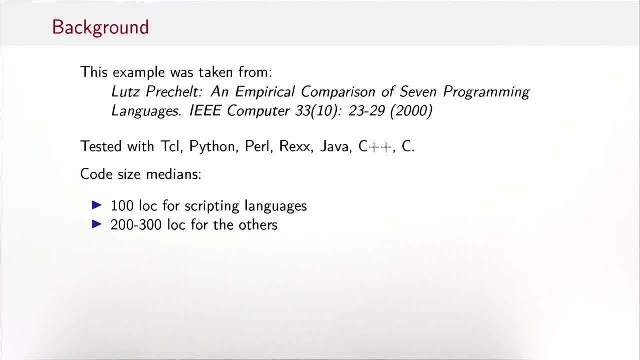 how long are the programs? how correct are the programs? how many bugs? how fast do they run? The interesting bit was the code size of the solutions. So the code size medians were about a hundred lines of code for the scripting languages. 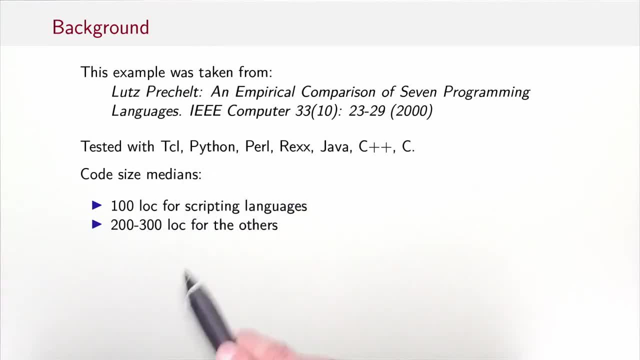 So essentially the first four here and two to three hundred lines of code for the others. What's also interesting was the run time. So you would expect naturally that C, C++ and maybe Java would run a lot faster than the scripting languages. But if you take the average running speed of the solution, 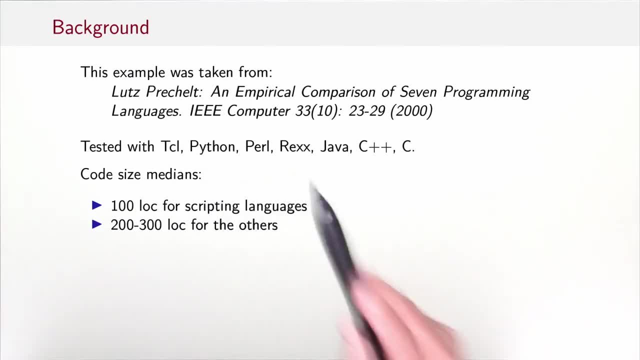 then the big surprise was that actually the scripting languages were quite competitive. Why was that? Well, it was because scripting languages have built-in collection data structures like maps and lists and all the things we were using, Whereas C++ and C had not and Java only had in a limited form. 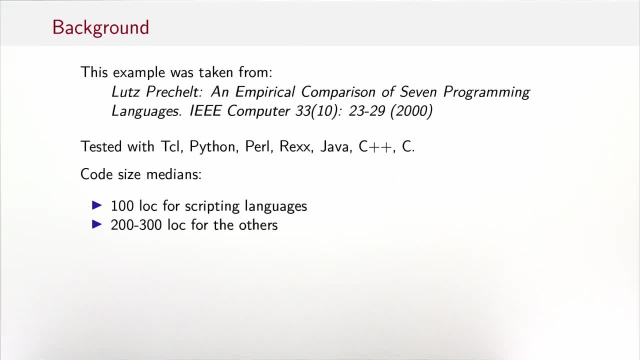 So that meant that people were essentially using the standard building blocks and not going terribly wrong, Whereas in C, C++, people would tend to essentially build their own data structures And sometimes they would get it horribly wrong in terms of performance And that would give you very, very slow solutions. 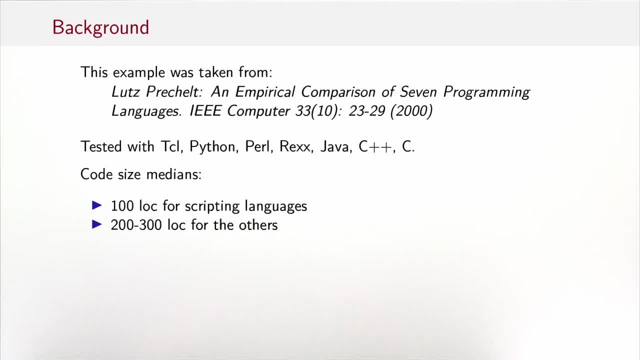 that then would ruin the average. The fastest solutions, of course, were again in C and C++ as well, It has to be said. But what's interesting in our case now is we have something which is very well performing and even much, much shorter. 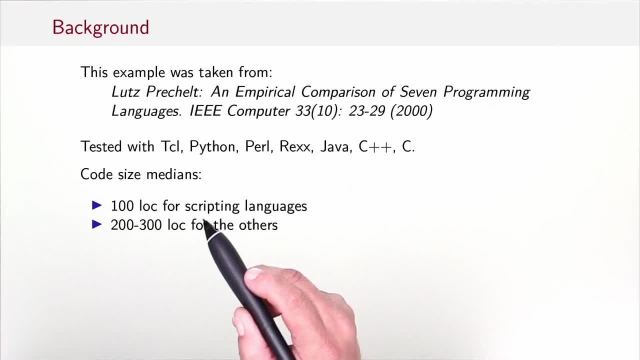 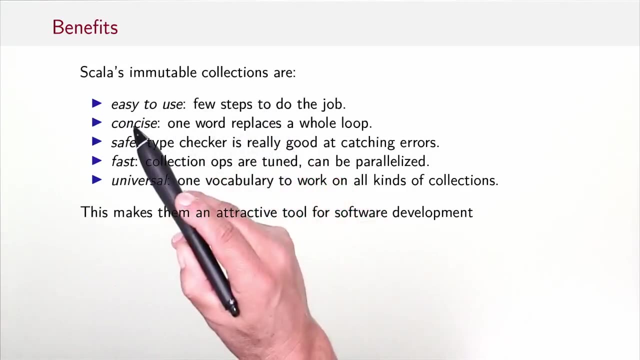 than the scripting languages. So we ended up with maybe 15 lines of code instead of 100 lines of code, And we have essentially strong type safety and pure functional programming as additional bonuses. So what we've seen is that Scala's immutable collections are very easy to use. 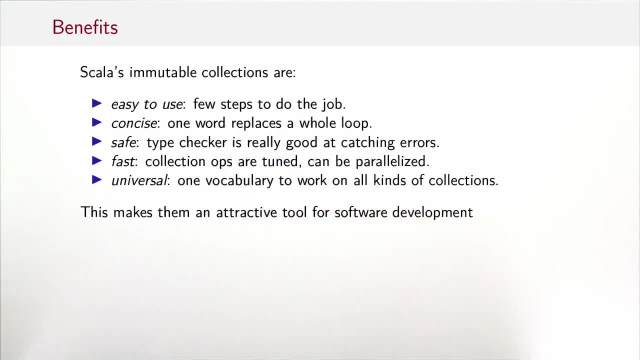 because there are only few steps to do the job. We have powerful operations, such as groupby, that do what in other languages sometimes takes a long sequence of steps. They're very concise: A single word like map replaces a whole loop. They're safe because the type checker 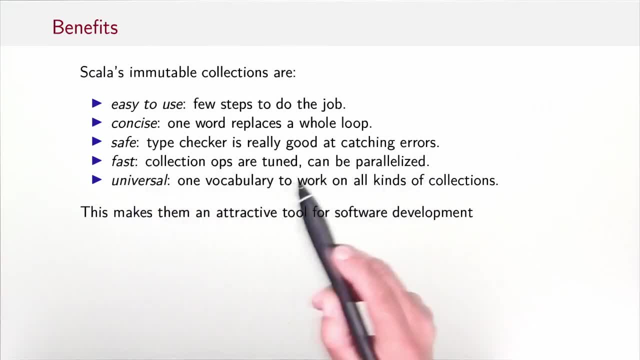 is really good at catching errors. They're very fast because collection ops are tuned and they can also be parallelized And they're universal, So there's one vocabulary to work on all kinds of collections. We've seen that essentially the same words- filter and map- can work on sequences. 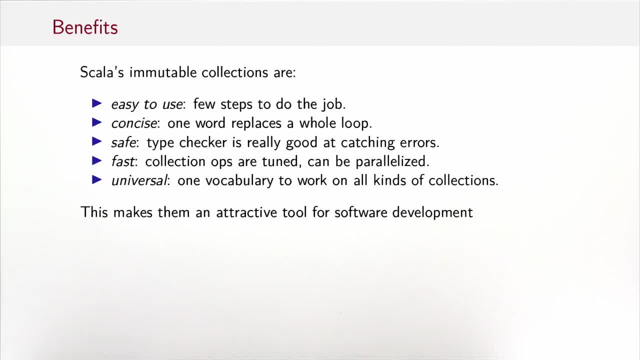 all kinds of sequences, even sort of degenerate sequences such as strings or arrays. But they can also work on sets and they can work on maps. And that's not the end of it. We'll see in the next units that this idea of collection-like structures 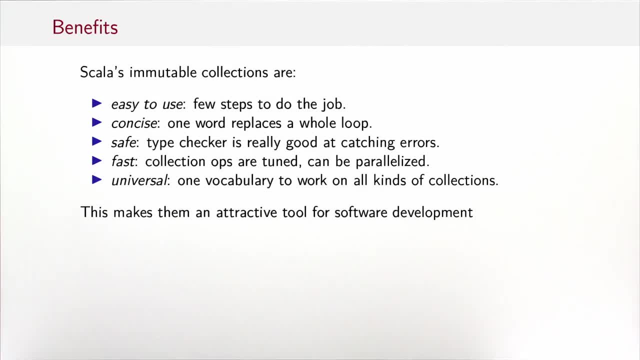 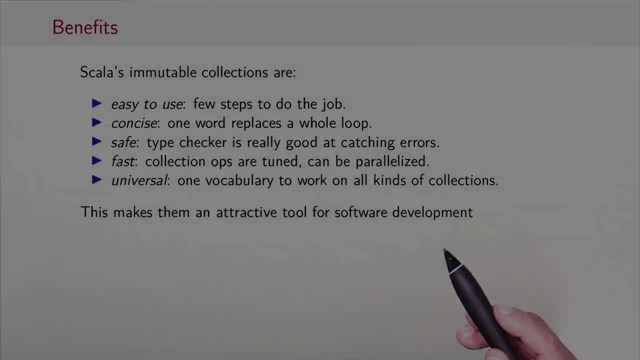 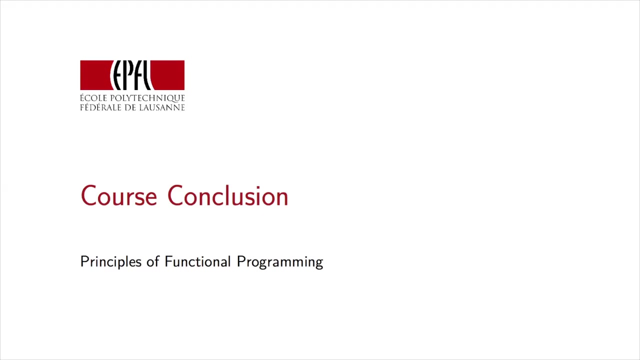 actually extends to a lot more things than just a narrow notion of collections. So we have essentially a universal vocabulary to attack many, many problems in a safe and fast way, And that makes them indeed a very attractive tool for software development. Over the past six weeks, 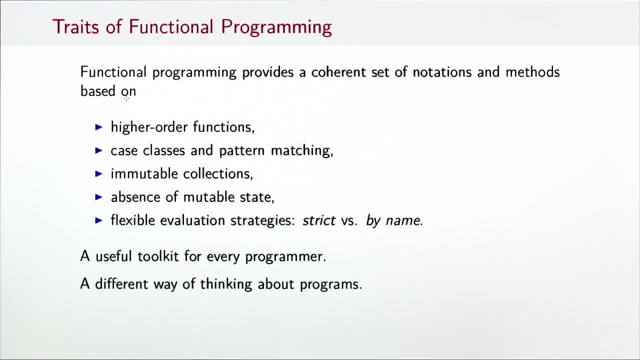 you have explored the traits of functional programming as they present themselves in the Scala language In particular. you've seen high-order functions and how they're composed. You've seen how to represent data with case classes and how to decompose it with pattern matching. 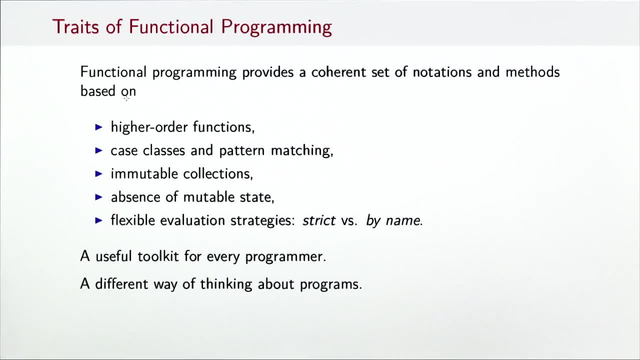 You've seen how to work in the app in the absence of mutable state, in particular with immutable collections, And you have seen several evaluation strategies, namely strict evaluation, call-by-value versus call-by-name, And you have seen how they can be mixed in flexible ways. 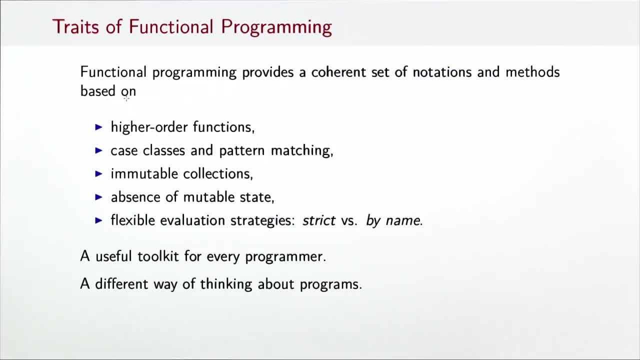 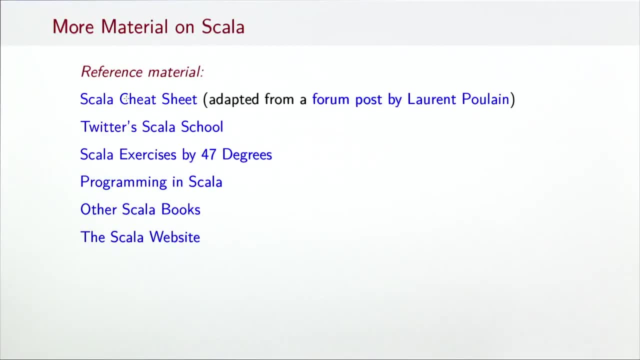 I hope you will find that a useful toolkit for your everyday programming, And I also hope that it has shown you a different way of thinking about programs. If you find out more about functional programming in Scala, there's actually a wealth of material out there. 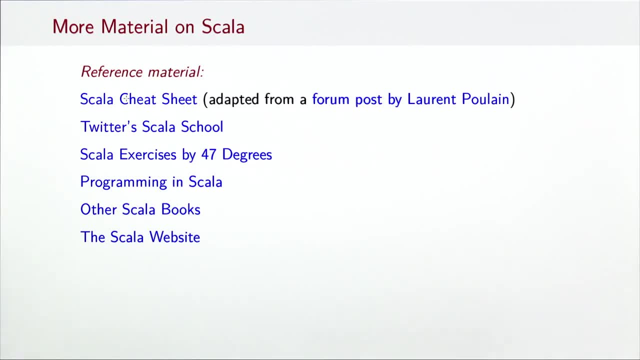 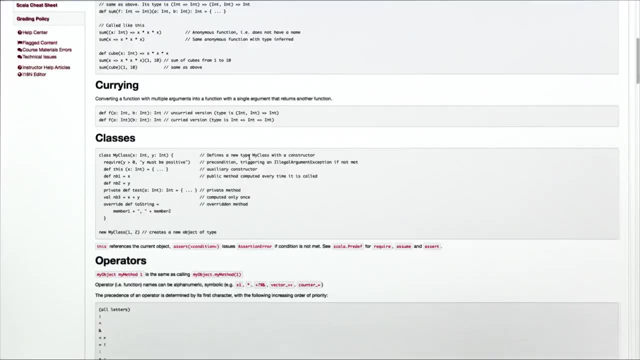 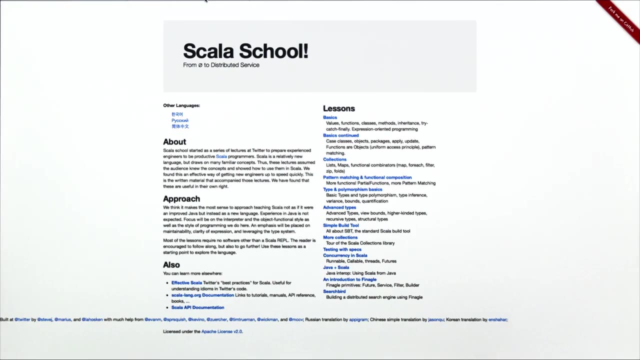 There's the Scala Cheat Sheet, which is actually from a post of a student of a previous course. The Cheat Sheet shows you the essential elements of the course in a condensed form. Another approach to learning Scala is the Scala School by Twitter. It gives you a lot of courses. 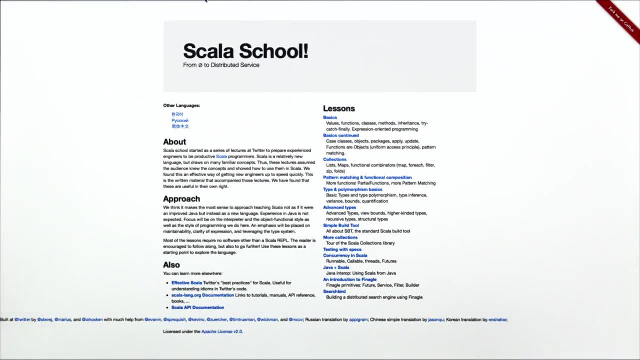 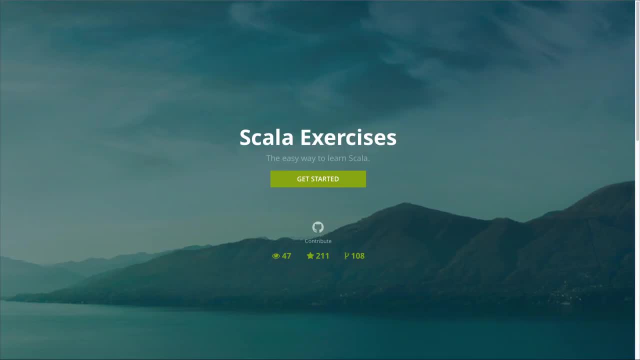 on the basics of functional programming up to the concurrency libraries that are used in Twitter's massive systems that are all written in Scala. Another fun way to continue your Scala experience and your Scala learning is doing some of the Scala exercises by 47 degrees. So that's a way to learn. 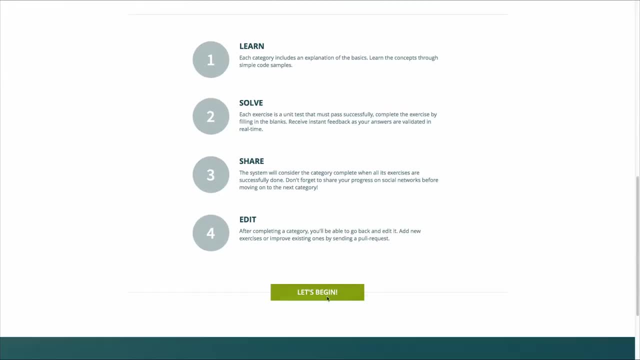 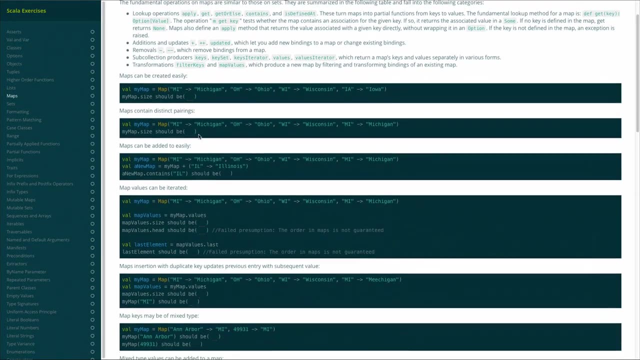 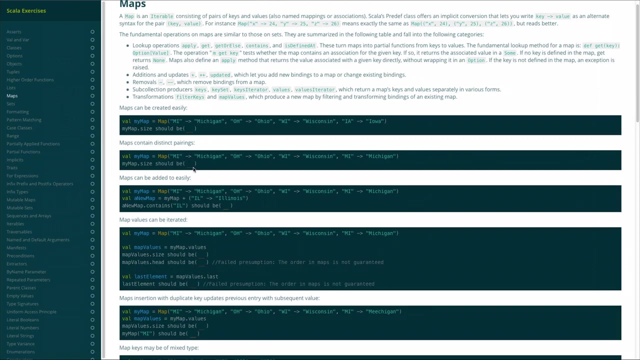 the individual features of programming by means of solving simple exercises. So, for instance, I can come up and have a look at the maps exercises. So here you see, essentially first some description and explanation And then it asks you to essentially fill in the blanks here, to say 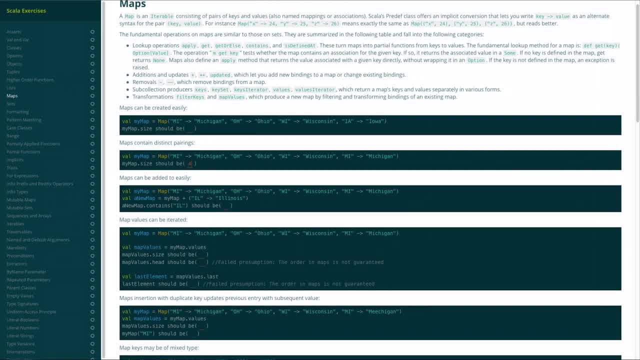 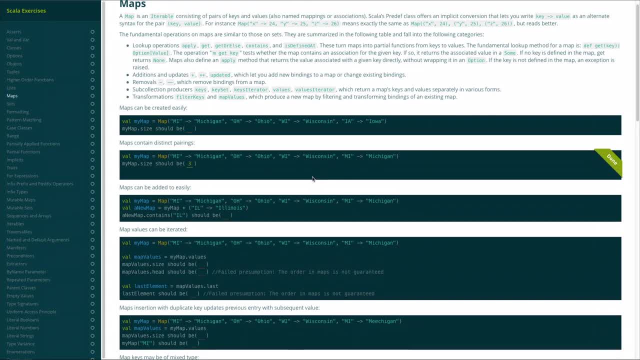 well, how many pairings does map have here? And it says four. No, that's actually wrong. So three is the right answer here. So it's a fun way to test your knowledge about Scala and also to extend it If you're more into reading a book. 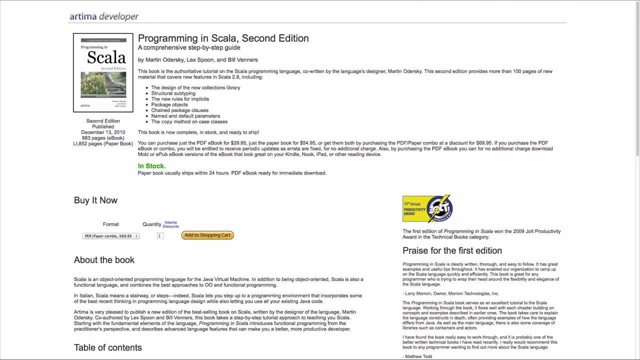 well, the reference book is Programming in Scala, which I co-wrote. It's currently out in second edition. The first edition is actually free download on the web. The second edition is available from the Artema publishers And finally there's the Scala website. 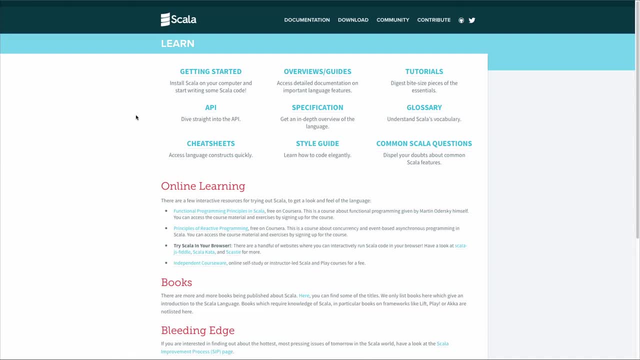 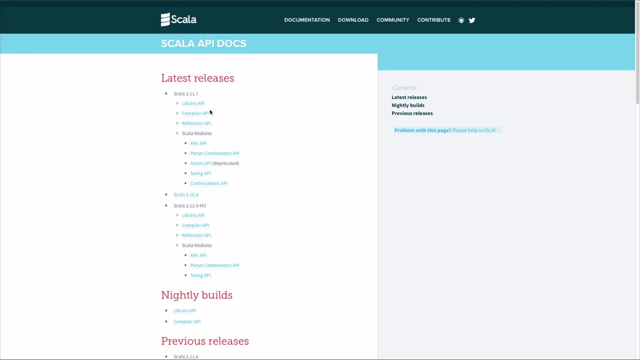 which contains a lot of documentation from again getting started and tutorials to a link to the Scala doc and a general API overview, to links to the community and a lot more. So it was quite a tour what you did over the last six weeks. 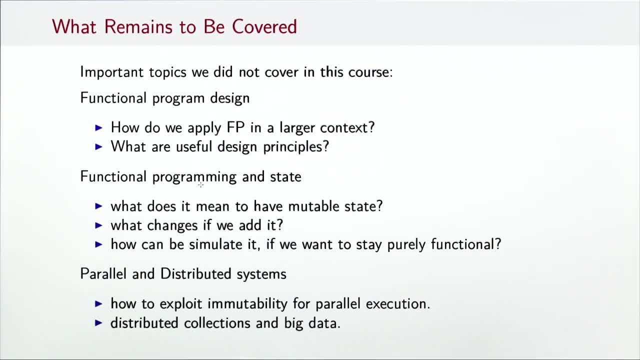 And I believe you learned a lot about functional programming, But there are also quite a few topics that we couldn't cover yet and that would be worthwhile to study in a future course. The first topic would be: well, how can we use the principles? 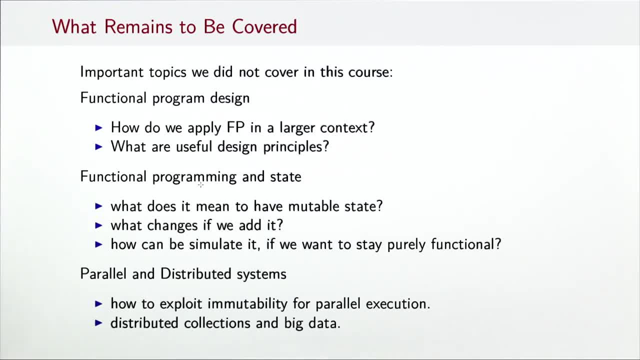 and the elements that we learned in this course in the design of larger programs. How can we apply functional programming in a larger context? Related to that is the question: what are some useful design principles of functional programming? We know all about design patterns in object-oriented programming languages. 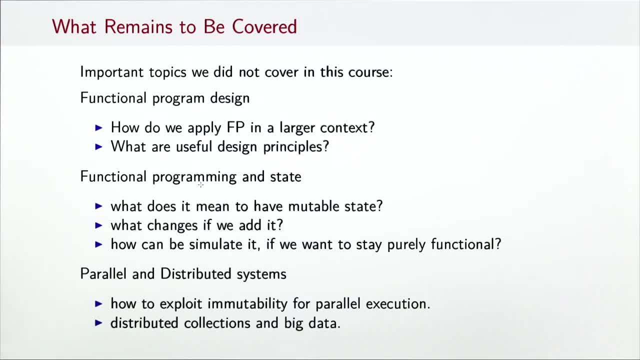 So do they carry over to functional programs? Probably not, But then the question is: well, what would be typical functional design principles? Another important and interesting question is about the relationship of functional programming and mutable state. So far, all our functions have been pure. 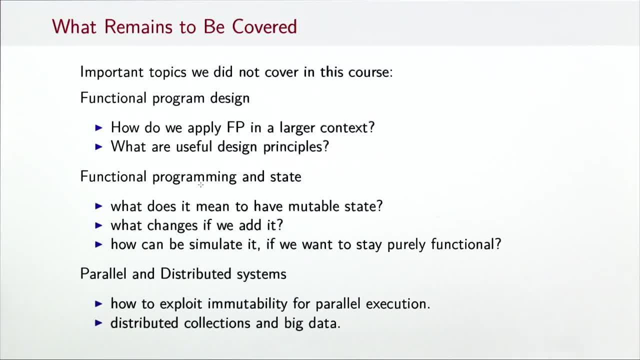 There were no side effects, And that meant we also had very powerful reasoning principles about functional programming that are all rooted in the idea of that substitution model that you have learned. Once we add mutable state, do things change? That's a very important question. 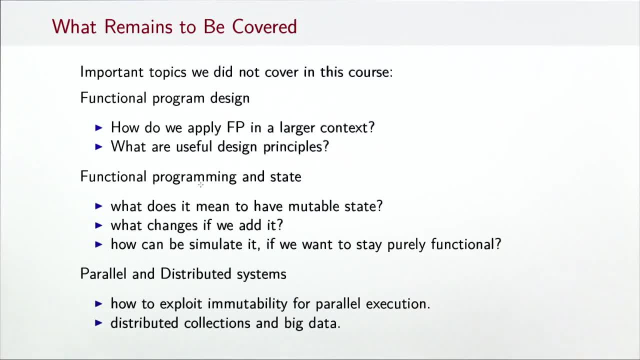 And also, if we don't want to add state in a straightforward way, can we maybe simulate state in a purely functional setting? Another important development is from sequential programming- what we have seen in this course- to parallel and distributed systems I've mentioned at the beginning of this course. 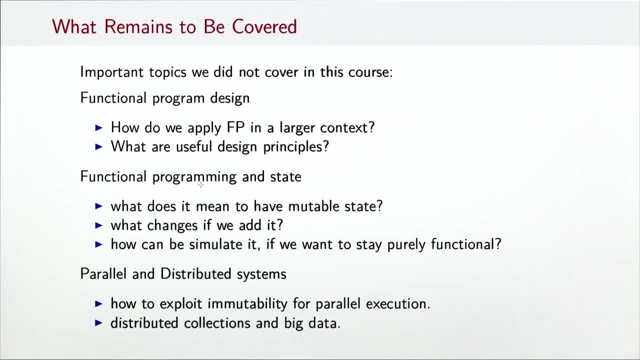 that functional programming is very suitable for parallel evaluation. But so far all our programs were sequential, no parallelism involved. So once we go parallel it would be interesting to see what are the data structures, what are the algorithm and programming techniques to do that. 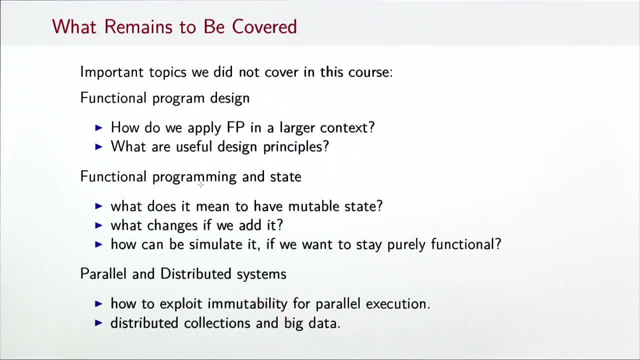 And one step beyond parallel programming are distributed systems, in particular, distributed collections that, it turns out, are very, very useful for big data and data science, data analytics. So there's a fascinating set of topics still to be explored And I hope I can see you back. 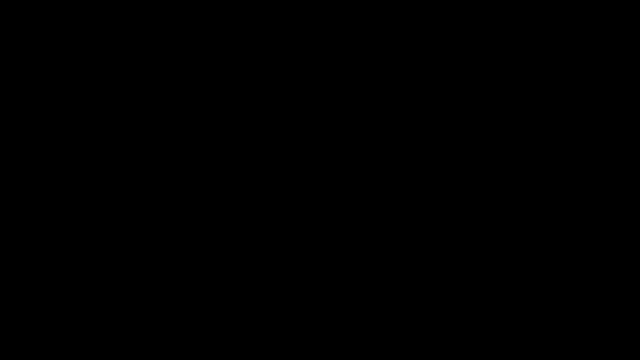 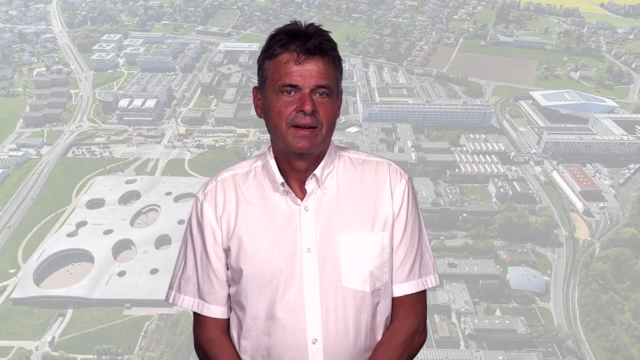 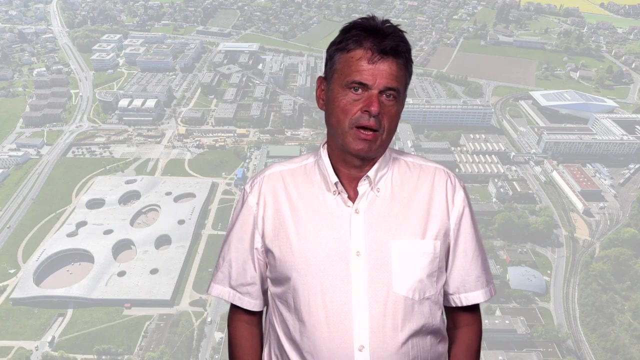 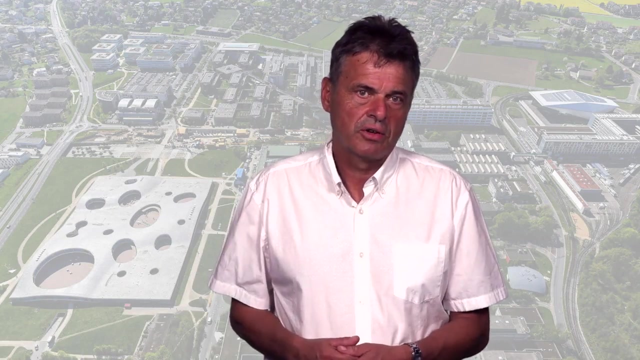 in future classes to do that. Welcome In this course. you'll learn how to apply the functional programming style in the design of larger applications. You'll get to know important new functional programming concepts, from lazy evaluation to type classes. We'll work on larger. 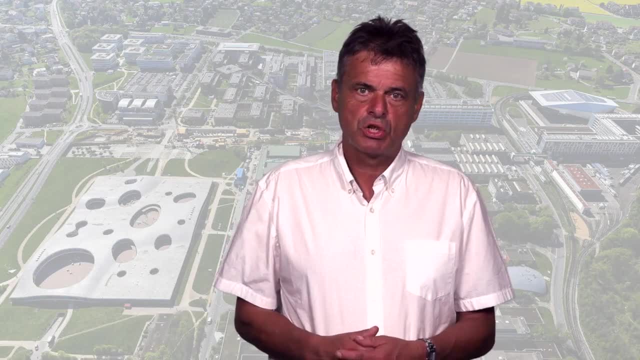 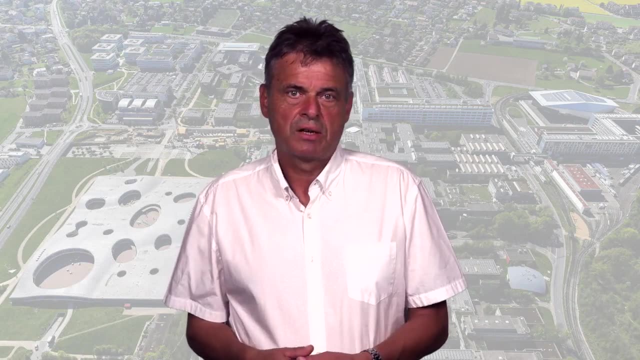 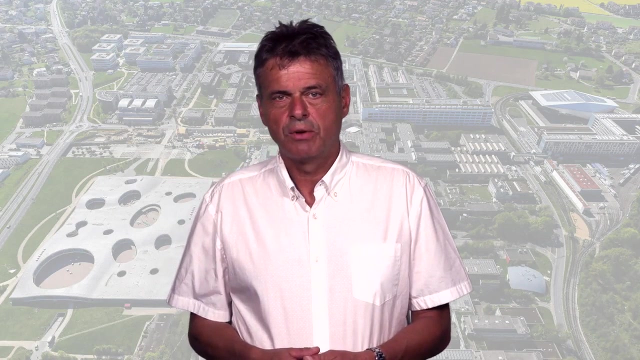 and more involved examples including state space exploration, random testing and discrete circuit simulation. In doing that, you'll also learn some best practices on how to write good scalar code in the real world. Several parts of this course deal with the question how functional programming interacts. 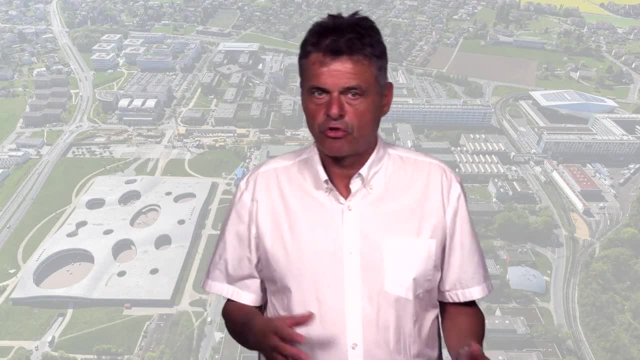 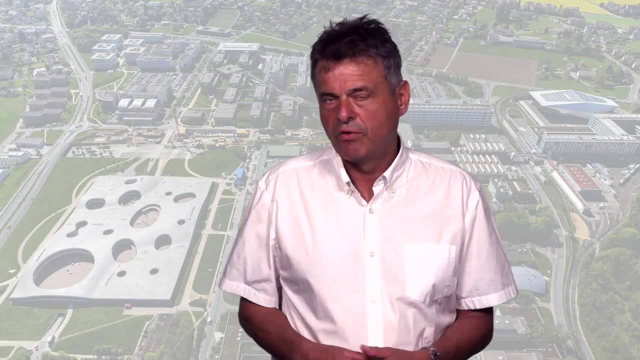 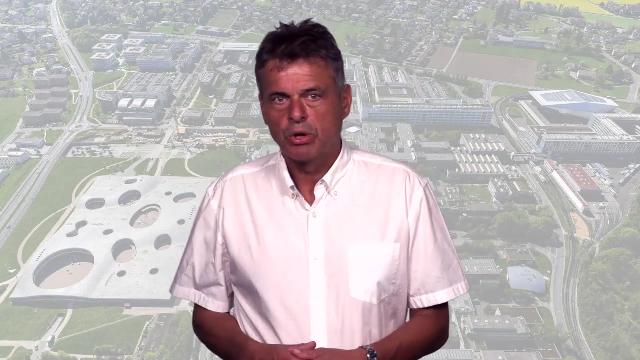 with mutable state. We'll explore the consequences of combining functions and state, And we'll also look at purely functional alternatives to mutable state using infinite data structures or functional reactive programming. Once you've finished this course, you should be able to recognize and apply design principles. 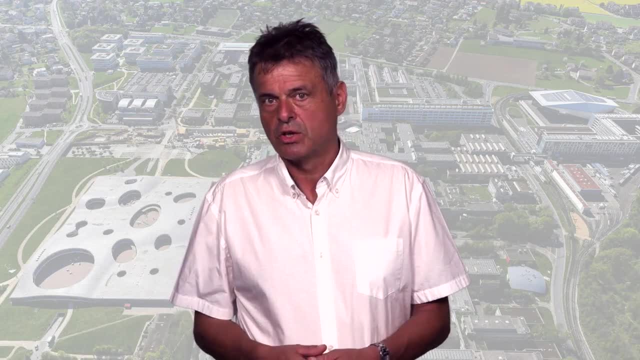 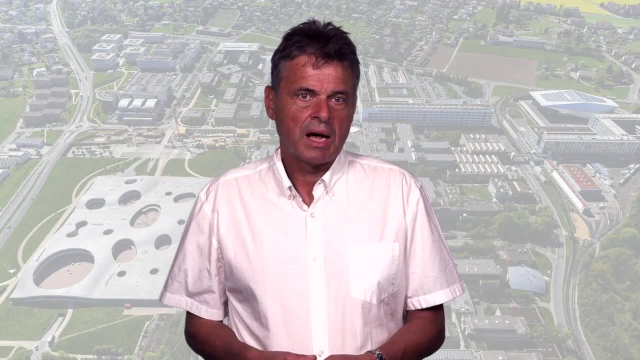 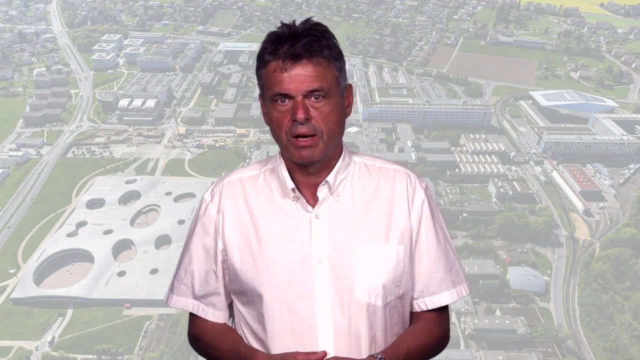 of functional programs. You should be able to design functional libraries and their APIs. You should be able to competently combine functions and state in one program and understand reasoning techniques for programs that do that. And finally, you should be able to write simple functional reactive applications. 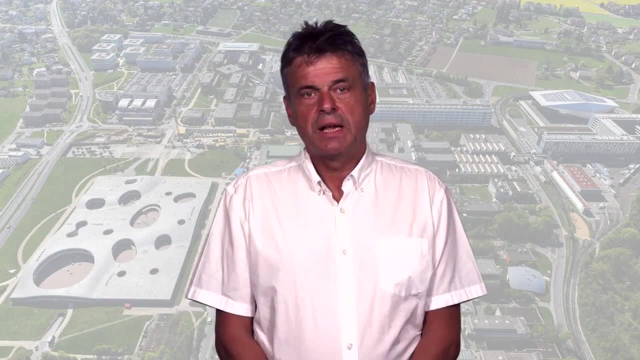 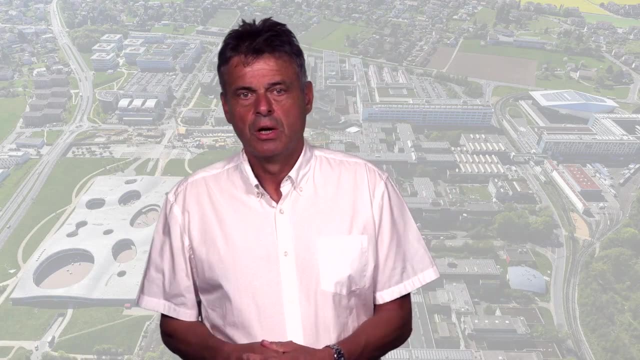 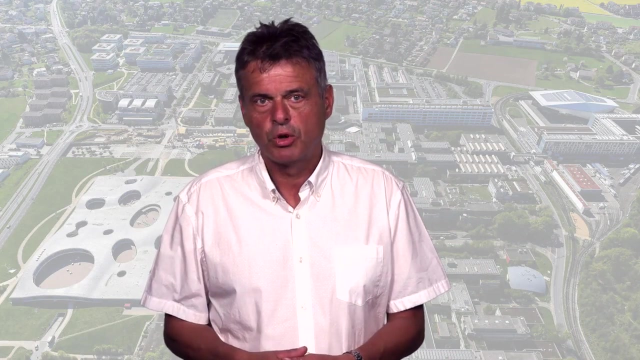 What about prerequisites? Well, this course is intended as a continuation of the course Functional Programming Principles in Scala. You typically will have taken that first To take both courses, a familiarity of maybe one year of programming is sufficient. Java and C-sharp would be ideal. 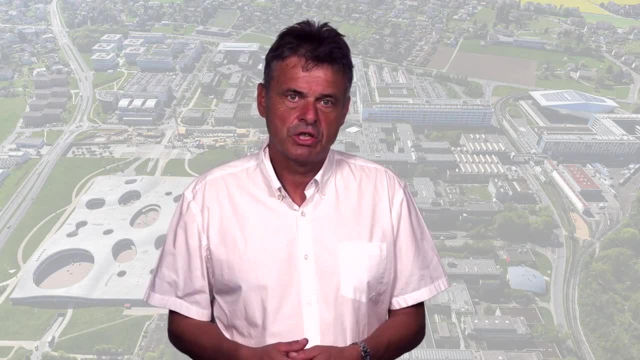 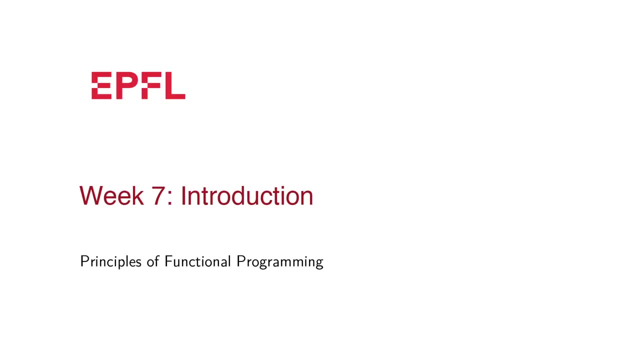 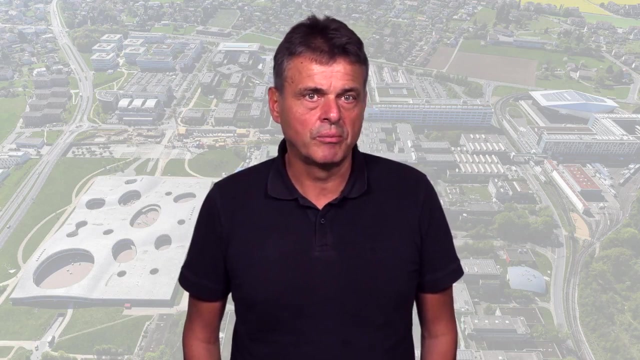 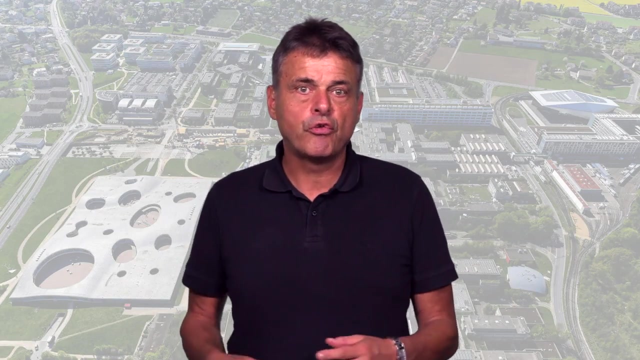 but Python, JavaScript, Ruby or many other languages would also be sufficient. Welcome. We'll start this week by revisiting some concepts that we've learned in Principles of Functional Programming, in Scala Collections, pattern matching functions. We'll then touch on four comprehensions. 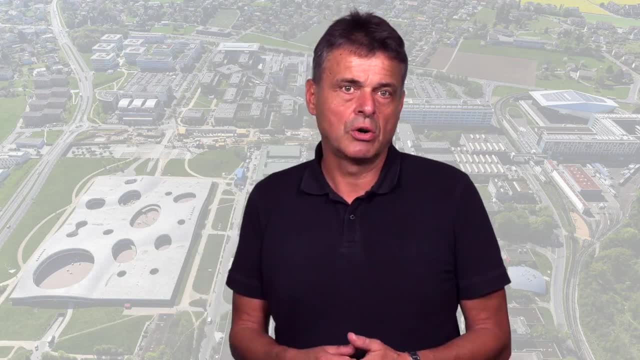 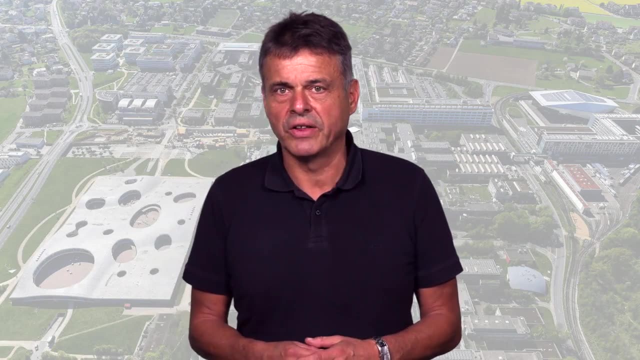 which are a powerful way in Scala to traverse a collection, process it and return a new collection. You'll see that four comprehensions are actually a lot more general than that. For instance, they can also be used as a query language for any kind of database. 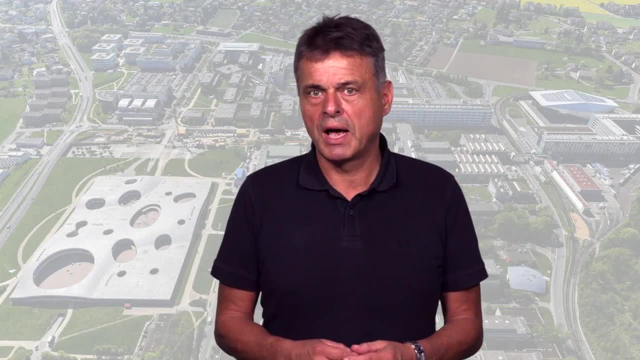 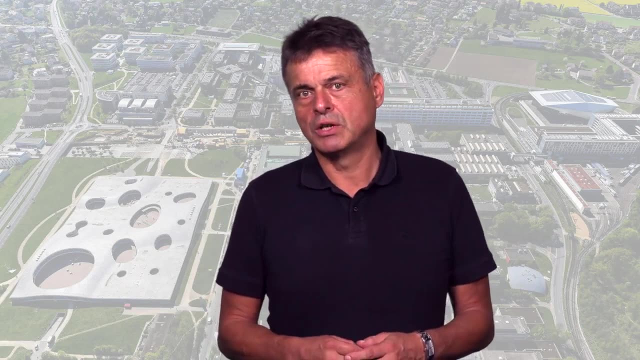 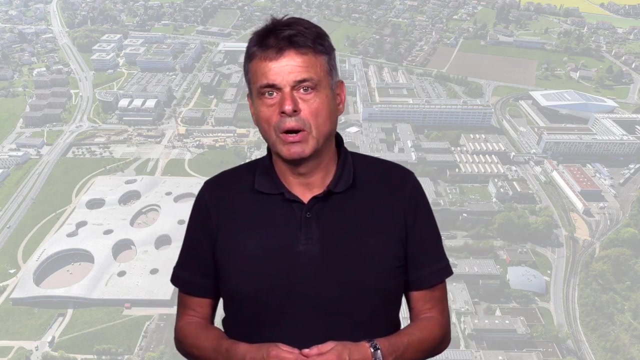 This generality is possible because of the way four comprehensions are translated into higher-order functions by the Scala compiler. In fact, four comprehensions are related to the concept of monads in category theory. You'll find out what monads are and will learn by means of examples. 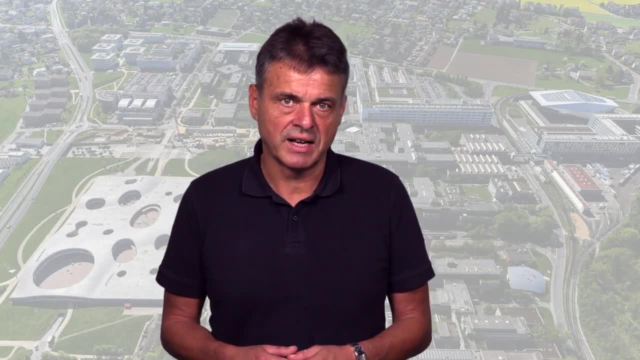 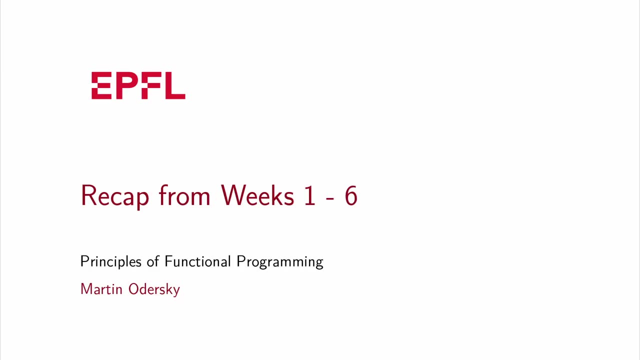 some techniques to verify that the monad laws are satisfied. In this session we are going to do a quick recap from weeks one to six of the Programming Principles in Scala course. The first topic to review is case classes. Case classes are Scala's preferred way. 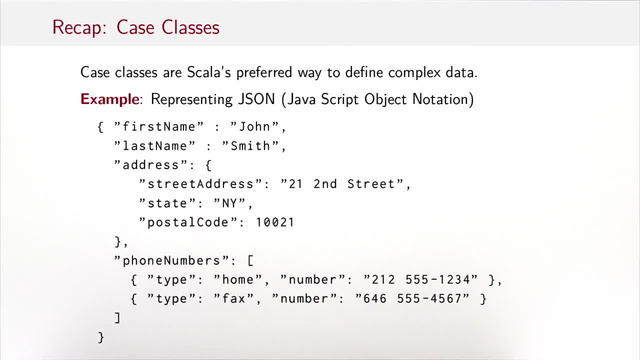 to define complex data. As an example, let's come up with a case class hierarchy to represent JSON, the JavaScript Object Notation. Here you see typical JSON data structure. You have fields and definitions of those fields. It can be recursive. a field can map to another JSON object, in braces. 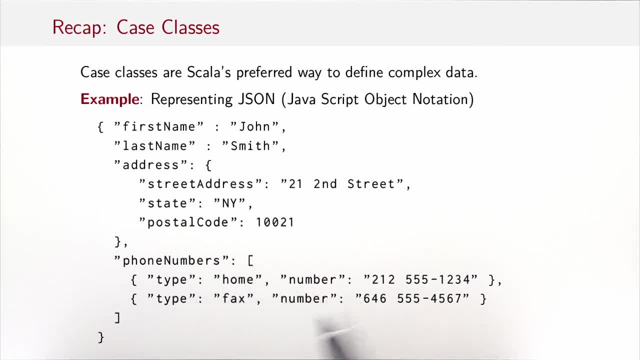 or it can map to a JSON sequence in brackets. The difference between an object and a sequence is that objects have names for the bindings here and sequences just have data. One advantage of JSON is that it's a very simple format, so it's also straightforward. 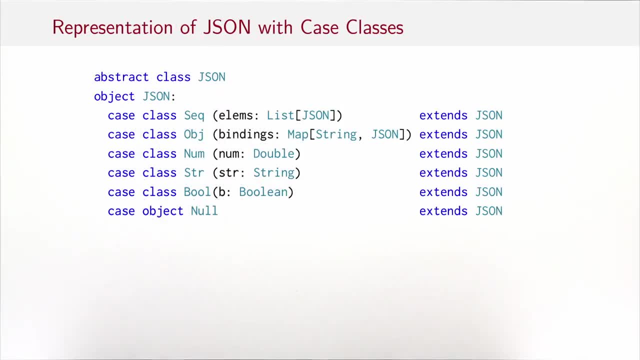 to come up with a hierarchy of case classes for it. So here's a possible representation. I have an abstract class, JSON, a companion object, JSON, and in that companion object the six cases that make up the alternatives of a JSON data structure. A JSON data structure can be a sequence of elements. 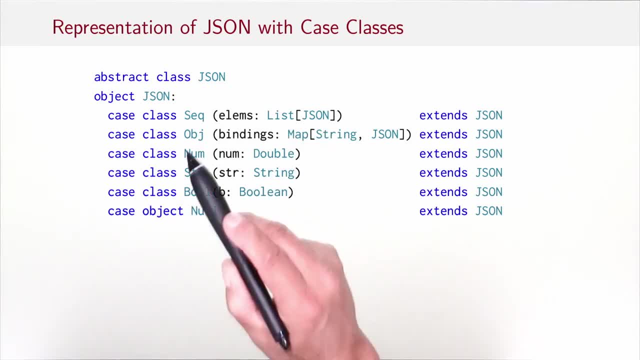 which would be represented as a list of JSON objects. It can be an object which would have bindings that are a map from string to JSON objects, So the strings are the field labels, the values are the embedded JSON objects. It could be a number which is a double. 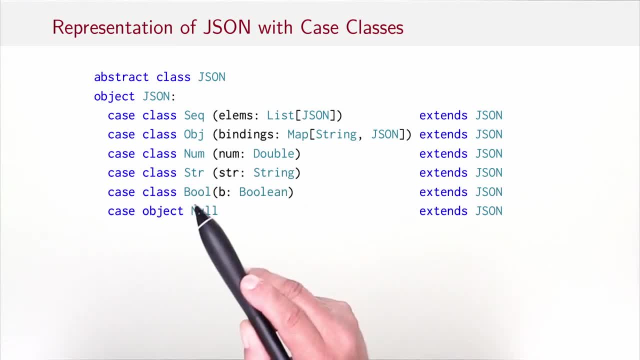 It could be a string which contains a string, It could be a boolean which contains a boolean, Or it could be null. So, unlike Scala, when null is discouraged, JSON data do have nulls in their definition. All these five case classes and this case object. 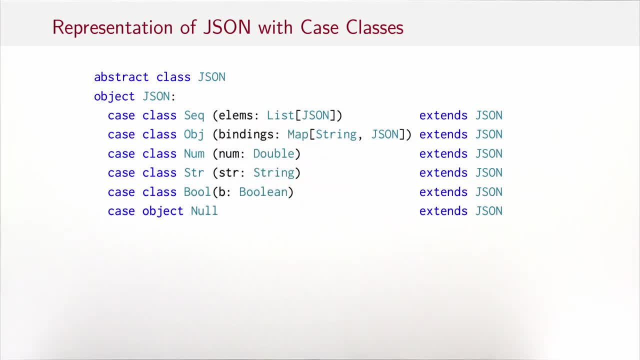 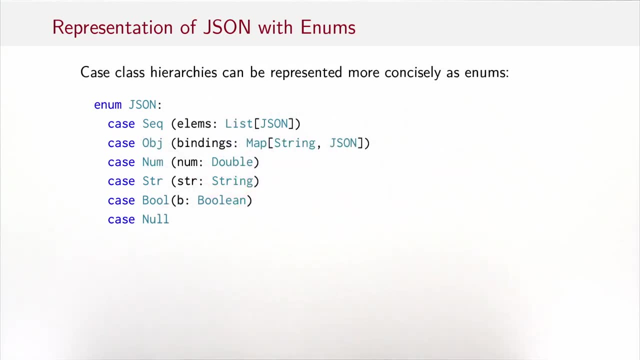 extend JSON, the abstract root class. We've also seen that we can represent case class hierarchies more concisely as enums. So here would be the same thing written as an enum. I would write just enum, JSON, and then the six cases without any extends classes. 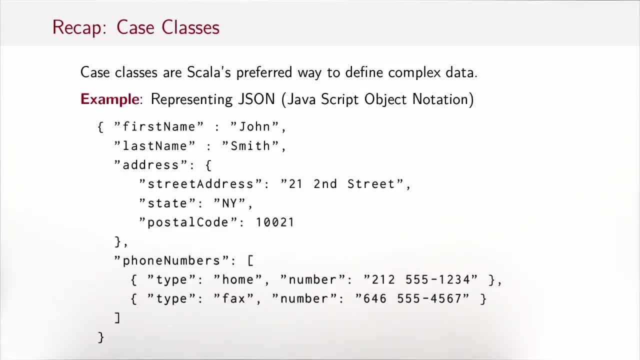 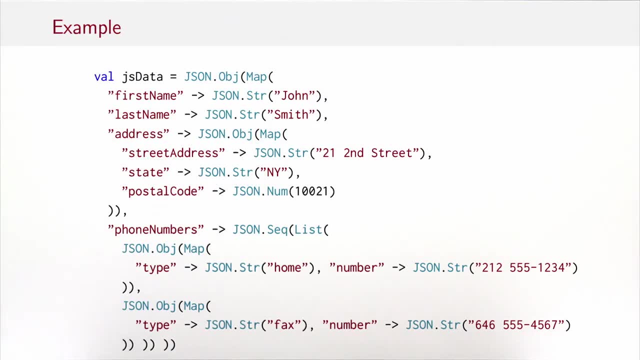 The extends classes would be redundant here. So let's do an example. Let's represent this data object in the enum that we have defined. So that's what it would look like. So our JS data. JS could mean JSON, or also John Smith. 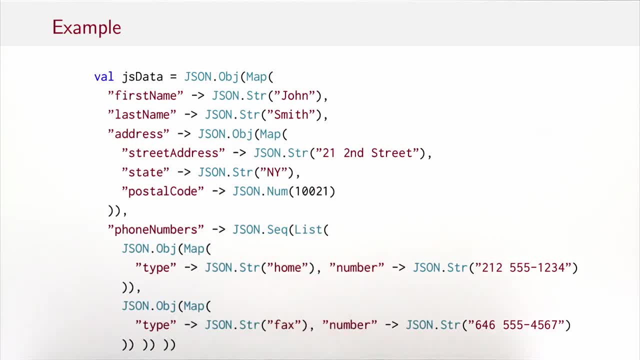 because that's the person we define- would be a JSON object which contains a map. The map contains bindings for: first name, That's the string John. Last name, that's the string Smith. Address, that's the JSON object that's recursively defined by. 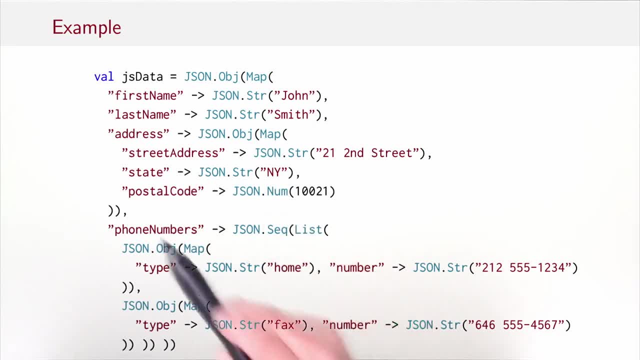 street address- what you see here, State New York. Postal code- what you see here. And it would have two phone numbers. so that would be a sequence. Each phone number has a type and an actual number. The type and the number are both strings. 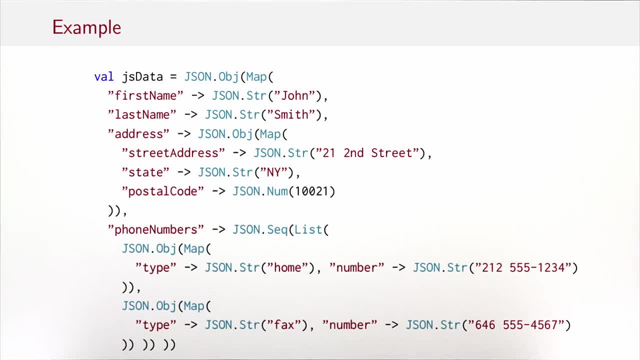 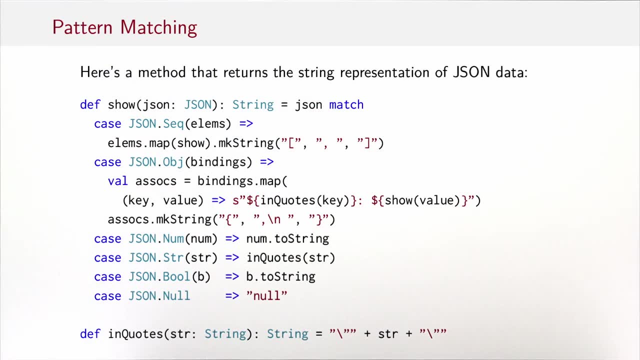 So it's just one example: data structure and the way how we can define it. So the canonical way to work with enums and case classes is by pattern matching. Here's a method, as an example, that returns the string representation of JSON data. So the method is called show. 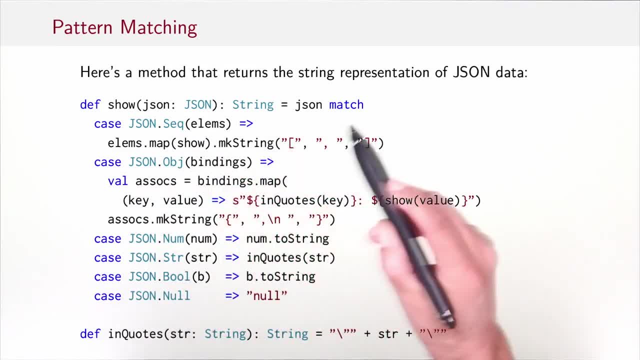 It takes a JSON object, returns a string and it does a match on the JSON object with those six cases. So we would have: if it's a JSON sequence, then we would recursively map the elements of the sequence and we would convert them with a string. 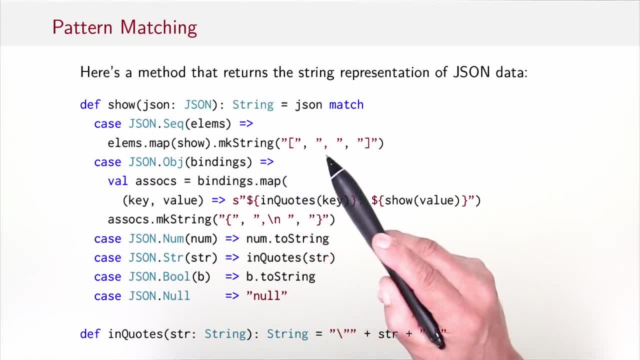 where the string starts with open brackets, We place a comma between ideation string elements and the string ends with close brackets. That's what that makeString function does. If the JSON is an object with bindings which are a map, then we go through the map. 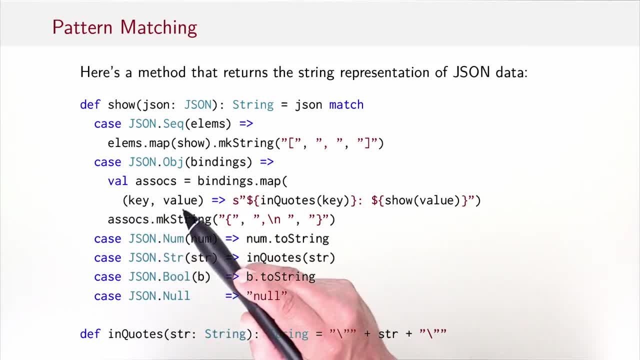 We take every key and value binding in the map and we convert that to a string by showing the key in quotes, because that's what JSON does, and showing the value. So inQuotes is an auxiliary method that takes a string and prints the string in quote marks. 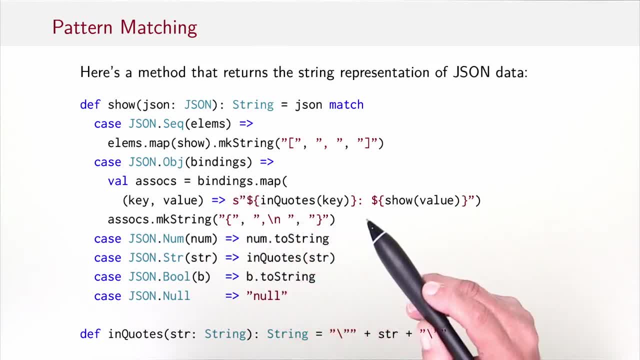 So that first operation gives us a list of strings, one string for each binding in the original bindings, and we now assemble them by placing them in braces and a comma new line between them, So we put each binding on its own line. The other cases are simpler. 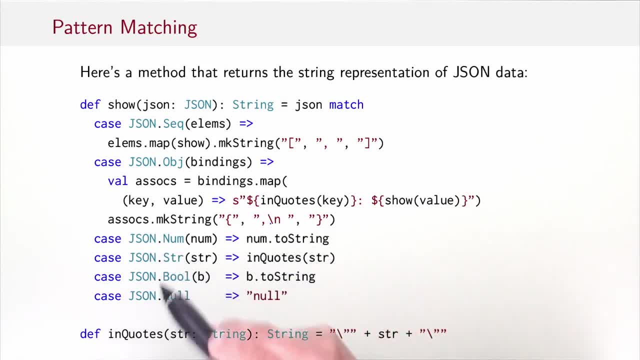 If it's a number, then we convert the number to a string. If it's a string, we print the string in quotes again. If it's a Boolean, we convert it to string, And if it's a JSON null, then we return the string null. 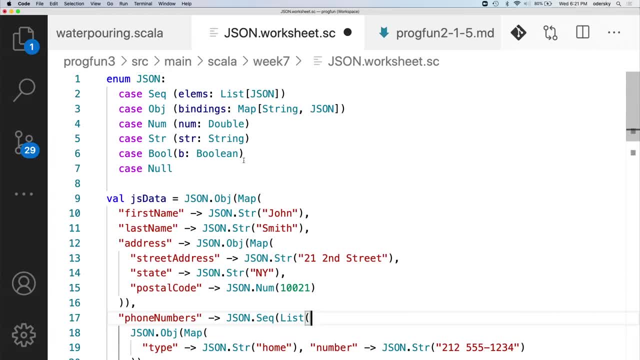 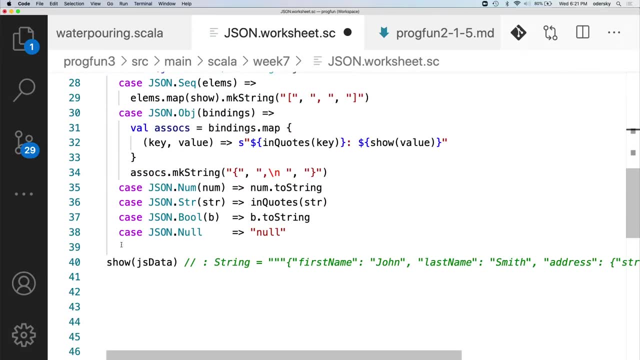 So I've pasted what we've discussed so far in a worksheet. Here's my enum, Here's the JS data example value and here's the show method. So what we can do to test it, we can do show of JS data. 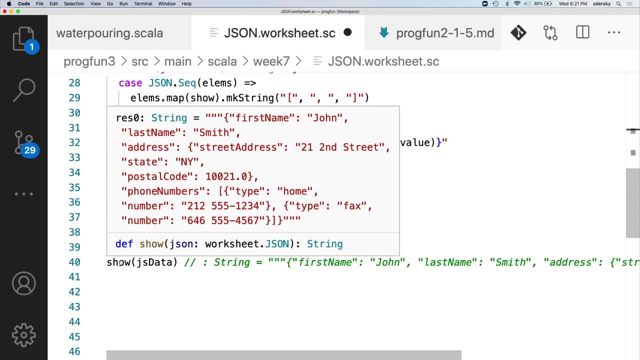 and that would give us the hover says it essentially the string that we see here: first name John, last name Smith. so it resembles very much the JSON value that we started with. So another topic to quickly recap are Scala's collections. 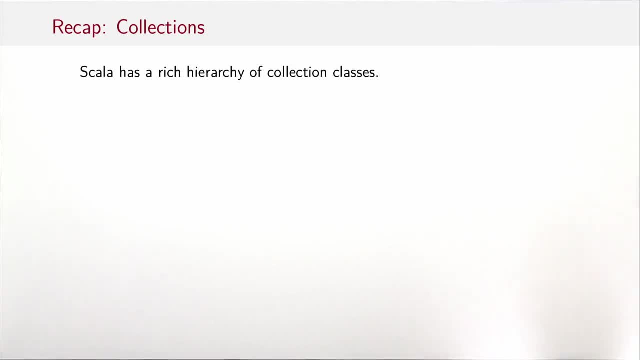 We've seen that Scala has a rich hierarchy of collection classes. They form a hierarchy in that sense that there's a base collection called iterable, and then three fundamental collection kinds, which are called sequence, set and map, And we have seen each in the previous six weeks. 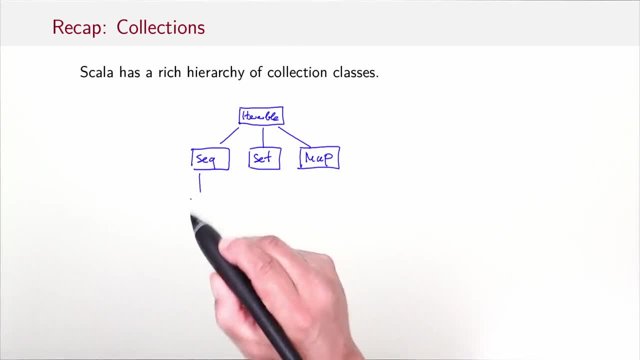 Sequence has multiple subtypes. One important one was the list, but there were also others like vector or array, which is not really a sequence but behaves like a sequence and has all sequence operations And sets and maps. all have multiple implementations with different efficiency, trade-offs. 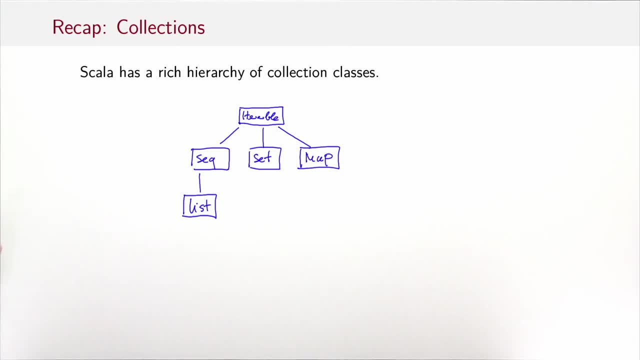 So all these different types could be quite confusing, except that they all really support the same operations with the same names. So that gives you an element of regularity that makes it easy to deal with these collections. So all collection types share a large set of general methods. 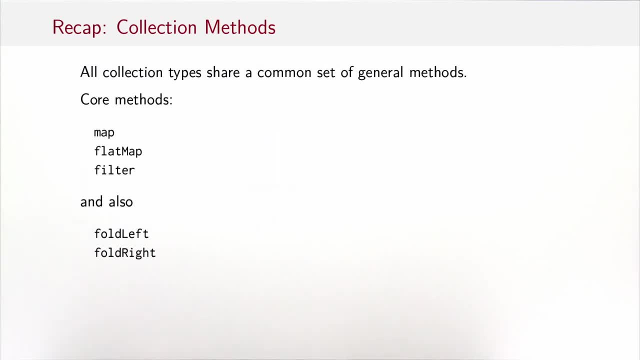 Some of the methods that are quite important, and that's why I wanted to point them out, are: the map method that transforms elements of a collection, creating a new collection. flat map that transforms elements and concatenates the collection results filter that picks all elements. 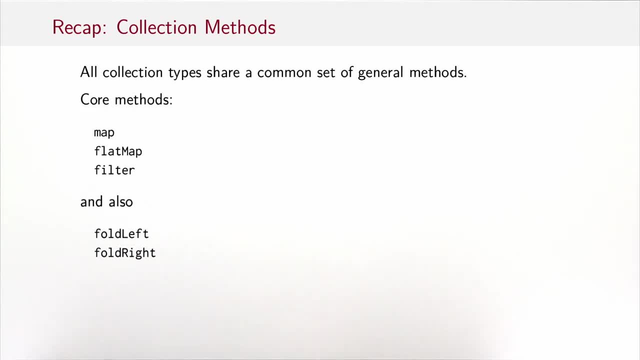 that satisfy a predicate. There's also fold left and fold right that do a reduction of a collection. that means they map the elements of a collection, with some binary operation, to a single value. Let's have a quick look at the idealized implementation of map on lists. 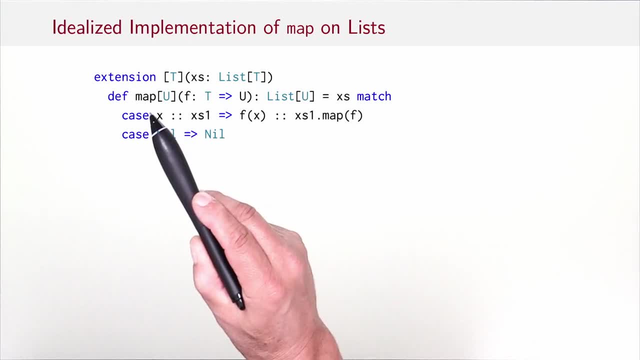 So map would be defined as an extension method that you see here. It takes a function from t to u, returns a list of u and it says: well, if the given list xs is non-empty, then it maps the first element using applying it to f. 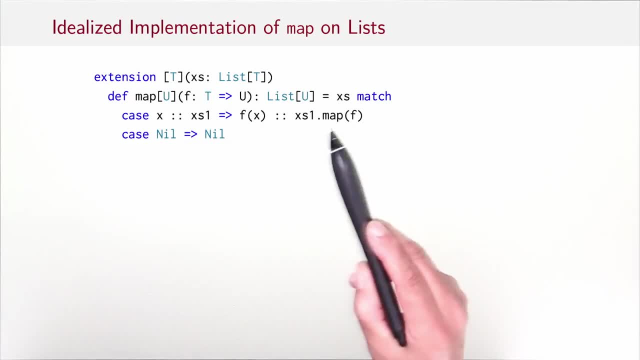 rather applying f to x and follows it with xs dot map f. If the list is nil, then the result is nil. Here's the implementation of flat map. It's almost like map. The only difference is flat map takes a function that returns lists of u's. 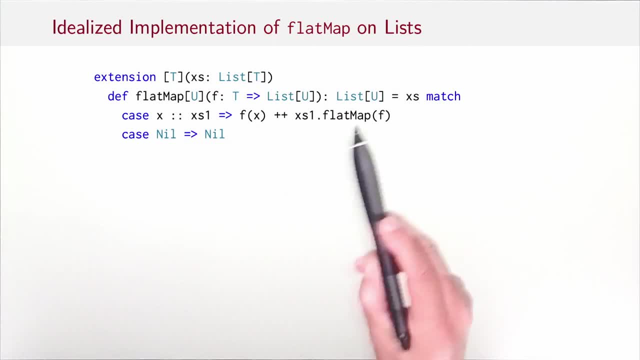 instead of single u's, and it concatenates the results with- not with cons, because that would give a list of lists, but with plus plus. So the list-valued result of f is concatenated with the result of xs. dot flat map f. 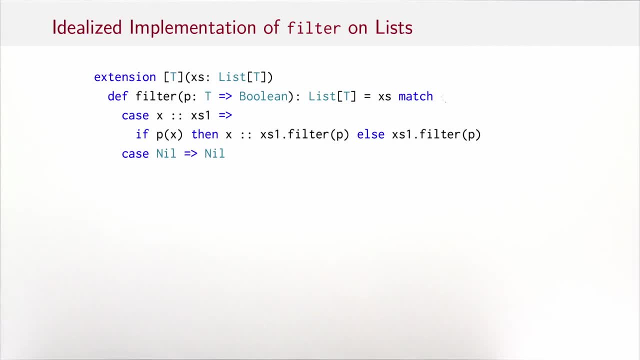 And finally we have filter, which can be defined like this: It's defined on xs of t's, takes a predicate from t to boolean and if the list is non-empty and the predicate is true for the first element, then it returns that element. 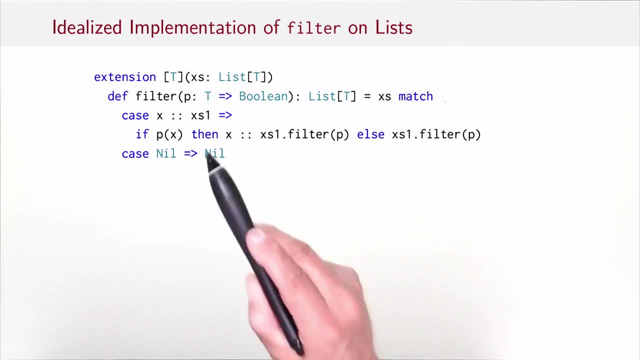 and the recursive filter of the rest of the list, and otherwise the first element is dropped and it just does the recursive filter of the rest of the list And, as always, empty lists are mapped to empty lists. In practice, the implementation of these methods. 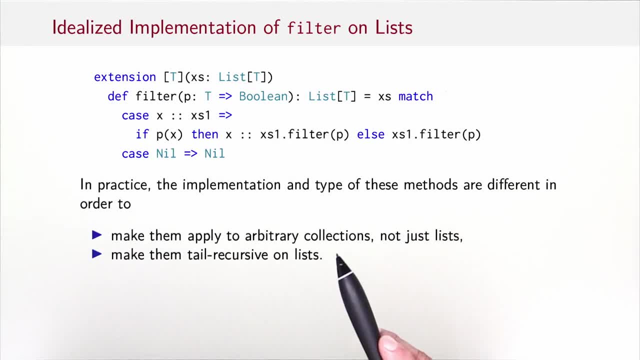 is a bit different, so that they can be applied to arbitrary collections, not just lists, and also to optimize them so that they can be tail recursive on lists. So these are some tweaks that are applied to the implementations of these methods, but you needn't be concerned with them. 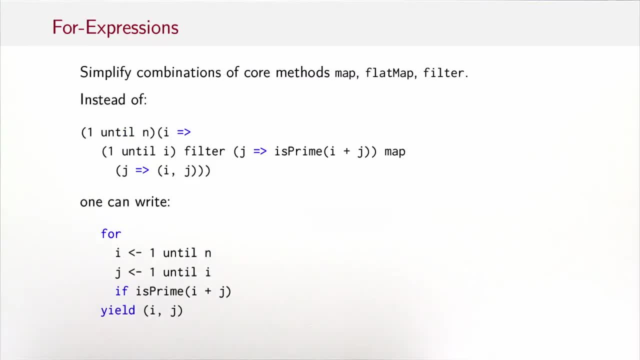 to understand how they work in principle. Besides collection operations, we also introduced forms, for example, for expressions, and for expressions they can simplify combinations of core methods: map, flat map and filter. So the example we've seen was instead of this rather incomprehensible expression. 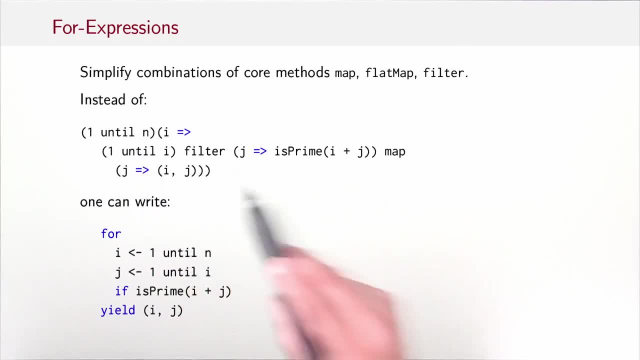 that essentially takes two ranges and then it does a map of a filter and whatever. we can write this, which is much, much clearer. So we can say: for i taken from 1 until n, so that's the range including 1,. 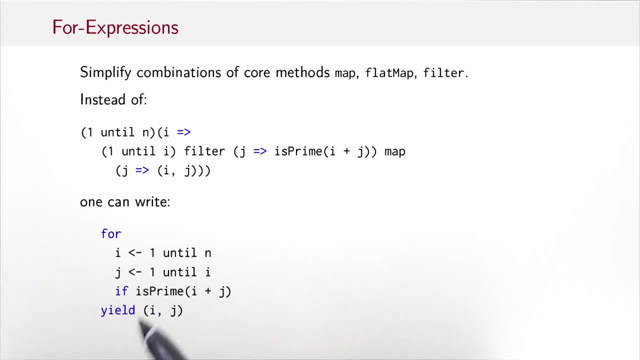 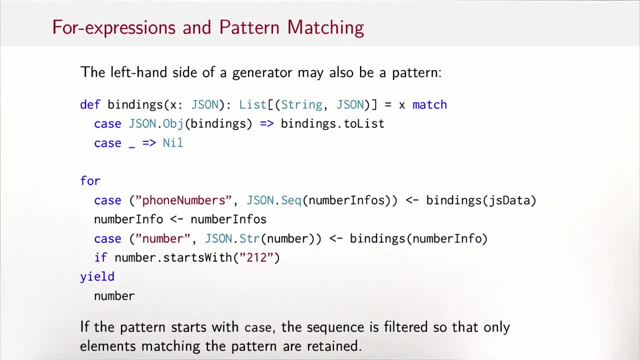 but excluding n for j, 1 until i. if i plus j is prime, then yield the pair of i and j. Here's something that we didn't cover yet in the previous six weeks, namely that the left-hand side of a generator of a for expression. 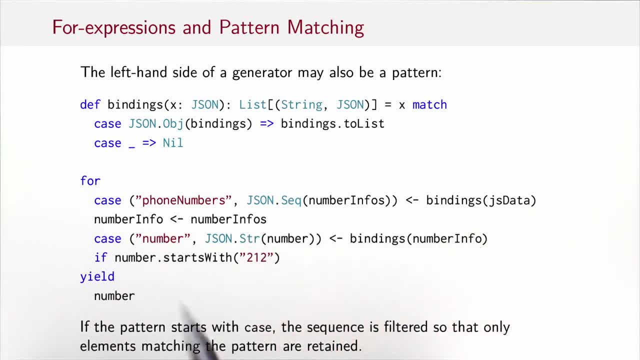 can also be a pattern. So previously we've seen only a single variable that is followed by the left arrow in a for expression. but in fact we can combine pattern matching with generation by placing a pattern on the left. So here's an example. 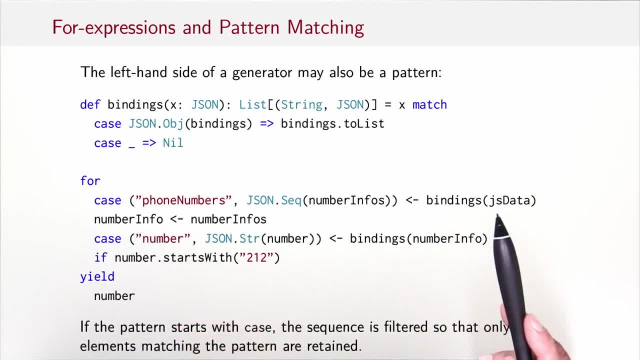 Let's say I want to get out of my JS data all phone numbers that start with 212.. To do that, I define an auxiliary method- bindings- that takes a JSON object and gives me, if it's an object, the list of strings and embedded JSON objects. 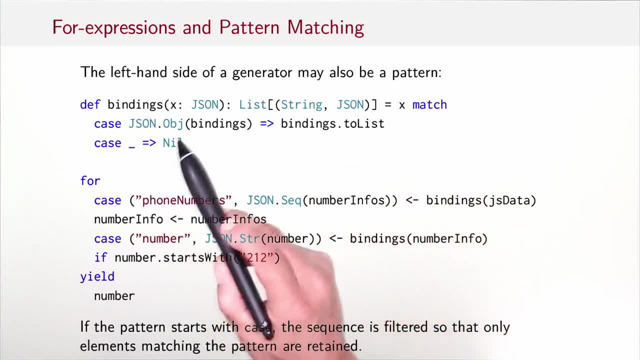 that make it up. So if x is a JSON object with bindings, then we convert the bindings to a list that gives us this list here, and otherwise we return nil to say that object doesn't have bindings. So now to get up the right phone numbers. 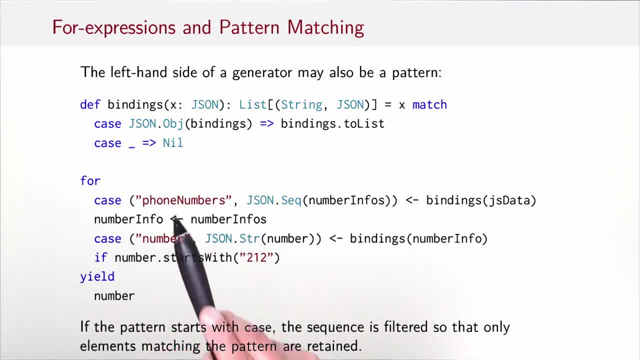 from JS data. we can write this, We can say for: and here we have a pattern: the binding that starts with phone numbers and that then on the right-hand side has a sequence of number infos. take that from the bindings of JS data. 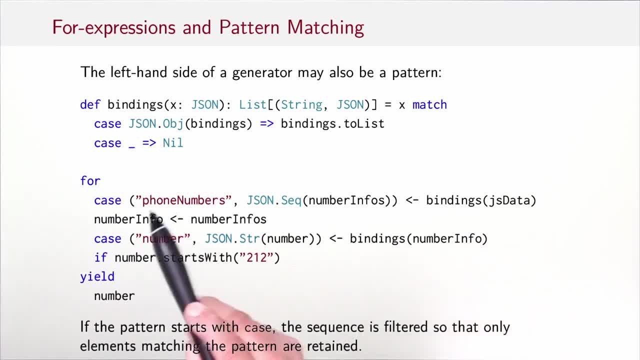 So what that does is it goes through all the bindings and the bindings that match this pattern. they are selected, Turns out there's only one in JS data, And then the fields that are embedded in the binding are recursively matched. So we would get the pattern match, to say. 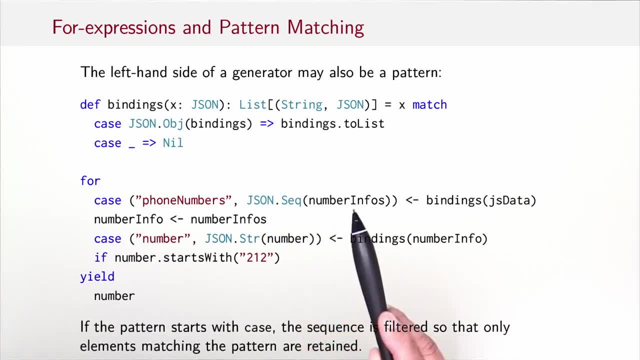 the right-hand side of phone numbers then would be matched against this pattern. here It is a sequence, So what's in the sequence would be matched with number info. Okay, so number infos is a list. We now let number info range over the elements of that list. 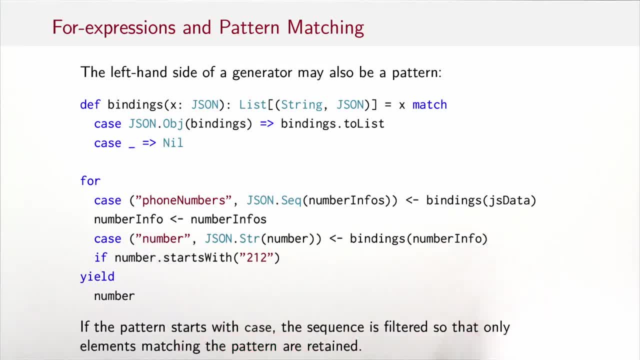 That gives us the info for each phone number in JS data. And that info for a phone number is another object. We take its bindings and we essentially match against the number field of that binding. So we want to find the number of that number info. 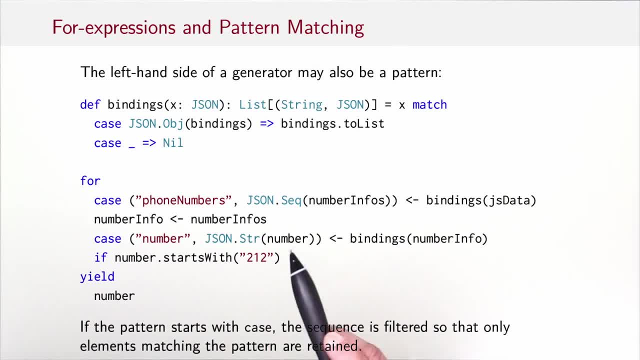 And that would have a JSON string on the right-hand side against which we match recursively. And then, finally, we have a condition: that that number should start with 212. And in that case we would return number. So we have combined in one four expressions. 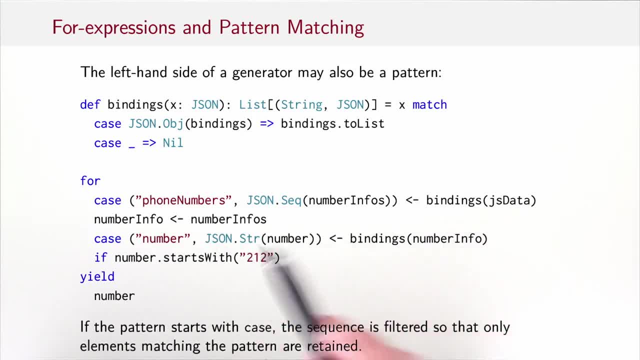 the traversal aspect- We generate essentially everything that is in here, in, here and here- And the filtering aspect. That means we only pick certain elements that match these patterns. To get the filtering behavior, you should prefix the pattern with case. If you leave out the case, 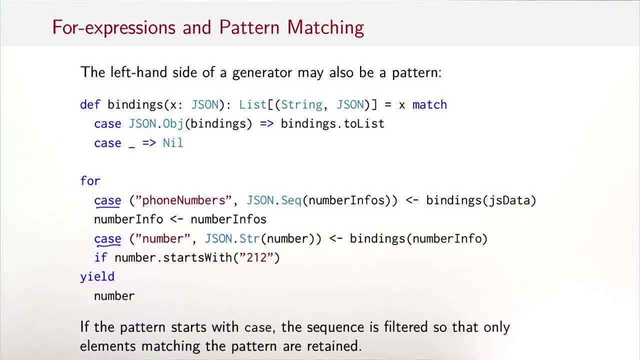 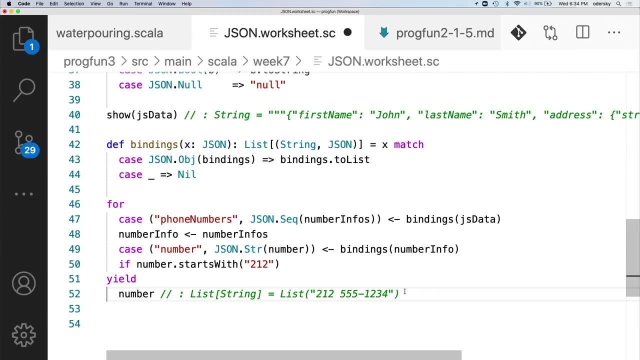 then essentially you are telling the compiler that your expectation is that every binding on the right will match that pattern. So case tells the compiler: please filter this. So if we add this code to the worksheet, then we will find that. indeed, yes, it pulls out the single phone number. 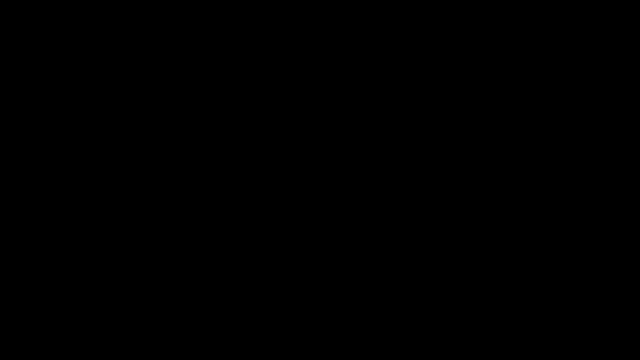 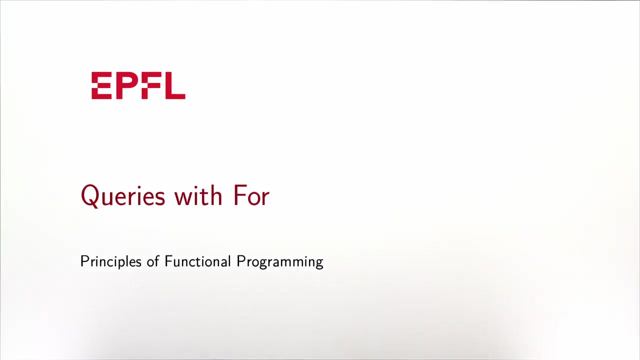 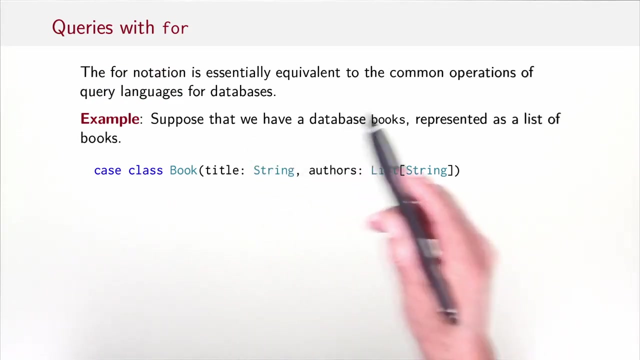 that starts with 212.. In this session we are going to look at how one can write common queries with four. In fact the four notation is essentially equivalent to the common operations of query languages for databases. To see that, let's do an example. let's say we have a little. 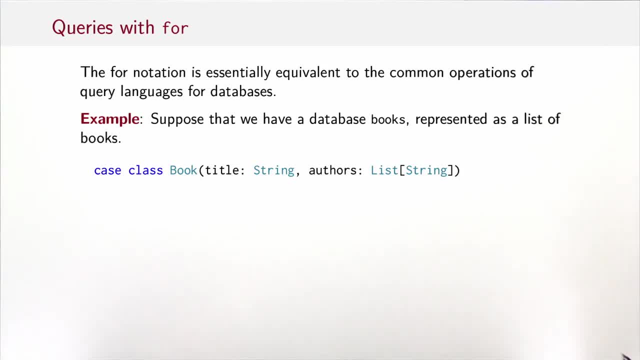 in-memory database of books and in this case we just represent it as a list of books where each book is a case class. The case class would have a title and a list of authors, which are all strings. Of course, often your database is much bigger than a simple list. 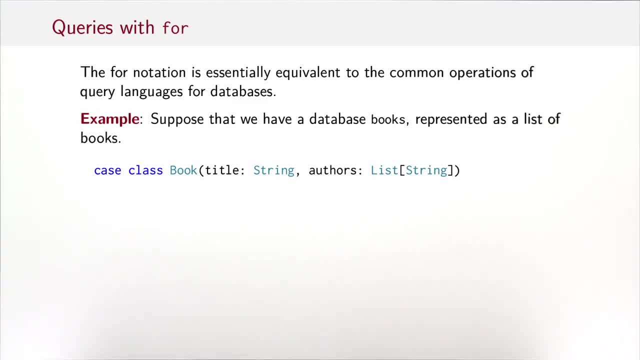 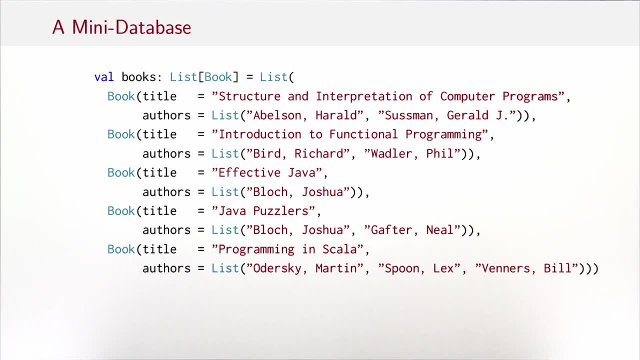 it could be a spark cluster or a postgres database on your computer, but the same principle applies for accessing all of these. So let's write our database. This is exactly big data, because it just contains five titles here. So here you have structure and interpretation. 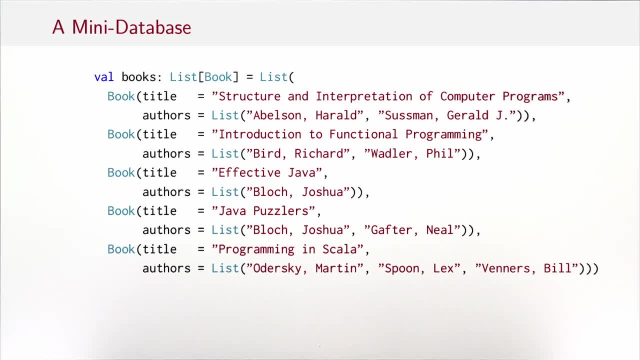 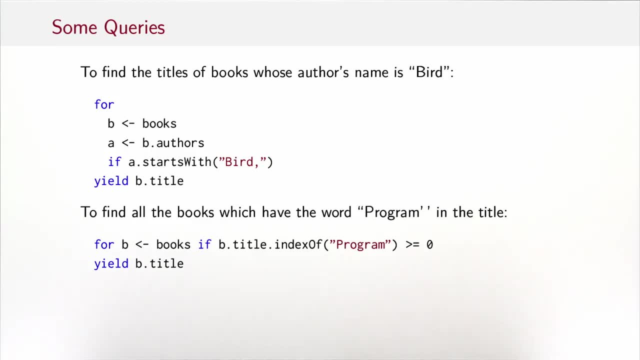 of computer programs, and here you have some other books in that library. Each book is an instance of the book case class, So here are some queries you might write To find the titles of books whose author's name is Bird. you could say, well, let B range over books. 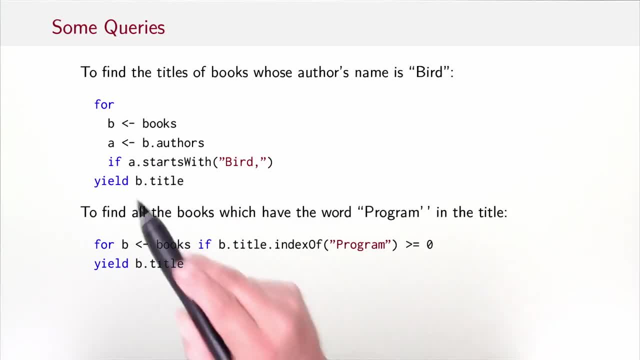 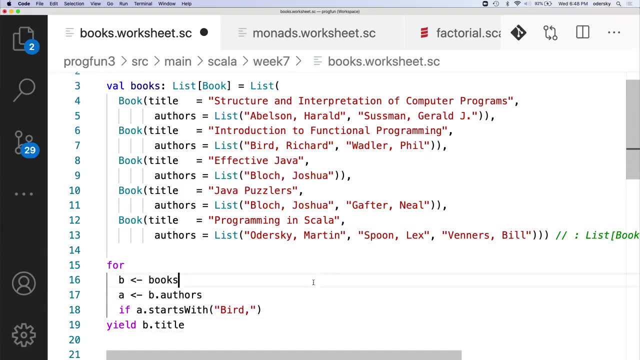 let A range over the authors of B. if A starts with Bird and then a comma, then yield B dot title. Okay, so let's see whether this works. I've written the query here and indeed I get the introduction to functional programming, which is the only book with Bird as the author. 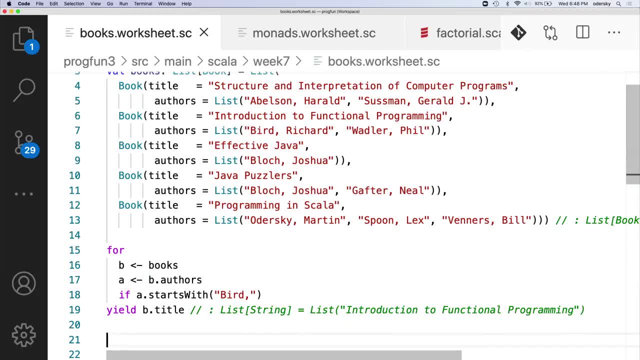 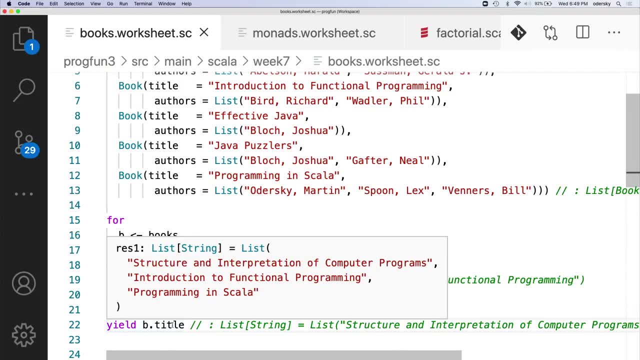 Or I could ask for all the books which have the word program in the title. So here's that query, and if I hover over that, I see that there are three books, and those are the three books that have the word program somewhere in the title. 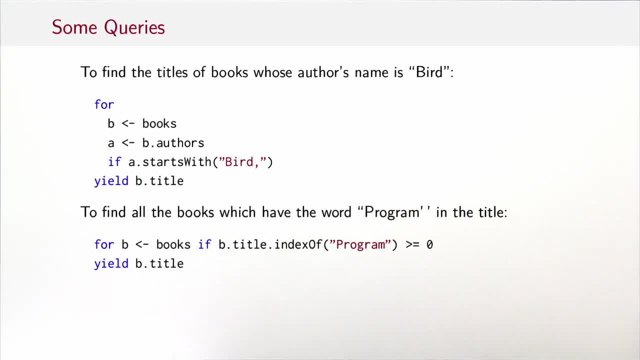 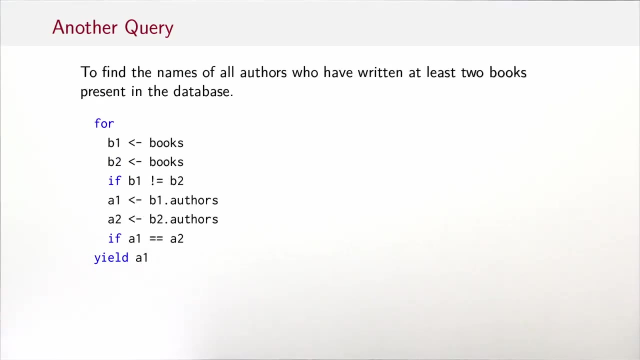 So you see that these four expressions, they are a very natural way to formulate what otherwise would be a database query. It's really quite natural. so it's a pretty obvious way to query databases or things that look like databases. So let's pursue this a bit further. 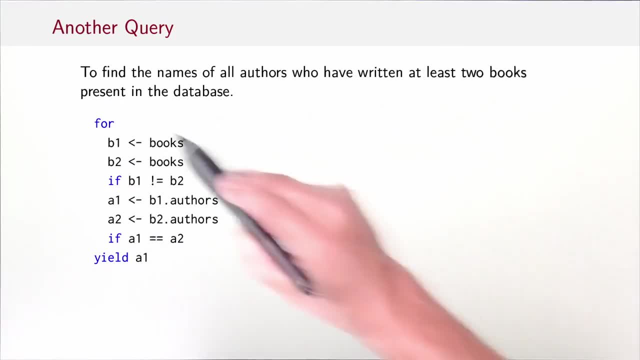 Let's find the names of all authors who have written at least two books that are present in the database. How would we do that? Well, we could say: let b1 range over the books and b2 range over the books. They must be two different books. 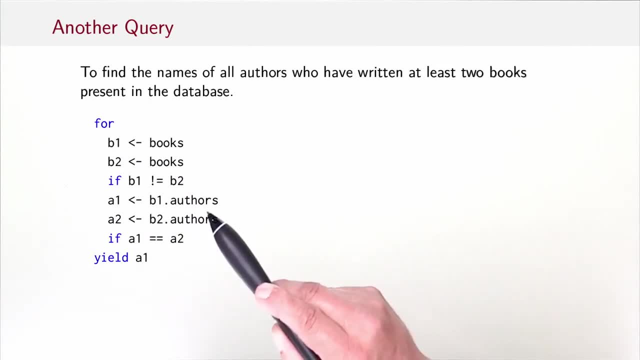 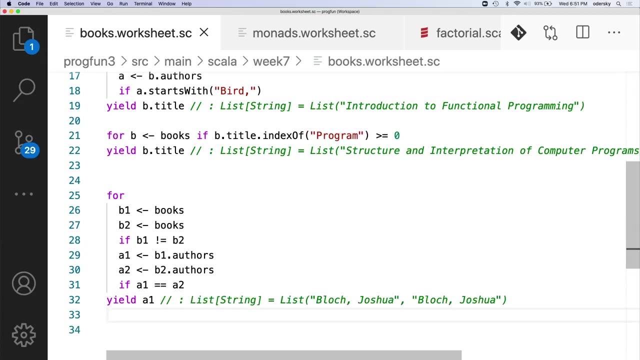 so that's a condition. Then let a1 range over the authors of b1 and a2 over the authors of b2.. If the authors are the same, then we have a hit and we return a1.. So let's look at what we get here. 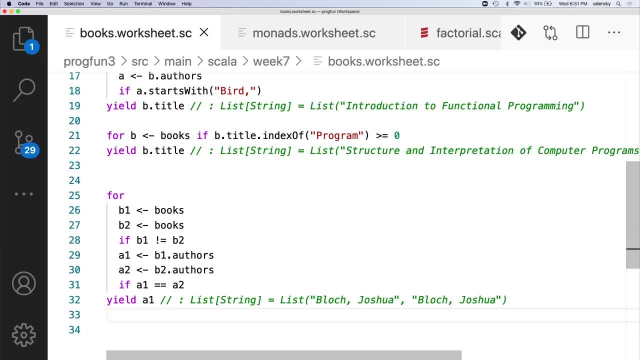 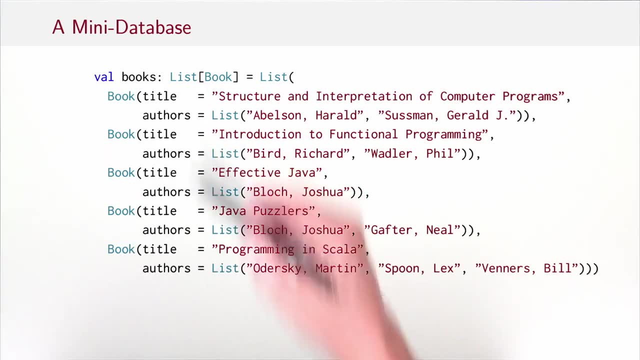 We get Bloch Joshua, Bloch Joshua. Why is that? We return the list of all possible pairs of books here And if you look through the book list then there are two pairs of books that match that. One is Effective Java and Java Puzzlers. 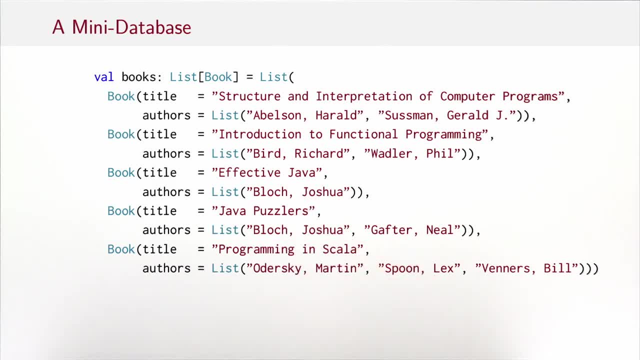 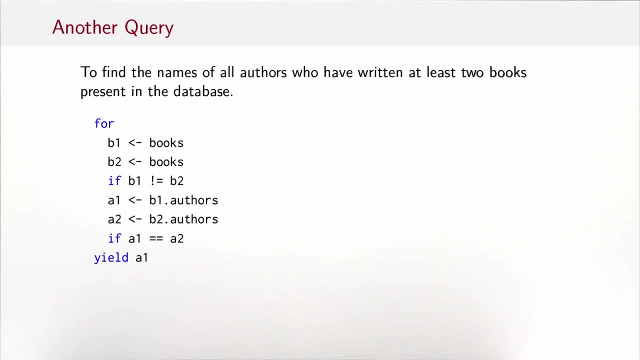 and the other is Java Puzzlers and Effective Java. So that's why the name appears twice. Can you think of a way to modify the query to prevent the duplication? Well, one thing we could do is we could discriminate and say that first in the pair of books. 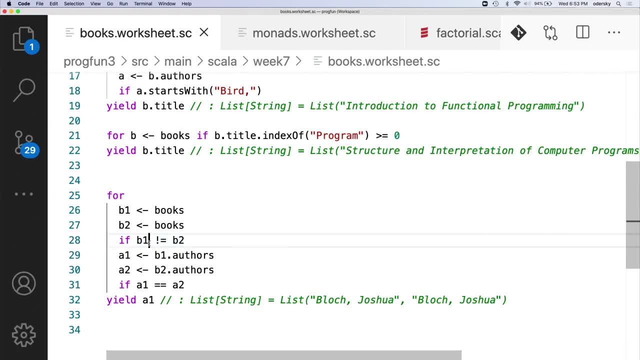 the first book must always have a title that is lexicographically smaller than the second book. So instead of saying b1 different from b2, we say b1.title is smaller than b2.title, And that would work, because now we have essentially only one pair. 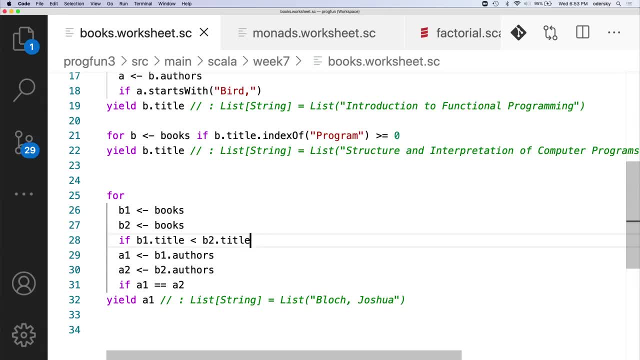 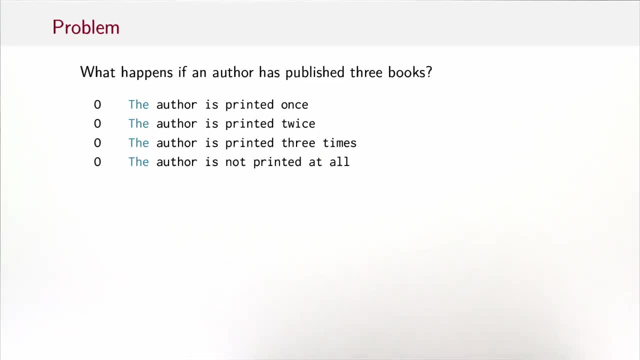 the pair that starts with a lexicographically smaller title. that is the left element of the pair and the other the right one. But does it scale? So what if an author has published three books? What would we get now with the new solution with the comparison of titles? 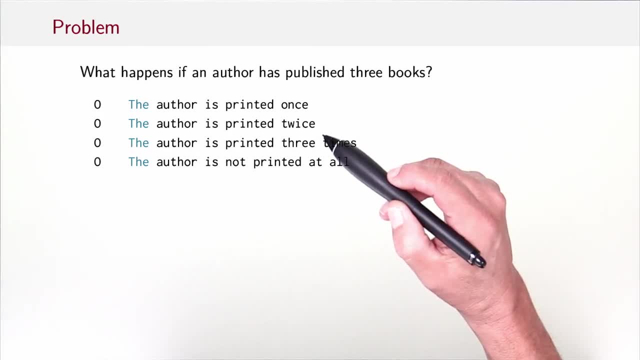 Would the author be printed once Or twice Or three times, Or maybe not at all? In fact, the answer is the author would be printed three times Because if you have three book titles, let's say a, b, c, then there are six possible pairs. 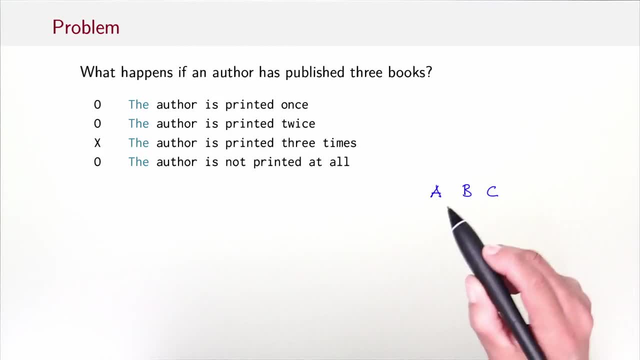 and three possible pairs where the first one is smaller than the second, namely a, b, b, c and a c. So for each of these pairs the author would show up. So we need a more robust way to deduplicate the authors. 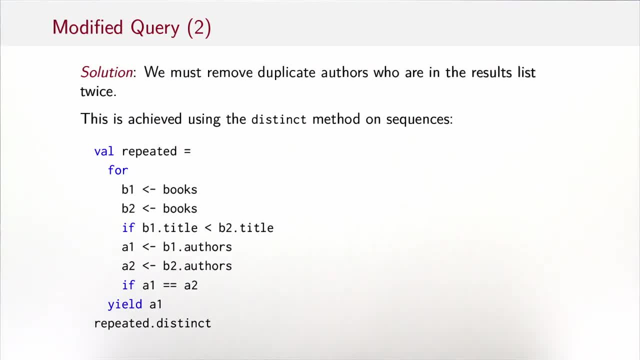 So one way we could do is we could use the distinct method on sequences. So here we define the query as before, name it repeated and then finally return repeateddistinct. So distinct would keep each element in the repeated list only once. Subsequent copies of the same element. 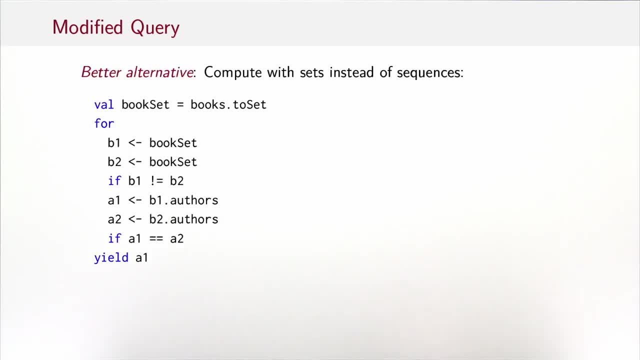 would be omitted. Or we could attack the problem at the root and compute with sets instead of lists, because after all, if you want to remove duplicates from the results, then we shouldn't introduce those duplicates in the first place. So by going to sets, we avoid any duplicates. 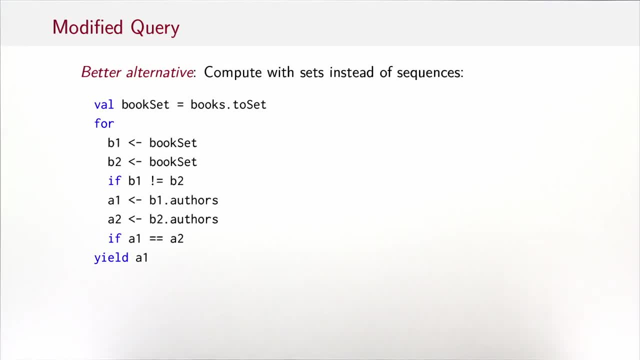 every set can contain an element only once. So what we could do here is we can write bookset equals books to set and then have the query range over sets, and that would also deduplicate all the results of the query. I can show that here in the worksheet. 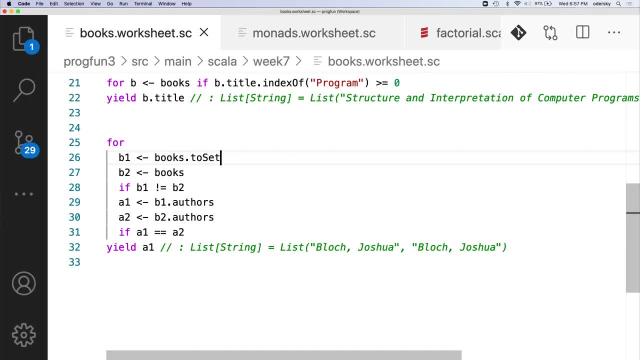 So that was the previous query. that contains the duplication and it actually suffices that we convert the first books to set, because then afterwards essentially all the computations will be done on the first collection type which is set. So that would now give us not a list with Brock Joshua twice. 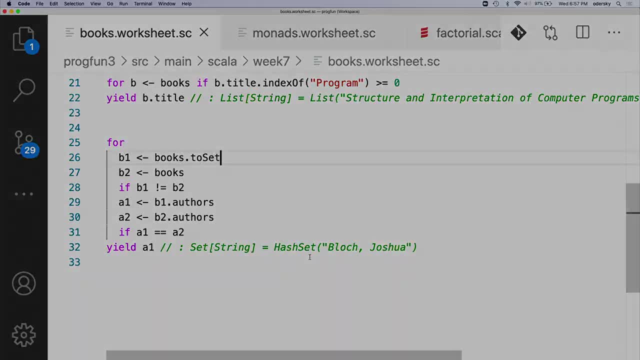 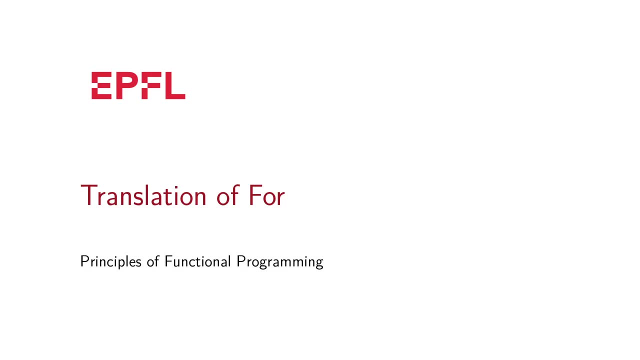 but a hash set where he appears only once. In this session we're going to look at the translation of four expressions. Four expressions have been a little bit of a mystery so far, in that we haven't really explained what they mean. I mean they're very natural. 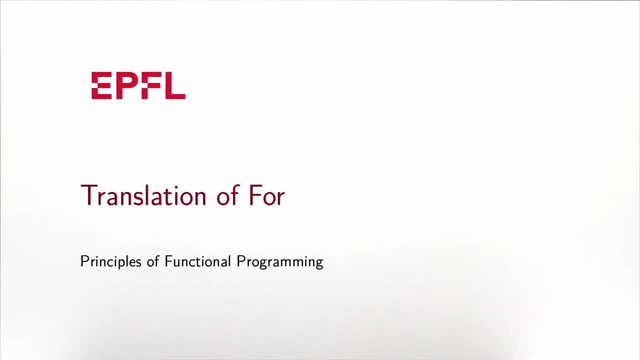 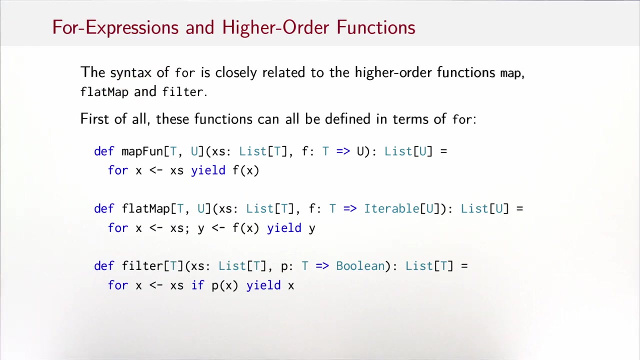 but you haven't seen a rewrite rule using the substitution model for them, for instance. In fact, what happens is that four expressions are translated to simpler elements that you know already, And in this session we will explain that in detail. So you've probably noticed already. 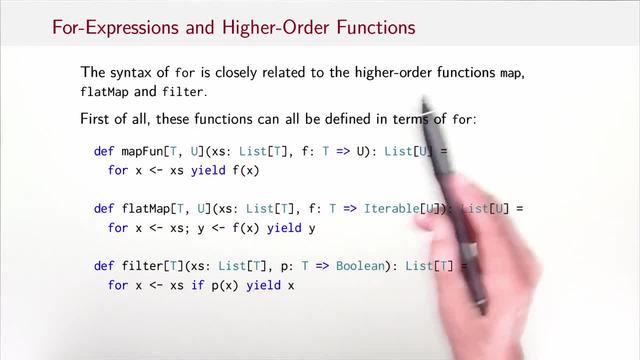 that the syntax of four is closely related to three higher order functions, namely map, flat map and filter. The first observation is that these functions can all be defined in terms of four. So we could define a function which is like map. let's call it map fun. 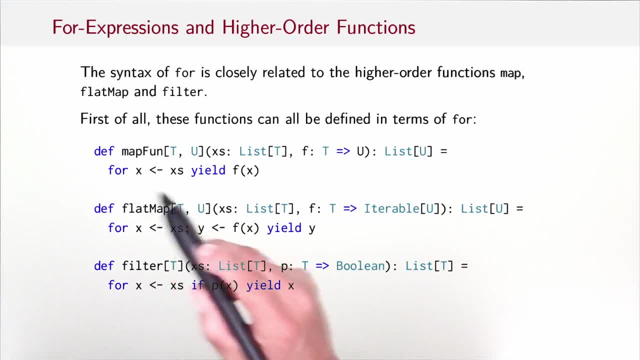 over xs and f. and map fun is just let x range over xs, yield f of x. That's the same as mapping f over xs. Or to do flat map over a list xs with a function f, we could let range x over xs, let range y over the result of f of x. 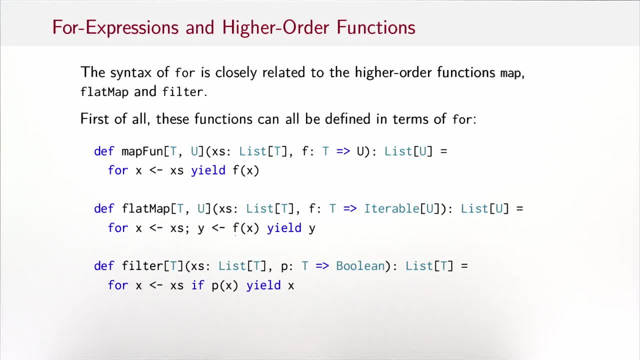 and yield y. That's in fact flat map. Or to do filter over a list xs with a predicate p. we let x range over xs. if p is true, then we yield x, otherwise we yield nothing. So these three methods can be naturally defined in terms of four. 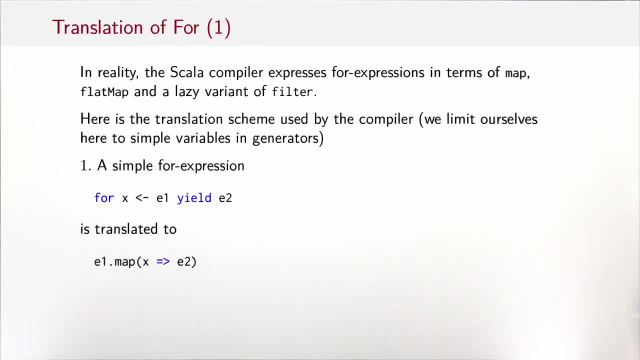 But in fact in reality it goes the other way around. The Scala compiler expresses four expressions in terms of map, flat map and a lazy variant of filter. Here's the translation scheme used by the compiler. We limit ourselves here to simple variables and generators. 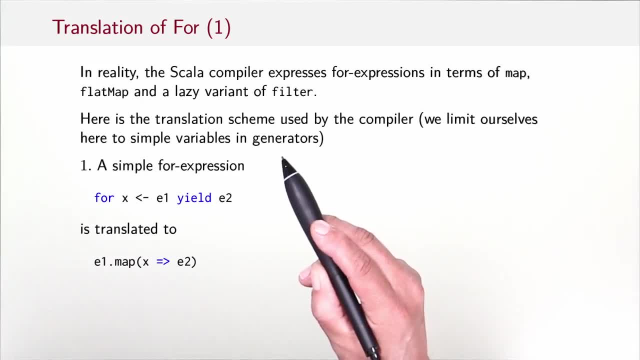 so this scheme also extends to patterns, but here we won't explain in detail how that works. So if we have a simple four expression, say for x taken from a generator e1, yield e2, then that's a map. so it's translated to: e1 dot map. 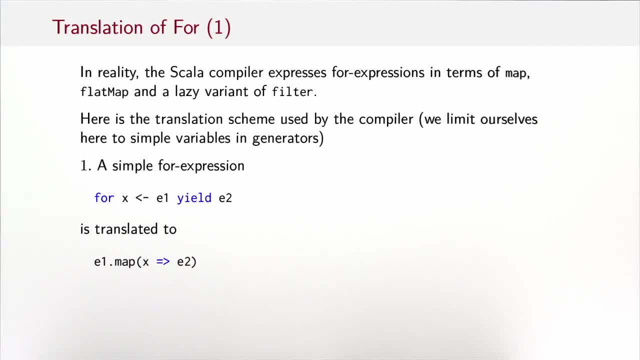 with the function that takes an x and returns e2.. So you see that we respect variable bindings here. The x is visible in e2 and it's also visible in the translation, because it is the parameter of a lambda that has e2 as its body. 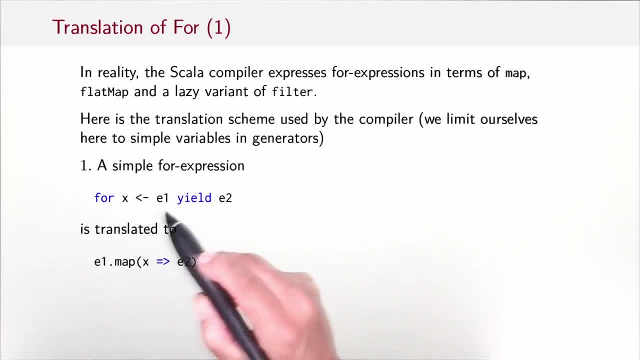 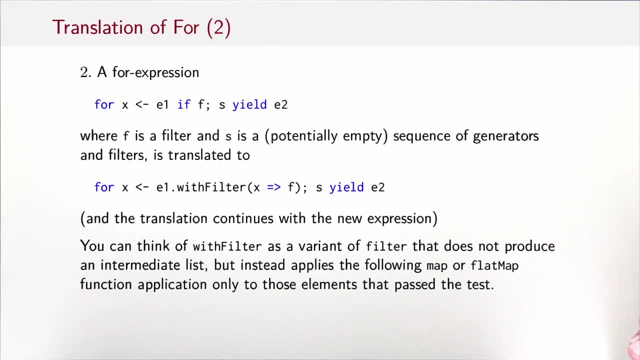 So that was the simplest case where our four expression consisted of exactly one generator. We now handle the cases for when the generator is followed by something. Let's assume first the generator is followed by an if and then possibly some other sequence of generators and filters. 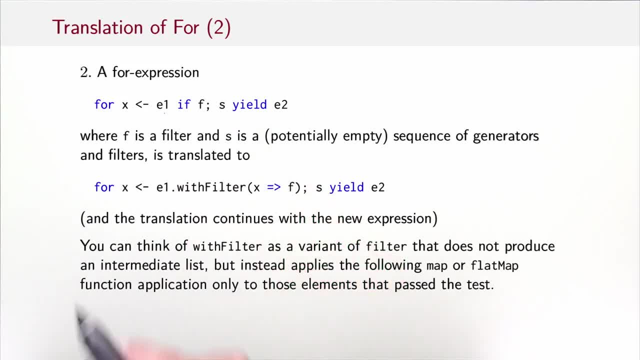 So we have a four expression of this form. That four expression is translated to what you see here. It's the four expression that uses the same generator, e1, but followed with a filter of the predicate that maps x to f. Then that's followed by: 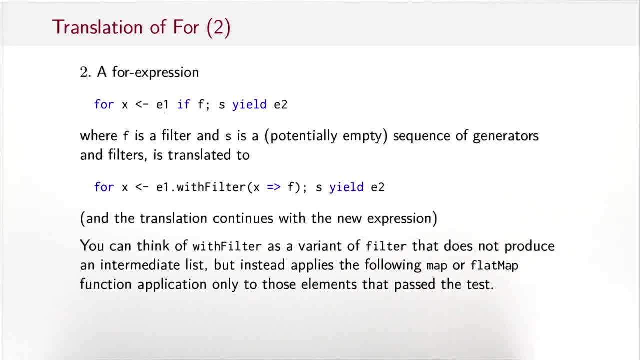 whatever followed the filter before, and the translation continues. You can think of with filter as a variant of filter that does not produce an intermediate list but instead applies the following map or flat map function application only to those elements that pass the test. So essentially, with filter is like filter. 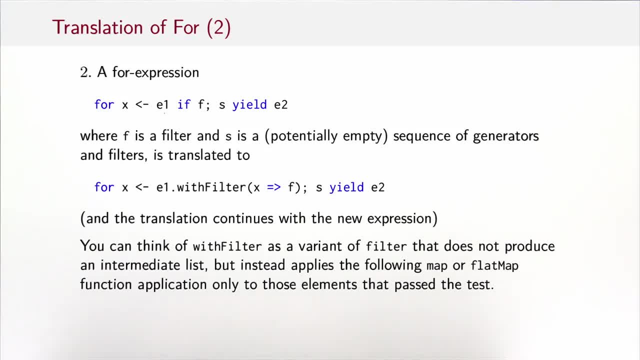 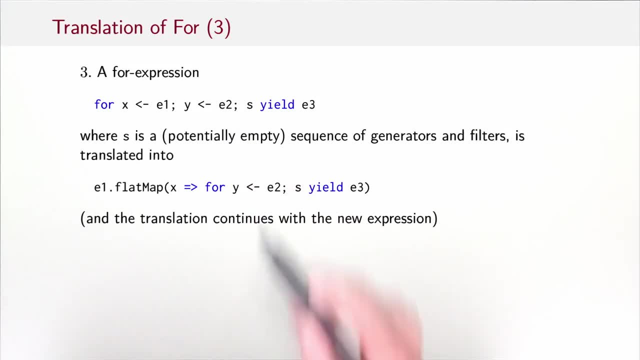 but it avoids the creation of an intermediate data structure. So the last remaining case is if our leading generator is followed by another generator and then possibly a sequence of filters and generators. That template is translated to what you see here, So the tail here. 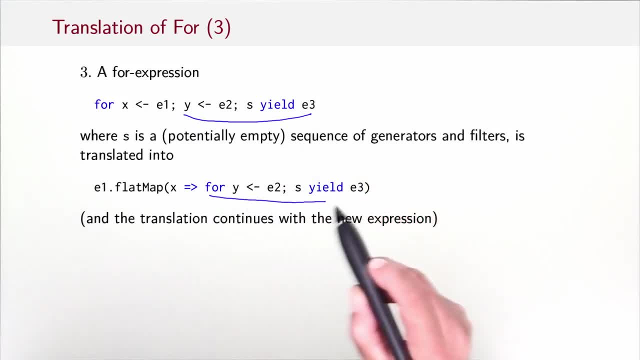 the remaining four expression you find here again. So that will give you a collection valued result. and then the results of that inner four expressions are concatenated via a flat map. So again we can verify that the variable bindings all work out. So the x here. 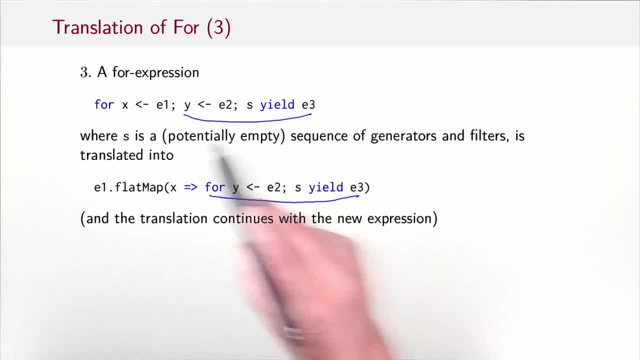 is visible in the remaining code from y to e3. and that's also the case here, because we have a lambda where we bind the same variable x, And once we have that, of course that inner four expression might itself be complicated. so translation continues recursively with that. 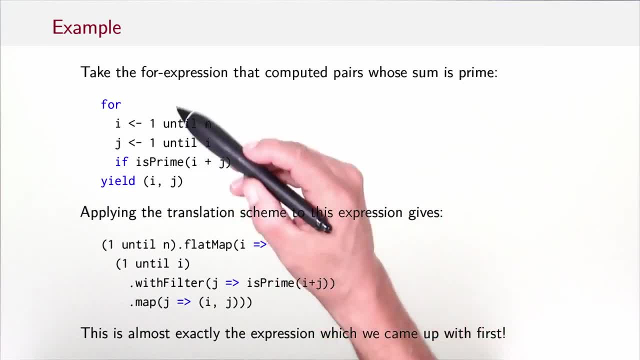 So as an example, take the four expression that computed pairs whose sum is prime, that we've seen already. So for i, taken from 1 to n, j taken from 1 until i, if is prime i plus j, yield i comma j. If we apply the translation scheme. 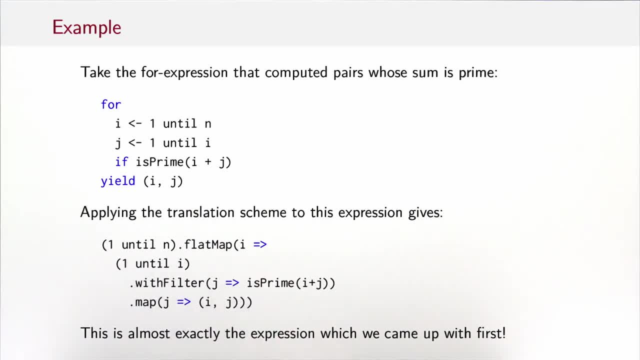 that we have seen. that's what we get. So it's exactly this expression here, which is almost exactly the expression which we came up with first before we mapped into the much clearer. it works in the other way. it translates a high level four expressions into low level code. 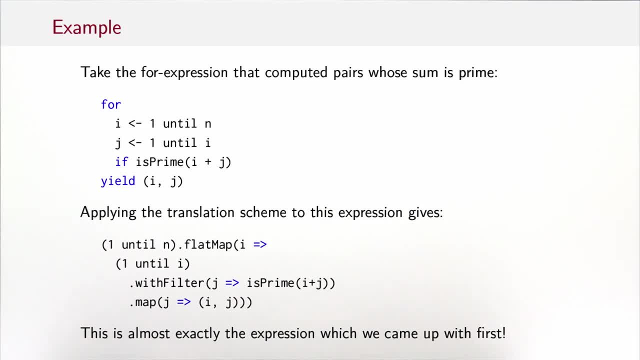 that, for our eyes, looks more obfuscated and less clear than the original four expression. On the other hand, that code that it maps to doesn't contain any four expressions anymore, it's just function applications, and we know how to deal with that in our substitution model. 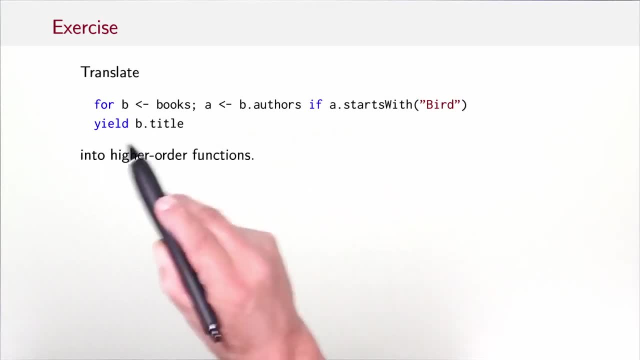 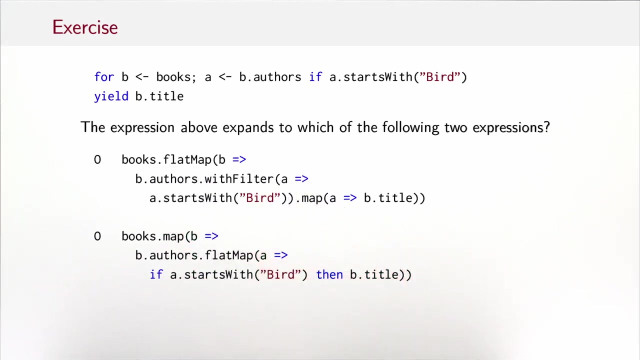 So here's an exercise for you: Translate the query here about books that you have seen already into higher order functions using the translation rules that we have just covered. What did you come up with? The expression above translates into one of the following two expressions: 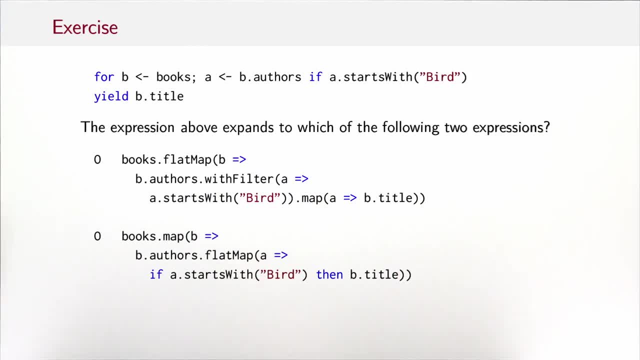 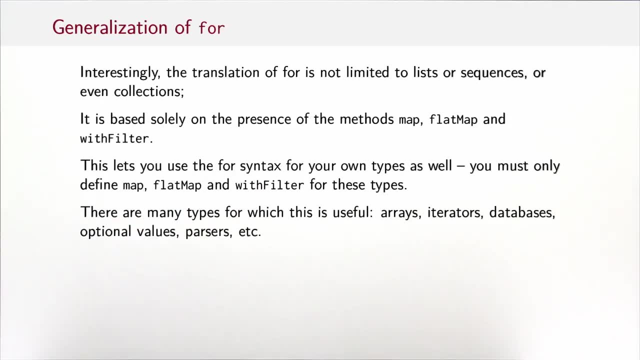 Which one? is it The first one here or the second one here? Well, if you've applied the rules correctly, you'll find out that the answer is the first one. So one interesting aspect of the translation rules for four that we've covered is that 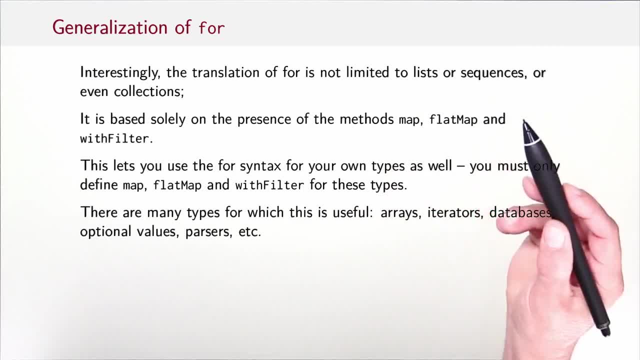 it's not limited to lists or sequences or even collections. All we need for the translation is the presence of the methods map, flatMap and withFilter on the data in question, And that means you could use the four syntax for your own types as well. 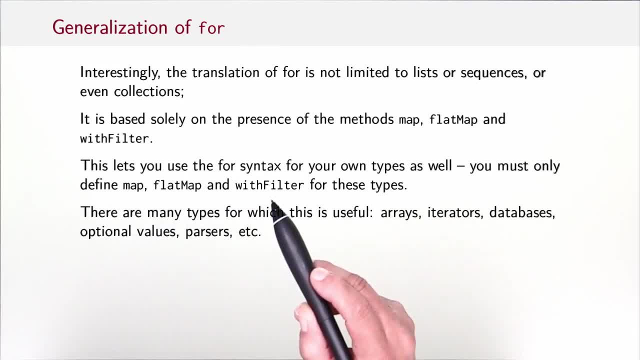 You must only define map, flatMap and withFilter for these types and you're done. It turns out there are surprisingly many types for which this is useful. Obvious examples are arrays or iterators, but also databases, optional values, parsers, random numbers and so on. 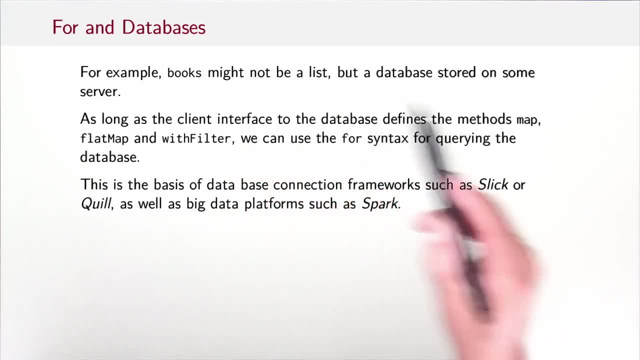 For example, books might not be a list but a database stored on some server or some cluster of servers. As long as the client interface to the database defines the methods map, flatMap and withFilter, you can use the four syntax for querying the database. 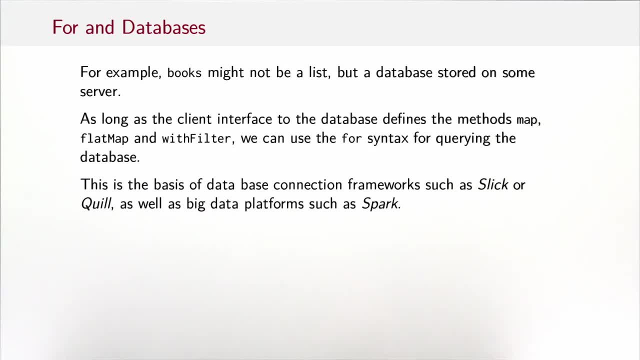 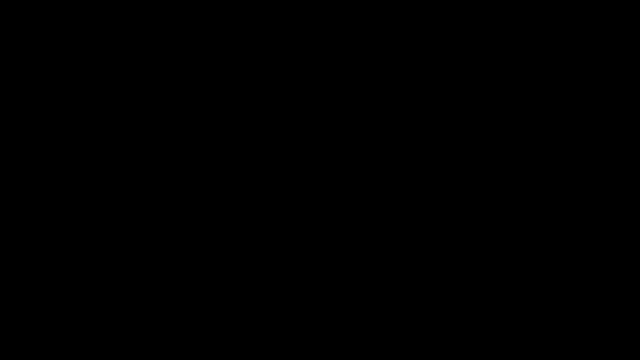 That's, in fact, the basis of many database connection frameworks in the Scala ecosystems, such as Slick or Quill, and it's also the basis of big data platforms such as Spark. In this session, we'll learn about a new abstraction which is very useful in testing. 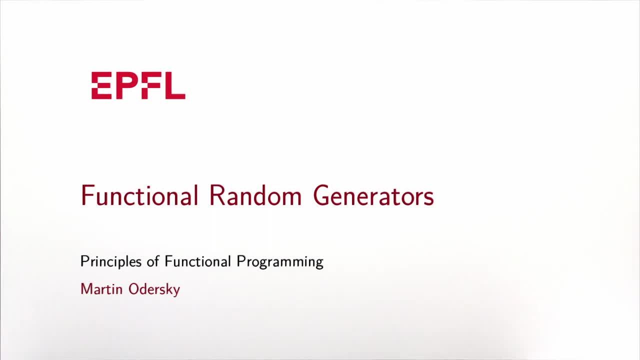 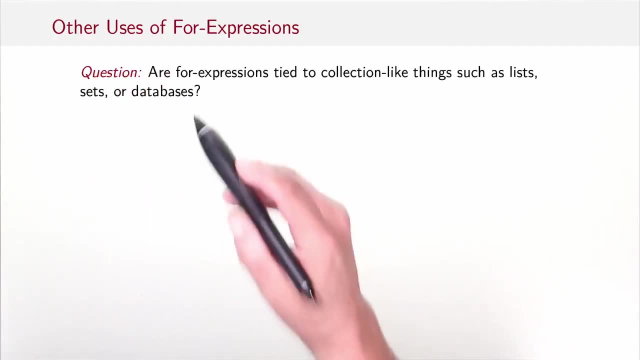 namely functional random generators. A question: Are four expressions tied to collection, like things such as lists, sets or databases? The answer is not really. All that's required is some interpretation of map, flatMap and withFilter, because in this case you can use the four syntax. 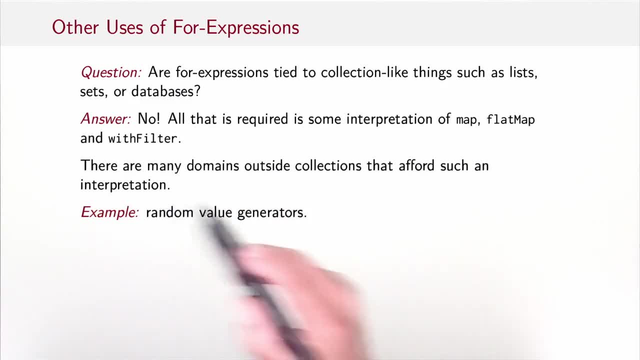 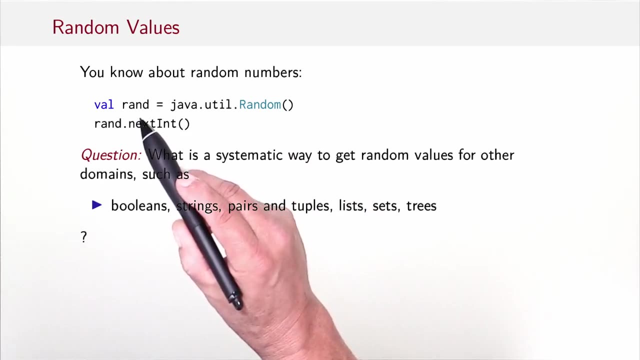 because that's the translation target of four expressions. There are many domains outside collections that afford such an interpretation. An example are random value generators. You probably know about random numbers from languages such as Java. So in Java you would create a random number generator like this: 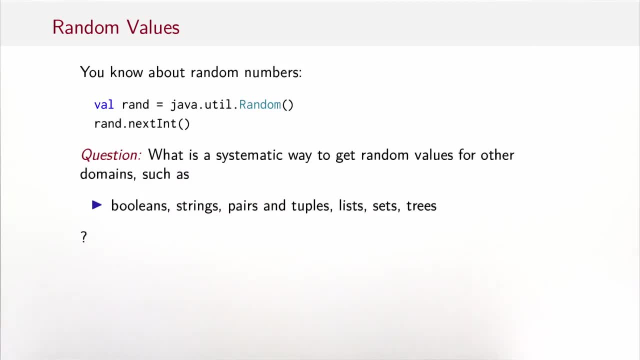 You invoke javautilrandom. that gives you a generator called rand here, and then you would get the next random number by calling randnextInt. You can do that arbitrarily often and each time you will get a new random number. So that works for integers. but the question would be: 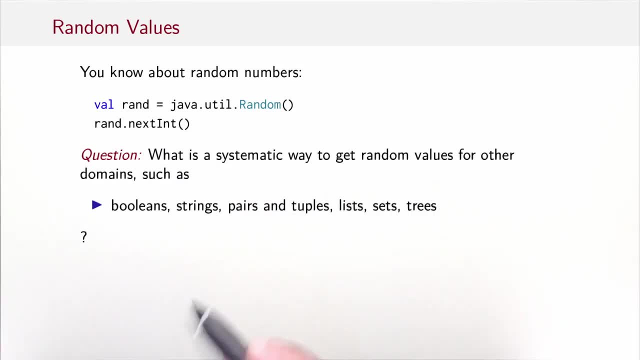 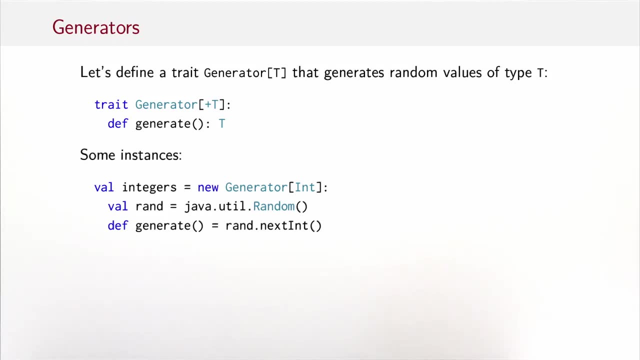 what are systematic ways to get random values for other domains, such as booleans, strings, pairs, tuples, lists, sets or trees. So that's what we are going to do now: We are going to define a trait generator of T that generates random values of type T. 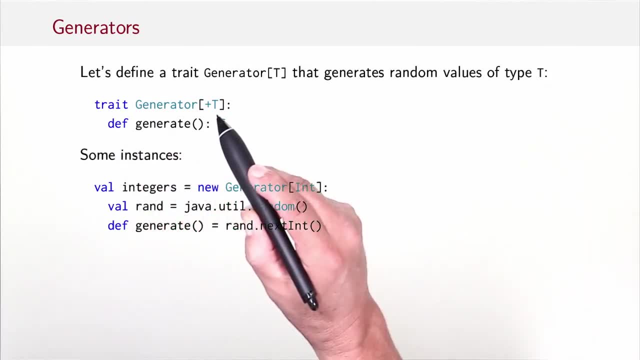 So here's the trait: It takes a covariant type parameter T and it has a generate method that, when called, returns a new random value of type T. Here's a possible instance of generator The integers. So that would be a generator of type int. 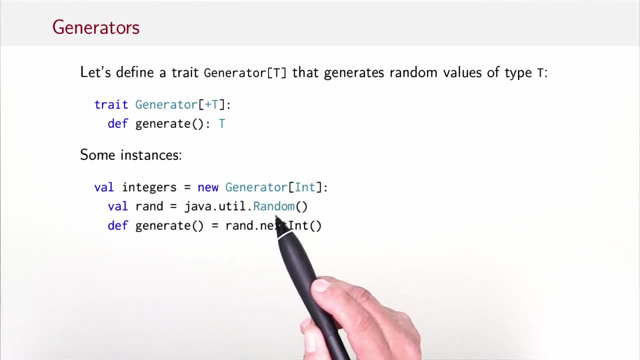 We create a new random value generator, so that's essentially our root generator, and then to generate a new integer we just call randnextInt, So it's just a wrapper around javautilrandom. really, What about generating random booleans? So here's a way to do it. 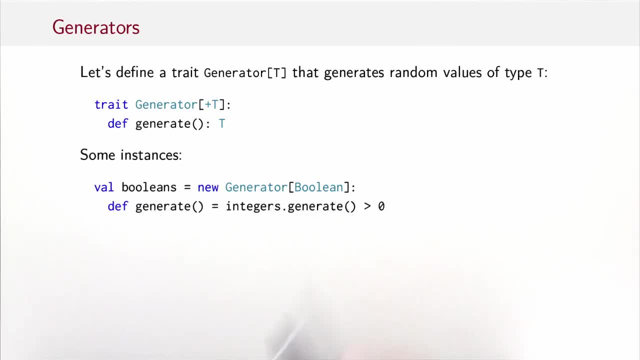 We define a val booleans. It's a new generator of type boolean and its generate method would call the integers generate and ask whether the result is greater than zero. So one half of the values generated by the integers generator would be greater than zero. so that would give true. 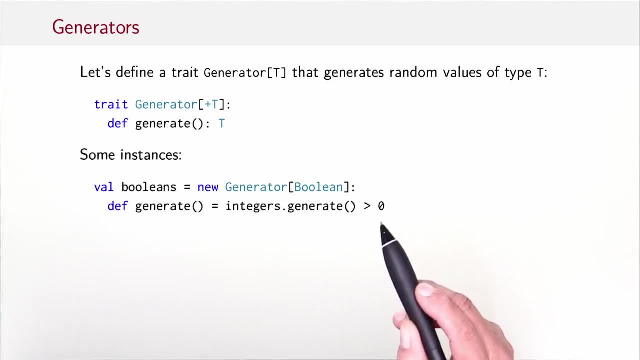 and the other half would be less than or equal to zero, so that would give false. Another thing we might want to do is generate random booleans. For that we define a new generator boolean. Its generate method calls the integers generate method and returns true. 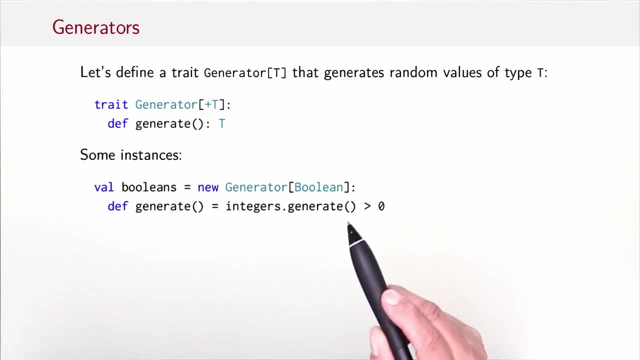 if the result is greater than zero and false. otherwise About half the values returned from integers generator will be greater or zero. so the distribution is about one half for true and false for the booleans generator. What about structured random data? It's a simple case. 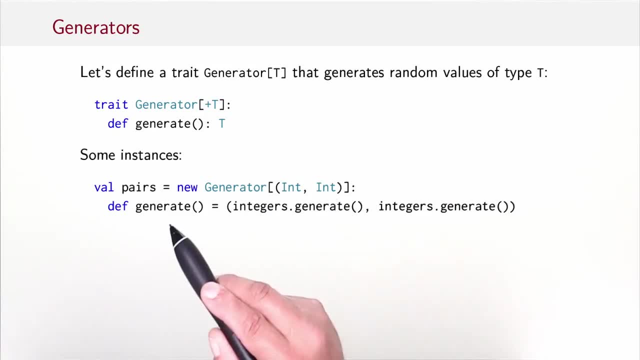 We define a generator for pairs of random integers. Its generate method would call integers: generate twice: once to produce the first half of the pair and the second time to produce the second half of the pair. So I've put what we have in a worksheet. 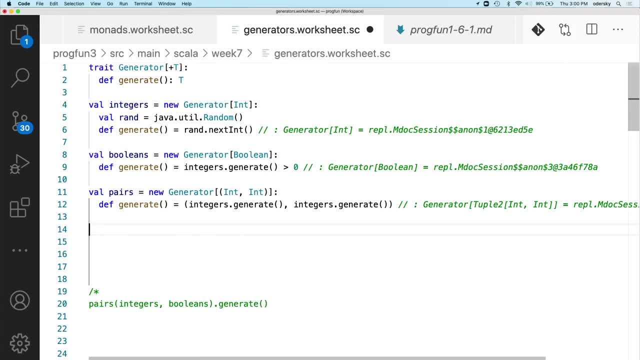 Let's test maybe by writing pairsgenerate, So that would give us two numbers, and if we call it again by saving again, it would give us two different numbers, and so on. That's the random number generation network. So you might object, haven't we left? 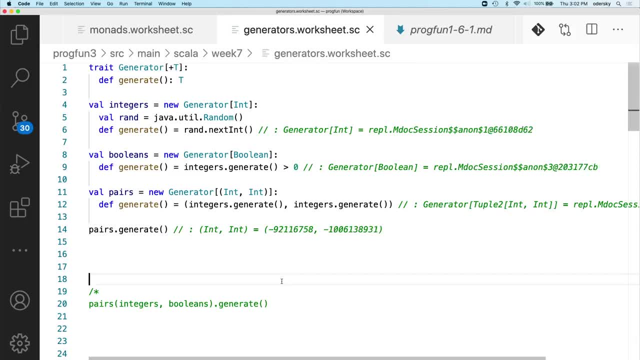 the domain of purely functional programming. after all, the more often I save this expression, I get a different value each time. so that's not really functional, is it? And I'd have to agree with you. The one saving grace here is to say: well, it doesn't really matter. 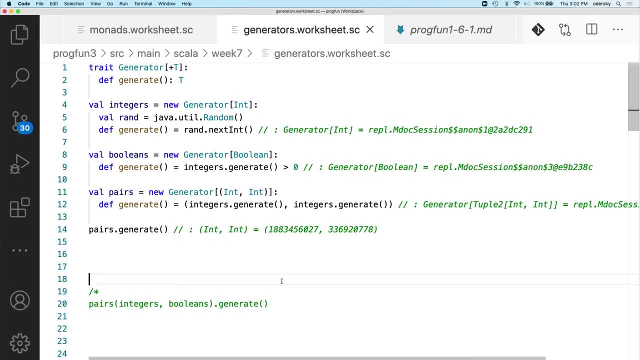 what the actual random number is. the whole point of random numbers is that they are random. One number does just as well as the other. So in that sense, while we are definitely outside purely functional programming, we are so in a relatively benevolent way. So as a next step, 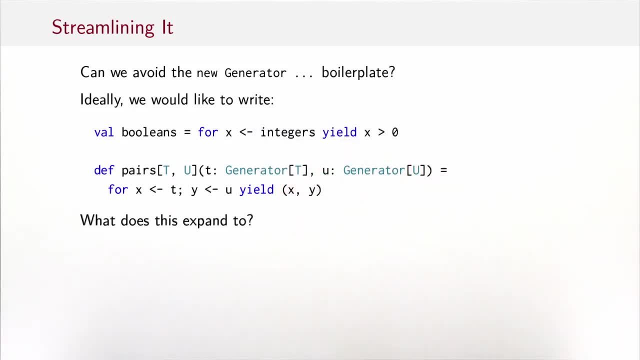 can we avoid the generator boilerplate, that every generator we create has to be a class instance of an anonymous class and we have to overwrite the generate method, and so on. Ideally, what we would like to write is this: we would like to write: well, booleans. 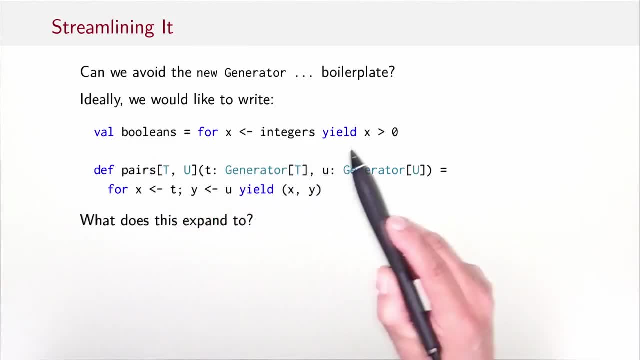 is: let x range over the integers, yield x greater than zero or def pairs of t, u. it takes a generator of t and it takes a generator of u and it gives you back any x ranging over t, y ranging over u, the pair of x and y. 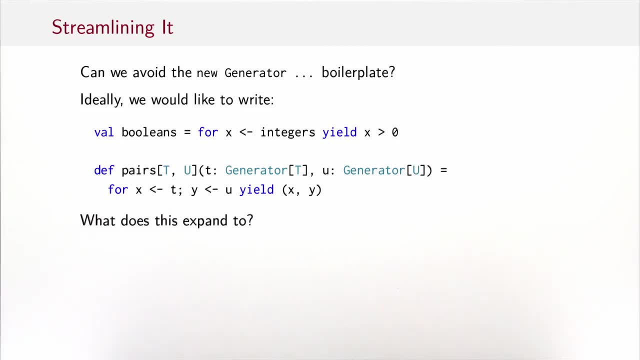 so in a sense that's more a streams view. we are no longer looking at individual random numbers, but at the stream of all random numbers that are generated, That's, the integers, and we convert that stream by saying well, to convert it to a stream of booleans. 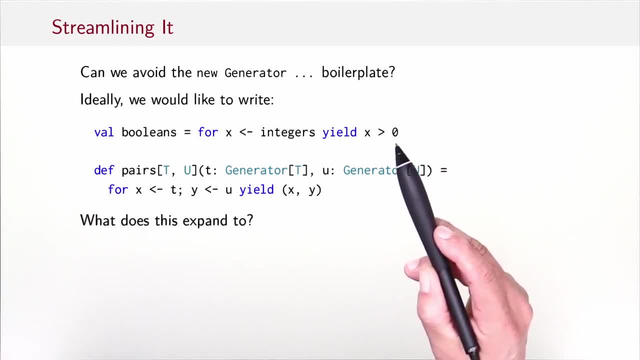 we just ask, each for each element, whether it's greater than zero. Well, here we produce a stream of pair random numbers by essentially composing the stream of t random numbers with the stream of u random numbers. So how do we achieve that? Well, what do these expressions expand to? 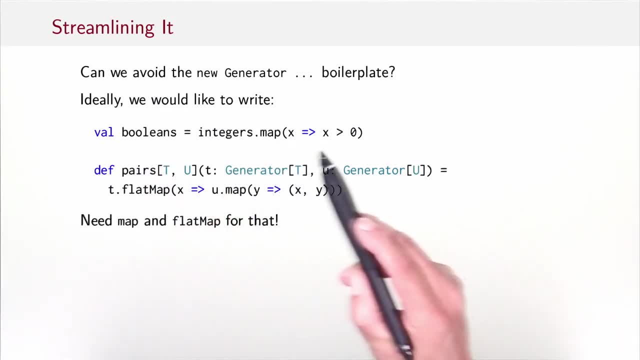 The first expression expands to integers: dot map x, x greater than zero. The second expression expands to a flat map of a map of the pair construction, as we have seen when we looked at the translation of four expressions. Ok, so to be able to do that. 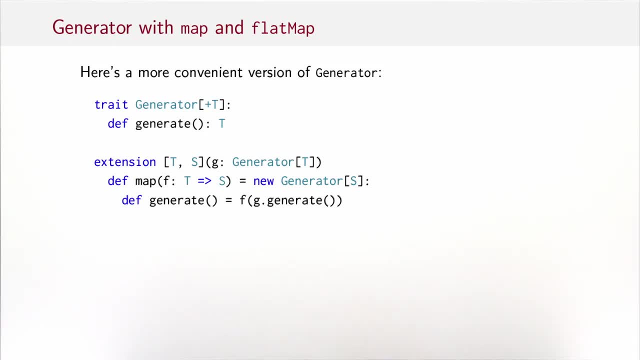 we need map and flat map. So here's how we can dress up generator to provide this new syntax: We just have to add map and flat map to it. So let's do that with extension methods. The map method you see here. it takes a generator of t. 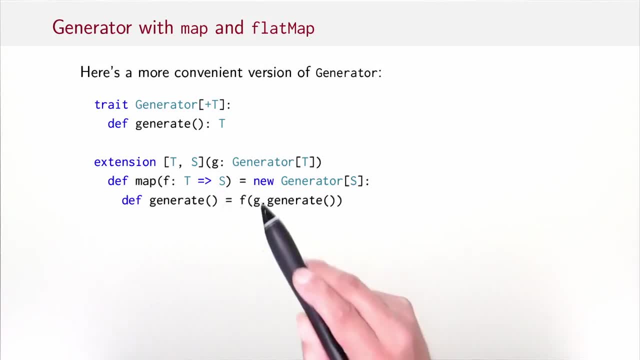 and a function from t to s, where s is some other type, and it creates a new generator of s whose generate method calls the g generate the original generate and transforms it with f. So that was map. What would flat map look like? Here it is. 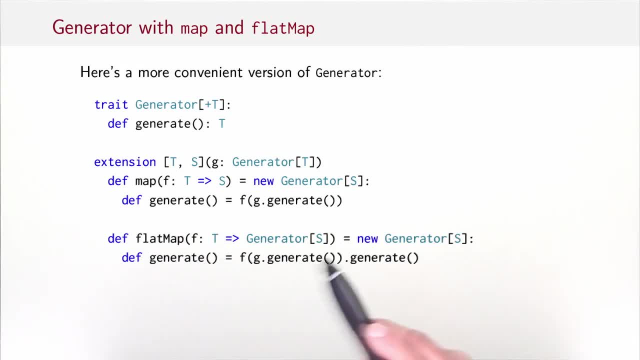 So flat map takes a function now that from t to some generator of s and itself produces a generator of s. So what its generate method does is it calls again the original generate from g, transforms it with f. that gives you a generator of s, so to produce an s random number. 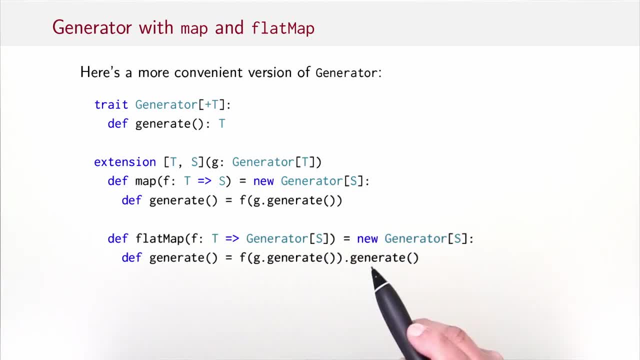 we call again generate on this second generator, So that gives you this right hand implementation of generate. So here we have defined map and flat map as extension methods of trade generator, but we could also have defined it as methods directly inside the trade. If we had done that, that's what it would look like. 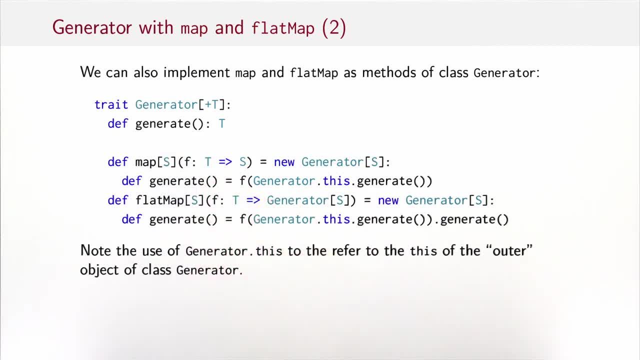 So we would put map and flat map inside trade generator and the implementation is very much the same as before. only now we refer to the enclosing generator object. That's the original generator. So there's actually a tricky bit going on. We can't just write this here. 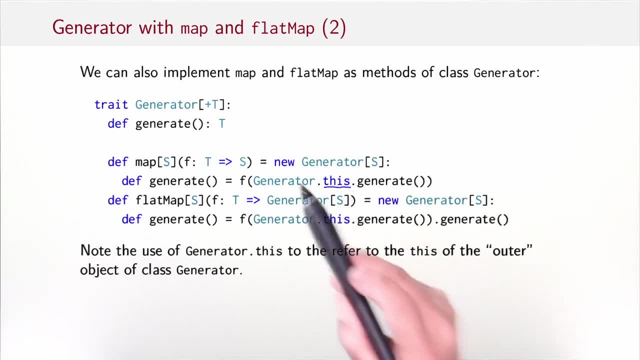 without the prefix, because if we write this in a new generator s, then remember that this expression creates an anonymous class and that this would reference to the anonymous class itself. So if we wrote just thisgenerate, we would get simply a recursive loop to the generate method. that was. 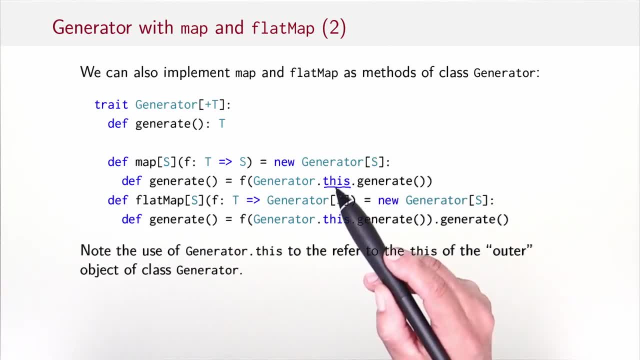 defined here To break out of the current class and refer to the this of the outer class. we prefix the this with the name of the class, in this case generatorthis. So generatorthis is used to refer to the this of the outer object of class generator. 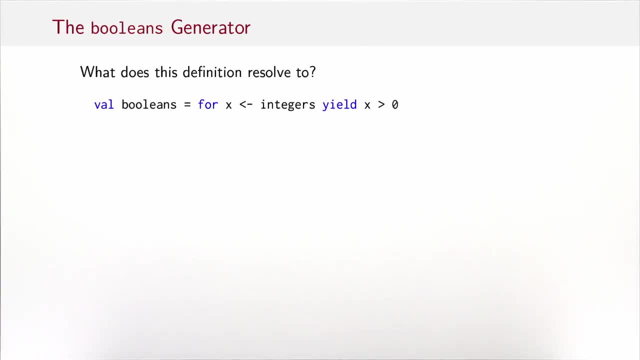 So this all looks very abstract. We define map and flat map for generators, and then some four expressions translate to them, and the original four expression then is supposed to be the right random generator. How do we know that? Well, we can apply some equational reasoning. 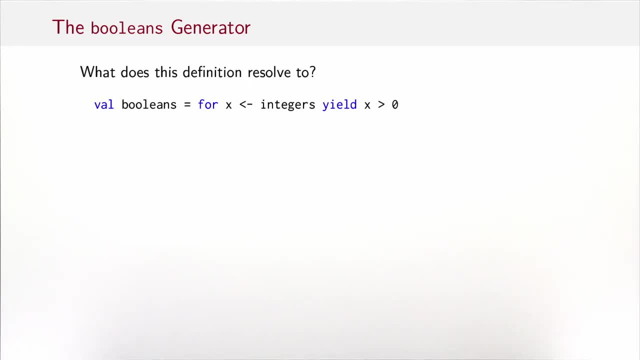 We can use what we know of the translation of four expressions and how the resulting expressions reduce to verify that, indeed, this expression that we write is the generator for booleans. Let's do that. So we've seen that the expression on the right translates to what we 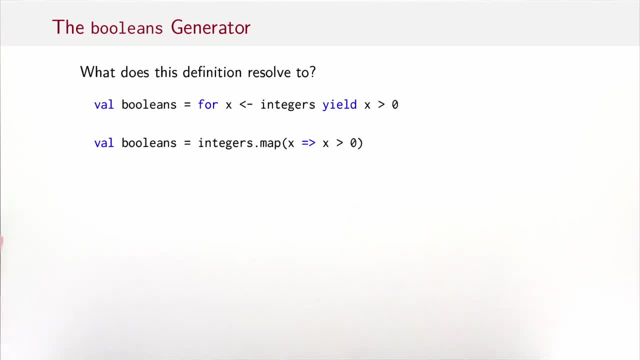 see here. That's what the compiler does when it translates four expressions. Now we plug in the implementation of map. So that's what we see here. The implementation of map says: take integersgenerate- so the left hand side here- and transform it with f where f is the. 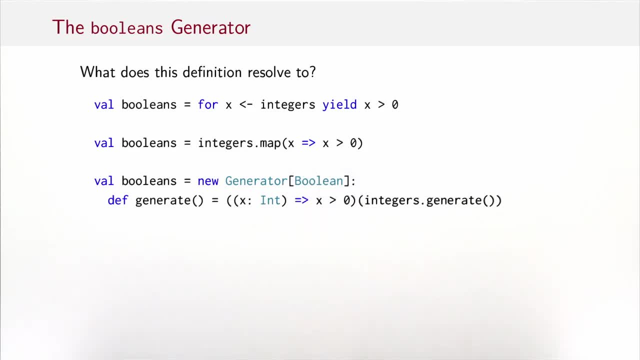 function that gets passed to map. So here we have that function again. It's a lambda. So now we have an anonymous function that's immediately applied to an argument. What we can do is essentially just rewrite. We rewrite it to the right hand side of the function. 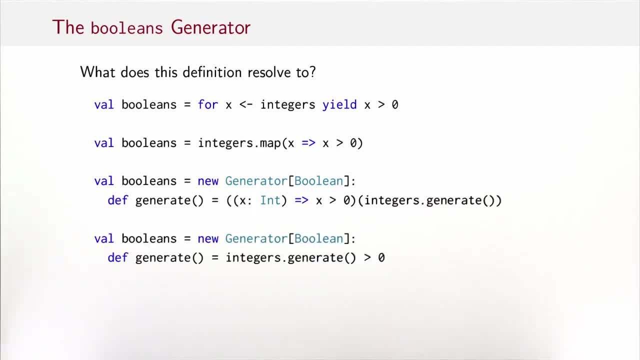 and replace the x by the actual argument. So that's what we get. then We get: def generator equals integersgenerate greater than zero, which, you notice, is exactly the generator for boolean that we have defined initially. Let's do the same exercise for the pass generator. 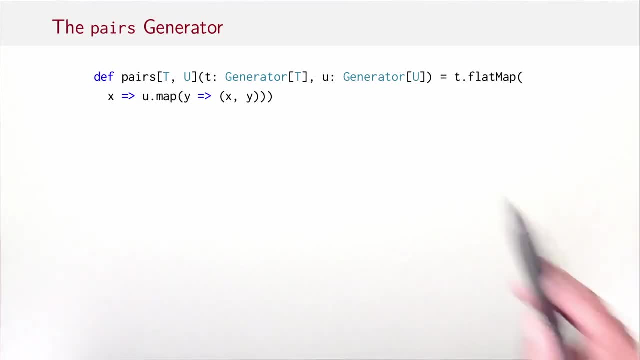 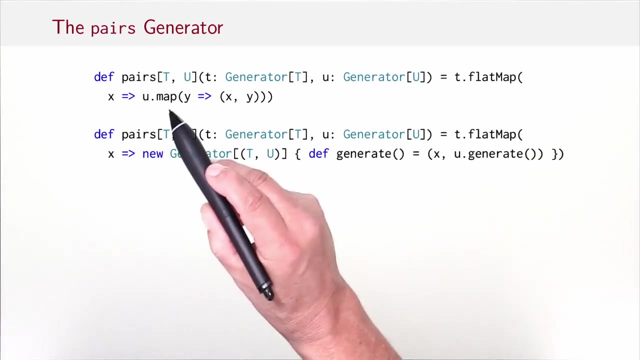 I've left out the initial four expressions. so we start directly with its translation into flat map and map. So that's what we start with. So if we look at the map function, here's what it expands to. So we create a new generator. 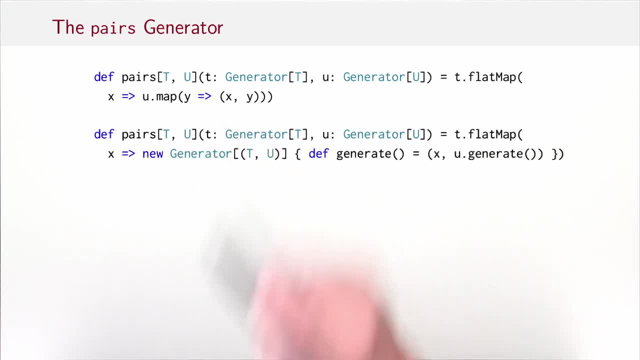 whose generate method is the application of this pairing function to the original generator from u, So it's ugenerate, then wrap with x as first element in a pair. I've done. I haven't written the anonymous function anymore, so I've directly written its expansion and that you see here. 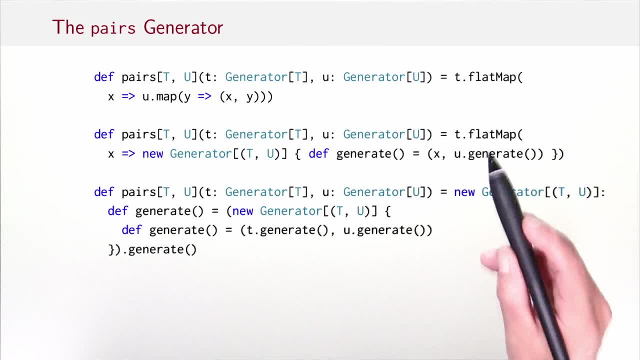 So let's expand flat map next. Here's what we get. So flat map gives us a new generator with a generate method that is the original generator. We call that and that would essentially give us a generator back and we call generate again on that generator. 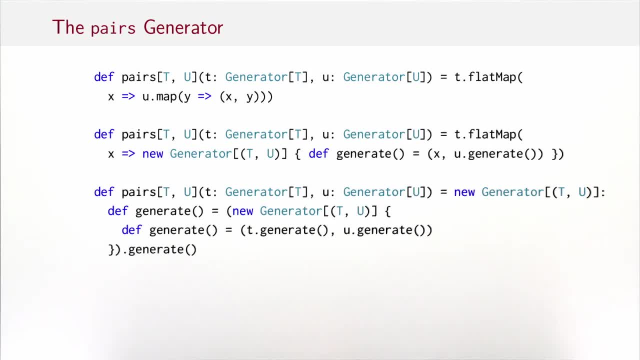 So that's the expression that we left out. Now we do rewriting again. We have here an object with a method and we call the method directly, so what we do, of course, is replace it with the right hand side of that method. So that would be. 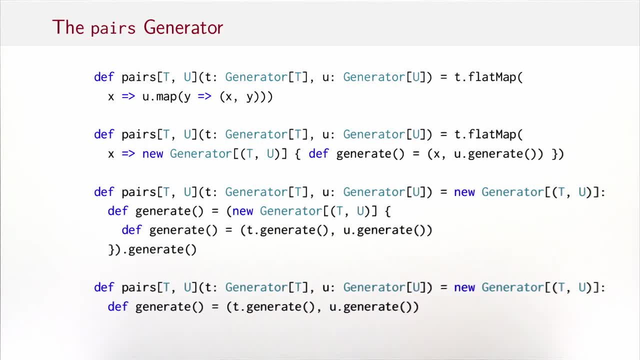 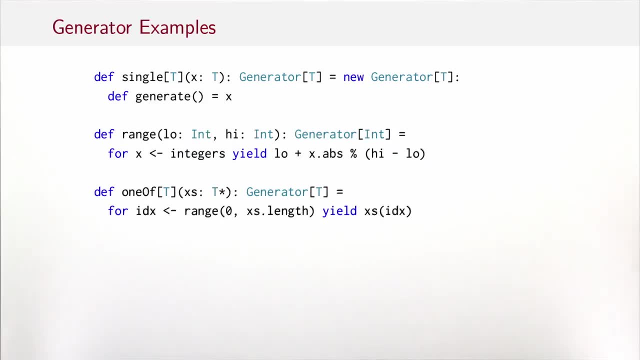 tgenerate and ugenerate, which is exactly the original generator for pairs that we started with. So here are some more example generators that are useful to build up more complicated generators. The single generator always returns the same value, x, So it's a generator that, when called, always returns. 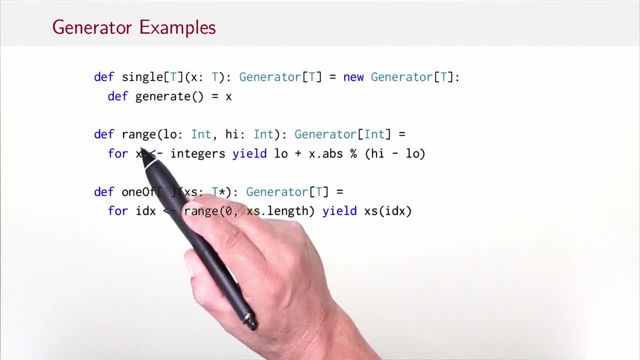 x. The range generator returns a random value between the low and the high values that are given here. So its implementation is: we let x range over the random integers and we yield the low value plus the absolute value of x modulo high minus low. So that would give us: 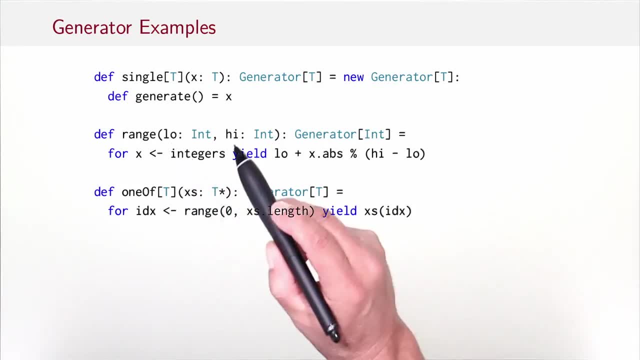 values in the interval between low inclusive and high excluded. Finally, the one off generator gives you random values that are taken from a list of values- xs here. So the way its implemented is: we let index range over the range of random values between zero and xs. 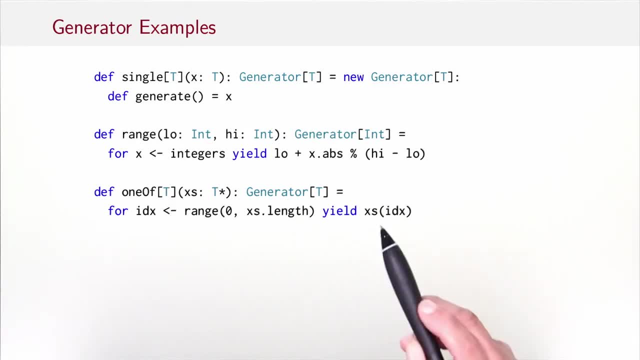 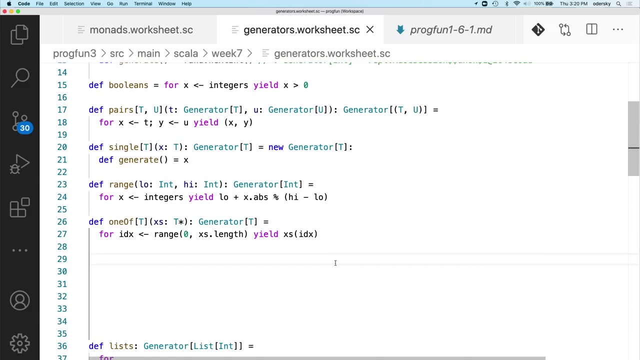 dot length, And for each such random integers we return the value of xs at the index of that integer. So I have added these definitions to the worksheet. Now we can define, let's say, a generator choice which is one of three colors: red, green or blue. 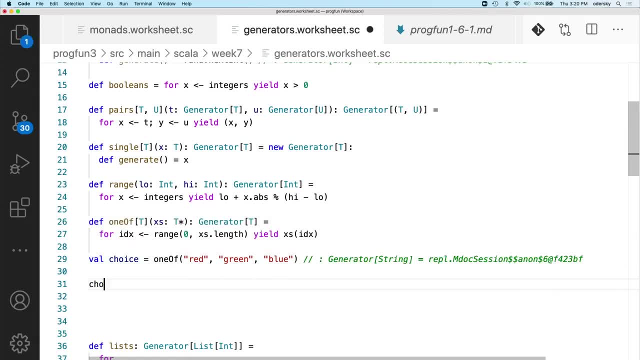 So that gives us a generator of strings And now we can write choice dot generate and that would give us a random string and if we go several times with saves then it would be essentially a sequence of random strings: Lots of greens, red, blue, blue and so on. 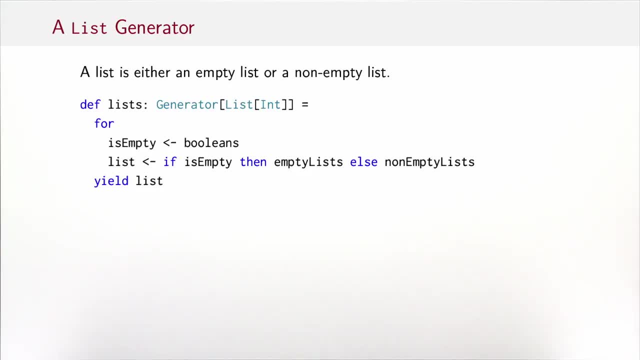 Can we also have generators for random values of recursive data types? Yeah, of course. So let's start with lists as a simple recursive data type. A list, as we know, is either an empty list or a non-empty list. So to generate a random list, we make first: 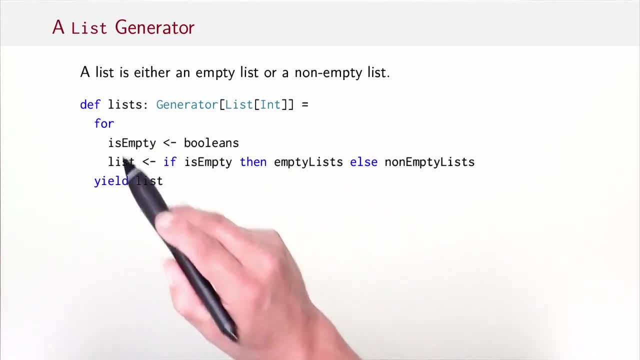 a coin toss, whether we want empty or non-empty, So we let isEmpty be taken from the Boolean random numbers And then the list that we produce is: if the coin toss says it should be empty, then we return an empty random list, which is always the empty list, and 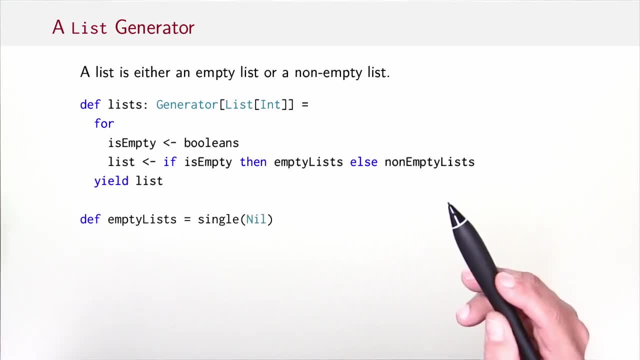 otherwise we return a non-empty random list. So what is an empty random list? Well, it's this generator, the single generator, nil, that will return nil every time it is asked to generate a new value. And what is a non-empty list's generator? 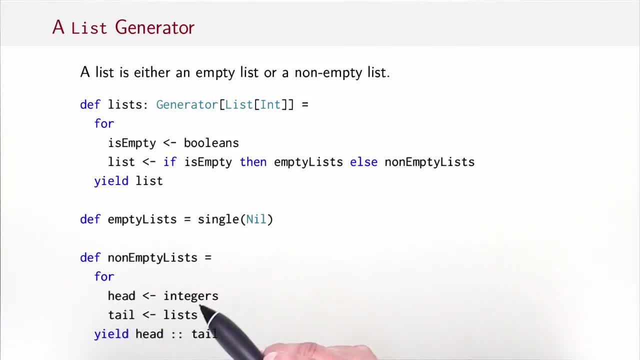 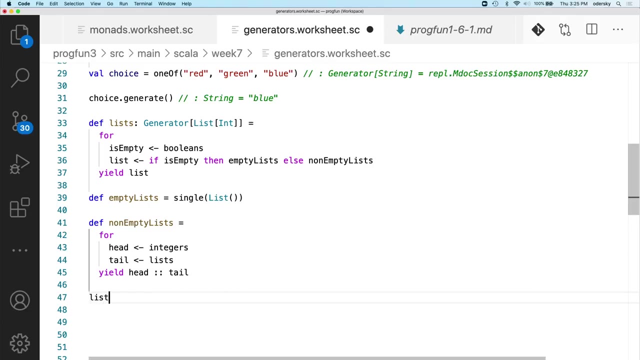 Well, it's a generator that generates a head, which is a random integer, and it generates a tail by calling recursively the list generator here, and that yields the list consisting of the head and the tail. So I've added the new definitions to the worksheet. If we now 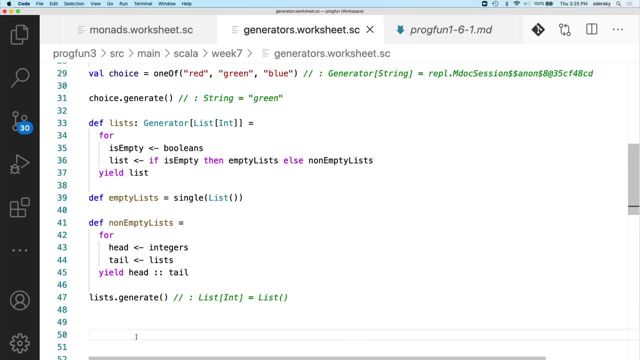 type listgenerate, we get a random list, and if we do that several times, we get, each in each case, a new random list, as you see here. One thing we notice here is that these lists tend to be rather short, Indeed, in about half of the cases, the expected length. 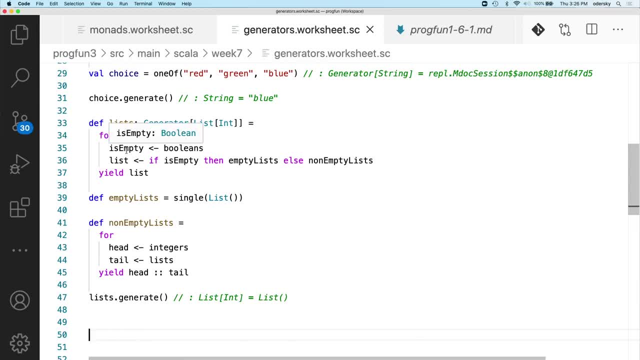 of the list would be zero because essentially then isEmpty, would be true. Can we find another generator that would generate lists that also can reach longer lengths with higher probability? Question to you: what would we have to change to get such a generator? Well, the thing we need to 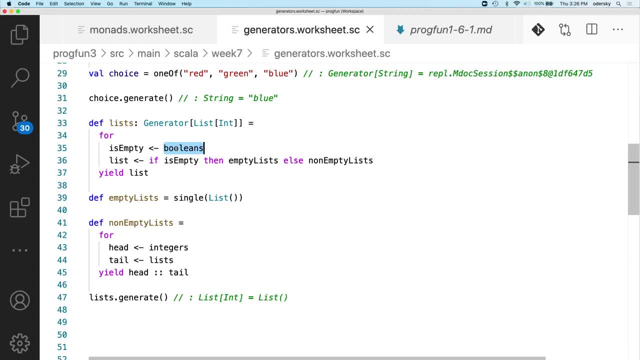 work on is this condition here, the booleans, which essentially split between empty and non-empty lists evenly, So we can reduce the probability that we generate an empty list by using a different generator. So let's say, use range and say we have essentially five slots of lists. 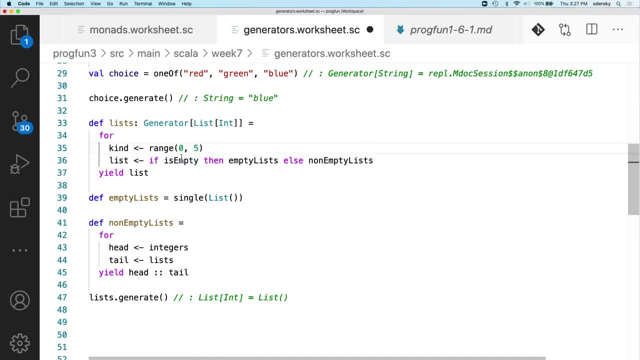 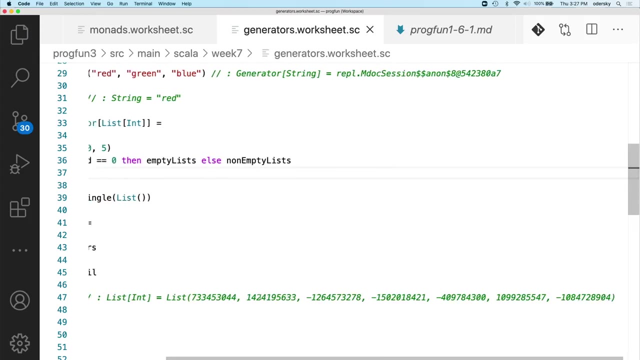 and so call that kind. we let kind range over that and we generate an empty list only if kind equals zero. So in one out of five choices we generate an empty list and otherwise we go on with a non-empty list. If we do that change, then you see the list. 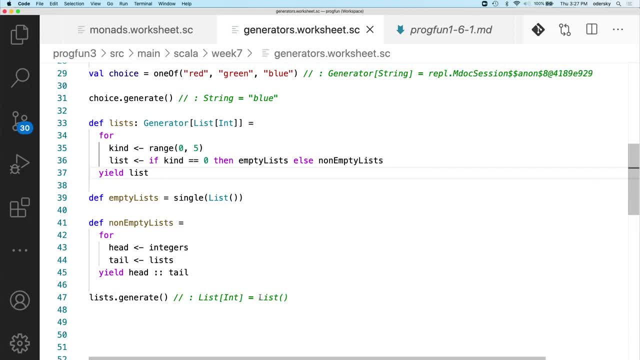 has gotten much longer, so of course it's still random what we get. sometimes we get the empty list, but we get it less often and we get longer lists with higher probability. Here's another exercise for you: Can you implement a generator that creates random? 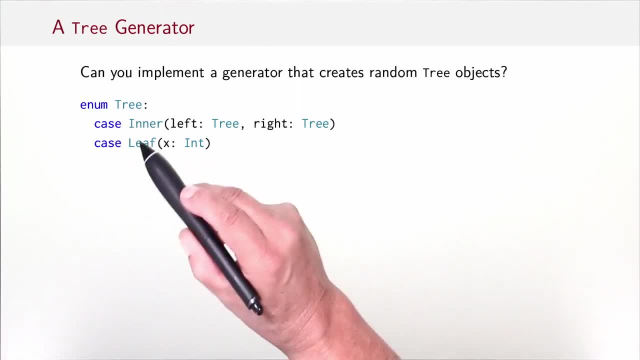 tree objects where the tree is an enum. that can be is either an inner tree with a left and right subtree, or it is a leaf, in which case it has a field of type int. Okay, so here's our tree type. let's write a generator for it. 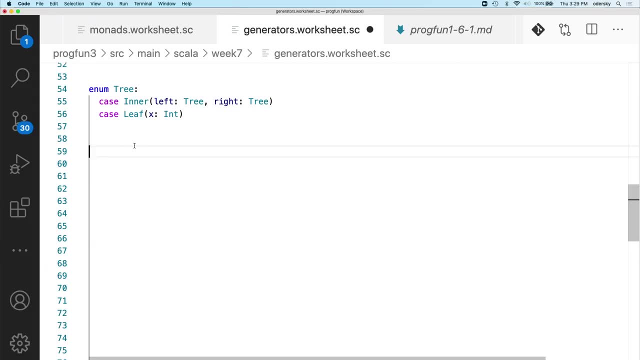 We would expect that this generator resembles quite a lot the list generator that we've written. after all, lists and trees are both recursive data types that are quite close together, So let's use the same schema. We use a for Now. we have first a test. 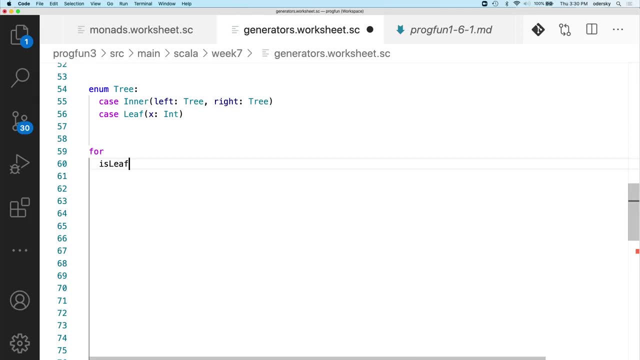 whether we should generate an inner node or a leaf. So let's say, is leaf taken from booleans, so that gives, is leaf is a random boolean, and then our tree would be well, if is leaf is true, then we generate an inner node and otherwise we generate a. 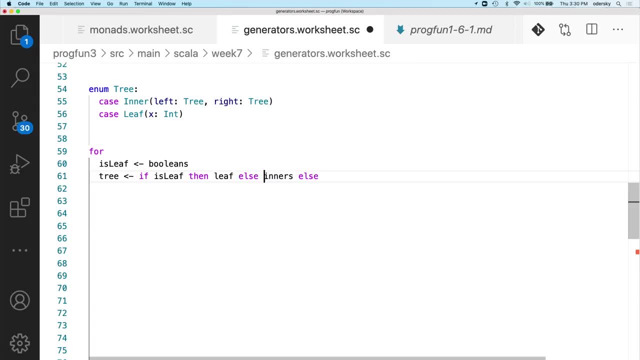 sorry, if leaf is true, then we generate a leaf node and otherwise we generate an inner node and that's the tree that we return in the end. So that would be the trees method, which has type generator of tree. Good Well, we still have to define. 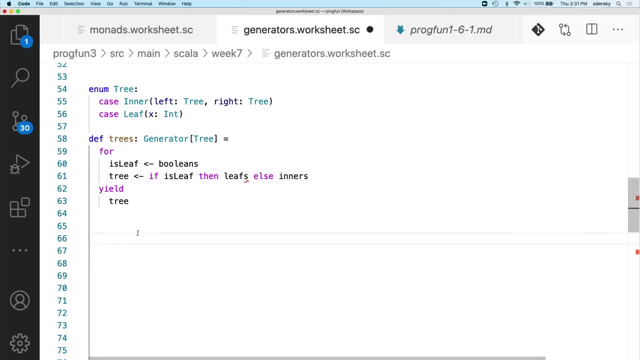 the leaves and inner generators. so let's do that next. So what would leaves be? So leaves would be for x taken from integers- yield tree dot- leaf of x. and inners would be for x taken from trees, y taken from trees- yield oops tree. 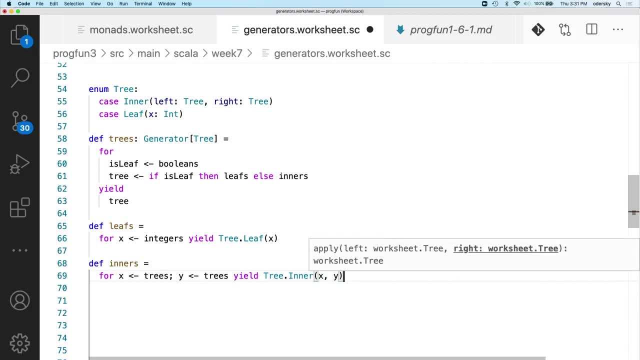 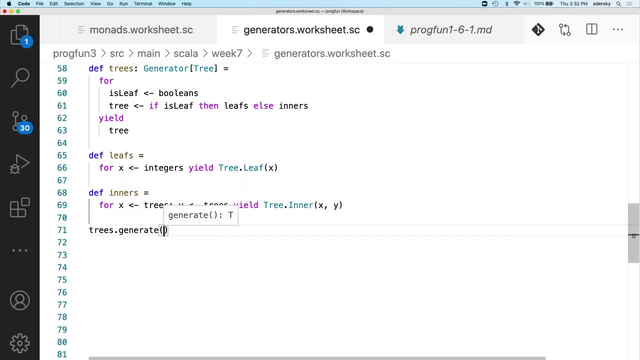 dot inner x, y. Let's test this. So we write trees, dot generate, and here is our tree Or other trees. we have a lot of leaves, but also some inner nodes and some nodes, some trees that are deeper. We can, of course, have less unevenly balanced trees. 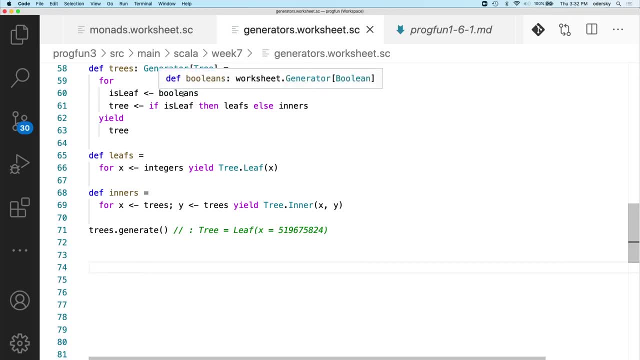 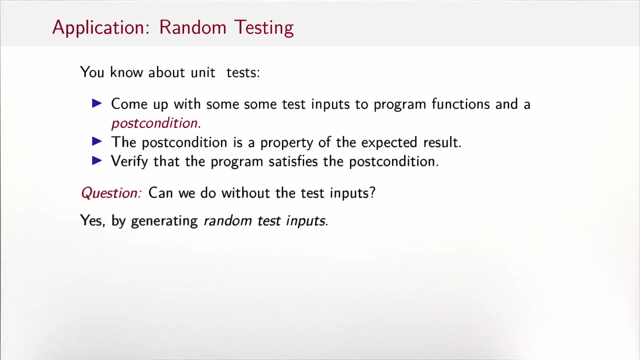 in the same way we did it for lists, by replacing the booleans criterion here with something that essentially is less oriented towards leaves, so that generates leaves less often as before. An interesting application of this random value generation scheme that we've seen is random testing. 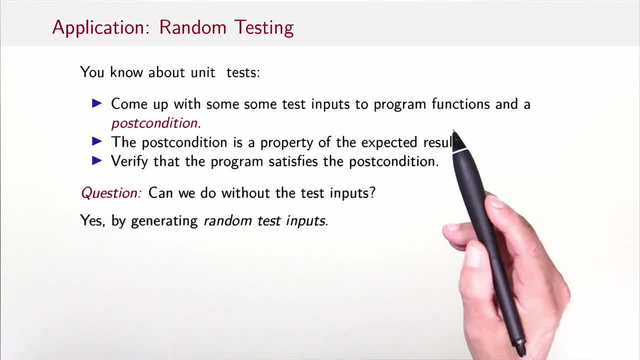 You probably know about unit tests. To test a function you need to come up with some test inputs and a post condition. The post condition is a property of the expected result of the function. Then we run the function on the inputs and we verify that the 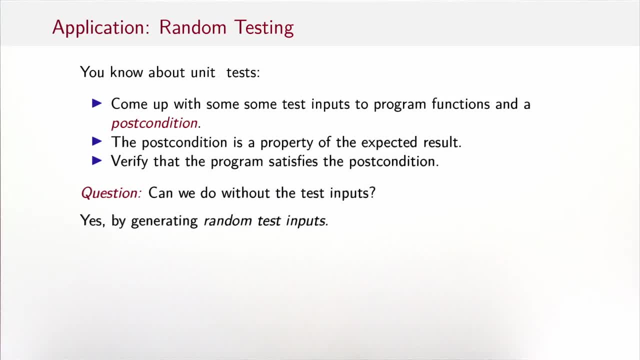 result satisfies the post condition. So a question: can we do without the test inputs? That would certainly be nice to be able to test program functions without having to come up with the arguments to them that we need to test And the answer is yes, we could generate random. 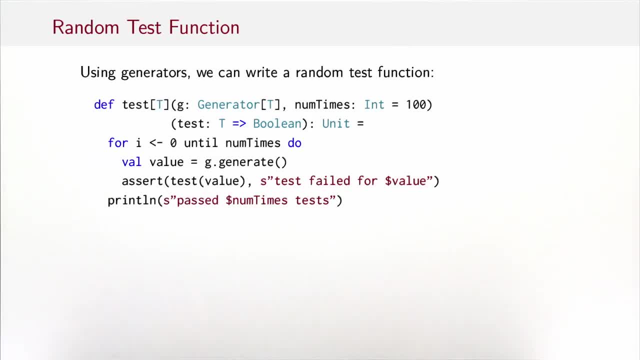 test inputs. So, basing ourselves on the generator framework that we've developed, we can now write a random test function. So here's a possible implementation. The function takes a function to test that you see here. That function has an argument type t and the result type boolean. 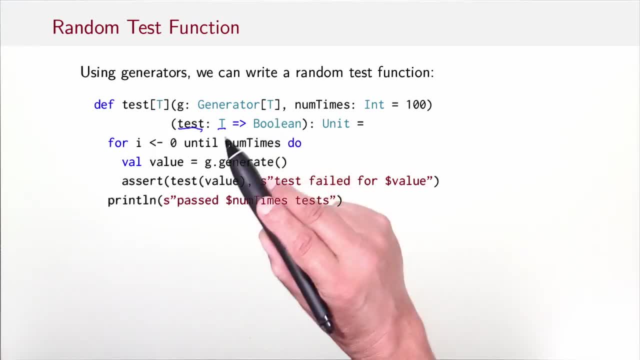 We then take a generator of t that generates random inputs of type t and an additional parameter, numTimes, that tells us how many tests should be run, And then the implementation is simply that we have a loop that goes through the input numTimes each time through the loop we generate. 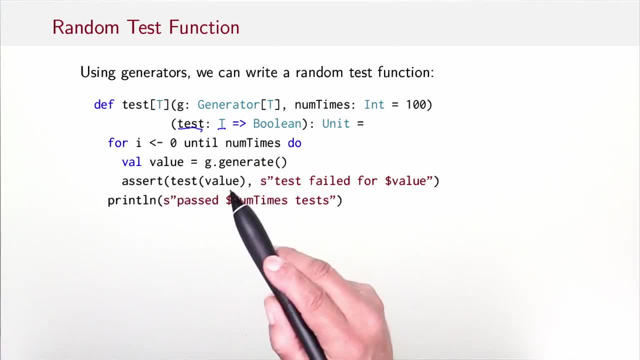 a new random value. we test the test function with that value and if the result of the test function is not true then we fail the assertion with the string. test failed for value. If we passed numTimes runs, then we print. we passed numTimes test, So that's a successful outcome. 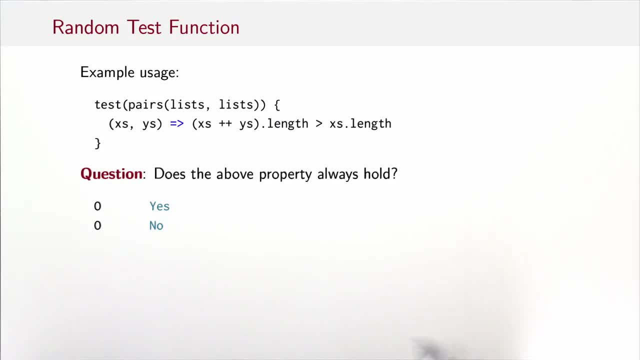 of the testing function. So here's an example usage of our test function. So we can say test pairs of lists and lists, under the condition that if we have two lists then the concatenation of these lists has a length that's always greater than the length of the first list. 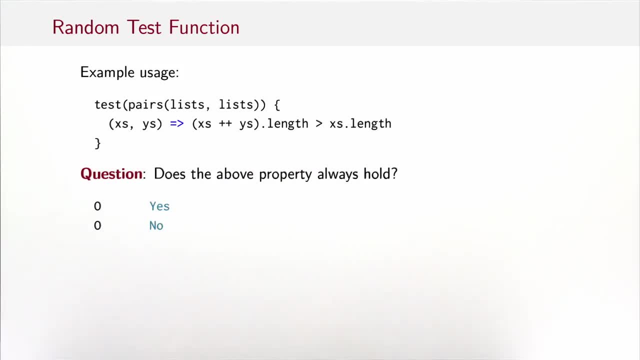 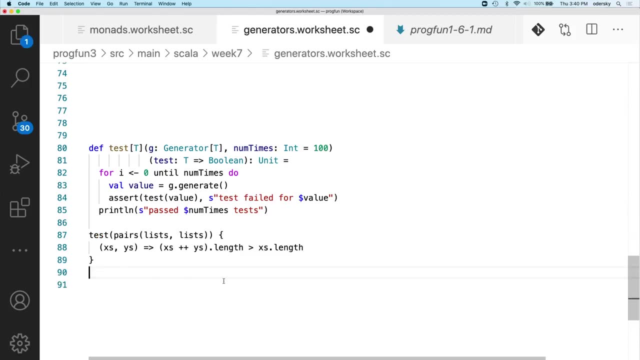 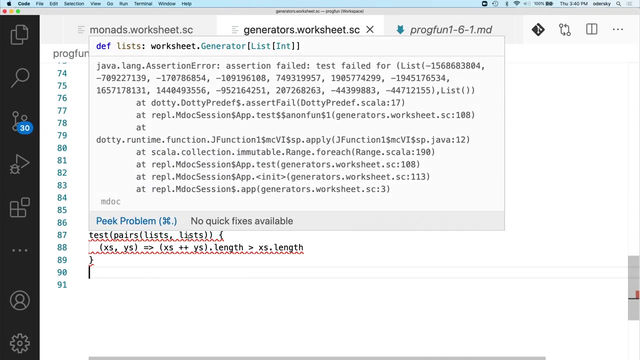 excess. Does that property always hold, Yes or no? Well, let's test it. So I've pasted our test function into the worksheet. Let's test it on the condition that we saw here. So we get a assertion error. that says the test. 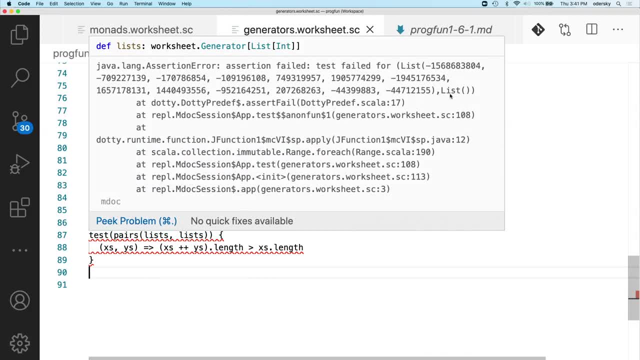 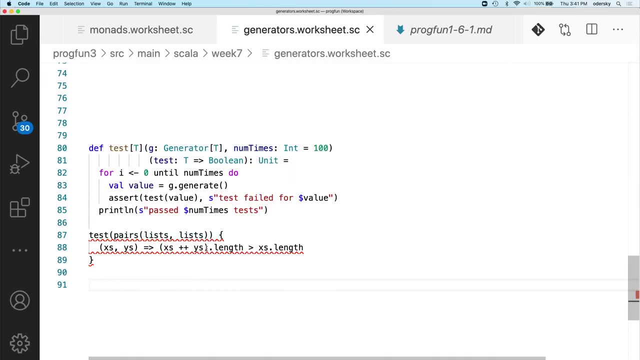 failed for some random list and the second list was empty. We can run it again and we get it now for the pair of empty lists. So what's of course the case under all these failing tests is that the second list, ys, was always empty. 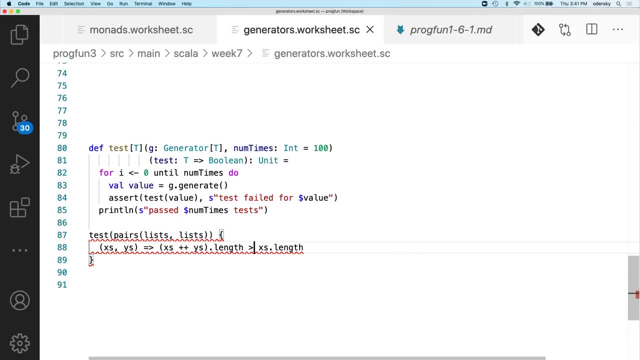 Now it's of course also clear that if ys is empty, then the concatenation doesn't have a length that's greater than excess, It's just greater or equal excess, And if we fix our condition in that way, then indeed we will get passed hundred tests. 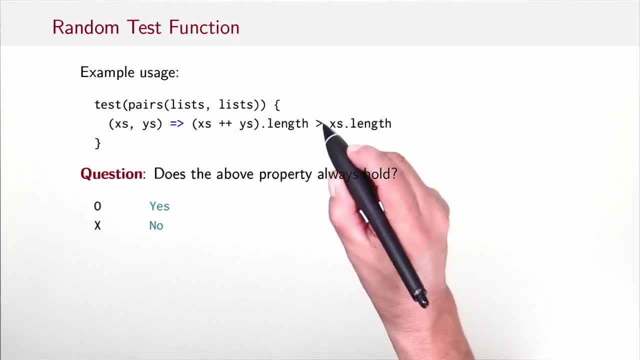 So the answer to the original question is no, and we also have learned that we have to change the condition by adding an equals here. So this looks quite cool. We can just write the property we're interested in and we give a generator for the data types in question, and then 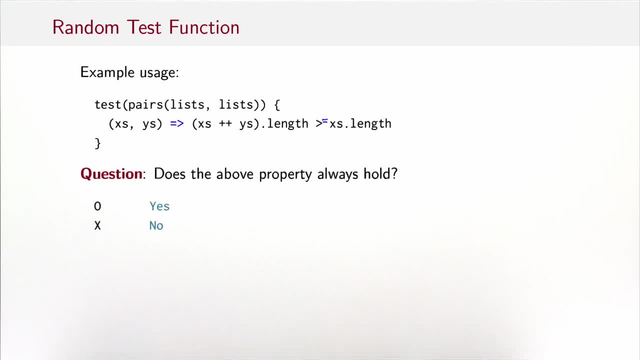 we can run tests for that property as many as we like without having to come up with different inputs. Of course, you might object that well, this naive random number generation is not really very good at detecting corner cases, which is true, and also that some of the 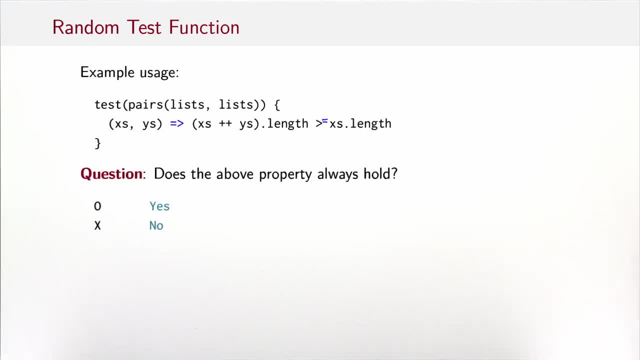 counter examples that we've seen. they were needlessly long. The first xs list, that was a counter example. It doesn't really matter whether it's ten or eleven or a thousand elements, any list would do. But these are things that can be overcome and indeed there are. 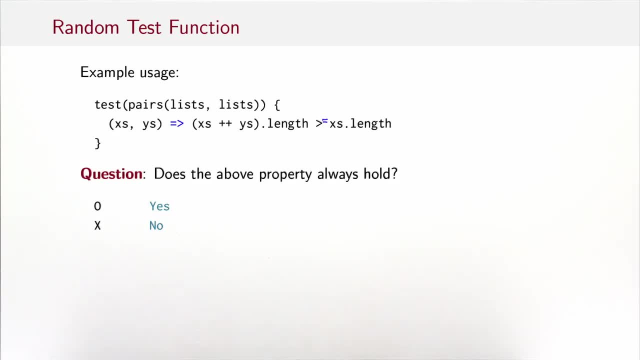 testing frameworks that are much better at finding good random distributions, that also execute the corner cases and that then can minimize the counter examples. So if it finds a counter example, let's say with a list of length ten for xs, then it would go and say, well, can I find a smaller one? 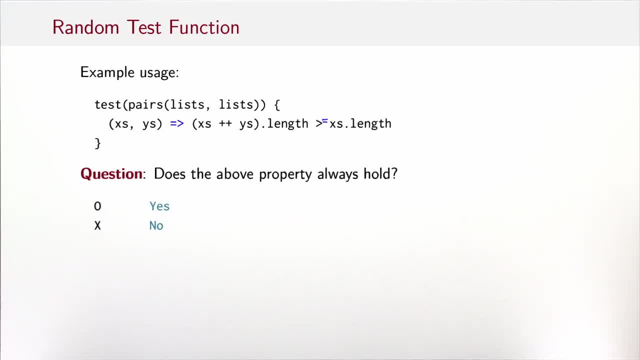 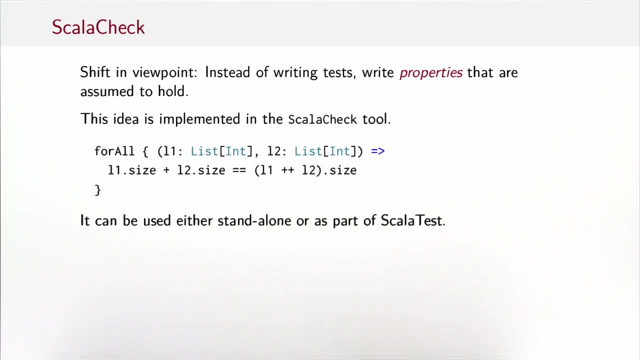 and it would continue until it found the smallest possible one, which in this case would be well nil plus plus. nil has the same length as nil, So what this leads to in the end is a shift in viewpoint. Instead of writing tests or traditional unit tests, 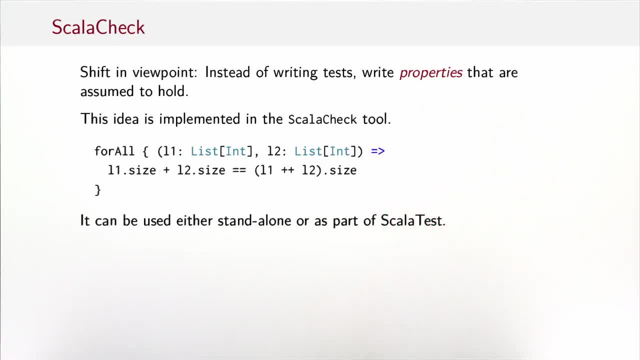 I should say: let's write properties that I assume to hold and then let's pass this to a random testing framework. This idea is implemented for Scala in the Scala Check tool to check a condition for lists that you see here. Here's some syntax you would use. 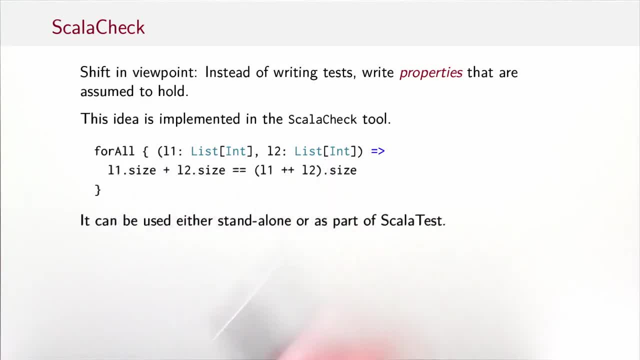 you would say for all, and then essentially come the arguments of type list, of int, and then comes the property. So if you look at this you might be puzzled. You might ask: where are the generators? We have just a function of a two list arguments, but 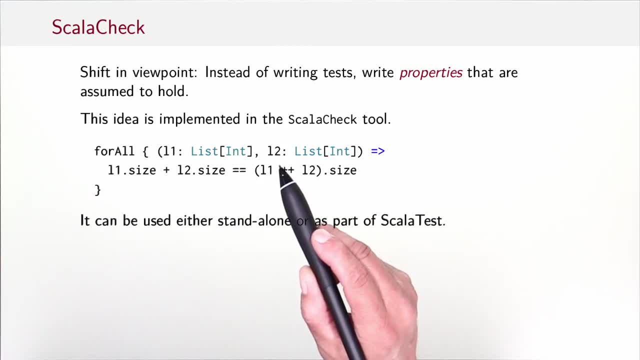 we see nowhere the lists generate that actually generates these random numbers. To solve the mystery, essentially the generators are provided by the for all method itself and it can do that automatically based on the types it has passed. We learn useful techniques to do that in two. 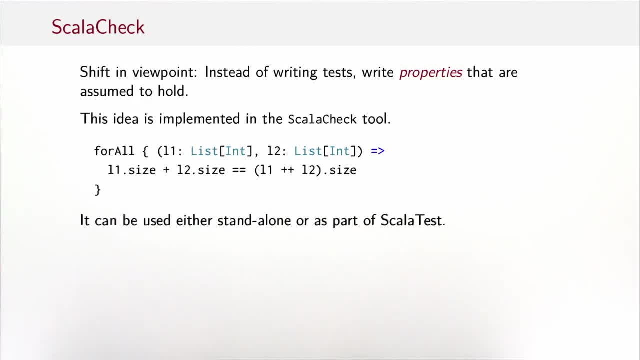 weeks time when we discuss type directed program generation. For the moment, let's just assume that we can write these generators ourselves, or let's just trust in the magic of Scala Check. I should say that Scala Check is not the first tool that did that. 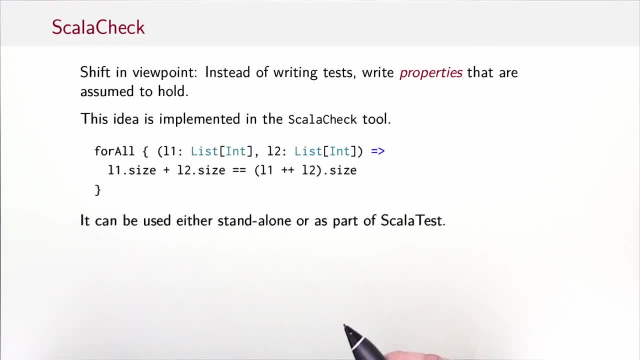 There are now a number of tools for different languages. The original tool that pioneered the domain was called Quick Check and was written for Haskell. Nowadays, the Scala Check tool is embedded in quite a few testing suites. It can, for instance, be used as part of Scala. 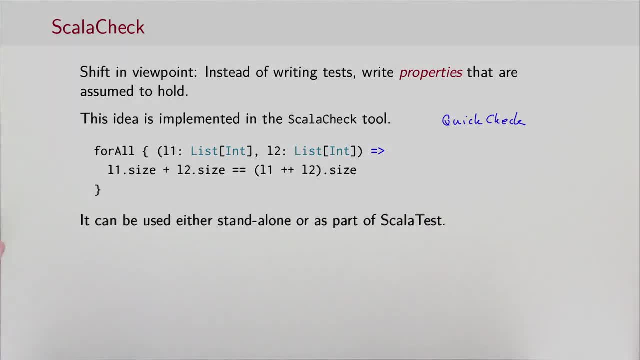 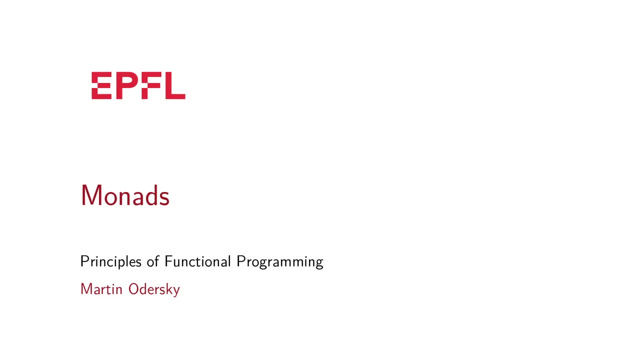 Test, but of course it can also be used stand alone. In this session we are going to talk about monads. If you are at all interested in functional programming, then you probably heard the term already or read an article of what monads are In fact. 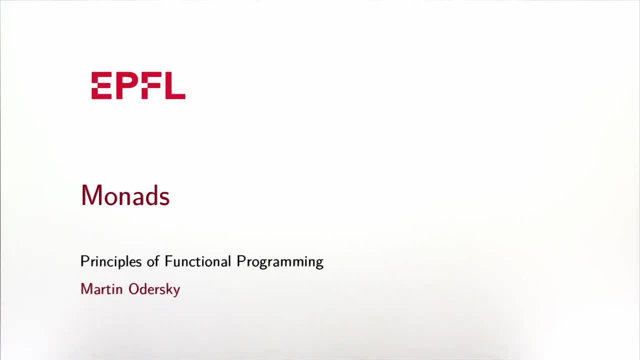 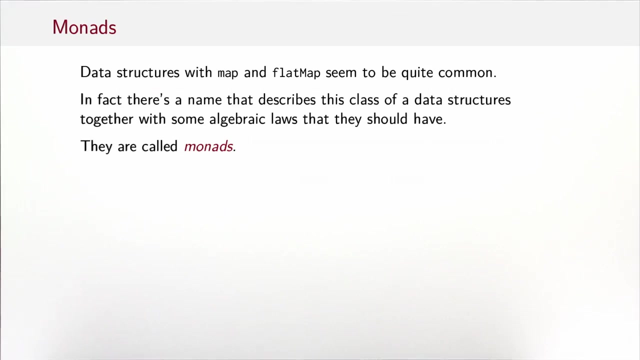 there is a zillion of such articles that compare monads to such exotic things as burritos or elephants. The truth is quite a bit more prosaic and in fact, once you have done this session, you probably will find out that you knew monads all along. So an observation. 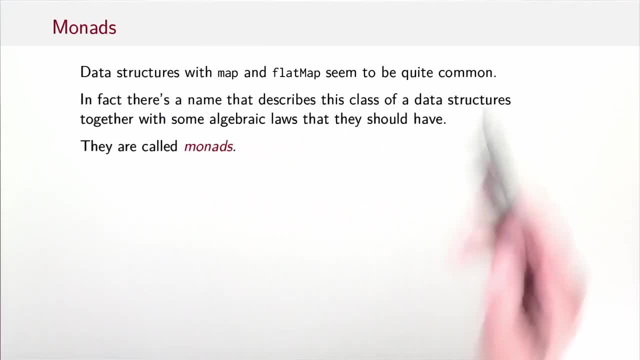 is that data structures with map and flat map seem to be quite common. We have seen quite a few of them And in fact, there is a name that describes this class of data structures, together with some algebraic laws that they should have, And that's. 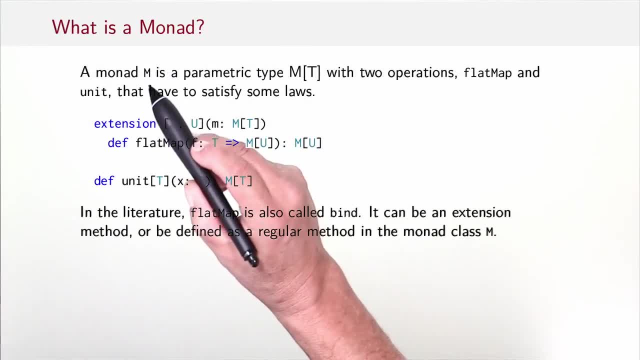 called a monad. So a monad M is a parametric type, so a type that takes a type parameter with two operations- flat map and unit- that have to satisfy some laws. The shape of these operations looks like this, So flat map is typically used. 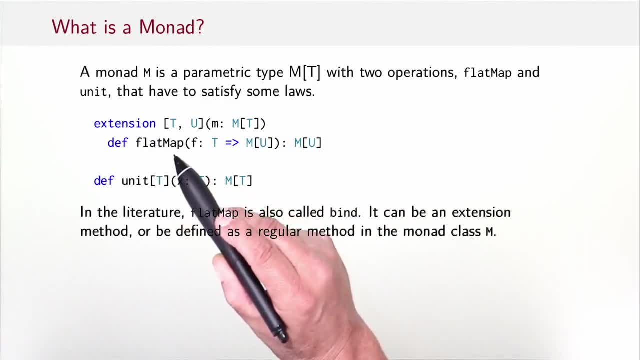 as an infix method. so we define it here as an abstract extension method. So it takes an instance of the monad type M and a function that takes a T, so what's in the monad to an M and it returns an M Unit. 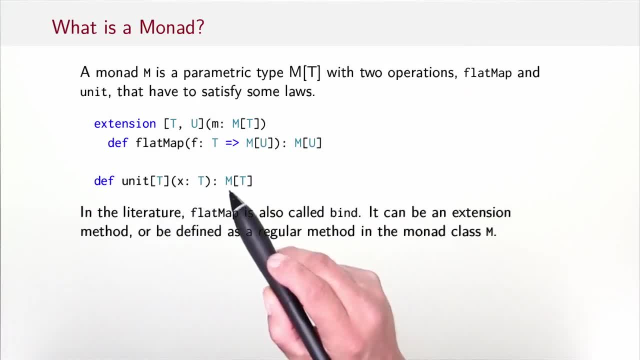 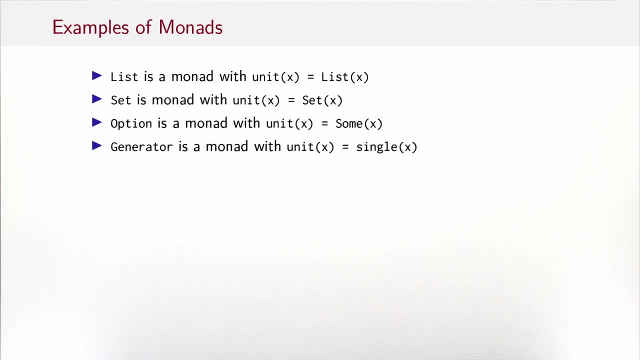 on the other hand, it takes an X and returns an M. In the literature, flat map is also called bind. It can be an extension method or it could also be defined as a regular method in the monad class M. So if you take this definition, 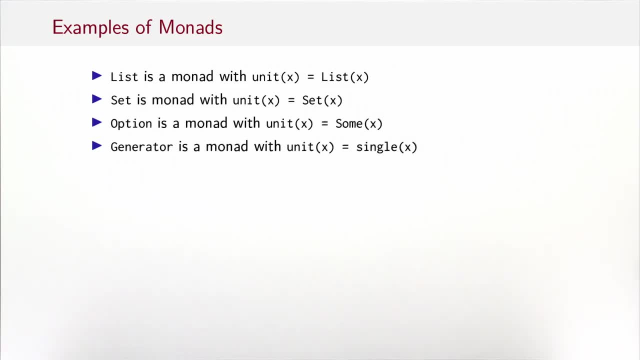 then we see that quite a few of the data structures that we encountered are monads. So list is a monad with unit of X is the single element list X and flat map being flat map on lists, Set is a monad with the unit element set of X. 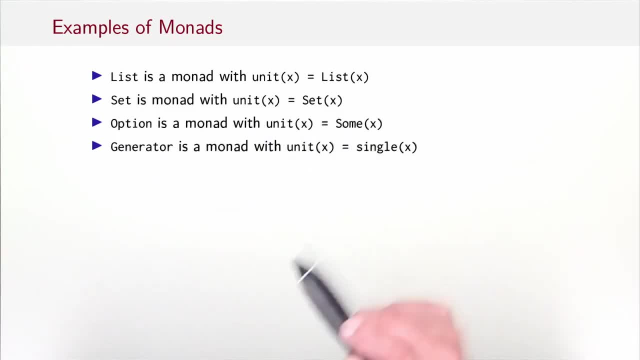 option is a monad with the unit element sum of X and generator is a monad with the unit element single of X. In each case, the flat map on the monad is just the flat map as defined on the type. So what about map Do we need? 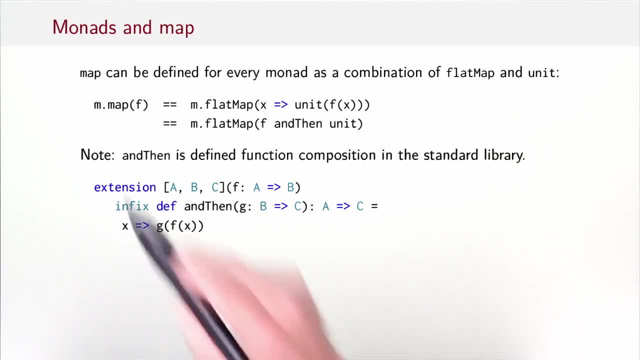 another definition of map. In fact, for monads we can define map as a combination of flat map and unit. So here is the general definition of map For any monadic value: M M dot. map f is defined to be M dot flat map with a function. 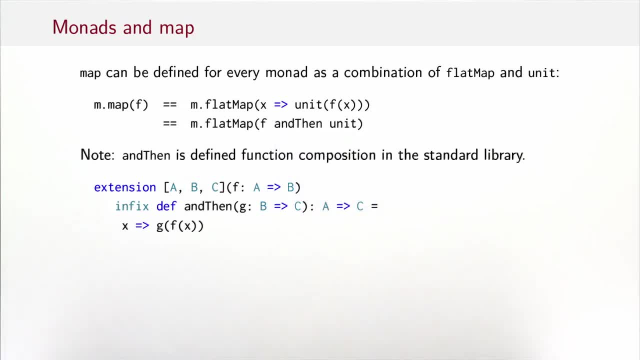 that takes an X and returns unit of f of X And that in turn is the same as M, dot, flat map, f and then unit, And then means function composition. It's defined in the standard library so you can think of and then as being defined like this: So it: 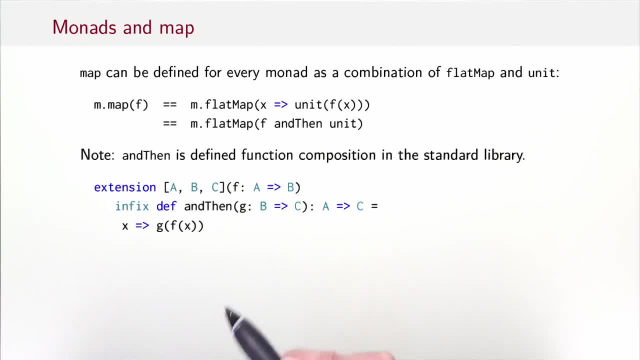 takes as left operand a function from A to B and as right operand a function from B to C, And it yields the composition of those two functions. So that's a function from A to C And its implementation is simply: take an X of type A, apply first f. 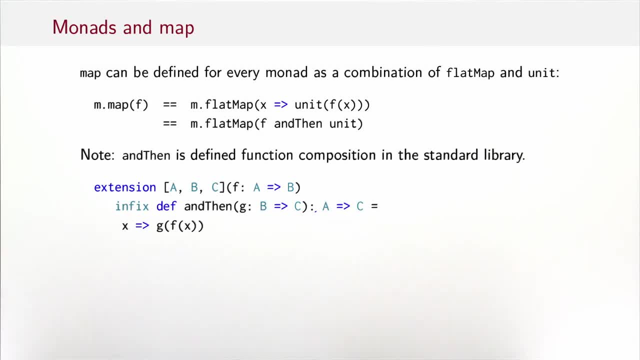 and then G to X, So that yields a value of type C. So let's see whether this makes sense with an example. Let's say M dot map f, where M is a list value. We know that lists are monadic values, So that 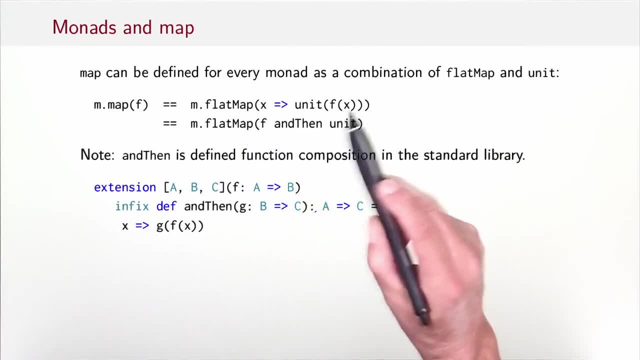 would be the same as M flat map, where we apply f yielding a single value and then pass it to unit and that gives essentially a singleton list of that value. And with flat map we concatenate all these singleton lists. So yes, mapping a function f over a list is the same as. 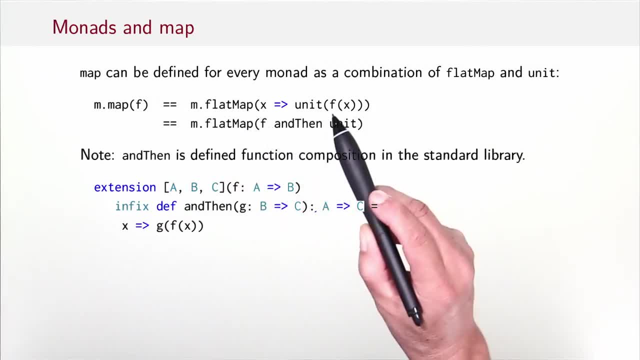 flat mapping. the function that arises from first taking f to the argument and then wrapping the result in a singleton list- In other words, boxing in a singleton list and concatenating the results- cancels each other out. So that was an argument why it makes sense to define. 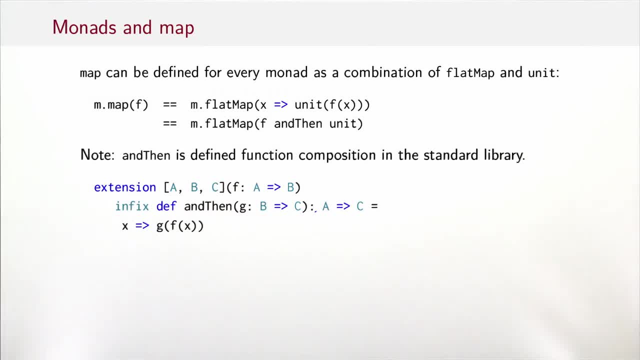 map that way. But if we argue in a monadic framework, then indeed we turn things around. We say we only define flat map and that here is the definition of map. So it can of course then be implemented more efficiently, like avoiding the boxing and the flat mapping. 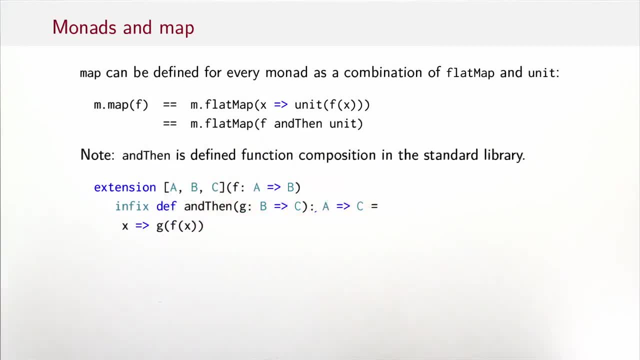 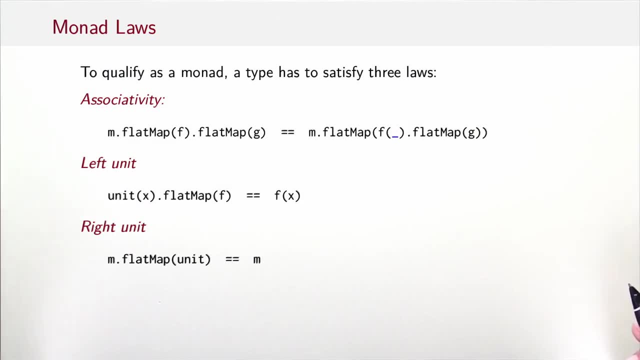 but any such implementation has to satisfy this equation. So having unit and flat map of the right shapes is necessary but not sufficient to be a monad. To qualify as a monad, a type also has to satisfy three laws that relate flat map and unit. 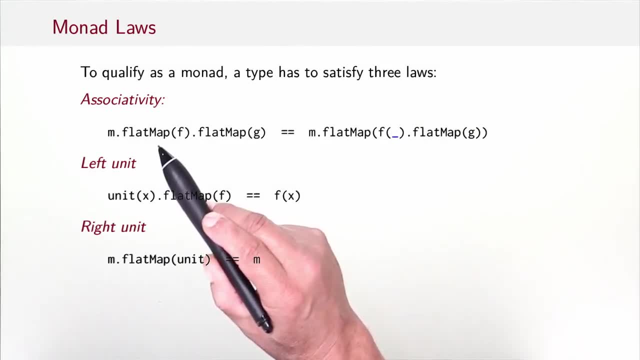 The first law is associativity. It says that m, flat map f and then flat map g is the same as m flat map, a combined function that first applies f and then flat maps with g. So here you can see the parentheses go like this: of course, that's how dot is defined. 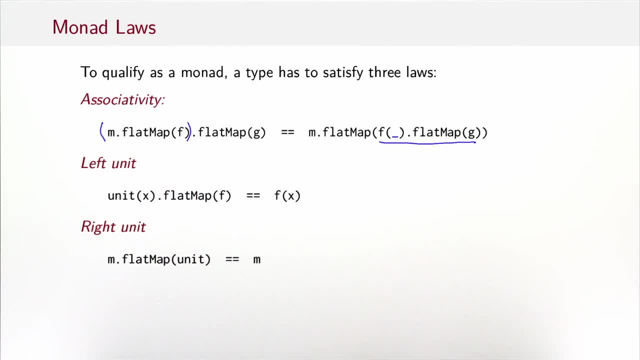 and here the parentheses are on the right, So that's an associative law. The second law is the left unit law. that says that if I take unit x of a monad and then I flat map with a function f, then that's the same as just. 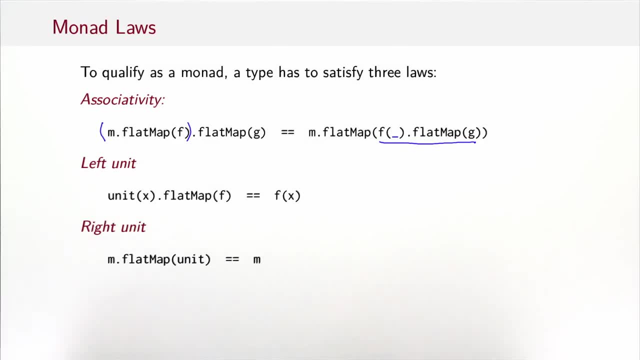 applying f to x. And the last law is the right unit law, which says that if I flat map a monadic value with unit then I get back the same monadic value, m. So these three laws of associativity- left unit and right unit- 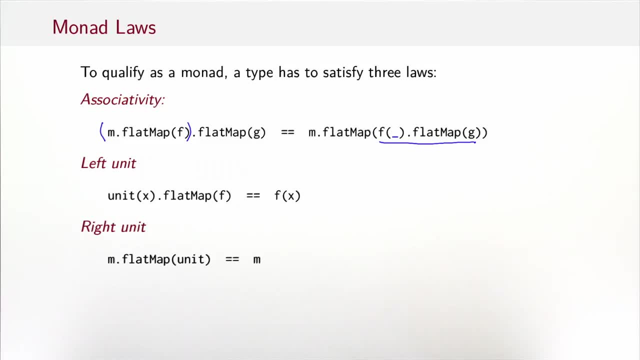 one typically knows from monoids. So a monoid is a structure with these three laws. So that observation gave rise to the often cited remark that monads are just monoids in the category of endofunctors, Which will probably leave you either. 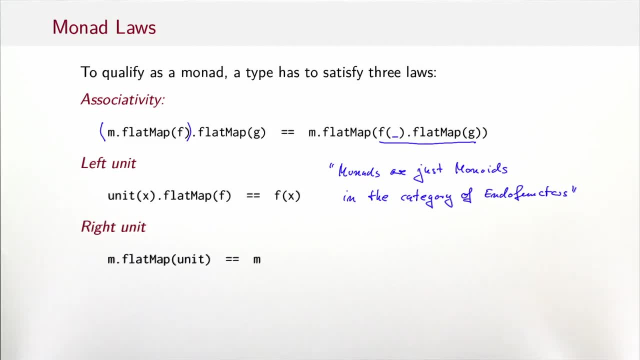 utterly confused or utterly impressed. But to go on. we don't need to know about endofunctors. so you can treat this as just a funny remark alongside the remarks that monads are burritos or monads are elephants. So those monad laws. 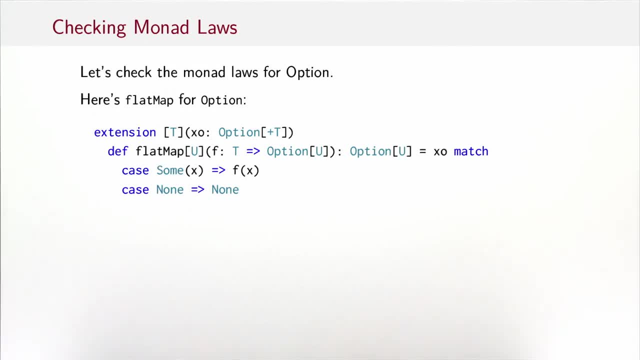 of course they have to be checked for each type that is a monad or that pretends to be a monad, So let's do that for option. So here's flat map for option. So flat map on option says we have a function from t to option u. 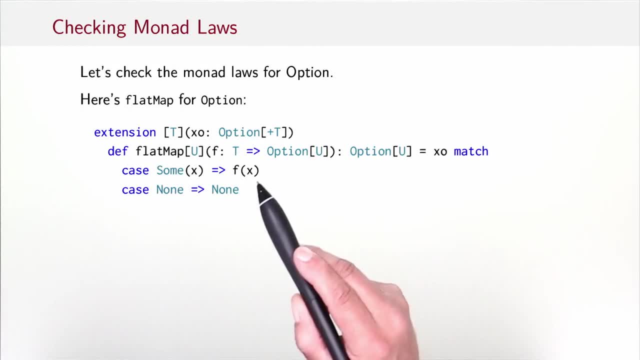 and it says: well, if the original optional value is sum of x, then we apply f to the original value That gives an option, And if it's none, then we return none. And we, for example, see that the unit for option was sum of x. So let's test. 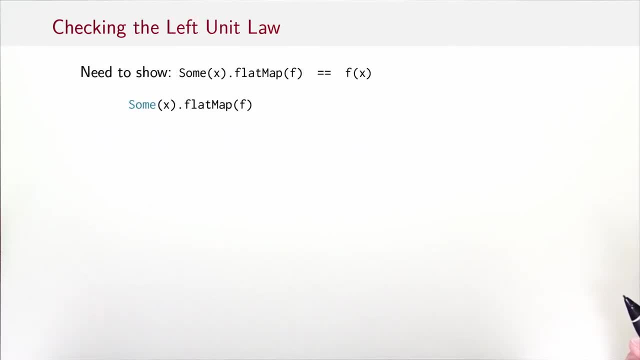 whether these two functions satisfy the monad laws. Let's check the left unit law first. We need to show that sum of x flat map f is the same as f of x. So sum of x flat map f by expanding flat map that gives sum of x match. 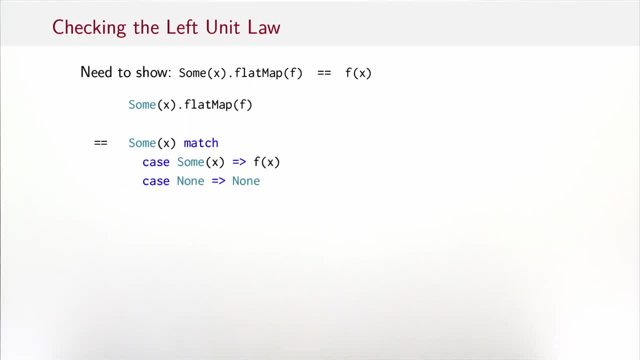 case: sum of x, f of x. case: none, none, And that gives by straightforward computation. we pattern match this with that pattern: f of x. So the left unit law holds. Now let's check the right unit law. So what we need to show is that optional. 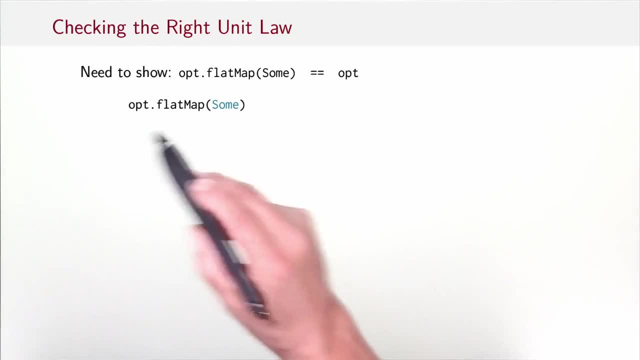 value: flat map sum is optional value. So optional value, flat map sum we plug in the definition of flat map. that's what we get. Optional value match: if it's sum of x, then sum of x. If it's none, then it's none. And now to 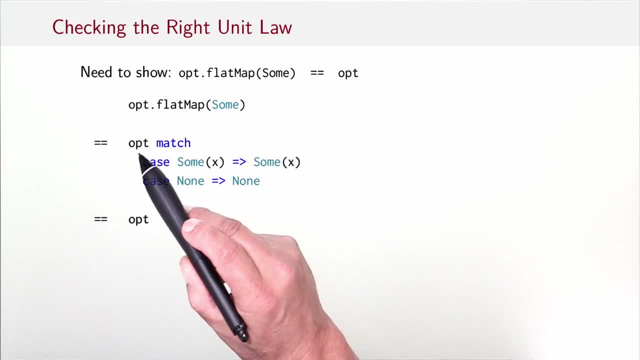 continue. we just make a case distinction: optional value is either sum of x, in which case we get back a sum of x, or it is a none, in which case we get back none. So in either case we get back the optional value itself, and that means that the right unit 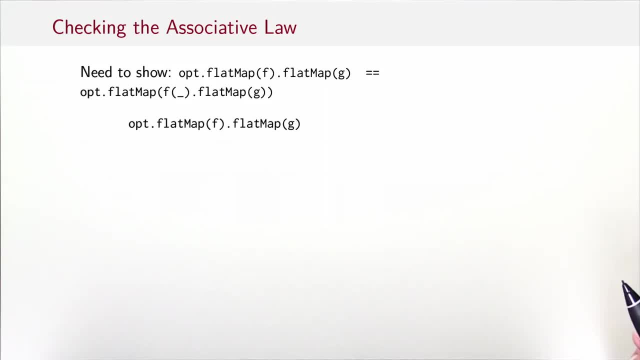 law holds. The most complicated to check is the associative law. So we need to check that optional value flat map f- flat map g is the same as optional value flat map f underscore flat map g. So let's start with the left hand side. 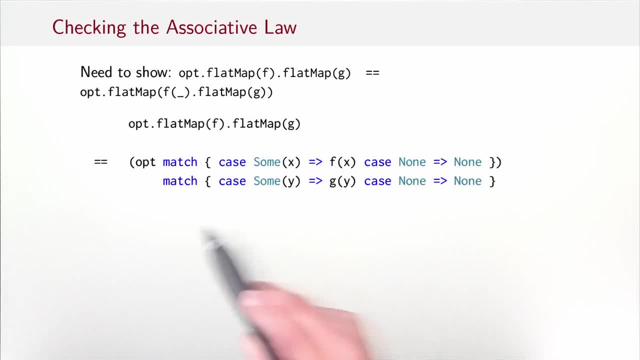 That left hand side is by expanding flat map twice this expression here. So the left expression here is: optional value: match case sum of x, f of x, Case none: none. So that's condition up to here. And then the second line is the second flat map. 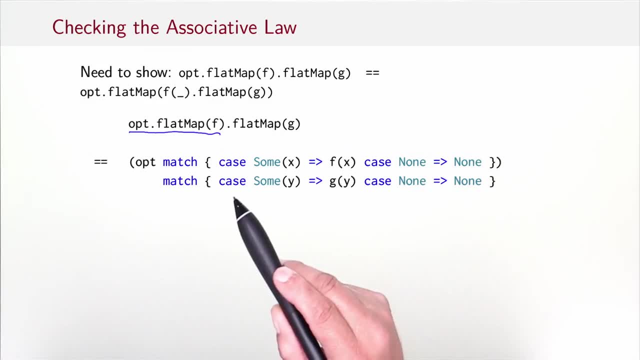 so that scrutiny would be matched against again: case sum of y, g of y, case none, none. So what we do next is distribute the second match into the first, So we have this optional value match: case sum of x, f of x. and then we continue. 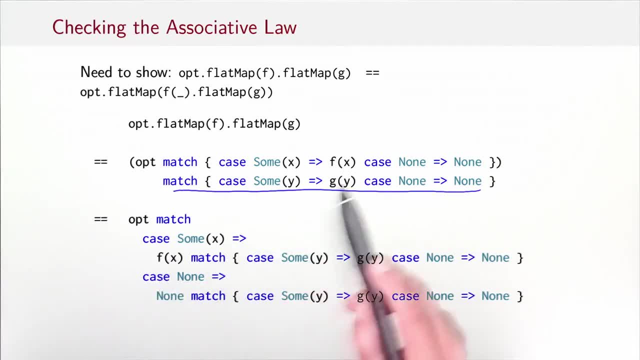 with the second match. Let's take the two together, So that gives f of x, continue with match case. sum of y, g of y, case: none, none. And the same way for the second case here. So we would say, well, if it's a none, then it's. 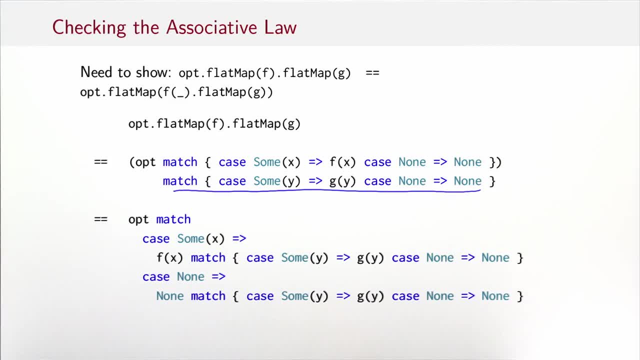 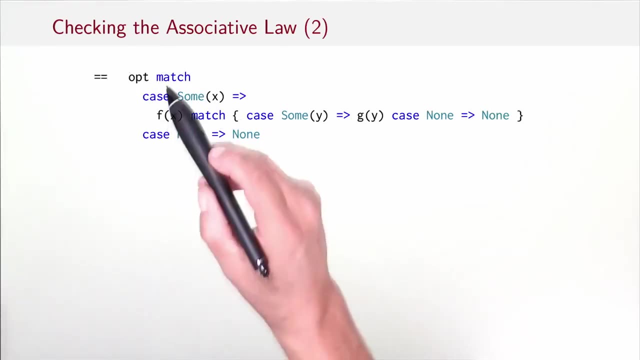 none match and then the same cases as before. So let's work on the second case first. So here we have none match this one here, So that would reduce directly to none, because that none match is up with that pattern. So that leaves us. 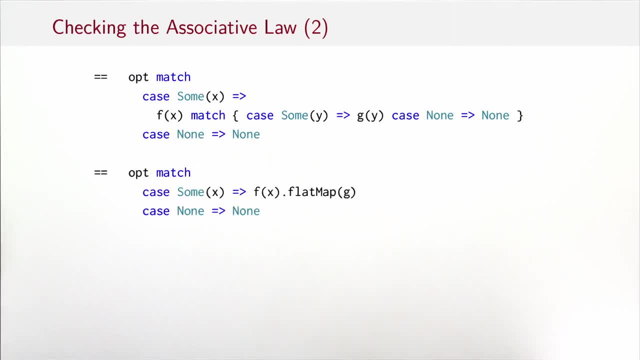 this expression here. Now let's work on the first one. So here, what we see is that this definition here is the right hand side of the definition of flat map, or more precisely, f of x, flat map g. If we expand flat map, we get. 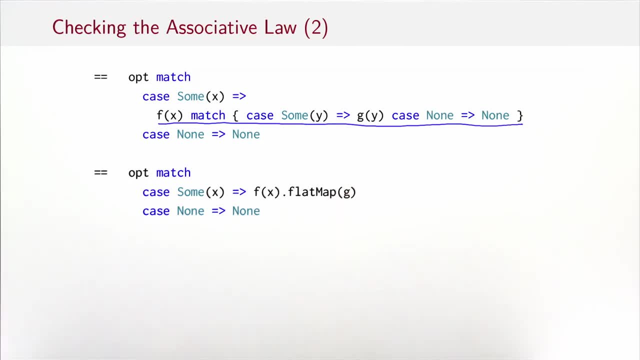 exactly that, And we have seen that the equations in our program, in our scalar program, are true equations. We can essentially expand them and reduce them in both ways. So here we go, from the expansion to flat map to the original call of flat map. 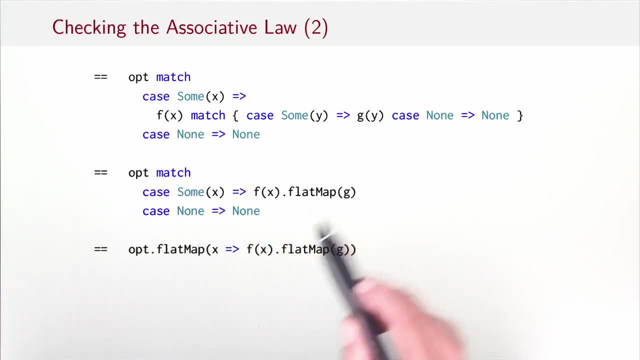 And we apply the same trick again. So now this thing here is the right hand side of this expression, here Opt flat map x, f of x flat map g. So if we expand that, we get that. So that's also an equality. And that last one is: 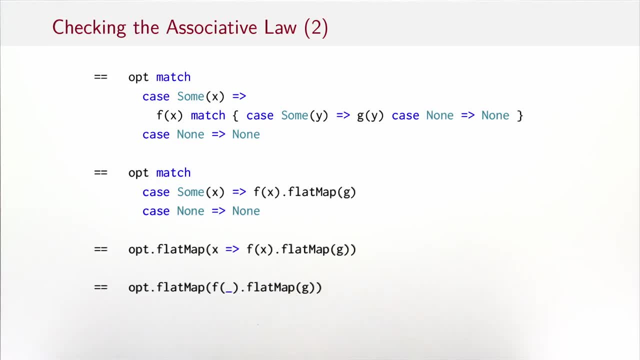 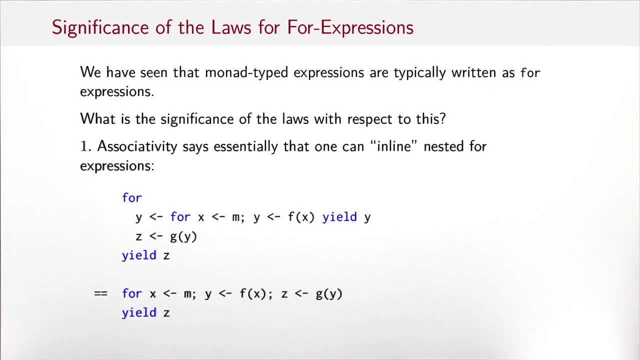 just another way to write the original right hand side of the equation. So that means that the associative law holds as well. So we've seen that monotyped expressions are typically written with four expressions. What's the significance of the laws we have developed with respect to four expressions? 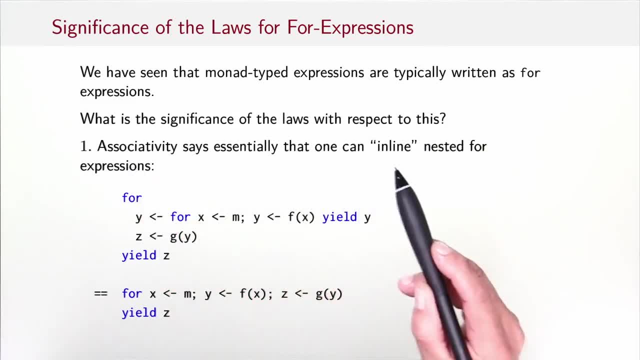 Well, associativity says essentially that one can inline nested four expressions. So if you have an expression like this four, and then y is taken from the result of another four expression and then z is taken from something else, then that's the same as inlining. 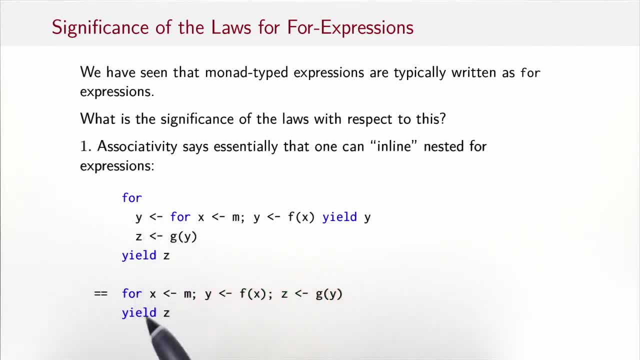 this inner four and putting it in front of the z. So it's the same as saying: well, let x range over m, then y range over f of x, and then z range over g of y, yield z. So we can take nested four expressions and: 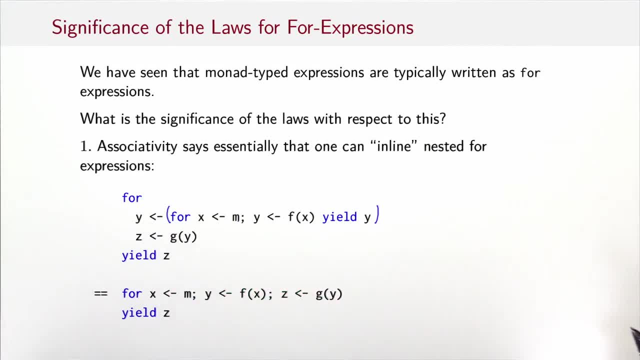 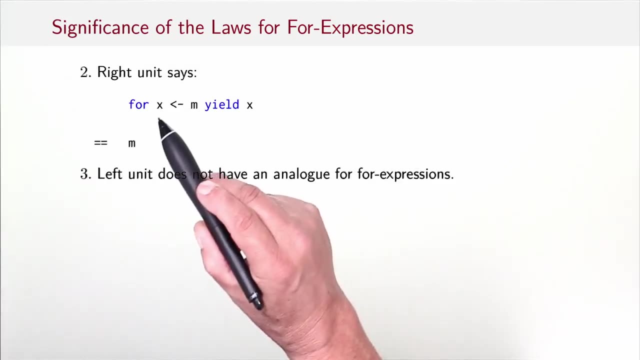 splice them in front of the things we define on the left hand side and what follows. So the significance of the associative law is that it lets us flatten four expressions in that way. The right unit also has significance with four expressions. It just says that 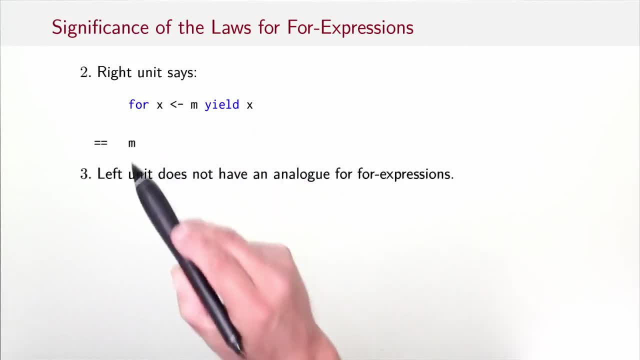 this is the identity. So four x taken from m yield x is the same as m Left unit interestingly doesn't have an analog for four expressions that I could discover, So it's right unit and associative that are relevant for four expressions here. 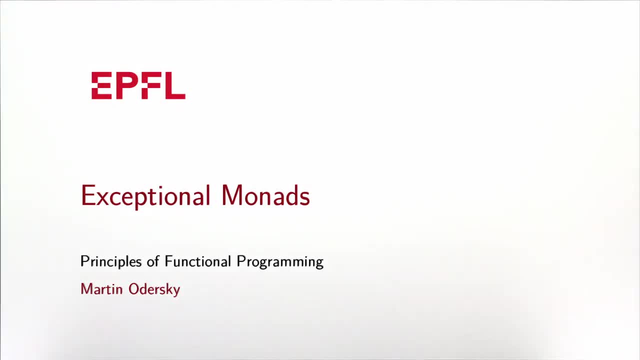 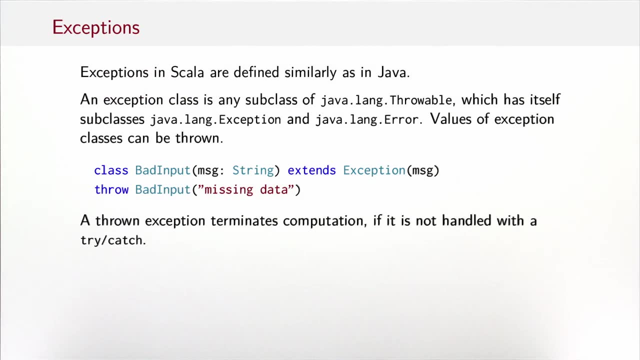 In this session we are going to talk about exception handling in Scala and what it has to do with monads. You've already seen exceptions as part of throws expressions. In fact, exceptions in Scala are defined similarly as in Java. An exception class is any subclass of javalangthrowable. 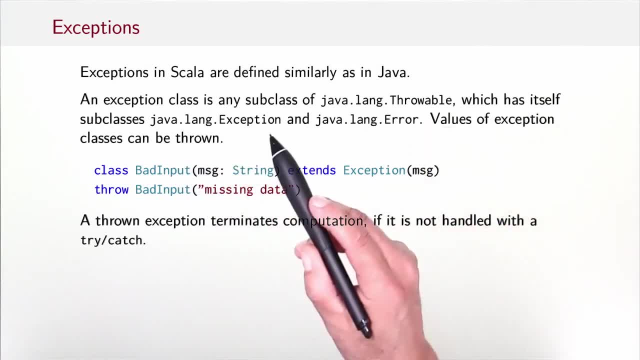 which has itself subclasses: javalangexception or javalangerror. So typically you inherit either from exception or error or from another class that in turn inherits from these Values of exception. classes can be thrown, So they can be parts of throw expressions. So here's an example You can. 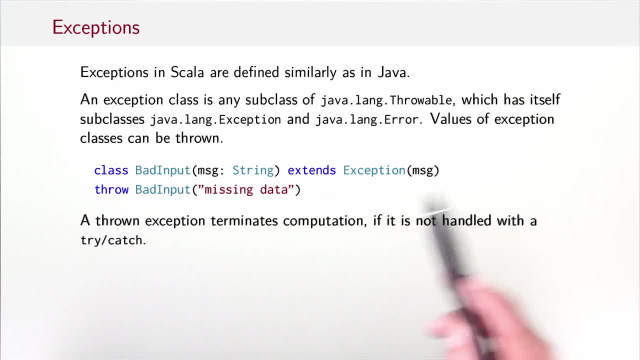 have a class badInput that extends exceptions. You typically have a message parameter, which is a string, as a parameter for these exceptions And once you have defined that, you can have a throw expression with badInput and missing data as the exception that is thrown- A thrown. 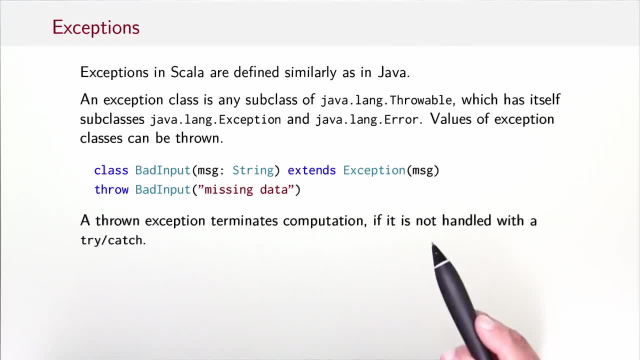 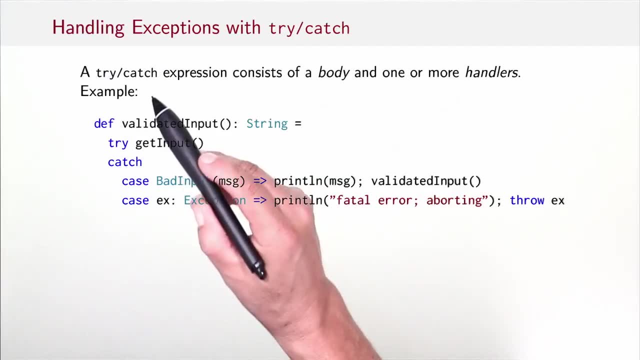 exception usually terminates computation unless it is handled with a try-catch expression. So we'll see those next. A try-catch expression consists of a body and one or more handlers. So here's an example. Let's say we want to write a function: validatedInput. 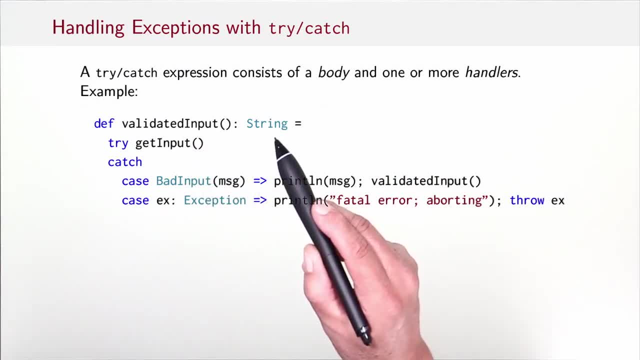 of type string that validates a user written input string. So it gets the input using getInput, And let's assume that this function here can throw a badInput exception if the input is not of the right format, say. So here we handle that exception with a catch clause. 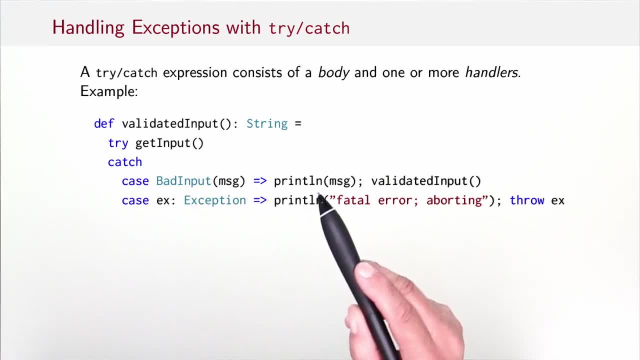 So we say: catch case: badInput message. In that case if the exception is thrown, then we print the message and we call validatedInput recursively, which means we invite the user to type in another input string. Here we also have a catch all or catch. 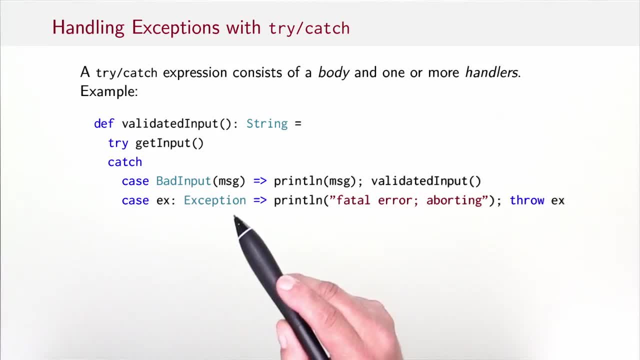 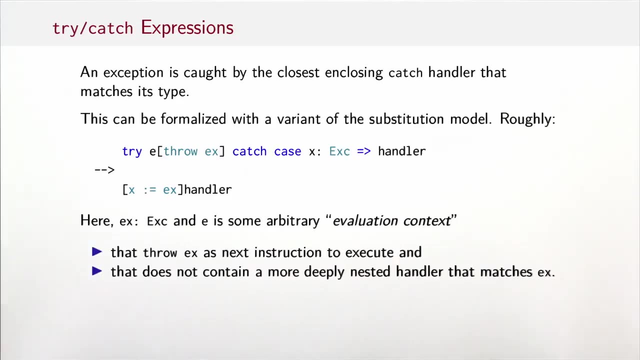 most exception. second clause that says: well, if it's some other exception, not badInput, then we print fatal error aborting and re-throw the exception. If there's no further try catch clause around validatedInput, this thing will abort the program. So generally, 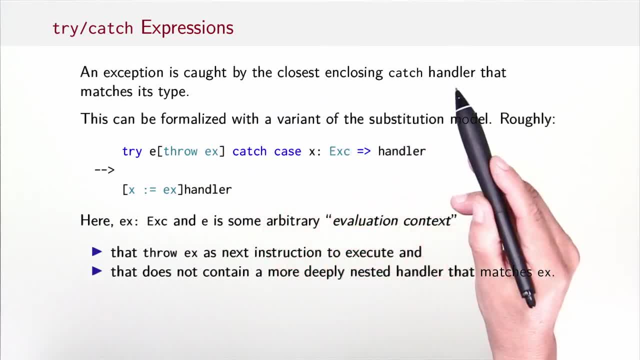 an exception is caught by the closest enclosing catch handler that matches its type. We can formalize this with a variant of the substitution model. So roughly we would formalize it like that. We would say, well, if we have a try and then we have somewhere. 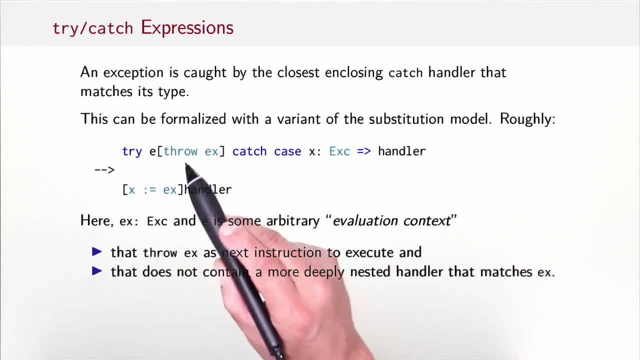 embedded in a so-called execution context e a throw exception expression, and then the try catches the exceptions with a catch clause, case x, xc arrow handler, such that the type of the expression x matches this type xc, in the catch clause. Then we continue the whole program. 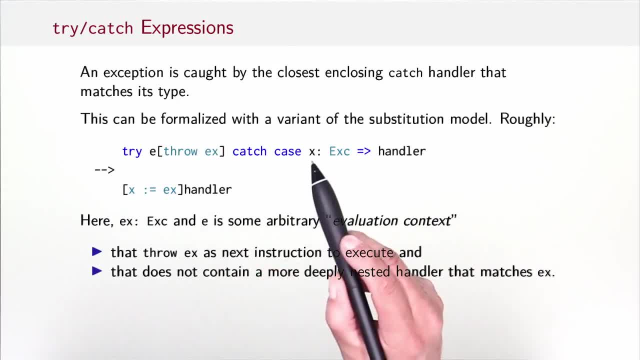 with the right hand side handler where the formal parameter x of the handler is replaced by the actual exception ex. So the evaluation context e here can also be defined formally, but we won't do that here. It's basically a context that has the throw x at some place. 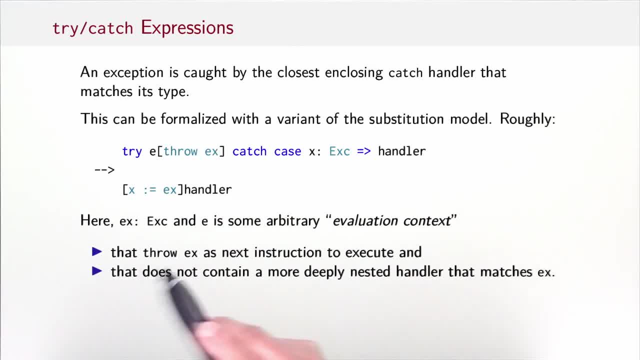 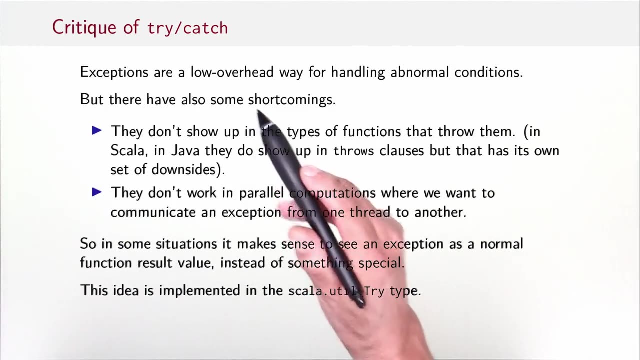 in some surrounding program code, such that the throw x is the next instruction to execute and that context does not contain a more deeply nested handler that also matches x. Exceptions and try catch are a convenient and low overhead way for handling abnormal conditions, But there are also some. 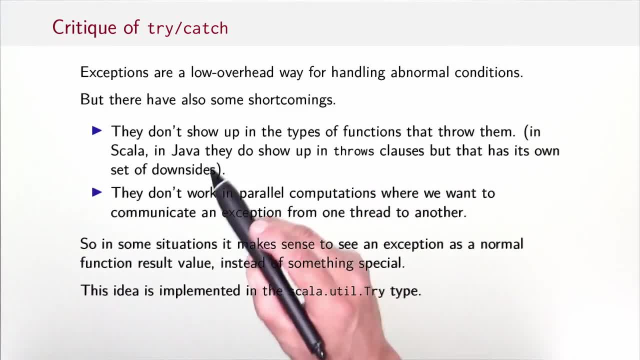 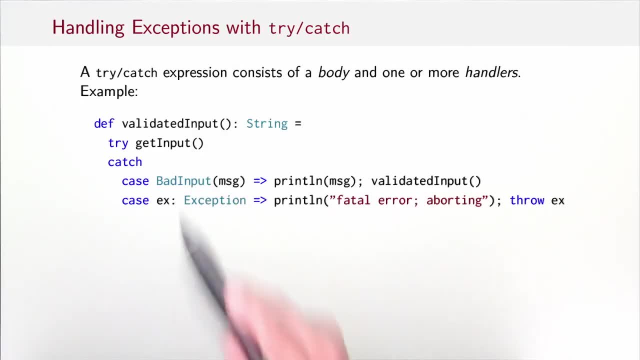 shortcomings. The first shortcoming is that exceptions don't show up in the types of functions that throw them. For instance, in the validated input example, that method here could throw an exception, but its type doesn't tell us that. Its type just says it will return a string. 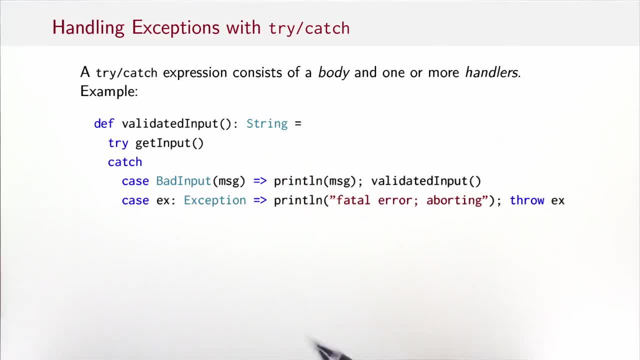 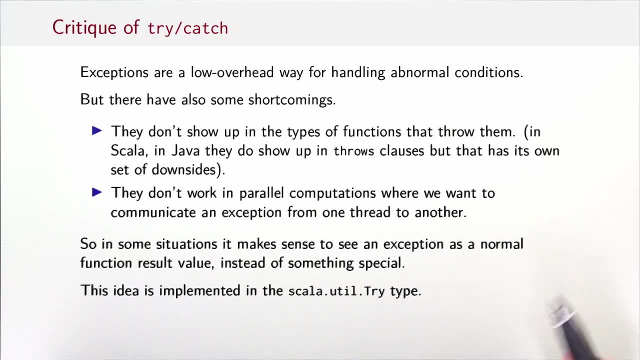 So exceptional values are not part of the return type of a function, which means that we are ignoring something which could be very important for software safety. That's the situation in Scala. Actually, in Java, certain exception types do show up in so called throws clauses, but it turns. 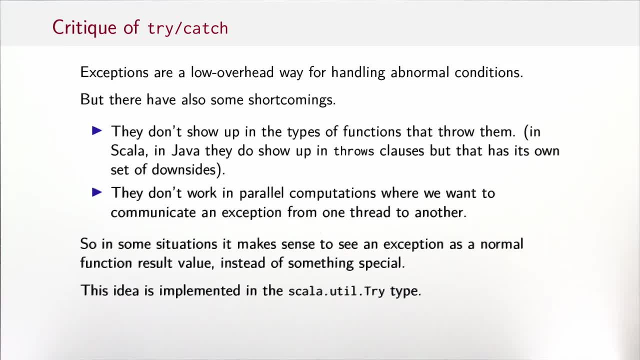 out that this has its own set of downsides. These throws clauses are typically quite inconvenient to write and not very flexible. It would be very hard, for instance, to write a function like map that handles throws clauses correctly in all circumstances. So that's why the example of Java 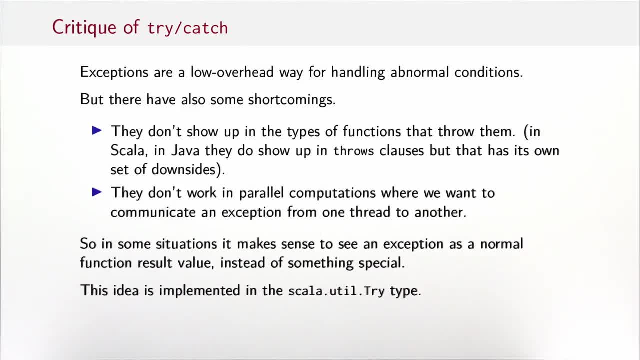 by and large, has not been followed by other languages. Most other languages do not have exceptions in the result types of functions But, as I said, this is a problem from the standpoint of program safety. One of the research topics of my group at EPFL is precisely 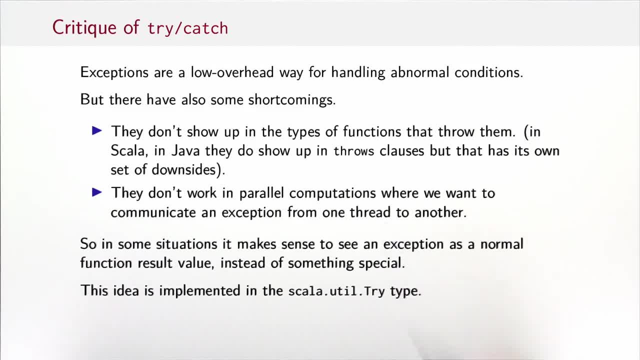 to find a new way to express effects- which what exceptions are? that doesn't have the shortcoming of the throws clauses in Java, So that can be written flexibly, that is polymorphic and can be used to augment the contract of a function to also represent its. 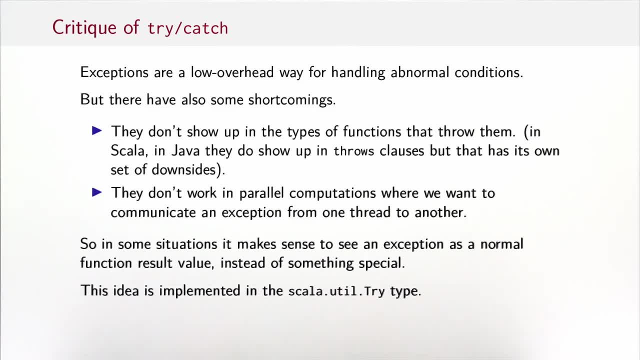 exception types. But that's research, so we are not there yet. The other shortcoming of exceptions is that they don't really work in parallel computations, where we want to communicate an exception from one thread to another, Exceptions are by their very nature tied to one thread. 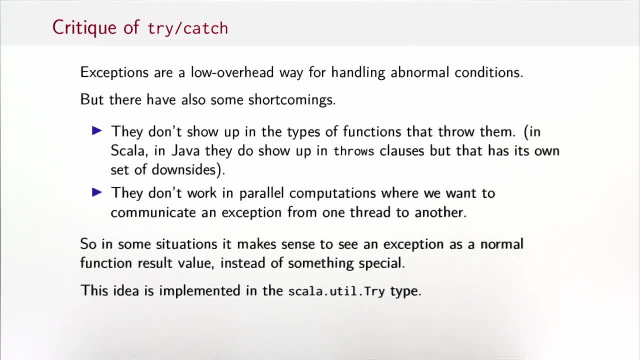 So it's in one thread that an exception gets thrown and caught. but to signal an exception condition from one thread to another we need something else. So definitely in some situations it makes sense to see an exception not as something special that gets thrown and caught, but as a 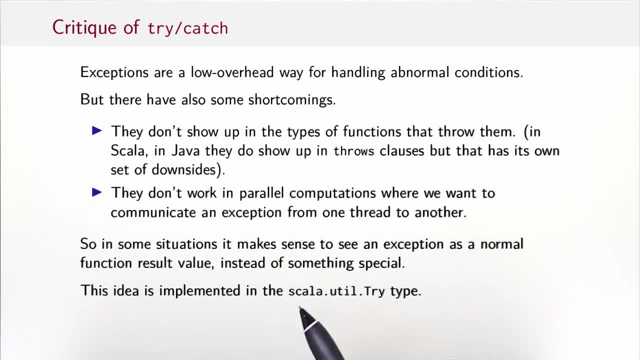 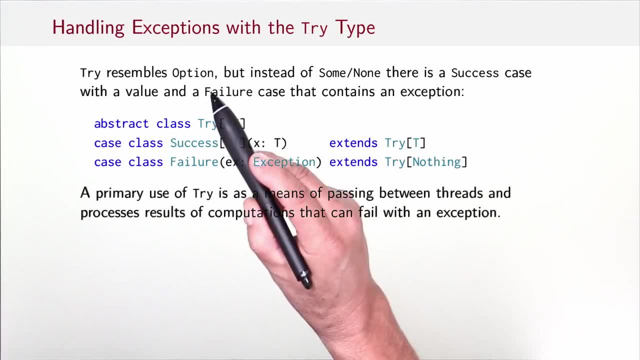 normal function result value. This idea is implemented in the type ScalaUtilTry. So here you see the definition of the try type. It resembles option, but instead of sum and none we have two cases: success and failure. So the success case is the analog of. 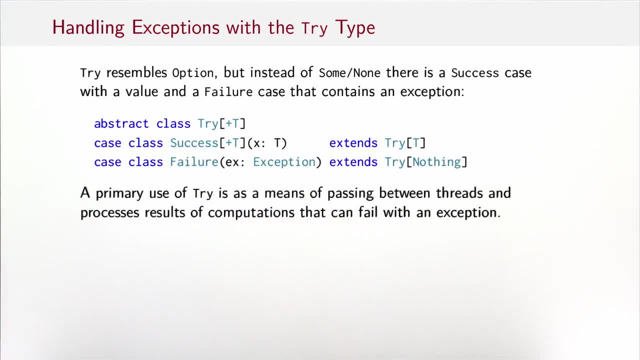 sum, It takes a single value that it returns. The failure case, however, has some additional information and that is an exception. So the failure case would be returned if the original computation through an exception, As is the case for sum and none success extends. 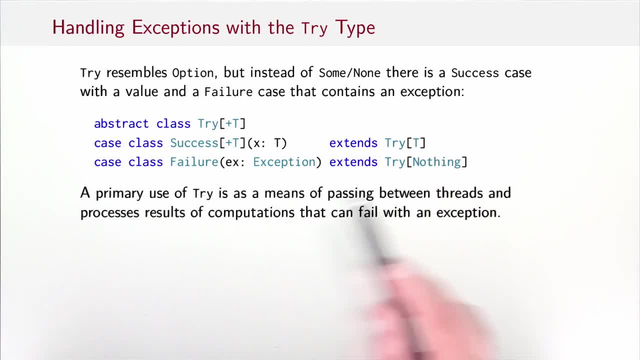 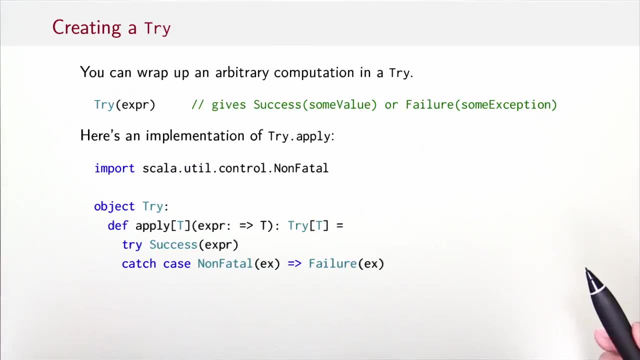 try of t with the type parameter t and failure extends try of nothing because no normal value is returned. in that case, A primary use of try is as a mean of passing between threads, and pauses is the results of computations that can fail with an exception. 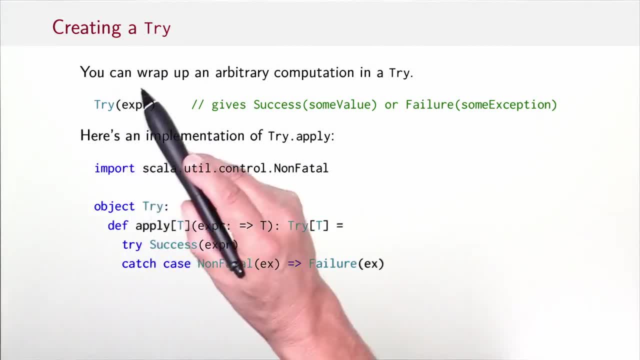 So how do you go from exceptions to tries? Well, you can wrap up an arbitrary computation in a capitalized try. here, Try of expression gives success with the value of the expression if there is no exception, and it gives failure with some exception if that expression, through that exception. 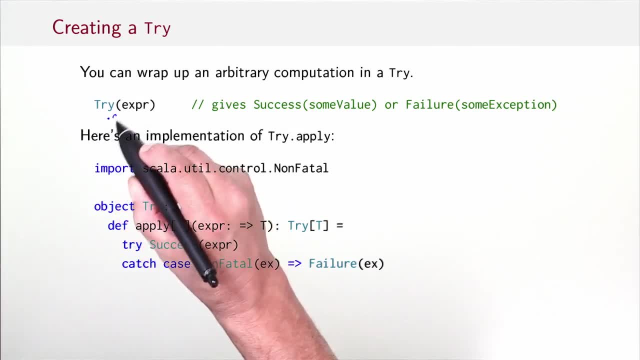 As usual, this is not magic, but simply an application of an apply method in an object named try, and here is its implementation. So apply takes a by name parameter expression. so expression is not yet evaluated when it is passed to apply and it returns a try of t. 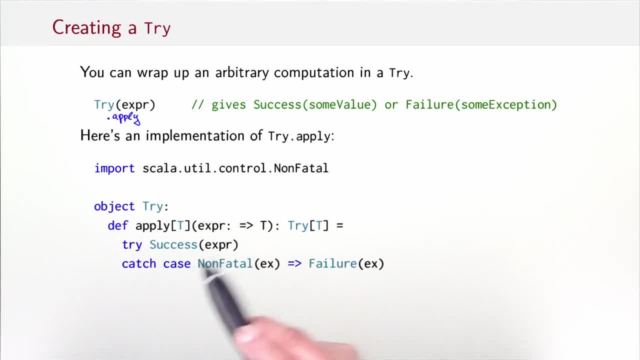 It says: okay, wrap the value of the expression in a success, unless there is an exception, a non-fatal exception, in which case we wrap the exception that got thrown in a failure. Here, non-fatal matches all exceptions that allow to continue the 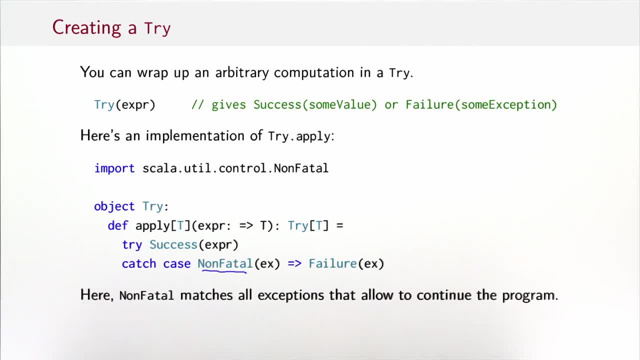 program. Among all the exceptions that can be thrown from a Java program, some of them really terminate the virtual machine and there is no good way to recover from them, So those are bypassed, but the others are caught in non-fatal Okay, just like with options. 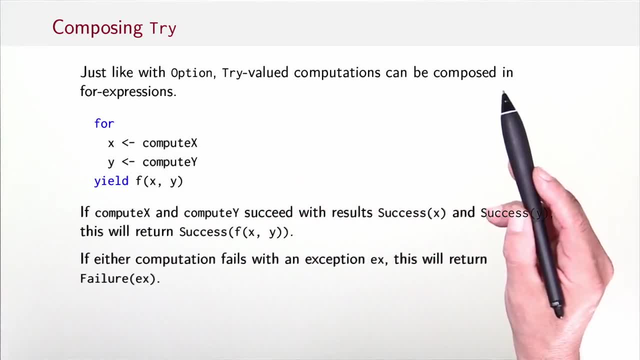 try valued computations can be composed in four expressions, which means that try has flat map and map defined. So you see an application here for x taken from some computation, y taken from some other computation, yield of the function f of x and y. So what this does is that 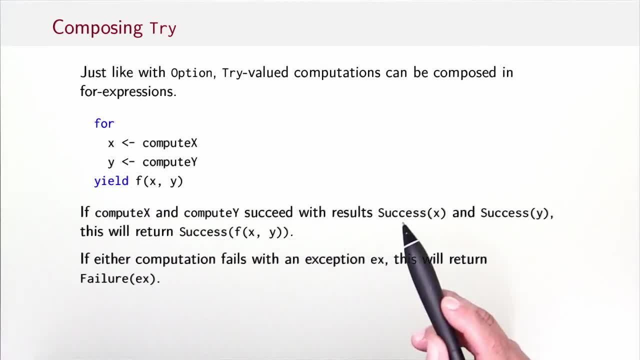 if compute x and compute y succeed, with results success x and success y, this will return success f of x and y. If either computation fails, with an exception e x, this will return failure of e x. So it will first do compute x and if that's successful do compute. 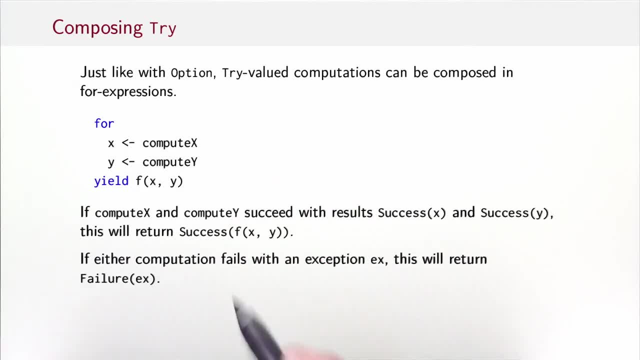 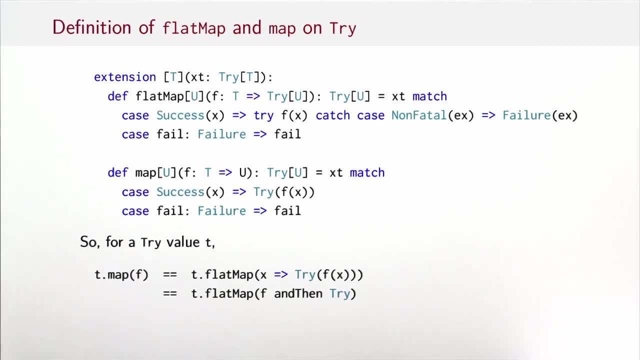 y. If either of them fails, you get a failure. If both of them succeed, you get this success value. So to be able to write four expressions on tries, we need a map and flat map. Here they are. Let's do flat map first. So it takes. 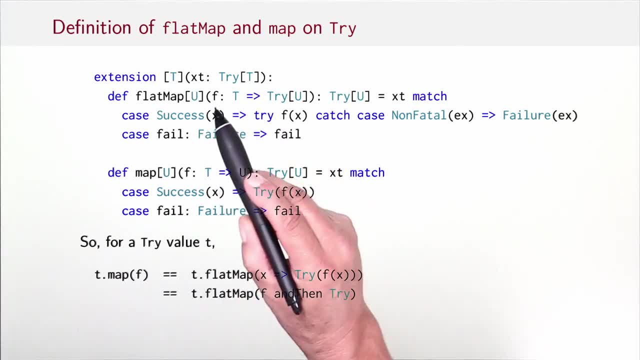 an xt of type try of t and a function f that maps a t to a try of u and returns a try of u. And here's the implementation: If xt is success of x, then it goes on with f of x. But there's 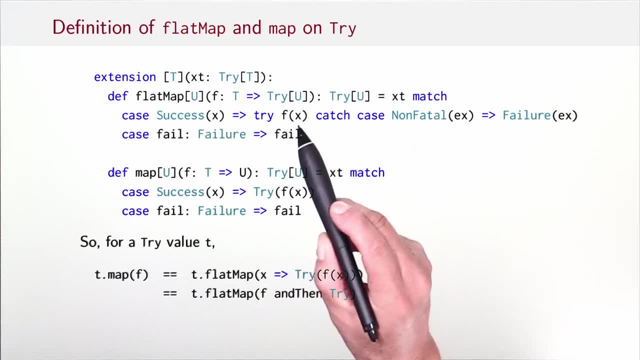 a catch clause that says: well, if the second operation throws an exception, a non-fatal exception, then we convert that to a failure x. So, in essence, what this does is we won't let exceptions escape the flat map of the try. If the first 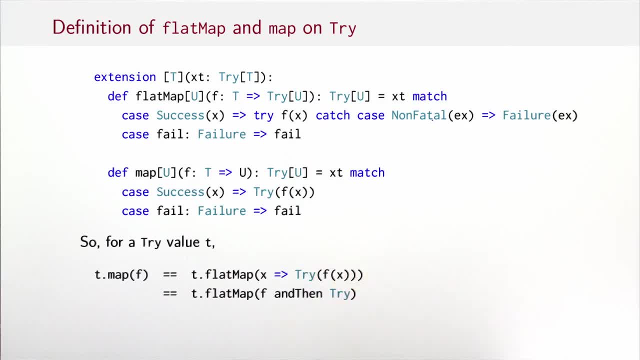 try was already a failure, then we just propagate that. Here's the definition of map. So it says: well, if the original try is a success, then apply f to x and wrap it again in a try, And if it's a failure, then fail. 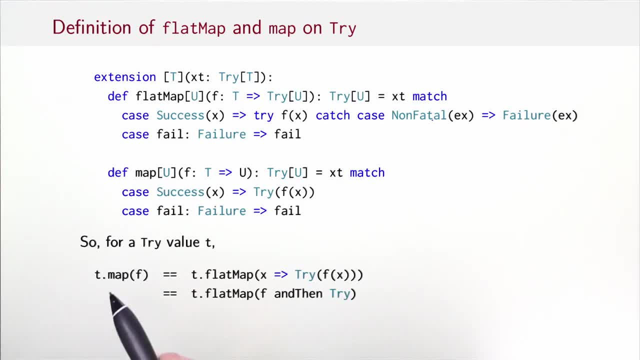 So we can establish a relationship between map and flat map as follows: So t dot map f is the same as t dot flat map x. try of f of x. So by working with these definitions, we can establish the following relationship between map and flat map. 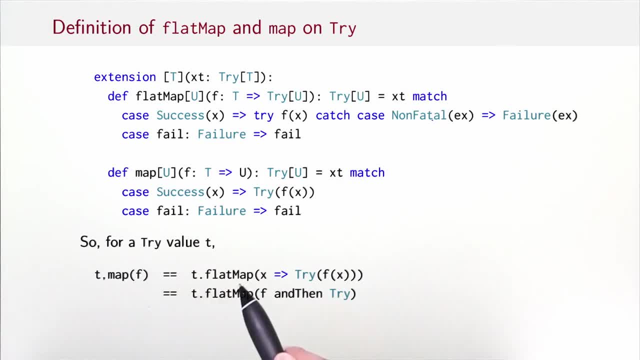 t dot map of f. is t dot flat map of the function that maps x to try of f of x, And that again is just t dot flat map f and then try. So that looks familiar. It's just a relationship between map and flat map in a monad. 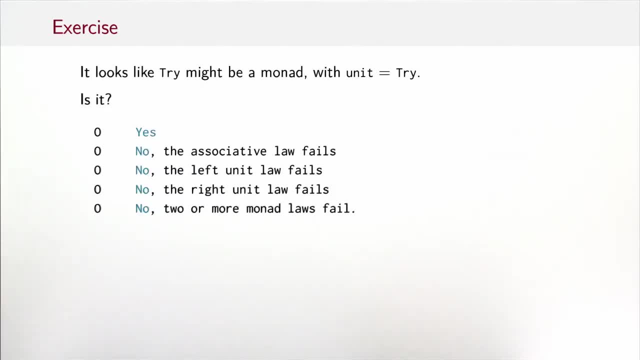 where the unit is try. So it looks like try might be a monad, with unit equals try. Is it Possible? answers are yes or no, because the associative law fails or no, since the left unit law fails or no, since the right unit law fails or no. 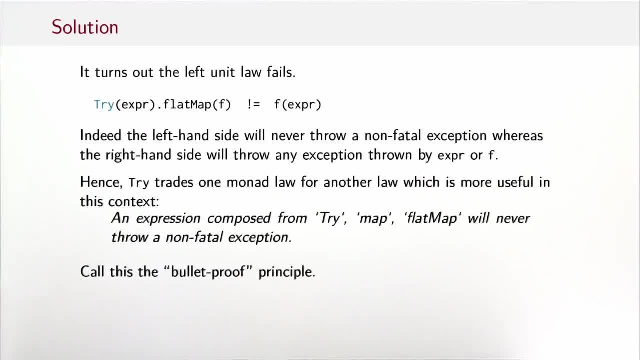 because two or more monads laws fail. The solution is, it turns out the left unit law fails. So try expression dot flat map. f is not the same as f of expression. Why not? Well, the left hand side? what we've seen, we know that it will never throw. 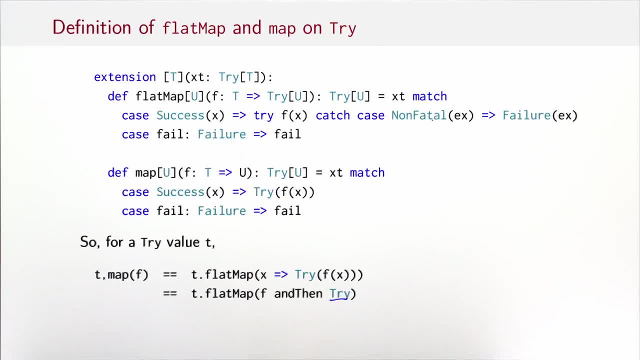 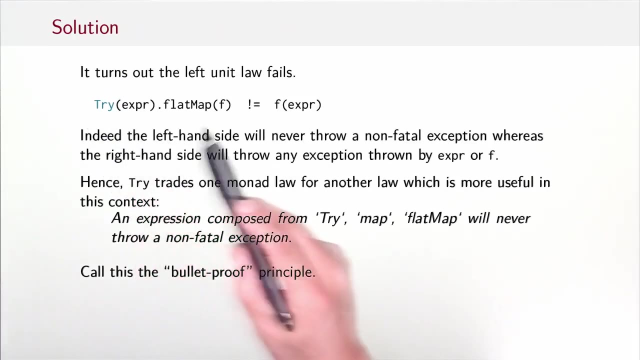 a non-fatal exception. That was the definition of flat map, Essentially everything we do here in the definition. if the computation of flat map gives a non-fatal exception, we catch it and return failure instead. So the left hand side doesn't return an exception, but the right hand side. 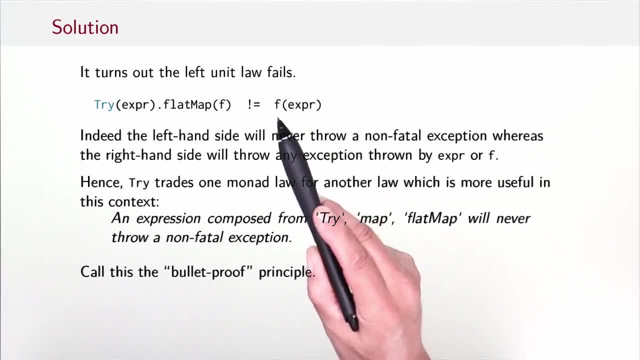 could of course Any exception thrown by either expression or f would be propagated in the result. So that means that the left unit law here doesn't hold. You can see it this way: Try: trades one monad law for another law, which is probably more. 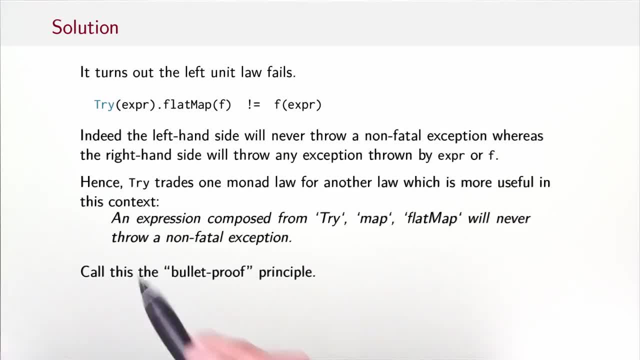 useful in this context. Let's call it the bullet proof law. The law says an expression composed from try, map and flat map will never throw a non-fatal exception, And that, of course, is another good property to have, Which just goes to show that. 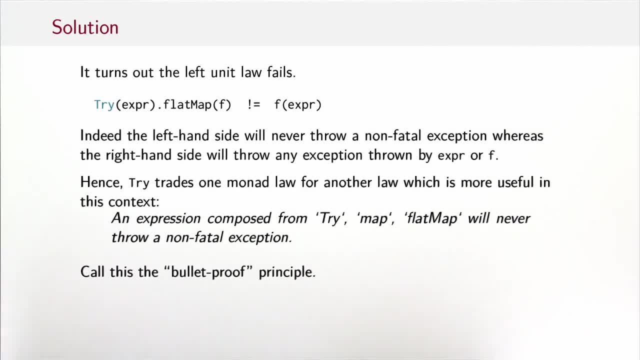 laws, whether monad laws or others, are not sacrosanct. It always depends on, essentially, what the situation is and what we need these laws for. Even if try is not completely a monad, it's still very useful and it's also possible to use. 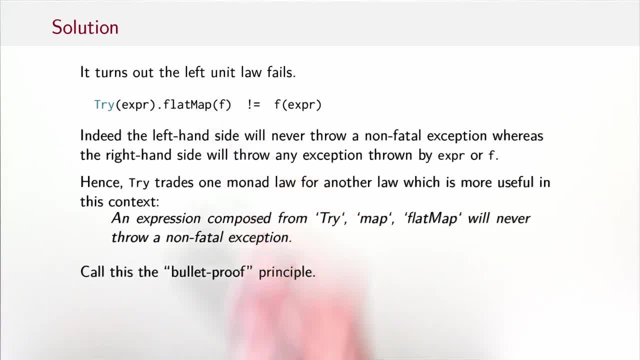 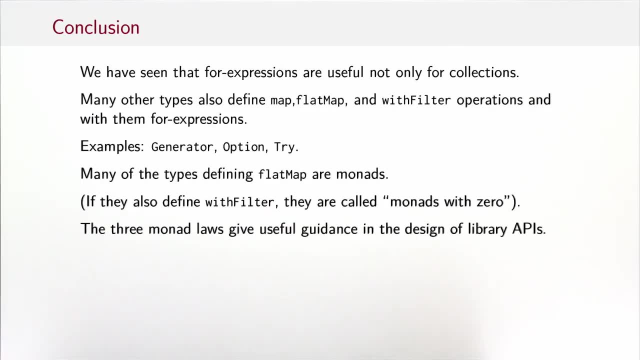 four expressions with try, because it turns out that the left unit law is the law that actually is not relevant for the correct expansion of four expressions. So to conclude, we've seen that four expressions are useful not only for collections. Many other types also define map, flat map and with filter. 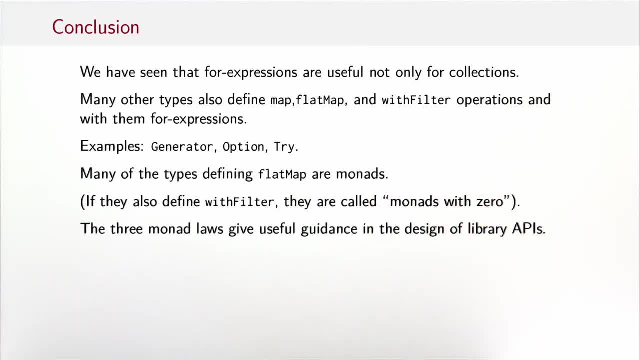 operations and with them four expressions. We've seen generators, we've seen option and we've seen try as examples. Many of the types that define flat map are indeed monads. If they're also defined with filter, they are called monads with zero. 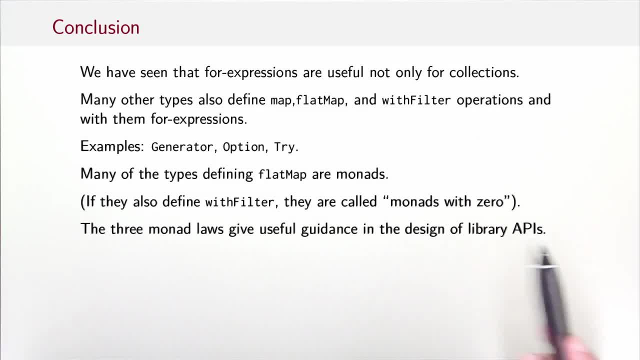 The three monad laws give useful guidance in the design of library APIs, So essentially break them at your peril. You should know what you're doing when one of the laws is broken and generally it's better to strive to actually have these laws and verify. 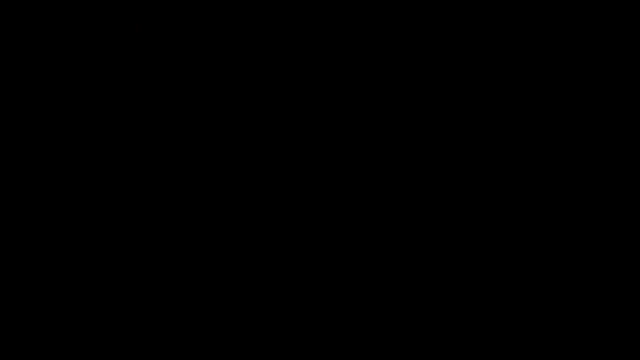 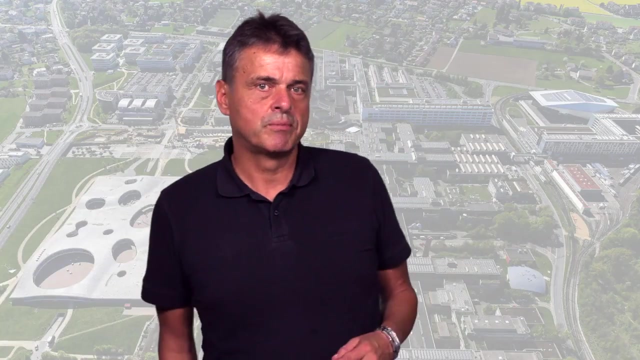 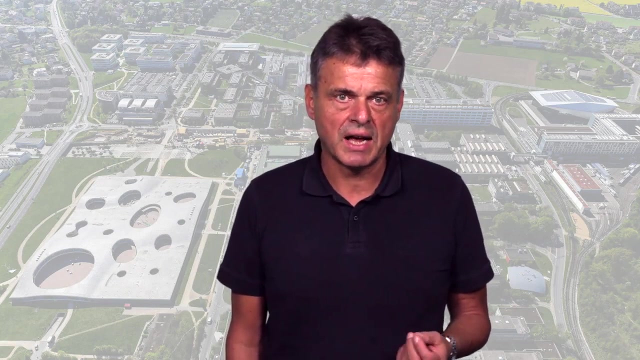 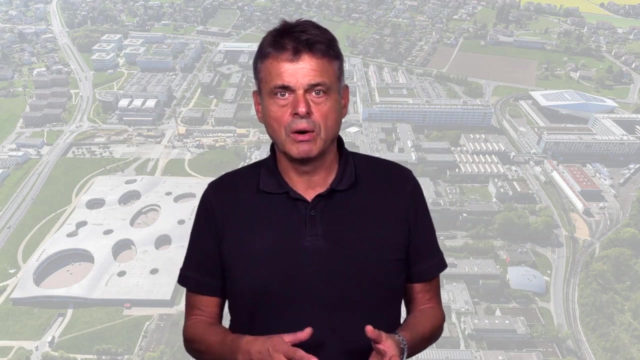 that they do hold. This week we'll revisit performance issues caused by combinatorial search and we'll discover an important concept in functional programming that can address these issues. The concept is laziness. Being lazy means computing a result only when it is needed. 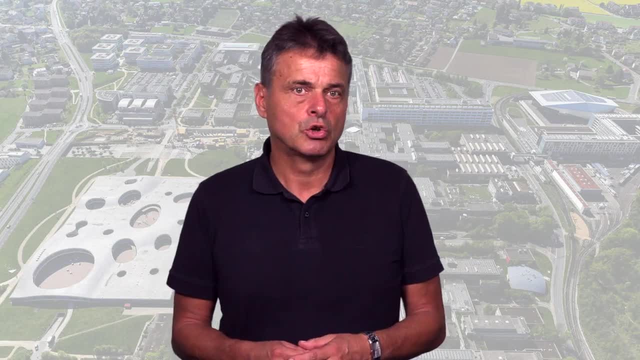 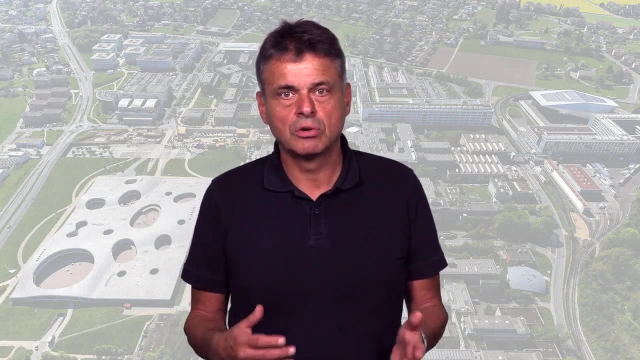 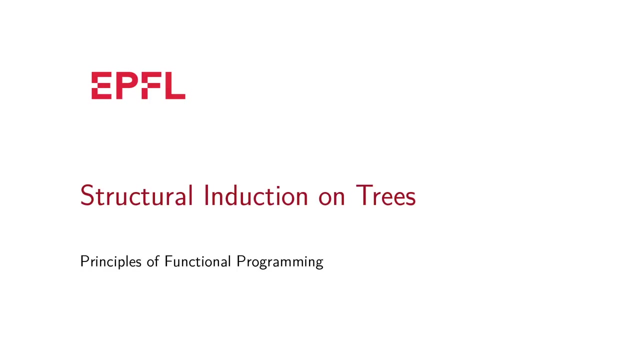 It turns out that this is a general and quite effective technique to speed up some functional code. You'll also learn a little bit about proofs on trees. In particular, we'll see how to extend structural induction to trees. In this session we're again looking at proving. 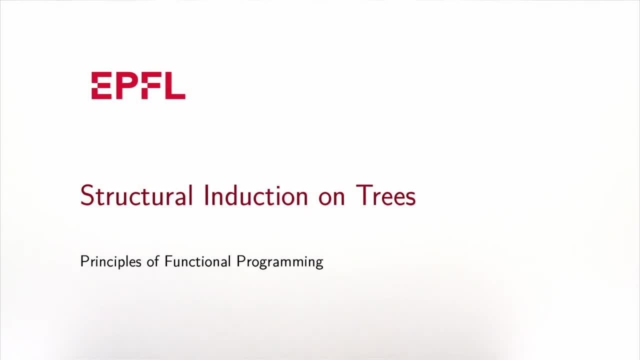 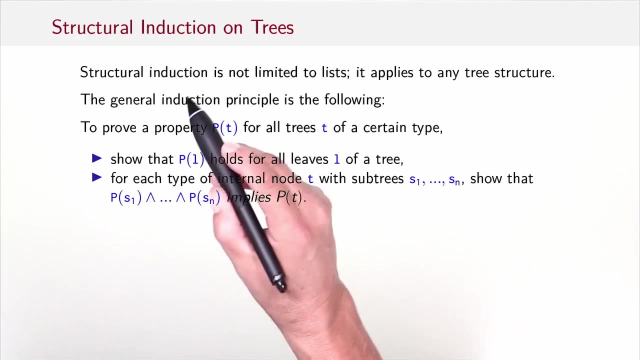 things about functional programs. More specifically, we are going to prove laws about data structures using structural induction on trees. You know structural induction on lists from the first half of the course, But structural induction is in fact not limited to lists. it applies to any tree. 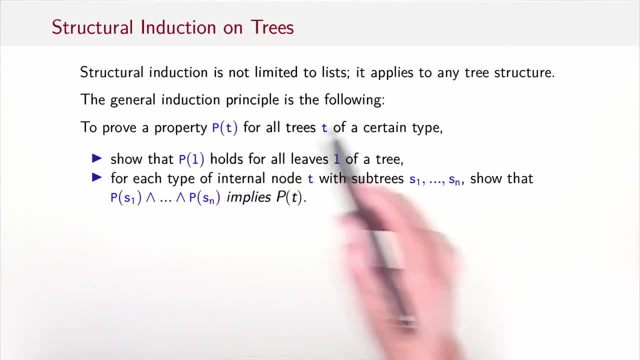 structure. The general structural induction principle is like this: To prove a property, P for all trees T of a certain type. show that P holds for all leaves L of a tree and for each type of internal node, T with subtrees S1 to. 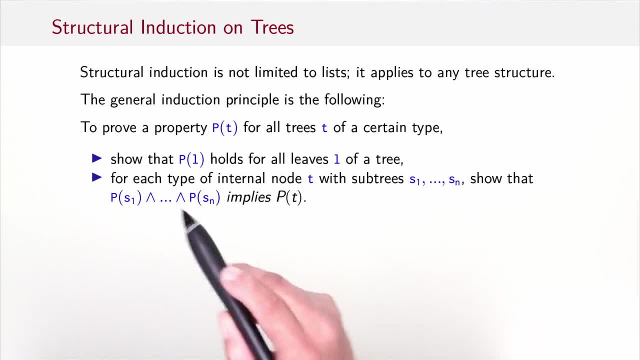 SN show that P of S1 and P of SN and so on implies P of T. So if you have a tree with leaves here and some internal nodes, something like that, then the structural induction principle says: well, prove it for all leaves. and assuming 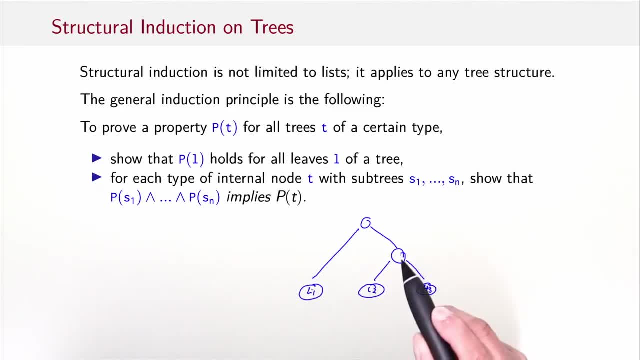 that you have already shown it for the subtrees, let's say for this one, and this one show it for the interior nodes as well. So if you can do that, then you have established the principle for all trees. So to demonstrate that proof principle, 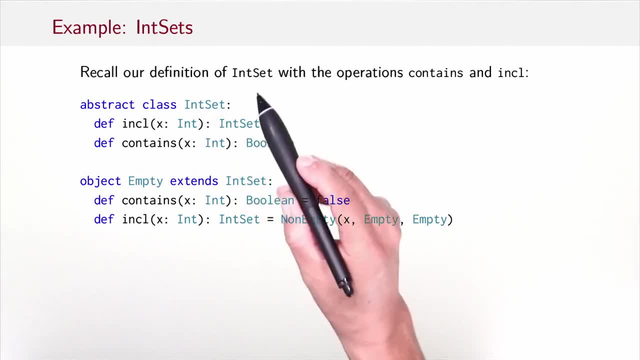 let's go back to int sets. Recall our definition of int set. There was an abstract trait with two operations- include and contains- And that was implemented either by an object empty- where you see the definition of contains and include like that- or by an object non-empty. 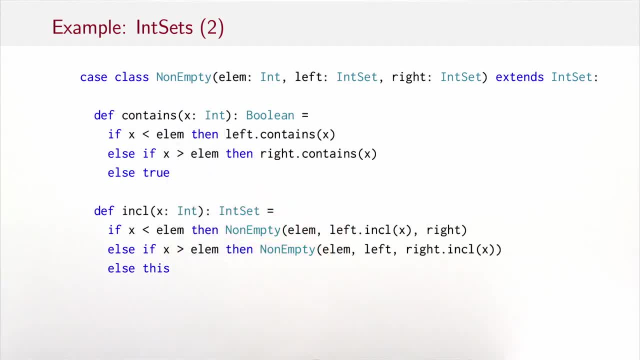 where you saw the definitions of contains and include, like that For a non-empty object. we always had a case distinction where the element to look up or to include is less than or equal or greater than the element on the right, And depending on that, we would then proceed. 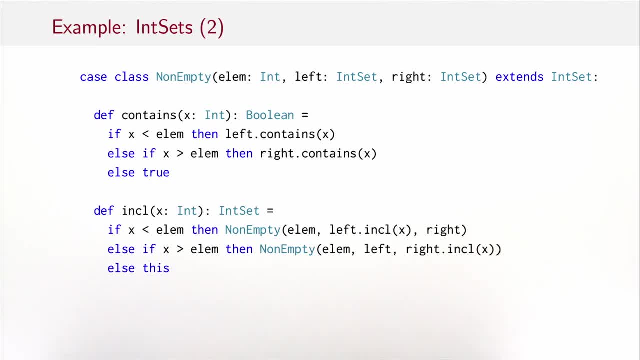 with the left or the right subtree. So the invariant of these sets was that elements are ordered in the sense that if we have a tree here, and so that's, let's say, lm equals 8, and then we have some subtrees here and some subtrees. 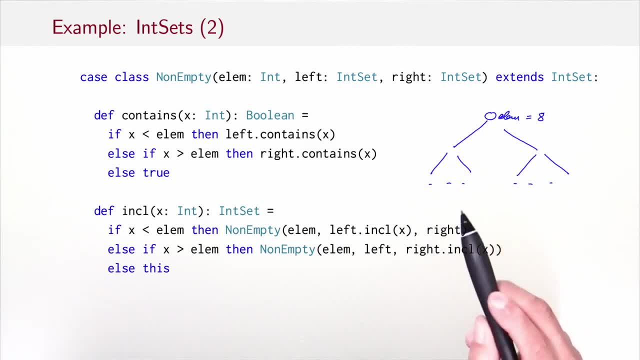 here. then all elements in the left subtree would be less than the element at the root, so less than 8 in this case- and all elements on the right subtree would be greater than that root element. So that's a class hierarchy that claims to. 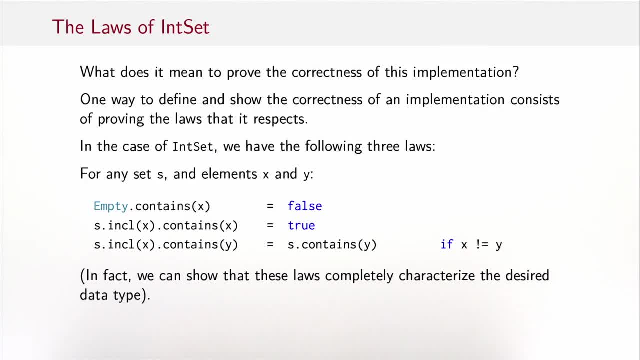 implement int set, but how do we know it's correct? Or what does it even mean to say an implementation is correct for int sets? Where is the specification of int set? Well, for that it's good to go back to the introduction of the very first. 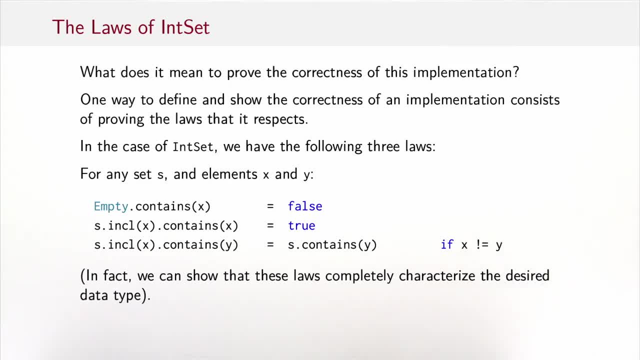 week of this course where we talked about paradigms and why functional programming is based on theories, And there we said: a theory is characterized by some values, operations on these values and laws that relate the operations. So we can do that for int set and then 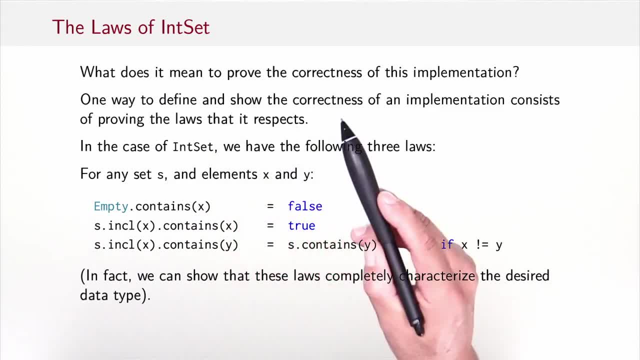 if you have laws for int set, then one way to define and show the correctness of an implementation means prove that the laws of int set holds for this implementation. So what are the laws of int sets? I propose those three here. So the first law says: 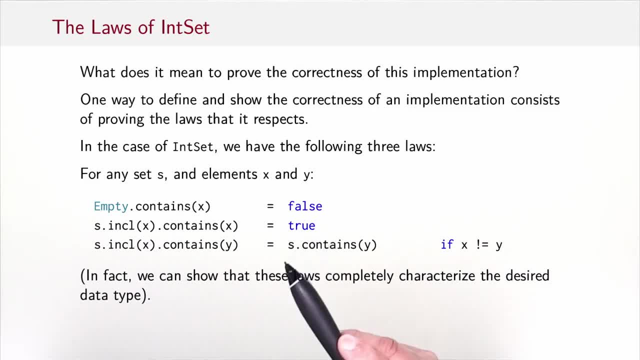 empty contains x is always false. The empty set contains nothing. The second law says s include x contains x is true for any set s. So if we include an element in the set and then ask whether the set contains the same element, then that's true. 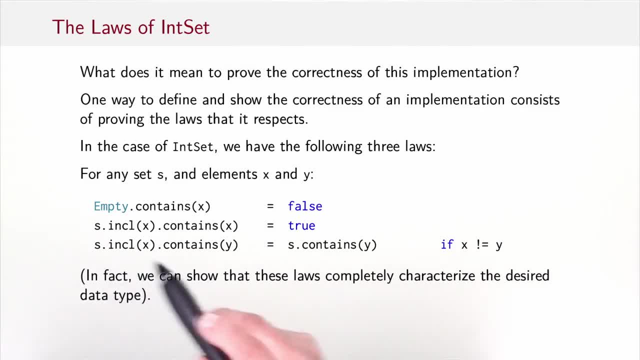 And the third law says that s include x contains y is s contains y If x not equal y. So that means if I include an element x in a set and then ask whether the set contains another element different from the included element, then that's the same as asking whether. 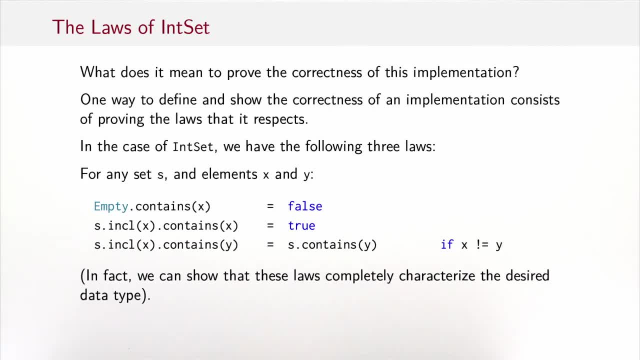 the original set contains that other element. So these laws obviously make all sense of int sets and furthermore, one can convince ourselves that these laws completely characterize what makes up an int set if we restrict ourselves to just the operations contains and includes. So we now proceed to. 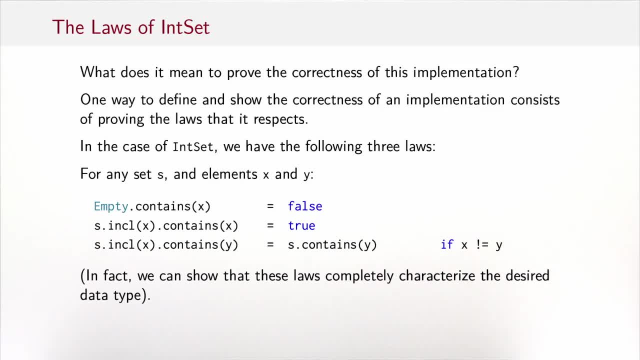 prove these three laws using structural induction on trees. The material that follows is a bit more on the theoretical side. If you are more practically minded, then you might want to just essentially quickly browse it or skip it altogether and continue with the next session after. 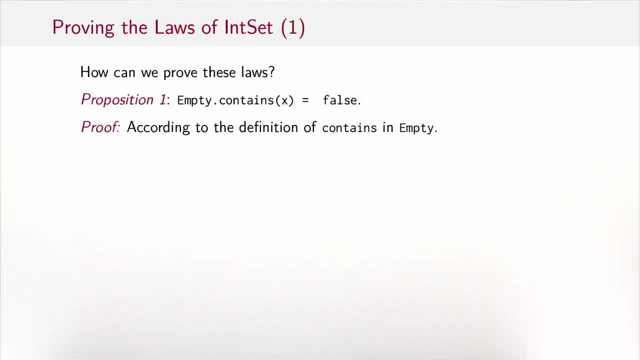 So let's go on and prove these laws. First law is empty contains x equals false. Well, that's obviously true, because that's how contains was defined on empty. So, according to the definition of contains, that's false. The second law is: s include x contains. 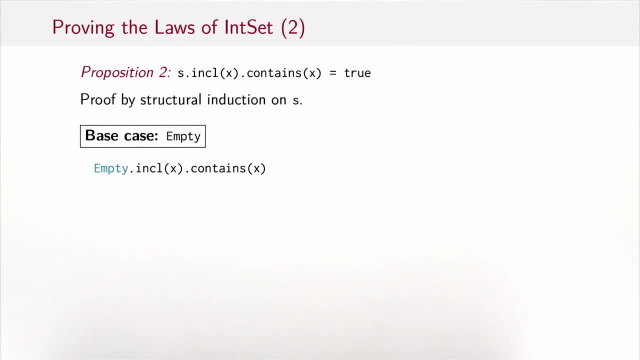 x equals true. We prove that by structural induction on the tree s. So the base case is: s is empty and we have to prove empty include x contains x. So that's by expanding include that gives us non-empty x. empty, empty contains x. 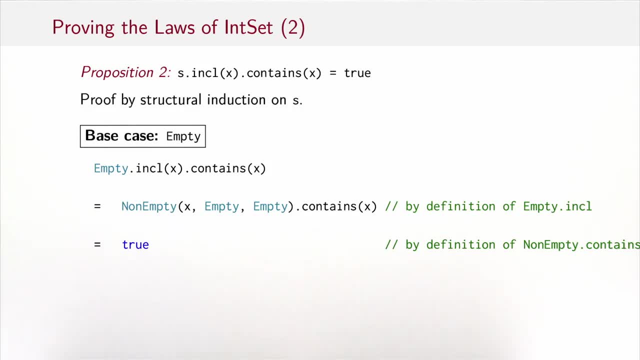 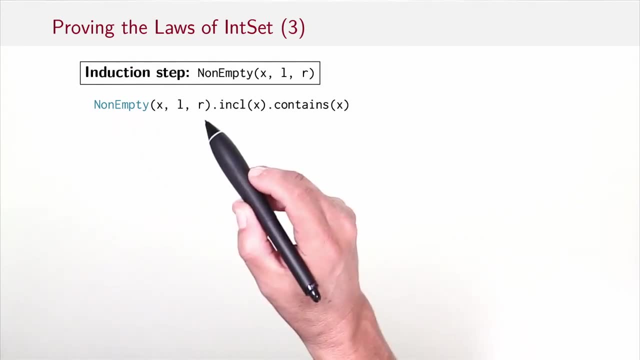 And then by the definition of contains for non-empty trees. that is true. So let's now prove the induction step. The induction step means that our set s here is of the form non-empty. then some root element, some left tree, some right tree, And there are several cases to consider. 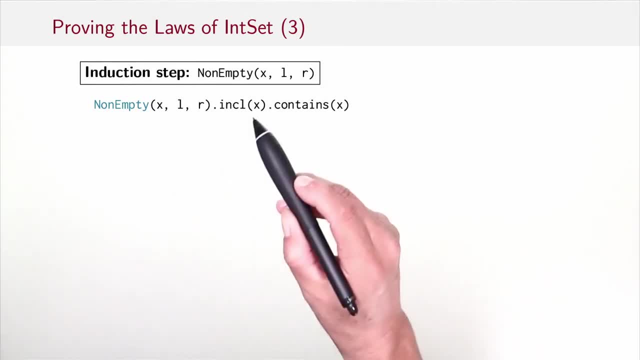 The first case we consider is that the root element x and the element we include is the same one. So we have this expression here and that one simplifies directly, because including an element in a set that already has that element at the top is the set itself. 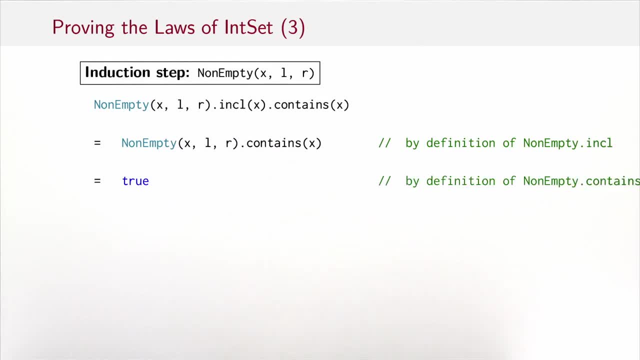 And asking whether this set contains x is, according to the definition of contains, true, So the law holds for that case. But that was just one of the possible cases for the induction step. Let's look at the other. So the next case would be: 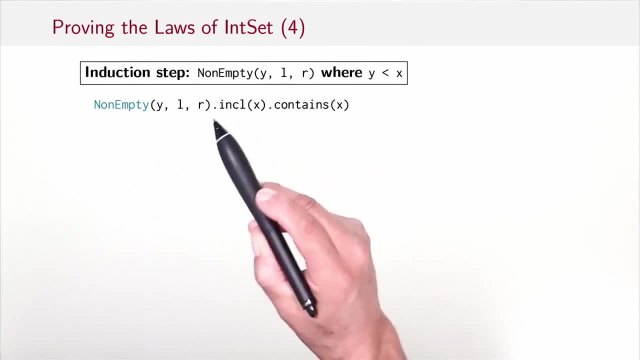 non-empty y l r for the set s where y is less than x. What do we have in that case? So we have non-empty y l r include x. What does that give? Well, according to the definition of include, it means that if we include x. 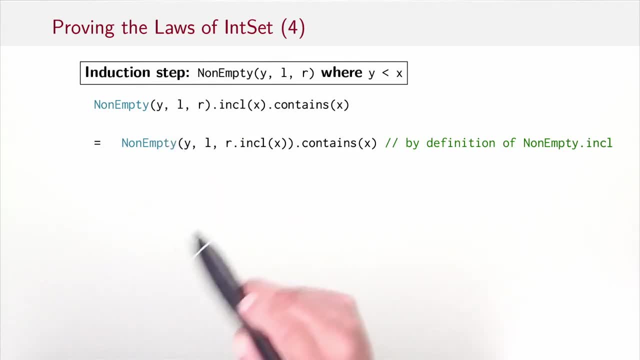 in a set where x is greater than the root element, we recursively include it on the right subtree and reform the set with the remaining elements. So that's what you see in this expression here, And we ask whether that expression contains x. Now we look at the. 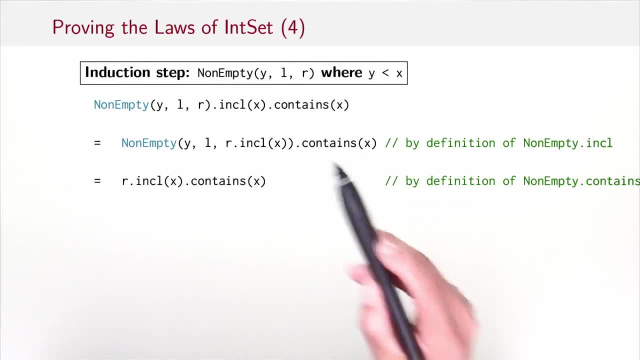 definition of contains. The definition of contains says: if x is greater than the root element y, then look in the right subtree That would give us r dot. include x contains x. And now we can use the induction hypothesis, because we are allowed to assume that. 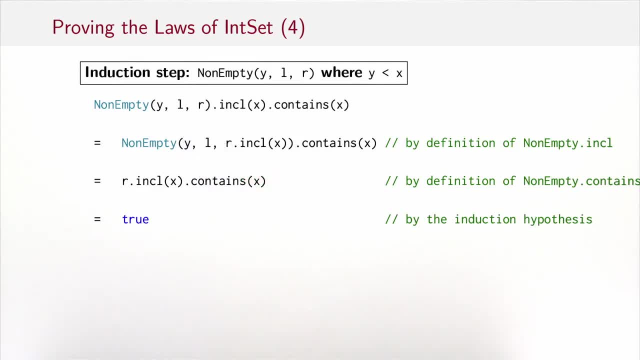 on each of the two subtrees of this non-empty set the condition holds. So we know for the tree r that r include x contains x, that the second law is true, and that means that the same holds for the non-empty tree. here There is a third case to consider. 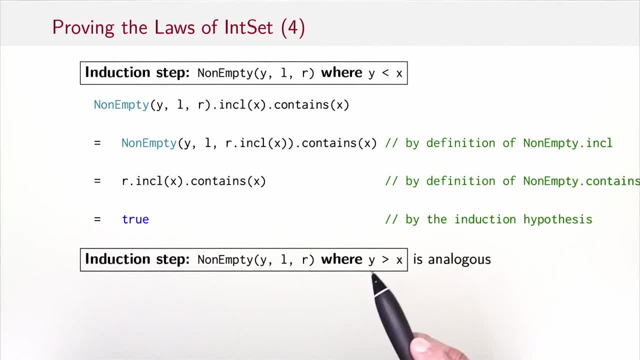 namely that we have a set of the form where now y is greater than x and that one is of course completely analogous. So I won't repeat the reasoning here. You can try it for yourself if you want. So the last proposition is this one here: 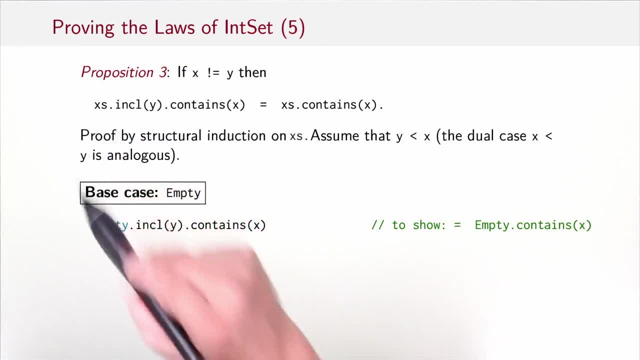 So if we have a set- let's call it xs- and an element x that's different from y, then xs include y contains x is the same as xs contains x. So asking whether a set contains an element after another element is included is the same as asking whether 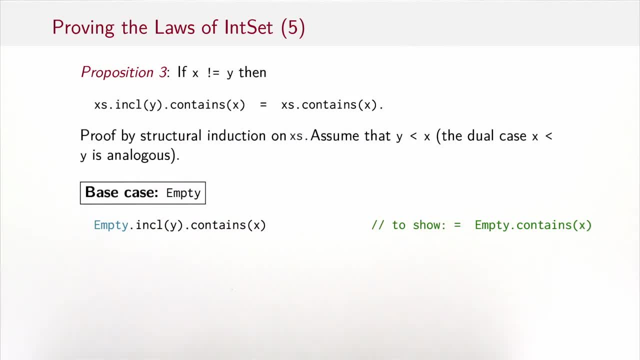 the original set contains that element. So we prove that law by structural induction. on the set xs There are two cases to consider. if x is different from y, then either x is smaller than y or larger than i, and we just assume the second case, that x is larger than y. 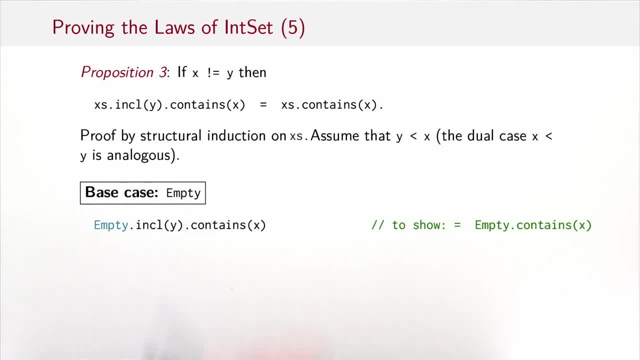 the case where x is smaller than i is, y is again completely analogous. We have empty include y contains x and we need to show that empty contains x. That's the right hand side here, So let's expand inclaw. that would give us nonempty. 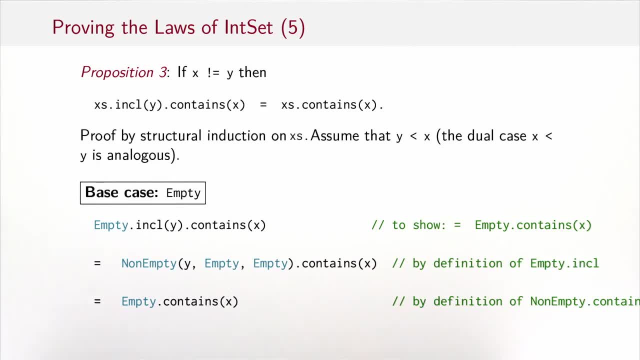 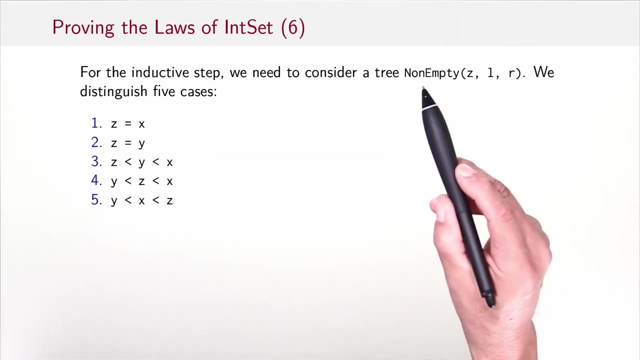 y empty. empty contains x, and that means we have to look in the right subtree. so it's empty, contains x. and that is our right hand side. so that's what we needed to prove here. So we've established the law for the case empty. Here we need to consider: 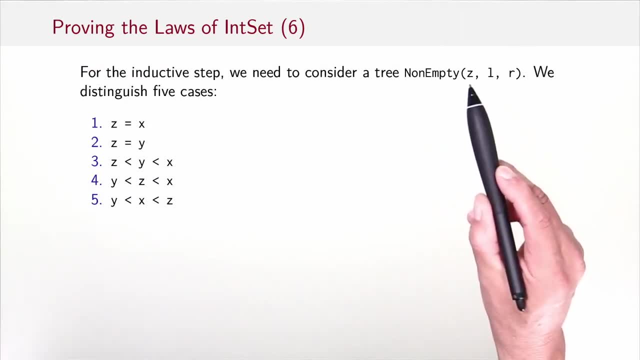 a tree, nonempty zlr, where the element z and the left and right subtrees l and r are arbitrary, And now it depends on where z is relative to y and x. So we have y and we have x and essentially the z could be. 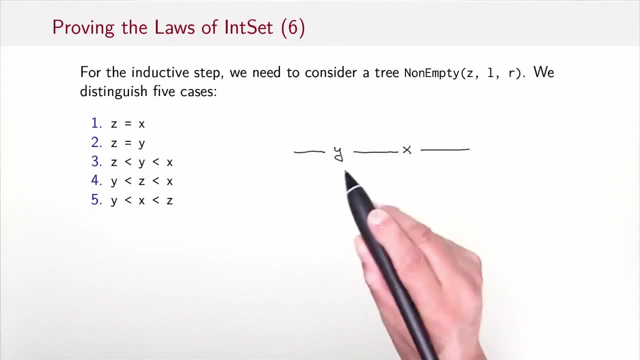 anywhere here. it could be less than y, it could be between y and x, it could be greater than x or it could be one of y and x. So that gives us five cases. z is x, z is y, z is less than y. 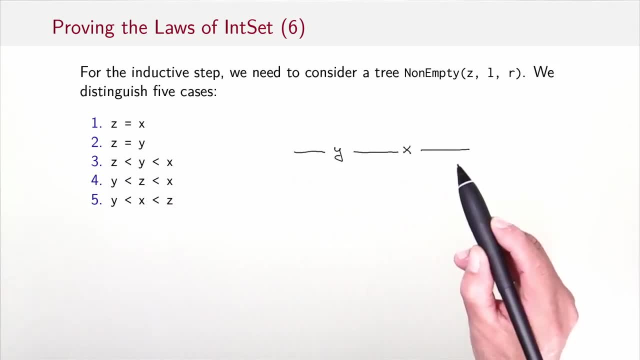 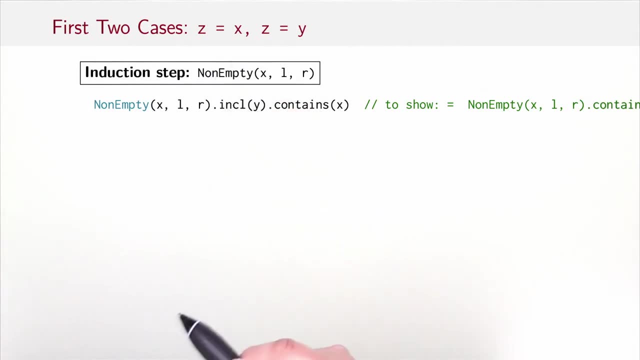 z is between y and x and z is greater than x. So let's tackle each of these five cases in turn. The first case is z equals x. so we have nonempty xlr include y contains x and we have to show that this is the same as. 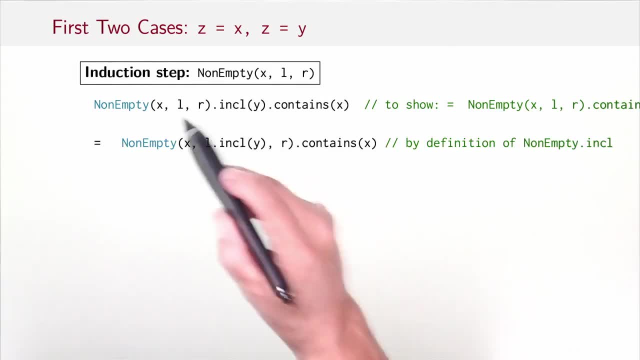 nonempty xlr contains x. So we know that y is less than x. so we construct a left subtree with y including and wrap the nonempty node around. that's what that looks like and we ask again whether it contains x. And now the answer. 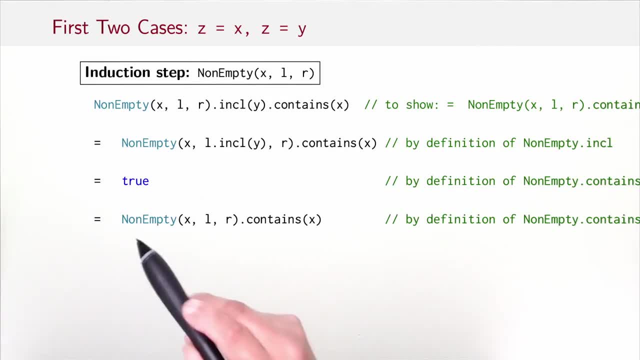 is true, of course, And that's also the answer. if we ask: nonempty xlr contains x. So we have established the equality. What if z equals y? Then our induction step would look like this: and we have to show that nonempty ylr contains x. 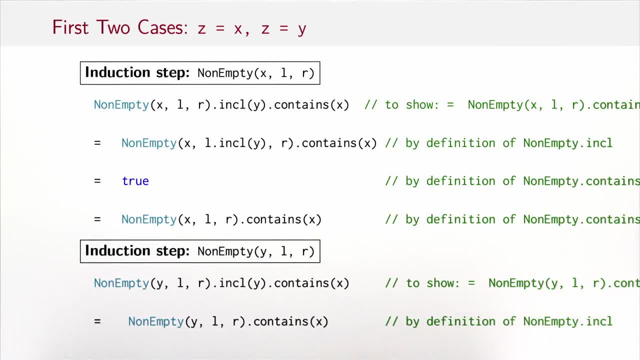 And that follows directly by the definition of nonemptyinclude, because that's how nonempty is defined: If we include an element that's already in the root, then we return the original z. So we're done for the two simple cases: z equals x and z equals y. 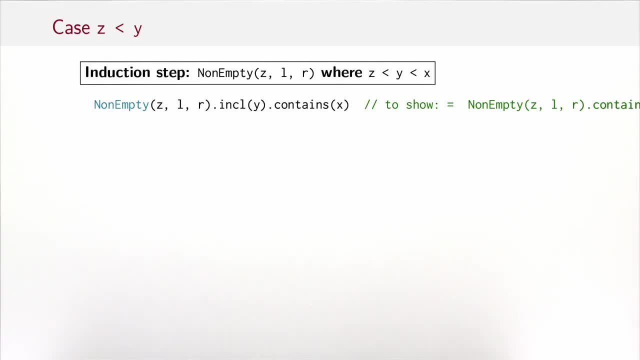 So what about the case where z is the smallest of the three elements, So z smaller than y. So we now have nonempty zlr where z is smaller than y and, as always, y is smaller than x. That's what our initial expression looks like. 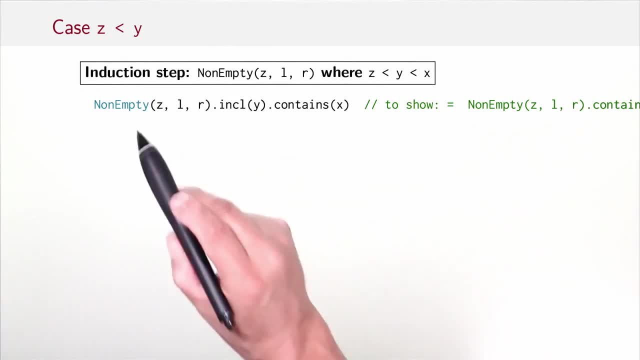 and we have to show that that's equal to nonempty. zlr contains x. So by definition of include, we now include y in the right subtree because y is greater than z. That gives this tree here and we ask whether it contains x. 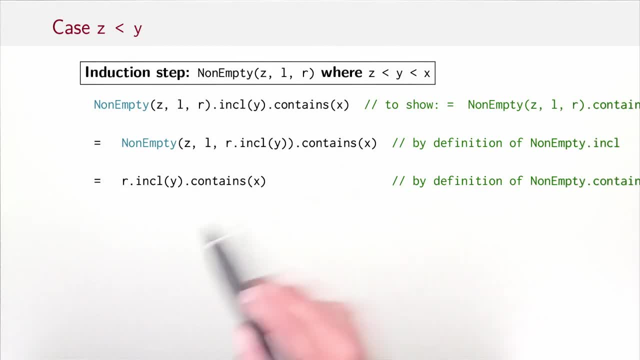 By the definition of contains z is smaller than x as well. so we look in the right subtree that gives this expression here and by the induction hypothesis, that is, r dot contains x. And if we compare that to the right hand side, nonempty zlr contains x. 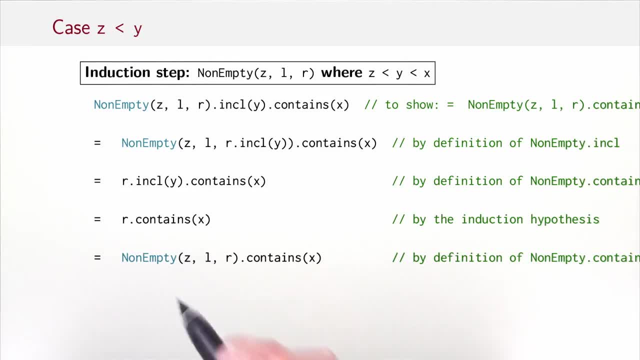 then we see that we again have equality, because that's how this contains is defined. on that node, x is greater than z. so we look in the right subtree. So we have established a four step equality between the left hand side of the law and the right hand side of the law. 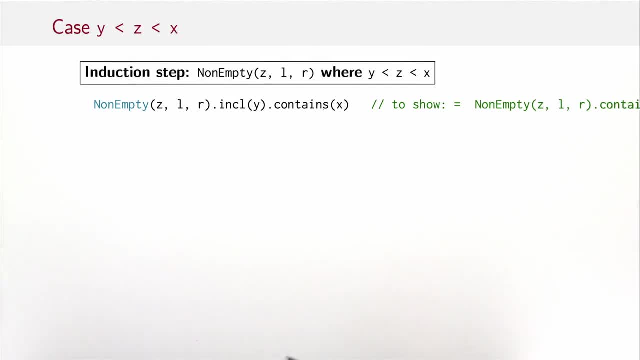 So the second case for the induction step to consider is where z is between y and x. We have the same left hand side as before and again we have to show that nonempty zlr contains x. So since y is now smaller than z, 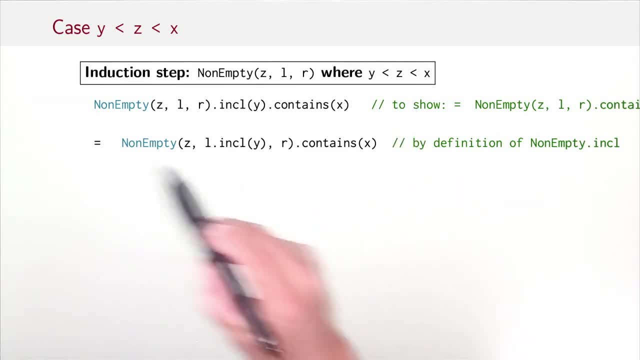 we include y in the left subtree and wrap the nonempty and we ask whether it contains x. So that's the same as right contains x because x is greater than z And that's the same as nonempty. zlr contains x by the definition of contains. 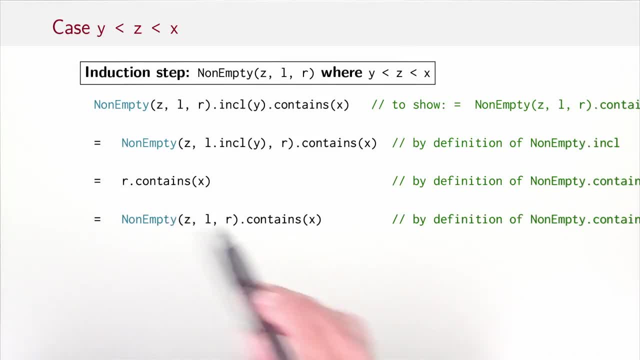 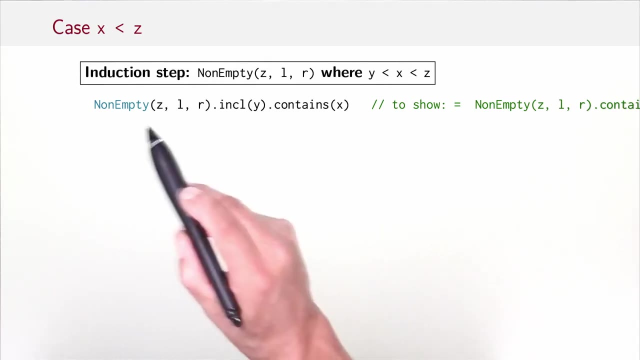 Since x is greater than z, we search in the right subtree, so this expands to that term over here. And the third step is the case where z is now greater than both y and x. So we have again the same left hand side and we need to prove again. 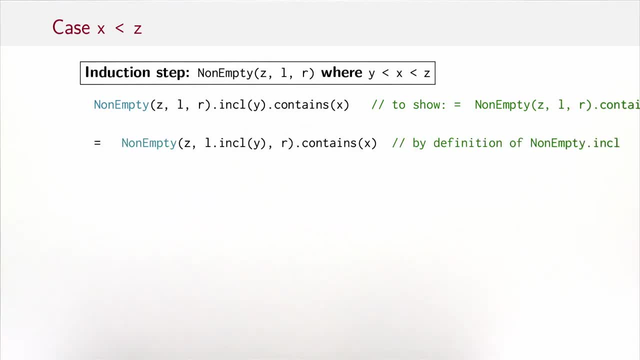 that nonempty zlr contains x in this case. If we do that, then we proceed as before in the first step. We know that include will expand to an inclusion of y in the left subtree. So we ask: contains x? and x is also less than z. 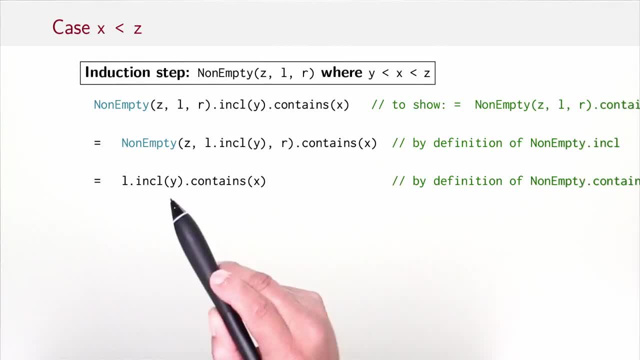 so to ask whether this set contains x, we look again in the left set so we have l include. y contains x. Now, by the induction hypothesis, that's the same as l contains x. And again, by the definition of nonempty, contains in reverse, that's the same as. 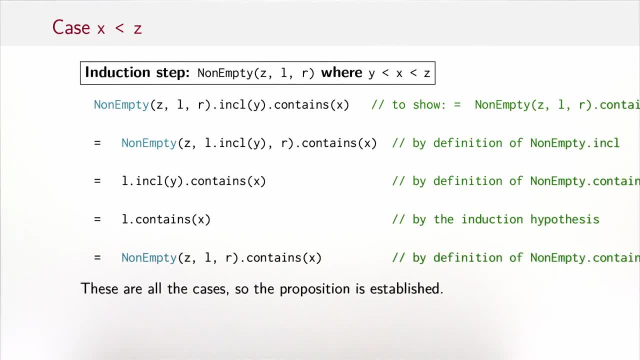 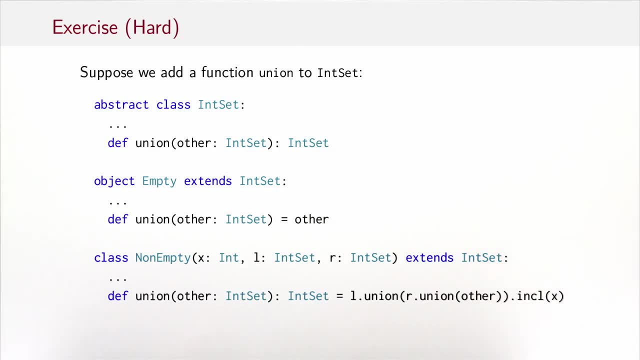 nonempty zlr contains x. These are all the cases, so the proposition is established. So if you want to explore this further, here is a harder optional exercise that you might consider. Let's suppose we add a function union to int set. We have seen it already. 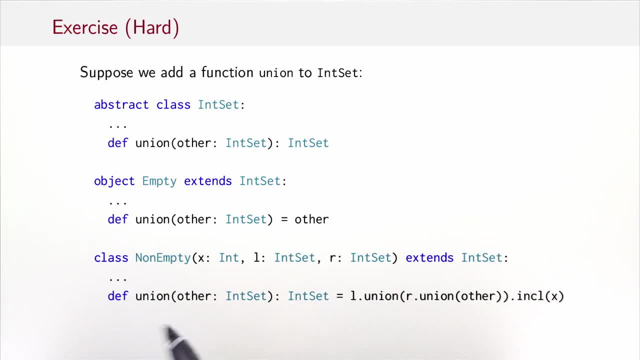 Here is a possible implementation of union. So for the nonempty set we say to take the union of a nonempty set with some other set, we take the left set union, right set union, the other set, and then we re-include x at the end. 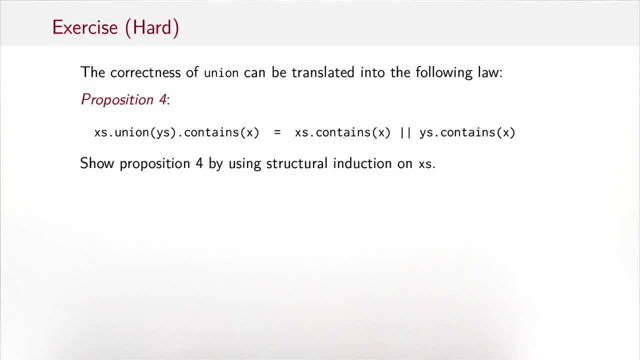 So what does it mean to say that this or any other implementation of union is correct? Well, we need to have a law for union, a way to relate it to the other operators that we have. There is one quite obvious law for union. it's this one here To say: well, 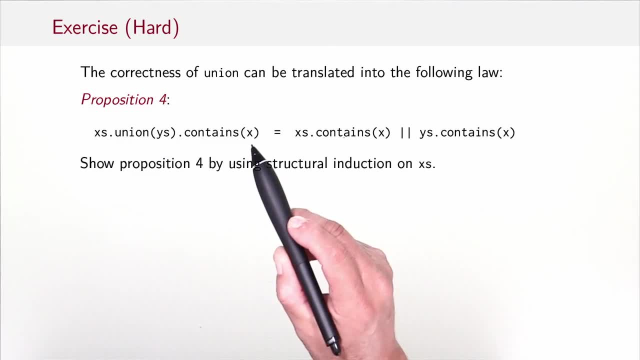 if we take the union of two sets and then ask whether that contains an element x, then that should be the same as asking whether the left operand contains x or the right operand contains x. So your task is to show this proposition by using structural induction on the set xs. 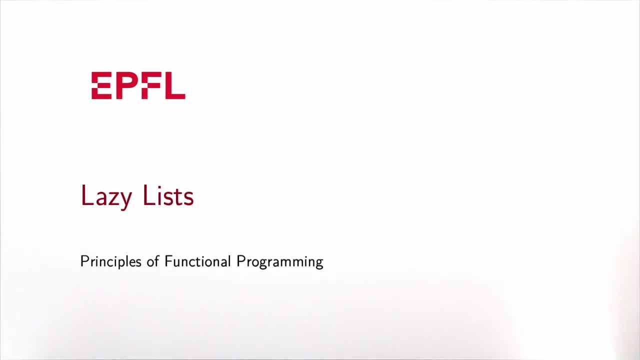 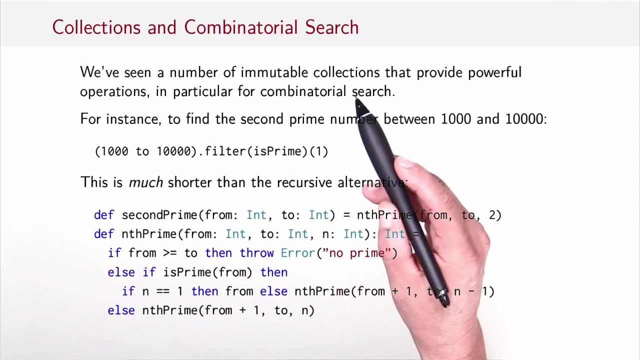 In this session and the next, we are dealing with laziness. Laziness means computing something as late as possible, Only computing it once it's first needed. We're starting with lazy lists, So for motivation, we've seen a number of immutable collections that provide 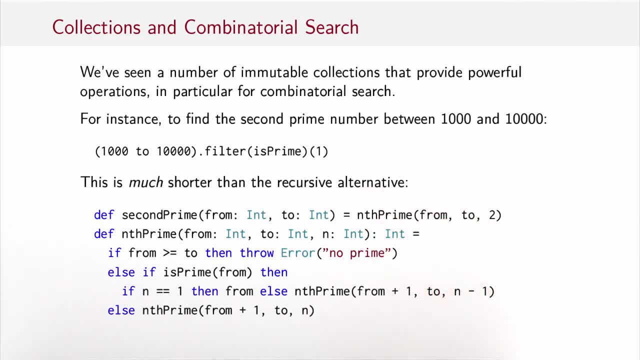 powerful operations, In particular for combinatorial search. For instance, to find the second prime number between thousand and ten thousand is really easy. You can write well, between thousand and ten thousand, filter with the is prime predicate and take the second number. So at index one. 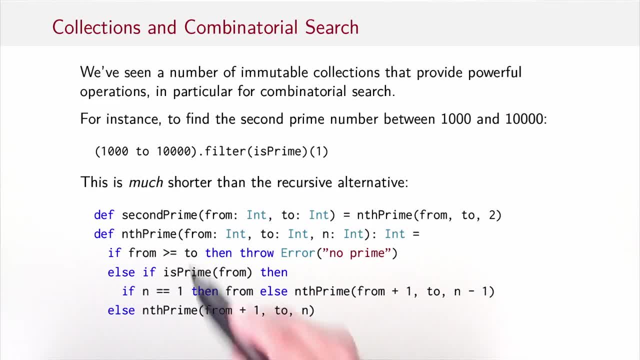 It's a lot more tedious to write this with a recursive function from scratch. So here you see a possible implementation. Second prime is implemented in terms of nth prime, and then, essentially, nth prime has this tedious thing with counters that essentially counts the number of primes that were found, and then 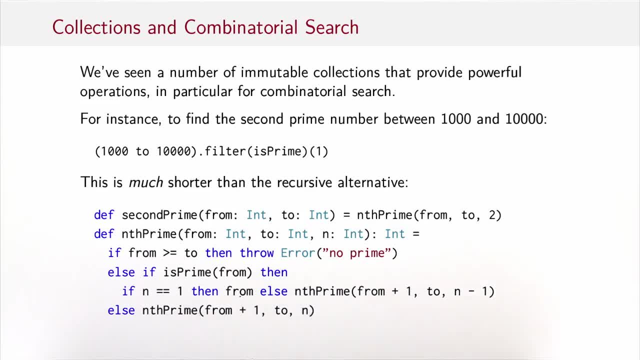 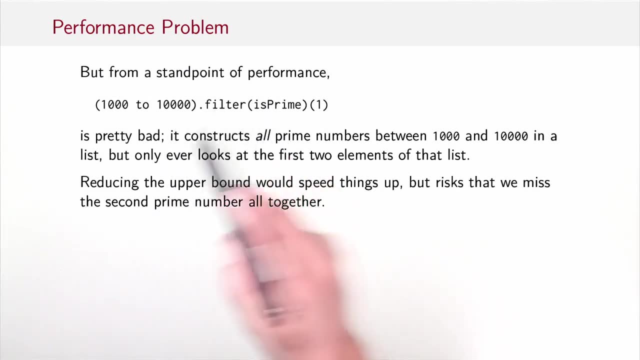 if it found the last prime that's necessary, it will return it, and otherwise it will go into the recursion one way or another. On the other hand, this more convoluted implementation is a lot faster than the one we wrote up here, Indeed from a standpoint of performance. 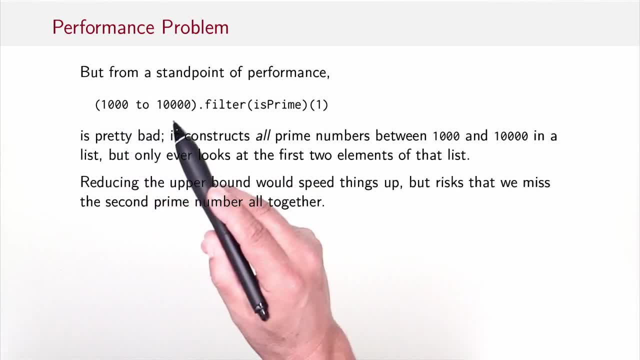 that expression is really bad. It constructs all prime numbers between thousand and ten thousand in a list but only ever looks at the first two elements of that list. The rest is thrown away. Of course we could reduce the upper bound. We know that the second prime number 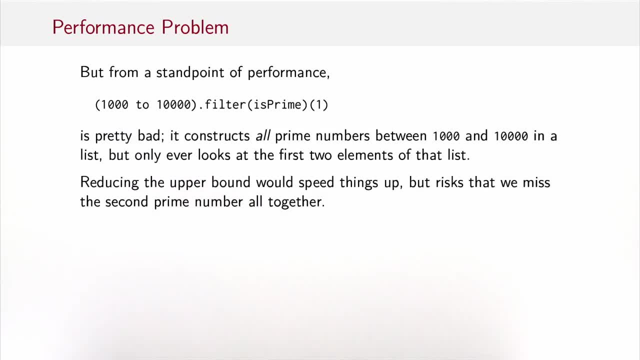 will be a lot closer to thousand than to ten thousand. but of course if we do that too much then we risk missing the second prime number altogether. So we have to put some knowledge in from the outside which we might not have. However, we can make the short code. 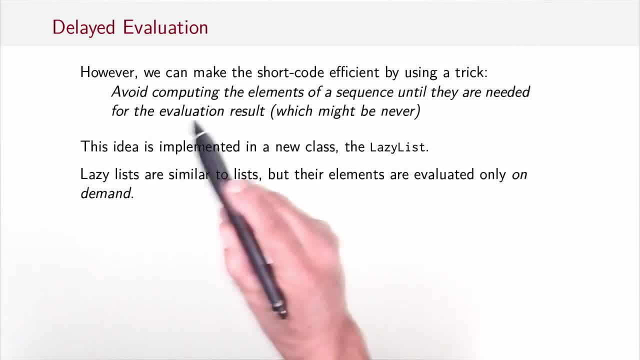 efficient by using a trick. The trick is that we want to avoid computing the elements of a sequence until they are needed for the evaluation result, which might be never. This idea is implemented in a new class in the Scala standard library, which is a lazy list. 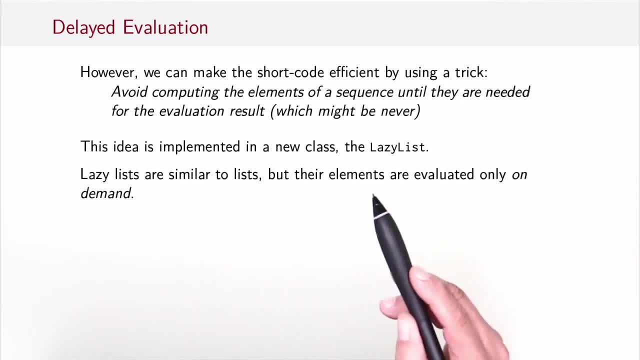 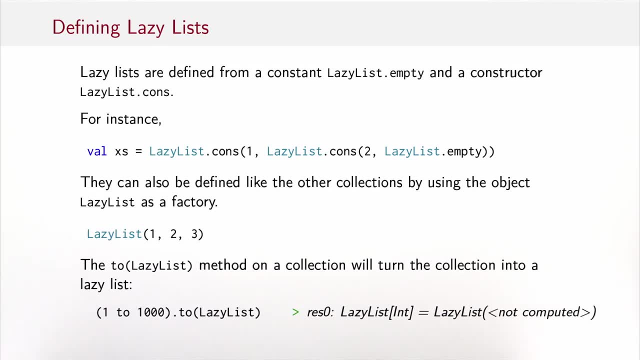 Lazy lists are similar to lists, but their elements are evaluated only on demand. So here is how you can work with lazy lists. They are defined from a constant lazy list dot empty, which is the analog of nil for strict lists, and a constructor lazy list dot. 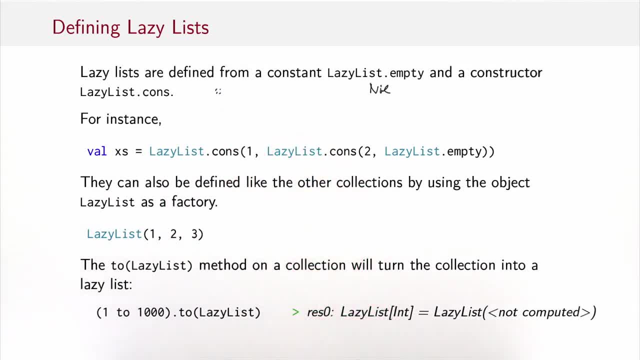 cons, which is the analog of colon, colon for strict lists. So, for instance, lazy list, dot cons one. lazy list, dot cons two. lazy list, dot empty is the lazy list one, followed by two, followed by empty. In what sense is it lazy? Well, it's lazy in the sense that a sub 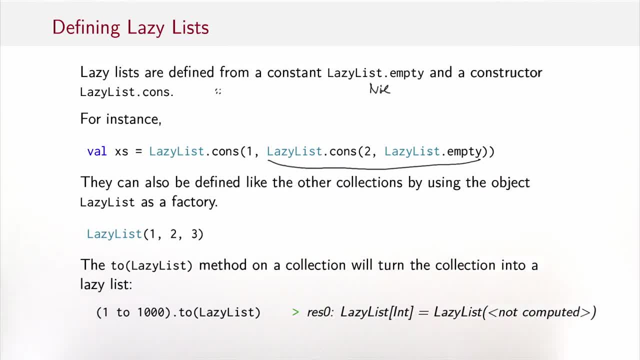 expression like this one here will be evaluated only when we need the second element of the lazy list. Lazy lists can be defined, just as the other collections, by using the object lazy list as a factory. So you can write lazy list one, two, three. that translates to lazy list dot. 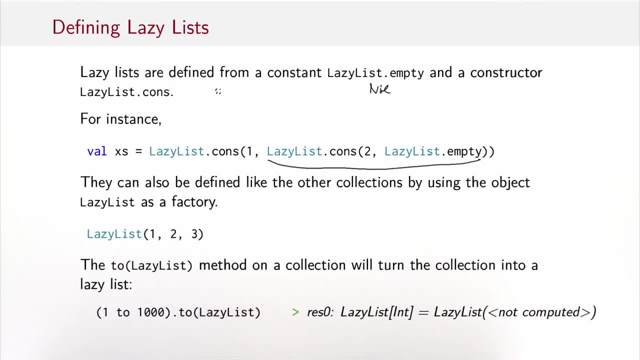 apply one, two, three and indeed the lazy list object has a suitable apply method that will convert these arguments to lazy lists. Another way to get lazy lists is by converting some other collections to lazy lists. You can do that with the to method, which is available on most collections. 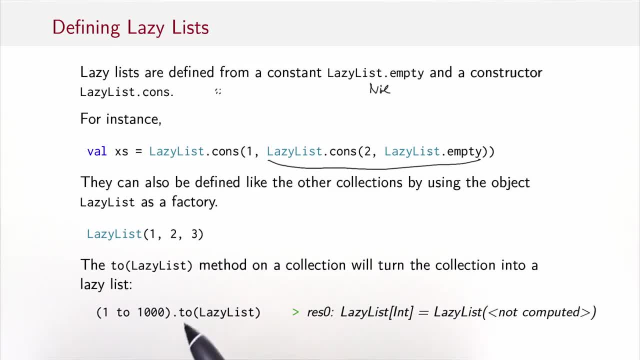 in the Scala library. So you write one, two thousand, dot two and then lazy list and that will turn this range one, two thousand into a lazy list. So two is another utility method defined on Scala collections. It essentially takes a object which is a factory. 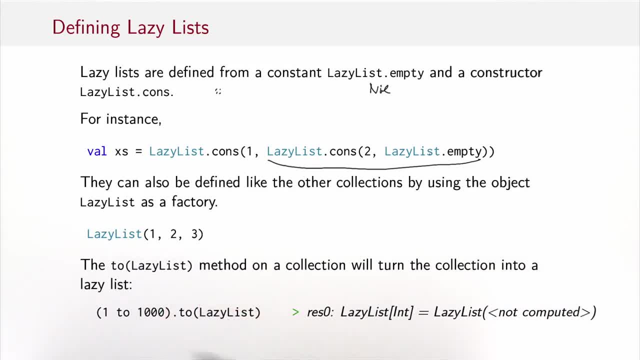 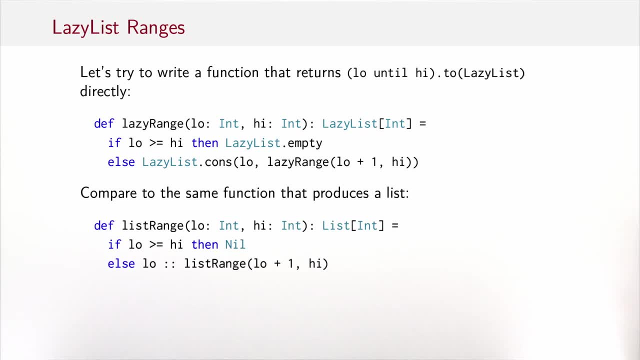 and calls the apply method on that object, on the elements that are to the left of the two. We can use some of these elements to define further methods that construct lazy lists, For instance lazy range here. So lazy range would be construct a lazy list of the numbers. 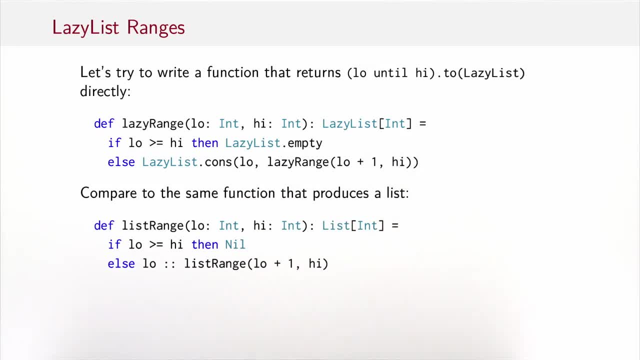 between low up to high. It's a lazy list of int and it's simply defined as you see here. If low is greater or equal high, then it's the empty lazy list. Otherwise it's the cons lazy list, with the first element being low and the rest 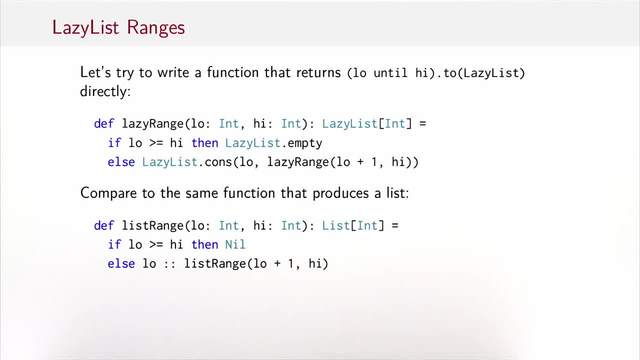 being the result of lazy range of low plus one and high. If you compare to the same function that produces a list, which you see here, then you see that the two functions are very, very similar. The only differences are that we use lazy list dot empty instead of nil. 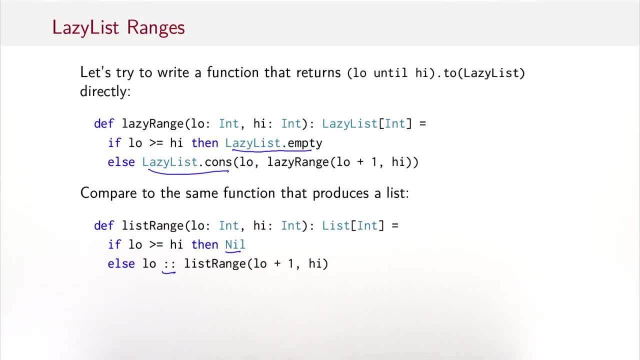 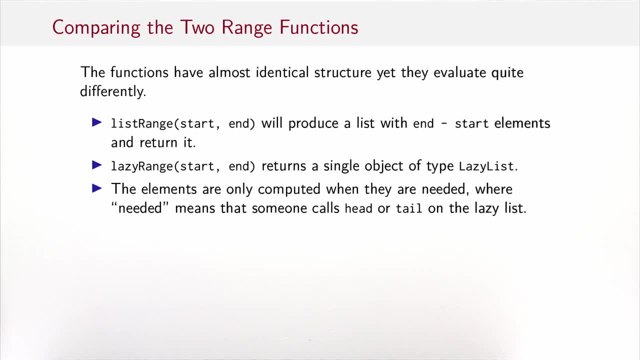 and lazy list of cons. instead of colon, colon. otherwise it's exactly the same. So the two functions have almost identical structure, Yet they're evaluated quite differently. List range- start, end will produce a list with end minus start elements and return it immediately Lazy range. 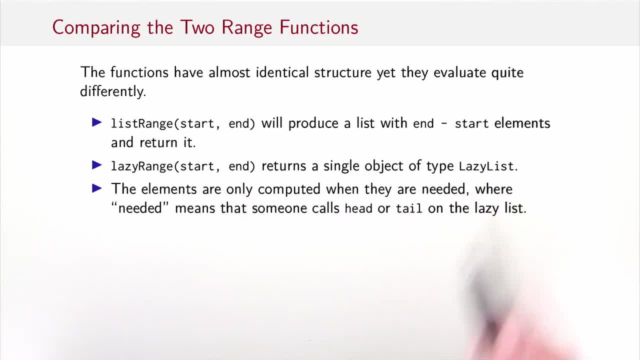 start end will return a single object of type lazy list. The elements are only computed when they're needed. where needed means that somebody calls head or tail on the lazy list or is empty, I should say. Until that time, the lazy list object is not evaluated. We don't know yet. 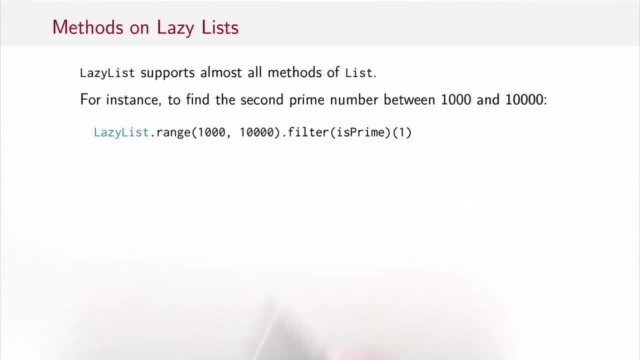 what's in it. So lazy list supports almost all methods of lists, including filter. so for instance, to find the second prime number between thousand and ten thousand, we can now write lazy list dot range: thousand, ten thousand and filter is prime element at index one, The one major exception. 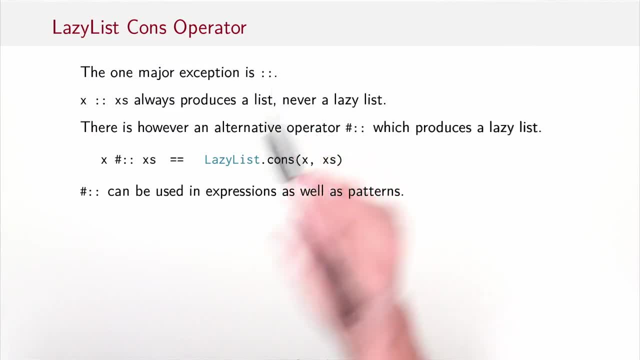 where the operations are different, is cons, So x. cons xs always produces a list, never a lazy list. There is, however, an alternative operator, hash cons, which produces a lazy list. So x. hash cons xs is the same thing as lazy list dot cons xxs, and what it does is: 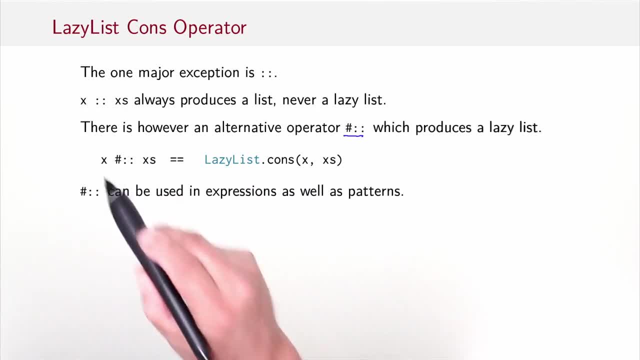 it produces a lazy list consisting of x as the first element, xs as the rest, and it does so lazily. That means the whole thing will be evaluated only when somebody needs to access an element of that list. Like cons, hash cons can be used in expressions. 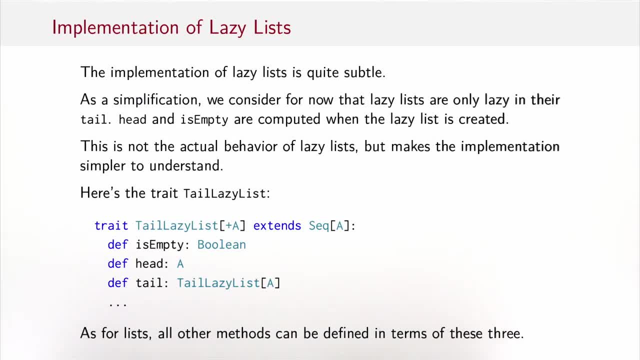 as well as in patterns. This idea of laziness looks a bit magic at the beginning and indeed the actual implementation of lazy lists is quite subtle. As a simplification to approach the subject, we consider for now that lazy lists are only lazy in their tail. 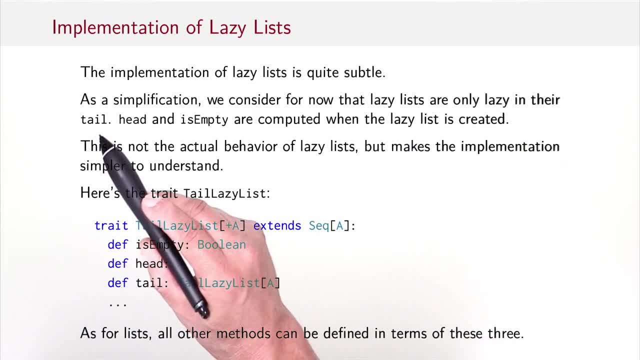 That means the tail of a lazy list is computed when the first time somebody needs it, but the head and the is empty predicate of a lazy list are already set when the lazy list is created. That's not the actual behavior of lazy lists, but it makes the implementation. 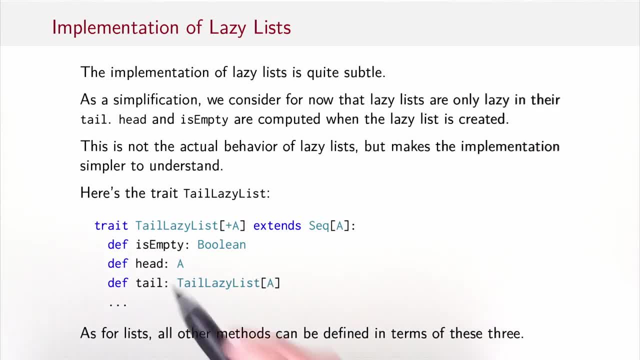 simpler to understand. So let's call this simplified lazy list tail lazy list because it's only lazy in the tail. So here's the basic trait. A tail lazy list should be a subtype of sequence. It has an is empty method and a head and tail method. 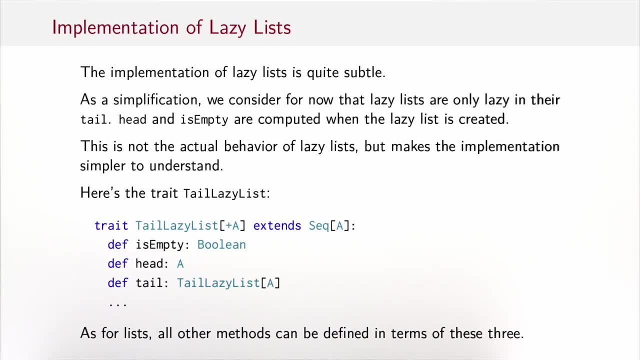 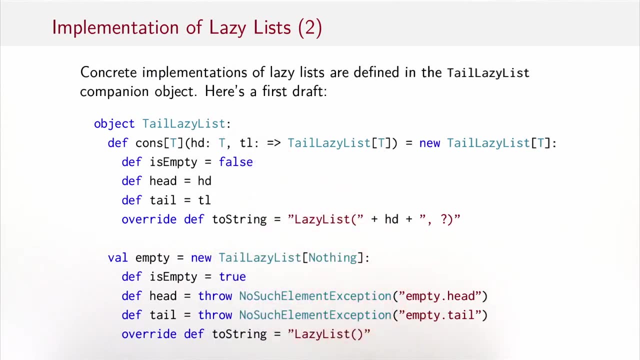 So the same fundamental operations as a normal list. As for normal lists, all other methods can be defined in terms of these three fundamental operations. So now to finish the implementation, we just have to give concrete implementations of empty and non-empty lazy lists that define these three methods. 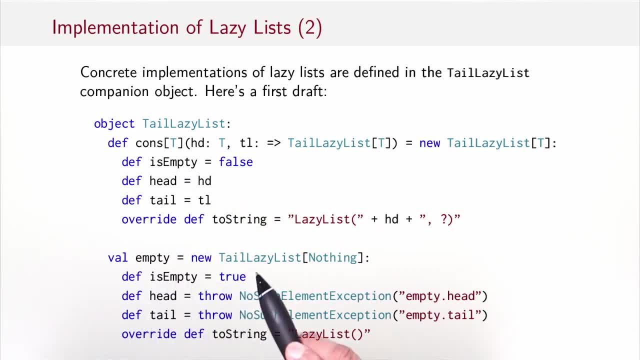 Here's the empty lazy list. So it's a tail lazy list of nothing Is empty, is true Head and tail. throw an exception. And there's also a toString method so that we can print these things nicely, which just says it's lazy list empty. 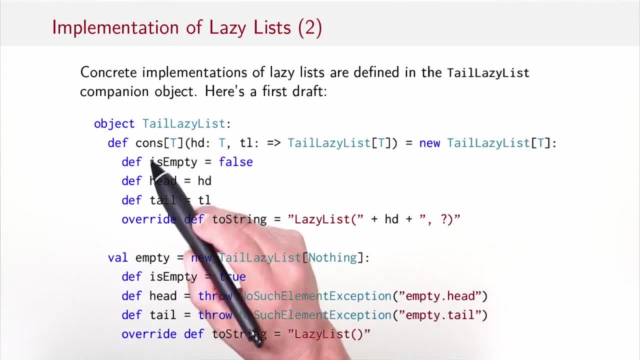 What about cons? So the main difference between cons and the list cons we have seen is this: The tail function now is a by name parameter, So it takes a head, which is a normal by value parameter, and a tail, which is a by name parameter of. 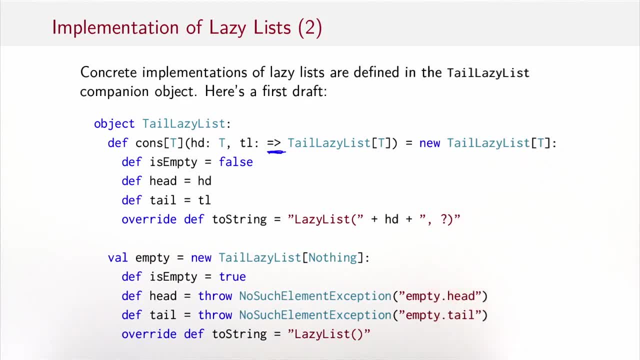 a lazy list of t And it returns a new lazy list of t where isEmpty is false. the head is the head, the tail is the tail argument here, and toString is lazy list, head and then comma. and then we just put a question mark in here in order not to force the lazy list. 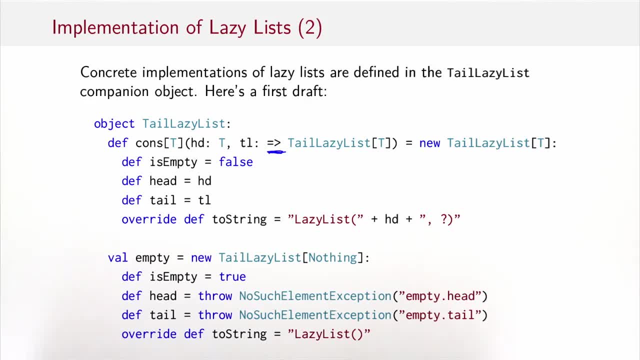 So we say, converting the lazy list to a string. we don't really want to find out what the elements are. by forcing the elements, we just print what we know And in this case, because the head is a by value parameter, we know what the head is. 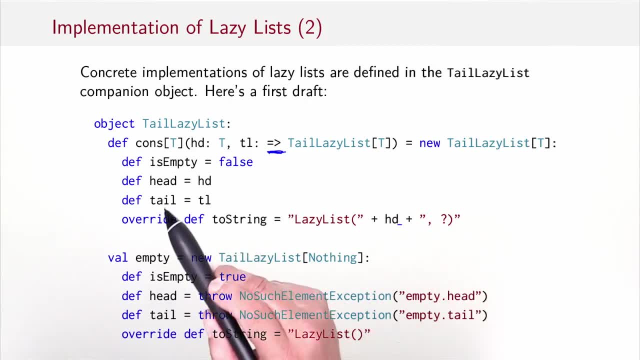 but we don't know what the tail is without calling tail. When we call tail, then it would call this by name parameter and that would in effect evaluate the expression that computes the tail of that lazy list. So the only difference between lists and lazy lists is really this: 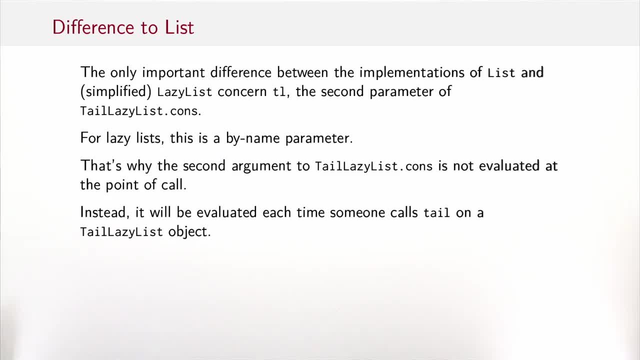 it's just the arrow in front of tail. So to reiterate: for lazy lists, tail is a by name parameter. for normal lists, it's a by value parameter. and that's why the second argument of tail-lazy-listcons is not evaluated at the point of call. 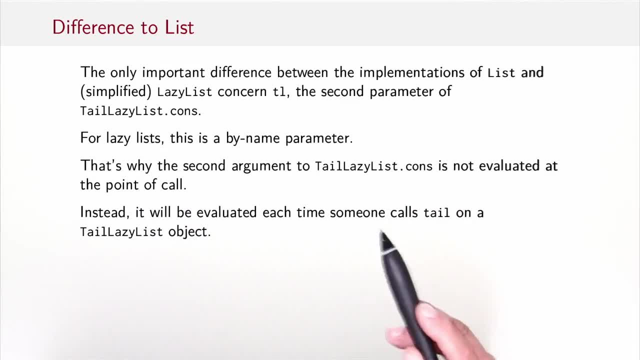 Instead, it will be evaluated each time someone calls tail on a lazy list object. You could argue: well, that's actually pretty bad because if tail could be called multiple times, which would lead to multiple evaluations of this by name parameter- and that's a correct objection and we will address that. 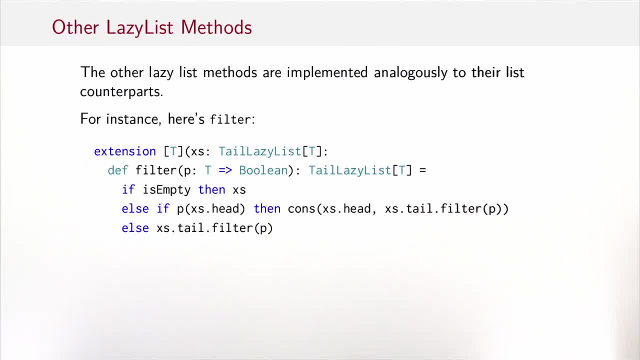 in the next session. Once we have defined lazy lists or tail-lazy lists like that, we can define other lazy list methods, just like the methods for lists. So, for instance, here's the implementation of filter on a tail-lazy list. it's really exactly the same. 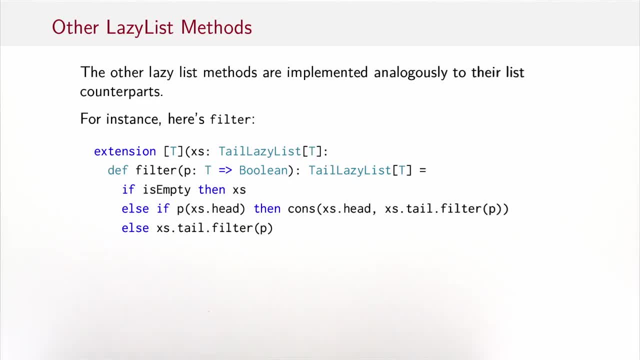 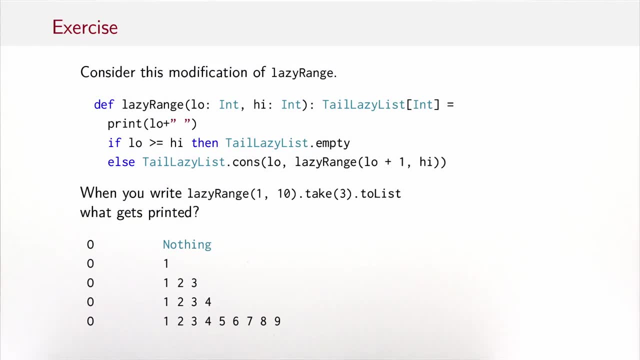 as we would define. filter on a normal list, if we wanted to base it on the three fundamental operations, is empty head and tail. So as an exercise for you, here's a slight instrumentation of lazy range. so it's what we had before, but each time we go into 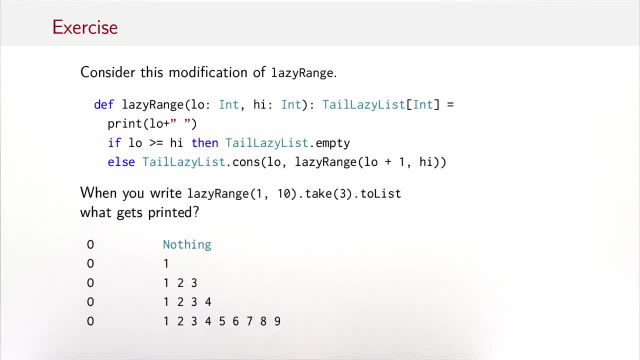 the body of lazy range, we print the current value of low. When you write lazy range: one, ten, take three, two, list what gets printed: Nothing. one one, two, three. one two, three, four or up to nine. 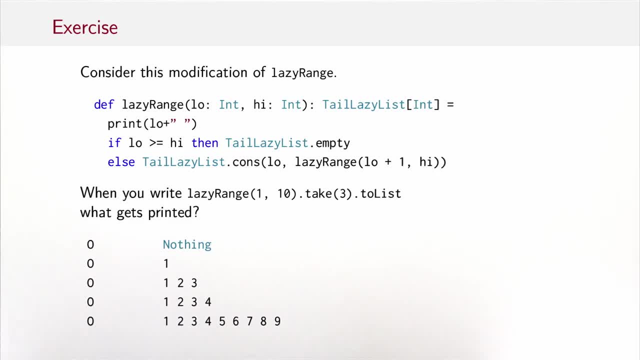 Ok, so let's see for a solution. If I just write lazy range one ten, what would be printed? Well, I would expand it to the right hand side, which would print one, and then, depending on the two branches, would in each case return. 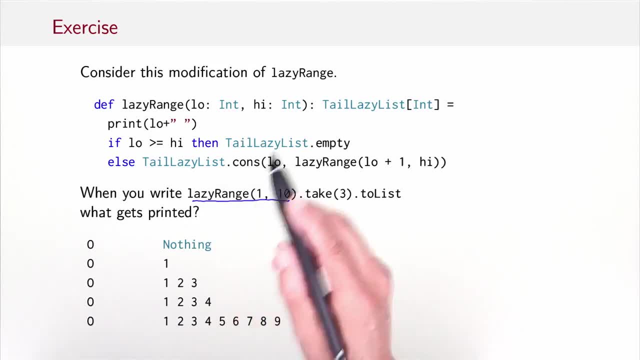 a lazy list, which means that nothing further needs to be printed because that expression is not executed. So, lazy range one, ten just prints one. What is lazy range one, ten. take three: Well, we don't have an implementation of take three. 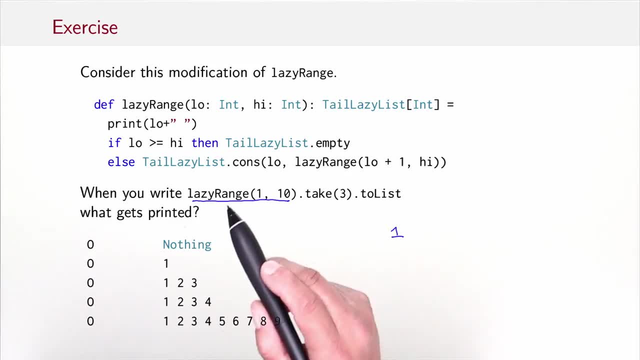 here. but essentially you can imagine that it takes the head of the list, it takes the head of the tail of the list and it takes the head of the tail of the tail of the list. That's the three elements it takes. So if it takes the 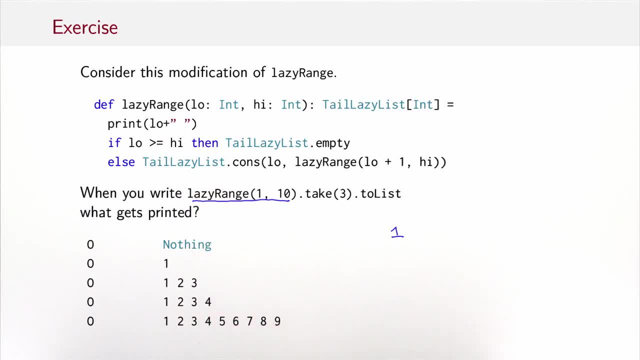 head of the list. nothing further is printed because the head is already evaluated. We already have the one. If it takes the head of the tail of the list, now we go into tail once. so we go into this recursive instance again, so we print the second. 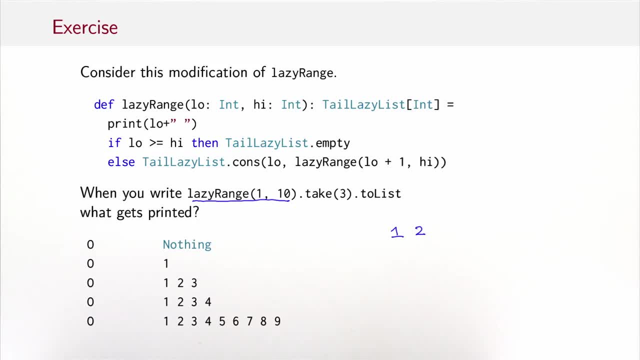 element two, And if we take the head of the tail of the tail of the list, we print the third element three And that's it. So that's all we need for take three. So if we convert it to a list, then of course we get the list. 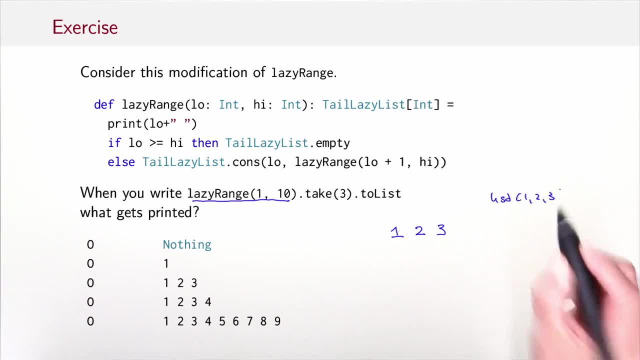 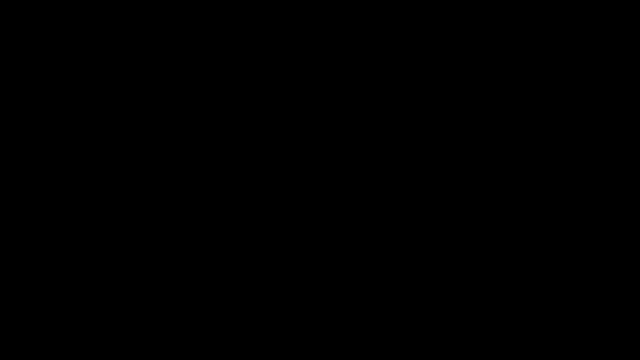 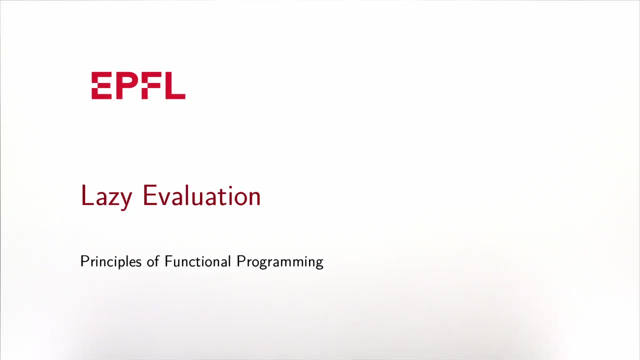 one, two, three. But before we get that, we print the elements one, two, three And not more than them. In this session we'll introduce the concept of lazy evaluation, which is some language, support and runtime constructs to make lazy computations more efficient. 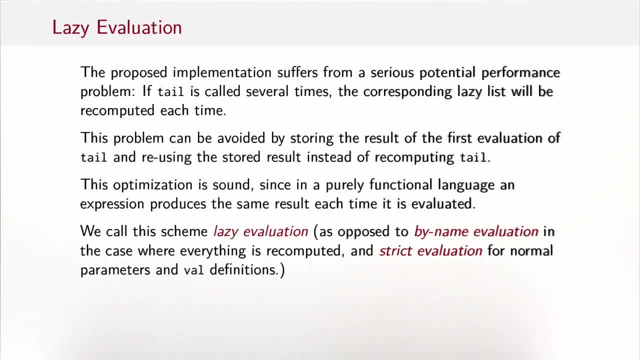 So we've seen that the previous implementation of tail lazy list suffers from a serious potential performance problem. If tail is called several times, the corresponding lazy list will be recomputed each time. This problem can be avoided if we store the result of the first evaluation of tail. 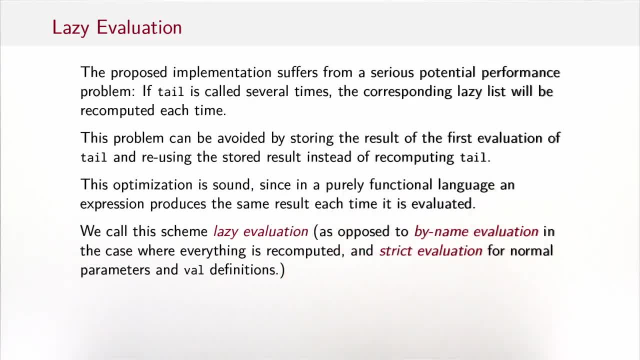 and reuse the stored result instead of recomputing tail another time. In a purely functional language, this optimization is sound, since the tail expression will produce the same result each time it is evaluated, So that means there's no need to actually do the evaluation several times since. 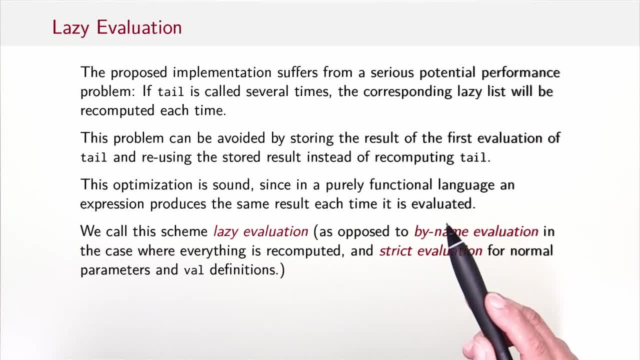 we know that every value will be the same. We can just use the first value that we have computed. We call this scheme lazy evaluation, and that's opposed to the by name evaluation in the case where everything is recomputed, and strict evaluation or for parameter. 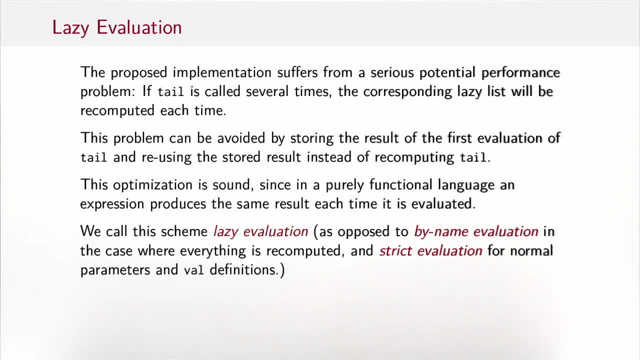 by value evaluation for normal parameters and value definitions. So by default Scala is strict by value. It has by name parameters that evaluate each time they are called, and we now also want to have lazy evaluation where we say we evaluate zero times or once, but not multiple. 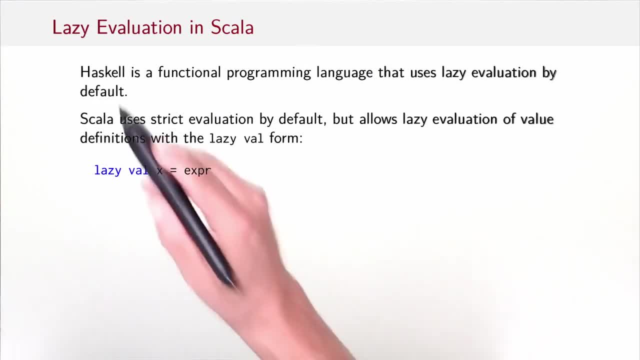 times. Some functional languages, including Haskell, use lazy evaluation by default. Scala, on the other hand, uses strict evaluation by default, but it still allows lazy evaluation of value definitions with a lazy val form, So you can write a lazy in front of a val and then the 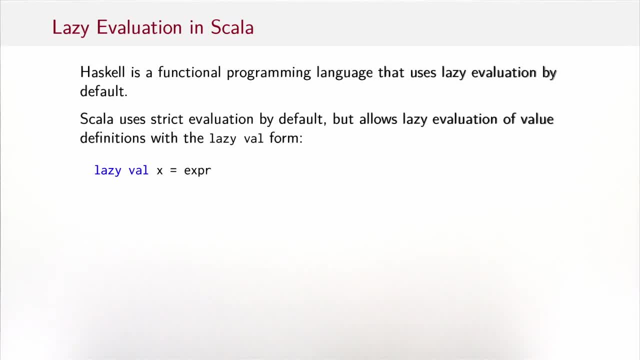 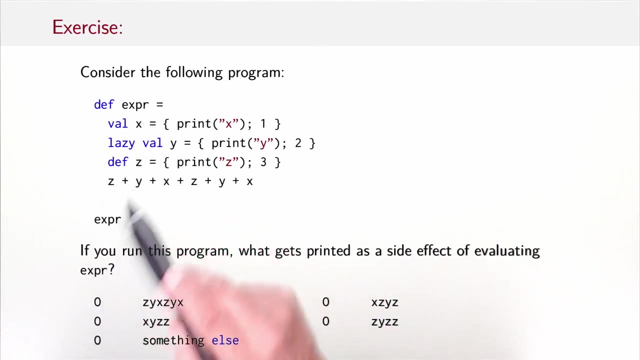 value definition is as usual, and what that means is that the right hand side of the val definition will be evaluated the first time x is used instead of immediately. So, as an example, let's consider the following program that you see here. So I have def x. 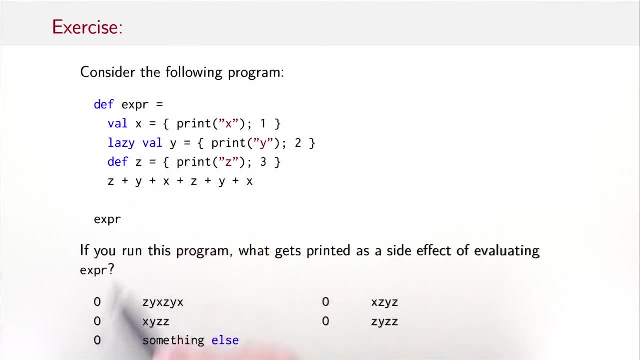 and then a val, and then a lazy val, and then a def, and then I sum them all up like this and for each definition I actually print what gets evaluated on the right hand side, If you run this program, what gets printed as a side effect of evaluating. 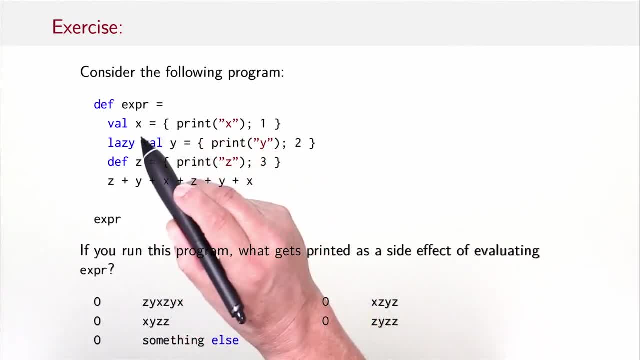 expr. So when I evaluate expr I have a strict value, definition x. so I evaluate its right hand side immediately, which gives me an x. So x is the first thing that is printed. The lazy val will not yet be printed because it's lazy. The 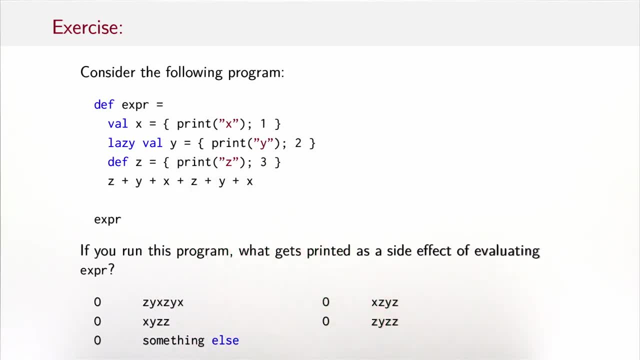 right hand side of the def will not yet be printed because it's a def. So then we look at the expression here. so now we call z and that prints z. so we have an x followed by a z. Now we evaluate y, so that would print y. 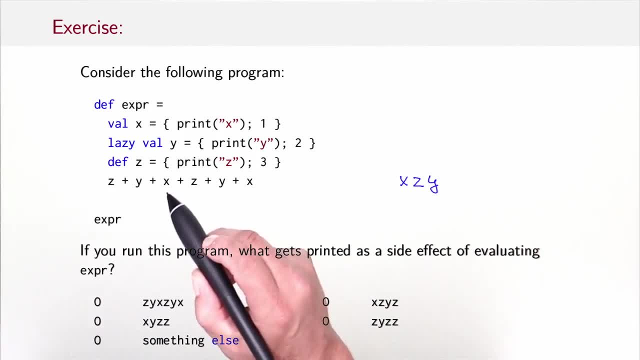 Now we want the value of x. that's already evaluated, so nothing gets printed. Now we want the value of z again, so that will re-evaluate the right hand side. That will print another z. Now we want the value of y again, In this case. 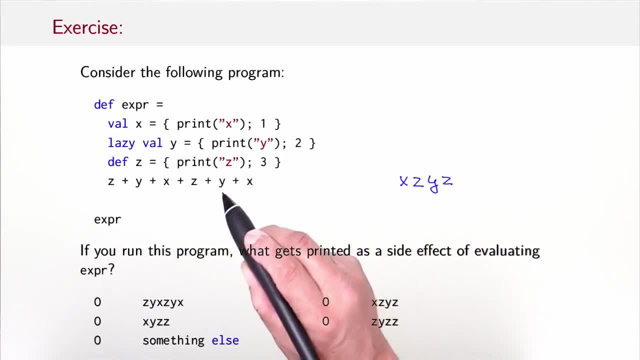 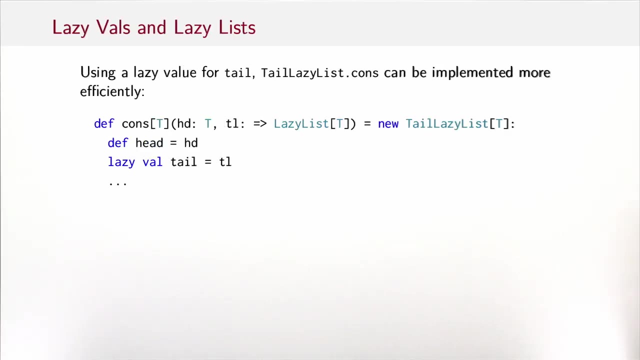 because y is lazy, it is already evaluated, It was already evaluated once, so nothing gets printed. And finally we want the value of x again, which of course is evaluated. so again that's what we get on the right hand side: xz, yz, So lazy. 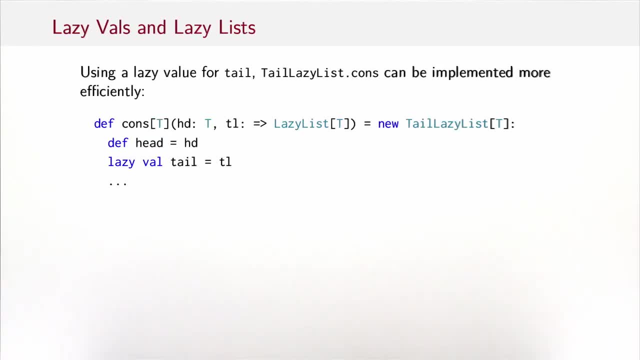 val's allow us to overcome our performance problems for lazy lists. So tail, lazy list dot cons can now be implemented. like you see here, Instead of a def tail equals tail, we have a lazy val tail equals tail. That's all that's needed, really that. 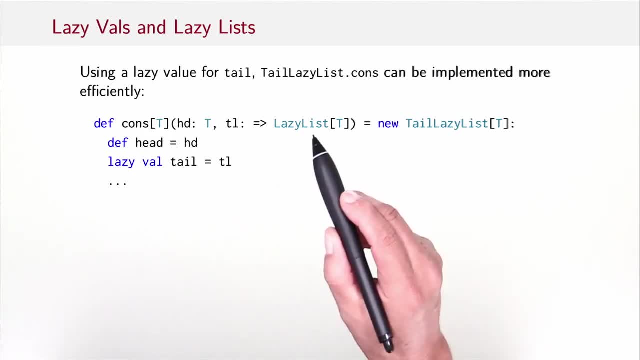 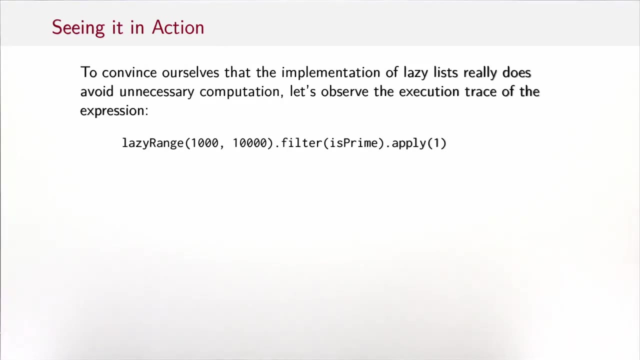 means that the first time somebody calls tail we will evaluate the call by name, parameter tl. but the next time somebody wants tail we have the value already stored here. so further evaluations of tail are avoided. So this laziness business might look a little bit like wizardry to. 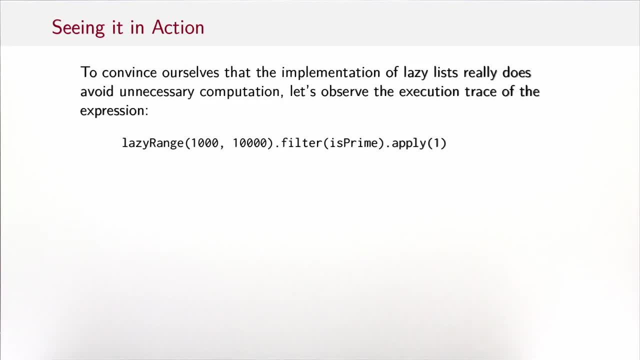 you in the sense that it's pretty smart at avoiding computations. To see it in action, we can just essentially use our basic substitution model and verify step by step that indeed laziness does what it promises. So let's start with the original expression that we have Lazy range. 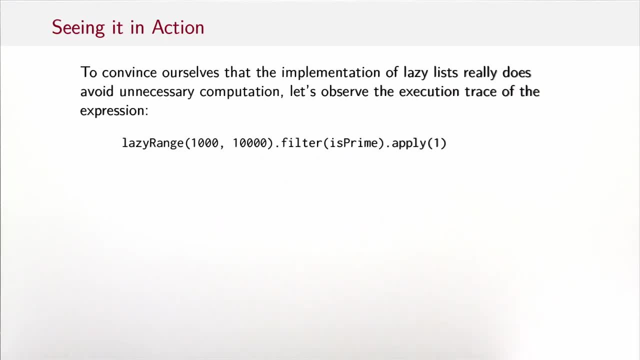 1000-10000 filter is prime apply 1. We want to reduce that from first principles using our standard rewrite rules and then verify how much of the list 1000-10000 actually gets constructed. So we first expand lazy range that. 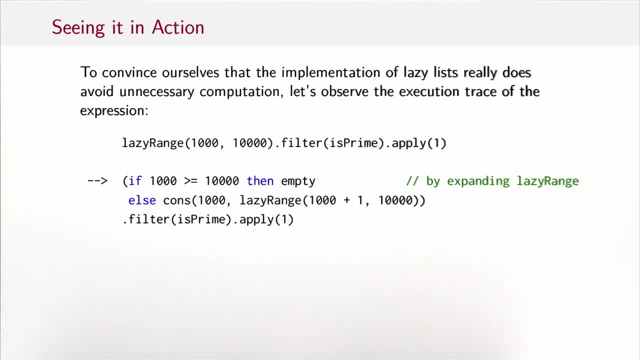 gives us this expression here with the parameter substituted, and then we plug that into the rest of the expression that you see here. Now we simplify the if, then else, so that reduces to the else part which you see here. So one thing that's important here is that this expression 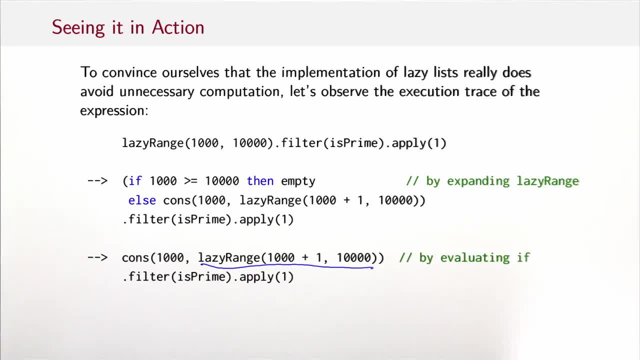 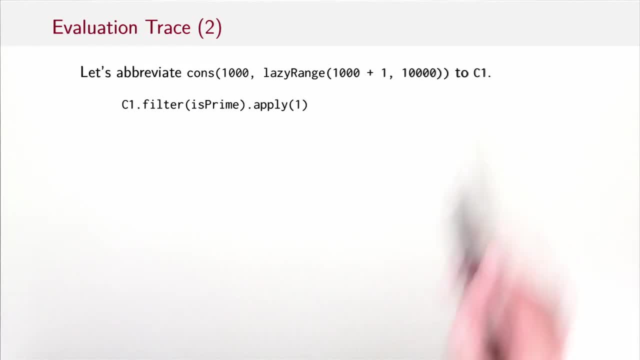 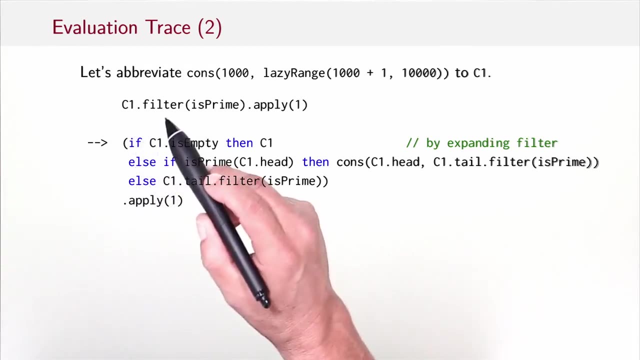 here hasn't been reduced yet. It's left as it is because it is a call by name parameter to const. Let's abbreviate this expression to just C1.. So we have C1.filter is prime apply 1.. So we now expand filter. 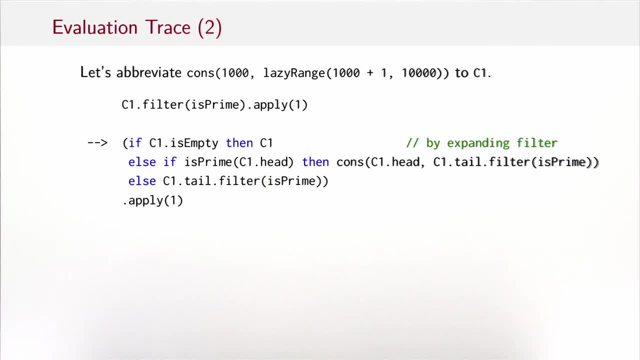 on the C1 value, which gives us here the right hand side of filter with the is prime method at the right place here. So if you simplify that, then we know that C1 is not empty. so it's going to be this one here if is prime C1.head. 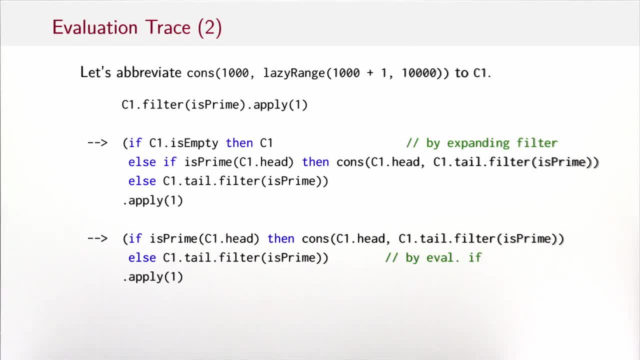 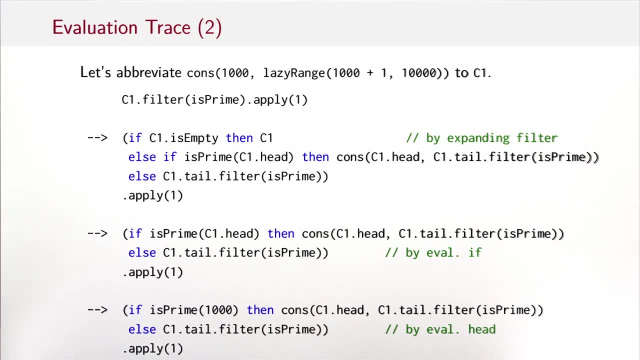 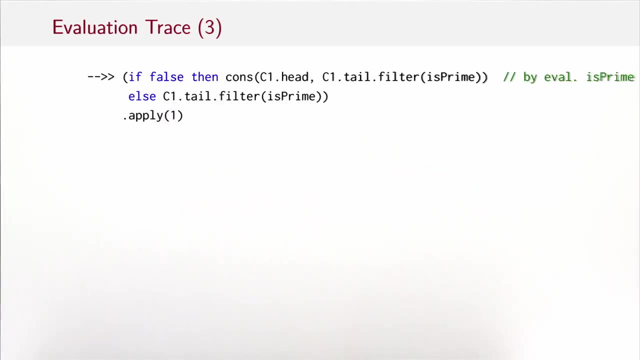 then this const expression, otherwise C1.tail filter. Now we evaluate C1.head, so that gives is prime 1000 and if we follow the computation of is prime, we will see that this reduces to false. So we are left with this expression here. 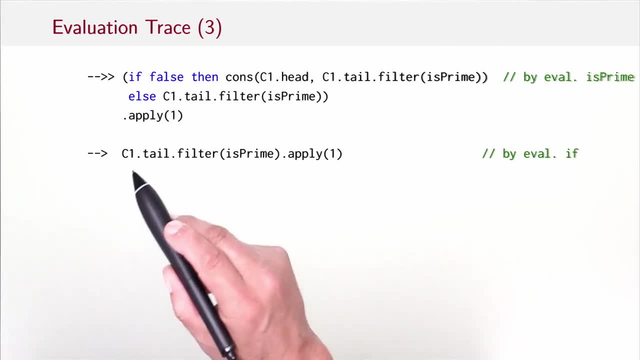 Now we can simplify the if, then else. so we are left with C1.tail filter is prime apply 1.. And now we go back to the actual argument of the C1 expression that corresponds to the tail. That was lazy range of 1000 plus 1, 10,000. 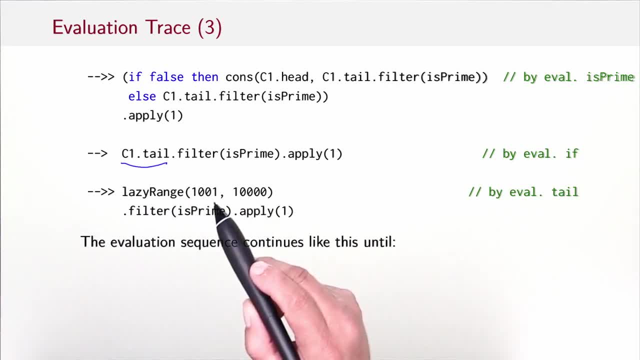 so at this point we compute that 1000 plus 1 is 1001 and we plug it into the expression here. So it's lazy range: 1001, 1000. filter is prime apply 1.. Which is basically what we started with, except that we have: 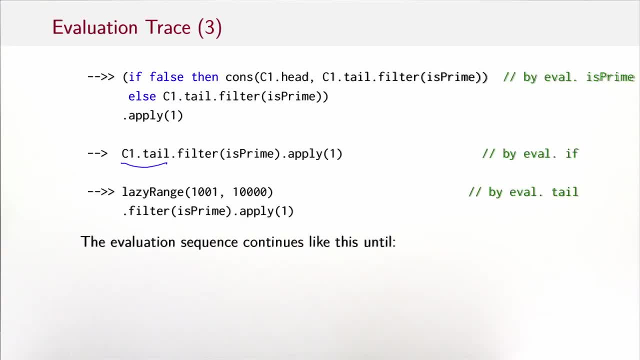 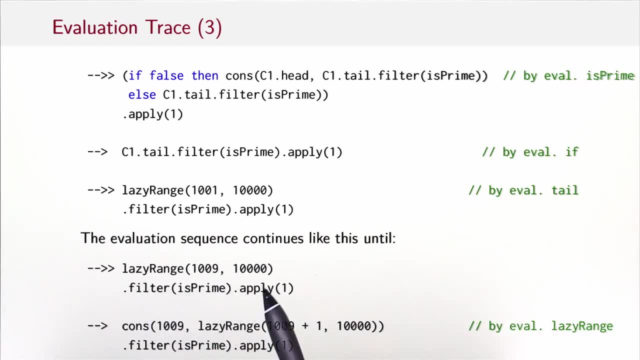 a 1 here now. And that evaluation sequence continues like this until we hit this situation here where we have lazy range 1009, 10,000 filter is prime apply 1.. And now by the evaluation of lazy range we get a const 1009 and 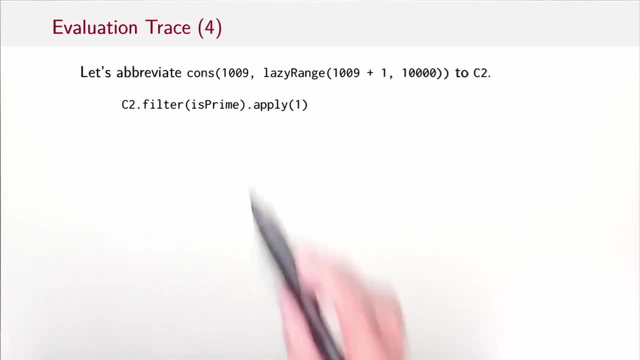 this expression here, Filter is prime. If we abbreviate that to C2 and we are left with C2, filter is prime, apply 1. Now, 1009 is a prime number. So we get the second case that we get, okay, our prime number. 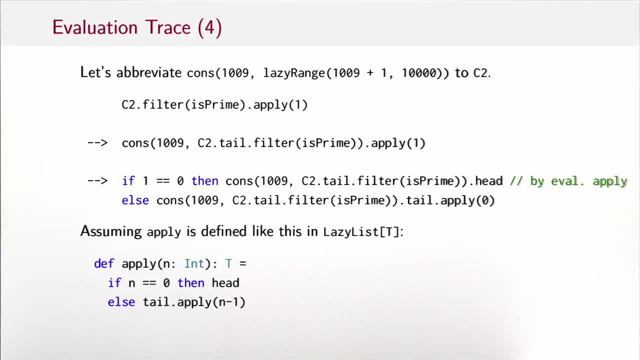 consists of a const followed by a tail, And now we have to finally evaluate the apply method. We get there. So let's assume apply is defined like this. So if n equals 0, then head is tail, apply n minus 1.. So what we would get here is: 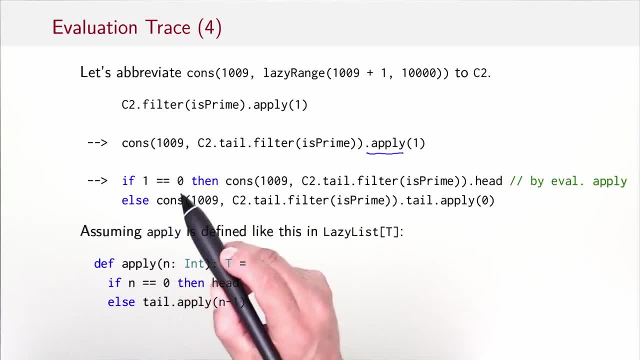 for the right hand side of the apply method, a 1 equals 0, because 1 is the index here. So that's false. So we continue with the cons in the else part that you see here, And that means now we have a call to tail. 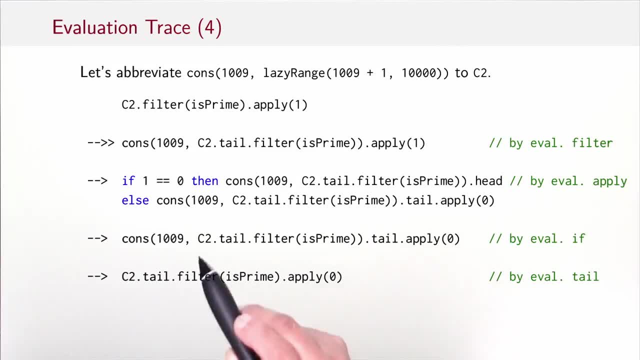 because that comes from the apply method. So we take essentially this tail of the cons which gives us C2 dot tail filter is prime, apply 0.. And that by computing what is the tail of C2 we get lazy range 1010, 10,000. filter is prime. 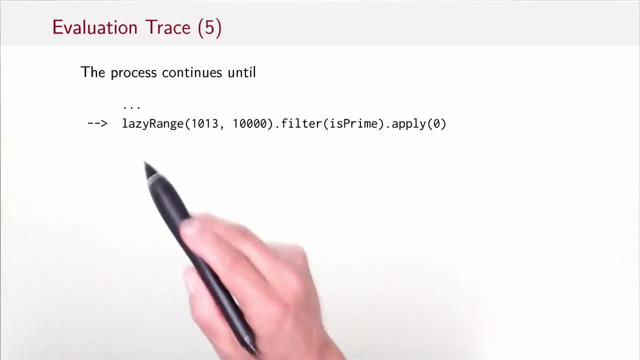 apply 0.. And that process continues until finally we have lazy range 1013,000. filter is prime: apply 0.. That then gives the cons expression as before, So it's cons 1013. lazy range of the rest: filter is prime: apply 0.. 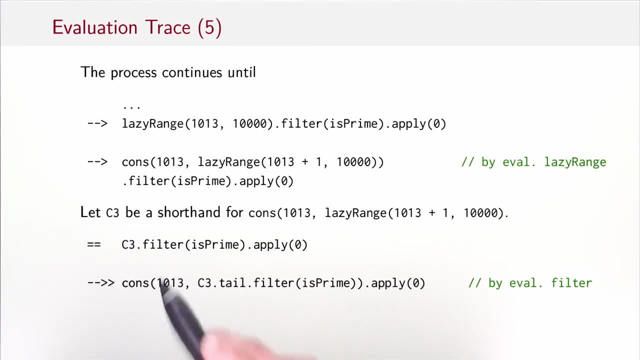 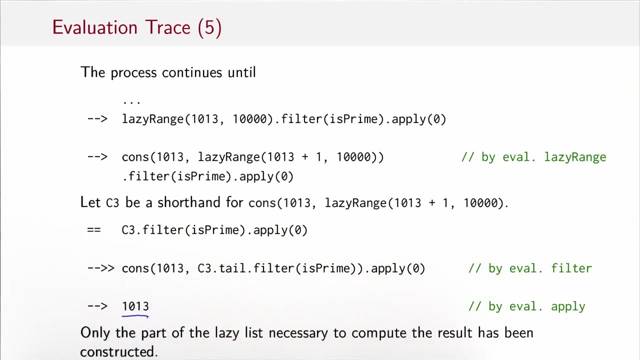 Let's call it C3.. If we filter that expression, we get cons 1013 and then this tail, because 1013 is in fact a prime, so the filter will include it as a first element, And that then is the final result. So if we look at our rewrite, 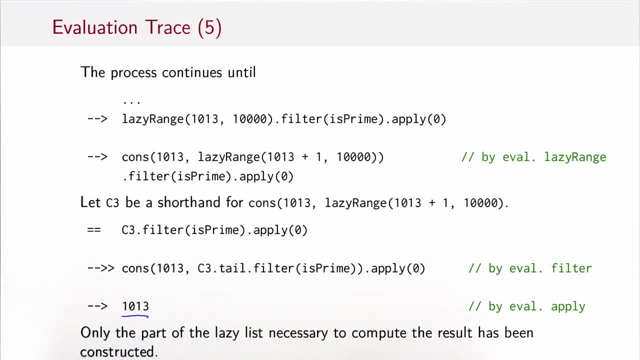 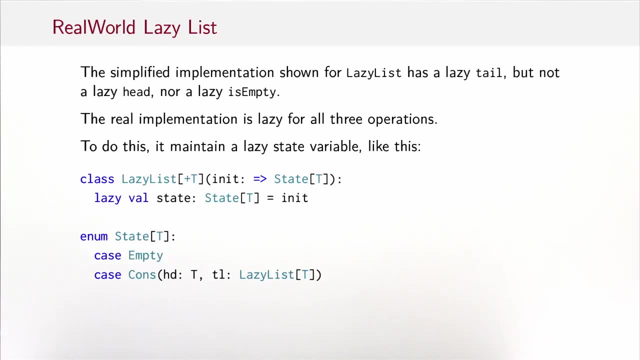 trace, then we will see that, indeed, we have never constructed a lazy list beyond the element 1013.. So we have computed exactly as many elements as we needed to verify that the second prime number following 1000 is 1013.. Good, So the simplified 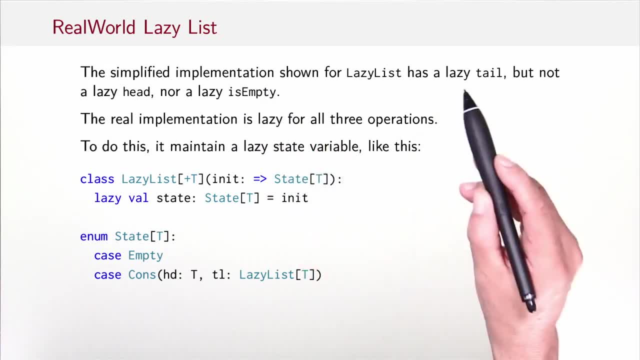 implementation of lazy list that we have worked with has a lazy tail, but not a lazy head, nor a lazy is empty. The real implementation of lazy list is lazy for all three operations. So lazy list is a lot lazier than tail lazy list To do this. 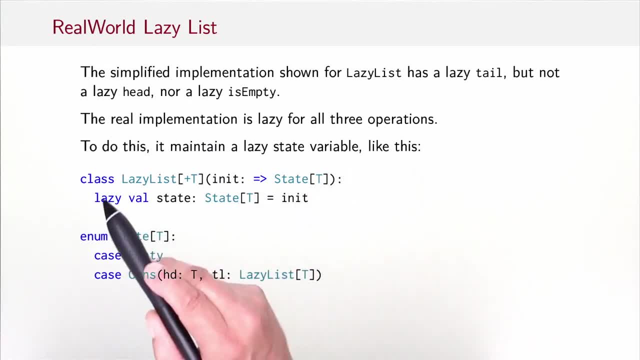 it maintains a lazy state variable, a bit like this. So there is a class lazy list in the standard library that has essentially an init parameter that computes the state of the lazy list, And the state of the lazy list is either that it is empty or that it is. 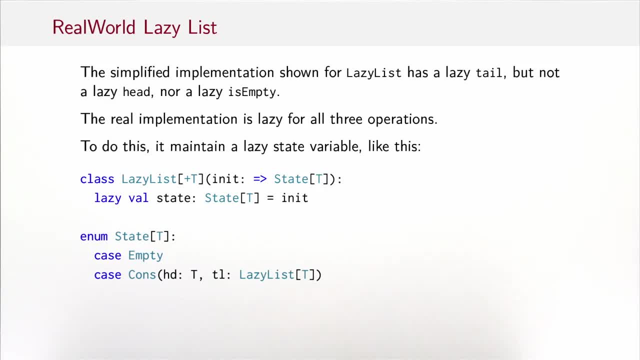 a cons of a head of type T and a tail, which is a lazy list, But that state so that the lazy list knows whether it is empty or a cons and what the head is. that is altogether computed lazily by this by name parameter. So that is the essential difference. 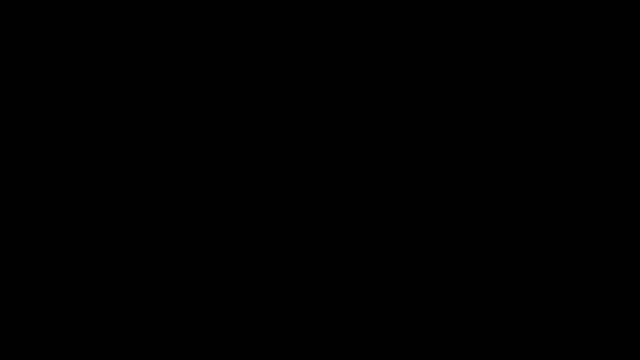 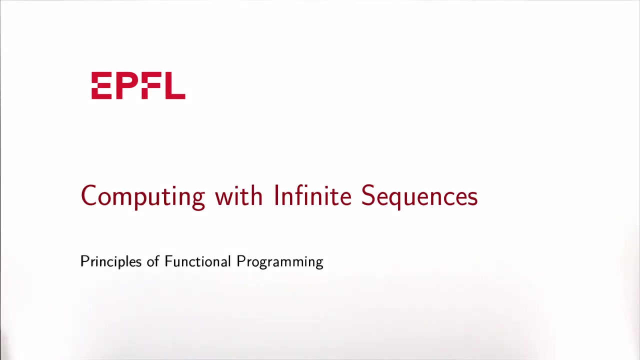 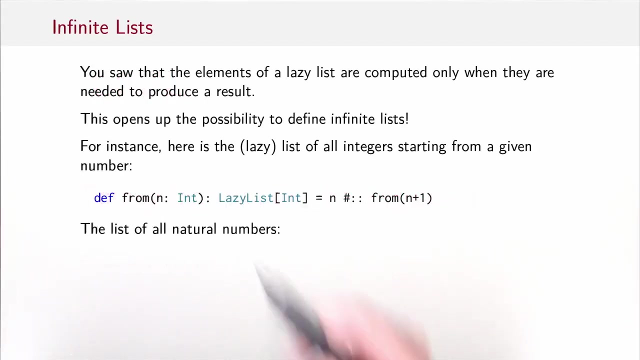 between the two. In this session we are looking at an interesting consequence of lazy computation, namely that we can compute with infinite sequences. You saw that the elements of a lazy list are computed only when they are needed to produce a result. That opens up the possibility. 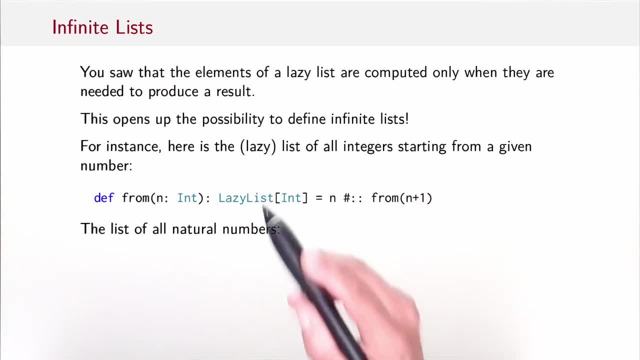 to define infinite lists. For instance, here is the lazy list of all integers starting from a given number, From n, int. It is a lazy list of int and it is defined to be n, followed by from n plus one, Or that is the list of all natural numbers. 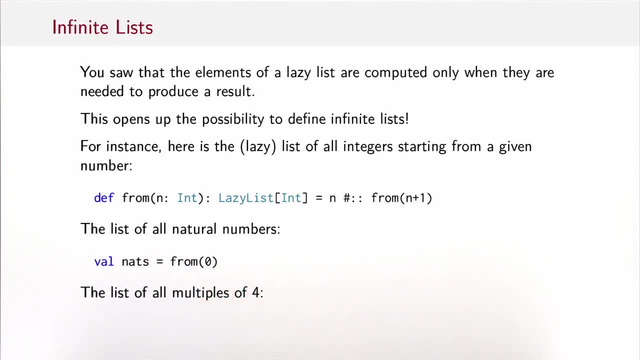 Well, nats equals from zero. Or to compute the list of all multiples of four, we can do: nats map times four. So why does this all work? Well, it works because when we create the lazy cons here, the expression here will actually not be evaluated. 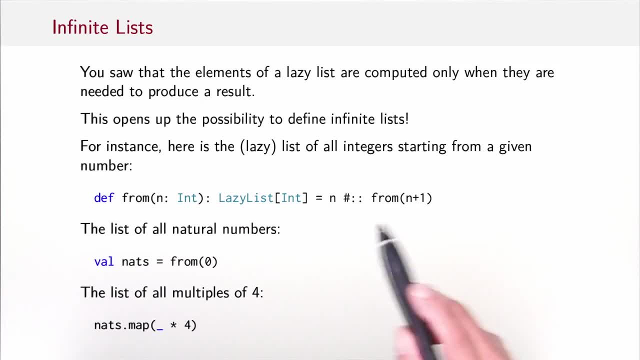 It will only be evaluated when we need the head of a tail of the resulting lazy list. So we can in complete confidence compute all natural numbers, because they will in fact be computed only once somebody asks for a particular natural number, And of course you can never ask for all of them at the same time. 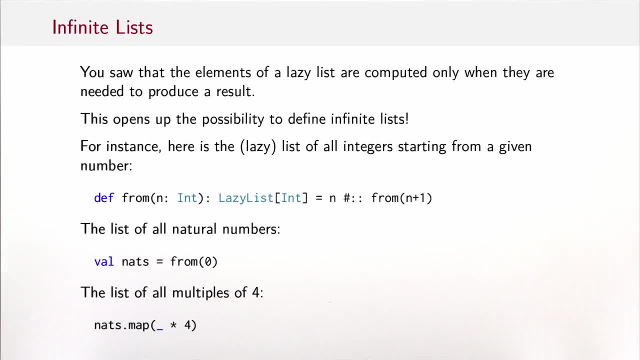 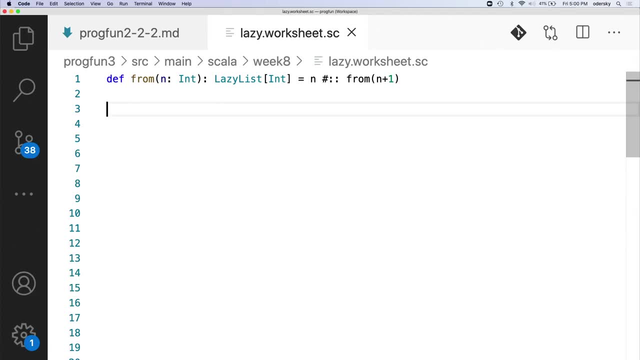 It is always a particular one, and then you compute the natural numbers up to that number. The same holds for the multiples of four. So I will show you that in a worksheet. Here is the definition of from that you saw from the slides, Let's define nats. 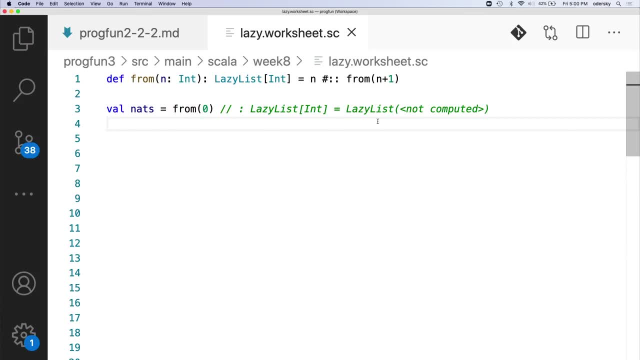 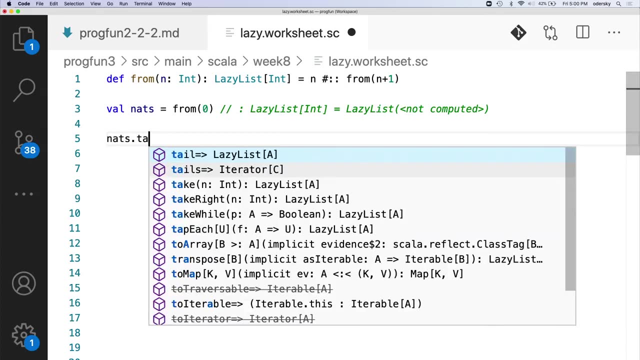 So that gives you a lazy list of int whose value is the lazy list that's not computed. So that's how it prints. Now, if you would write nats, let's say, take ten, Let's take the first ten element of the natural numbers. 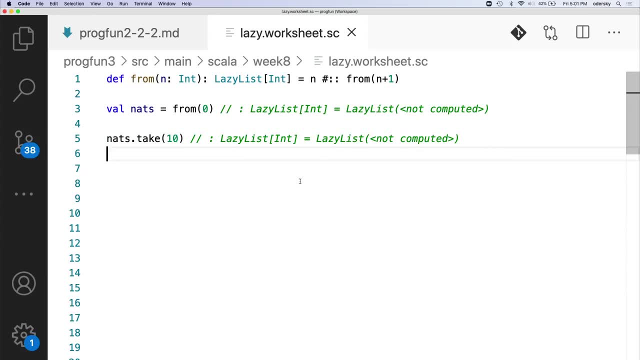 And we still get lazy list not computed. So when do we see anything in a lazy list? Well, one good way is to convert it to lists So we can do nats dot, take ten dot to list, And now we see something. What? 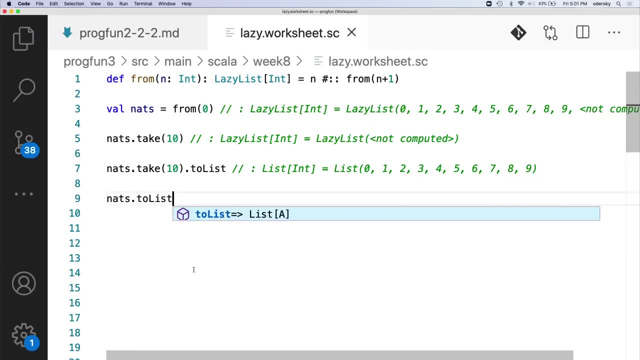 happens if we just write nats dot to list. So I saved and we get a valiant worksheet. so nothing happens, Of course, because to convert all natural numbers to a list, that would never finish, The list would be infinite. So I stop that computation. So you might say: 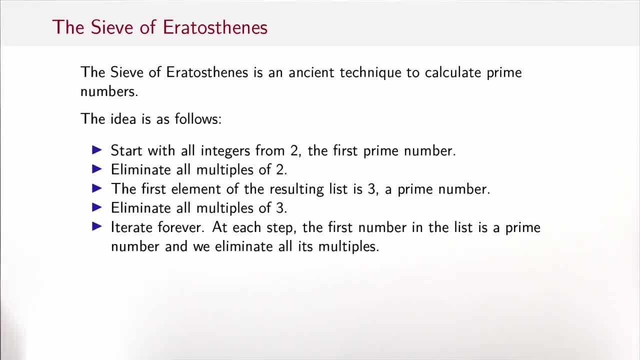 that's cute, but is it useful? Yes, actually you can do quite a few very useful things with infinite lists and other infinite data structures. One useful application is an ancient technique to compute prime numbers, called the sieve of Eratosthenes. The idea can be visualized. 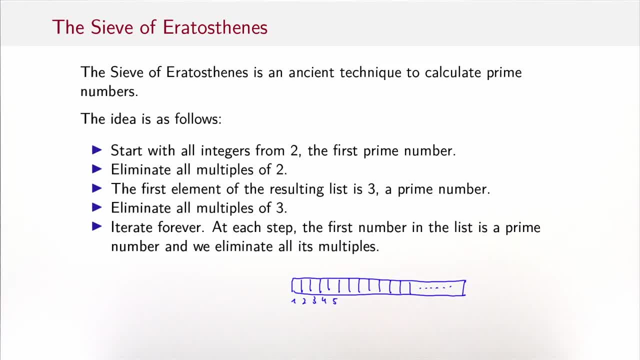 as follows. So we have an array of all numbers here and we start with two. So we say two is a prime number, so that's it. And now we cross out all multiples of two. Now the next number, that's three, is three. So three is a prime. 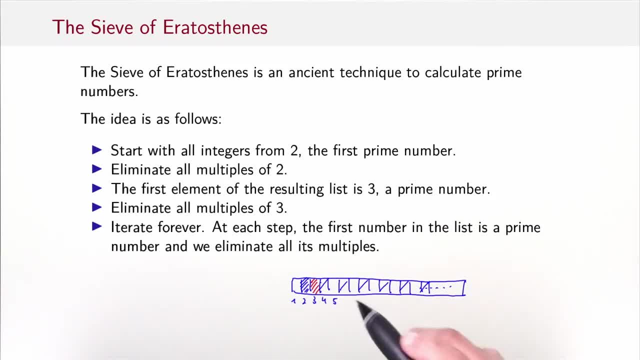 number, and we cross out all multiples of three, So that one is already crossed out, That one is freshly crossed out, That one is already crashed out, That one is freshly crossed out, and so on. Now we see the next empty field, That's five. 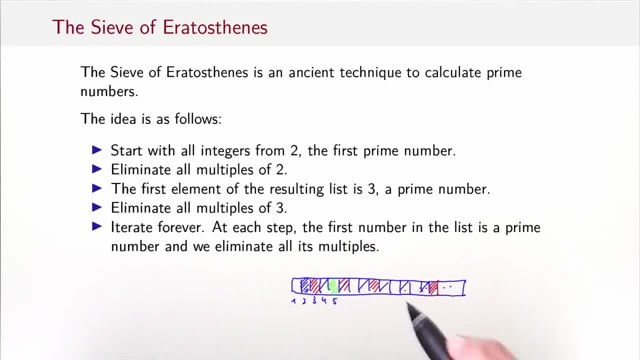 So five is a prime number and we cross out all multiples of five. So at each step we take the next free field. that field is a prime number and then we cross out all its multiples In the traditional formulation of the sieve of Eratosthenes. 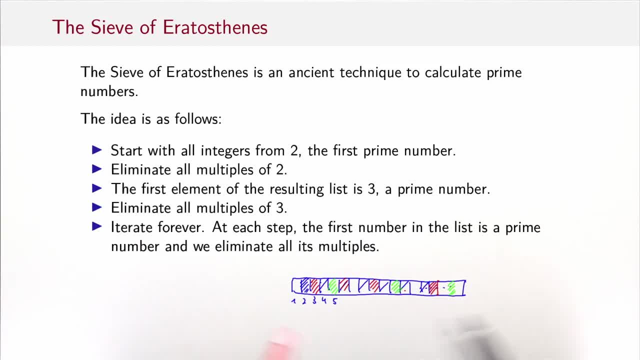 the array here was finite, so you computed prime numbers in a certain interval, from two up to the last field of that array. What we want to do now is we want to generalize the technique to compute arbitrarily many prime numbers without having an a priori upper bound. 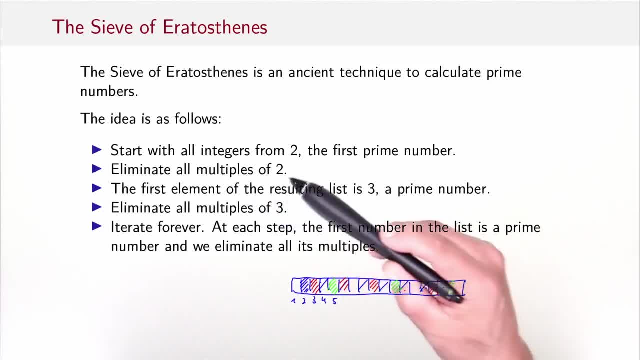 So, to review the algorithm, we want to start with all integers from two, which is the first prime numbers. We eliminate all multiples of two. The first element of the resulting list is three. We eliminate all multiples of three, and like that we iterate forever. 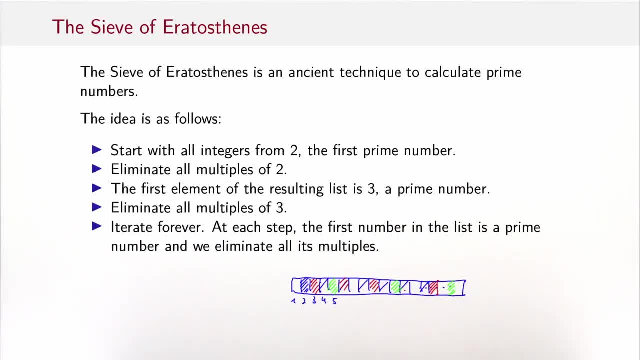 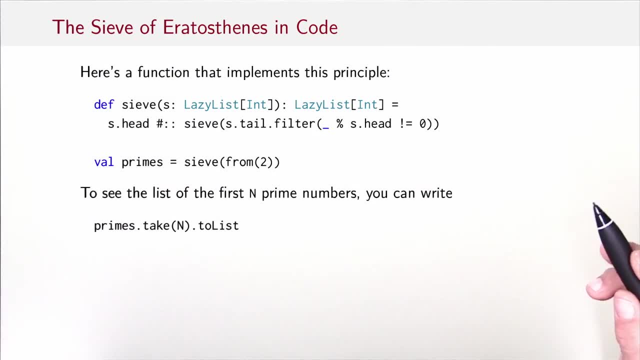 So the list we work with needs to be a lazy list because it doesn't have an upper bound. So here's the sieve function that implements this principle. It's surprisingly short. So here we have def sieve. It takes a given list of integers. 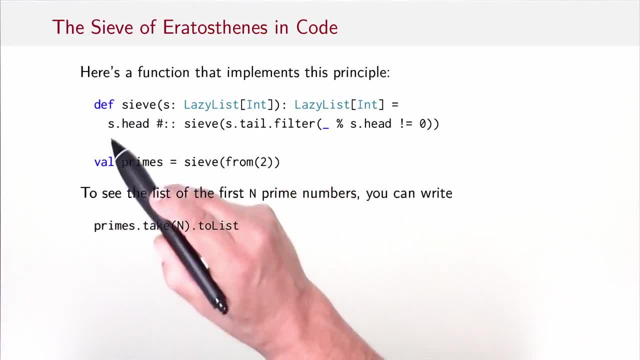 and it filters them so that it takes the head of that list. Then all remaining of the remaining elements, we keep only those that do not have the head as a divisor, So that we keep only those elements. x where x modulo s dot head is different. 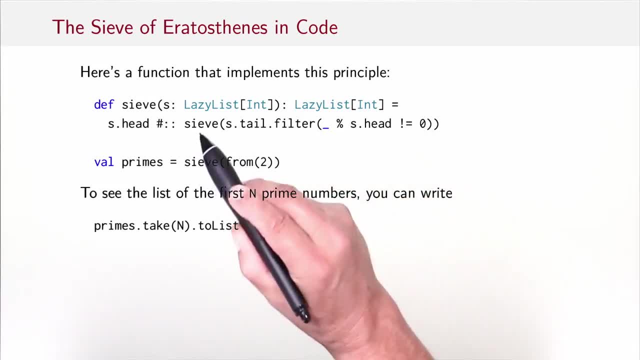 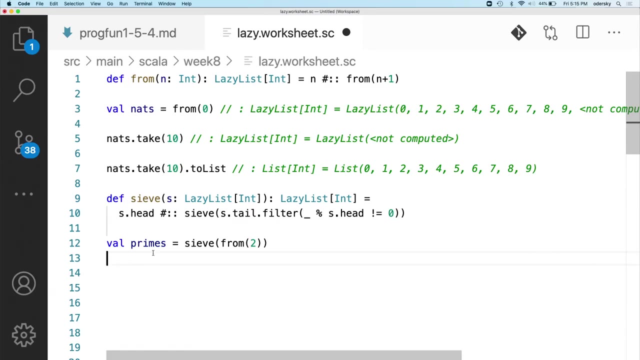 from zero And that remainder of the list gets recursively sieved again. So the prime numbers now would be the sieve applied to all the natural numbers from two. So let's test this. in the worksheet I have copied the definition of sieve and primes. 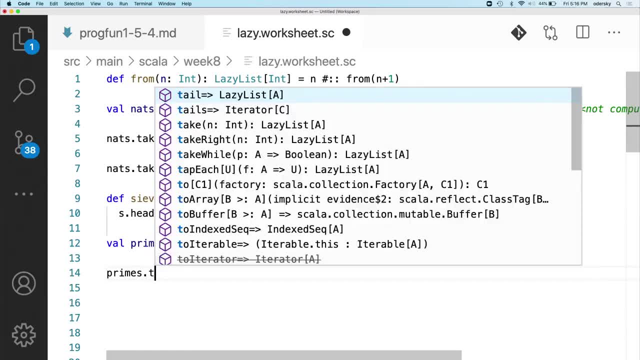 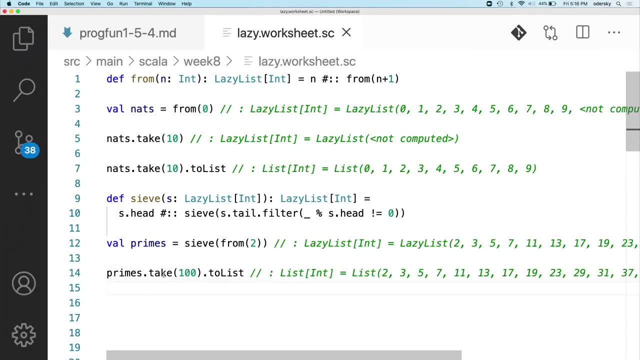 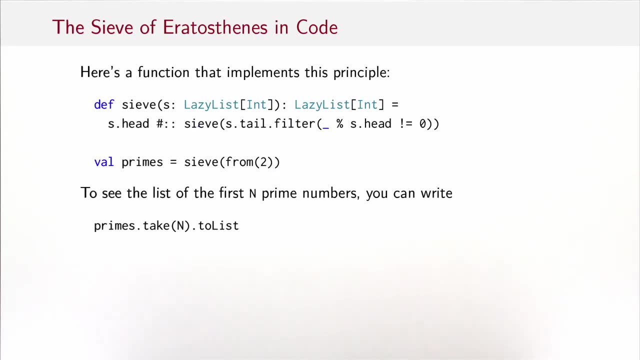 And now let's just find out what are the first hundred primes. So here we see the list, or we see it also if you hover over it. So yes, that looks correct. Those are the first hundred primes. So the lesson to take home here is that 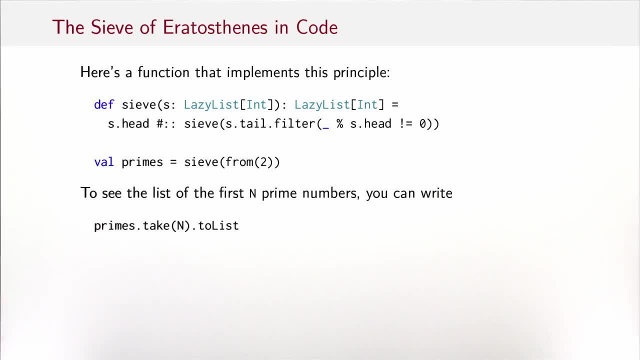 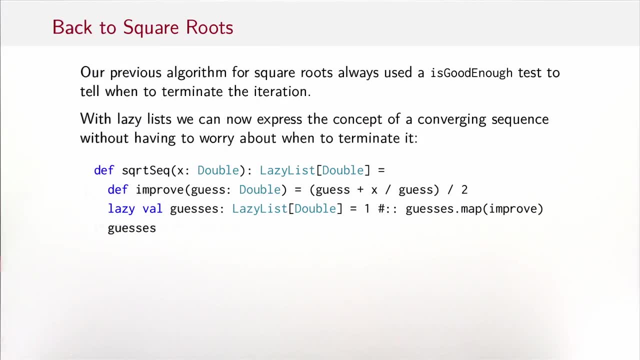 many algorithms that previously required an upper bound can now be extended to arbitrary size by using lazy data structures such as lazy lists. Lazy lists are also useful to define components that can be put together in very flexible ways. For instance, if we come back to our previous algorithm for 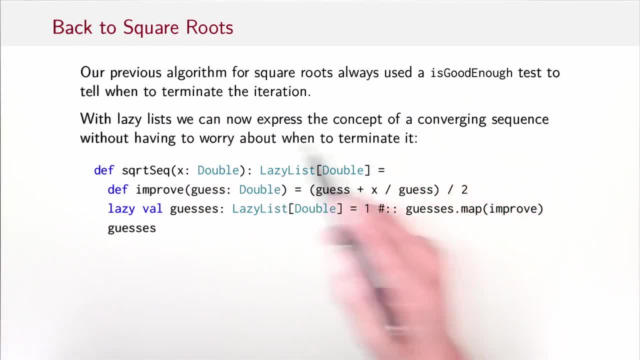 square roots there. we always used the is good enough test to tell when to terminate the iteration. So we had in one loop the iteration, so the next step and the test when it was good enough and we could return the result. With lazy lists we can separate these. 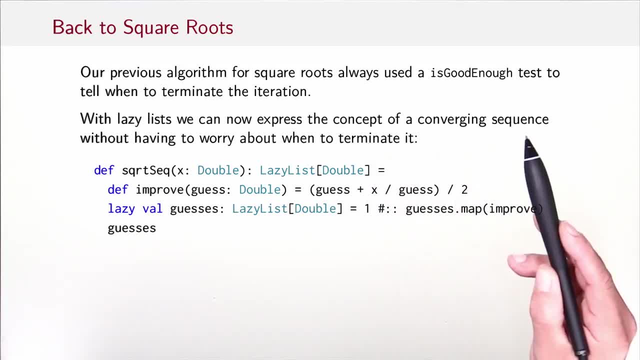 two concerns. We can now express the concept of a converging sequence without having to worry about when to terminate it. So here we could have a square root sequence that, essentially, instead of computing the final value of square root, gives us the sequence of the approximations. 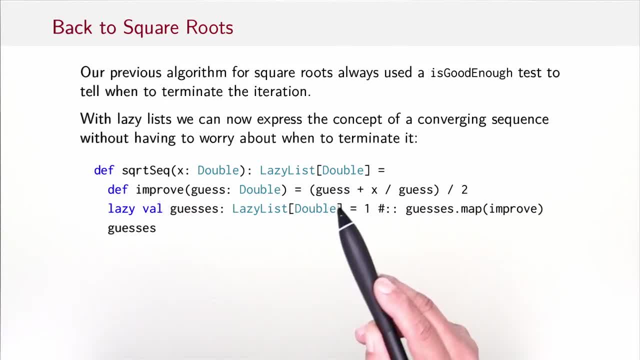 So each improved step is what we had before, so it's the average of the existing guess and x divided by guess, And then we have a lazy list of guesses that starts with 1 and is followed by guesses map improve. Now you might be puzzled, and 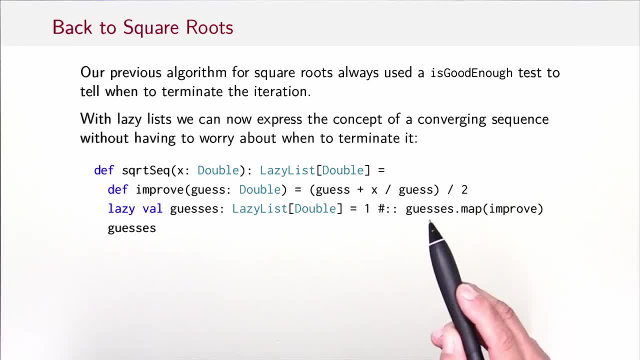 ask. well, that looks weird. guesses uses itself its own value in its right hand side, but yet it is a val and not a def. So how can that work? Well, it can work in some situations if the value of the valdef is a lazy list. 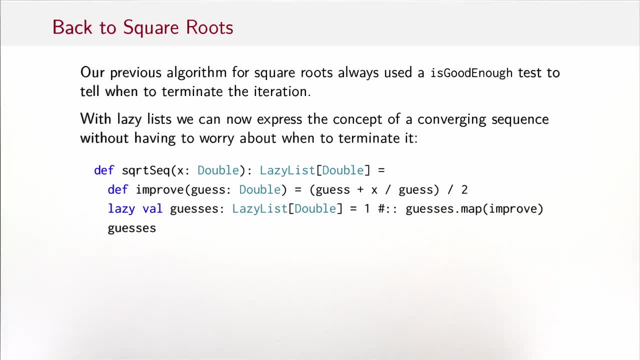 or other lazy data structure. So let's trace the construction of the first few values of the list that we do here. The first value is clearly 1.. It's followed by the guesses map improve. So the first value of what follows is the. 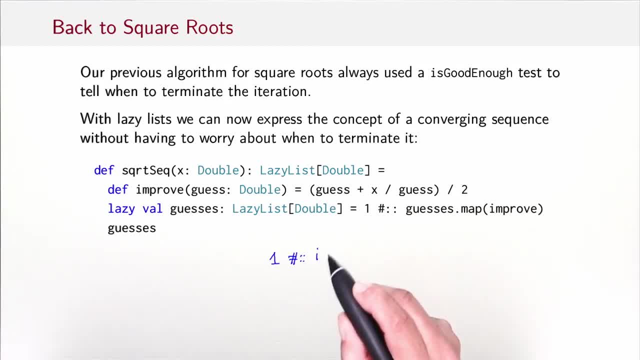 first value of the original list map with improve, So it's i of 1 where I abbreviate improve to i to save some space. What's the next value of the list? Well, the next value of the list is the second value of guesses. 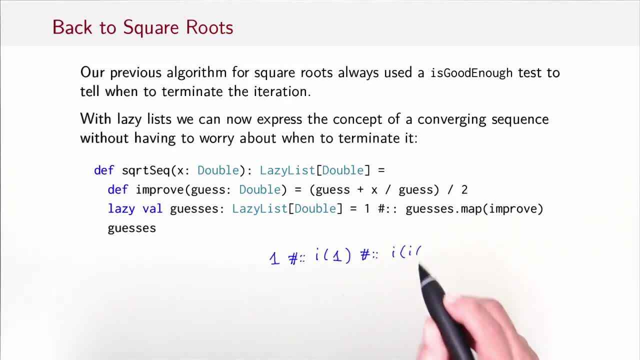 mapped with improve. So it would be i of i of 1.. And the fourth value would be the third value with improve. So you see, every value contains one further application of improve. So what you have here is essentially the iterate of improve, where every value applies. 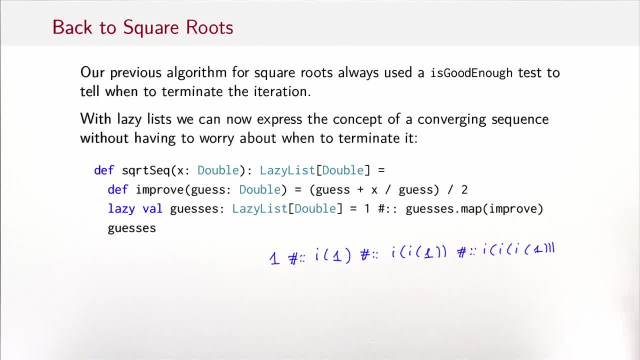 improve one more time, And that's precisely the converging sequence that gives you a square root. So all you need to do in the end is return that guesses. You might still not be quite satisfied and ask: well, why is this a lazy val? 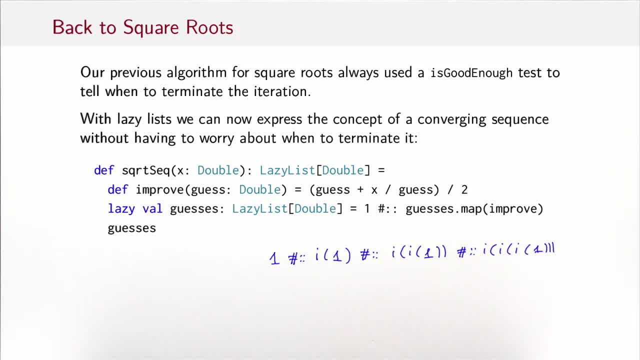 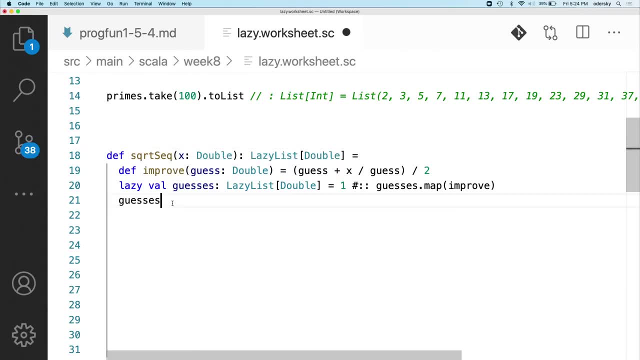 Why can't it be a normal val if you have argued so convincingly that the resulting sequence is ok? So, as always, let's try it out. So we have here our original square root sequence. Let's remove the lazy val. What do we get? 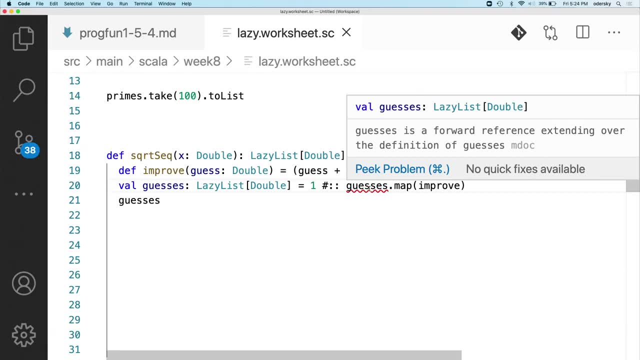 Well, we get a type error. It says guesses is a forward reference extending over the definition of guesses. So what Scala has is essentially it has built in checks that verify that we cannot have a recursive or mutually recursive or forward definition of a val in a local list. 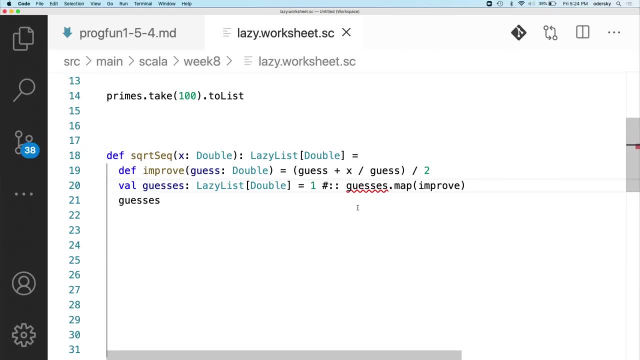 And that check here refuses the program. But the check is conservative. So in principle in this, if the compiler would let this program pass, then the execution would still give us the same result. So in principle it would be ok, But the compiler is overly conservative. However, 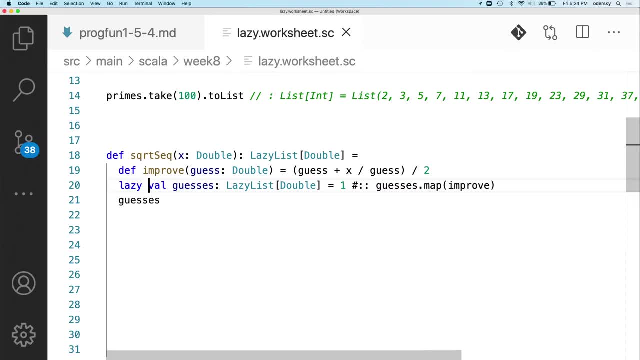 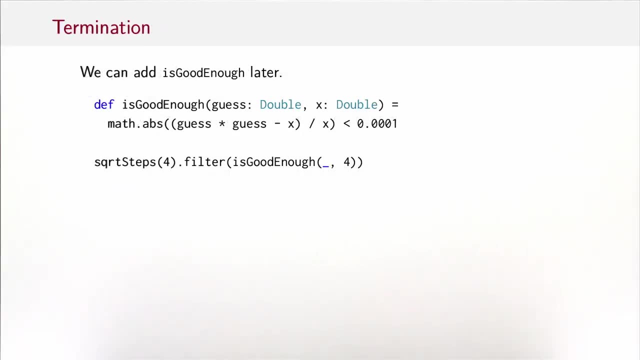 we can avoid the check if we declare the value a lazy val. So that is the solution of the mystery why we need a lazy here. Ok, So the point of having a sequence of approximations is that we can add the criterion when to terminate the sequence. 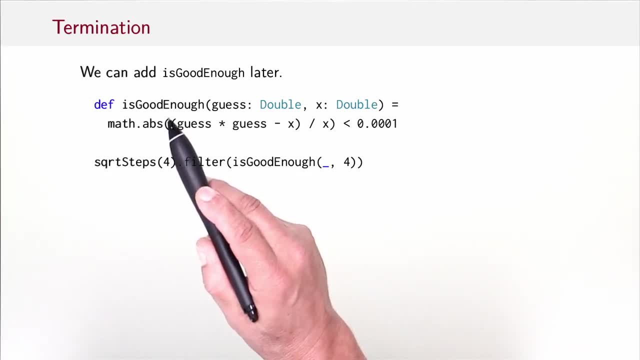 later So we could have now a separate method is good enough. that takes the current guess and the original value from which we want to take the square root and it just says well, if the square of the guess minus x divided by x absolute is less than. 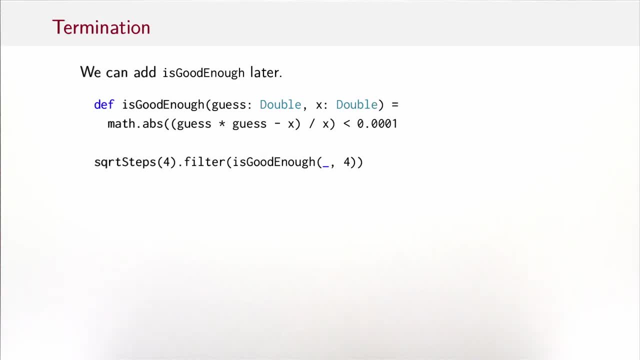 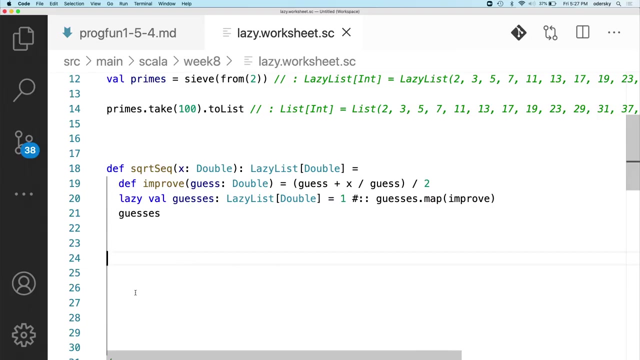 0.001, then that is good enough, And then we can compose square root steps with good enough. So what this expression would do, it would keep only those approximations that are close enough to the value that we want. So let me show you that in the worksheet. 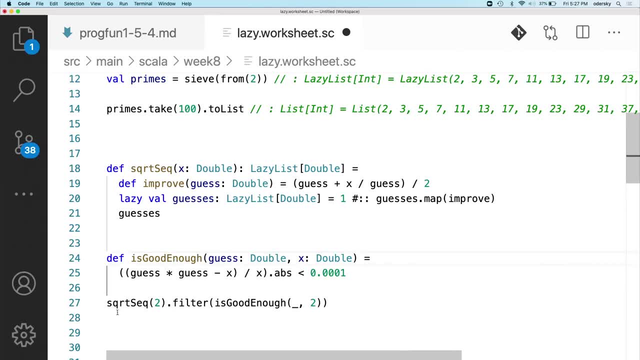 We have the good enough test here, and here we have the expression that filters the original square root sequence with the is good enough test, Assuming that the value we want to take the square root of is 2.. So if we save that, we get a lazy. 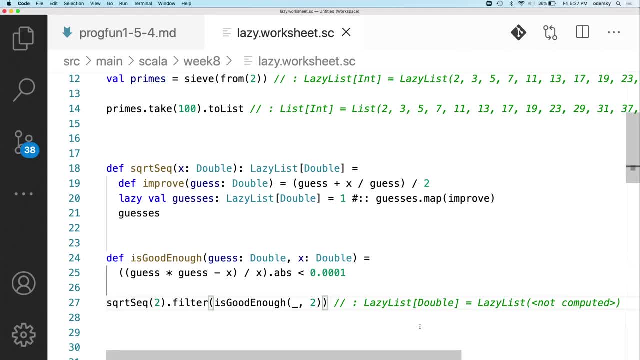 list. It is not computed So to actually get the final value of square root. we just take the head of that list. So we have a series of approximations. We take those that are good enough and we take the first one that is good enough. That is the value. 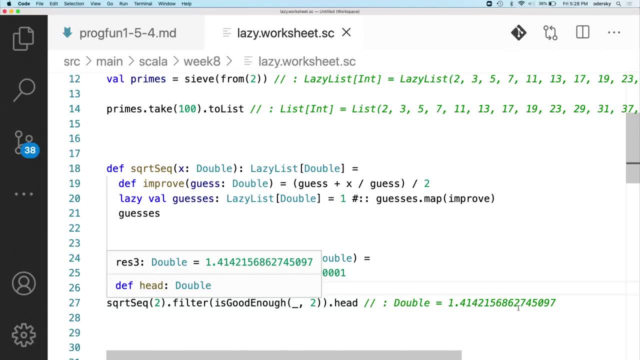 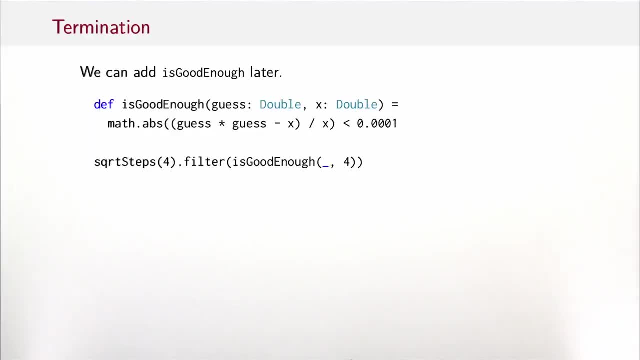 of our square root algorithm. So this is a very nice decomposition of the original square root problem into smaller and smaller steps. It was used as the original argument of quite an influential paper which is called Why Functional Programming Matters. The author of that paper was John Hughes, So let's 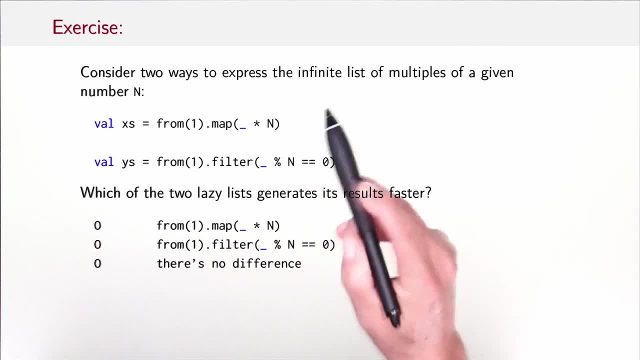 finish with an exercise. Consider two ways to express the infinite list of multiples of a given number, n. So we could say the multiples of n is: take the list of all natural numbers and map each by times n. Or we could say: take the list of all natural numbers. 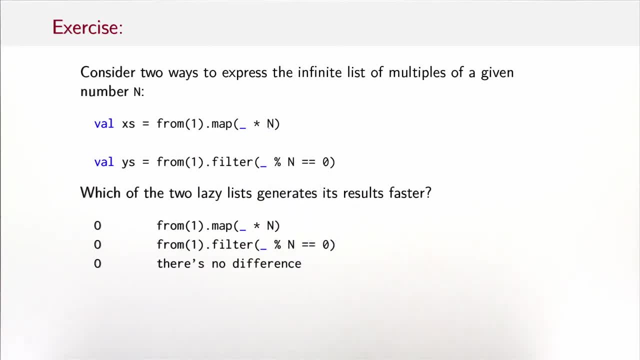 and filter those numbers that modulo n are 0.. Which of the two lazy lists, which both compute the same result, generates the results faster? The first, the second or is there no difference? And the answer is the first, simply because the first doesn't compute. 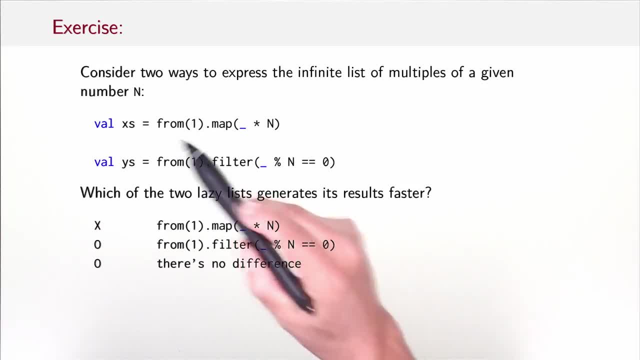 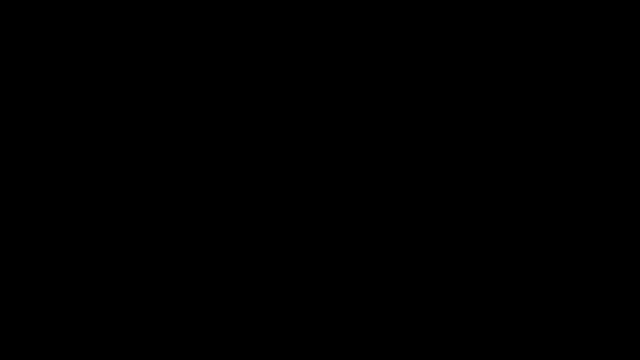 any elements that then are later dropped. So for the first, every element we compute in the list will contribute to the result immediately with the map, whereas the second list generates more elements that then are discarded by the filter. So the first technique is faster. We conclude this week. 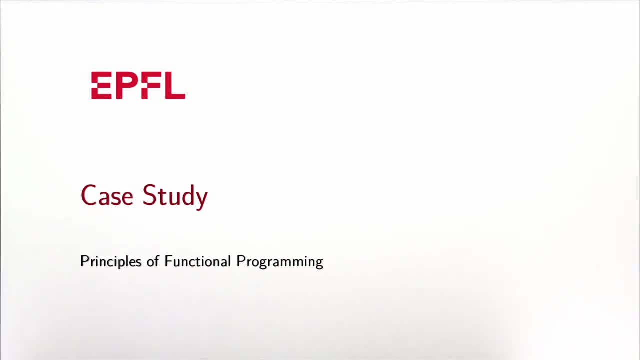 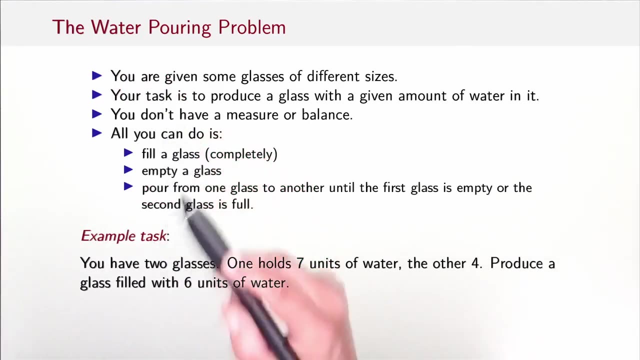 with a case study where we solve another well-known programming problem with the help of lazy data structures. The problem is the water pouring problem. So the water pouring problem is formulated like this: You are given some glasses of different sizes. For instance, you might. 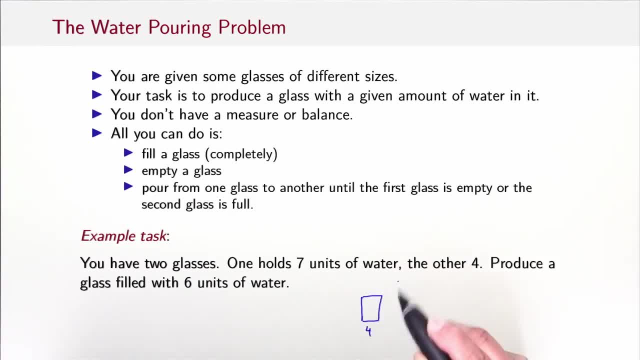 have a glass of size 4, 4 units, and a bigger glass of size 7.. Your task is to produce a glass with a given amount of water in it. So, for instance, you could say: well, we want 6 units of water in one of the glasses. so 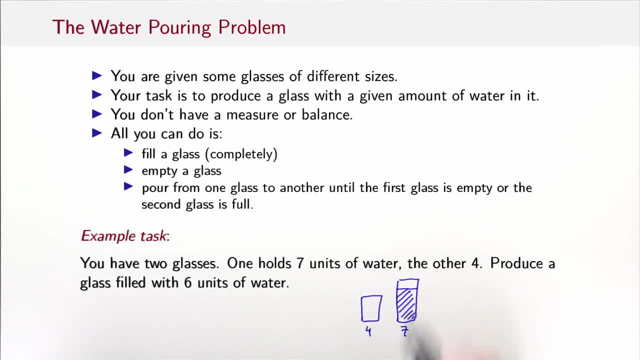 clearly has to be the second one. So we want 6 units of water in here. However, you don't have a measure or a balance. All you can do is fill a glass completely, empty a glass or pour from one glass to another until the first glass is empty. 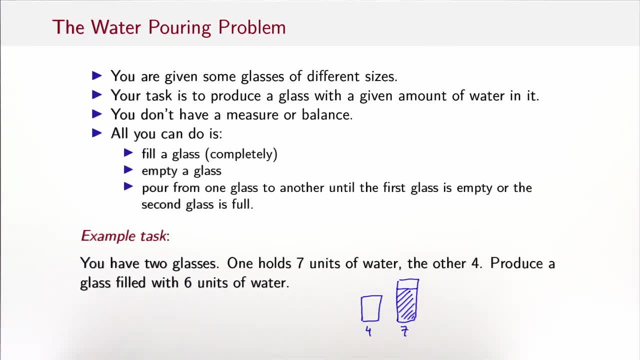 or the second glass is full. So what we are after is an algorithm that will produce a sequence of moves where a move can be one of these three that ends in a situation where one of the glasses holds the required amount of liquid Before we jump into the code. 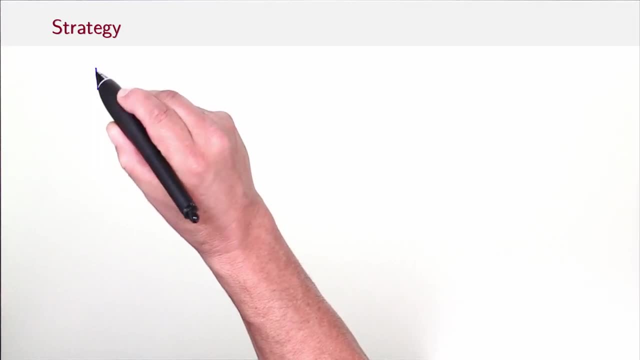 let's develop a strategy. So we are given these glasses- I keep the same example as before, so 4 and 7 just as an example, and we need to produce a target in one of the glasses. So what we can do is, well, we would start in the empty state. 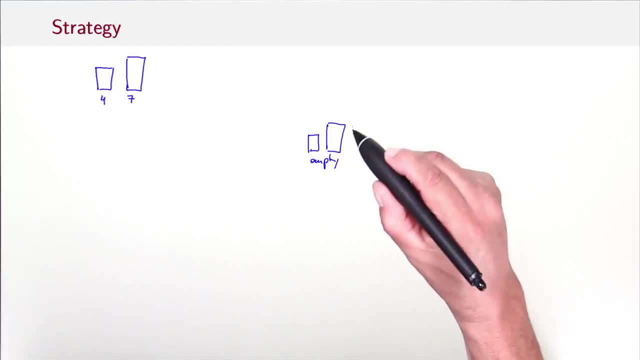 and then from that state we can do moves. For instance, we can do the move which says: fill the first glass, I am going to start the indices at zero, so the first glass has index zero, the second glass index one. So I would have a move. 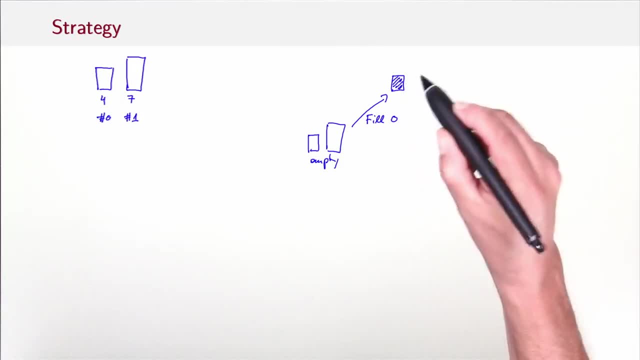 fill zero, and that would give us a new state where the small glass is filled and the big glass is still empty. Or I could have another move which says: fill one, and that would give us a state where the small glass is full, sorry, where the small glass is empty. 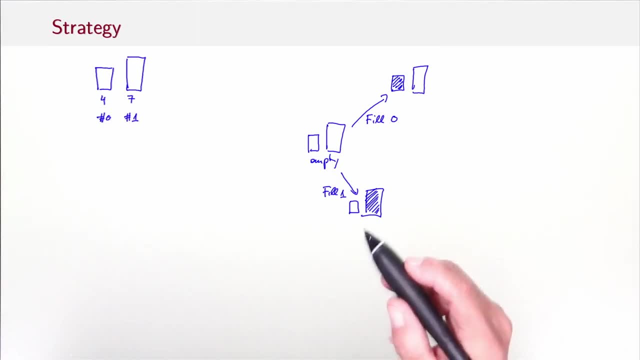 and the big glass is full. Or I could have another move, let's say empty glass, number zero, and that would of course do nothing because the glass zero is already empty, so that would lead back to itself. So those are possible results of an initial move. 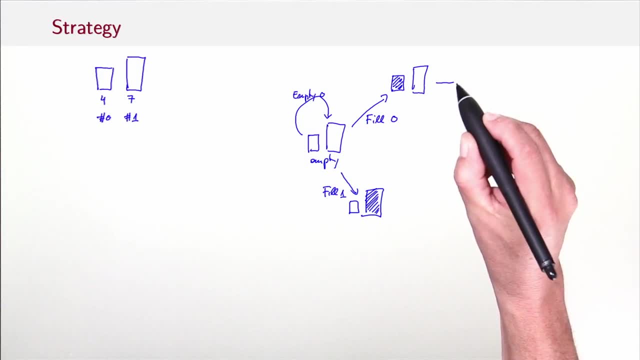 I can then follow that with further moves. for instance, here I could have a move pour from one, from zero to one, sorry, so that now would give me a state where the first glass is zero and the second glass is filled with four, And I could go on. I could then. 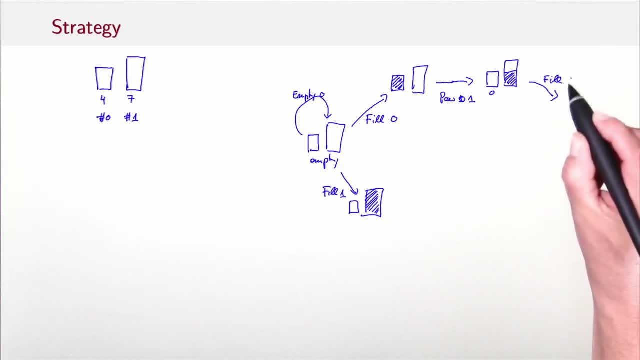 say: okay, for instance here, fill zero would give me four in zero and four in one, so that's four, four. then I could say again: pour zero, one, so that would give me a glass where now the second glass is full seven and the first glass has three units. 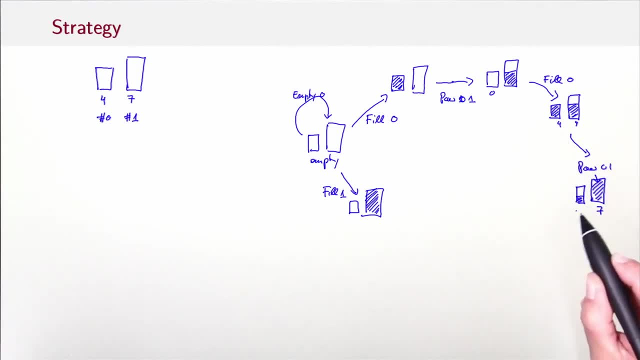 in there because I could- pour sorry, the first glass has one unit in there, because I pour three units from the first to the second and so on, and similarly I can expand here the paths as well, and the idea is then, I would essentially do this exploration until I find: 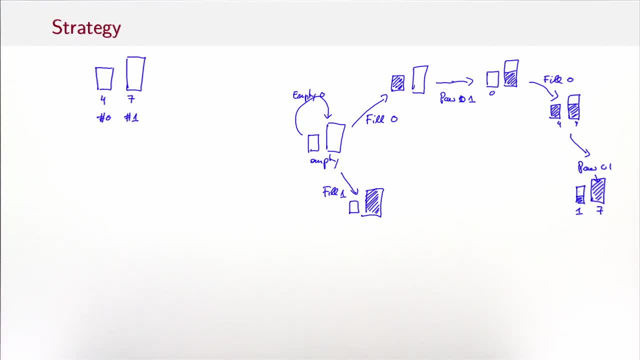 a path that ends in the required target state. but how do I do the exploration? well, one idea is using a lazy data structure. I could simply compute all possible paths and then pick one that ends in the correct target state, but of course, there's an infinite number of such paths. 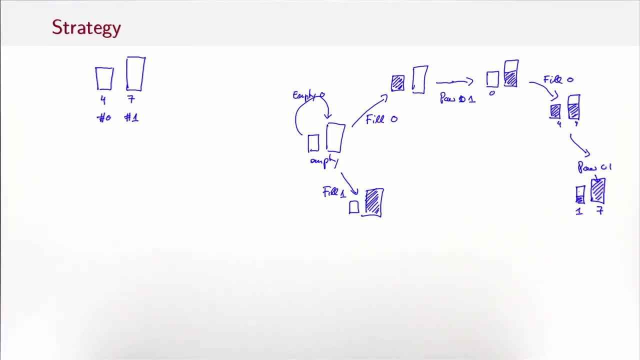 so I have to answer the question: how do I avoid exploring a subspace of of the search space without finding the correct solution where the solution is somewhere else? so the idea to avoid that would be that we produce shorter paths before longer paths, so we first produce essentially all paths. 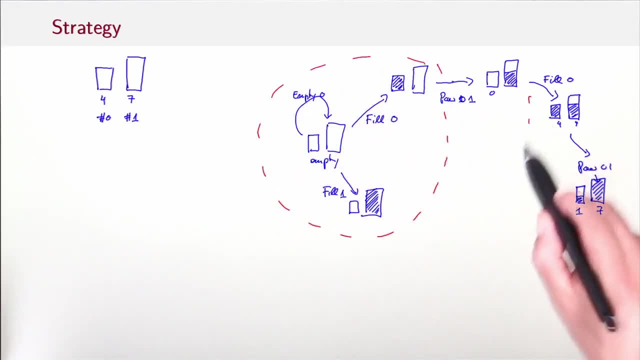 of length one, then we produce all paths of length two, then length three, length four and so on. so at each step we produce all possible paths that originate in the empty state and that have a length up to the length of that step. that avoids falling into an. 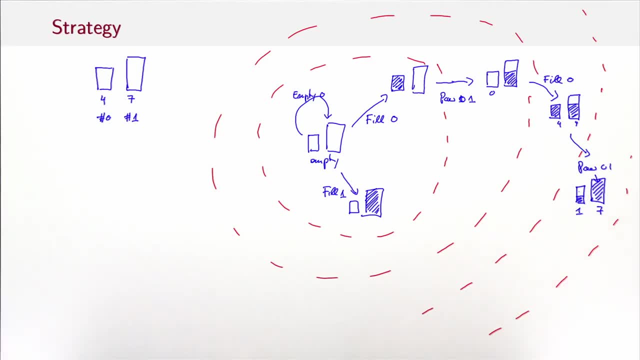 hole of infinite paths, because we go essentially from smaller to larger. the second thing to watch out for is cycles. so another thing I could do here from this state is a move pour one zero, which would go back to the original state, and that's essentially useless because I have just done needless work. 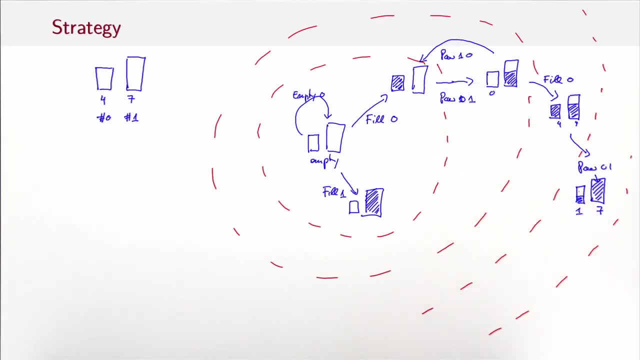 and that will never be on the shortest solution to the target state. so I want to avoid such cycles, and the way I do that is that I simply will keep track of what target states have already been reached and if a path leads to one of the target states, that. 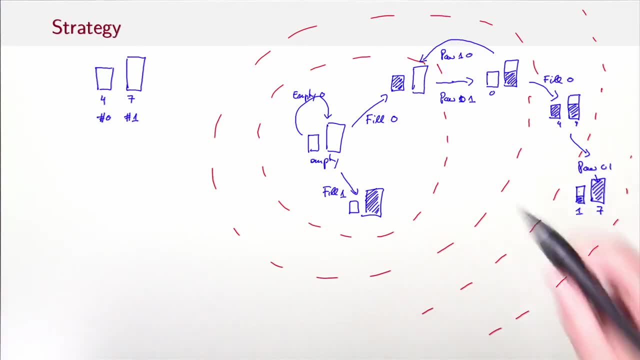 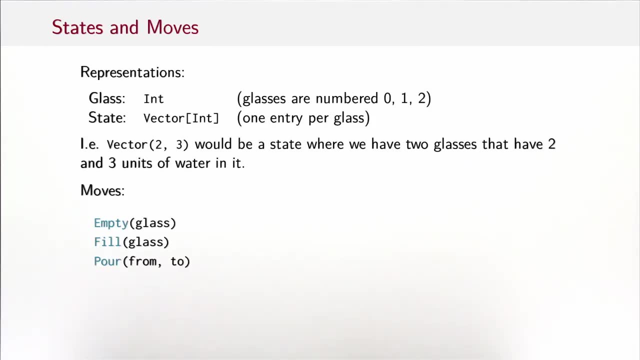 have already been reached, then it's discarded. so that edge here would be discarded by this step of the algorithm. so before we put that in code, let's spend some thought on how we are going to represent things. I've already said, glasses are indices numbered from zero for the first glass, one for the. 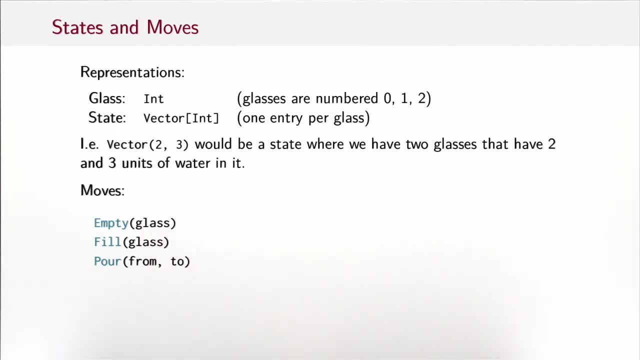 second and so on. so the type glass is just an alias for the int type. and then we have to represent states or configurations. that means how much water is in what glass. so a state can be represented as a vector of int with one entry per glass. so that means 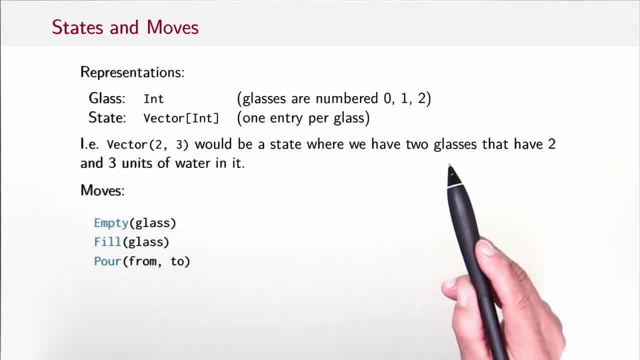 for instance, the vector would be a state where we have two glasses that have two and three units of water in it. so, for instance, vector would be a state where we have two glasses and the first glass has two units of water in it, whereas the second glass 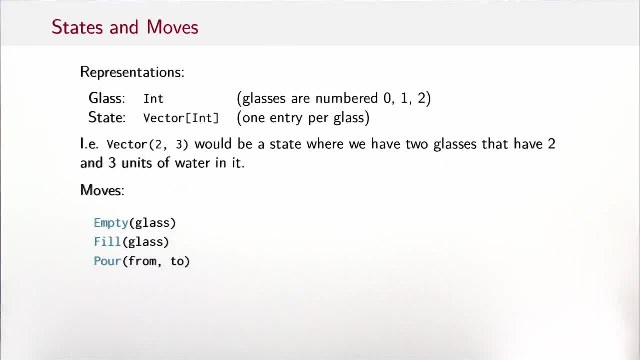 has three units of water in it. so those were the states. what about the moves between states? a natural representation for them would be as an enum, where one case would be empty a glass, another move could be fill a glass and the third move could be pour the content of glass. 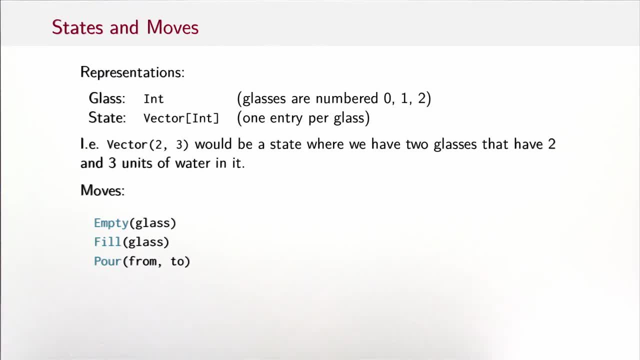 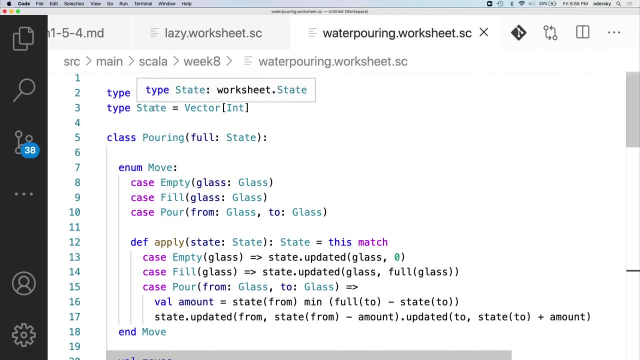 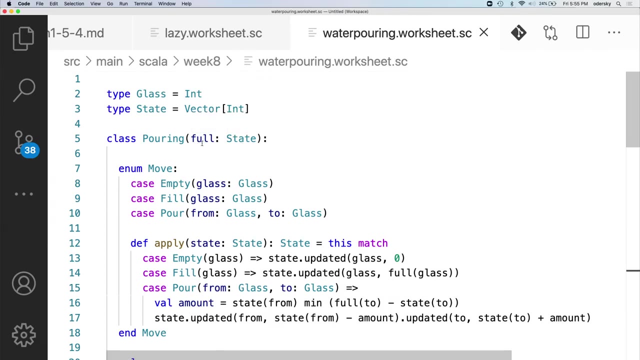 from two glass, two until either from is empty or two is full. okay, so let's set up things in the worksheet. we have the type glass and state, as discussed, and then we have a class pouring which contains as parameters the state with all glasses full. so that means for every. 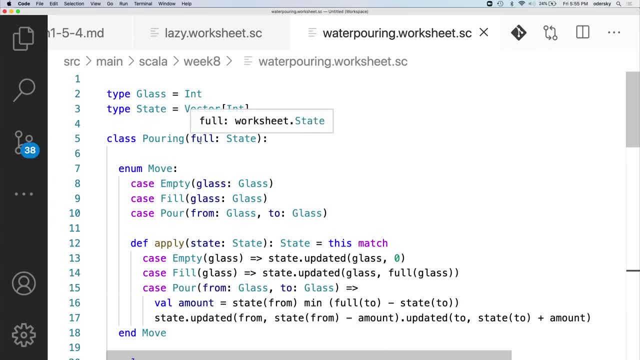 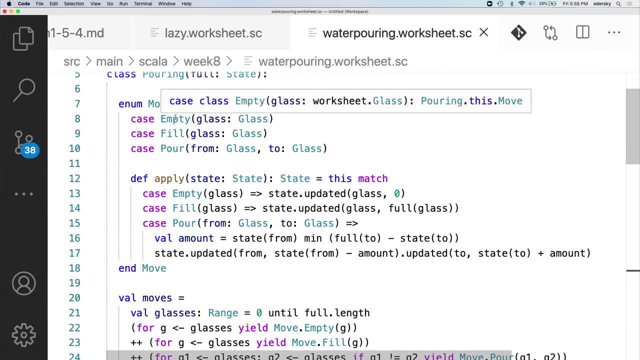 glass. we know what the capacity of the glass is because that's in the full state. so that's the parameter for my pouring class. then we have our enum of moves, which is empty, fill or pour, and what i'll do is i'll already describe what each of these moves 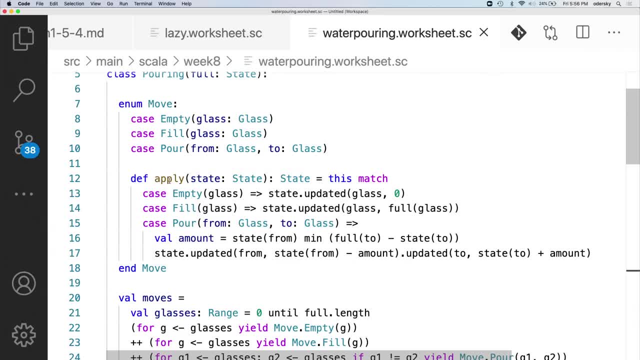 does to the current state, and i do that in an apply function so i can apply a move to a state and that gives me a new state. so what does the application do? so if the enum- so that's this here- is empty, so if the move is empty glass? 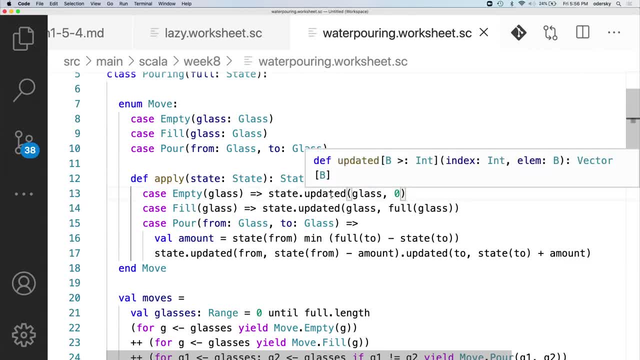 then the state would be the state updated. so it's the old state, except at the index glass, where the state will be zero. if the move is fill glass, then the state is the state updated, such that at the index glass now the glass will be full. so we have the original. 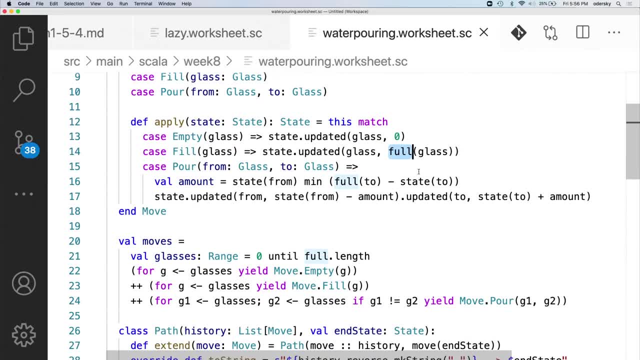 state where the glass is at capacity. and the third move is pour from one glass to the other. where is here? we first compute the amount that is going to be poured from one state to the other, so the amount would be. well, we can only pour what we have in from. 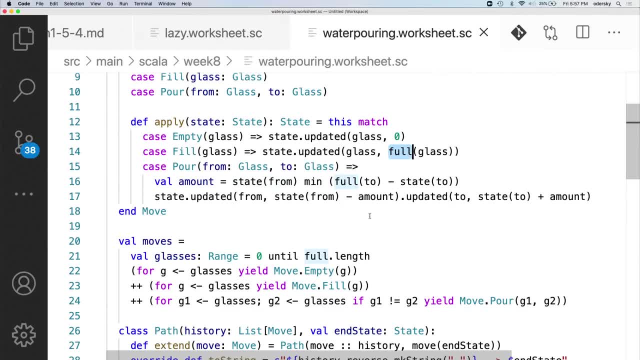 so that state of from and we can also only pour what remains in two, so that would be full of two minus state of two is what's still empty in glass two, so that those are two upper bounds for what we can do. so the amount that we will pour is the minimum. 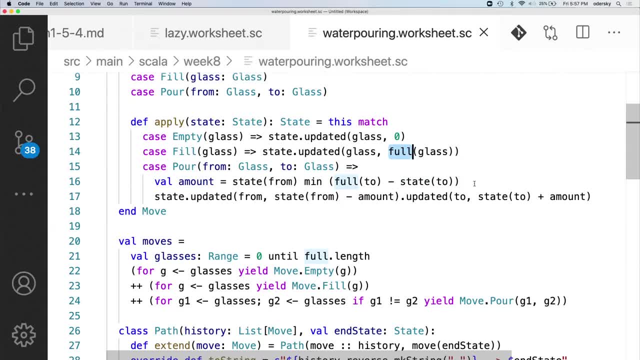 of those two amounts. once we have computed that, then the new state would be the state where the from glass has its contents diminished by amount, so its state of from minus amount, and the two glass has its state augmented by amount, so its state of two plus amount. 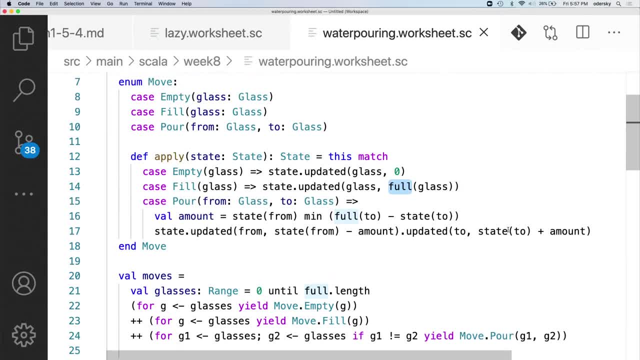 so that's the move. the next thing we could do is: well, what moves do we have? can we enumerate all the moves? because that will be useful if we want to enumerate all the solutions and, yes, that's an easy exercise. so, to enumerate all the moves, let's first enumerate all the 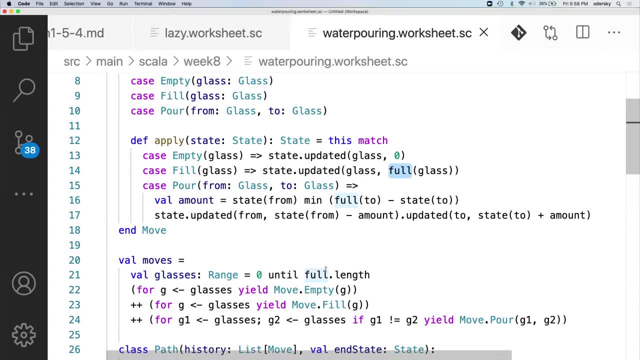 glasses. so the glasses is just the range from zero until full dot length. so that's the possible indices we have. and then what moves could we do? well, we could empty one of these glasses. so that's the expression four g taken from glasses: yield, move dot, empty g. 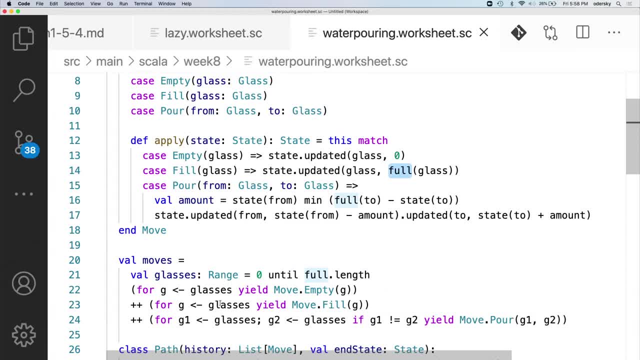 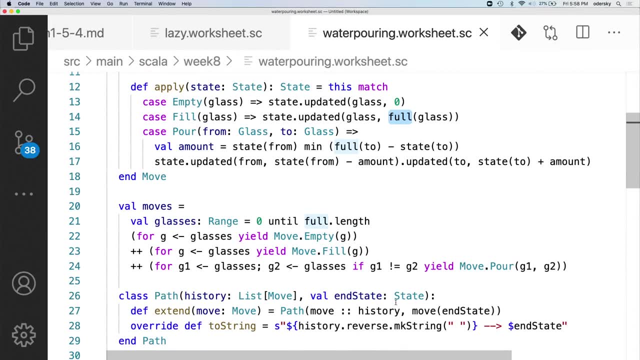 or we could fill of one of these glasses, so that's the second one. four g taken from glasses. yield move dot fill g. or we could pour from one glass to another, so that would be four g, one taken from glasses, g two taken from glasses. if g one is different from g two, we can't. 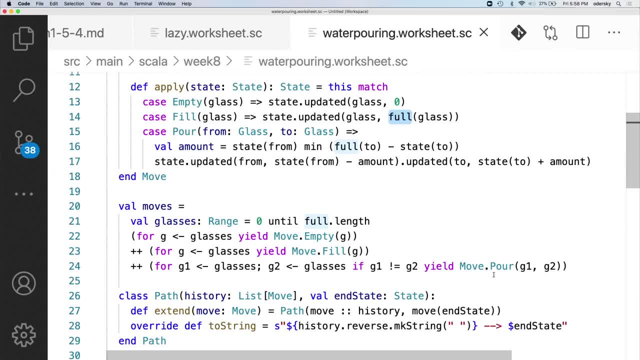 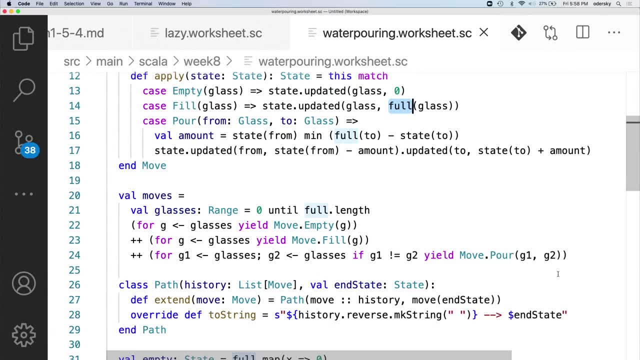 pour from one glass into itself, then yield, move dot pour g one to t two. ok, so the next step to model is a path. so how do we do that? so the way we want to do that is that we want to essentially record paths in reverse order. 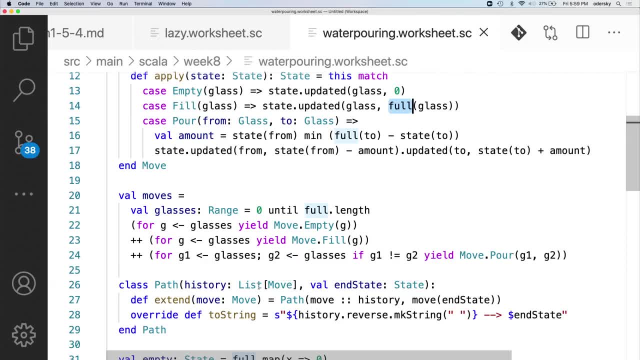 so a path is a list of moves, but what we want is essentially the history. so the last move in the path should come first and the first move from the initial empty state would come last in that history. so a path would be: have a history which is a list of moves. 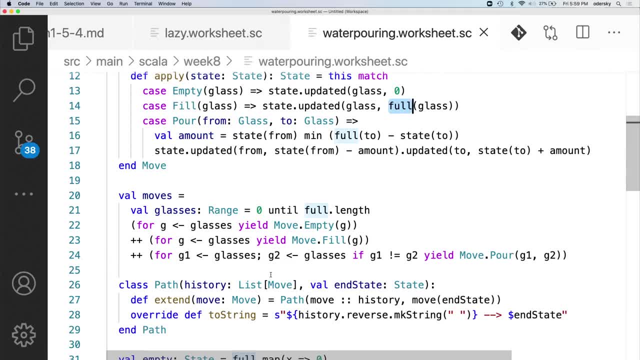 and then it's also useful to already record what the end state of that path would be. so that's the two elements of a path. so if we want to print a path, then what we do is we print the history in reverse, so that now we go forward from the 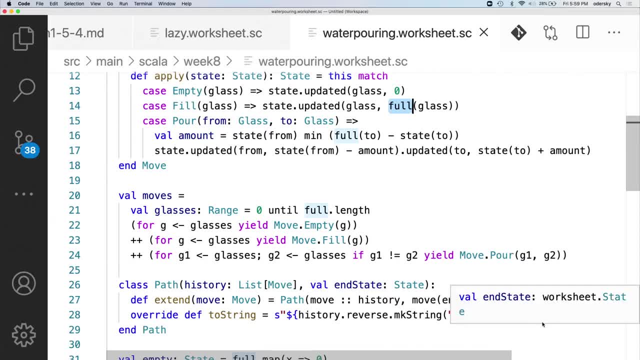 empty state and then we print an arrow and we print the end state. so that's the end state, the configuration that that path leads to. we also have a utility method, extend. so that's tells us what path results if we add and move. move to the existing. 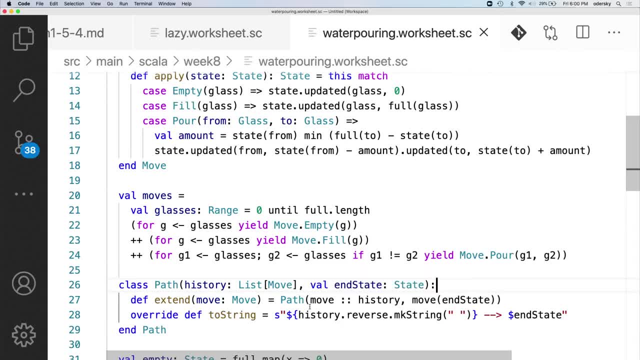 path and the path that results is given here on the right. so the history of the path would be the move that we extended with and the existing history and the end state of the path is simply the move applied to the end state of the current path. that's the apply. 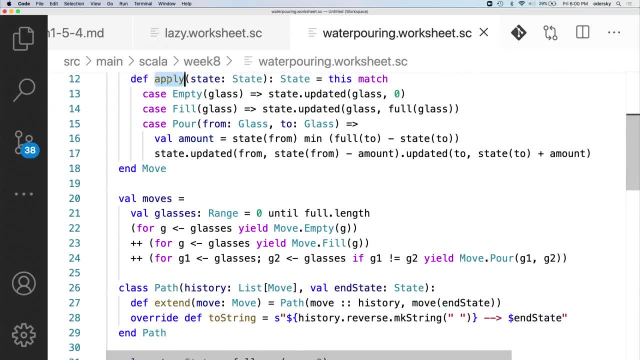 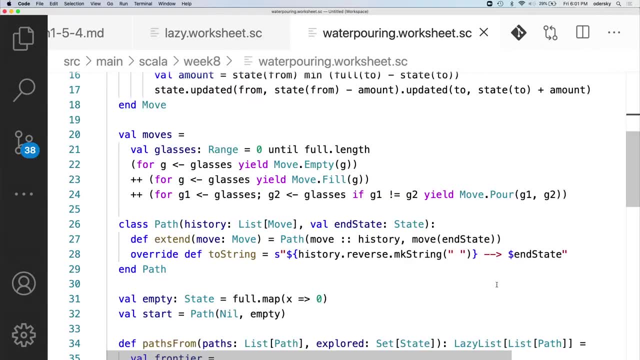 function that we have defined up here, which precisely tells us essentially what moves do to state. so the new end state is the move applied to the old end state. okay, and then we start from the empty state. so that empty state is simply the full state where we 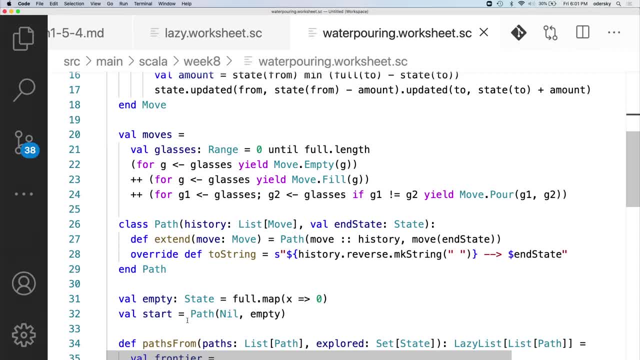 map all content to zero, and our start path is then the path that has no history because we just started and has the empty state as current state. so one interesting observation is that so far we haven't actually written an algorithm to compute the solution. we just modeled the domain. 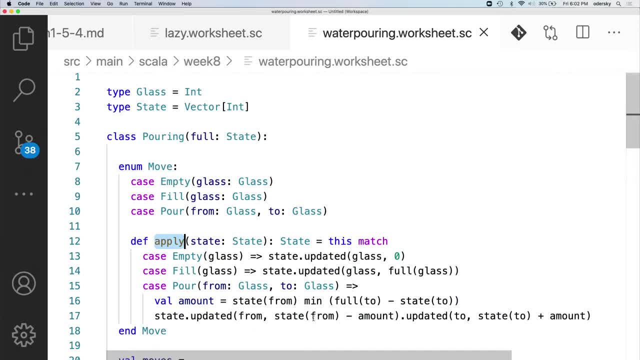 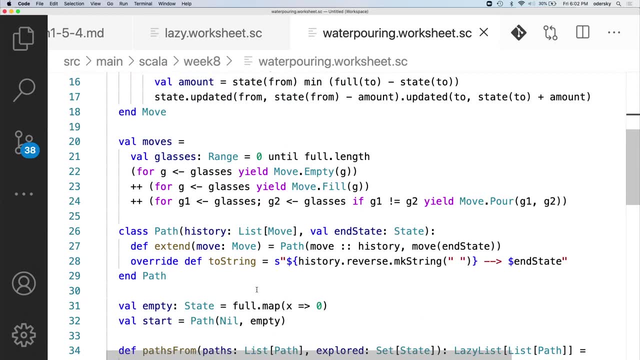 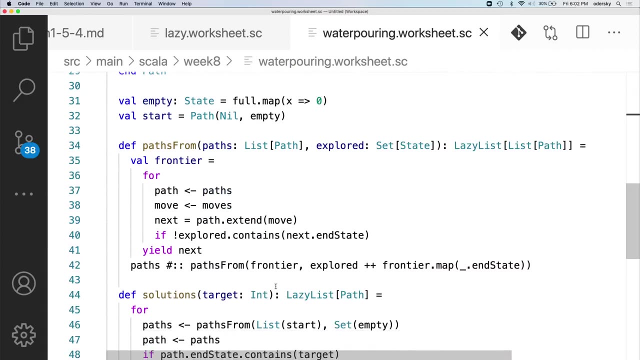 we said, okay, how do we represent classes, states, moves, what moves do we have? what are paths? and that was it, basically a good domain model that helps to keep the actual search algorithm very clear and very short. so let's go to the algorithm next. there are two parts to it. 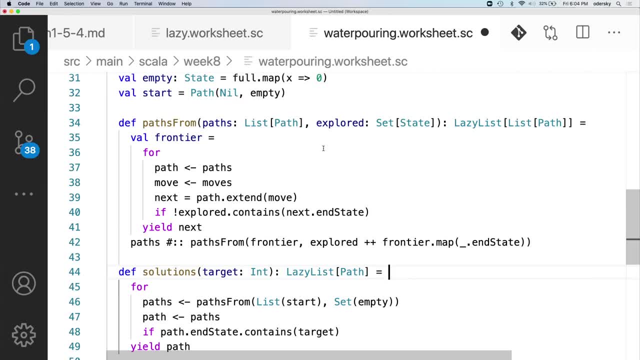 one part builds the infinite list of possible paths and the second part then picks out the right solution from that very, very large list. so the first part is done with the paths from method. so paths from is similar to the from method on natural numbers that we've seen it. 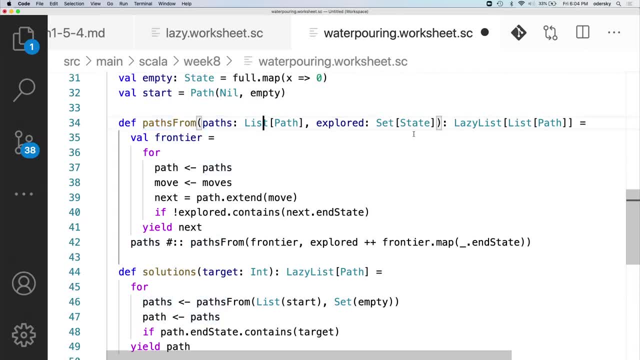 takes an initial list of paths and an initial set of states that were already encountered and it gives us essentially all lists that start in these paths. so that would be a lazy list of lists of paths. the idea here is that the path from that it gives is ordered by length. 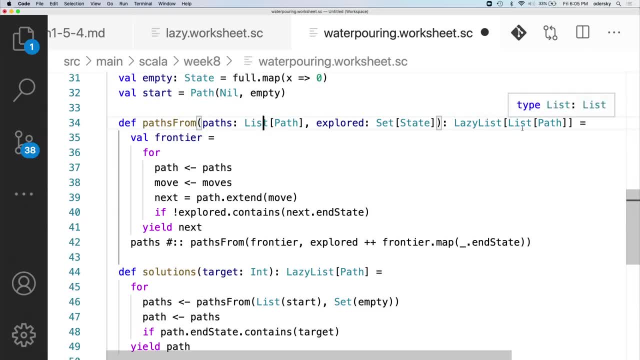 so each element in that lazy list is a list of paths and the first element, if we start from the empty state, would be all the paths that have length one. the second element in that lazy list would be the list of all the paths of length two and so on. so the 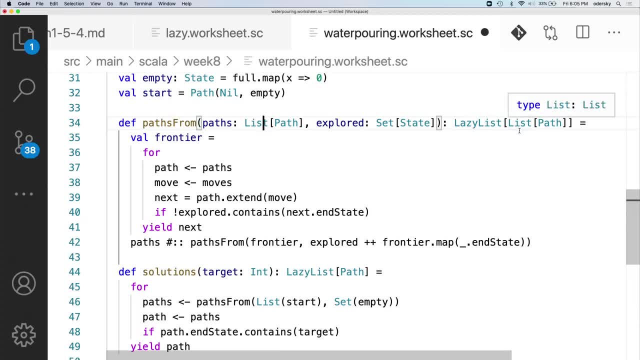 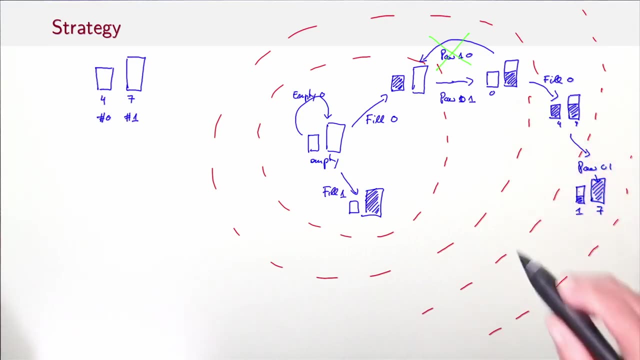 paths that are in the outer lazy list are ordered by length. ok, so how would we produce that right hand side in paths from? so if we go back to our strategy, so we're given a list of paths all of the same length and we want to extend. 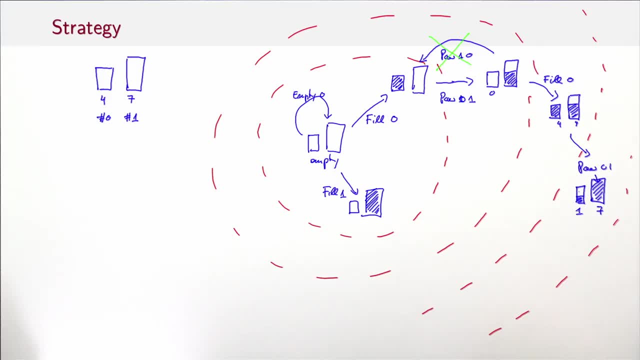 it by essentially one move each of those paths. so what we are after is essentially the next circle around here. call that the frontier. so the frontier is essentially the set of paths extended by one. the frontier is computed here, so we say, ok, let path range over all. 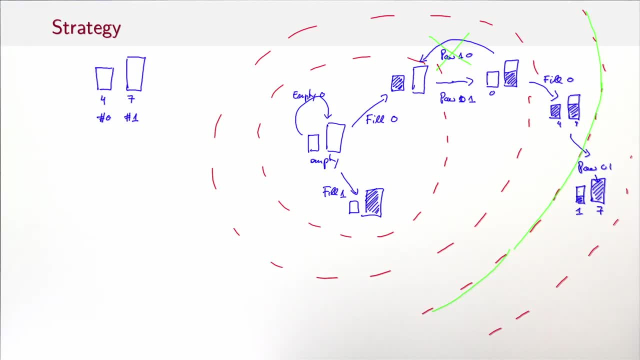 the paths that we have now let move range over all the possible moves. let's extend the path with the move that gives us essentially the next path and then let's keep the path if its end state is not already in explored. if it's already in explored, then that would be a 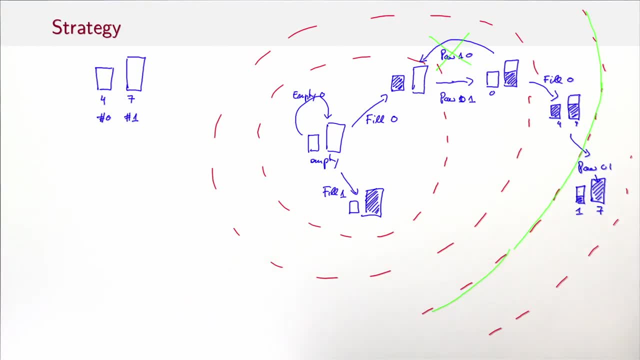 cycle and we can drop that path. so the paths that survive that criterion form part of the frontier here, so they are returned. ok, so that gives the frontier. so now we want to compute all the possible paths that start from an initial set, so that that would then be. 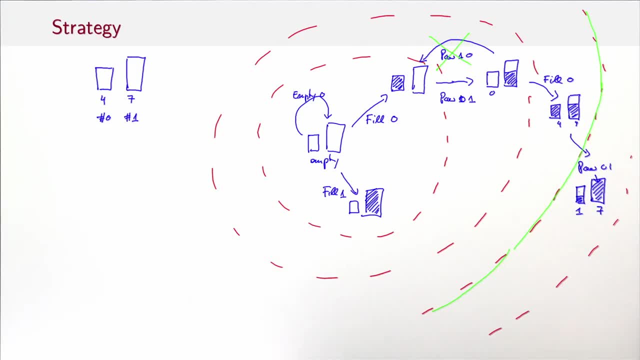 the initial paths that we have followed by the paths from now, the new frontier and the set that we have explored is the previous set that we have explored plus all the end states of the frontier paths. so frontier map, end state, so we combine the two. that gives us a set of paths. 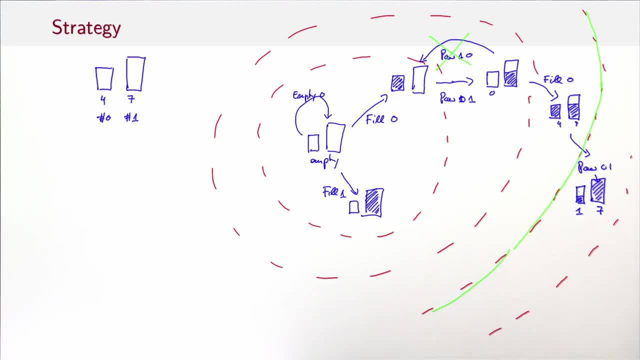 that's explored now and of course that gives us an infinite list of paths. but that's not a problem, because this thing here is a lazy cons and we produce a lazy list, so we will expand that list only into the degree where somebody wants to find an element. 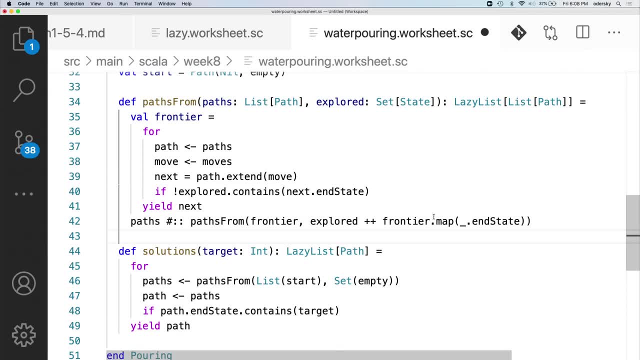 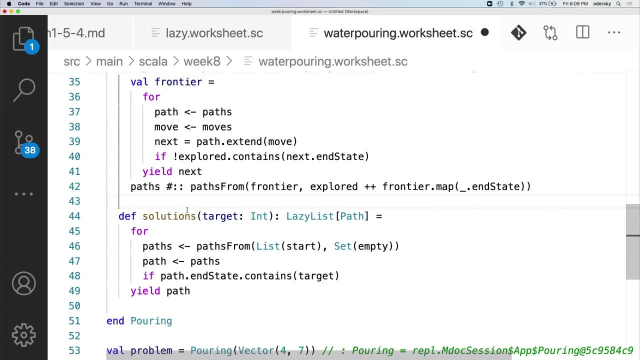 in the list. ok, so now that we have explored the search space using paths from, so that we can now span an infinite list of list of paths, let's find this path that lead to a solution in that infinite list. so that's the solutions method. it gives us again a lazy. 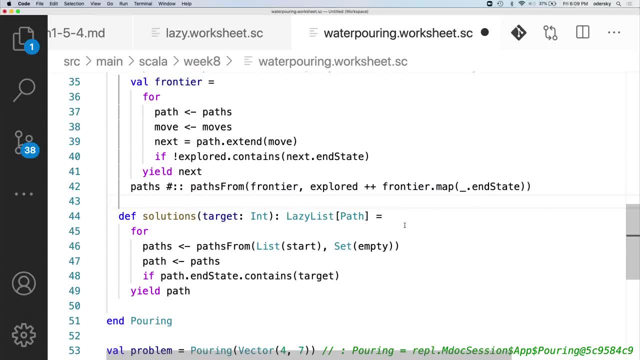 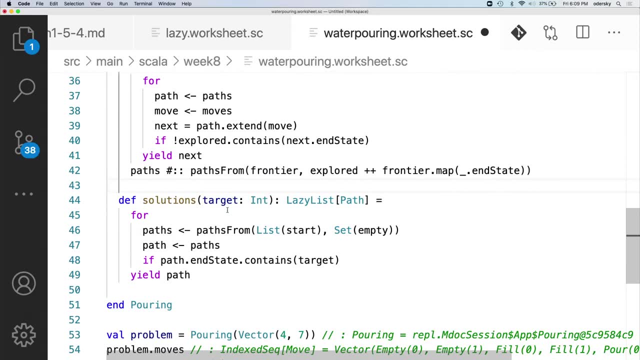 list of paths and it contains all the possible paths that we have constructed in paths from that end in the target state, so that have a class that contains the required amount target of units of liquid. so what we do then is we construct the search space here in paths from: 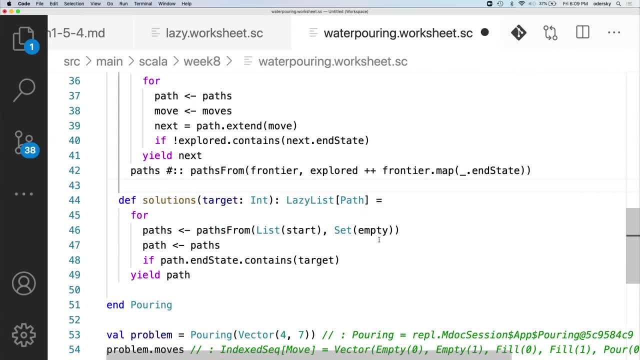 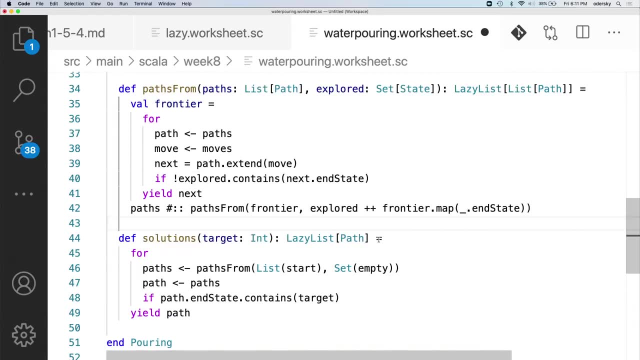 we start with the empty state and what we have explored: nothing so far, so no state has been explored. so now that we can construct all possible paths that start in the empty state using paths from, we use that to pick those paths that end in the required state. so we want to. 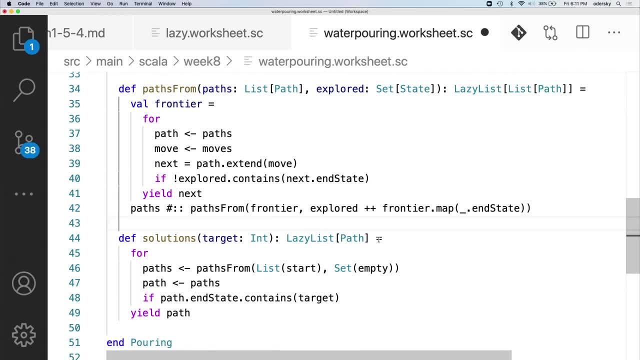 pick those paths that end in a state such that there is a class with target unit in it. so the way we do that is we span the possible search state with paths from. the initial path is just the start and the initial set of explored state is just empty because initially 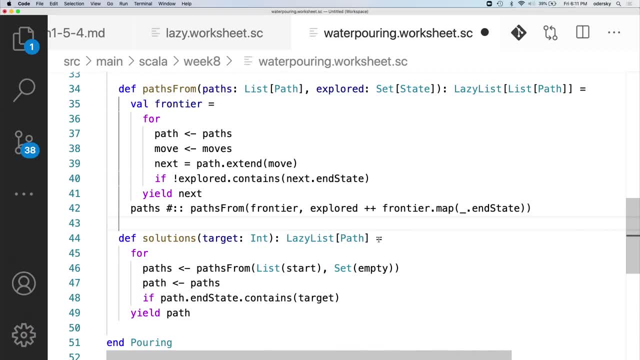 all classes are empty. so that's the state. we know that's the original state and that's the only state in the set. so then we take an arbitrary path from the search space. we ask whether the end state of the path contains the target and if that's the 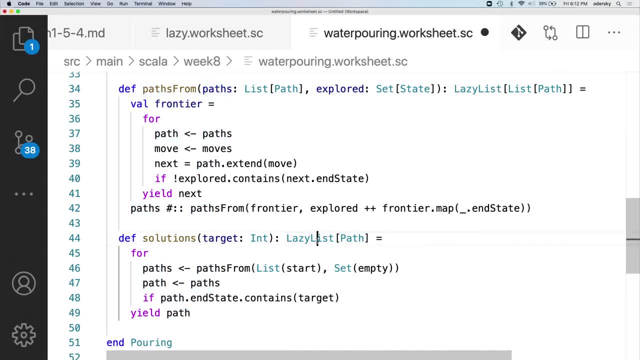 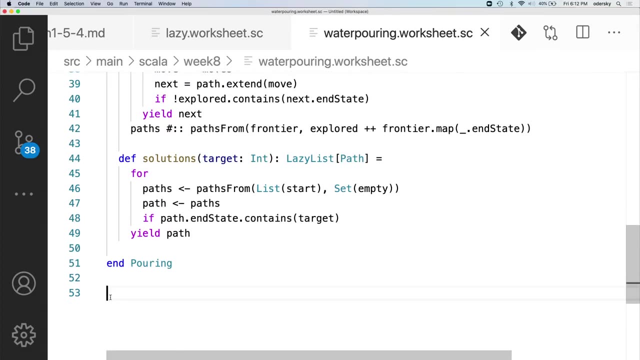 case we yield the path. so now we have a lazy list of paths where every path is a solution to the original problem and, furthermore, the lazy list will be ordered that shorter paths come before longer paths. so that's the whole algorithm. so to use it for an example problem: 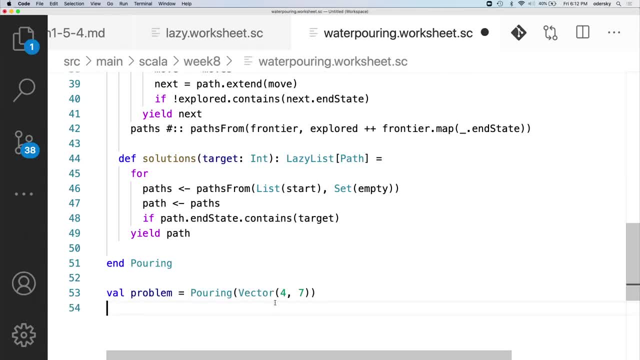 let's define a problem. let's say it's pouring with the vector of two glasses of size 4 and 7, as discussed. and now to find a solution to have a certain target state, what we write is: problem dot solutions with the target. let's say we want a glass with 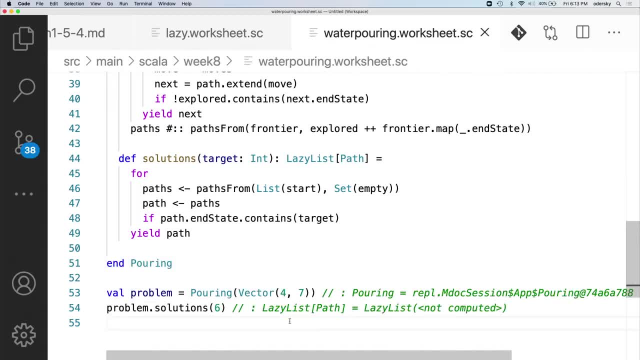 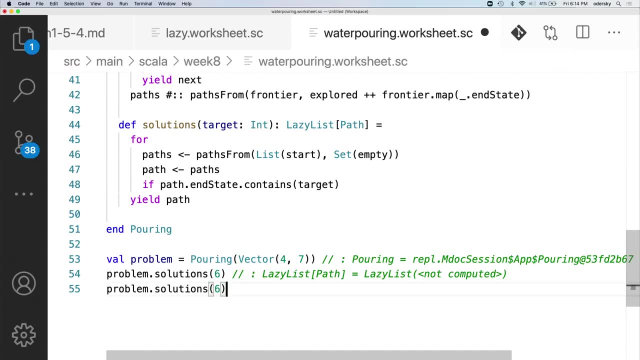 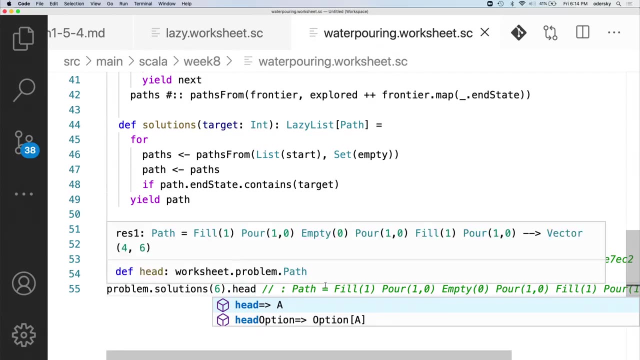 size 6 in it. that would give us a lazy list of paths and what we want is the shortest. now to get one solution, we just take the head of that list. that will give us the shortest possible solution to the target state, if one exists, and indeed it has found one. 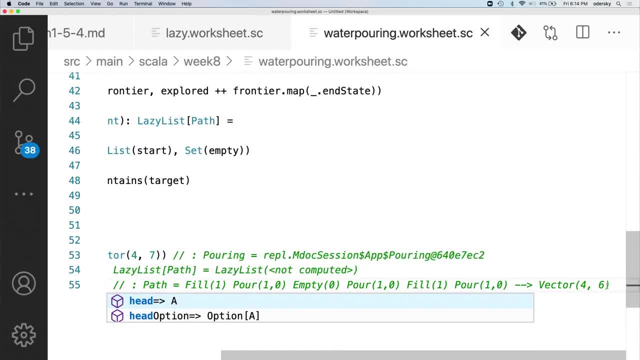 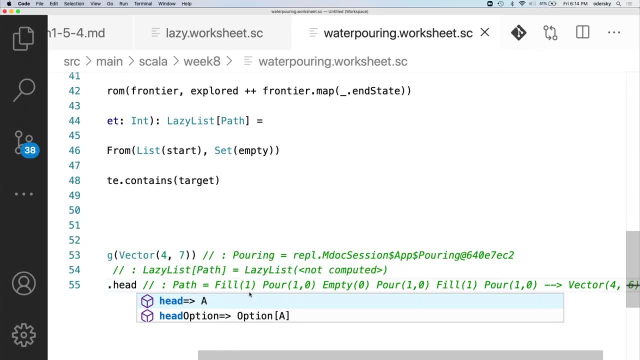 so here it is. it ends in the vector 4- 6, so one of the glasses has 6 in it. and here's the sequence of moves. we fill first the first glass, the one that, no, sorry, we fill the second glass, the one that contains 7 units. 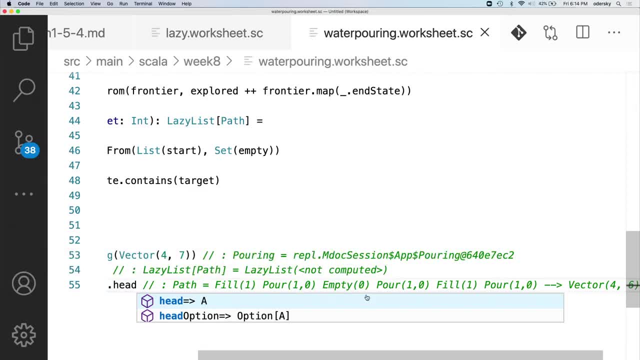 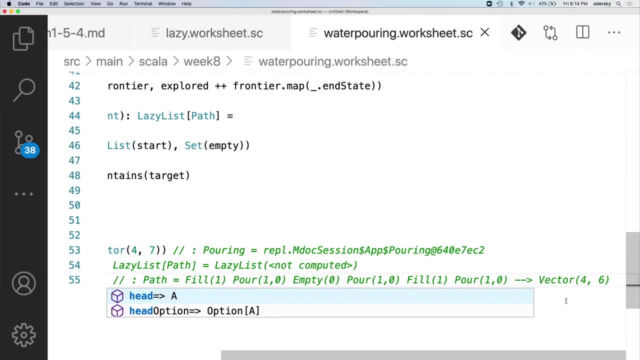 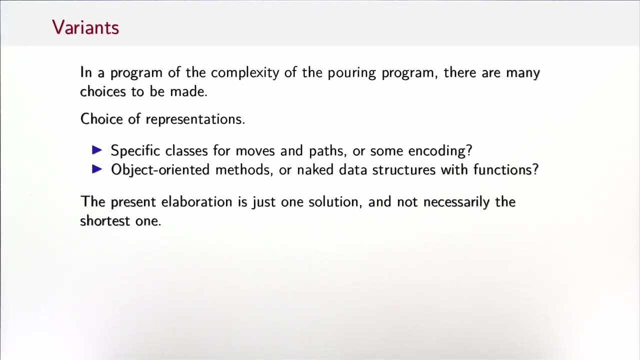 we pour from the second glass to the first, we empty the first, and so on. so I invite you to try it out and verify that we will indeed get the vector that it claims to get here at the end. so that was the solution to the water pouring problem. that was. 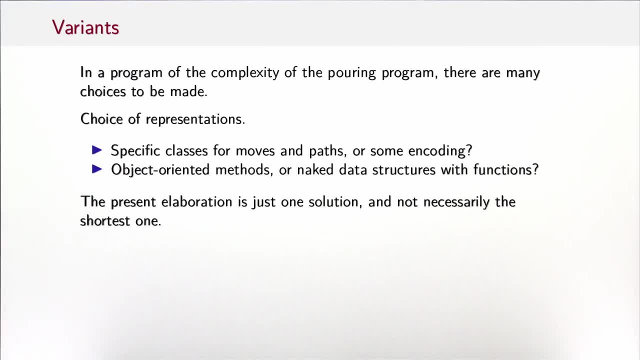 quite elegant and short and that made crucial use of lazy, infinite data structures to achieve that. of course, it's not the only possible solutions. there are many variants possible. we could, for instance, do a different choice of representations here. we define specific classes or enums for moves and paths. one could have also: 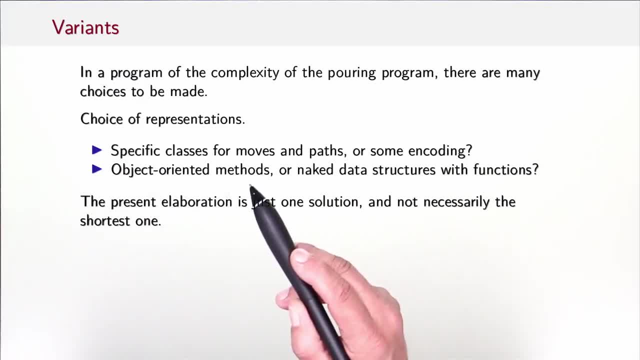 encoded them. we defined object oriented methods where it was natural. one could have also used naked data structures with functions. so the present elaboration is just one solution, not necessarily the shortest or most efficient ones, but it's reasonably short and reasonably efficient. some guiding principles for good design that. 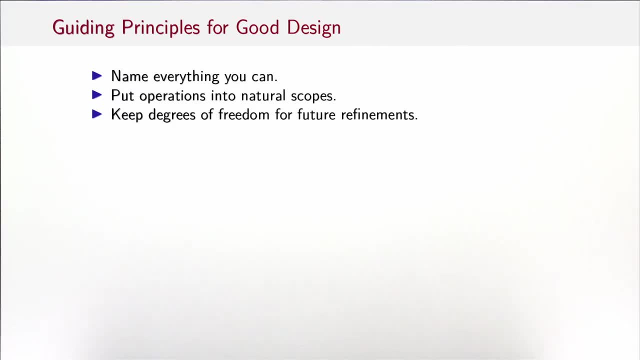 are employed implicitly everywhere one is. naming is really important. name everything you can avoid long expressions with lots of anonymous functions and things like that. so it's true that sometimes it's hard to come up with a good name, but it's definitely always worth the effort. so try to name. 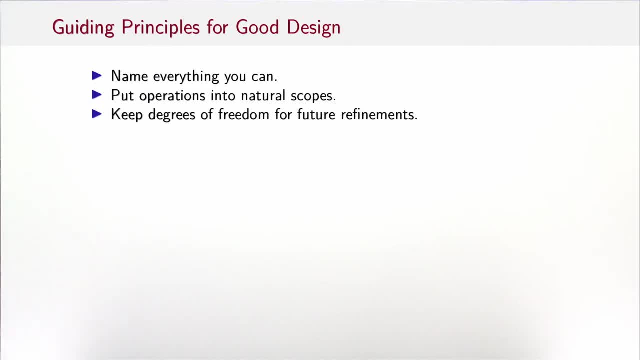 everything you can and try to find good names for the definitions that you have. the second observation is that scoping is important. you should put operations in the scope where they fit, naturally. and the third observation is essentially to come back to data abstraction. one should keep degrees of freedom. 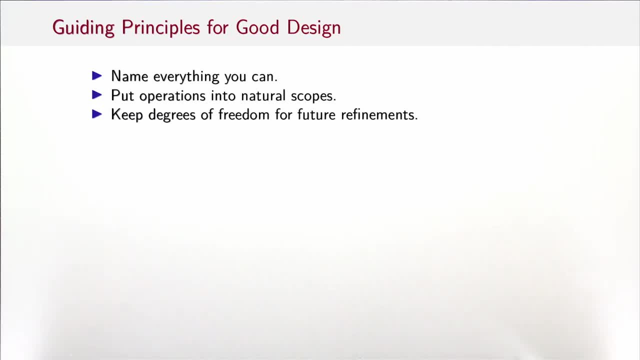 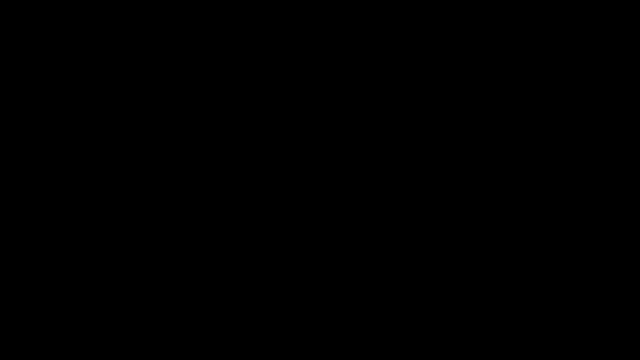 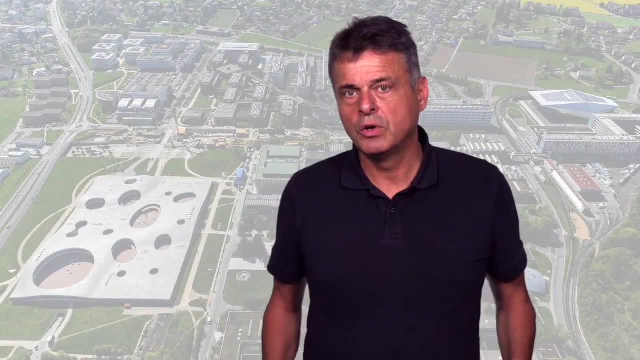 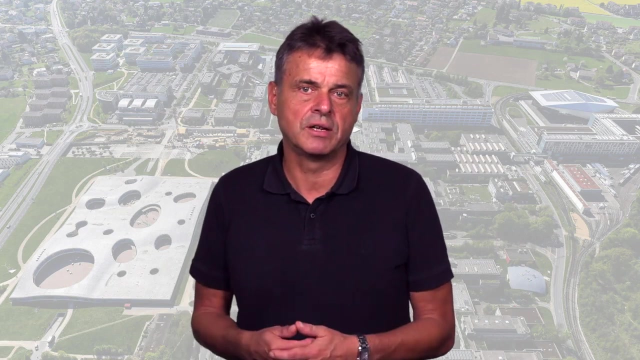 for future refinements. so the interface of a module should not be concerned with the implementation details in that module. by now you've gained quite a bit of experience with type inference, which lets you omit type parameters and type annotations. in many situations type inference comes down to the compiler filling in certain 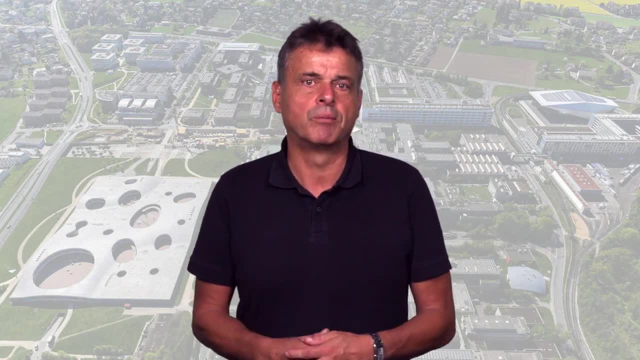 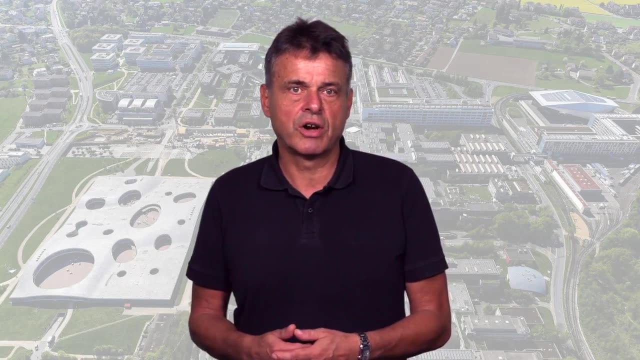 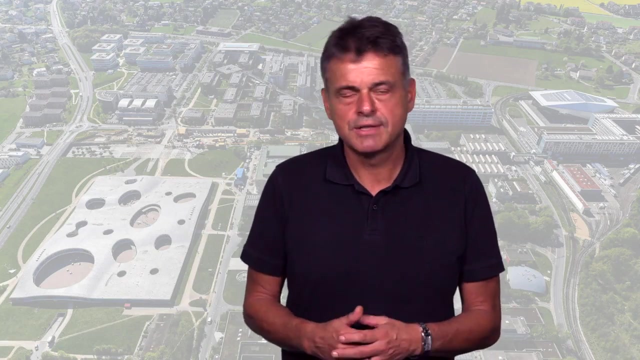 types from values or expressions that you as a programmer provide. typically, type parameters for a function are inferred from argument values to that function and result types of definitions are inferred from their right hand sides. in this week we'll cover the dual type inference, which is also very powerful. 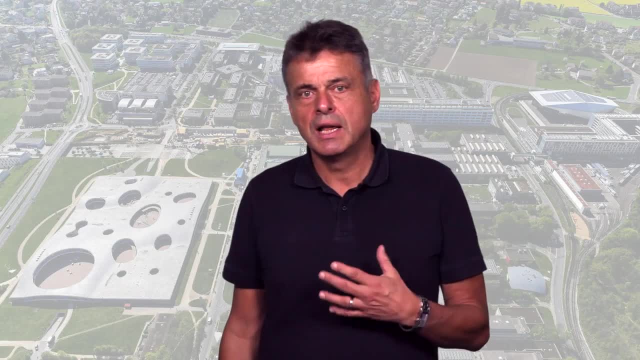 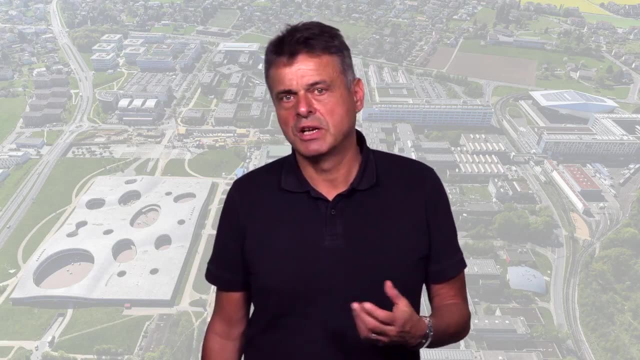 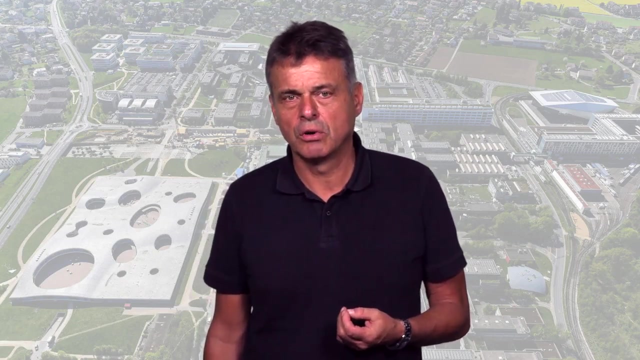 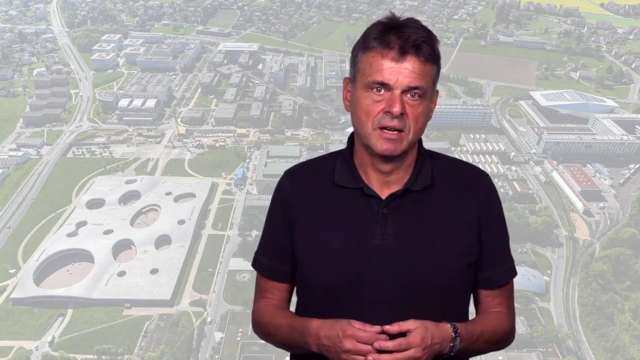 and useful term. inference means that the Scala compiler can, in certain situations, infer a value or expression from a type. values and expressions are also called terms, hence the name term inference. there are several cases where this is useful, and we covered two important ones this week. the first one is 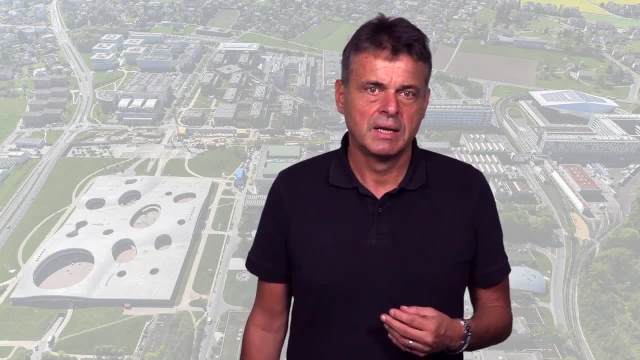 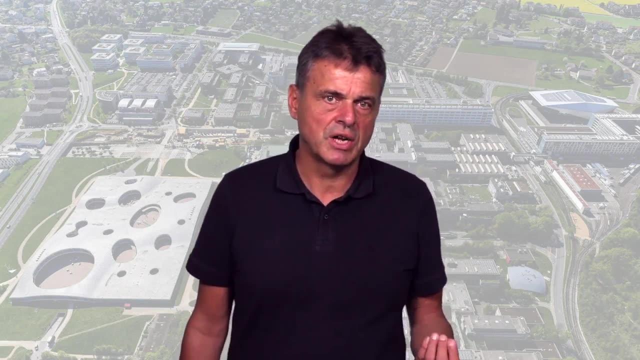 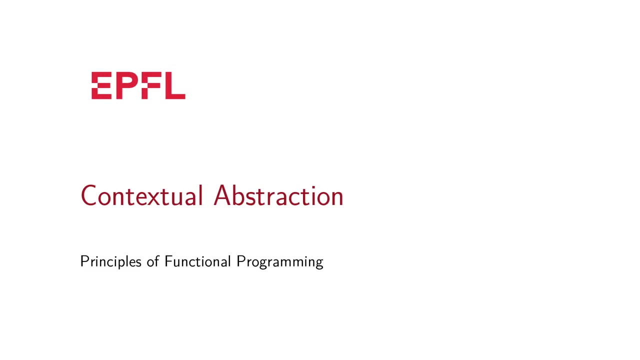 the type of the type which is generated by the compiler, knowing just the required types. second, this gives us a rather general way to pass contextual data from the points where it is generated to the points where it is accessed. in this session, we are going to talk about contextual abstraction. 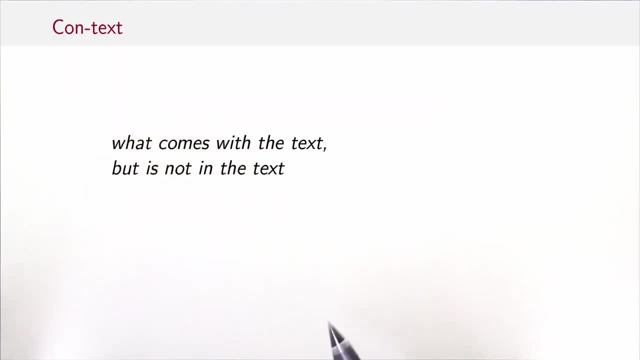 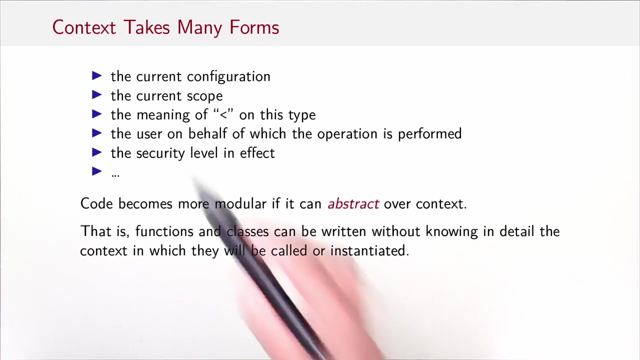 in a little bit. so if we look at the word context, it's formed from con, which means latin with, and text. so it means what comes with the text but is not in the text. so it's a very general concept which in fact comes in many forms. 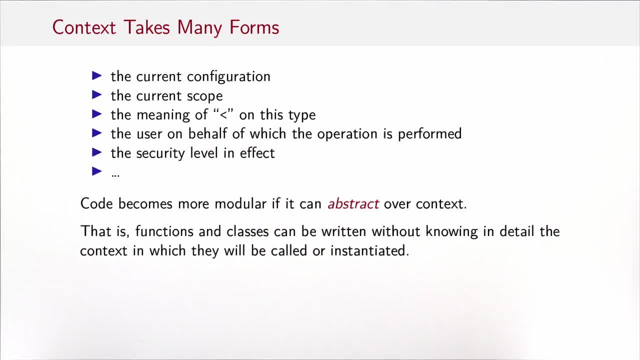 so context could mean the current configuration, which is the same everywhere, except maybe at some point you want to change it in some parts of your code, or the meaning of an operation, like less than on this type, or, going out further, the user on behalf of which an operation is performed. 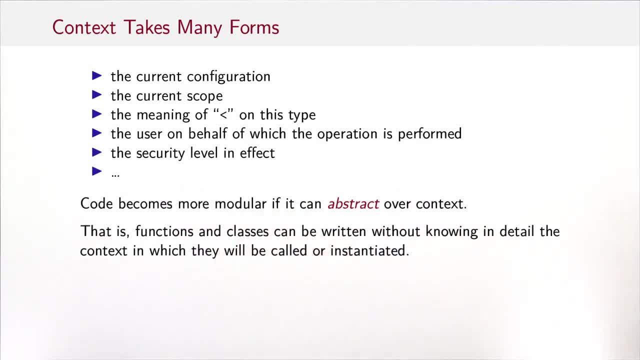 or the security level. in effect, it's really very general. it could mean many things. code becomes more modular if it can abstract over contexts. abstracting over context means that functions and classes can be written without knowing in detail the context in which they will be called and instantiated. 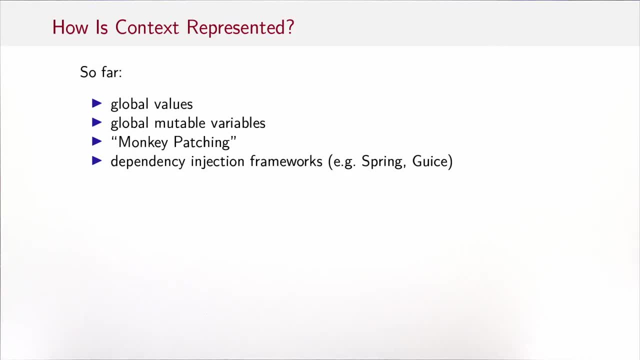 so how can we represent context in programming? there have been so far several techniques to do that, and they all have downsides. so what we can see is we can represent context as just global values accessible to the program, but that means we have no abstraction, and that's often too rigid. 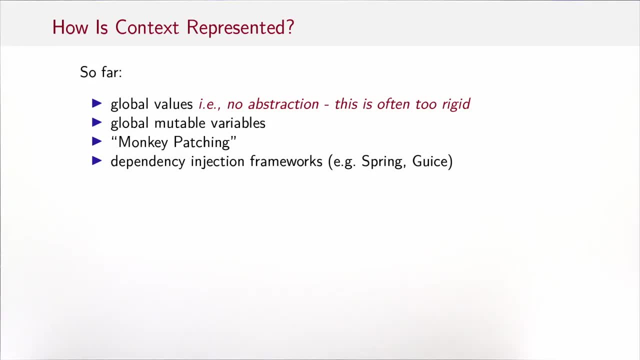 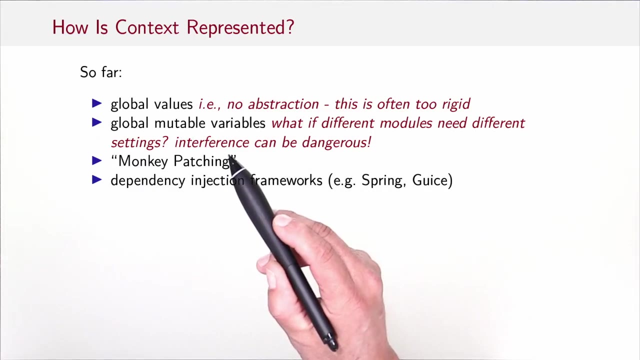 that means that global value is just known for everybody and we can't change it anywhere. so we might change that to global mutable variables that can be set according to the needs of various program parts. however, what if different modules need different settings? that could give you interference. 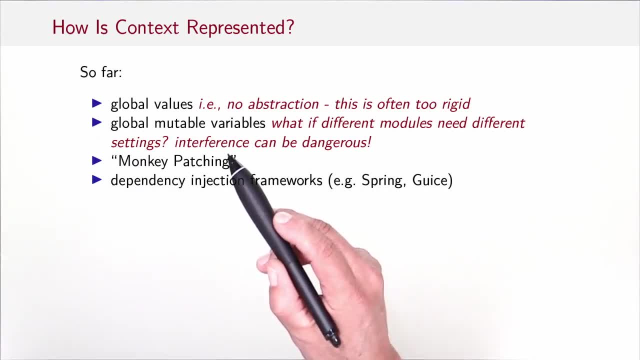 where you think you have one setting, but in fact somebody has changed the variable and you have a different one, and such interference can, of course, be very dangerous. some dynamically typed object-oriented languages have introduced a concept called monkey patching. what that means is something similar to global variables. 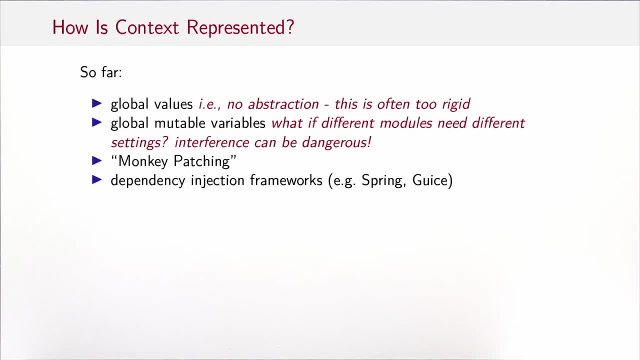 but instead of changing a global variable, you change the property of a root class, so, for instance, you might have the base class object and you add a new method to object that's visible for everyone, or you change the behavior of a method so that has a slightly more limited scope. 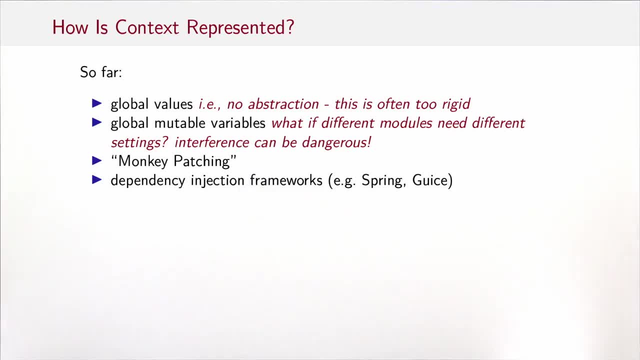 than globals, because it affects only classes inheriting that root class, but it's nevertheless. it's essentially just a more powerful way to shoot yourself in the foot. I think another solution is provided by programming frameworks. examples are spring or juice in the java world. these have sprung up because 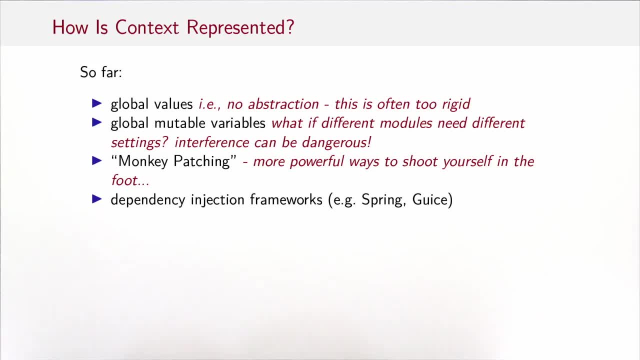 programming languages haven't offered out of the box solutions to the problem of how to abstract over contexts. what they do is they are outside the language and essentially rely on bytecode rewriting to add dependencies to programs. so that's powerful, but it also makes programs harder to understand. 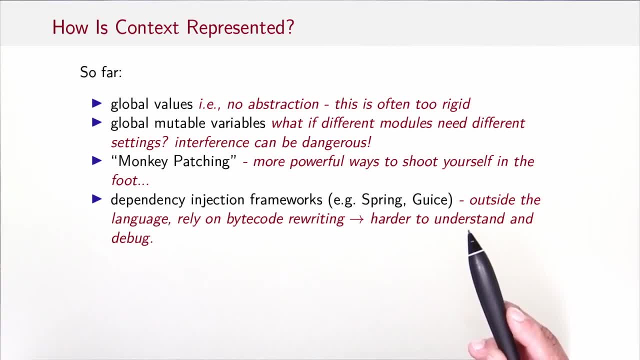 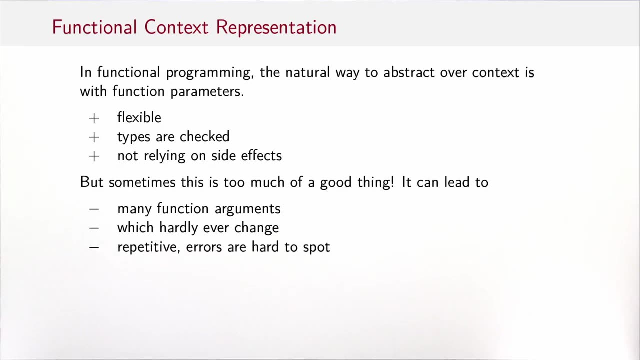 because now you have to understand the programming language and the bytecode rewriting framework, and it's, in particular, harder to debug because there's now a lot of code in your way that you haven't written yourself, but some framework has written. so all this was very imperative: what would be a functional way to represent? 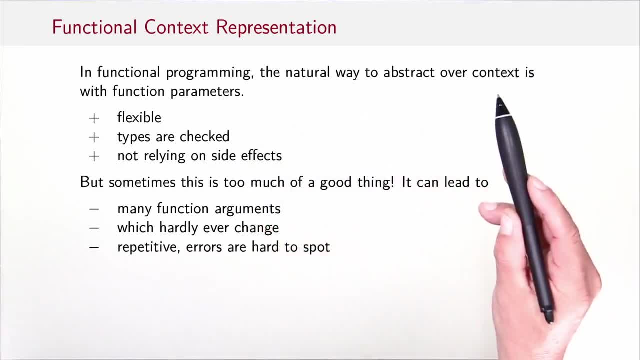 context. well, in functional programming, the natural way to abstract over context is with function parameters. so if you want to abstract over something that is known from the outside of a function, then make it a function parameter. that's, of course, very flexible, type safe, since parameters have types. 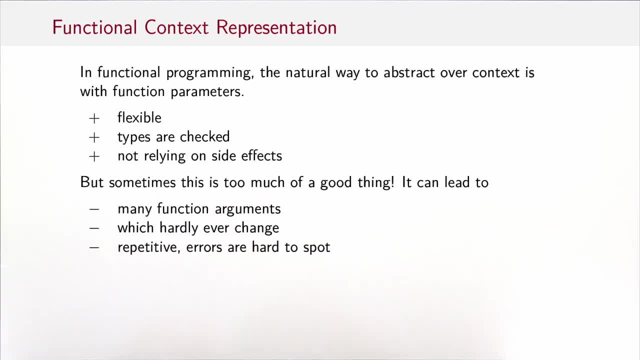 and the types are checked. your programs become safer. you can't have a type error when you read something from the context, and it's not relying on side effects, which is definitely a bonus. so why is not everybody doing that? well, sometimes this is too much of a good thing. 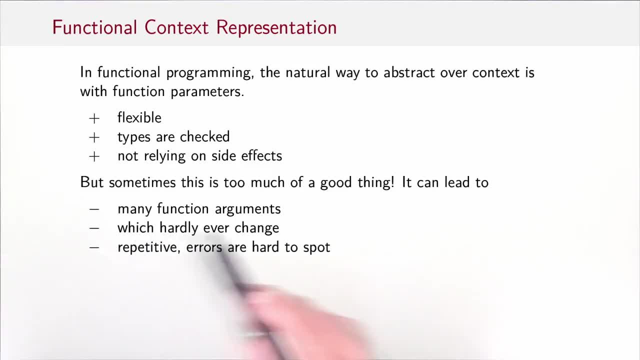 if you use that technique extensively, it can lead to many function arguments, and most of them are the same from one call to the next, so they hardly ever change, and this of course means your code will be very repetitive, and in all these repetitions, errors will be hard to spot. 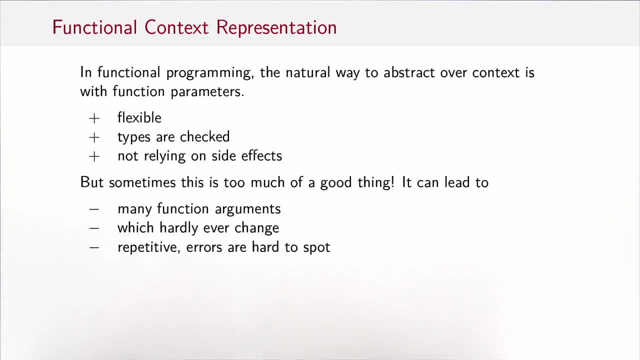 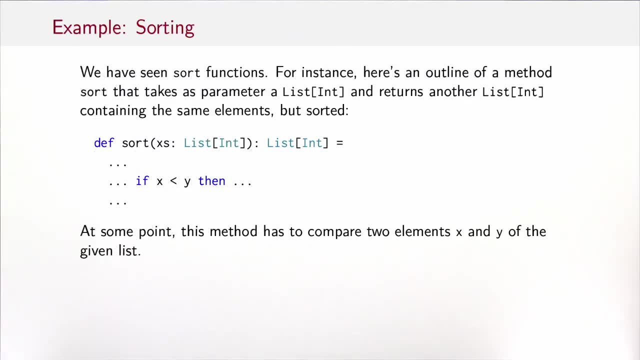 so that's the downside of essentially overdoing this functional parameter approach to context representation. but, as we will see, it has a solution in Scala. let's demonstrate the problem with an example. you've already seen sort functions, for instance. here is the outline of a method: sort. 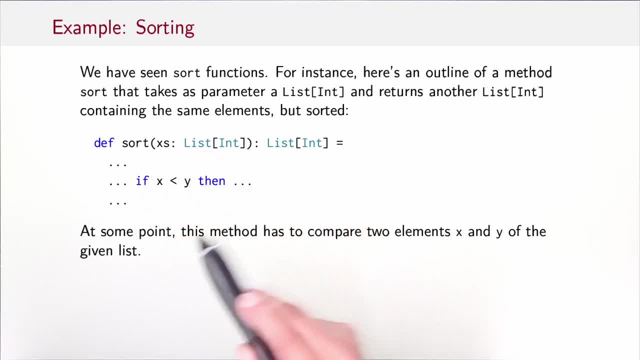 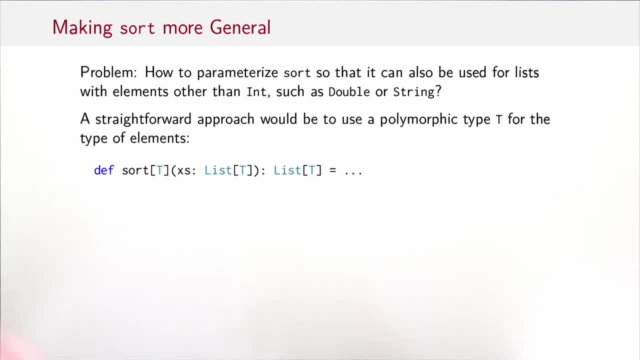 that takes as a parameter a list of ints, somewhere in the body of sort you would find a comparison of two list elements. so if x less than y, something like that. now, that worked for list of ints, but of course we want a more general sort that works for lists of arbitrary types. 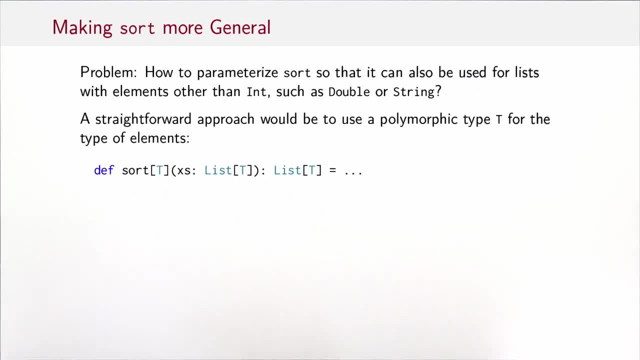 so here it is. that's a sort function which now takes a type parameter. but this does not work because there is not a single comparison method. less than that works for all types t. so if you would write less than here, you would get a type error which said that the type parameter t. 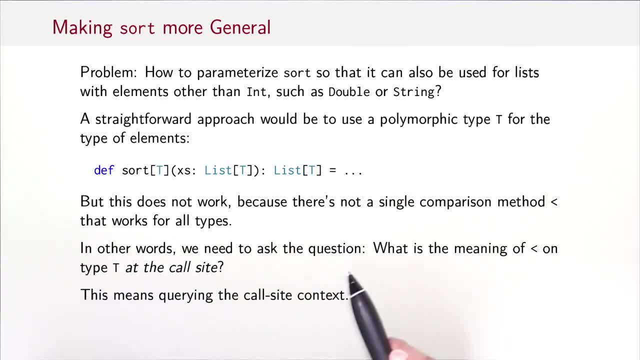 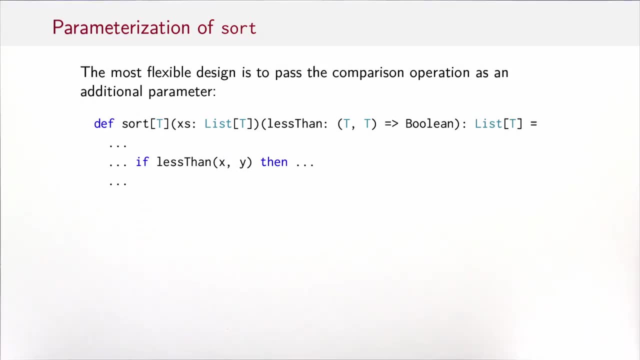 doesn't have a less than method. in other words, we need to ask the question: what is the meaning of less than on type t, so the actual instance of type t at the call site? and this means we need to query the call site context. so let's apply our strategy. 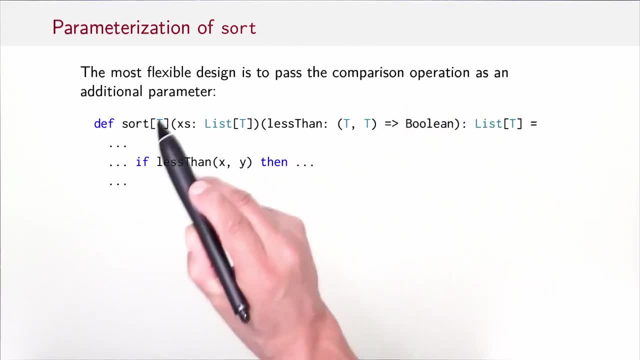 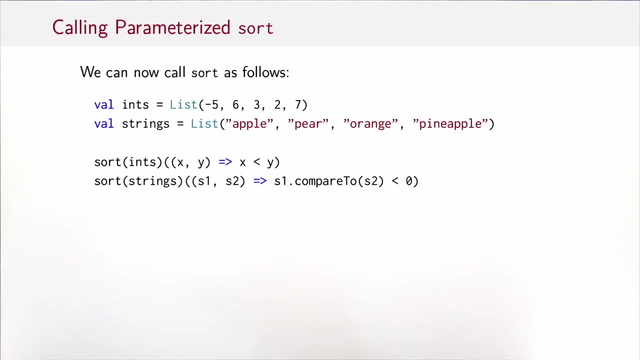 to represent context as parameters. that's the most flexible design. as an additional parameter, so sort would now take a list and a less than method which compares to element of type t, and instead of having the less method directly, we write less than xy. that works. we can now call sort as follows: 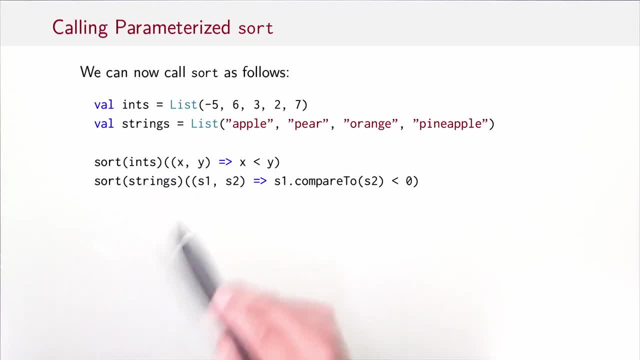 so let's say we have a list of ints and a list of strings like that. then we would write: sort ints with the less than method, which is integer comparison here, and sort strings with the less than method to less than zero here. so in each case we have passed. 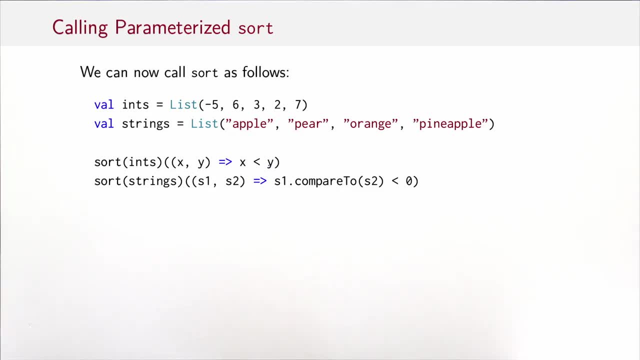 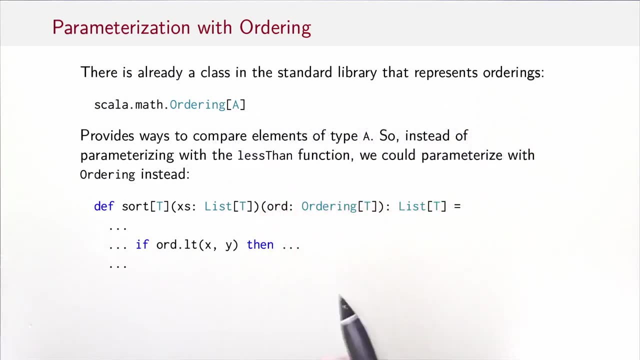 the appropriate method to compare the elements of the list. in fact, there's already a class in the standard library that represents orderings with less than methods, and also less than or equal, greater and so on. it's called scalar math ordering and it's parameterized by the type. 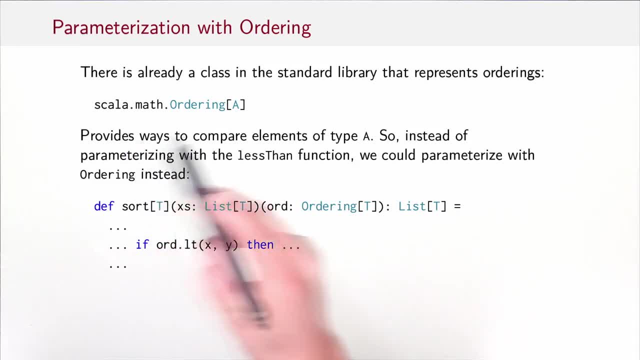 for which the ordering is defined. so that method provides ways to compare elements of type a, which means that instead of parameterizing with the less than function, we could parameterize with ordering instead. so that's what this would look like: we would have the sort method and it takes an ordering of t. 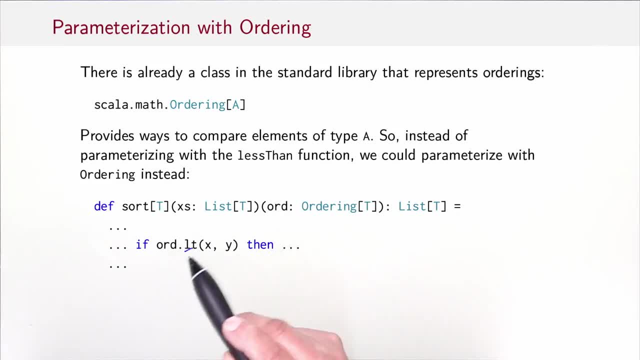 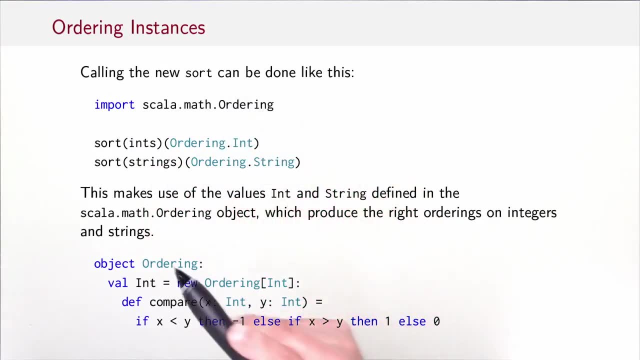 and then instead of less than, we would write orglt, which is essentially the less than method defined in that ordering and calling the new sort method would look like this: we would import scalar math ordering and then we sort the integers list with the integer ordering, orderingint and the strings list. 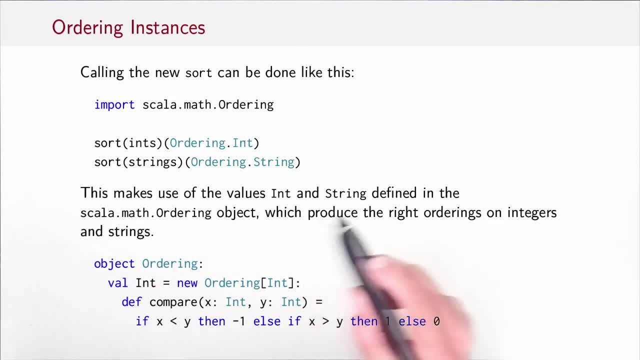 with orderingstring that makes use of the values int and string in the ordering object, which define the orderings for the types int and string respectively. so, for instance, here would be the int value in the ordering object, so it's an ordering for int and what we have to do is we have to define a. 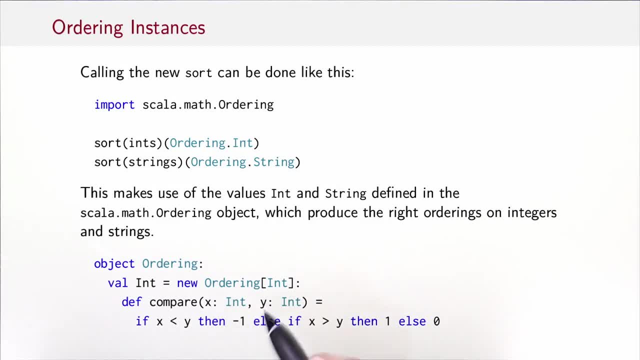 compare method that will give us back: minus one if x is less than y, plus one if x is greater than y and zero if there equal. so it would have the typical compare method for integers and then the lt and the other less than greater than comparison methods would all be defined. 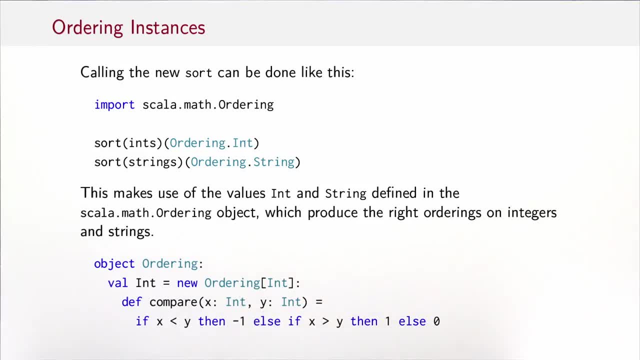 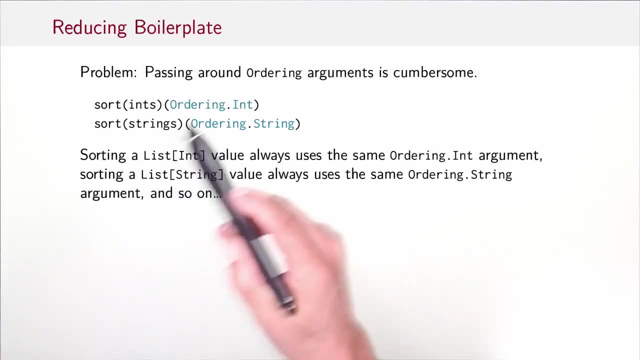 in the class ordering in terms of compare, and of course the orderingstring would be defined analogously. so this works. but there's a problem, namely that passing around these ordering arguments is quite cumbersome. so sort ints: ordering of int. sort strings: ordering of strings looks heavy and you could. 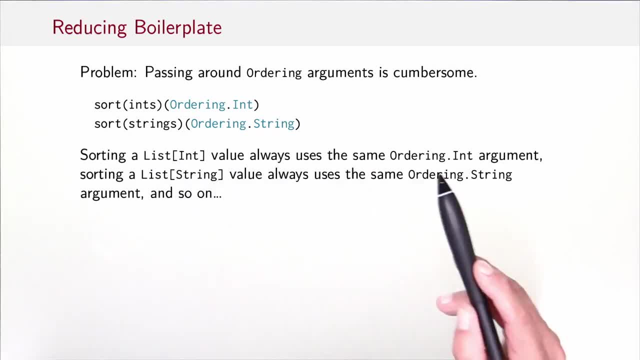 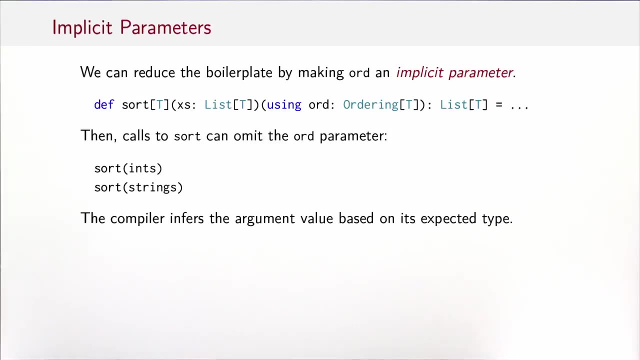 argue that sorting a list of int value should always use the same ordering int as an argument, where sort list of string value should always use ordering of string. so why make it mandatory to add these things? can't the compiler figure that out? and in fact we can let the compiler. 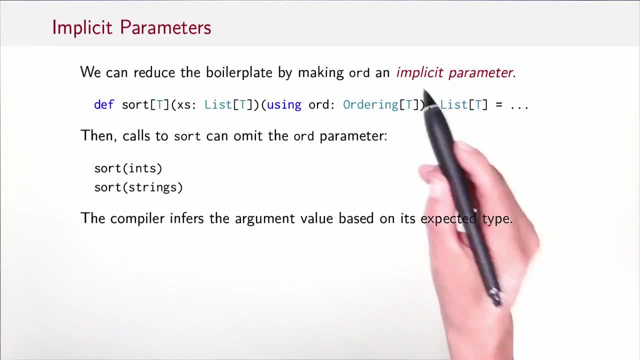 infer that and reduce the boilerplate by making ort an implicit parameter. we make it an implicit parameter just by prefixing it with the keyword using, as you see here. so now ort is an implicit parameter, which means that the compiler can synthesize the correct arguments that match the ort parameter. 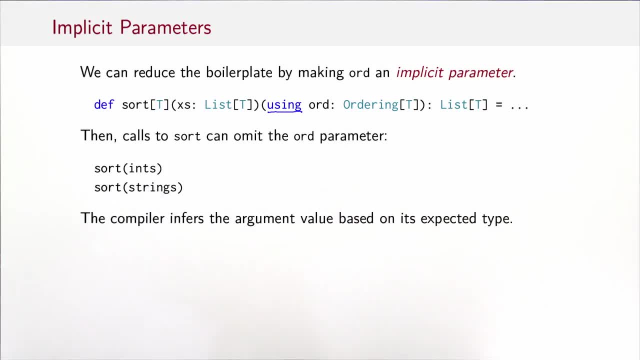 so you can omit the parameter and just write sort of ints and the compiler will figure out it needs an ordering dot int argument here. or you can write sort of strings and the compiler will supply an ordering dot string. so in general the compiler infers the argument value. 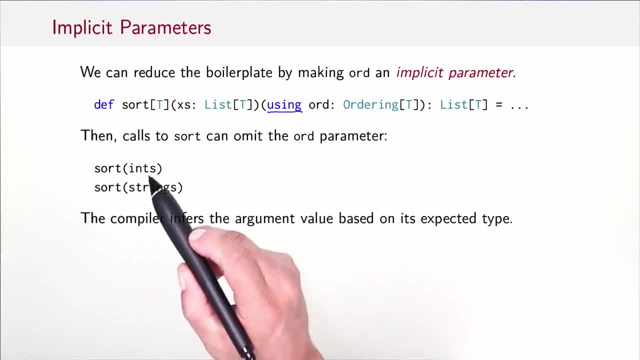 based on its expected type. and of course, here you know, the compiler knows at this point that since you sort a list of ints, you need an ordering of type int and here it needs an ordering of type string. so the expected type is known and with that expected type, 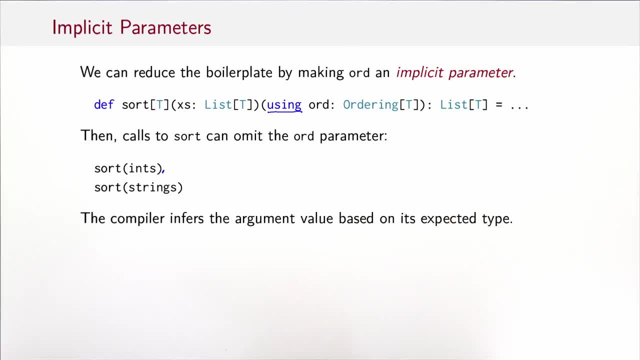 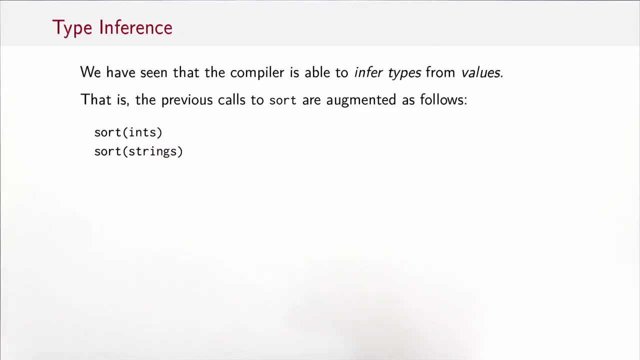 you tell the compiler to figure out what the right argument value here is. so what happens? there is, in a sense, the dual of type inference. type inference is when the compiler infers types from values, for instance in the previous calls to sort that. we see here what the compiler 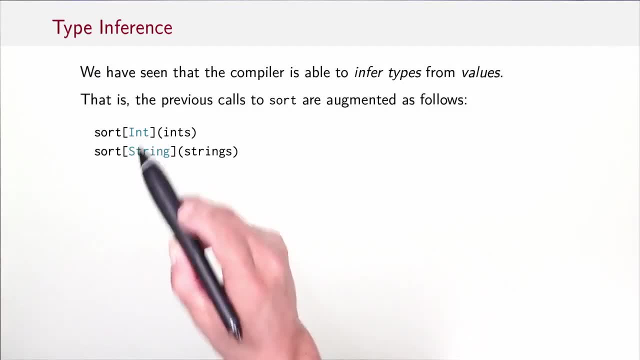 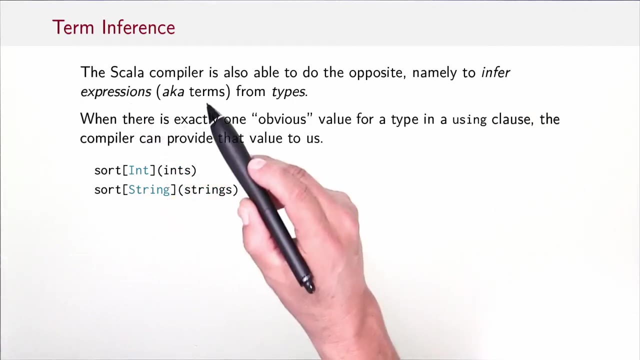 really does. it supplies the type parameter- int in the first case and string in the second case- and that it infers from the type of the actual values that get passed to sort. but the Scala compiler is also able to do the opposite, namely to infer expressions which we 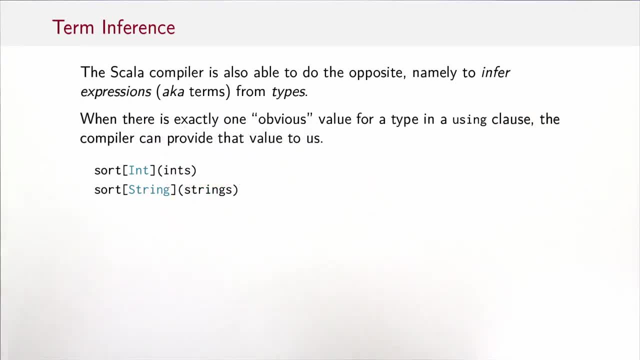 sometimes call terms from types and so consequently this is called term inference. when there is exactly one obvious value for a type in a using clause, the compiler can provide that value to us. so it will further go and say: well, sort int ints will actually be augmented with the argument. 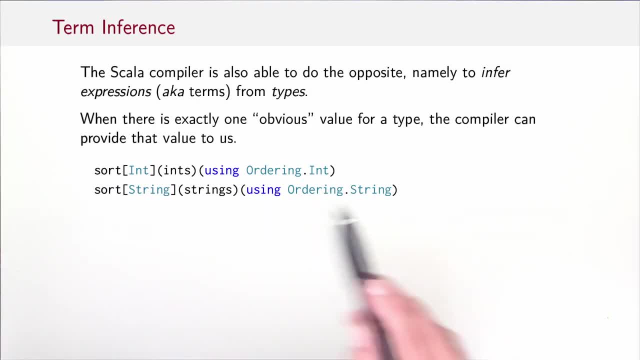 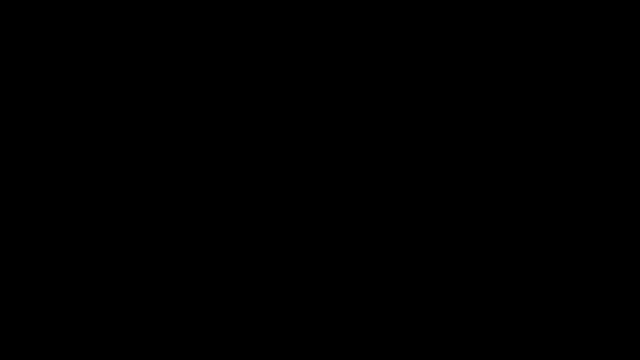 ordering dot int and sort string strings will be augmented with the argument ordering dot string. so this looks very useful and at the moment it also looks a little bit like magic. so in the following sessions we will explain the precise rules for this to happen. in this session we will explain the magic. 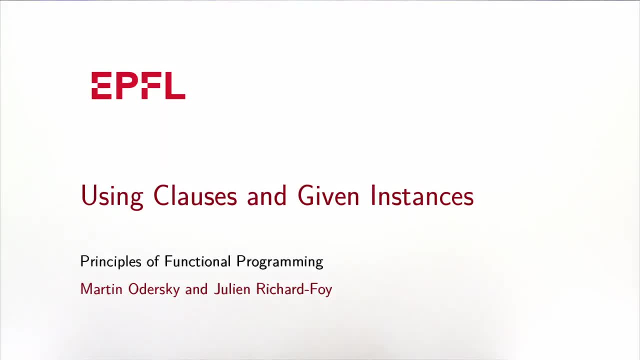 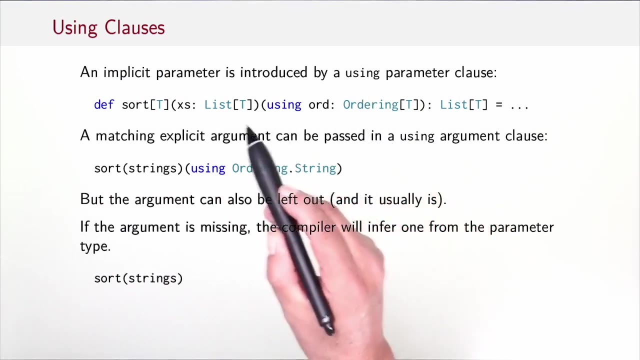 I alluded to in the last session, where the compiler could infer a value for a type. it comes down to using clauses and given instances, so an implicit parameter is introduced by a using parameter clause. that is the one you have seen using, or ordering of t if we have a parameter clause. 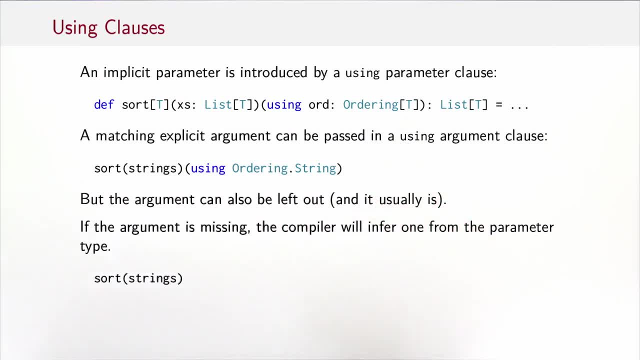 like that. we can pass a matching explicit argument- that is the one you have seen using- or ordering of t in a using argument clause. so you repeat, using again: you write sort strings using ordering of string and that would match up with this parameter. but the point is that arguments 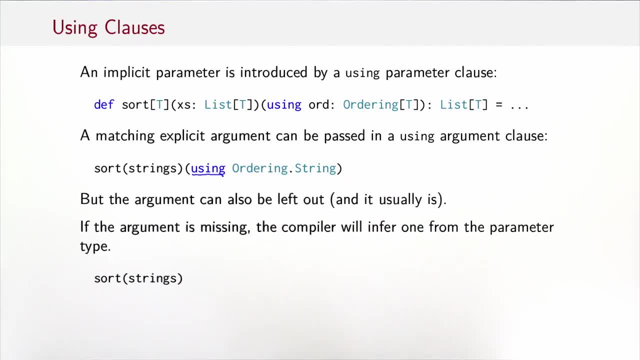 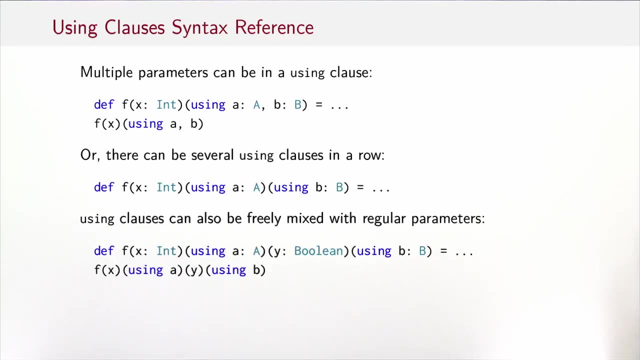 for implicit parameters can also be left out, and they usually are. if the argument is missing, the compiler will infer one from the parameter type, so sort of strings will become sort of strings using ordering of string. here are some variations of using clauses. you can have multiple parameters. 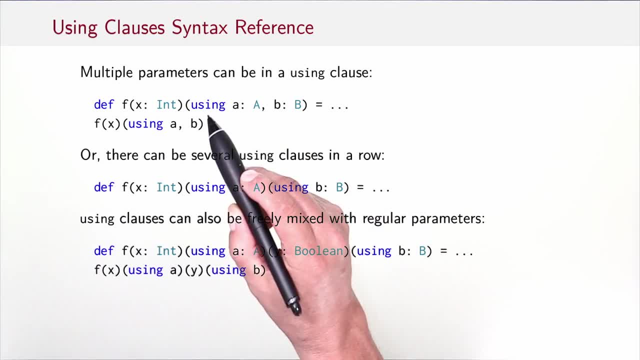 in a using clause, but then you write the keyword using only once at the front of them all. analogously, you can also have multiple arguments with a single using in the front, or you can have several using clauses in a row. so, for instance, you could have a using clause for a here. 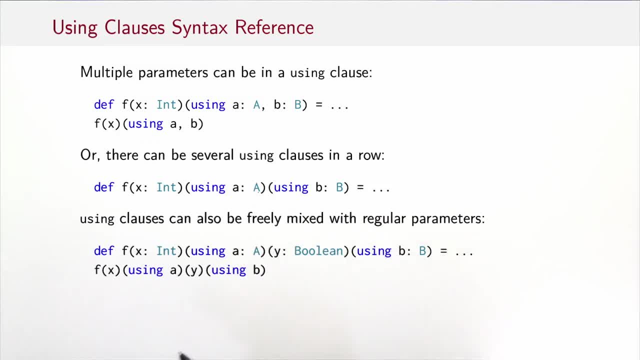 followed by a using clause for b, or you can mix using clauses freely with regular parameters. so here you would have a case f, where you have a regular parameter x, a regular parameter y, a using clause b, and if you pass arguments explicitly, then they follow exactly that pattern. 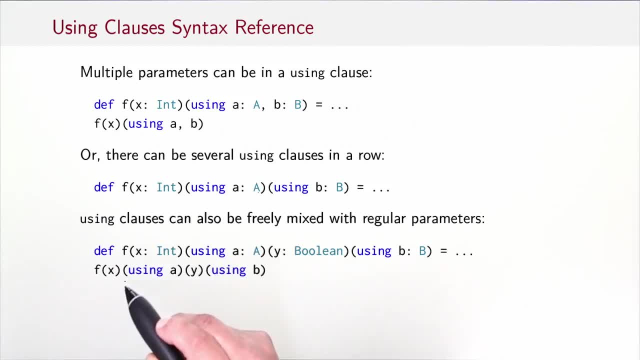 x using a, y using b, but this one here or this one here can also be left out. you might ask if I have two using clauses that follow each other and then I write a single using argument clause, like as in this using y, which one will be matched? 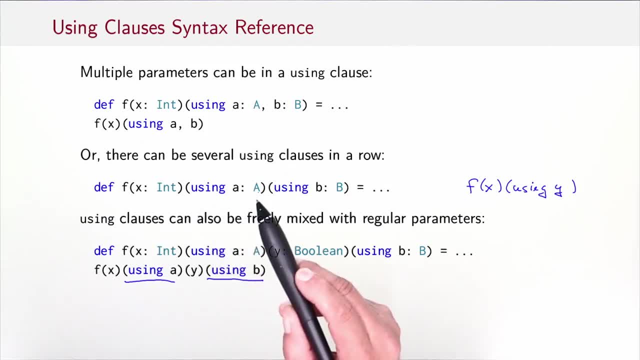 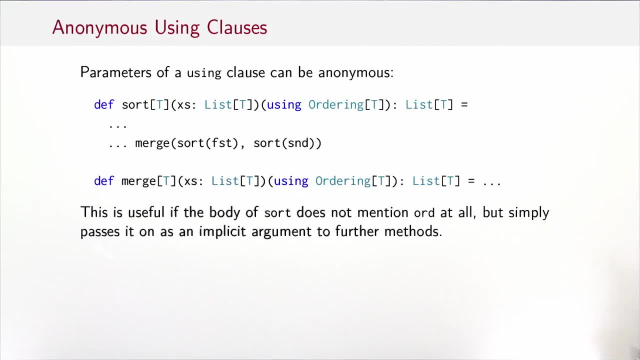 and the answer is: it's the first one. you fill in using clauses from the left, and if there are no using argument clauses left, then the rest will be inferred by the compiler. parameters of a using clause can also be anonymous. you could write just using ordering of t. 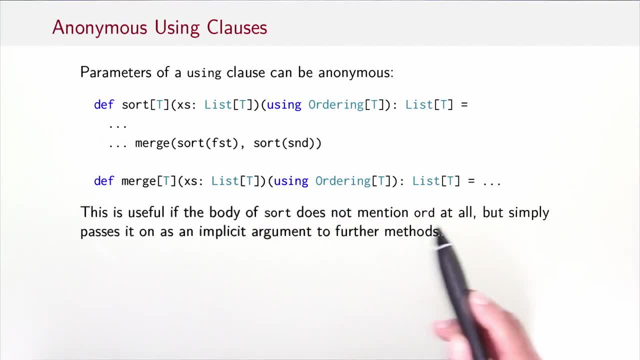 and leave out the ord parameter. that's useful if the body of sort does not mention ord at all, but simply passes it on as an implicit argument to further methods. you see the situation here where the only use of the ord parameter is to pass it on to the merge method. 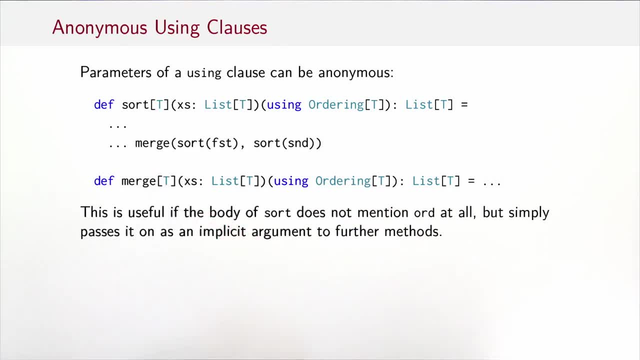 that does. the actual comparisons code that you see here is analogous to the following code, where the parameter names are put back and the arguments are made explicit. so here everything is named and I pass ord explicitly, and here the parameters are anonymous and the implicit argument is inferred. 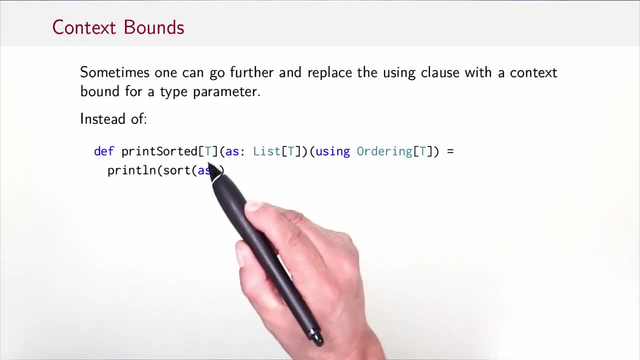 so this pattern where you have a type parameter, t, and then a using clause that uses t like ordering, is actually quite common. so this syntax colon ordering is called a context bound, in analogy to an upper bound or a lower bound, which you know already. so instead of having, let's say, an upper bound for t, 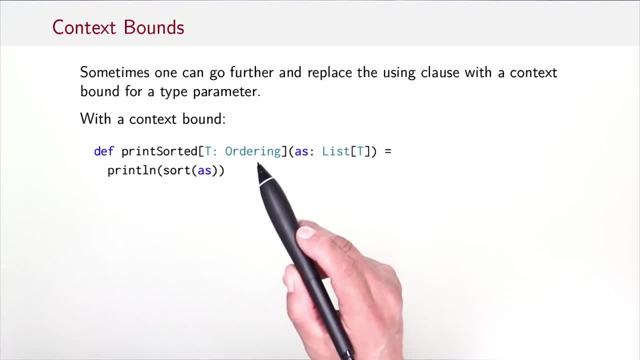 we have essentially a constraint that says there must be an instance for ordering that is defined on t, and that's another form of bound which is called context bound because it refers to the situation at the call site of the print sorted method in this case. so, more generally, a method definition. 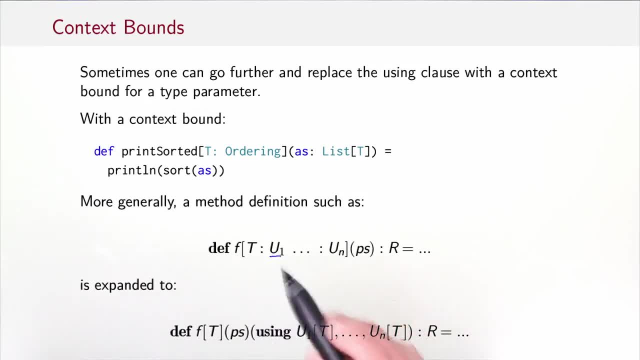 such as this one here, where t is followed by a number of types, each following a colon, would be expanded to just a simple type parameter, t, and then for each of these types, here you have a using parameter, an implicit parameter: u1 of t up to un of t. 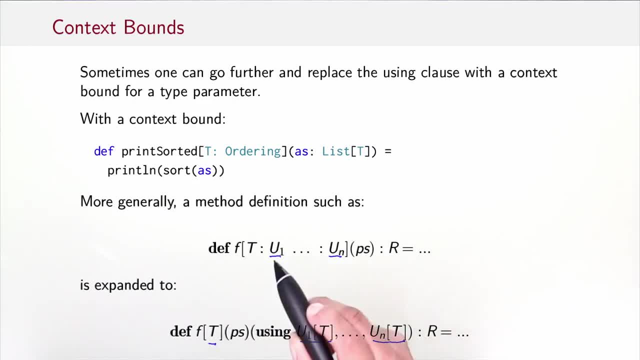 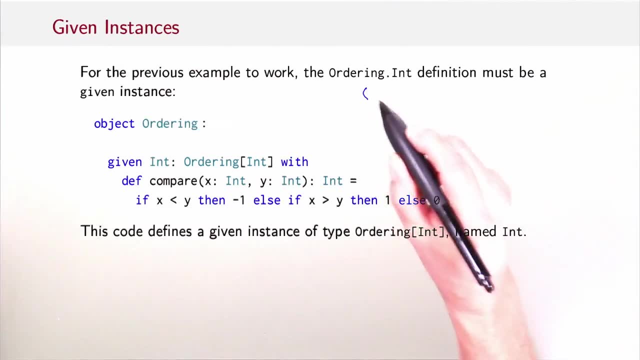 so the t gets repeated each time in the argument of these type constructors u1 to un. so we've seen previously that a parameter in a using clause, such as using ordering of int, gets instantiated with an ordering of int value. for this to work, that ordering of int must be. 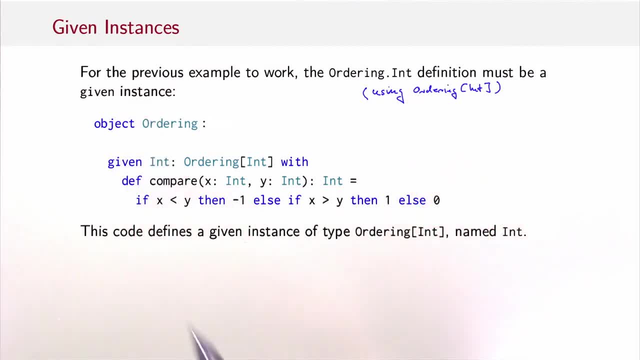 defined as a given instance. so you see here the given instance for that value, int is written. given int its name, then the type it implements- that's ordering of int- and then the methods that need to be implemented for an instance of that type. in our case, ordering of was a trait. 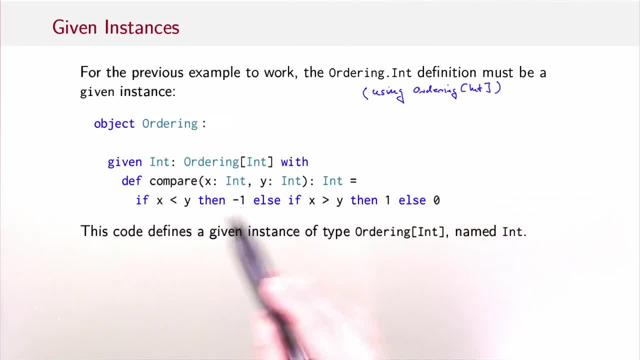 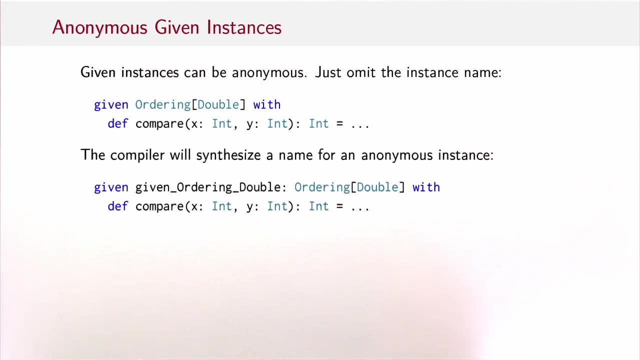 that had a compare method that gets implemented here in the given instance so that code defines a given instance of type ordering of int named int. given instances can also be defined as an anonymous instance. you can just omit the instance name. an example you see here to define an anonymous instance. 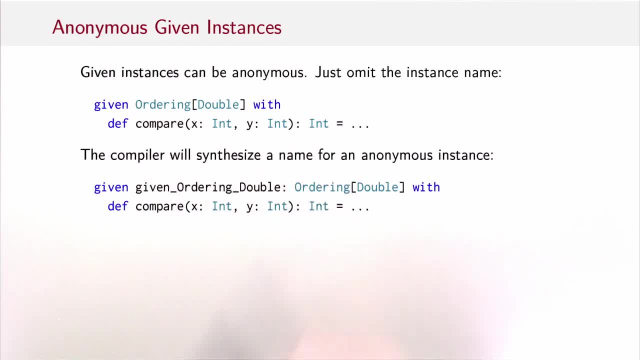 of type: ordering of double. you just write given, ordering of double and then the definition of compare for that type. you can leave out the name for the given instance. in that case the compiler will synthesize a name here. you see it, the name would read here the same as what you have defined. 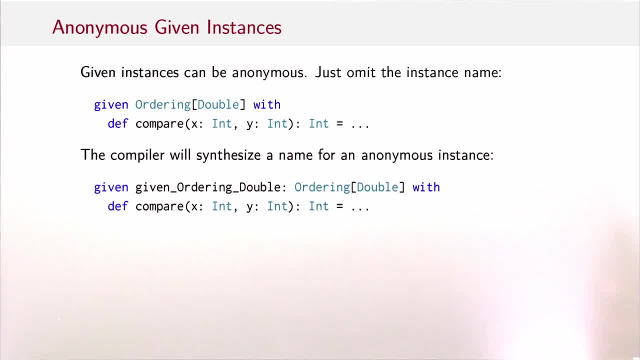 anonymous givens are nice because they're concise and concentrate on what's most important, namely what type do you implement? the name usually doesn't matter to the same degree. sometimes you might find that two given instances give you a name clash because the generated name is the same. 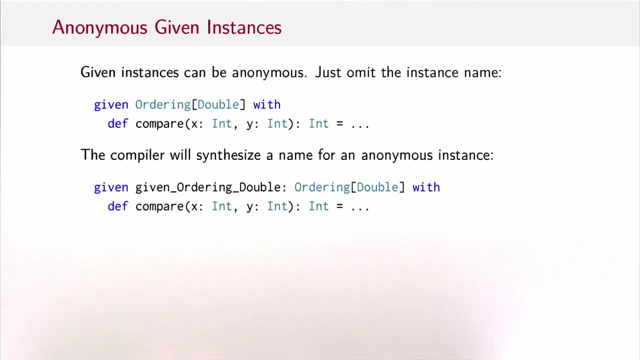 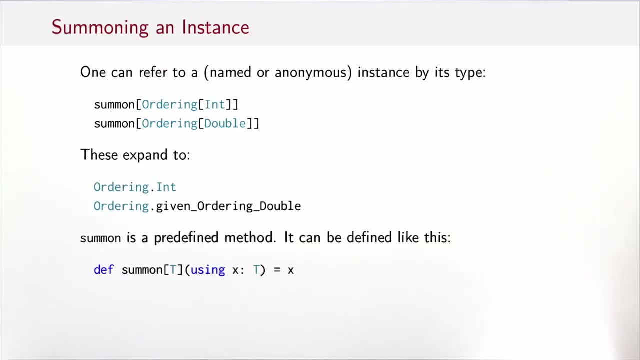 essentially, the two types were too close to each other, they led to the same generated name in that case, basically, you just fall back to the given instances. to avoid the clash, we can summon an instance, which means we can refer to the instance, whether it's named or anonymous, by its type. 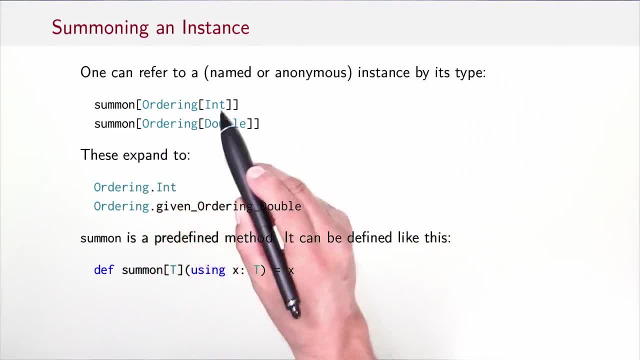 that's done with the summon method. so summon followed by a type will create the value, the instance that is the given instance for that type. summon ordering of int would expand to ordering of int. that's the given instance. or summon ordering of double would expand to ordering and then the name. 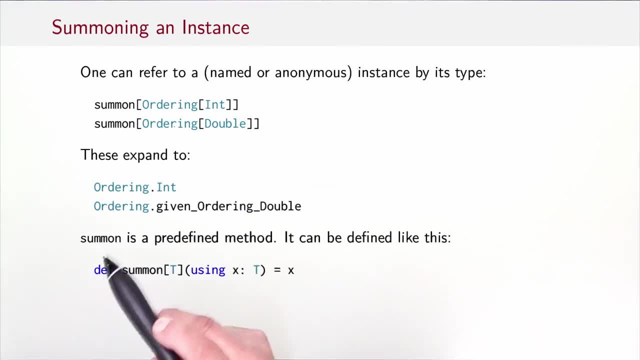 that the compiler has generated for this double ordering. so summon is a regular method. it's in the pre-dev object which is imported automatically into every Scala code. but it could also be defined like this. you could define: summon takes a type parameter t and an instance of type t. 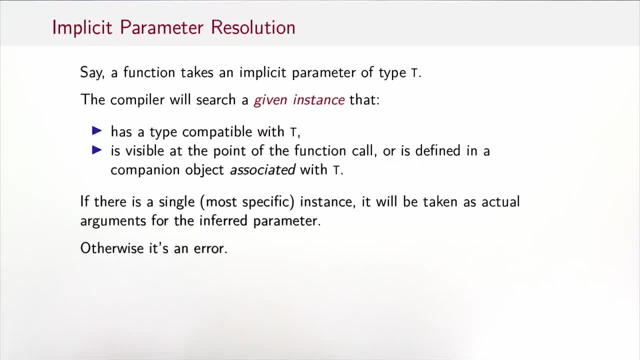 with a using clause and it simply returns the instance. that's all there is to summon. so now for the fine print. say you have a function that takes an implicit parameter and a corresponding argument. in that case the compiler will search a given instance that has a type which is compatible with t. 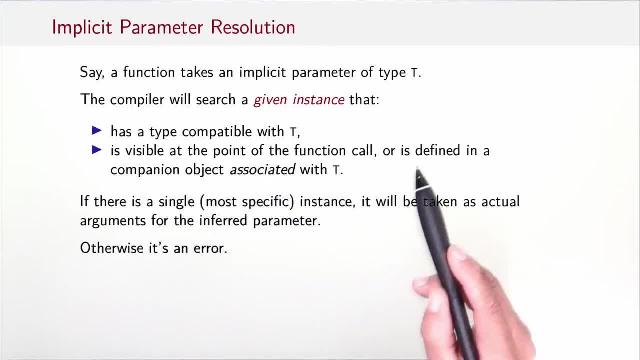 and that is visible at the point of the function call, or it is defined in a companion object associated with t. we'll get to that, what that means, in detail in the next slides. if there is a single such instance or a most specific instance, we'll get to that as well. 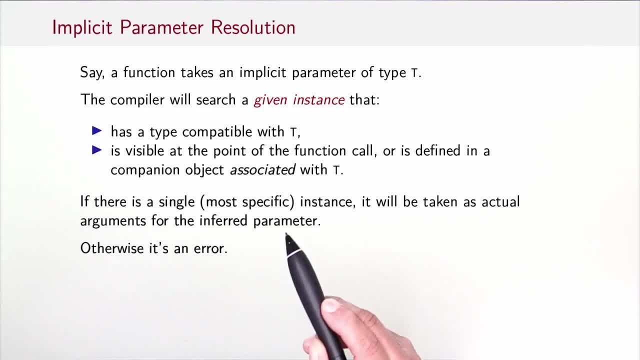 then that instance will be taken as a preferred parameter, and if there is not such an instance, it will be a type error. so what we still have to clarify is where exactly is the compiler looking for given instances, and how does it decide whether an instance is more specific than another? 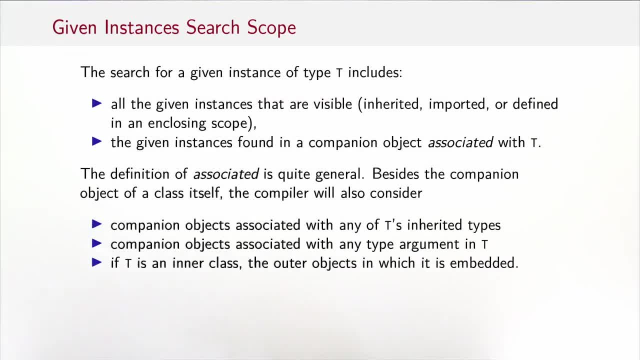 so these two points need to be clarified now. where does the compiler look for a given instance? the search for an instance includes all the instances that are visible at the point of call. visible means they could be defined by an enclosing scope or they could be inherited by an enclosing class. 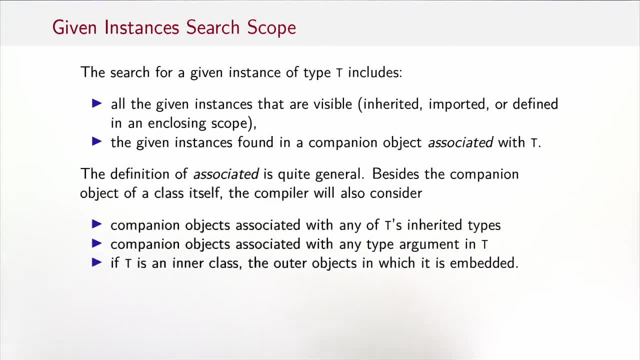 or they could be imported. if it doesn't find a given instance in the enclosing scope, it will also look at given instances in the companion objects that are associated for the query type t, and this definition of when a companion object is associated is actually quite general, so it means that if t is a class, 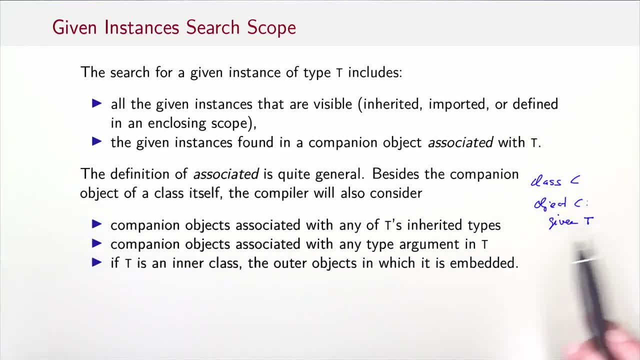 and the class has a companion object here, then a given instance in that companion object will be found, because the companion object is associated with the class type c. beyond that companion object of the class itself, the compiler will also look in the companion objects that are associated in any of t's inherited types. 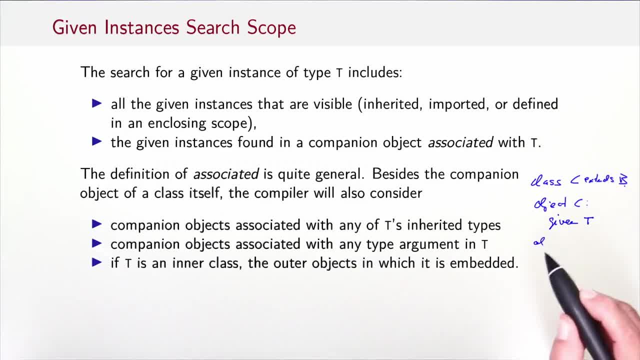 so if class t extends, let's say, a base class b, then it will also look in the companion object of b. then the companion object might be associated with any type argument of t. so it's not just the type as a whole but any part of a type. 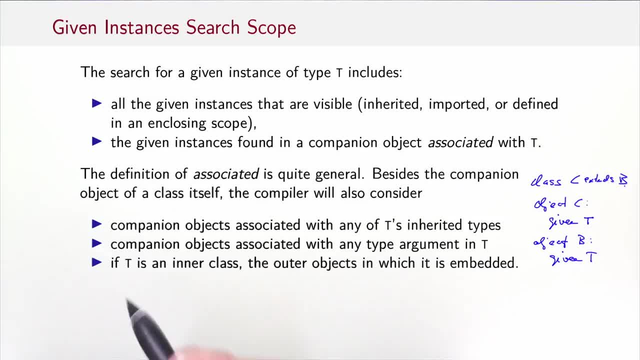 that gives can give rise to companion objects that are searched for given instances. or, finally, if t is an inner class, the outer objects in which it is embedded also contribute to the companion objects associated with t. so if we look at, let's say, we have an object o, 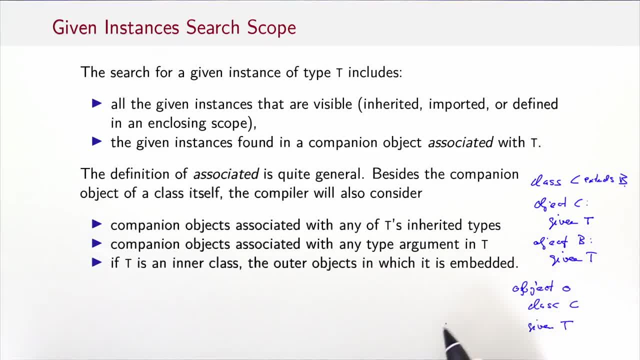 and a class c and we look for we need a given instance for the type oc. then that t here would be eligible because it's not a companion object of c but it's defined in an outer object. so in summary, basically every object that sort of can be reasonably. 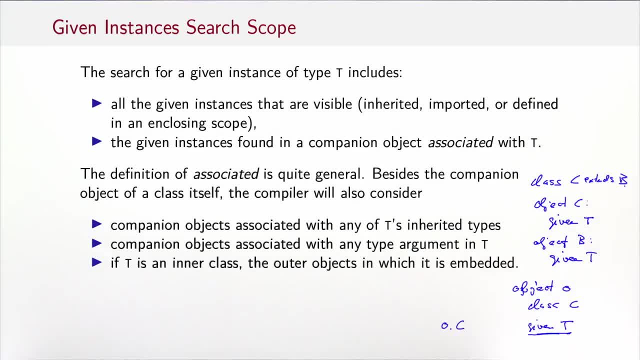 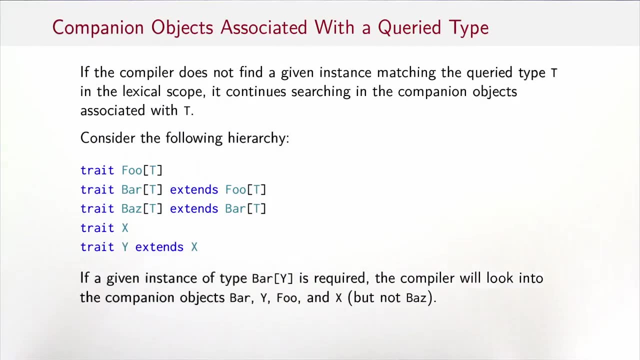 connected with the type t will be searched and that means that you don't need to worry too much where you put your given instances, as long as they have some connection with the type and it will be an associated companion and the given instance will be found. the search for given instances. 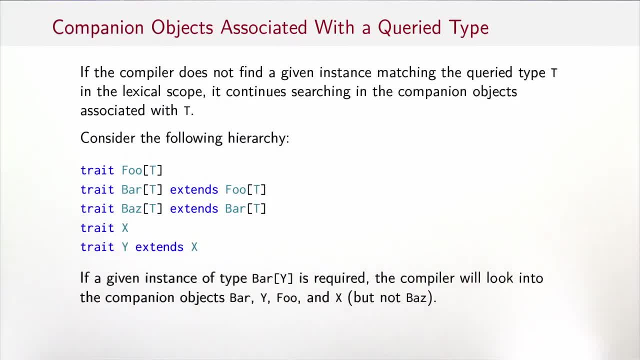 is done in two phases. it will first look in the lexically enclosing scope for something that's visible, and only if that fails it will look for companion objects associated with t. so here's an example. we have the class hierarchy that you see here and we want to know: 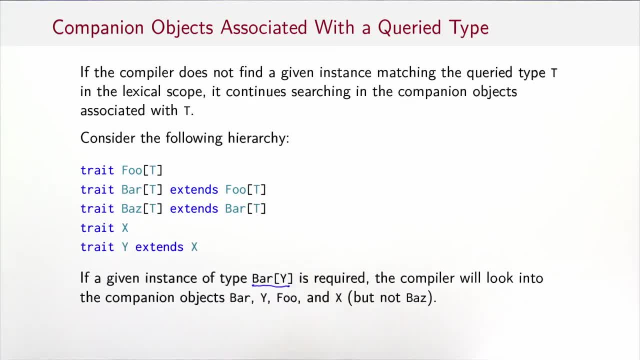 what are the companion objects associated with the type bar of y, so which companion objects would be searched for, given instances? in fact, in this case, the companion objects would be the companion object of bar, because, well, that's the class that you have here. the companion object of y. 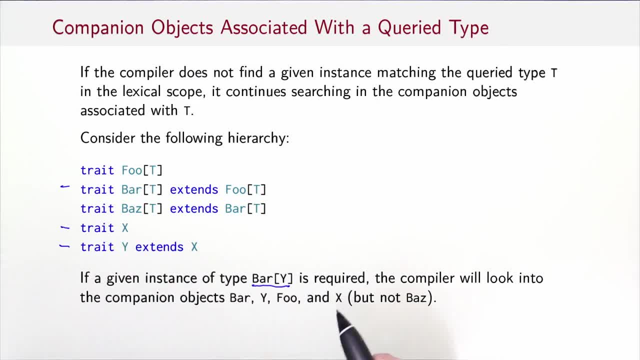 because that's a parameter of bar, companion object of x because that's a base type of y and the companion object of foo because that's a base type of bar. but bars of t doesn't count because it's not a companion object of a base type of either bar or y. 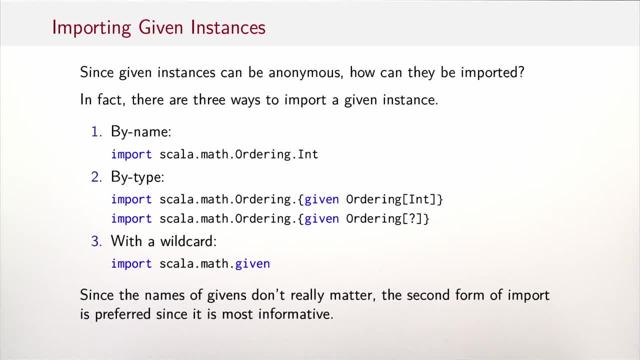 So I said, one way to make a given instance visible is to import it. But that raises a question. Given instances can be anonymous, so how can we import given instances that don't have a name? In fact, there are three ways to import a given instance. 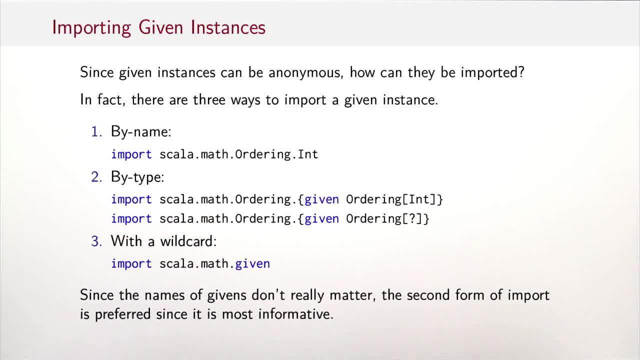 The first way is by name, so that's just the same as importing any other definition by name. For instance, ScalaMathOrderingint would import the given instance with the name int from the ScalaMathOrdering object. The second form is new and it applies only to given instances. 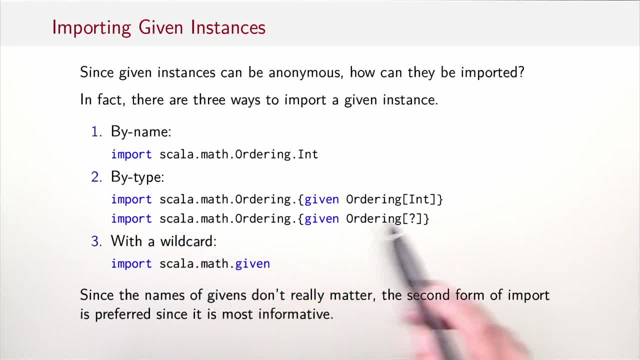 We can also import them by type. So for instance, here you see, we import ScalaMathOrdering and then we write: given ordering of int embraces. What that does is that it will import the given instance in that object that implements ordering at type int, so that it is a given instance of that type. 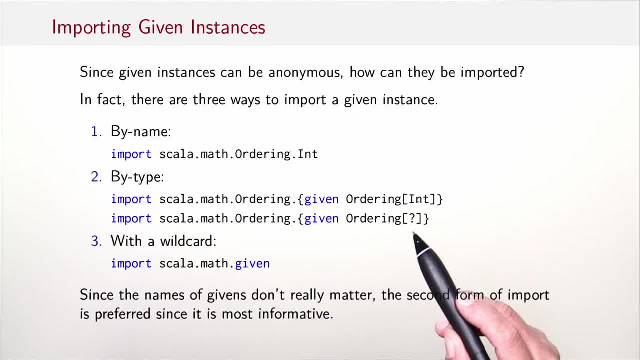 And we can also be more general. Instead of having a particular argument, like int, we can also have a question mark, which is a wildcard. So here we can. there's the second import would import any given instance that implements an ordering object of an arbitrary type. 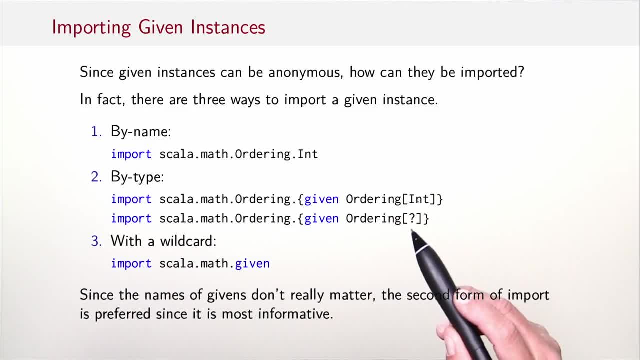 So it would import the ordering of int and the ordering of boolean and the ordering of double and any other orderings that were in this ScalaMathOrdering object. And the third way to import a given instance. The third way to import a given instance is as a wildcard. 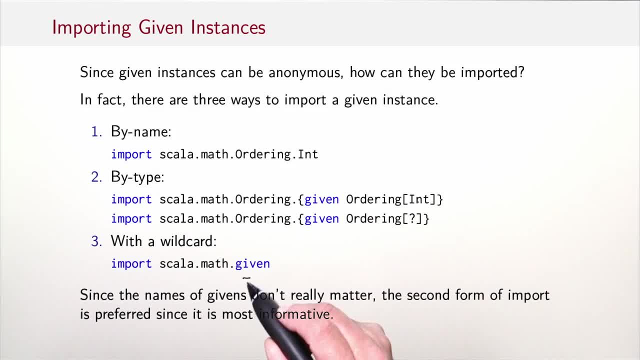 But the wildcard is different. Instead of using an underscore for a wildcard for normal values, we write given, And that makes it explicit that we in fact want the given instances, and only the given instances, from the ScalaMath objects, but not the normal values. 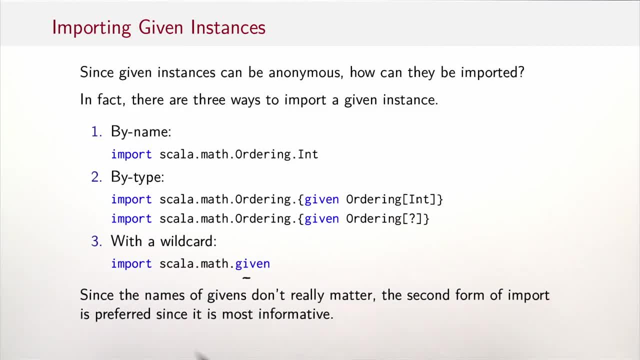 So which form of import should you use normally? Well, I would say, since the names of given don't really matter, use the second form. It's the most informative. It tells you exactly what you need. It tells you exactly what you want to know, namely that we get the given instances for. 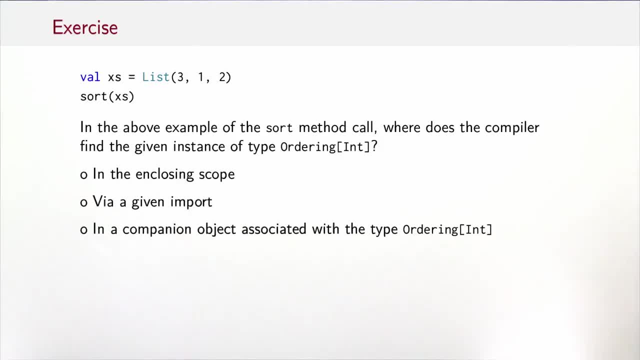 a specific type. So here's a little exercise. If you have this program here. so we define the list, we sort it with the sort method call that we've seen before. Where does the compiler, in this case, find the given instance of type? ordering of int. 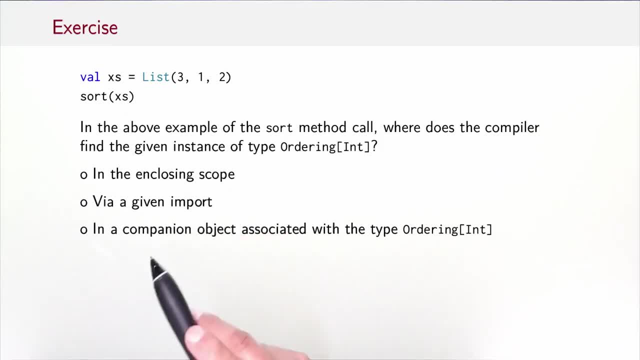 Was it in the enclosing scope via an import, or in a companion object associated with the type? Well, in this case the ordering of int is in the compiling object. So it's in the compiling object associated with the type. The ordering of int was defined in a different module. 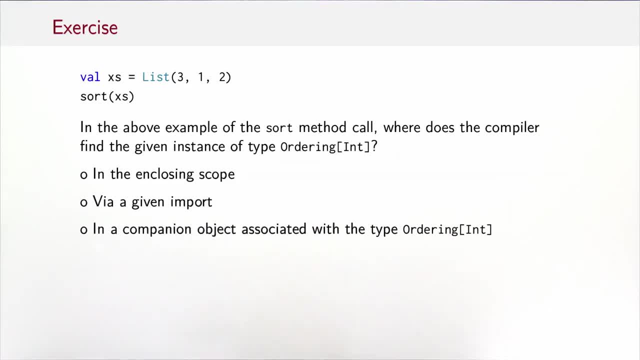 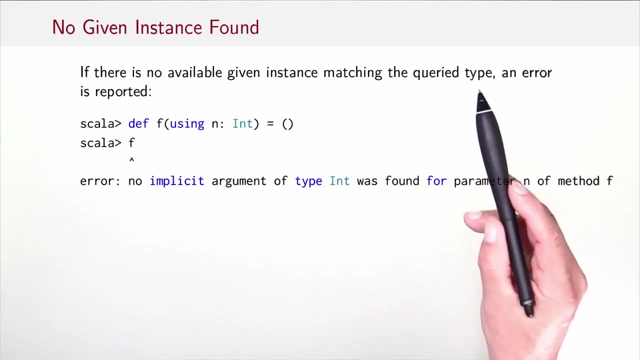 So it wasn't in the enclosing scope and we didn't have to import it explicitly. So it was found because it was a companion object of the type ordering Given instance is found in that companion object. So if there's no available given instance that matches the query type, you get an error. 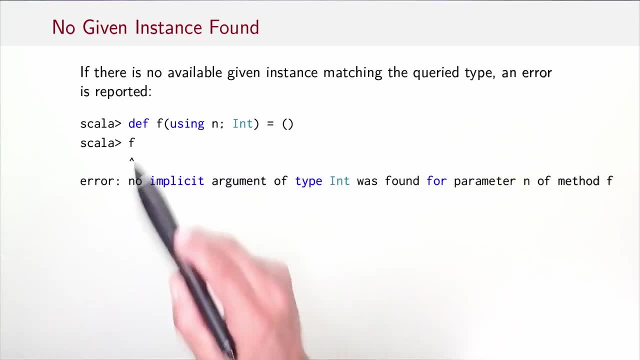 So for instance, here you write def f using an int and you just write f, you will get no implicit argument of type int was found. So you can just write def f using int and you just write f, You will get no implicit argument of type int was found. 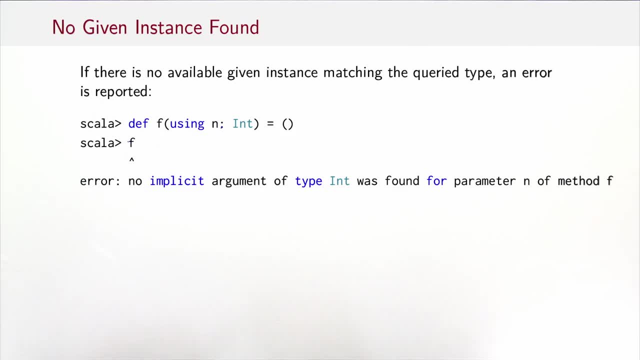 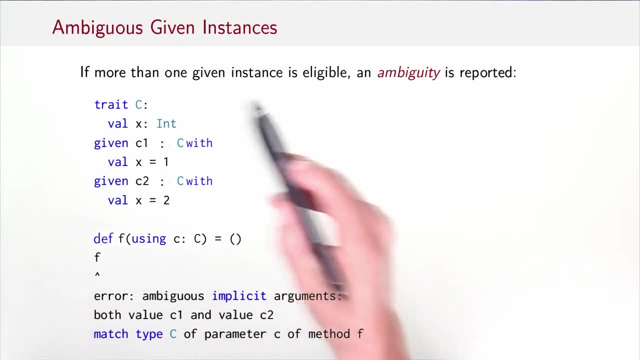 For the parameter n of method f. The other kind of error you might get is an ambiguity. That happens if there's more than one given instance that's eligible. So here you see an example. You have a trait c and you have two given instances of c- c1 and c2, which both define. 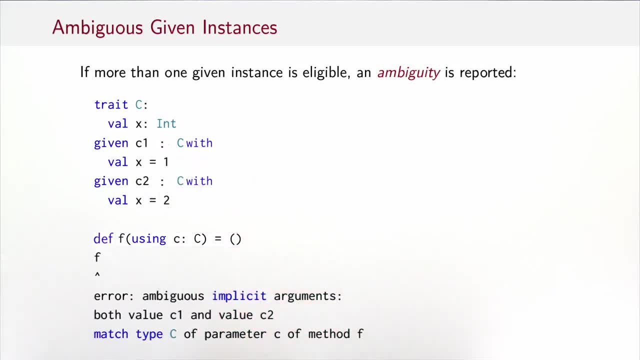 the value x to be different values, 1 or 2.. And we have a function definition f With an implicit parameter of type c. Now if you just call f, then we would get an error which says ambiguous implicit arguments. both value c1 and value c2 match type c of the parameter c of method f. 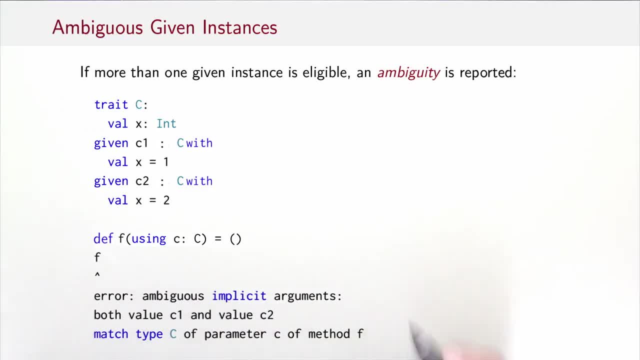 So what do you do when you get an error like that? Well, one thing you could do is just pass the argument explicitly, So, for instance, you could write f using c2.. If it was c2, you want it. 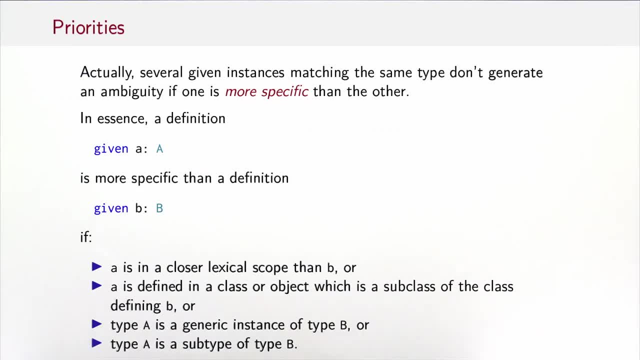 So you don't always get an ambiguity if there's several given instances that match the same type, because it could be that one of them is more specific than the others. In essence, a definition given a of type a is more specific than a definition given b. 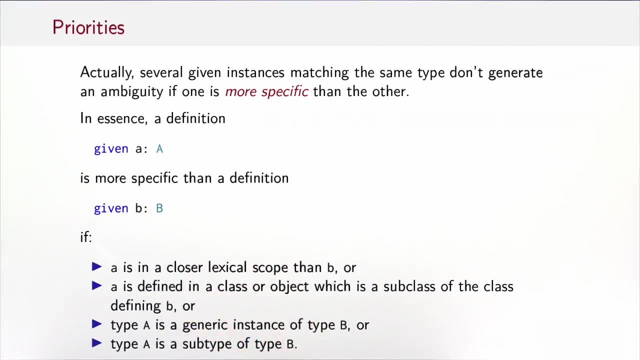 of type b if one of several conditions apply. So if a is in a closer lexical scope than b, so it's nested more deeply than b, then it takes priority. It will be selected instead. It will be selected instead of b. 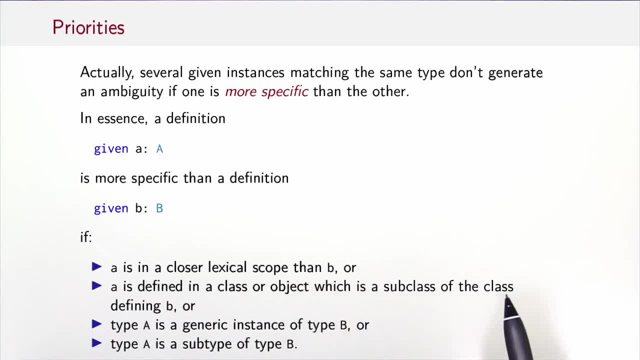 Or if a is defined in a class or object which is a subclass of the class which defines b, then again a takes priority. Or if these conditions don't apply but the type a is a generic instance of type b or is a subtype of type b, then again the a instance will be chosen over the b instance. 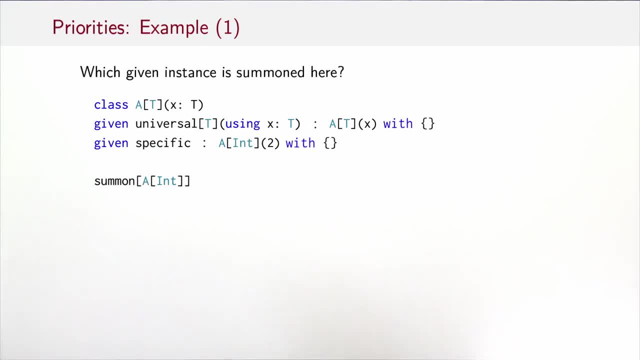 So let's demonstrate this with some examples. What given instance is summoned here? Summon a int. You have these two things. So you have a universal one, which takes a type, parameter and a using argument, and that is an instance of a, of t, for any t, and you have a specific one that is an instance of. 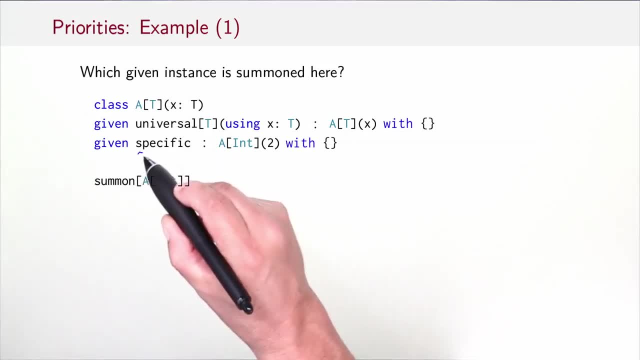 just a of int. So the answer is: the specific one will be chosen because it's an instance of the generic type. So the more specific the type is, the more specific the given instance is as well, and more specific instances will be chosen over more general ones. 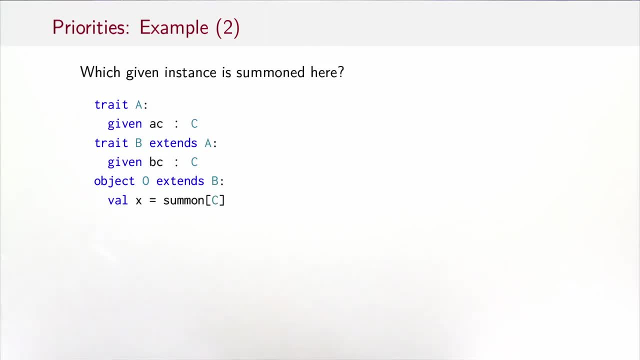 What given instance is summoned here? So you have a trait a and a given instance ac and a trait b and a given instance bc, then an object o that extends b, and we want a c. Well, it will be this one here, because it's defined in a subclass. 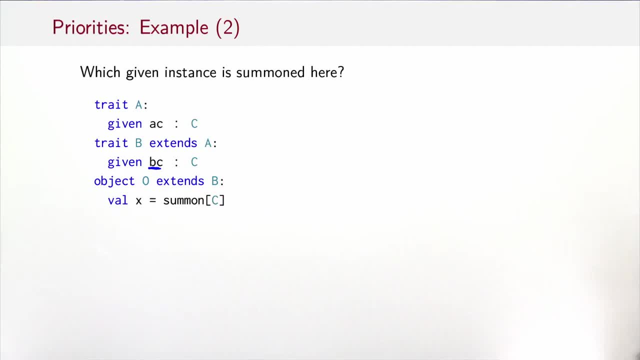 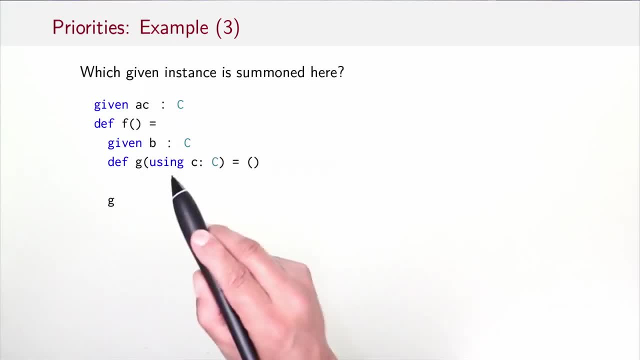 Subclass, Subclass And finally, what given instance is summoned here. So you have an outer instance ac, then a function f with an instance b inside f and then a definition that needs a c. So it will be the inner instance that is chosen, this one here. 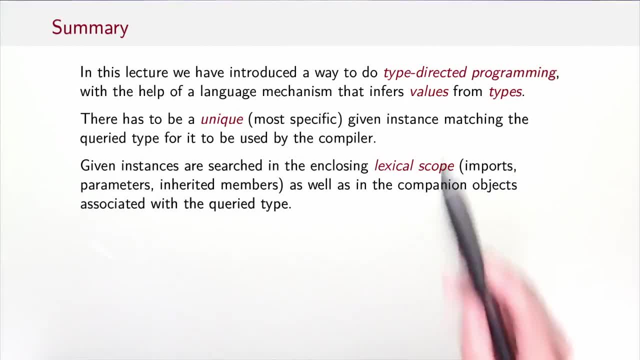 So, to conclude, in this lecture we've introduced a way to do type directed programming. So the types direct our programming and they even generate parts of our program with the help of a language like C, The language mechanism that infers values from types. 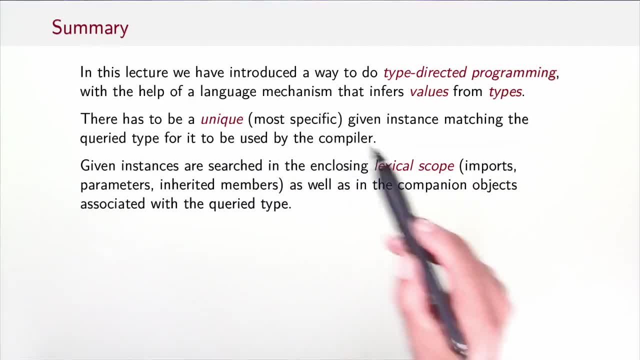 So the idea is that there has to be a unique or at least more specific given instance that matches a query type for it to be used by the compiler for synthesizing a value of that type. Given instances are searched in the enclosing lexical scope. so imports, parameters inherited. 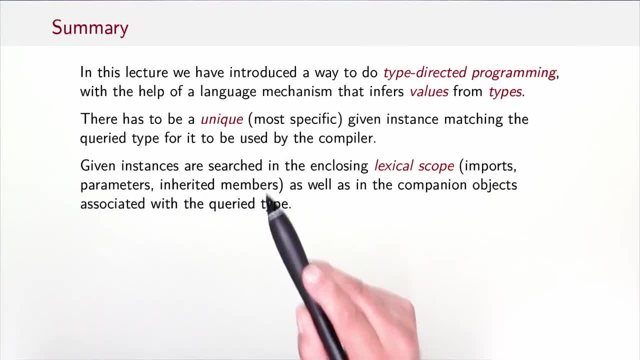 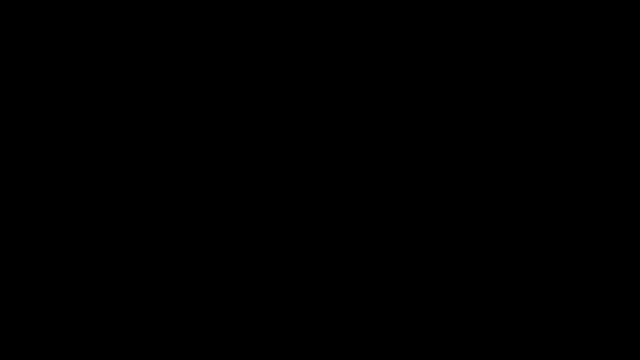 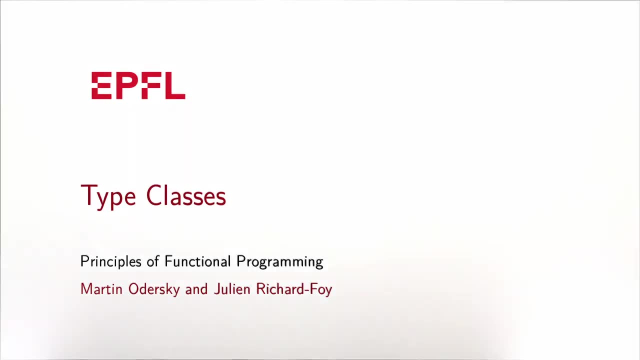 members, as well as normal definitions, and then, if that doesn't give a match, in the companion objects that are associated with the query type. In this session, you'll learn about a particular way to do context abstractions and to turn types into values, which is called type classes. 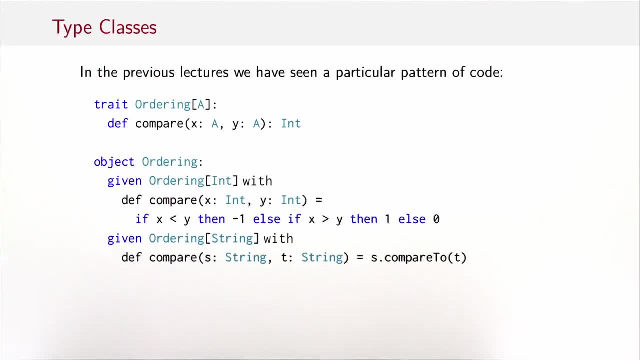 In fact, you've seen the pattern of type classes already. Here it is again. So we have a trait like ordering and a compare method. So we have a trait like ordering and a compare method. So we have a trait like ordering and a compare method. 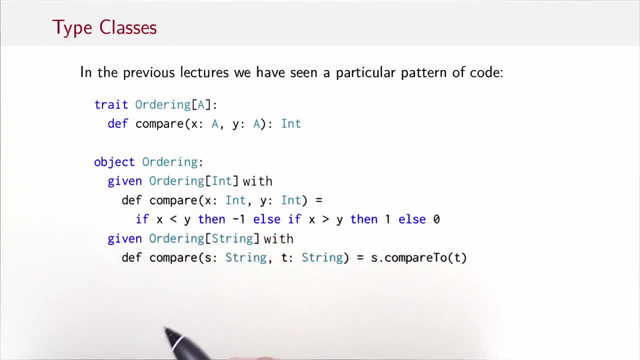 And then we have an object, a companion object, with given instances for particular type, instances of that trait. So we have a given instance for ordering of int and we have a given instance for ordering of string, and both of these instances define the compare method as is appropriate for that. 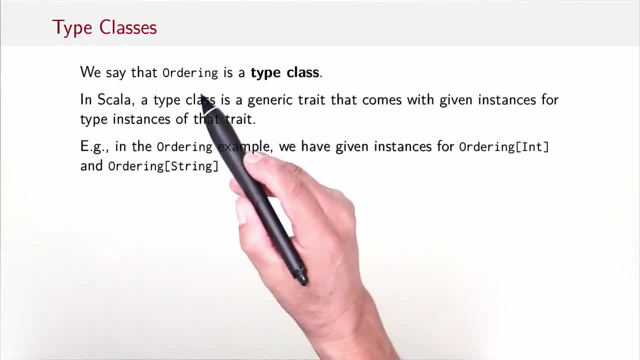 argument type. here. If you have a pattern like that, we say ordering is a type class. In Scala, a type class is made up of a generic type class. In Scala, a type class is made up of a generic type class. In Scala, a type class is made up of a generic type, so a type with a type parameter and 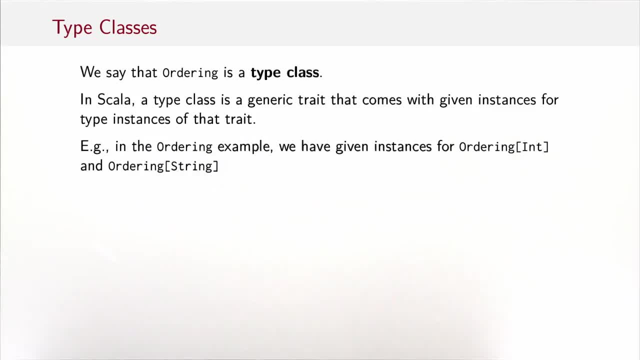 given instances for type instances of that trait. In Scala a type class is made up of a generic type class. In Scala a type class is made up of a generic type class. So in the ordering example we have the given instances for ordering of int and ordering. 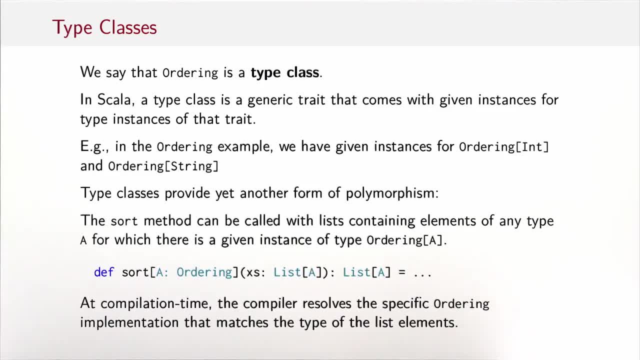 of string And the type class is ordering. Type classes provide yet another form of polymorphism, being able to come in many forms, And that form is sometimes also called ad hoc polymorphism. To see what I mean, look at the sort method. 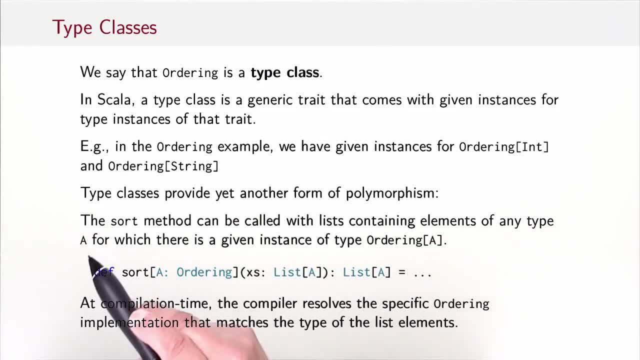 To see what I mean, look at the sort method with lists containing elements of any type a for which there is a given instance of type. ordering of a so sort can be called on arguments of many types and its functioning is different depending on what type it is, because its functioning will depend on the given instance for the actual type a. 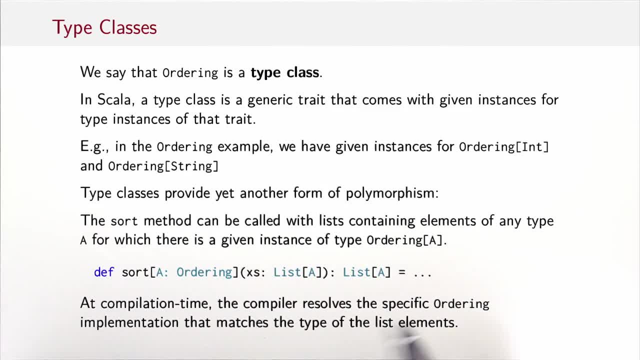 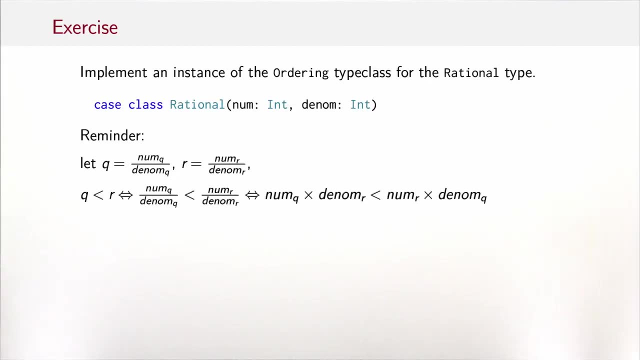 that you see here. at compilation time, the compiler resolves the specific ordering implementation that matches the type of the list elements. resolving simply means providing an argument in a using clause that matches this ordering context bound. so, as an exercise, let's implement an instance of the ordering type class for the rational type. i'm going to simplify a lot. 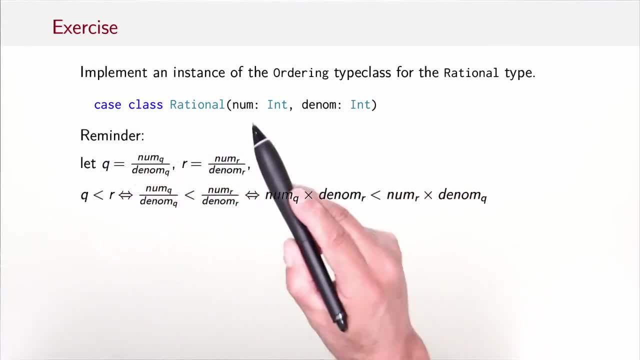 for now, the class rational will simply be a case class with a numerator and denominator and no additional methods. we don't need any for this particular behavior. so for the ordering type class we need to implement a compare operation, and here's a reminder what less than is on rational numbers q and r. what we do is we simply multiply the numerator. 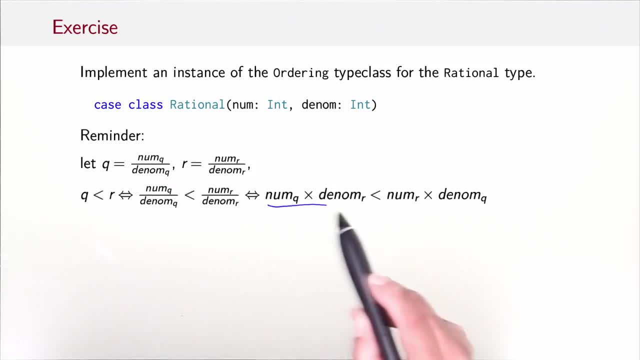 of one side with the denominator of the other. so that gives this here. and do the same thing on the right hand side. so its numerator gets multiplied with the denominator on the left hand side, and then we compare those two products. so let's do this in the way that we did in the previous class. 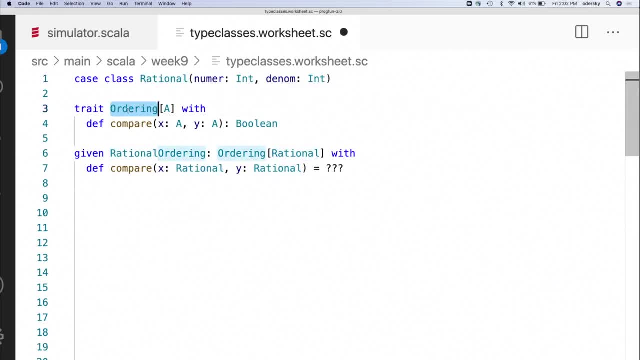 we have our class rational here, our trade ordering here, and we have a given instance- let's call it rational ordering- of ordering of rational, which has a compare method, and we have to implement the right hand side of that method. so, according to the formula, we define two helper. 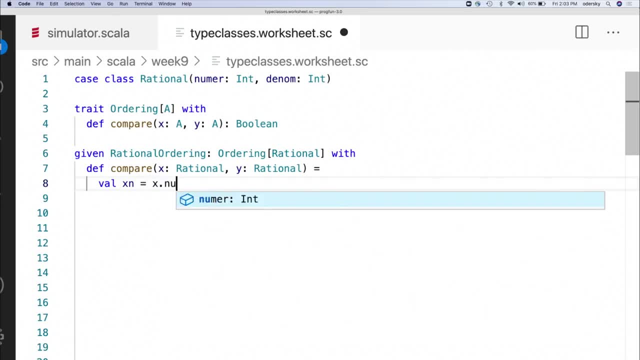 values x, and the normalized is a numerator of x times the denominator of y, while yn would be then the numerator of y times the denominator of x, and then we have the usual comparison. so if xn is less than yn, then we return minus one. else if xn greater yn, 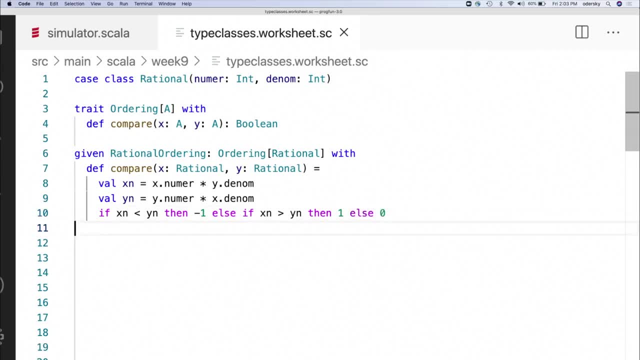 we return one, else return zero. so you might ask, why haven't i written simply x and minus yn? because that gives you arguments of the same sign as this expression here. the answer is this one here is placed better with integer overflow. if i compare two numbers that differ by a very large amount, then that subtraction might overflow, whereas here the 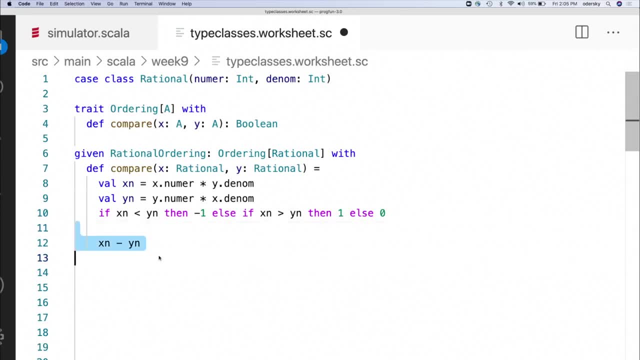 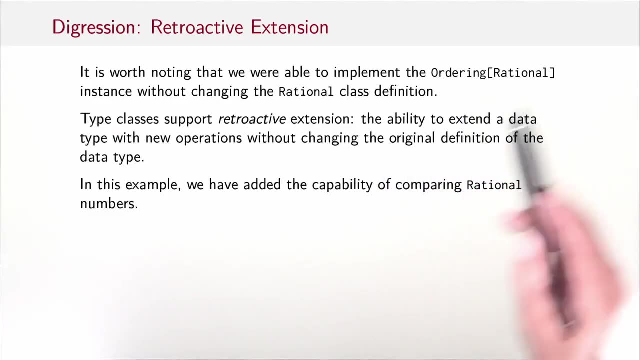 comparison will still give you the good result, so that's why it's written that way. so it's worth noting that we were able to implement the ordering rational instance without changing the rational class definition. that means that type classes support retroactive extension. we can extend a data type with new. 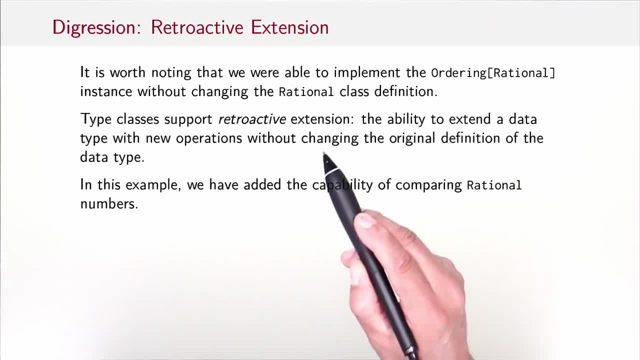 operations such as compare, in this case, without changing the original definition of the data type. in this example, we've added the capability of comparing rational numbers without changing the class rational. so that's one of the advantages of using type classes over using regular classes: that you can do that. here's another advantage. 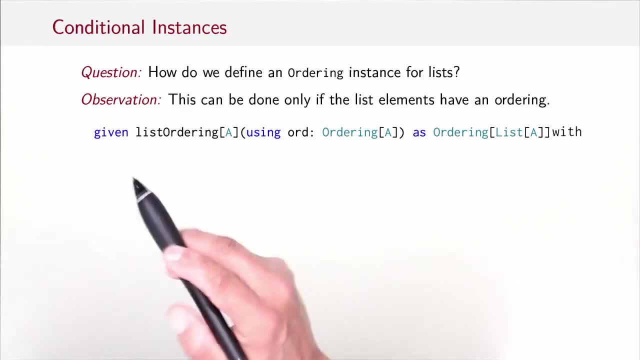 you can do conditional instances. so the question arises: how do we define an ordering instance for lists? and well, it depends what lists of what elements. right, because we can define an ordering on a list only if the elements have an ordering. so that leads us to a definition like this one here: 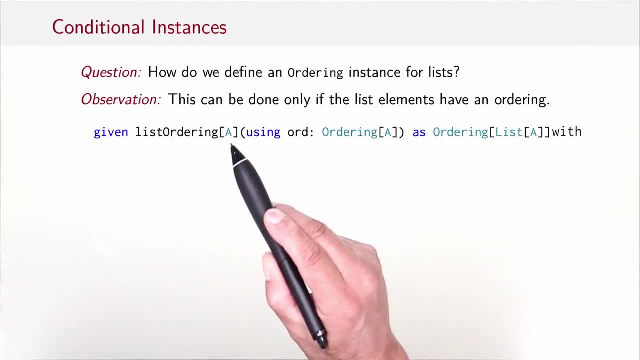 we have a list ordering of with some type parameter a and that is an implementation of an ordering of list of a. but we need an ordering of a as well, which we can express here by adding a using parameter clause to the given name here that you see over there. 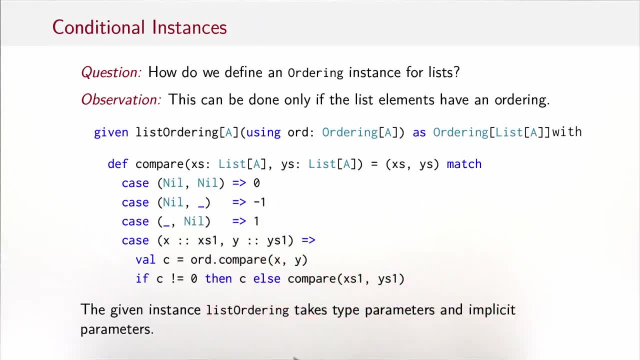 and then we need to define the compare method. here it is. so the compare takes two lists of a and it does a pattern match on the pair of xs and ys. if they're both nil, then they're equal. You can define it, but the graph on the graphinarian doesn't�. if the first one is 0, 0 and the second one is 10, then if ls and ls are even, then you know that there's a double freeze over it, then opening, and there's a double freeze also, and many of us will do that. so this should prepare a отвеч. 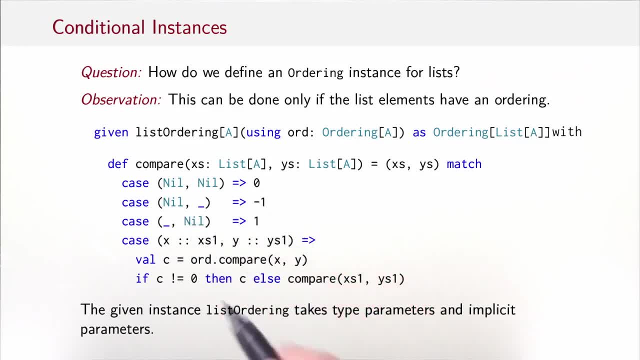 one is nil and the second is not nil, then the first one is smaller. If the second one is nil and the first one is not, then the first one is smaller. If they are both non-nil, so they are both constants, with heads x and y and tails x as 1, y as 1, then we compare. 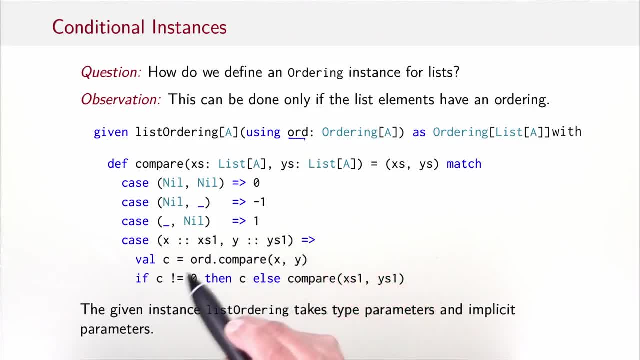 the heads, and for that we need our type class, here our ORT. So we use ORT to compare x and y. That gives the result c, And then if that result is 0, then we compare furthermore the list x as 1 and y as 1, we compare the tails If the result is different from 0,. 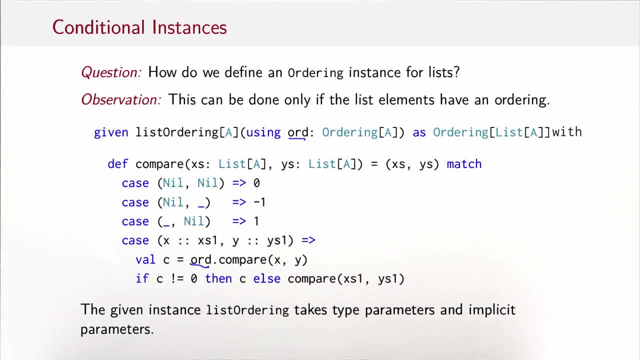 then we have our result and that's what we return. So one new syntax that we've seen is that a given instance list ordering can take type parameters and implicit parameters. You could also leave out the list name, in which case you would just have a given instance without a name and type. 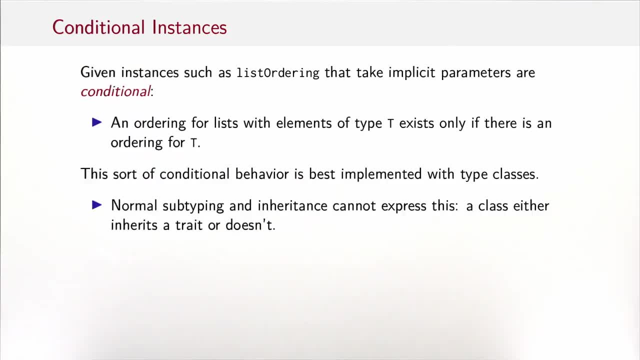 parameters, given parameters that would work as well. So we observe that, given instances such as list ordering that take implicit, parameters are conditional. That means an ordering for lists with elements of type T exists only if there is an ordering for T, because otherwise the compiler couldn't synthesize an. 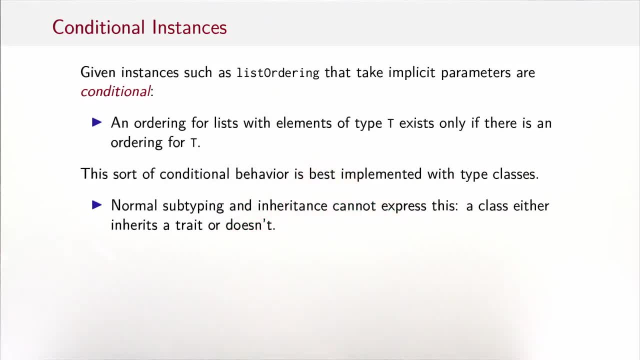 actual argument for the using clause in list ordering. So this sort of conditional behavior is really best implemented with type classes. Normal subtyping and inheritance cannot express this. A class either inherits a trait or it doesn't. But you can't make a class inherit a trait depending on a condition. 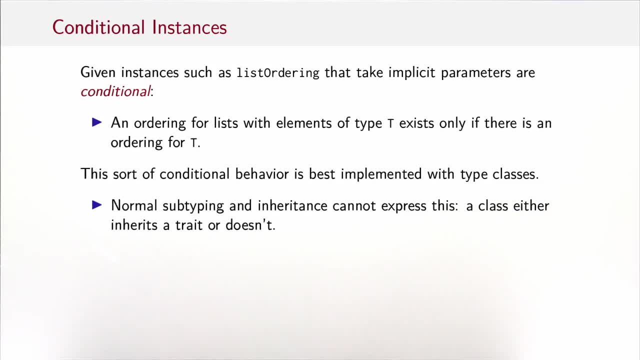 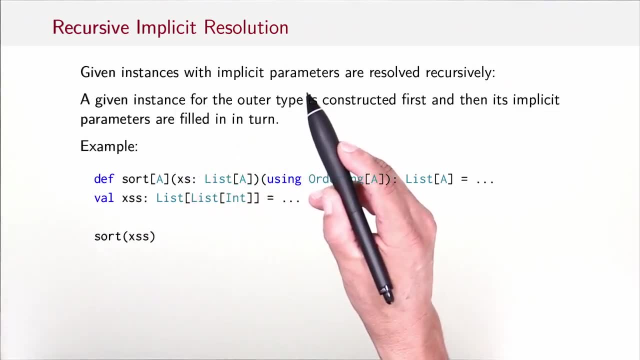 of its parameter types. That's not possible, But with type classes it is. Things get interesting if we look at how instances of conditional implicit parameters are resolved. In fact, the resolution proceeds recursively. That means a given instance can be used to solve a conditional condition. If we look at how instances of conditional implicit parameters are resolved- In fact, the resolution proceeds recursively- That means a given. 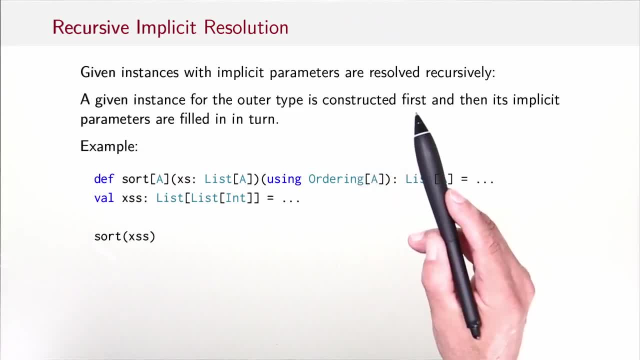 instance for the outer type list in this case, is constructed first and then its implicit parameters are filled in in turn. So for instance, let's say we have the sort method which takes an ordering, A type class instance, and we want now to sort a list of list of int. So that's the original call Type inference gives us. 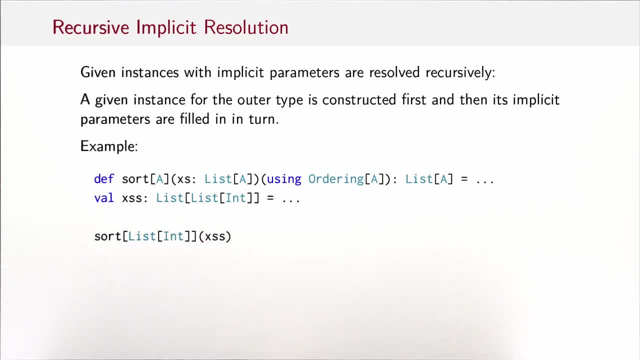 list of int as the element type A that we want to sort. So now we need an ordering instance for list of int. So the ordering instance we find is list ordering, So that's what we pass, And list ordering itself needs a ordering instance for the element type, which is 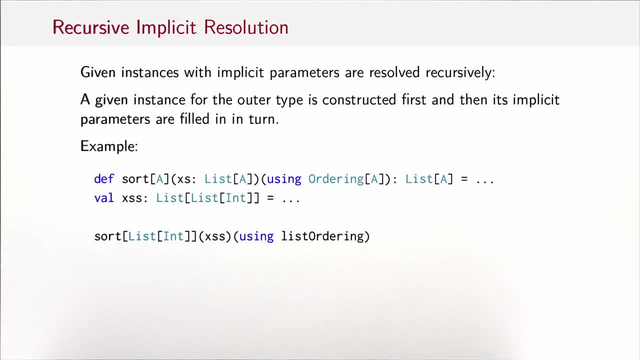 int in this case. So this expression in turn is expanded to this one here, using list ordering that takes an ordering of int parameter. So we started with this and we got this. That is essentially the work of the compiler that added the missing pieces. 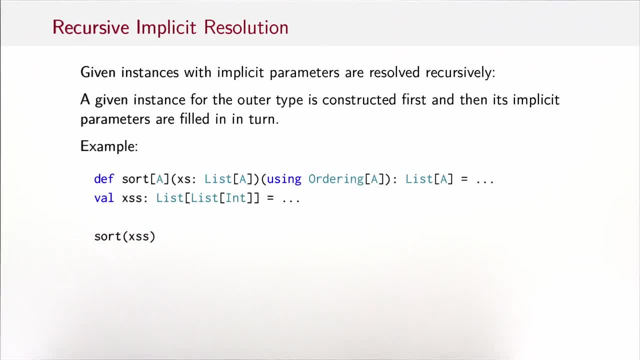 It's also worth noting that each of the intermediate result is actually a valid scalar program. So you can write this, of course. You can also pass the type parameter explicitly, of course, But you could also add just list ordering, essentially to help the compiler along and says: well, I need a list ordering. But 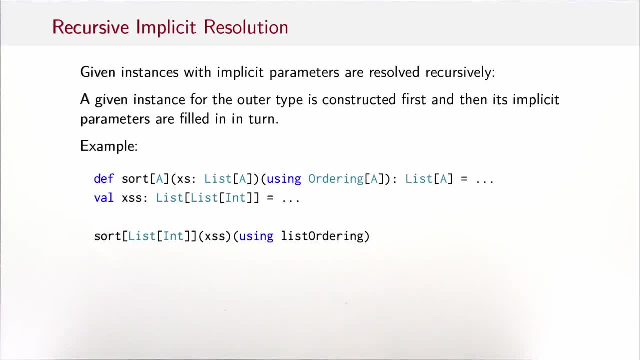 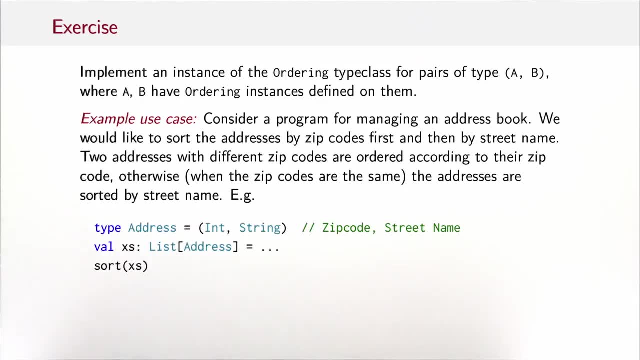 now you can figure out yourself what parameter, what argument to pass to the list ordering instance here. So you could either write this last thing or leave it out. So here's another exercise. Let's implement an instance of the ordering type class for pairs of type A and B, where A and B must have ordering instances defined on them. 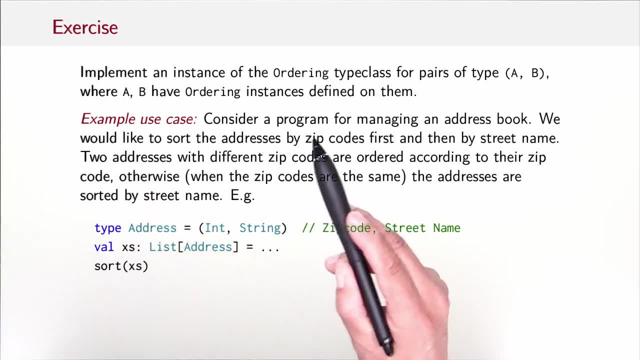 That's useful for examples like this one. here Let's consider a program for managing an address book. We would like to sort the addresses by zip codes first and then by street name, So two addresses with different zip codes are ordered according to their zip code. 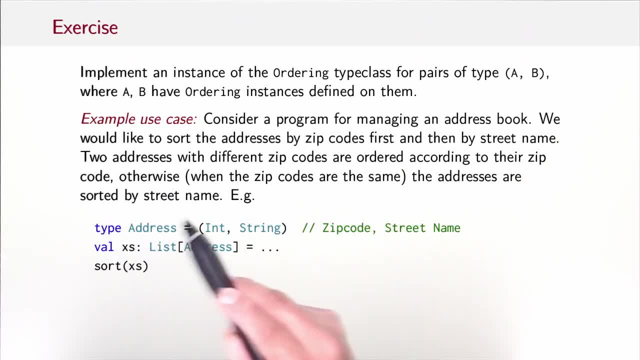 Otherwise, when the zip codes are the same, the addresses are ordered by street name. So that would lead to the setup that you see here. We have a type address, which is a pair of int and string. We have a list of addresses and we want to sort that list. What is the given instance that we can pass to that sort function? 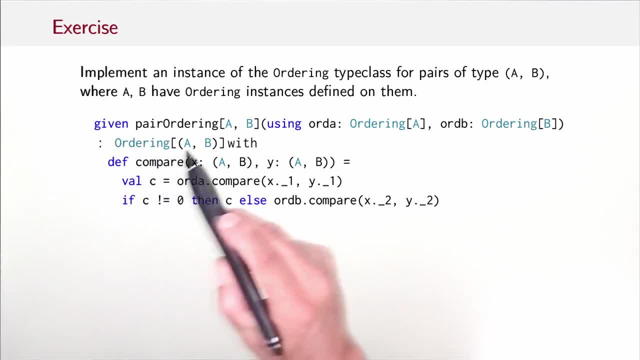 So here's a solution. We have a given instance- Let's call it pair ordering- of ordering of A and B. Here A and B are type parameters, So that works for any pairs of types A and B, But they must both have an ordering instance. So we must have an ordering instance for A and one for 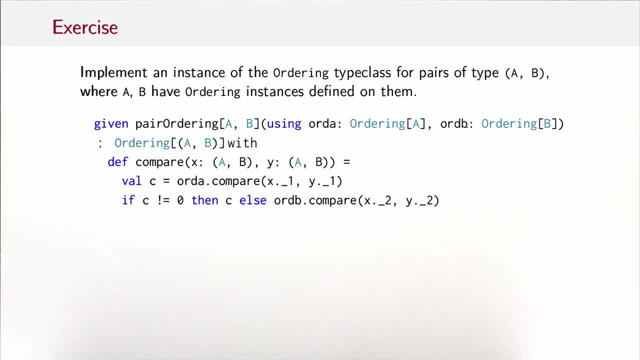 B. We give them names: ordA for the one, for A and ordB for the other one. So now we have to define a compare method for pairs. So the compare method takes two elements, x and y, both of type pair of A- B, And what we do is we compare the first. 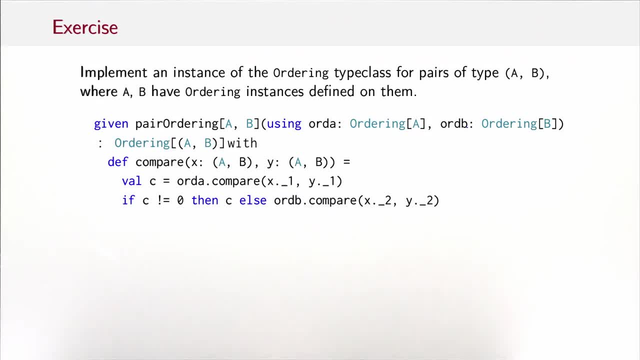 half of these pairs. So that's x dot underscore one and y dot underscore one. That gives us a result. If that result is different from zero, then that's what we return, And otherwise, if the result is zero, we go on and compare the second halves of the two pairs. 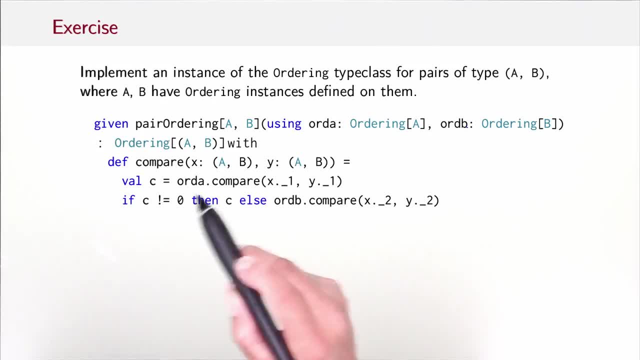 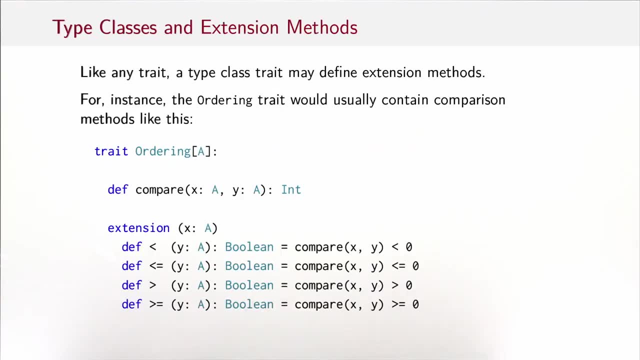 And for the comparisons. we use ordA in the first case because that's the comparison we need to use for the A parameter, And we use ordB in the second case. Good, So we've seen that ordering has a compare method. 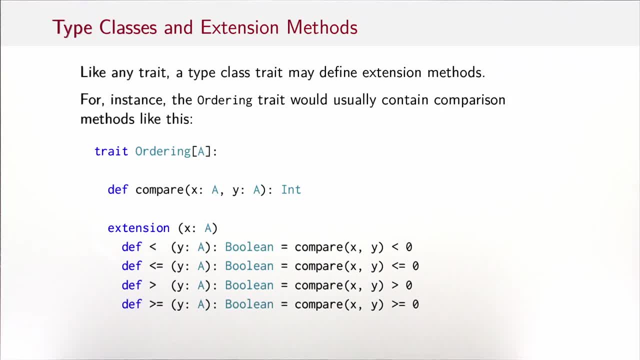 But typically when we use an ordering, we don't really want to use compare. We want to use less than or greater than or methods like that. So that's possible because, like any trait, a type class trait can define extension methods. 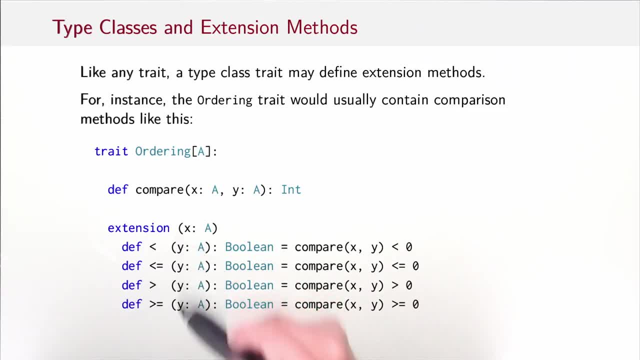 For instance, the ordering trait would usually contain comparison methods like this. So there's the compare method, which is abstract, And then we have extension methods- less than less than or equal, greater than greater than or equal- which all use compare to produce. 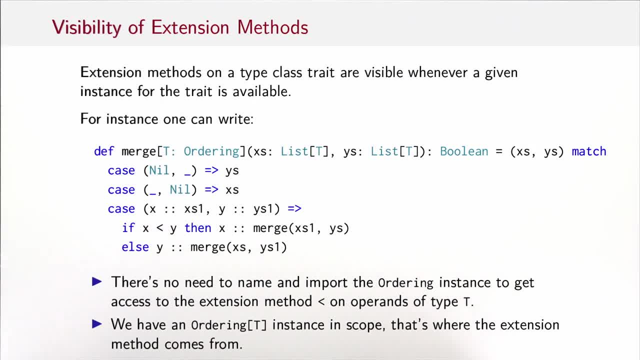 their results. So that's handy, because now we can use the natural less than operators and the others for comparisons. So here's an example in the merge method of merge sort. So merge works for any type T that has an ordering, So that's an implicit parameter. 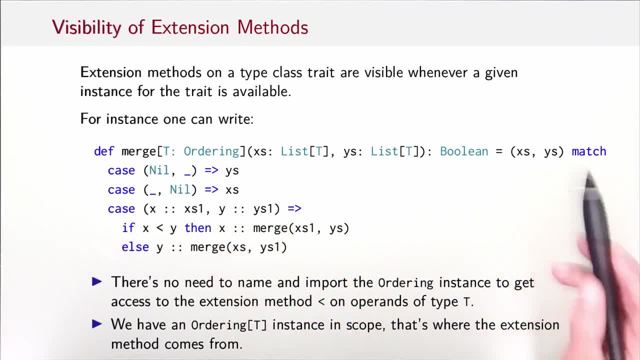 ordering of T that we assume here, And there's the usual pattern match which says: well, if one of them is nil, then take the other, And if they're both non-nil, then we compare x and y. So that uses a comparison operation. less than which is the less in ordering, So that less. 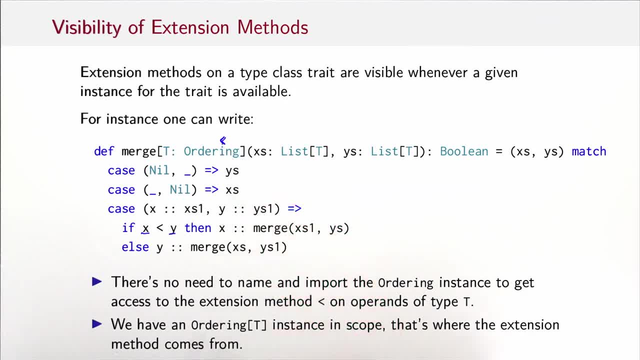 is really the less that we have here defined as an extension method in the ordering class. Now you might wonder how does the compiler know that this less than means the ordering, less than It's not defined in the environment, It's not imported, In fact we don't even have 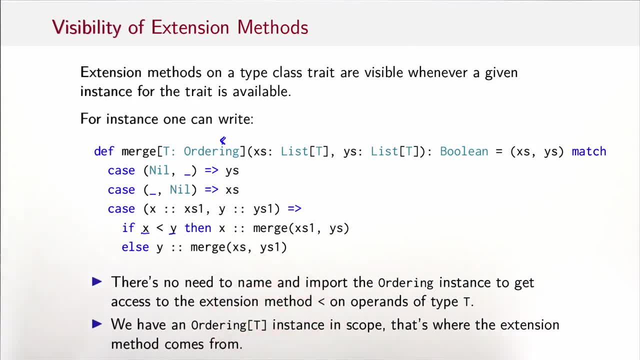 a name we could import it from. Ordering is just a context bound. It isn't a name parameter. The trick is that there's an additional rule which says that if we have a type class instance, such as ordering in scope, then its extension methods are eligible for the type that is. 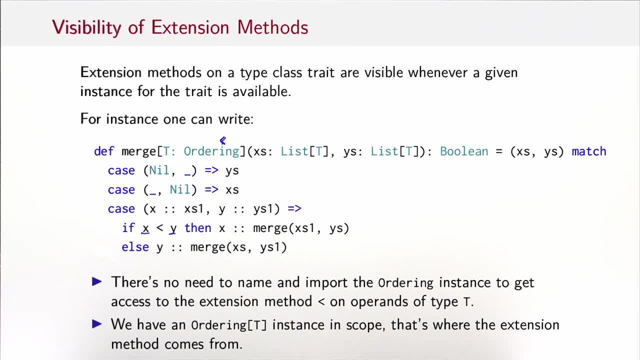 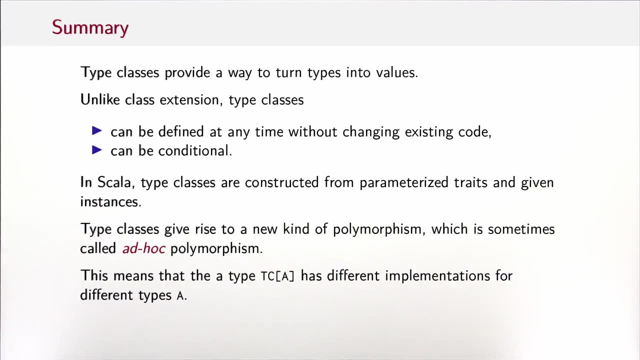 the argument of the type class. So we have ordering T in scope, and that means its extension methods are defined on values of type T. That's what makes it work without any additional boilerplate. So, to summarize, type classes provide a new systematic way to turn type into values. 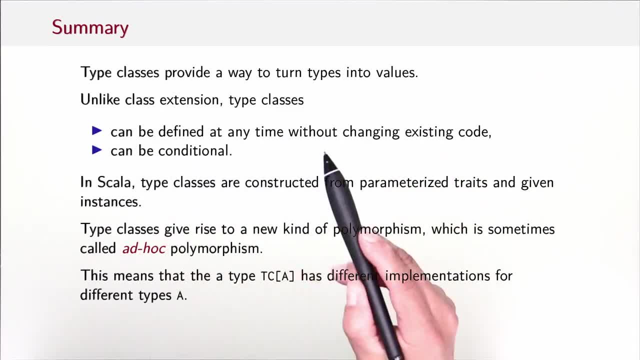 Unlike class extensions, type classes can be defined at any time without changing existing code, and they can be conditional. That makes them a lot more flexible and powerful than plain class extensions that we have seen before In SCALA. type classes are constructed from parameterized traits. that's a type class. 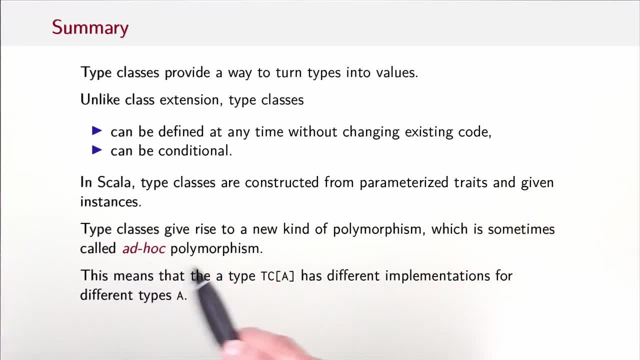 and given instances for that trait. Type classes provide a new systematic way of turning types into values You can have. Type classes give rise to a new kind of polymorphism, which is sometimes called ad hoc polymorphism. That means that the type TCA has different implementations for different types A. 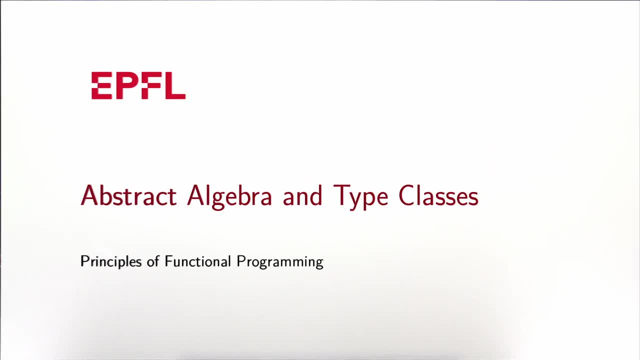 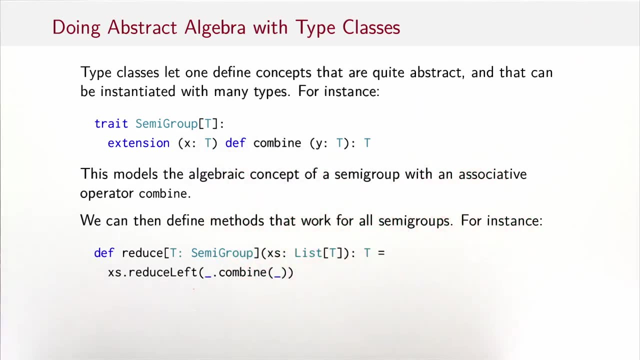 In this session you'll get some taste how you can implement abstract algebra with type classes. Type classes: let one define concepts that are quite abstract and that can be instantiated with many types. For instance, we could come up with the concept of a semi-group. A type is an instance. 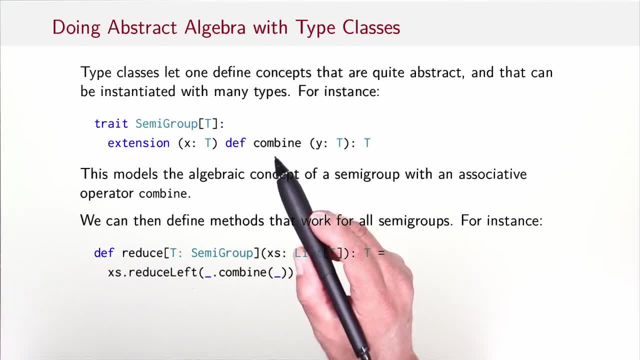 of a semi-group if it has a combined method, a binary operator that takes two T's and returns a T. There are many possible instance types of semi-groups. For instance, int with addition is a semi-group, so is int with multiplication. So we have a choice what operator we want to. 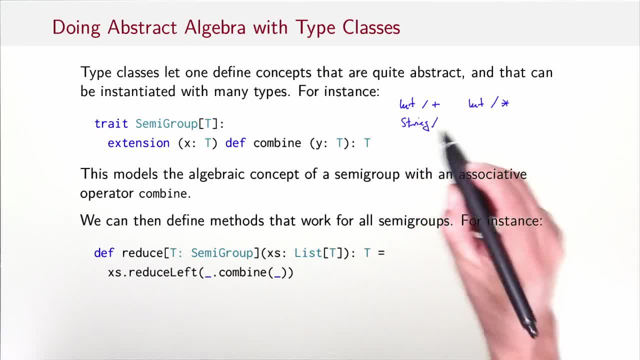 use here. So it's string with concatenation, so that would be string plus. So it's any sequence really. So seek of some A type A with concatenation again, And you can find many, many other examples. It's really very general. So semi-group is a concept that comes from abstract algebra. 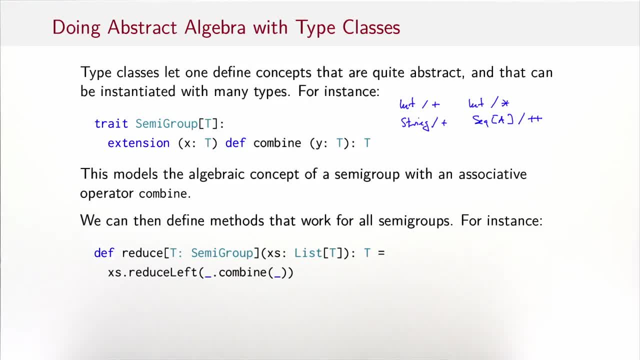 from mathematics And there to be a semi-group, it's required that the operator is associative. In fact, if you look at these examples, then each of these operators is indeed associative. Once we have defined semi-groups, we can now define methods that work for all semi-groups, So very general methods that work for all of these combinations. 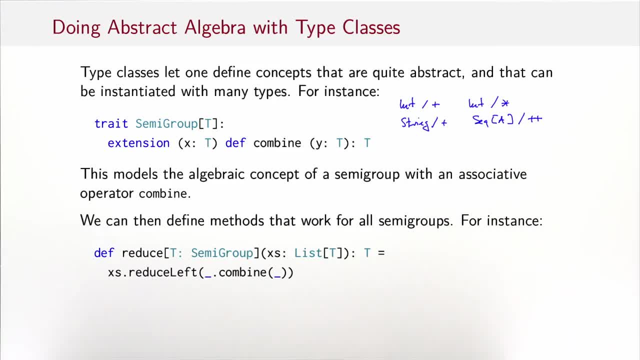 up here. For instance, we could have a reduce method that reduces lists of T elements where T is a semi-group. So it would take the operator that is defined by the semi-group and use that operator, called combine, to reduce the elements of the list. 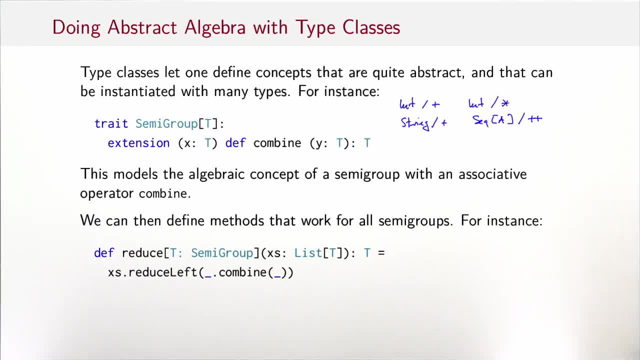 Yielding a single value of type T. So depending on what the type T and its semi-group instance are, reduce could do many different things. If you give it a list of ints and an instance of the sum semi-group here, then it would give you back the sum of the numbers in the list. 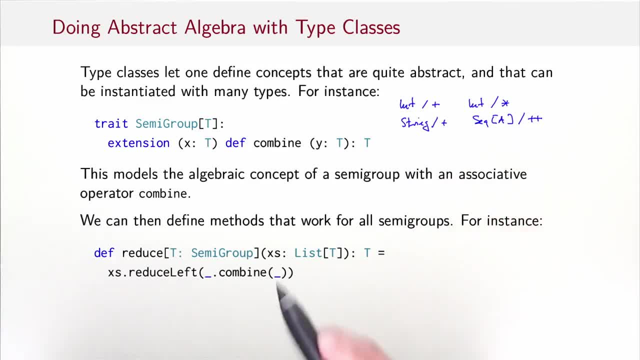 Or if it's a product, semi-group, the product, Or if you give it a list of strings, then it could would give you back the concatenation of all these strings. It's a very general method that exists in many forms. In fact, if we look at abstract algebra, then the type classes that we 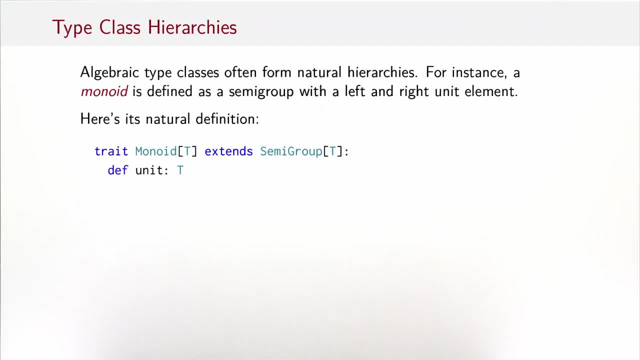 find there form natural hierarchies. For instance, the next element down from a semi-group is usually called monoid. that's defined as a semi-group with a left and right unit element. So here's its natural definition. A monoid of T is a semi-group of T and it has, in addition to the 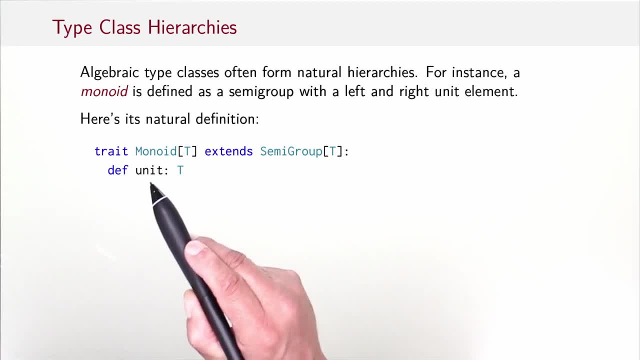 combine method: the binary operator. it has, in addition, a unit method. This is a method that returns the unit element of type T. So unit means that if you combine it to the left or to the right with anything, you get back the other operand, the anything. 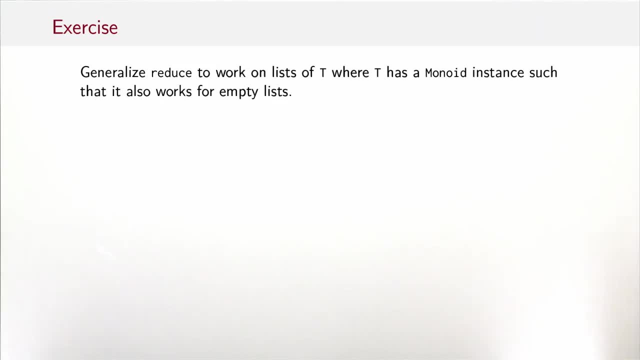 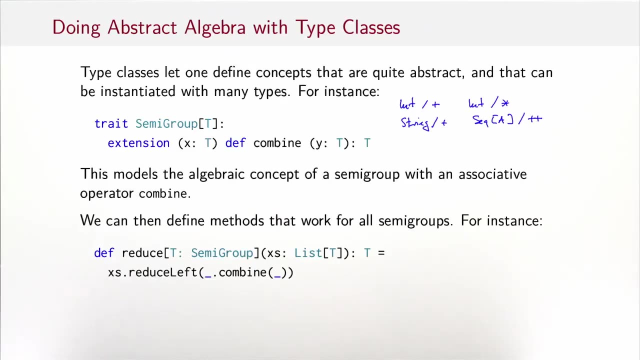 So as an exercise, let's generalize reduce to work on list of T, where list has a monoid instance, such that it also works for empty lists. If you look at the reduce operator before, it wouldn't work for empty list, because reduce left doesn't work for empty list. It gives you an exception. 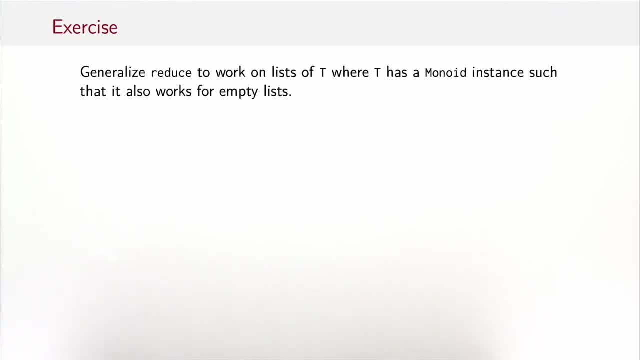 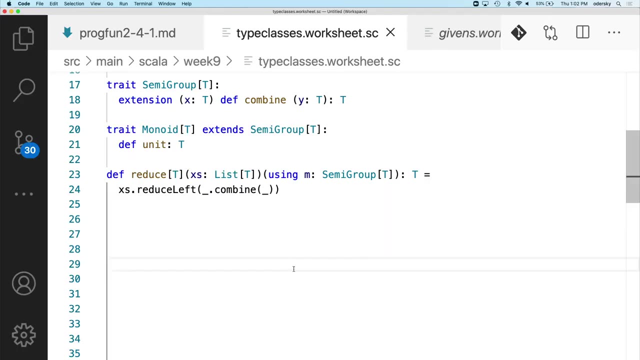 illegal operation. So now we want to get a version of reduce that works on monoids, so that it returns the unit element for an empty list. So I have pasted what we have so far in a worksheet. So here's the old definition on reduce on semi-groups. Let's make it work for monoids and empty lists. 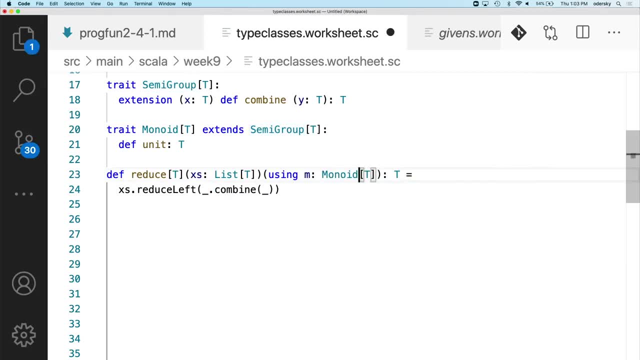 So we replace semi-group by monoid. And now we don't want to use a reduce left, because reduce left doesn't work for empty lists. We want to use a fold left. It could also be a fold right, It doesn't matter, because combine is associative. 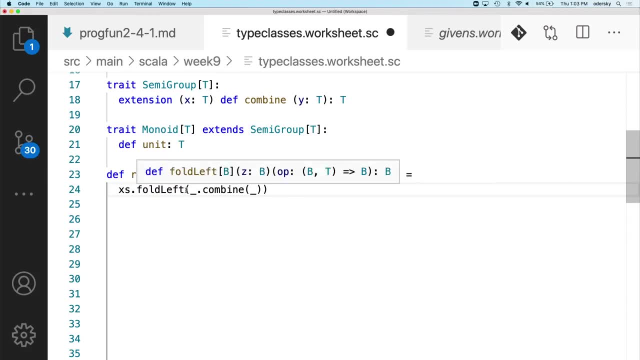 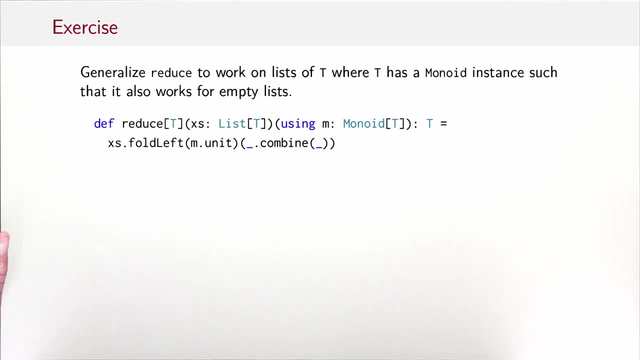 But let's use a fold left. Okay, so we do a fold left. So for fold left we need a unit element, So that would be m dot unit, And we have the same combine method as before. So that's the definition of reduce that we came up with. But one thing you have noticed is that I 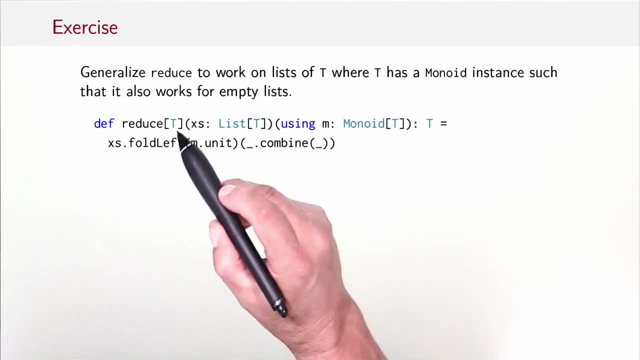 changed the header of reduce a little bit. Instead of a context bound, I was using a plane type parameter and a using clause because I needed a name for the actual monoid in question to select the unit element from that. The question is: can we also do without? Can we do with a context bound? What would we have to do to work with that? 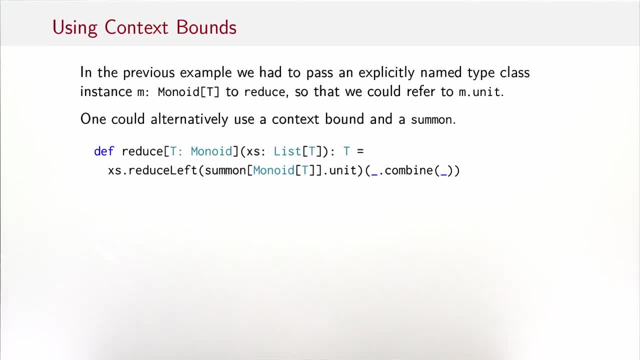 So if we keep the context bound, then reduce would look like this: So then to actually get the monoid of t instance that we need, we can use a summon here. So we say reduce left and then summon monoid of t, So that would give us the monoid that's implied by this implicit parameter. 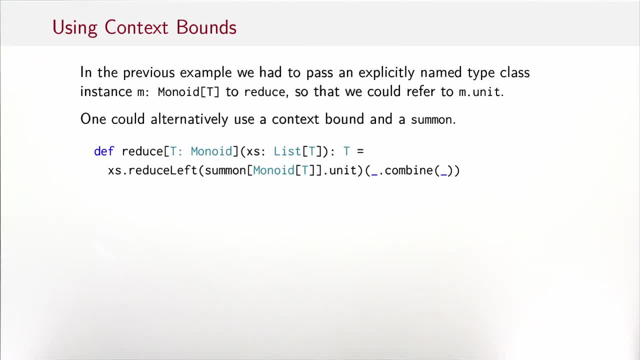 and take the unit from that. So this works, but it's unfortunately a bit clunky. So if monoid is used a lot, which is maybe too expected because it's a very general type class- then it might be worthwhile to streamline the notation a little bit, And we can do this by: 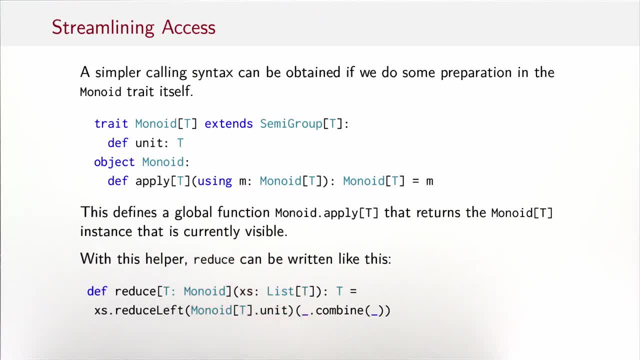 adding a helper method to the companion object of monoid. So we define a companion object, monoid, and we give it an apply method, and that apply method is essentially a summon. So it says: well, I need an implicit parameter of type monoid of t for type parameter t and I return that implicit. 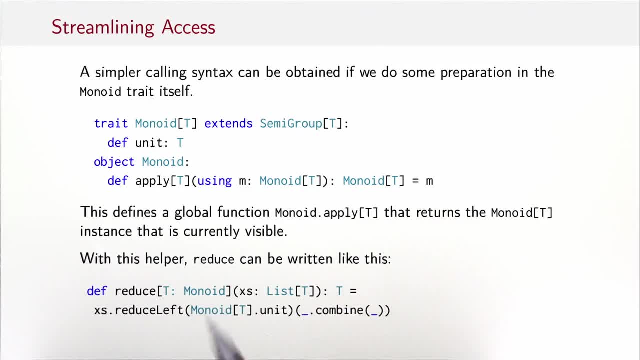 argument. So I return the current monoid of t instance. So that defines a, now a global function. monoid dot apply of t. that returns the monoid t instance that's currently visible And with that helper we can now write reduce like this: 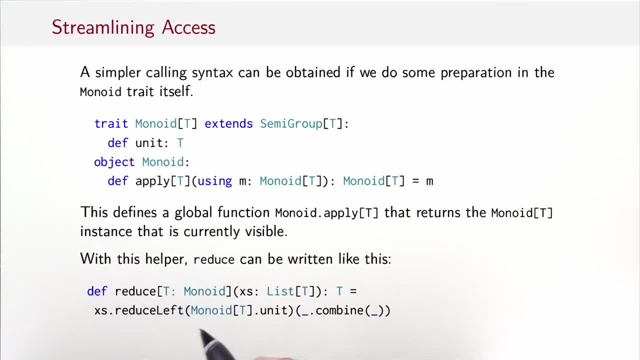 So reduce Context bound as before, and we do reduce left with monoid of t dot unit. So monoid of t is of course monoid dot apply of t. as always, we insert an apply. So it's this method here, and what it returns is: 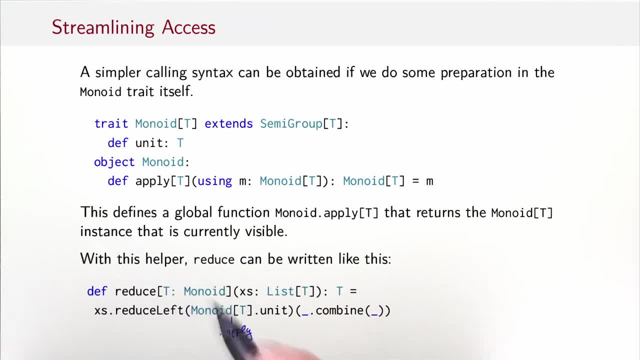 the current monoid of t instance that is in scope and we take the unit element of that. So that's precisely what we want. So that's a way to keep context bounds, because they're nice and concise and streamline the access to things that are not extension methods in the type class. 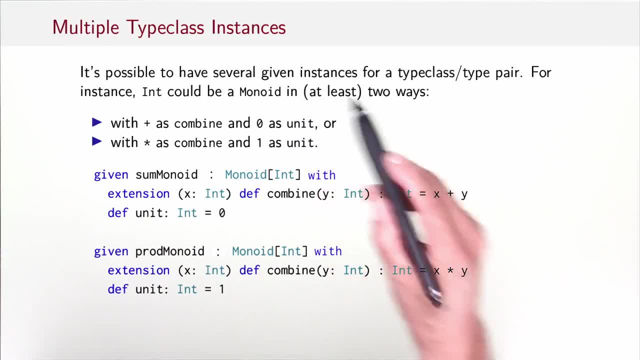 a little bit Now. it's possible to have several given instances for a type, class, type pair. For instance, int could be a monoid in at least two ways. So it could be a monoid with plus as combine and zero as unit, or it could be a monoid with times as combine and one as unit. So those 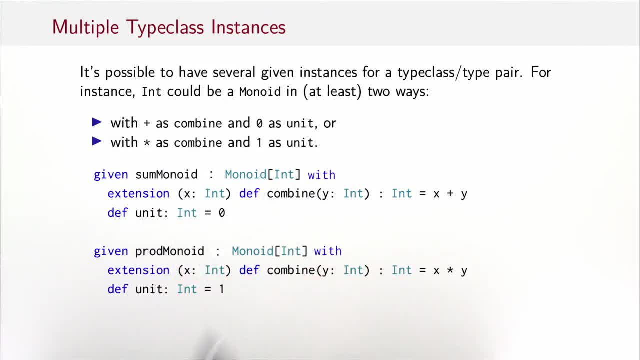 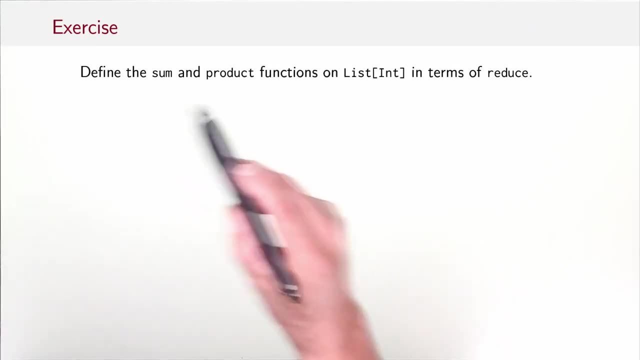 are the two instance definitions. The given sum, monoid, is this: So combine is plus and unit is zero. and the product, monoid is this: Combine is times and unit is one. Assuming we have these given instances, define as an exercise the sum and product functions on list of int in terms of: 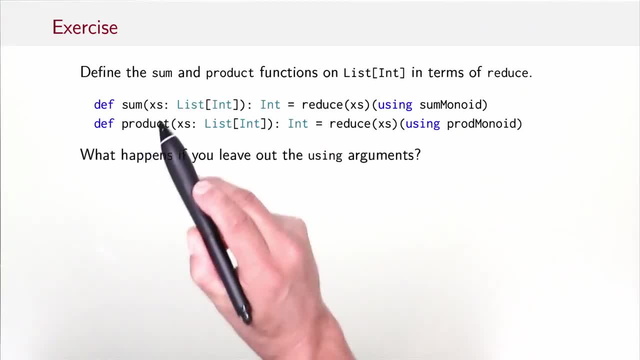 reduce. Well, here's what you would get. So sum of xs is just reduce xs with the sum monoid, and product xs is reduce xs with the product monoid. That's all there is to it. Now question to you: if you have done that in the worksheet, Could you just quickly try out? 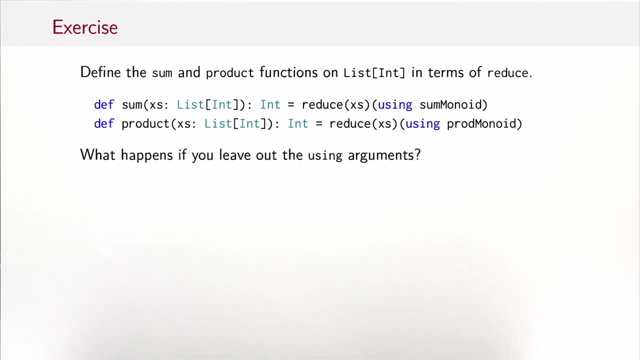 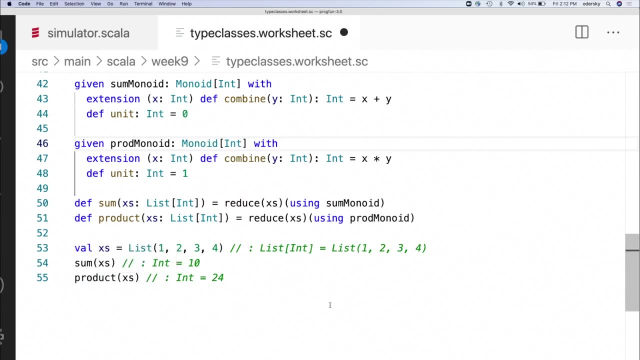 what happens if you leave out those two using arguments? So I have the worksheet here with all definitions and you see that indeed, sum of xs and product xs work as expected. So what happens if I leave out the using clauses in the arguments here? I'll comment them out here. 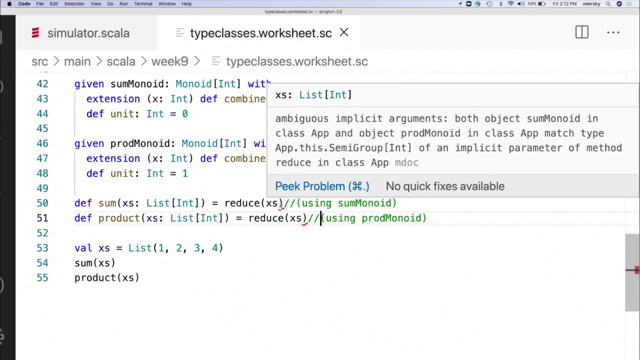 So I get two errors. They say both ambiguous implicit arguments. Both the sum of monoid object and the product monoid in a class app match the type that's expected, which is semi-group. So that's quite normal because indeed I have two given instances: sum monoid and product monoid. They're both applicable, They can be both passed. 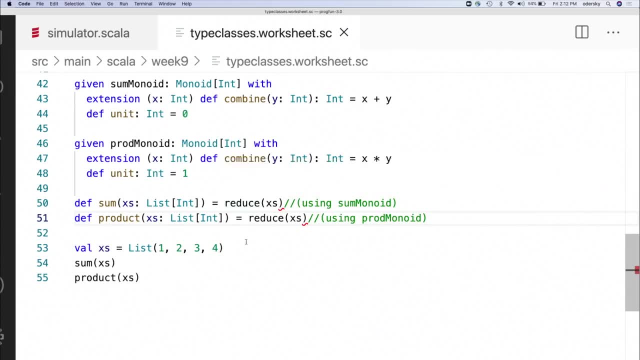 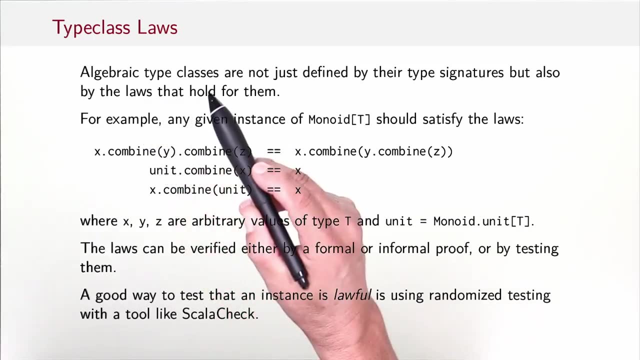 to the using clause of reduce, and neither is better than the other. So you get the classic ambiguity error. Now, one thing that's important is that algebraic type classes are not just defined by their type signatures, but also by the laws that hold for them. So, for instance, if you have a given instance of 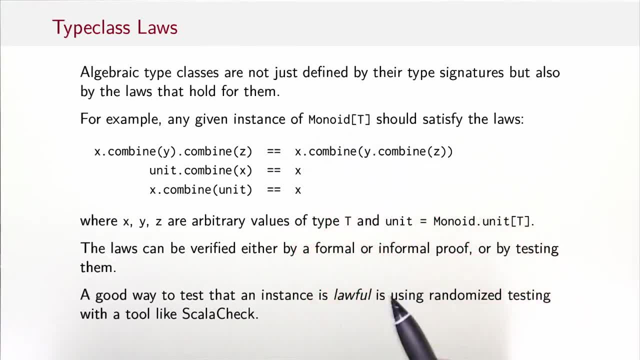 monoid of t, then that instance should satisfy the laws of monoid, which are that combine is associative and that unit is a left and right unit. So it should satisfy these laws for arbitrary values, xyz of type t. How do you verify the laws? Well, the type. 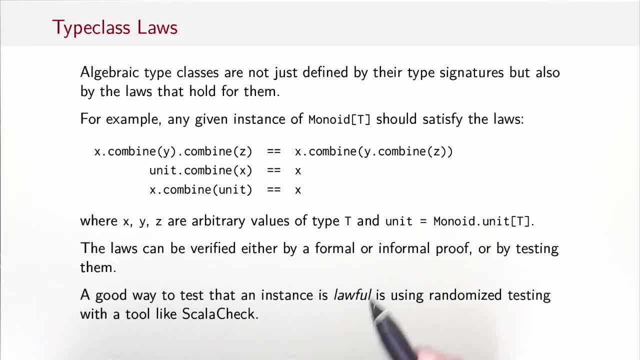 checker is not yet up to it to do that, So you'll need a proof. that could be a formal proof on paper or an informal proof, or it could be a proof with a mechanized proof assistant, such as Coq or Agda or Isabel or one of these, Or you could just test them And a good way to test these laws, or a good 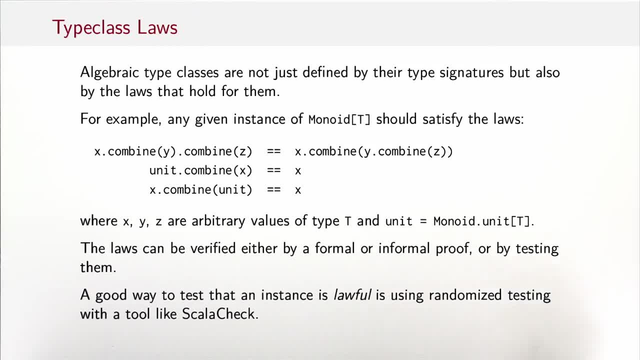 way to test that an instance is lawful is by using randomized testing, because that will exercise these laws at many different random values And that you can do by using randomize testing. So you can do that with a tool like ScalarCheck that we have seen a couple of sessions ago. 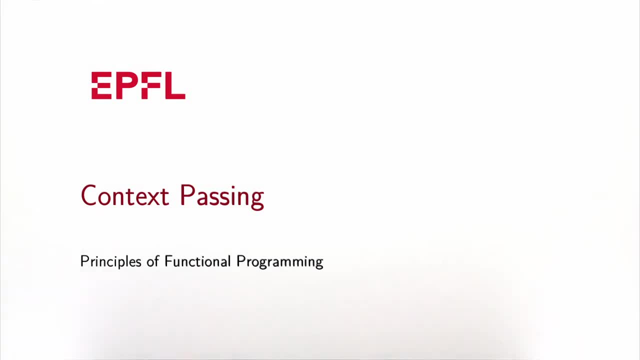 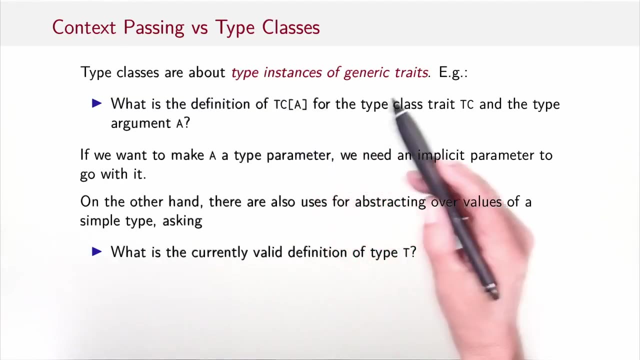 In this session I'm going to cover another broad category of contextual abstractions, which I call context passing. You've seen that type classes are about type instances of generic traits. That is, they answer the question: what is the definition of t c, a for the type class trait t c and the type argument a If you want to make a a type parameter? 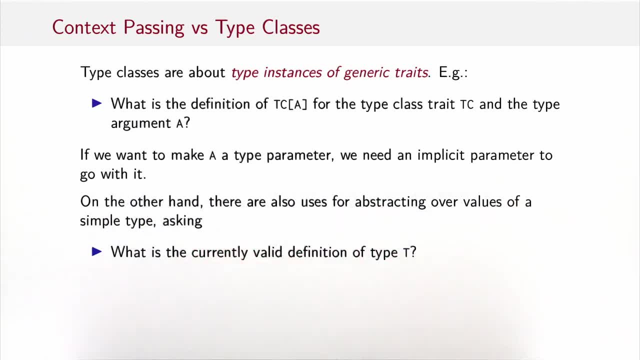 we need an implicit parameter to go with it that conveys this information: what the actual definition of t, c, a is. On the other hand, there are also uses for abstracting over a values of a simple type which is not parameterized, And then the question to ask would be: what's the currently? 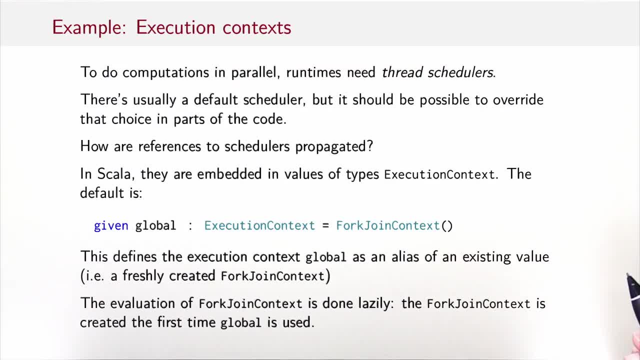 valid definition of type t. So here's an example that comes up a lot in code that uses concrete or parallelism. To do computation in parallel, runtimes need thread schedulers. A thread scheduler is essentially a piece of software that allocates a runtime on processor cores. 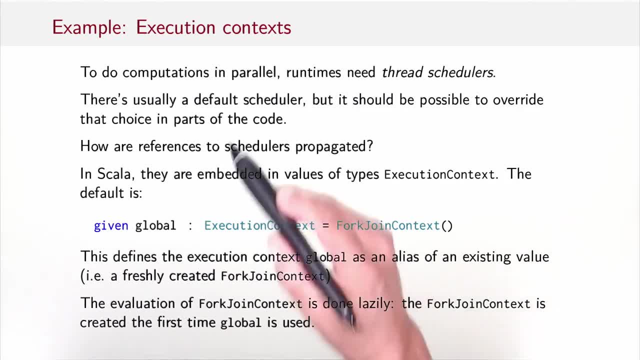 to individual parallel processing threads. There's usually a default scheduler, but it should be possible to override that choice in parts of the code, because a different scheduler might have better performance characteristics or better availability guarantees and so on. So the question is: how are references to schedulers propagated In Scala? they are. 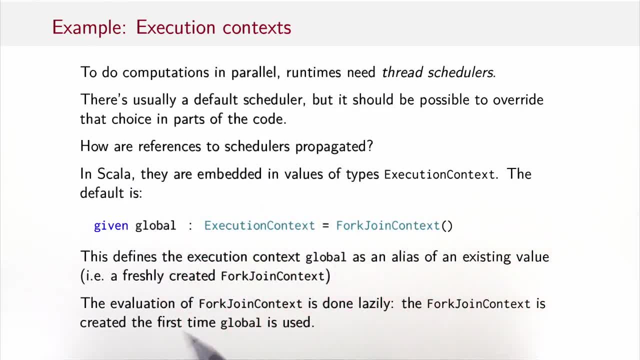 embedded in values of type execution context, The default you see here. so there's a global execution context, which is a so-called fork join context. So that example illustrates a second form of given instances. You can also define a given instance as an alias, like that. 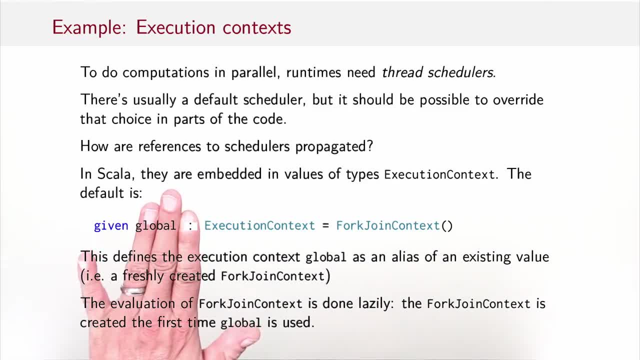 and, as as always, the name is optional, So you could also write: given execution context equals fork join context. What happens here at execution is that the evaluation of join context is done lazily. The fork join context is created the first time global is used either. 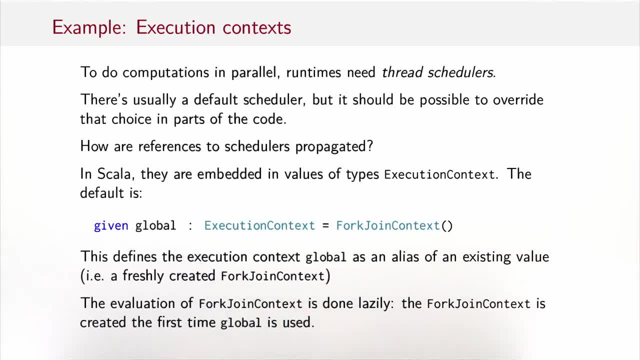 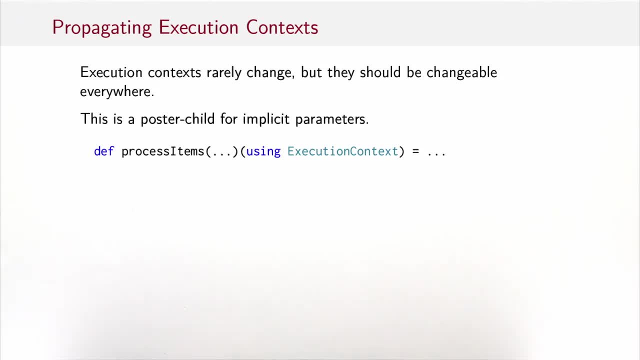 directly or as an argument to an implicit parameter. So execution contexts have this property that they rarely change. Most applications would be happy with the default execution context everywhere, but on the other hand, they should be changeable everywhere, So it should be possible at any point to override the execution context that's given by default and use a custom one. 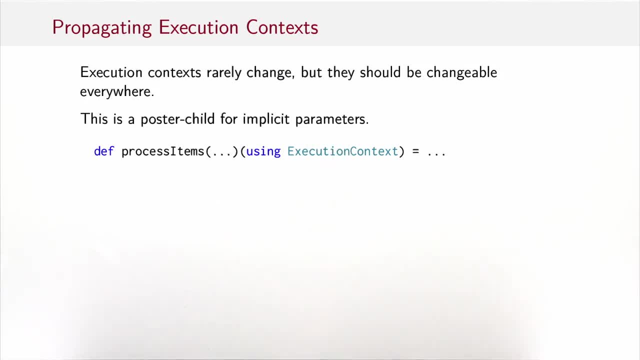 So this profile is a poster child for using implicit parameters. It means that we pass execution context as an implicit parameter to all code that needs it, and usually you'll just pick the execution context from the caller one. but at any point where you need to, you can use a different execution context just by having an 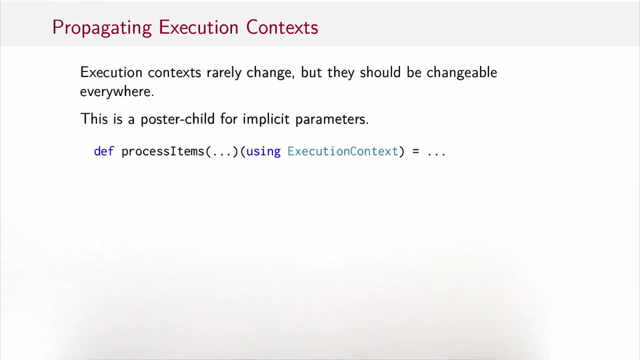 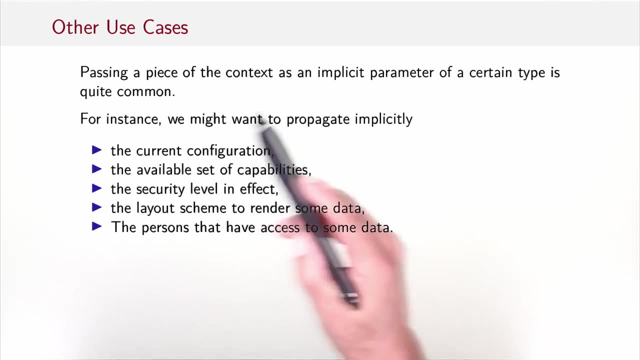 explicit argument here instead of the implicitly synthesized one that the compiler gives you. So that was one example, but there are many other use cases. Passing a piece of context as an implicit parameter is actually quite common. For instance, we might want to propagate implicitly the current configuration or some capabilities and a set of available capabilities or a security. 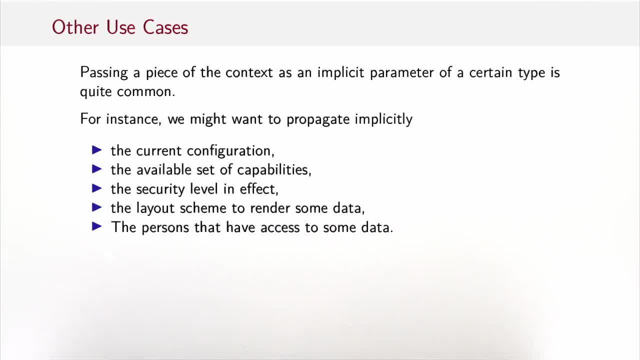 level, or let's say a layout scheme to render some data, or persons that have access to some data, and there are many more examples. In all of these cases, the idea is that a certain information has to be propagated widely to many places in your program and it changes relatively rarely. That means, and of course it should change. 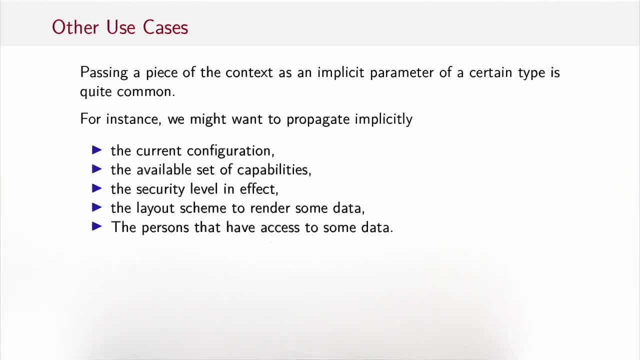 functionally. you don't want to update it. So that means that this piece of information, it gets propagated down the call graph in the trees and it's always the same point. you might want to change it and then in the subtree there will be a change, and at another. 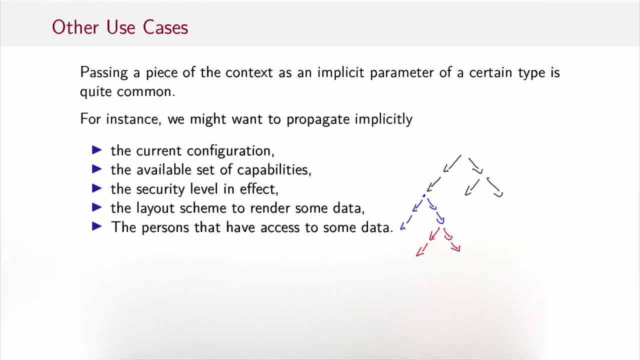 point. you might want to change it again and so on, But these changes would happen rarely because otherwise, if they happen often, then the right choice is an explicit parameter. It matters what the value of this parameter is. It's only if that, if the usual case is that it's just the same- that 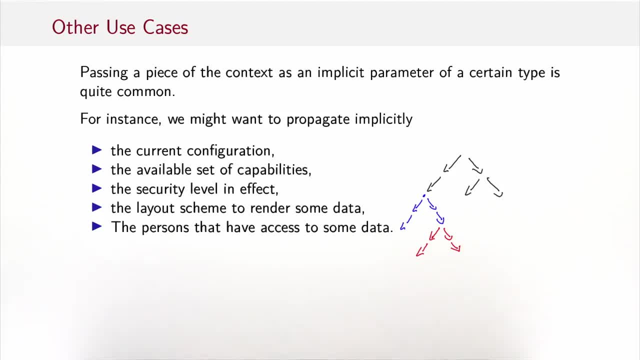 we want to suppress the noise. we don't want to pass it everywhere explicitly If it's everywhere the same. So as this example implies, implicit parameters and context passing really are important for larger systems, Small systems rarely need them, So let's do a slightly. 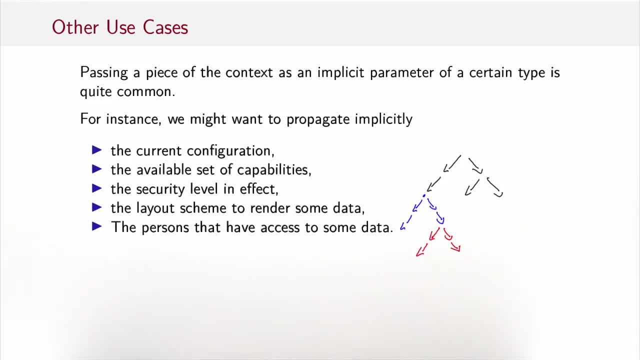 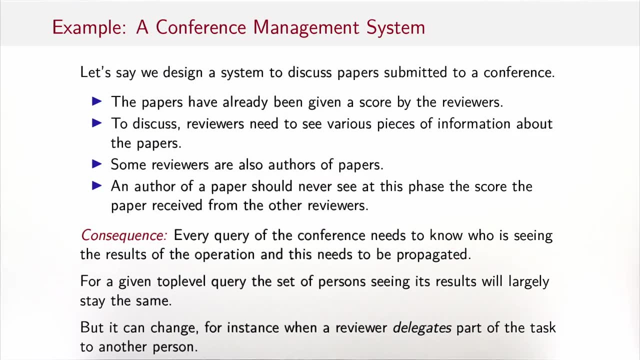 larger application that points to essentially something even bigger, and what we want to track here is persons that have access to some data. So what we are going to do is a conference management system or, to stay modest, just one part of a conference management system. So we want to design a system to discuss papers submitted to a conference and we assume that the 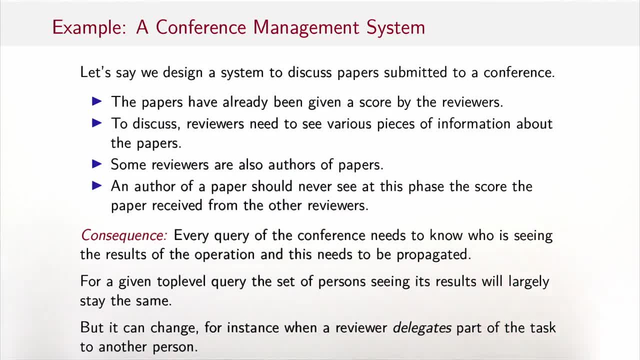 papers have already been given a score by the reviewers. That's another part of the conference system that we leave out here. So to discuss, reviewers need to see various pieces of information about the papers, But some reviewers are also authors of papers and an author of a. 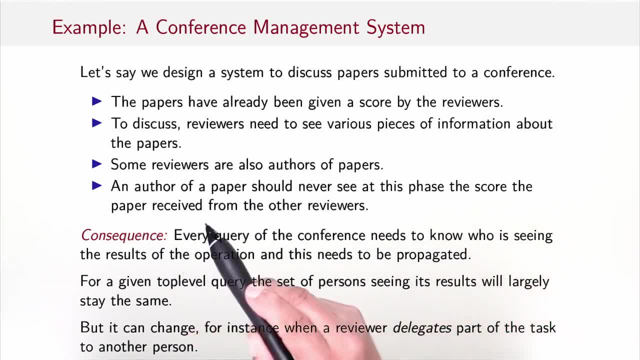 paper should never see, at this phase, the score the paper received from the other reviewers. The consequence of this is that every query of the conference needs to know who is seeing the results of the operations, and this needs to be propagated everywhere, Because if one of the persons who sees 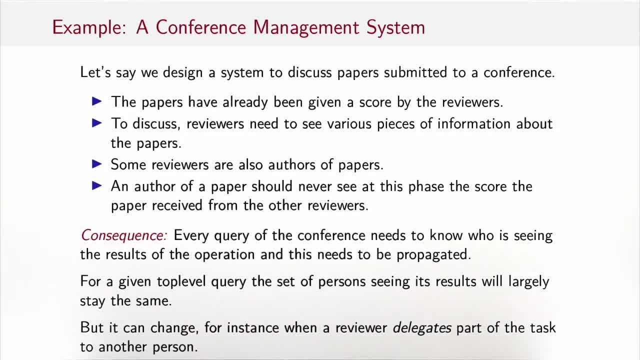 the result of a query is the author of a paper, then that person shouldn't see the real score of the paper or be able to infer the real score of the paper. So some action has to be taken, and for that action to be taken we need to know first who is seeing the results of an operation. 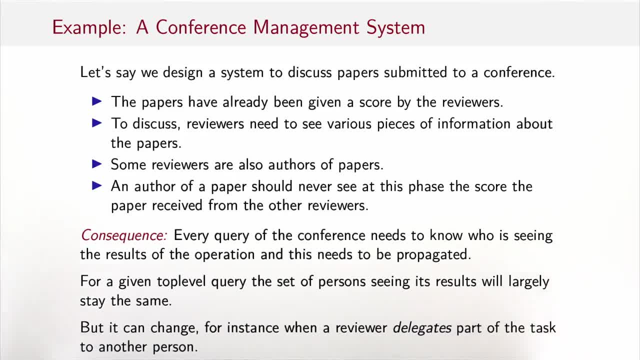 For a given top level query, the set of persons seeing its results will largely stay the same. So I initiate a query and then basically, it's just me who will see the results. But that's not always the case. There are scenarios where we imagine this could change. For instance, I could delegate part. 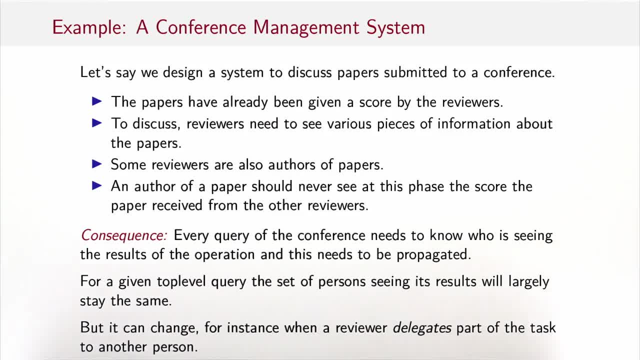 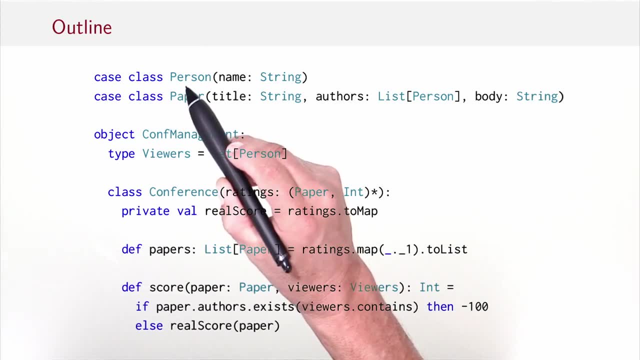 of a task to another person, and if I do that then it's myself and the other person who has access to the scores of that paper. So if either of us is the author, then the scores should be suppressed. So here's the outline of that conference management system. So we model persons with a 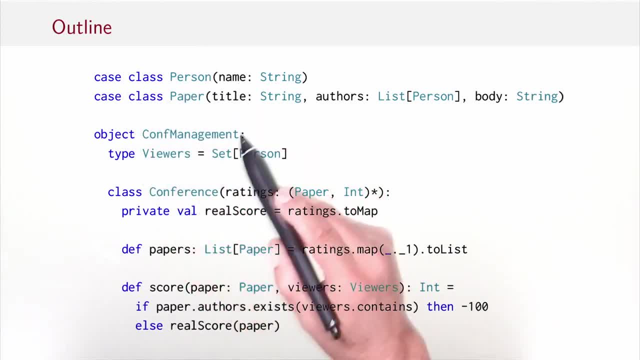 case class and a name. A paper is a case class that consists of a title, the authors, which are a list of persons, and a body. The conference management system itself provides a class conference. that essentially already gets the ratings, So ratings are a repeated argument. 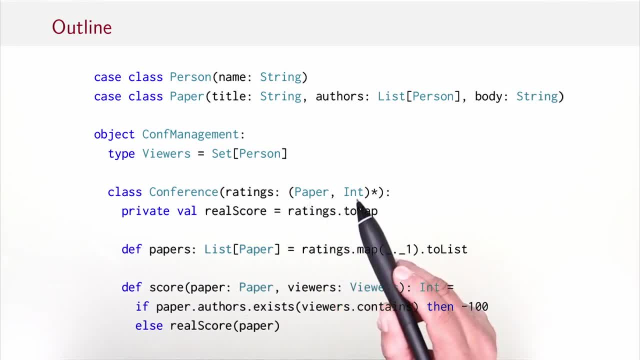 which consists of pairs paper and int, where int is the score. So I can immediately convert that to a map with just two map of the sequence and that would give me the real score of a paper. So the actual score that comes from the actual 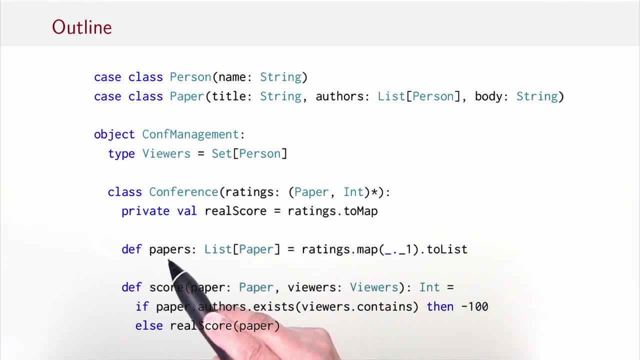 ratings. Then another thing I can compute immediately is the list of papers that have been submitted to the conference, because that's just the first part of the ratings- and convert it to a list. The next function we look at is score, which gives us the score of a paper. 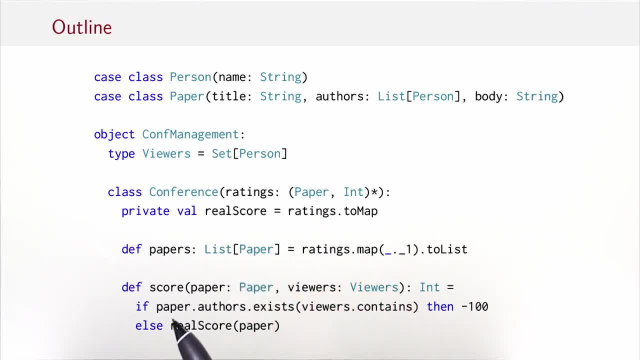 And that's not always the real score, because if there is an author of the paper that is also a viewer of the result, then we should mask the real score. So what we do, instead of giving you back the real score, is just give back a very low made up value minus hundred. 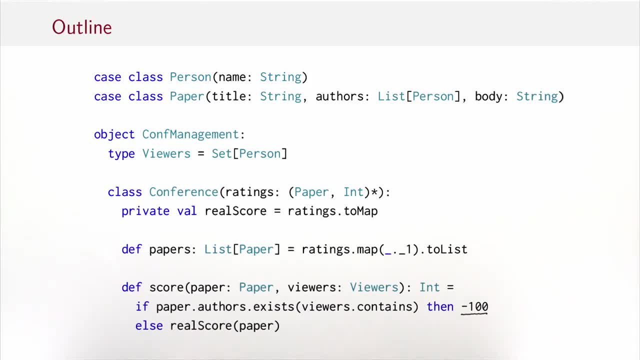 And if that's not the case- so the authors of the paper are disjoint from the viewers- then we give you back the real score. So what this implies is that the scoring function must know who who is the viewer of the paper, And finally we'll see the result of this. 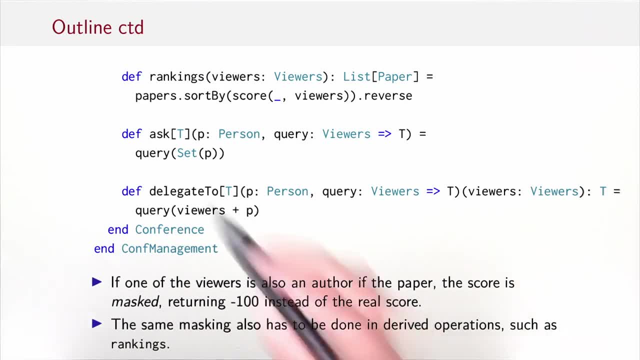 But it's not just score that needs to see the viewers, It's also functions that use score, such as this one. So the rankings functions ranks the list of papers according to scores. So papers with a higher score would come first and papers with the lowest score would come last. 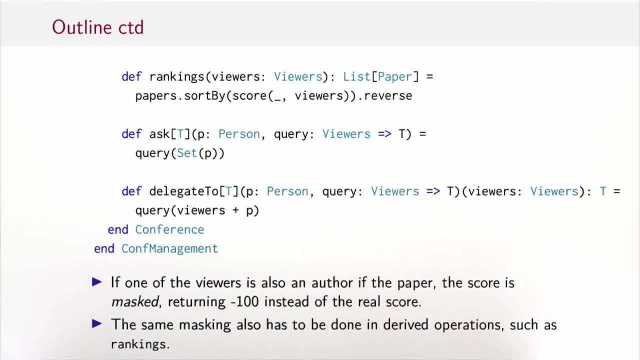 So here's the definition of ranking, So it's papers sort by score in reverse, And of course also needs to know who the viewers are. The next function here is called ask, So that's essentially a top level query. So we have the person who asks a query And the query is a. 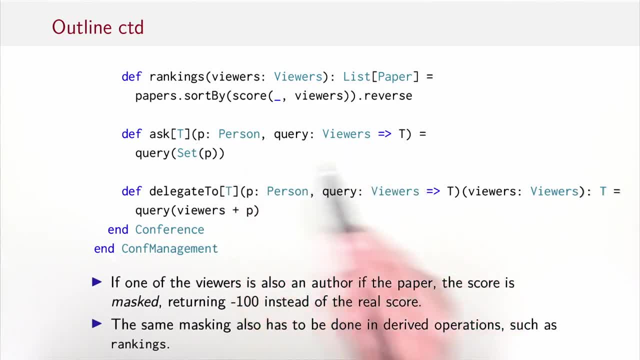 function from viewers to key. So if the person submits a query, the query takes the viewers argument and gives you back the result that the person is interested in, which is a type parameter, so can be arbitrary, And the implementation is simply: we call the query with the person. 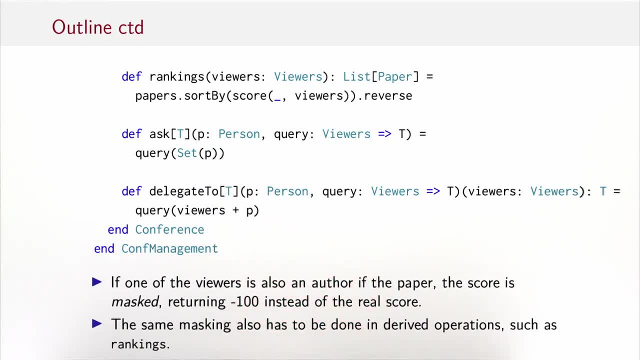 as the viewer. So it's a set of P. And finally we have the delegate to method, which solves the task of delegating a part of the computation in a query to some other person. So query will be run with the current viewers which has to be passed into delegate to. 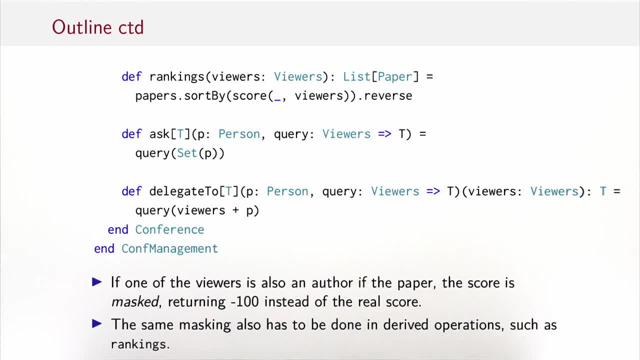 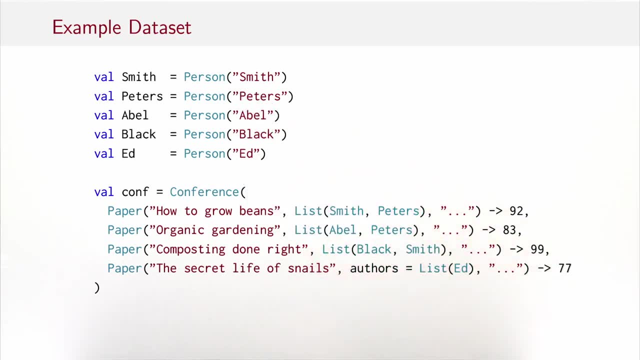 and, in addition, this other person, both the current viewers and person, can now see the scores of the paper. So here we have an example data set. So we have five persons, both reviewers and authors, And we have four submitted papers that you see here. So here's. 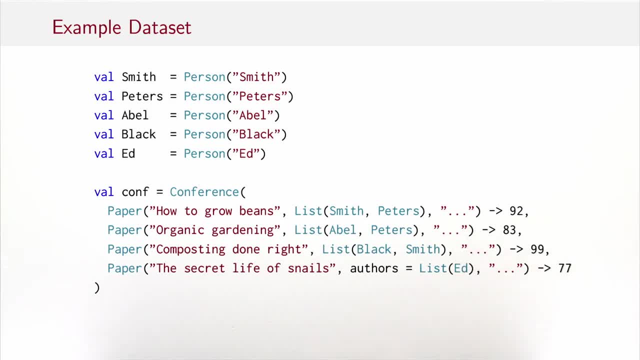 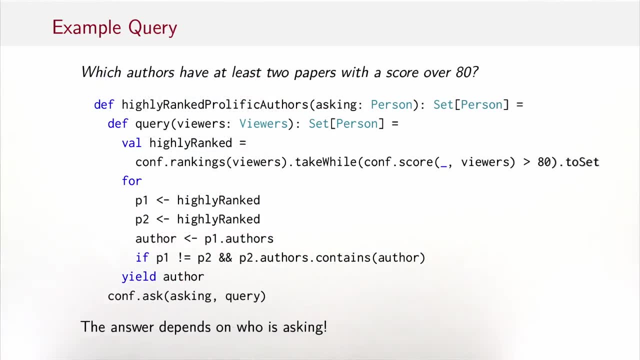 the titles. here are the authors and the body I leave out in each of the cases And they all. each paper has a score that you see here on the right Now. here's an example query. The query is which authors have at least two papers with a score over 80.. 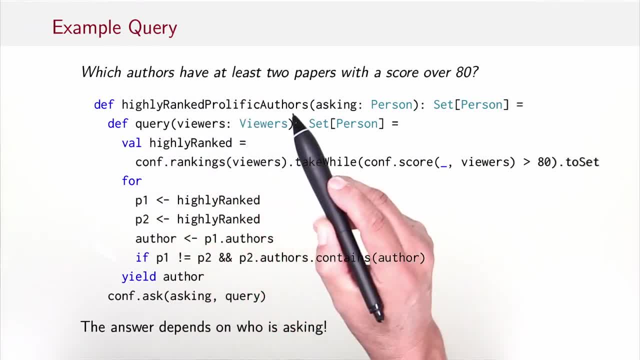 So we define that query in a method- highly ranked, prolific authors- And, as we will see, the record result of that query will depend on who's asking. so we also pass the person that's asking the query as a parameter and we get back a set of persons which 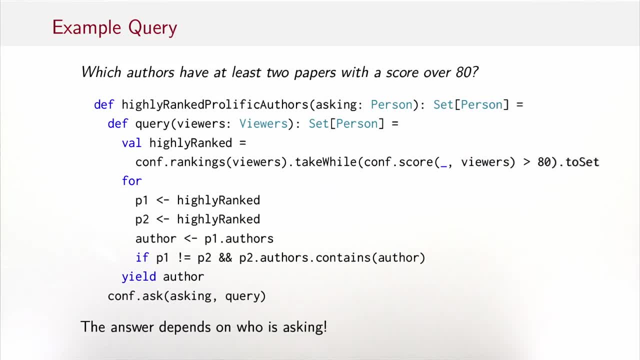 are the highly ranked, prolific authors. so what we do is we ask the conference system with the current person, so that's asking, and this query here that you see here locally, so that query, as every query, has to take a viewers parameter, so a set of persons parameter, and it gives you back a set of persons, so what it does. 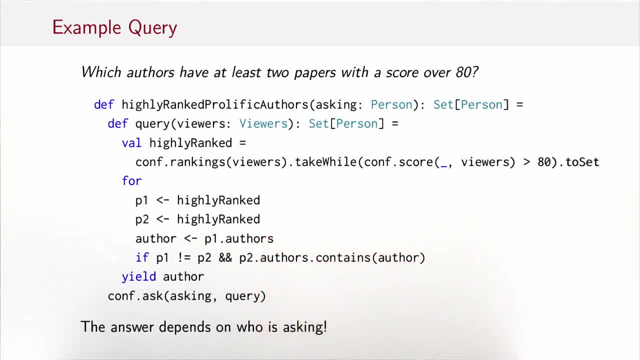 is it first computes the highly ranked papers. highly ranked papers means we get the rankings and we take the top papers, so we have a take, while here top papers means that the score of a paper would be greater than 80, so we take them from the rankings list until the ranking is lower than 80 or equal to 80, and these top 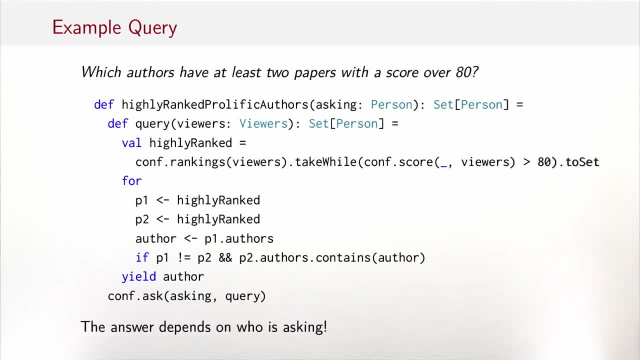 papers are converted to the top papers, to a set here. so once we have highly ranked papers we can complete the query with this for expression that you see here. we let p1 range over all highly ranked papers. p2- the same. we let author range over the authors of paper. p1 if p1. 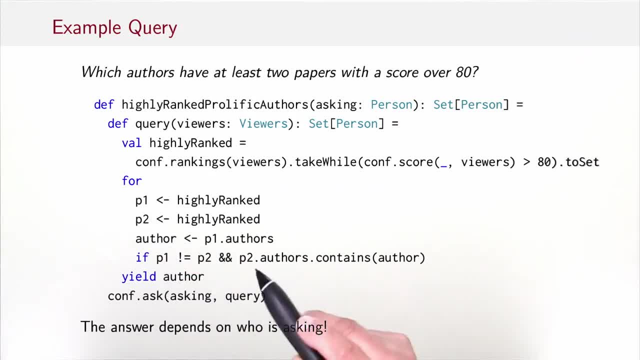 and p2 are two different papers and the author list of paper p2 also contains our author. then the author is a highly ranked, prolific author and we return it. so that's the way it works. so now you see, the rankings function is parameterized with the current viewers, so is the score function. 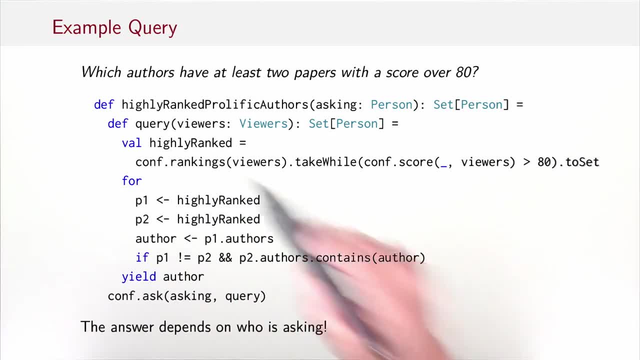 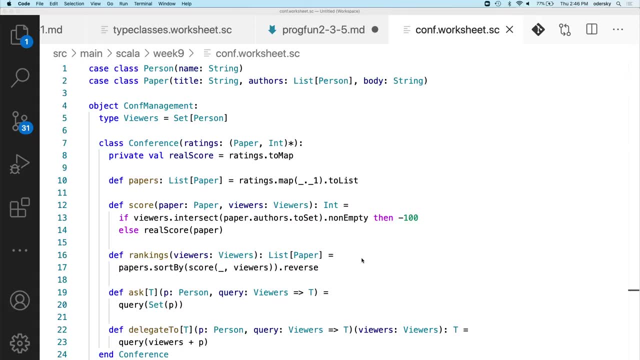 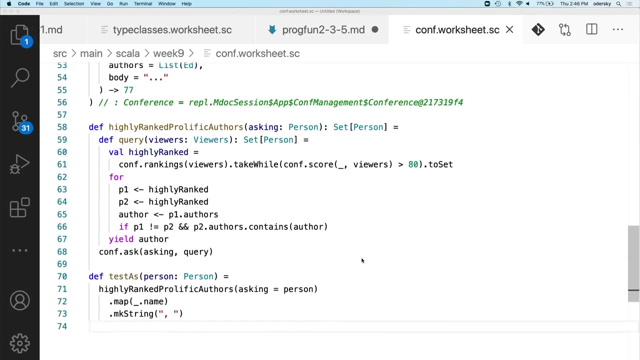 so the answer of these functions will depend on who is the current viewer and that in turn depends on who is asking. so i've put the conference management in the worksheet. you see it here. we have the query here and now we have a test as method which says: well, we called the. 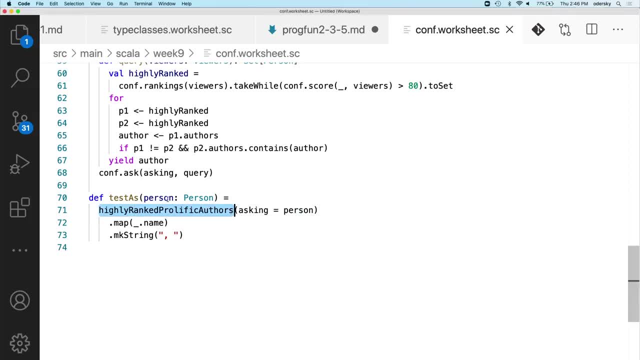 highly ranked, prolific authors, with the given person as the person who's asking, and we just essentially printed out slightly prettified, taking the name and separating with commas. and if we now do run this test as different persons who are asking- so blacksmith, able or red- then you get different answers because 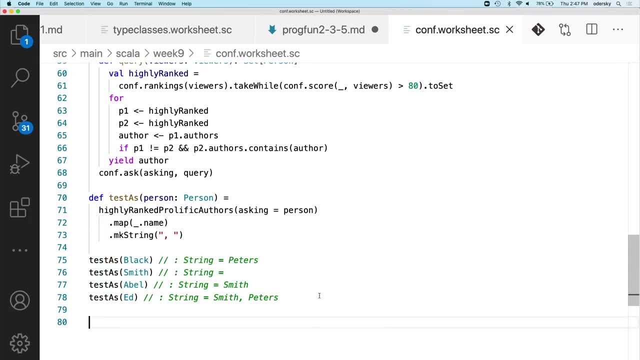 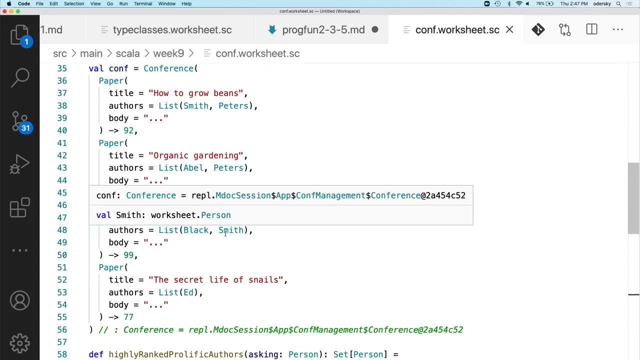 let's say, in the first case, where it's a mrs black that asks: you see, here mrs black is a co-author with mr Smith and that means that she won't see this paper, or the score of this paper will be minus hundred. so that means that the other 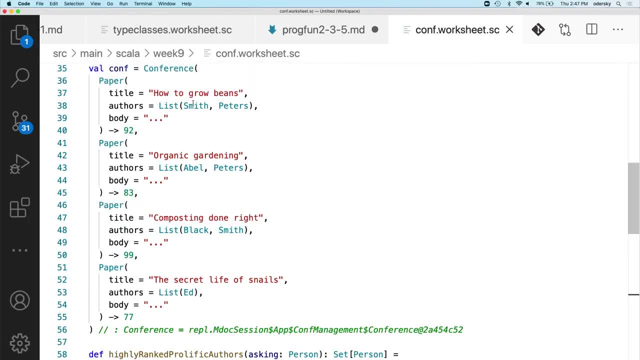 paper of mr Smith, who is a highly prolific author, is is seen, but this one. this one is not so from the viewpoint of mrs black. mr Smith has only seen the first paper of mrs black, so that means that the other paper of mrs 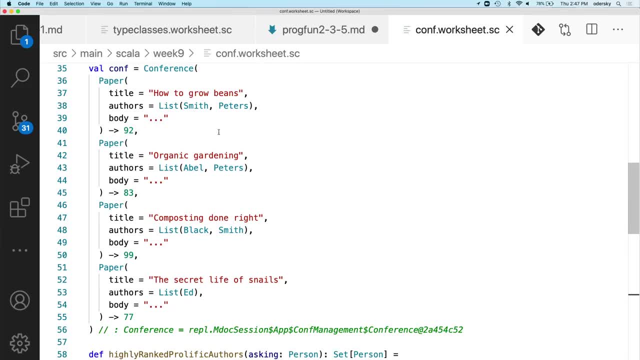 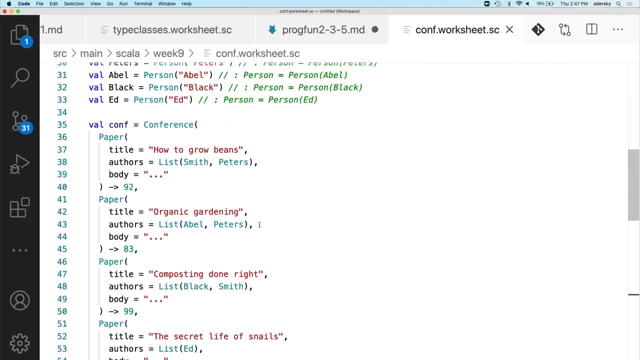 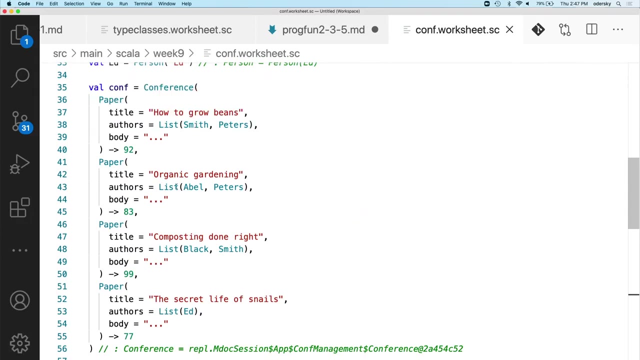 black is only one highly ranked paper, the first one. if we ask as mr Smith, then we'll find that mr Smith is has these two papers, so I can't see their scores, and in the other papers the author doesn't figure. so from the viewpoint of mr Smith they he doesn't see himself as a highly ranked prolific. 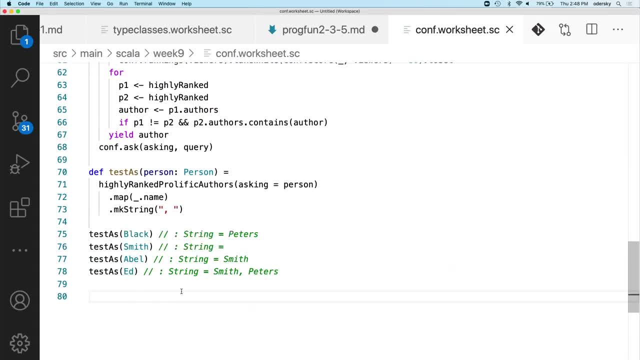 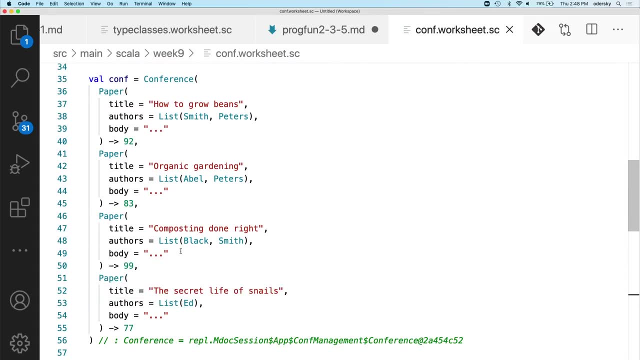 author. and if you finally look at mr ed, so mr ed he is, he he's here, he hasn't published with the other, so he has a complete picture of these first three papers. so for him, both Smith and mrs Peters are highly ranked prolific authors. they both have two papers in the 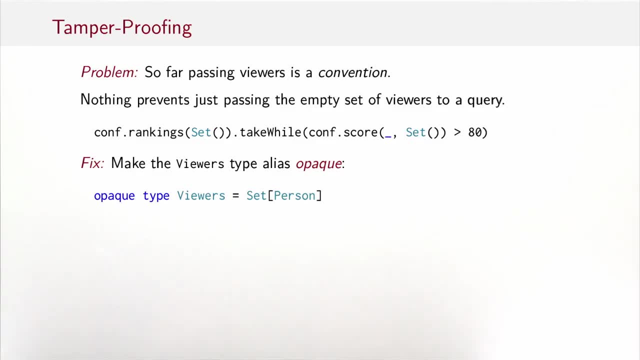 in the list of these three. okay, nice, but there is a problem. so far, passing the viewer set is a convention. that means nothing prevents just passing the empty set of viewers to a query. so our query- highly ranked, prolific authors- could also have looked like that. it would be type correct. we? 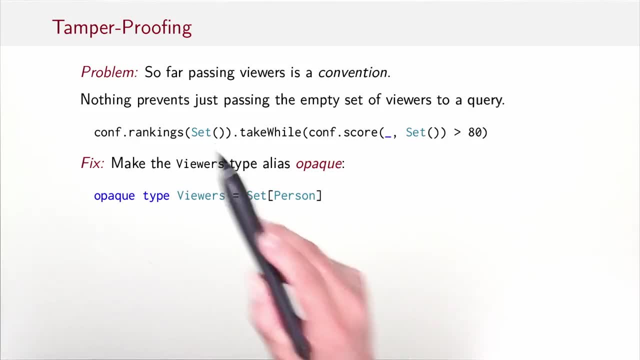 would say: well, we want the rankings and nobody's seeing that really. and and then we take the top ranked papers according to the score, which again, nobody is seen. that's a lie, of course, but the type system will not catch us out with that, so we can fix that by making the viewers type, alias opaque. previously we've seen: 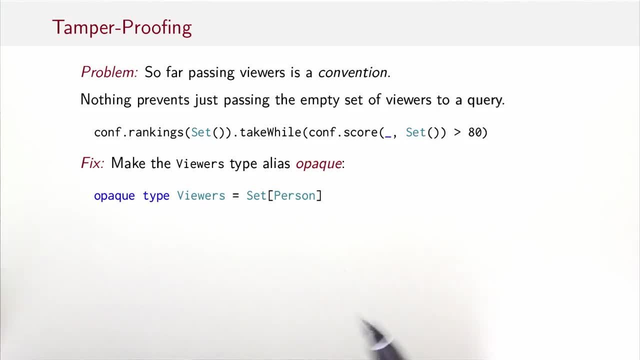 that viewers was just an alias for set of persons and that's something that essentially is for everyone to see, so we can everywhere freely exchange viewers with set of persons. the left-hand side and the right-hand side are the same, but if we write the type alias with an opaque modifier that you see here, then 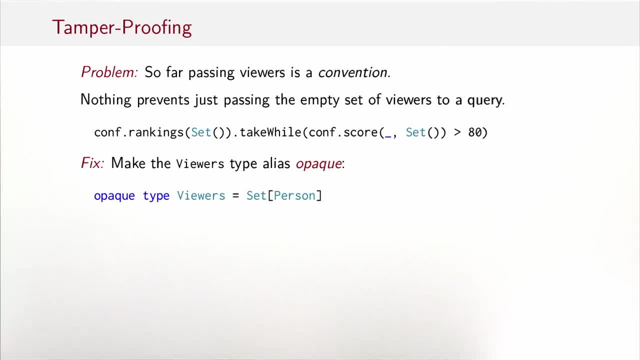 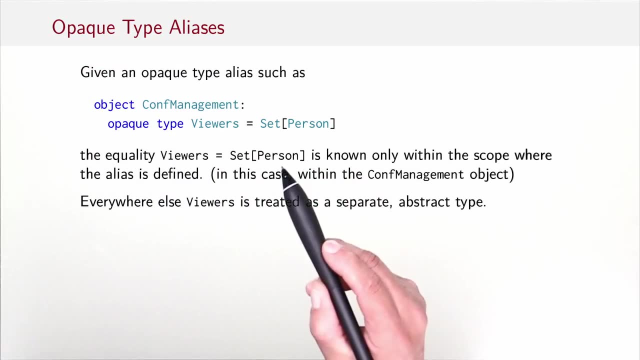 it becomes an opaque type alias and the rules change. in fact, given an opaque alias such as this one here, the equality that viewers and set of persons is the same is known only within the scope where the alias is defined, in this case within the conference management object, everywhere. 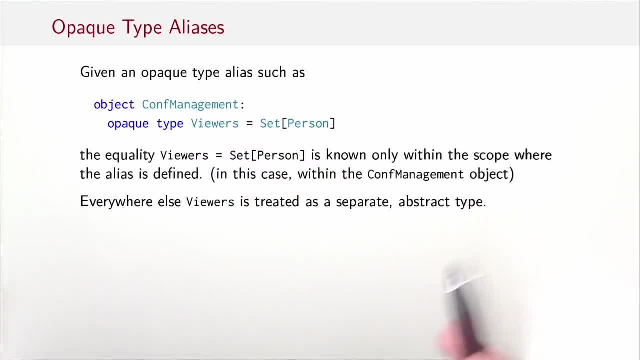 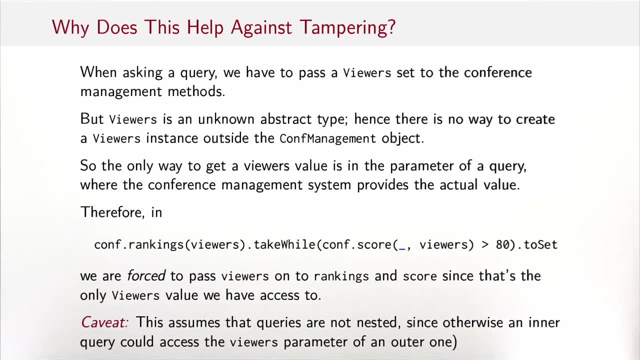 else viewers is treated as a separate abstract type. so it's just a new type about which we know nothing. we certainly do not know it's an alias of set of person. so if we do that, how does it help against tampering? well, when asking a query, we have to pass a viewer set to the conference management methods like 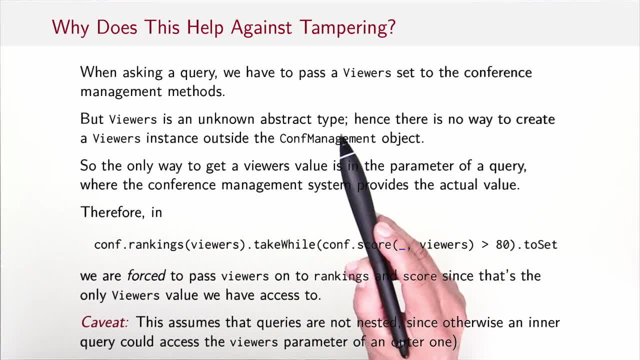 rankings or score, but viewers is an unknown abstract type. now so. but because the queries are formulated outside the conference objects, viewers for them is an unknown abstract type. hence there's no way to create a viewers value outside the conference management object. so the only way to get a viewers value is in the 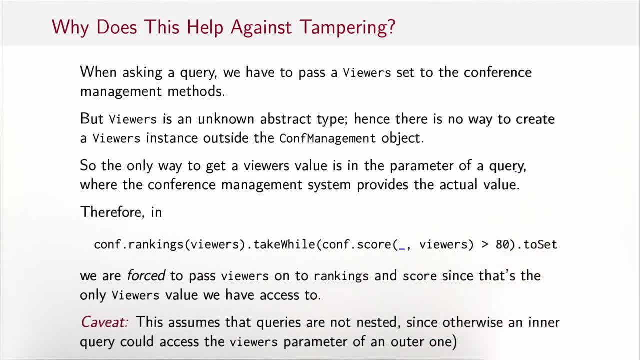 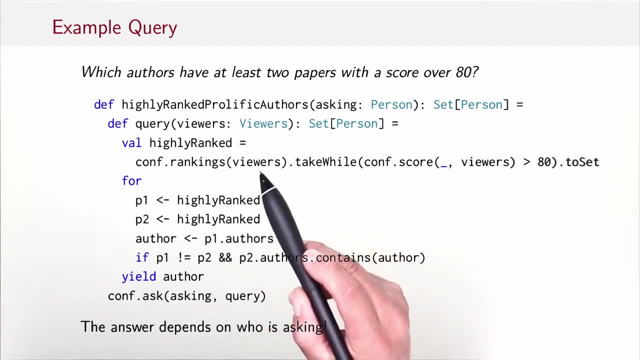 parameter of a query where the conference management system provides the actual value. so that means in this query here, we are forced to pass viewers here and here because that's the only viewers value we have access to. indeed, if you look here, so if we can't create a viewers value, then the only viewers value we see is 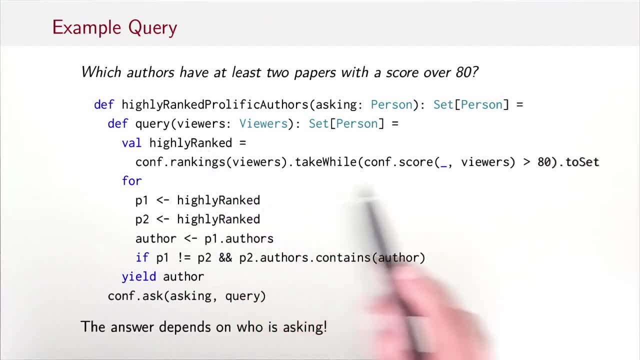 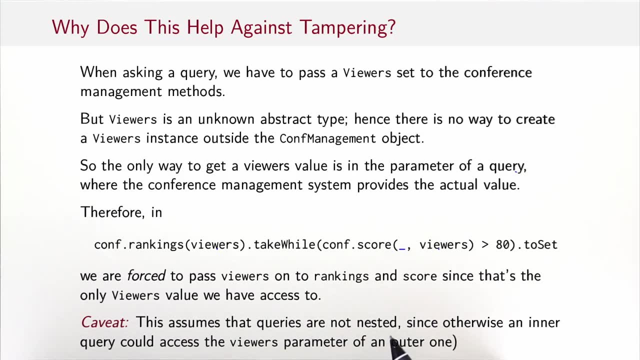 that one here in the parameter of the query, so we're forced to pass this on to rankings and score. there's a caveat that actually works only if queries are not nested. if queries would be nested, then we would have a choice. we could pick an outer parameter of an outer query or a parameter of an inner query, so that 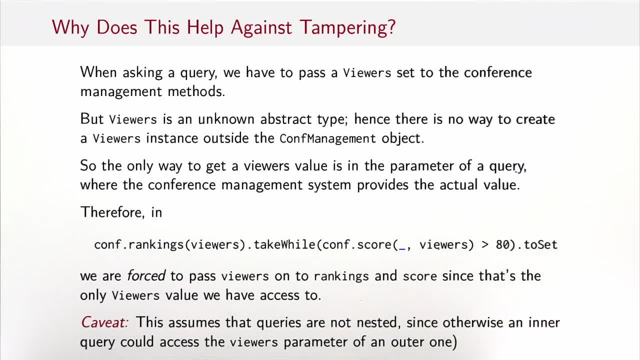 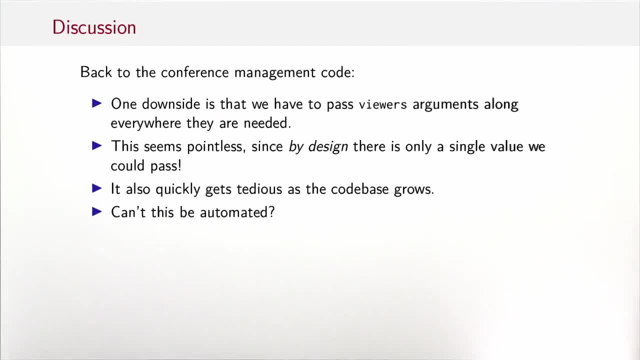 would still allow cheating. so for the moment let's assume that queries are not nested, that every query we formulate is a top-level query. so let's look back to the conference management code. one downside is that we have to pass viewers arguments along everywhere they're needed, and that's tedious and it also 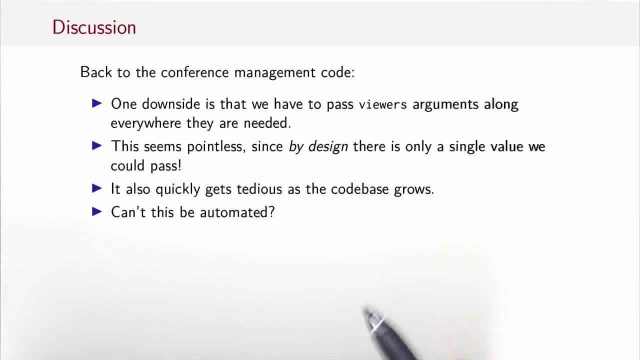 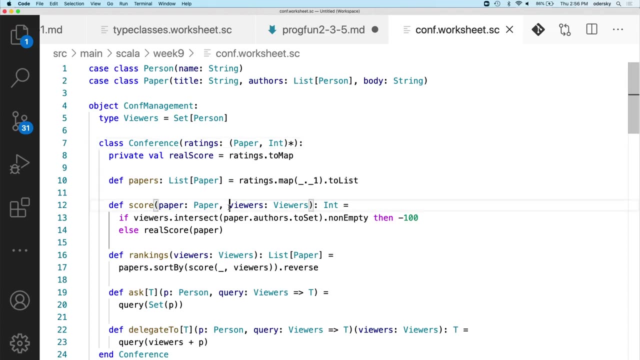 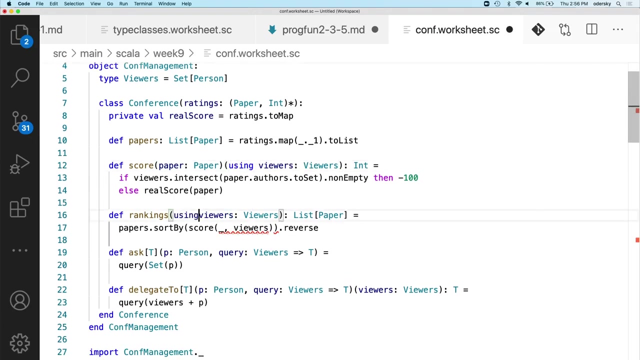 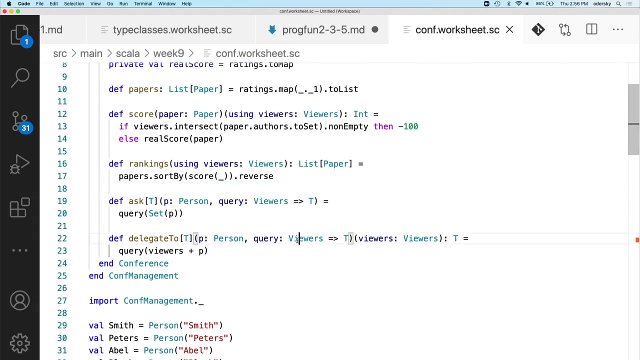 seems pointless, since, by design, there's only a single value we could pass. so the question is: can't we automate that? and the answer is, of course, just use implicit parameters. so let's apply this change to the worksheet: we make every viewers parameter a using clause and at the same time we avoid explicit arguments. 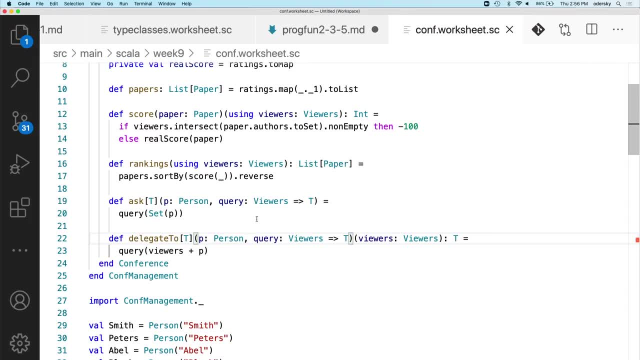 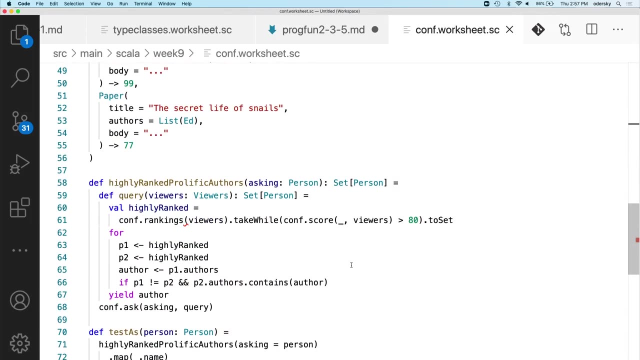 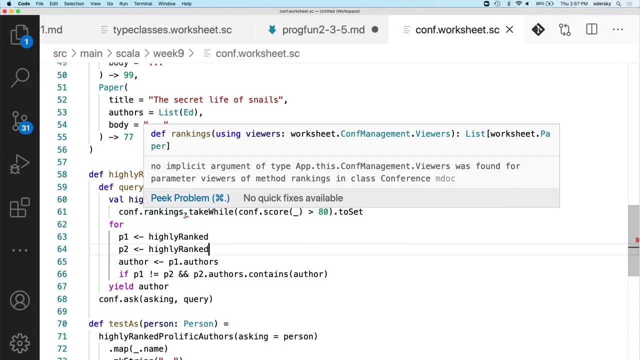 with viewers because they can be passed implicitly now. so we still have a problem here. it says that there's no implicit argument of the viewers type available, and that's because here we actually haven't passed the viewers type and we have to pass the viewers type, and that's because here we actually haven't. 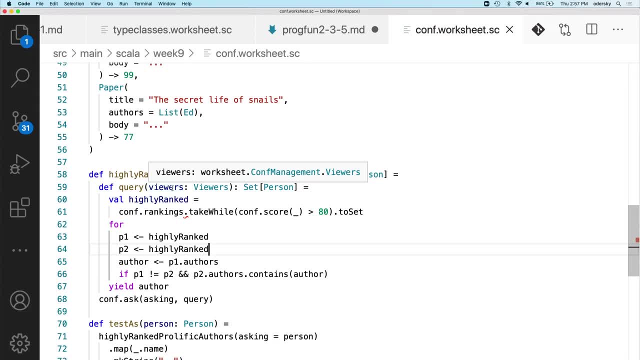 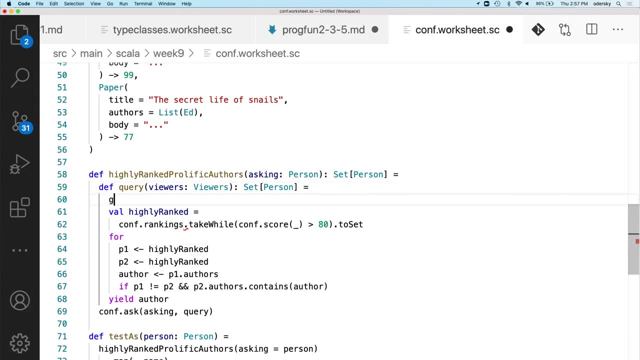 passed the viewers type, and that's because here we actually haven't made viewers a using clause, because that was essentially the function type prevented us from doing that. so we need to correct that by essentially making it a given instance. that's possible implicitly, so what we can write is given. 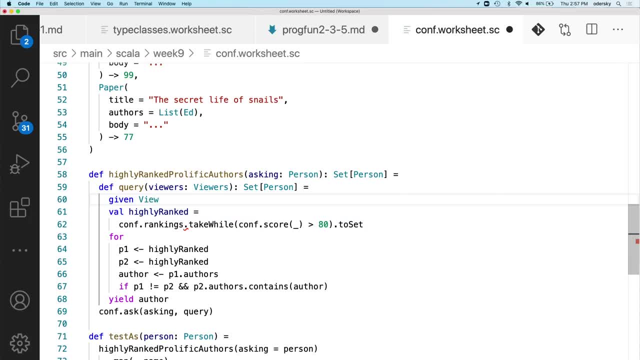 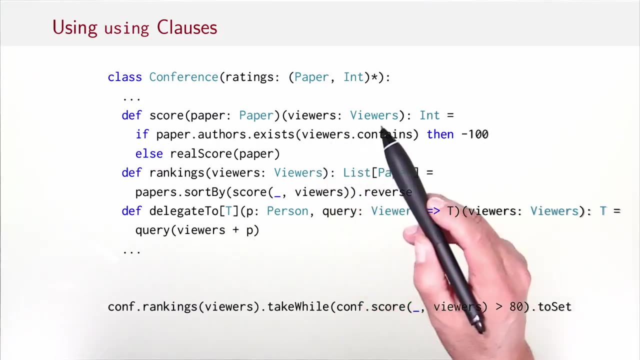 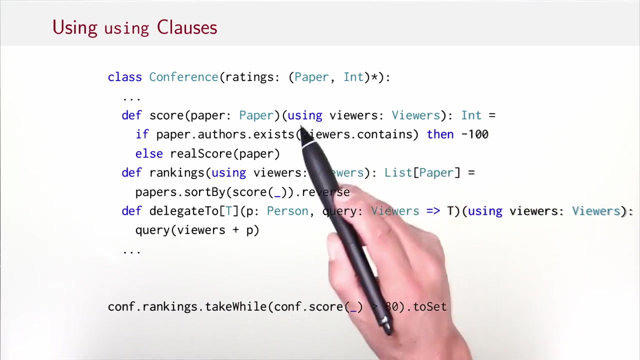 viewers equals viewers, and that's it. so now things are good, okay. so what we've done is we have we have changed every explicit parameter- viewers- to a using clause, and we have have omitted the actual arguments that refer to these viewers. so we've, in a nutshell, gone from this to this, so the parameters get the using. 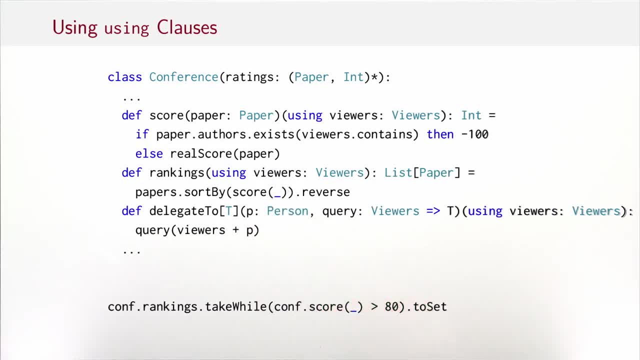 keywords and the applications get the viewers arguments dropped. so here we have viewers in score and now it's gone. and here's, here's the same thing. so there, we pass viewers twice, but afterwards we don't need to do that anymore. so you might say, adding all these, using clauses, just to save three. 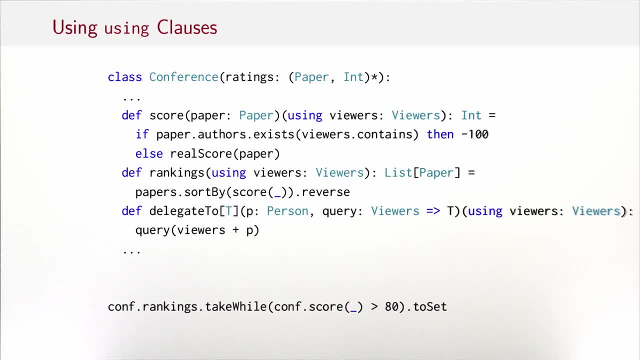 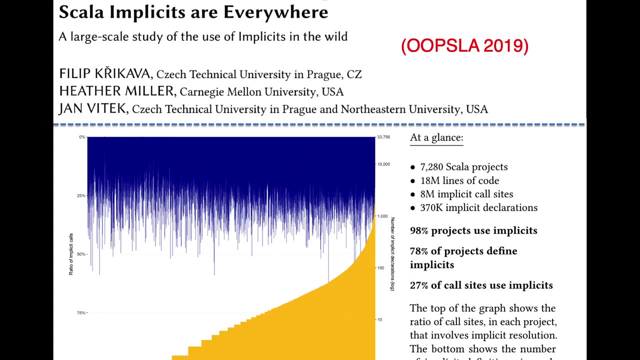 explicit arguments is not really worth. it is it, and I'd have to agree with you. but remember, this is sort of a extremely minimized natural system. real systems are much, much larger and you would have many, many more implicit parameters where the savings would actually add up. so data about this have been collected in. 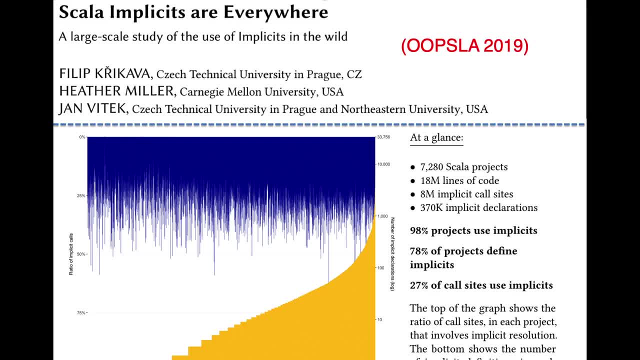 a paper called Scala implicits are everywhere and that appeared at the Uppsala conference in 2019. it analyzed a large body of code consisting of 7,280 Scala projects with together 18 million lines of code, and it found that 98% of 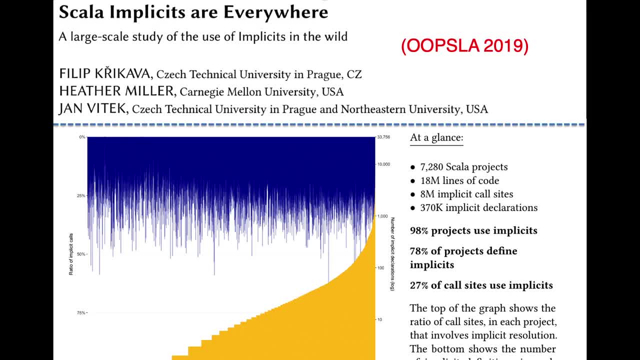 projects use implicits, 78% of projects define implicits and 27% of call sites use implicits. so it means these 27% of call sites. if they all had needed explicit parameters, then that would lead to a significant blow-up in code size for these projects. 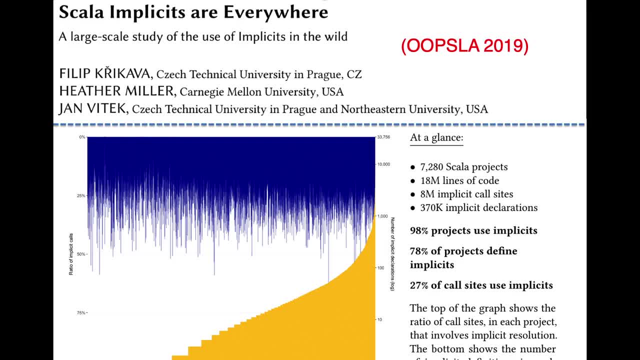 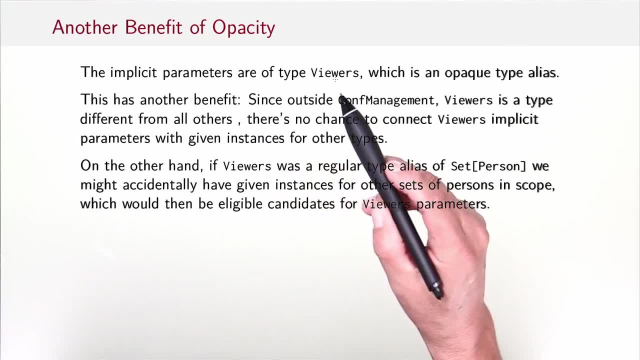 implicit really do save a lot of tedium and repetition in these real-world code bases. so in our case, the implicit parameters were of type viewers, which is an opaque type alias, and that has another benefit: since outside conference management viewers is a type different from all others, there's no chance to 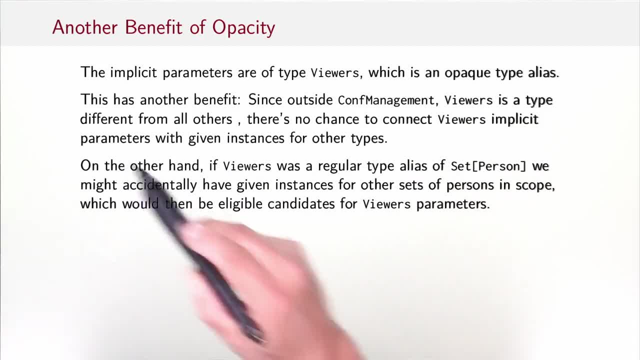 connect the viewers implicit parameter given instance with given instances for other types. on the other hand, if yours was a regular type alias of set of persons, we might accidentally have given instances for other set of persons in scope, and then we would get crosstalk. we would then get sets that are not 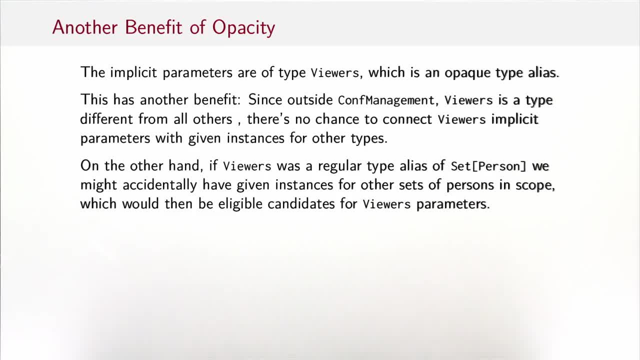 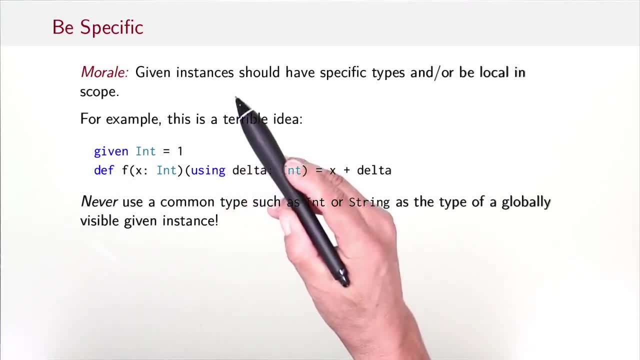 intended as eligible candidates for viewers parameters that are eligible nevertheless. so that's a problem. so the moral of that is that, given instances that you defined, should have specific types. that means types that are don't appear very often in the rest of the program, outside this use case of passing implicits, or there should be. 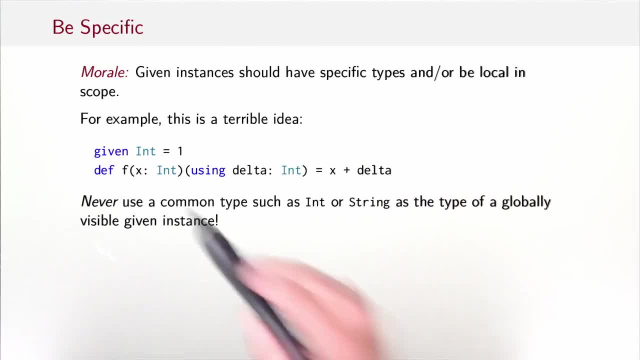 local in scope, or there should be both. So, for instance, this would be a really terrible idea that you write a global given int equals one, so that means we have a default integer- that's one- and then use that in some functions, like this f function that uses a delta and returns x plus. 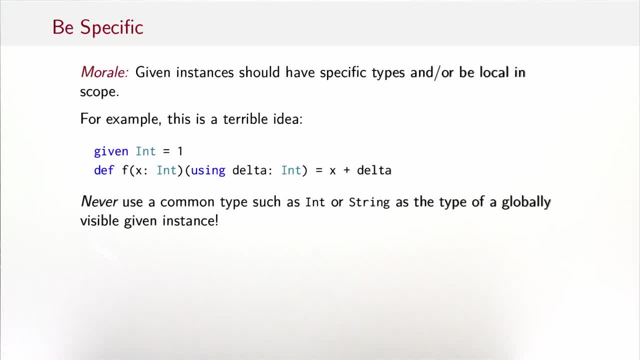 delta. That's really bad because you can do that once in your program, but if somebody else does the same thing then you would get spurious, ambiguous instances and generally a huge mess. So never use a common type such as int or string as a type of a globally visible given instance. 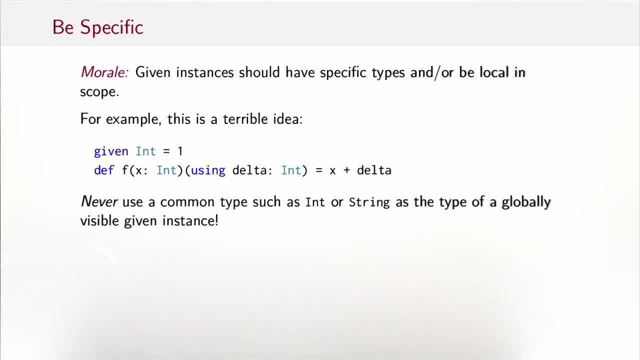 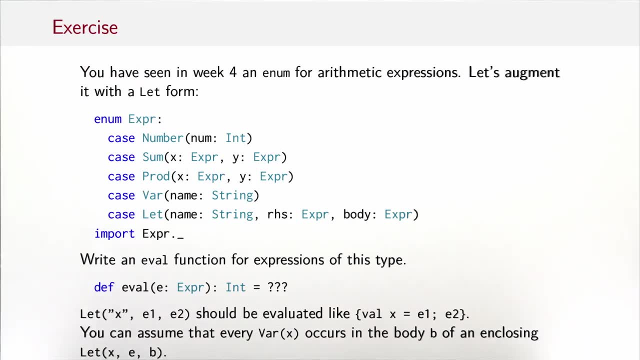 The best thing is you define your own class that essentially lives mostly for being passed as an implicit, or you define an opaque type. So here's an exercise You've seen in week four of the first course, an enum for arithmetic expressions. It consisted of numbers, sums, products and variable cases. That's augmented with a let form. 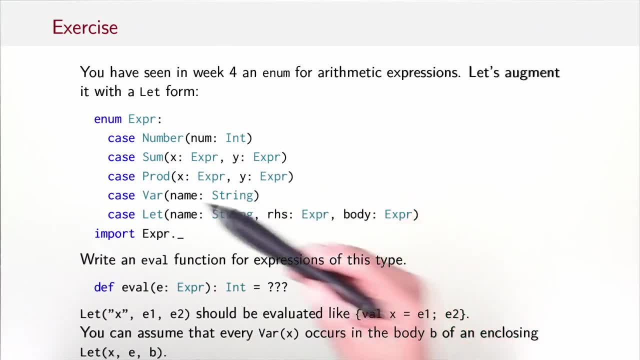 So now an expression is a number or a sum of two expressions, or a product of two expressions, or a variable with a name or a let binding that says the variable with this name is defined to be this right hand side in the scope which is given by this body here. 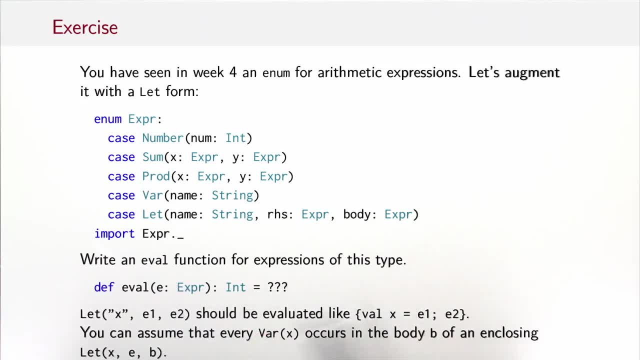 The task is to write an evaluation function for expressions of this type. def eval takes an expression, returns an int, and you should fill in the triple question marks here. So this let node, let x, e1, e2 should be evaluated as you would evaluate in Scala: the block val x equals e1. 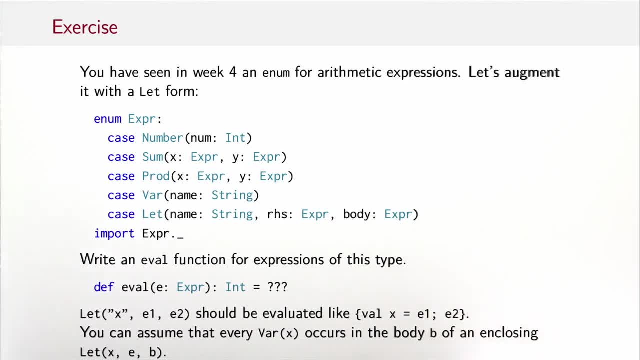 and then e2.. And you can furthermore assume that every variable x occurs in the body b of an enclosed closing let x- e2.. So you can furthermore assume that every variable x occurs in the body b of an enclosed closing let x- e2.. 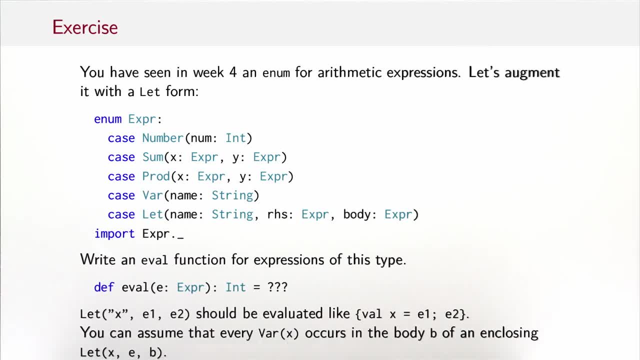 So that means it won't have variables that don't have an enclosing definition. I have a hint for a solution on the next slide. If you want the hint, then keep viewing. If not, you might stop the video here. So here's the solution hint. 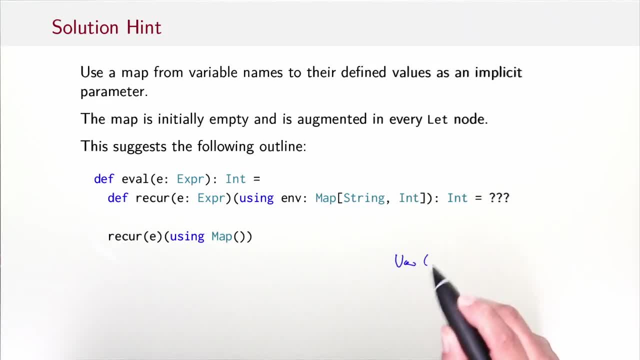 One issue we have is that, given a var node like var abc, we need to know the value of abc. So we'd have to look in an enclosing, let binding that defines abc. So how do we figure that out? Well, the idea is to use a map from variable names to their defined values. 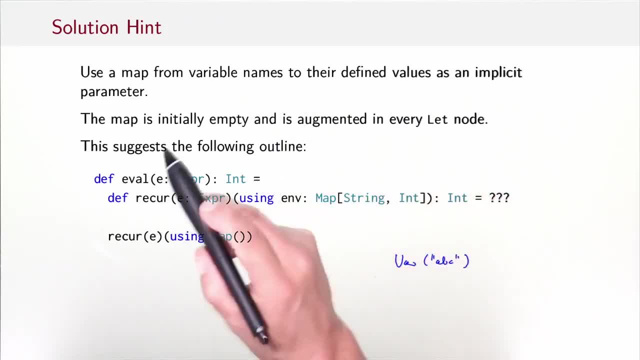 and to use that map as an implicit parameter. Initially the map is empty, no variables are defined, and at every let node, like here, we augment the map with the binding that is here the right hand side r. So this suggests the following code outline In our evaluation function: 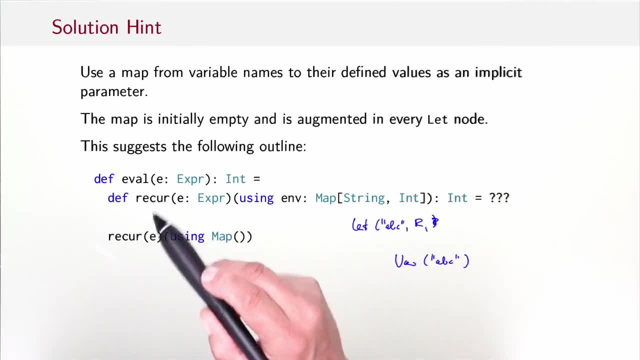 we have a local function called that recur, because it has to be defined in the right hand side, the actual recursion, going through the expression tree. It takes the actual expression to evaluate and it also takes this environment, which is a map from strings to int, and it returns an int. 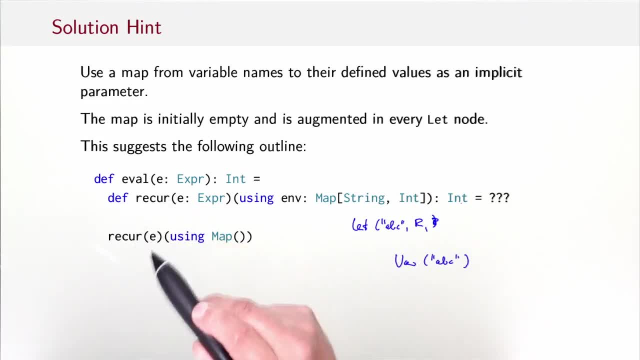 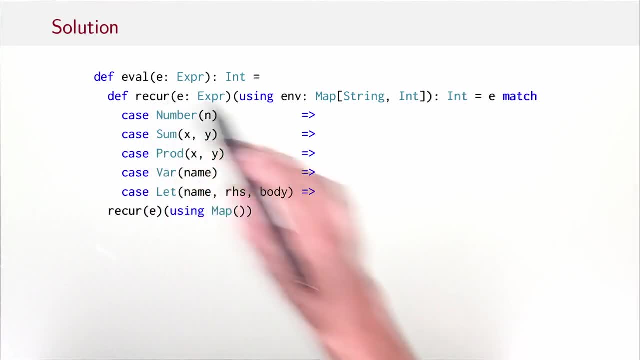 Then we start the computation off by calling recur with the original expression and the empty map. So let's develop the solution step by step. We have our original outline, we have the recur function and it's pretty obvious that we would proceed by a pattern. 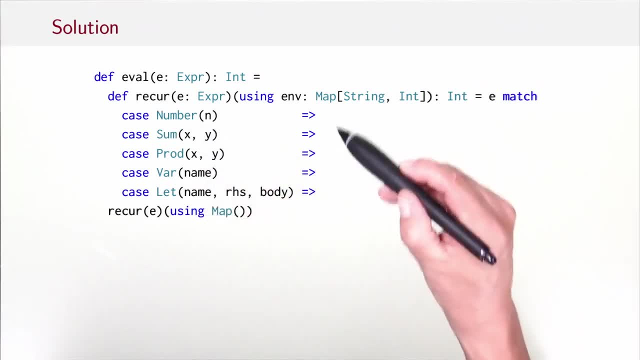 match on what the expression is. So we have five cases and we have to fill in all five of them. If the expression is a number, then its value is just the number that's stored in the node. If the expression is a sum, then the value is recur x plus recur y, Both recurrences. 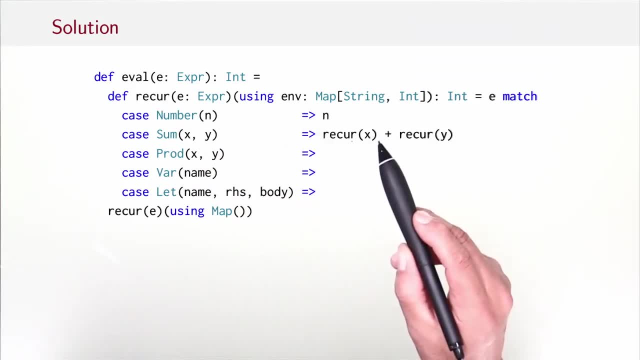 of course need an environment, but that environment is passed implicitly. You don't need to write it here. in the same vein, Product x- y. The value of the source function can also be added to recur y. in the expression value is recur x times recur y. Now what's the value of a variable? Well, we need to. 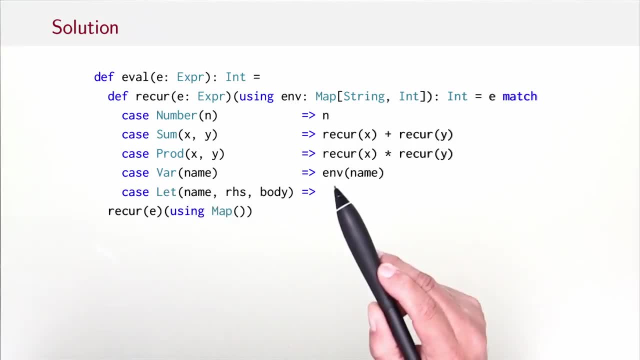 look it up in the environment. We say the value of a variable is whatever is the entry in env under that name. And since we assume the global condition that every name is declared, we know that every name will be in the map and we can use a map apply here safely. Otherwise. 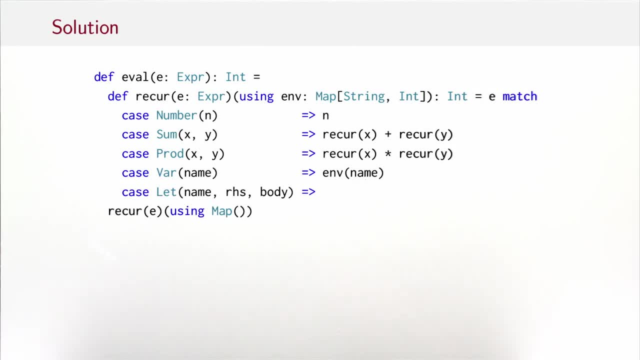 we would have to use an environmentget name and handle the error case appropriately. Finally, for a let node like this, the result is a recur of the body part using an augmented environment. So the new environment is the old one, env, and the additional binding that. 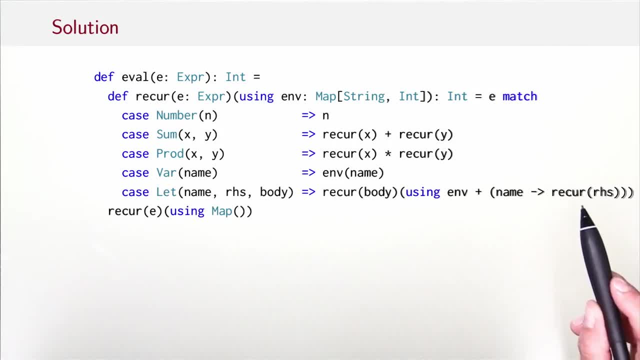 the name here has now the value that's given by recur of the right-hand side. So we compute the right-hand side with recur, Combine it with the name, add it to the environment and compute the body with that augmented environment. So again you might ask: well, was it worth using an implicit argument for the environment? 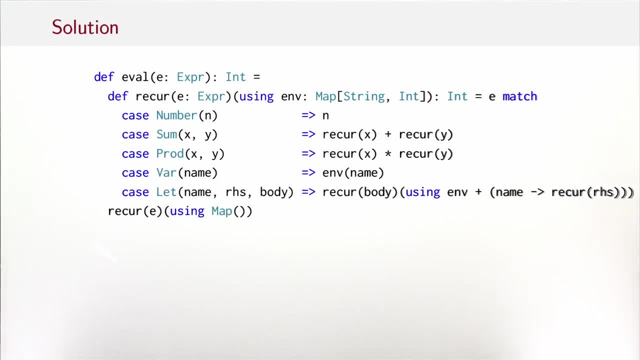 And I guess in this small example not. But again, this example is just essentially an illustrator for something much larger. A real compiler interpreter would have maybe not five cases but 50. And it would not call itself or something else that needs the environment. 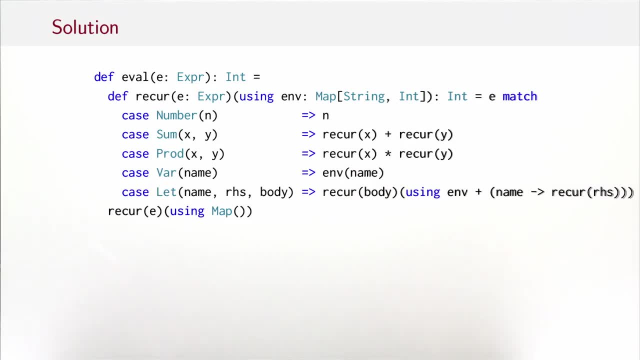 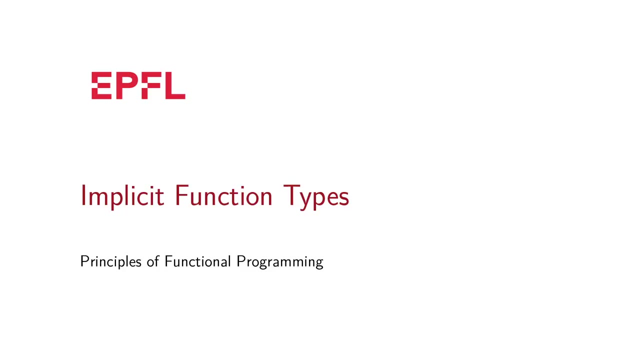 twice, But dozens of times. So then of course these things multiply and you get numbers where it's really worthwhile not to have to pass the environment manually to every little nook of your computation graph. In this session you'll find out ways to streamline our contextual abstractions even further. 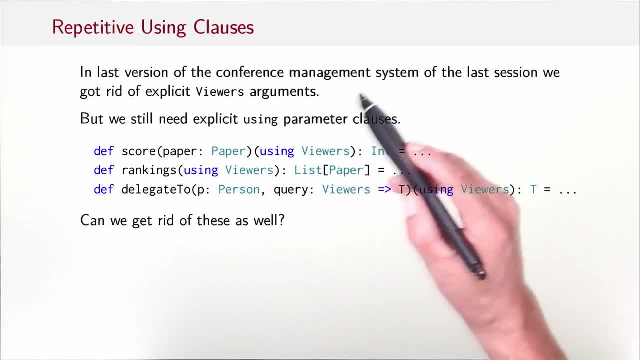 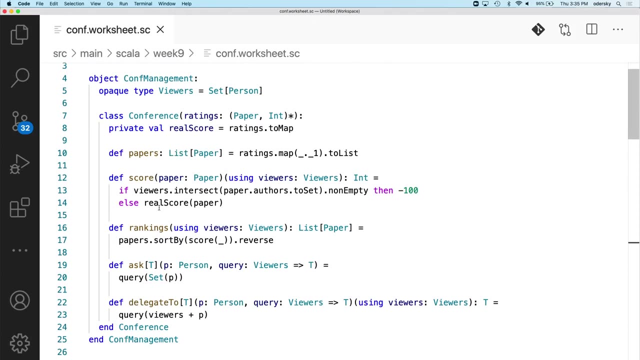 using implicit function types. In the last version of the conference management system of the last session we got rid of explicit viewers' arguments, But we still need them for using parameter clauses. So if I look at the worksheet here, then score rankings, delegate2, all have these. 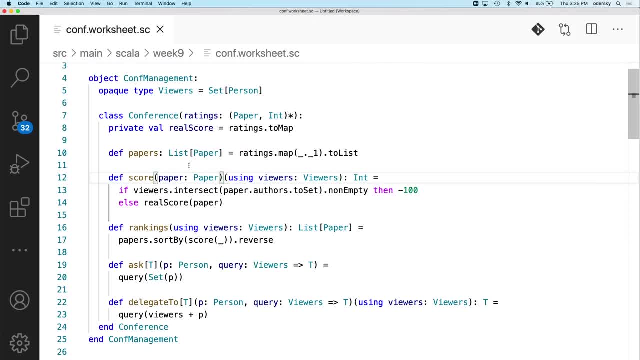 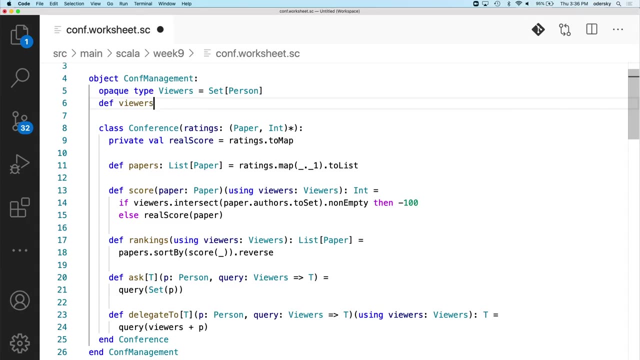 additional using clauses to track the set of viewers. One thing we could do to make this slightly more streamlined is to avoid the names of the viewers' parameters. Okay names. we just define a new global viewers function that takes the viewers and returns it. So now, essentially whenever we have an implicit viewers in, 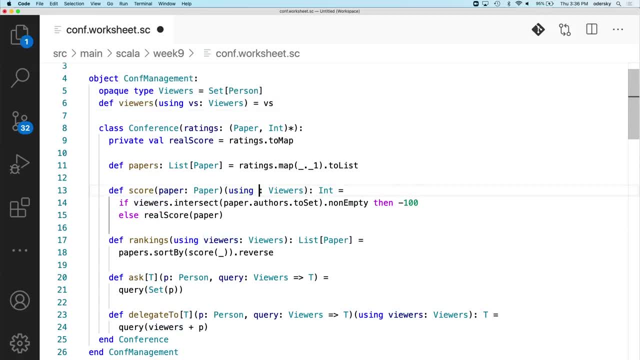 scope. we can just refer to it with this viewers function and consequently we don't need to name the parameters anymore. That's a trick that one can basically apply everywhere. one does context passing, So now it looks slightly more streamlined, but of course there's still the overhead of writing these. 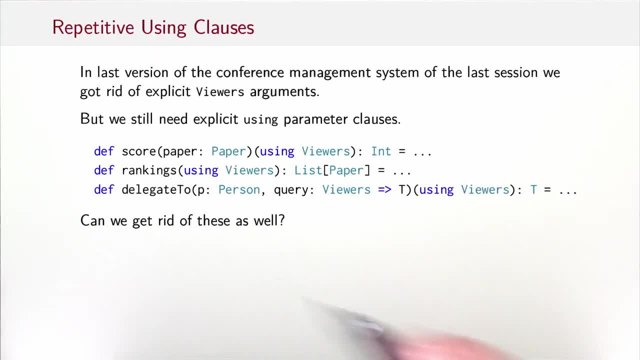 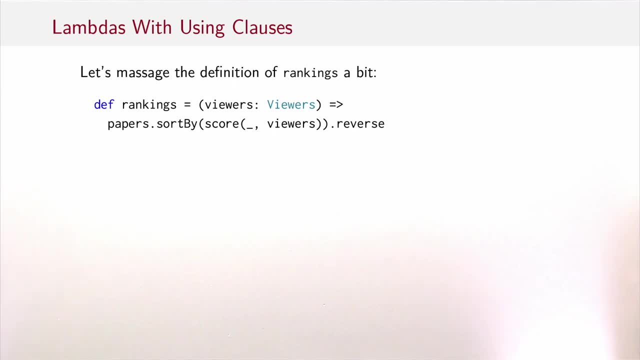 anonymous using clauses. So the question is, can we get rid of these as well? So to get to an answer, let's massage the definitions of rankings a bit. You know from the first half of the course that we can write any function with parameters. alternatively, as a function without any parameters, like this, def rankings here. 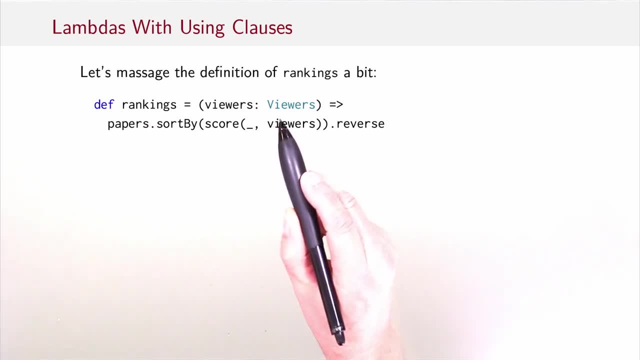 that takes a little bit more time. So let's get to the definition of rankings. So we have here a function that takes, on the right hand side, an anonymous function. The anonymous function has all the parameters of the original function and then continues with the functions body. So rankings, alternatively, could be: 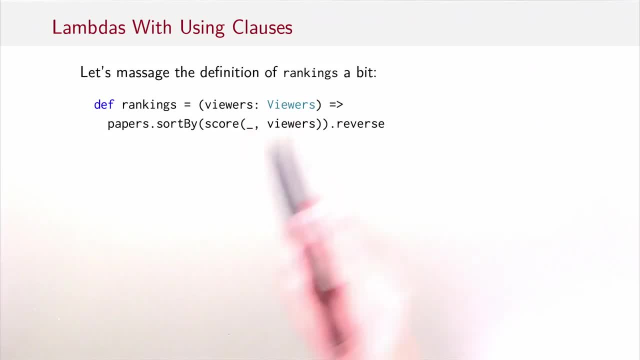 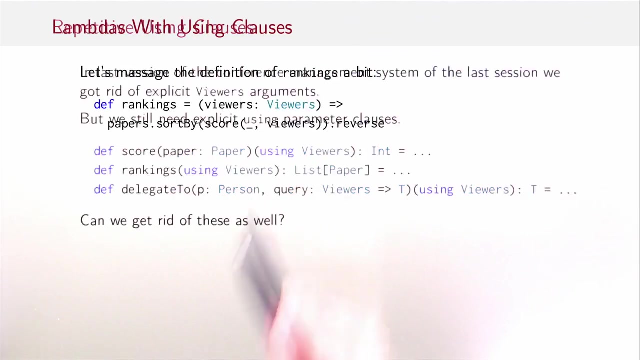 written as the anonymous function that takes some viewers and does the sort by. But something important got lost now in this translation. Namely, previously the viewers parameter was with a using clause, so it was an implicit parameter, but now in the anonymous function it's just a regular parameter. that has to be. 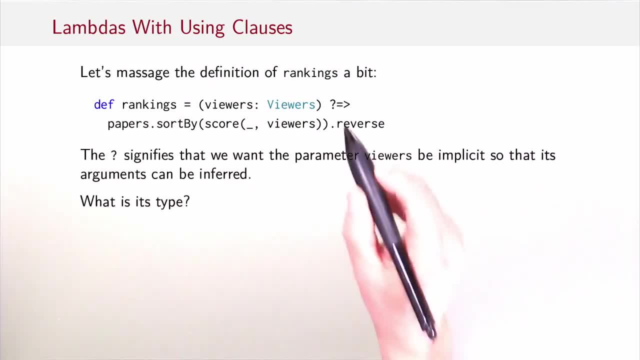 passed explicitly, So we can get back to parity by writing a new kind of function arrow: question mark arrow. here The question mark signifies that we want the parameter viewers to be implicit, so that its argument can be inferred. In other words, that parameter now plays exactly the same role as the using clause on the 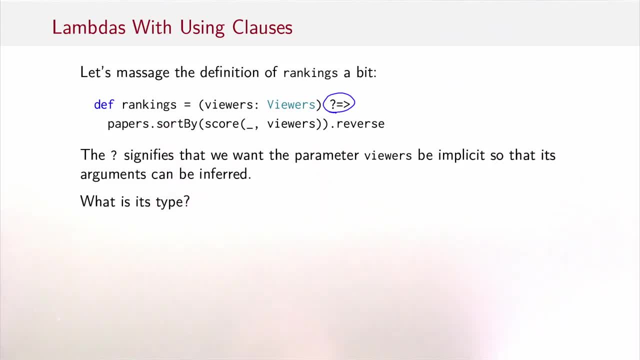 left plate before. One interesting question is: if you have a function like that, why does it have to be implicit? What is its type? For a normal anonymous function, the type would be viewers arrow list of paper- A normal function type, But for an 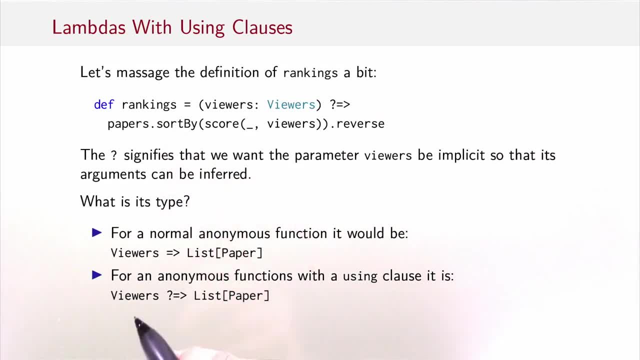 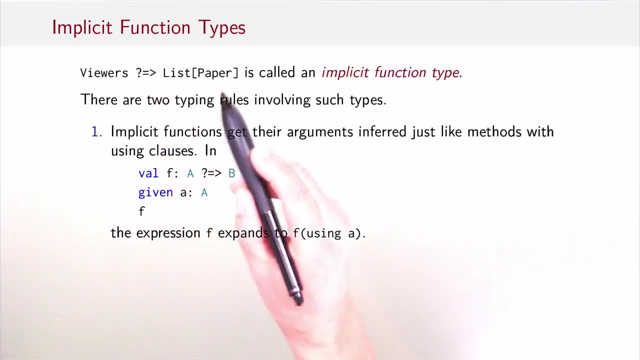 anonymous function that represents a using clause. on the left the type is again written with a question mark. So the type is viewers- question mark arrow list of paper, and that type is called an implicit function type. So viewers question mark arrow list of paper is an implicit function type. What can we do to? 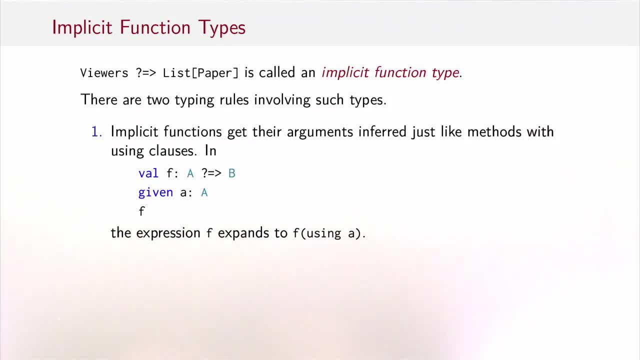 with such types. Well, there are two rules that are relevant. The first rule says that values of implicit function types behave essentially like methods with using clauses. They get their arguments inferred in the same way. So if you have a value like f here of an implicit function type, a question mark arrow b. 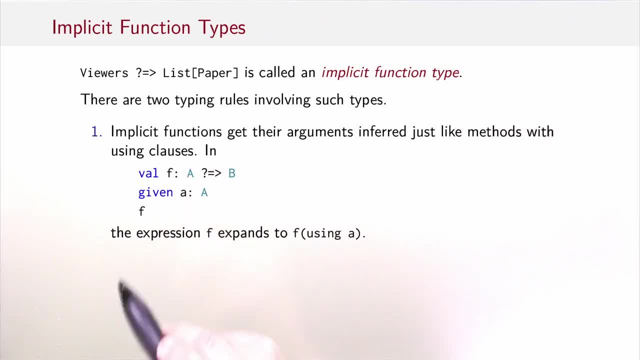 and a given instance of type a. then the expression f expands to f using a. So the compiler will infer the value a as the correct parameter for the implicit parameter a of f here. So that's exactly the same as if f had been. 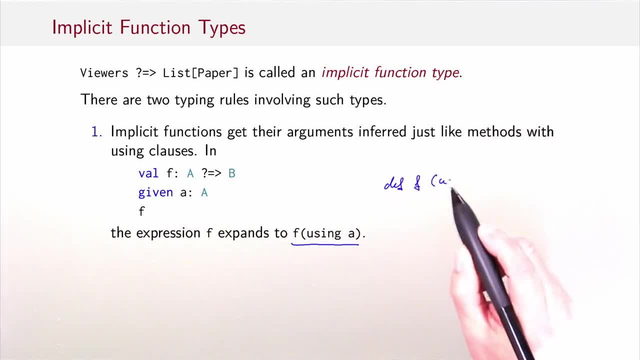 defined as a method like this: f, def, f and then a using clause with a. The parameter inference is the same in each case, And then there's a second rule which makes implicit function types in a sense similar. So if you have a method like this, then the expression f expands to f using a, And then there's a second rule which makes implicit function types in a sense. 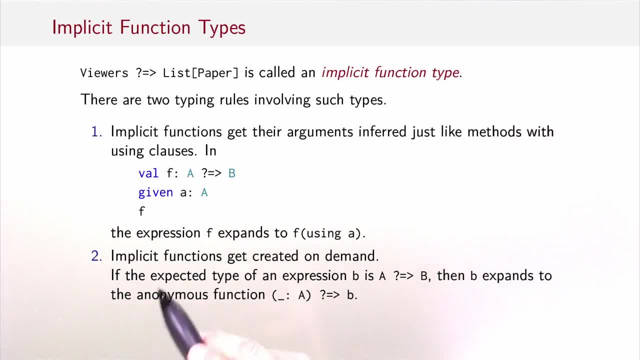 more powerful than just methods with using clauses. The rule is that implicit functions can get created on demand. What that means is that if the expected type of an expression, say b, is an implicit function type from a to b, then b will expand to an anonymous function where the parameter a, which is an implicit 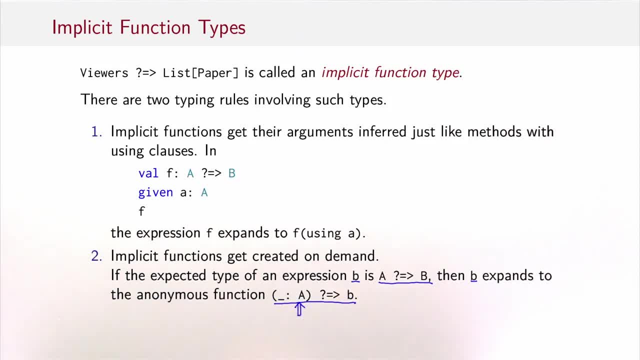 parameter is synthesized is inferred And that expansion happens before the parameter b is type checked. So that means when the compiler type checks parameter b there will be evidence of an implicit value of type a in scope which can be used inside b. Now this might all seem quite abstract. Let's see how it. 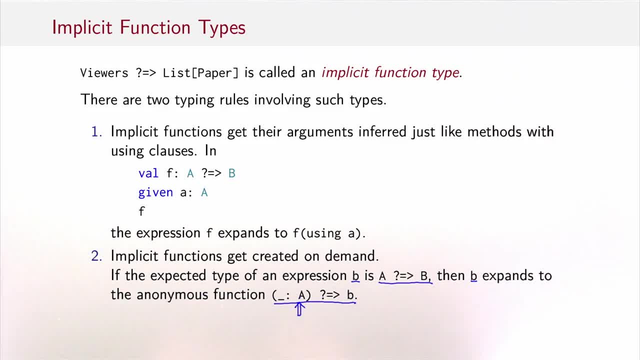 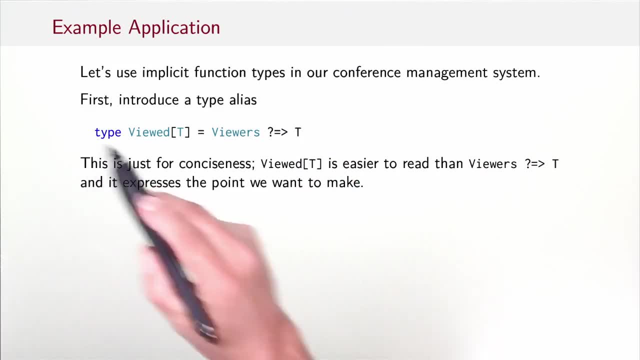 applies in the concrete example of the conference management system. So let's use implicit function types in our conference management system. The first thing we do is introduce a type alias. We say: type view of t is viewers question mark arrow t. That's in a sense just for conciseness. 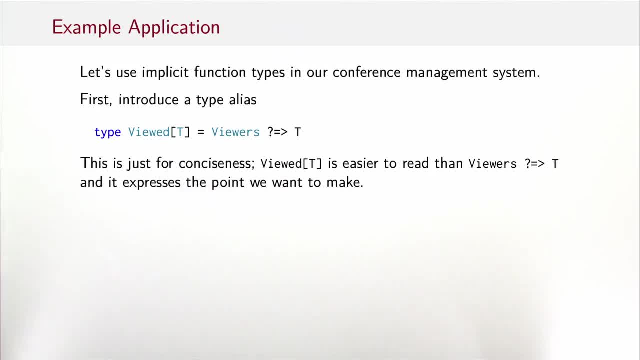 Viewed of t expresses the fact that while we return a result of type t and we also have the info, who's viewing that result. So it's the same thing as the implicit function types here on the right, but it expresses that thing with a custom-made name, namely the view thing. here Now we can apply two changes. 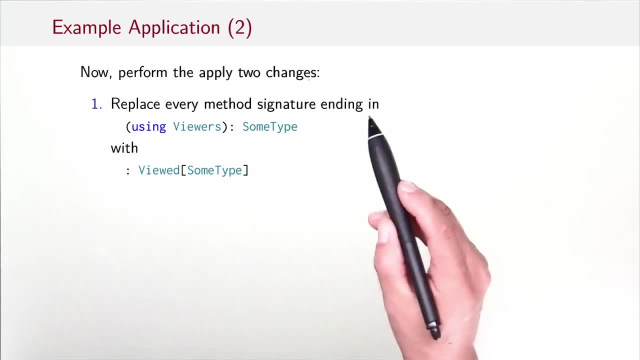 to our code. First, we can replace every method signature that ends in a using clause and some result type with just the result type wrapped in a viewed. It's the same thing. We just essentially trade a parameter to the left to a using clause in the implicit function type And second, we replace every parameter query. 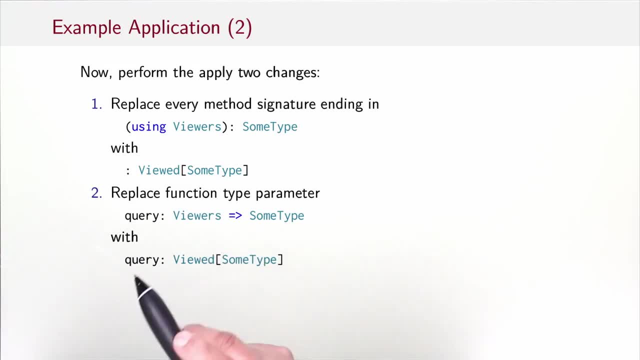 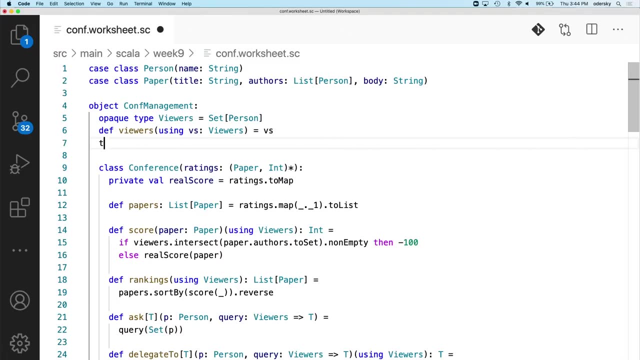 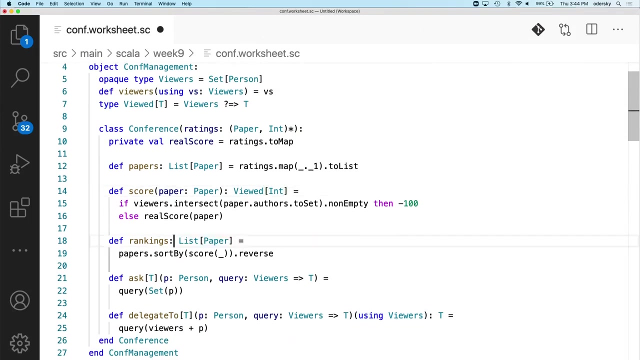 that has a function type like viewers arrow, some type to be query which is a viewed of some type. So let's apply these changes to our worksheet, So we have a new type viewed Like this, And now we can replace all using clauses by viewed instances and we 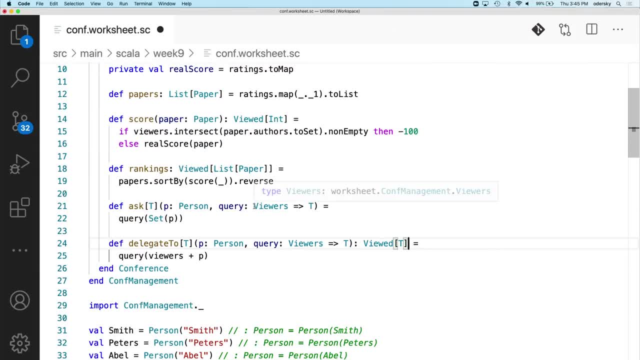 further replace every query argument with an explicit function type with the same implicit function type, Or rather it's viewed alias. And that means that if we pass an explicit one now to query because it's an implicit function type, we have to add a using clause here. 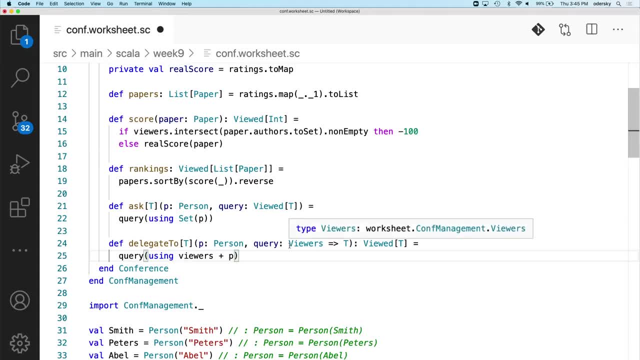 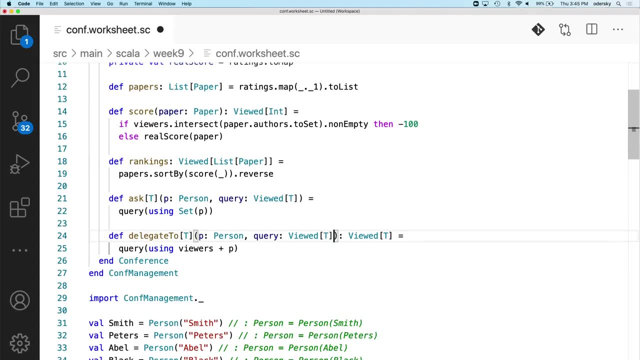 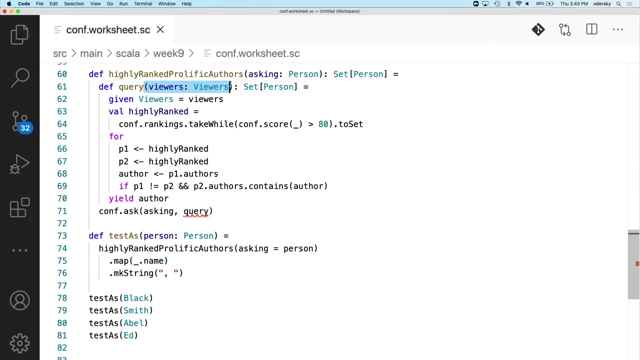 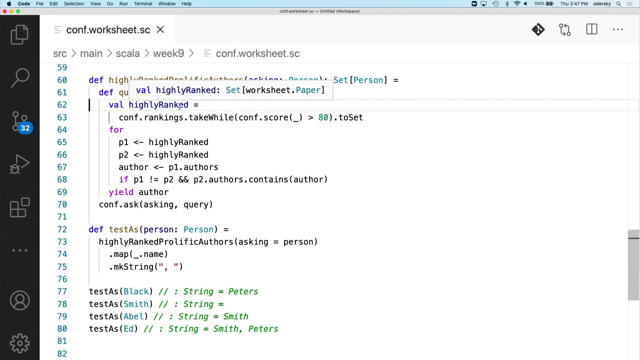 And we have to do the same thing here. So let's see, we have some more problems here. But query now is the same thing. It's a viewed offset of person and we can remove the viewers here, which is no longer needed, because now query is already an implicit function type, so it will get an implicitly. 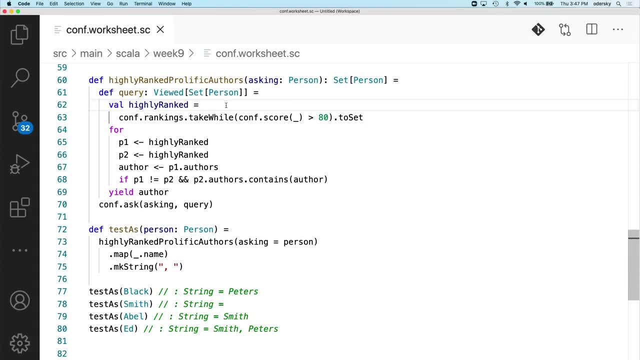 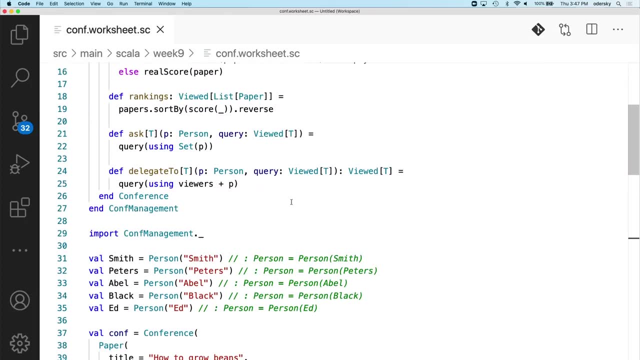 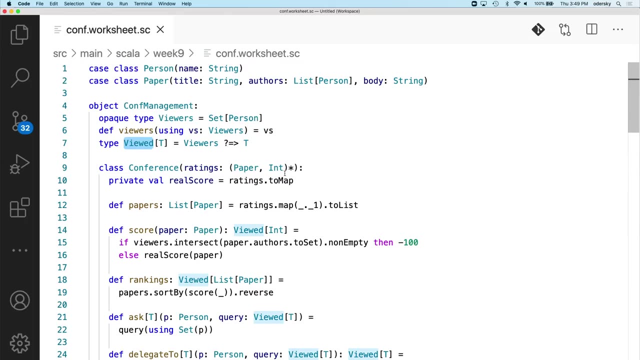 supplied viewers argument that will be used then in the body of query. So what we've achieved in the end is code that is quite streamlined. so essentially all we need to do is mention the viewed in the result type of the methods or in the type. 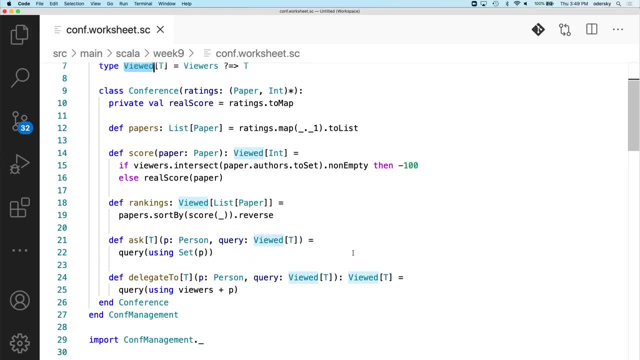 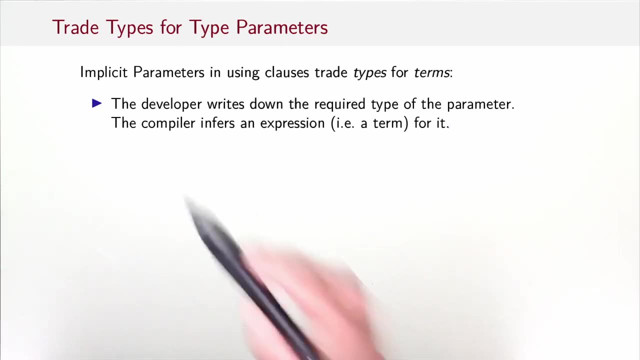 of the query parameters and that will automatically track through the correct viewers set as implicit parameters. So it all works without us having to do anything explicitly in this example. So let's see what we have done here. We know that implicit parameters in using clauses, trade types for terms. 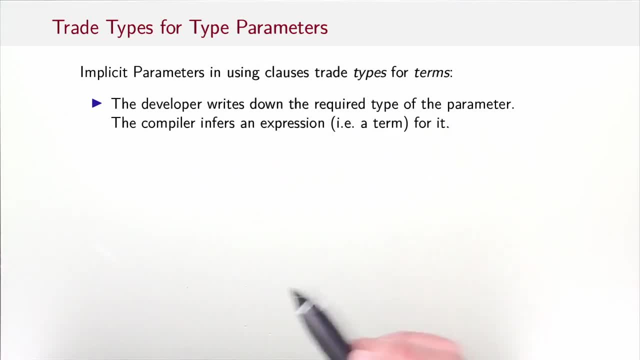 That means the developer writes down the required type of the parameter and the compiler infers a term that is an expression or a value for it. Implicit function types go one step further. They trade types. now, For the parameters, the developer just needs to write down the return type of the method. 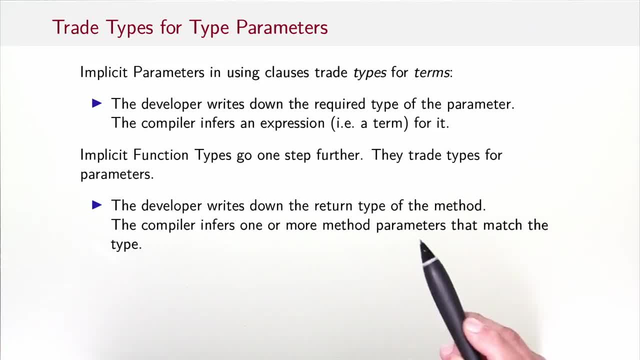 and the compiler infers one or more method parameters that match the type, And from those parameters, of course, it will infer the correct anonymous function bodies and also the arguments to the parameters. So basically, at a very high level, you just essentially specify a single type and the 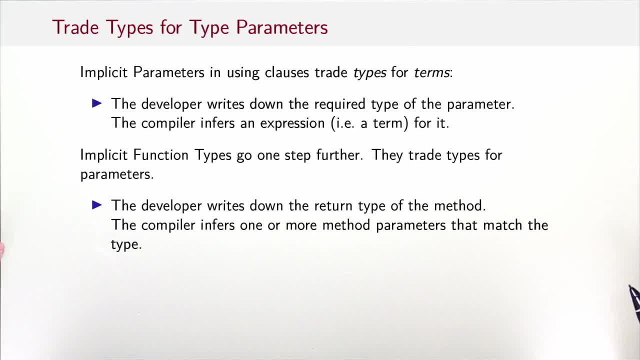 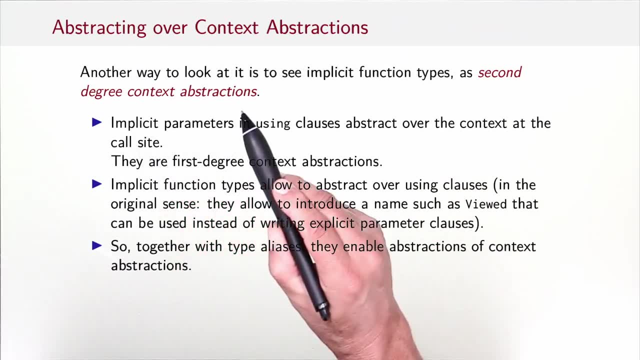 whole machinery will be generated for you by the compiler. Another way to see this: Implicit function types are second degree context abstractions. So what do I mean by that? Well, implicit parameters, in using clauses, abstract over the context at the call site. So they are first degree context abstractions. 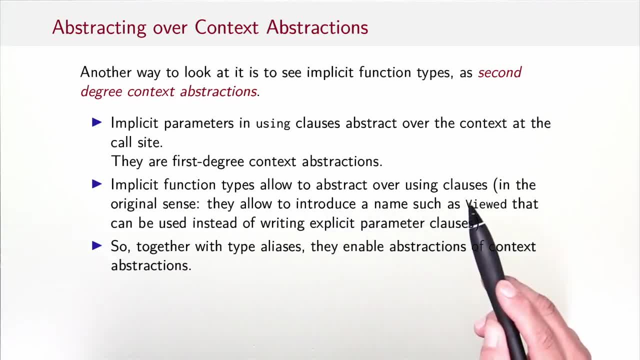 And implicit function types allow to abstract over using clauses as we have seen. Abstract in the original sense They allow to introduce a name, such as viewed, that can be used instead of writing an explicit parameter clause. So, together with type aliases, they enable abstractions of context abstractions. 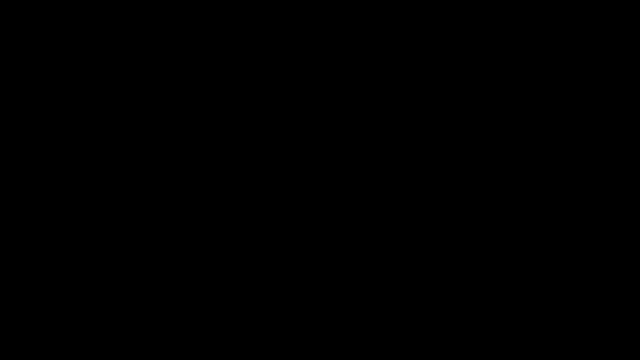 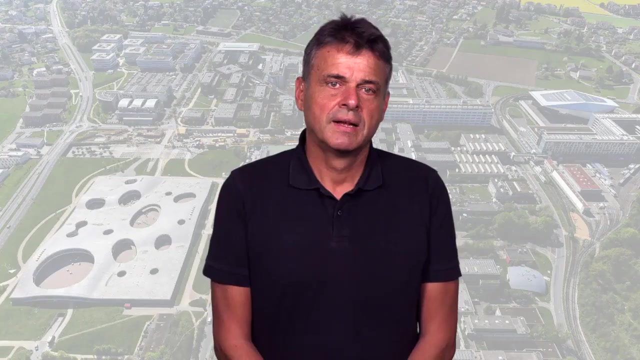 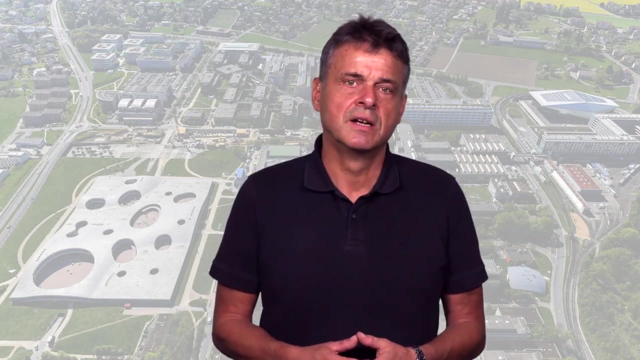 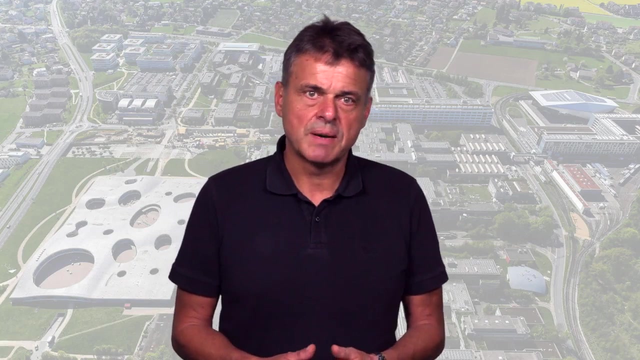 Hence context abstractions of the second degree. This week we'll extend our scope from pure functional programming to also cover mutable states and side effects And we'll study what happens when we combine these with an otherwise functional program. It turns out that some of our techniques for reasoning about functional programs will 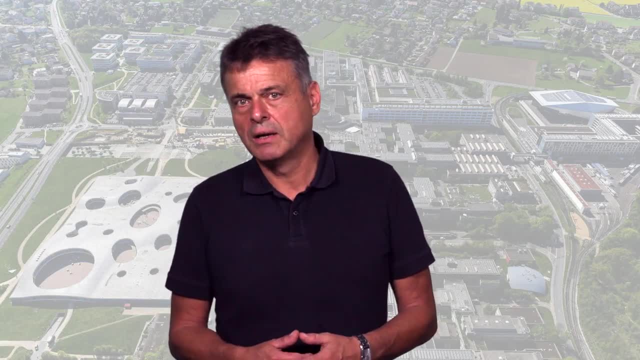 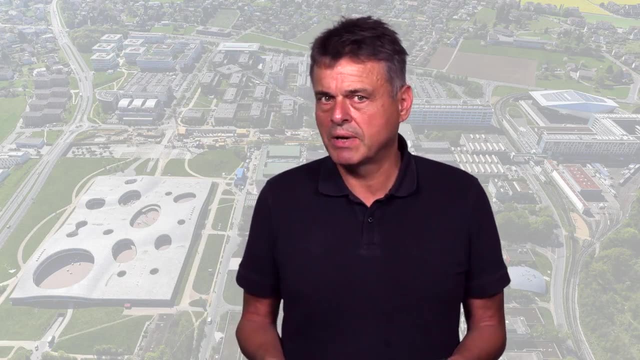 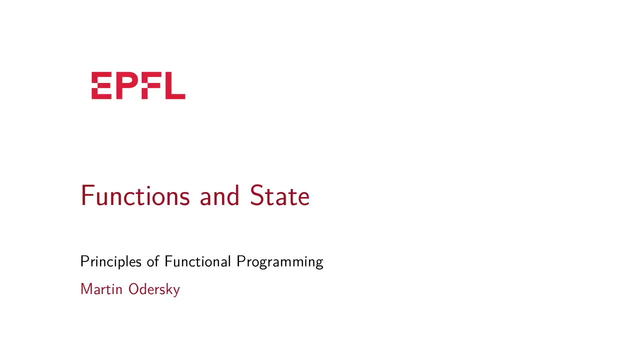 no longer work in that case. On the other hand, the combination of mutable states and high order functions gives us added expressiveness that allows an efficient and sometimes also elegant formulation of certain programming patterns. In this session we take a first look. what happens when we add states? 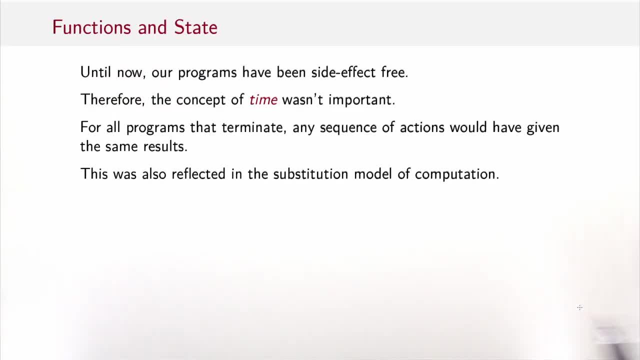 Where do we start to functional programming? Until now, our programs have been side effect free. Therefore the concept of time wasn't important, For all programs that terminate any sequence of actions would have given the same results. This was also reflected in the substitution model of computation, So as a reminder, let's look at that. 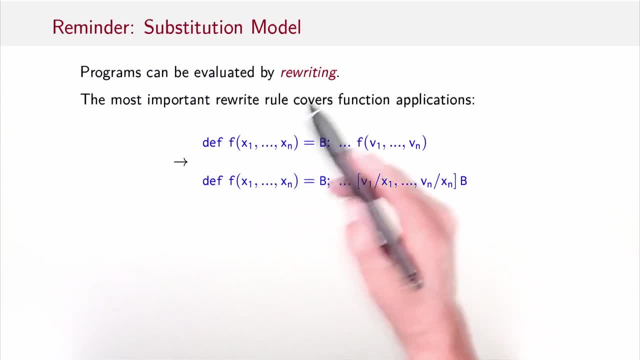 substitution model. again, Here programs are evaluated by rewriting. The most important rewrite rule covers function applications. So it says that if you have a function definition with parameters x1 to xn and body B somewhere and you have a call to that function with actual arguments, values v1 to vn, then the 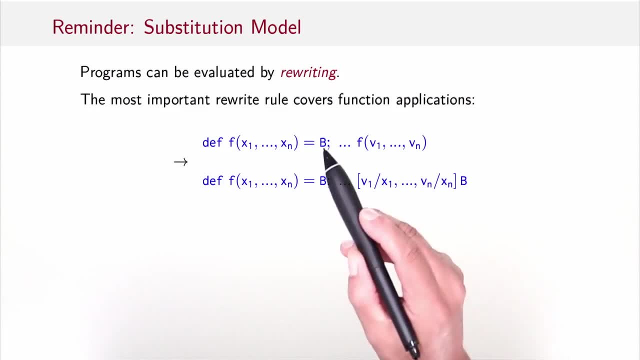 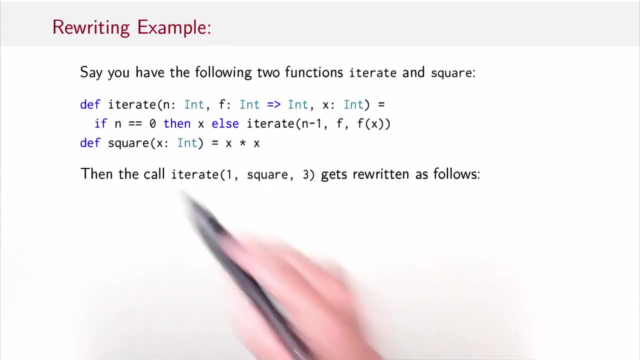 program would be rewritten so that the call gets replaced by the body of the function, where the formal parameters x1 to xn are replaced by the actual values v1 to vn. So that's the substitution model. Let's see it in action in an example. Say you have the following two: 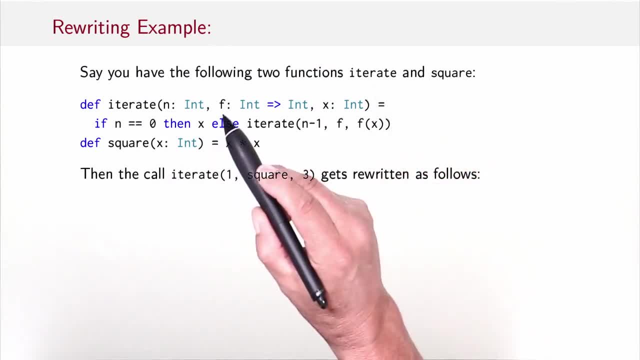 functions iterate and square. Iterate applies function f n times on an initial value x. So if n equals 0, then that's x, and otherwise it's iterate n minus 1, f, f of x. And then you have the square functions that we have seen a lot of. 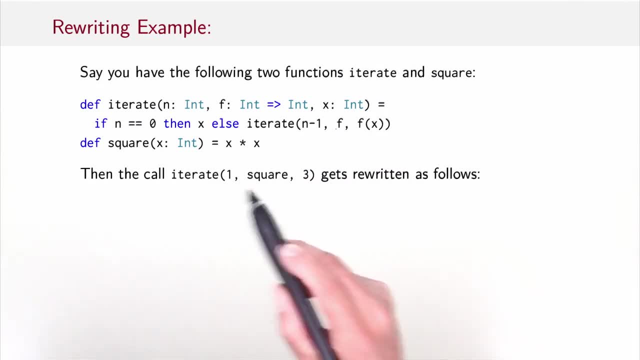 times already. So now the call iterate one square three gets rewritten as follows: We expand the body that gives you this. We simplify the if and pick the else branch and simplify the argument here. that gives you this: We convert the square three call to a in its body three times three and then to a value which gives this: 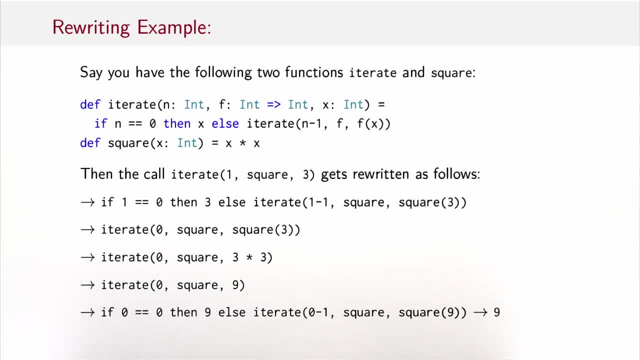 call here, which expands in turn to another body with an if-then-else, where now 0 equals 0 evaluates to true, So this would in the end give you 9.. So in that sequence we always picked one particular place where we would do the next rewriting step, But in fact rewriting could have been done. 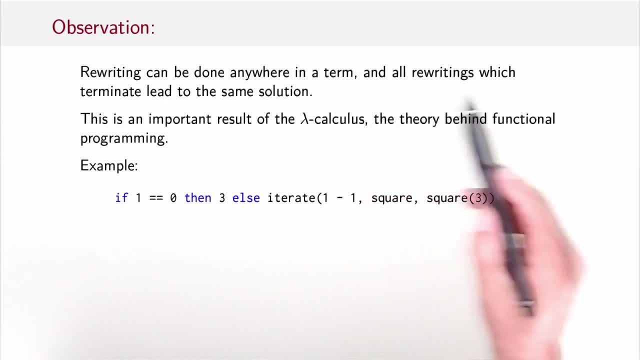 elsewhere. In fact, it can be done anywhere in a term and all rewritings which terminate lead to the same solution. That's an important result of the lambda calculus, the theory behind functional programming. It's sometimes called the Church-Rossa theorem or the confluence theorem. That's 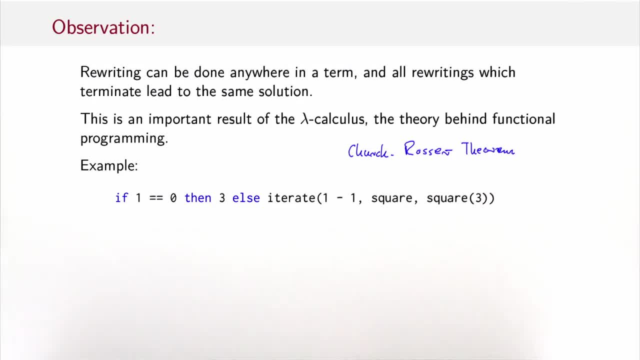 another name. So to demonstrate that, let's take the expression that we started with here again and we have here our sequence that we performed. So that would lead us here. But another possibility would be to say: well, let's just keep the if-then-else as it is and concentrate on this call first, So that 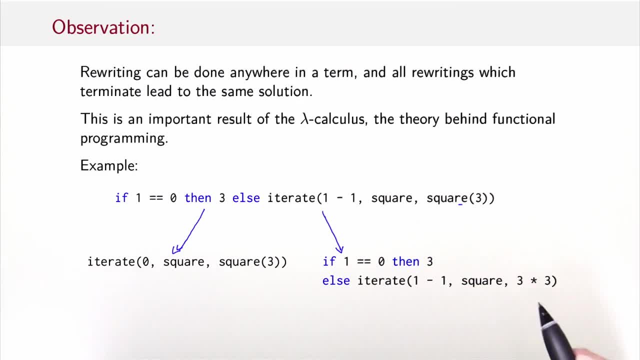 expression could also have been rewritten to this expression here by going deep inside the else part and rewriting the square here to 3 times 3.. So the Church-Rossa theorem, or confluence theorem, says that what we can do is we can then find another reduction. 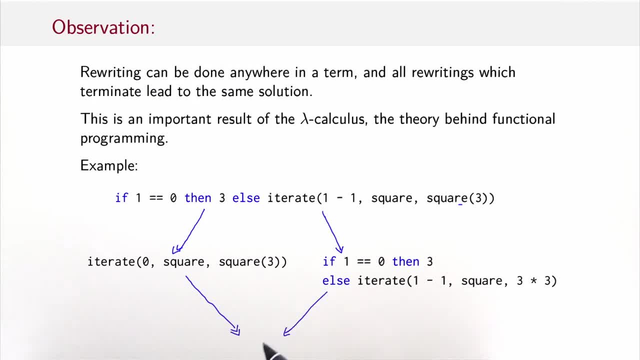 sequence from both sides to end in the same result: 9.. In other words, it doesn't really matter where you reduce first. You'll always get the same result, And that in turn tells you that time cannot matter. The sequence of operations is immaterial. 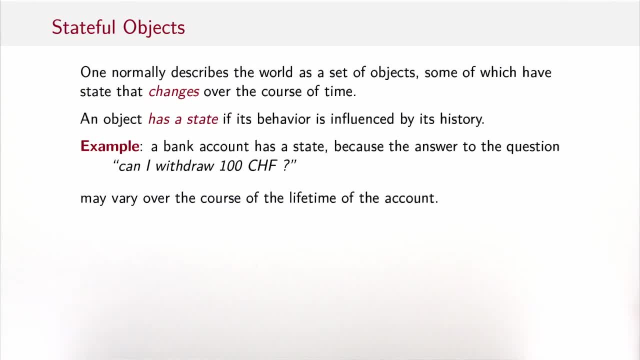 Time is just a set of objects that we can actually move around the world, And this is the final result that you get. On the other hand, of course, time is around us in the real world. One normally describes the world as a set of objects, some of which have state that changes over the course. 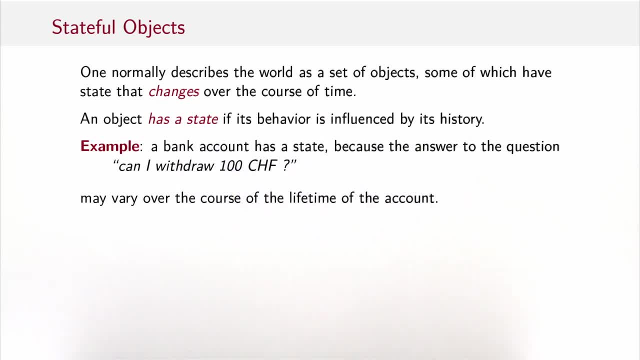 of time And we say an object has a state if its behavior is influenced by its history. So, for instance, a bank account has a state. because the answer to the question: can I withdraw 100 Swiss francs? Initially it might be false because I have no money in. then I might do a deposit. 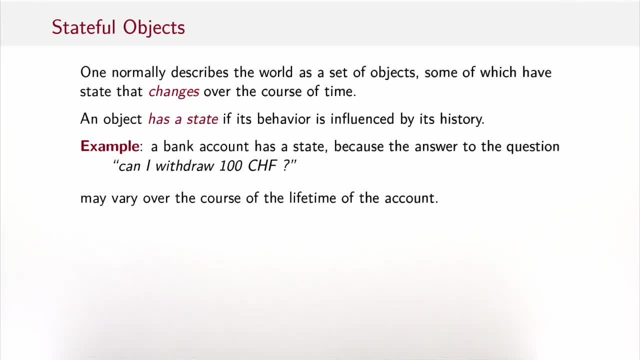 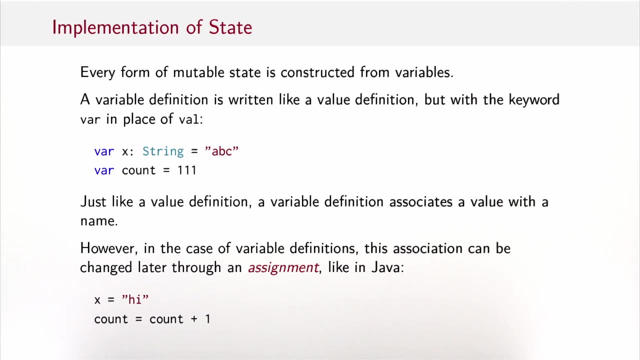 then it will be true. And if I withdraw and the account is overdrawn, then the answer might become false again. So the answer to that question depends on the previous history of operations on that account. So that was a very abstract notion. what it means to have a state, namely to be influenced. 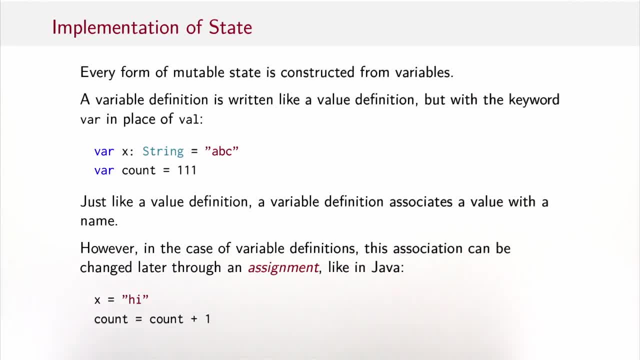 by one's history. But in practice, and if we disregard input-output, then every form of mutable state comes down to be constructed from variables. A variable definition in Scala is written like a value definition, but with the keyword var instead of val. So here you have a variable, here you have another one, Just. 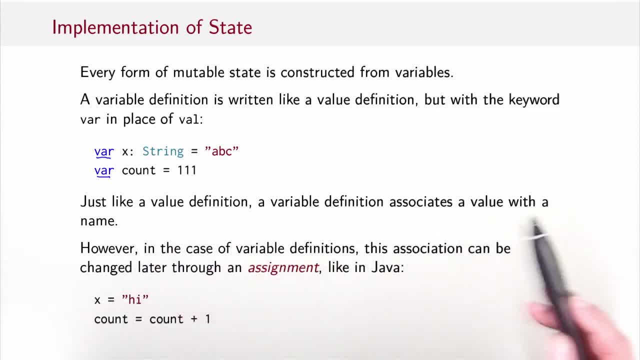 like a value definition. a variable definition associates a value with a name. So if it would be just that, then the variable definitions would behave like two vals. But in the case of variable definitions this association can be changed later on. If you look at this with the eyes of a mathematician, you might cringe a bit, because at the end 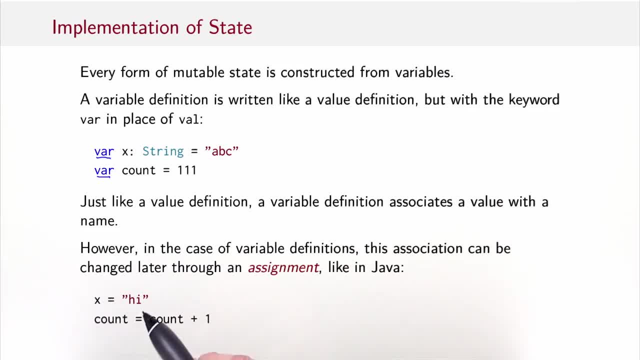 of the day, the value definition is the same as the value definition of the variable x. So you could write later: x equals high and then, after that statement is executed, the variable x would have the value high and no longer abc. Or you could write: count equals. 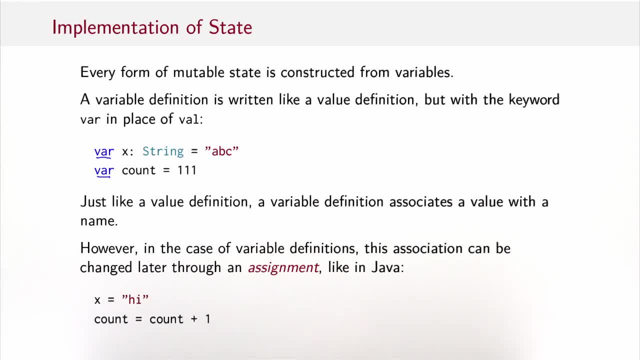 count plus one and then, after that statement took effect, the count would be 112, and no longer 111.. If you look at this with the eyes of a mathematician, you might cringe a bit, because, at the end of the day, this association exists. 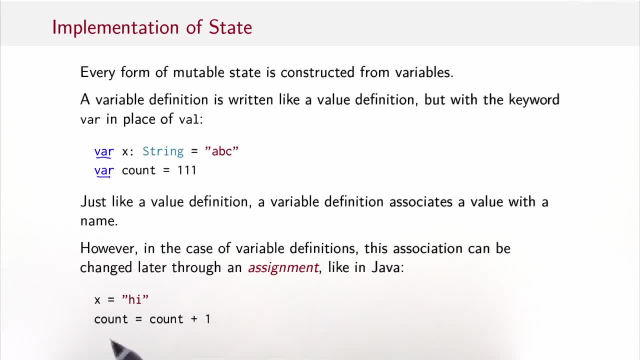 Well, that's all for the next video. I hope that you 되ico'sy, And that's it now. Take care, Ciao, I'll see you the next one. bye, Ciao, Good bye, ciao, Ciao. 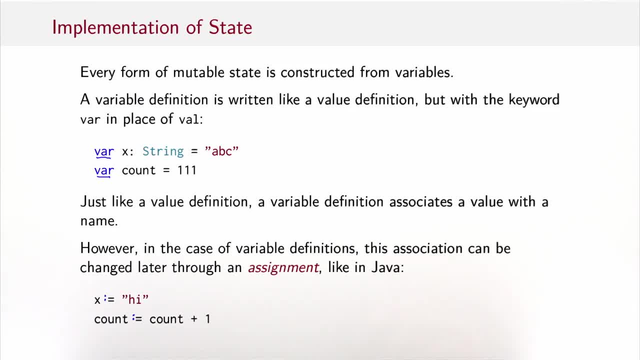 Ciao, Bye, I'll see you as well. Bye, Ciao, Bye, Bye, Bye, Bye, Sie Xiao Dad. so use equals. so Scala unfortunately followed along, and now it's too late to change that. So we have to live with equals In practice. real world objects with state are usually represented. 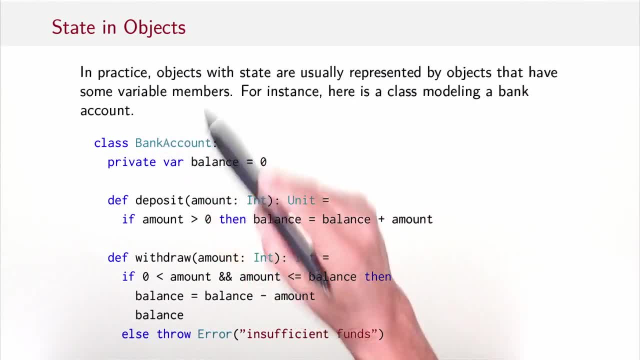 by programming language objects that have some variable members. For instance, here is a class that models a bank account. We have class bank account and then we have a balance, which is the current balance on the account, Initially zero, and that balance is private, so that not everybody. 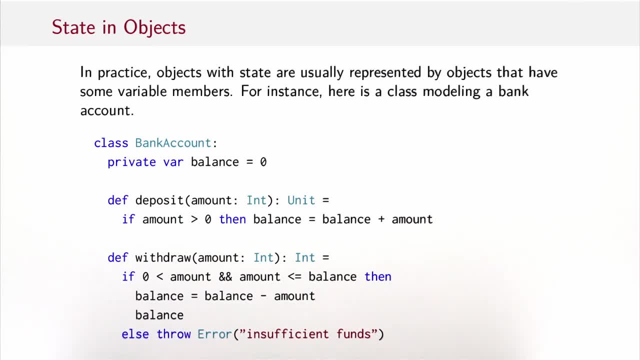 outside the account can just fiddle with the balance and maybe add some Swiss francs to it. That would be very convenient, but I believe the banks wouldn't like such a class. So there are two methods that regulate the changes in balance: There's deposit and there's withdrawal. So to 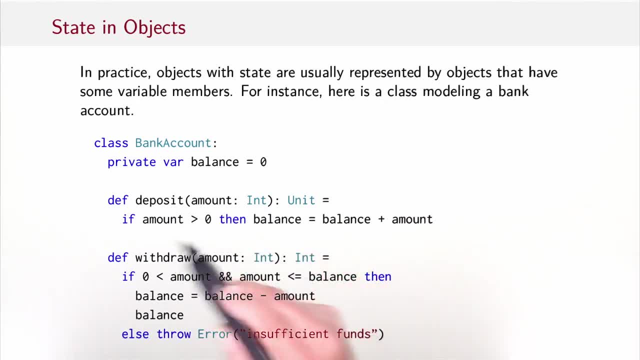 deposit an amount of currency, you ask: well, the amount should better be positive. You can't deposit a negative amount, and if that's the case, then the balance is augmented by the given amount And the other method is withdraw. So to withdraw an amount of money, again, the amount should be: 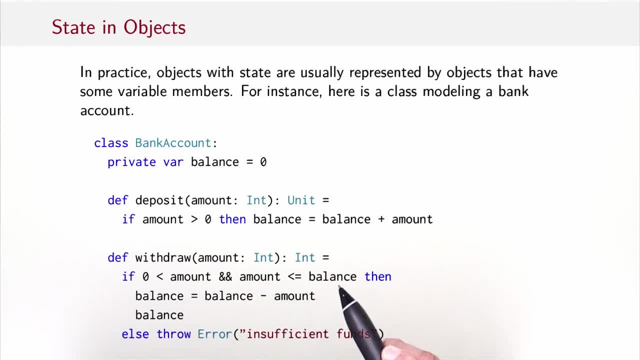 positive and the amount should be less or equal than balance. so no overdraws allowed. In that case balance equals balance minus amount, so deducted by amount and you return the balance. So the result of the withdrawal method is the current balance, And if the condition is not fulfilled then you throw an error with a error message insufficient. 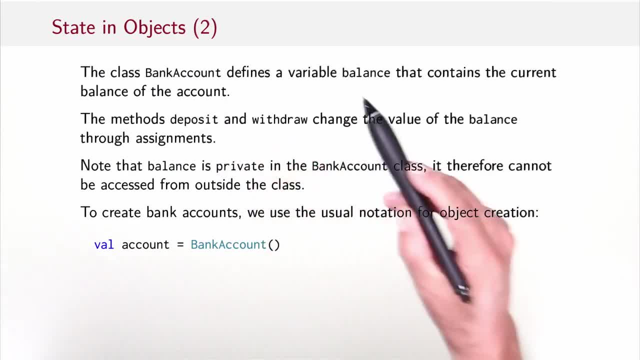 funds. So in essence, the class bank account defines a variable balance that contains the current balance of the account. The methods deposit and withdraw change that value through assignments. Note that balance is private in the bank account class. it therefore cannot be accessed from outside the class. To create bank accounts we use an usual notation for object creation. So 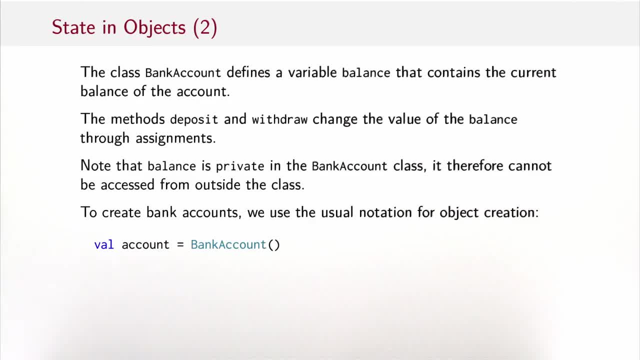 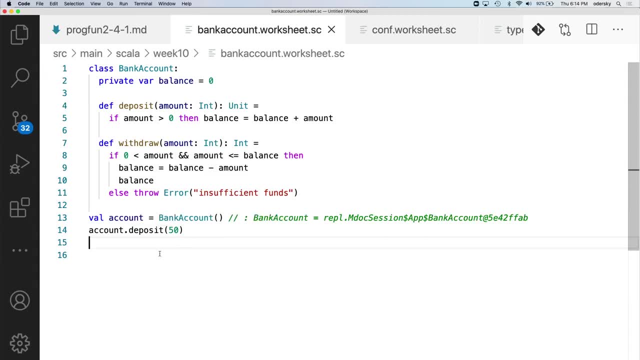 if the account is open, parents close, parents would create a fresh account. So here's a worksheet with bank accounts. So I have defined my class as shown. I define a new bank account and I deposit 50 units initially. I then withdraw 20 units and it responds that the balance is now 30.. 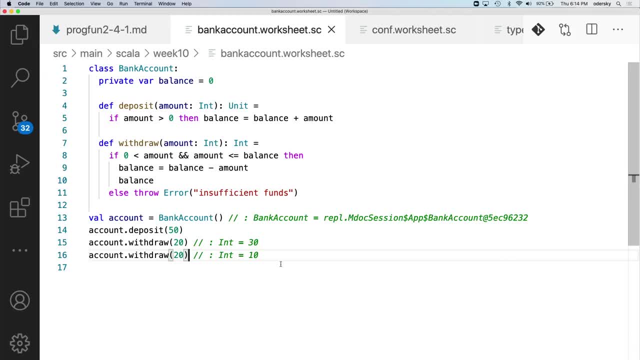 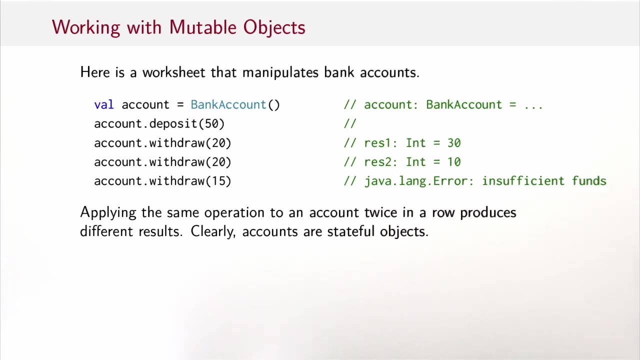 And I withdraw a further 20 units and it responds that the balance is now 10.. Let's say 15 units and I get an error: insufficient funds. So what you've seen here is that, applying the same operation, account, withdraw 20 from the account. 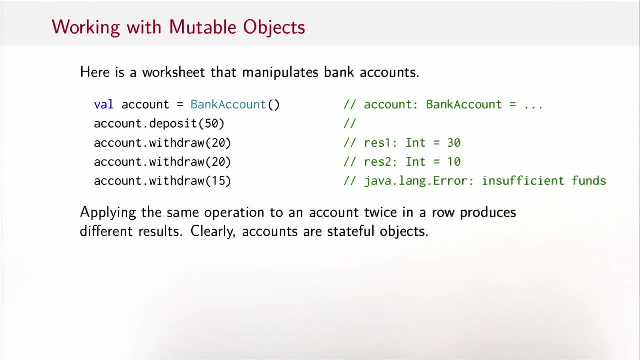 twice in a row produces different results: first 30 and then 10.. So clearly, accounts are stateful objects. If they were stateless, that would mean that the result of withdrawal is always the same, But clearly that's not the case. So accounts have state and that we know even without looking inside the account. and 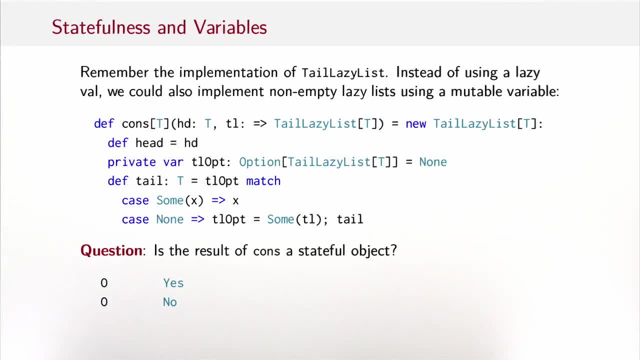 discovering a variable there. Mutable variables can play a useful role even in purely functional programs. For instance, remember the implementation of tail lazy list or simplified variant of lazy lists. It used the lazy val to compute the tail operation. But instead of using a lazy val we 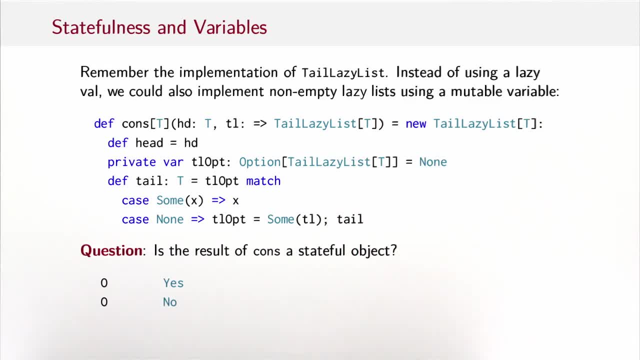 could also implement non-empty lazy lists using a mutable variable. So here's a example of a lazy val. Here's how that would be done. So here's the non-empty lazy list. constructor cons creates a lazy list whose head is as given, and then it has a variable which is private. 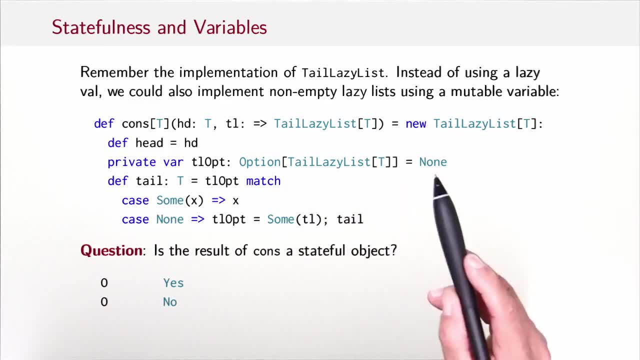 tailopt of type. option of tail. lazy list of t initialized to none. So now to take the tail of a list, it would query tailopt. if it's none, that means nobody has asked the result yet. then the result will be computed here. So tail will compute the by name. 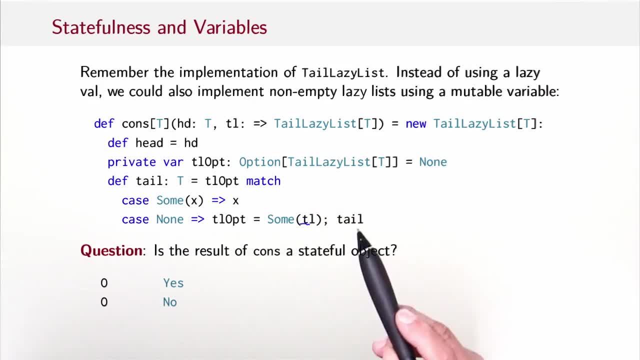 And then the result will be called recursively, which would go into the first case. So if someone had already evaluated the tail, then there's no need to evaluate it again. In this case, tailopt would return sum of x and we would return the result x directly. It's an interesting question. 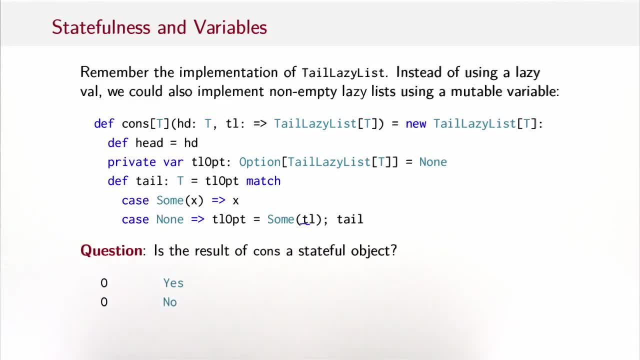 to ask: according to our definition of statefulness as being history dependent, Is the result of cons a stateful object? It's a tricky question and I would respond with it depends. It's not a stateful object if the rest of the program is purely functional. So to see why, let's make the argument. 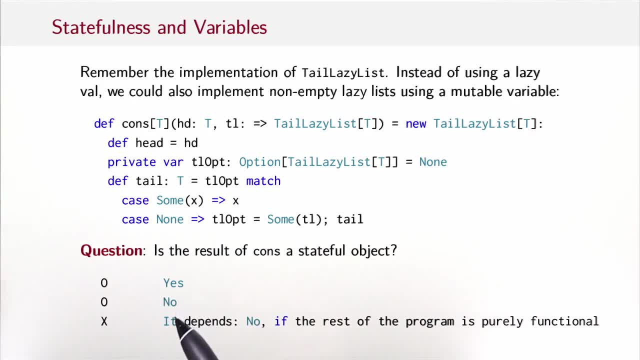 first that it is in fact not a stateful object, that it is purely functional. That argument goes as follows. It says: well, all this tailopt does, it avoids a recomputation of the tail definition here. But in a purely functional world tail will always return the stateful object. 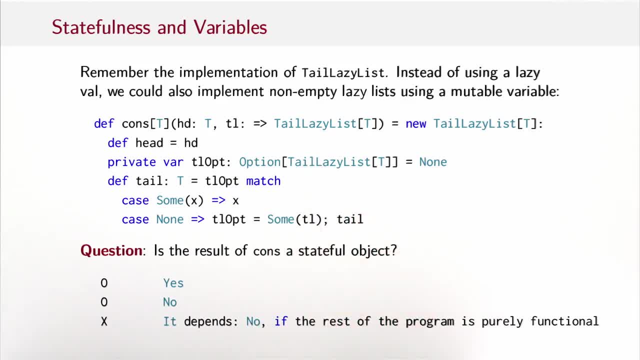 The same value, even if it's, if it's called several times. So clearly there's no point in evaluating tail several times. We can just use the cached value and that will not change any observation that we could make from this tail lazy list. And that's true, but it's only 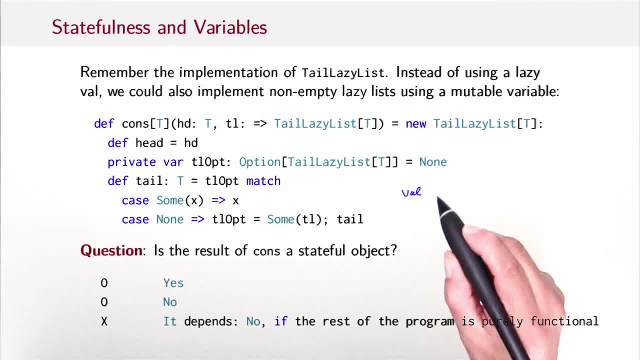 true if the environment is purely functional. Here's a counter example where it would be false. So we do a cons of some number one and the tail of the cons would print something- So that's a side effect- and return nil, or rather lazy list empty. This should be empty. 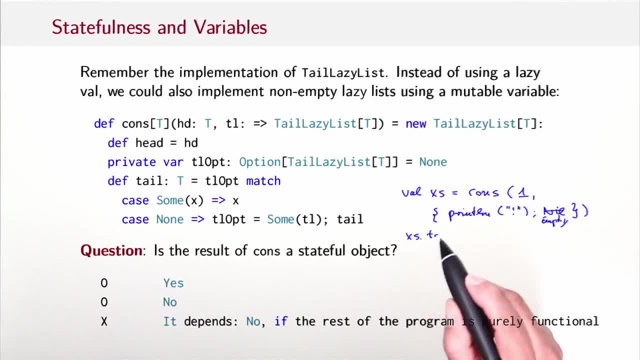 And now we do xs dot tail and we do xs dot tail again. So in the first execution what you would see is an exclamation mark. It would print something, And in the second execution we would see nothing. So okay, so that's a output println, But we could turn this easily into an. 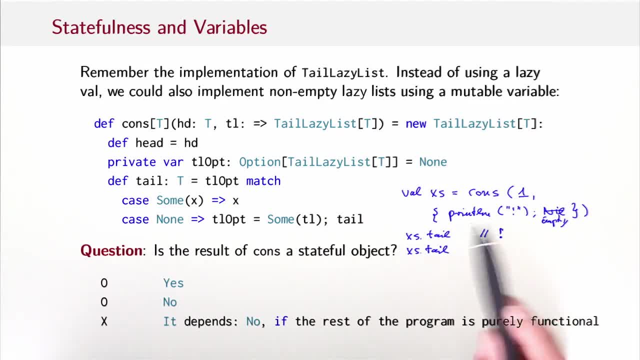 observable effect inside the program by essentially changing a variable instead of doing a println. The println was just essentially to demonstrate what goes on. So the morale is that if the environment can have side effects, then the tail optimization with mutable state is not purely functional. But ironically, in a purely functional world it would be, Which means 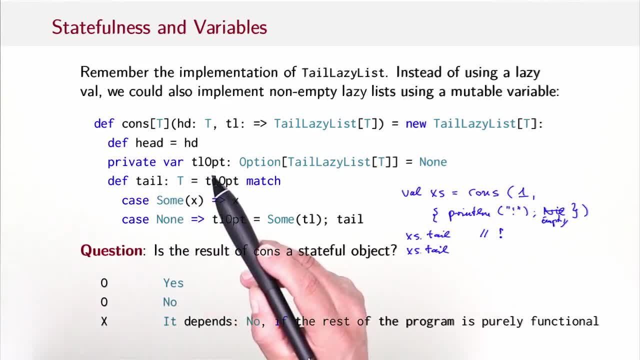 there is a role for having variables, essentially as caches, that work very well in a purely functional architecture and that are in fact, not observable in that architecture, Whereas they would be observable if the architecture was not purely functional. That's something to chew on. So, staying with this line of questioning, consider the following class: bank account proxy. 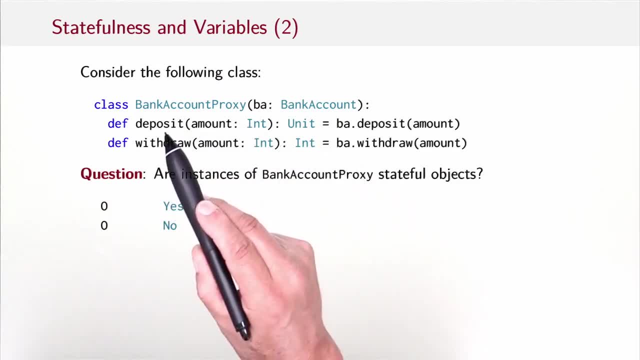 It's a proxy of a bank account and it simply forwards its deposit and withdraw methods to the bank account that's given here. The question is: are instances of bank account proxy stateful objects? The case for no would be to say: well, there's not a variable inside, How can there be stateful objects? 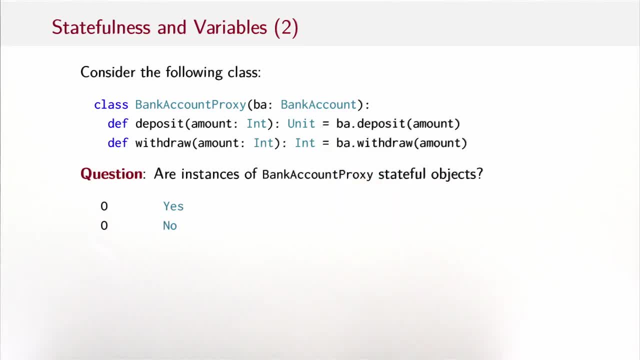 But of course they can be stateful objects, because bank account is a stateful object And that means the history of the deposit and withdraw methods here will mirror the histories of those methods on the original bank account And that means the result will depend on what happened. 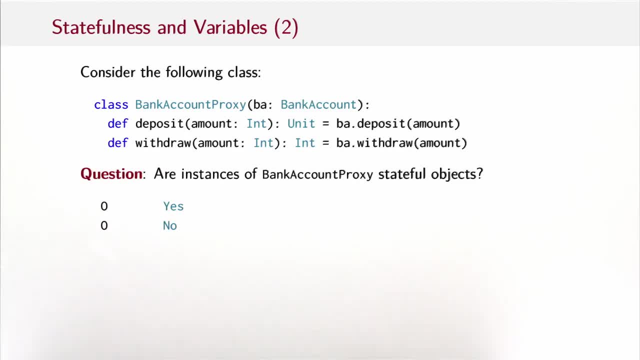 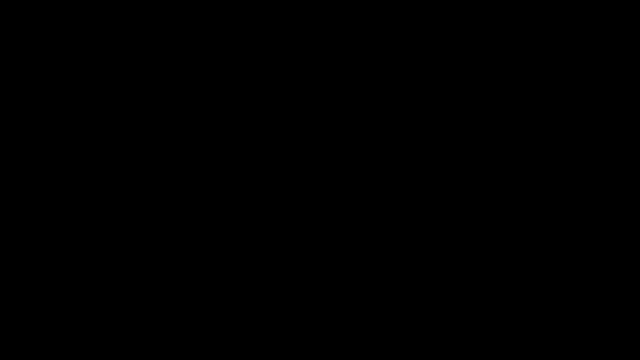 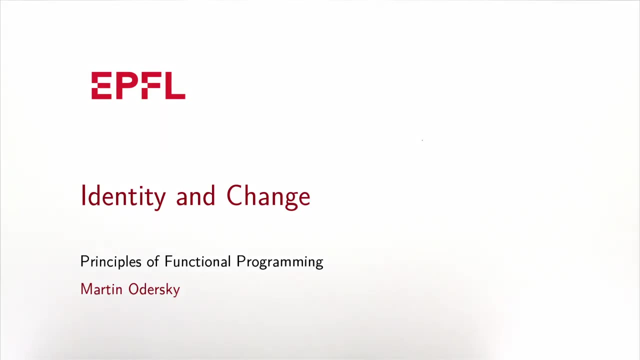 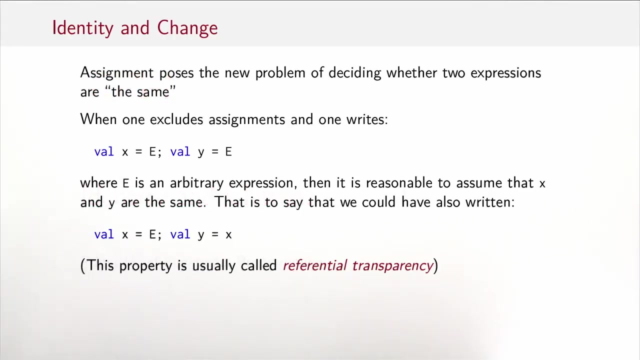 before. So by that more abstract definition, indeed, bank account proxy is a stateful object, even though it doesn't contain any variables itself. In this session, you'll learn how the introduction of assignments affects our notions of identity and change. In fact, assignment poses new problems for deciding whether two expressions are the same. 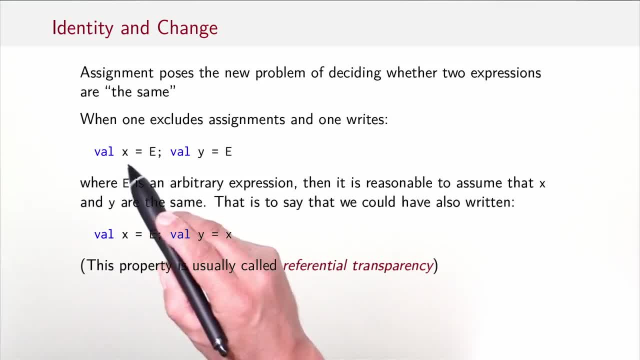 If one excludes the two expressions, the two expressions are the same. If one excludes the assignments and one simply writes val x equals e and val y equals e- for some expression e, then it's reasonable to assume that x and y are the same. 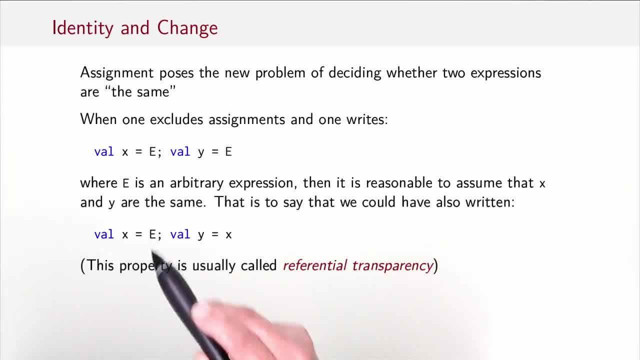 That is to say that we could also have written val x equals e and then, instead of repeating e again, we just write val y equals x. x is the same as e, so we might as well use the value of x instead of e, or so it goes This property, that we can do these changes in confidence. 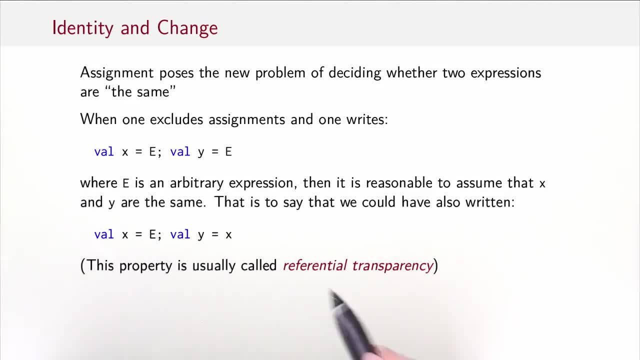 is usually called referential transparency. Referential transparency means that a reference such as x is really the same as the thing it's bound to. So it doesn't matter whether you use x or the things it's defined as, namely the expression e. It comes down to the same thing. 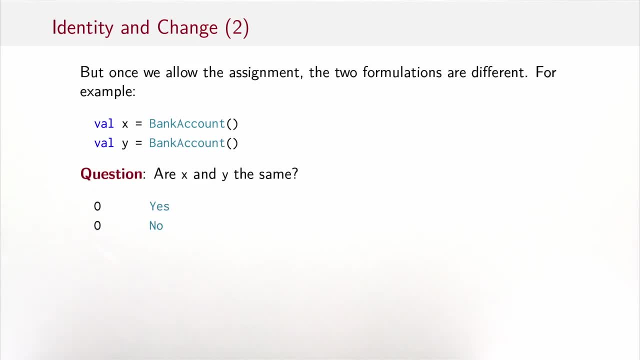 But once we allow assignments, things become more complicated. For instance, if now we would write: val x equals bank account, val y equals bank account, are x and y still the same? Well, intuitively no, because we have created two different bank accounts. But according to our previous definition, x and y would be the same. 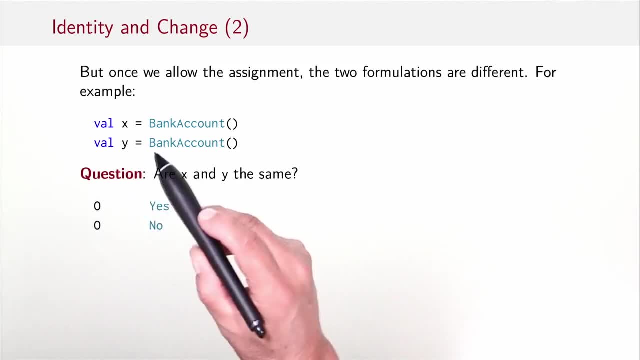 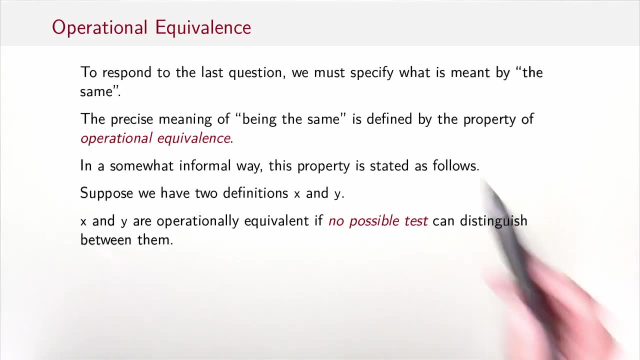 They have the same right hand side, so we might as well write: val y equals x. So what happens here? Well, to respond to this question whether x and y are the same, we should specify what is meant by the same. The precise meaning of being the same is defined by a property. 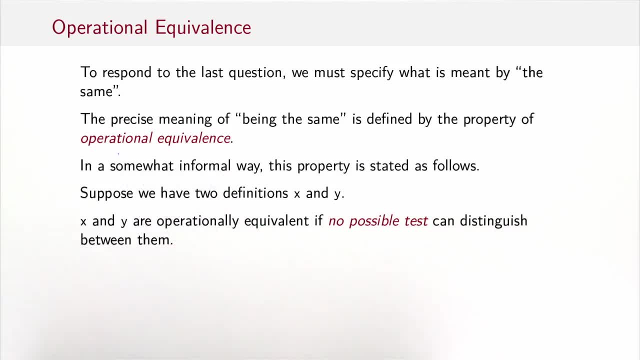 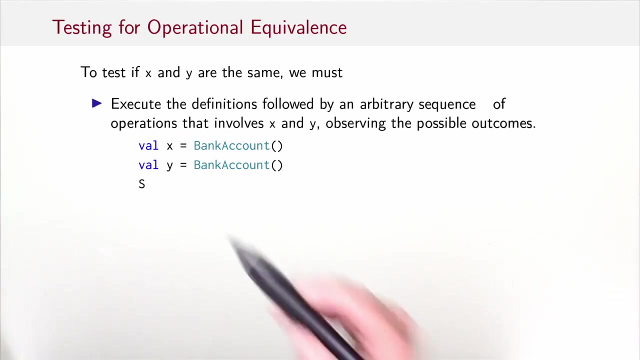 called operational expression. In a somewhat informal way this property is stated as follows: Suppose we have two definitions, x and y. x and y are operationally equivalent if no possible test can distinguish between them. So that begs the question: what is a possible test? So let's make that concrete, To test whether 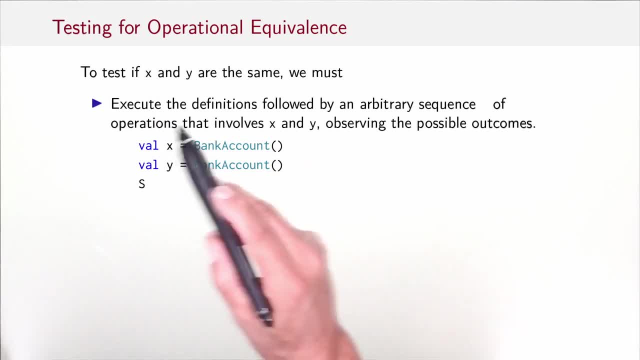 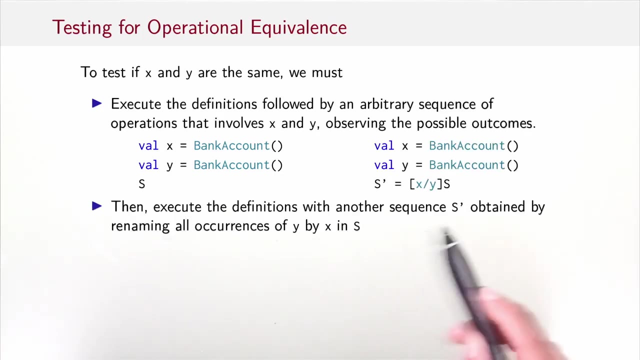 two definitions, x and y, are the same. we must execute the definitions and then follow it by an arbitrary sequence of operations, here called s, and that can involve both x and y, and we observe the possible outcomes. Then we execute the definitions with another sequence s prime. 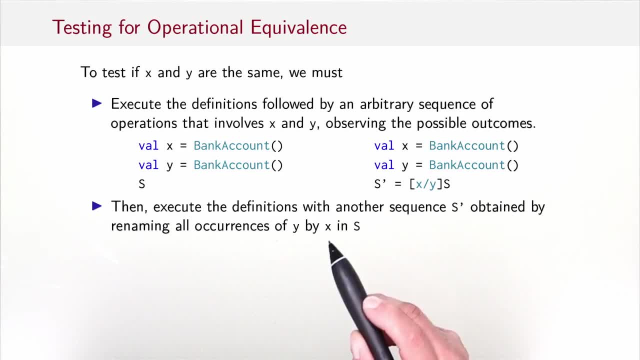 that is the same as s, but every occurrence of y is replaced by x. So instead of using y, we use x in this new sequence here. If the results are different, then the expressions x and y are certainly different. It makes a difference whether I use x or y. 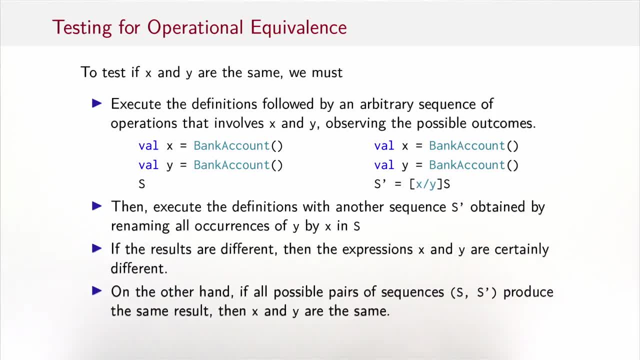 Or y in the sequence of operations. On the other hand, if all possible pairs of sequences s and s prime produce the same result, then I can't observe a difference and that means I have to conclude that x and y are the same. Note that this is not a test I can do mechanically, To be sure to observe. 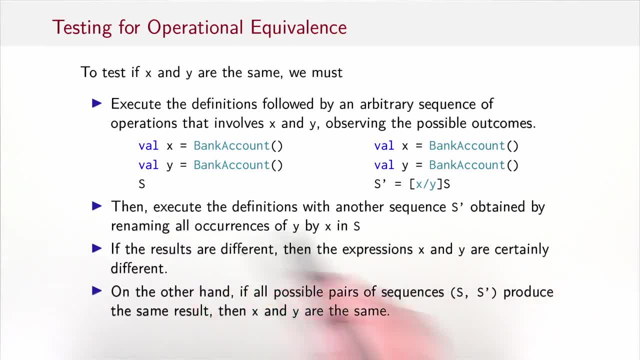 a difference. it's. I just need a single sequence s that when I do the renaming here yields a different result. So that's easy. But on the other hand, to prove that two definitions are operational equivalents, I have to reason about all possible sequences of actions that follow the definitions, and there are infinitely many of those, So I can't really. 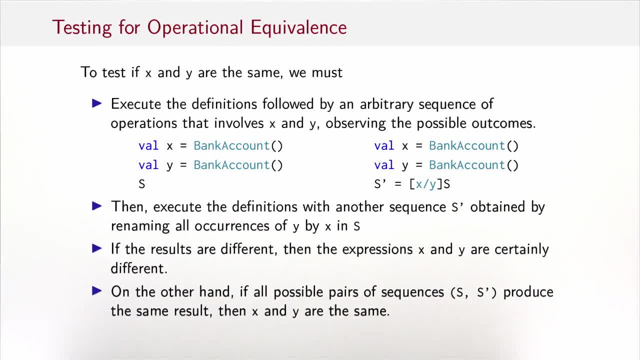 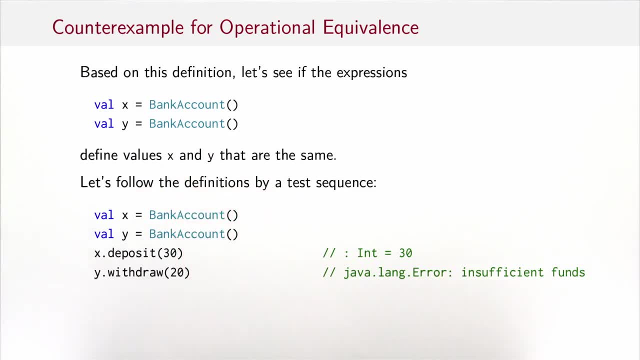 do that in an experimental fashion. I have to find another way to prove that. So let's see, Based on these definitions, let's prove that these two bank accounts, x and y, are different. So let's see, Based on this definition, let's see whether the expressions val x equals bank account val y. 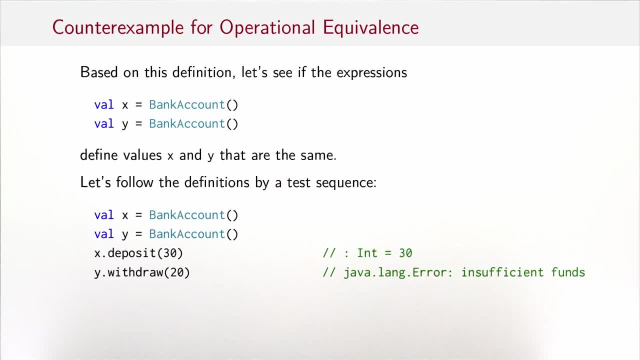 equals bank account differ. Let's find values x and y that are the same. Let's follow the definitions by a test sequence. Let's say, deposit 30 units into bank account x and withdraw 20 units from y, So what you will get. 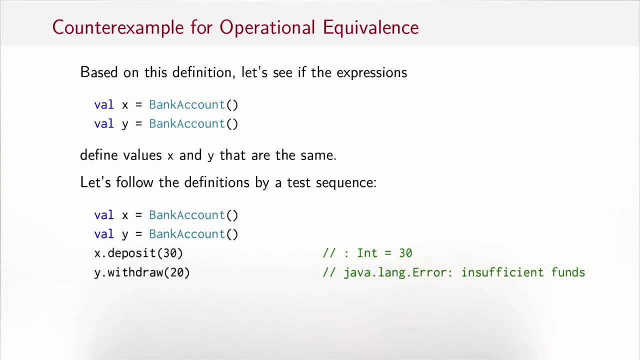 is a result of 30 in the first case and an error insufficient funds in the second case, because y was empty before the withdrawal. On the other hand, if we rename all occurrences of y in the sequence with x, then what we would get is x, log, x. 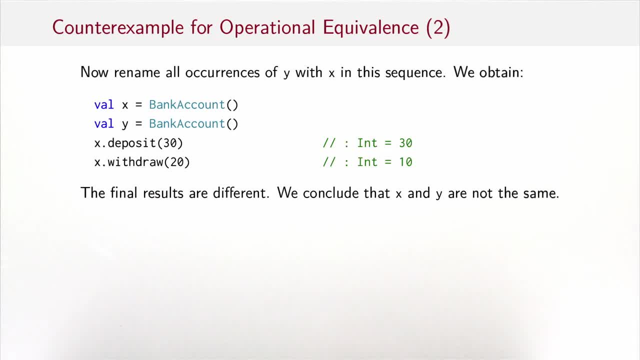 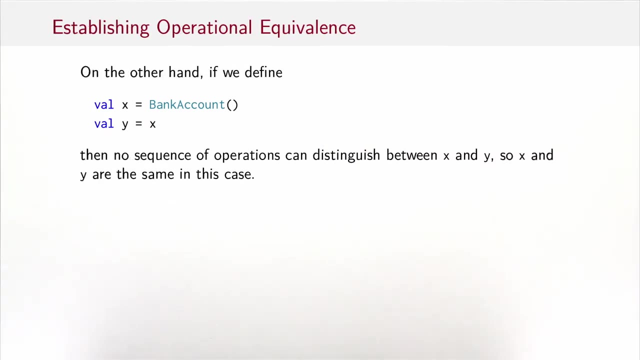 So we would get this sequence here and we would observe 30 after line 3 and 10 after line 4.. So the final results are different, The result of this withdrawal operation, and therefore we conclude that x and y are not the same. That's the proof. On the other hand, if we define val, x equals bank. 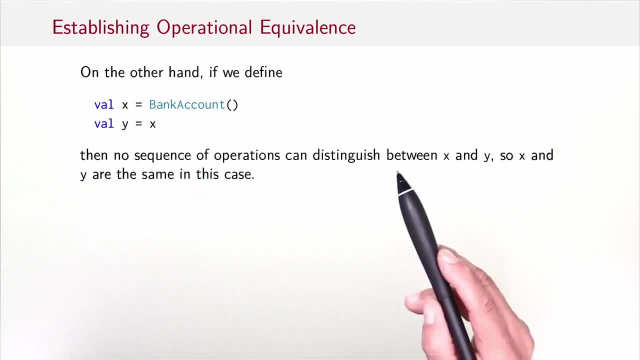 account val y equals x, then no sequence of operations can distinguish between x and y, So x and y are the same in this case. One can do a formal proof of the statement by essentially formalizing the semantics of programming languages, but that's beyond the scope of this course. The preceding examples show that. 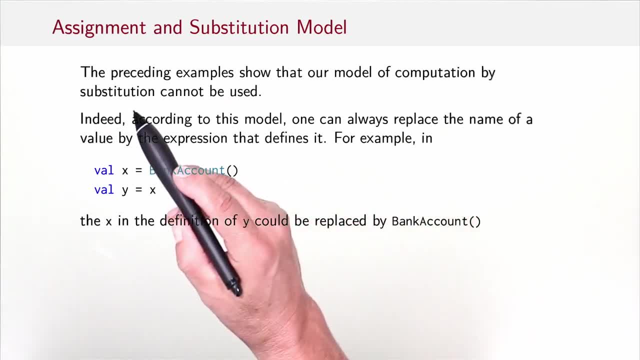 our model of computation by rewriting or by substitution cannot be used anymore. Indeed, according to the substitution model, one can always replace the name of a value by the expression that defines it. For instance, if we have these statements here: x equals bank account, y equals x, then the x in the definition of y would be replaced by bank account. That's what the 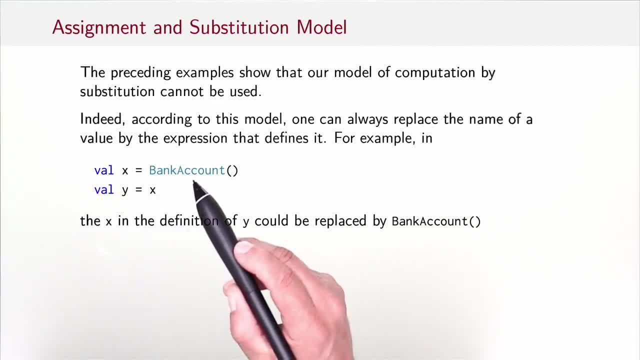 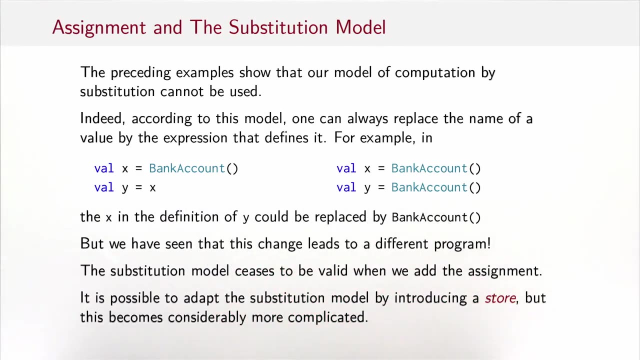 substitution model predicts. It says: simplify this to a value where an object reference is already a value and then replace the reference by the value that you find here. So the substitution model tells us that that rewrites to that, and if you rewrite things then they're necessarily the same. 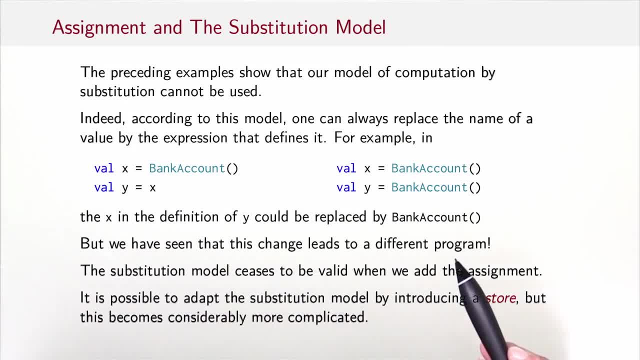 But now we have seen that this change leads in fact to a different program. So that means the substitution model clearly is no longer valid. if we add assignments, It's possible to rescue the situation, to adapt the substitution model by introducing a store that essentially tracks all variable bindings that you have in your program. 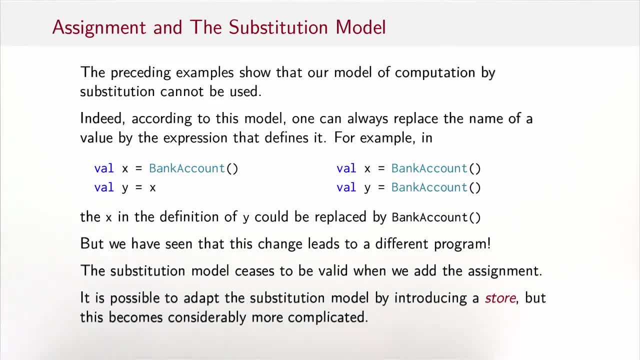 But then things become considerably more complicated. So we see that adding variables and mutable state to functional programming gives us additional expressive power. but we pay for this with a loss of simple semantic foundations and also with a loss of reasoning capabilities, because we have seen that the substitution model actually was used extensively. 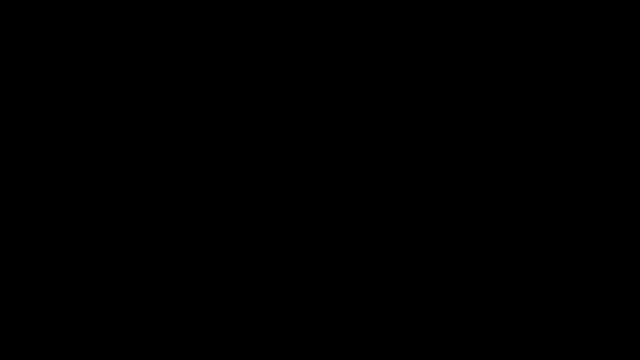 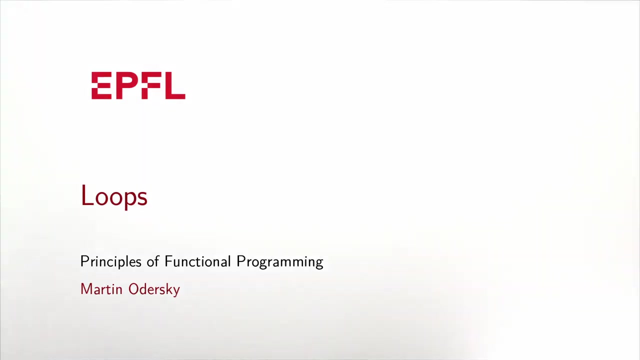 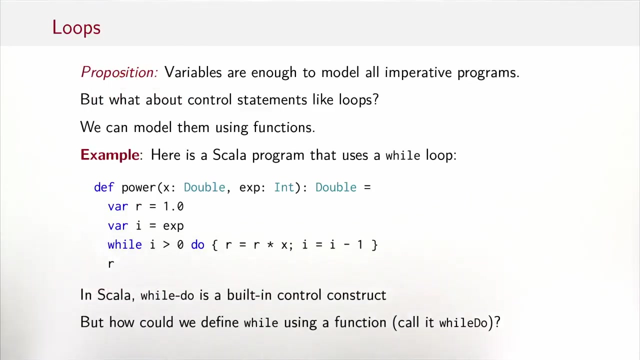 in proofs about programs based on structural induction. In this session, we're going to look at a core concept of imperative programming, namely loops. In fact, our proposition is that variables are enough to model all imperative programs. So what about control statements such as loops? 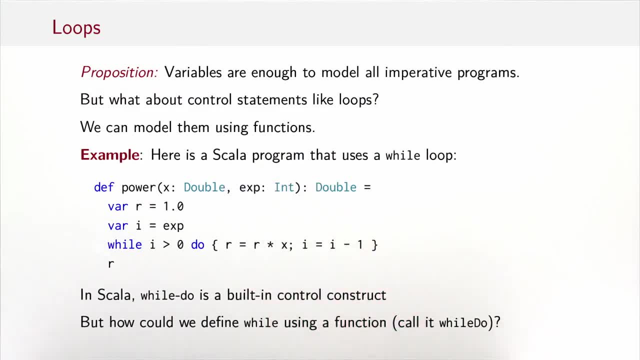 In fact, we can model them just using functions. For instance, here is a scalar program that uses a while loop. So it's the imperative. computation of the power function takes a double and an exponent, and then you have a loop that, while the exponent is greater than zero, you multiply the value. 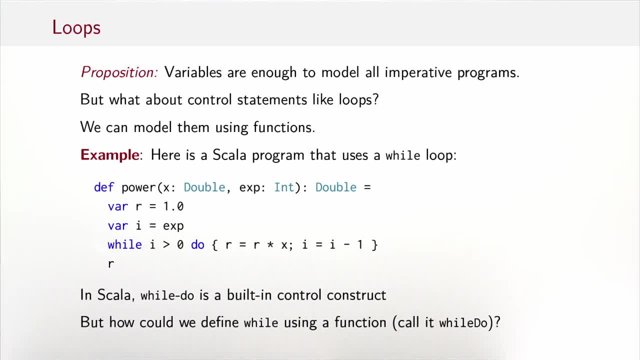 of r, here with x, and you decrement i by one and finally you return r. So in Scala, while do is a built-in construct, but we could define it also using a function. Let's call it while do. How would that work? 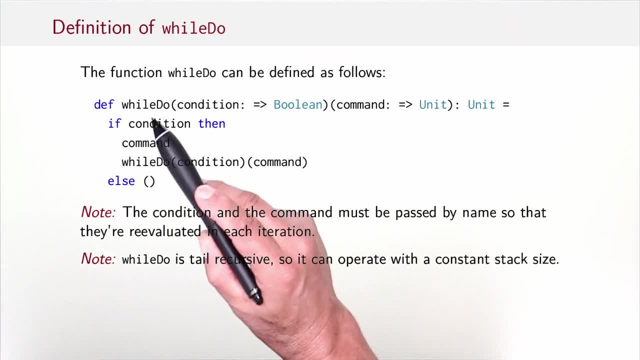 Well, here's how we could define that function. We have: while do. it would take a condition and a command. So here's an example: application of while do. You would write while do. while do x greater or zero. y equals y times y. x equals x minus one. let's say: 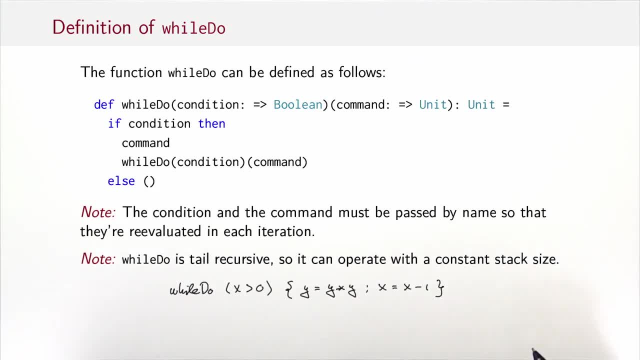 Something like that, Assuming we have two variables, y and x, defined. So what that translates to is a function call for while do, with a first argument, x, greater than zero, and a second argument which is two. That's the body that you see here. 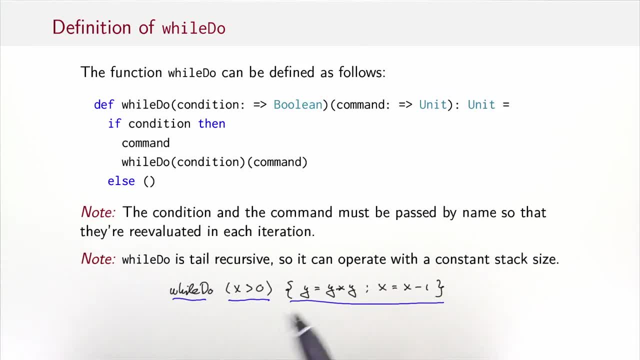 So these are just plain function arguments. They can be written in parents or in braces, It doesn't make a difference. So to make this call syntax work, we need a definition of while do with two parameter sections. The first has type boolean and the second has type unit, which is essentially the uninteresting. 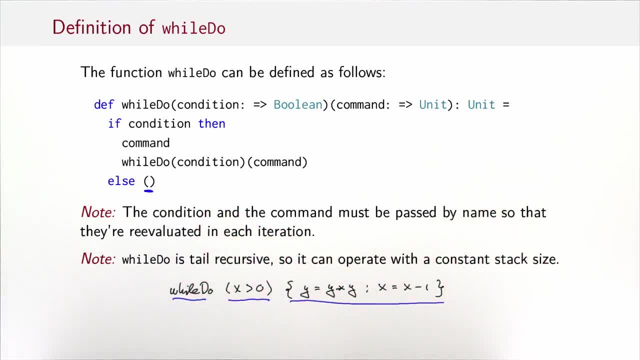 type that only has the single value: open parents, closed parents. The result return type of the while do is also unit. It's important to note that both The condition and the command are by name parameters because the actual arguments will need to be evaluated multiple times as we go through the loop. 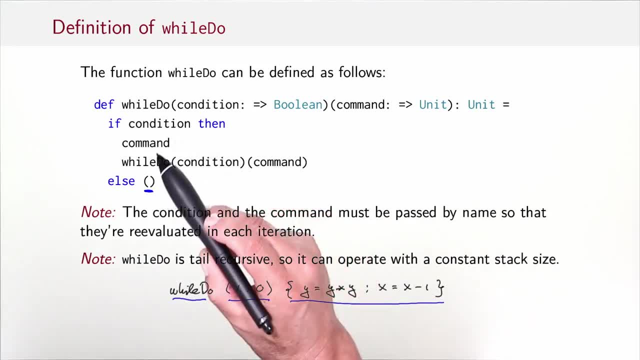 The body of the while then is as follows: If the condition holds, then execute the command and recursively call while do with the same condition and the same command, Otherwise terminate. that means return the unit value as a result. So quick check is: while do tail recursive. 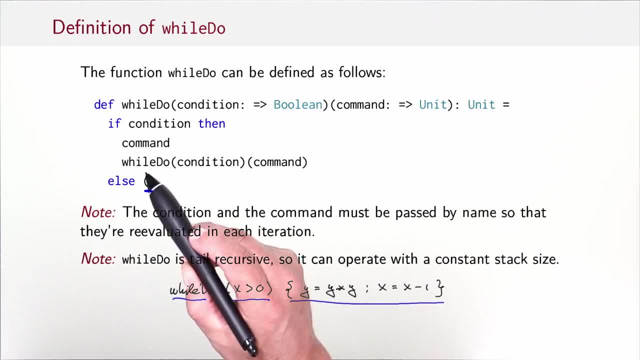 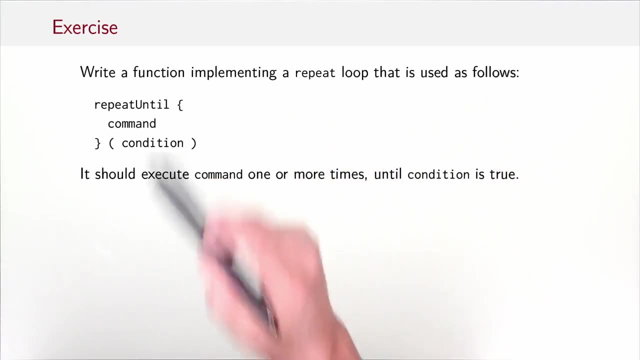 The answer is yes. It calls itself only as its last action here. So that means while do can operate with constant stack size, just like a native while loop. So here's an exercise for you: Write a function implementing a repeat loop that is used as follows: 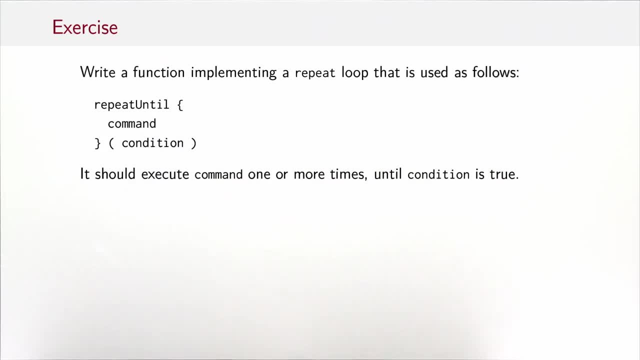 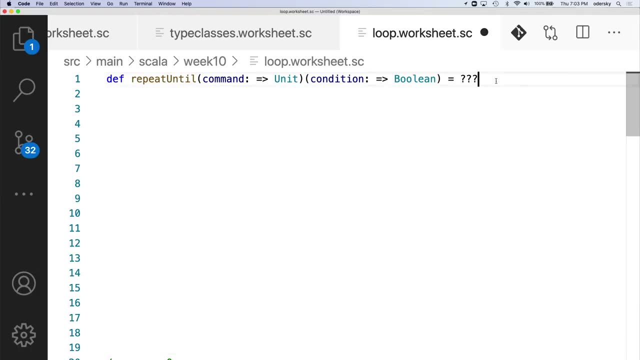 Repeat until then a command and then a condition. It should execute command one or more times until condition is true. So let's look at the worksheet. We need to implement this function here So it will execute command at least once. So let's do that and get it out of the way. 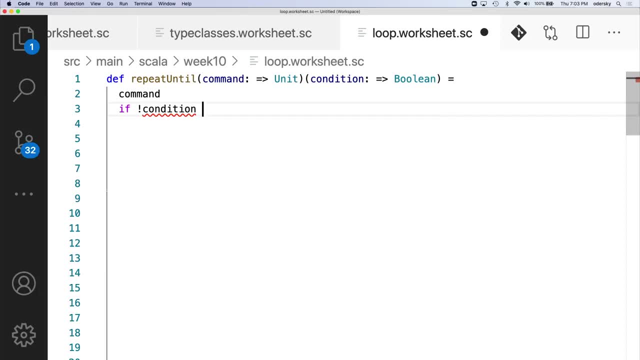 And then we say: if the condition is not true, if the condition is true, we finish, But if the condition is not true, then we will do another iteration through the loop, Else we will return the unit. Okay, Bye, Bye. 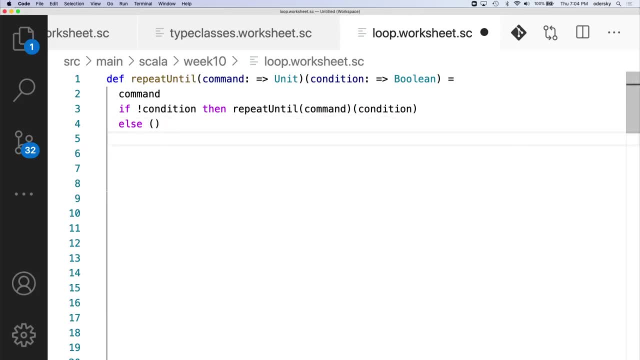 So let's see what happens And take the classe type And sorry, it's over loaded. And let's go to aíveis And let's after how many And say unit value. You get an error here. It says over loaded or recursive method. repeat until needs return type. 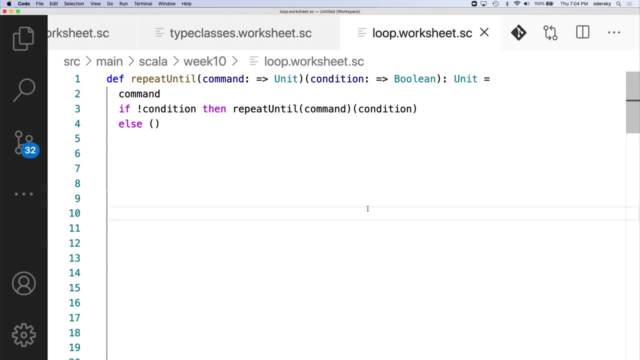 Yes, that's a limitation of starlass type inference that as soon as a method is recursive it needs a return type. In this case it's just unit, As a simplification. if you have an if, then else returning unit values, so of type unit. 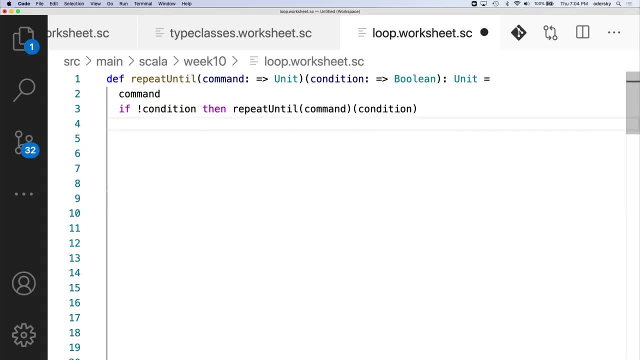 then you can leave out this else: unit value. so this would work just as well. So let's put it to the test. I have here this little program involving variables x and y, and we go through the loop until x is 5, doubling y at each iteration. So what we get are the initial 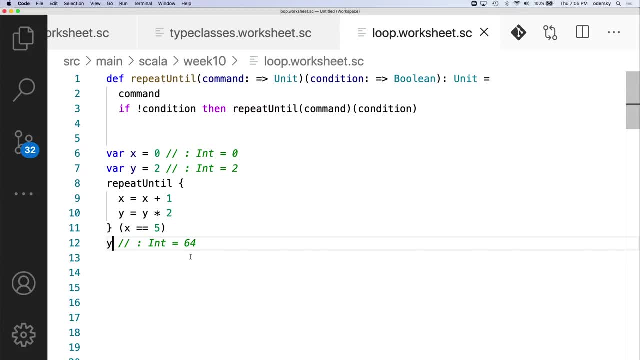 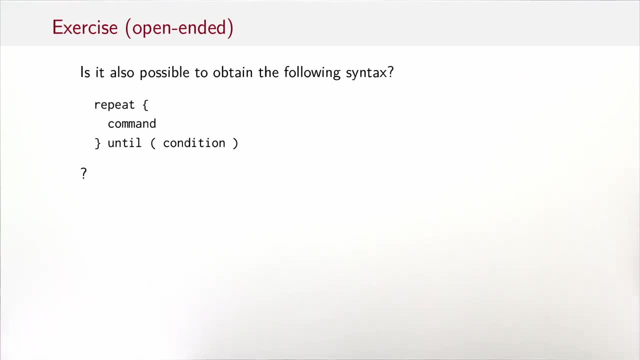 values, and the final value for y is 64, as expected. So here's another exercise which is optional and more open-ended. Is it also possible to obtain the following syntax, which would look more like a repeat: until in a traditional language, We want to write repeat and then a command, and then we want to write. 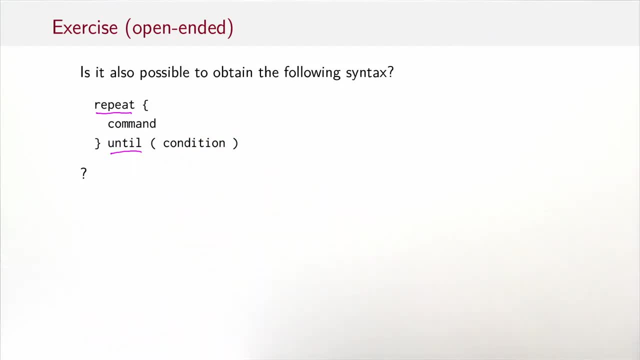 until like this, and the condition should follow the until. Can we write a scalar definitions that support that calling syntax? So to find a solution, let's analyze what this dsugars to. It would be repeat of the command in parents or not, or braces, it doesn't matter. and then it 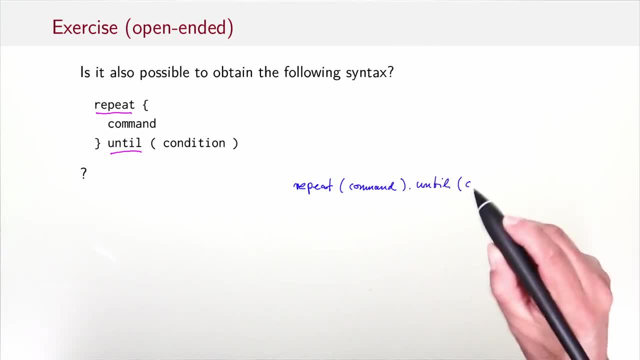 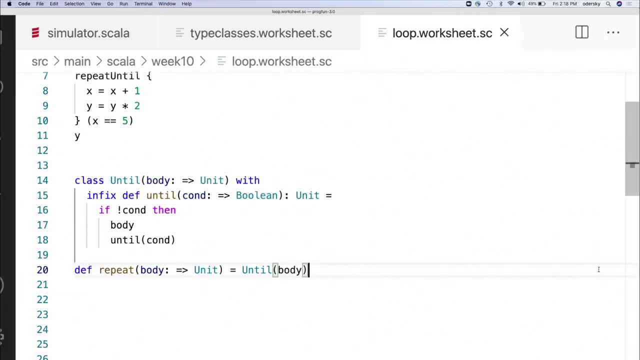 would come down to a method call until, which gets the condition as additional argument. So that means we are after a repeat function that returns something that has an until method. So you see a possible solution in the worksheet. I define a repeat method which takes a. 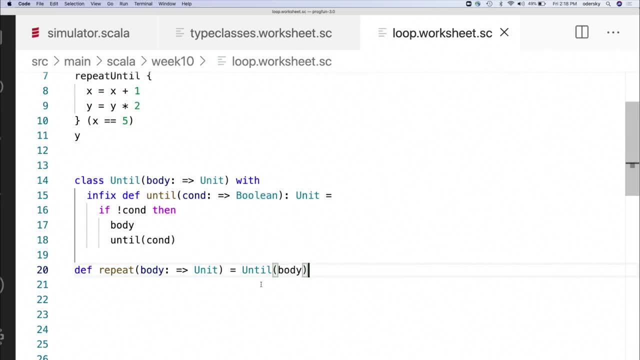 by name parameter body, and it creates an object of class until capital, until passing it. the same body, So until, takes body as a by name parameter again and it has an until method lowercase now which takes another condition also by name and its body. then would say, well, if the condition doesn't hold, then I go once. 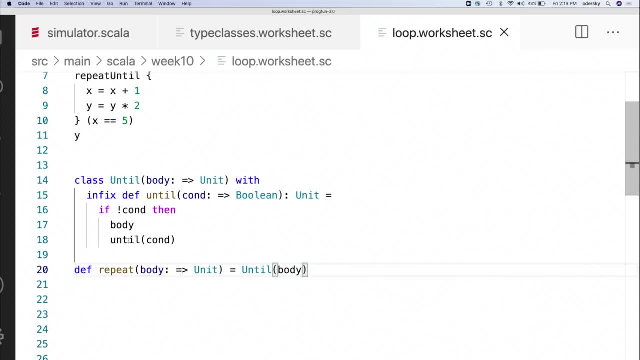 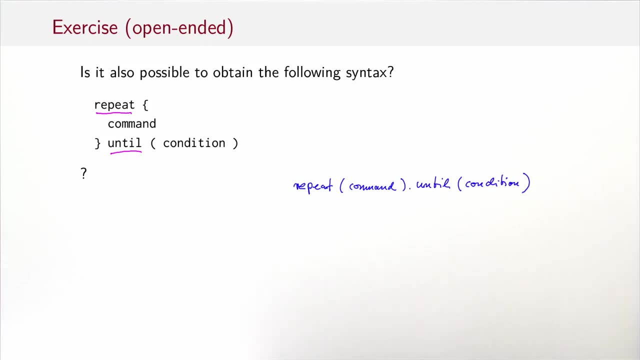 more around the body. So execute body and recursively call until with the same condition. So that would be a solution In future Scala versions to be able to write this without a warning. I should declare until infix, because otherwise it would insist on a dot in front and 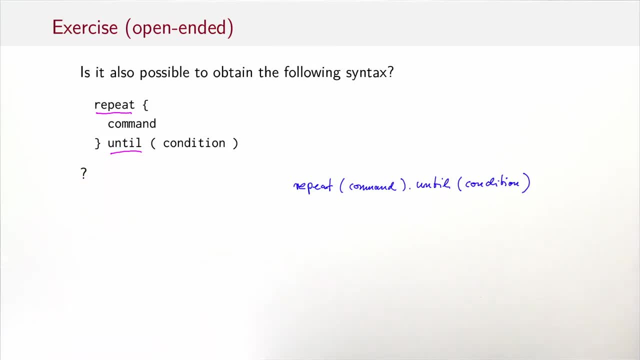 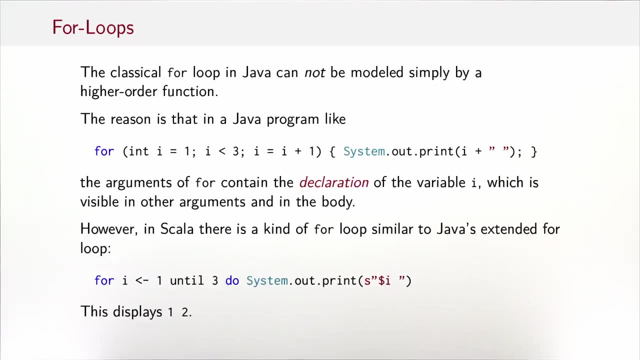 to keep the sort of more traditional command syntax. I don't want that, So that's why we have an infix annotation in front of the until at the worksheet. So we've seen that we can do while loops and repeat loops credibly using just functions in. 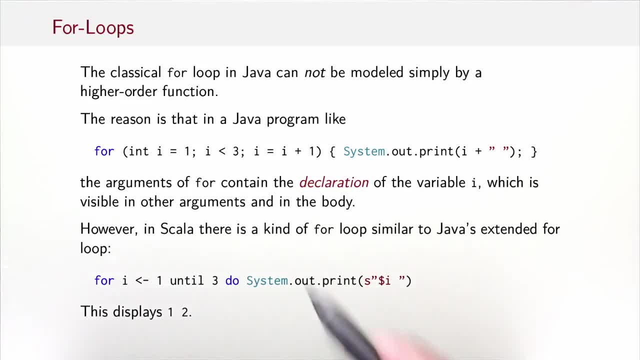 Scala. What about the classical for loop of C or Java? So the classical for loop cannot be modeled simply by a higher function. The reason is that in a Java program like this one, the argument of for contain a declaration. this one here. so that's a new declaration of i. it defines a new i inside. 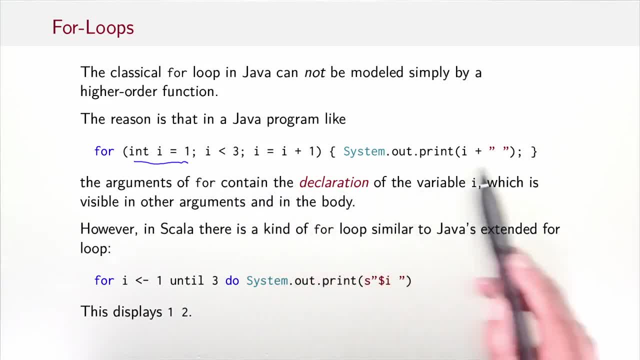 an argument which then is visible in the other arguments and in the body, and that wouldn't work, because whatever we write as actual arguments for a function in Scala would stay there. so anything we define here, its scope would just be the first argument here and the remainder wouldn't see that. 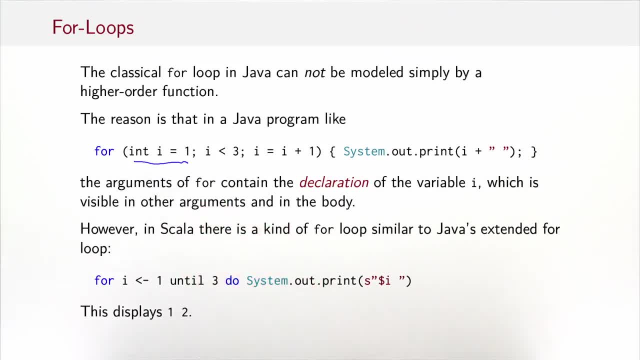 the thing we define here. However, in Scala there is a kind of for loop similar to Java's extended for loop. so what we can write is: for i taken from one to three, do, system out dot print and then the value of i. So for loop like this is very similar to a for. 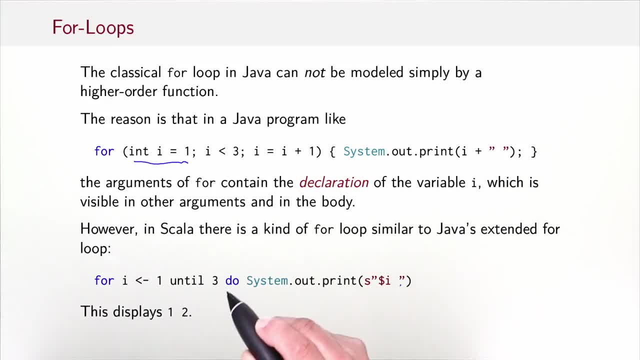 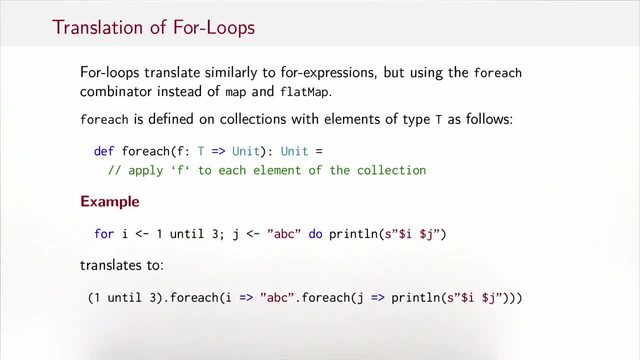 expression that you have seen already, except that where we have yield in a for expression, we have do in a for loop. Like for expressions, for loops also translate into combinations of higher order functions. but instead of a map and flat map, they translate into the function for each. 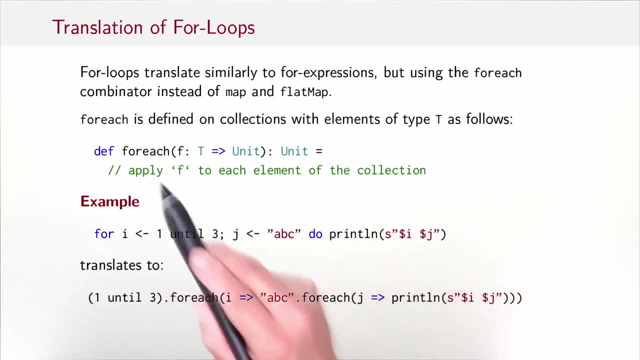 for each is defined on collections with elements of type t, as you see here. So for each takes a function that maps t to unit and returns unit, and what it does is it applies the given function to each element of the collection. So, for instance, this, for expression: 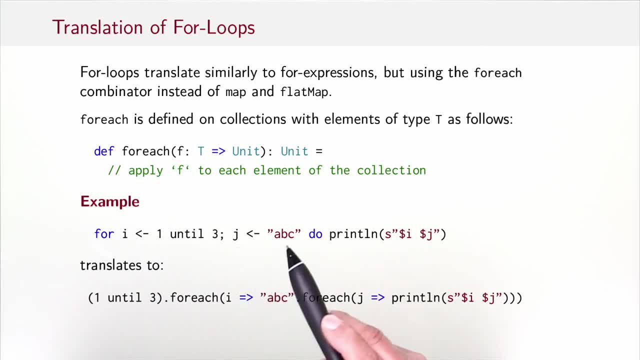 for i, taken from one until three, j, taken from the string a, b, c. do print on i and then g- that would translate to one until three- the range dot for each i, a, b, c, the string dot for each j, and then print on the body that we have seen up here. 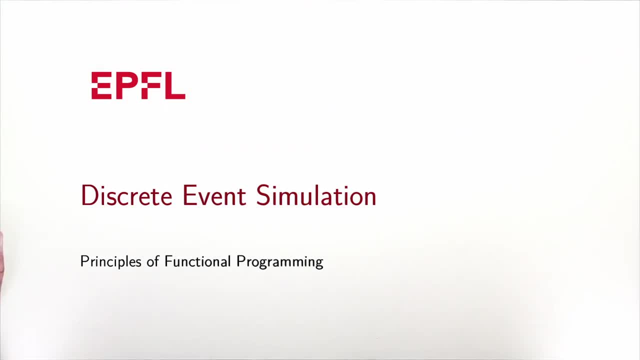 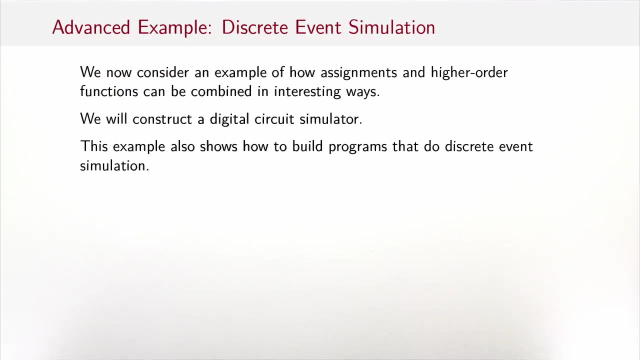 This session will be all about an extended example program dealing with discrete event simulation of digital circuits. This example will show interesting ways how one can combine assignments and higher order functions. Our task will be to construct a digital circuit simulator. There are a number of things that we need to do. We need to define a way to specify. 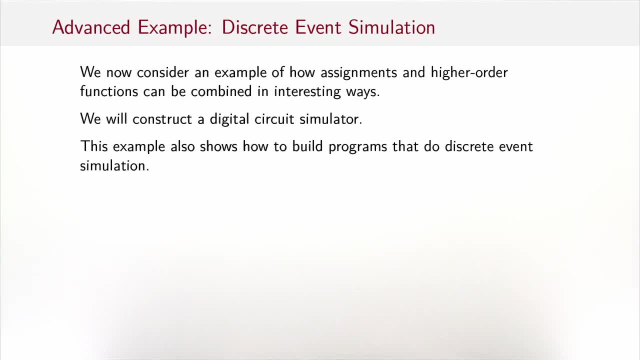 digital circuits. We need to define a way to how to run simulations, and then we have to put everything together so that the circuits can actually drive the simulator. This is also a great example that shows how to build programs that do discrete event simulation. So we start. 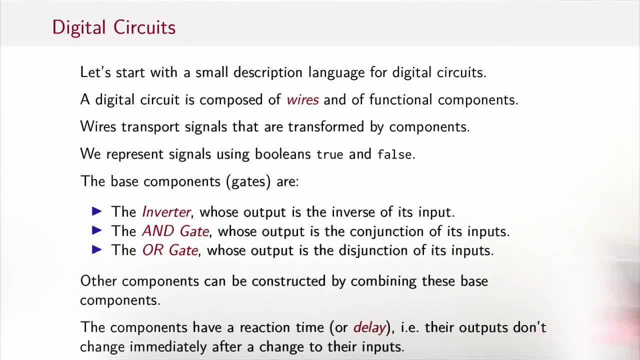 with a small description language for digital circuits. A digital circuit is composed of wires and functional components. Wires transport signals and components transform signals. We represent signals using booleans- true and false- So it's a digital circuit simulator, not an analog one. A signal is either true or false and not, but not something in between. 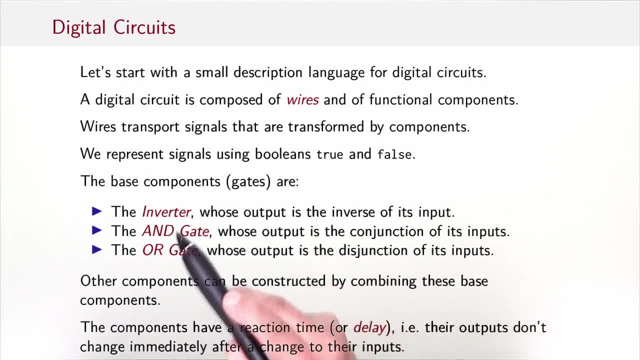 The base components are also called gates. They are the inverter, whose output is the inverse of its input, The AND gate, whose output is the conjunction, the logical AND of its inputs, and the OR gate, whose output is the disjunction logical OR of its inputs. Once 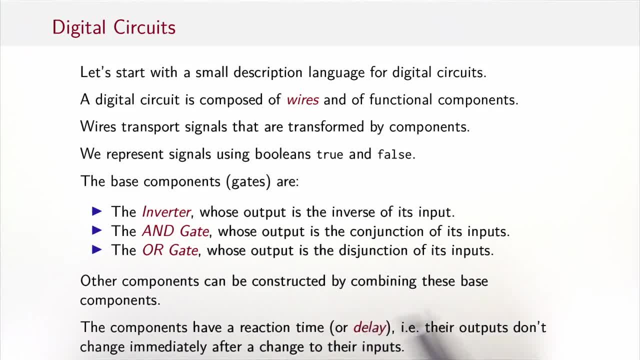 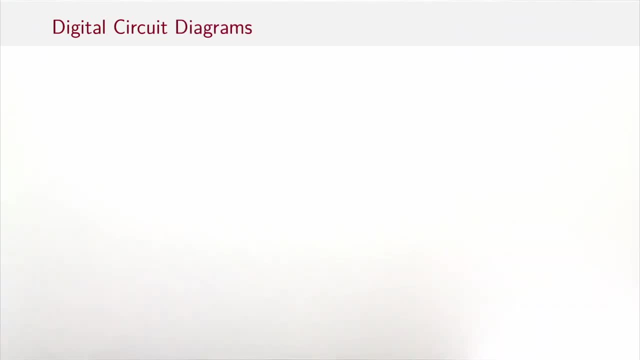 we have these three. we can construct the other components by combining the base components. One thing important for the simulation is that the components have a reaction time or a delay. That means their outputs don't change immediately after a change in their inputs. Logical gates are usually drawn with standard symbols, So this would be an AND gate. This 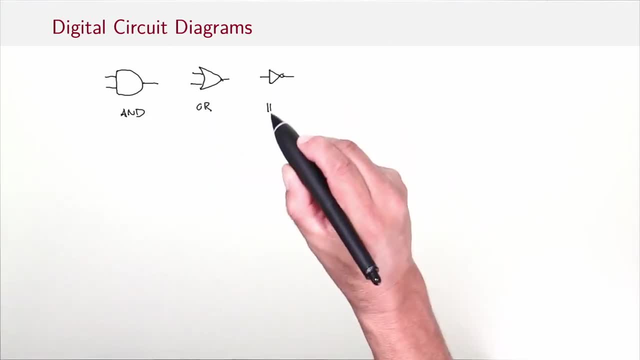 would be an OR gate and this would be an inverter. We can use the basic gates to build more complicated structures. For instance, here we have created a half adder. The half adder takes two inputs, A and B, and then it has two outputs, the sum and the carry. The carry is set if both. 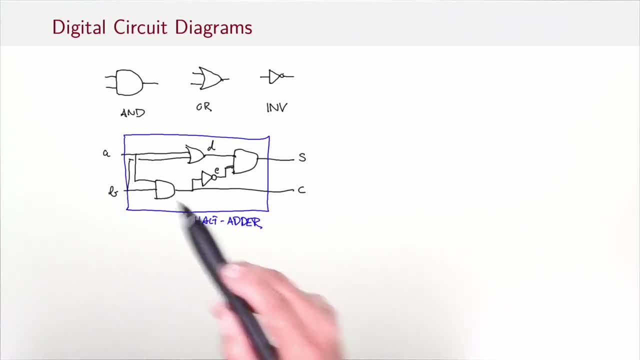 A and B are set. So we have a logical AND gate that goes into the carry output. The sum is set if either A or B is set. We have an OR gate here and the carry is not set. So we have an inverter. 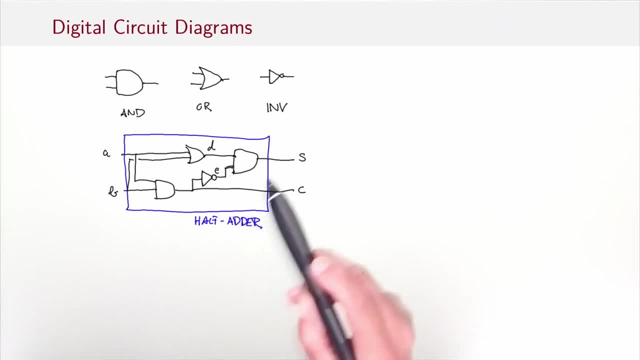 here, So that one is set if the carry is false. and here we have an AND gate, So the sum is true only if either A or B is true and carry is false. Once we have defined a circuit like a half adder, we can use it in turn to define more complicated circuits. For instance, we can use two half adders. 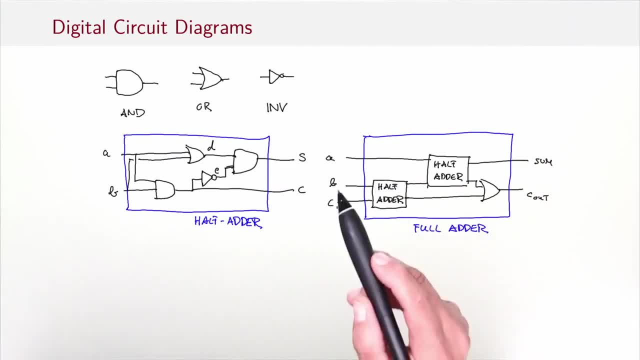 to define a full adder. What we do here is we first have a half adder that adds B and C in producing a carry here and a sum here. We take the sum and add A, so with another half adder. So the final sum is the sum. 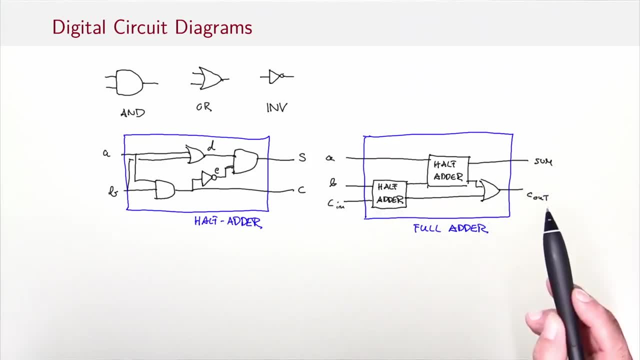 of the whole full adder, and the output carry is then the logical OR of the carries of the two half adders that you see here. So our next question is: how do we put that in code? What we have to do is essentially find code representations for these three basic circuit diagrams so that they can be composed to. 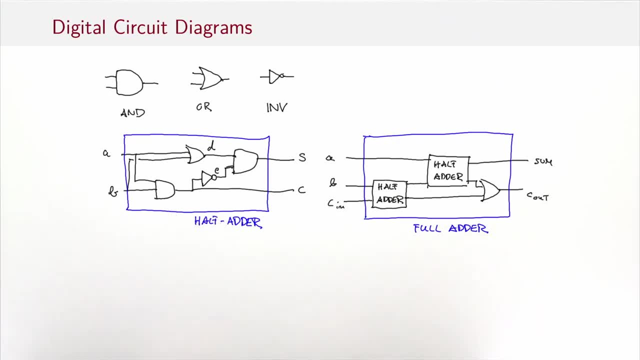 give you half adders, full adders and any other components you might wish to construct. So our basic language then consists of the three gates here plus the wires. So a wire is needed to connect gates, and here it should be noted that a wire is not, doesn't necessarily have two ends, Essentially, 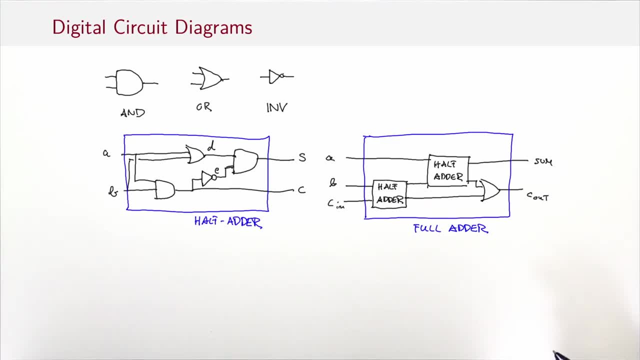 any network that has the same current electrically counts as a wire. So for instance, the A wire would be not just this line here, but it would also. that would be part of the A wire and the C wire would consequently be the whole network that you see here. So these colored things are wires, and then 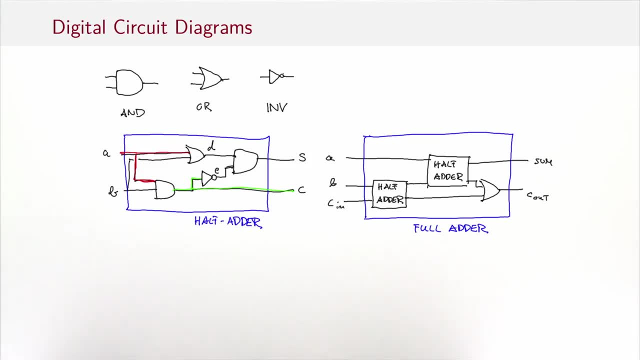 we have gates that connect the wires. That's the basic situation. You see also that the circuits are not necessarily hierarchical. They're potentially complex networks of components connected by wires. The way we're going to represent that is that we are going to have a 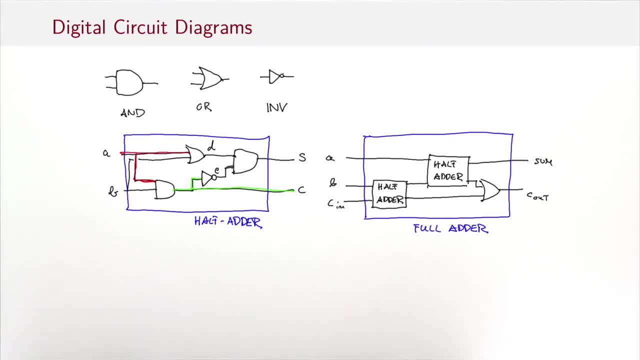 class for wires. and then we have a model where, essentially, we drop a gate, a component, onto a circuit board, connecting it with the wires that are there. So essentially, our idea to construct a circuit is based on side effects. We you can think of it as 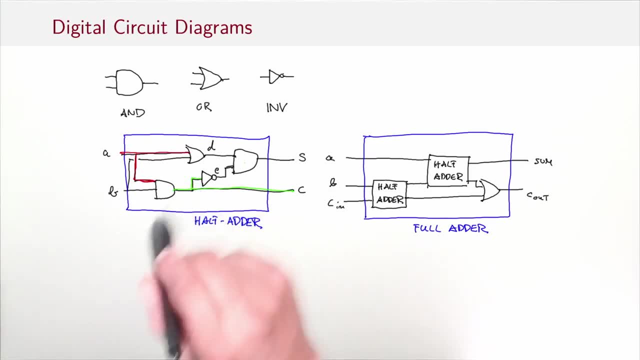 essentially, you have a circuit board, you have some wires and then, essentially, you put the gates as an action onto this board and connect them with the wires. That's the mental model that we are going to pursue. So to start, we need a class wire to model wires, So wires can then be. 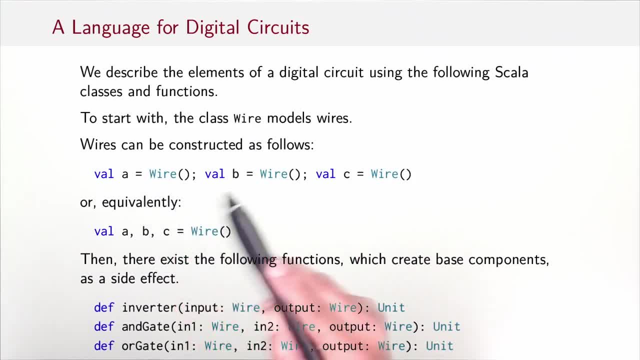 constructed as follows. You can say: A equals a new wire, B is a new wire, C is a new wire or a scalar allows you to shorten that. You can just write well, ABC equals wire. That means each of these three names will get the same right hand side, namely create a new wire, And then we need 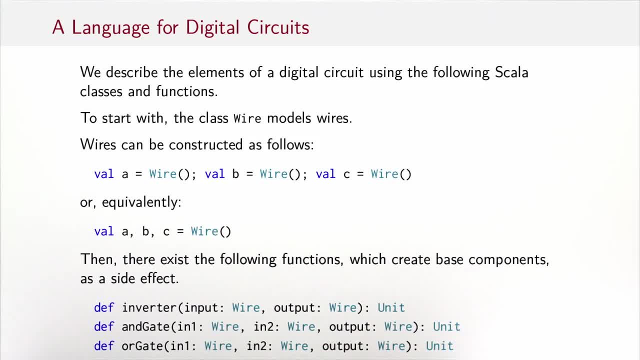 functions that create the base components. as a side effect We drop them on the board. So inverter says place an inverter between the input wire here and the output wire there. AND gate says place an AND gate between the two inputs here and the output there, And OR gate says 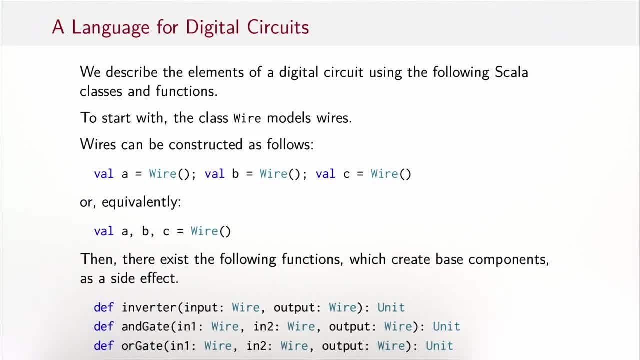 create an OR gate with those two inputs and the output. All three methods have unit as the result type. That means they act only as a side effect. by essentially connecting themselves to the wires, They don't return anything interesting. Starting with these basic elements- wires and 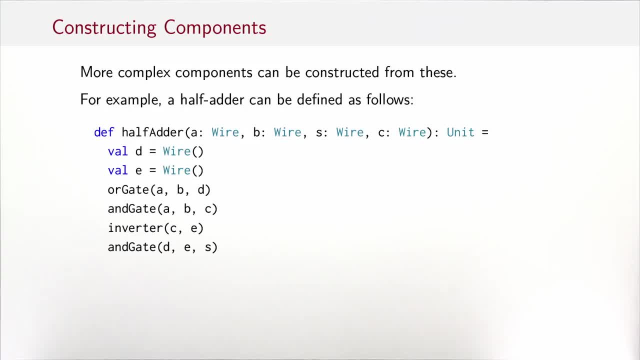 three kinds of gates. we can construct more complex components. For instance, here's how we can define a half adder. So it says we have four wires: A, B, S and C. We create some internal circuits which we're going to use later. We place an OR gate between A, B and D. So that would be an. 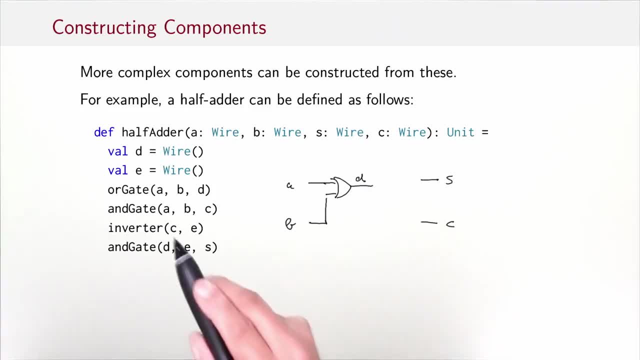 OR gate here, and that would be D. We place an AND gate between A, B and C, So that would be my AND gate here, and that would be C. You can connect that already. We place an inverter between C and E, So that would be E now, And we place an AND gate between D, E and S. Okay, and that's an AND. 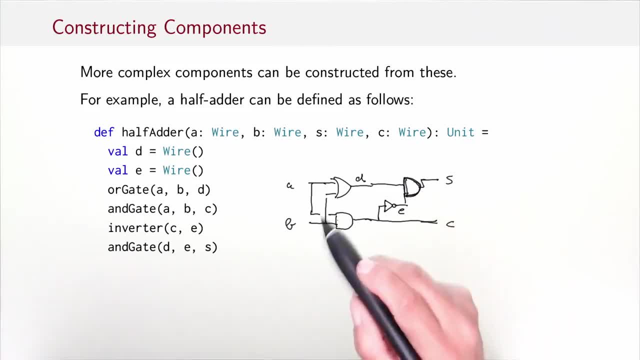 gate, not an OR gate. Okay, and that's my half adder. So I define a method which means I draw a box around it and now I can use this thing as its separate component. So now I can start to drop half adders on my circuit board and connect them to further wires. So here's how you would do a. 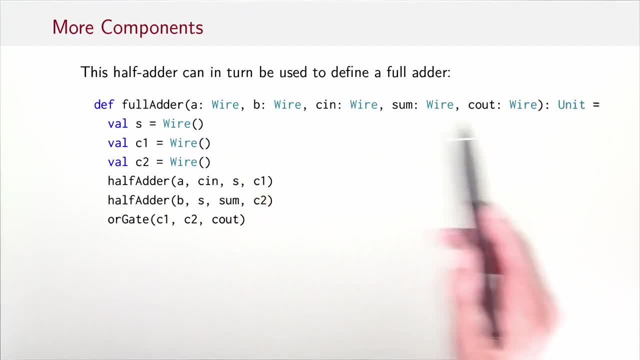 full adder. It takes three input wires, two output wires has three internal wires and you place two half adders on the board, connected as you see here, and an OR gate for the two output carries. that gives you the final C out signal. I invite you to do that yourself just following. 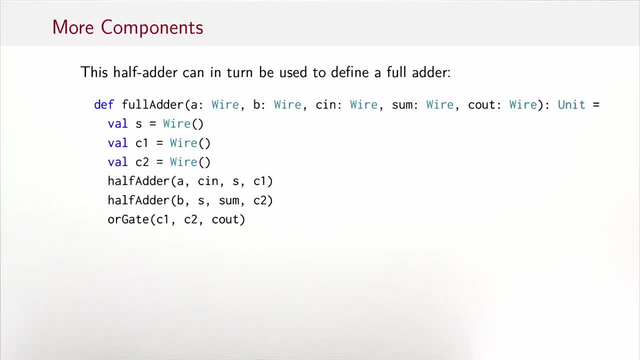 these instructions and verifying that you will get the full adder that we've seen some slides ago. So here's an exercise for you. What logical function does this program describe? There's a function f- our mystery function- that takes two input wires A and B. 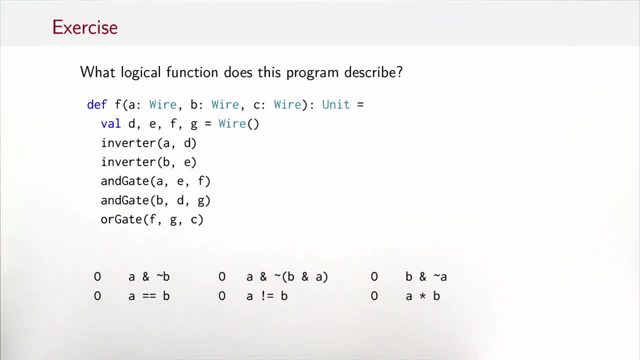 And has an output, wire C. And here are its internal workings. What's the logical function that gives? Is it one of these six that you see here below? So one way to solve this puzzle is to look at these gates as describing logical formulas, For 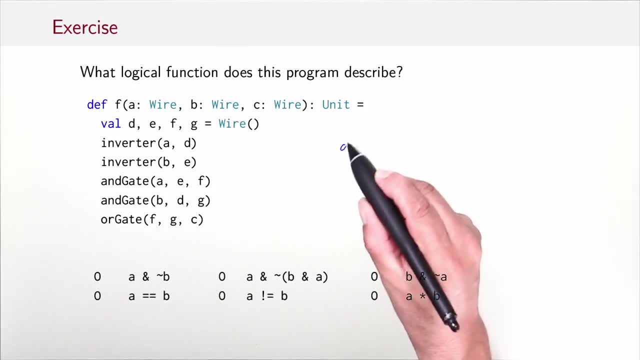 instance, this inverter here would define the signal D to be NOT A. Similarly E equals NOT B. Then f is A and E. So f is A and NOT B, G is B and NOT A, And the final result c is f or g. So the final result is true if either A is true and B is false or B is true. 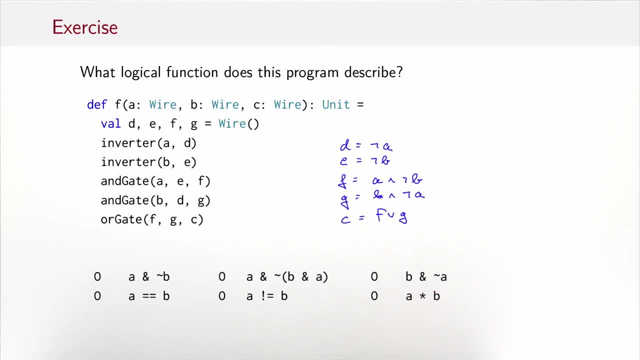 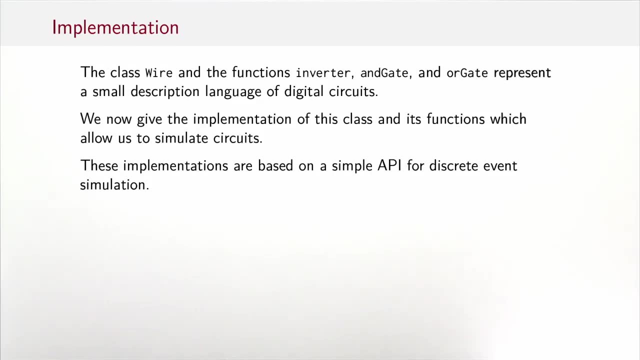 and A is false, Which means to say that the final result is true if a and b are different signals. So that's the answer to our puzzle. Okay, let's proceed to an implementation of all this. So the class wire and the functions inverter AND gate and OR gate represent a small description language. 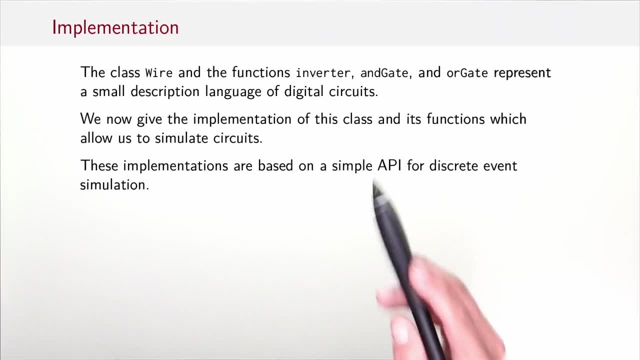 for digital circuits. We now need an implementation of this class and these methods to allow us to simulate circuits. So to be able to do this, we first have to clarify how do we do simulation? what interface do we have to run a simulation? So what we do next is develop a simple API for discrete event. 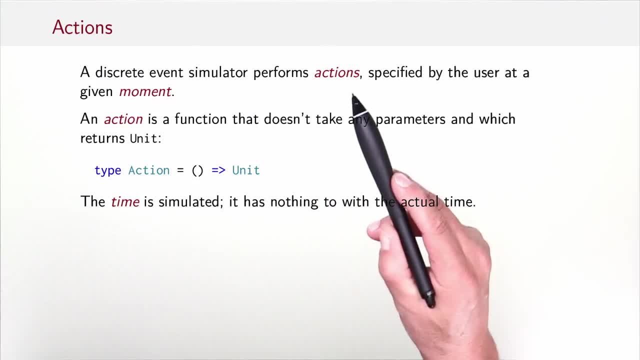 simulation. So a discrete event simulator performs actions that are specified by the user to be performed at a given moment, And an action is a function that doesn't take any parameters and which returns unit. So an action is really just something that lives for the action, the side effect. 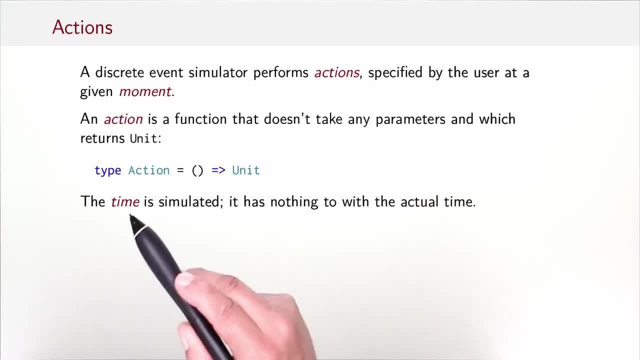 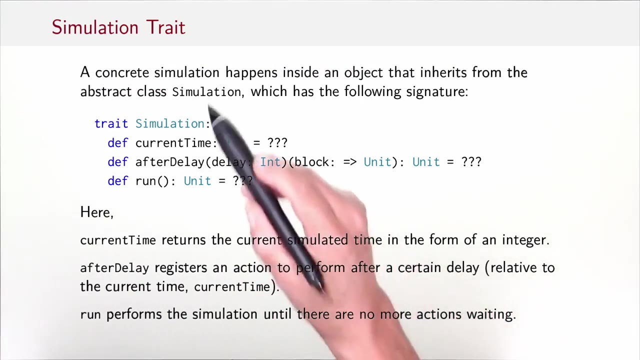 that it performs, And the time when an action is performed is simulated. It has nothing to do with the actual time. So there's an internal timekeeping unit that essentially advances the time as the simulation progresses. So the way we'll set it up is that a concrete simulation will be inside an object that inherits. 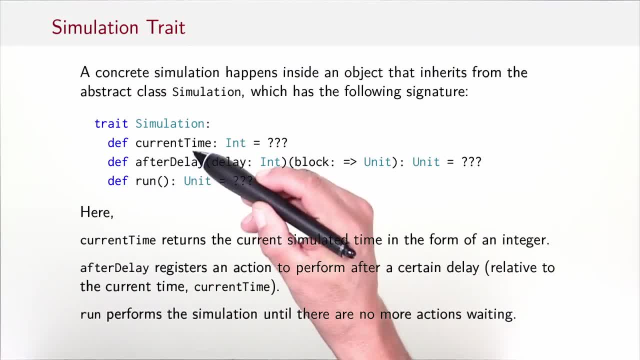 from the trait simulation. and the trait simulation has the following signature of methods and members that we can use in simulation. object: So first there's the current time, which is the simulated time, So that's the current time in our simulation. Then there's a method after. 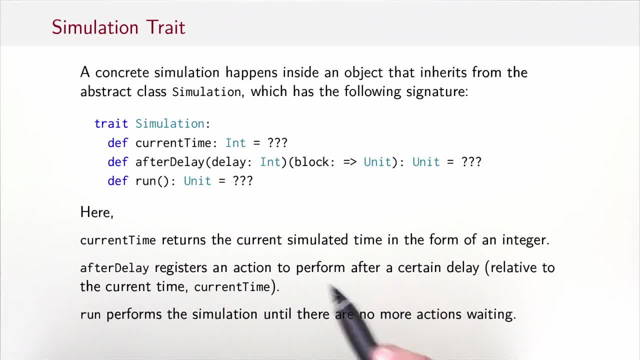 delay: that registers an action to be performed after a certain delay relative to the current time. So we say, after delay, n units run this block of statements. So what this does is it essentially stores this block to be run once the simulation has reached the time that's specified by current time. 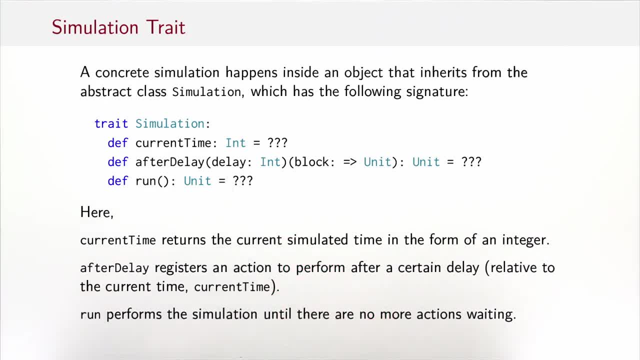 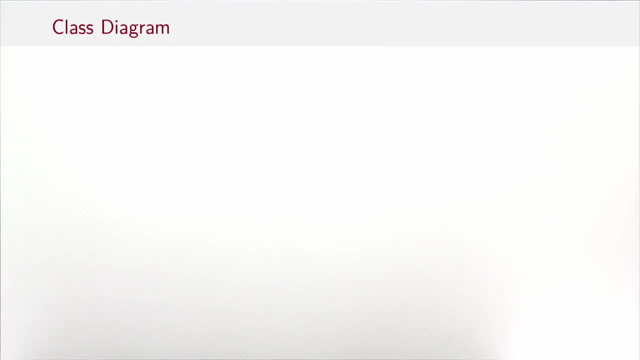 plus delay. But after delay doesn't run the simulation by itself. that's done by a separate method called run. So run essentially says: well, these actions that are now stored for the simulation, they should be performed. at this point, Before going into details, I want to show you the outline of the different components. 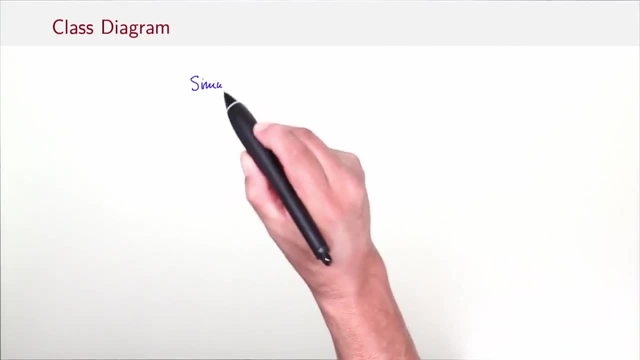 that we are going to assemble. So at the very top is the simulation trait and that will be inherited by essentially our structure. that defines the basic gates. Gates need simulation because they will. it's in the end them that will be simulated. And then from gates we will have another trait. 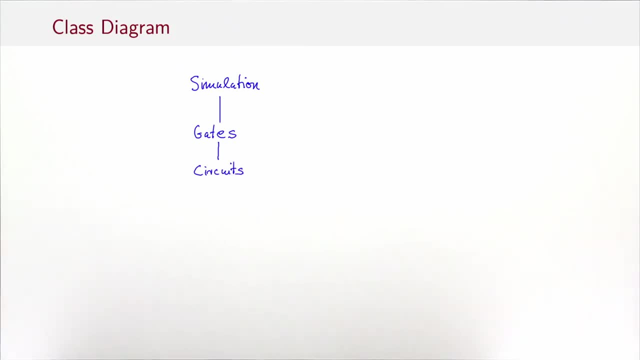 called circuits. that contains things like half adders, full adders or other circuits that a user might want to define. So here we sort of up here. that's essentially. the system provides a simulation package and it provides the basic gates. When we define circuits then maybe some of them are provided by the 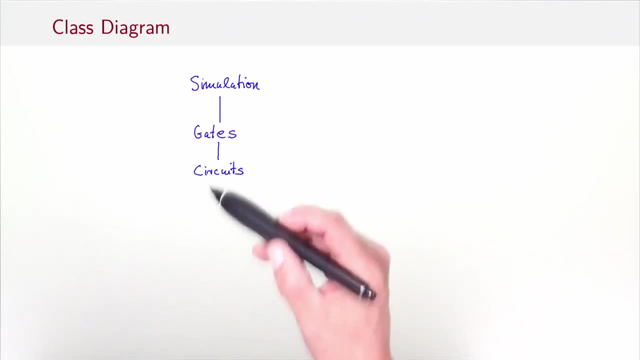 system, and others could be provided by the user. So we could also have several classes here that essentially define different libraries of circuits. In our example we just need a single one, And then finally we will have an object called, called its simulator, which is the concrete simulation, So the concrete. 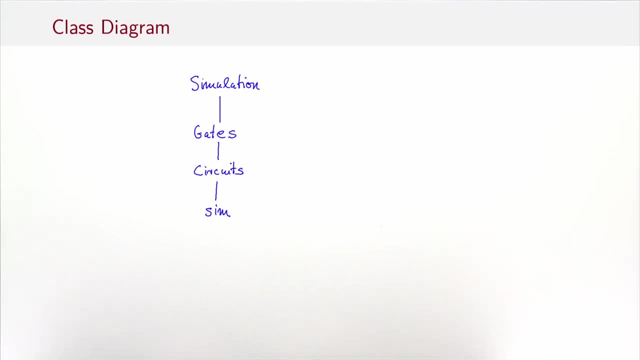 simulation essentially defines a test circuit that we now define as a simulation. So this is the concrete simulation that we now want to run and simulate. So we have already shown the circuits layer when we defined half adders and full adders. So that showed how to define these circuits. 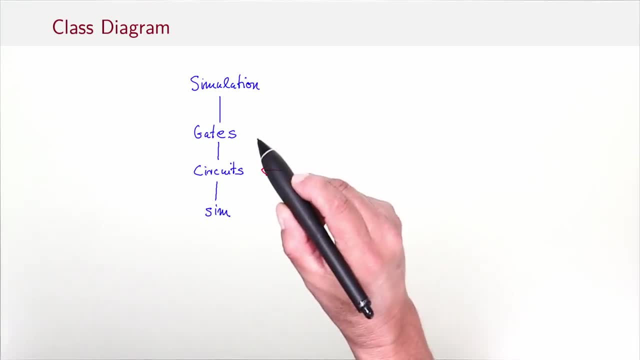 What we still need to do is we need to fill in the blanks for the gates class- What do inverter and AND gate OR gate actually do, and how is wire defined? and we have to fill in the simulation class to implement the API that we have. 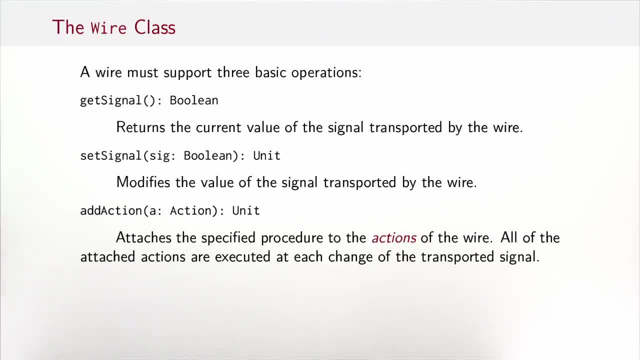 defined. So let's turn next to gates and in gates. let's turn to wire. So a wire must support three basic operations. The simulation might want to know what is the current signal on the wire. Is it true or false? It might want to set. 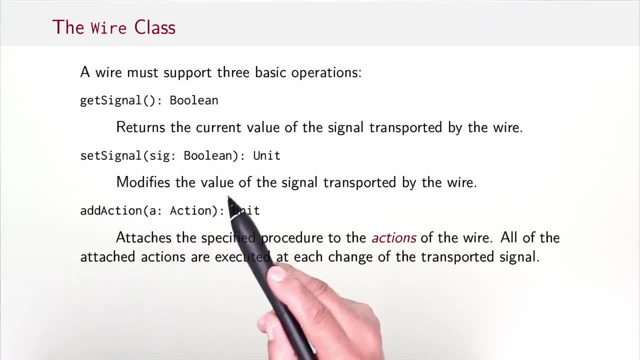 the signal of a wire as an action, So that would modify the value of the signal transported by the wire. And the third basic operation, add action, allows the simulation to customize what should happen when the signal of a wire changes. We can add an action, we can attach that to the actions of a wire and all of 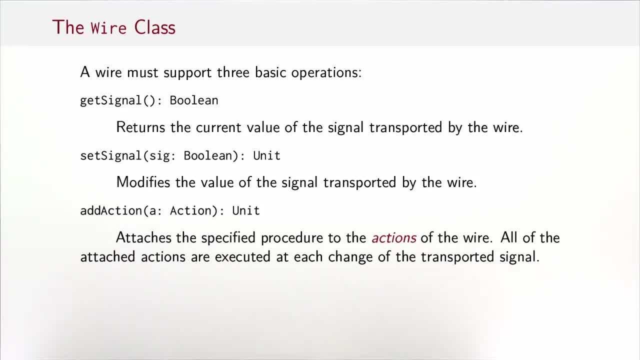 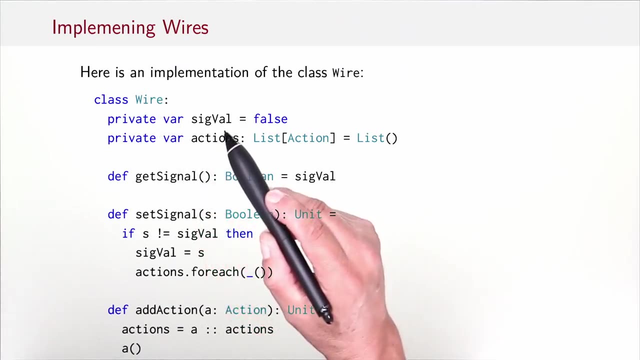 these attached actions are executed at each change of the transported signal. So basically, we register an action to say perform this action when the signal of the wire changes. So here's an implementation of class wire. Internally a wire would have a signal value. 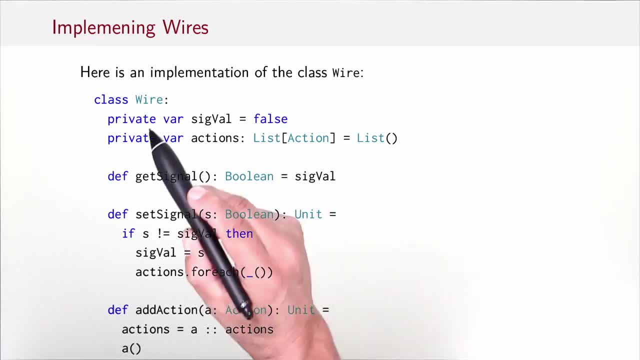 Initially it's from the beginning false, so no current and that's private. so you can't access it from the outside. And the other piece of state in a wire is the list of actions that are currently attached to the wire. Initially that's the empty list. 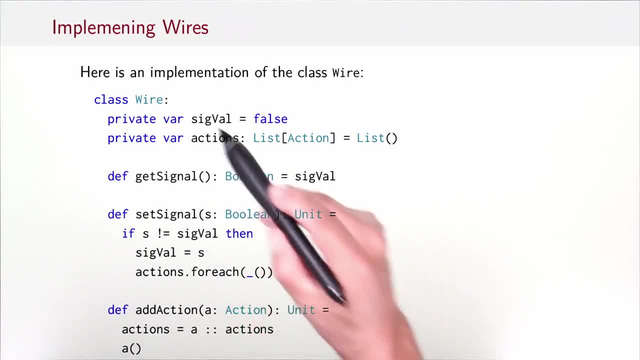 Now here are the three methods. GetSignal simply returns the current signal value. So the setSignal operation sets the current signal value to the signal s and it also executes all the stored actions if the signal value changes. So this line, here it's maybe a bit cryptic. so let's analyze what this is. 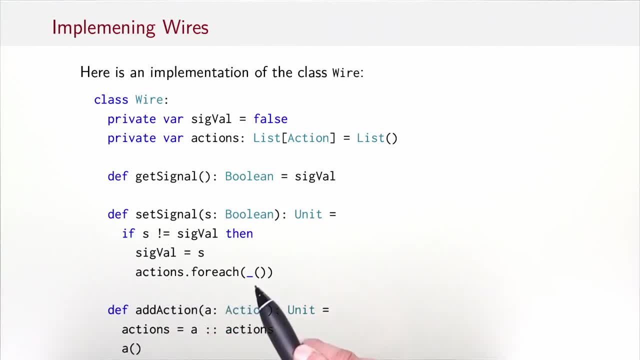 It does a forEach on all the actions. and what does it do? Well, it calls the action with the empty parameter list. So that's what that does. You could write this also a bit more expansive to say: for a taken from actions, do a for. 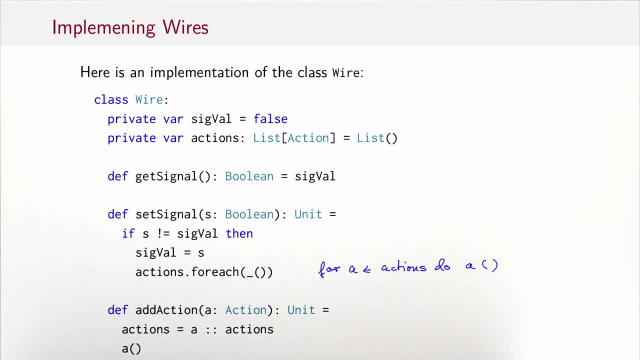 execute the action a. That's probably a bit clearer. The last operation, addAction, simply adds the given action to the list of actions on the front, and then it immediately calls the action. So why is that? Well, you can think of the circuit initially to be in an undefined state. 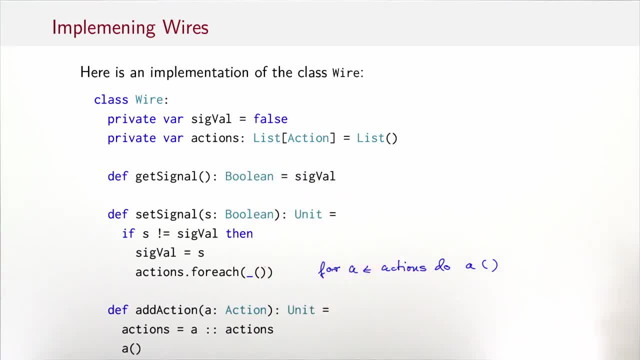 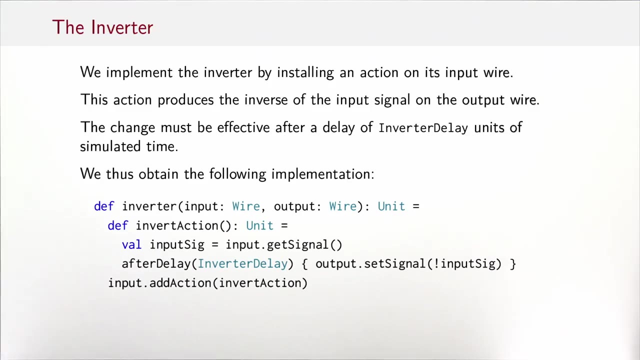 So when I said signal value equals false, I really should have said undefined. So once we have an action, essentially we immediately execute it to essentially force the signal to be defined, namely to be the output value of that action. So once we have wires, we can now proceed to define the basic gates. 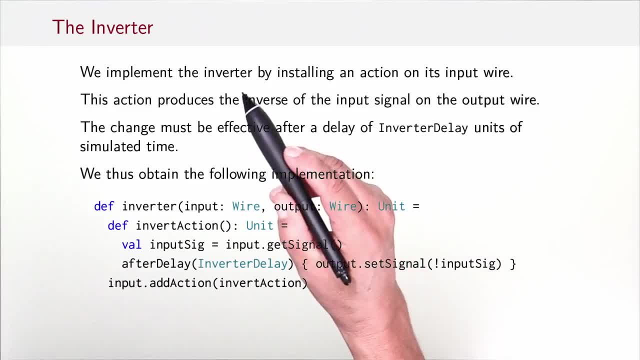 So let's start with inverter. We implement an inverter by installing an action on its input wire. So we have here input, addAction, invertAction. And what does invertAction do? Well, it will sample the signal on the input wire and set the output to be. 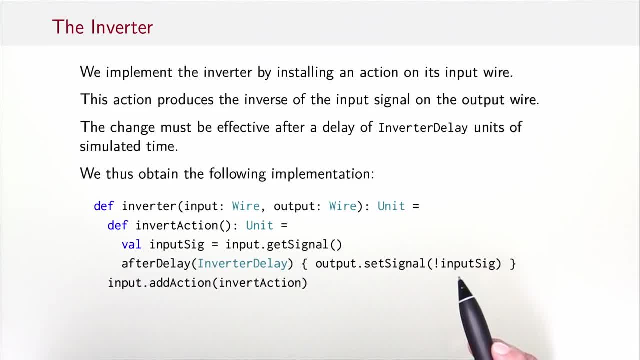 the negation, the not of the input signal. That's what inversion means. But it will do so not immediately but only after the inverter delay that we still have to specify. So to summarize, we have said before that placing an inverter on the board, essentially 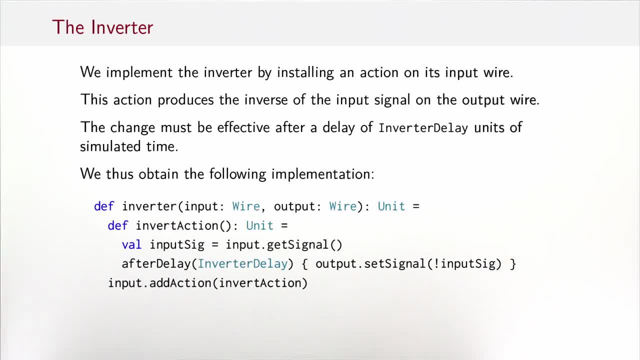 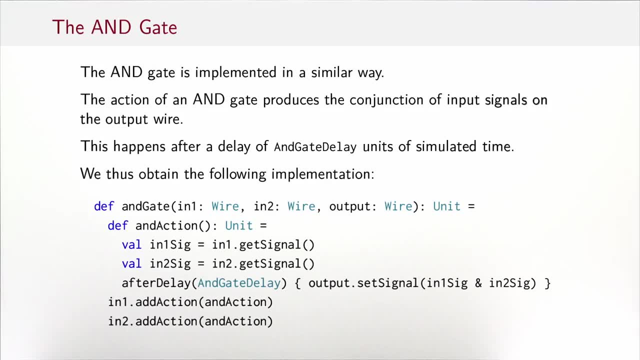 produces a side effect. What the side effect is is to add the invertAction to the set of actions on the input wire. If we now look at AND gates, It's implemented in a very similar way. So again, the AND gate function here has a side effect. 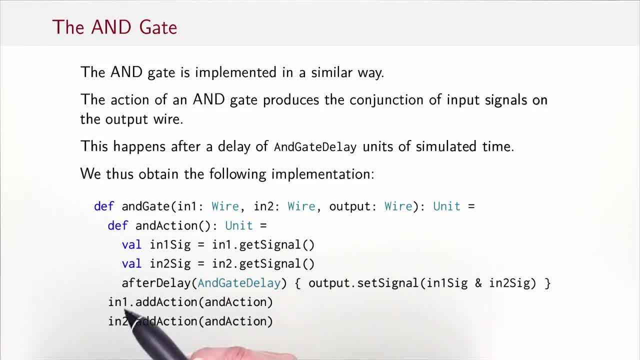 And the side effect is to add the AND action on its two input wires, in one and in two. So what is AND action? Well, we get the signal from the two input wires here and here, And then we set the output signal to be the AND of the two input signals. 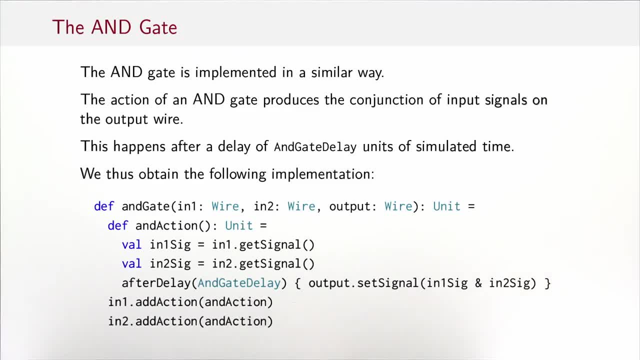 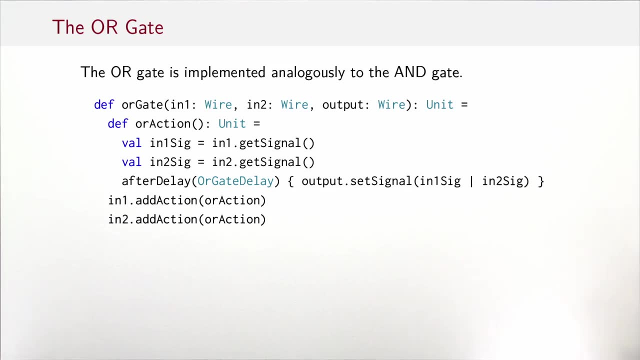 And we do so only after a delay, namely AND gate delay, So this action will be registered in the simulation to be take place at a point in time and gate delay from the current time, that is now, And the OR gate is now implemented. quite analogously, 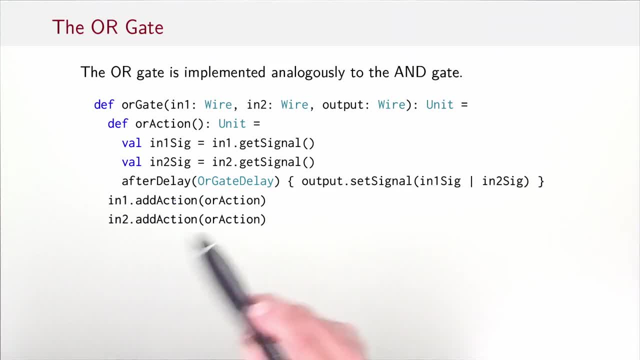 So again, it adds an action to its input wires, That's the OR action, And the OR action that simply would take the disjunction, the OR of the two input signals and do so after OR gate delay. So here's a question to you. 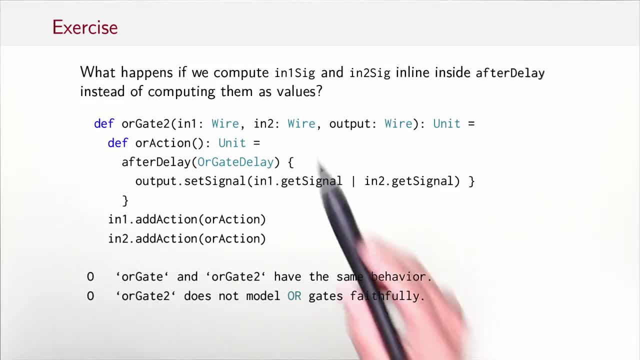 To see. if you have any questions, feel free to ask in the Q&A section. What would happen if we compute IN1-sig and IN2-sig directly inside the after delay, as you see here? So I don't bother to define them as two values in front. 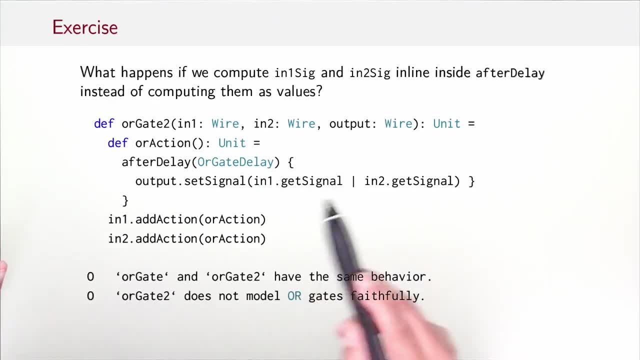 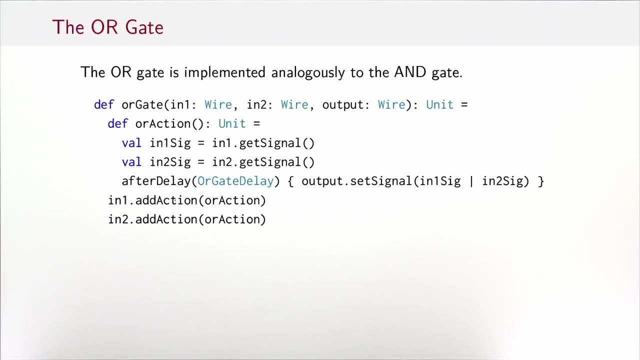 I just essentially inline them here and here, as you see there. Would that give us the same behavior Or would the behavior be different? and in this case, OR gate 2 would not model the OR gate faithfully? And the answer is, of course, that would be something different. 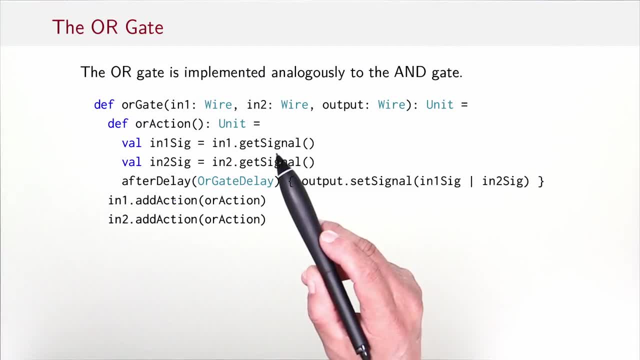 So here we get the signal at the current simulated time, That's just the GET signal, And then we wait OR gate delays and then we set the output signal, Whereas in the modified program we again wait OR gate delay units, but we set the output. 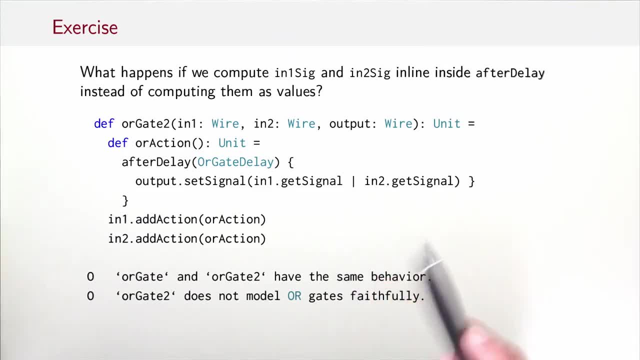 signal to the disjunction of the input signals at this point in the future. And of course, at this point in the future something else might already have happened. So this is not a faithful model of an OR gate. So let's see where we are in the worksheet. 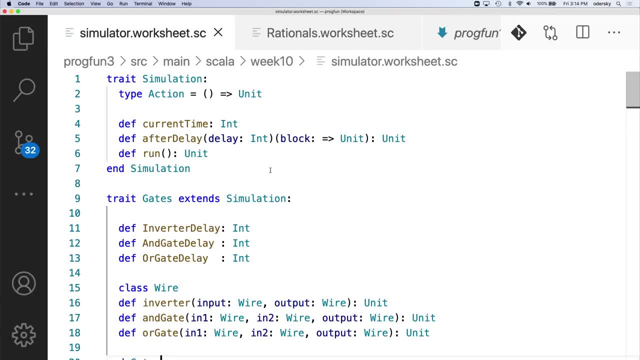 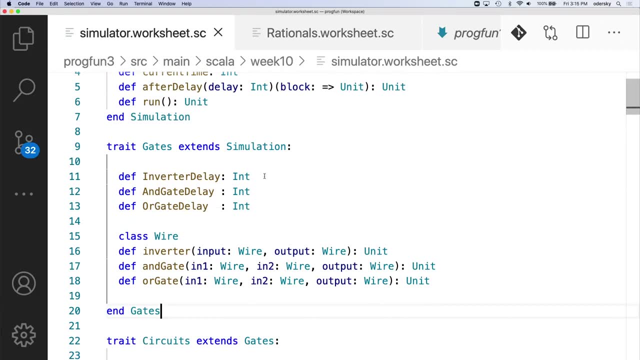 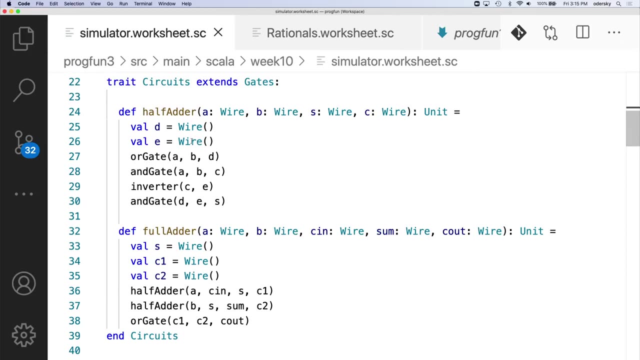 So I have here my simulation trait, which is still empty. I have my gates trait, which is again empty. I just have the class wire and the three methods, And I have the delays that are also defined here. And finally I have circuits, and there I've already added half adder and full adder. 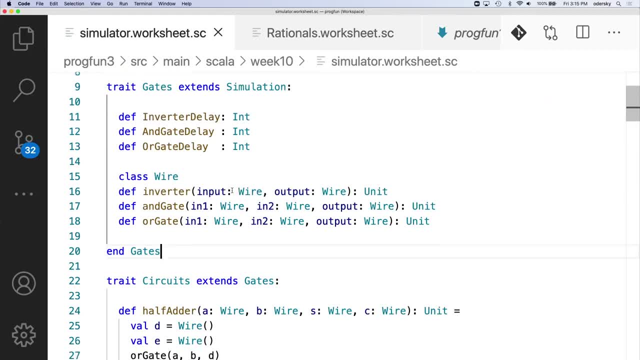 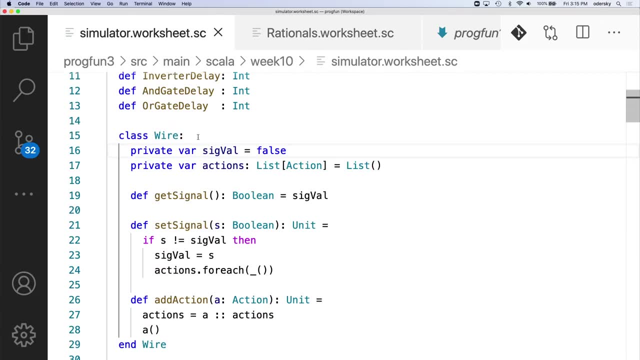 I just need the interface of the gates class, And I just need the interface of the gates class, And that interface is provided, just the implementation that is still missing. So what we've done, then, is we have implemented the class wire as you see here. 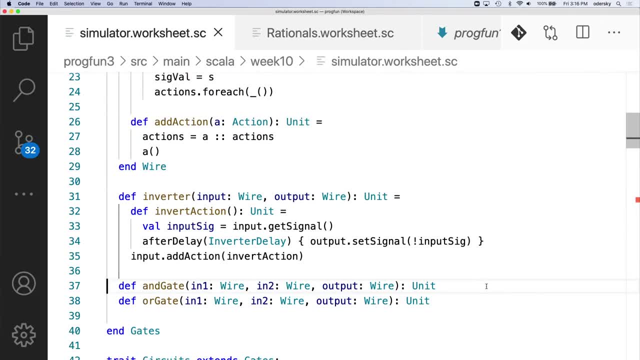 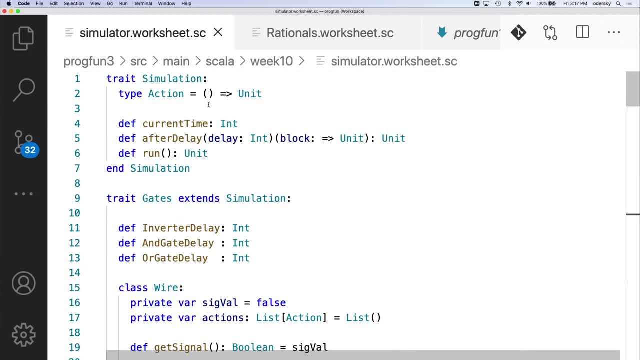 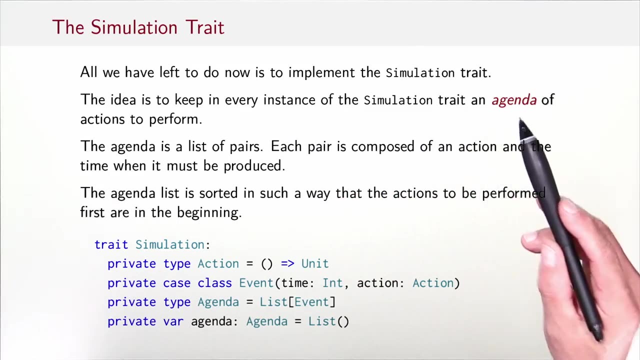 We have implemented the inverter, as you see here, And we have implemented AND gate and OR gate. So what we have to do next is flesh out the simulation trait. So the idea is to keep, in every instance of the simulation trait, an agenda of actions. 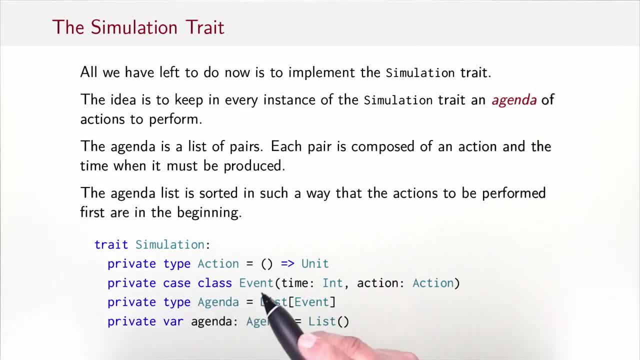 to perform. An agenda is simply a list of events, And each event is composed of an action and the time when the action must be executed must be produced. The time is simulated time. as we said before. The agenda is sorted in such a way that the actions to be performed first are in the beginning. 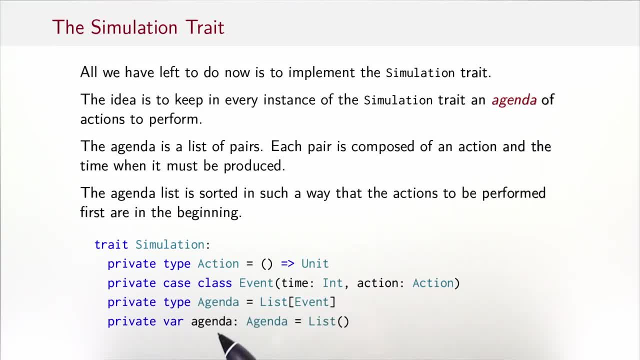 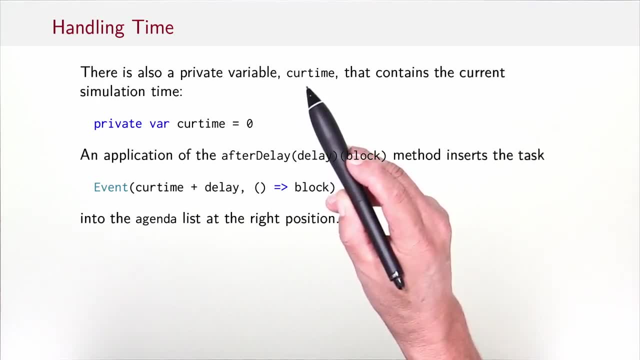 of the agenda. So agenda is a list of events, And here is our agenda, which is initially nil. There's also a private gate. There's also a private gate. There's also a variable- call it current time or code time- that contains the current. 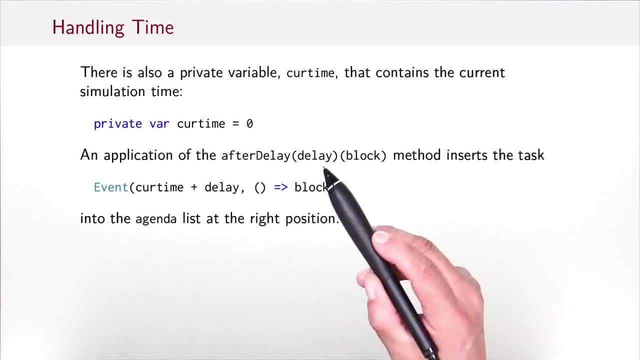 simulation time. An application of the after delay method, with some delay and some block given, inserts the task event to be produced at current time plus delay to consist of the actions in block, into the agenda at the right position. So here's after delay. 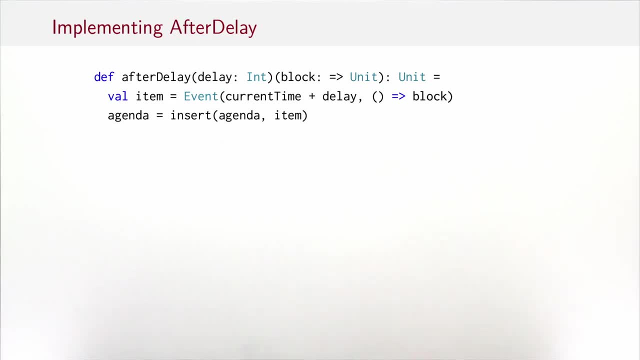 We produce the right event here And we insert it into the agenda. That's all. The insertion function is straightforward. That's essentially just what we did when we did sorting as well. So we just go through the agenda. If the time of the first item in the agenda is less or equal to the time of the item that 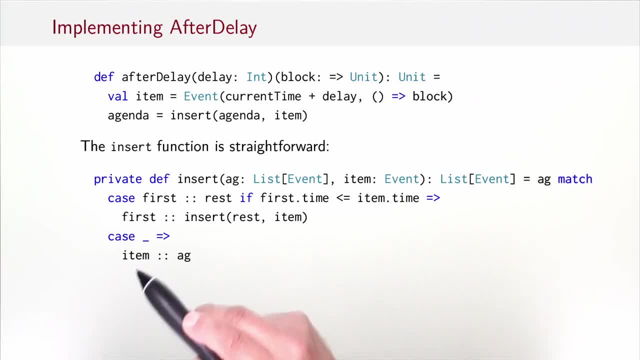 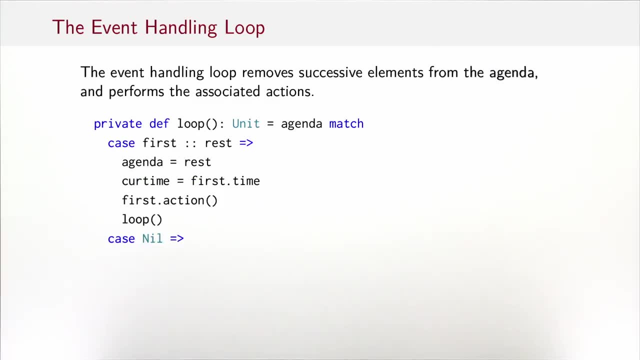 we want to insert, then we insert in the tail of the agenda. Otherwise we put the item at the top of the agenda and follow it with the previous agenda. So once we have an agenda, we need to execute it. That's done in a transaction. 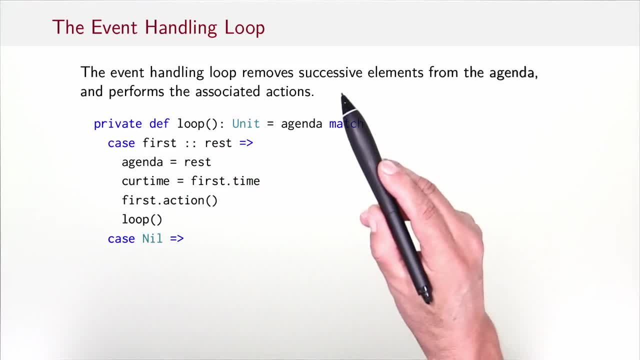 an event handling loop. The event handling loop removes successive elements from the agenda and performs the associated actions. So here's an implementation of the event loop. It does a pattern match on agenda. As long as the agenda is non-empty, it executes the first item on the 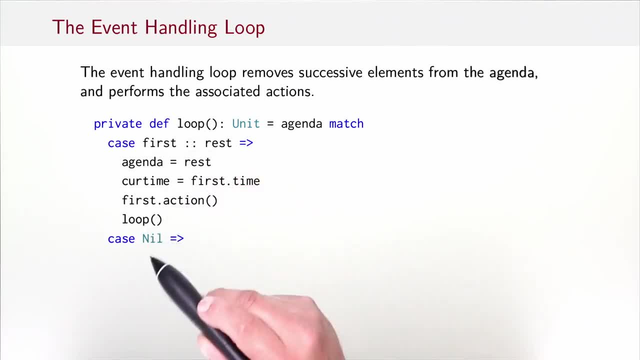 agenda and it recursively calls itself: If the agenda is empty, it terminates. What does it mean to execute the first item of the agenda? Well, we strip off the item from the agenda. so the agenda now becomes the rest. here It sets the current time to the time stored in the first entry. 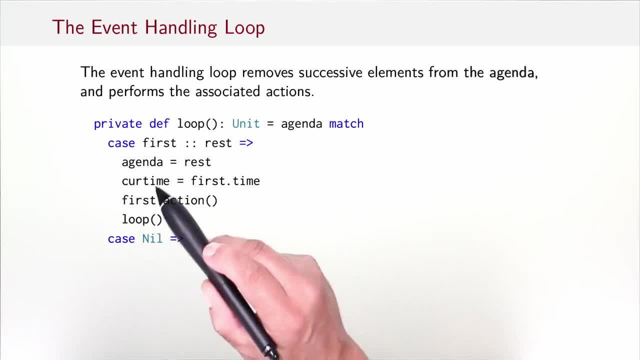 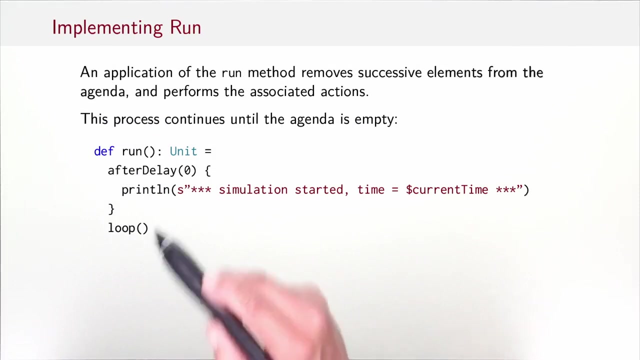 and it performs the action of the first event at this time, at the simulated time. Quick check whether the loop function is tail recursive. Yes, indeed, it calls itself as last action. That's important because, of course, the agendas for simulations might become quite long. So now, finally, the run method. Run method simply calls loop after it prints. essentially: 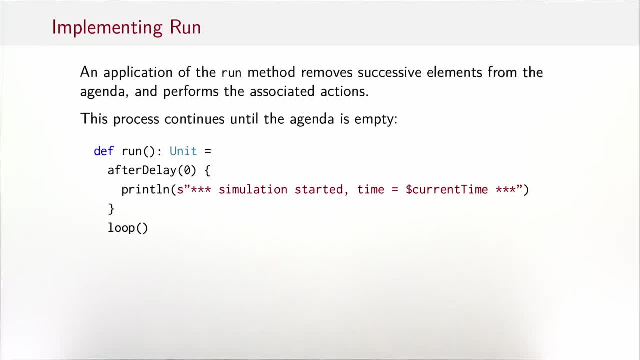 a header. It installs a first action after delay zero. that says simulation has started and here's the current time. So it puts that at the front of the agenda and executes loop. One question for you: Does every simulation terminate after a finite number of steps? At first glance it might seem so. 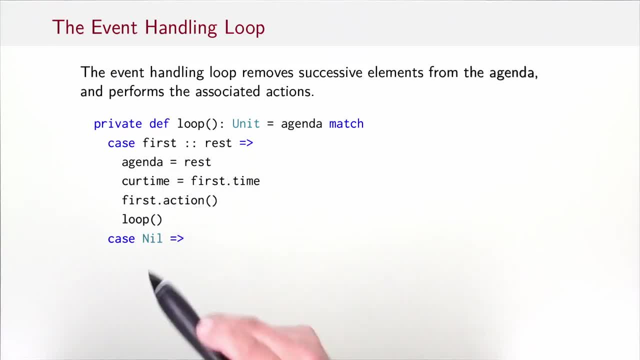 since loop just goes through the agenda left to right until the agenda is nil. However, remember that actions that are performed here can install further actions in the agenda through after delay, And that means that, in fact, we might never finish the simulation because every action will install one or more further actions in the agenda. 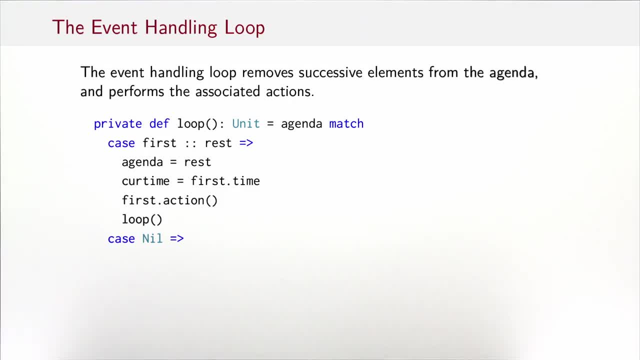 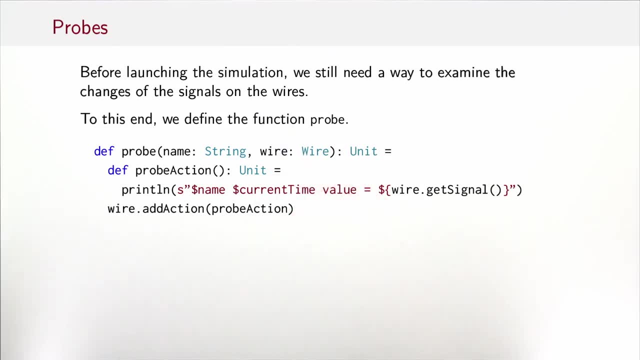 and the agenda could even grow without bounds if every action installs more than one action into the agenda. So time to try it out. But before we can launch the simulation, we still need a way to examine the changes of the signals on the wires. So far it's a black box. Something happens. 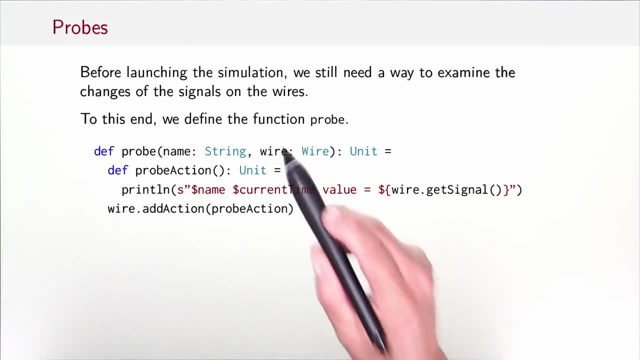 but we don't know what. So to this end, we define another function called probe. So probe is essentially: you have a wire and then you have a pair of pliers- I'm very bad at drawing- And then you have something like this: This is a very old-fashioned oscilloscope, or something like that. 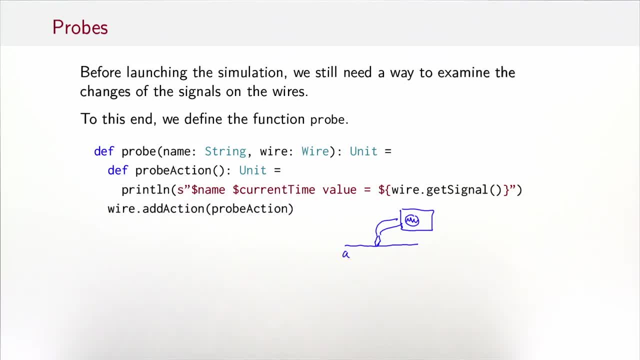 that would tell you what goes on in these wires. So that's what the probe is. So a probe gets attached to this wire here and it has a name, because we are actually going to print out the signal of the wire just, rather than throwing it, showing it as a curve like here. So what we 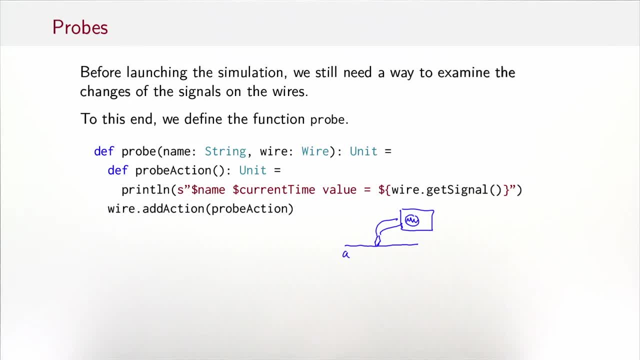 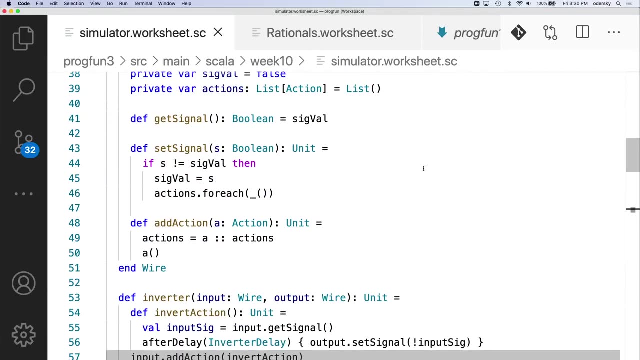 want to print is the probe action says: print the name of the wire, print the current time and print every time the signal on the wire changes. this probe action will be executed because we have added probe action as an action to that wire. i have added all these implementations to the worksheet. 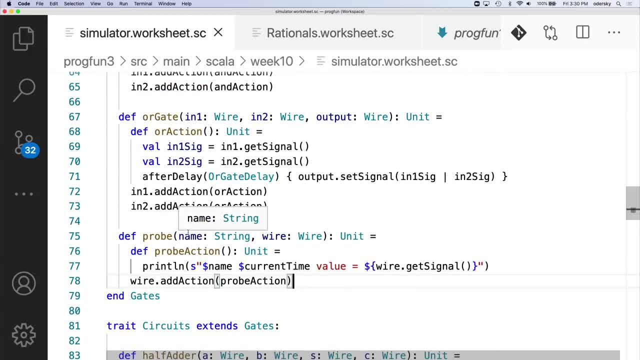 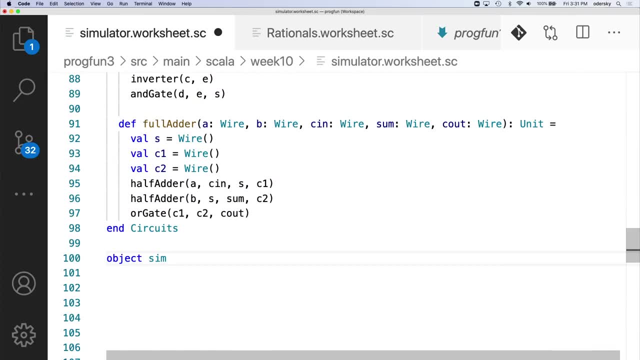 here's probe. so that's the last thing i've added here. so it's time to set up a simulation. to set up a simulation, we define an object, sim, and that extends essentially the circuits that we want to simulate, and we get an error and says: okay. so there are three things that i haven't defined yet. 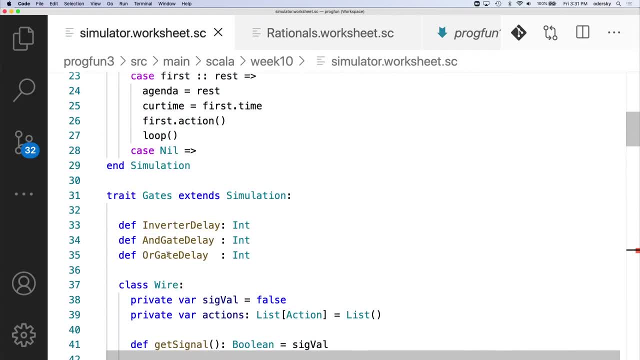 indeed those were the methods: inverter delay and gate delay and or gate delay. i could define them right here, but that wouldn't be very systematic, because when we define a library of gates then we don't really want to fix these delays at this point. the delays of these gates is technology dependent. with a new generation of silicon it might be. 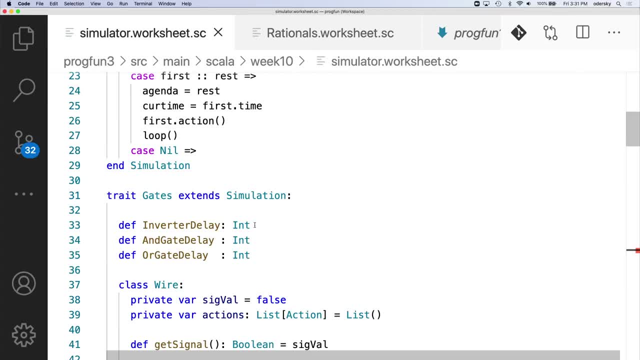 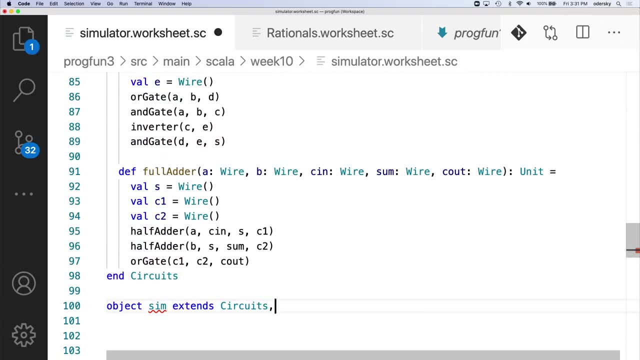 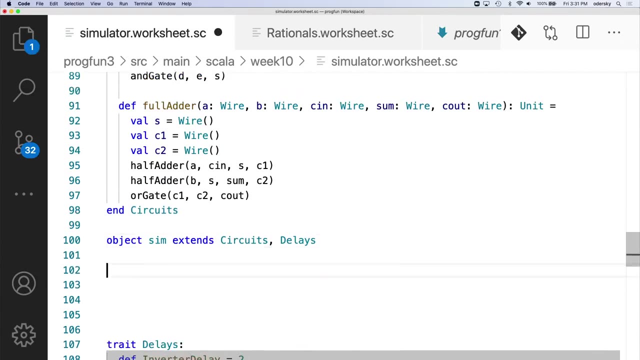 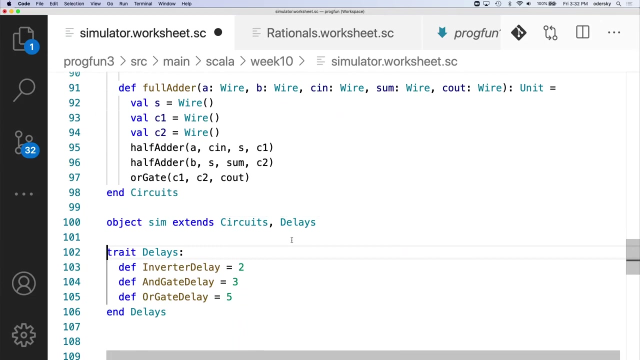 different, so we want to define them somewhere else, further towards the actual simulation class. so what we do instead is we create a separate trait for the delays which you see here. so essentially, our simulation object extends circuits and delays so it gets the circuits from one part and the delays from from another, and here are the delays that i have. 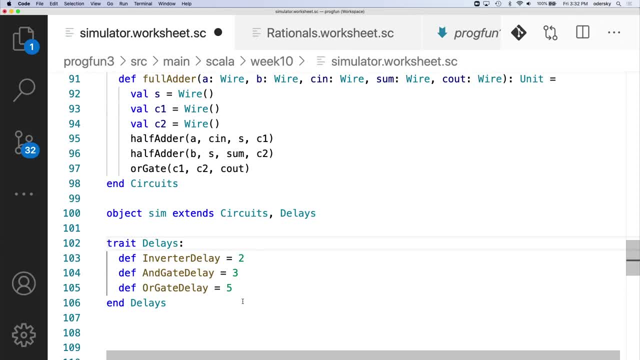 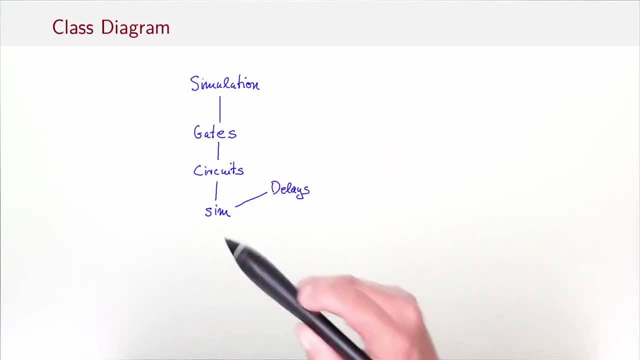 defined just to to do an example. so if i look at my class diagram again, i have the classes, simulation, gates, circuits and my concrete simulation. and the concrete simulation now also inherits from a trait that fixes the technology dependent delays. so here's a sample simulation that we're going to. 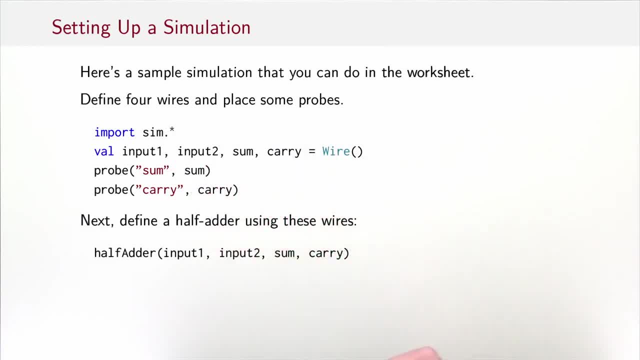 do in the worksheet. we define four wires and place some probes on each of them, and then we're going to place some probes, so two input wires, some, and a carry wire and we want to place the probes on the sum and the carry. next we want to define a half adder using these wires, so we place a half adder. 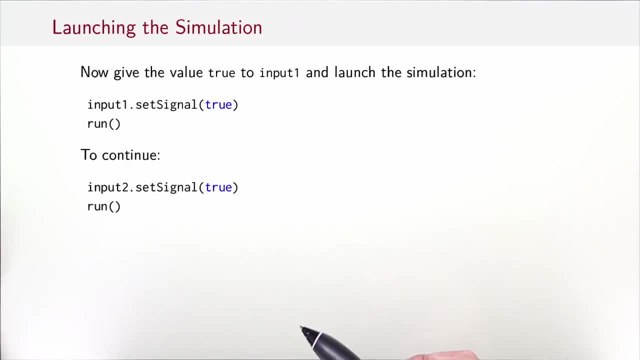 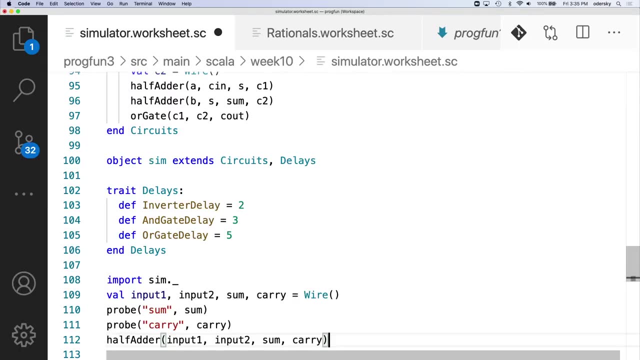 between input one, input two, sum and carry. now we want to give the value true to input one and launch the simulation. so let's set up the simulation like this: i have the wires, i have the probes and the half adder to do this. i need to transform the simulation so we could use again these probes here. 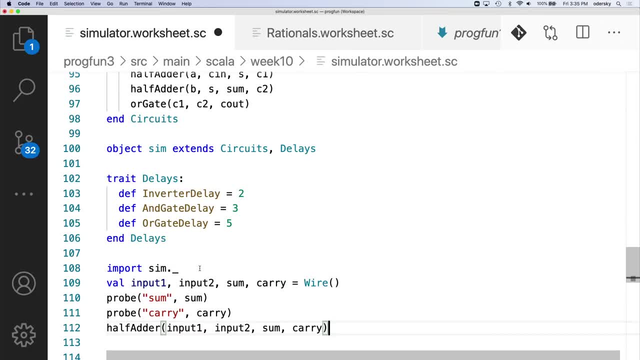 so first one, the half goes here, next we have two here, the other's down. we have improved, so let's without prefixing. I've just imported the simulation object, so that way I have access to everything that's defined in here. So we get the initial values of 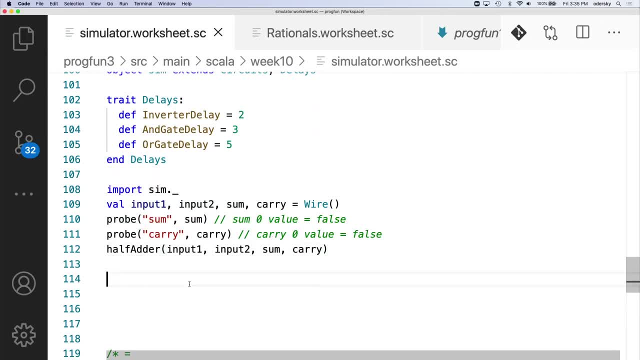 sum and carry, which are both zero. Now to do something, let's change the symbol of one of the inputs and run the simulation. So it says simulation started and not more. but if we hover over it then we will see. ok, the sum probe gave us at: 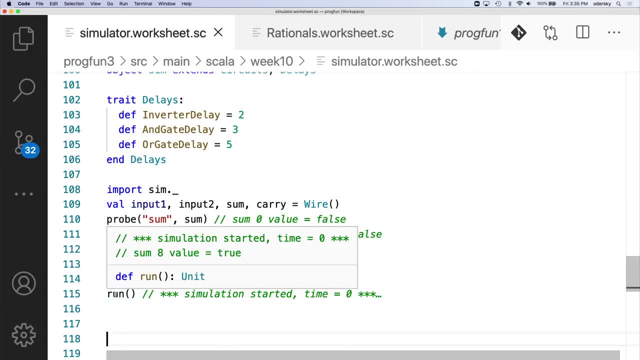 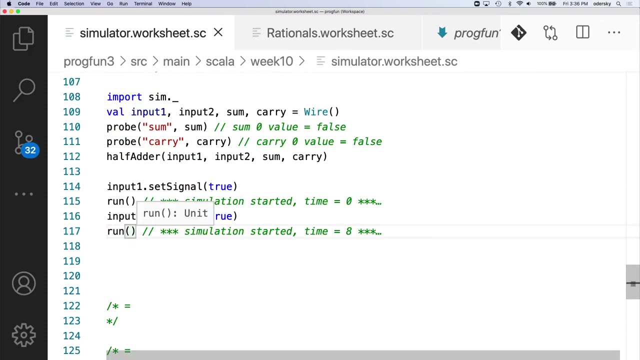 time 8. a new value: true. So after eight simulated units, the sum signal went to true. What we could do now is we could also set a signal for input 2 and run again, and what we see now is that the carry and sum signals have. 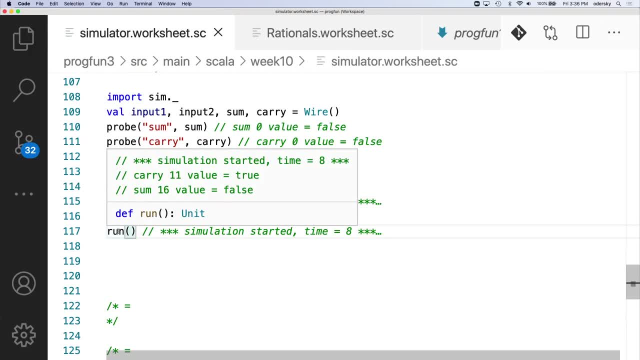 changed, so we can run the simulation. let's see if that works. we can also set the signal for the carry, and some values have changed and the carry signal at simulated time 11 became true and the sum signal at simulated time 16 became false again. so that just shows that the basic of simulations work. 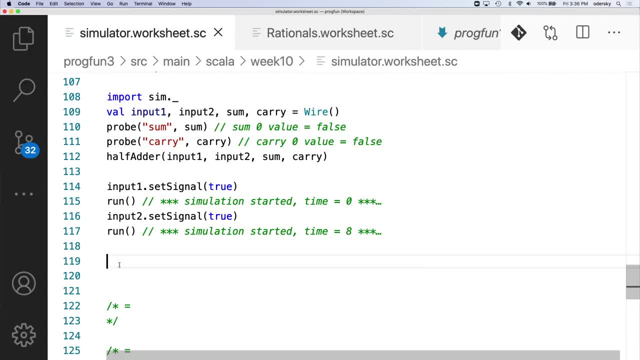 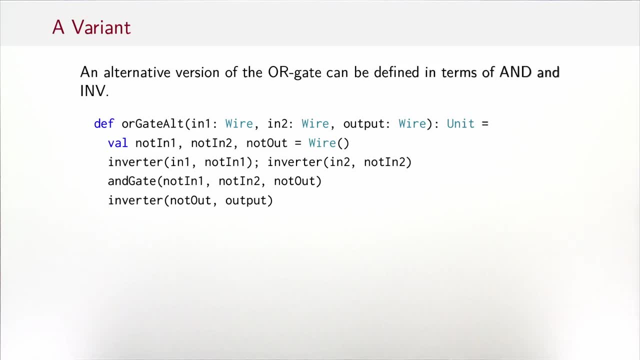 as expected, i invite you to define more circuits and have more simulation runs to play with it. so, in fact, logically speaking, we wouldn't have needed three gates since, for instance, the or gate can be defined in terms of and or inf, so an alternative for the or gate would be to define it. 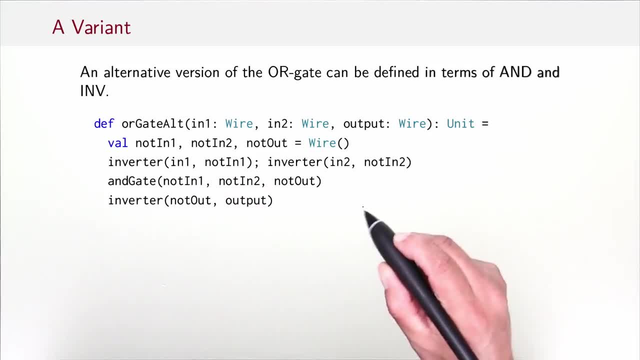 as a circuit. that would then correspond to to this circuit here, where we first put an inverter here and an inverter there, and then we have an and gate of the negated symbols and then we put a final inverter on the result wire. that's of course, just a consequence of the formula that a or b is the same as. 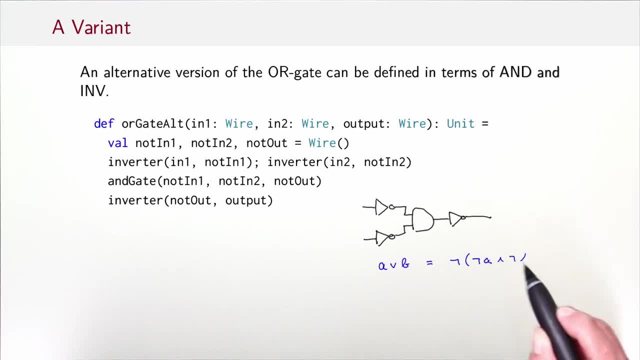 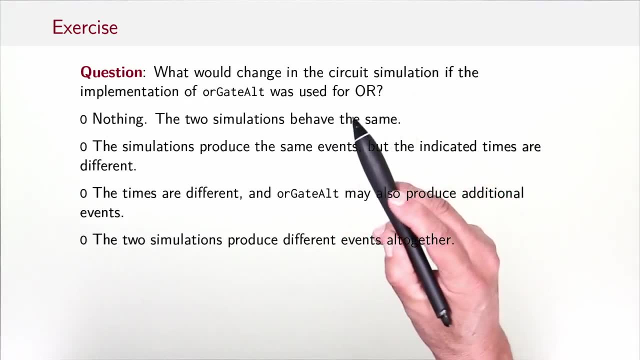 not, not a and not b. so that's the circuit that we have drawn here. so question to you: what would change in the circuit simulation if the implementation of or gate out that you have just seen was used for, or would it be nothing? the two simulations behave the same, or would the simulations? 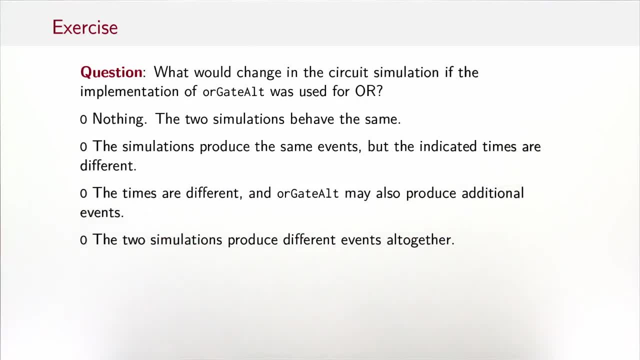 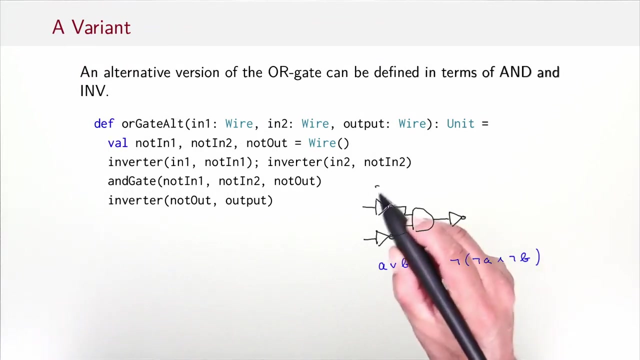 produce the same events but the indicated times are different, or would the times be different and or gate alt might also produce additional events? or would the two simulations produce different events all together? what do you think so clearly the timings would be different in general. if you take our current example values, then an inverter delay would be two and an end gate delay. 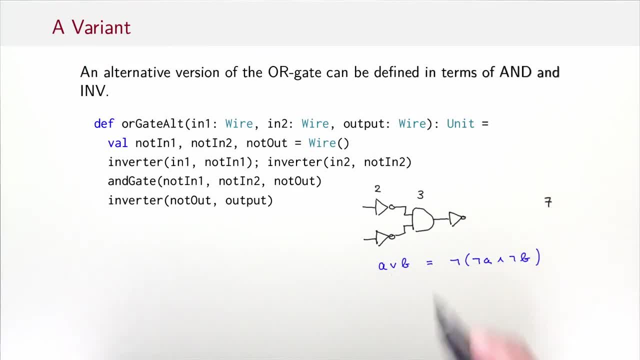 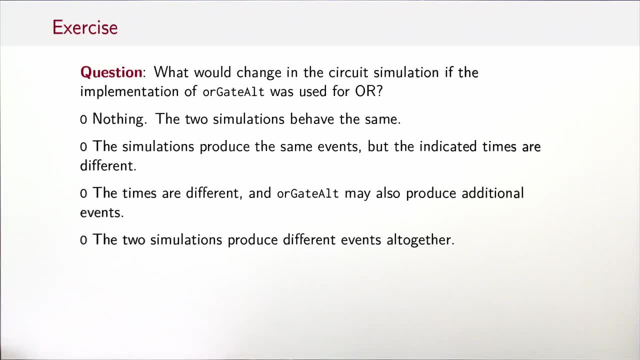 would be three. so you get would get a total delay of seven, whereas an or gate delay in our example values had a delay of five. so that would give you different times and you might think that's it. so it would be number two. but if you have actually tried this, 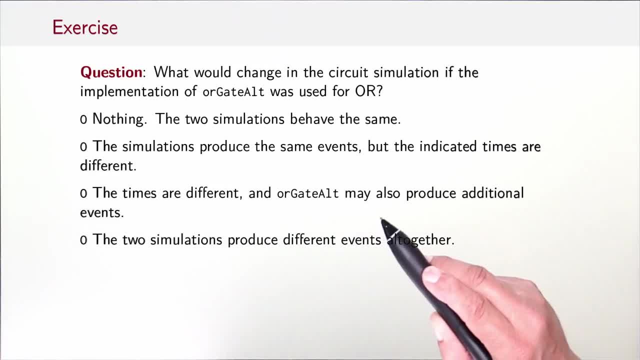 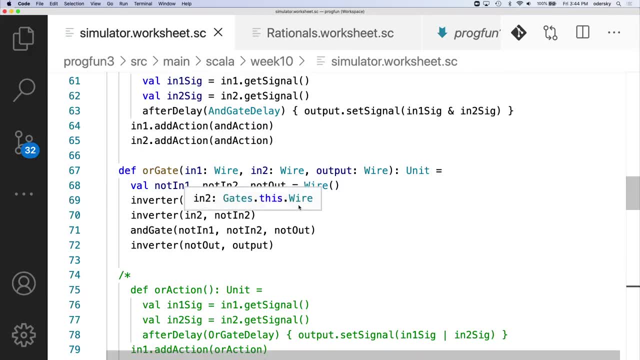 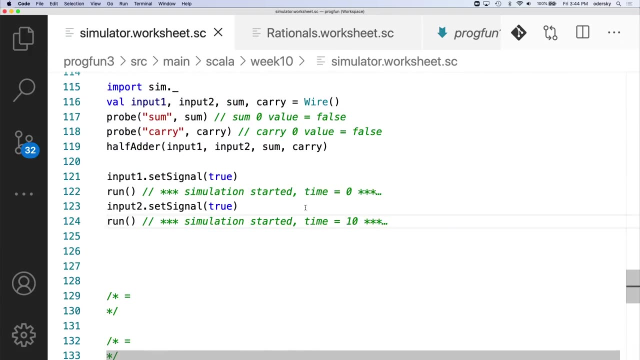 in the worksheet. then you will actually see something else. the times are different and or gate out might also produce additional events. so, to demonstrate, i have plugged in the new version of the or gate in the worksheet and now we have the uh run here. uh, where we get for the first run. uh, at at time number five, the value is true. 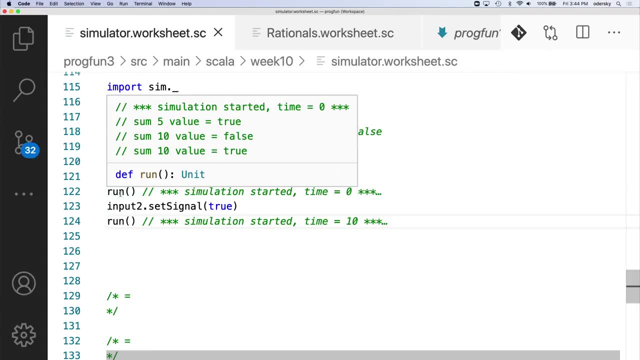 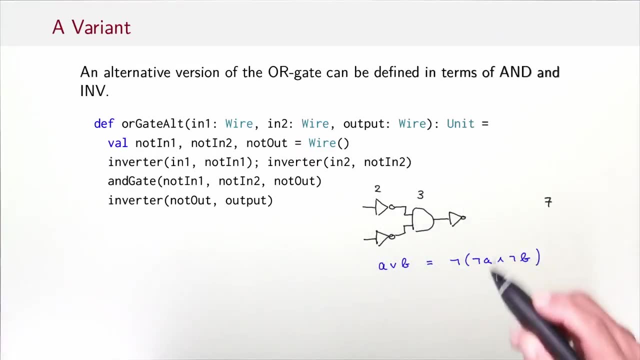 and then at ten. uh, the value is first false and then true again. so that looks at first really mysterious. to explain the mystery, let's have another look at this diagram again. so what we have here is essentially not a single event, as in the or gate, where essentially we have a single 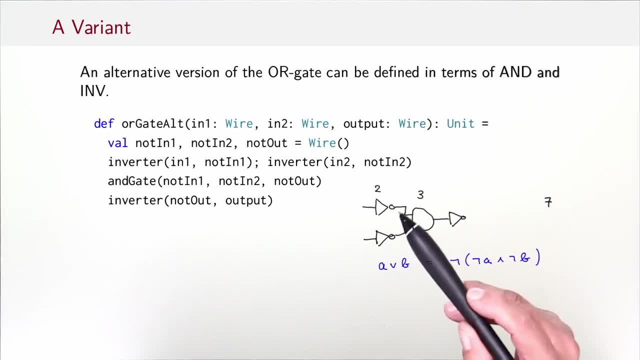 action to be produced used, but we have multiple actions. we have the two invert actions and the and action and then the final invert actions. so we get many more actions in our agenda that also will be executed, sometimes at the same time and when you have several items in the agenda that are executed. 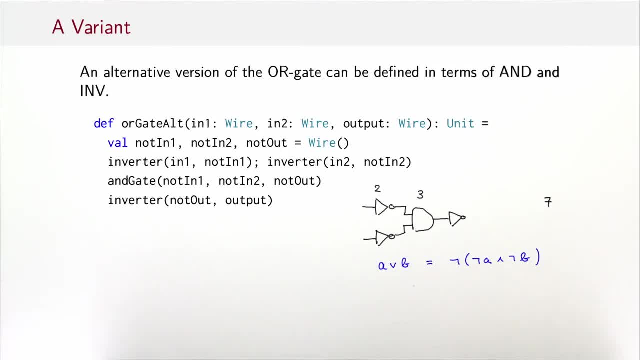 at the same time, you can essentially get interleavings. you can have some things that happen at some moment before something else happened, and that was essentially here what we observed: that at time 10 you got one item in the agenda that just decided that the signal should be false and at the same time you got another item that put the signal back to true. 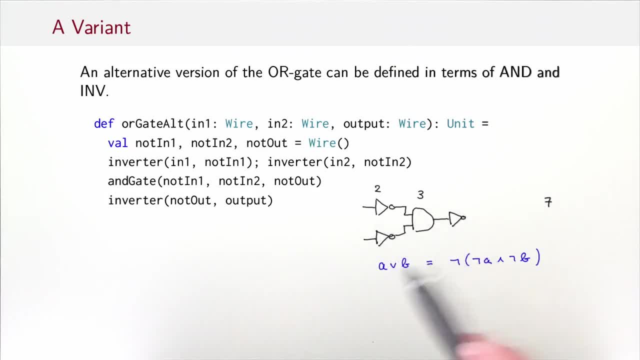 so, essentially, it's the fact that you have, instead of a single item in the agenda, you have multiple items, which are not executed atomically as a whole. they get interspersed with each other and that causes this fluttering behavior where you see events that you didn't see before. so, to summarize, state and assignments make our mental model. 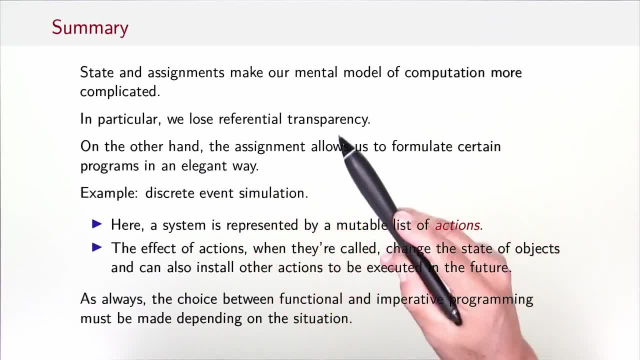 of computation more complicated, in particular because we lose referential transparency. on the other hand, assignments allow us to formulate certain programs in an elegant way. an example that we saw was discrete event simulation. here, a system is represented by a mutable list of actions, and the effect of actions when they're called are to change. 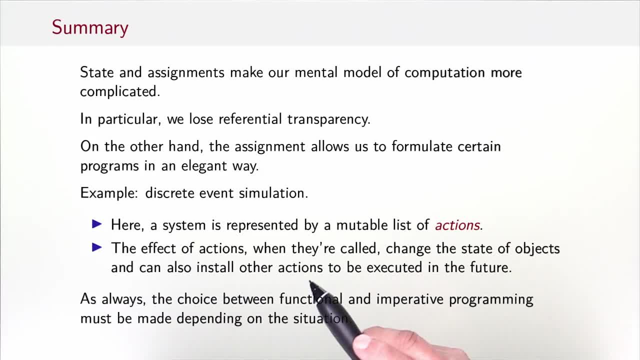 the state of objects and also to install other actions to be executed in the future. as always, the choice between functional and imperative programming must be made depending on the situation. the digital circuit simulation was a good example for a mixture of functional and imperative programming, for essentially two reasons. one reason is that the non-hierarchical 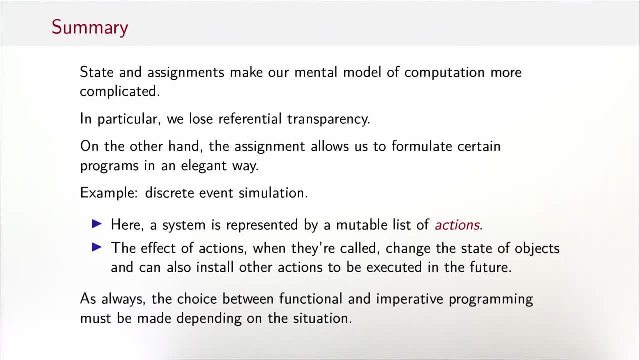 nature of circuit networks lends itself well to an imperative programming for the forecasting of results. the right network is able to support the functional and imperative programming and therefore the Definition of the Robot circuit could be a pretty good example for future execution and production by大destry. that's exactly why we were able to continue with this. 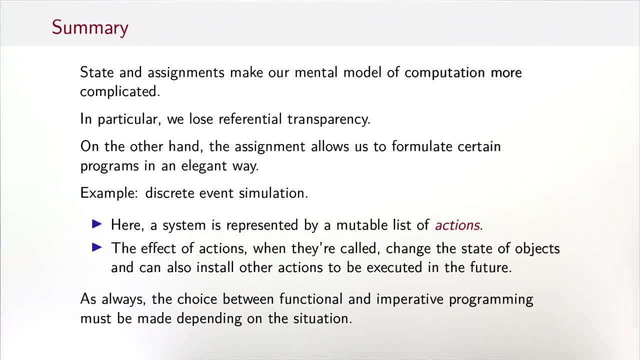 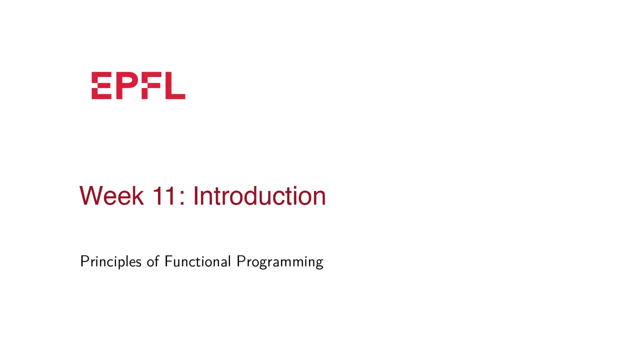 imperative formulation where we essentially place gates and circuits between wires. The other reason is that we simulated a real world system where things change, with a system where the internal state also changes, so this is quite natural. In this final week of the course we cover functional reactive programming. 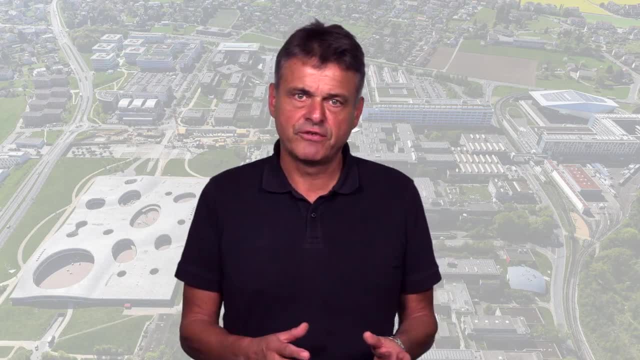 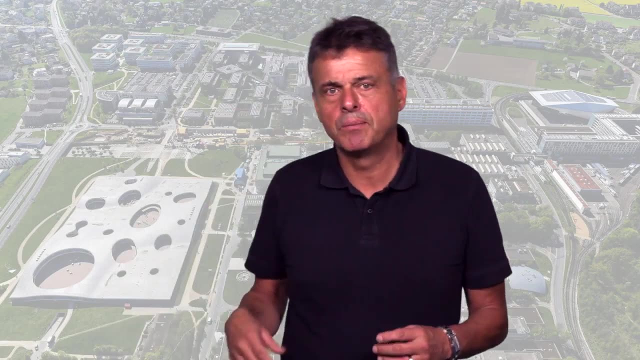 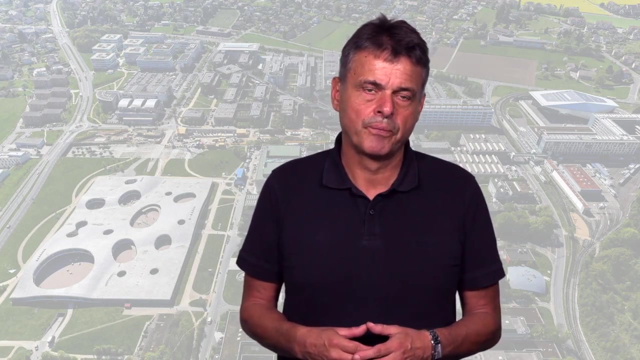 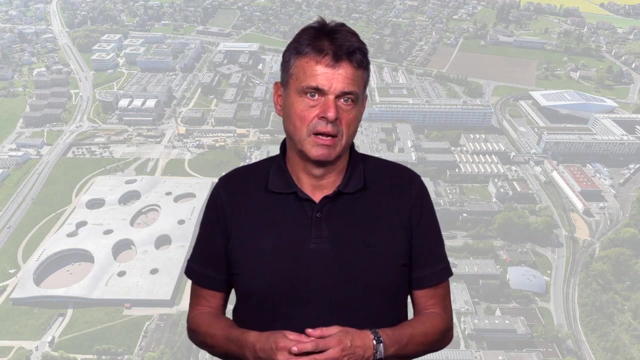 You'll find out how functional reactive programming shifts the focus from singular events to time-varying signals. This lets us express in a purely functional way event-based programs that are traditionally expressed with imperative state changes. To be sure, our implementation of functional reactive programming also uses internal state. 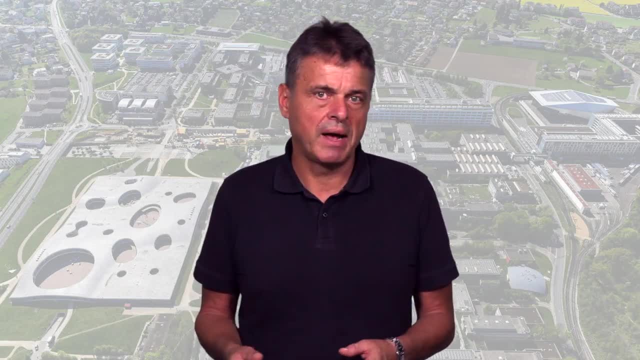 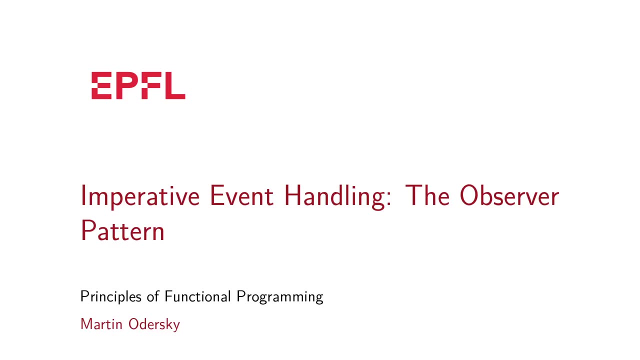 But that state is not always functional. It is now encapsulated so it does not impair the reasoning one can do about the functional surface language. In this session we are reviewing the observer pattern, which is the standard, imperative way to do event handling. 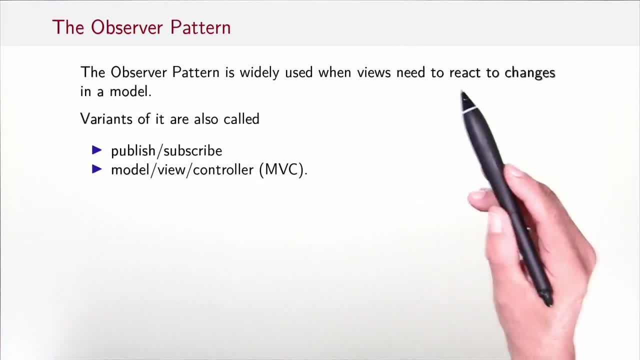 The observer pattern is widely used when views need to react to changes in a model. Variants of it are also called publicist patterns. The observer pattern is the model view controller. So here we have a model which is some stateful object or set of objects. 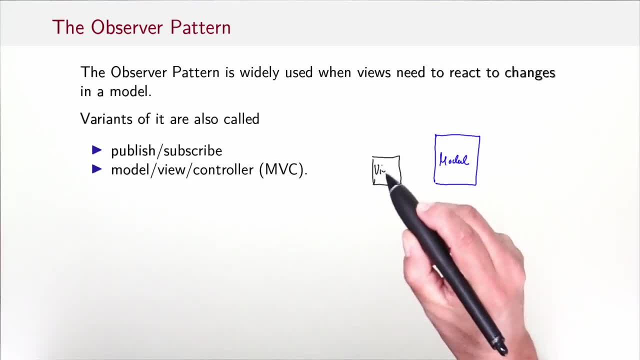 And then we have views that show some aspect of the model, And the model typically doesn't know how views are implemented or how many there are, And the views can also change dynamically in number. So the task then is: whenever the model gets updated, all the views have to be. 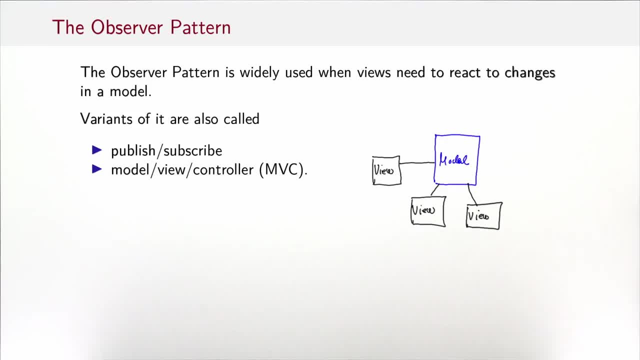 notified so that they can update themselves as well. So a typical scheme to do this is to declare the model to be a publisher and the views would be subscribers. So a subscriber contacts the publisher to say I want to be notified of any updates. 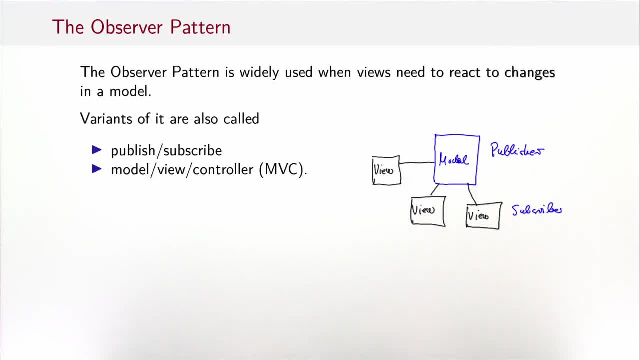 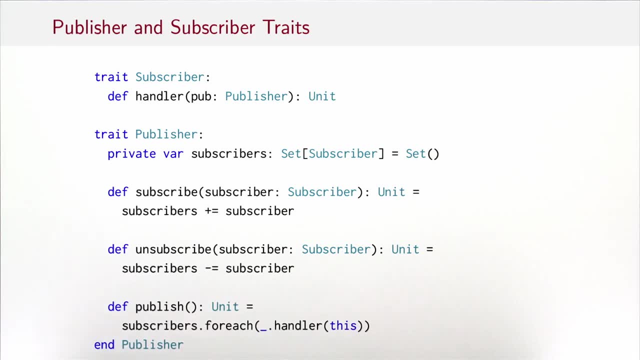 And when there are updates, a publisher will essentially notify all the subscribers of these updates. So here's an implementation of this principle. in Scala, We have two traits: subscriber and publisher. So subscriber is the base traits of all views, And they offer a handler method that will be called by the publisher whenever there's. 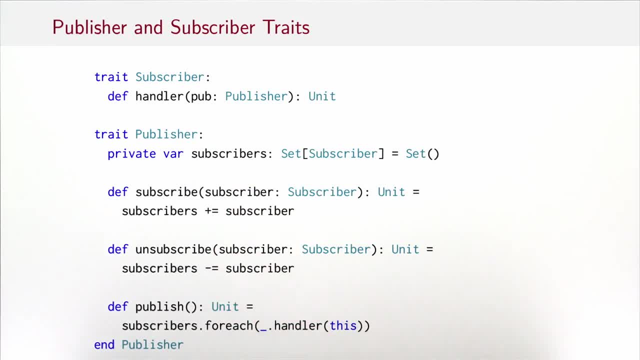 a state change in the publisher. And then the trade publisher maintains a set of subscribers. here in this private variable, A subscribe method would add a subscriber to the set. An unsubscribe method called from a subscriber would remove the subscriber from the set. And finally, the publish method would go through all subscribers and for each subscriber. 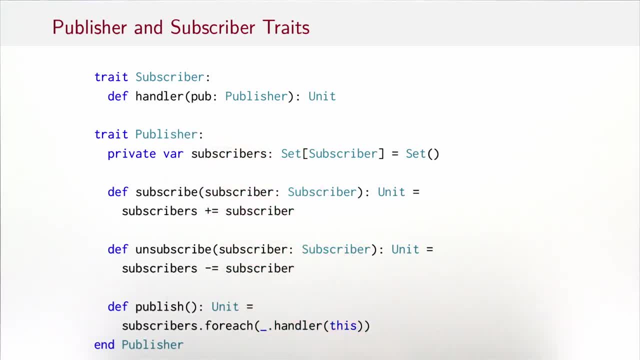 call the handler method that the subscriber has defined here And the publisher passes itself along as the publisher here. So that means the subscriber could actually subscribe to several publishers And when handler is called it would know what publisher pushed the change from this parameter here. 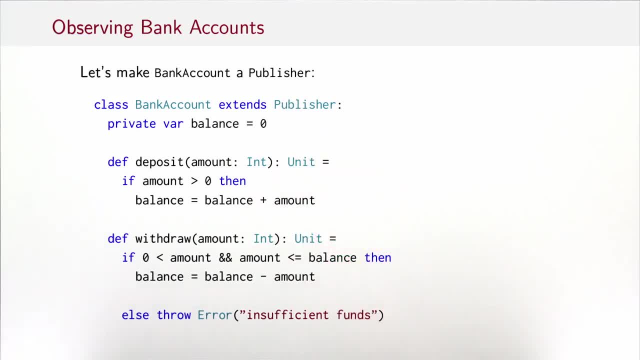 Okay, so once we have that, we can make bank account a publisher. That means that one can subscribe to a bank account To be notified of any changes in that account. So bank account now extends publisher, And what else do we have to do? 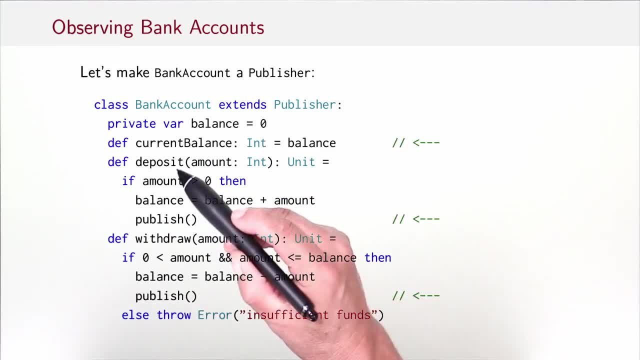 Well, essentially three things. First, is any state change in deposit or withdraw has to call the publish method Here and here, So that way all subscribers are notified. Second, when a subscriber is notified, they would like to find out what the current balance. 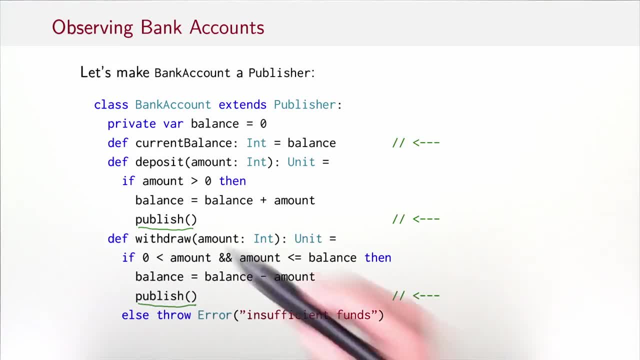 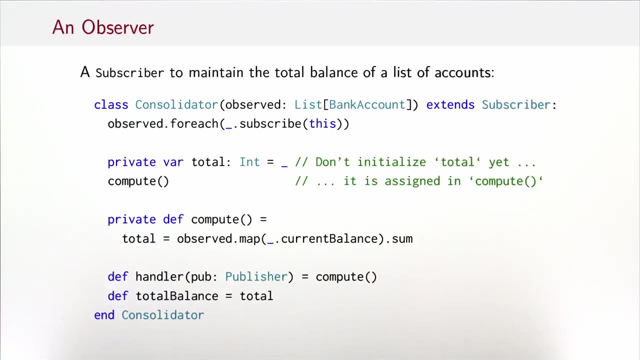 on the account is now Because it typically wasn't them to have done a deposit or withdraw method, So they don't know. So we will add another method: current balance- that just returns the current balance without depositing or withdrawing anything. That's all the changes that we needed to do. 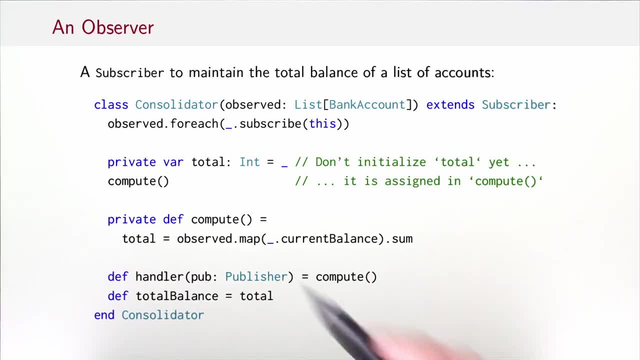 So let's use this model to define a subscriber. One example of a subscriber I call here a consolidator. Let's say you have a list of bank accounts and we want to know at each point the balance overall of these accounts. So whenever one of these bank accounts changes, then the consolidator should be notified about. 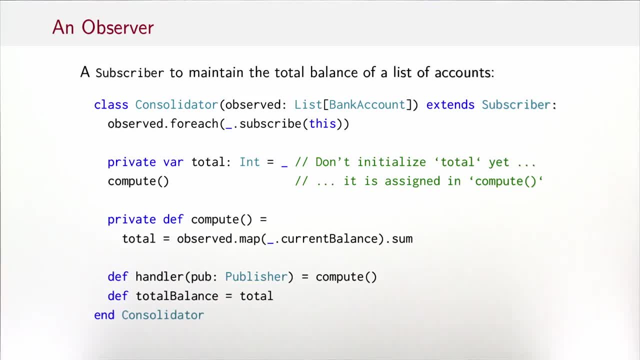 the change and it should recompute the total balance. So a consolidator is a subscriber And as part of its initialization it will subscribe to each of the bank accounts in Observe. So for each of the bank accounts it will add itself as a subscriber. 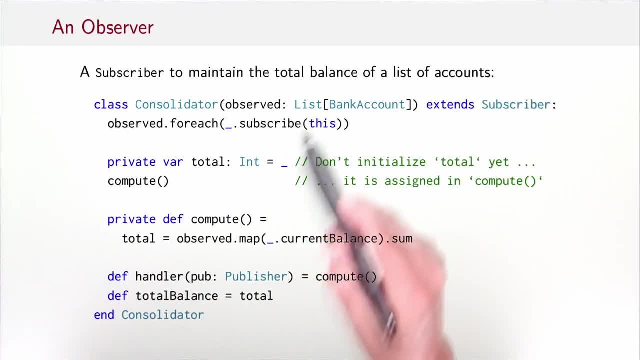 Then we have the variable total, which reflects the total balance in all the accounts. That variable is initialized by the call to compute that follows immediately. Here's the definition of compute: It sets total to the sum of the current balances of all accounts in Observed. 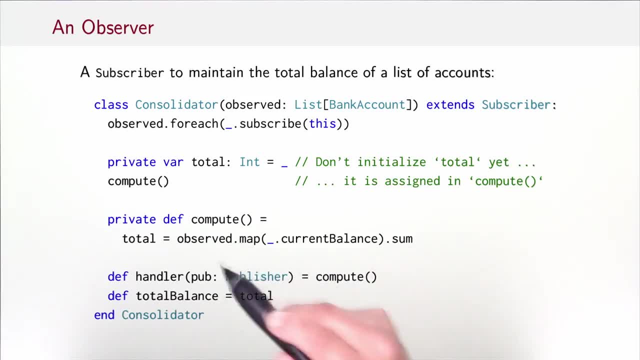 Observed map: current balance sum. So compute is called once when we start the consolidator, but it will also be called each time one of the accounts changes. That's done by calling compute from handler. So if one of the accounts changes, it will publish the change by calling handler and. 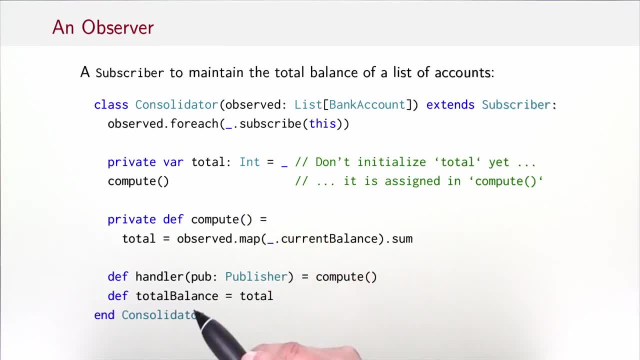 that will recompute the total balance. And finally, the total balance method here is simply a public interface to this private variable total. So there's one little syntax twist here. It's this: equals underscore. What does that mean? Well, if I would leave out equals underscore, like this, then what I would get is not an 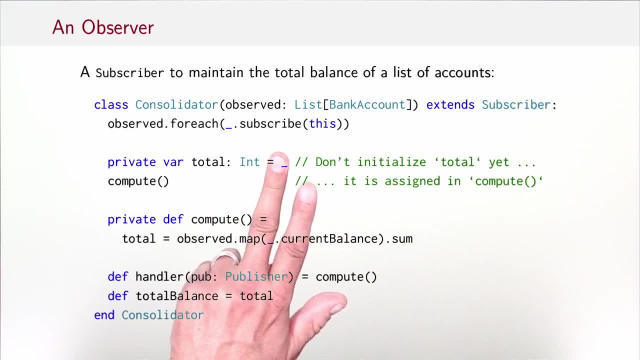 uninitialized variable. It's an abstract variable. That's basically a variable that only has a way to get the variable and to store the variable, but it's not backed by a field. The field, the variable, would have to be implemented in a subclass. 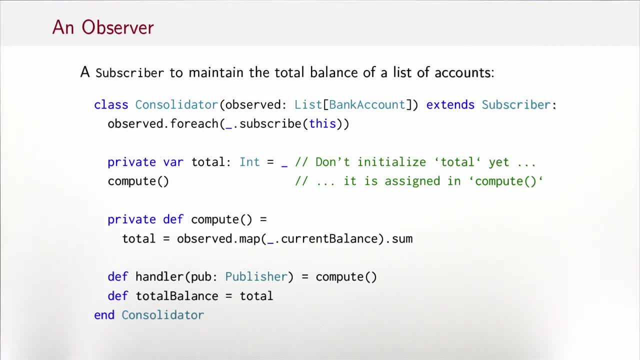 So to have a variable where I just say: well, I choose to not initialize the variable here because it will be initialized later, I write equals underscore. That means don't initialize total yet. So that concludes our example. Let's review what we have seen. 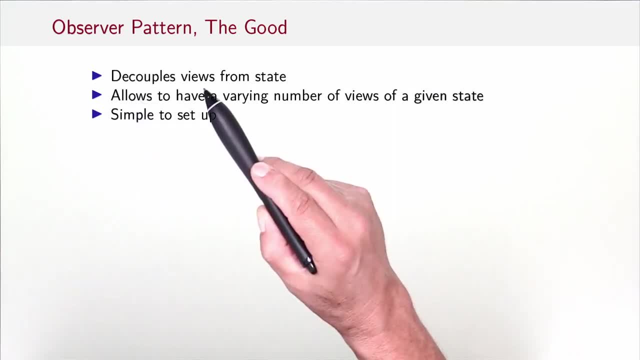 The good thing about the observer pattern is that it manages to decouple views from state. The views are quite different from the state in the model. It allows us to have a varying numbers of views of a given state And it was actually quite simple to set up. 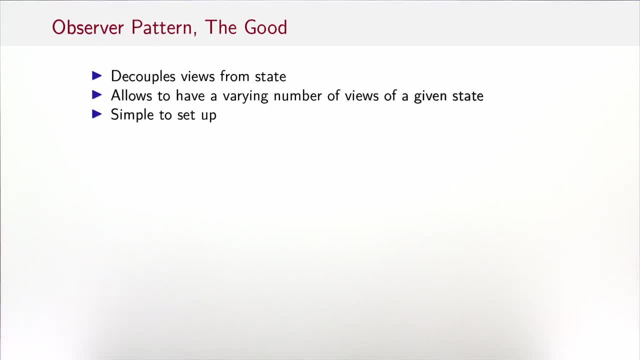 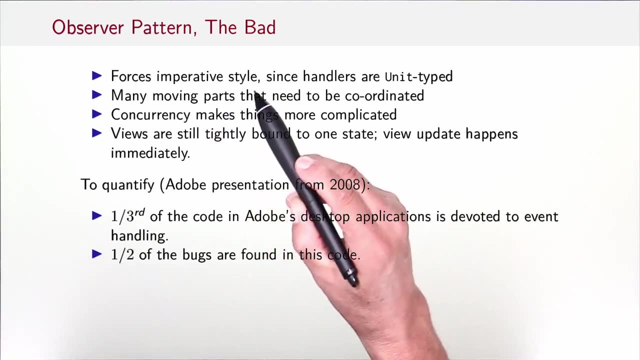 It's fairly easy to turn the thing like a bank account or another stateful object into a publisher. The downsides of this pattern are, first, that it forces an imperative style, since handlers are unit type. So a handler never returns anything. It can't because it's called from the publisher. 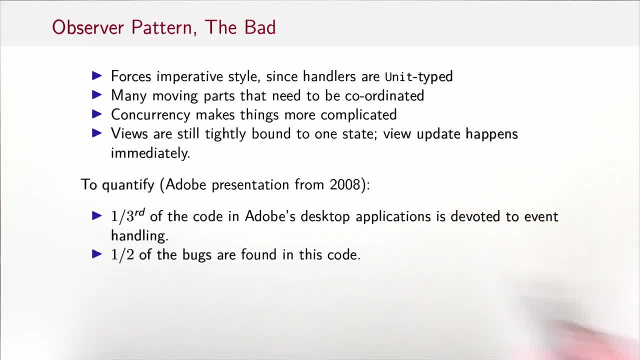 So everything a handler does, it has to do with a side effect. There are quite a lot of moving parts that need to be coordinated. In particular, subscribers are fairly complex classes. A third downside is that the observer pattern as we've seen it here really works well only 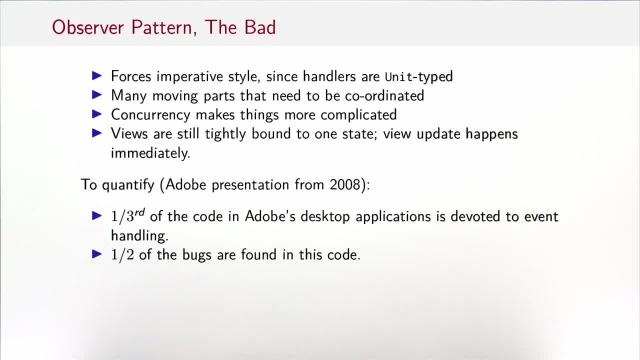 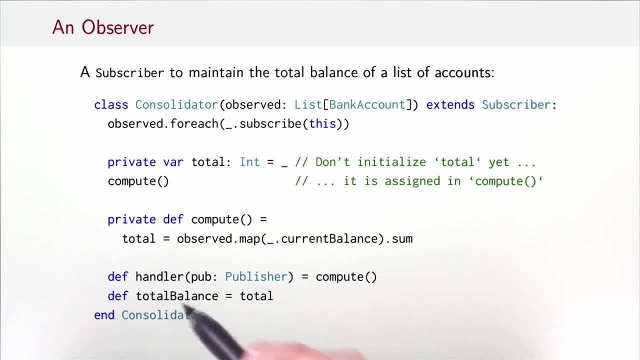 in a single threaded model. Once we add concurrent execution, things get a lot more complicated. If I look back at the consolidator, what could happen in a concurrent execution? What could happen in a concurrent execution is that several handlers will be called in. 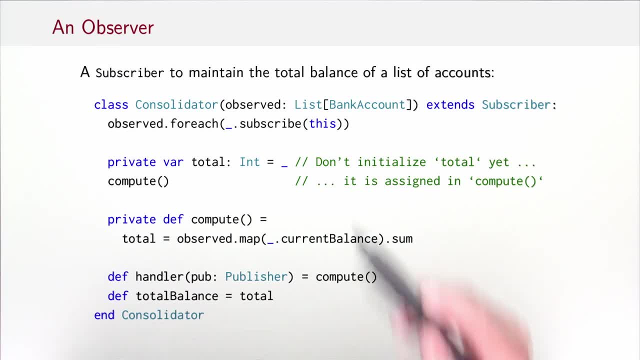 parallel at the same time maybe, And that means the consolidator has to protect itself from race conditions. Of course that can be done. We can make it a monitor with synchronized and so on, But it's additional steps that we have to do and those steps have additional downsides. 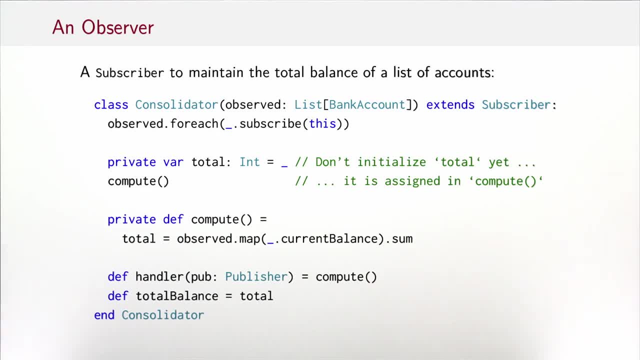 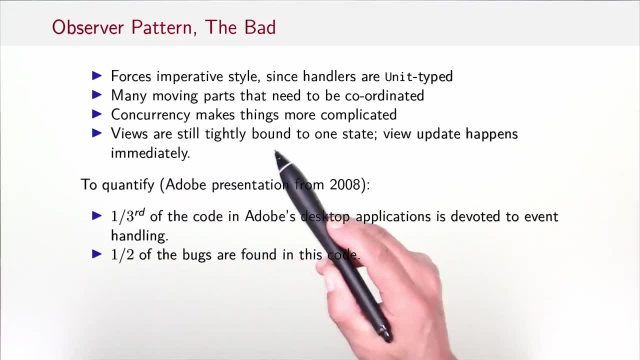 like they might produce deadlocks or other unwanted effects in concurrency. So observers in a concurrent scenario, And the fourth downside might be that views are still tightly bound to one state, to one model where the view update happens immediately. So these issues are actually quite relevant because the observer pattern is not a little. 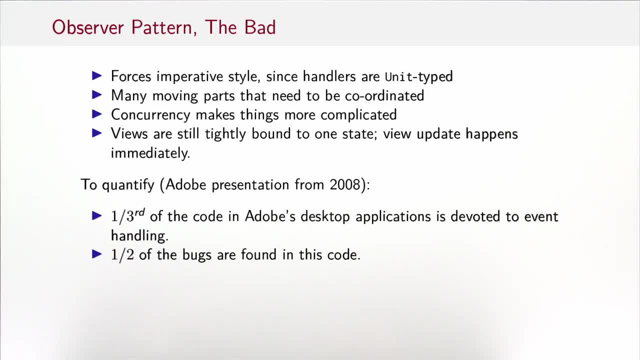 niche thing. For instance, if we look at Adobe, which is the producer of Photoshop, with which this recording was made, and also of PDF, then we learn that one third of the code in the desktop applications Is devoted to event handling. So one third of all code, of a pretty humongous code base. 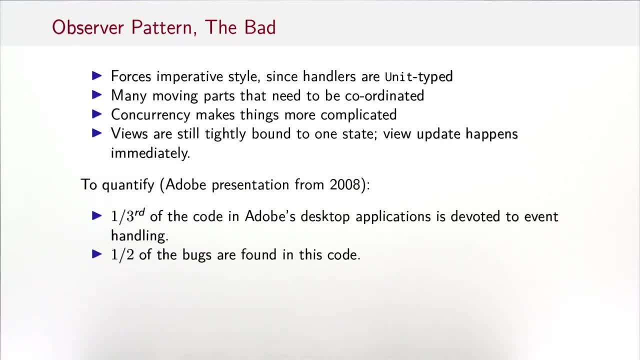 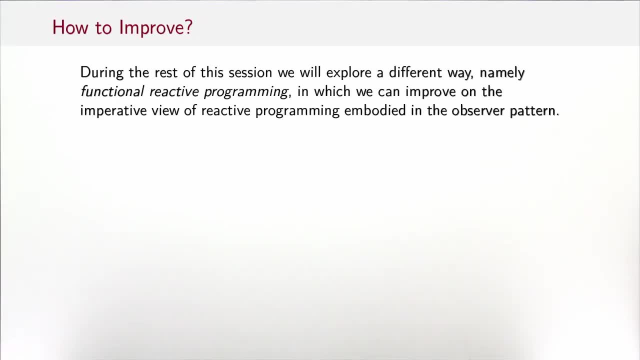 And, furthermore, one half of the bugs are found in this code. So not only is it a lot of code, but it's code that tends to be more difficult and more buggy than the rest. So can we do better? The answer is yes, maybe. 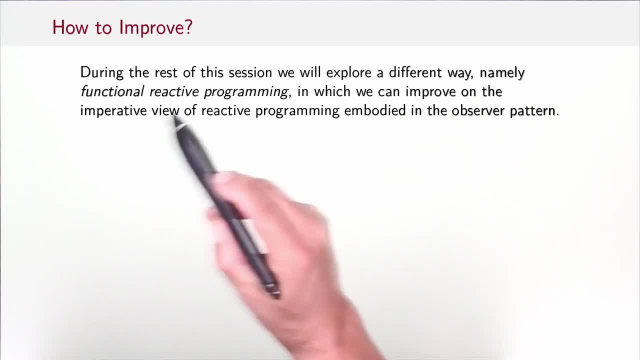 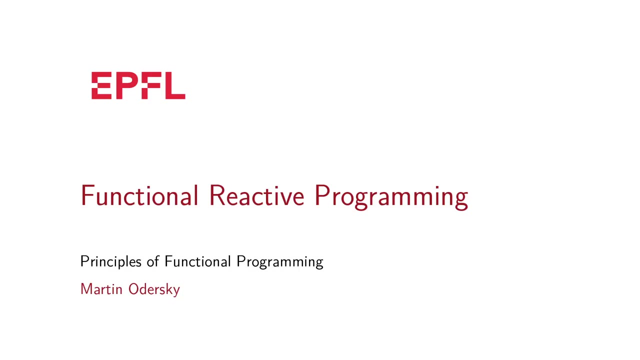 In the next sessions we'll explore a different way, namely functional reactive programming, And that can improve on the imperative view of reactive programming that's embodied in the observer pattern. In this session you'll learn about a functional way to do event handling, called functional. 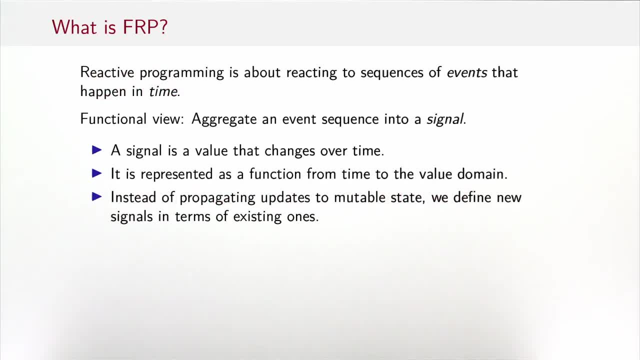 reactive programming. So what is functional reactive programming, or FRP, to which it is often abbreviated? Well, if you just talk about reactive programming, it's about reacting to sequences of events that happen in time, And the functional view of this is, in a nutshell, to aggregate an event sequence into a signal. 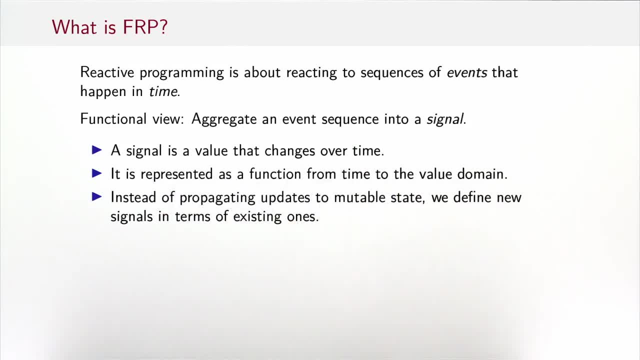 So a signal is a value that changes over time. But we're no longer looking at the individual events as they fire, we're looking at the signal as a whole. So an abstract view of a signal is to say it's a function from time to the value domain. 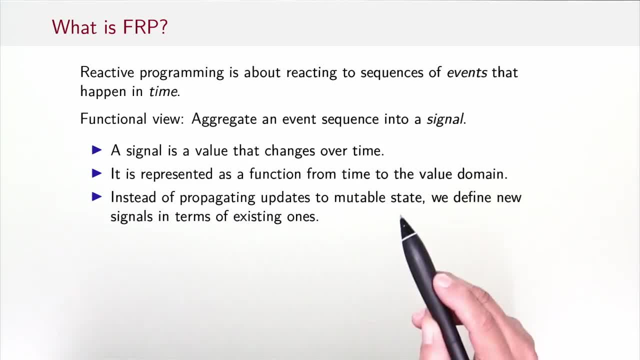 And once we have that, We can replace Propagating updates to mutable state by defining new signals in terms of existing ones. So instead of having the individual events and their updates, we see the signals as a whole. So so let's make this concrete with an example. 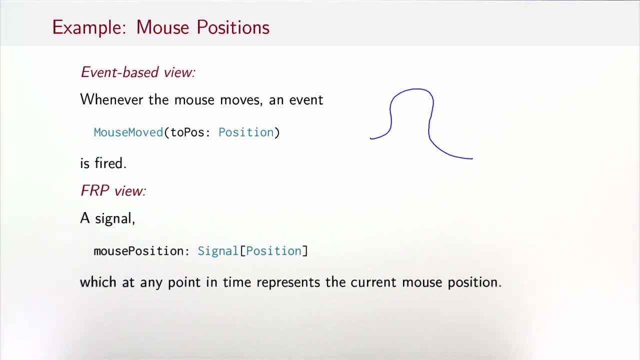 Let's say you have a mouse that moves around the surface, The event based imperative view would be that whenever the mouse moves, you get an event that says mouse moved. and the new position where it is now, By contrast, the FRP view of that- would be to say: well, we represent this curve as 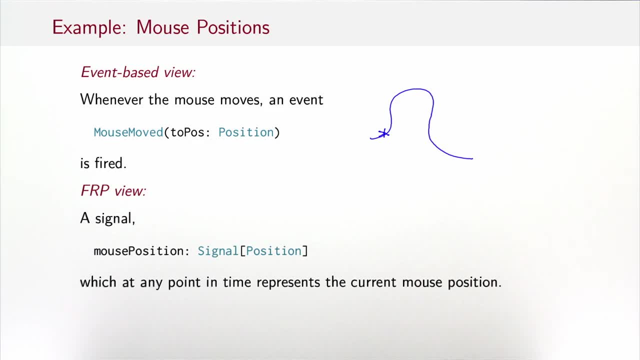 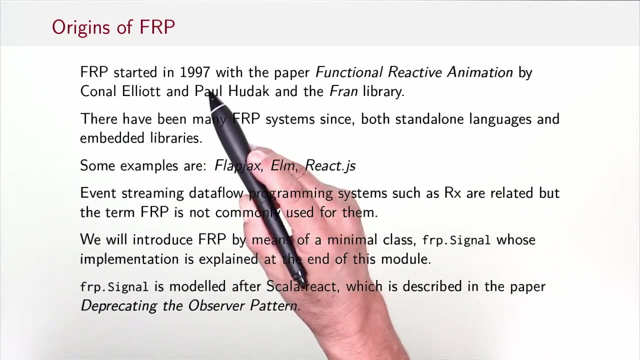 a signal from time to the current mouse position. So it's a function from time to points in a two dimensional space that you see here. So how was this change in viewpoint invented? Well, FRP really started in 1997 with the paper Functional Reactive Animation by Conal. 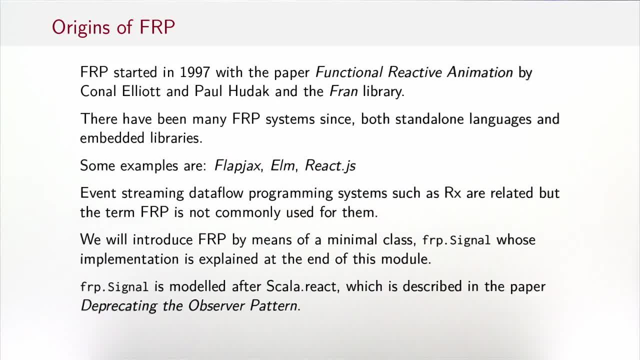 Elliott and Paul Hudak, And they also published a library to go with it, which was called FRAN. That was very influential. There have been many FRP systems since, both standalone languages and embedded libraries. Some popular examples today are Flapjacks, Elm, ReactJS or also React Native. 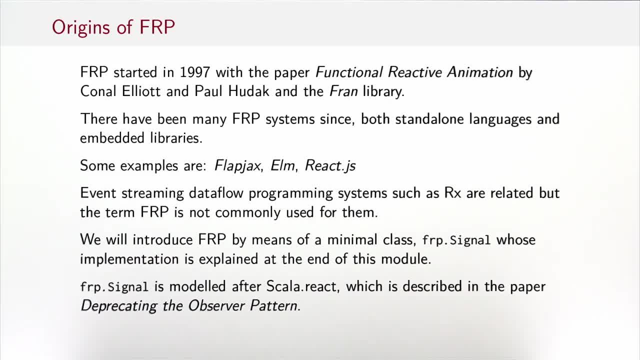 So a lot of the event propagation on JavaScript frameworks is now done in a functional reactive way, using ReactJS, for instance. There's another branch of reactive programming, Which is essentially data flow programming systems based on event streaming. An example is RX. Those are related, but the term FRP is not commonly used for them. 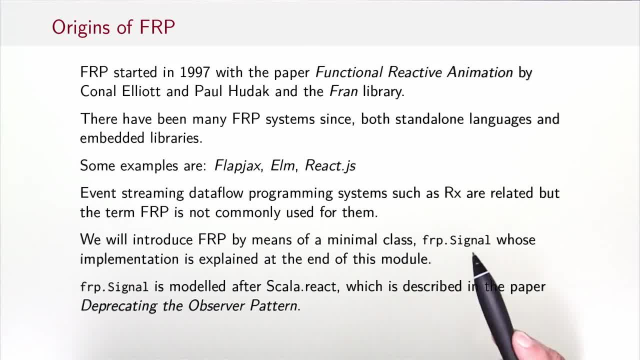 We use FRP by means of a minimal class which we define ourselves and whose implementation is explained at the end of this module. This implementation is modeled after a system called Scala React, which is described in the paper, deprecating the observer pattern. 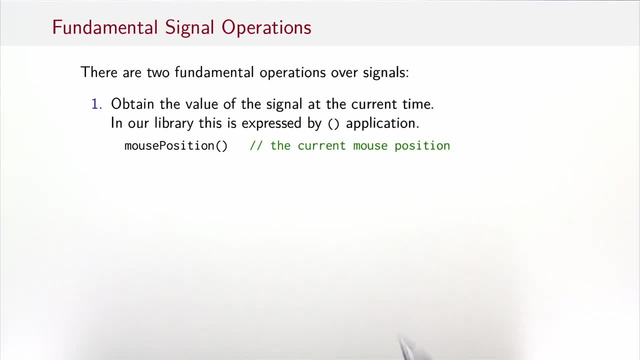 So what can we do with a signal? There are two fundamental operations. The first operation is to obtain the value of the signal at the current time. So if signals are functions, then obtaining the value of a signal at a current time is function application. 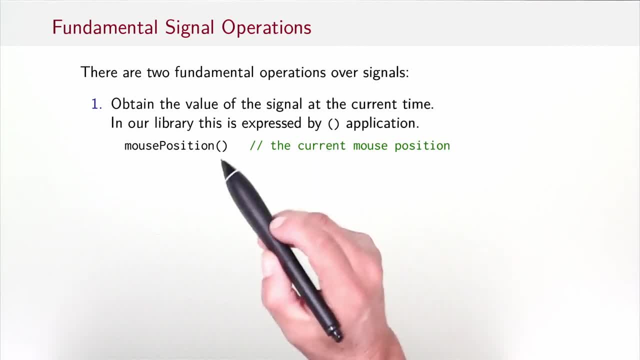 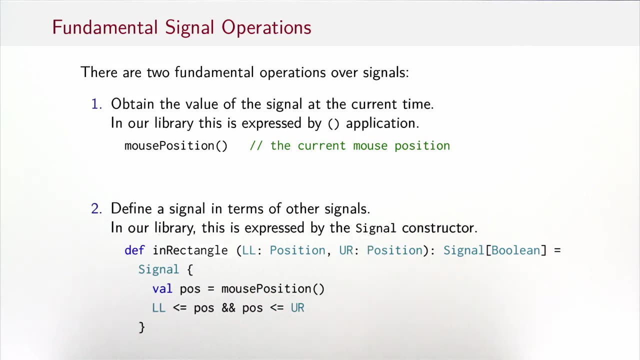 In our library. this is consequently expressed by just writing function application like this. So the current time is implicit. So mouse position: open parents, close parents would say the mouse position at the current time. The second fundamental operation is to define a signal in terms of other signals. 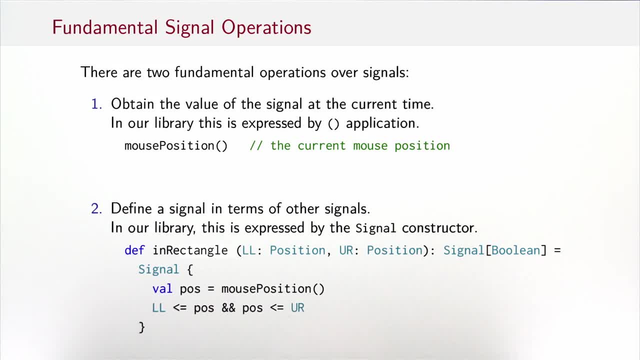 In our library this is expressed with the signal constructor. So, for instance, we could define a signal in rectangle that says: is a position in the rectangle given by the lower left and upper right corners. That's a signal that gets the mouse position: the mouse position at this point in time. 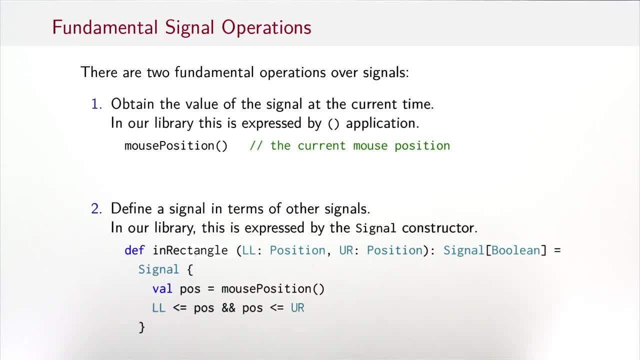 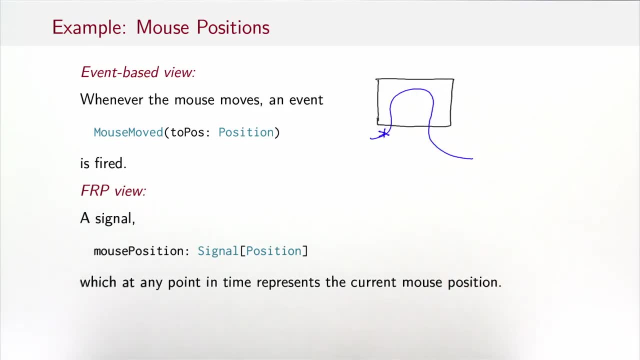 And it then asked whether the position is between LL and UR. So that can be visualized like this: So now you have from this original signal, you have the bounding box between LL and UR And your new signal would be a function in time that goes essentially like this: 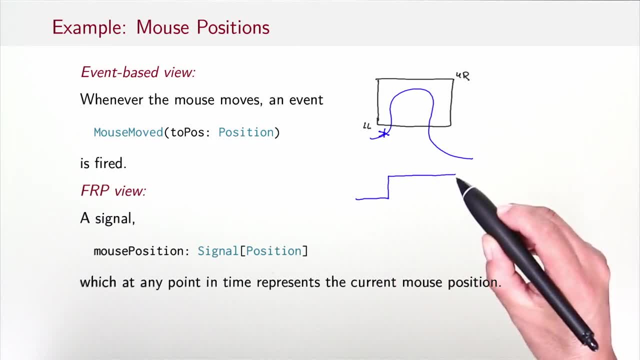 First it's not in the bounding box, it's false, Then it's true, And then, after some time, it's again false. So this would be true, This would be false. So you see, we can transform one signal into another using the signal constructor. 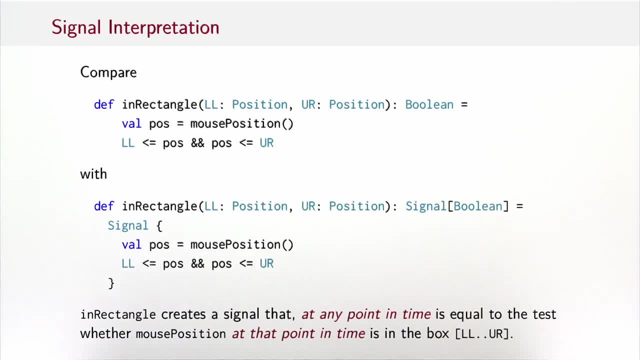 It's worthwhile taking a step back and see what we've done here. Here's the in rectangle function that we would define normally without functional reactive programming. So it's just the body of the signal here and it returns a boolean. Now that means that every time we call in rectangle, it will tell us whether the current 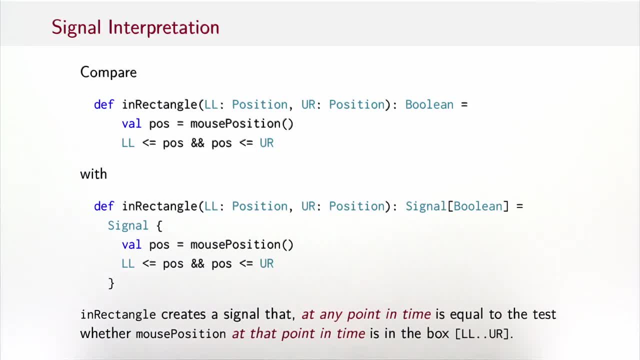 mouse position is between LL and UR. Contrast that with a new definition of is in rectangle. that returns a signal of boolean, So in rectangular, creates a signal that at any point of time is equal to the test, whether mouse position at that point in time is in the box LL or UR. 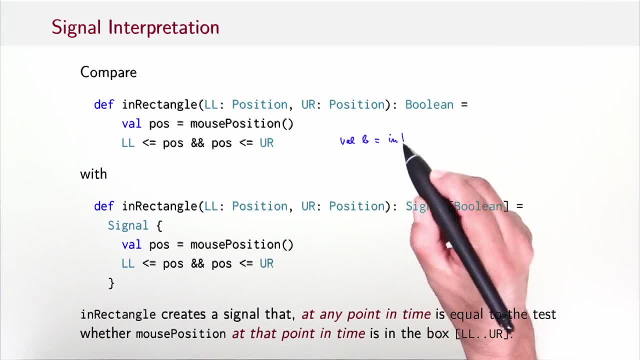 So that means if we write, let's say, val b equals in rectangle some corners L and R, that will give us a boolean result that reflects whether, at the time when we evaluated this call, mouse position was between L and R, and the result will stay the same forever. 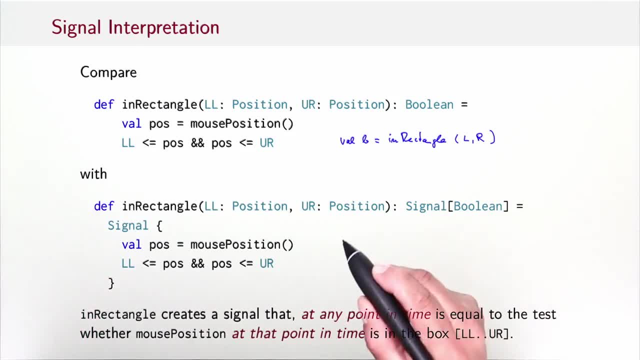 afterwards, Whereas for the signal version, we, if we set it up like this, well, signal equals in rectangle L, R, so that would give us a signal which we can query its arbitrary times in the future, and each time we query the signal it might give us a different result, depending on the mouse position at the 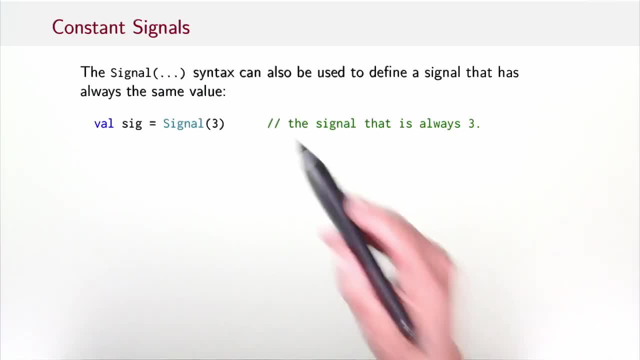 time when we query the signal. The signal syntax can also be used to define a signal that has always the same value, so that's a constant signal. For instance, val sig equals signal 3, is a signal that is always 3.. So the idea of functional 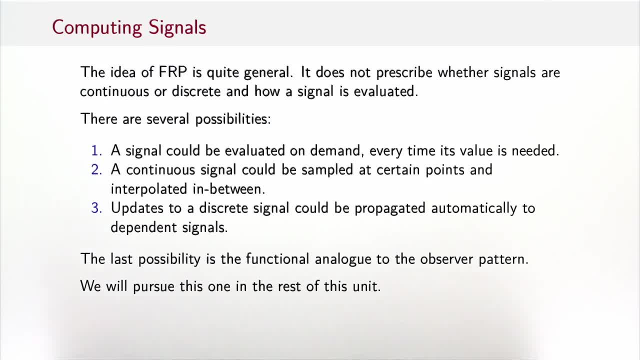 reactive programming to see signals as essentially time-varying functions is quite general. It doesn't prescribe whether signals are continuous or discrete, and also it doesn't prescribe how a signal is evaluated. We could think of several possibilities to evaluate a signal. One way would be to evaluate it on demand to. 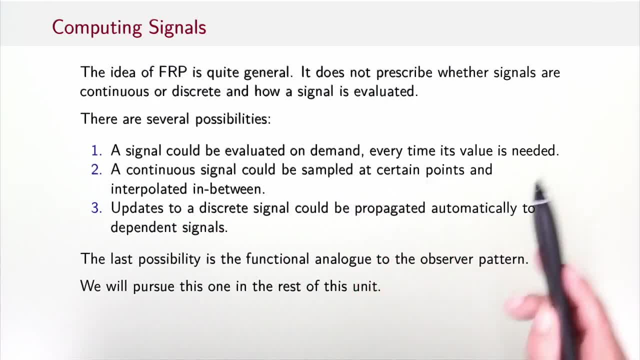 store the signal as essentially a formula, and every time its value is needed, we evaluate it. Another idea is to sample a signal that's continuous at a fixed or varying time interval at certain points and to interpolate in between. Or if the signal is discrete, we could also update it internally and 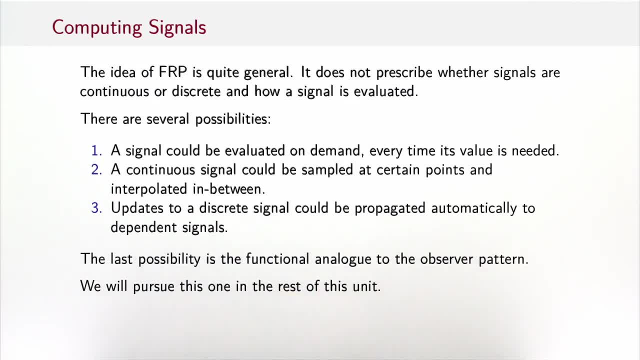 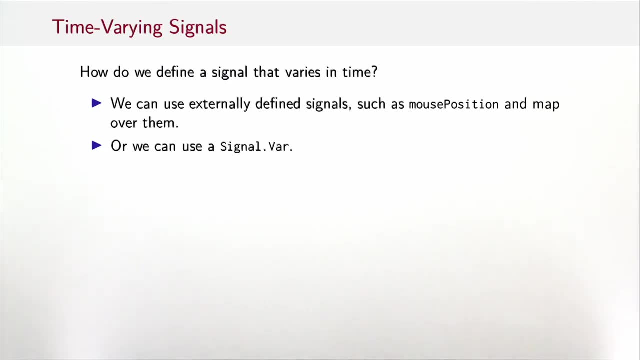 propagate the updated signal in the same way. That last possibility is, in a sense, the functional analog to the observer pattern, and that's what we will pursue in the rest of this session. How do we define a signal that varies in time? The possibility we've seen so far was to take an externally defined signal, such as mouse position, and then map over them. that means define derived signals in terms of mouse position. so since mouse positions varies over time, so do the derived signals. 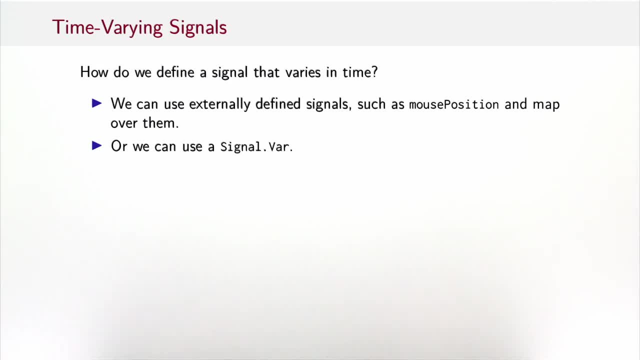 So if the signal is continuous at a fixed or varying time interval, at certain points and the value is greater than the value of the signal at the particular point in time, then we can easily get the signal to be the dependent signal, Or we can do that internally using a signalvar. 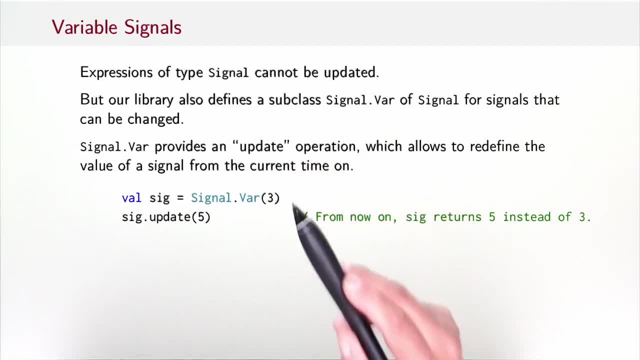 So expressions of type signal cannot be updated. But our library also defines a subclass var inside signal, so signalvar for signals that can be changed. Signalvar provides an update operation which allows to redefine the value of a signal from the current time on. 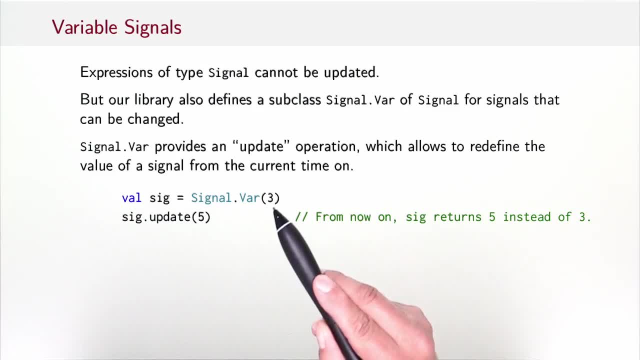 So for instance, we could set up a signal like this: it's a signalvar 3.. So it is at this point in the computation always 3.. But at some later point we could say sig update 5.. That means from that point on the signal would return 5 instead of 3.. 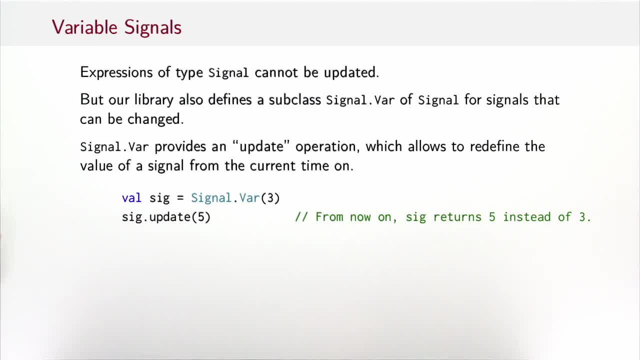 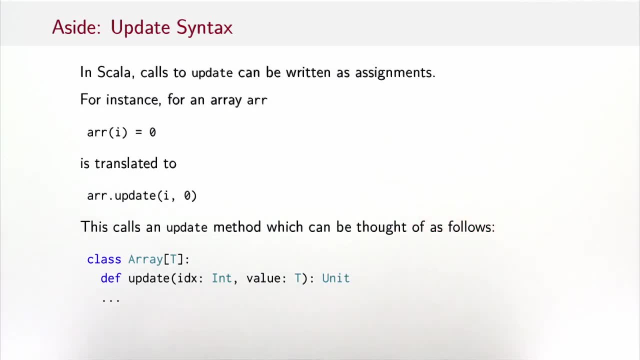 In fact, we can make this somewhat nicer by using Scala's special update syntax. In Scala, calls to update can be written as assignments. You might have seen this already when you worked with arrays. For instance, for an array r, we can write: r of i equals 0. 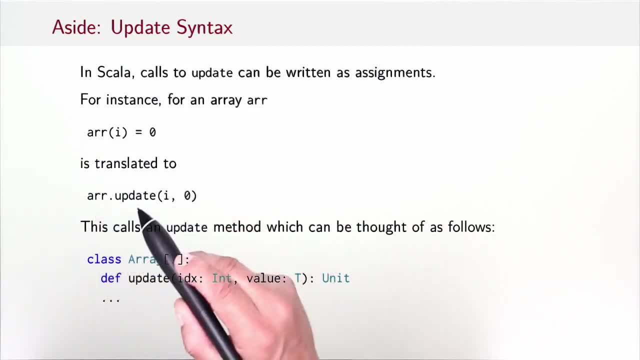 In case you wondered what that is, it's actually translated to rupdate, So it's really a call of an update method on an array. This update method can be thought of as you see here, So it's in class array, The update method takes an index and a value and it would then set the element of the array. 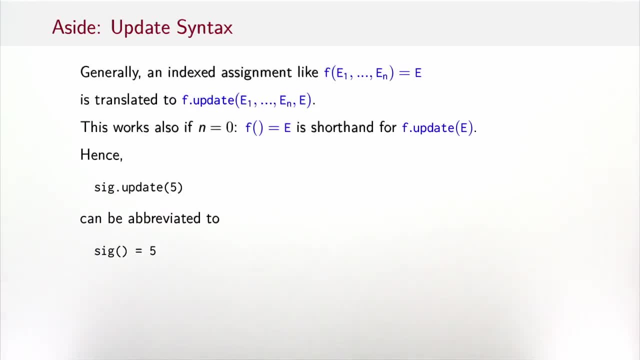 at that index to the new value. So there's a general rule in Scala that enables it. The rule is that If you have an assignment like this one here, so on the left hand side you have something that looks like a function call and then an equals and then a right hand side, then that's. 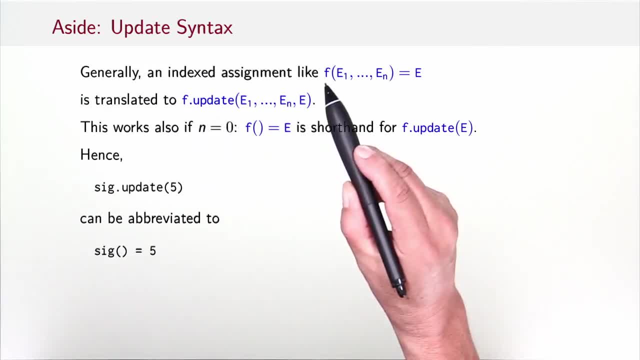 translated to an update method on the f here with all indices and then the right hand side as arguments, And that works also if n equals 0. So if n equals 0, then that means that f equals e is a shorthand for fupdate e. 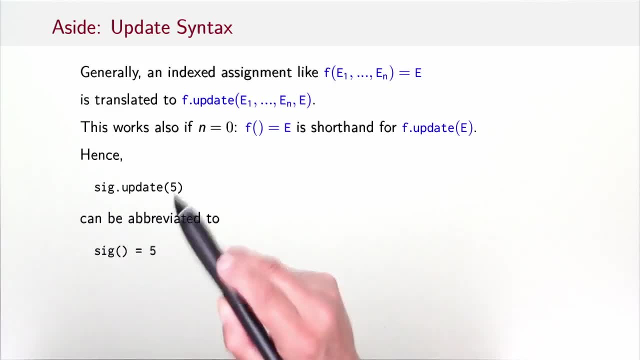 So because of that You can also write, instead of sigupdate, sig equals 5.. Which is quite nice, because we say, okay, sig is the current value of signal, and then sig update equals 5 would mean the current value of signal after this assignment will be 5.. 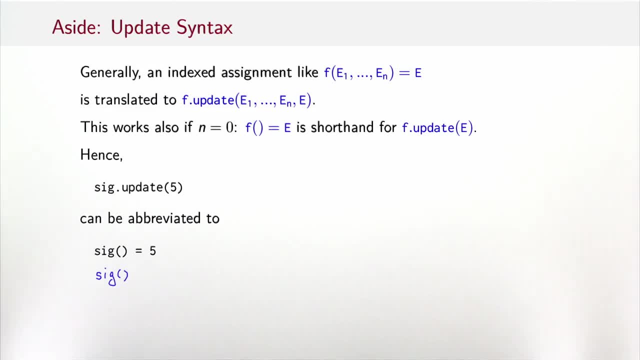 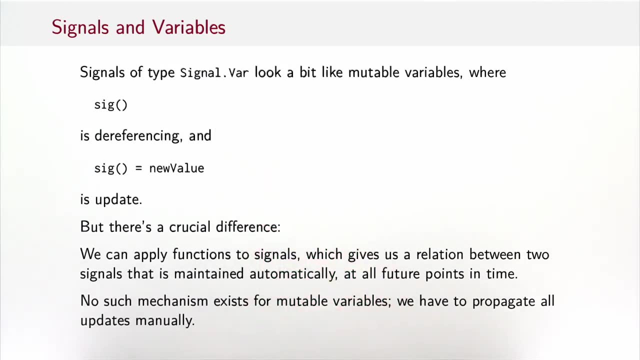 So in both cases you can read sig as current value of signal sig. So now you might wonder: how does a signal var differ from a regular var? Well, these signal variables look a bit like mutable variables where sig open parents, close parents is simply dereferencing, and that would be assignment. 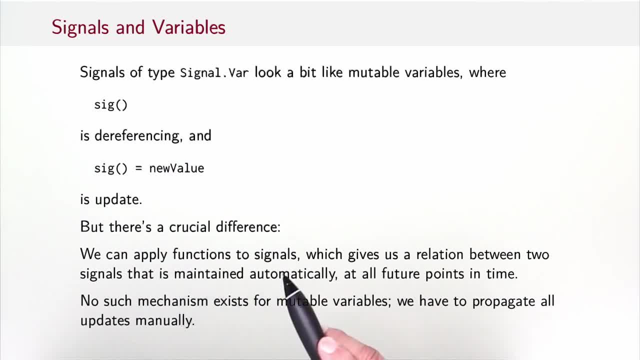 But there's a crucial difference: We can apply functions to signals, which gives us a relation between two signals that's maintained automatically at all future points in time. No such mechanism exists for mutable variables. We have to propagate all updates manually. So to illustrate the difference, I'm going to write down the same sequence of operations. 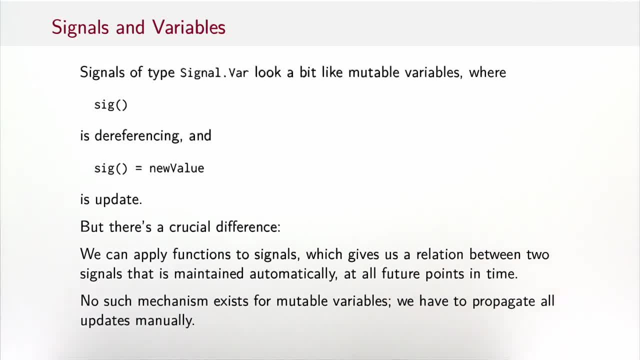 once for regular variables and once for signal vars. So here's a list of operations. I define a variable x to be 1.. I define a variable y to be x times 2.. And then I set x to 3.. Now I do the same thing with signal vars. 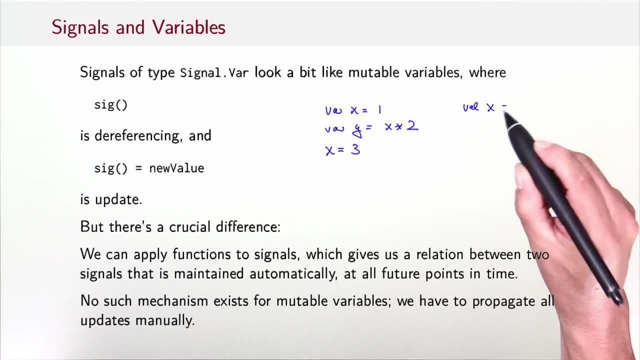 So the analog here would be: I define a signal Which is a signal var. 1. I define another signal, y, Which is the signal that is x times 2. And I update the signal var to be: 3. What is the value of y at the end in each case? 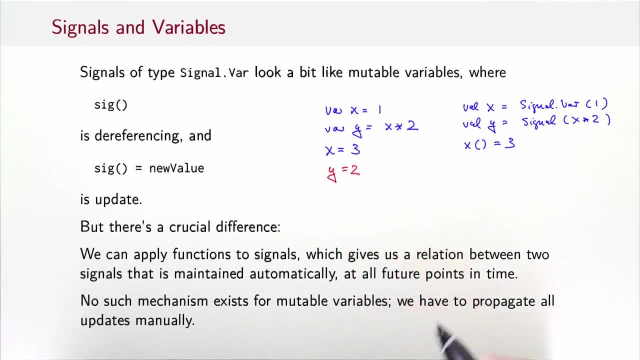 So here we would have clearly y equals 2. And here we would have the dereferenced y is 6. Because the variable x is now the signal 3. And y always maintains its relationship with that signal to be x times 2.. 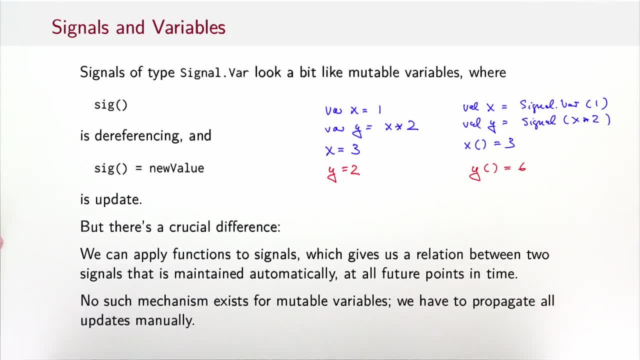 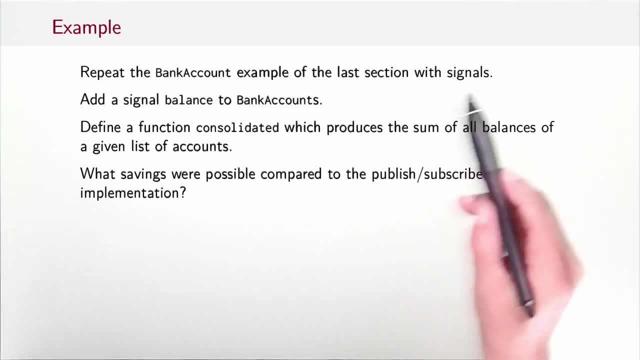 So that nicely demonstrates the difference between regular variables and signal vars. Okay, let's do an exercise. Let's repeat the bank account example of the last session, but with signals. That means we want to add a signal balance to bank accounts and then, instead of having 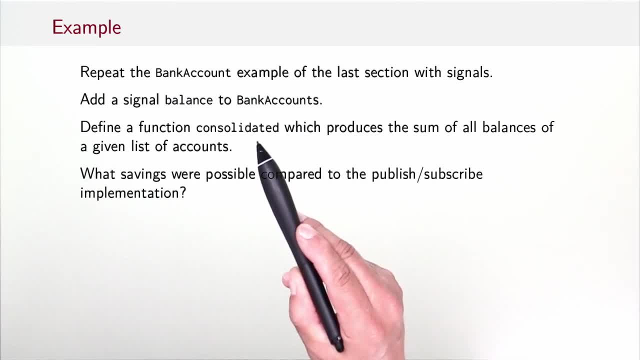 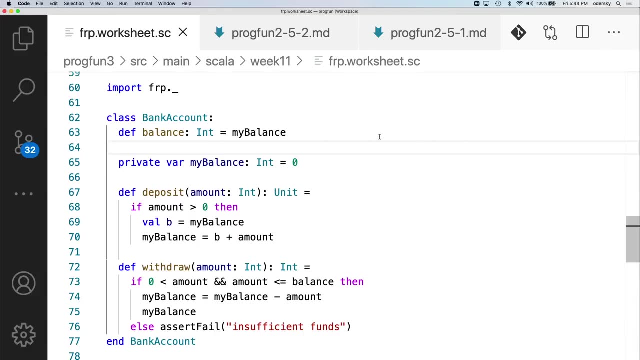 the consolidated signal With subscriber. we want to define a function consolidated which produces the sum of all balances of a given list of accounts as a signal. So the interesting question then is whether there were any savings compared to the publish subscribe implementation. So here we have entered the previous non-reactive bank account. 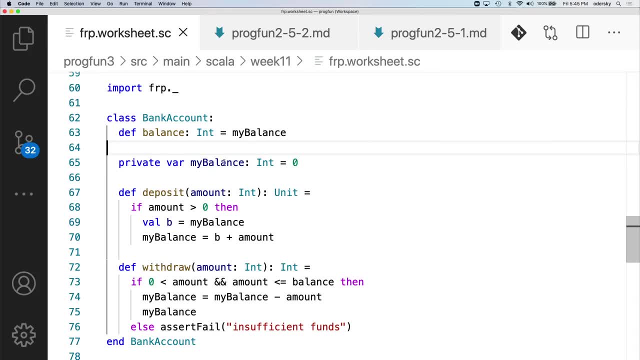 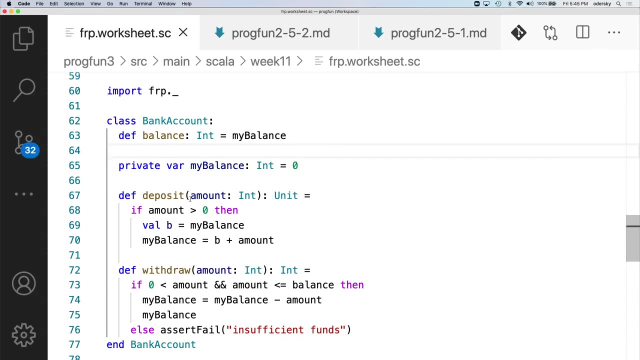 So it's just an imperative object with a private variable, myBalance- And the only thing I have done, compared to the previous versions of bank accounts, is that I have added a method balance that allows to inquire what the current balance is, But otherwise it's still the same as before. deposit deposits something into the account. 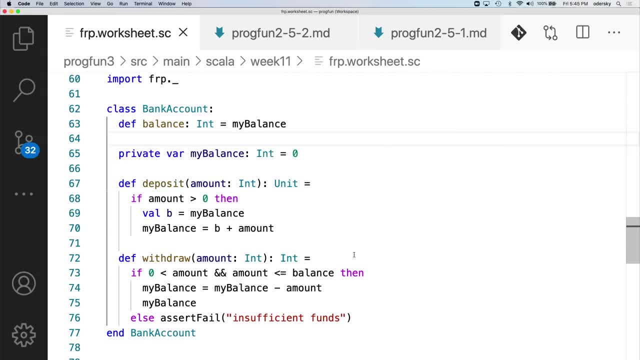 returns a unit, withdraw, withdraws something. Now, what we want to do now is turn balance into a signal, So it should be signal int, And that means my. my balance would also be a signal, and it should be a variable signal. So we don't need a var here. 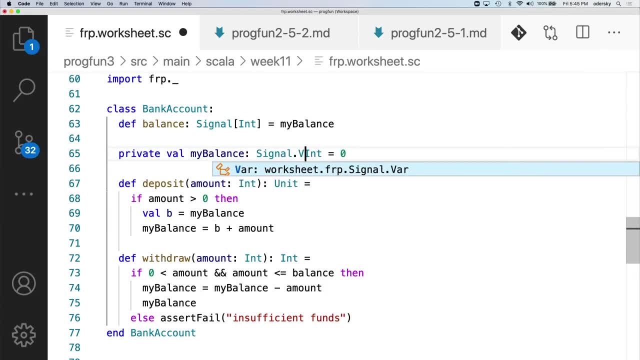 Here at the outside. but it will be a signal dot var of int And that's initialized to zero. So we can roll the type and the initializer into one and write that OK. so now what we have to do is that at each point when we want to know the current value. 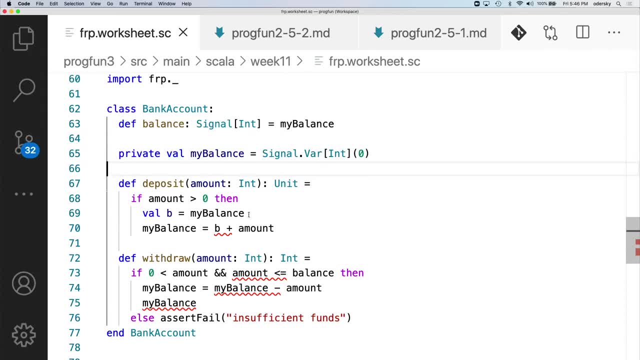 of a signal, like balance and my balance, we have to dereference it. So when we inquire what is the current value of my balance, We need the parents here, And if we update my balance, we need the parents here. Same thing would hold here. 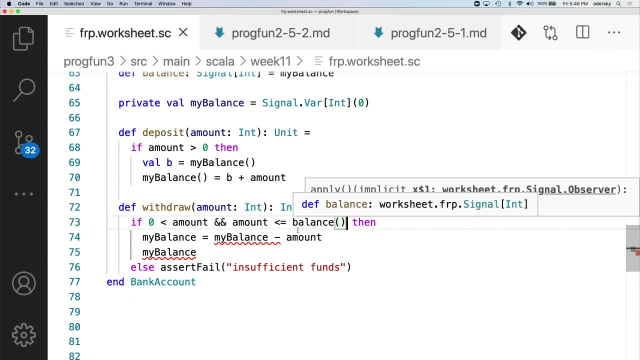 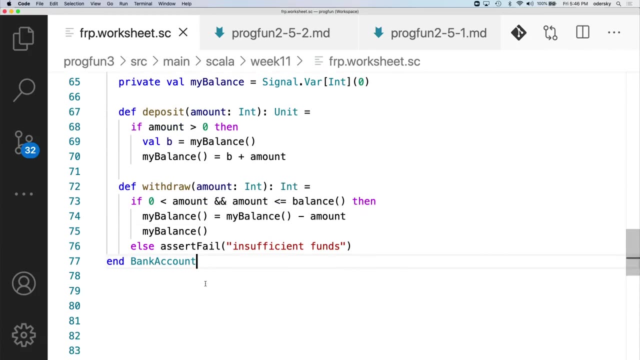 So here's an inquiry. put the parents. here is an update and an inquiry, And finally, we return the current value of my balance. OK, so let's do the next step, then, and define the consolidated method. Here is its signature. It takes a list of accounts. 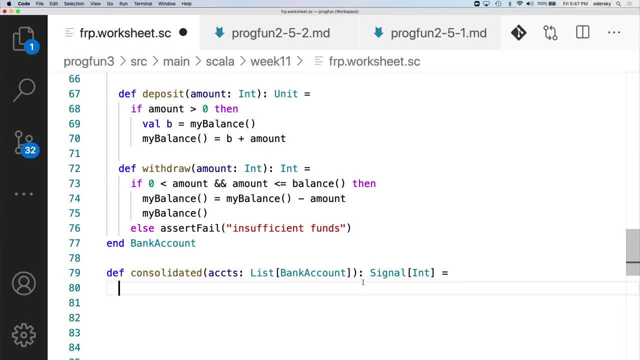 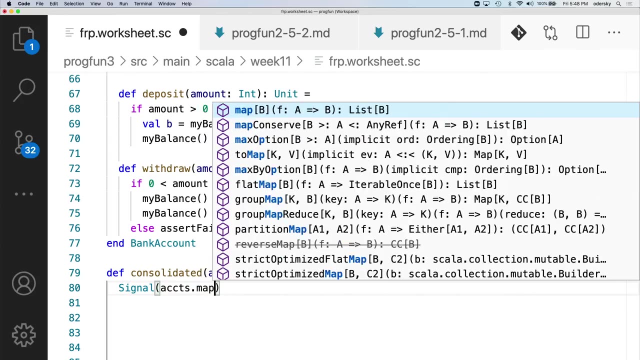 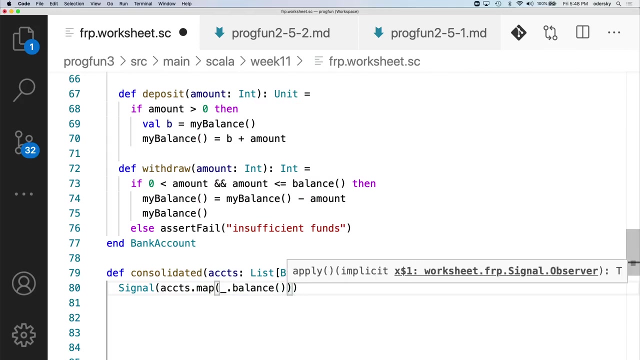 And gives us back a signal int that, at any point in time, tells us what the total balance of the accounts is. So, to implement consolidated, what we need to do is define a signal where we go through all the accounts, Take the balance of each, or it would be on that. 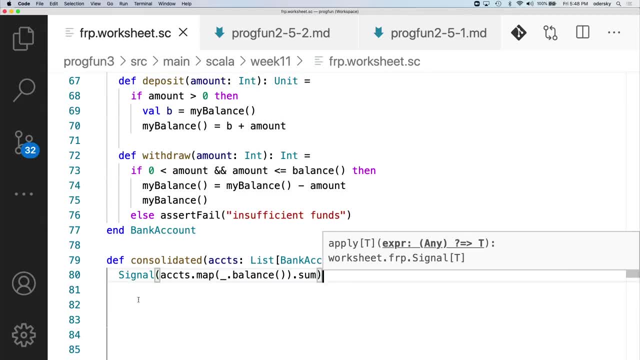 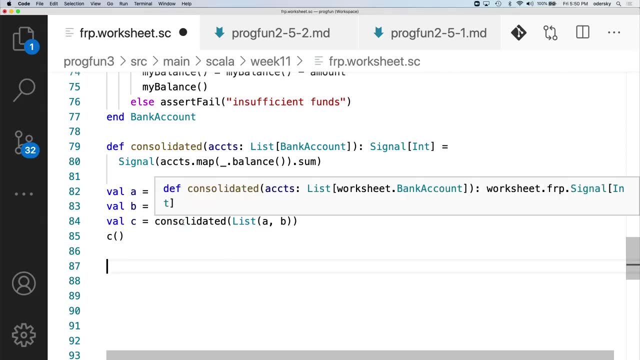 And take the sum of the results. OK, So we can test this by setting up, let's say, two bank accounts and forming the consolidated bank total in the C signal and asking what the signal is. So that gives us two bank accounts a signal and that signal is initially zero because 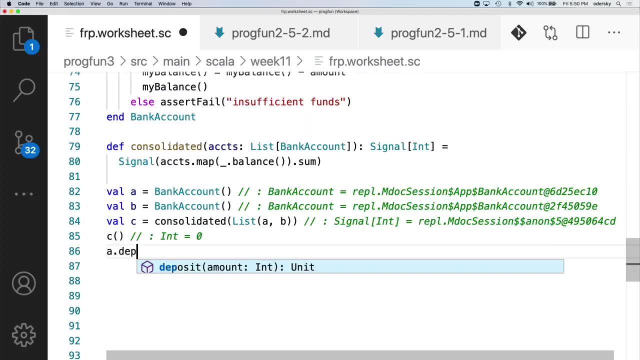 all the bank accounts are zero. So let's deposit something into account A And ask what the signal is, And ask what the signal is. OK, So it's 10.. Let's deposit something into account B, So now the total is 30.. 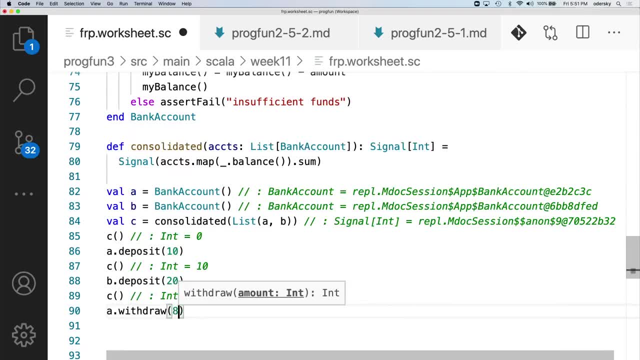 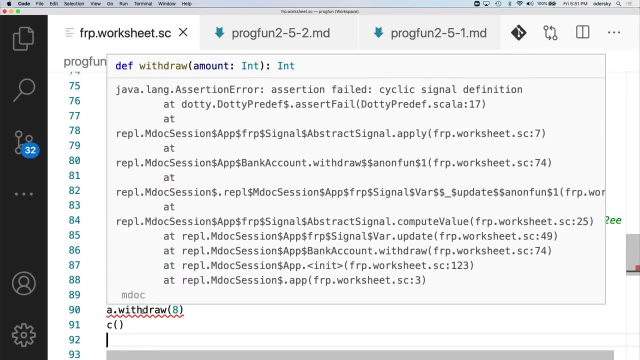 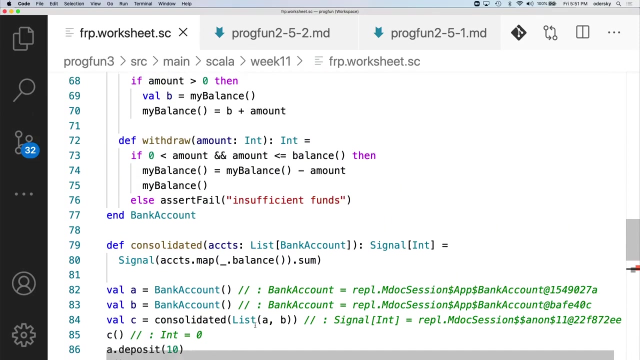 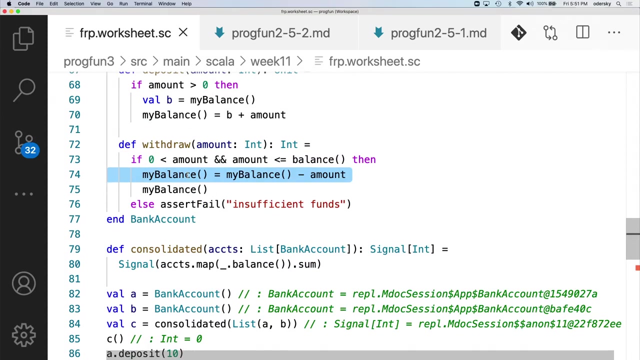 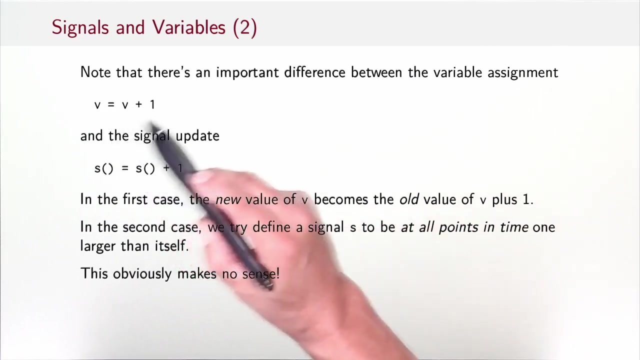 Let's withdraw something from account A And we get an error. So what does the error say? It says assertion failed. The error is that we overlapped an important difference between the variable assignments, such as v equals v plus 1 and a signal update: s parents equals s parents plus 1.. 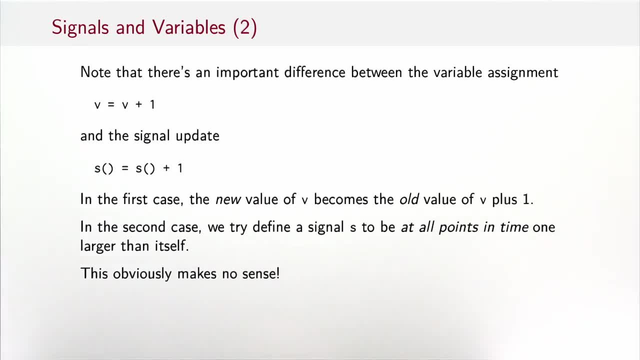 So why would we get a cyclic signal definition when we write something like this? In fact, our error was that we overlooked an important difference between the variable assignments, such as v equals v plus 1 and a signal update s parents plus 1.. The first makes sense, but the second doesn't. 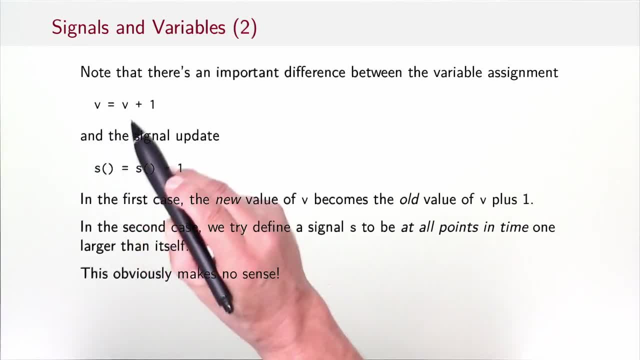 In the first case, what happens is that the new value of v becomes the old value of v plus 1.. But in the second case, what we did here is we try to define a signal, s, so that all points in time from this assignment on s is one larger than itself. 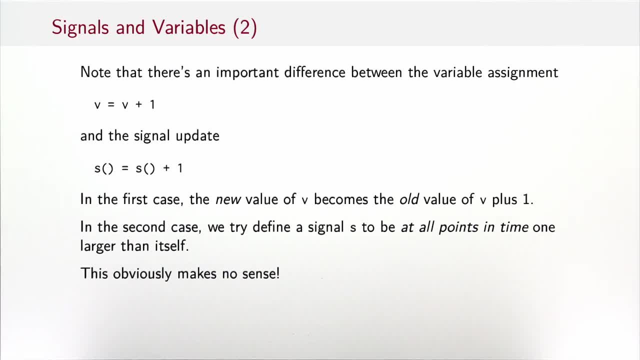 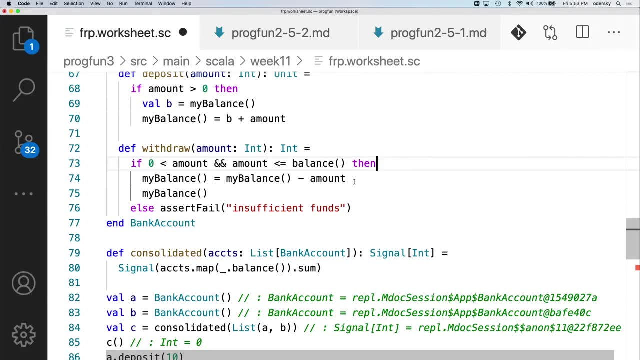 And that obviously makes no sense. It is indeed a cyclic signal definition. The definition of the signal depends on itself, and that's, of course, forbidden. So how do we fix this? Well, we do the same, what we have already done in the deposit method. 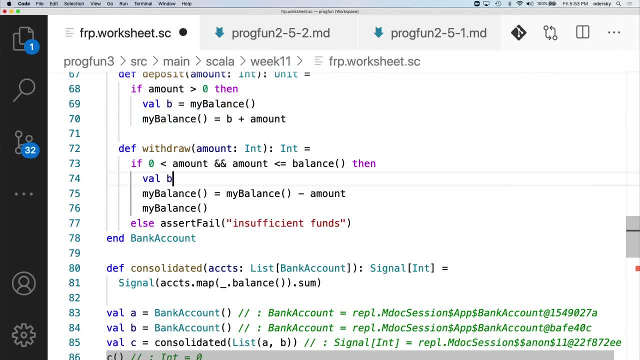 We get the value of the signal beforehand And then we use that value in the subtraction. So what we see now, the sequence of action, is okay, Let b be the signal, my balance, at this current point in time only, not all future points in time. 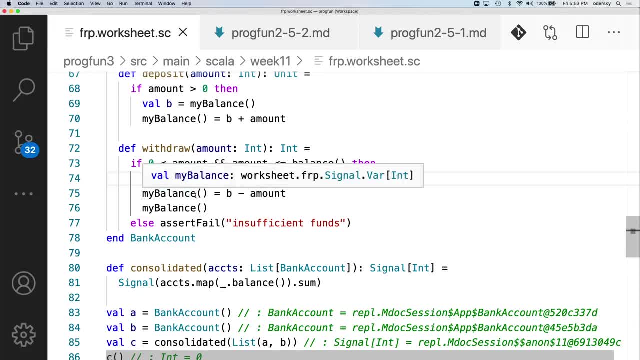 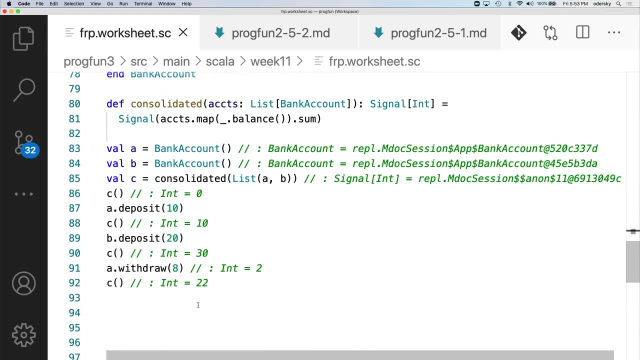 And now define the next value of my balance at all following points in time, to be b minus amount. So now it makes sense. Let's see what consolidated says. Yes, it gives us the right value after the withdrawal. So here's another exercise for you. 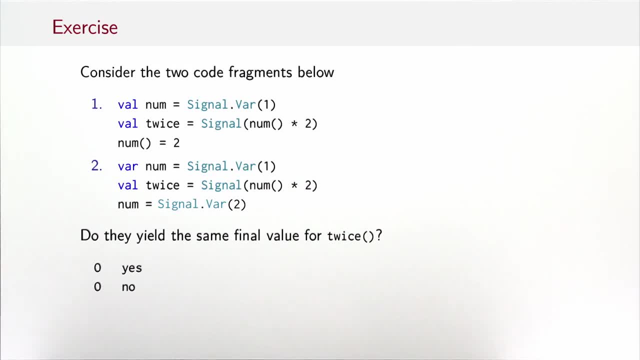 Consider the two code fragments here and here They look very similar. Are they in fact the same? In particular, do they yield the same final value for twice parents, Yes or no? Well, let's see. What are the differences? The differences are here. 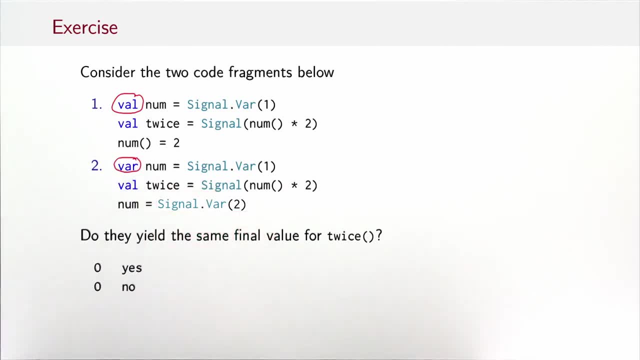 Num is a val and whereas here it is a var. And furthermore here I did a signal update: Num equals two and here I defined the variable number to be a new signal: two. Okay, So the value of twice after each of these sequences, after the first sequence, the value. 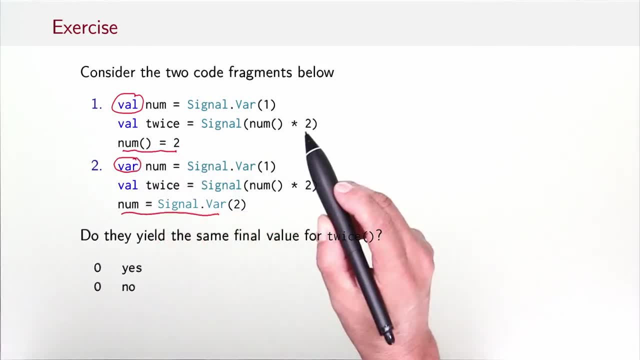 of twice will be the value of num times two. That's the relationship that we have established, And the value of num at this point will be two, So we will have twice equals four. After the second sequence, however, the value of twice will still be two. 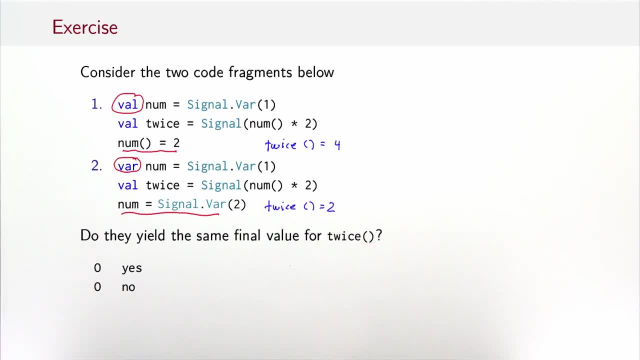 Okay, Let's see. Okay, Why? Well, because twice is linked to this first signal. What we have done in the second case is we have defined a signal var with value one and called it num. So num is a reference that points to the signal var. 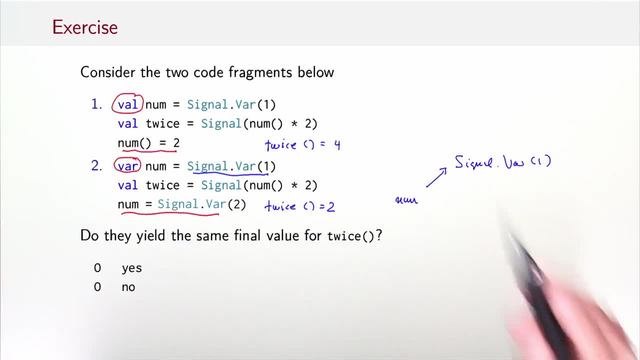 And then we have defined twice to be num times two. So it's that signal var, So twice would be the signal var. Okay, So we have defined a signal var of the num signal times two, where the num signal really points to this one here. 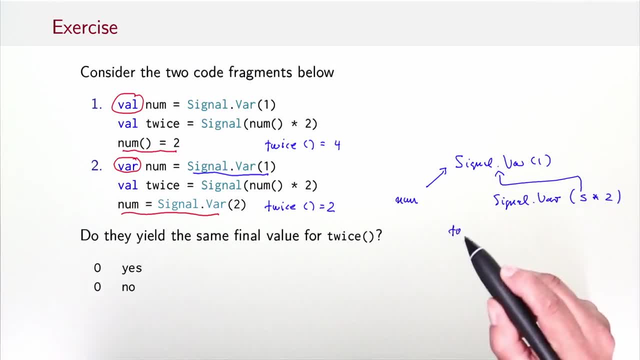 So we said: whatever that signal is, the twice signal, is that signal times two. But what we have done here in the last statement is we have now defined num to be a new signal var. Okay, That is initialized. Okay, That is initialized to two. 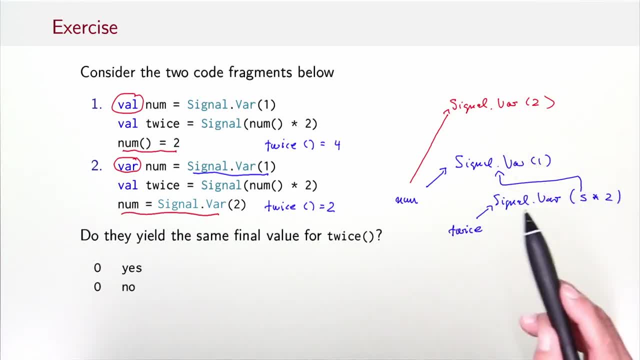 So num now refers to this different signal, but the link between twice is established to the signal that num referred to previously. So twice is still two, even though num points to a new signal which has nothing to do with what happens over here. So the answer to the question is no. 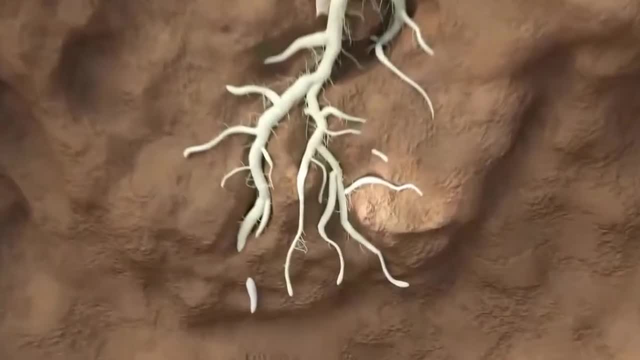 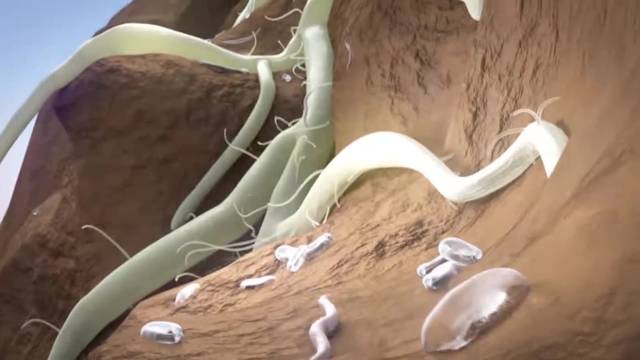 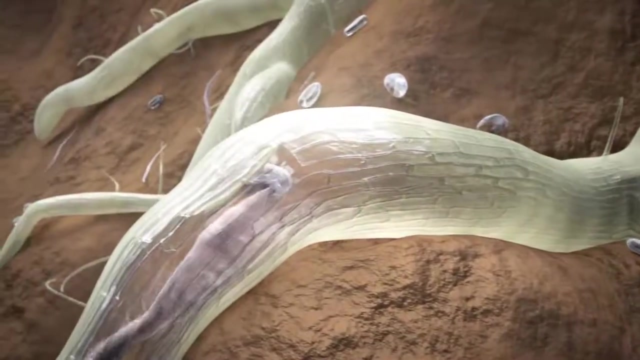 Nematodes are responsible for heavy yield and crop losses in fruits and vegetables all over the globe. Tiny eelworms, like the root knot nematode, live in the soil and the larvae, attack plant roots. Nematodes penetrate the root, start to reproduce and cause root galling. 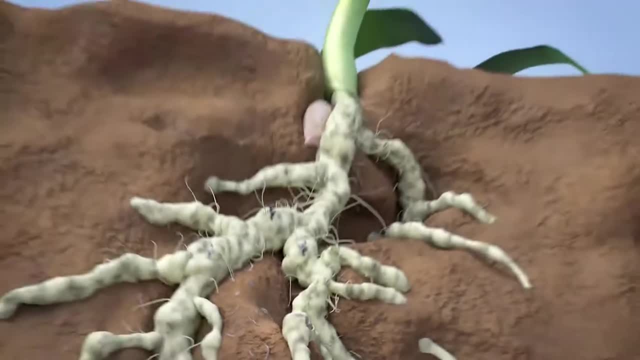 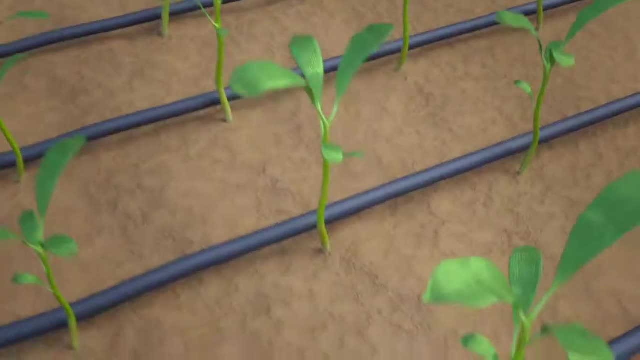 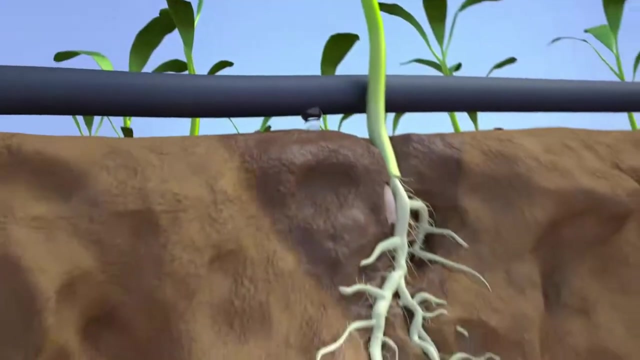 They suck water and nutrients from the root system. Infested plants suffer and show poor growth. Fluopuram from Bayer stops the attack. The active substance is applied to the soil via a drip irrigation system, allowing it to precisely target the root system.